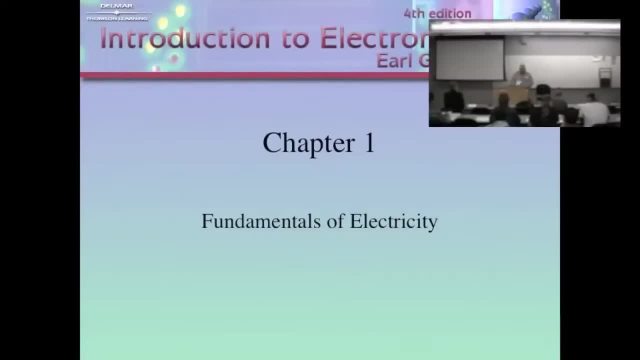 Okay, since you know who I am and you know how I operate, I'm all about protocols, not putting the proverbial cart before the horse. That being said, tonight, one night, and one night only, we're going to put the cart before the horse, The way that I want you to approach. 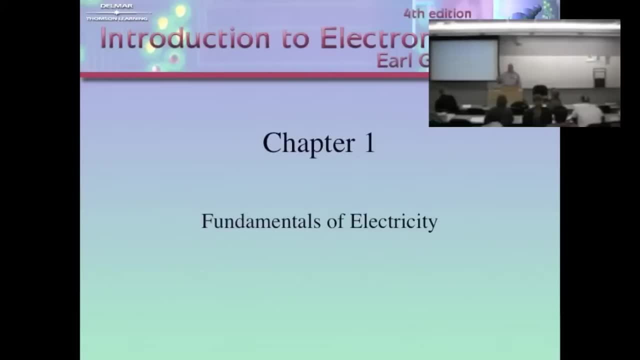 E-L-E-C-1-10,. and this is a recipe for success because, like I said, I've been doing this for a couple years. I know what works and I know what doesn't, And I guarantee you, I guarantee you, if you follow the syllabus, if you do all the assignments, that you're. 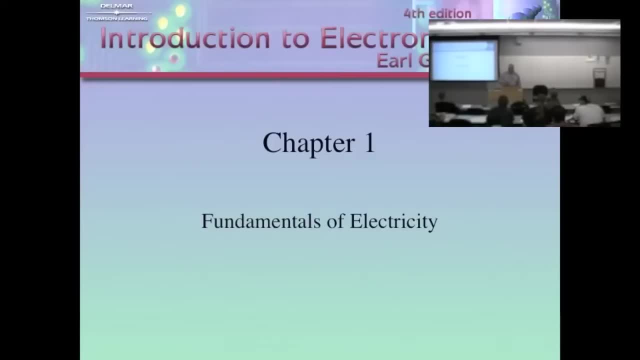 given. if you follow that recipe for success, you will be successful. You'll pass this class, Guarantee it. I don't know if any of you also know. Lake Washington Technical College has a guarantee that if you graduate our class you're going to be a successful student. 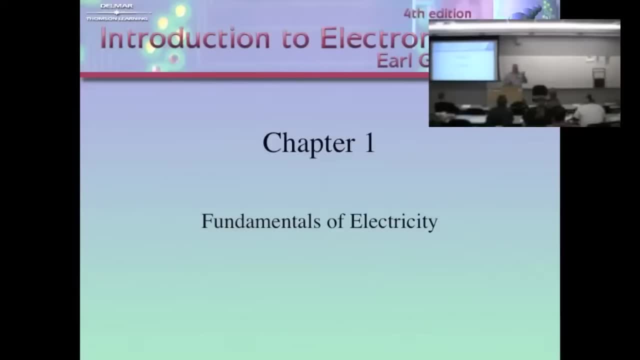 If you graduate our program, go into industry and your local, whoever you go to work for, says: you don't know what you're talking about. we will re-educate you for free to get you to the standard that industry says. How many students have been sent back to the electronics? 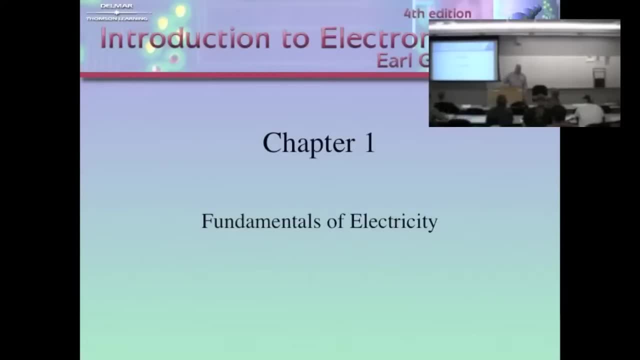 program Zero Zero, So I know it's working. So keep in mind the way that this is supposed to work. I think this really is the best recipe for success is I like to read the chapter very quickly, And what that does is like format your hard drive for what you're. 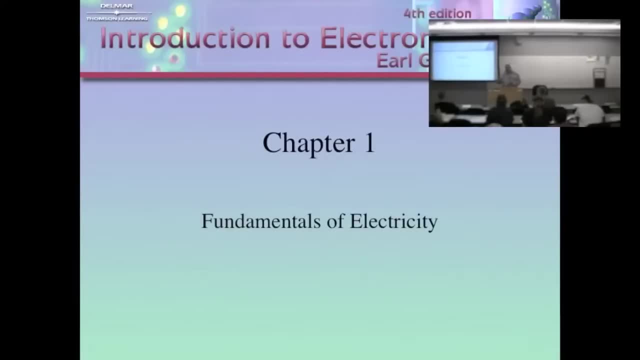 about to receive. That, of course, is a given that you've already reviewed the syllabus. In reviewing the syllabus, that shows you specifically like on page one they start the course outcomes and objectives And then you look at how those course outcomes and 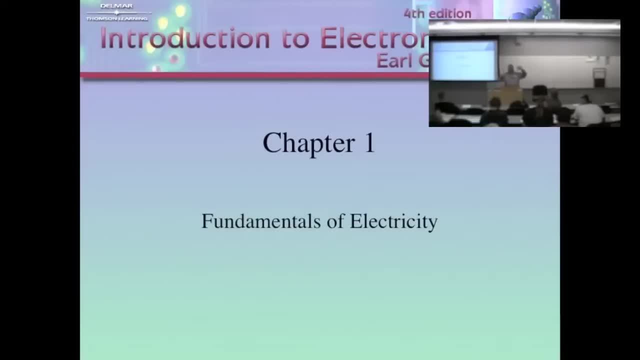 objectives of the syllabus, which is really the training contract between you and I, how closely the book and the chapter works meet those objectives. So read through the objectives in the syllabus first, then read through chapter one or chapter 17,, whatever. 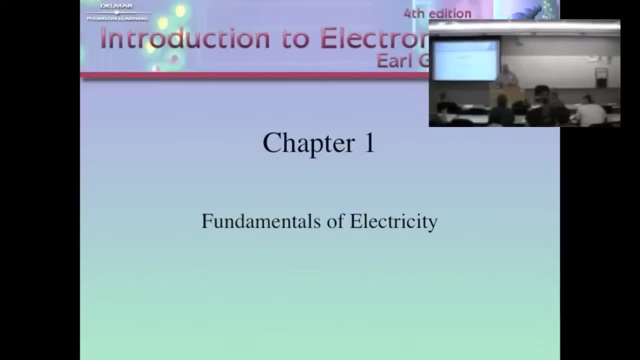 chapter you're on just like a book. But this isn't a book, it's a textbook. So when you get to the end it's not going to be like, oh, I never knew it was going to turn out like that. I mean, this is a textbook, It's a text slash reference book. After you've. 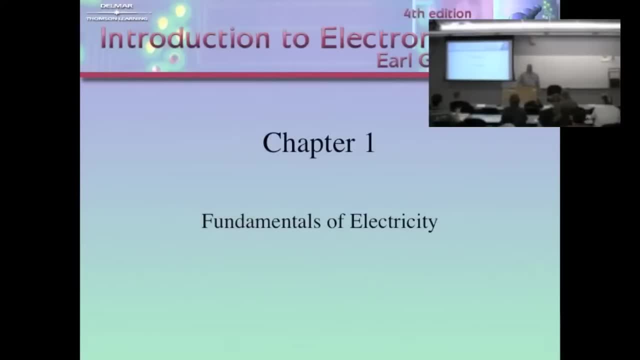 read through the chapter, then you're going to read through the syllabus And then you're going to go through it with a fine-tooth comb. Whenever you come to an example or a problem, take out your calculator and do the math And follow along and do every practice. 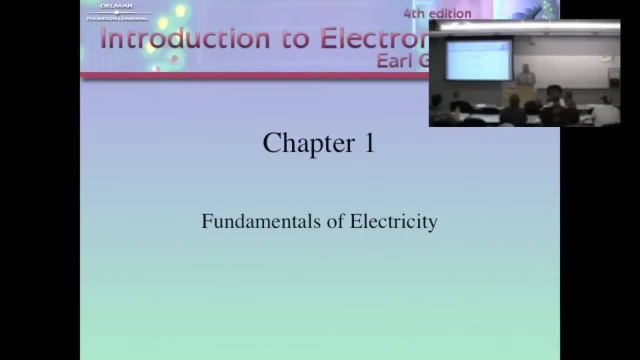 problem. Keep note of that, because that's going to be part of your written assignment. Then, when you're all done with the chapter, then I'd read through it again very, very quickly, just to make sure you retained all that information, Some of the stuff that we're 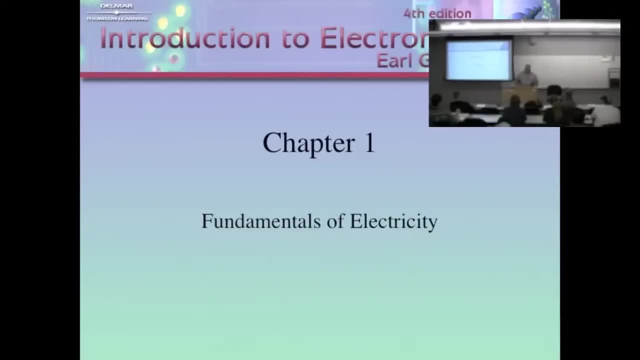 going to talk about tonight in chapter one, like atoms, molecules. you probably have heard before right The periodic table. A lot of you have heard that already before, So keep that in mind that if you're going through the book and the book is talking about stuff that you already know, you don't need to beat. 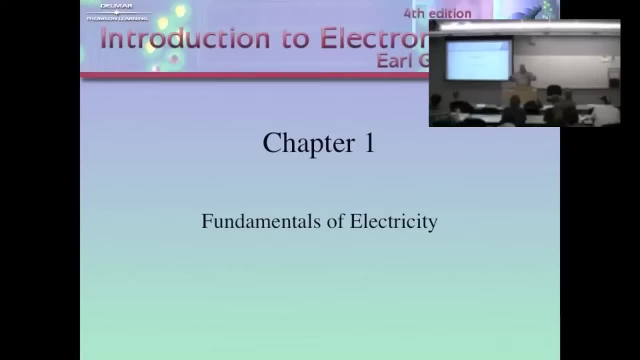 that to death, And that's actually good, because it's going to draw you to focus your attention on those areas that you don't understand, And you're going to be able to dump all of your energy into the stuff you don't understand. 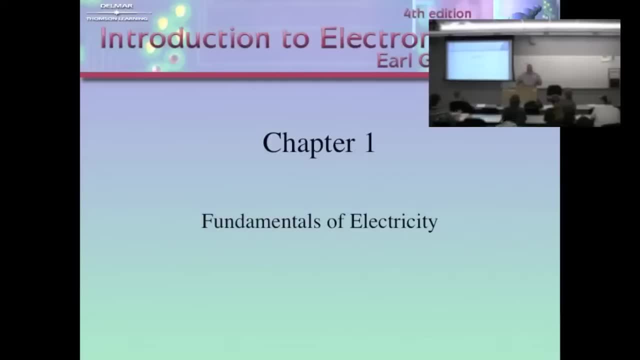 Does that make sense? I mean, it sounds really basic when you think about it like that, but that's really what's going to be the most effective means of traversing this. Normally, I will not lecture on a chapter until you've read the chapter, done your homework and 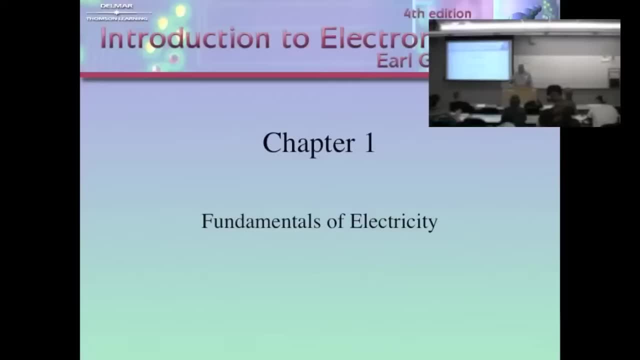 gotten together in your teams and completed a peer review right of your homework. Once your homework has gone through the chapter, then you're going to have to go back to the peer review- that process- And then you've got completed homework. then come into lecture. 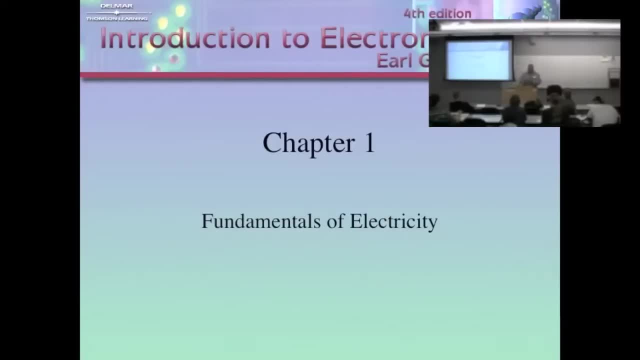 Because you know what? I want to spend my time in lecture, lecturing on What you didn't get out of the book, What you didn't get out of the assignments. That's how I want to spend the majority of my time in lecture. Fair enough, Okay, Let's get started. These slides here. 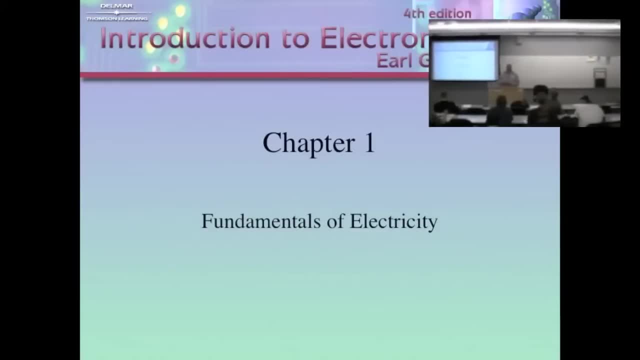 actually follow the book, And these slides, by the way, are available online On the web On the Google site. The TAs helped you out on how to get that site. The links are right there in your syllabus, So what you could do is you could download these from the site. 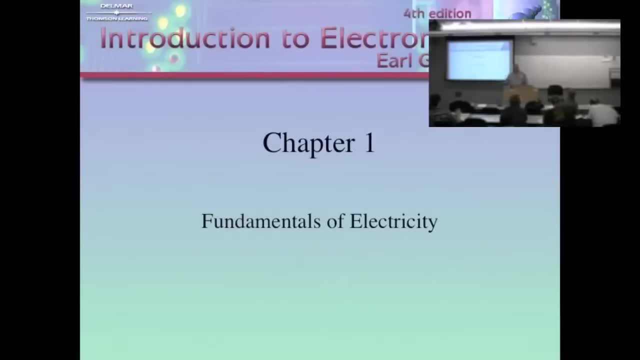 to your computer and then put them on your laptop or home computer and have the same slides that I'm showing you tonight. Also, there are audio files of this lecture in MP3 format that you could download. Joe Grinnick on MP3, right, And listen to me, I'm going. 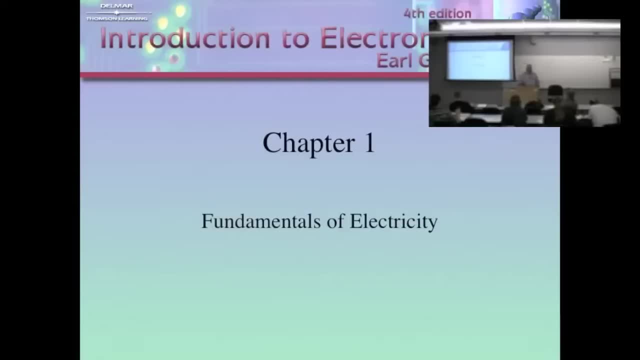 to show you When you're working out at the gym or running from the police or whatever it is you do when you listen to MP3s. And then also we're going to be adding to this now videotape of the lecture that we've got our TAs back there working on right now. So ultimately we'll 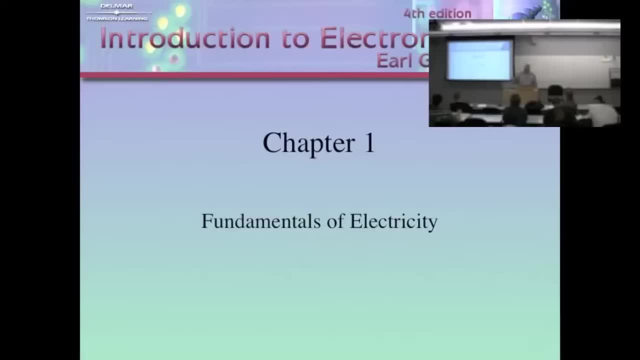 be able to upload that, And the reason that I go out of my way with recordings, with the slides. I've got nothing to hide. I've got nothing to hide As a matter of fact. I want to give you as much information as I possibly can. 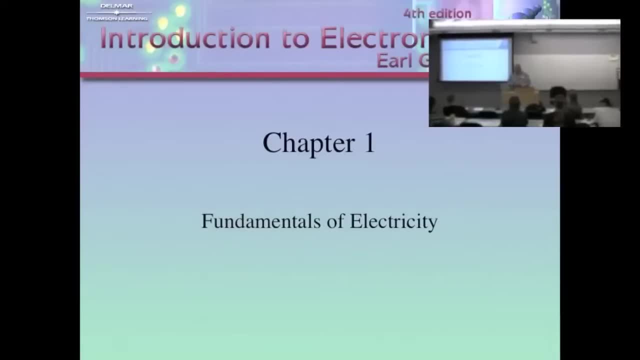 So that you could benefit from that information And you know what. How many of you here own any DVDs- Your favorite movies? Why would you own a copy of a movie? Why would you do that? Isn't seeing it once good enough? Why would you go out and buy DVDs of a movie? 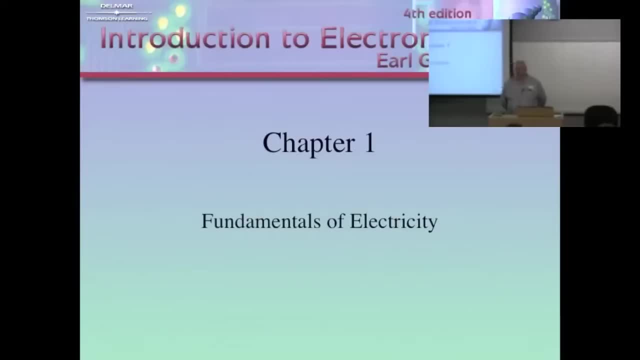 Because they're cheap, Unless they're giving it away. so it costs money. Why do you? What's that? You couldn't bid for it? That's a big one. What's that You couldn't bid for it? That's a big one. You couldn't bid for it. That's a big one. 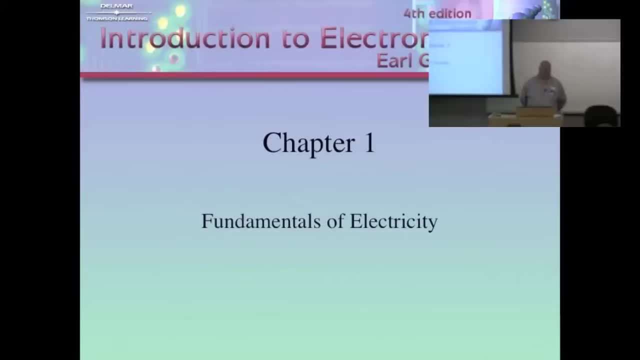 Yeah, You can watch it any time you want. You can watch it any time you want, But why specifically would you purchase a particular movie? Because it encompasses your interest. Exactly, It encompasses your interest. And for those of you that have movies, how many? 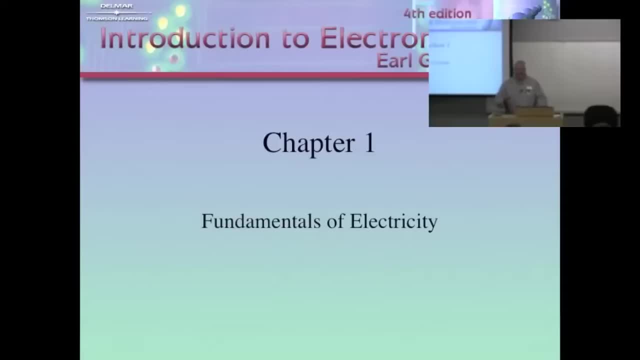 of you have watched a movie the second time and picked up stuff out of it the second time around- that There's some movies I've seen in the theater that I'm like I've got to go out and get that DVD because I want to see this again. Yeah, I know how to do it. 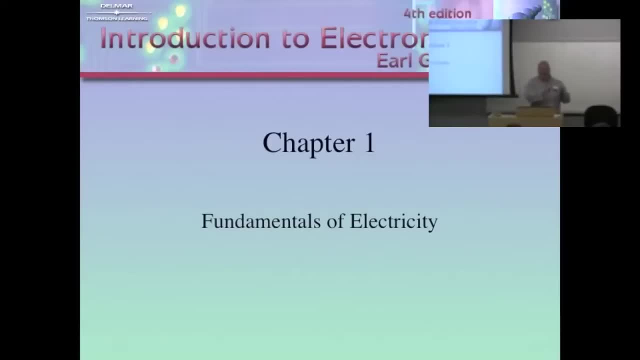 Yeah, I know how it ends up, But I want to see it because I missed something in the beginning and I want to look for that thing that I missed in the beginning or whatever. So it's perfectly natural for you to want to hear this lecture over and over again, I mean for some of you. 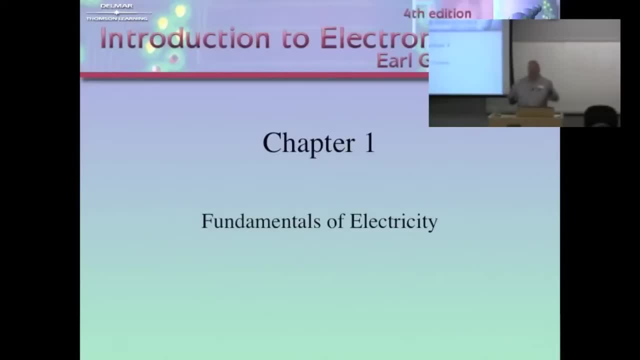 once might be good enough. Okay, I go to church on Sunday, My pastor. normally he gets up there and he preaches. I get it right the first time, I don't need to hear it again. Okay, For some other people, though- and actually at my church they do audio recordings and 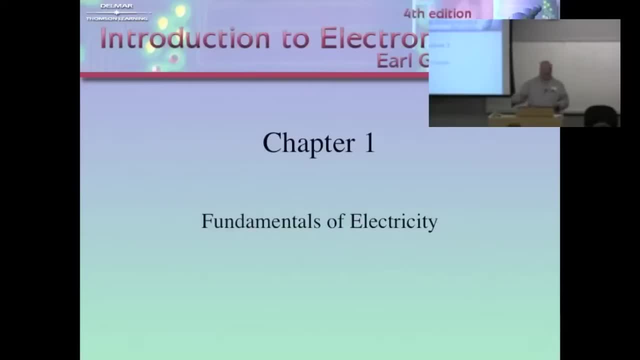 then people can listen to that content And I think that's a good thing. But I think that's a good thing. People can listen to that content. They want to hear it again. Normally I get it the first time. That's the kind of guy that I am. That's the type of learner that. 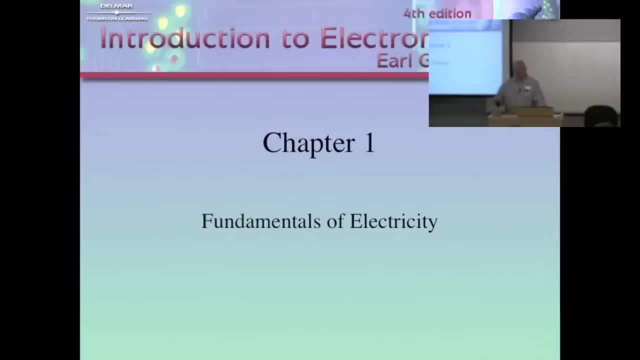 I am. But look at that. That's the other thing too with taking notes. Some of you- it's been a while since you've been in school- Try to hone your note-taking skills. When I emphasize something, I'm usually emphasizing it for a reason, And that reason is: you may see it. 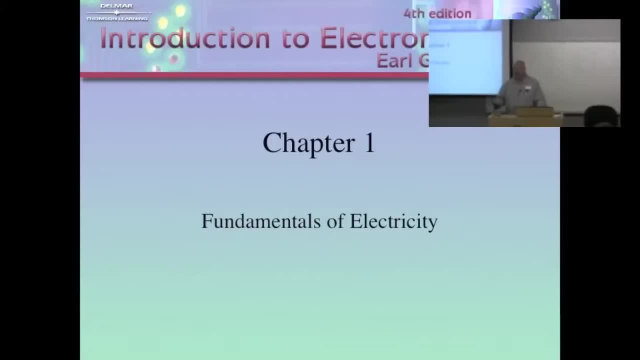 again in the future on a quiz, on an exam, But, most importantly, you may see it again in industry, Because one of the things I don't want to do is teach you the exam, teach you the quiz. That's not what it's all about. One of the things that I want to share with: 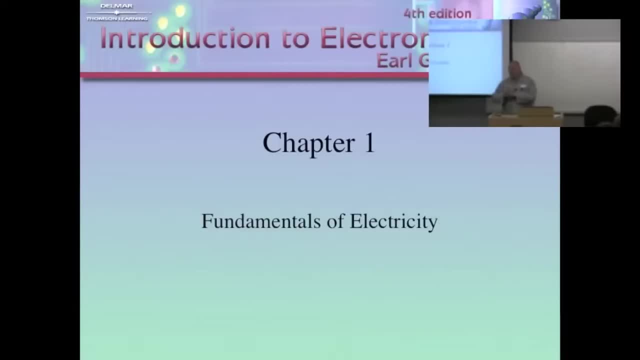 you is, I'm not really concerned. I mean, I want all of you to pass my quizzes. I want you to all pass my exam. I want you to all pass this class. But to be totally honest with you, do you know how I measure your success? I measure your success as to where are you. 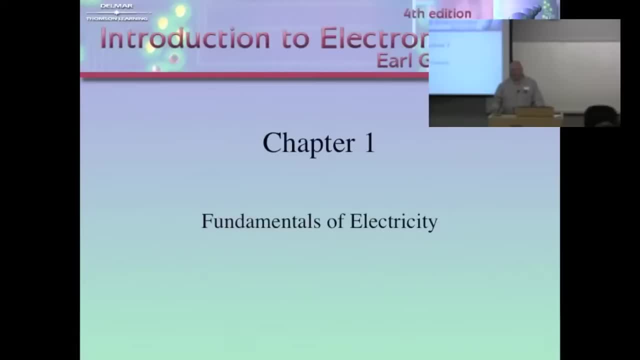 going to be five years from now, And did I give you an example? Did I give you an example of that? I wouldn't give you anything out of this course that helps you in that position you're in in five years, in ten years. The payoff for me is when you call me and say: 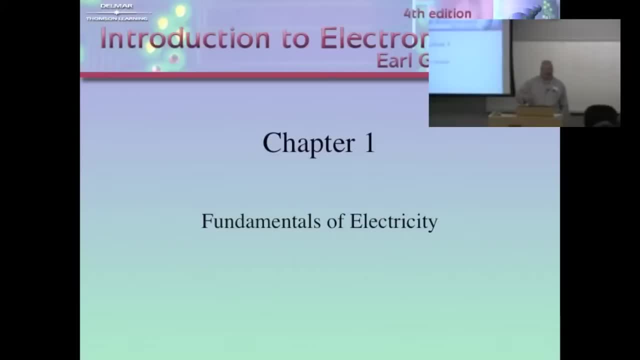 Joe, I'm in town or I'm passing through, I'd like to buy you lunch. I like lunch. Swing by and buy me lunch. Tell me what's going on, Tell me what you're doing now and how I had an impact on that. I actually I went on a cruise over Spring Break, Caribbean. 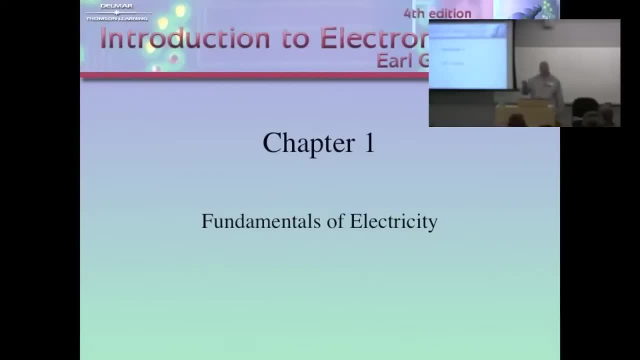 I was just getting ready to get on the ship and I get all my emails forwarded to my phone and I got an email from a student that I had in 1993.. And he introduced himself and he says: I don't know if you remember me. My response back to him: of course I remember you. 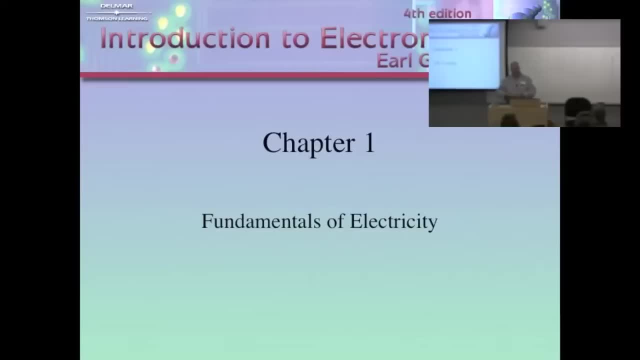 Because, again, we established a relationship, a professional relationship, But he graduated, he went down to California, kind of dropped off the radar. He was going to be in the area and was wondering if I'd be available next Friday to get together and we could visit And I said, well, unfortunately I'm out of town. 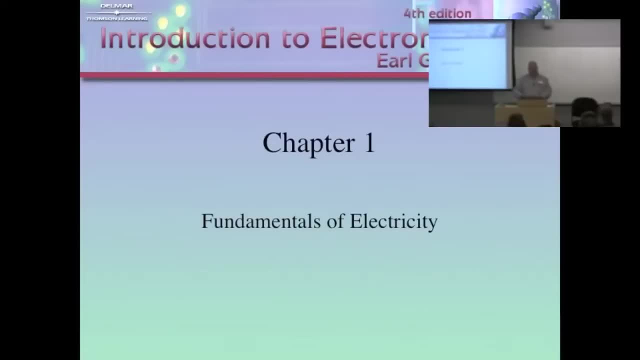 But you know, that is how I measured the success. Number one, that he remembered me. Number two: what he learned here is part of his present reality. So that's what I want all of you to think about. Yeah, you want to pass the quiz, you want to pass the exam, you want to pass the class, but where are you really going to use this stuff? 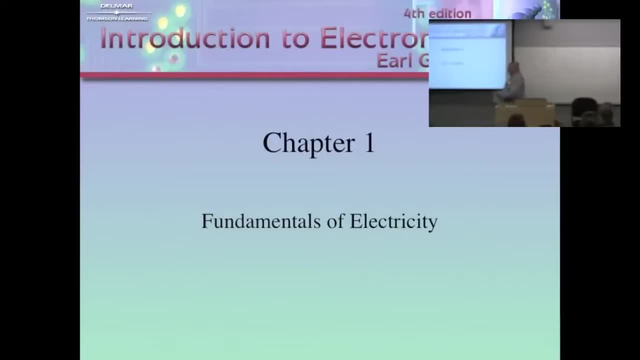 Anyway, kicking things off here, this is section one of the book, Section one of the book Area of the text that deals with what are called DC circuits. DC stands for direct current And we're going to talk about the difference between direct current and alternating current throughout this. 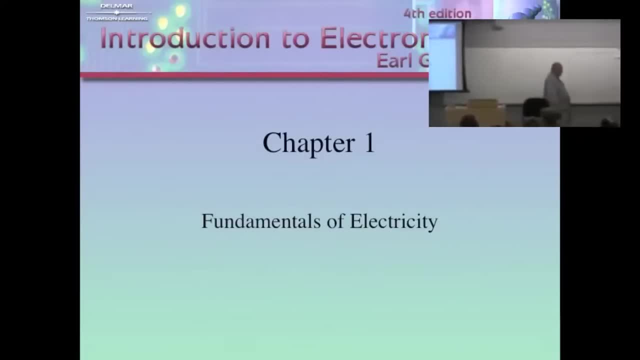 Chapter one deals with the fundamentals of electricity And I got to tell you That these first few chapters are like sacred chapters. You know, we should like ring bells and like hit gongs and chimes or whatever when we speak of some of this stuff. 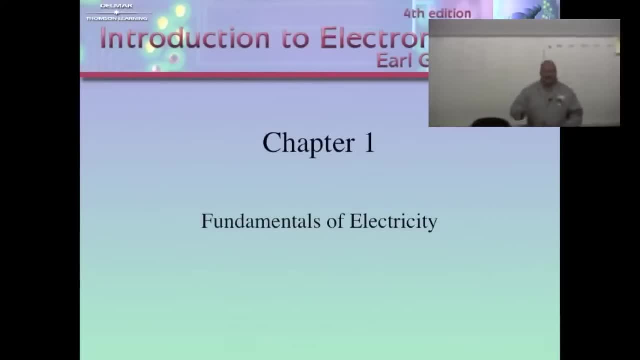 Because if you want to be successful in electricity and electronics, these things that we're going to speak of are critical attributes of what makes stuff work. As far as I know, I'm concerned, I'm going to let the cat out of the bag from the get-go. 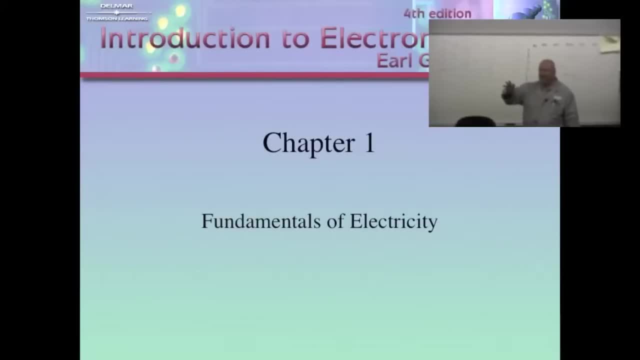 Okay, The four. the big four things that we're looking at that drive this entire industry are four properties. The properties are: voltage, current resistance and power. Voltage, current resistance and power. Voltage, current resistance and power. 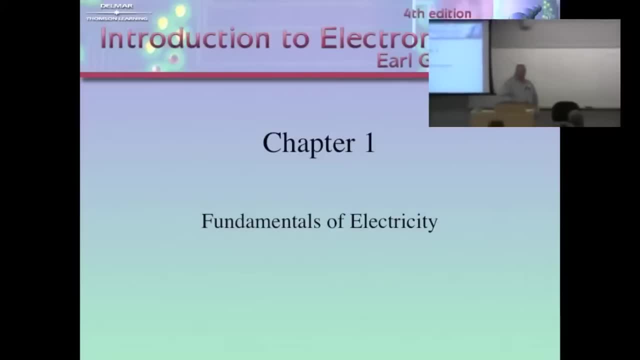 My cell phone works because of voltage, Current, resistance and power. My car computer works because of voltage, current, resistance and power. Satellite TV works because of voltage, current, resistance and power. Anything electrical or electronic works because of those four. 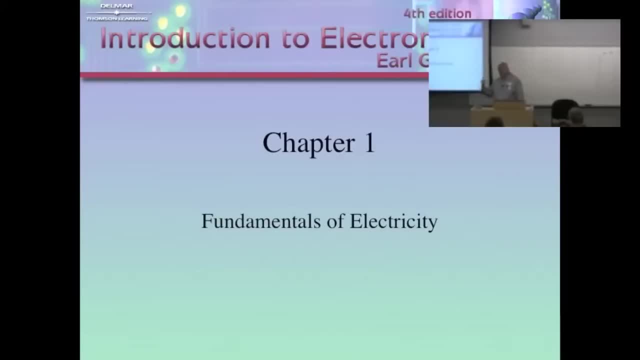 So what we really need to ensure is that these four properties that we're going to discuss we fully understand, up one side and down the other. As I said earlier, I've been doing this like since puberty, So you would think that I know everything there is to know about voltage, current resistance and power. 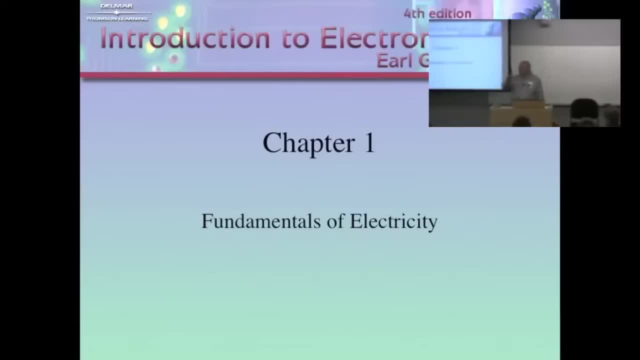 No, I do not. Occasionally I get questions from students that are associated with those properties that I can't quite answer, even though I've been doing this for so long. So I'm on a continual journey to learn as much as I can about those four properties. 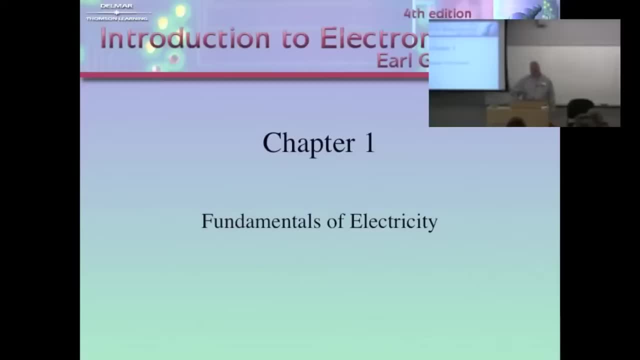 So we're going to kick things off with chapter one here, dealing with the fundamentals of electricity, but pay special attention to those four properties: Voltage, current resistance and power. The big four. I like to call them the big four because they are the big four. 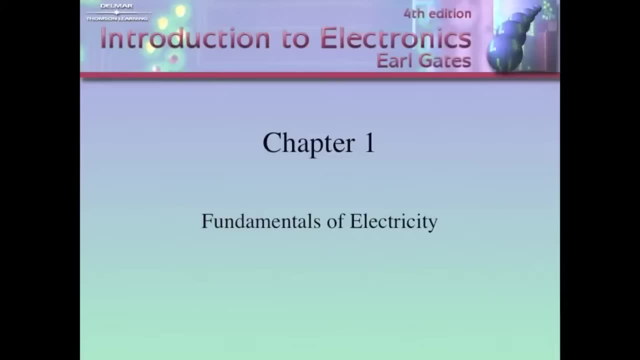 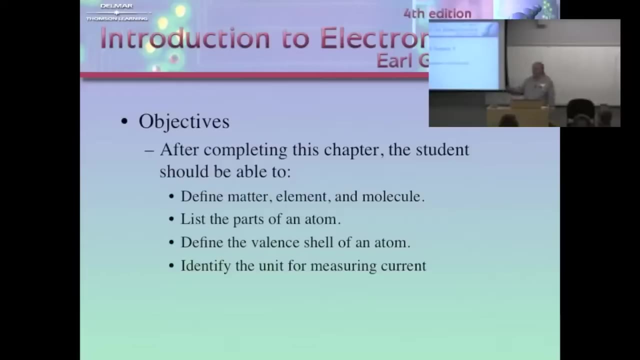 It's what everything is based on. If you know what's going on with voltage, current, resistance and power, you know what's going on inside the circuit. We're going to talk about that. So kicking things off, fundamentals of electricity. 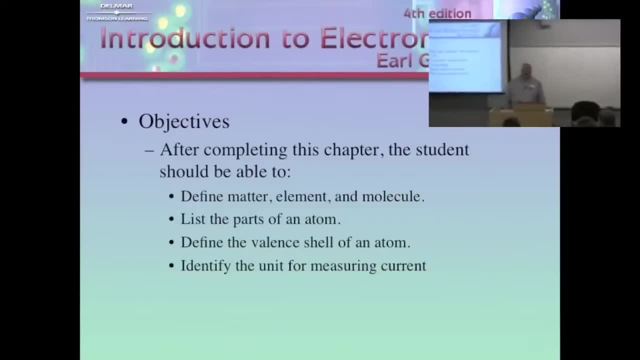 One of the things that I do at the start of every lecture is I review the objectives. The objectives that I review are the same objectives that are on the syllabus. That's a pretty good reason why I select the objectives. The objectives in the textbook reflect the objectives in the syllabus. 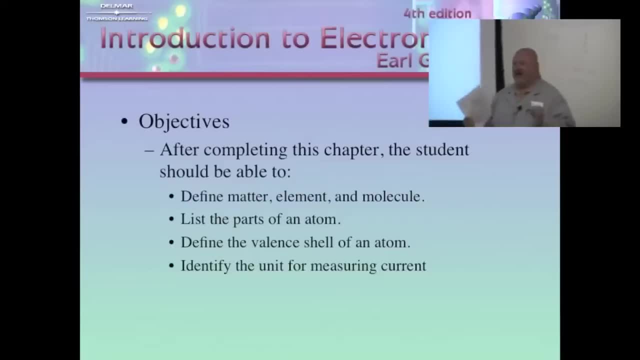 One of the other things I want you to fully understand is: I don't teach the textbook, I teach the curriculum. The curriculum is contained in the syllabus. The curriculum is derived. The curriculum is derived through input from our local industry advisory committee. 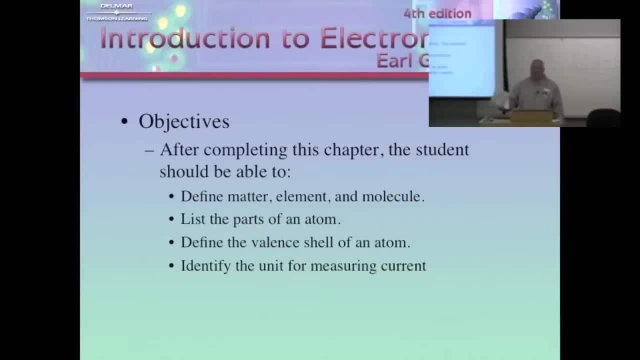 This is a group of volunteers that get together on a regular basis, sit down and tell us what we need to be doing for this program to stay competitive. So this book works really good because you're going to do all the chapters in it. 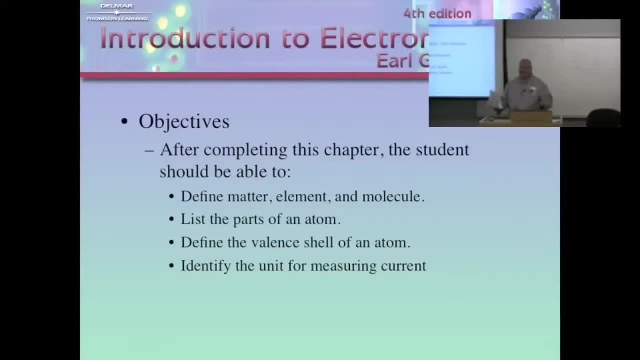 But occasionally in the future you may get some textbooks that the instructor is going to say you don't need to do this chapter Why It's not part of the curriculum. Local industry really doesn't think it's important that you learn that aspect. 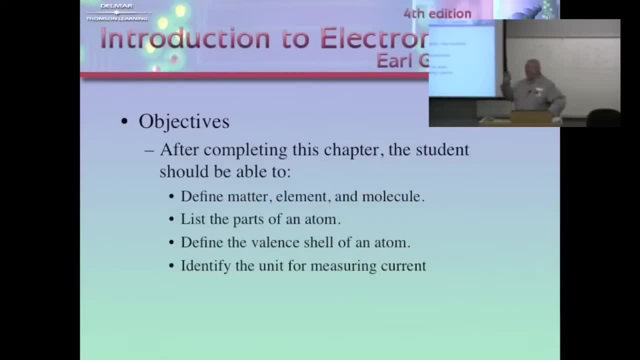 So does that make sense? Okay, One of the reasons that I review the objectives as well is to prepare you for what you're about to receive. It's like formatting your hard drive So that when I start talking about this stuff, you're kind of like ready to store that information away on your hard drive, your mental hard drive, your brain. 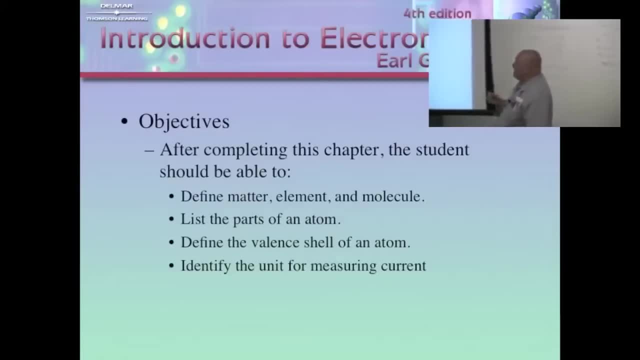 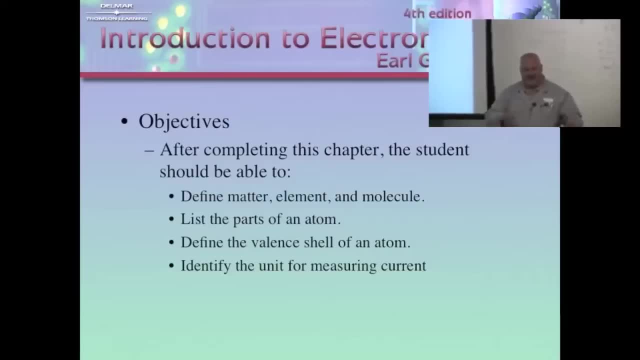 right off the quiz: Define matter, define element, define molecule. It's an objective. I hope at the end of this chapter you could define those, List the parts of an atom, define the valence shell of an atom and identify the unit. 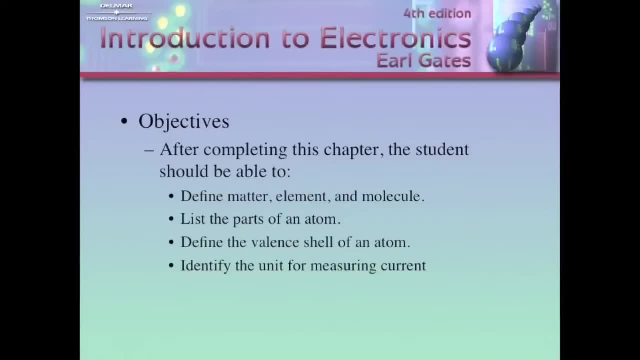 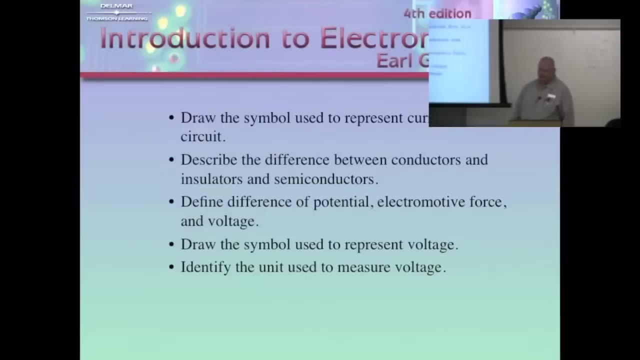 for measuring current Draw the symbol used to represent current flow in a circuit. Describe the difference between conductors and insulators and semiconductors. Define difference of potential, electromotive force and voltage. Voltage, wasn't that one of the big four? So again, if this was like church would be ringing bells, or 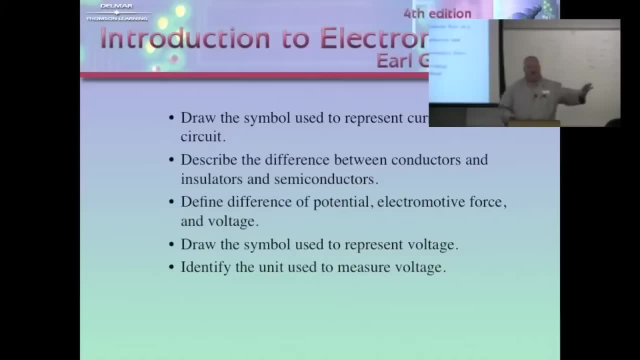 gong. you know We'll talk about projects later. Some of you may want to build sound effects so that we could you know whenever do that stuff or dim the lights. Voltage- Draw the symbol used to represent voltage. Identify the unit used to measure. 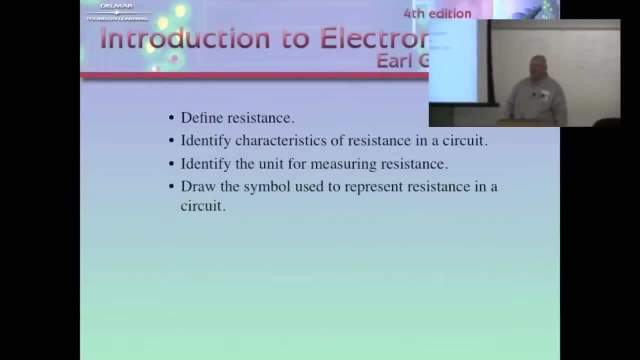 voltage to measure voltage. Define resistance gong, one of the big four. Identify characteristics of resistance gong in a circuit. Identify the unit for measuring resistance and draw the symbol used to represent resistance in a circuit- a circuit. 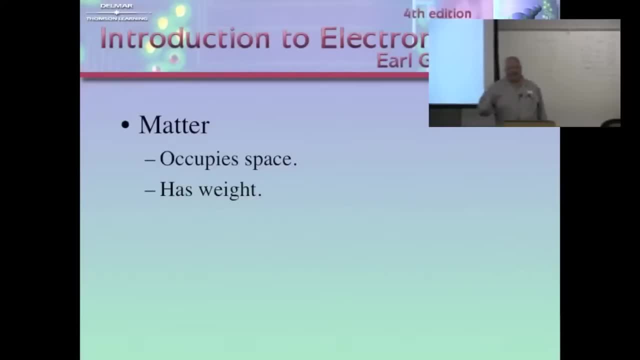 Everything you are about to learn, as it pertains to electricity and electronics, is traceable back to matter. Do any of you here know anything about matter? Do you know what matters? Matter is anything that occupies space and has weight. Does anybody know where we could find the absence of matter? 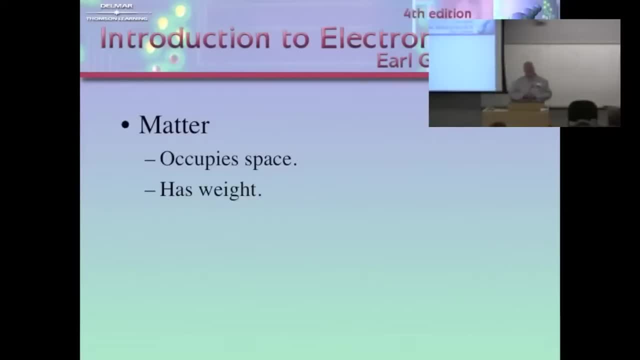 Does anybody know? can we create this condition here on planet Earth Vacuum- and I'm not talking about the auric-5-pound, upright, I don't think that's what you're talking about, right? What kind of vacuum are you talking about? It's called industrial vacuum, And 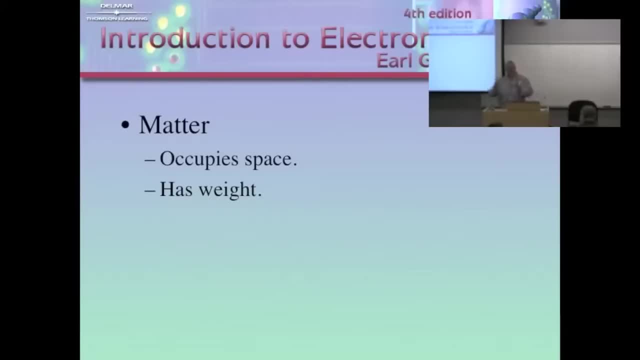 And, in essence, what we're talking about is pumping all of the matter out of a vessel so that all that's left inside is space- empty space. It's used a lot. A lot of you that go into high-tech careers you're going to see this process used in the manufacturing process. 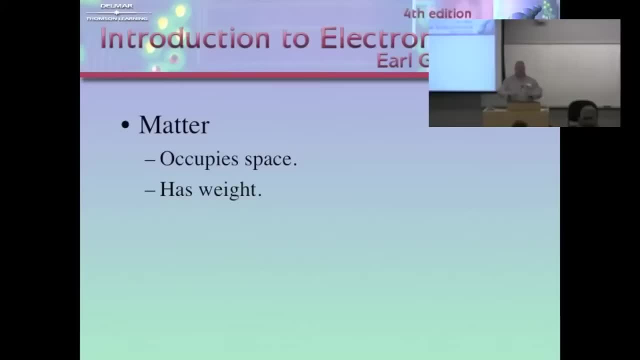 because it allows us to only put into the chamber what we want to be into the chamber. Where can we find a large abundance of an absence of matter? Space, And you know, the odd thing about it is that's why it's called space. 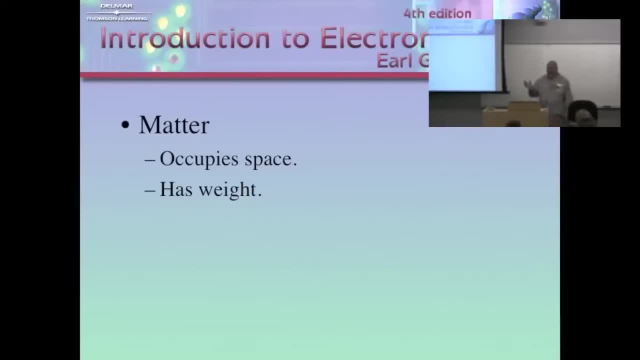 Because there's no matter. There's no matter Now if you're in a spaceship traveling through space and you roll the window down and you stick your butterfly net out and you pick up some cosmic debris and your butterfly net- pretty odd thing to do. 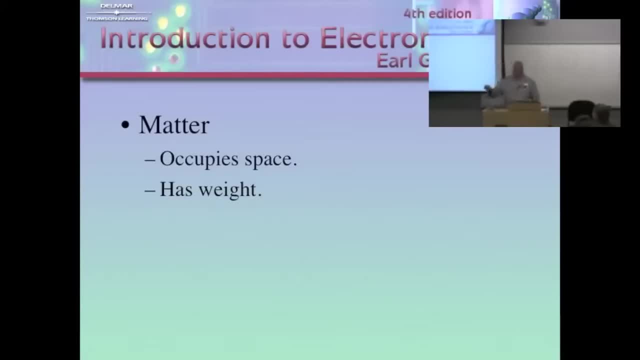 Down a spacesuit, if you're going to roll the window down on the spaceship and do that. But if you find any cosmic debris in your net, that means that you have found matter, Because if it's something and it occupies space and it has weight, therefore it's matter. 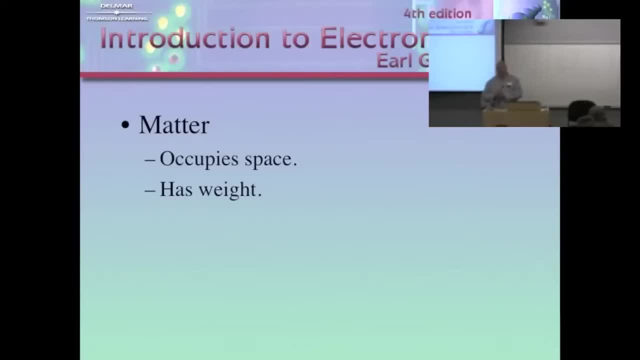 Have any of you heard of antimatter? We will not be talking about that. We're not going to be talking about that here in this program. Okay, I used to think it was science fiction until I was talking about it in a lecture like this. 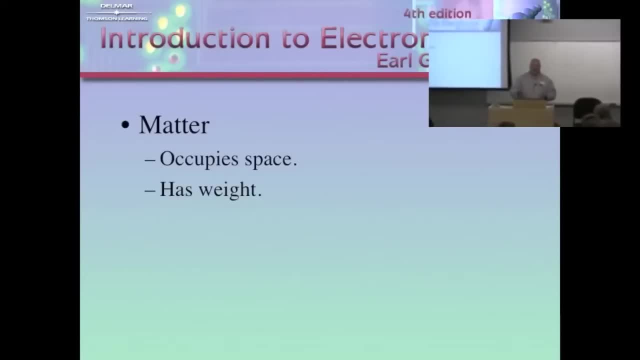 And I had a student raise their hand and we're not going to talk about it because I don't know anything. you know the absence of matter, antimatter, the opposite of matter. And he brought in an article the next week about a NASA project. 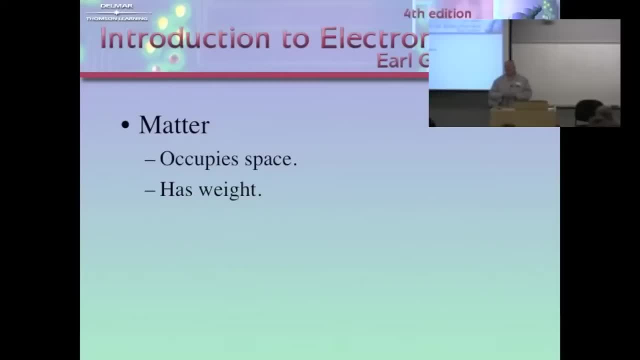 And these NASA teams are all about funding. So all these PhDs and all these scientists: it's all about getting money for them to continue their research. Well, NASA was running out of money and there was a particular group that was doing research. 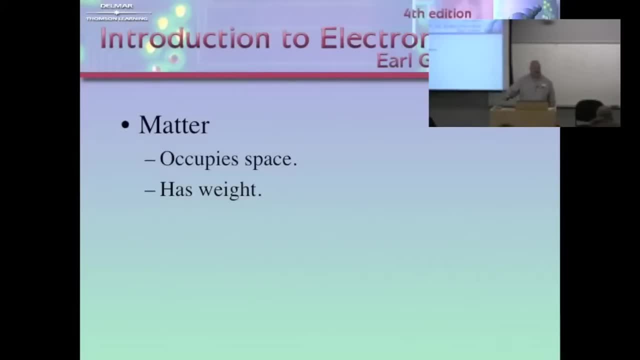 And they were going to get their operation shut down. So as soon as they all were basically put on notice, you all are no longer going to have a job at NASA. They're like, oh sheesh, you know that's too bad. 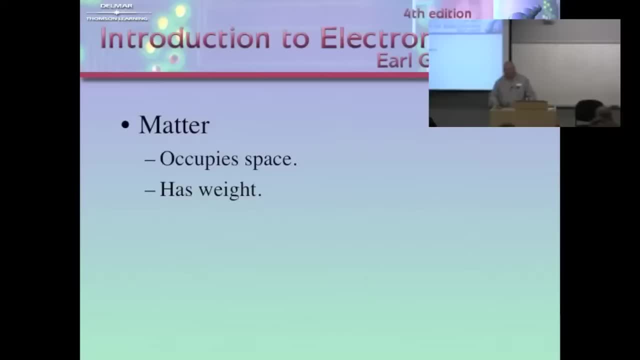 You know that's really bad. Well, why is it so bad? Well, we just discovered a cloud of antimatter And we think it's headed this way. You know, Right away, you know, NASA gives them more money to continue the research. 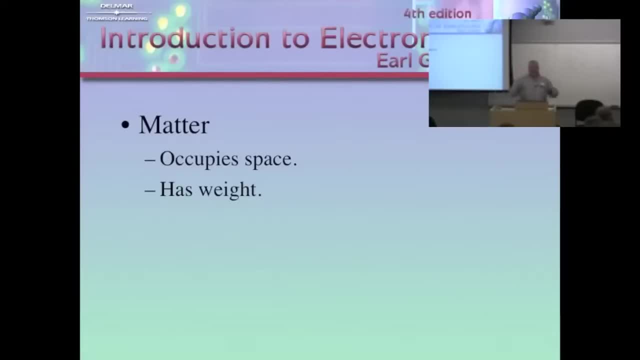 And somewhere in my archives I've actually got a picture of this antimatter cloud that you know. I mean, who knows if it even exists? But obviously if antimatter collides with matter, they cancel each other out. So if there was antimatter cloud that inundated our solar system, 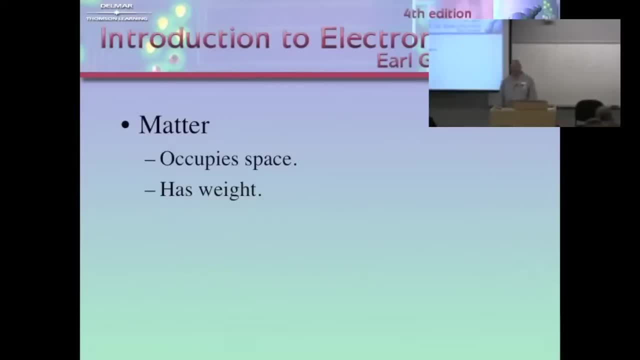 we'd be gone. You know, I don't know where we'd go, But this is what they say. Enough said We won't be talking about antimatter in this class. We're more concerned about matter Now, the basic building block of all matter that we're aware of. 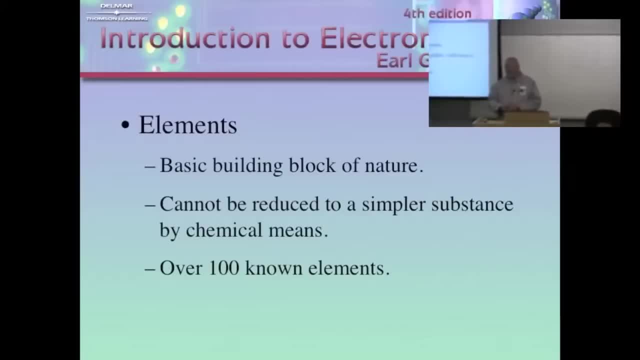 and this is really interesting- is what's known as an element. An element can be found on the periodic table. I must not be a real professor. If I was a real professor, I'd have one of those pull-down charts that's got the periodic table and all the squares you know. 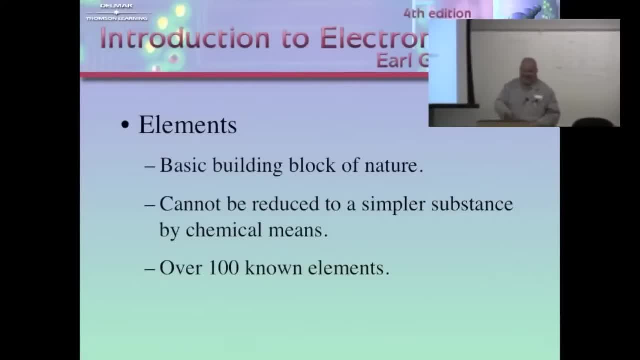 That's the sign of a true professor. I don't have one of those. I could probably call it up on my computer screen, but it wouldn't be the same of having one of those pull-down charts where you go with the pointer right. 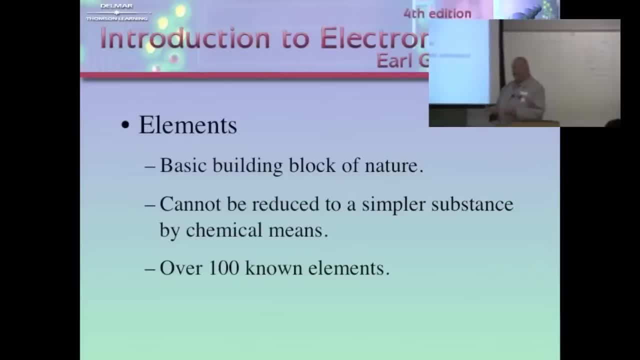 And you've all seen that. You all know what I'm talking about, right? Probably saw it back in elementary school. Elements of the basic building block of nature cannot be reduced to a simpler substance by chemical means And, believe it or not, there are only about 100 known elements in existence period. 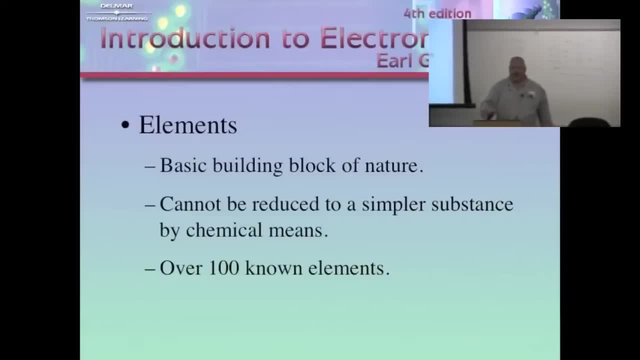 Period: Over 100 known elements Period. That means me, you, that desktop, the chair, a cow, a monkey, a sports car, an airplane- we're all made up of 100 of the same ingredients period. Isn't that amazing? That was one of the things they really didn't know about going to the moon. Were they going to go to the moon and find some new element? They went to the moon and they found the same stuff we got here on Earth. So basically, the assumption is in the scientific community. 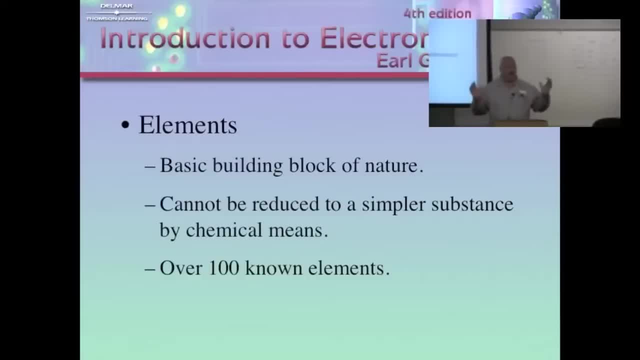 that really the entire universe is made up of about 100 of the same ingredients. I mean I got more crap in my pantry at home: Spices, seasonings, you know, I got all kinds of stuff all over the place. But the fundamental essence of it all, 100 plus elements period. 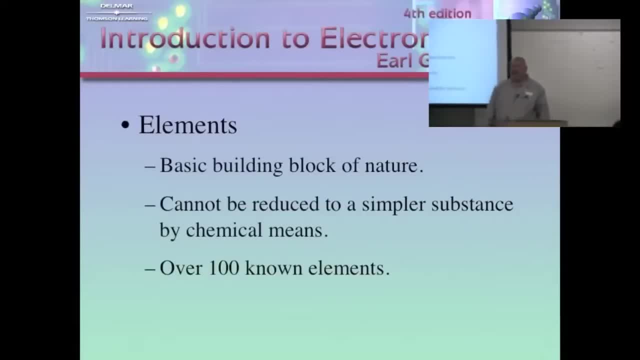 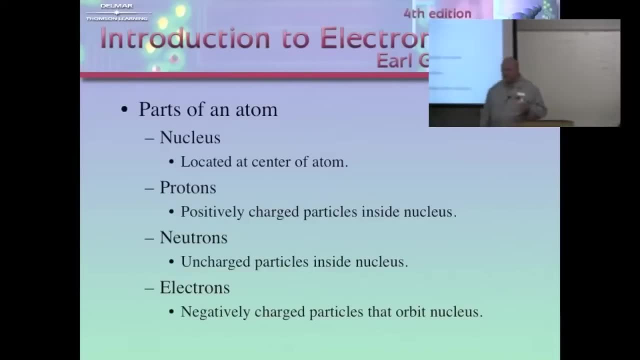 Everything's made up of those. Everything's made up of the same 100 plus ingredients. Now we're really focused on the parts of an atom. So when we have an element, the smallest particle that we could break that element down into and have it retain its identity is an atom. 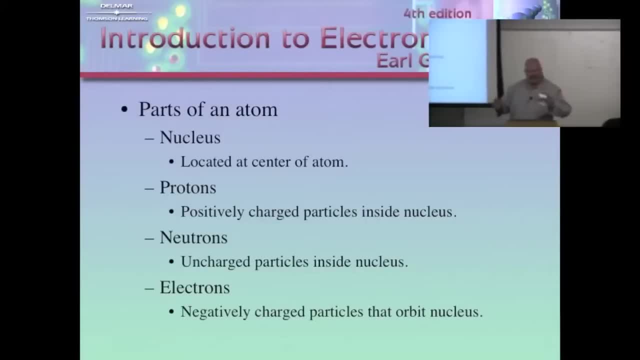 So I know you think I'm going all wacky like chemistry on ya and everything. okay, bear with me. We have to understand the essence of matter so that we can understand it, so that we can get electricity out of matter. That's where we're going with this. 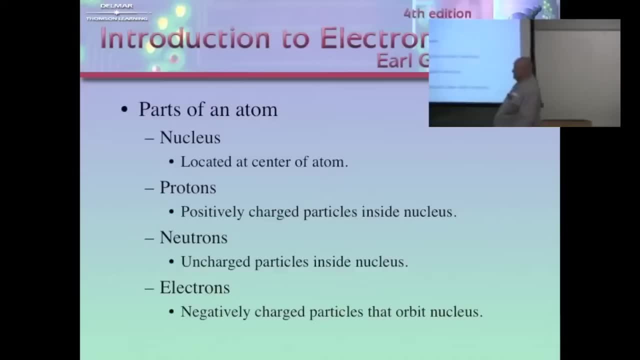 The first part of the atom you need to understand is called the nucleus, And the nucleus is not even really a part. I misspoke that. It's not a part, it's a place, And that place is simply the center of the atom. 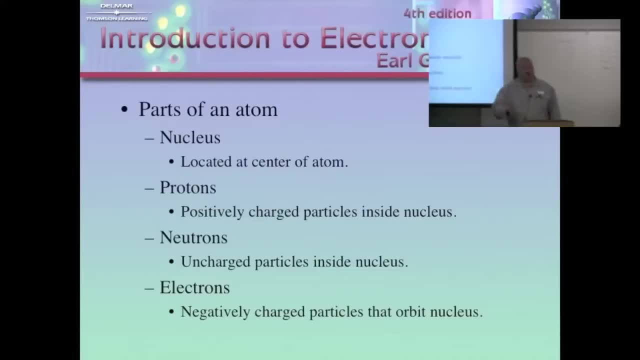 The first true subatomic particle that we're going to talk about is the proton. Proton is a positively charged particle that's located in the nucleus, And I just said something that's very, very significant. I just said the word positively charged. 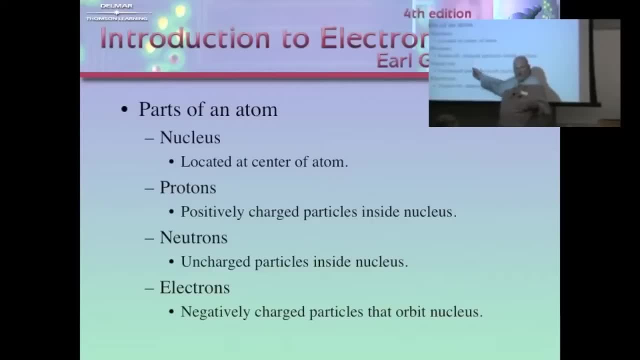 For the first time in this program, we just spoke of something that has an electrical characteristic, a positive charge. So a proton has a positive charge. The other subatomic particle that's located in the nucleus of an atom is called the neutron, And neutrons are uncharged particles. 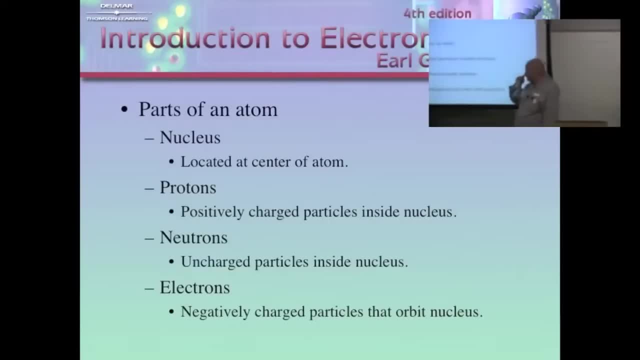 meaning no charge. One of the ways that I remember it always is: proton p-p-p-proton positively charged. Both start with the letter P: Neutron n-n-n-n-n-neutrally charged. Okay, They're not positive or negative. 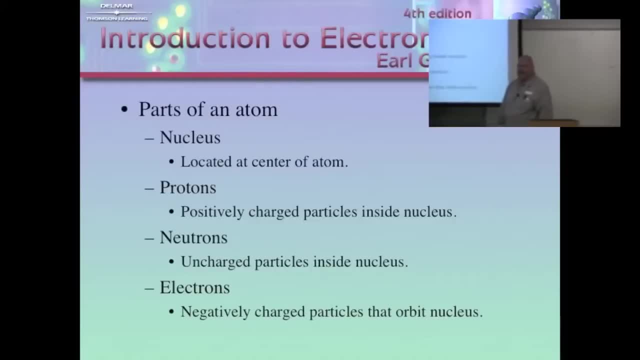 They're uncharged, They're n-n-n-n-neutrally charged. That's why they're called n-n-n-neutrons Electrons. well, that's the other subatomic particle, And if one's charged positive and one is neutral, 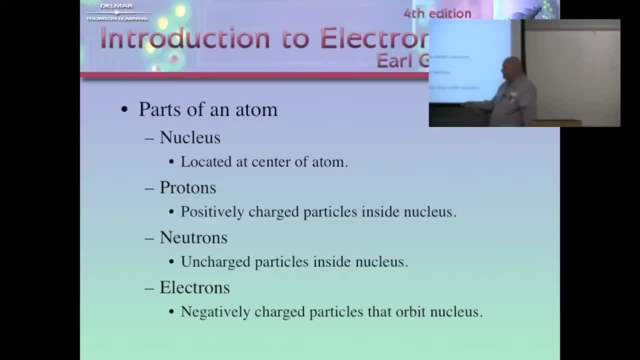 then therefore, the electron must be negatively charged particles. The electron actually orbits the nucleus where the protons and the neutrons are located. This is a very, very significant slide. Remember earlier I shared with you a little bit about my background. I wasn't the sharpest tool in the shed. 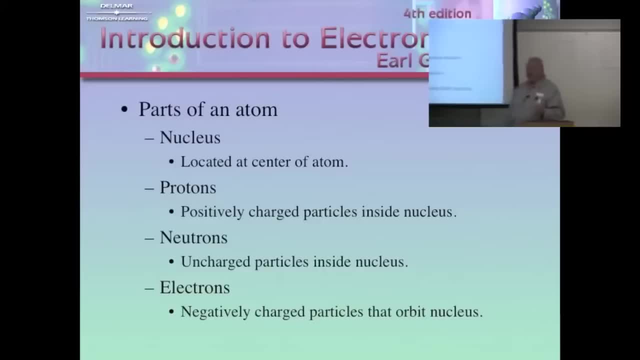 And, as a matter of fact, when I was in the Navy on active duty, my uniform, the Navy- even if you sail on a cruise, even if you sail on a cruise, even if you sail on a cruise, you have a symbol that identifies what division you're part of. 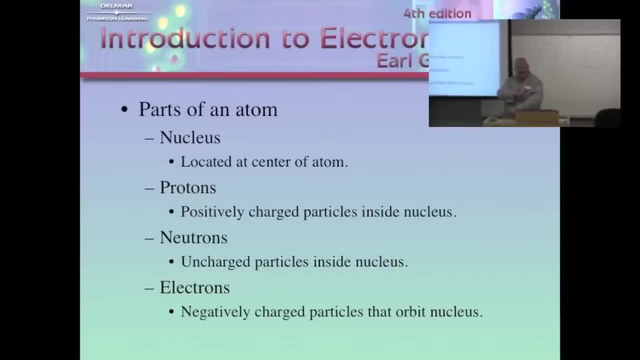 And for me, I had on my arm my chevrons. you know that signified you know my rank. But then I had a helium atom on my arm And that helium atom was to signify matter. And the helium atom with the electron orbiting around the outside. 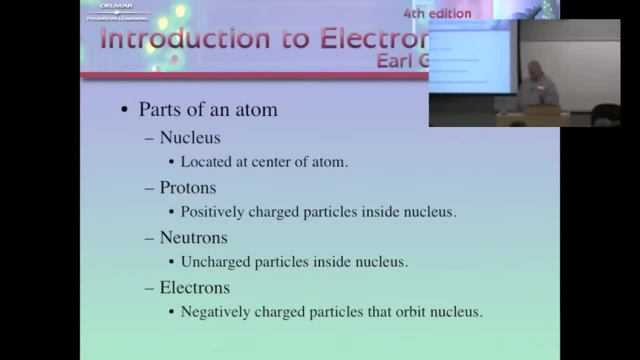 was to signify electrons orbiting the nucleus. Why? Because I was an electronic technician And I basically went for like three years of my career before I realized. why is there like an atom on my arm? Okay, What does that mean? What it means is the electrons orbiting the nucleus. 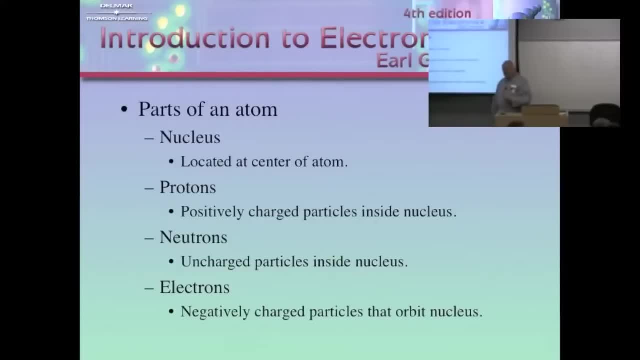 because I was a subject matter expert, a technician, on the behavior of electrons. That's what you're all here to learn. If you're here to learn about electronics, you're here to study the behavior, the behavior of the electron, And that's what we're really going to talk about. 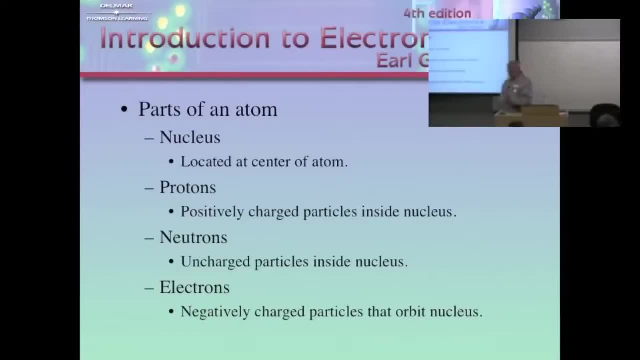 Make sense. One of the things I do not want you to study while you're here in this program- and I'm pretty open-minded If you want to go off and do some projects and stuff like that, I'm all about it. One of the things I really don't want you doing. 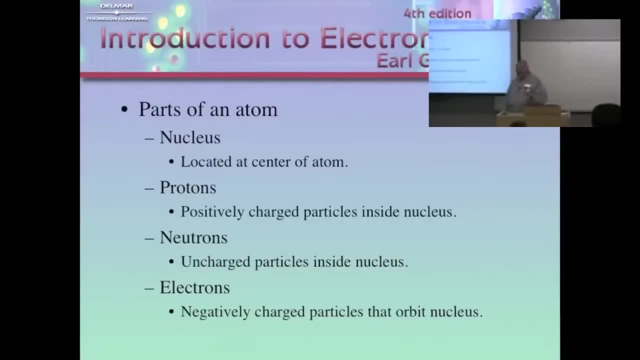 is anything with the nucleus of the atom. Okay. And if you plan on doing anything with the nucleus of the atom, give me fair warning And I think I'll stay in federal way that day, Okay, And then you can have at it and try to split the atom. 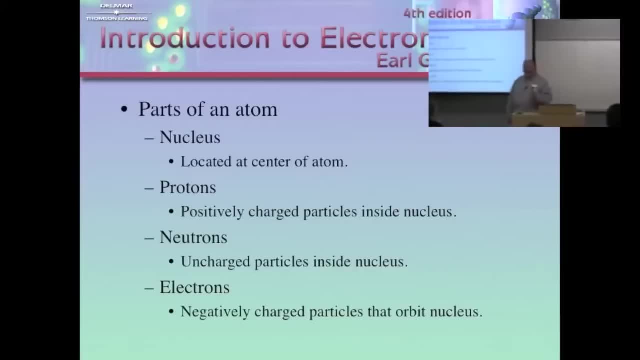 or do whatever it is you're going to do, But when you start playing around with the nucleus of the atom, bad things happen. As electronics professionals, we're only going to play around with electrons. As a matter of fact, we're only going to play around with certain electrons. 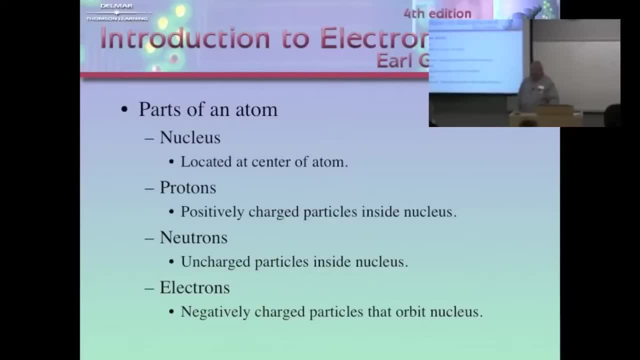 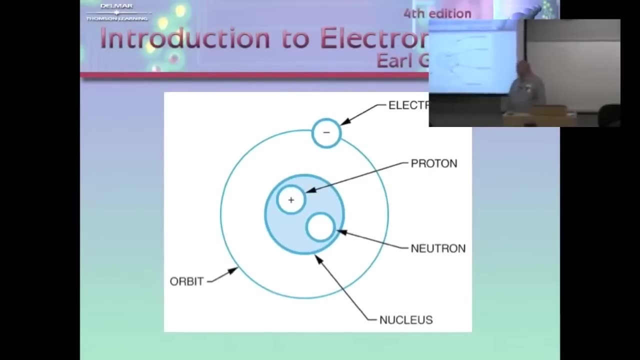 I'm going to share what those electrons are with you in a moment. This is kind of sort of what it looks like. maybe This is an artist's depiction and the scale is really, really off. The proton is a very big particle. The neutron is a very big particle. 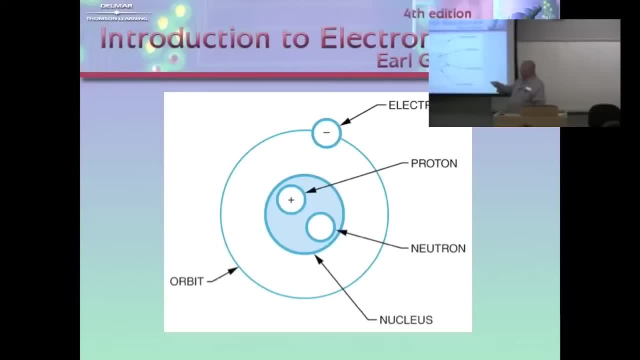 So the nucleus, this is kind of working. okay, This is kind of working for me. The electron, though, is not the same physical size as the proton. The electron would be like the spot of my laser pointer, But, in actuality, if this truly was the neutron and the proton, 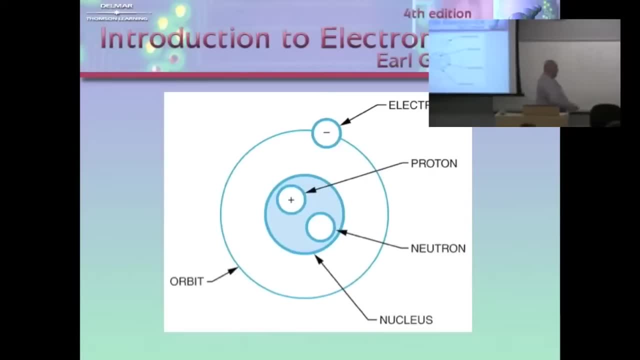 I don't think this spot of my laser pointer would even be in the room anymore. That's how far the orbit is around the nucleus. I heard it once explained as like a cathedral If you had the size of a grapefruit in the center of the cathedral. 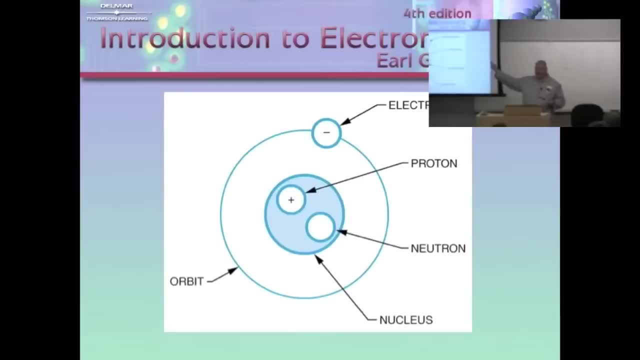 the electrons orbiting would actually be like on the outer walls. It'd be, you know, really really far out there. So the scales here are off, But this gives you an idea of what's going on. One thing I want you to understand also: 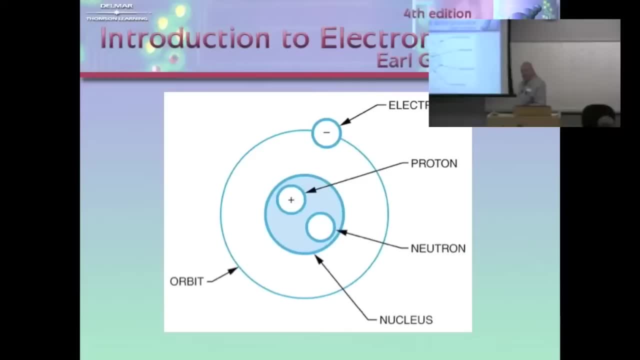 is that, all matter when, in its neutral natural state, has an equal number of protons and electrons. Protons are positively charged, Electrons are negatively charged. They're equal number, so they cancel each other out. That means that matter is equal. 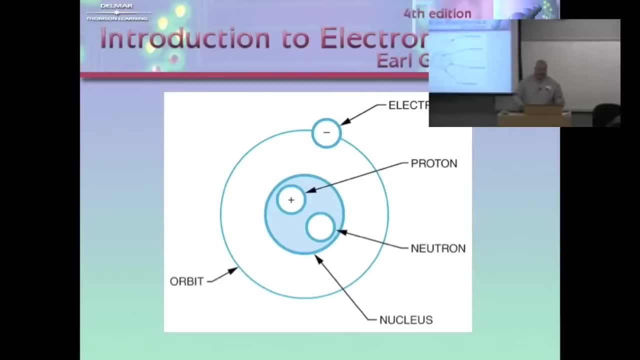 It is in a neutral natural state. Did that answer your question? You had a Balanced, Balanced Right. So there's an equal number of electrons and protons in atoms, until we do something to it- And we're going to talk about that in a minute too. 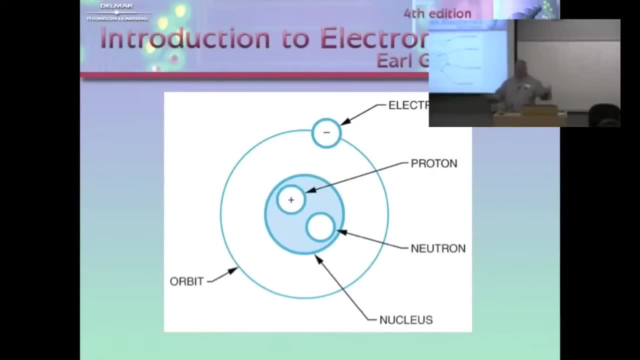 Because we're not just going to let everything stay in a neutral natural state. If we did, we wouldn't have- We'd be out of jobs, We wouldn't have current flow. We wouldn't have current flow, It'd be a drag. 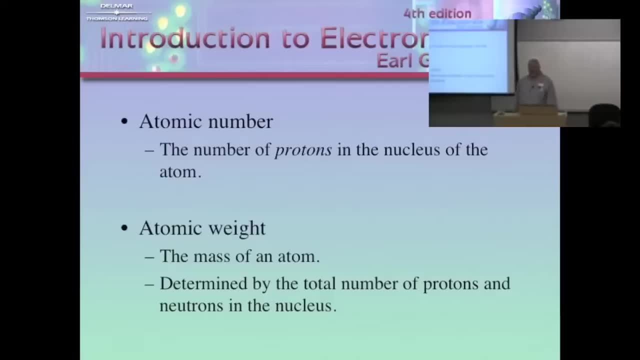 A couple of the numbers that you need to familiarize yourself with, And one of the things that I want to stress to you is that all of you are here taking electronics courses. You're here to learn the language of electricity and electronics. That's really what it is. 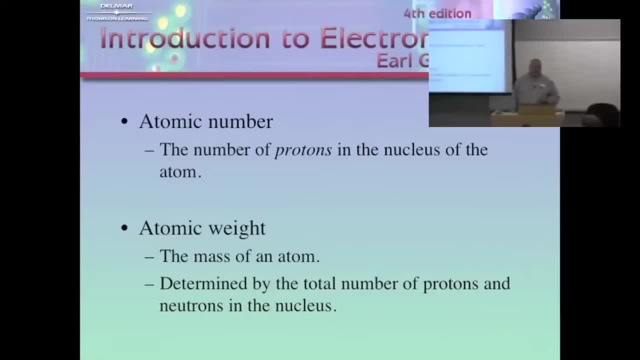 It's just like taking a second language. I've actually had a lot of students that speak different languages and English is a second language and they wonder if they could come in and do it. It's like, yeah, you could come in and do it. 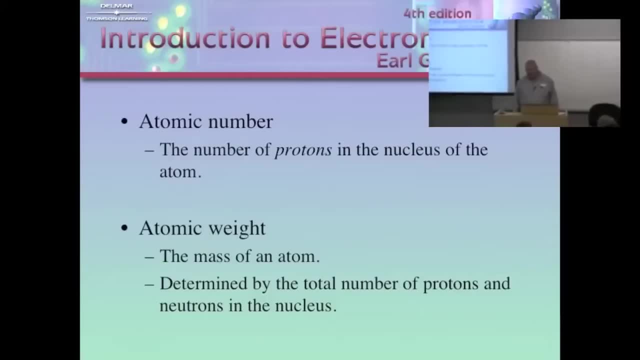 Because you know what. What I'm talking about here is another language, So I'm going to give you a couple of examples. So one of the technical terms that we may use in the future is a number called atomic number. An atomic number simply is the number of protons. 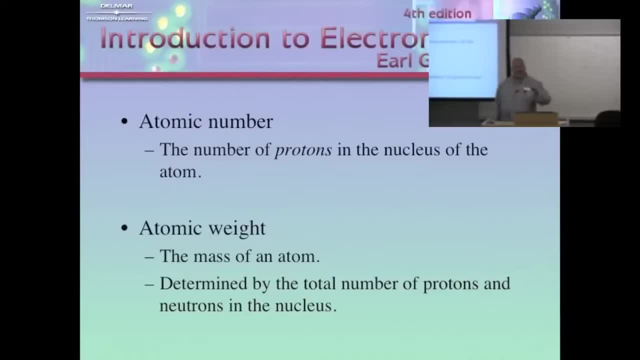 in the nucleus of the atom, And every one of those hundred plus elements that I talked to you about earlier has a unique number of protons. You don't have two different elements that have the same number of protons. So the scientific community embraced this. 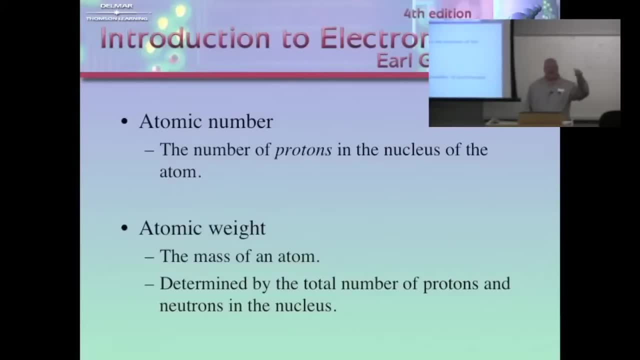 and they said: you know what? Why don't we just use the number of protons? and that's going to give it its position on the periodic table. Make sense, Okay? The next number I want you to familiarize yourself with is the atomic weight. 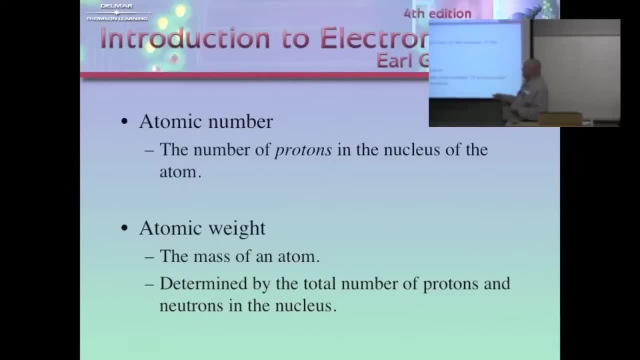 And the atomic weight deals with the mass of the atom, its weight, its physical weight. And remember when I said that protons and neutrons were big and they were contained in the nucleus and the electron was just like a little tiny subatomic particle. 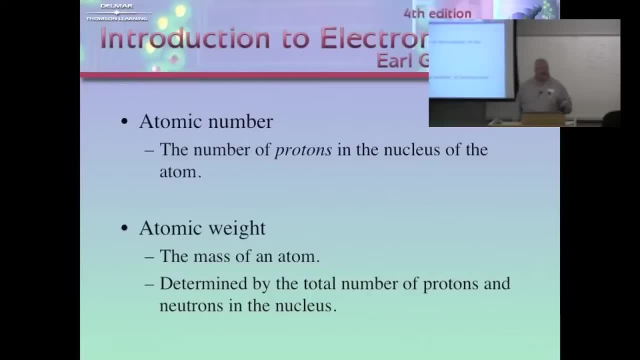 orbiting way outside. Basically, to end up with atomic weight, all you do is count up the total number of protons and neutrons in the nucleus. Count that up. that gives you the atomic weight. Every weight of every element on the periodic table is unique. 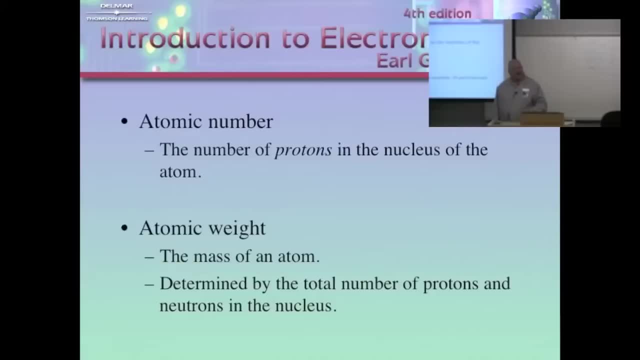 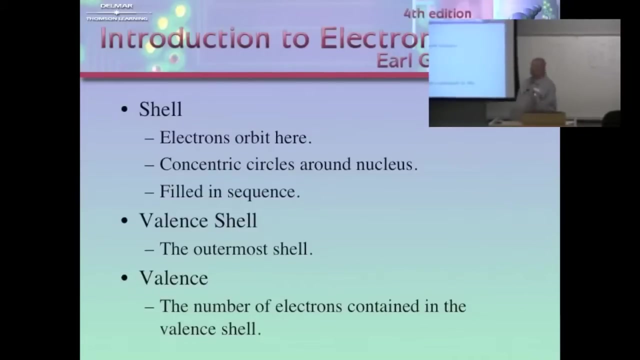 And basically the mass of the electron is so insignificant we don't even take that into account in determining the atomic weight. Make sense, Now? this is where things get interesting. First term: shell. This isn't the kind of shell you find by the seashore. 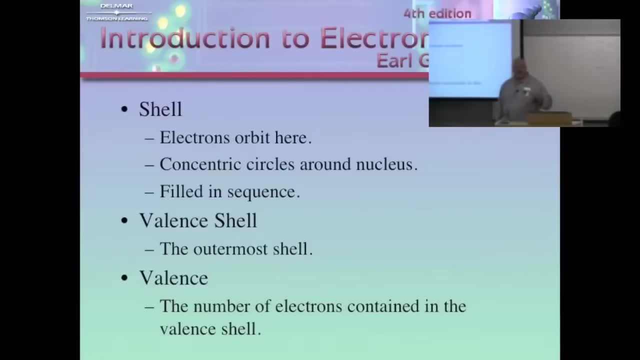 What we're talking about here for shells is simply an orbital path around the nucleus. This is where the electrons orbit. They form concentric circles around the nucleus and they're filled in sequence. Have any of you here been to a parking garage like down at Sea-Tac Airport or Bellevue Square? 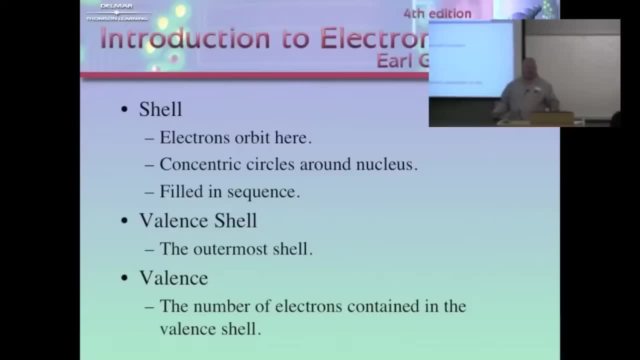 I don't know about you and again, I'm not the smartest guy, but normally I want to park at the first level I can find a space at. So what I'll do is I'll go to the first level and I'll drive around. 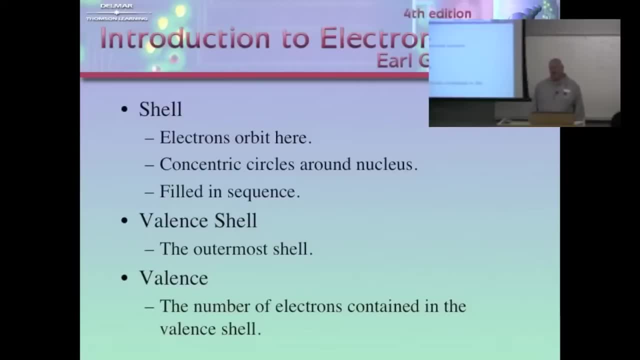 And if I can't find a parking space, where do I go? Up to the next level? And then I drive around. And if I can't find a space there, where do I go The next level? And I keep doing that. 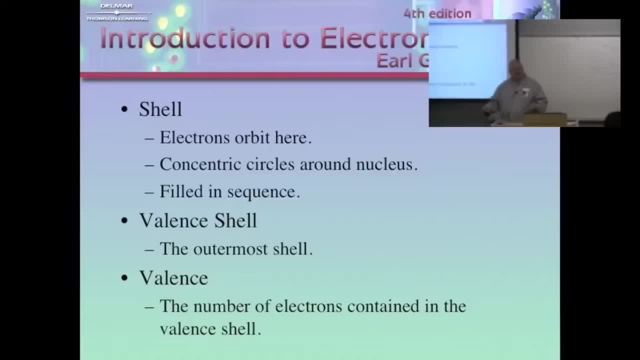 This is how shells are filled in atomic structure. When the first shell gets filled, then electrons start going out to the second shell, and then the next shell, and then the next shell. So our most complex atoms in existence have electrons in shells that are way out there. 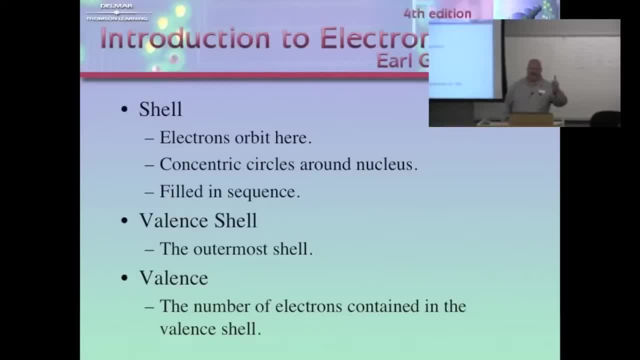 Because they have the highest number of electrons, And the higher the number of electrons, the higher the number of protons, Because, remember, they have to be equal. Make sense Now. the shell that should most concern you is this valence shell. 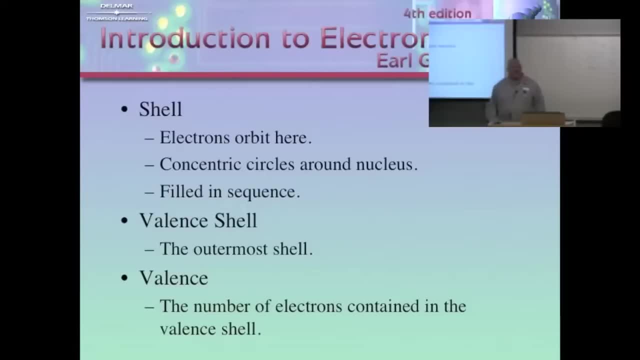 This is the outermost shell. If it's a complex atom, it may be way out there. If it's a simple atom, it's going to be real close to the nucleus, And I'll talk to you in a minute why that's. 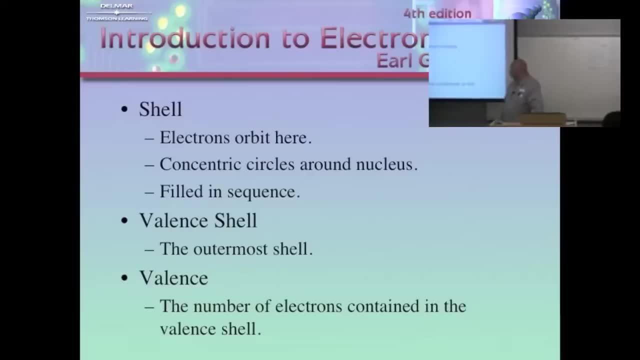 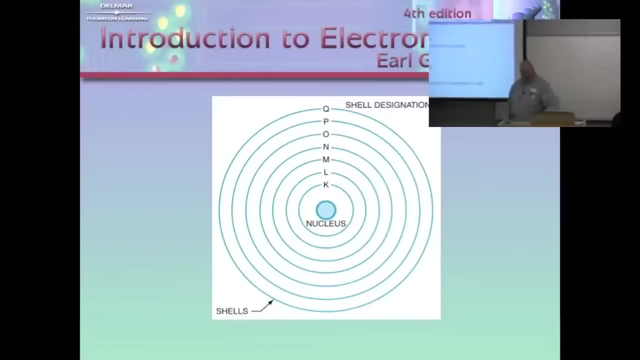 It's important for two different reasons. The number of electrons contained in the valence shell also refers to the term valence. Now, this is the scheme that they came up with in naming the shells. If we have a simple atom, let's say we've got an atom that contains one electron. 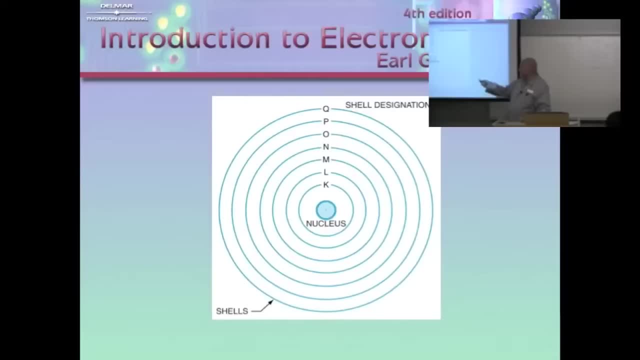 That one electron is going to be parked in the lowest level, And we're not going to call it the lowest level- No, that'd be too easy. We're not going to park it in what's called the first shell, because that would be too easy. 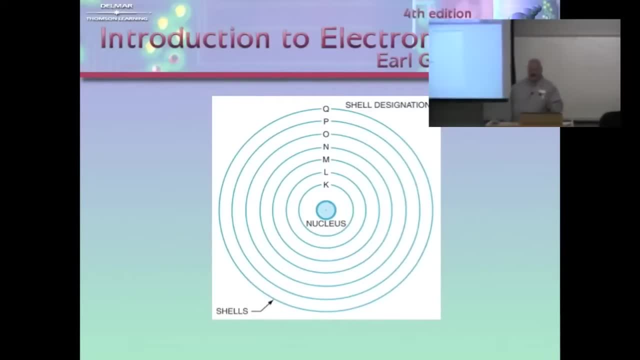 You're here to attend college, okay, to get educated. So we've got to not call this the first shell or the A shell. We're going to call this innermost shell, the K shell. Why, I don't know. It helps us educated people justify our existence. 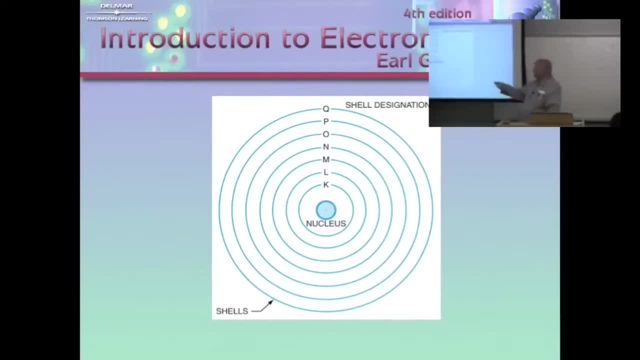 After the K shell comes the. This is the part that actually makes sense to me. After K comes L, M, N, O, P, Q. So I did okay with the alphabet, So it kind of makes sense. So what this means is the Q shell. 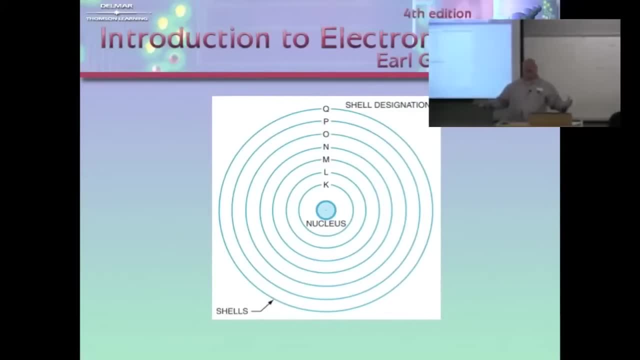 the most complex element that we have found in the universe contains electrons in the Q shell. Does that make sense? If it's a simpler element, an element with a lower atomic number, that means it's going to have electrons, maybe only in some of these shells. 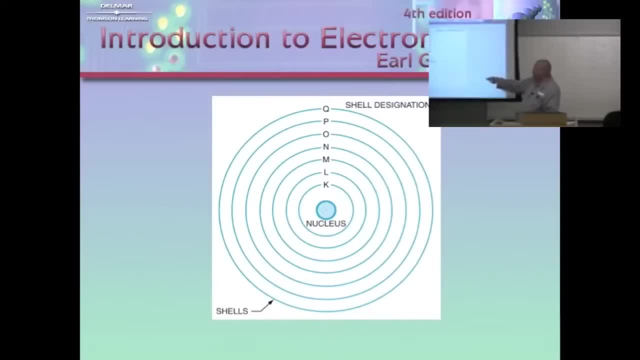 But we have to fill a sequence: first fill this K shell before we bump an electron up into the L shell. when L gets filled- And some of you that have maybe taken chemistry and some physics classes know there's a certain number. I don't want you to memorize that. 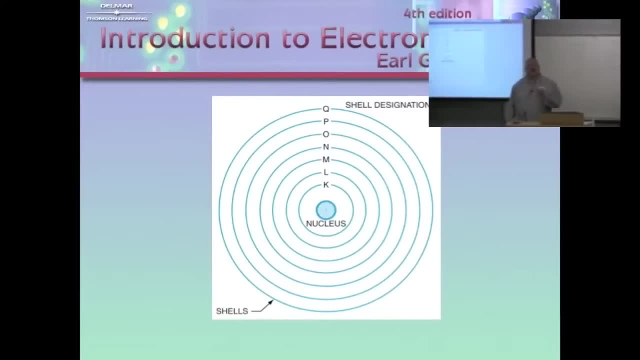 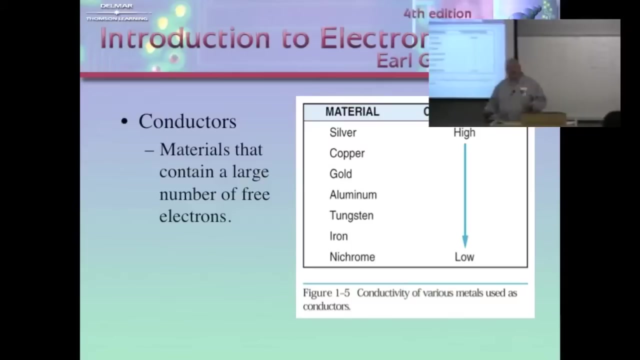 That's not going to help you become an electronics professional, But just remember, there is a limit of how many electrons you could park in a shell before the electrons have to go into the outer shell. Now why am I talking to you about all of this stuff? 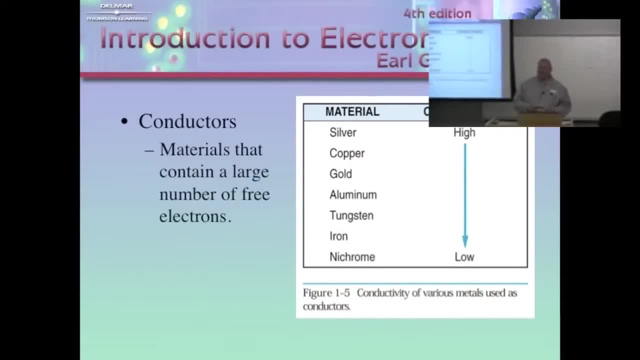 Again. this was a question that plagued me for about three years since I was educated, Like: why were they teaching me about all the subatomic stuff? I'm not going to be some mad scientist, you know. Why do I need to know about the periodic table? 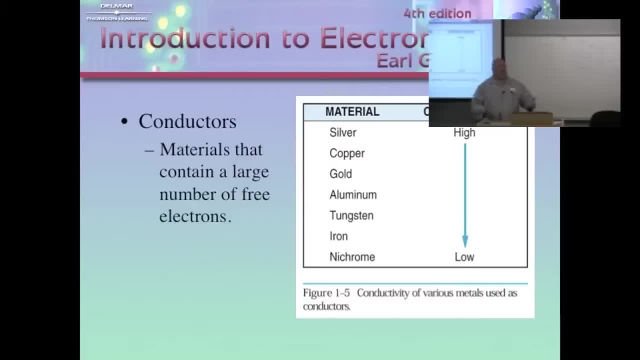 Why do I need to know about subatomic structure? You know. I want to learn how to use a multimeter to take voltage readings. I want to know how to use an oscilloscope to take readings. Why do I have to understand subatomic shrubbery? 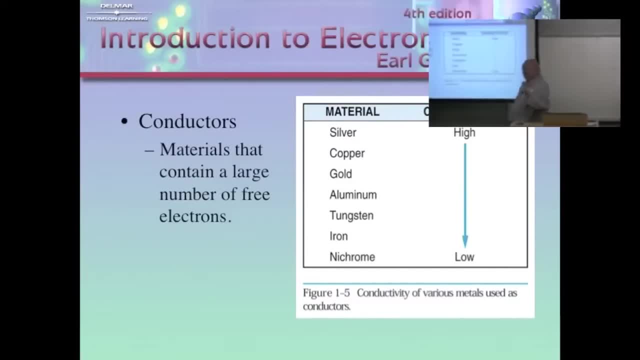 Two reasons you need to understand subatomic structure. Number one is so you could identify the properties of materials that we use in electronics. That's first and foremost. Secondly, you need to understand where voltage comes from, And we're going to talk about that in a minute. 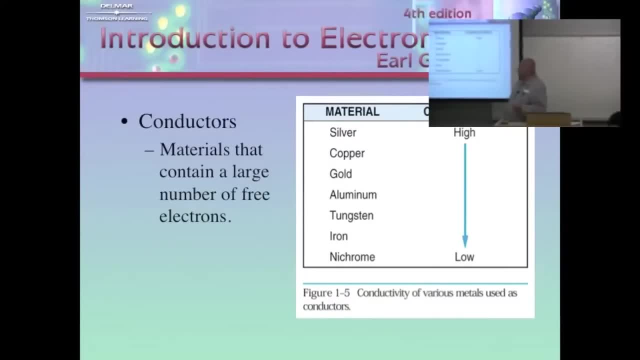 First, let's talk about some of these materials and their properties: Conductors: How many of you are familiar with conductors? Conductors: That's the guy that runs the train. Is that the conductor? I actually saw that the other night. 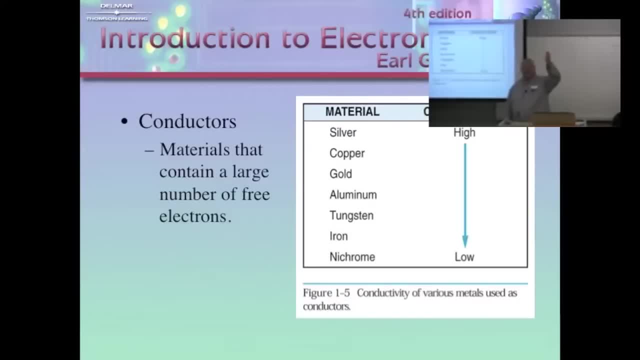 What's that movie Unstoppable? How many of you have seen the movie Unstoppable? It was actually a pretty good movie. You haven't seen that one. It was pretty good, wasn't it? Train running out of control. 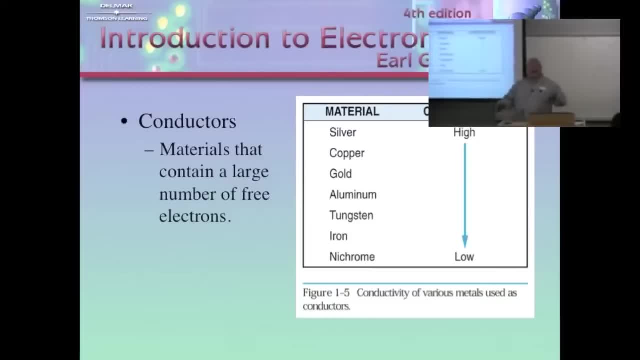 Based on true stories. It was based on a true story. Let's set the throttle and jump off the train and switch the track and jump back on it. It just didn't work out very well. Anyway, that's not even what we're talking about. 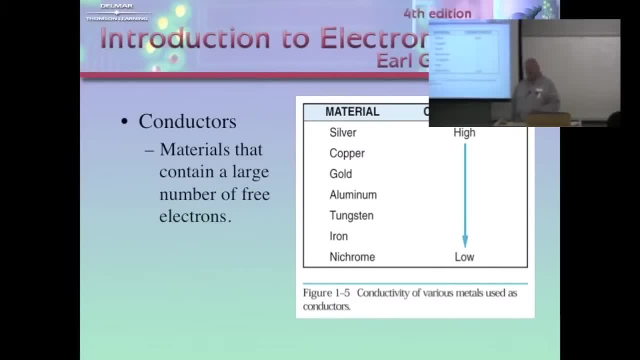 Conductors. We're not talking about train conductors. We're talking about conductors, electrical conductors, Materials that readily accept the flow of electrons, or electricity, if you will, Categories. Categorically, the textbook says they're materials that contain a large number of free electrons. 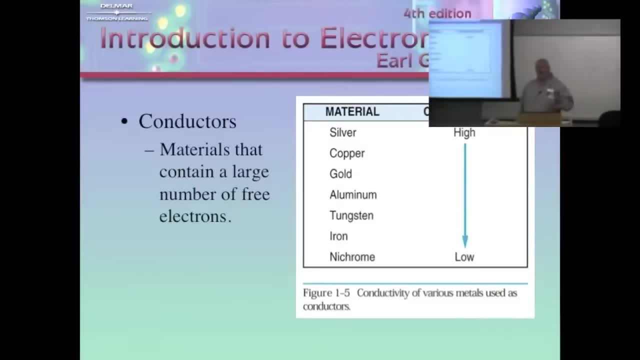 However, I want you to think of it in a different way. When I speak of conductors, I am speaking of materials that have three or fewer electrons in the valence shell And, by the way, in this class, in this program. 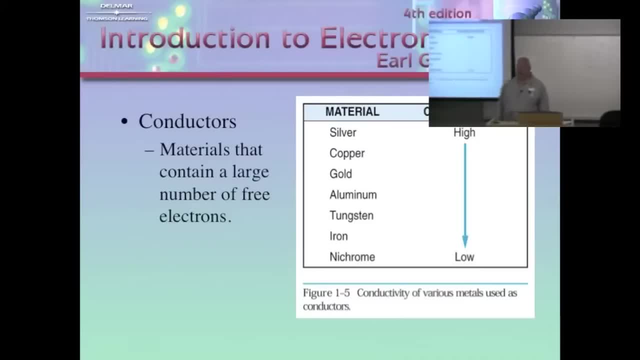 the only shell that you will ever work with for safety reasons is the valence shell. If you plan to experiment beyond the valence shell again, let me know And I'll probably stay home that day. Okay, So it's only the valence shell. 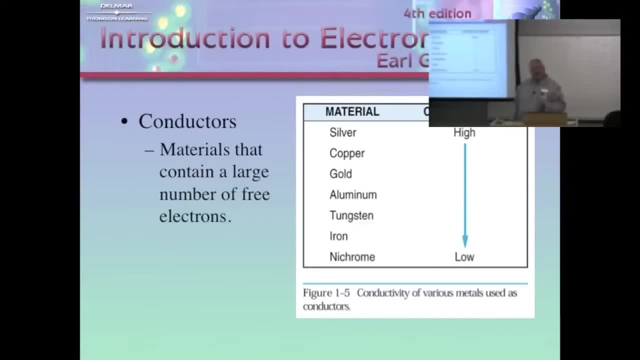 So if you've got an element that has three or fewer electrons in the valence shell, it's going to potentially be a good conductor. Now, in order of precedence, the material that has the best conductivity or conductance is that of silver. 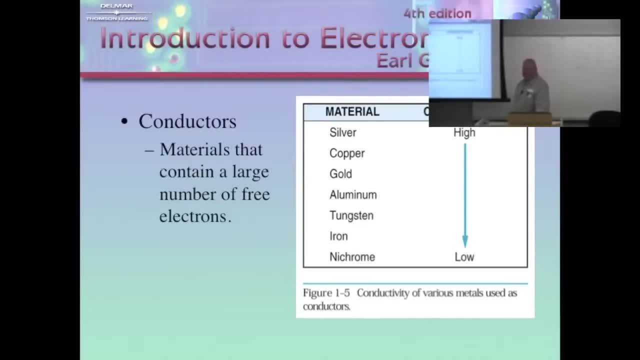 Silver. believe it or not, that's the best found in nature Out of all the elements, silver is the best, Followed by copper, gold, aluminum, tungsten, iron, nichrome and silver. Okay, Silver is the best. 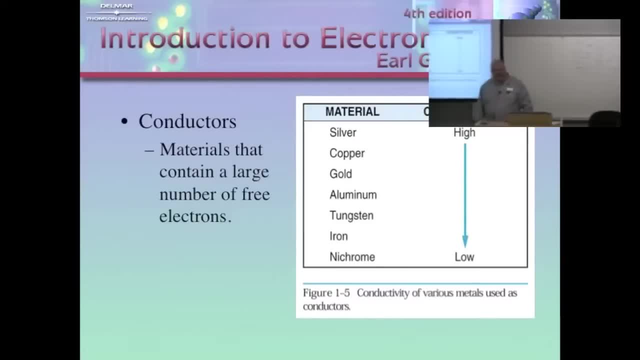 If silver is the best, why, when you buy a stereo, why, when you buy audio-video equipment, do they try to sell you gold-plated patch cords? Okay, we've got one response there: Money. yeah, They could get more money out of you. 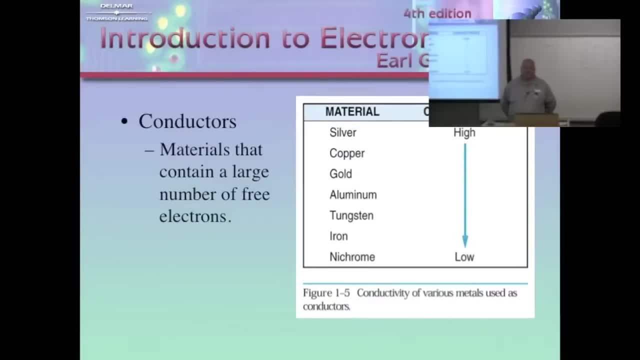 It's corrosion. Silver has a higher corrosive potential than gold, Absolutely, Absolutely. Copper is a little bit more corrosive than gold, but not as much as silver. So basically, gold is the least likely to oxidize and corrode. 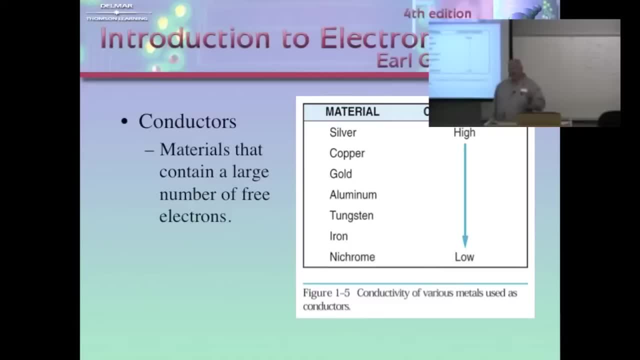 So when we get copper wire and plate it with gold, we get a good conductor, because gold is still a good conductor, but it won't oxidize. If you're scuba diving in the Caribbean and you find a treasure chest full of gold, 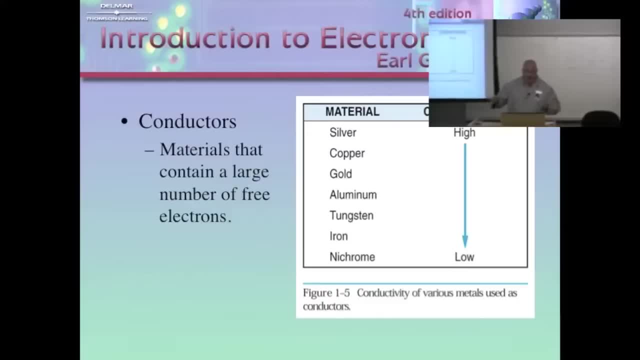 that's been sunken hundreds of years under water and you dig it out of the sand and you open it up under water, salt water, hundreds of years. you open it up. you would know that you found gold because it would look as good. 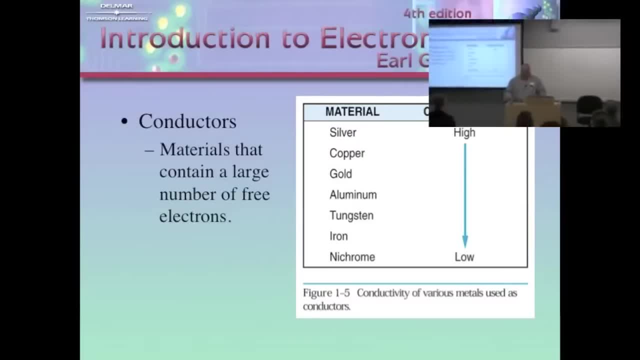 as the day that that treasure chest fell off the pirate ship. If you found a treasure chest under the ocean in the Caribbean and it was filled with silver and you pried it open, you'd be like ugh, what happened in there. 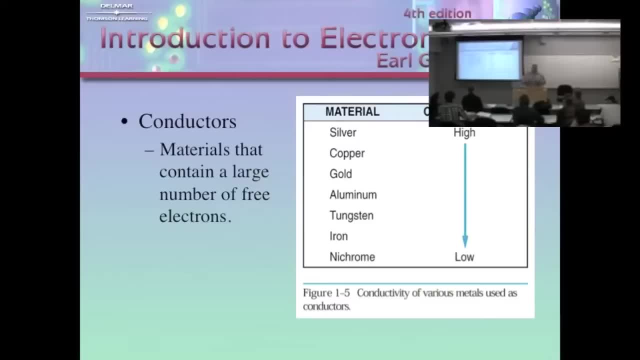 Because it's all oxidized. Of course there's still good silver in there, but the exterior would be oxidized. So that is why we use gold-plated connectors. Don't oxidize. We live in an oxygen-rich environment. so if I could have gold-plated connectors. 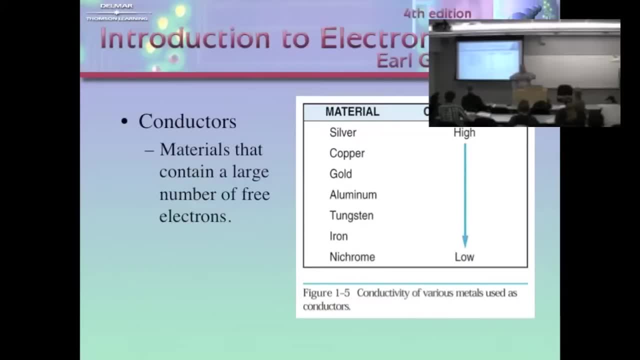 gold-plated connector to connector and I could mate the two. I'm going to get the best possible electrical connection that I can Now. do you really need to go out and buy those gold-plated audio-video connectors? It's actually kind of funny. 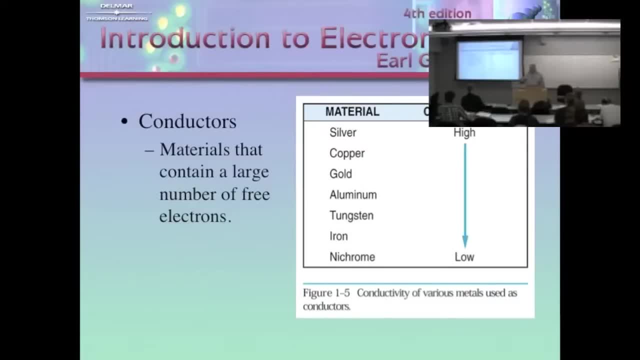 because I've seen a lot of people go out and spend good money on those and then they plug it into the back of a dusty amplifier. It would have been better for you to go out and get some technical-grade alcohol clean the male-female connectors. 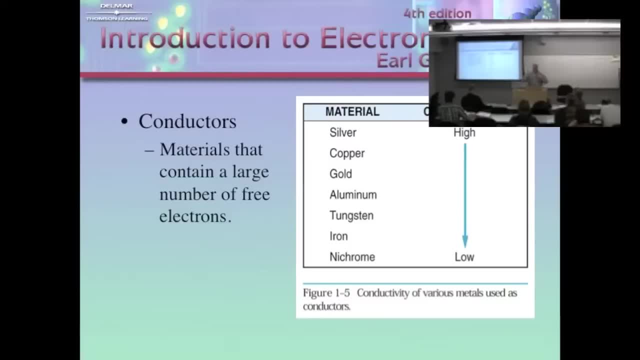 connect them and you'd get a better electrical connection. Now, in a perfect world, a totally clean gold to totally clean gold- clean, nice, no dust- is going to give you a superior connection. We actually learned a lot of this. 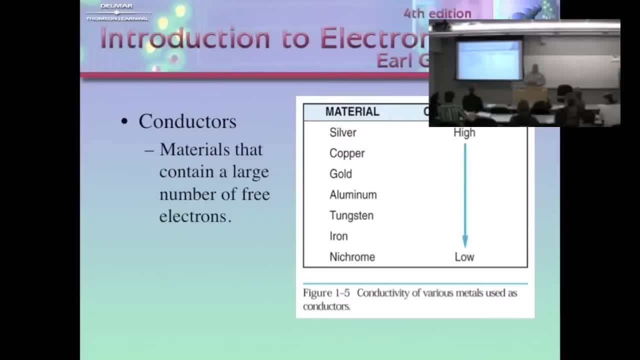 was developed in the space program Because- think about it- to basically send people to the moon and have them get back and have those electronic circuits needed to be highly reliable. So this is where NASA started playing around with. everything is interconnected. You can't permanently wire everything up. 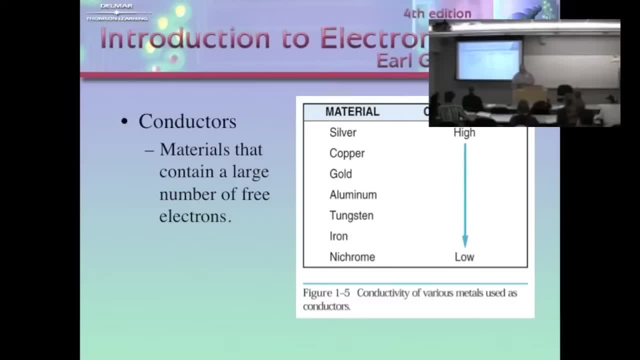 You have to have boards and sockets and everything is interconnected like that. So NASA did a lot of research and they said, hey, we plate the stuff with gold, we'll be golden, you know. And literally that started that whole trend in electronics. 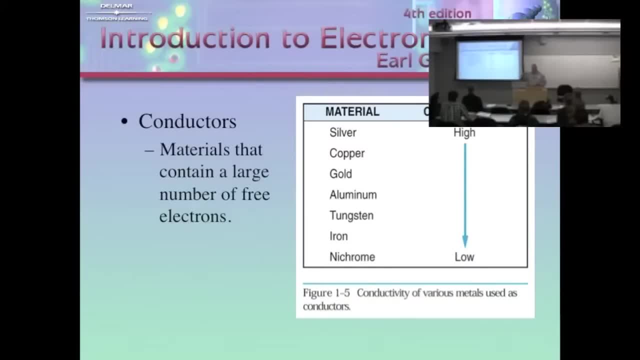 A lot of the circuit boards and stuff that you buy your computer motherboard, you know your video card have gold plating on it, so they make that connection and it's a highly reliable connection. Big thing I want you to remember though. 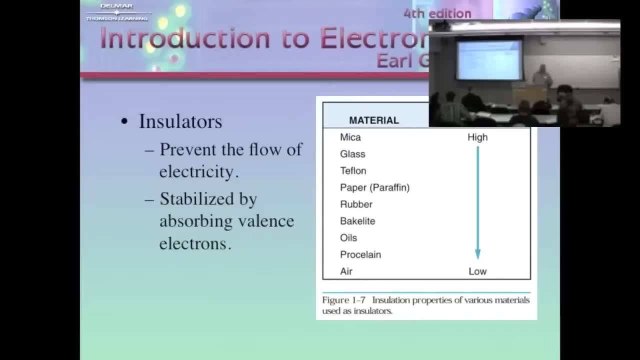 three or fewer electrons in a valence shell. Insulators are materials that prevent the flow of electricity. The textbook says they're stabilized by absorbing valence electrons. The material found on planet Earth that has the highest insulative quality in nature is mica. 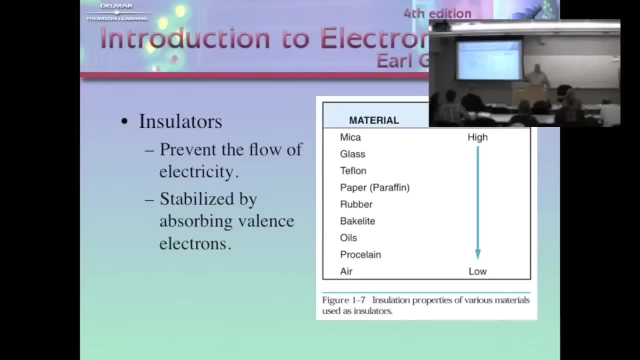 Any of you know what mica is. It's found in rock formations. It's very fragile, It's a good thermal insulator and it's a good electrical insulator. A lot of times it's found in quartz formations and it's almost like paper. 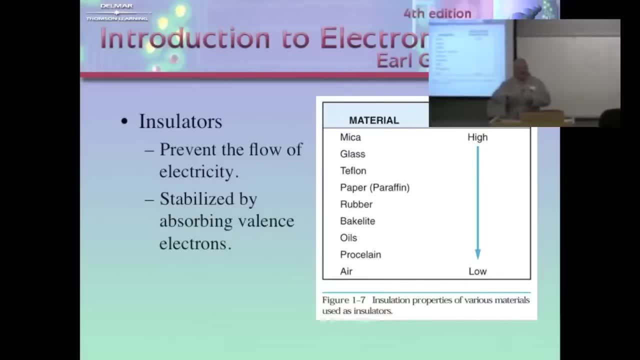 like you can kind of peel. There's one layer and another layer and another layer, but it's highly fragile. That, for thickness, is the best insulator that we have found in nature. That's why it's at the top of the list. 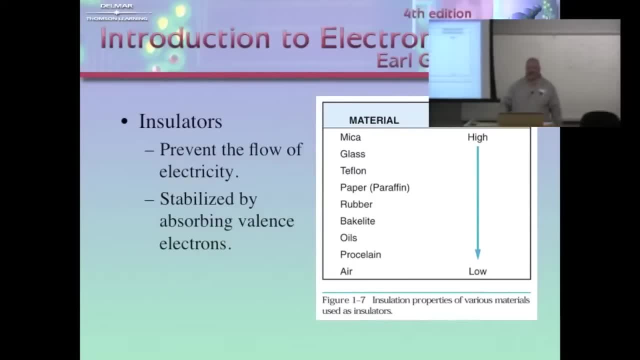 That's what we compare everything to. Glass is high, but not as high as mica, followed by Teflon paper, wax paper, which is used in the manufacturing of some electronic components, rubber, bakelite- You know what bakelite is? 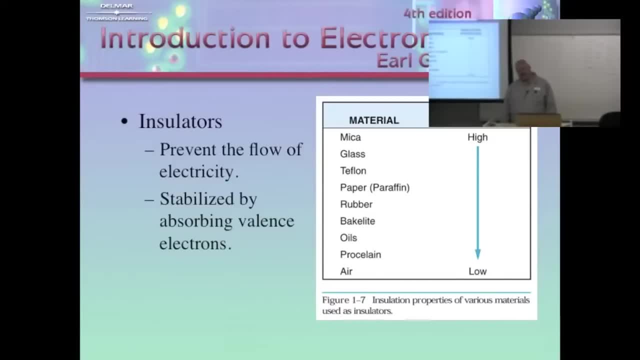 Bakelite is like the handle on your toaster oven and like when you drop it it chips it and you can't glue it back together. It's not only a good electrical insulator, it's a good thermal insulator. It's that black stuff, that again. 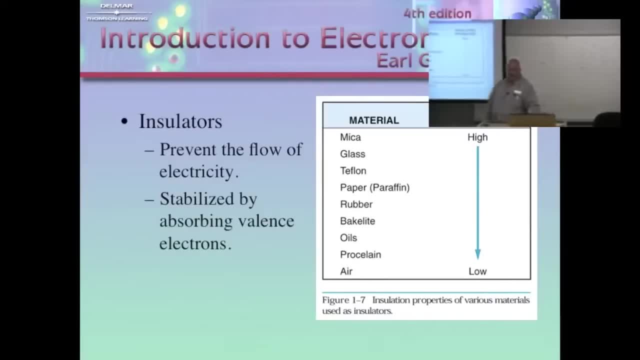 you chip on your pots or pans and you can't fix. Isn't that the original form of plastic? Yes, Yeah, it is one of the original forms of plastic, if you will, that they used as a composite, if you will. 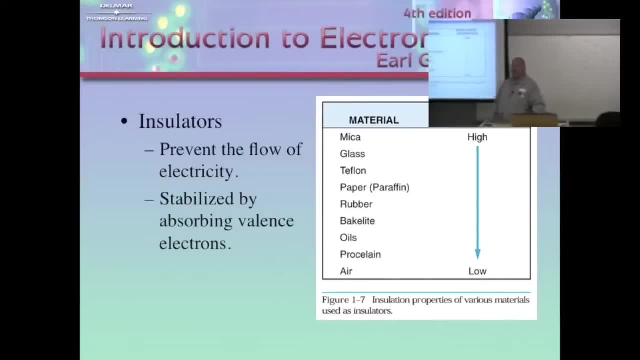 Oils. A lot of oils are used. They used to use a lot of oils that had a lot of poison in them for, like, electrical transformers, But we kind of got out of that because oil is an insulator. And it's nice because oil 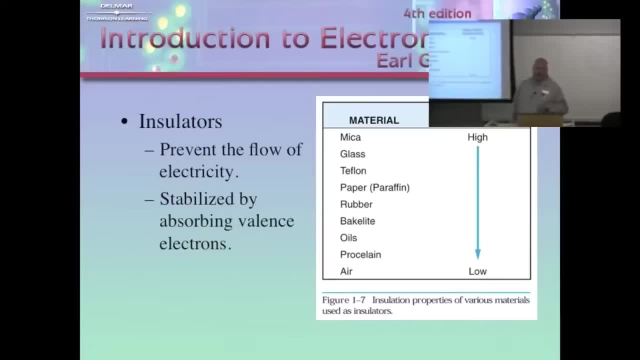 will draw heat away from circuits. So if you had a circuit submerged in oil, if any, what do you call them? computer heads here, PC files. you know, one of the big problems we know with PCs are heat, the generation of heat. 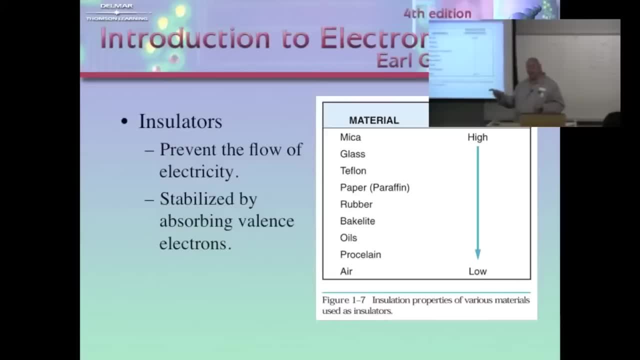 in the processing. So one of the big things is, if you could super cool a computer, you'd get more performance out of that computer. So if we got the computer, don't try it again with my computers, but if we got it and submerged it. 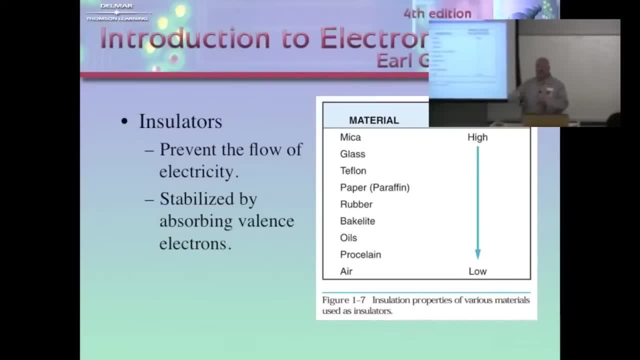 into a vat of oil, and then we cooled the oil and recirculated it. we could draw more heat away from the circuit and then we could start bumping up the speed of the computer and, in the industry, overdrive the chip. 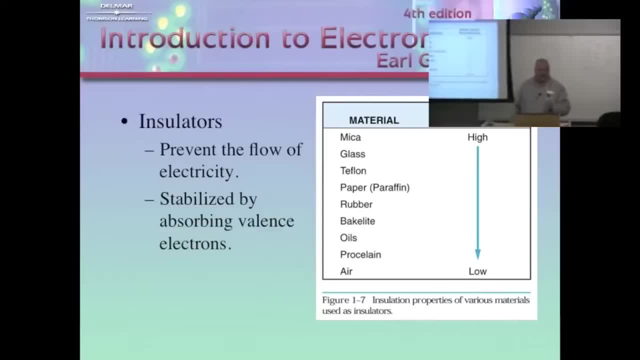 Ask more of the chip than what it's rated for Yup, Porcelain. And, of course, air. Air is an insulator, isn't it? If you've driven under power lines, what's between the power lines, Air? I don't know if you've ever driven under. 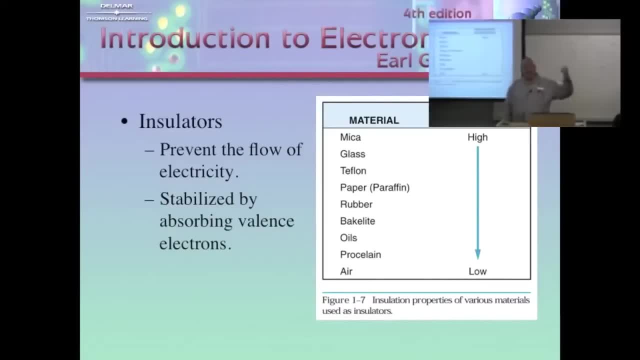 or walked. do some walking, hiking under the BPA power lines down south, and on a day that's damp you could actually hear the. It's like wow, Air is the insulator and I guess it ain't working too good right now. 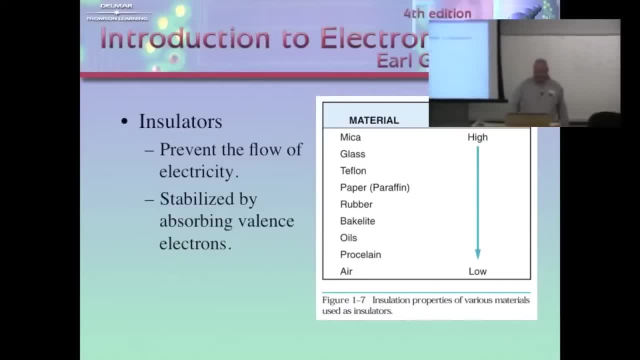 Hope it doesn't arc to me. There's also a category of materials that are called semiconductors. Semiconductors are materials that could be altered to function as either a conductor or an insulator. Let me go back. I left out one thing here. 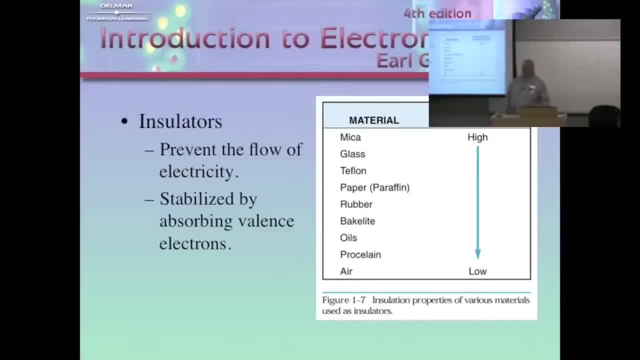 Insulators are materials that have five or more electrons in the valence shell. Five or more electrons in the valence shell. So conductors were three or fewer, Insulators, five or more, Five or more. Anybody want to take a wild guess? 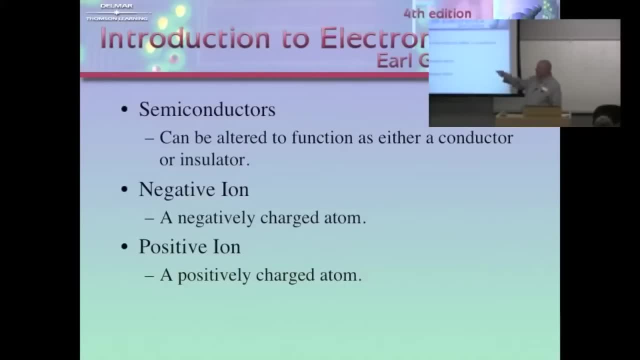 what a semiconductor might be, One that could be altered to function as either a conductor or an insulator. Anybody want to take a wild guess? Four: You all could have been scientists back in the 1940s, Because that's basically. 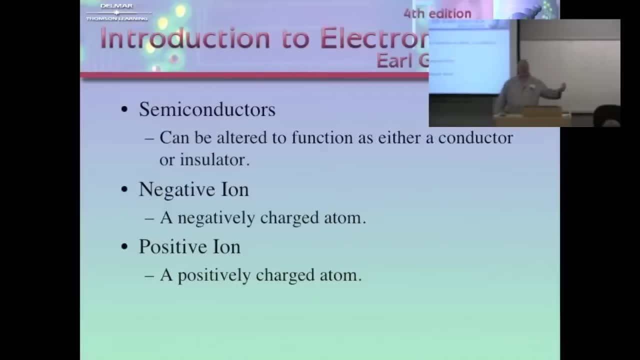 what they came to the conclusion. We know the properties of conductors. We know the properties of insulators. What happens if we start playing around with something that has four electrons in the valence shell? We could get it maybe to swing both ways. 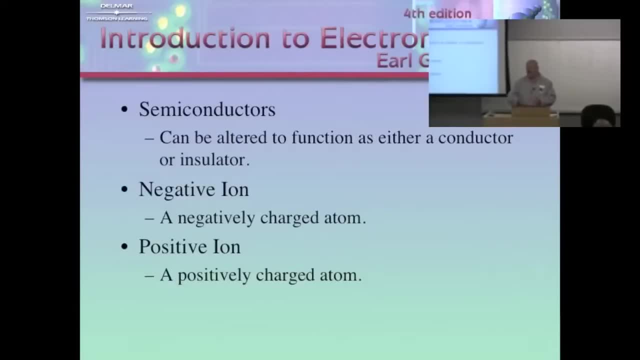 depending on how we want it to behave at that moment in time. And, as you know, semiconductors are the fundamental building block of diodes and transistors. Transistors are the fundamental building block of computer microprocessors. That's all a microprocessor is. 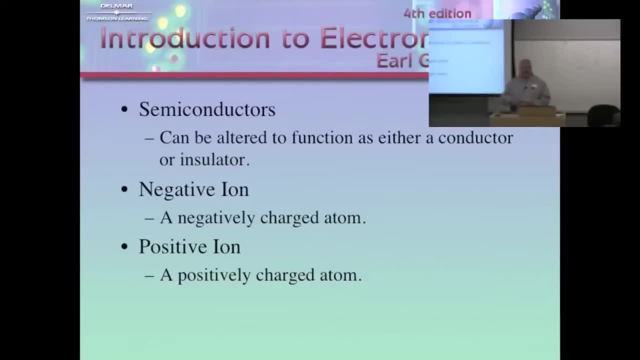 Now, in essence, billions of transistors on something the size of a postage stamp, Made of materials that have four electrons in the valence shell, Those materials that you're going to study later on in the program, not real important now for you to know. 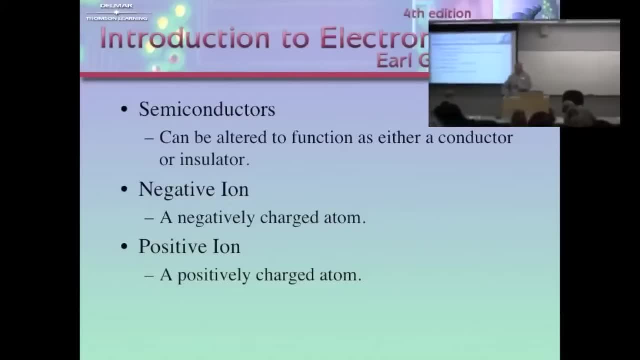 but I think you'll recognize one of the names: Germanium, That's not geraniums, that's what grows in the gardens. Germanium, it's an element. Carbon, that's an element, And the most prevalent Silicon. 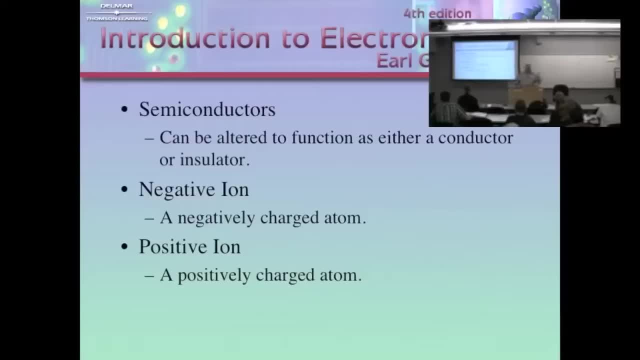 Silicon, Silicon Valley. You've all heard of Silicon Valley. Have any of you know where Silicon Valley is? Have you ever been there? Vast mountains of silicon everywhere. Now it's fabrication facilities, labs. Okay, You're talking about the Bay Area. 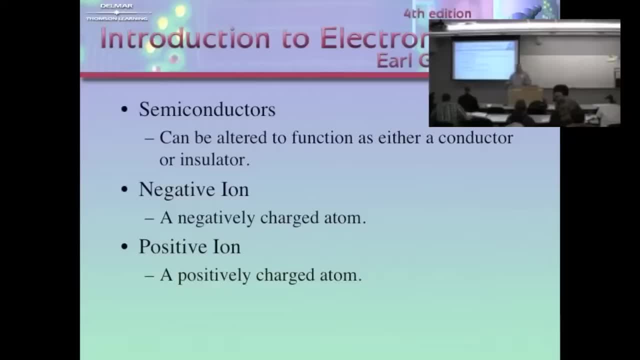 Make sense. And what they did is they harnessed the power of semiconductors and made transformers or transistors- excuse me, not transformers, That's another line. Trust me, we'll enjoy that lecture when we get to it. 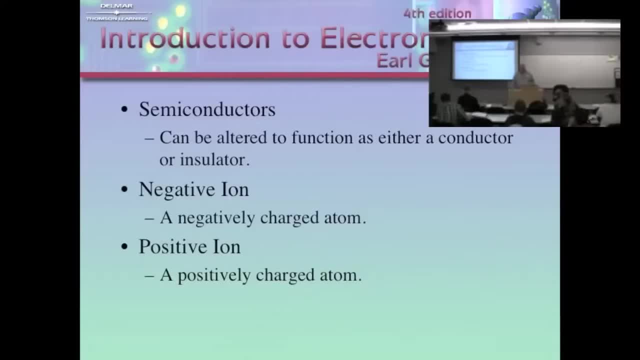 The other big thing I want to address with you is negative ion, Positive ion, Because in essence, this is where voltage comes from. This is where voltage comes from If I get this calculator here on the desktop. it's just been sitting on the desktop all day. 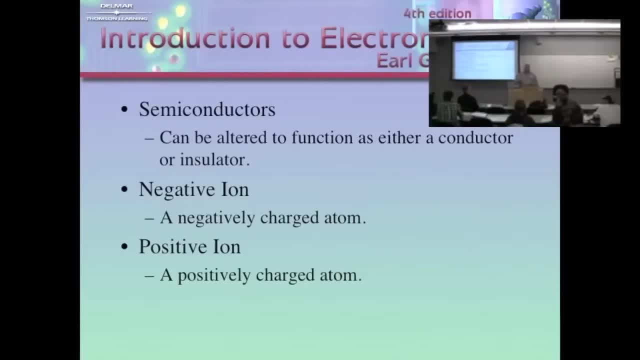 just your average everyday calculator. I assume that, since it was sitting on the desktop minding its own business, it's electrically in a neutral natural state, Because this calculator is made up of matter, which is made up of elements Sitting here, neutral natural state. 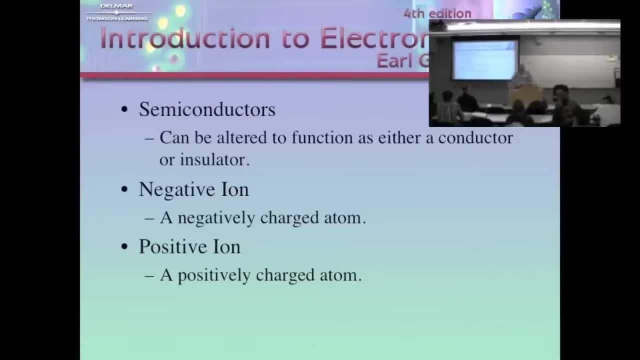 So if I get this now and I start rubbing it, I start rubbing it. what effect do you think that's going to have on the calculator? I'm cleaning it. No, it's a different class. That program's down the hall. 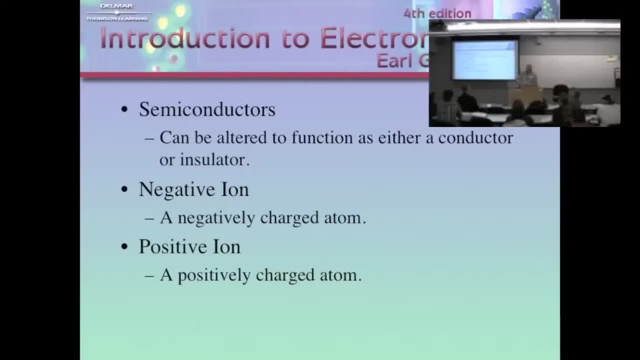 Go out the double doors. Static electricity causes friction. The friction does what, How and why? Through the resistance of the fabric going across the plastic. Close, Close, kind of The difference of the electrical potential, in that you're rubbing that cloth on the plastic calculator. 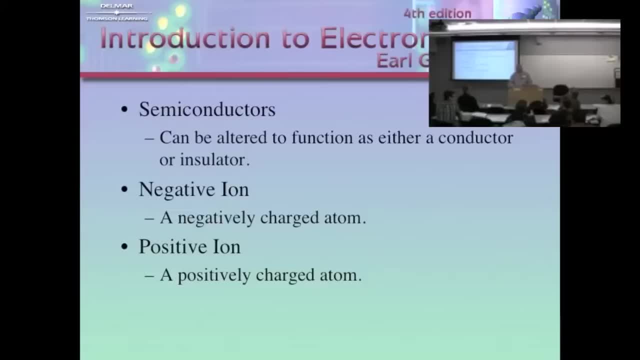 which creates charge on there, And then when you touch it, you have less charge. Yup, that's pretty good. That's pretty good In essence, by me rubbing this and applying friction, which is a form of energy, when I apply energy to matter. 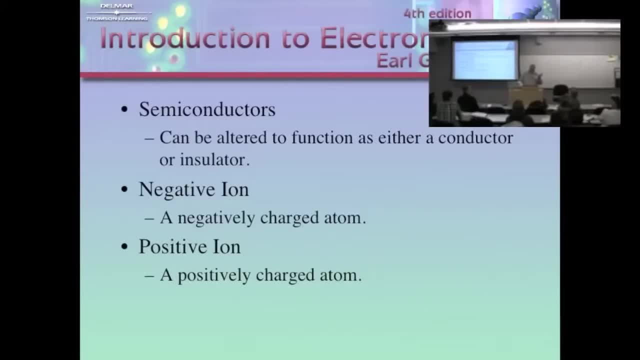 and I rub this, there's a pretty good chance that I am going to knock some subatomic particles. Which ones? Electrons, Electrons Off of what shell? Valence, Valence, shell. If I rub this so hard that smoke starts coming out of it. 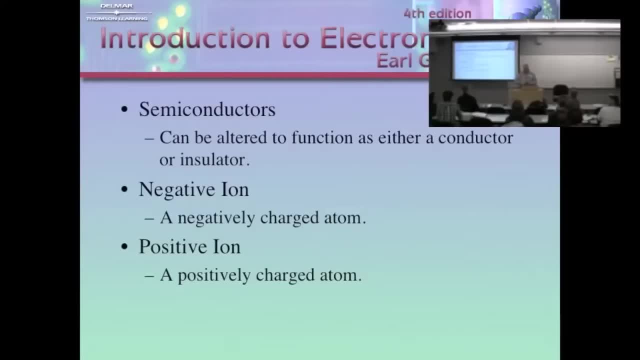 and it bursts into flames. chances are I've gone in too far. But if I just rub the valence shells and I knock some of those electrons from this onto this, now we've got a disparity. Now no longer if I've removed electrons. 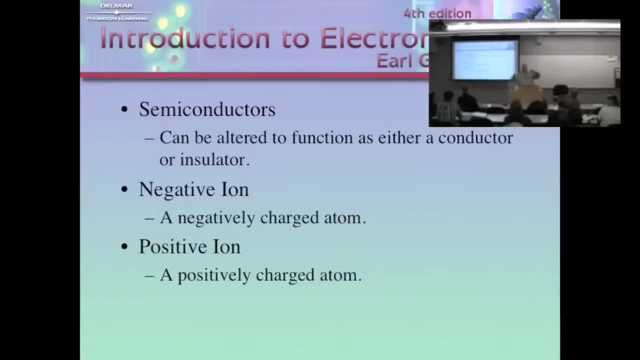 from something that was neutral-natural and I've taken electrons from it. what is the predominant Positive? Positive Why? Because electrons are negatively charged. taking them away Exactly Now, I'm left with more protons on this than I have electrons. 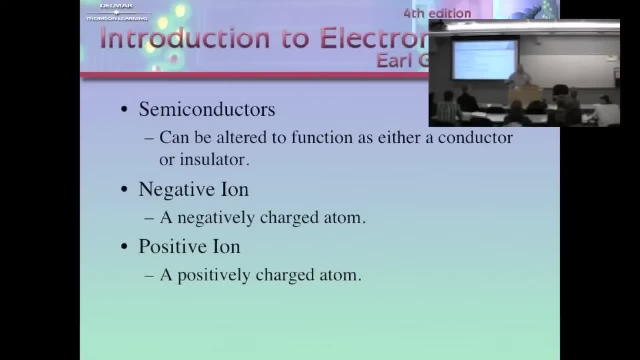 It was in a neutral-natural state, so I started rubbing it. Okay, So that's exactly what I've done, So I just made this a positive ion. I just made this a positive ion by removing electrons from it If this was also in a neutral-natural state. 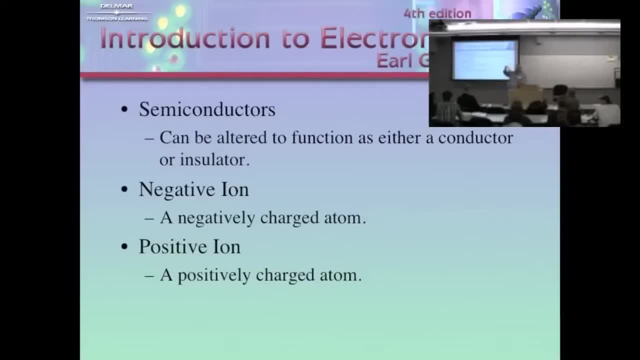 until I started monkeying with it. now I rubbed electrons from the calculator onto the cloth. What does this mean for the cloth? It's now negatively charged. Why is that? Because it contains more electrons than it had when it was in its neutral-natural state. 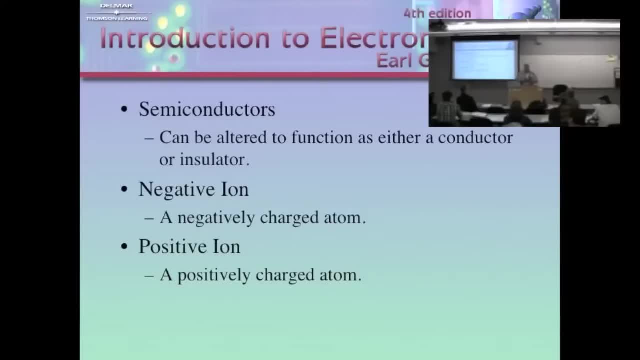 Now you know what, When I do this, when I do this- both of these items- I don't want to make it sound like they have consciousness or whatever, but their whole freaking goal in life now is to get back into a neutral-natural state. 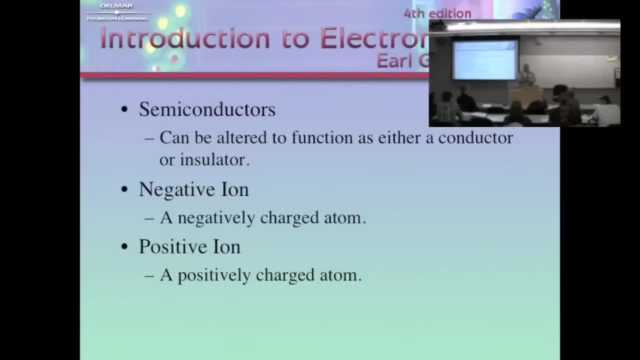 They cannot wait until I put them together and the electrons could jump off the cloth back onto the calculator and they could be at rest in a neutral-natural state in a perfect world. Does that make sense? What I just shared with you is how we generate electricity. 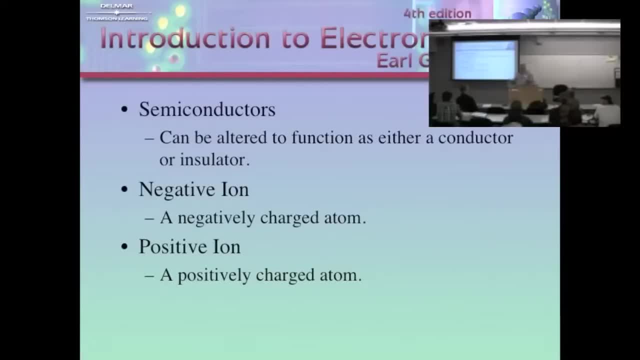 That's how we generate electricity. In order for us to generate electricity, we must apply energy to matter. When we apply enough energy to matter, we could knock electrons off the valence shell, gather them and then say, hey, what? 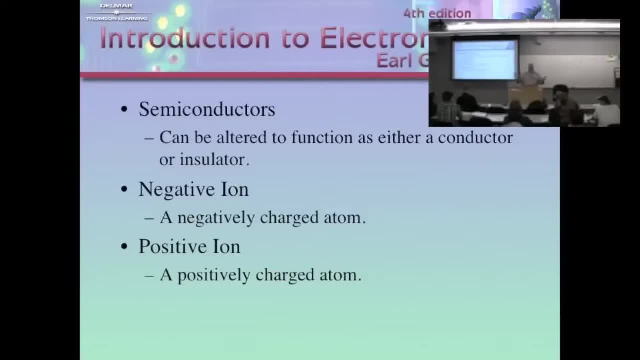 You want to get back to the positive, Have I got a deal for you? Come Travel through my circuit, Make this light bulb illuminate and I'll give you a complete path back to your neutral-natural state. That's what we end up doing as a career. 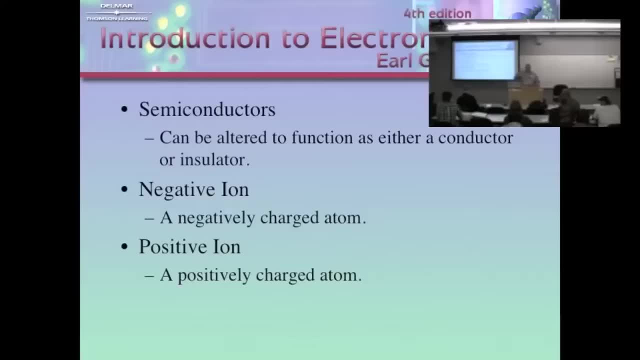 Making sure electrons that were harnessed are ready, able and willing to do work for us, and then we make sure that they follow the correct path and do something for us. We just don't let them complete the path. If you're just letting them complete the path, 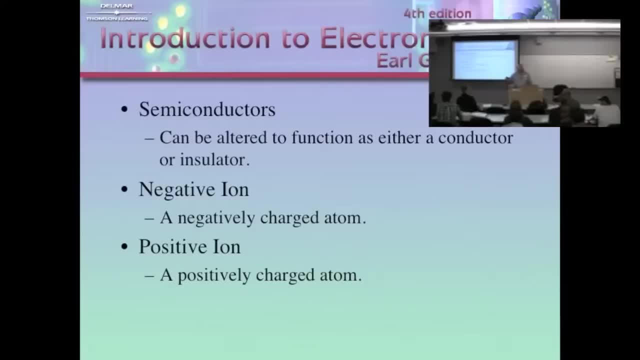 that's called a short circuit. That's not a good thing. We'll talk more about that in future chapters. We just want to make sure that the electrons follow the path and complete that path, Make sense, Very critical. Talked about two big things already. 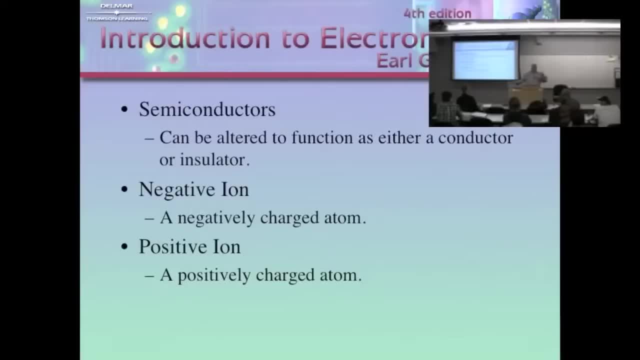 The properties of materials we use in electronics and also the property of how we create voltage or electricity. There's one other thing here the book does not go into. We have conductors, we have insulators, we have semiconductors. There's a fourth property that's floating around. 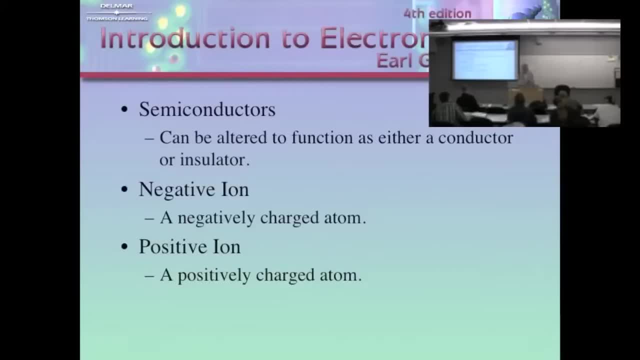 out there in science right now. Does anybody know what property I'm talking about? Superconductor, very good, Very good. A superconductor, all of these materials, whether you're a conductor, whether you're an insulator, whether you're a semiconductor. 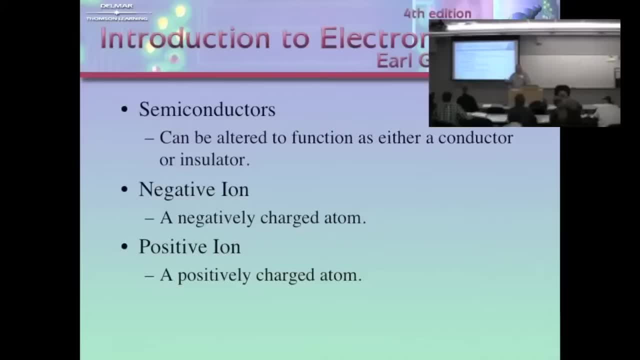 you have one property associated with you. Everything has that property associated with it. It's a property of resistance. We're going to talk about it in a bit. There is a material that exists. It's called a superconductor. It has no resistance. 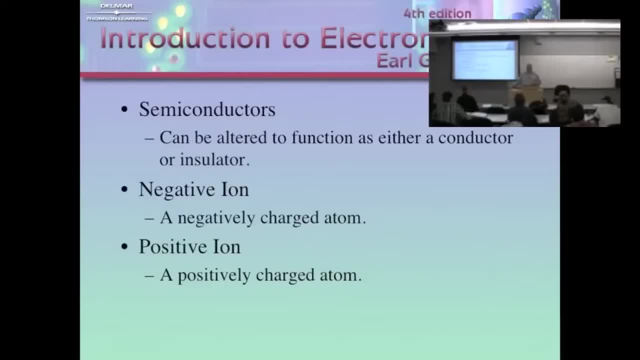 The problem is: does anybody know where it exists? It is at low temperatures, So therefore where it's going to exist is in a laboratory. They don't have it operating at room temperature. I can't bring you next door and give you a tour. 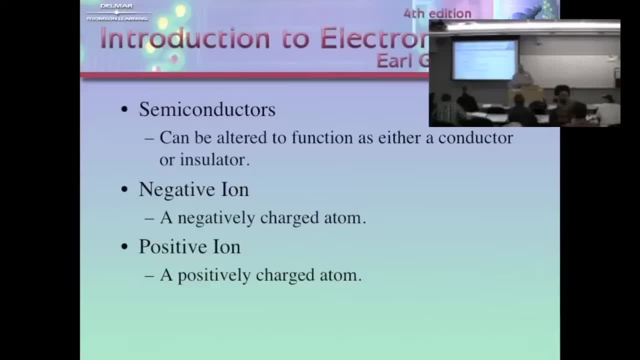 of my superconductor that I have set up over on a bench over here. I could if I had a cryogenics plant and I was a research facility and playing around with it, But when they harness superconductivity it's really going to rewrite the textbooks. 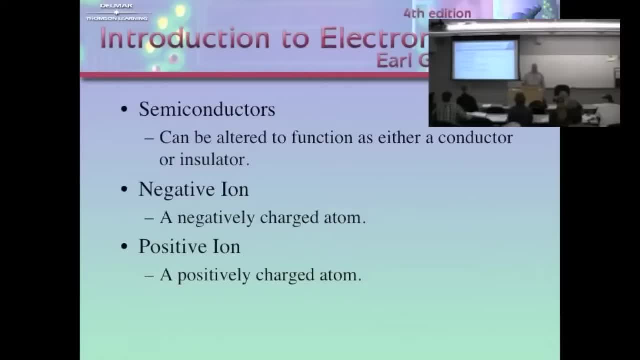 on how we manage electricity and electronics. You think Bill Gates got a lot of money. The dude that captures and harnesses superconductivity at room temperature is going to be very, very wealthy. Very, very wealthy. Make sense, By the way? does anybody know what material 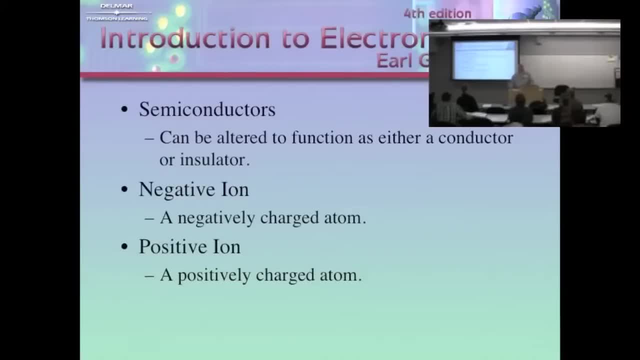 they're having the best luck with as it pertains to superconductivity. What's that Graphene? They're doing some stuff with that. That's not the best results yet. Believe it or not, it is ceramic. Ceramic at room temperature is an insulator. 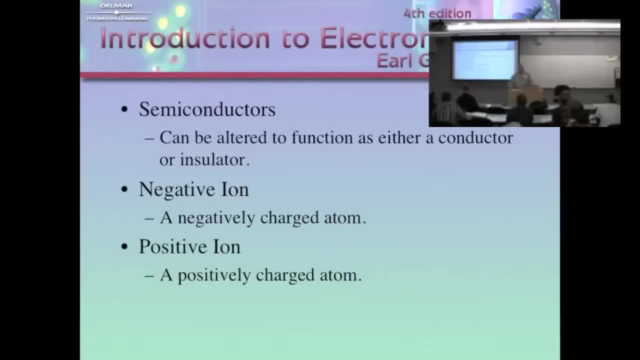 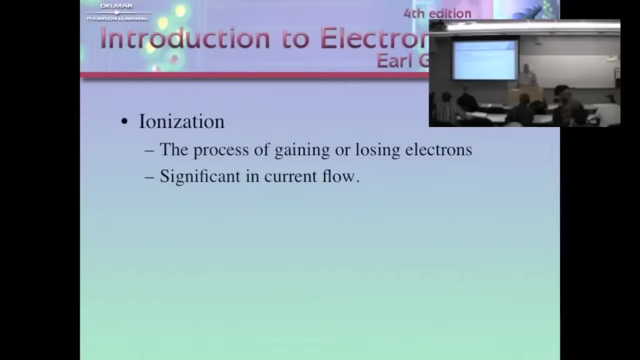 It's a great insulator. We use it as an electrical insulator, But when they bring these ceramics to really really cold, extreme temperatures, they take on conductive properties and they conduct, with no resistance, Pretty cool Ionization. that's the process I just described. 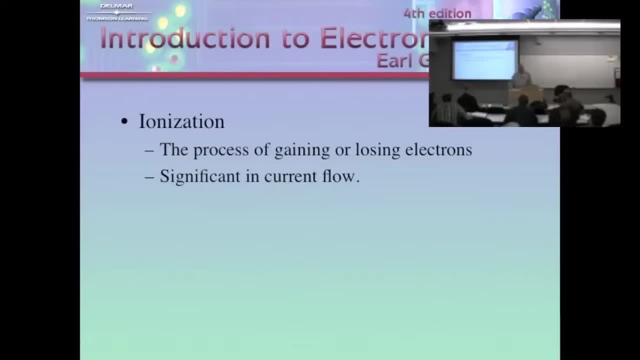 It's the process of gaining and losing electrons and it's significant in current flow. Without ionization you wouldn't have voltage. Without voltage you would not have current flow, Current- again, we should ring bells. Current is the movement of electrons. 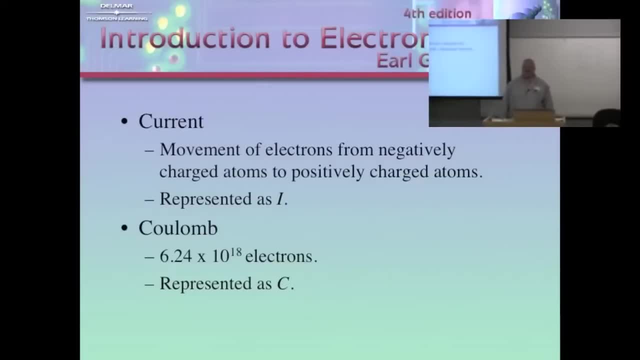 from negatively charged atoms to positively charged atoms. The letter that we use to abbreviate current with is the capital letter I: Capital letter I. One of the terms we need to familiarize ourselves with when dealing with these electrical properties is the term Coulomb. 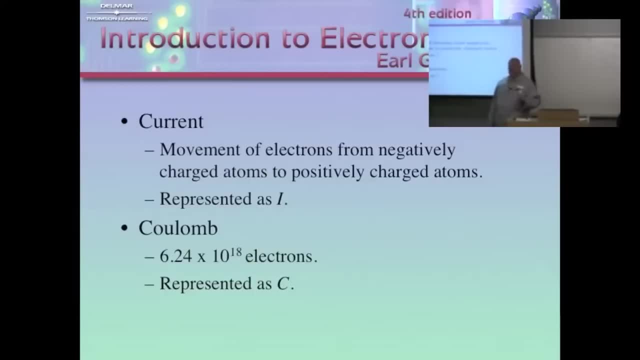 We'll talk more about the Coulomb next chapter, but what a Coulomb is is 6.24 times 10 to the 18th electrons. This is a big, huge number. This is basically 6.24 and 16 zeros after that 4.. 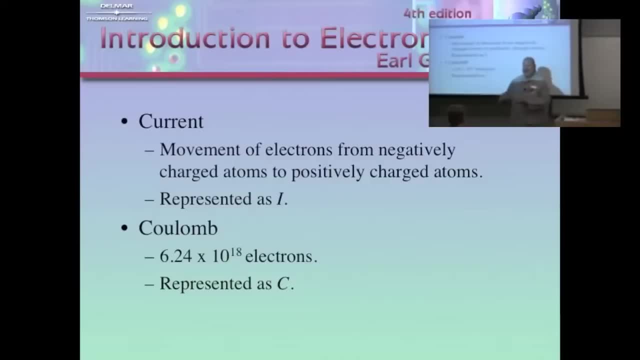 It's too big to fit in your calculator. That's why we refer to it in this as an engineering notation. We'll talk more about engineering notation again in future chapters because we get you used to dealing with these extreme numbers. In electronics we deal with a lot of extreme numbers. 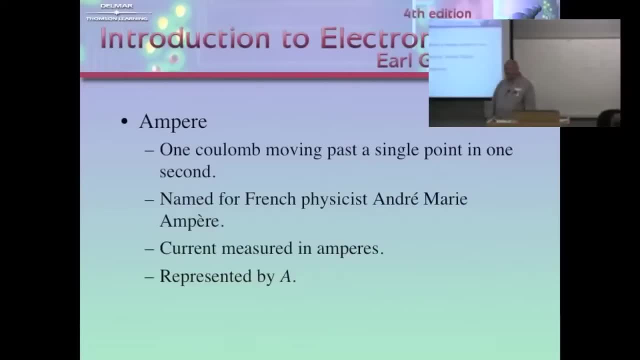 And we represent it with the capital letter C, Now in Ampere, named after André-Marie Ampere, French physicist. one Coulomb, that big number of electrons, 6.24, with 16 zeros after it, that number of electrons moving past. 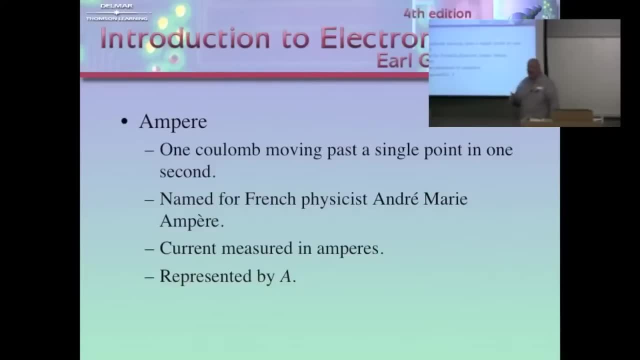 a single point in one second is called the Ampere. Have you all familiar with the term Ampere before? If you've ever burnt out a fuse, you make sure you get the fuse. that's the proper Ampere rating If you pop your circuit breaker. 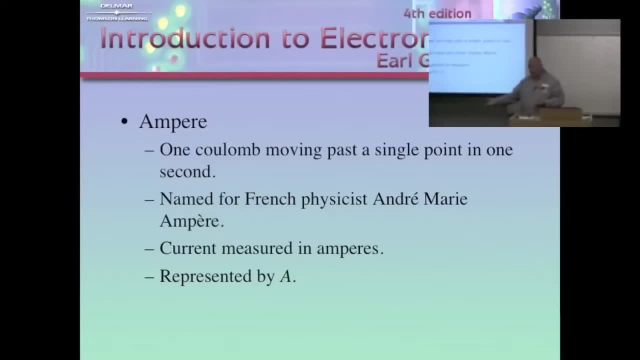 you need to make sure, when you're resetting it, that you're not overloading the circuit and exceeding the amperage rating of the circuit, And what that is is physically a given number of electrons that you're forcing through a conductor in one second's time. 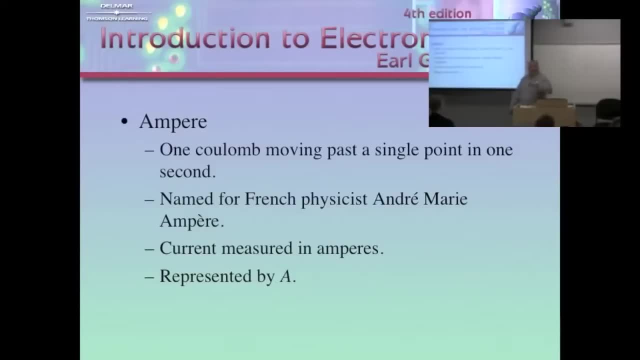 One Coulomb per second is one Ampere. 15 Coulombs per second is 15 Amperes. We'll talk again more next chapter on that. Currents measured in Amperes and it's represented by the capital letter A. 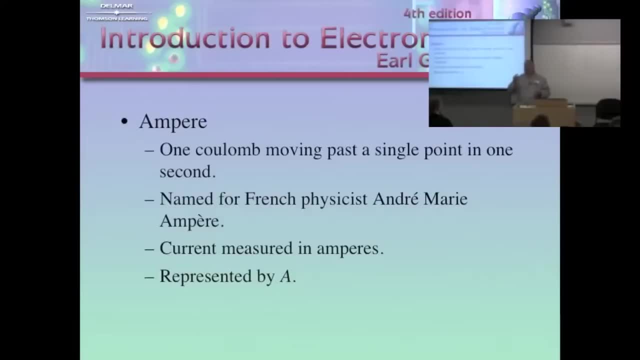 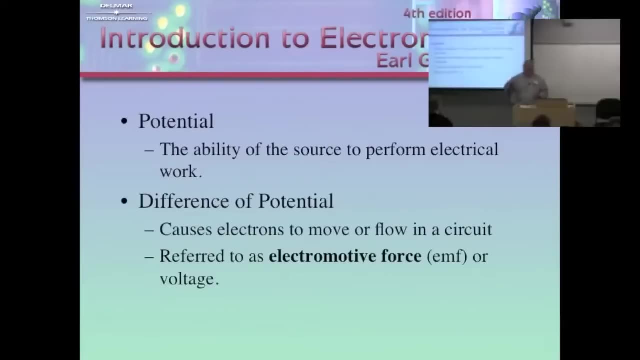 So if you go out to your fuse box in your car, pull a fuse out and it says 15A next to it, that stands for 15 Amps, Universally accepted. Universally accepted, Universally accepted Potential, the ability of a source. 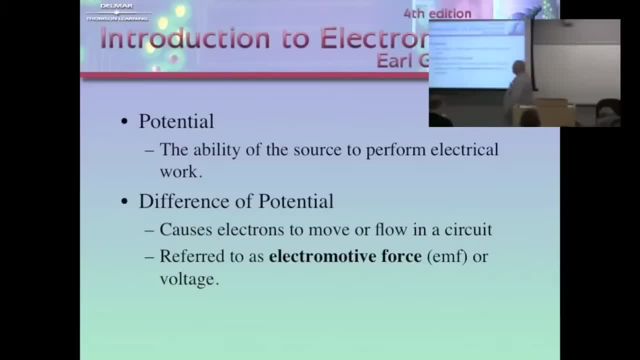 to perform electrical work. What we're talking about here with potential is voltage. Difference of potential causes electrons to move or flow in a circuit. This is referred to as EMF, or electromotive force, or voltage. EMF, electromotive force, voltage. 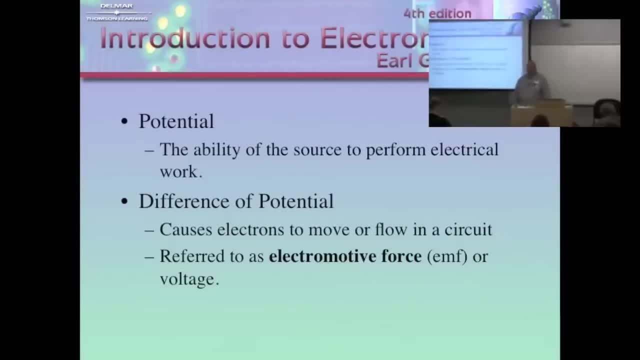 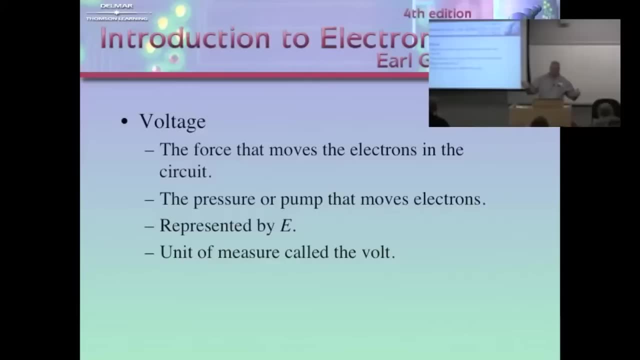 difference of potential. they're all synonymous. Voltage- ring bells, chimes hit the gong- is the force that moves electrons in the circuit. It's the pressure or pump that moves electrons represented by the capital letter E or the capital letter V. 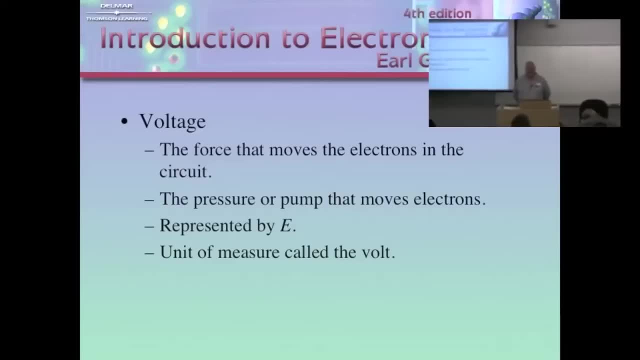 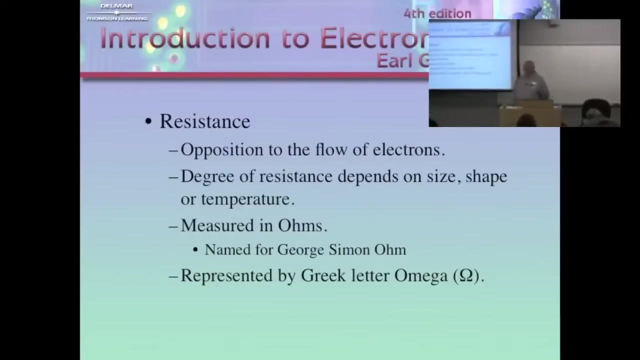 Whether you use E or V here. the textbook uses E. you could use V if you want. As long as you know what we're talking about, It's universally accepted. The unit of measure is called the voltage. The unit of measure is called the volt. 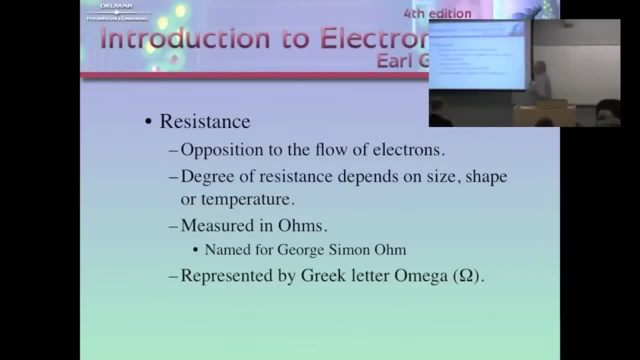 Resistance, the opposition to the flow of electrons. The degree of resistance depends on size, shape and temperature, and it's measured in ohms, Named after George Simon Ohm, represented by the Greek letter omega. One of the things I want you to familiarize yourself with is 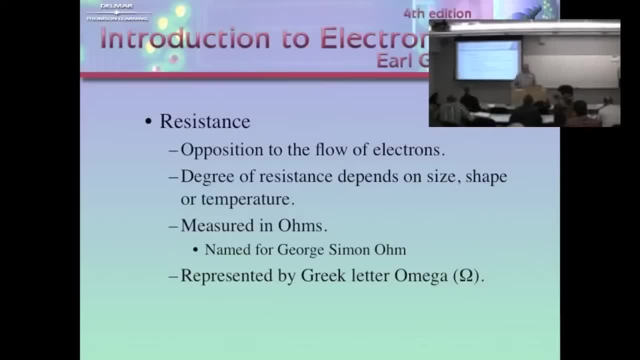 you know what has resistance? Everything, Everything except superconductors, And superconductors only exist in a laboratory right now. Hopefully, when you buy an extension cord, that extension cord has a low amount of resistance. Okay, Hopefully when you buy new spark plug wires. 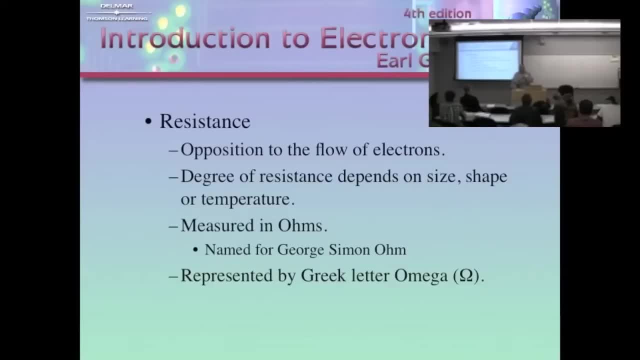 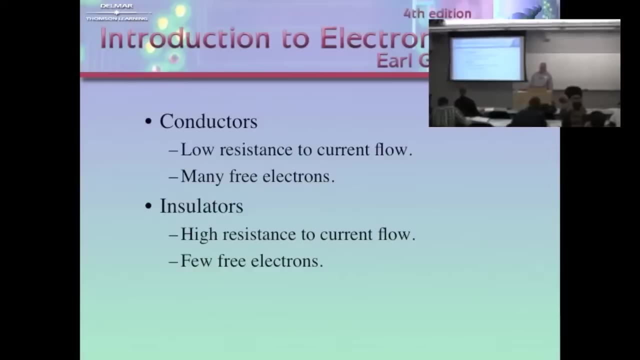 for your car and they're insulated, hopefully. the outside of the spark plug wires has a high amount of resistance. Make sense: Conductors have low resistance to current flow. That's why they're called conductors. They have many free electrons to transfer the energy. 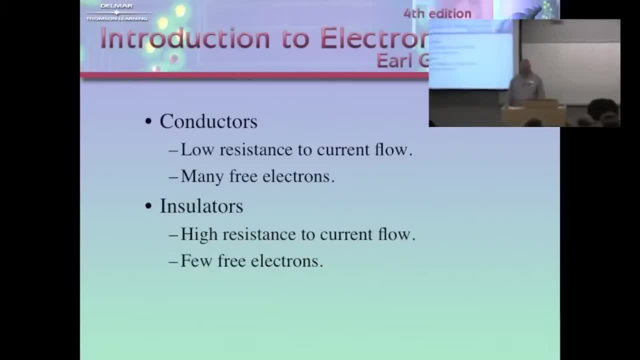 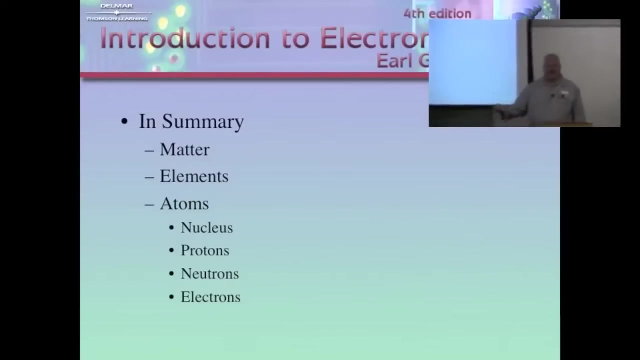 Insulators have high resistance to current flow, very few electrons. In summary, tonight we talked about matter. we talked about elements, the fundamental building block in nature. we talked about atomic structure, specifically subatomic particles, and a place. Nucleus is not a particle, it's a place. 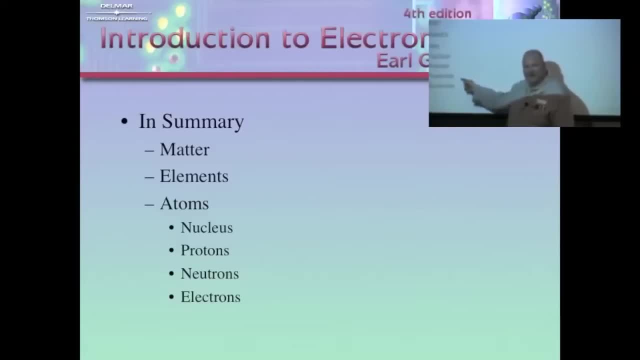 That place contains the protons, the neutrons and the electrons. Protons are positively charged, neutrons are neutrally charged and electrons, well, those are the other ones. they're negatively charged. We talked about atomic number: number of protons in an atom. 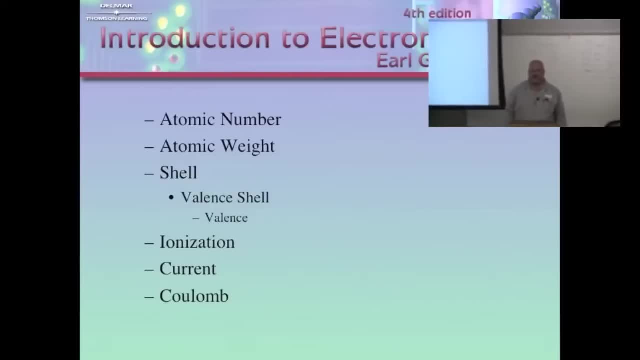 Atomic weight, number of protons and number of neutrons in an atom. We talked about shell. these are the orbital arrangements of the electrons, starting with the K shell, going all the way up to the Q shell. We talked about ionization. 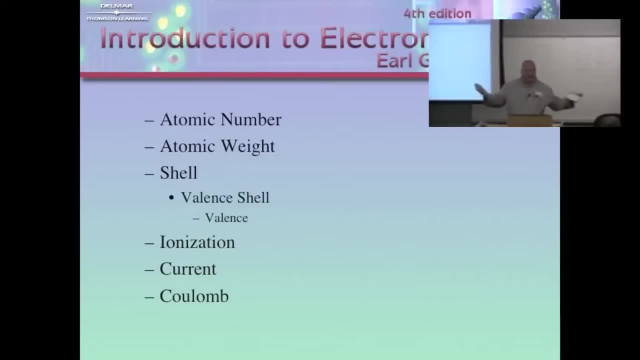 the process of taking things out of a neutral natural state. We talked about current. current is the flow of electrons from negative to positive. Why? Because it wants to get back into a neutral natural state. We talked about the Coulomb: 6.24 times 10 to the 18th electrons. 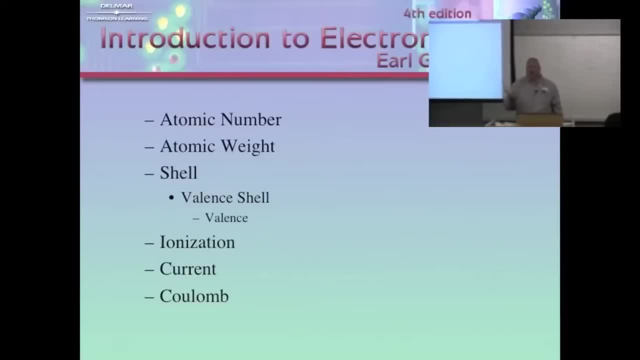 it's a number of electrons, Like a dozen eggs, a bushel of apples, a gallon of gasoline. We talked about the ampere. The ampere is one coulomb per second. We talked about electronic or electric current. that is measured in the ampere. 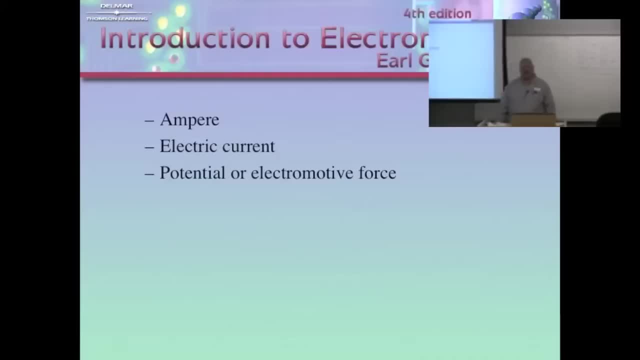 And then, finally, we talked about potential or electromotive force. what we're talking about there is difference in potential or voltage. Does anybody have any questions on anything that I covered in a lecture for chapter one? Going once, Going twice, What's that? 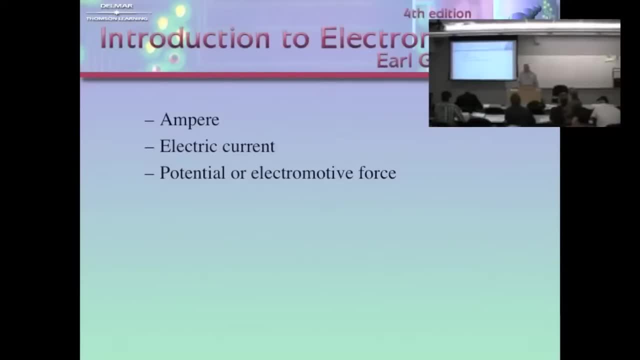 Yes, these slides are on the website. The audio recording is on the website and eventually we're going to get the video uploaded as well, But the content will remain the same. It will be the new Google site. New Google site. Any other questions? 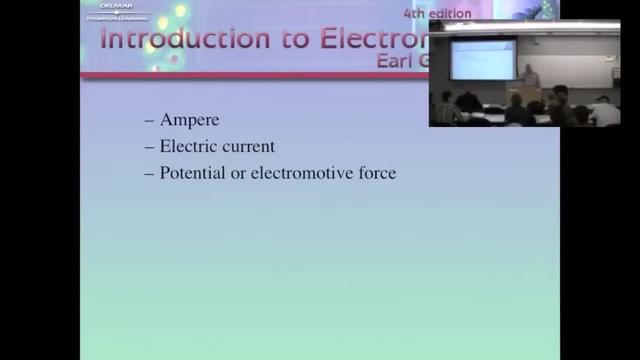 Going once, going, twice going going. The new Google site, the last one that's listed there, the HTTPS sites, googlecom site, LWTC electronics- I've got that turned on. Anybody with the address should be able to get in there. 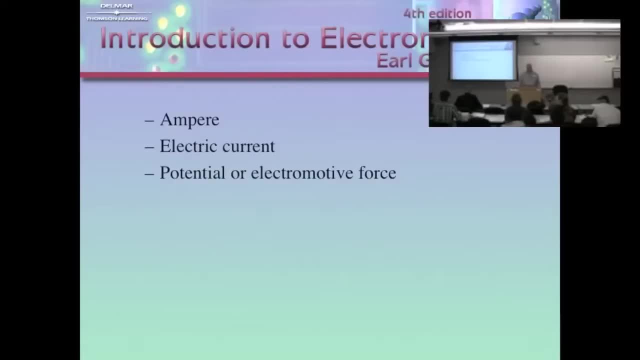 We haven't uploaded this material to it yet, but it should be there. Really, Yeah, I think the S means that there's somebody with administrator access walking on secure action. So I like messed up. Is that what you're saying? Yeah, 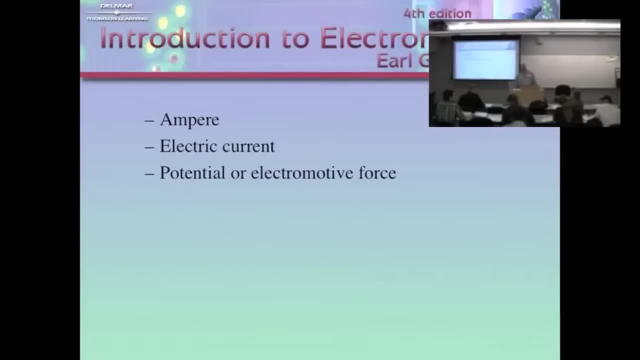 All right, I messed up. I think so Cool, Cool. That's why you got the job as TA. You're here to keep me honest. Any other questions? Once, twice, I should know where lead falls on the. I honestly don't know. 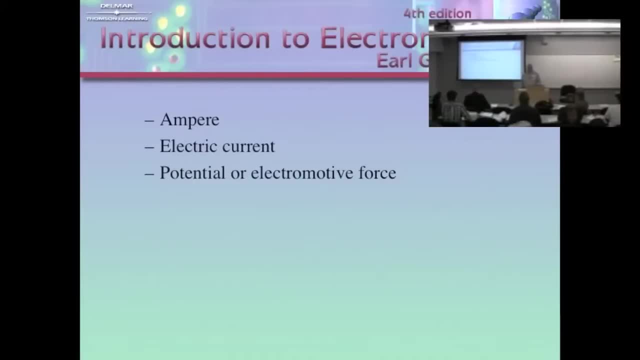 I mean, it's pretty far down. I think it's amazingly good. It's real close On a periodic table. it's amazingly close to silver. Yeah, It is good, but it's Oh yeah, And that's why. 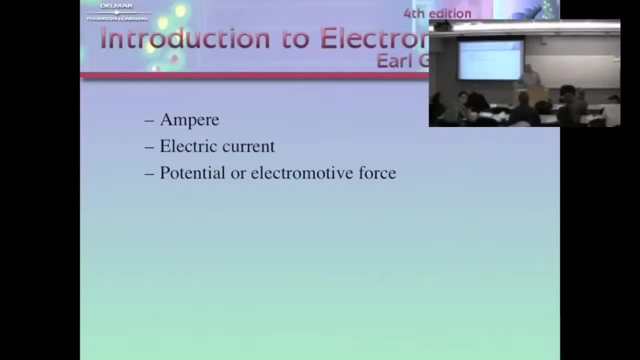 actually in solder we used to contain lead, but because lead is lead and it's bad, they realized it was really really bad so we pulled it out of solder. but it was used to join in complete electrical circuits, So it's. 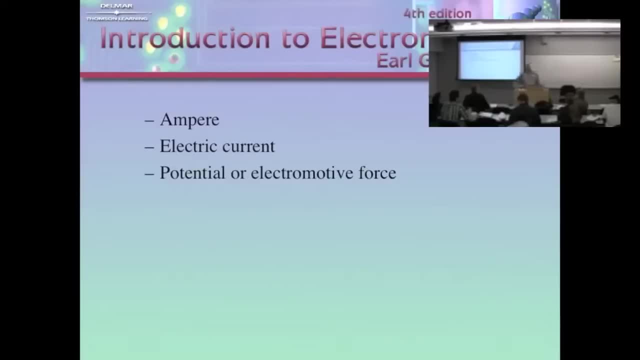 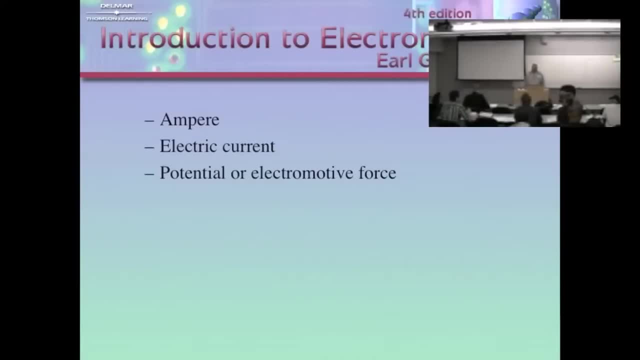 And once going, twice going going, Gone, We're black. The next questions that I have for ELEC 110, Chapter 1,. you'll be answering for me on a quiz, But don't worry, Well you'll have. 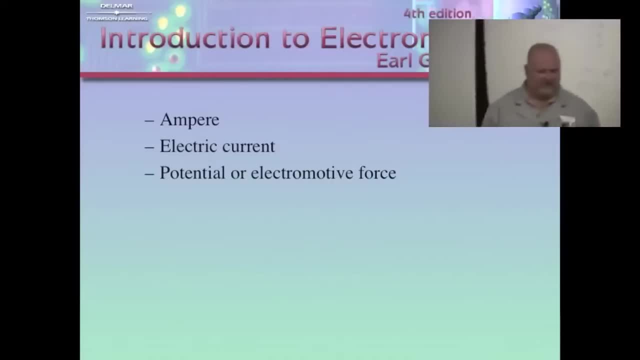 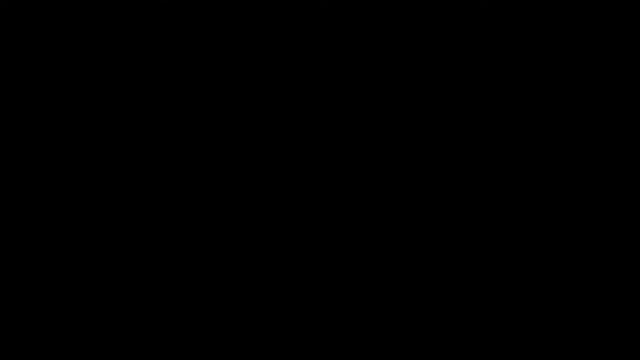 another week or so before we take the quiz. I'll coordinate with the class lead on that. Any other questions about protocol? anything else we're doing here? All right? Um, we don't have. Okay last week. um, wrapping up lecture. 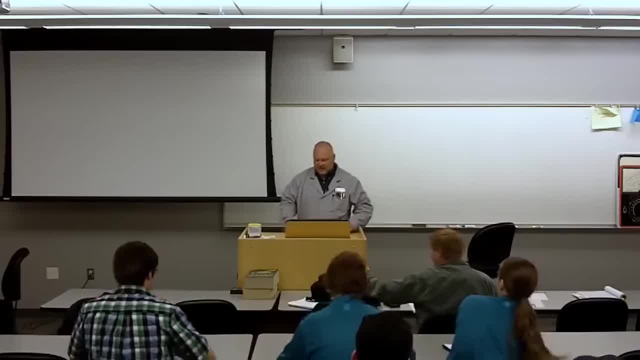 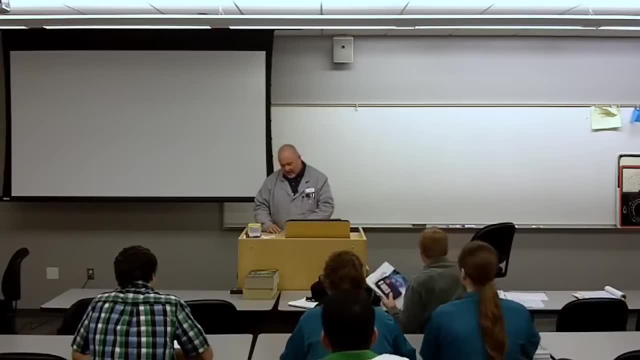 we're talking about electrical insulators, we're talking about conductors, things of this nature, right? Um, I dug out of my archives here. Remember I talked to you about mica Mica. I found my stash, my private stash. 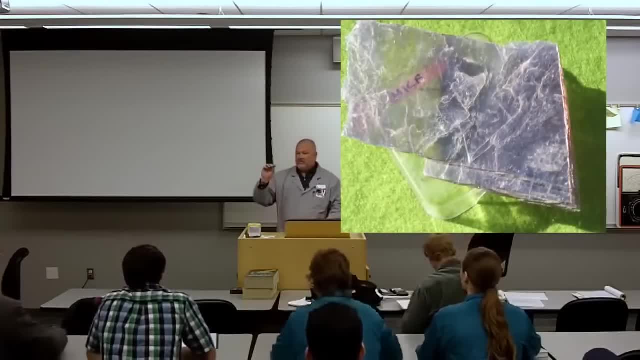 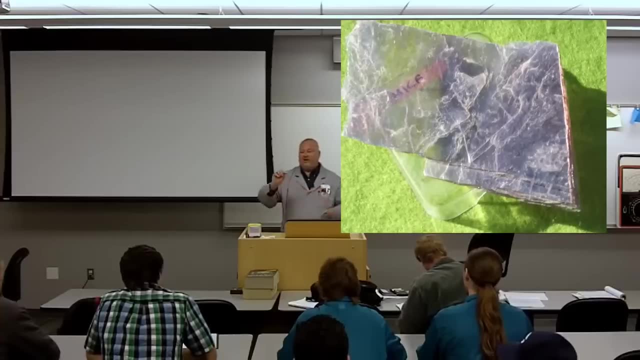 of mica. Please be very careful passing this around. Um, I don't know if you have any questions about this, but it actually kind of flakes off, So you can just handle it. look at it, This is found in nature. 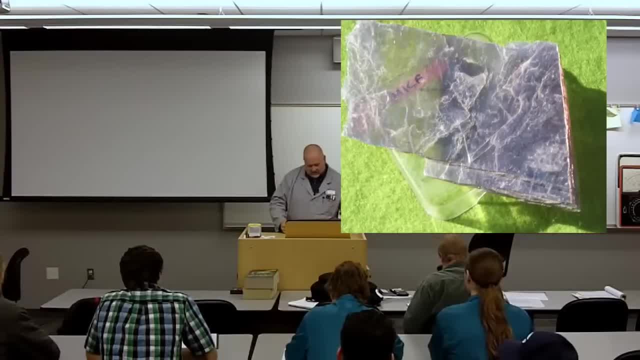 It's found in rock formations And this is the best insulator found in nature. This is a washer, an insulator washer that's been made out of mica. Okay, so we'll pass these things around so you can see, But these are very fragile. 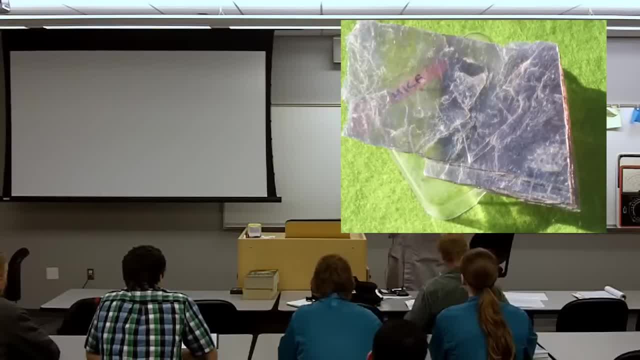 Don't try to bend it, You'll break it. It's uh almost like a real thin piece of glass, if you will. So this is uh mica in the raw And this is a processed piece that could be used. 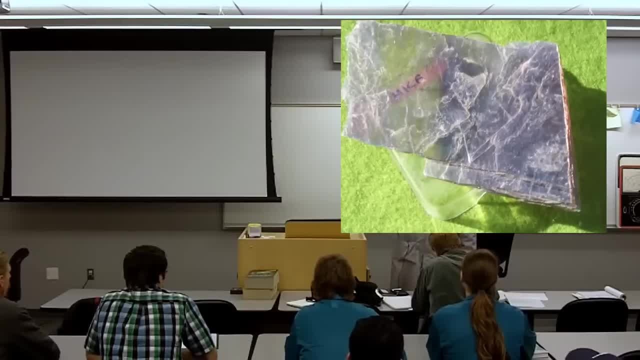 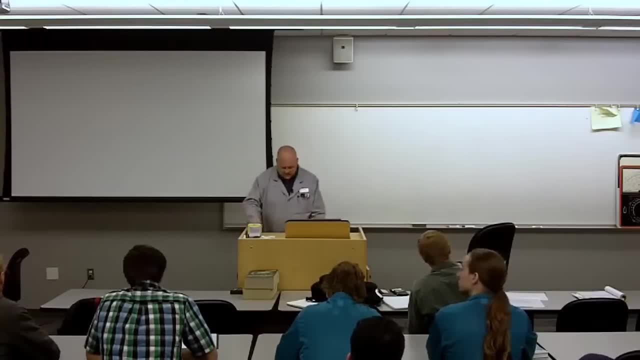 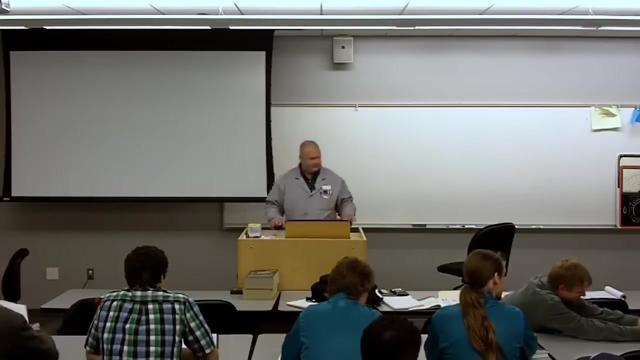 as an electrical insulator. So cool stuff. Does anybody have any questions on anything else before we get started here? Chapter chapter number two. Okay, so we're going to go through this and see if there's any other questions that we have. 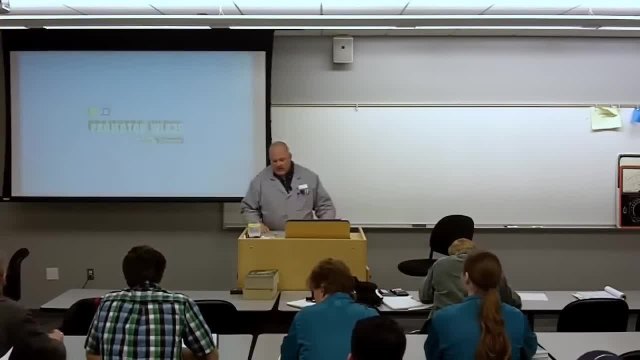 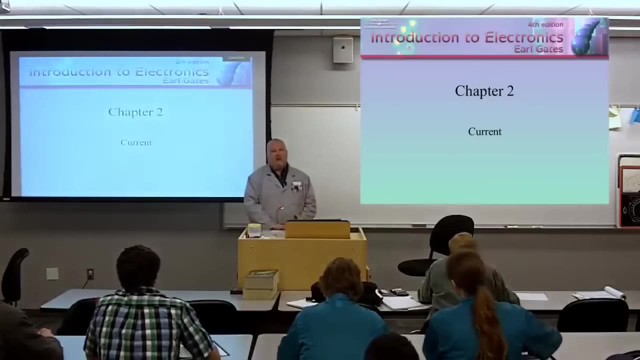 Okay, just to get us kind of ramped up from where we left off last week. um, we really started our discussions last week talking about the fundamental properties of of electricity. Um, and that discussion really started off with a discussion about matter. 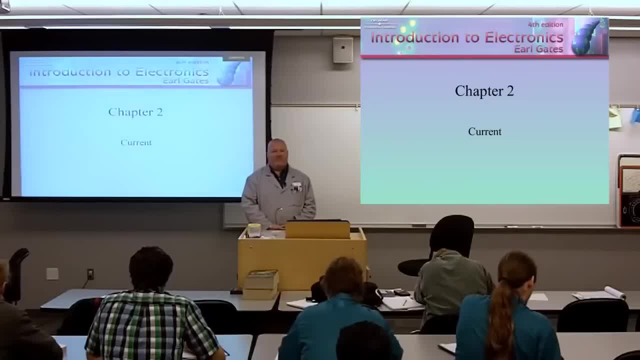 Matter is uh. if there is no matter, the absence of matter is called space. We could recreate the absence of matter here on planet Earth by using an industrial vacuum vacuum chamber. That's where we pump all the gases out of the chamber. 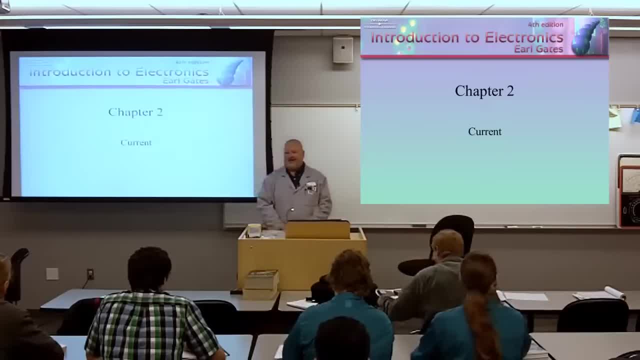 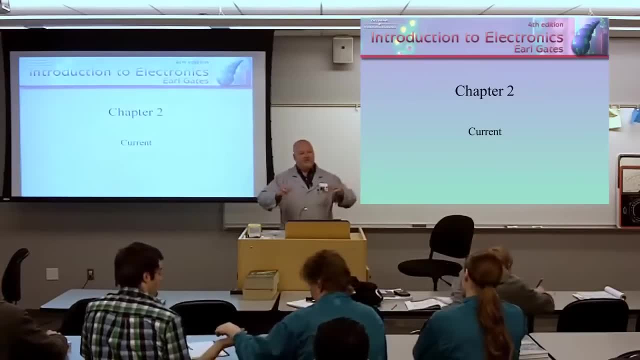 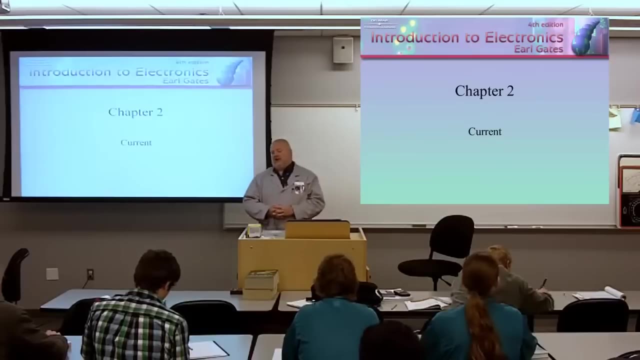 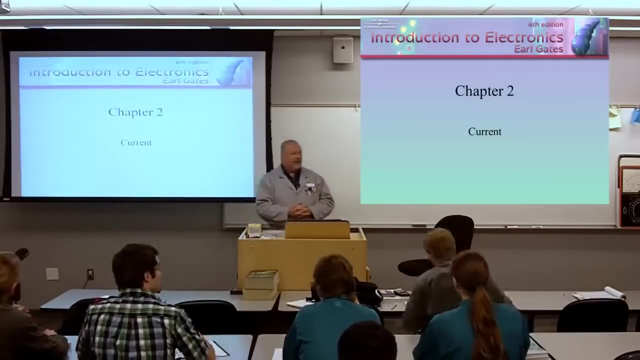 and we're left with nothing inside. Um, industrial vacuum is used a lot to separate from it and only introduce those materials that they want to be inside the chamber. Remember that discussion? Okay, The next thing we talked about, which is uh. 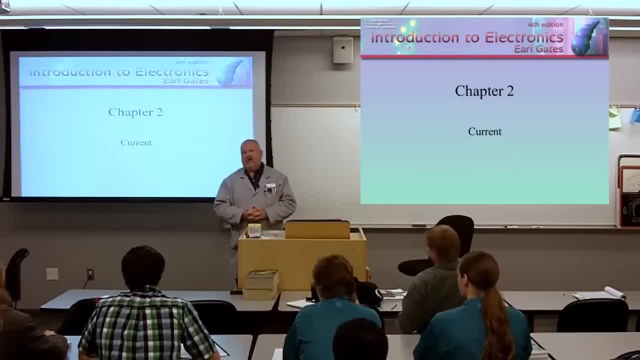 which is very, very critical are the properties, the fundamental physics properties, if you will, of materials that are used in electrical production. So let's say you have fewer valence electrons, electrons in the valence shell. Okay, That means. 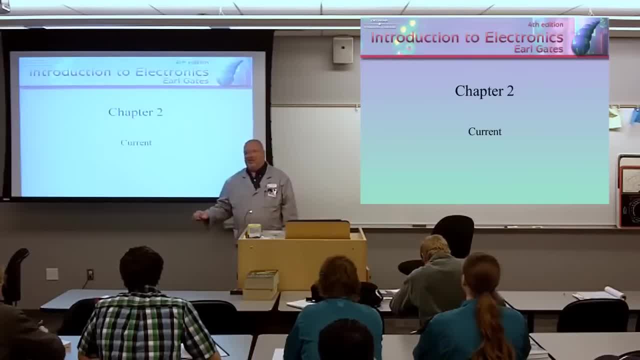 there's- basically we talked about it like a parking garage. There's room for electrons to park in this valence shell. Therefore it's going to make it a good conductor. Materials that have five or more electrons are not going to have any. 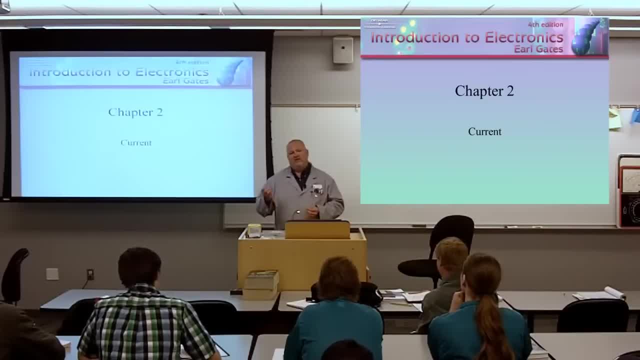 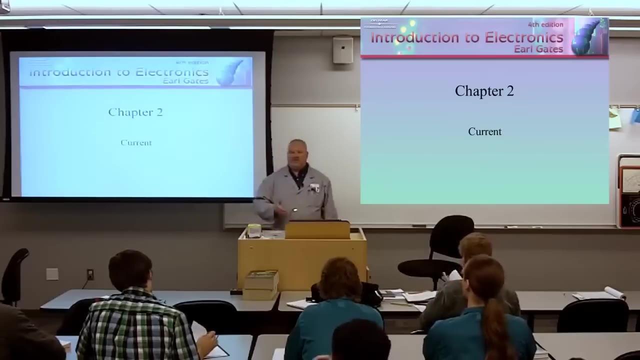 place to park on that piece of mica. We also talked about semiconductor materials. Those are materials that have four electrons in the valence shell And- uh, for those of you that continue on in this program, ELEC 120, that's right. 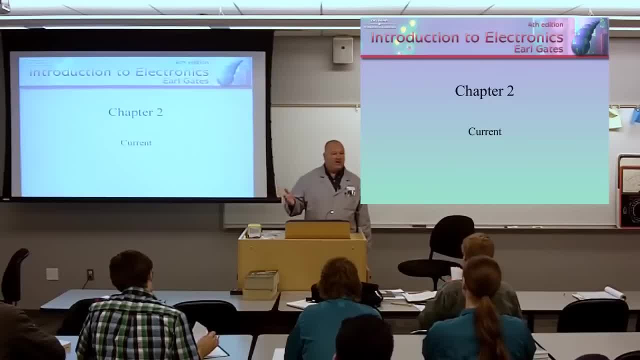 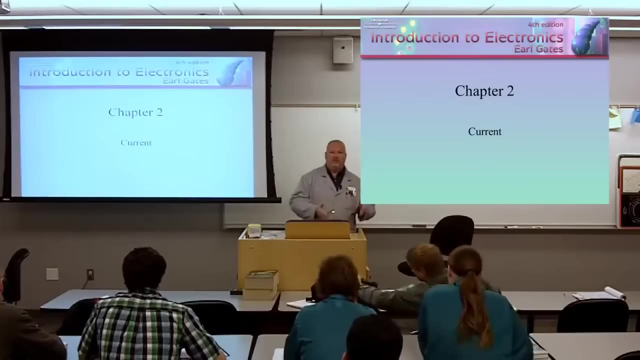 where we're going to pick up the discussion back to fundamental properties of physics. when we were talking about these fundamental properties of atomic structure, because that discussion was all about solid state materials- Silicon germanium- that we use in the manufacturing of transistors and integrated 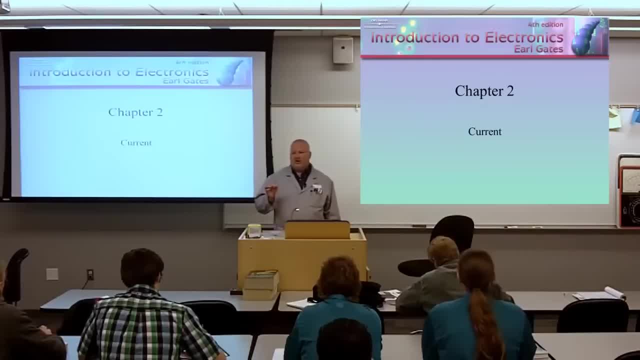 circuits. Um, the other big thing we talked about is, in essence, the beginning, the creation of electricity When we have matter and we could knock an electron off that valence shell. When we knock an electron off that valence shell, we end up. 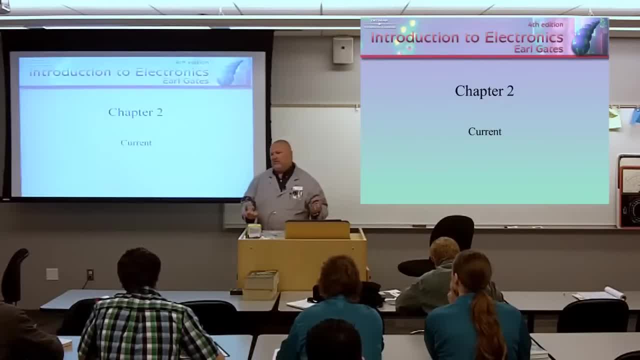 with what's known as a positive ion. A positive ion Because, remember, in nature matter is typically in a neutral state. That means it has an equal number of protons and an equal number of electrons. Remember that What's your atomic number? 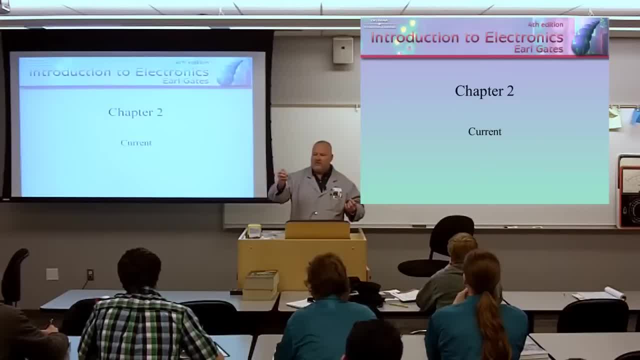 Which one is it? A is weight, B is number on the quiz, C is both. D is none of the above. Which one's it gonna be? The number of protons Is number, Okay, So that number, whatever number. 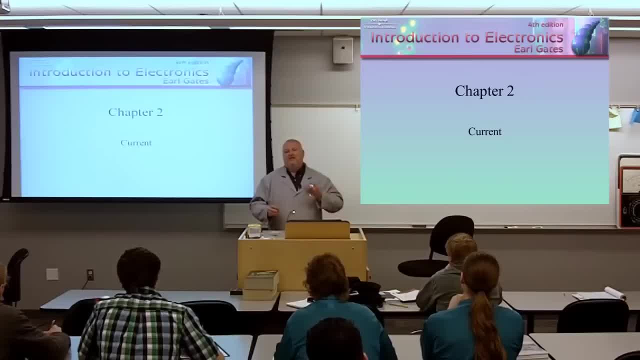 of protons we have, we also have the same number of electrons. That's what puts it in a neutral natural state. So when I impart energy on matter and I knock an electron off now, I have more protons that have a positive charge than I. 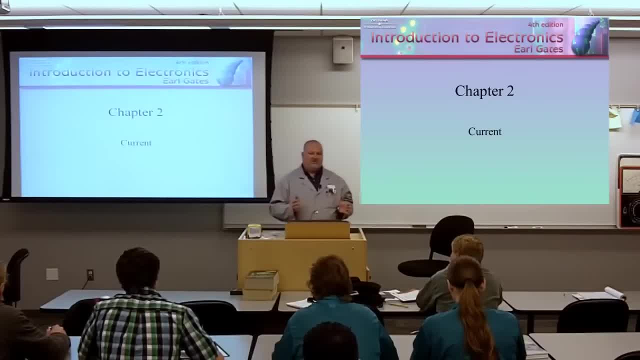 have electrons in the atom. that makes it a positive ion. In essence, what I just did is created electricity. That's what electricity is. Electricity is us applying energy to matter, knocking an electron off, gathering those electrons and then saying, hey, electrons. 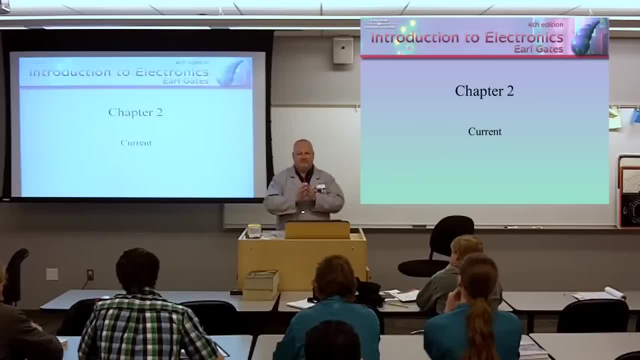 have? I got a deal with you. Get it into a neutral natural state. Come this way, Go through this circuit, Do a little bit of work for me and then I'll give you a path back to neutrality And electrons. they do this. 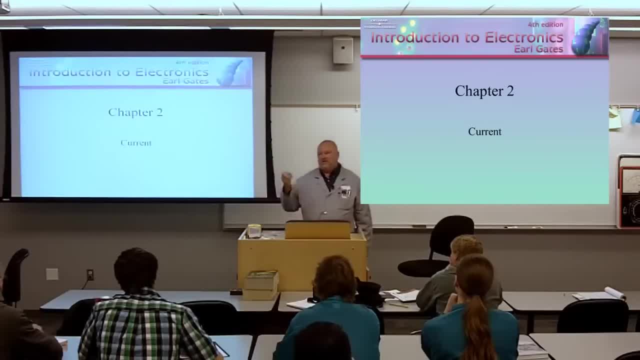 So part of your careers in the electronics industry is gonna be simply managing the behavior of electrons, Making sure the electrons do what they're supposed to do. I guess that's why they call this electronics Electronics, Right Electronics: The study of the 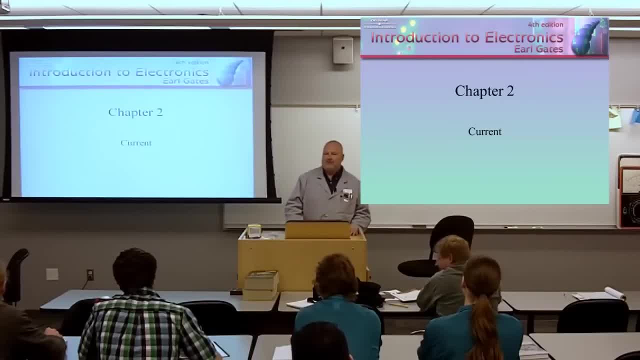 behavior of the electron. That's what this is all about. The other thing we talked about last week, briefly, was the coulomb, a unit of measure. Right, A coulomb is like a gallon of gas, a dozen eggs, a bushel of apples. 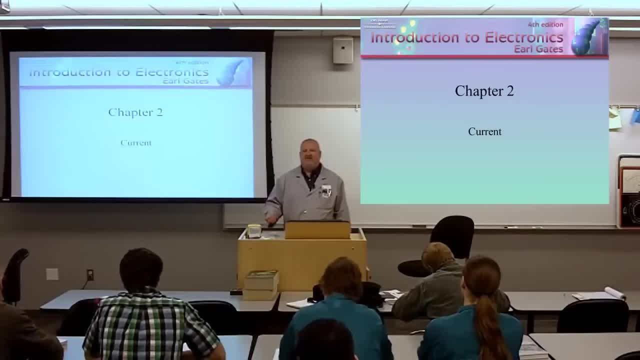 A coulomb is 6.24 times 10 to the 18th electrons. It's a big, huge hurricane number of electrons. There was a guy by the name of Charles. He was counting electrons for a living and then he died. 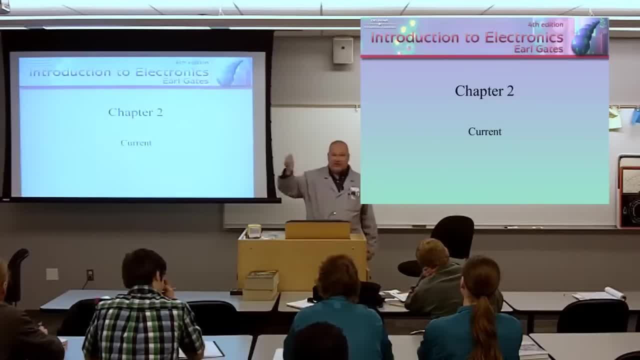 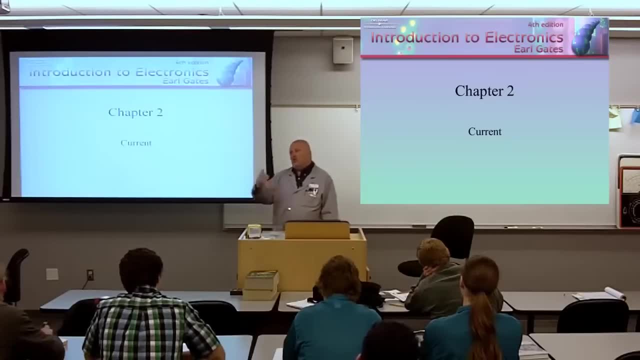 You know. And then he said: hey, anybody here want to continue on Chuck's work? Anyone, Anyone? Alright, we'll just call it. even We'll call you know the number that he came up with: 6.24 times 10 to. 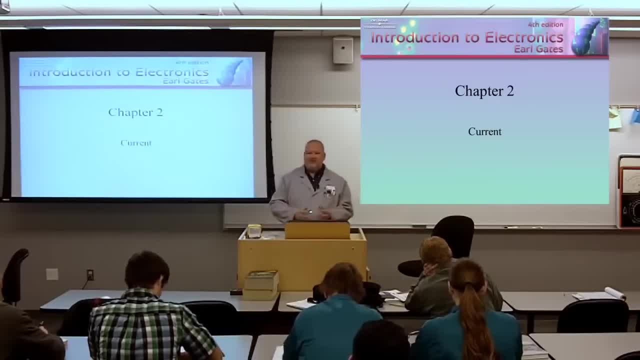 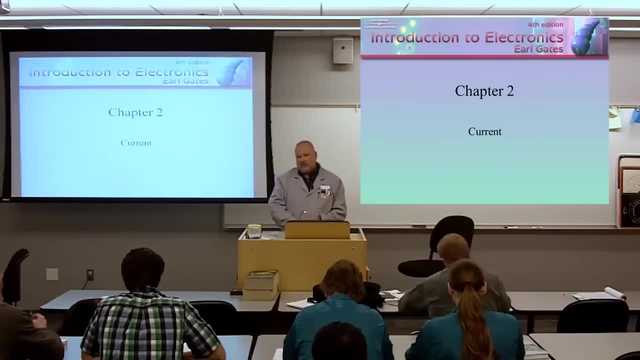 the 18th. we'll call that a coulomb. One coulomb per second is the ampere That was put together by a guy by the name of Charles Charles Ampere, Andre Marie Ampere, And you know what? 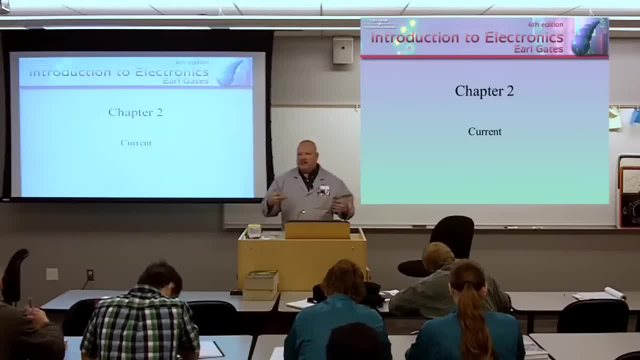 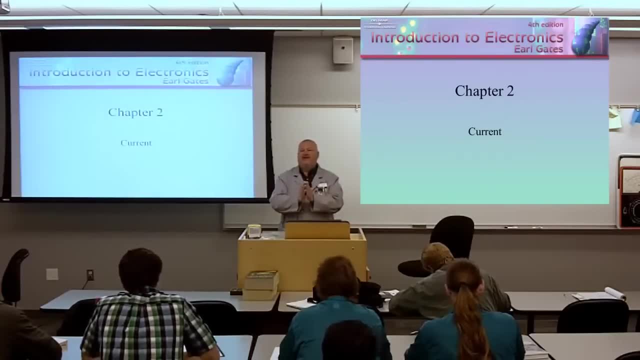 Universally. that's accepted. See the amazing thing: I enjoy travel, travel all around the world. People speak different languages. We use different coins, different monetary values. When it comes to current worldwide, the ampere is the accepted value. 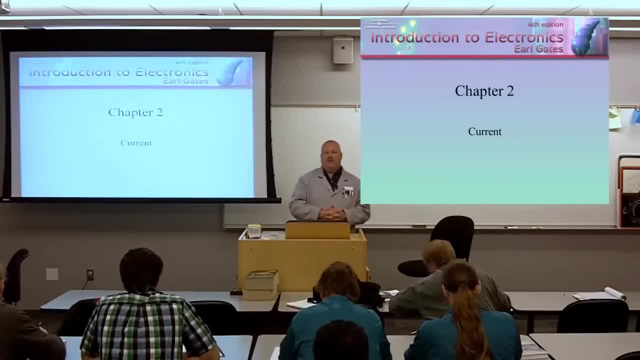 that we use, no matter where you go. So those of you that are learning, or if you have English as a second language, you know when you struggle with this we're all learning a new language. It's the language of electronics. 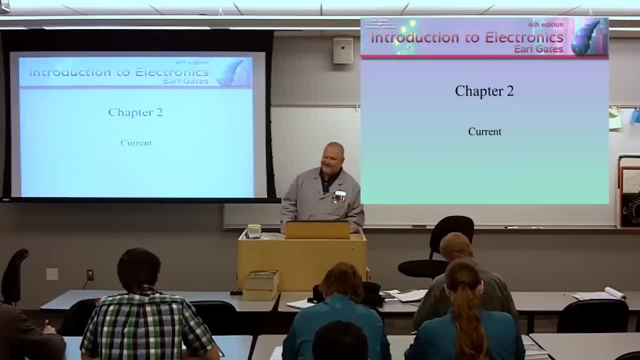 And the word we're gonna study tonight is current, Current, And you already know kinda a little bit about current based on our lecture last week. Well, we're gonna pull back the curtains and study a little bit more tonight After completing this chapter. 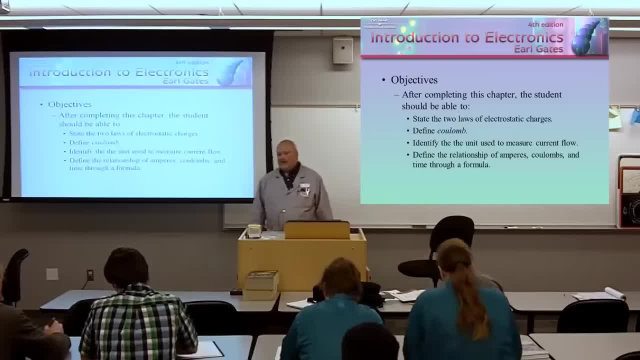 you're gonna be able to state two laws of electrostatic charges. I'm gonna give you a heads up. If it's a law, you should like sit up straight and like take note, Because if it's a law, 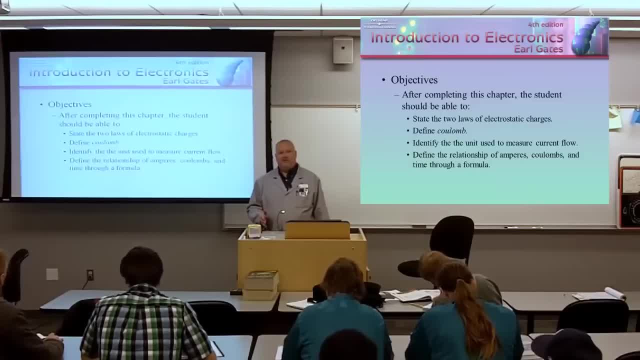 the type of laws we're talking about here are not laws that we can go to Olympia and have repealed. Okay, They're not talking about laws that we can go to the Supreme Court and have overturned. That actually would be kinda fun, wouldn't it? 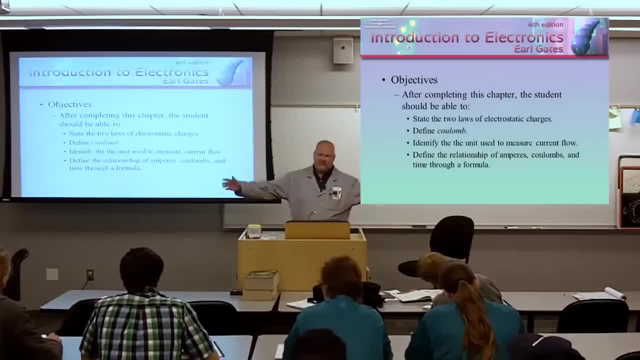 Go to Washington DC. Students from Lake Washington Technical College in Kirkland, Washington, protested against it. okay, So these electrostatic charge laws are kinda critical. We're gonna be able to define Coulomb: Identify the unit used to measure current flow. 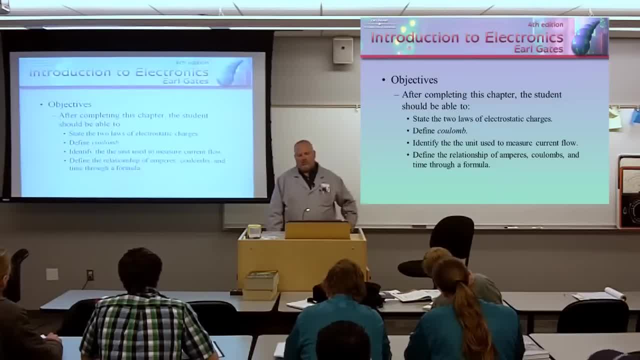 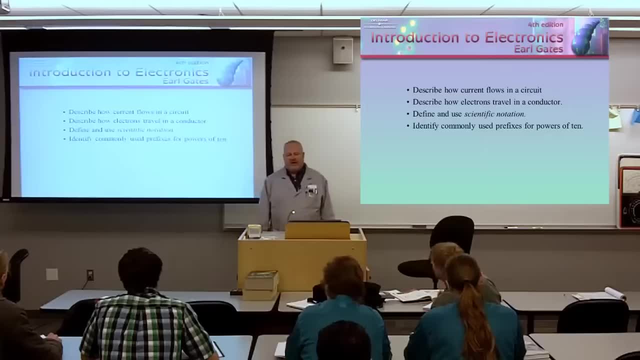 Define the relationship of amps, Coulombs and time through formula. Describe how current flows in a circuit. Describe how electrons travel in a conductor. Define and use scientific notations And identify commonly used prefixes for powers of 10.. Some of you may be. 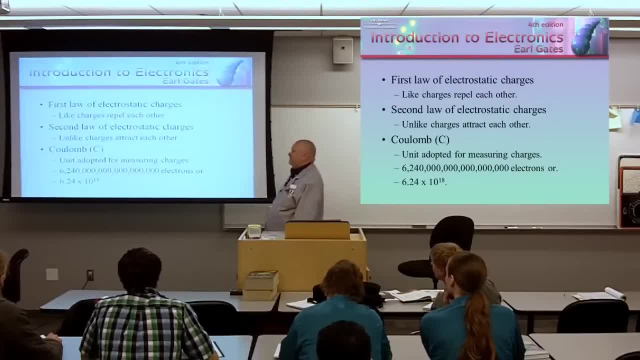 familiar with this law. You've probably heard it before. The first law of electrostatic charges are like charges repel each other. Have all of you heard that one before? Okay, The other thing that you're probably familiar with is like opposites. 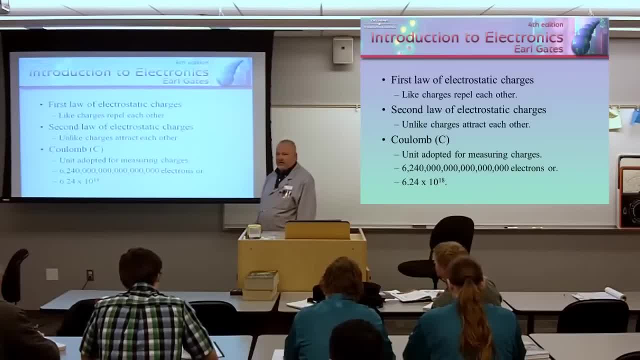 attract right, Opposites attract, and that's not only in relationships but also in relationships. okay, So the first law of electrostatic charges in relationships, that's actually the laws of electrostatic charges Opposites attract is actually the second law of. 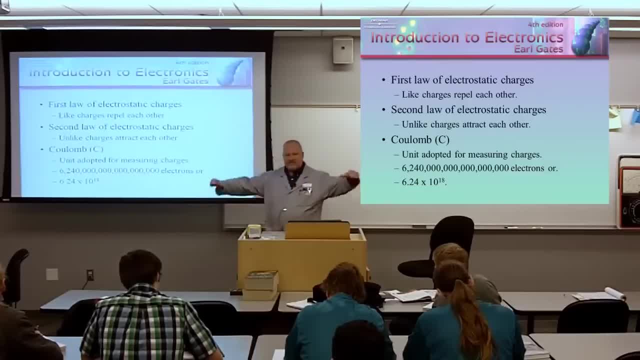 electrostatic charges. So if I got a negative and a negative, they're gonna oppose each other. If I have a positive and a positive, they're gonna oppose each other. If I got a negative and a positive, pow they're gonna be. 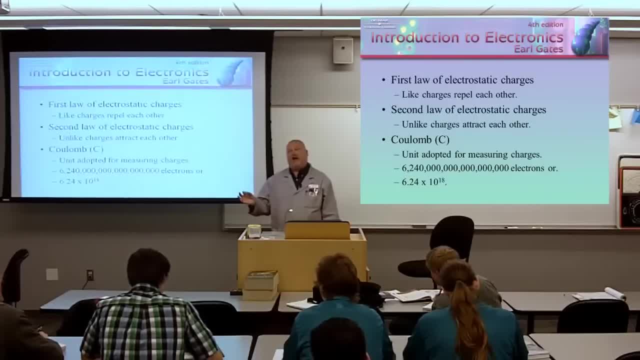 attracted to each other. Yup, very similar, But the same thing. North is gonna be attracted to south. You got two north poles. they're not gonna be attracted. They're actually gonna push back on each other. Two south poles, the same thing. 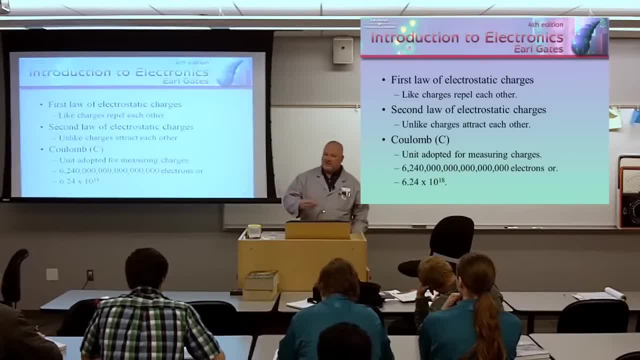 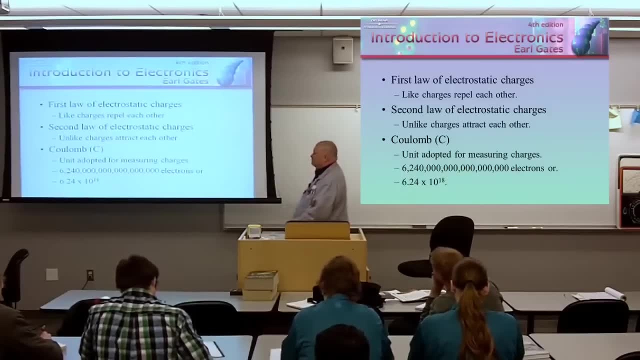 So we're actually gonna study that in future chapters. But this is the law of electrostatic, not electromagnetic, So just keep those two separate. Coulomb: Coulomb is the unit adopted for measuring charges. In last week in lecture I gave you the. 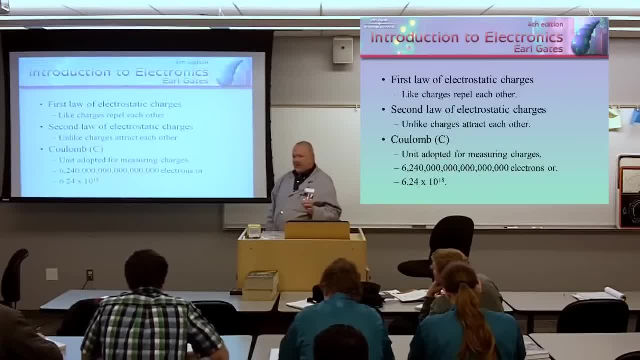 two, fourth times tenth of the eighteenth. I figured I'd wait a week before I actually showed you what that number looks like. I mean, it's one thing for me to say up on the board, it's six point two, four, then sixteen zeros. 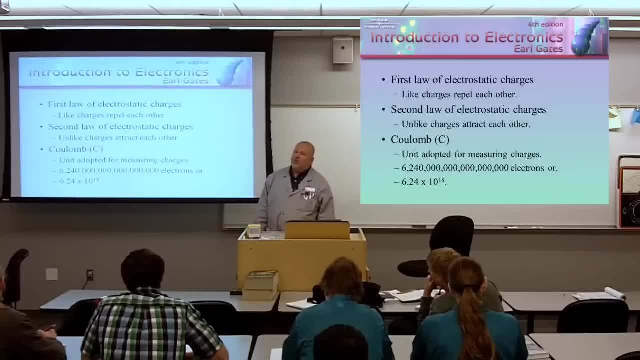 after. But this is really what the number looks like. Okay, It's really what the number looks like. One of the reasons that we need to use this form of notation is that this number right here will not fit. It won't fit in. 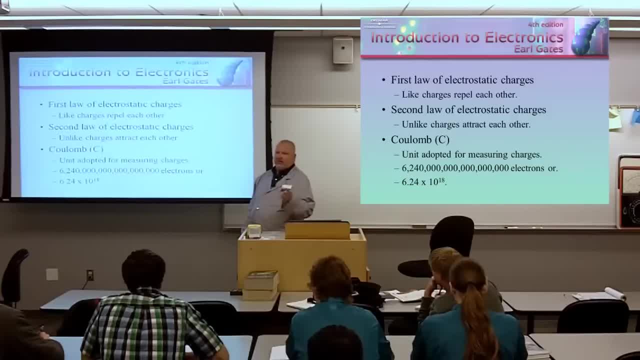 your calculator unless you enter it in this form, And I'll show you By the end of the lecture. I'll show you how to make sure you know how to enter it in that form. It's kind of funny because if you had some, your neighbor 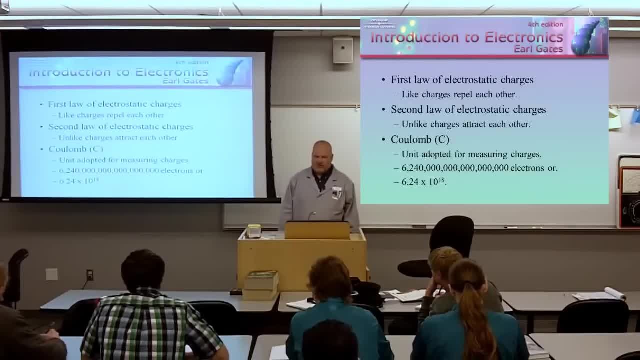 down the street or whatever, and you found out that they were going to college in an accounting program. Right, If they're going to go to school to become an accountant, you'd probably say, wow, that is a lot If you're a Bill. 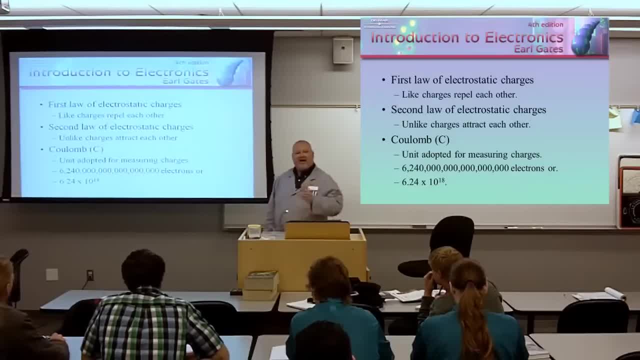 Gates, accountant, you're not dealing with a number like this, Okay, But yeah, regularly, on a daily basis in the study of electronics, we're going to be dealing with numbers like this. So if you're struggling with this form of notation, 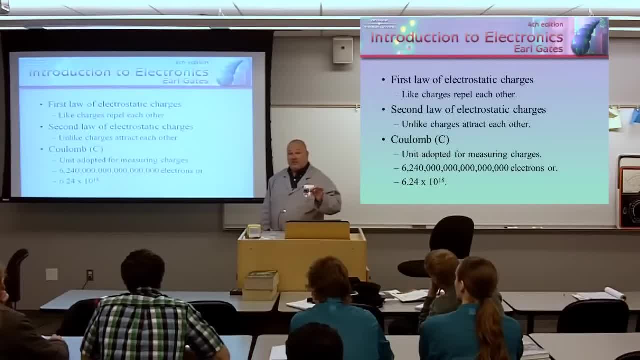 we'll work with you, But don't be like me. When I was in school initially like this, I looked at this number and I looked at this stuff and, ah man, I don't know, that's too close to the 18th. 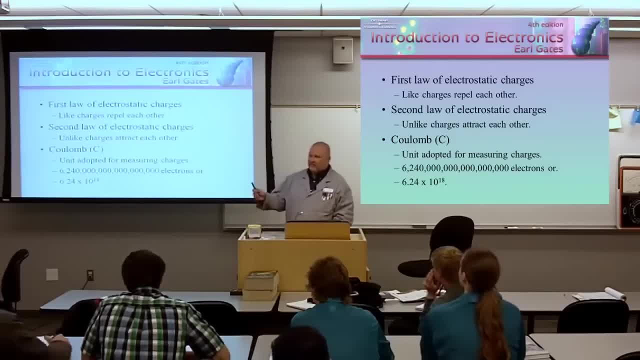 That's a number like Mr Spock would use or something on the Starship Enterprise, And I'm a more down-to-earth guy, so I'm going to keep it basic. you know, And in very short order I realized you can't keep it. 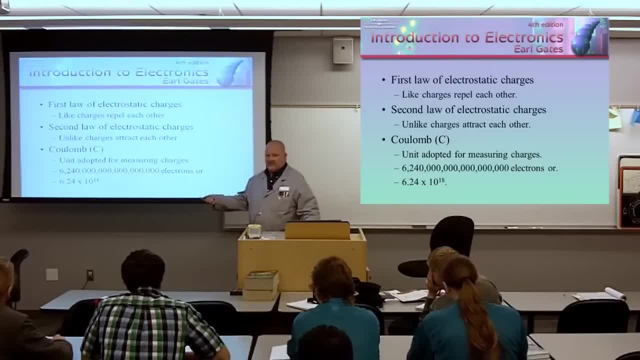 basic in electronics because we're going to be dealing with these extreme numbers, So we have to use this form of notation. So you see how we came up with this: 6.24 times 10 to the 18th. The decimal point here means: 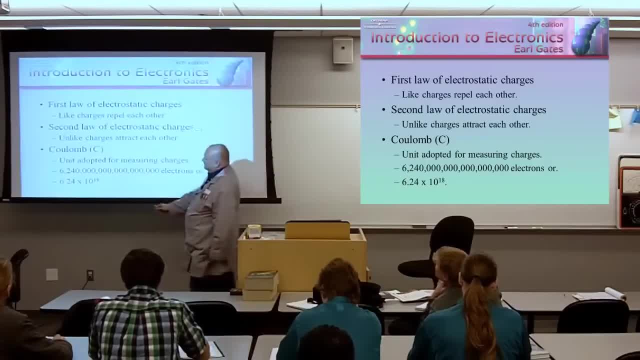 there's 18 places here. So if we went ahead and actually counted here, right, that's like us moving the decimal place from here all the way up to here. So if we went ahead and count 1,, 2,, 3,, 4,, 5,, 6,. 7,, 8,, 9,, 10,, 11,, 12,, 13,, 14,, 15,, 16,, 17, 18.. So 6, decimal point, 2,, 4,, 10,, 11,, 12,. 13,, 14,, 15,, 16,, 17,, 18.. So 6, decimal, point, 2,, 4,, 10,, 11,, 12,, 13,, 14,, 15,, 16,, 17,. 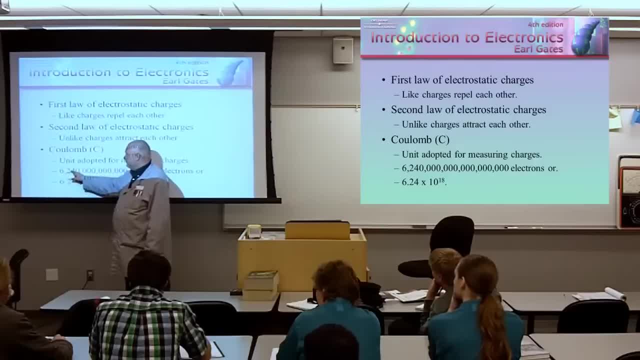 18.. So 6, decimal point, 2,, 4, 10,, 11,, 12,, 13,, 14,, 15,, 16,, 17,, 18.. So that's what we're going to do. 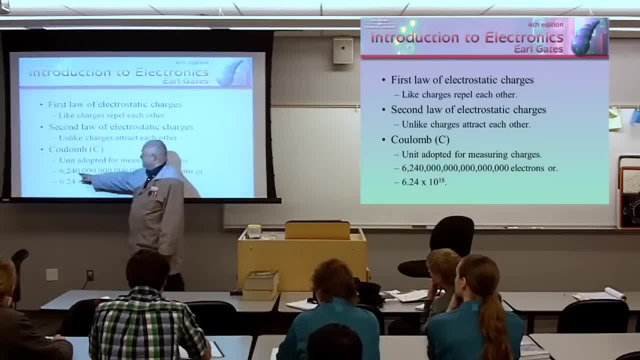 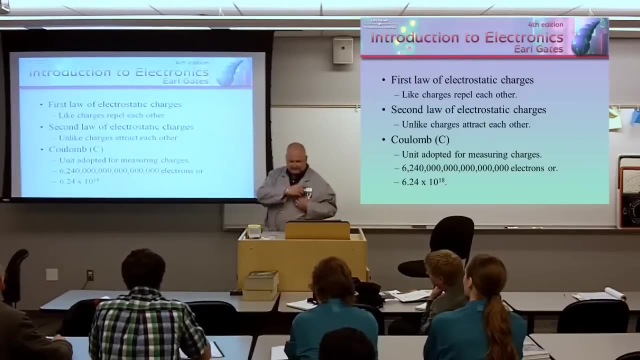 here. We're going to go back to the original formula. We're going to go back to our formula. We're going to go back to our formula And we're going to go back to our formula And we're going to go back. 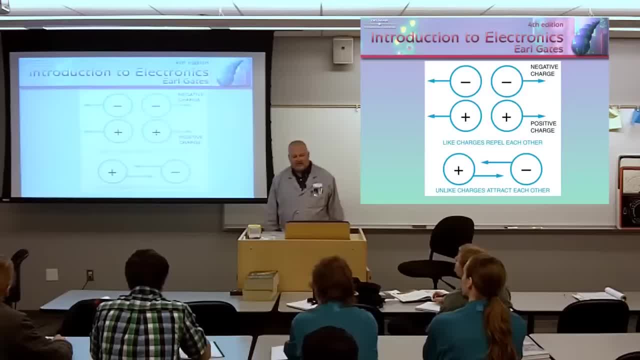 to our formula again. So we are going positive, Uh-uh, Negative on a positive Uh-huh, Uh-huh, Because remember, in the beginning everything was in a neutral natural state anyway, right? So originally everything was. 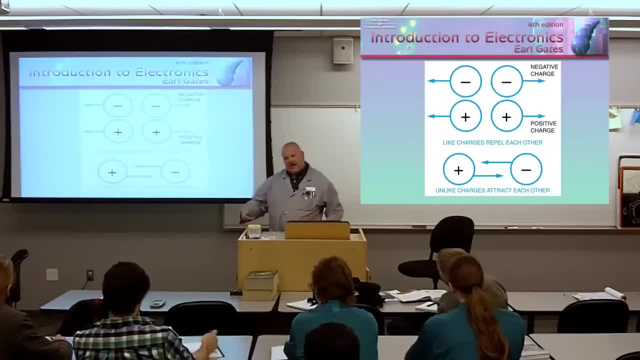 like harmonious, balanced. When we apply energy to matter, we knock an electron off that valence shell And all is that valence shell. that electron that we knocked off has in mind is getting back and putting that atom in a neutral natural state. So if you put an electron in 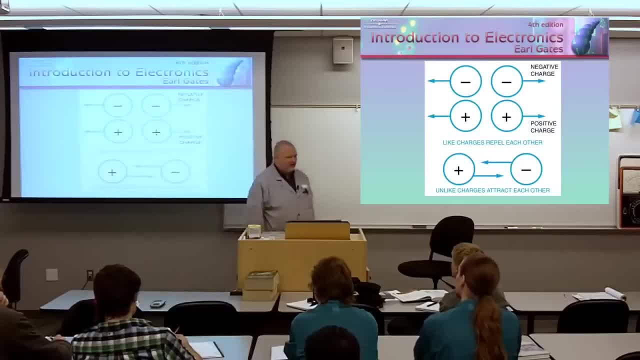 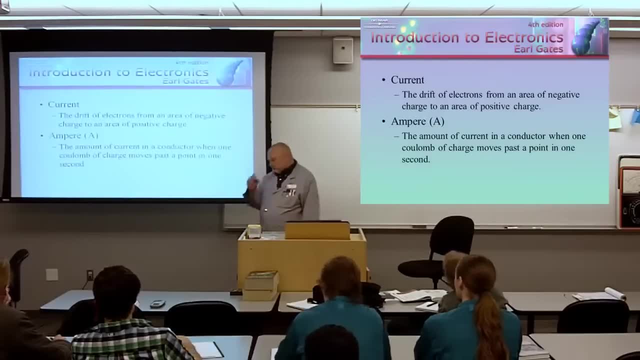 the same room with a positive ion. they're going to seek each other out. They want to achieve balance and harmony, Make sense, Current, Current, And every time I use this word here we should like ring bells, chimes, hit a gong, something like that. Because this: 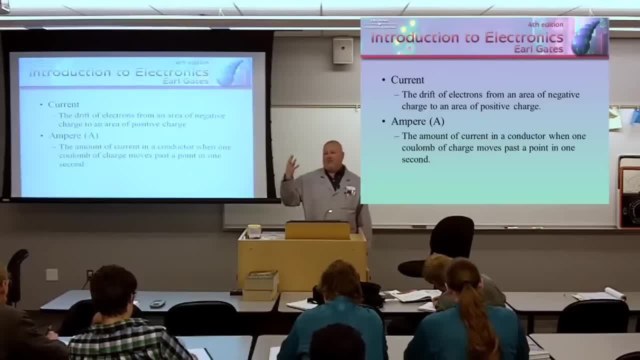 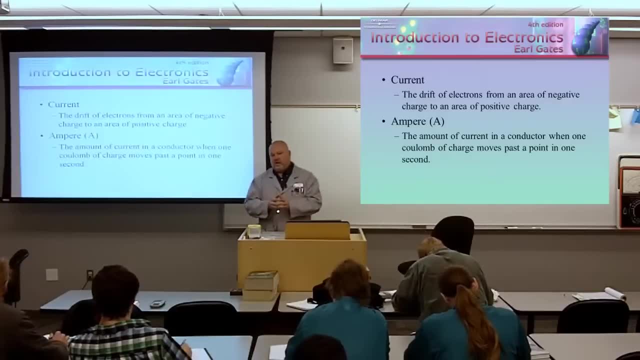 is like a holy word- A holy word in electronics. There's four properties that you really need to be infatuated with, And when I say infatuated with, I'm not talking about just as a student. I'm talking about later on, when you continue on with your career, The worst day you have in this industry. 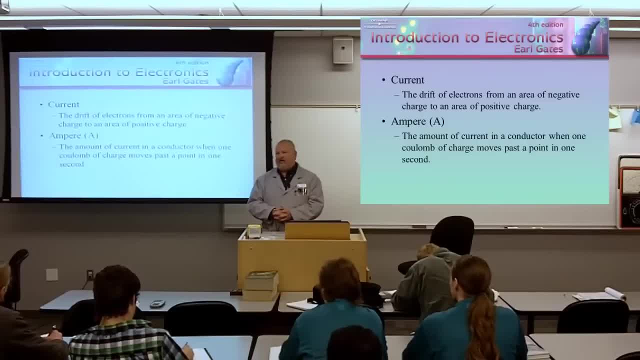 is a paid electronics professional. The problem will be solved by understanding and knowing the behavior of voltage, current, resistance and power period. Do I sound like I'm oversimplifying it? I'm not. It gets that basic If they've got an electrical problem with the space shuttle and they can't hit the button. 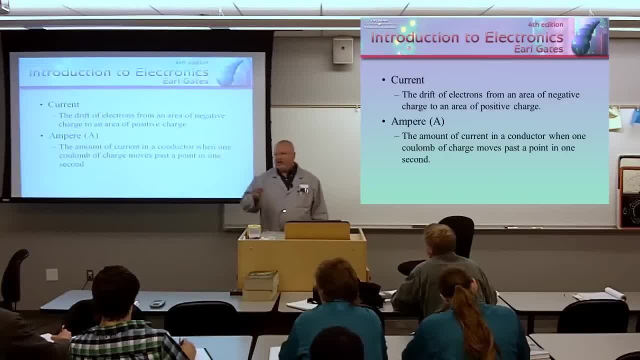 and have it blast off. it's because voltage, current, resistance or power isn't doing what it's supposed to be doing. So if you know everything about those four parameters on the space shuttle, you can get in and look at those four parameters and quickly find. 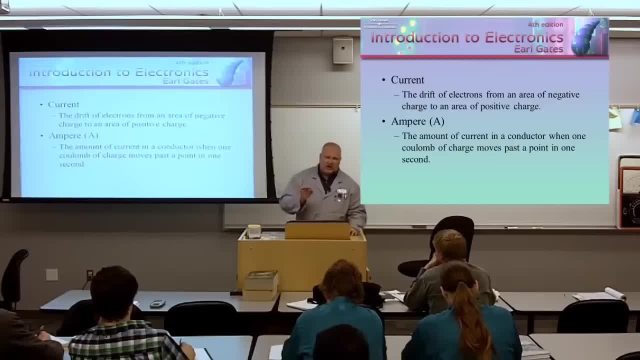 where the problem is. So today we're talking about current. We should ring bells, hit chimes, hit a gong or something, because current is one of the big four properties. Now the textbook talks about current. Current is being the drift of electrons from an area of negative charge to an area of positive. 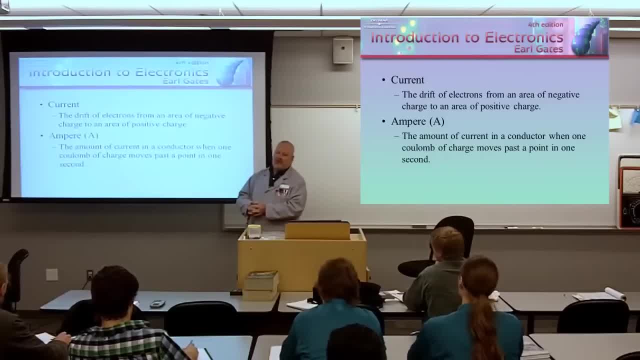 charge. I don't like this definition, the drift of electrons. It makes it look like I'm an electron and I'm drifting. floating An electron is more like if I'm negative charge and there's like positive ions out in the freaking hall, I'm going to be like I'm going. 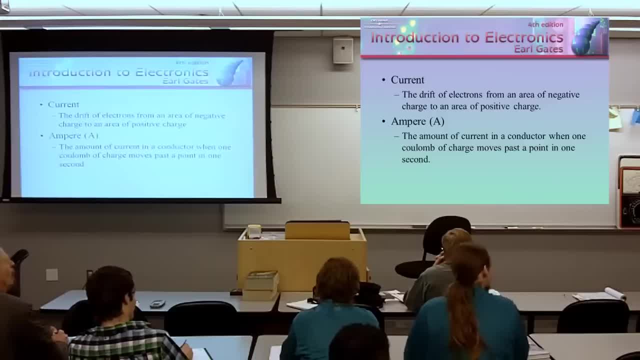 to be like I'm going to be trying to get over there. Why? Because I want to fill those holes. I want to fill the void that was created when energy was imparted on matter. Does that make sense? So that's really the behavior of current. As a matter of fact, that was kind of a mad. 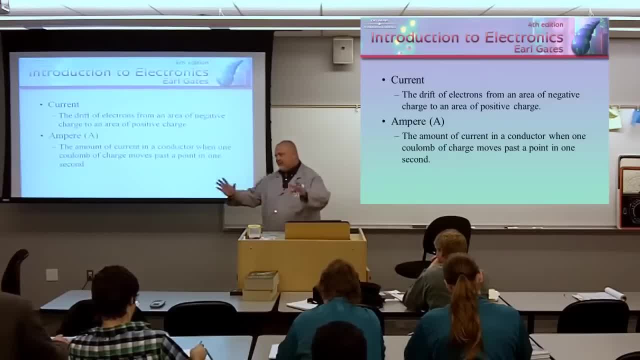 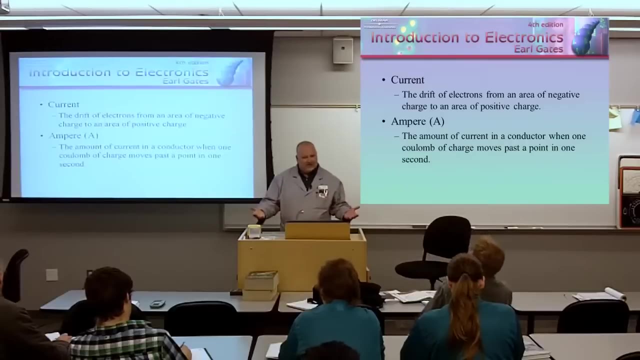 dash, I bet you didn't think I had it in me. huh, It gets better than that. You know how quickly electrons are going to go over there if you can complete the path At the speed of light. At the speed of light, If we allow electrons to complete the path, it's going to travel. 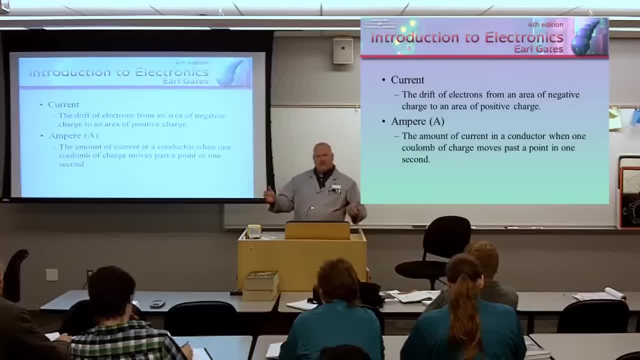 at the speed of light. So I don't call that the drift of electrons negative to positive. Now, Andre-Marie Ampere came up with this term that he called the. Ampere named it after himself. These dudes didn't have egos, You kidding, They didn't have egos, Andre-Marie. 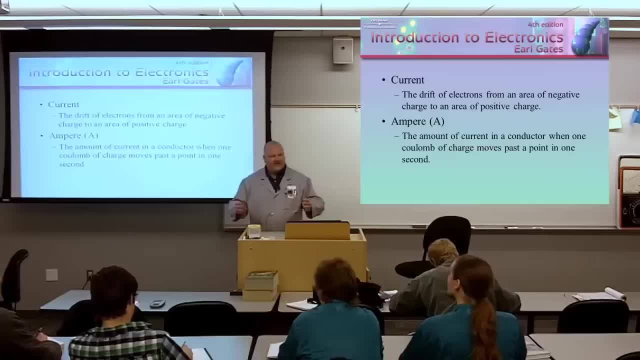 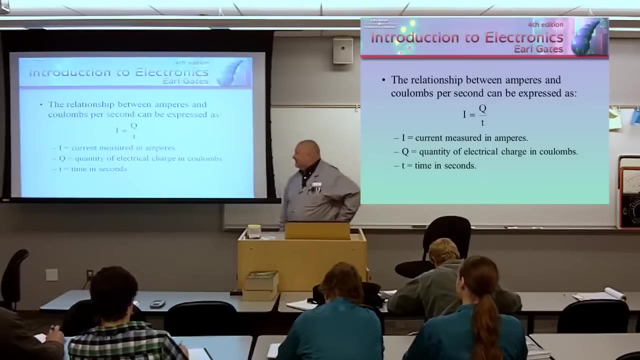 Ampere invented a, A unit of measure called the Smith, Now the Ampere. The Ampere is the amount of current in a conductor when one coulomb of charge moves past a point in one second. This is kind of emotional. This is your first rule formula. It's your first rule formula: The 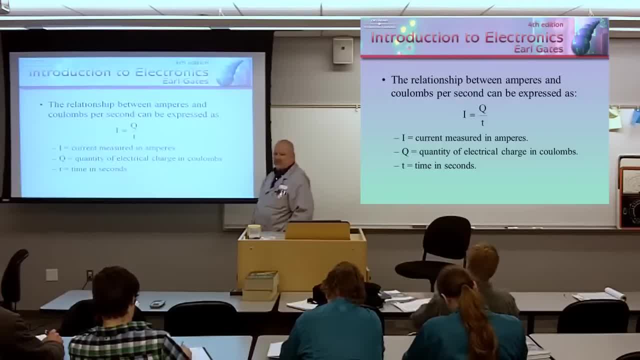 relationship between Amperes and coulombs per second can be as expressed as I, which is current, is equal to Q charge Current measured in coulombs divided by T time measured in seconds. So what we're. 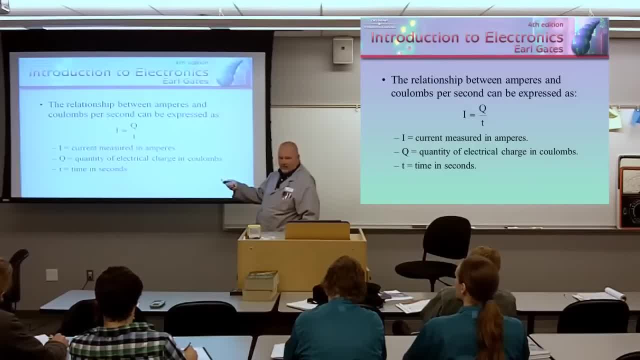 saying here is one amp, or Ampere is equal to one coulomb per second. Now be careful with this, because I could ask you a question about number of electrons. Is number of electrons coulombs? Number of electrons is number of electrons. 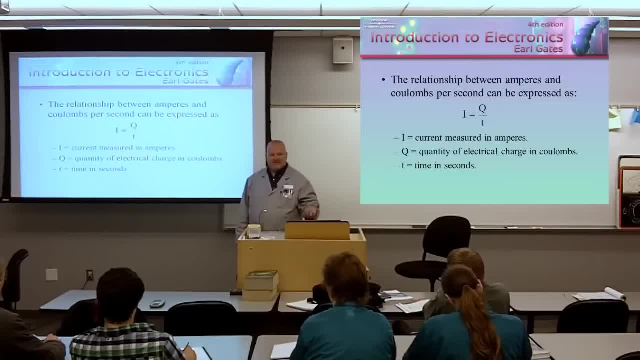 Coolum is 6.24 times 10 to the 18th electrons. So this formula only works if you're using coulombs. What happens if I have half a coulomb per second? It's not a trick question If. 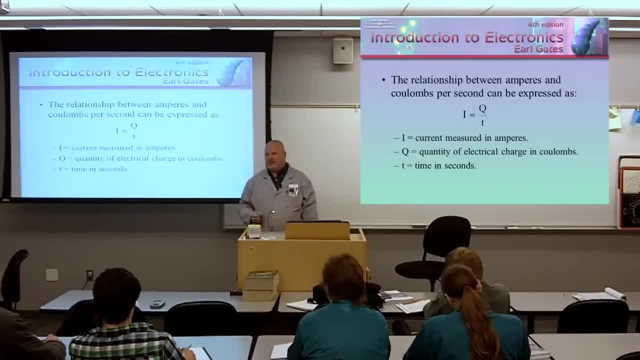 I have half a coulomb per second. what's my current going to be Half an amp If I have a quarter of a coulomb per second? what's it going to be A quarter of an amp If I have two coulombs per second? this is a trick question, No, just kidding Two coulombs. 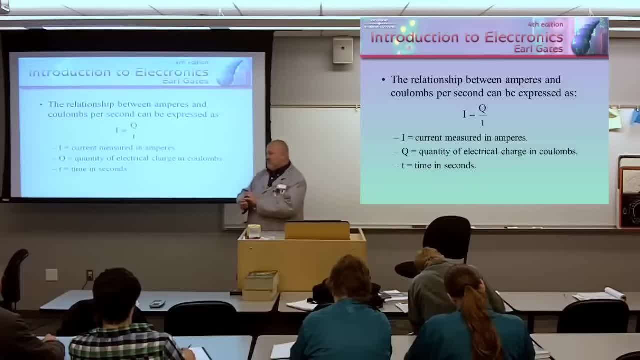 per second. That means I'm going to have two amps. So typically for household current in your home. we talked about this last week. What was that number? What's your typical utility connection from the power company to your home? That's the voltage. What's a. 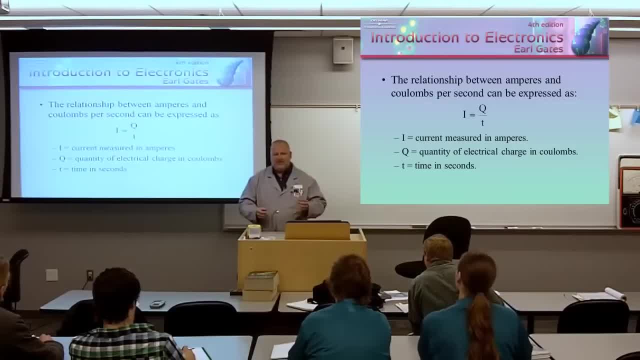 typical box. 250. Typically about 200 amps is a typical residential connection. You buy a home you're going to see that it's typically 200 amp connection from the power pole. or if you have underground service to your box- that big gray box that's in your house, 200 amps From that box. the 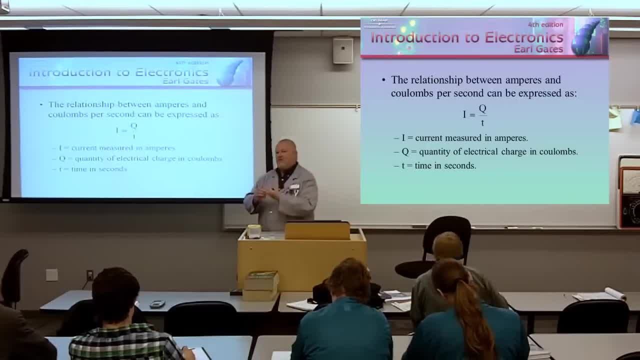 circuits in your home get distributed to circuits that are typically either 15 amps or, in some cases, 20 amps, And for some of your appliances, You know, they'll be a little bit higher in some cases If you have an electric hot. 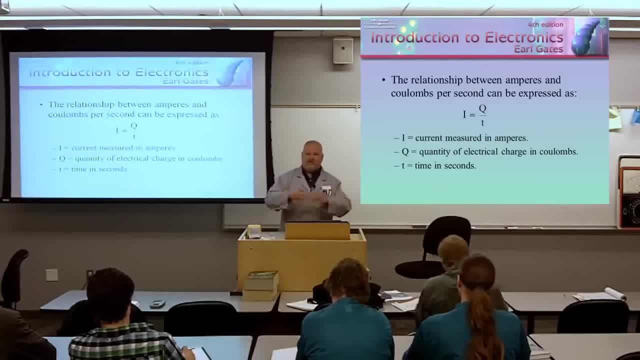 water heater or things like that. I've got a hot tub. It requires more than 15 amps, more than 20 amps, So I've got a high current connection going to that. So if you've got 15 amp outlet in your home, that means that outlet is capable of handling. 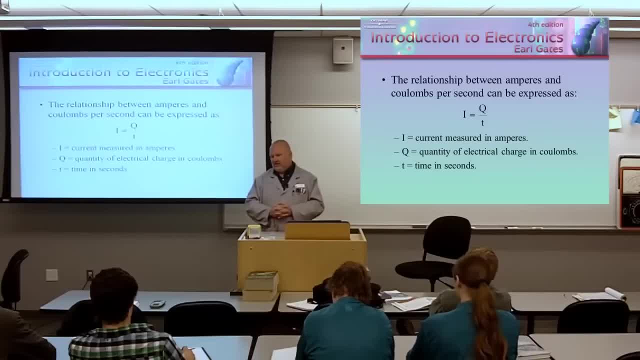 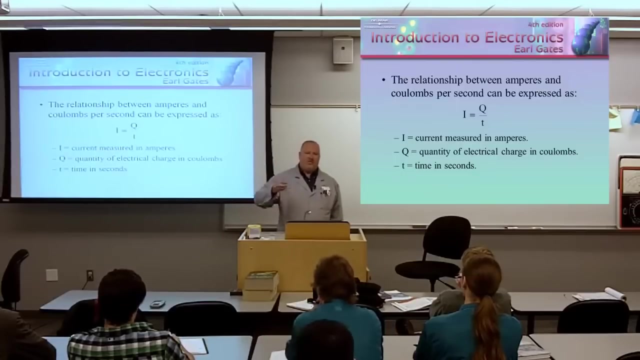 how many coulombs per second? 15. 15. 15. 15. 15. 15. 15. Right Right, Exactly Right 回. I mean the first time you're going to see that we're trying to leave that parent. 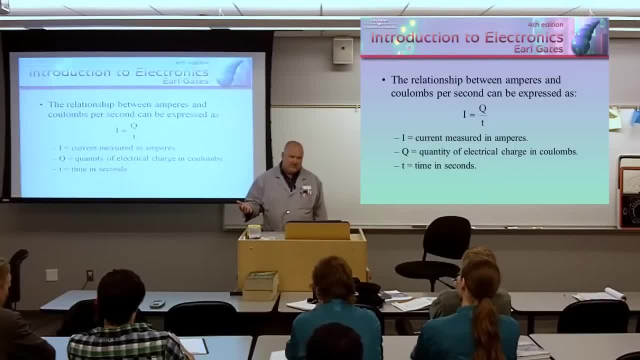 care complex as simple as I can. associated with it current ratings and this is why Physically it can't handle any more electrons. If you try pumping, you know if you got a garden hose and connected it to a fire engine. okay. 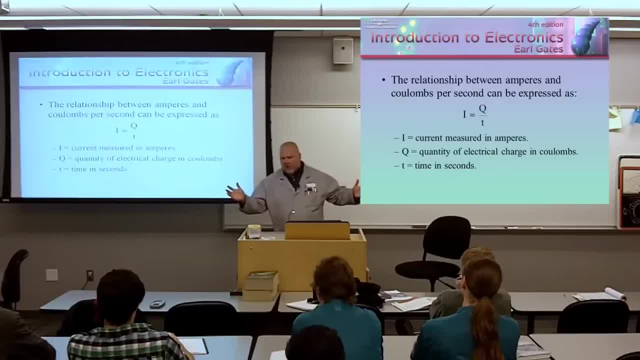 and turned the pumps on high. what do you think's going to happen to that garden hose? It's probably going to blow up. It's probably going to explode, right. It can't handle that volume. That's why firemen have like big hoses okay. 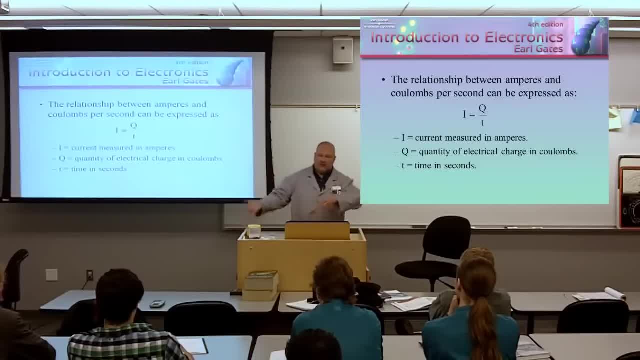 because they have a higher volume of water that they try to put, you know, from the truck onto the fire. That's why they're fire firefighters. fire people Make sense. The other thing I want to share with you about formulas: okay. 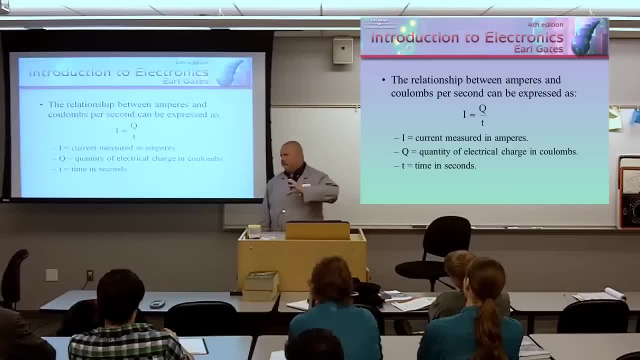 if there's shortcuts that I could teach you and you could remember. I'm all about that. This is college. so whenever I give you a formula, I'm just going to give you this formula and assume that all of you are like college students. 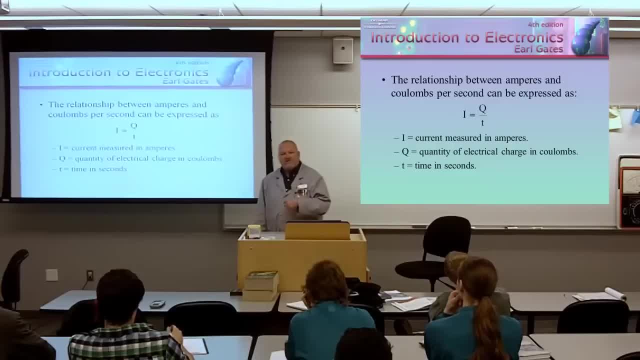 that have paid your dues and are here for the right reasons. So I'm not going to show you every possible variation of the formula. I'm going to expect you to know how to do it on your own, But I don't expect you to know how to do it on your own. 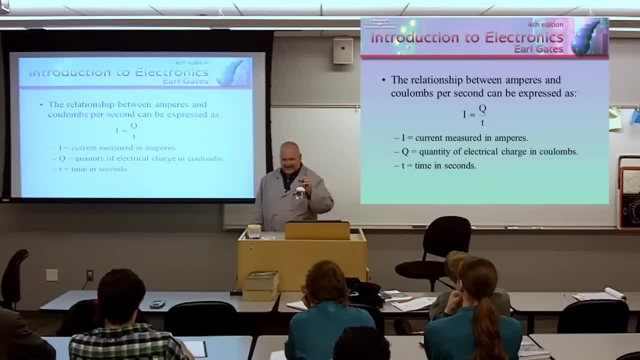 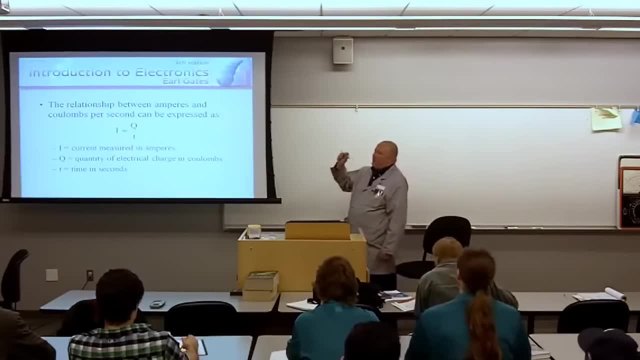 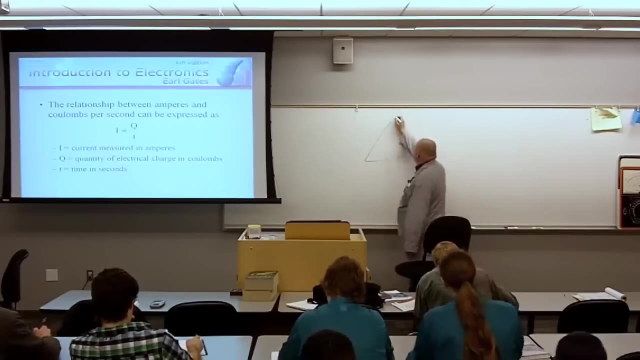 because all of you don't have a comprehensive algebra background yet. So I'm going to show you a couple shortcuts here. a way to cheat: What I want you to do is start off with drawing a triangle. A triangle I want you to draw. 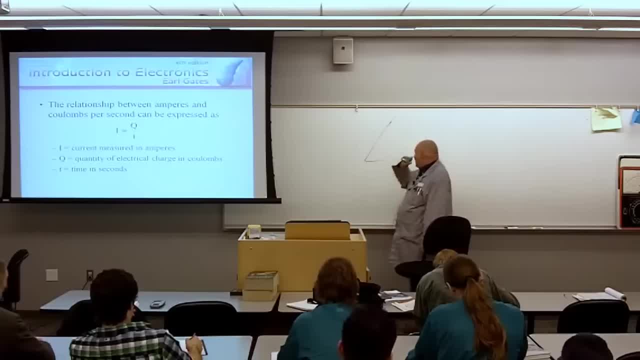 I want you to draw a simple triangle. Then, inside the triangle, I want you to draw a T, The one formula that you know. I want you to plug into this triangle. So I, in this particular case I, is equal to Q over T. 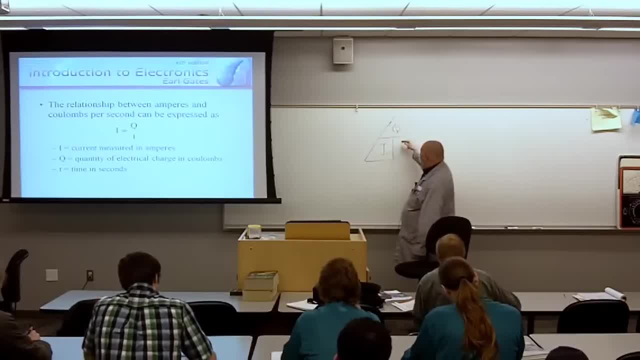 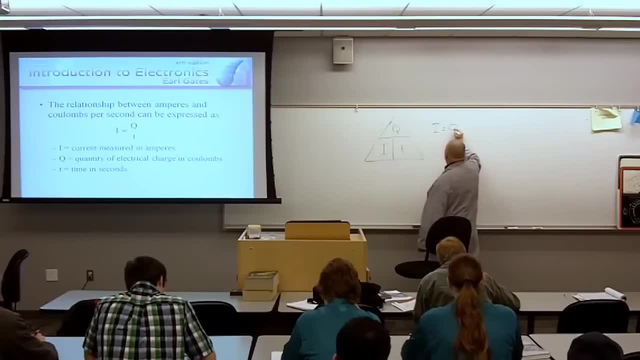 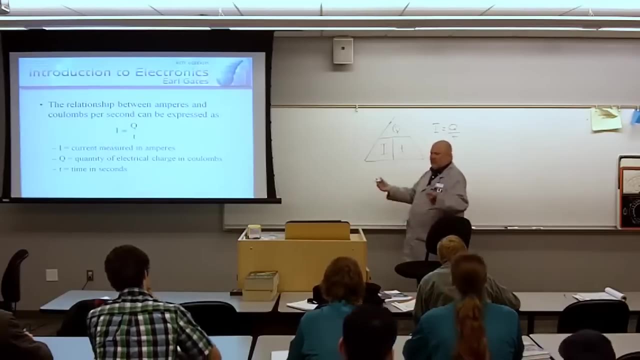 Does everybody see how I did that? I is equal to Q divided by T, So that's the first formula that I gave you. I is equal to Q over T. Now, on a quiz or an exam, or simply when you're hanging out together. 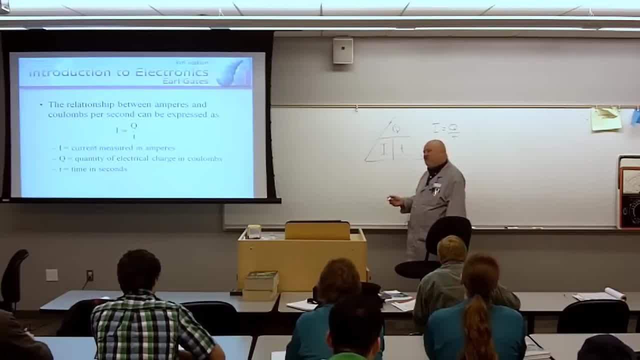 working with each other in the lab. what happens if I gave you coulombs and I gave you current? Then what we could do is simply cover up the letter T and say: T is equal to Q over I. So I did that. 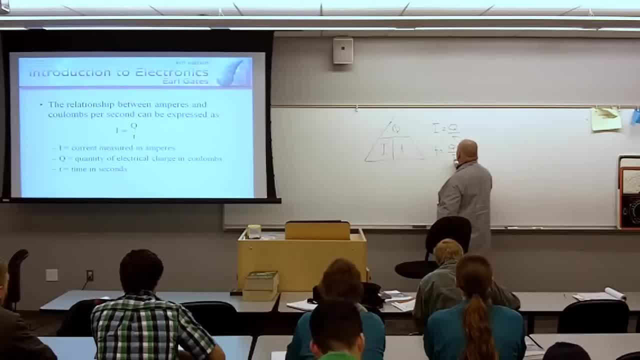 So T is equal to Q over I. That's the other algebraic manipulation of this. If I asked you on a quiz, if I said, if I gave you current and I gave you time and I wanted you to figure out how many coulombs 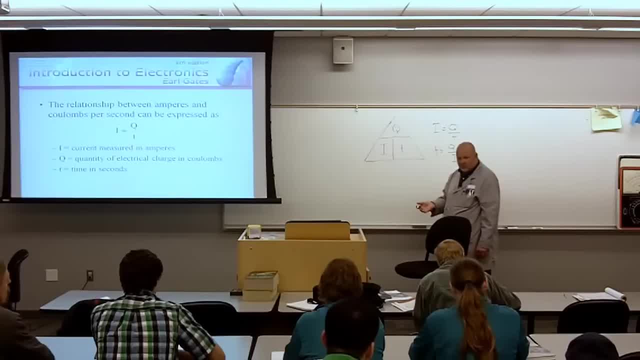 what the value of coulombs would be. then we simply cover up the Q and then it's going to be I times T. See, the I is next to the T. So it's going to be I times T. So that's going to be our other variation. 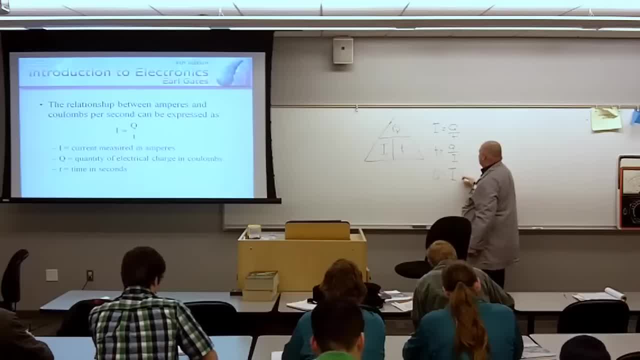 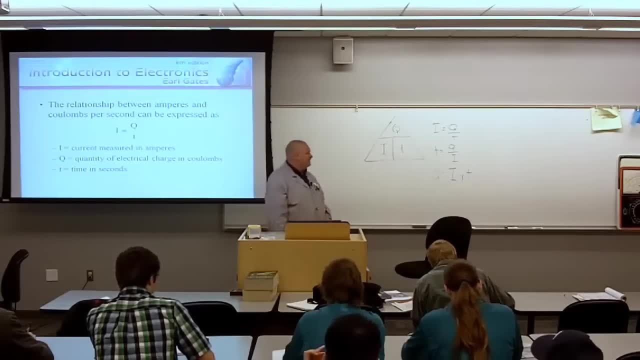 Q is equal to I times T. So with that one formula that I gave you, there's three basic algebraic manipulations that we could have, and this is all of them. So do you have to memorize these? No, Remember do the triangle. 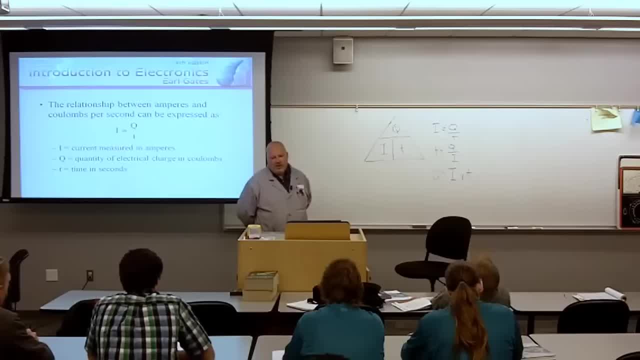 put the T in the center and then lay that one formula out, and then now you have all the algebraic variations of that formula And you know what. You need to know how to do this, because I could ask you. I'll be honest with you. 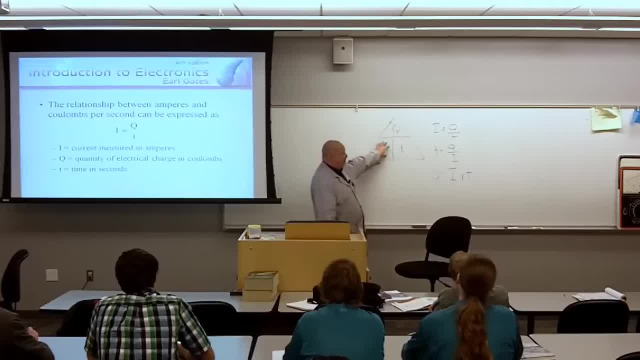 Everything right now is fair game. I could ask you to solve for current- You should be able to do it. I could ask you to solve for time- You should be able to do it. I should ask you to be able to solve for coulombs. 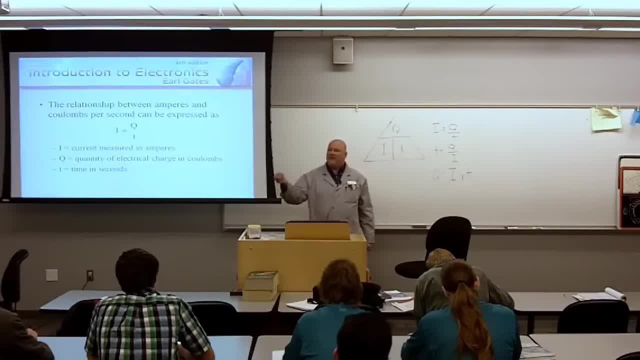 and you should be able to do it. I should be able to give you a number of electrons, right? You have 30 gazillion electrons. How many coulombs is that That gives you this value? Then you could figure out the rest. 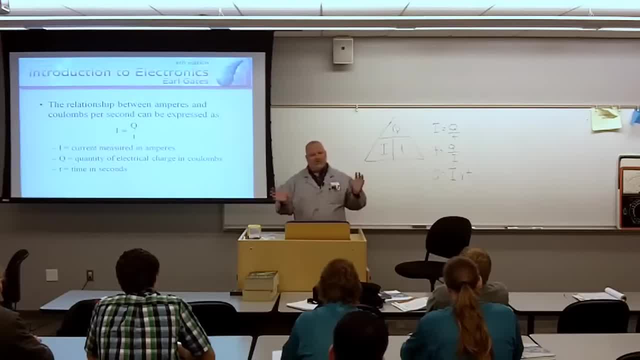 Does that make sense? So it's a stepping stone, But don't get hung up on what you don't know. Focus always on what you do know, And the one thing to remember is: one amp is one coulomb per second. I is equal to Q over T. 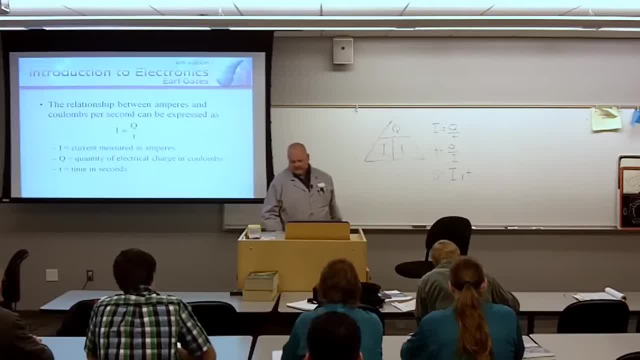 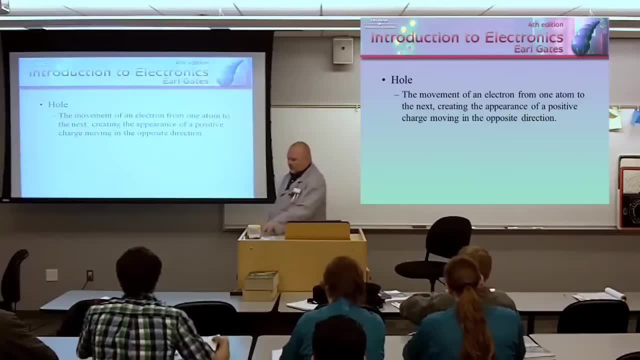 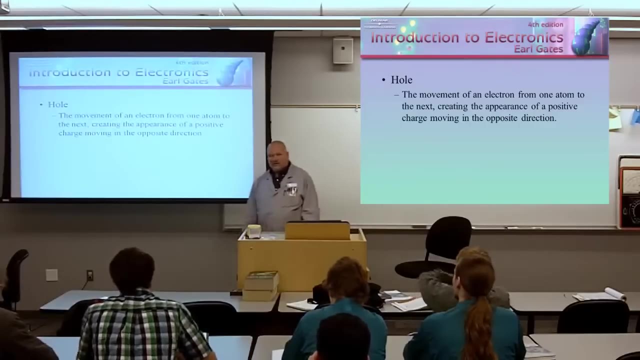 And then lay that out. It gives you all the other variations. Make sense? Sight Hole, An all-female progressive rock band from Seattle, Washington. Hole Hole- That was a joke- Is hole even still around. No, No. 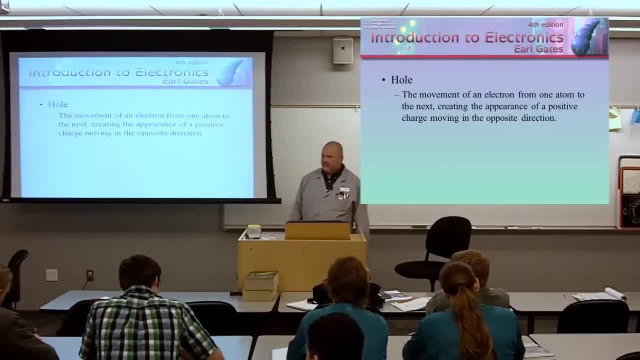 No, They're not. When did they disband? Where did they go? No, She's doing her own thing, Dad. that's what I understand. She's doing her own thing. It's a reference: What Beavis and Butthead do America? 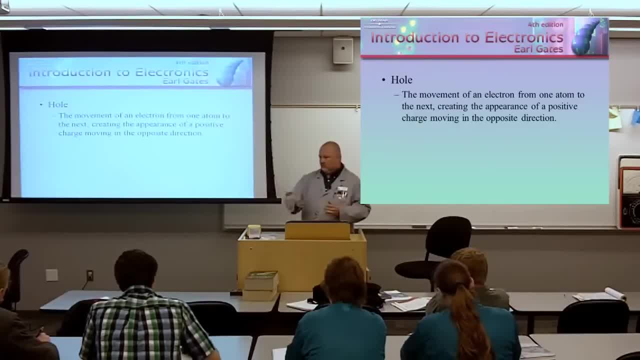 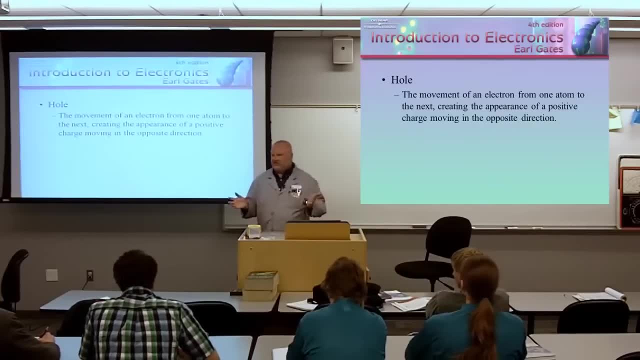 Right, There's a reference to hole, Not this hole, but the other hole. Remember they were No seriously, They were going. Remember Beavis and Butthead. do America They're looking for their TV or the TV broke and they stole one. 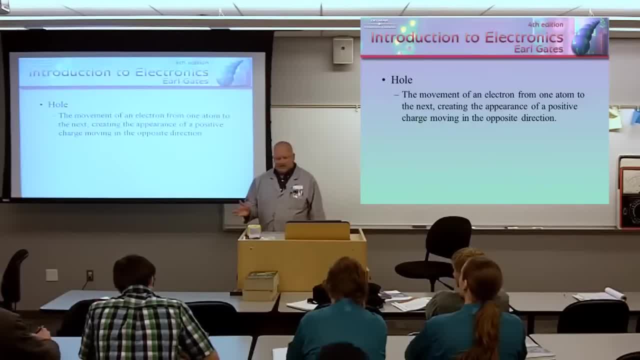 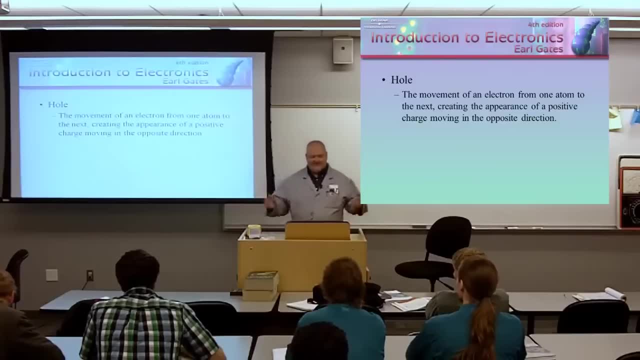 and whatever they were doing. But they were going to go to Washington Like DC. But when they heard about Washington they were like Washington, That's cool, That's like where Seattle is. We could go see Hole Anyway. 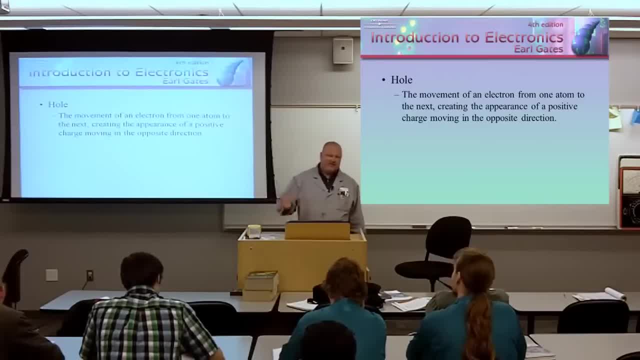 That's required viewing for all of you. Beavis and Butthead, do America. That's going to help you understand. Anyway, no, I'm talking about a different type of hole. Hole that I'm talking about here is the absence of an electron. 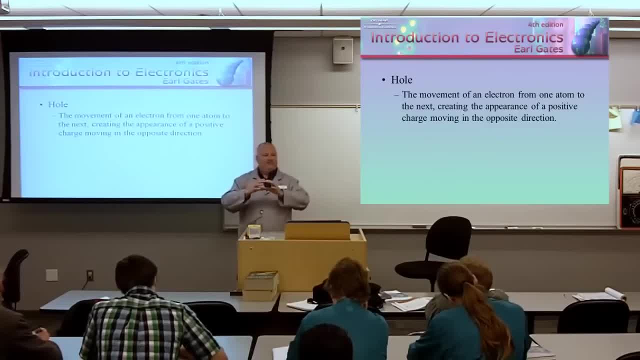 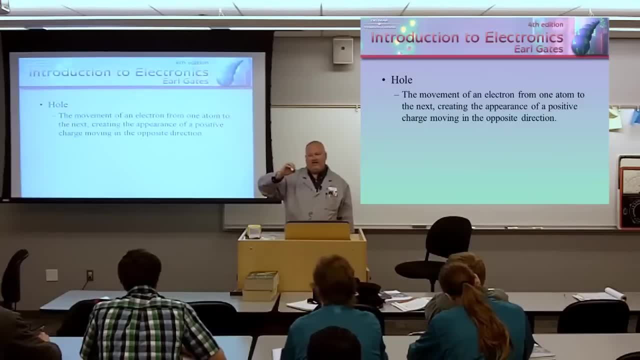 If I have an atom and I apply energy to matter and I knock that electron loose, what do I leave? What do I leave behind? A hole. So a hole is nothing more than the absence of an electron. The reason I want to point this out to you. 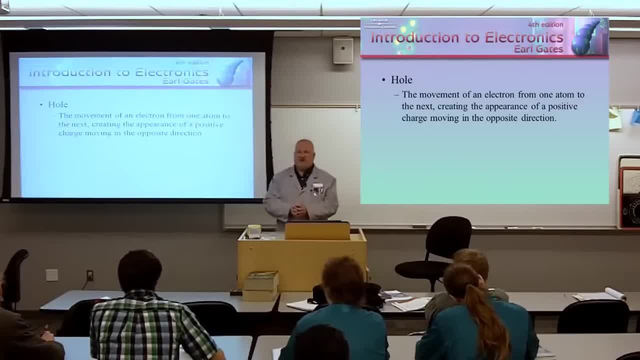 is that here at Lake Washington Technical College, every other technical and community college in Washington State, in the country, the US military, all branches of the US military, technical schools, a lot of universities, all embrace what we embrace. 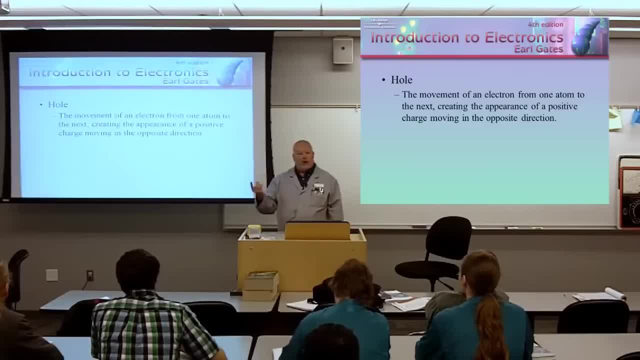 and that is electron flow. We call one amp 6.24 times 10 to the 18th electrons traveling per second. That's what we call one amp. right, Engineers, scientists embrace what's called hole flow. They think that the holes are flowing. 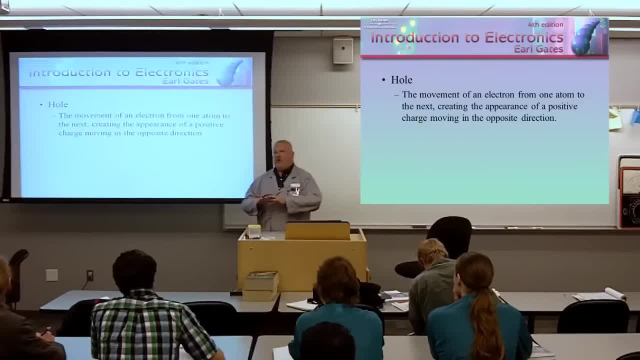 to get filled by the electrons. I don't want any of you to lose sleep over this. Whether 6.24 times 10 to the 18th, electrons travel in that direction per second, that's an amp. or 6.24 times 10 to the 18th holes. 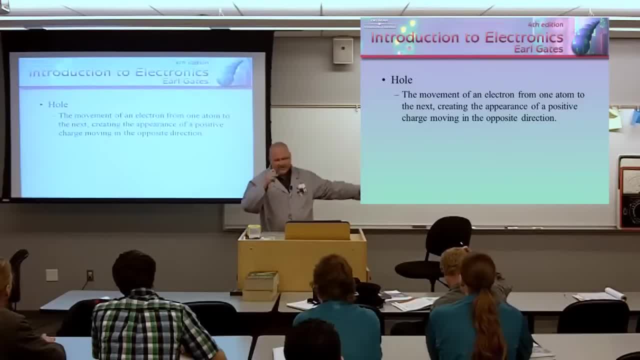 that travel in that direction per second. that's going to be an amp, But hole is the absence of the electron, And the reason I'm pointing this out to you is I know all of you this weekend, as soon as you get a little bit of time off. 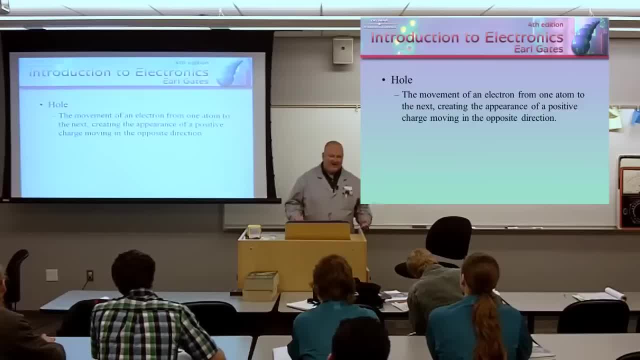 you're probably going to go to the library and pick up some electronic books, start reading. I don't want you to call me a liar. I don't want you to open up that book and say, hold on, This book shows that current flow. 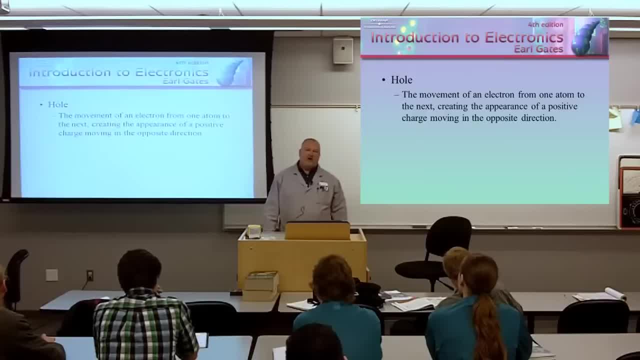 is positive to negative. That Joe Greenick over there at that lake wash- he doesn't know what he's talking about- He said that current flow is negative to positive. Current does flow negative to positive Electron flow. Current also flows positive to negative. 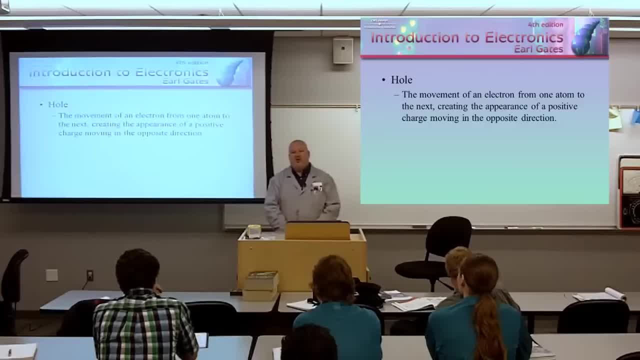 Hole flow. Are any of you going to go home and lose sleep over this? Be honest with me. Let me know, because I did. I honestly. when I was in school, I got the same lecture I'm giving you right now. 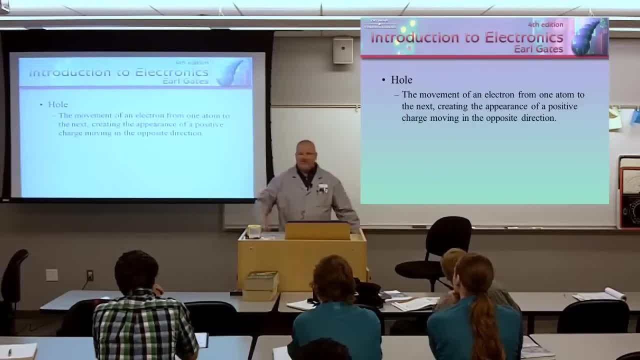 and I'm like, oh no, I didn't raise my hand. But then I went home and I'm like, scratching my head, What the heck was he talking about? And I, like months, for months, I freaking tried to analyze. 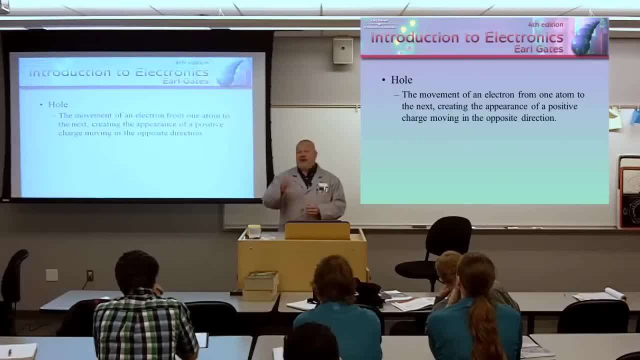 It's not that difficult of a concept. You just got to hit the I believe button. Joe says 6.24 times 70 to the 18th electrons per second equals 1 amp. So be it. We do want to talk about hole briefly. 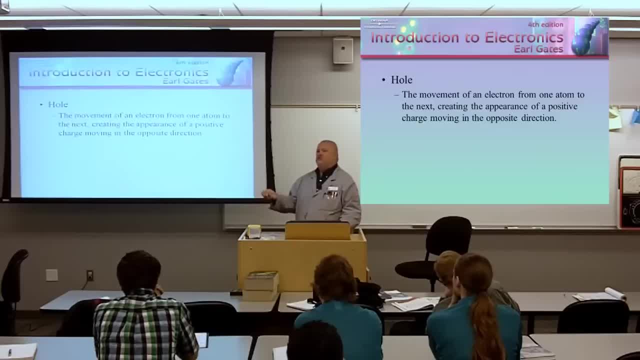 so you can differentiate between electron flow and hole flow, and also to prepare you for what you are about to receive in the future. Because, again, if you sat in on my lecture last week on ELEC 120, guess what? We started talking about hole flow again. 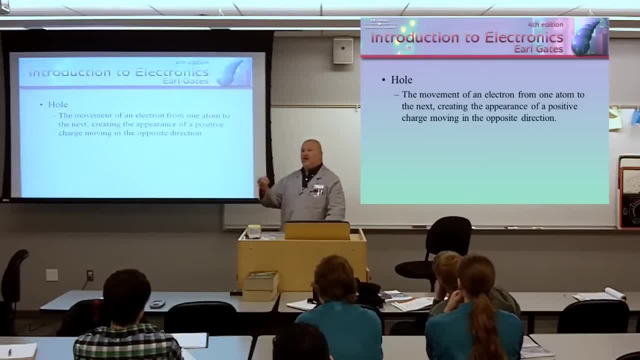 Because hole flow is significant in the study of semiconductor devices, solid state devices. If you want to understand how a transistor really works, you have to embrace hole flow. So we are going to talk about it more here at Lake Washington, but you don't need to beat yourself to death on it. 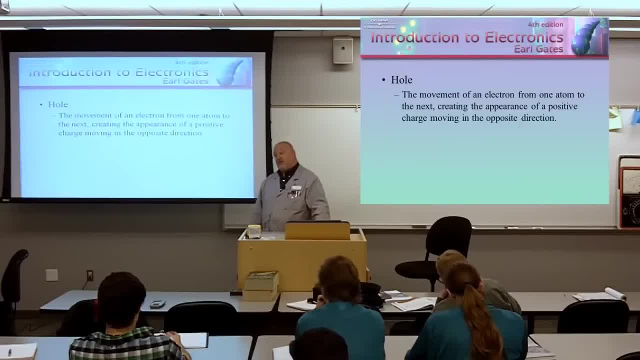 Question: Do holes have matter in them? Well, you've got to realize that the hole itself, though, is the absence, But if you're talking about matter that exists, and it's the absence of the electron, then we're really talking about a positive ion. 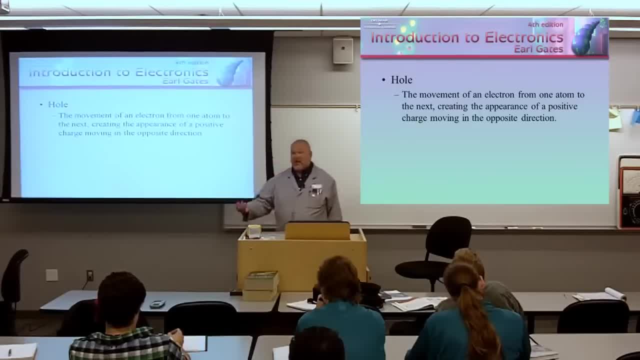 And a positive ion does have mass, because you've got all your protons, you've got all your neutrons and of course that's how we determine atomic weight. Very good Answer. A Fill in the A Atomic weight, number of protons and neutrons. 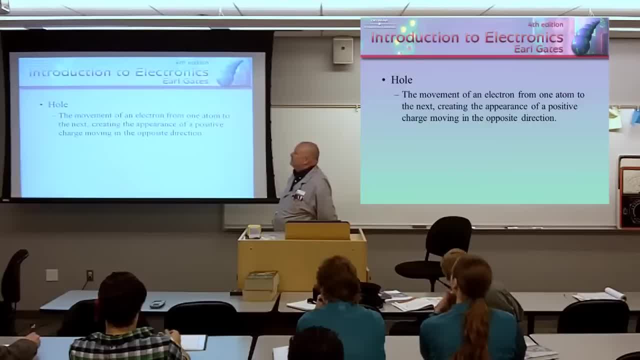 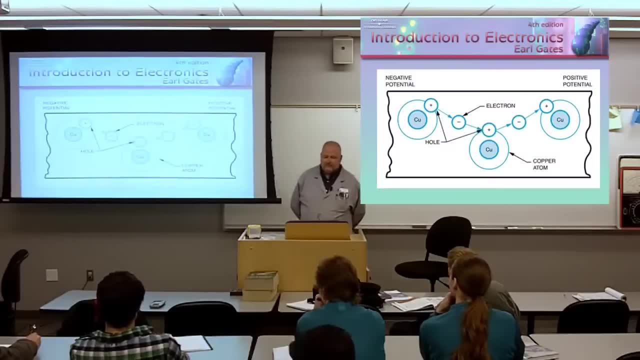 So hole is the movement of an electron from one atom to the next, creating the appearance of a positive charge moving in the opposite direction. So that's what we call hole flow. If you had a piece of copper, which we know, copper is a good, abundant conductor. 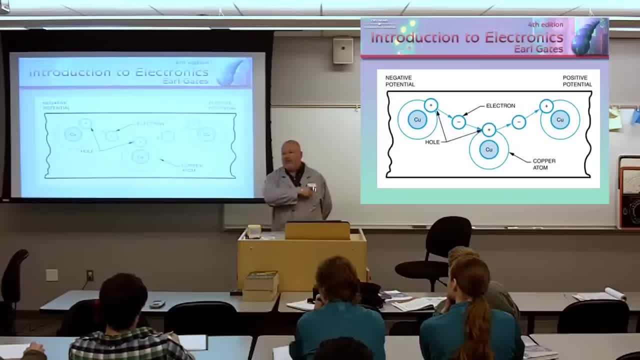 this is kind of how the electron path, how it would work: Negative to positive kind of copper atom. it would jump over here to copper atom, jump over here to copper atom. Make sense, Drifting along, Drifting, Drifting along at the speed of light. 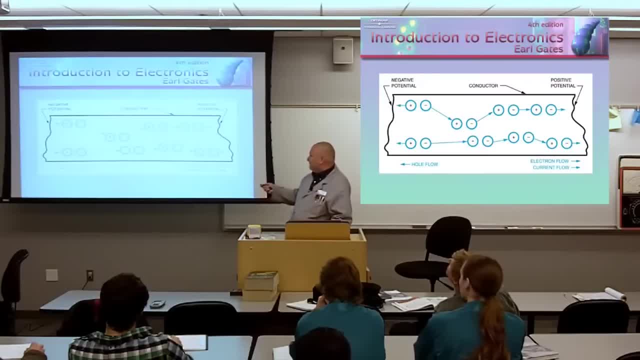 This. here we see again a conductor. We've got electron flow left to right, current flow left to right, hole flow right to left. Make sense? Okay, I want to show you something how this really works, Because the way they're making this look, 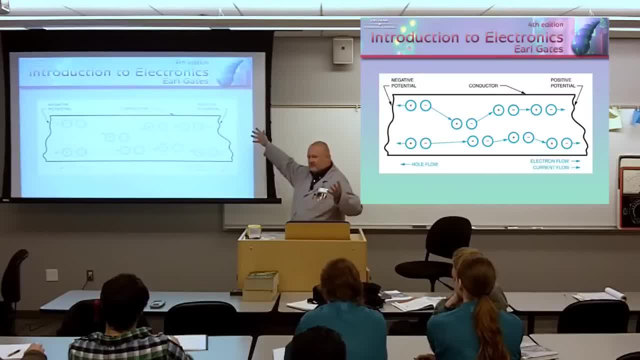 and I think you guys are all buying this right Because again you kind of got to believe me. But this is kind of like the free electron is kind of like hopping from copper atom to copper atom, because there's three or fewer electrons in a valence shell. 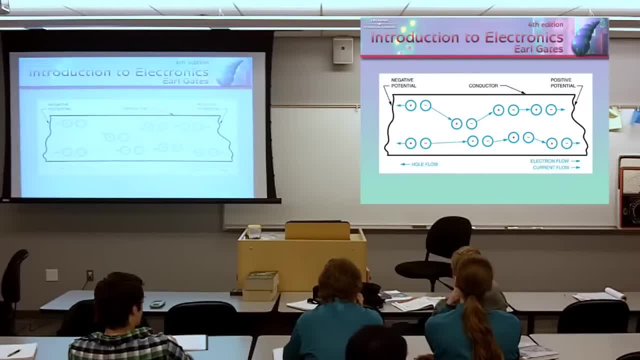 It's kind of hopping along, hopping along, there's another copper atom. You ever jump across a stream. It's kind of what they make it look like here. right, Everybody at this table here can you just back up here? Nobody has a coffee or anything on here. 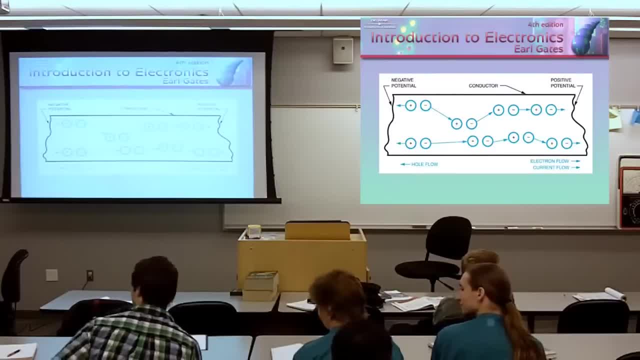 Okay, Can you put your hand on the on the end of the table, just like this, Okay, Okay, Let me know how quickly you feel this. That is how current flows through a conductor. That's how current flows through a conductor. 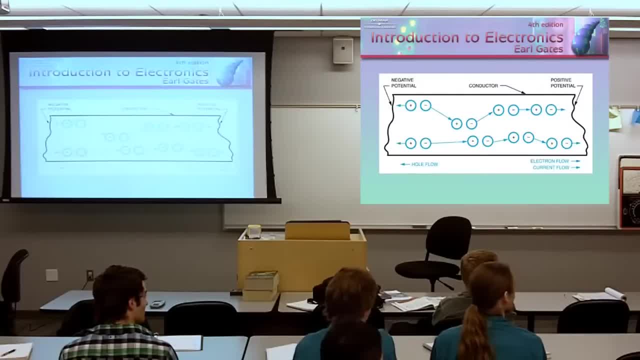 The speed of light: Instantaneous, Instantaneous. If I've got a negative here and I've got a positive there, pow, instantly. that is going to be felt on the other side. That's how current flows through a conductor. So it's not. 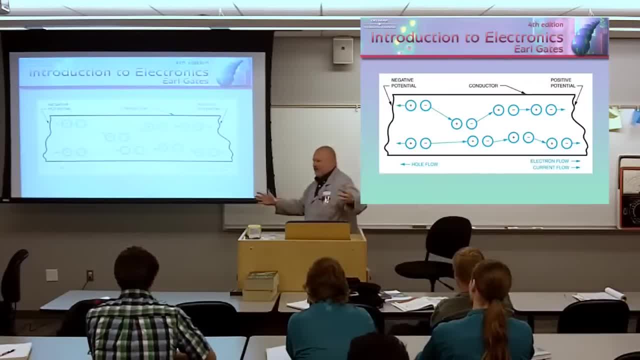 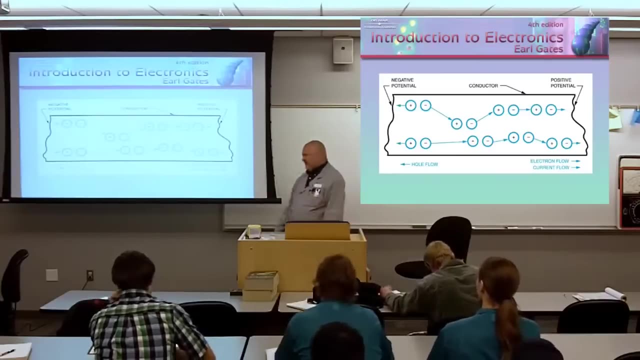 you've got to do this, Got to have your tongue out when you're doing it too right? It doesn't work like that. it's instantaneous. The speed of light, Which is important: 186,000 miles per second. The speed of light is 186,000 miles per second. 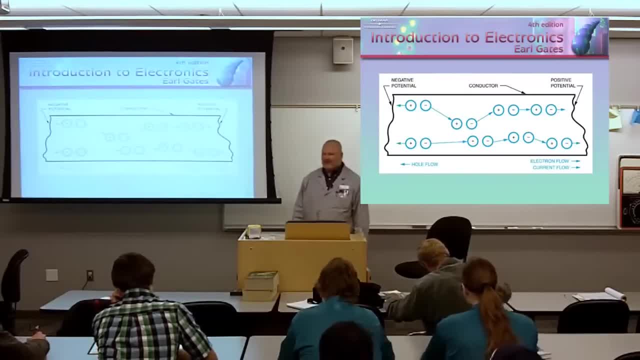 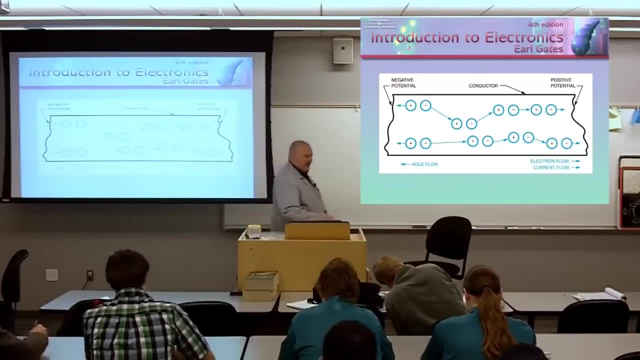 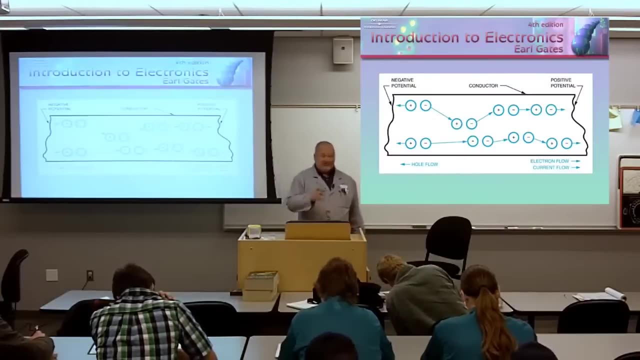 Or for those of you in the metric system, 300 million meters per second. 300 million meters per second. Or for those of you that keep track of all things nautical, 161,000 nautical miles per second. And I've got a couple of chuckles out there. 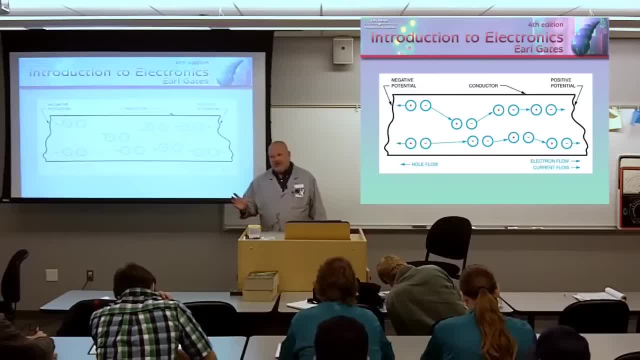 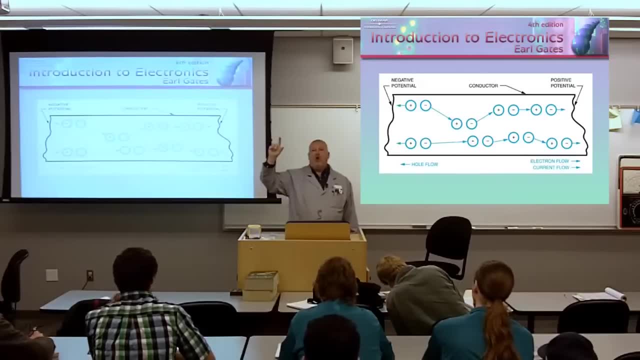 It's kind of like well Joe's ex-Navy. he would probably know that. No, I'll tell you what, If you know those three numbers: 186,000 miles per second. 300 million meters per second. 161,000 nautical miles per second. 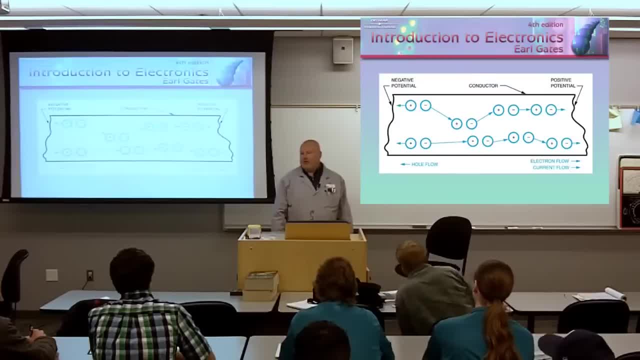 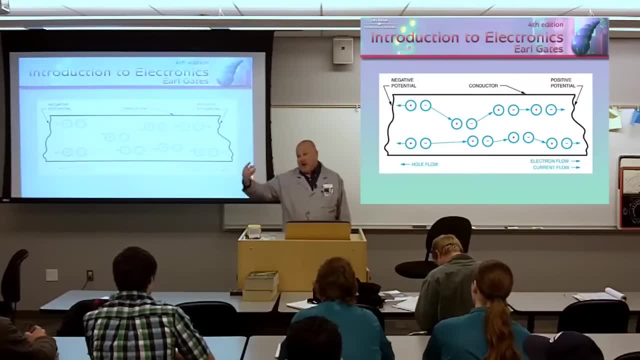 if you know those three numbers, you could probably get about eight or nine questions right on your FCC license exam, Because it's how RF energy transmits as well. If you're working on a radar, you want to get your radar endorsement to be able to work on a radar. 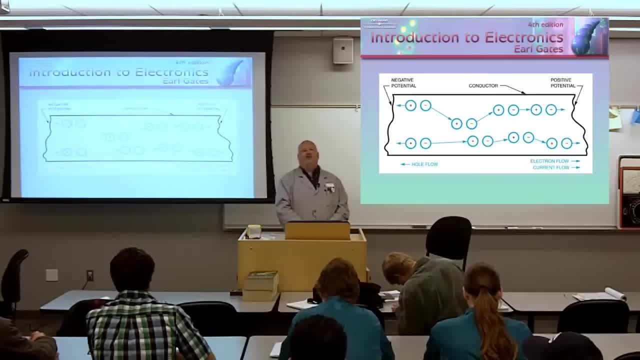 The only radar in the world that I am familiar with that operates in statute miles is the radar that's operated by the police. If you're on a Washington State ferry and they're looking at a radar, that radar is calibrated for nautical miles. 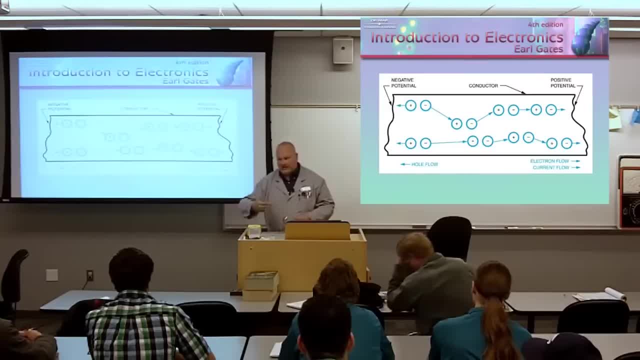 So all the math that takes place internal is 161,000 nautical miles per second If you go to work for the Federal Aviation Administration and you work at Seattle TRACON, that keeps track of all the aircraft arriving to Seattle and departing Seattle. 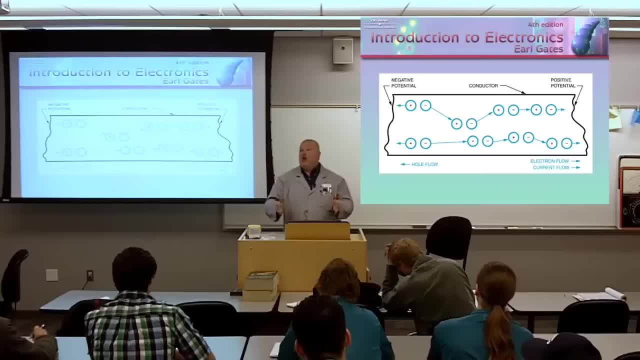 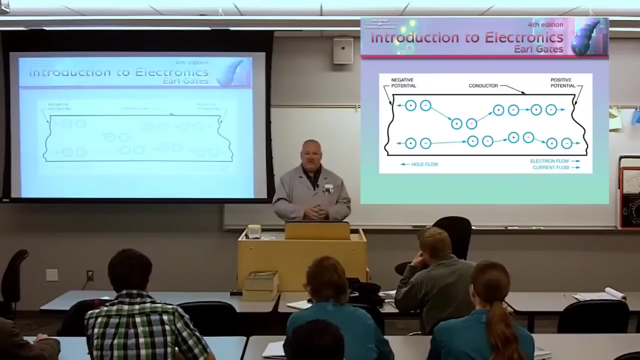 the radar that they're looking at is calibrated in nautical miles And the aircraft also travel speed-wise in knots. In knots, which is nautical miles calibration standard. So that's why those numbers are very important. That's how fast current travels. that's how fast radio frequency energy travels- at the speed of light. 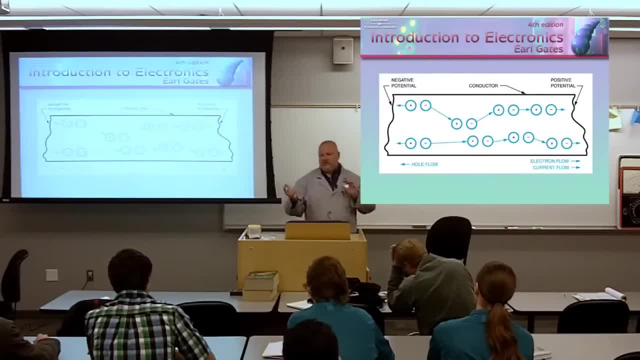 Or close to the speed of light. There's actually some atmospheric anomalies that kind of slow it up a little bit, but generally speaking, it's the speed of light Which is also important to realize. that's why it's so great you got me as an instructor, because you could learn from all of my goofy mistakes. 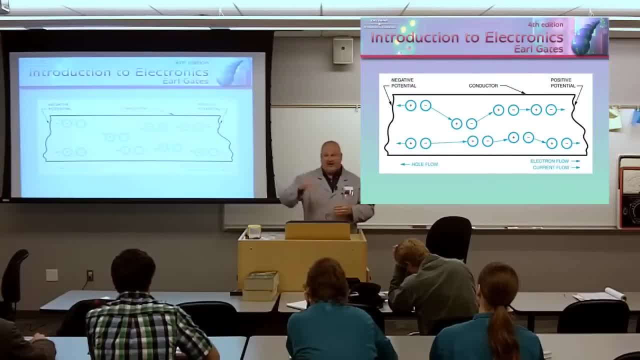 Back when I was in the Navy, the only way that I could get a raise, the only way that I could increase rank, was obviously not getting in trouble for a period of time, Which is actually another funny story. I'll show you that one within a second. 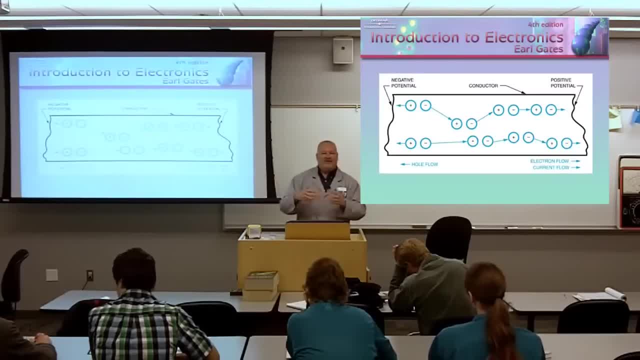 I forgot all about it, But anyway. the other thing is by taking professional examinations twice a year- And I remember one of the exams you would have thought I would have been ramped up with this stuff- I got to this whole section of the exam once when I was trying to go up and rank. 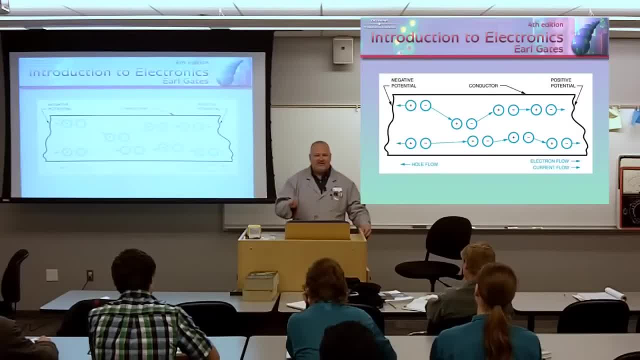 and they started talking about this, talking about the behavior of antennas in outer space, And I was like I'm a submarine guy. I have no freaking clue how this antenna is going to behave in outer space. What the heck are they talking about? The Navy's got like people in outer space. 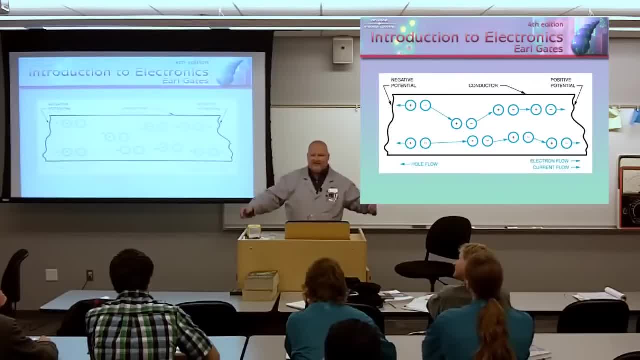 And I just got myself into a tailspin and I couldn't even answer anything. instead of looking at the obvious, How do antennas behave in outer space? Perfectly, Theoretically perfectly. That's what they were looking at. So I got all those questions wrong because 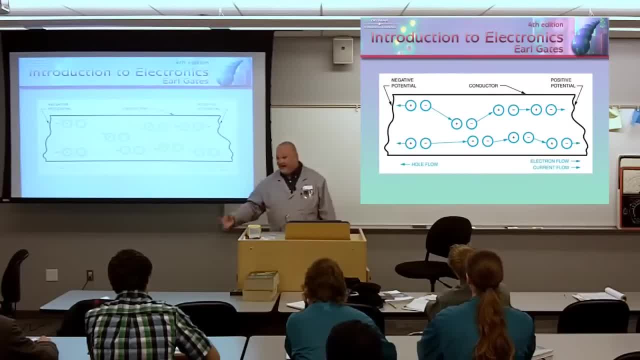 they're talking about going to freaking outer space. I'm not going to outer space, I'm going to live beneath the sea. More on keeping out of trouble. Can't make this stuff up. I was looking at a copy of my medical record. I have a copy of my military medical 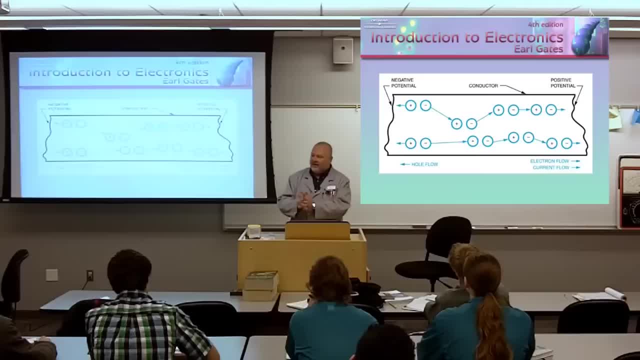 record at home and I was looking through it And I came upon a page. I got into a slight altercation And actually the medical record, uh, uh, reveals 25-year-old Caucasian reported to sick call Reports being worked over by two bouncers. 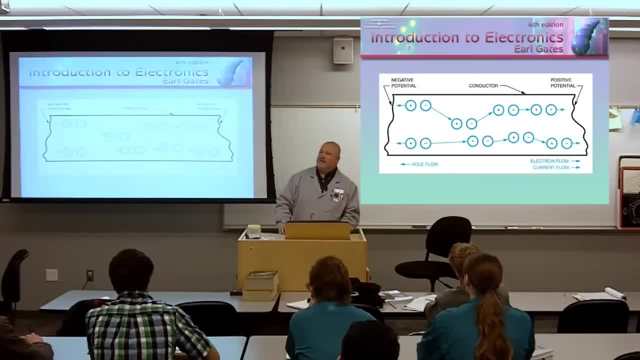 And then it goes into how I slept well and I woke up somewhat sore And, um, basically I reported to sick call and it was: I had a crushed, my cheekbone got broken And one eye was pointing one way and the other eye was pointing the other way And finally they said: you gotta go get that. 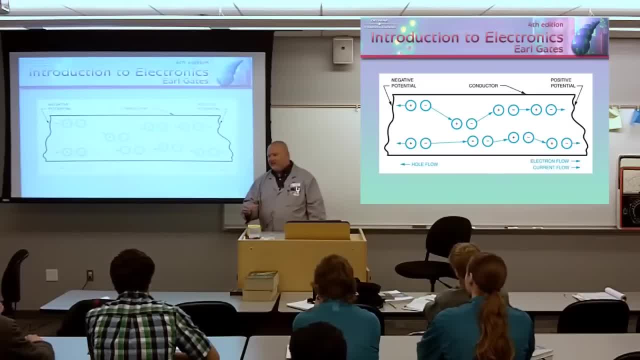 looked at. But right in there in print reports being worked over by two bouncers, Called my son over. I said: check this out, It's kinda cool. I should have that framed, Put that in my office, My medical record, you know. 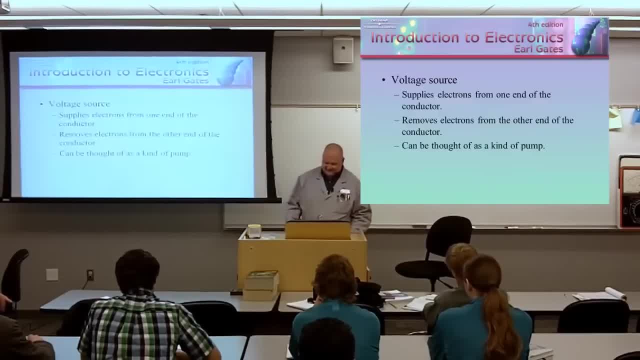 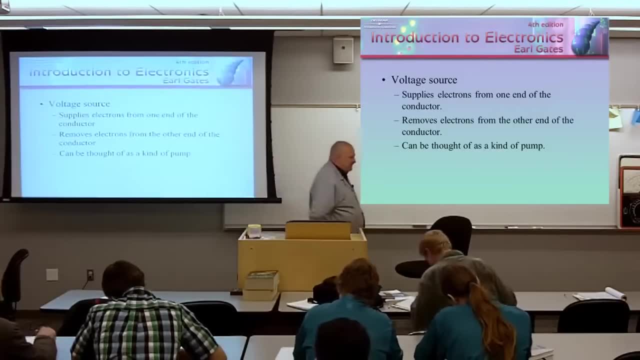 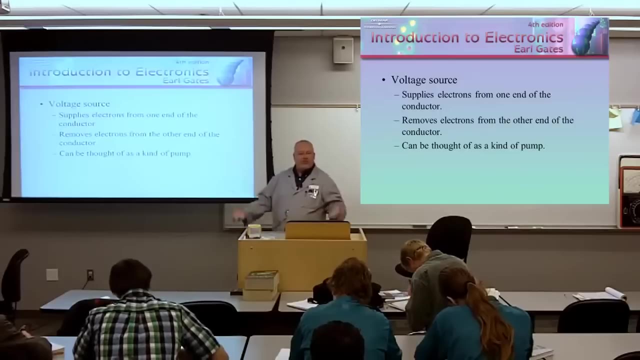 But anyway, I was a good sailor. Voltage source: And again we should almost ring bells, chimes hit gongs when we're talking about voltage source And I hope you don't think that I'm over exaggerating this, These first few chapters of what we're talking about. 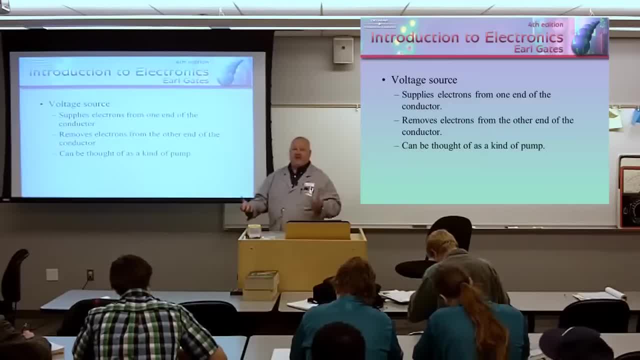 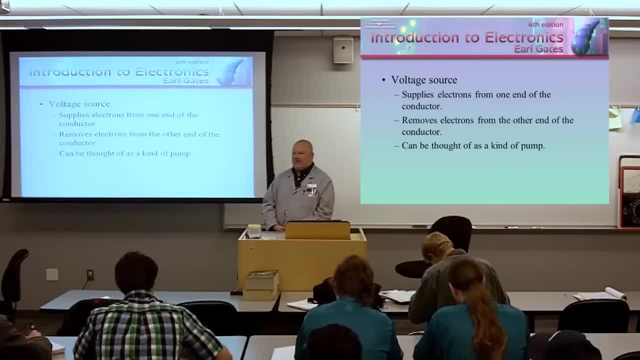 are the fundamentals. You have to understand this stuff 100%. Now you need at least a 70% to pass this class. If I were truly the pope of electronics, I'd say: no, You don't move on to the next module. 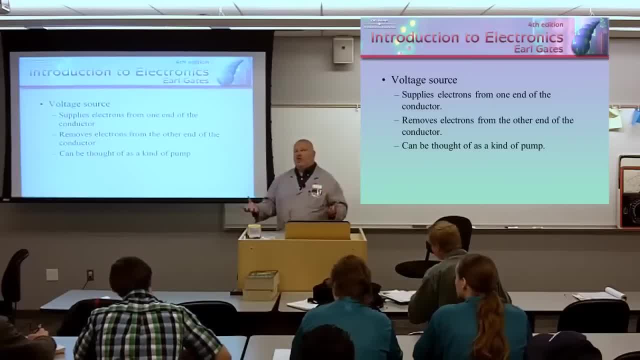 the next chapter until you prove 100%, Because this is how critical this information is. Voltage source. What we're talking about here is a power supply. It supplies electrons from one end of the conductor And it removes electrons from the other end of the conductor. It can be thought of for those of you that 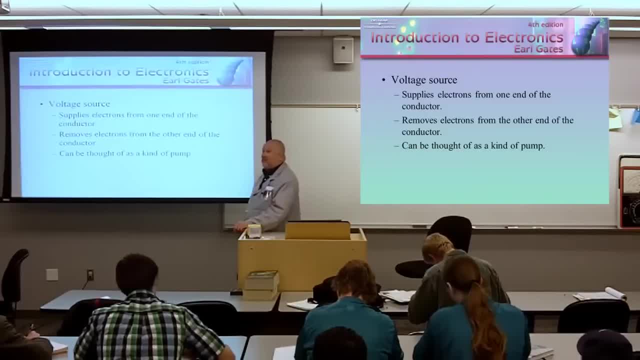 like, using analogies, fluid systems. it could be like a pump. What does a pump do? It sucks from one end. it pushes out from the other end. Right, This is what a voltage source does. It basically supplies electrons from one. 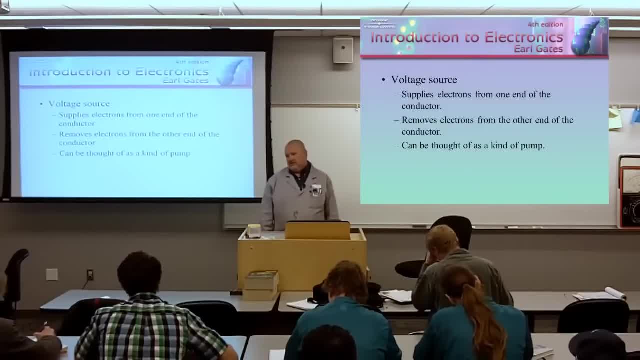 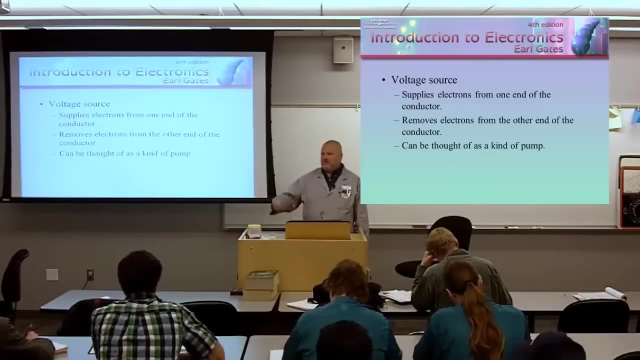 end and then sucks them back from the other end. That has to be taking place or it's not a valid voltage source. So a battery is a voltage source. We're going to talk more about batteries in future chapters. right, It provides electrons on the negative end of the battery. 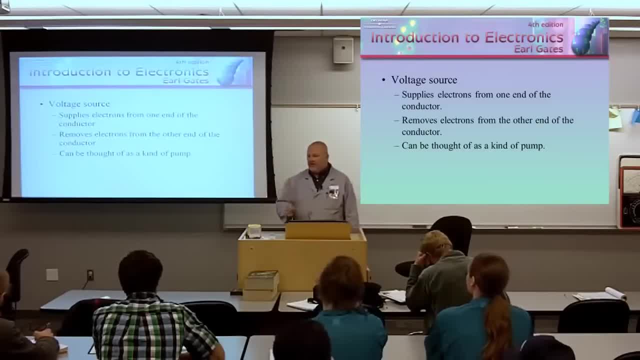 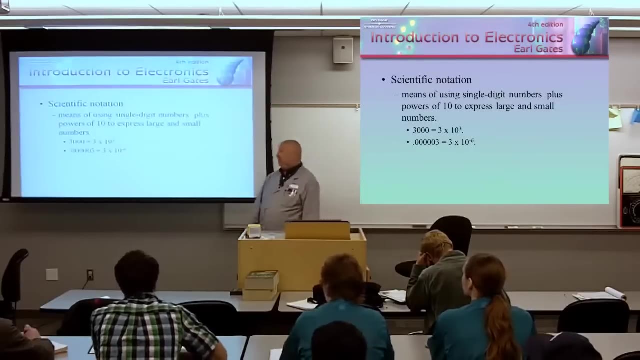 and it collects those electrons on the positive end of the battery. That's what makes it a battery, It's what makes it a voltage source, And we need a viable voltage source in order for us to have a viable circuit. Finally, we're going to talk about scientific notation, but we're not. 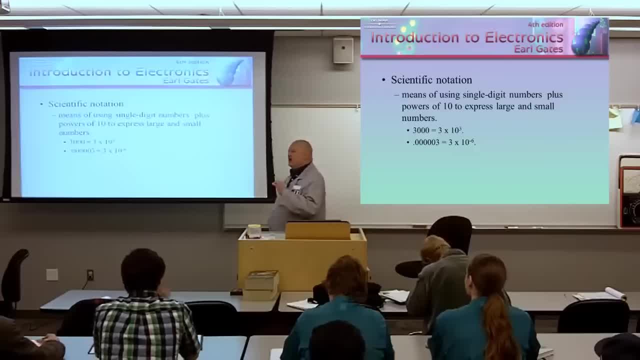 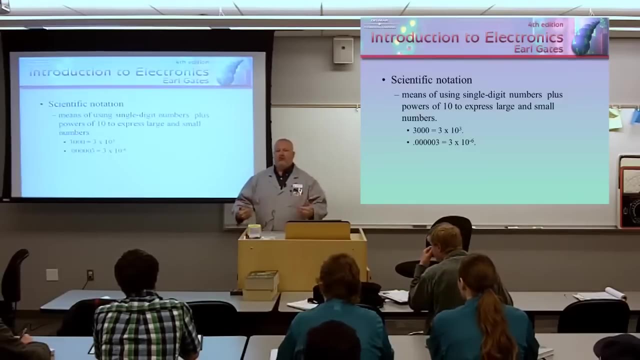 Actually, what I want to talk to all of you about tonight is what's known as engineering notation. Anybody here really comfortable using scientific notation? If you're really comfortable using scientific notation, I guess you can keep using it, but I would encourage you instead to use 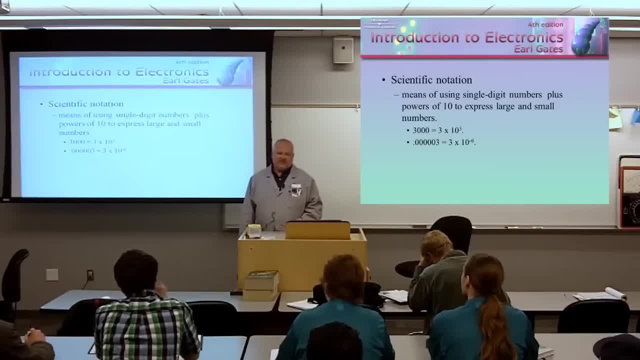 engineering notation. The difference is scientific notation can be times ten to the first power. second, third, fourth, fifth, sixth, seventh. it can be anything. You follow what I'm saying. Can you dig it? Engineering notation is always going to be in groups of three. 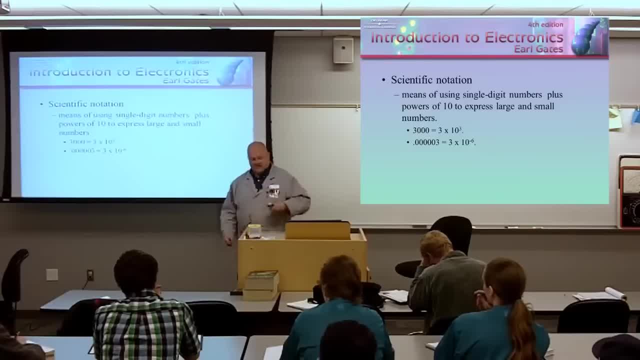 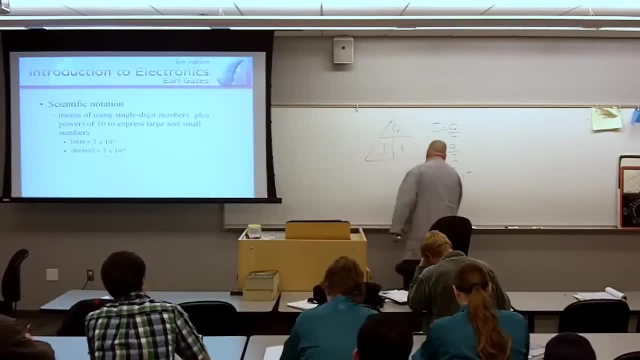 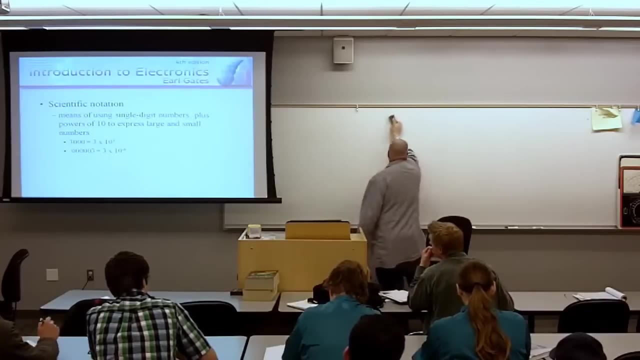 It's always going to be in groups of three, which lends itself very well to what we're doing here in electronics. Let me show you. Let's start off with a decimal point. Oops, there it is. There's the decimal point. 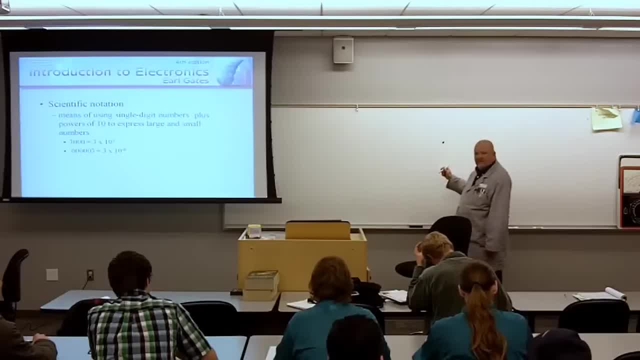 So if I put something to the left of the decimal point, this is going to be my base ten, This is going to be my ones column. So this number here could be anywhere from zero to nine. If I get nine and I add one to it, nine plus one equals. 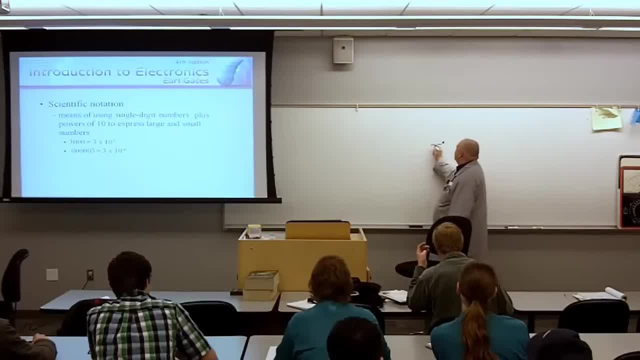 ten. So I've got to go to my tens column. So this is my tens column. this is my ones column. Can you dig it? This is the part that I did well in school too, the number line If I get up to. 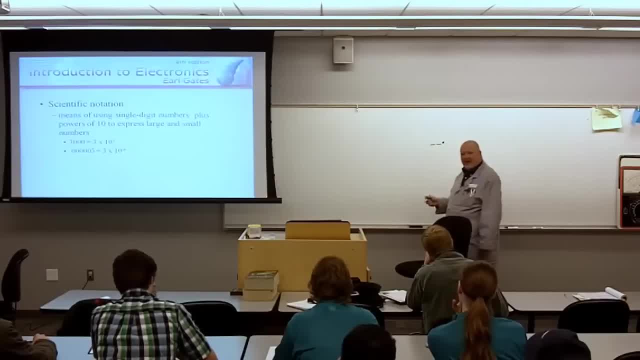 the number ninety-nine and I add one to ninety-nine. now I increment to the hundreds column, So we're familiar ones: tens, hundreds. So those are going to be my basic units of measure. This could be pounds, ounces, volts, amps. 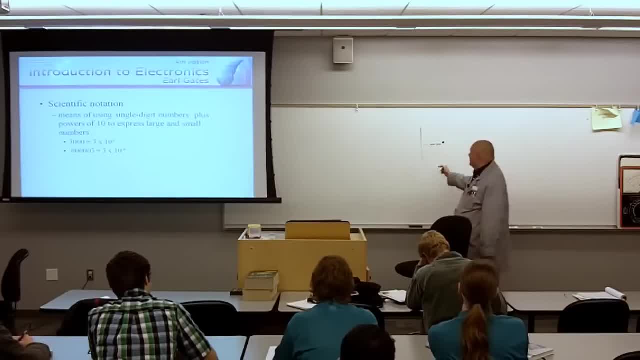 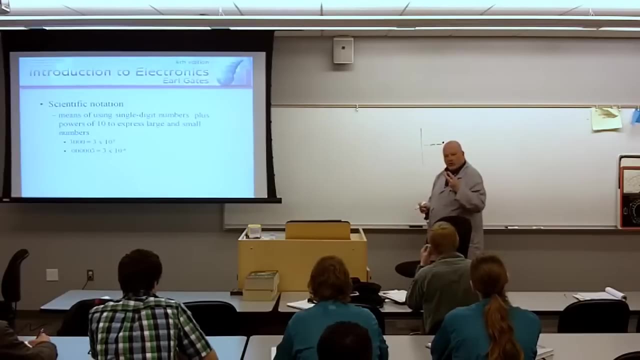 miles, whatever. Now, if I go here to my thousands column, one thousand column. basically, what I'm doing now is this is times ten to the third, Times ten to the third. Everything in here will be times ten to the third. 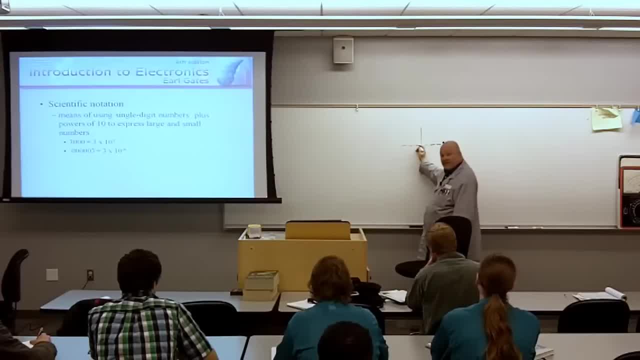 This could be one times ten to the third, twenty-two times ten to the third, nine hundred and forty-three times ten to the third. Make sense. The reason that I'm so infatuated with having you put it in engineering notation is by ten to the third. 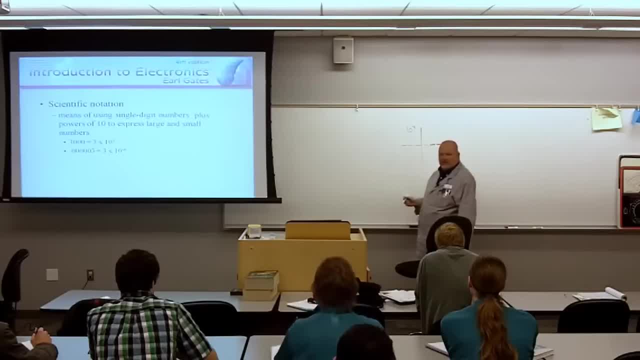 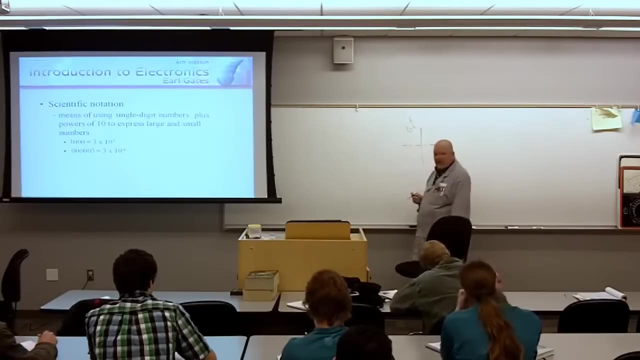 we're going to call this value here in the metric system. what? What's thousands in in metric Kilo? Very good Kilo. So what we're going to do is we're going to call this small letter k kilo. 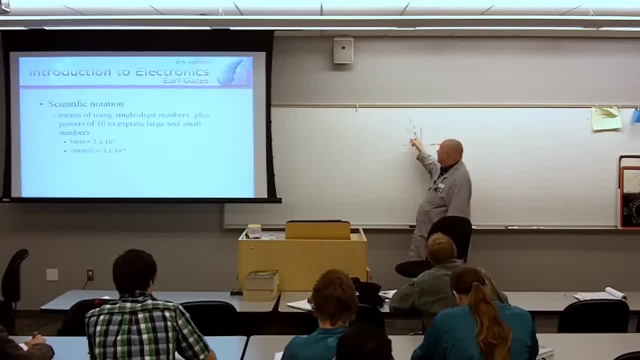 So instead of saying one thousand, I'll say one k, Instead of saying nine hundred and forty-three thousand, I'll say nine hundred and forty-three. kilo, Kilo pounds, kilo ounces, kilo miles, kilo volts, kilo ohms Make sense. 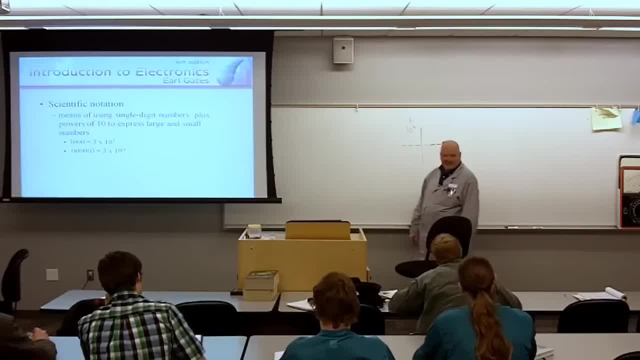 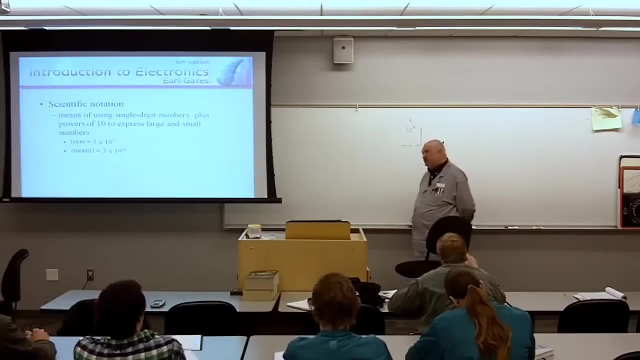 Kilo miles. There's a new one for you. So resistors expressed in k, meg kilo, or that's all. basically, it's scientific or it's engineering notation. Well, metrics, it's in metrics. but if you put, 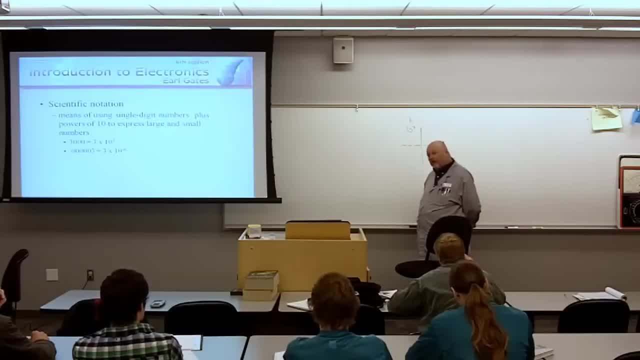 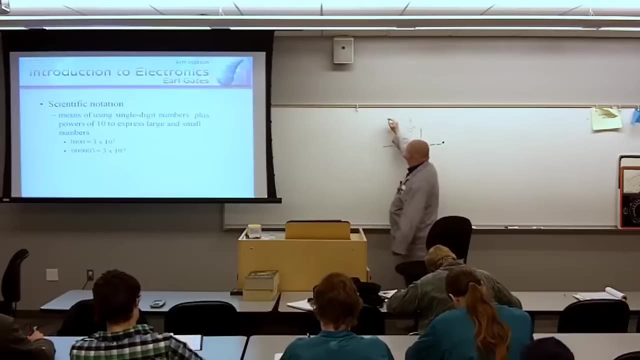 it into engineering groups of three, then it's going to fit directly into those prefixes, those metric prefixes. So three more places past the decimal point. One, two, three. This is times ten to the sixth. We're going to call this. 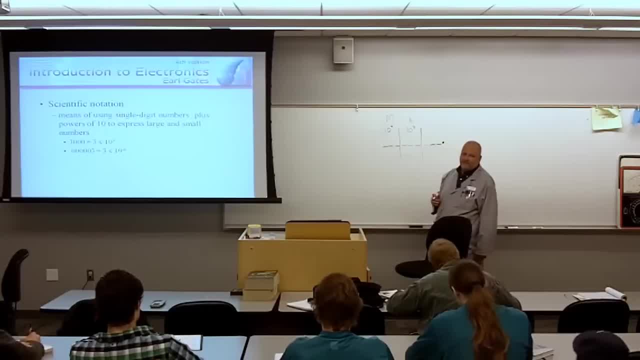 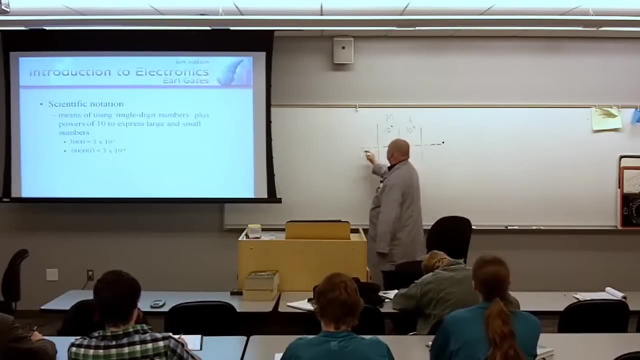 mega, Mega And in actuality it's like millions, right, One million, ten millions, hundred millions, Mega Ten to the ninth. What's that Giga? Very good Capital letter: G Giga. When I first got into this industry. 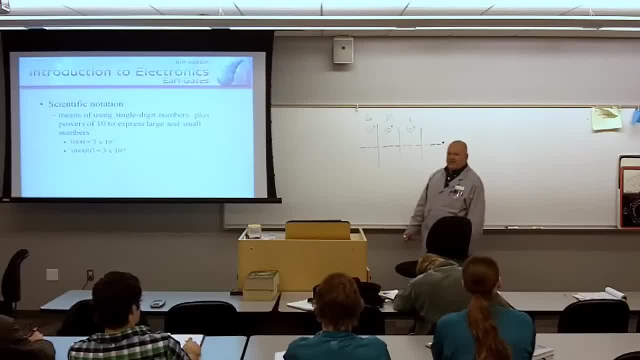 I'm dating myself. I don't know why I say that I make myself feel old. This is as far as we had gone in the electronics industry- General electronics, Giga Wow, And I'll be honest with you Where I used to. 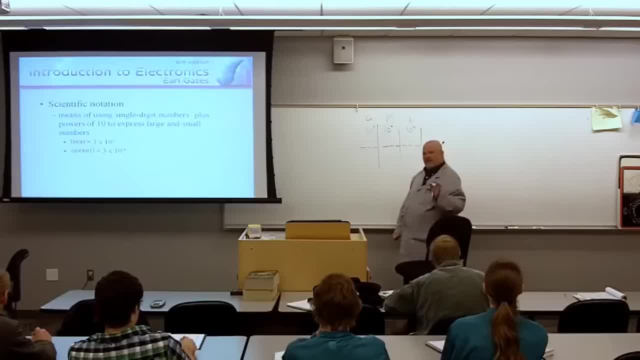 work in electronic intelligence. the only people that could afford to play up here in giga values were superpowers. It was either us or the Soviets, And we knew what we had. so if I detected something that was in gigahertz, it had to be the Soviets. 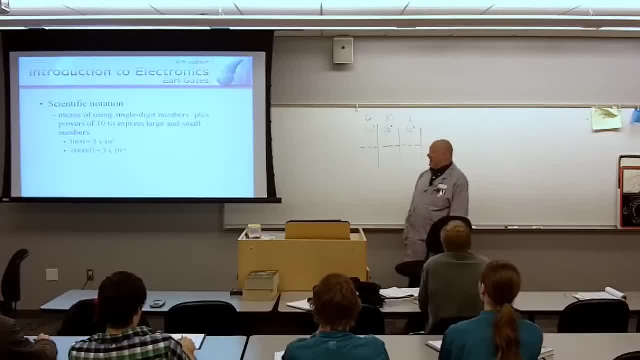 Okay Now giga Commonplace After school today you could probably stop at Fred Meyer, pick up a laptop computer that's got a you know eighty gigabyte drive in it for forty-nine dollars. That's actually too much money. Forty-nine bucks you could get. 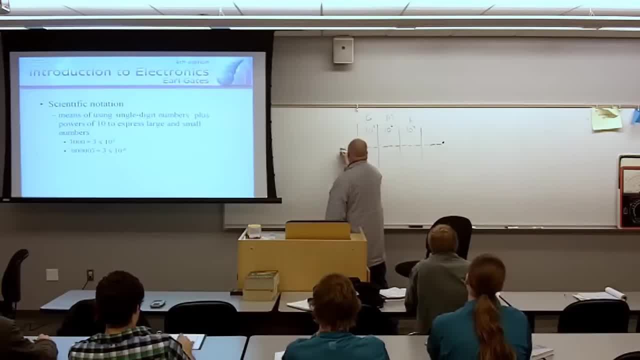 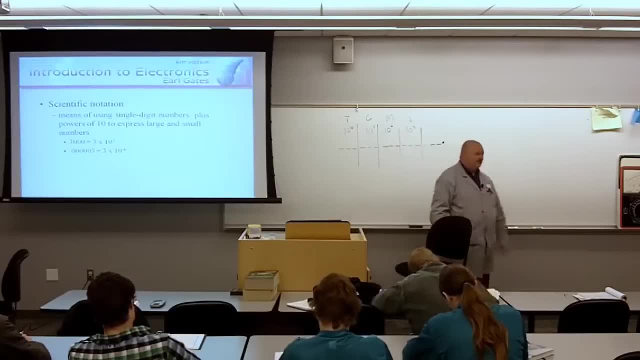 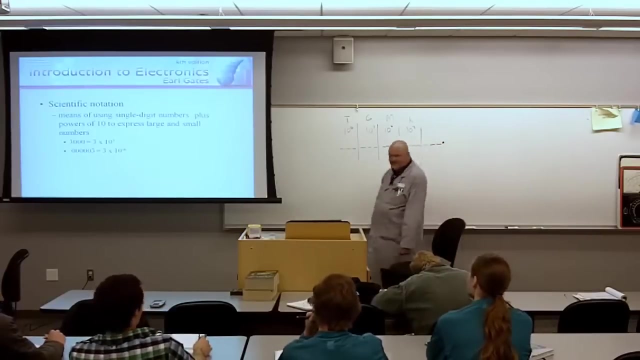 a times ten to the twelfth Terra. Terra also happens to be a barista down in Federal Way. that's kind of got it going on, if you know what I mean. I don't even know what I mean. I don't even know what that is, Terra. 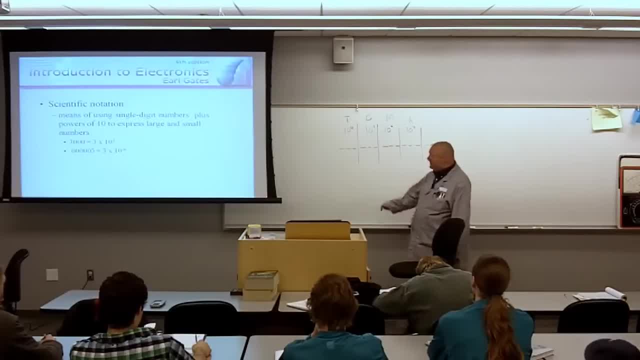 When I first started teaching here twenty years ago at Lake Washington Technical College, I can't even remember. I think I might have had like an eighty meg hard drive or something. I remember getting super jazzed by getting the Sunday Seattle Times and I saw an ad in the paper that I could get. 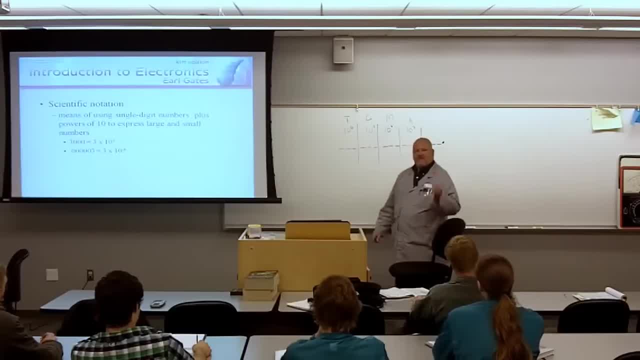 like a two hundred and fifty megabyte hard drive for less than a dollar per megabyte, And I'm like you gotta be kidding me- I could get less than a dollar per megabyte of storage. I'm gonna go out and get one of those, You know. so I went out and paid my 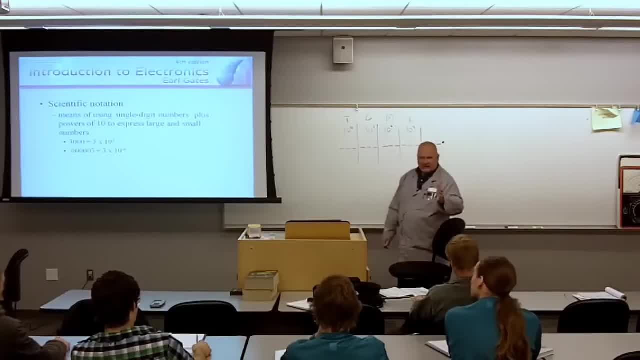 two hundred and fifty bucks or whatever. Now you're getting a terabyte hard drive for forty nine dollars. Now they have two terabyte hard drives they could get for ninety nine dollars. So this is. Have I made my point about the numbers we're gonna work with in high tech industry? 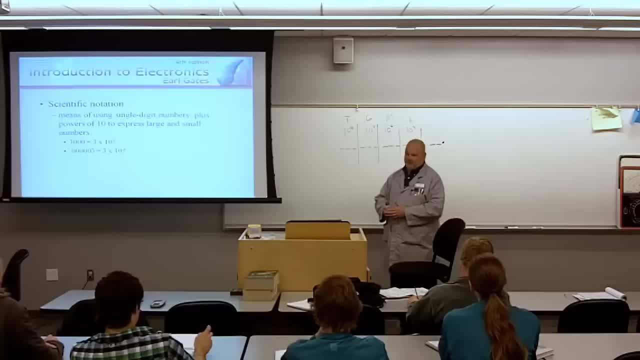 I mean, the numbers are extreme, They're extreme. So again, if you use engineering notation and put it into groups of three- and most of you on your calculators have a mode that you could put it into engineering notation, So ultimately the answer's gonna be given to you in either times: ten to the third. 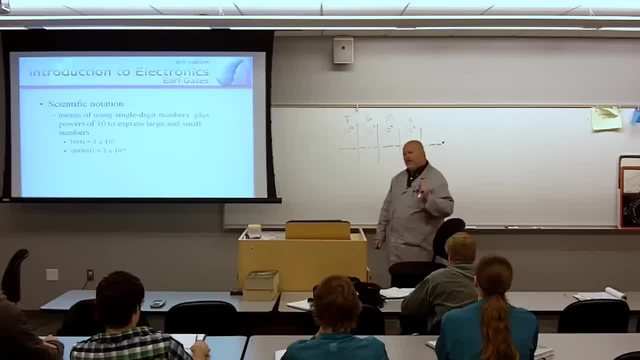 ten to the sixth, ten to the ninth, ten to the twelfth. If you don't know how to do that, you might wanna look at your owner's manual. If you already threw your owner's manual away, do a Google search on your. 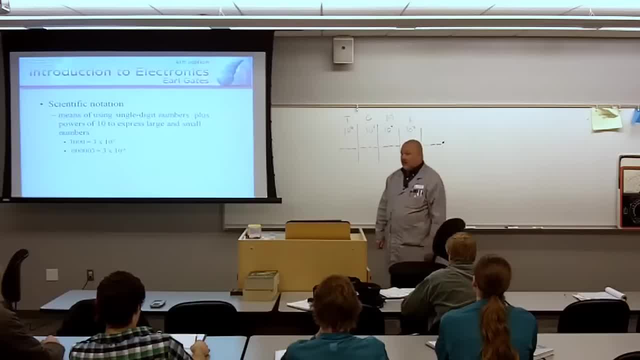 model and it'll come up with a PDF of it. You wanna make sure you know how to access those modes in your calculator, Because again, we're gonna be using some extreme numbers. But you know what I'm not done, I've yet to begin. We're about. 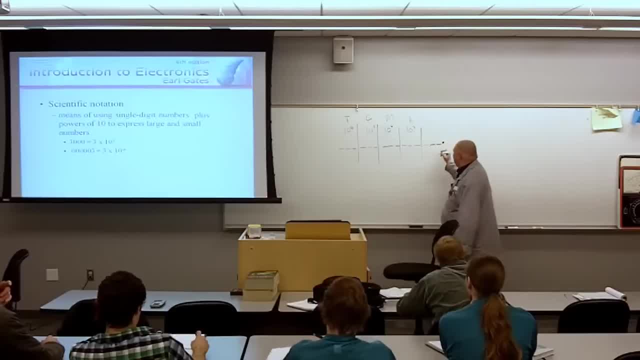 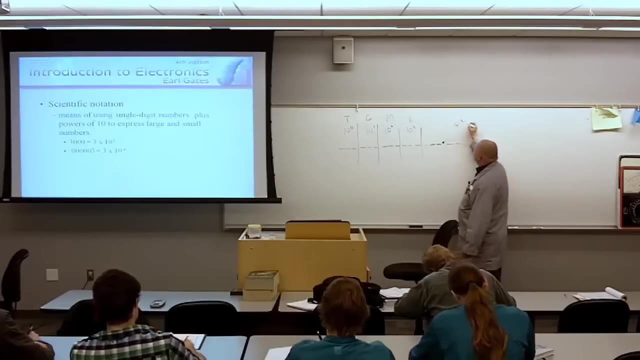 halfway done. We're also gonna be dealing with numbers that are smaller than one. So when I go back, one, two, three places- Anybody know what we call these Times- ten to the negative. third, Three places to the right of the decimal plates, Millie, And actually, if any of you come, 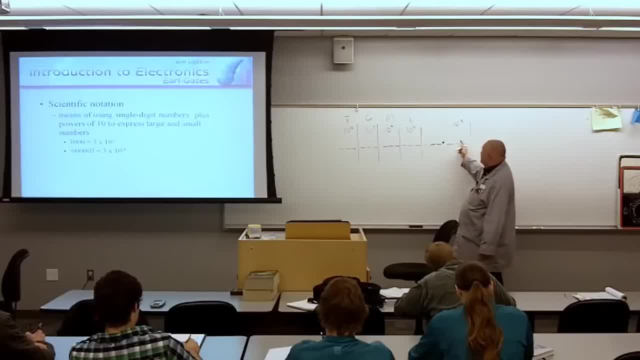 from a machining background or whatever, like thousandths of an inch. This would be a tenth of an inch. Right, This would be hundredths of an inch. This would be thousandths of an inch. And you use the term mill, Right. How thick is that? 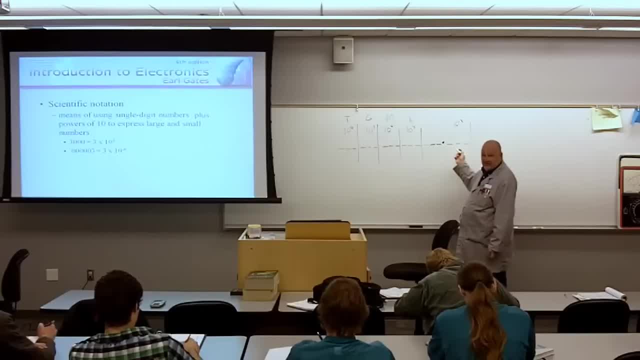 plastic. Three mil, Three millie. Okay, So we're gonna call this small letter M for millie, M-I-L-L-I: Millie, Millie. Three more places past the decimal point Gives me times ten to the negative sixth. Anybody know what we call this? 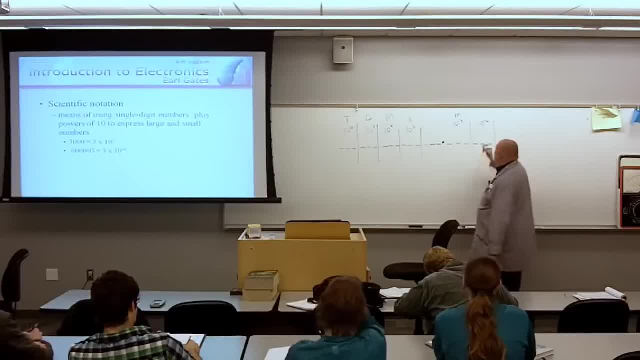 Micro. Very good Micro. Micro is kinda weird too. It's a Greek symbol. Kinda looks like this, Kinda like a backwards U. It's actually the Greek symbol called mu Mu. Dirty jobs. Really, He does that Micro. 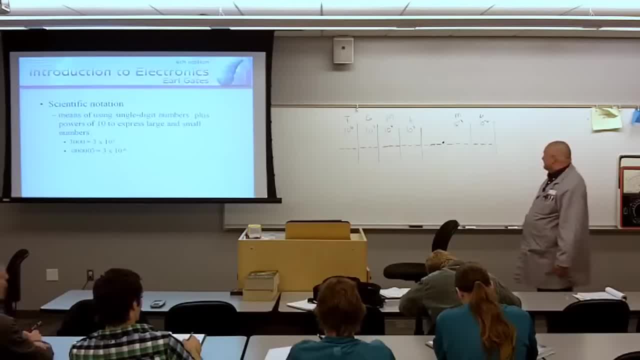 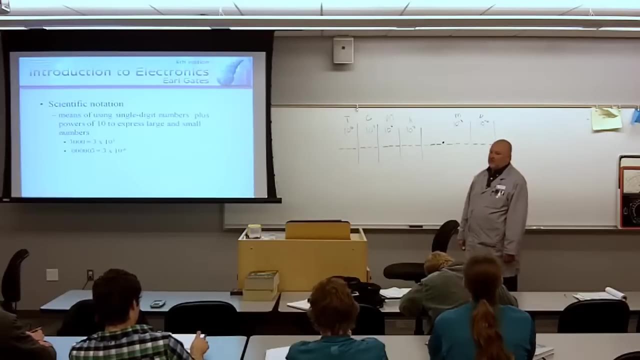 Micro, Micro For our friends at home. Yeah, Micro, He actually participated in a fundraiser here in the fall of Lake Washington Technical College Via satellite. Actually, the producer from that show, Dirty Jobs, was here and they did a fundraiser for our college foundation. But Micro was live. 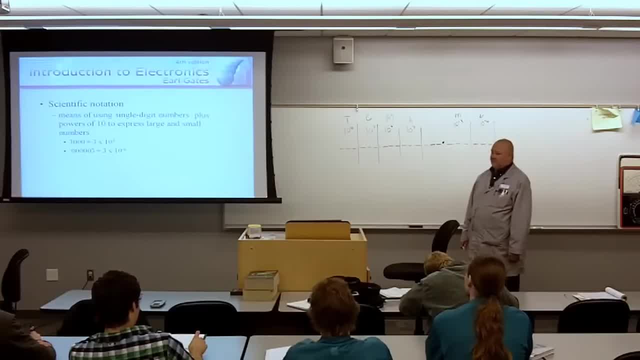 via satellite, Speaking directly with all those that went to breakfast Washington Technical College. I slept in that morning. I was hoping they were gonna TiVo the event so I could watch it at my leisure, but nobody TiVo'd it. Three more places past the decimal point Times ten to the 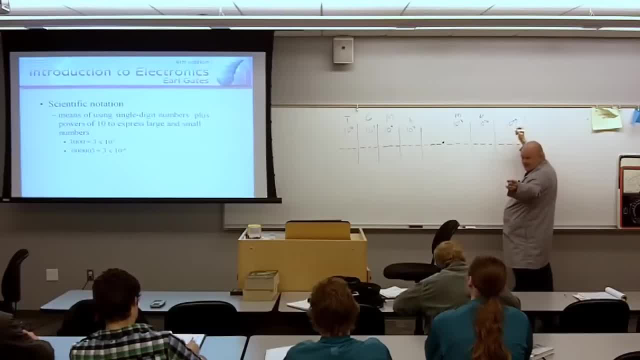 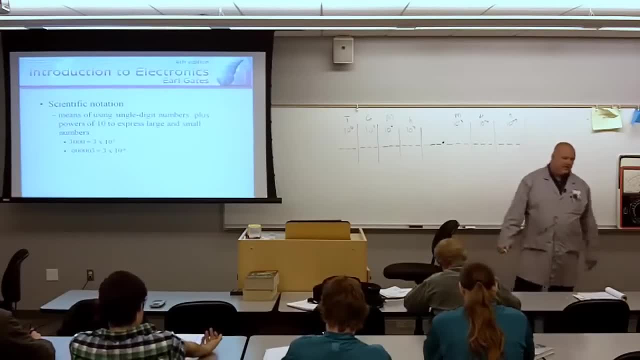 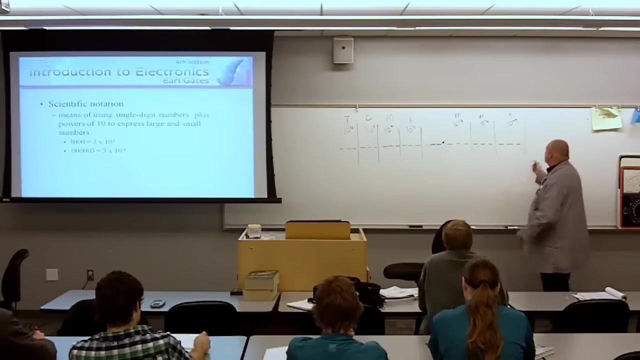 negative. ninth: Nano, Yup Nano. Very good. Small letter N. Small letter N- Nano. Any of you have heard about nanotechnology. This is kinda like where nanotechnology is playing around with now Three more places past the decimal point Times. ten to the negative. 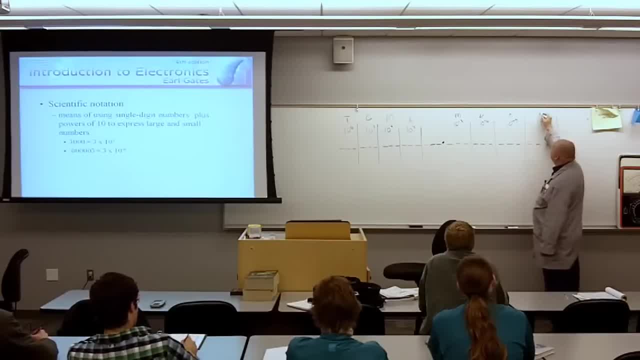 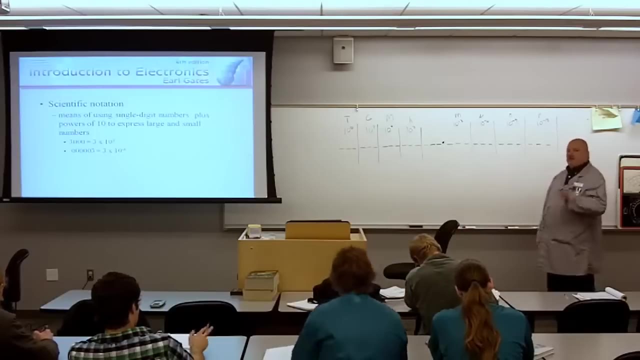 twelfth Pico: Pico. Small letter P Pico. Suffice to say, I could go further. There's a couple places past this, but it's beyond the scope of what we're talking about right now. But as students at Lake Washington Technical College, 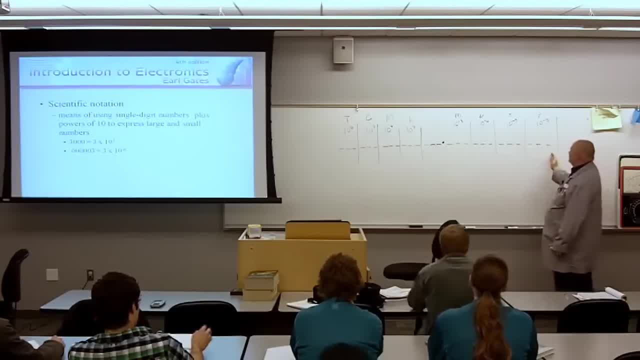 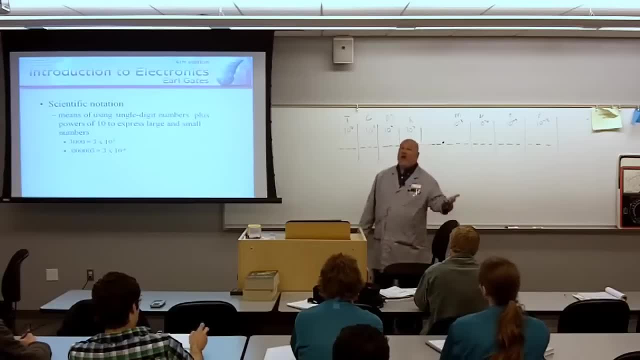 you, on a regular basis, are gonna be dealing with numbers, times ten to the negative twelfth to times ten to the positive twelfth, Sometimes in the same problem. So, like I said earlier, even if you're Bill Gates accountant, even if you're the IRS, 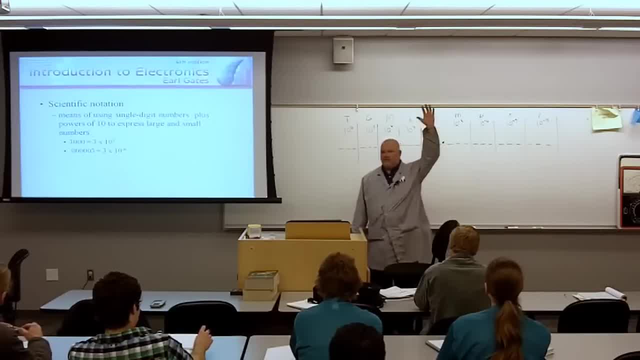 itself. anybody here not filed their taxes yet. Two of us, Three, Be honest, Four. It's actually funny. I was with some friends on Saturday. We stopped at Starbucks for a cup of coffee and my friend saw this woman that she thought she recognized. 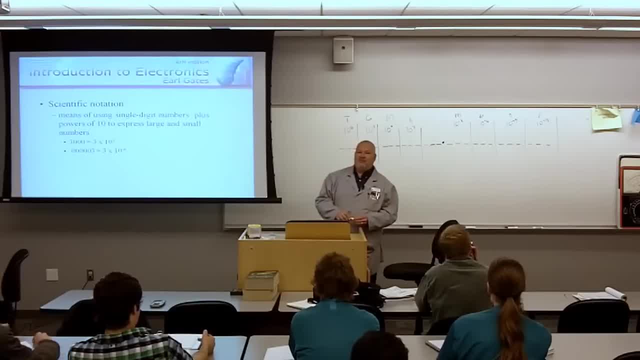 that she knew, And you can't make this stuff up. It's like she's like you look like a good friend of mine. blah, blah, blah. Do you work for Quest? No, I don't work for Quest. Well, you know, I work for the IRS. 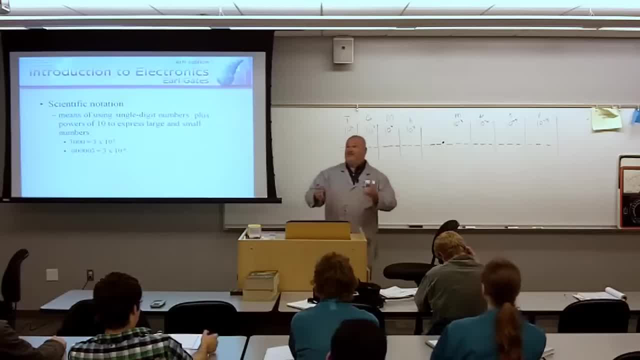 Really Excuse me, ma'am, but you look lovely today. Can I buy you a pastry to go with a cup of coffee? You don't want to tick those people off. You finally brought down Al Capone, wasn't it Right? The IRS. 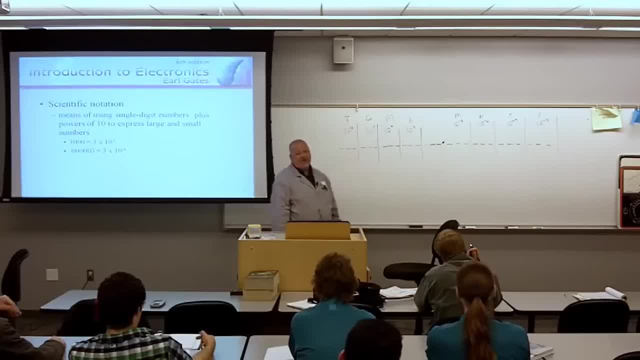 Anyway, we're gonna be dealing with numbers like this, so we have to make sure we get it right. So in most of your calculators you'll have a key ee, a key ee, and you could enter that. Whatever you do, do not enter it as it appears. 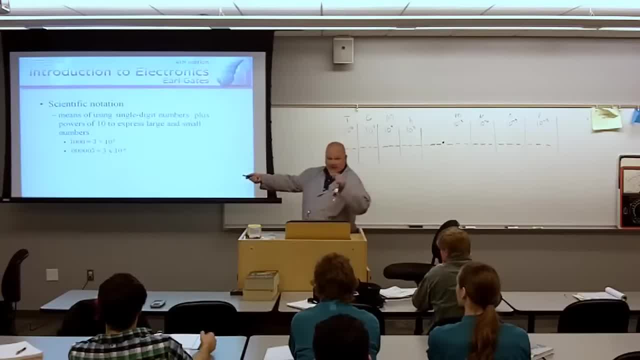 here on the don't go three hit the times. key ten to the third power. You're actually gonna end up a decimal place off with that. You have to enter it. the ee key exponential notation. Any questions on that? Alright? 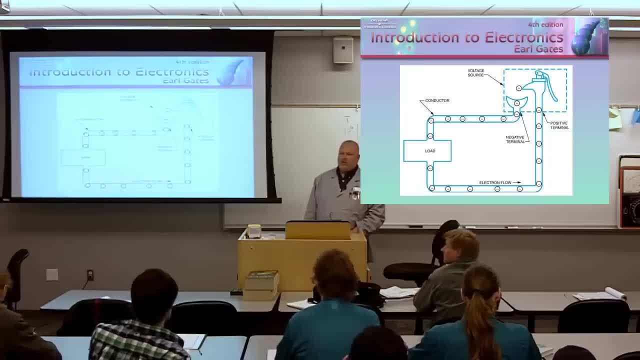 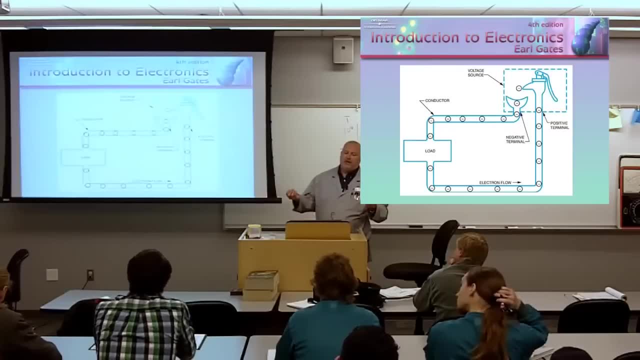 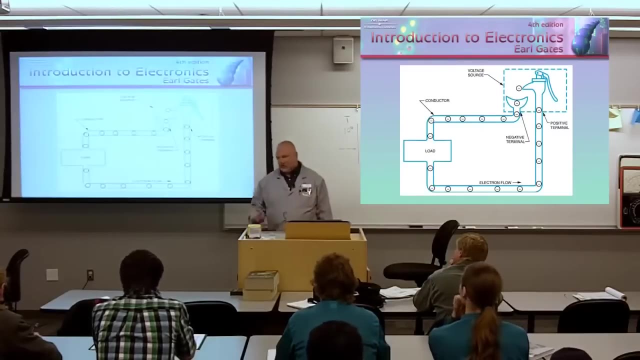 There's no harm in using your imagination when you're dealing with an electrical system, in equating it to a fluid system, Because, let's be brutally honest, you can't see electricity coursing through wires. You can't see it. Our five senses are very, very limited, So sometimes 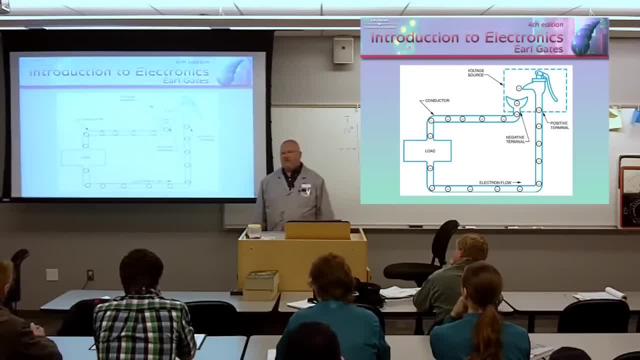 analogies really, really help us out. So for those of you that understand fluid systems, you know it all rolls downhill and pressure and pumps and that kind of stuff. you could use the same analogies to figure out what's taking place inside an electrical circuit. One of the things that I do because I just love 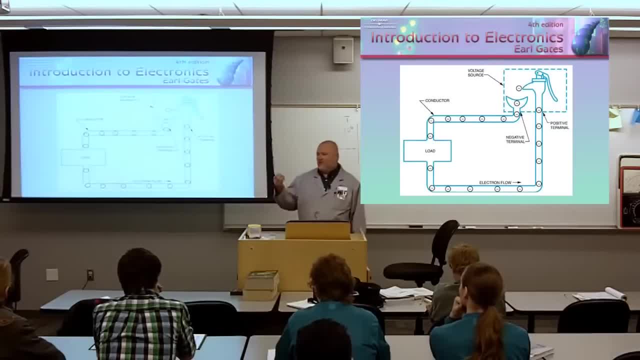 Seattle is. I'll use the Seattle freeway system to sometimes explain the behavior of current in a circuit I-5,, 405,, 520, and we'll use those as analogies of how current behaves, How traffic behaves on a Friday before a 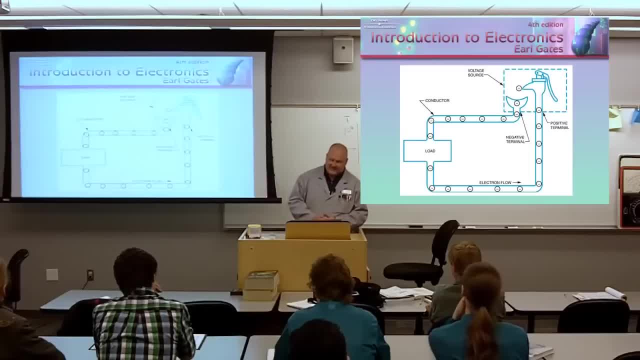 three-day holiday weekend And it's sunny out And raining In the convergence zone And we'll use those analogies to kind of figure out what's taking place in a circuit. So this here, this analogy, shows us the pump. This would act like our voltage source. 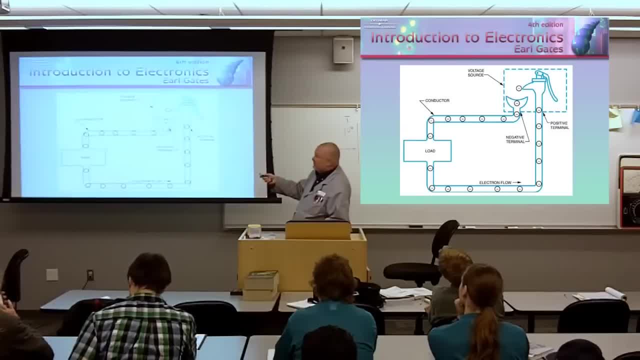 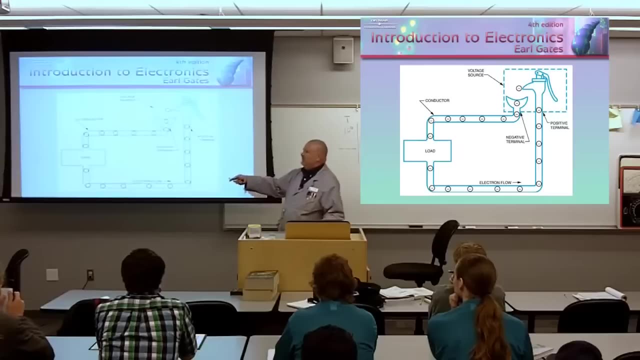 right, It's sucking and then discharging, right. So this is our source of electrons and this is where it's drawing the electrons through. So the pump, The current flows through the plumbing, The electrons flow through the circuit. The only thing that I would have done differently if I drew this illustration. I can't. 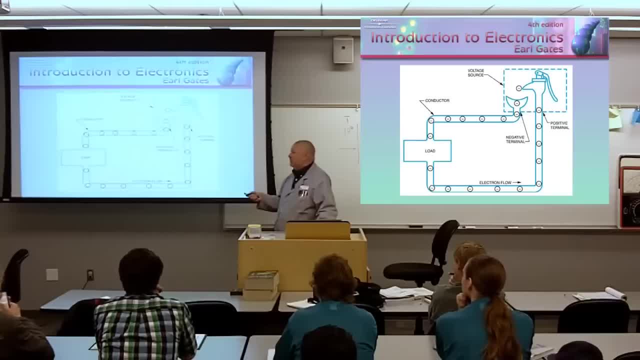 take credit for this. I simply pulled it out of the text. is the load. This would have been nice if they had, like, a water wheel right here, So as the water runs by, it turns the wheel, Because that's what a load does. A load. 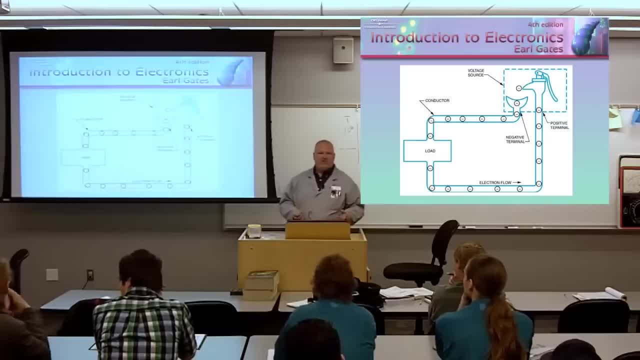 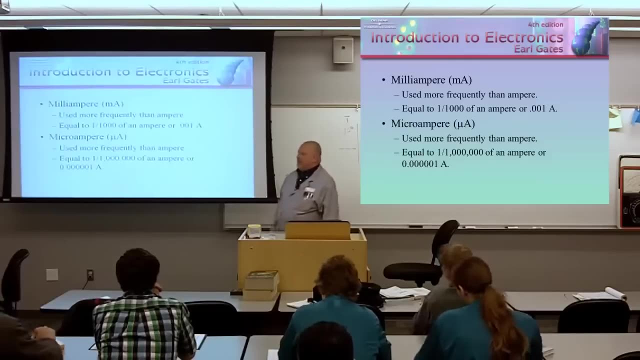 converts one form of energy to another form of energy. An electrical load converts electric energy into light energy or electric energy into motion or some other form. Does that make sense? So you can use this if you care to, Since this chapter's talking about current, typically in the study of electronics. 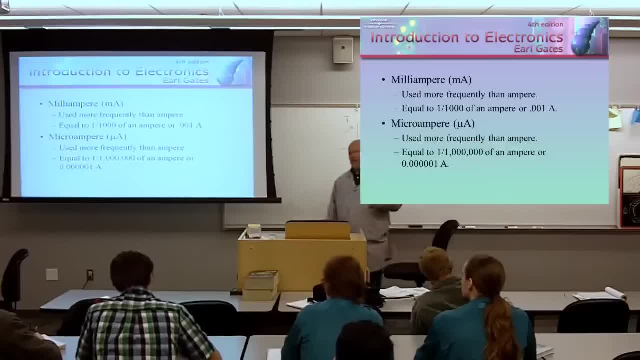 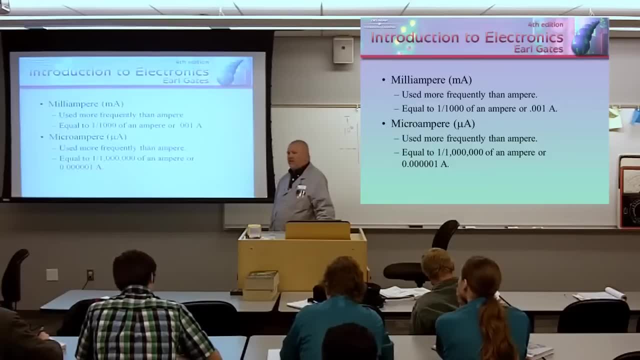 electronics- Not electrical, but electronics. We're typically only going to be using values associated with milli times 10 to the negative third, milliamps- Which, don't be fooled, milliamps could kill you. There's enough, even though it's thousandths of an amp. 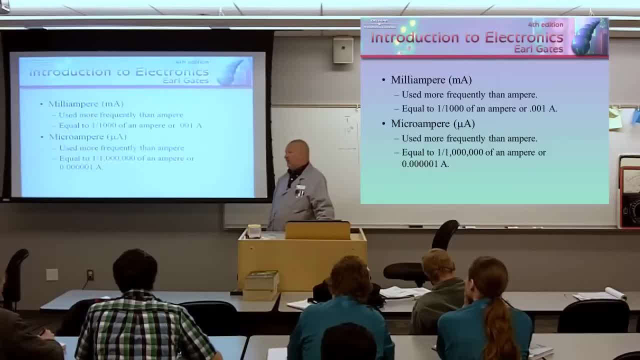 it's still enough to kill you, More than enough to kill you. And also we're going to be dealing with micro amps, Typically as a student here in the electronics program Lake Washington Technical College. For those of you that go into the electrical trades at all, 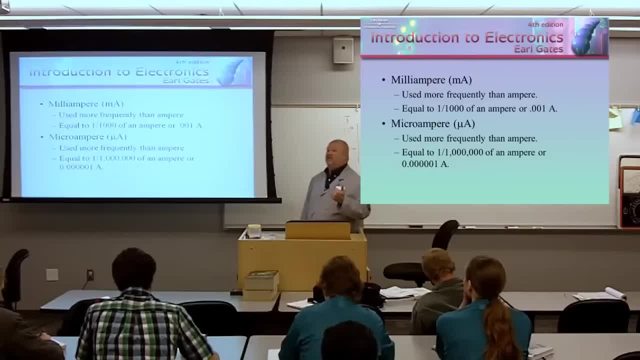 you're going to be dealing with amps And lots of them. We had a student that just got hired by Bonneville Power Administration BPA. He's going to be working substations. I don't even know how many amps you're dealing with at a substation. What makes a substation a substation? 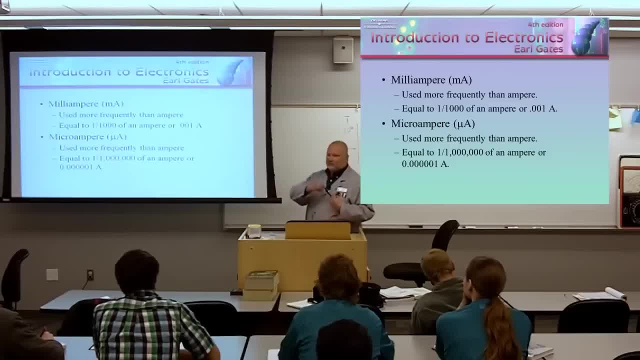 Lots of amps. I would imagine I never had an interest to working with that many amps. Since milliamps could kill you, why would I want to work with more than enough to kill me? In summary, we talked about the laws of electrostatic. 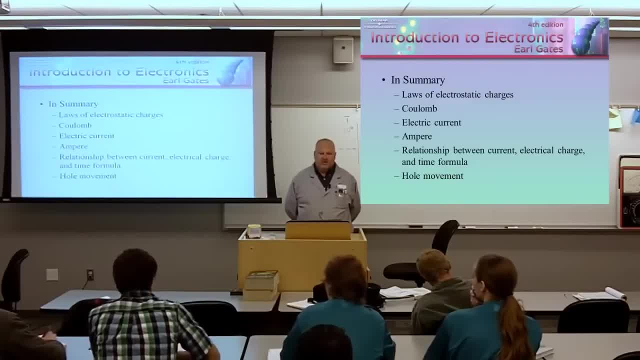 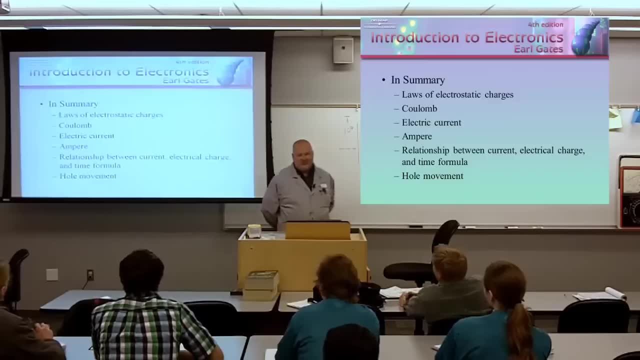 charges. The first law is that like charges oppose each other. The second law is: unlike charges attract each other. A coulomb is 6.24 times 10 to the 18th electrons. Electric current is the flow, not the drift. the flow of electrons. 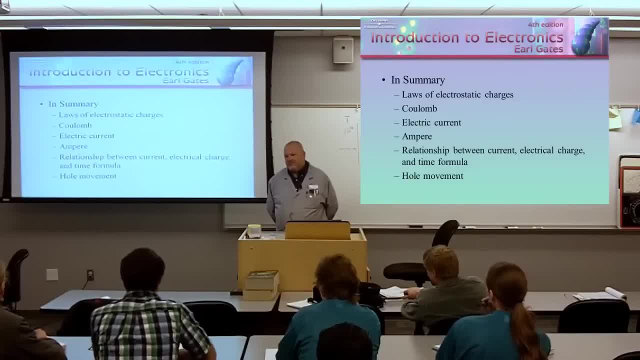 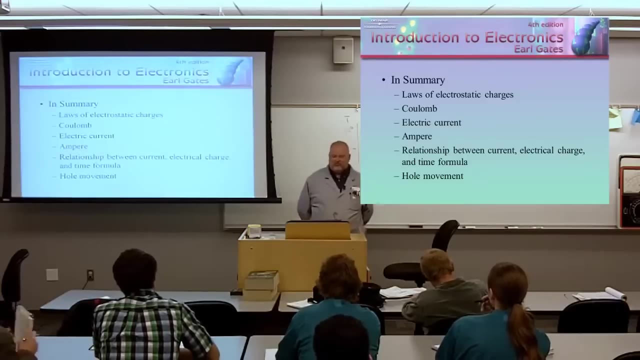 in a specified direction, Measured in amps conceived by the dude by the name of Andre Marie Ampere. and Andre Marie Ampere stated that one amp is equal to one coulomb per second. That's the relationship between current electrical charge and time formula. 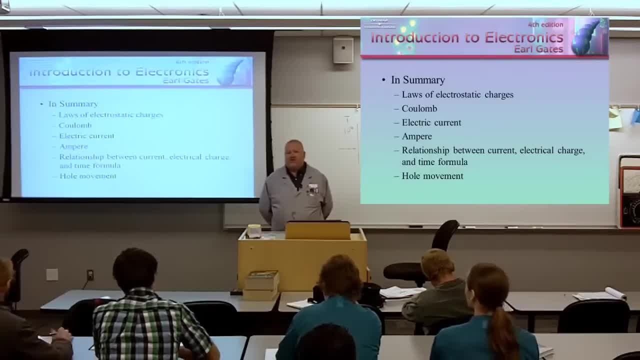 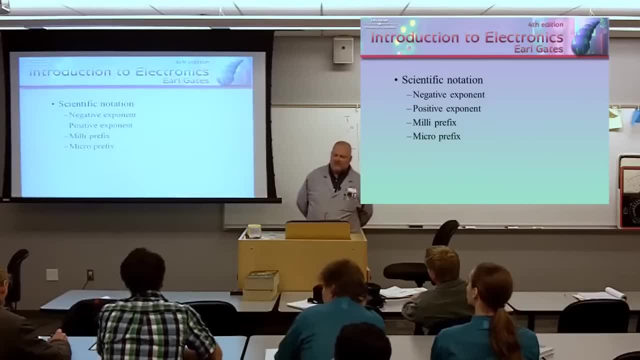 We talked about holes moving. Holes move in the opposite direction of electrons. Electrons travel negative to positive. holes travel positive to negative. We talked about scientific notation, Negative exponents, specifically milli, micro nano and pico. 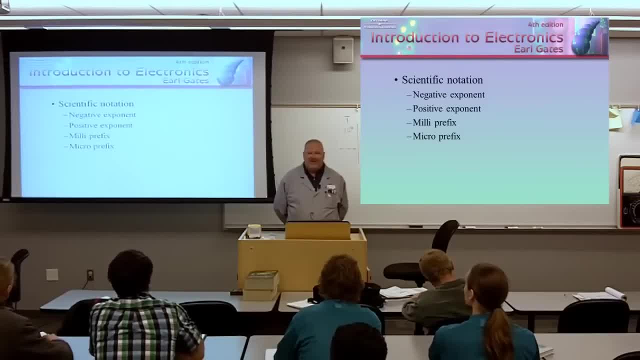 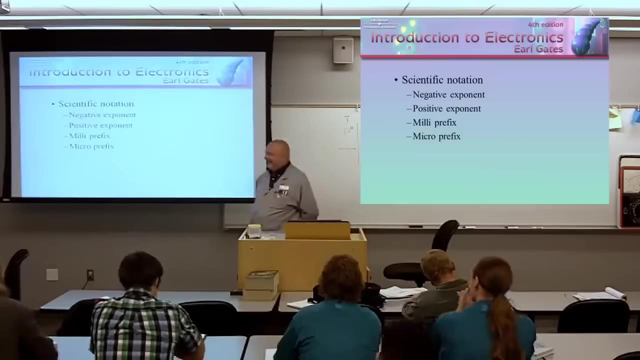 And we talked about positive exponents, specifically kilo, mega, giga and tera, And tera also happens to be a. That's kind of got it Outstanding, If you know what I mean. I don't even know what I mean We're going to talk about. 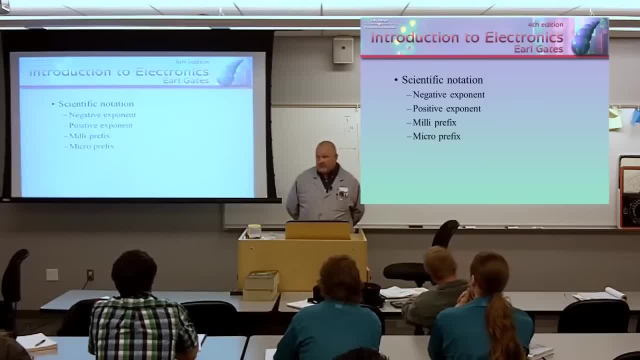 milli prefix. Typically these are the values of current that we'll see in an electronic circuit And also micro times: 10 to the negative 6. These are also values of current we'll typically see inside an electronic circuit. Make sense? Anybody have any questions? 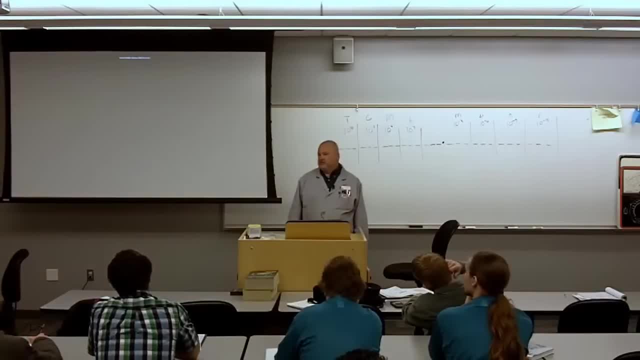 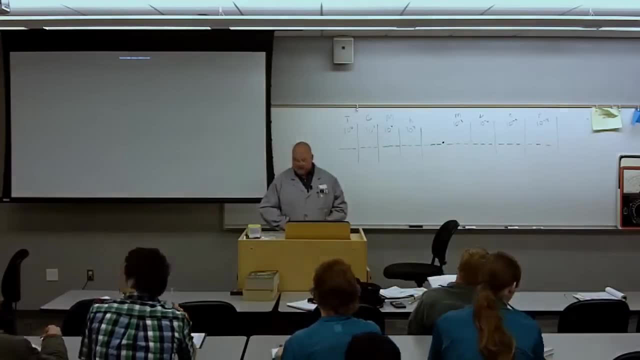 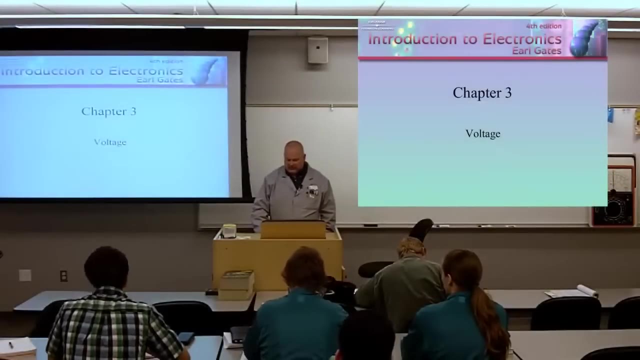 on anything that we covered in chapter 2?? Chapter 2.. Alright, let's go ahead and take about a 15 minute break, and at 6.45 we'll go ahead and kick things off again. Okay, chapter 3, voltage. Chapter 3, voltage. 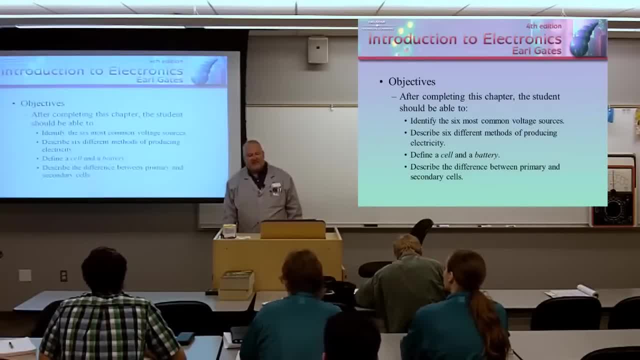 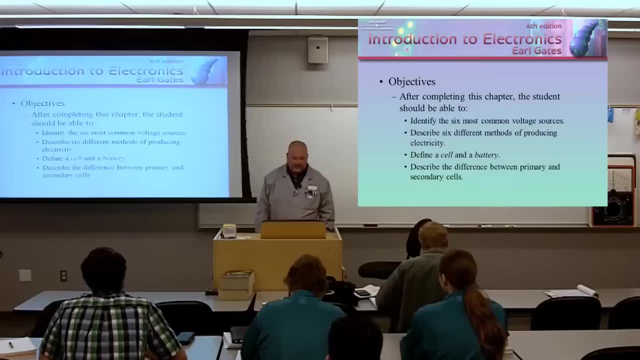 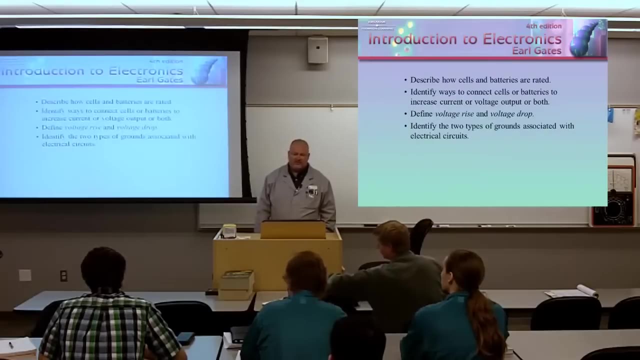 After completing this chapter, you're going to be able to identify the six most common voltage sources. Describe six different methods of producing electricity. Define cell and a battery. Describe the difference between primary and secondary cells. Describe how cells and batteries are rated. Identify ways to connect cells or batteries. 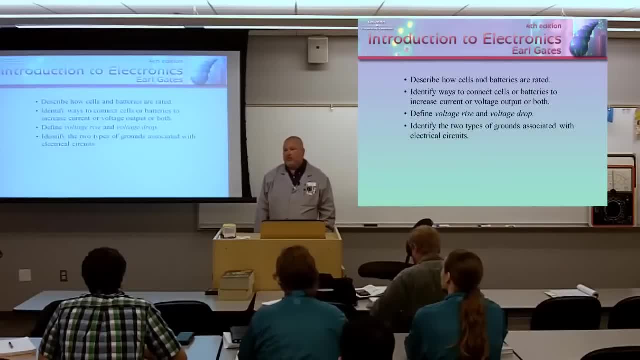 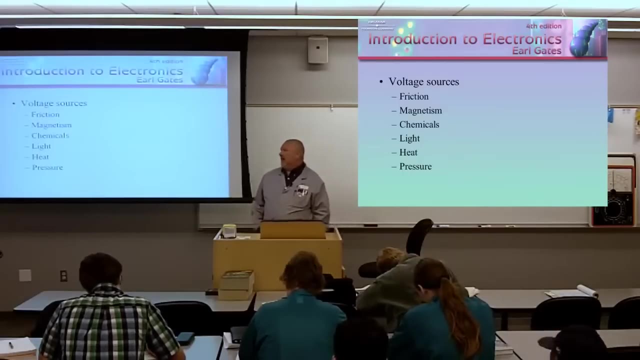 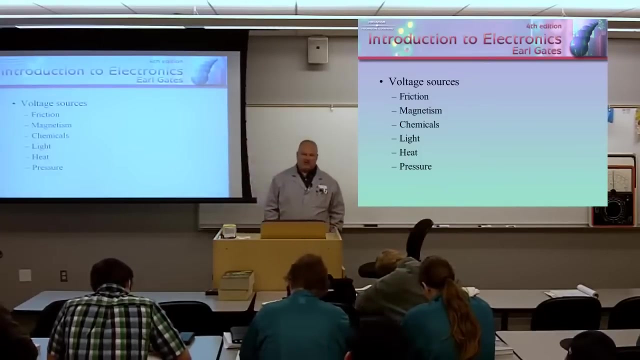 to increase current or voltage output, or both, Define voltage rise and voltage drop And identify the two types of grounds associated with electrical circuits. This kind of makes me laugh. You know, the big buzz word now is alternative energy. Right, Alternative energy And. 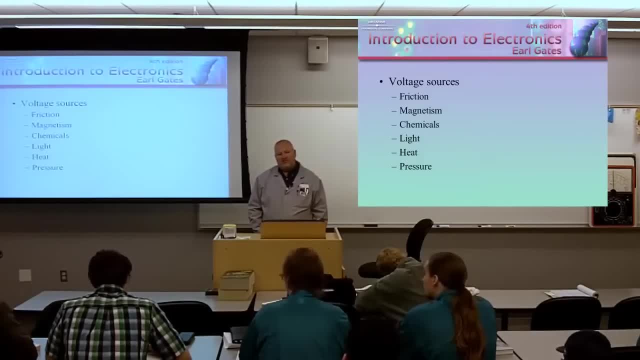 really worldwide. we consume electricity. That's the form that we've pretty much chosen: Electronics electricity. You know, I don't think there's any places that are installing oil lamps. You know, new hotel in the Caribbean. We light our place with oil lamps. 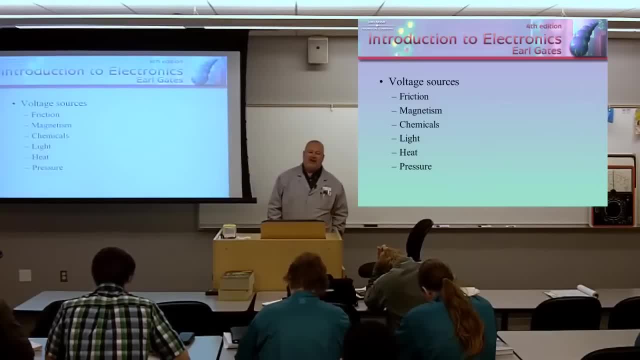 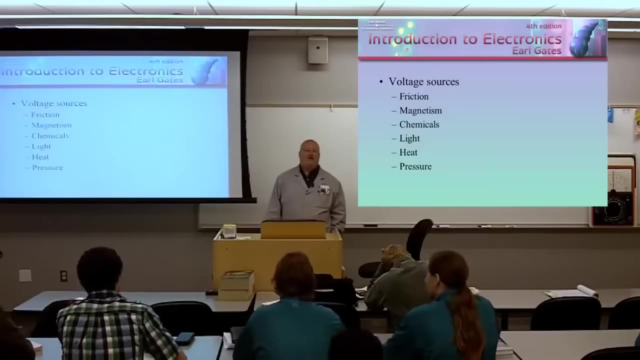 No, we use electricity And there are six methods of producing electricity period. So when I hear about alternative energy, I kind of sit up. I'm like wow, have they come up with a seventh method? No, As long as I have been in this industry, there have been six methods. 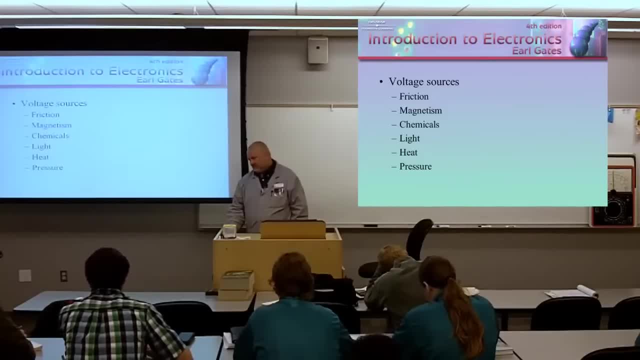 There are only six methods. If you come up with a seventh now, maybe you're onto something. Those six methods are friction, magnetism, chemicals, light heat and pressure period. The first one we're going to talk about is friction, Probably the most. 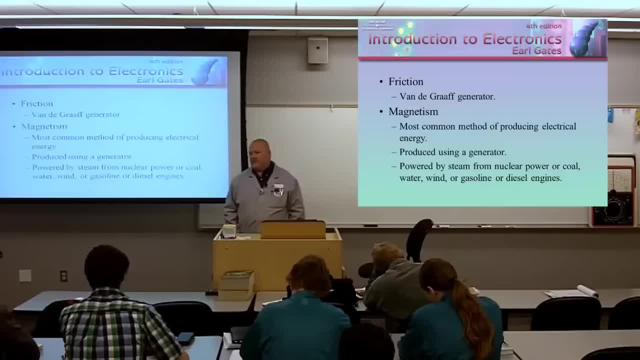 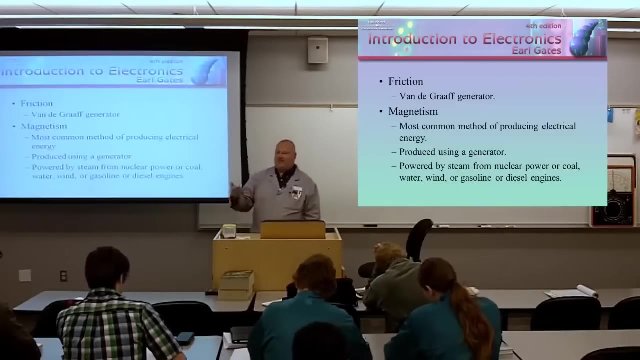 familiar is the Van de Graaff generator. How many of you are here familiar with the Van de Graaff generator? Let me try that again. How many of you here are familiar with lightning storms? That's probably the best example of friction producing electricity. 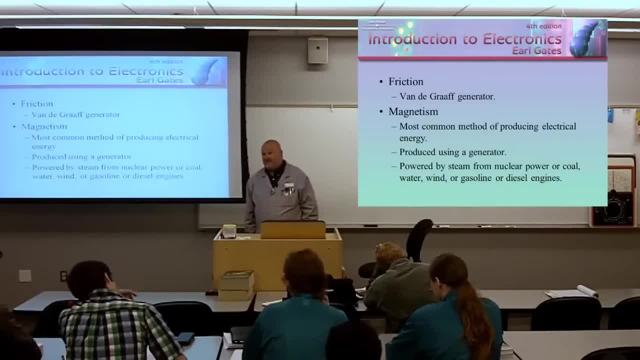 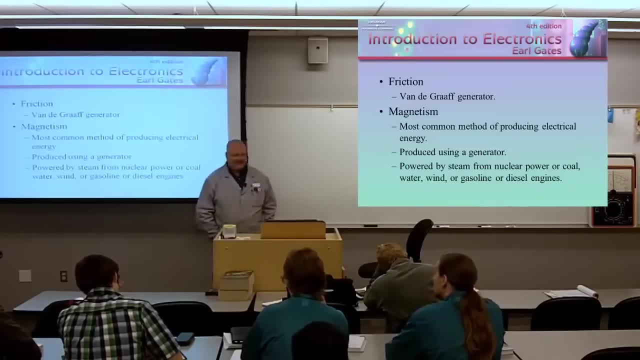 Friction producing electricity. A guy by the name of Ben Franklin figured that out by flying a kite in an electrical storm- One of our brilliant forefathers. It's amazing he didn't get electrocuted in the process. So lightning is a form. 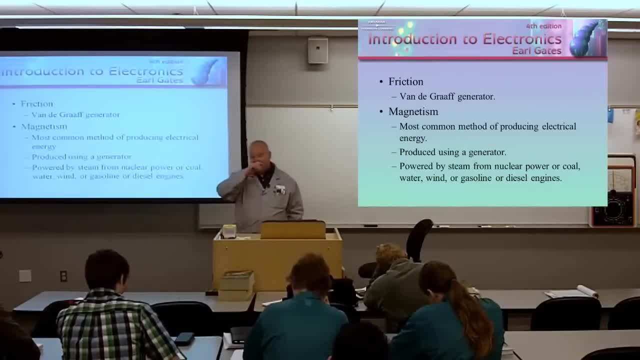 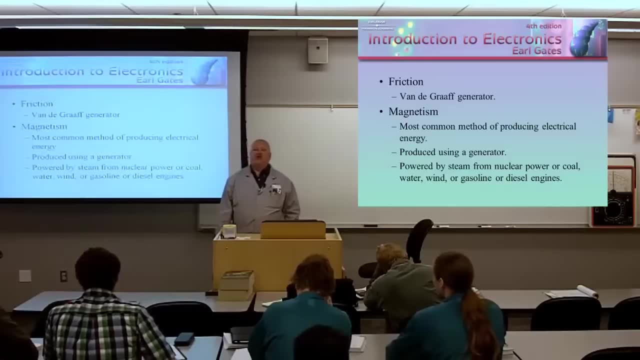 of friction caused by atmospheric friction, if you will- And that produces lightning. Another example is electrostatic discharge. when you walk across a carpet or you move, if you're wearing clothes- Just that movement, You could generate static electricity Tens of thousands of volts. 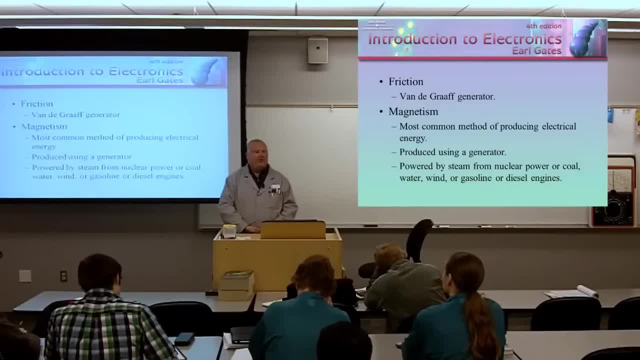 could be generated by you simply wearing clothes. The alternative is not wearing clothes. You wouldn't generate static electricity by doing so, but of course the world would be a different place. The Van de Graaff generator Some of you have maybe seen in a museum before. I've got one in the back room. It's out of commission right now. 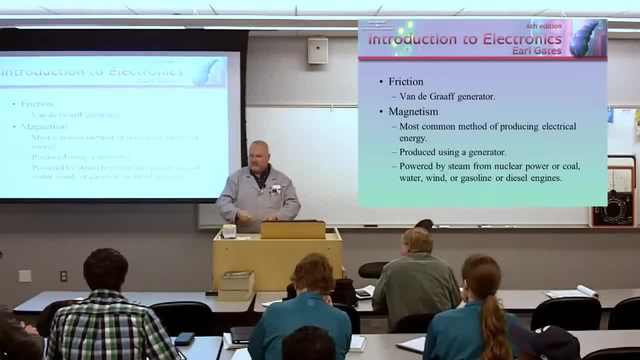 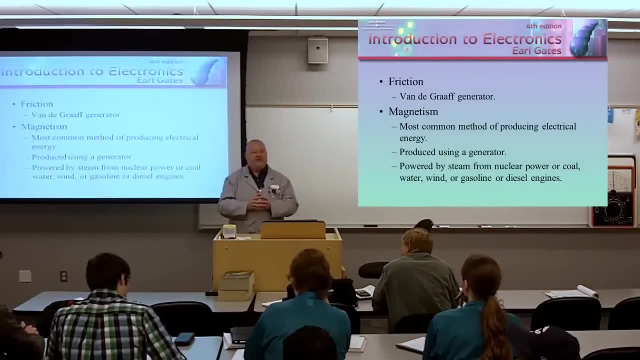 But there's a big sphere on the top of it, And then what it is is a belt: Pulls electrons off the bottom, Brings it up to the top, so the sphere becomes charged. And what we could do with that is if you were insulating. 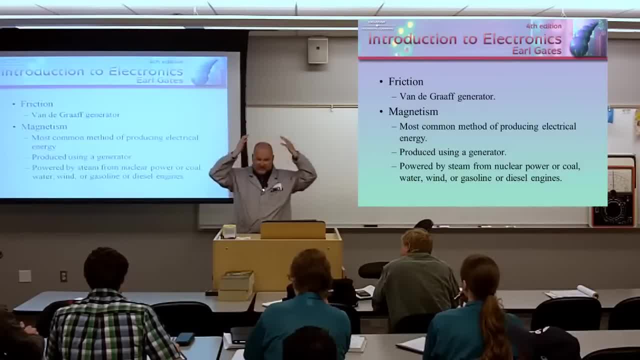 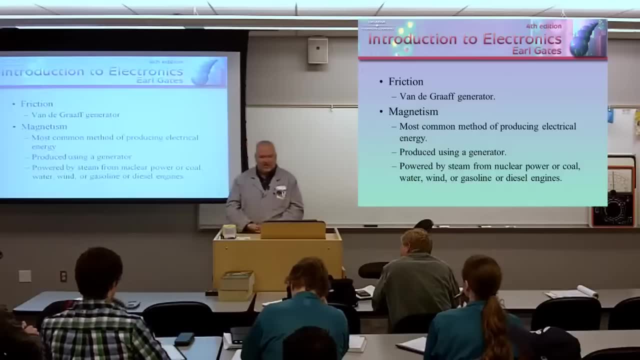 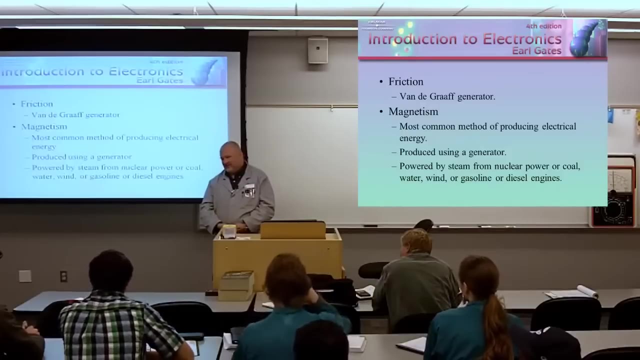 you put yourself at that electrical potential. You've maybe seen the pictures where people's hair is standing straight out on end. That effect could be created with a Van de Graaff generator- Friction- Not really the best method of producing electricity, Not going to hire tens of thousands of people. 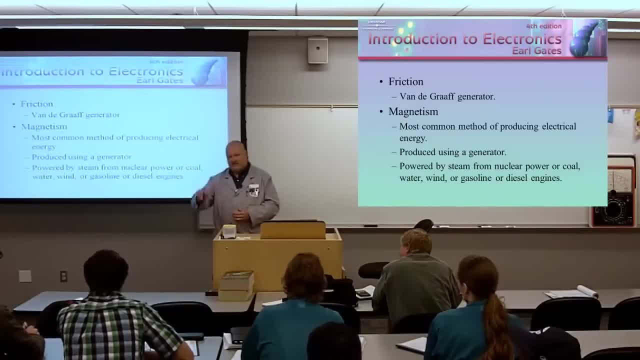 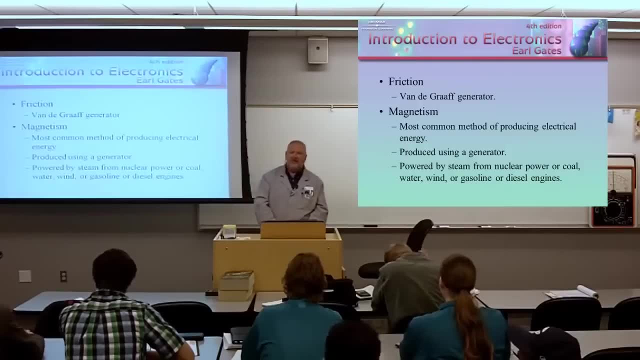 to walk around on carpets and then touch a conductor and power cities that way. It just doesn't make sense. On the other hand, if there was a method of somehow harnessing lightning, Now that would be something. That would be something. I don't know How many of you. are from the Seattle area, northwest, originally- your whole life. I don't know if you've ever had the opportunity to travel to the east coast, the midwest: Monster storms, Tropics, Monster storms, Storms that even jet airliners can't get above. 60,000 foot thunderstorms- Just amazing. I remember a few years ago I was flying commercially down to the Caribbean and on the way back, this monster storm outside and even the pilot was talking about it, and he's like. you know, in my 30 years of flying I have never seen a storm this. 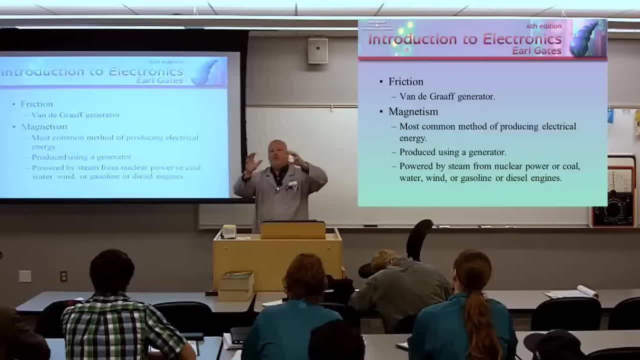 big And you just looked out and the whole thing was just glowing, Constantly glowing. It wasn't like lightning flash, Lightning flash was just constantly sitting there, just like throbbing glowing. Pretty frightening. So if you could somehow harness that lightning, 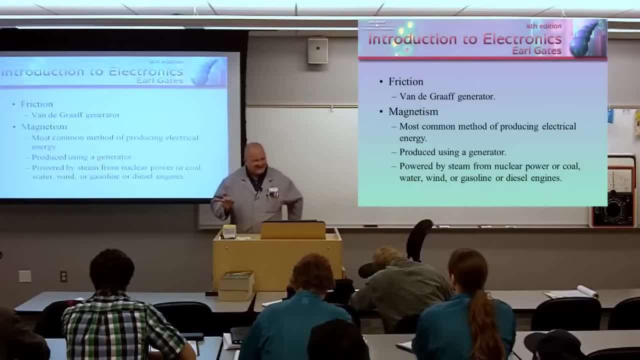 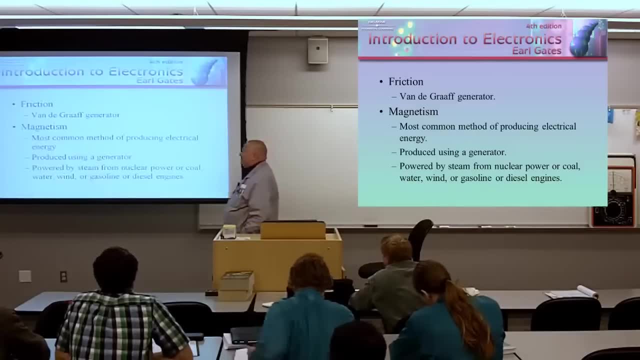 that would almost constitute a form of alternative energy. Magnetism is the most common method of producing electrical energy. This is how we produce electricity: using something called a generator. That generator could be powered by steam. That steam could be generated from nuclear power, coal, water, wind gas, diesel. 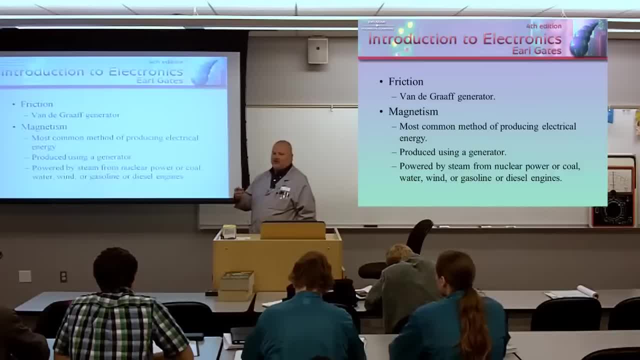 It doesn't matter how you rotate the shaft. The goal is you gotta rotate the shaft. It's actually very devastating the news from Japan. I was watching the news this morning and I guess they upgraded it to a level 7 accident now, which is on. 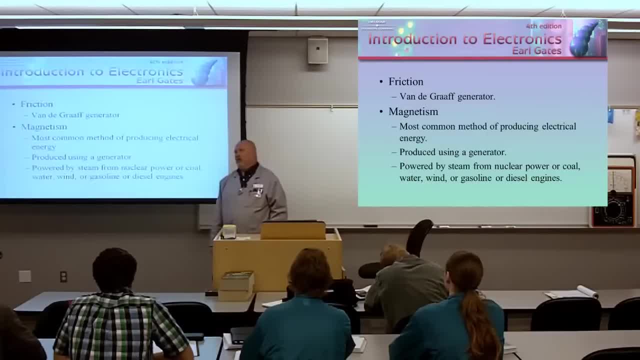 par with Chernobyl. Actually, the amount of radioactivity that that puts out could exceed Chernobyl if they don't get it figured out. It's really too bad. I'm not necessarily- I don't know if you want to call me- a proponent of nuclear- I mean I worked on nuclear submarines. 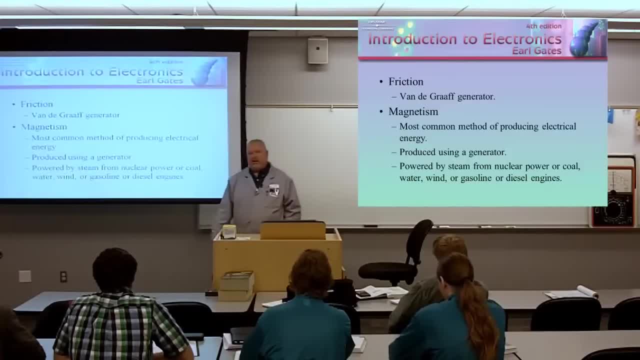 for you know 8 and a half years of my life And it's pretty cool. I mean, it's hot because it generates steam, but you know what I'm saying, It's pretty innovative technology. You know how often we- you know I commute. 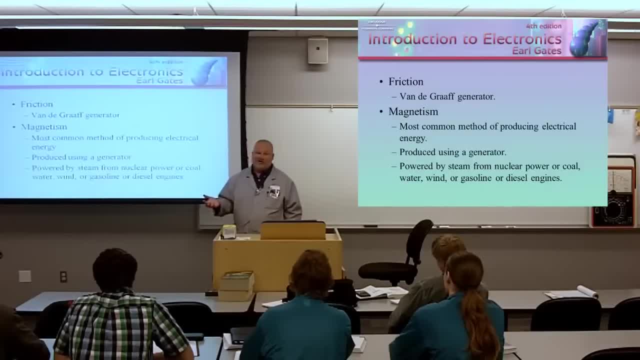 and I gotta go to the gas pumps about twice a week with my car And my car burns premium High compression engine. I gotta burn premium in it. You're talking about 50 bucks a pop Just to fill up my car for me to commute. You know how many times I saw my nuclear submarine. 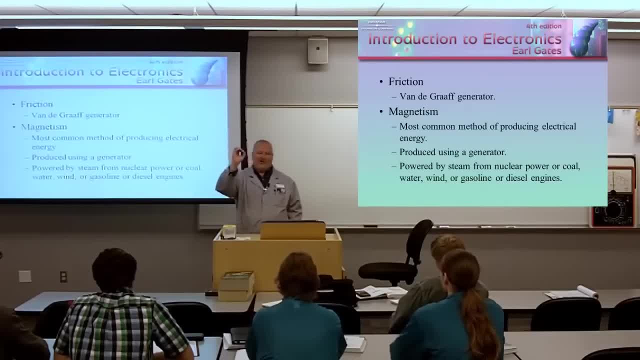 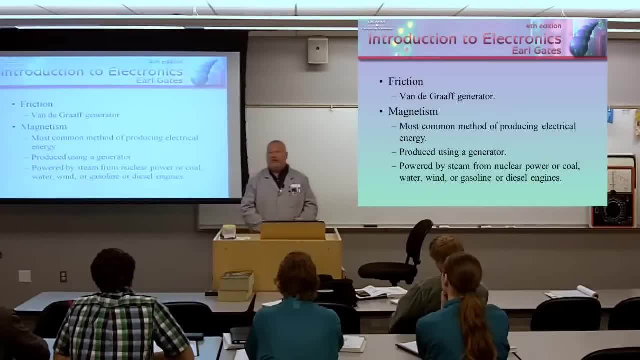 So it was actually getting quite a bit of momentum in the green movement. A lot of the folks in the green movement were like no nukes, no nukes, and they realized that it's pretty clean energy. Yeah, you gotta worry about the nuclear waste afterwards, but it's really a devastating 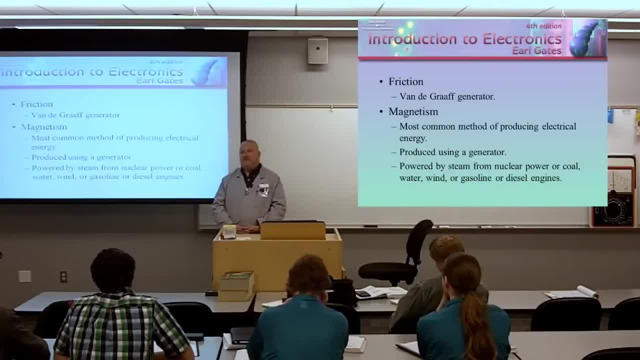 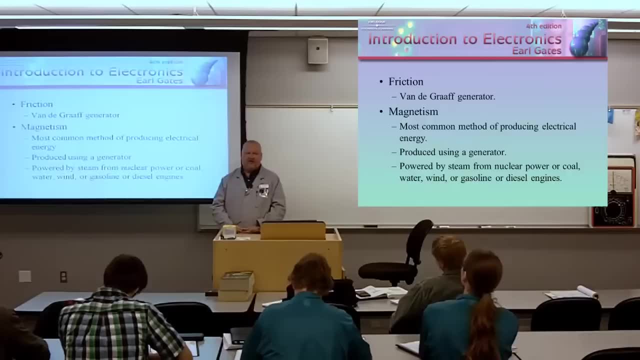 you know, not only for the folks in Japan but also really for, you know, energy efficiency and non-dependency on fossil fuel burning, So hopefully they can get a handle on it. I mean nuclear power. all forms of energy are inherently dangerous, you know, I mean my. 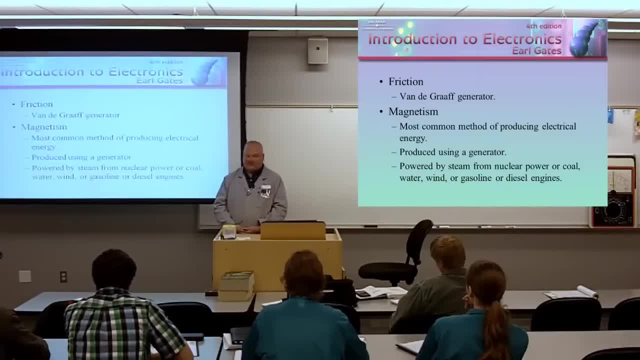 fuel tank splits open on my car on the drive home and I burst into flames that'll kill me just as dead as radiation. you know what I'm saying. So it's a matter of mitigating those risks, But I want you to keep that in mind. 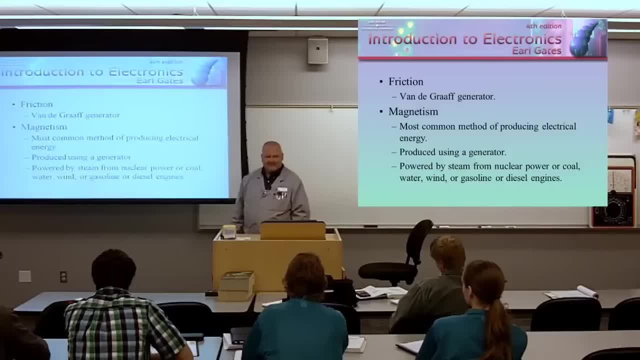 This is why, again, alternative energy. you know I've been to Holland before. they got freaking windmills over there. Windmills, They were harnessing windmills, Wind energy, You know. now we wind turbines. you know All you're doing is rotating the shaft and you're turning a generator as opposed to 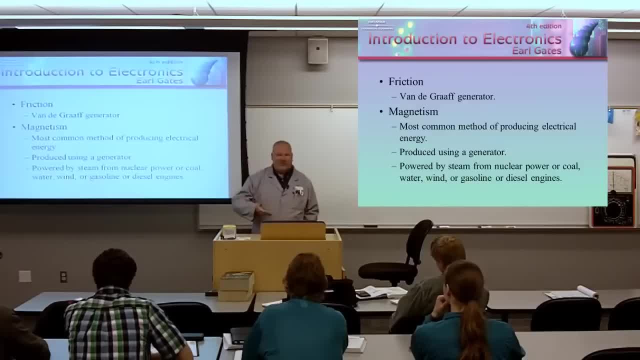 grinding your grain with power from the wind. So is it really alternative energy? Nah, there's just a different spin on it, Which is interesting because I've known this stuff since like puberty And I always, in the back of my mind, was thinking about like energy. 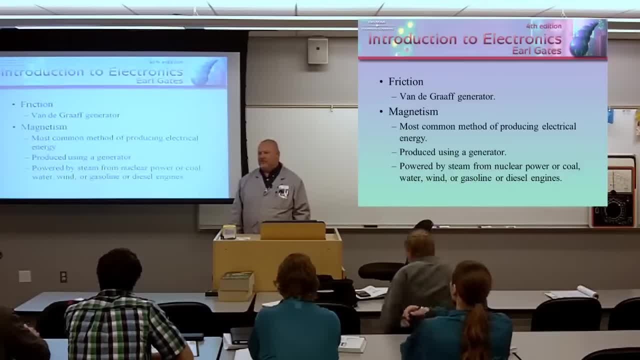 in different forms, Because I was always getting yelled at by my parents. you know, Shut the door, Shut off the lights, What do you think? you live in a barn, You know this type of stuff. So I was, yeah, at a very young age. I was thinking, wow, you know. 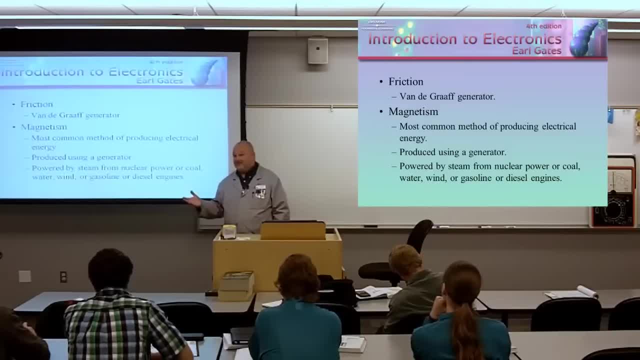 one of my duties as a child was cutting the grass, And it used to amaze me the small amount of gas I could put. I was always hoping I'd run out of gas, so, like I don't have to, I couldn't finish the lawn. Why I ran out of gas? you know The thing would never. 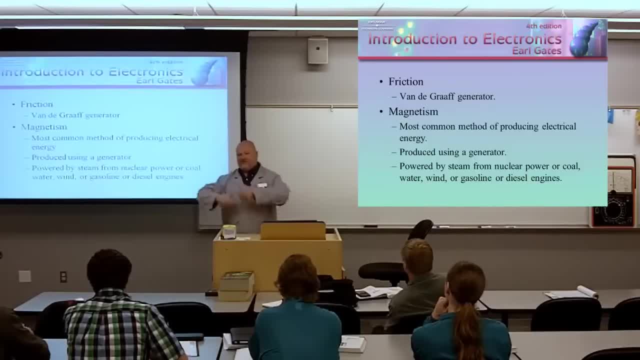 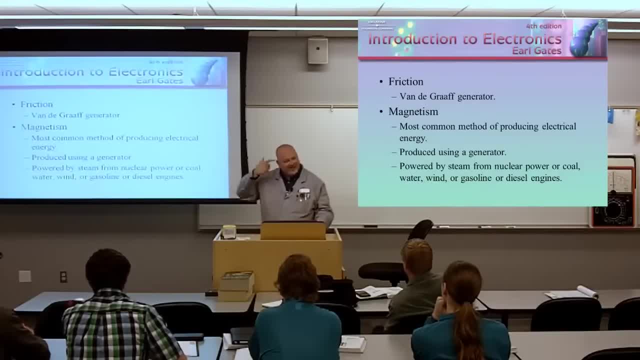 on, I could leave the doors open, I could get my parents off my back. you know, At a young age I was thinking about alternative energy And obviously I didn't understand all the formulas associated with it. So no, you can't necessarily power a home. 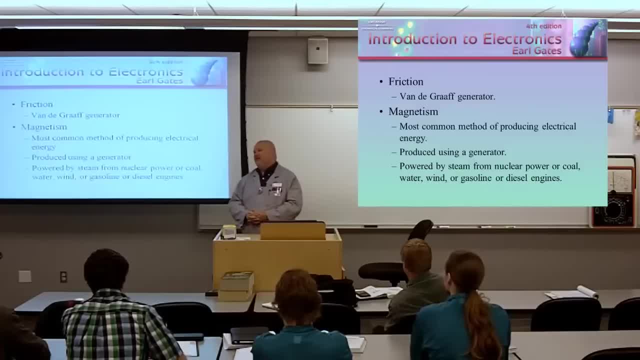 with a small three and a half horsepower Briggs and Stratton engine, But with a ten horsepower you could do it, And if you've got a backup generator that's a good enough size generator to power a home. Anyway, that's how we harness magnetism. The generator: 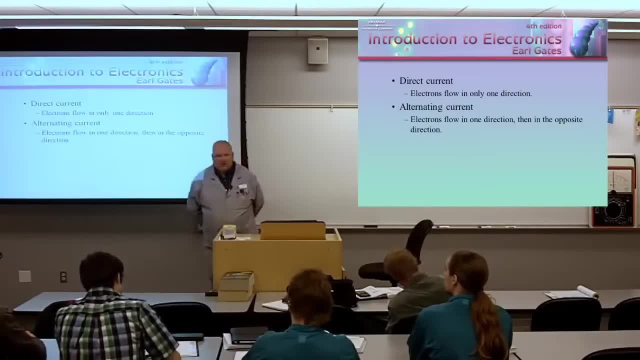 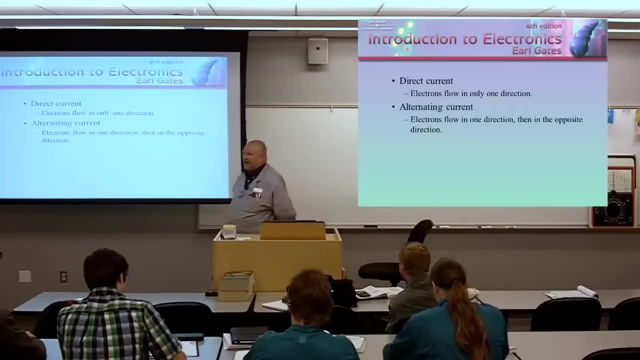 could be configured to produce either direct current. direct current is the flow of electrons in only one direction, Negative to positive, period Negative to positive Or alternating current. Alternating current is actually current. that goes back and forth, back and forth. What comes out of the outlets here in the school. 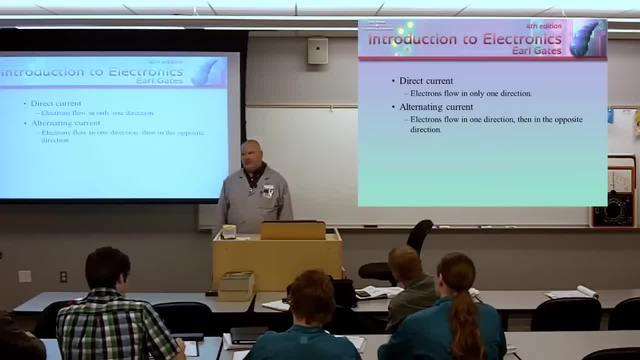 and at your home is alternating current. The electrons never really go anywhere, But they're getting shaken back and forth, back and forth, back and forth. That's the harness, That's the energy that we harness. So we could have a generator connected to a shaft that 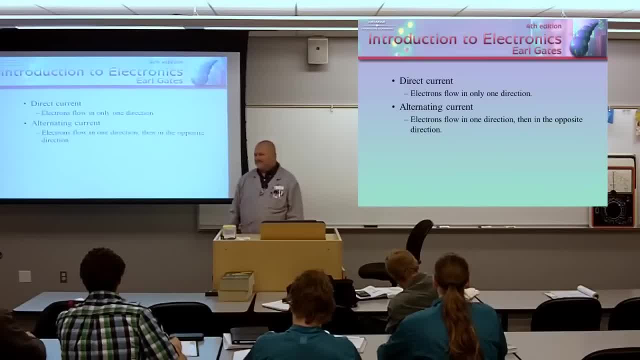 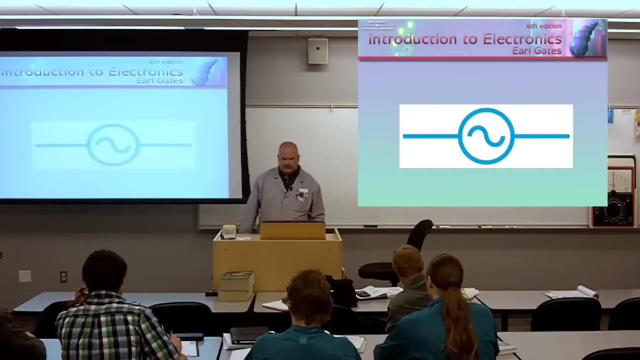 produces either DC or AC. DC generators are not that prevalent. They're not that prevalent, Really. AC is used predominantly throughout the industry because of it's a higher level of efficiency in transmitting the power. This is the schematic symbol for an AC generator. 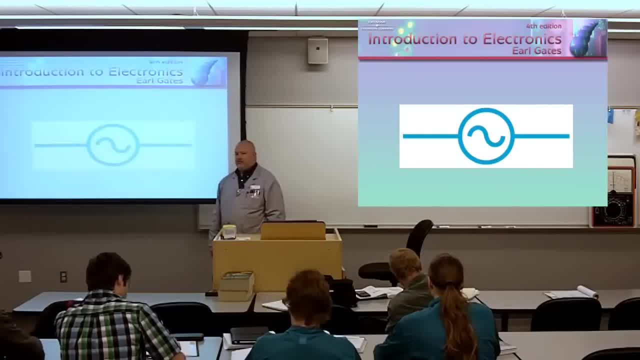 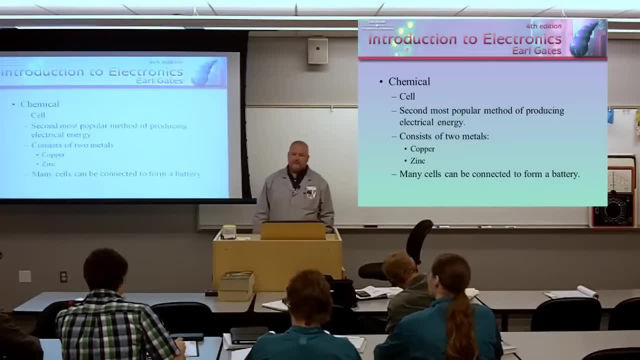 So if you saw this on a schematic you would say, ah, this means an AC power source, AC generator, Chemical Chemical- The most common is a cell. Chemical means is the second most popular method of producing electrical energy: A chemical cell. What we're talking about here is batteries. 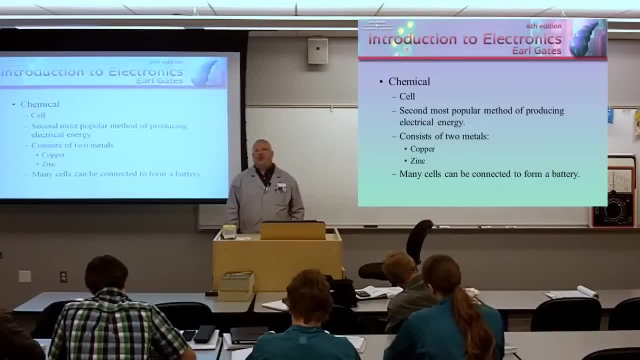 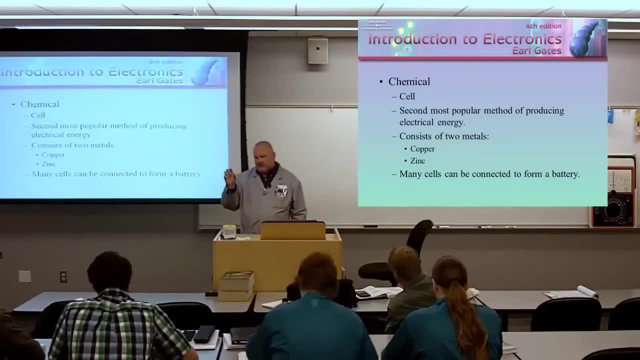 The original chemical cell consisted of two metals: copper and zinc. These were the old school batteries. Remember the kind that if you left them in your device too long they'd start to like ooze and ruin your portable electronic device. Those were just standard. 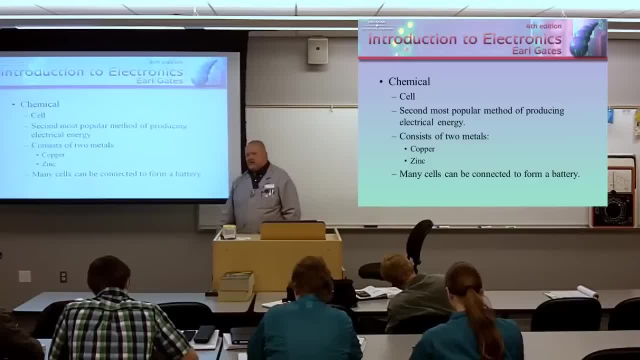 carbon or, yeah, zinc cells, Copper zinc cells. Typically, many cells can be connected to form a battery. When we use the term battery, we're actually talking about something that's made of multiple cells, And part of why I'm telling you this is that you're all here to learn a second language and that second language. 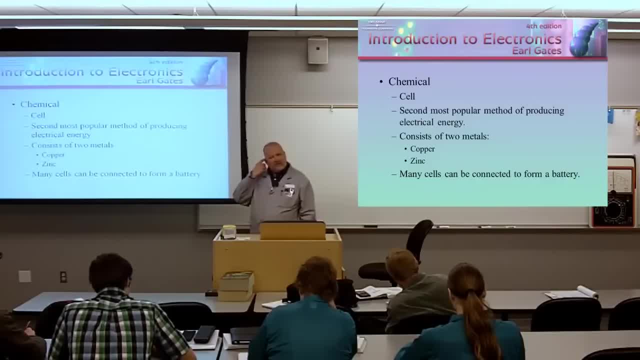 is electronics. So if you were going to go to Fred Meyer, where are you going? I'm going to Fred Meyer to get me some batteries. If you said that to me, I'm going to assume that you're going to get batteries, and batteries are multiple cells that are put together. 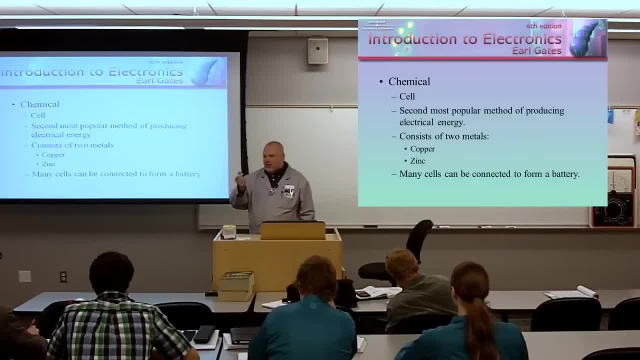 Where are you going? I'm going to Fred Meyer to get me some batteries. What do you need batteries for? For this here flashlight That battery doesn't take. that flashlight doesn't take batteries. That flashlight takes cells, And cells are the typical size. 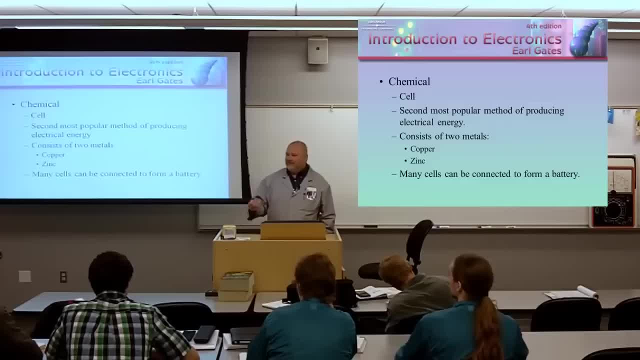 batteries that we've come to know and love: Triple A, double A C and, my personal favorite, the D size. cell D size means it's bigger. Since it's bigger, it means it's got more chemical in it. More chemical means it's going to last. 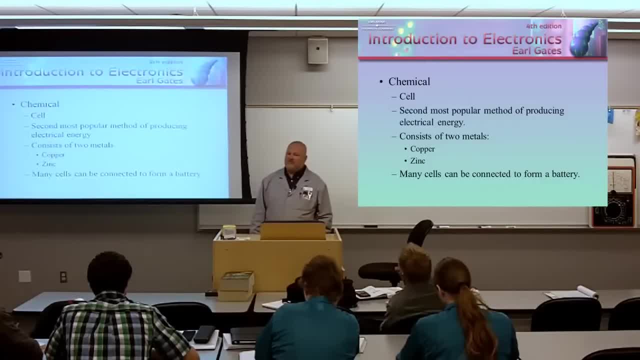 longer. If you had a D size battery and you connected it to your remote control. it would look stupid, but it would last forever. I put triple A batteries in my remote and they last for longer than my TV lasts. I just had some cells go out in a remote. 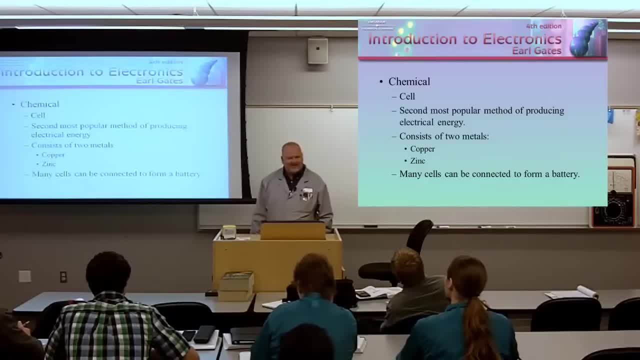 and I looked and they were the original cells in the remote. I'm like man. I've had this thing for freaking 14 years. It's got the original goofy brand batteries that came with it, So typically many cells can be connected to create what's known as a battery. 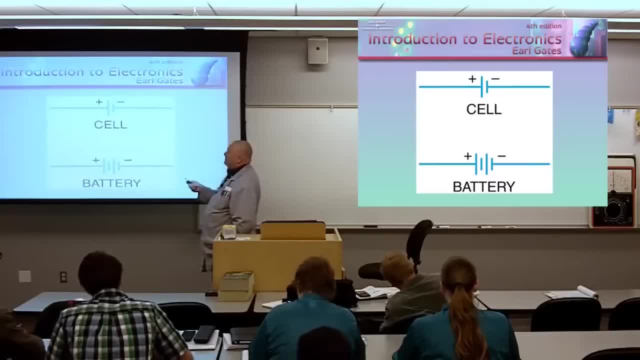 Now in schematic diagrams, when you see this symbol right here, you can assume that this is a cell. The short line is the negative lead, The long line is the positive lead. On a schematic diagram, if you put a short one, a long one, a short one and a long one together, we could make. 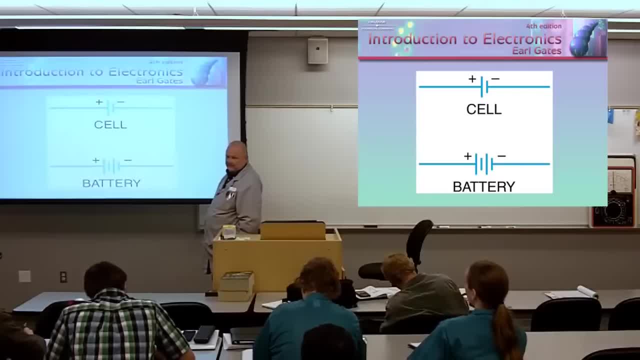 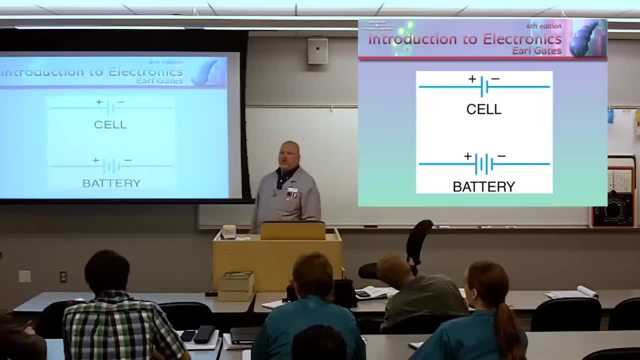 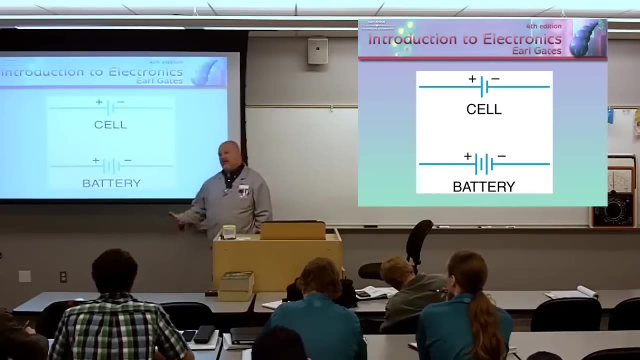 the assumption that this is a battery. The other assumption that you could make on a schematic diagram is when you see this: assume 1.5 volts, Because most cells- triple A, double A, C and D- all produce 1.5 volts DC. 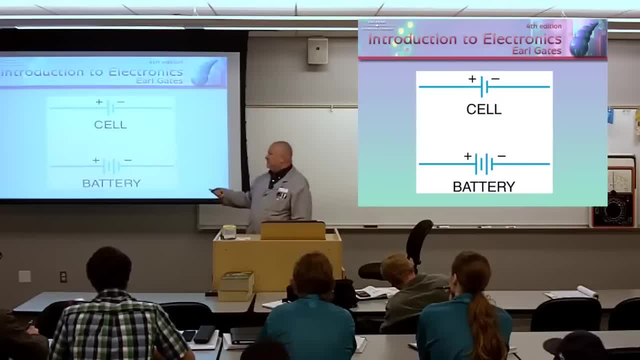 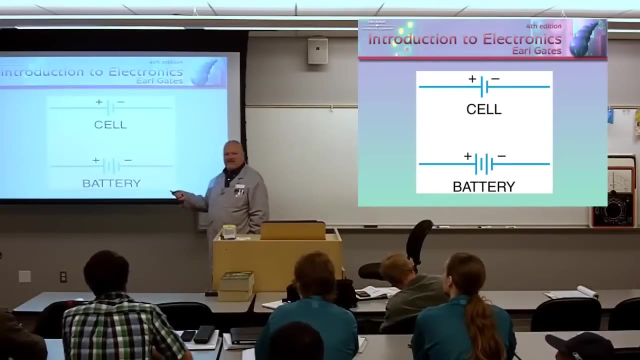 So if we saw this, what can we assume? 1.5 plus 1.5 is 3.. So normally on a schematic diagram, sometimes they'll draw two of these side by side, sometimes they'll draw three, but they won't draw any. 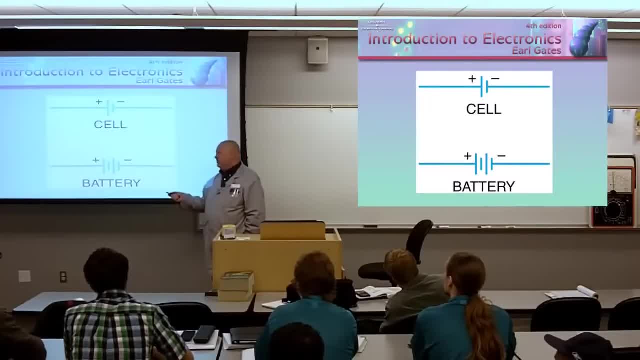 more than three. So any time you see two or more, assume, assume that it's either the value here or right next to this. I could write 12V. And if I write 12V, well it's a 12 volt battery pack. And if you split that battery pack open. 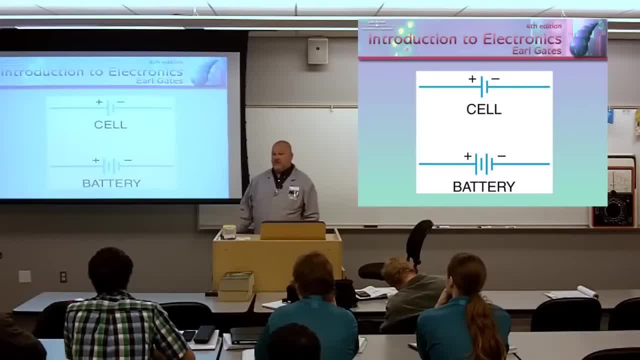 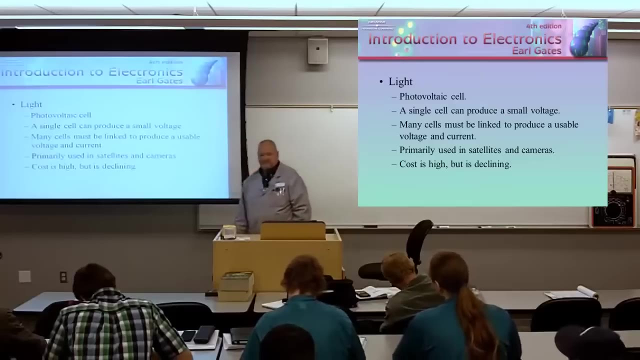 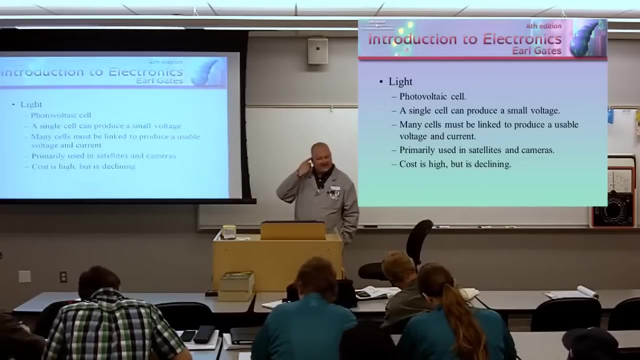 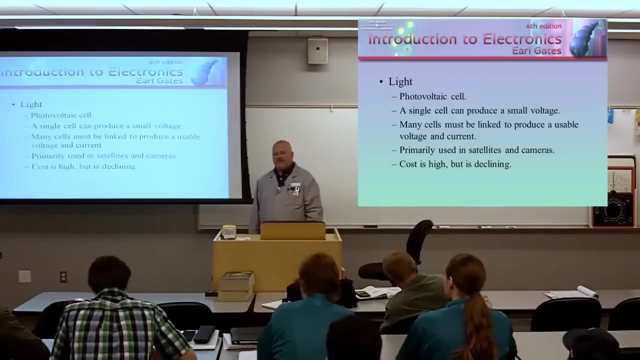 you would find that it's actually made up of multiple cells that are wired together internal to that battery pack. Make sense: Light Light. Photovoltaic cell harnesses light. A single cell can produce a very small voltage, So therefore many cells must be linked together to produce a 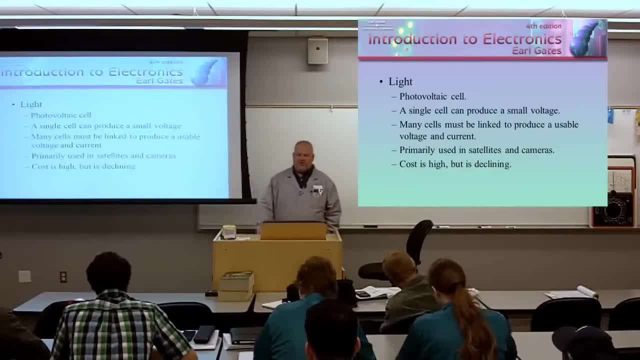 usable voltage and current. These are primarily used in satellites, because satellites would look stupid if they had, like an extension cord connected to them. You know you'd be like what the heck is that going up into the sky, you know? Well, it's an extension cord. 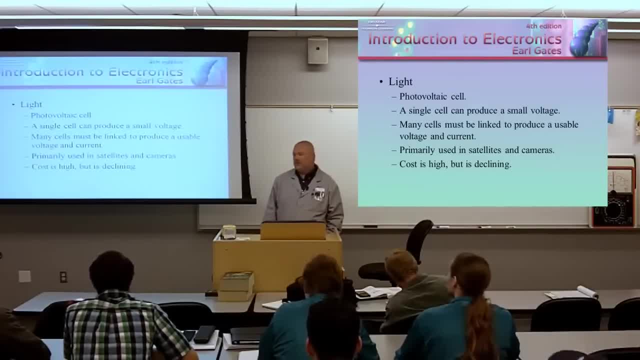 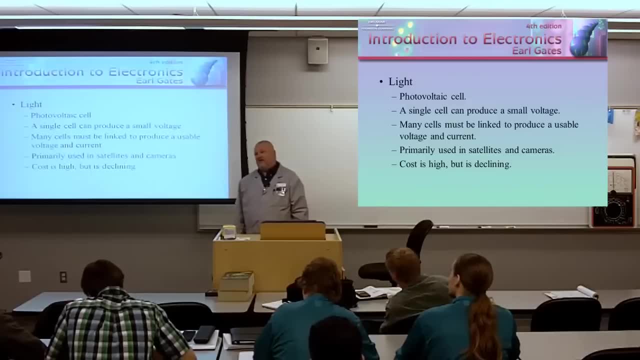 for, you know, a communications satellite. So we can't do that. Cost is high but it's declining. What I suspect is going to happen with this photovoltaic? basically to make a solar panel. it uses the same technology that is used to make microchips, So it's a pretty costly. 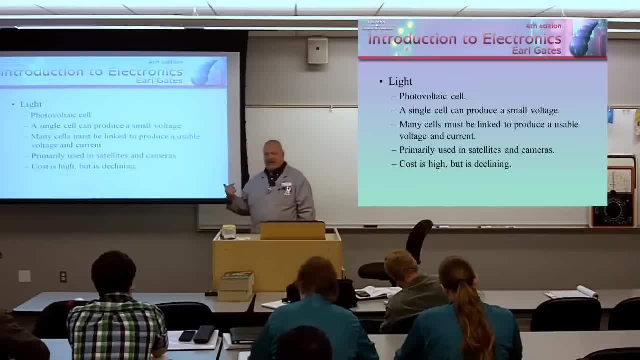 process. What I suspect to see- and you're not going to find this in any textbook- what I suspect you're going to see- is a marriage between photovoltaic and nanotechnology, And when those two merge together, you're going to be able to go to Sherwin Williams. 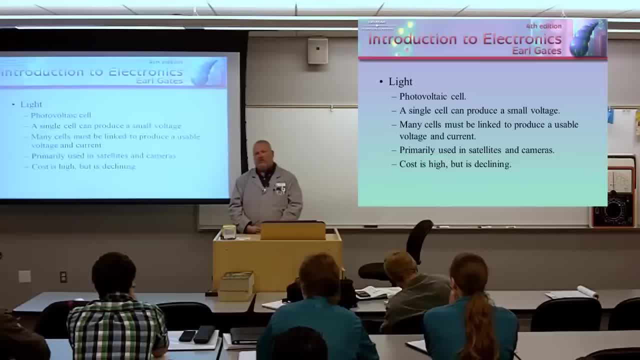 get paint for your house and they're going to say, sir, would you like the photovoltaic additive today For $19.95?? Sure, go ahead And they'll add a photovoltaic additive and the fact that your paint on your house is outside. 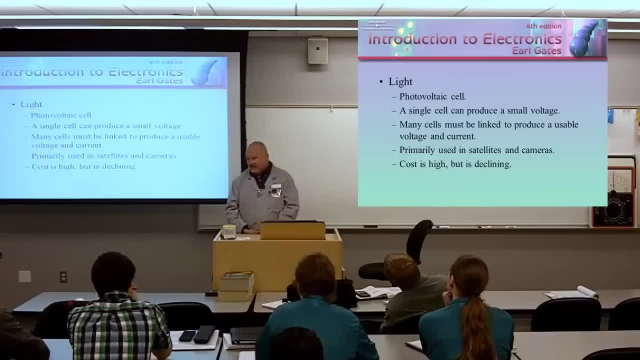 and it's in daylight part of the time. it's going to be producing voltage Now. we're not quite there yet, but I suspect that that's where we're going to be. They do have the technology now that there are companies that basically could spit out photovoltaic film. 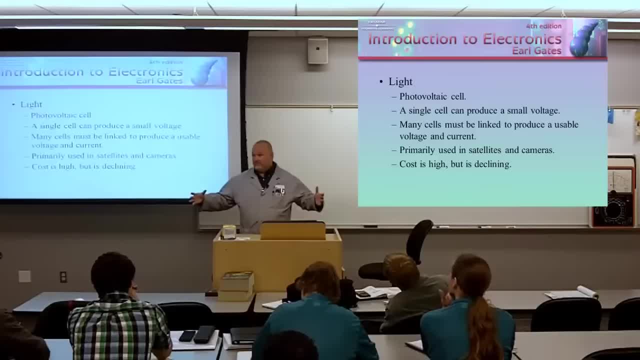 almost like Reynolds Wrap, So you could go out and buy a roll of photovoltaic and roll it out and connect your connections and you're producing electricity. So the cost is coming down on this stuff And think about it. free voltage from the sun. I mean how cool is that? I mean it really is Here in western Washington. well, you know, you probably have to pressure wash it twice a year to keep the moss from growing on your panels. I've got moss growing on my car. 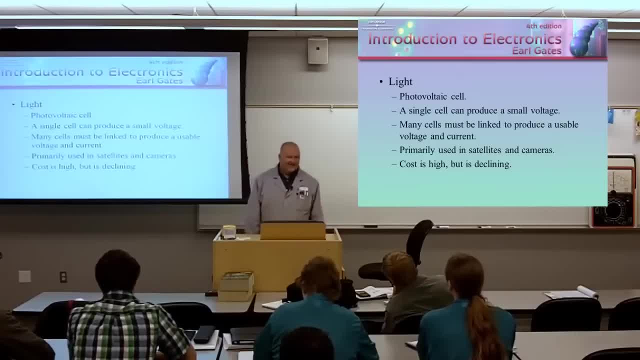 I'm getting it the other day and I'm like what the heck is moss growing on it? But other areas of the country, they're doing us, They're doing us. I was in Arizona Flagstaff several years ago and I checked into the hotel late at night. 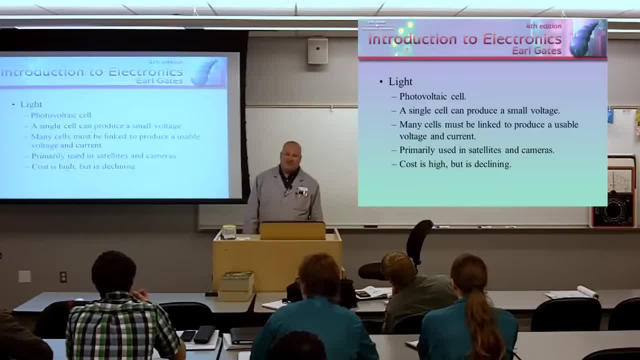 and got up in the morning and opened my curtain in the hotel room. I was on an upper floor and I was shocked Number one. it had snowed out the night before and it was like six inches of snow out there. I'm like holy crap, this is Arizona. 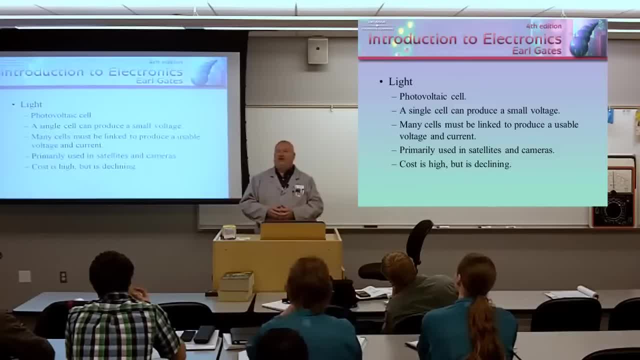 What's there snow doing out there? It's Flagstaff, You know, you're in the mountains. The other thing that shocked me is: wow, look at this. Across the street was a solar farm and it was all photovoltaic panels connected directly. 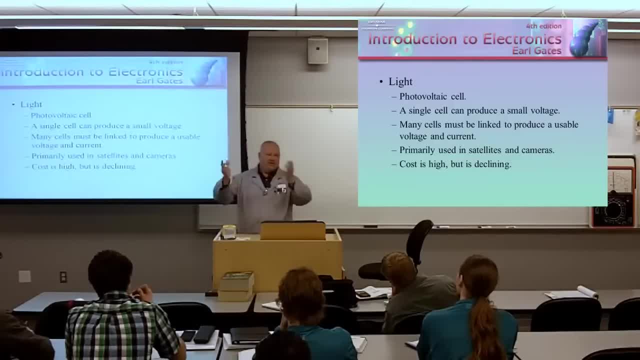 to the power grid And these panels would all track the sun and, you know, basically supplying energy to the power grid. So in some areas of the country they're already doing that And they're doing this. Would I run out tonight and buy solar panels for your home? 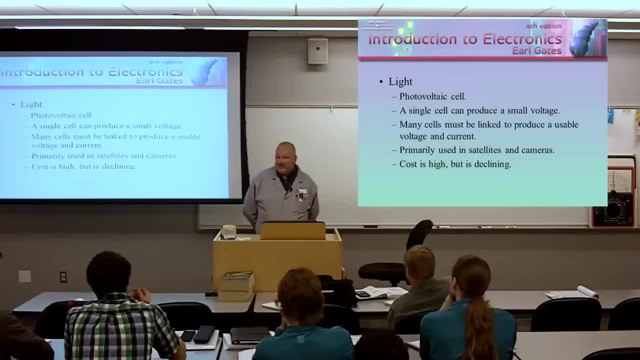 Probably not. But again, it's free energy, free voltage. So keep your eye on this technology, because I'd love to be an investor in the company that gets that photovoltaic nanotechnology harnessed. You know, just add a little pinch of it to your paint or whatever. and 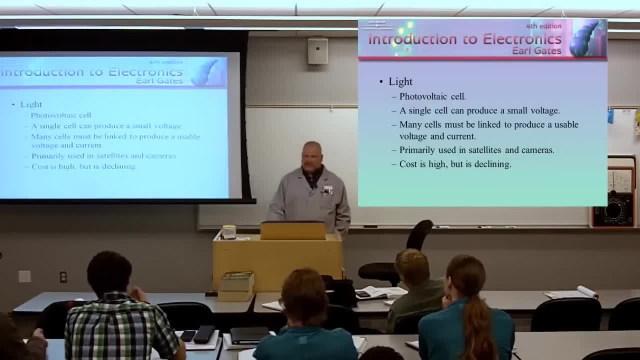 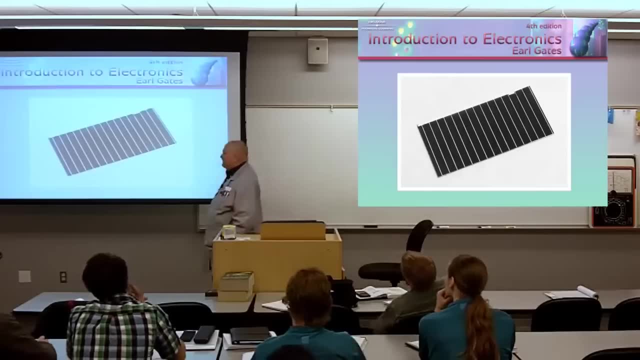 paint, whatever. you just turned it into a solar panel. No, Guarantee you, within the next few years we're going to be seeing that technology. This is what one of those solar panels look like, And the problem is this is on a metal backing, but basically it's glass. 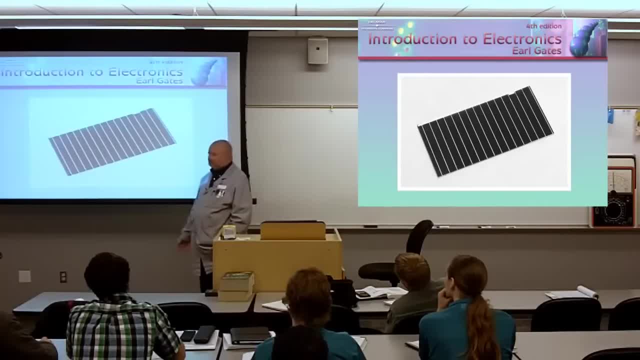 It's pretty fragile. You know you want to have it permanently mounted. Still, for outer space, satellite is the best option. Point it towards the sun. The sun comes out every day. Actually, if you're in outer space it never goes out because you know you're not rotating. 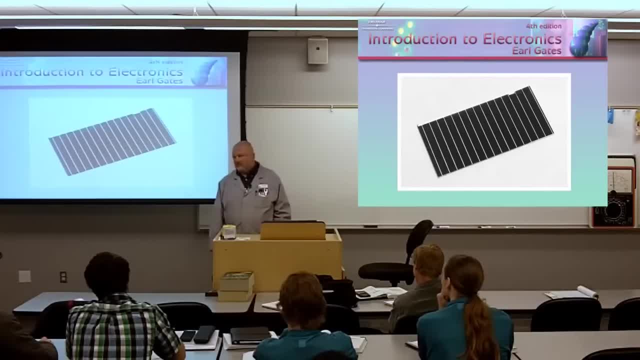 If you're a stationary satellite just looking at it, unlimited electrical resources. It was actually interesting. I was at a conference. I spoke at a conference a month ago- That was like a month ago today- in Milwaukee, Wisconsin. It was at the Green Energy Summit. I was an invited guest speaker. 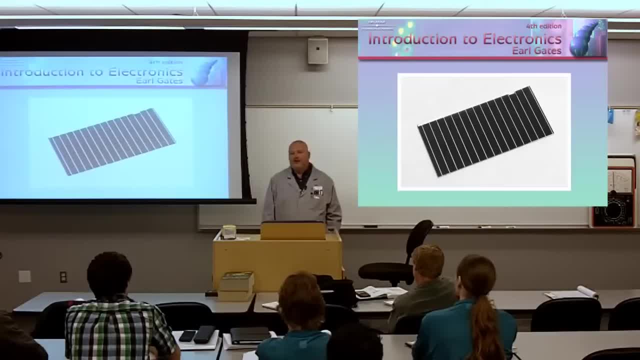 And one of the other speakers was very interesting. He had one of our first satellites, a mock-up of it, And when they were developing the satellite, this was in response to the Russians launching Sputnik, And it was the whole thing with the space race. 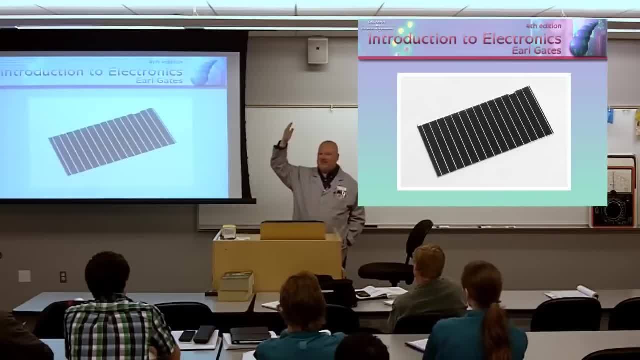 And basically, you know, he who gets the satellite in space first and goes to space first is going to rule, dominate the Earth. So this is all stuff that was going down in the 1950s. They in a push to get our satellite up there in response to 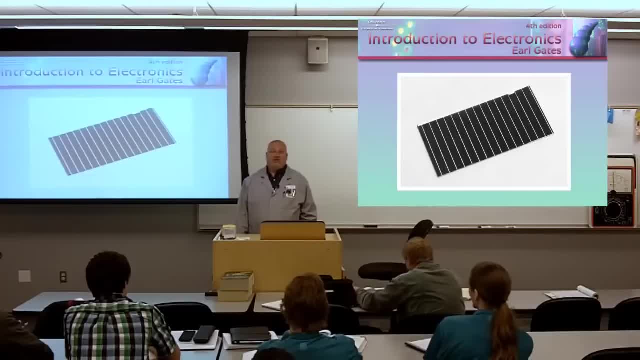 the Russian satellite. basically, what they had was a battery-operated satellite Launch. it Goes up, Beep beep, beep, beep, And that's literally all this thing did. It was a beacon Just beeping in space. And then, as an afterthought though, the engineers were like: 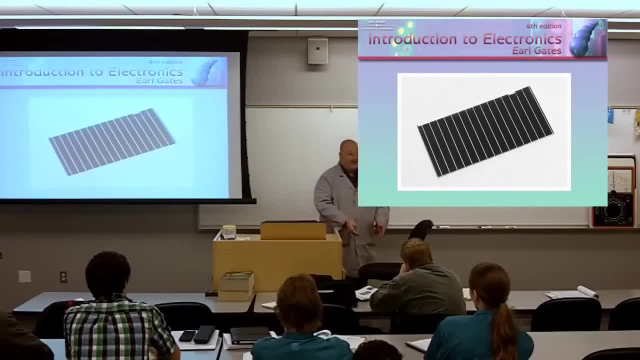 let's put this on it. This here is a photovoltaic cell. Let's put this on it so that when the battery dies, it'll continue to beep. And they're like: what are you doing? This is stupid. This is stupid. 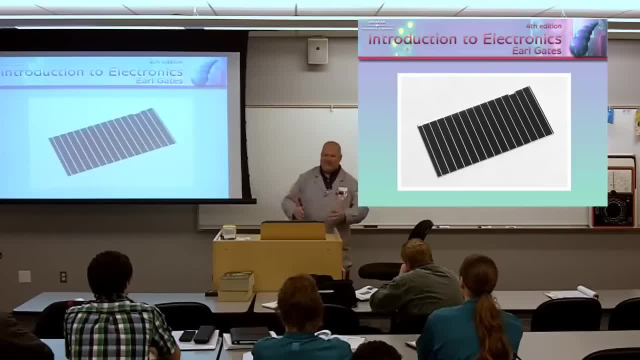 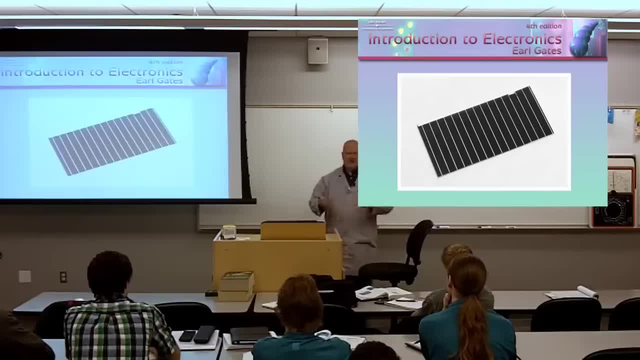 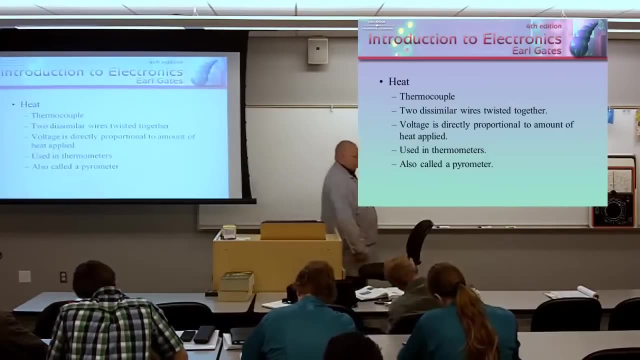 And I think finally it was like interfering with some other communication technology that had developed. They finally had to shut the thing off. So that was proof of concept that photovoltaics really work. It's been mainstream ever since. This is a cool way, No, it's a hot way actually. 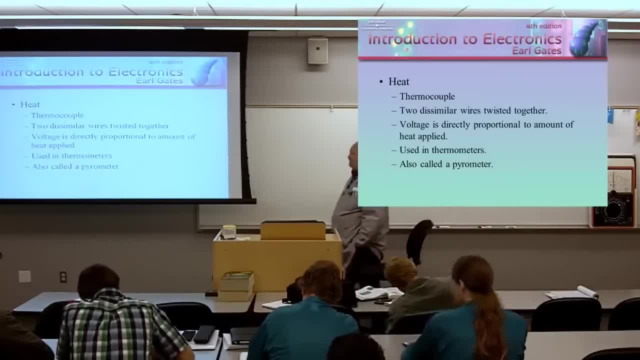 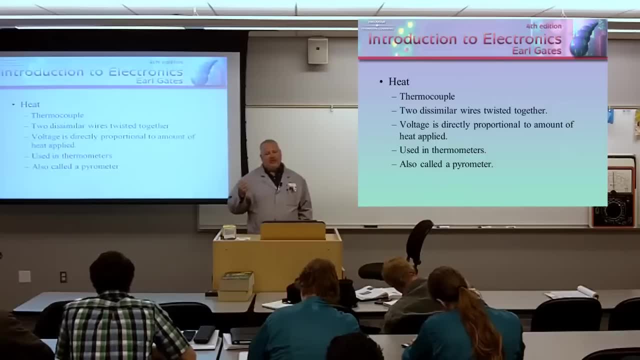 of producing voltage. We could use heat to produce voltage with what's called a thermocouple. These are two dissimilar wires twisted together. When I say dissimilar, I don't mean one blue wire and one red wire. I'm talking about two dissimilar metals And they're not actually twisted. 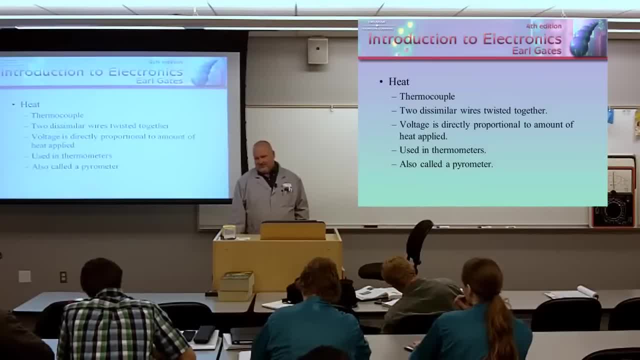 together. They're actually welded together. So you get the two dissimilar metals and then you weld them together Where they're welded together. when you heat that joint because they're dissimilar metals, it's going to produce a voltage. Voltage produced is directly. 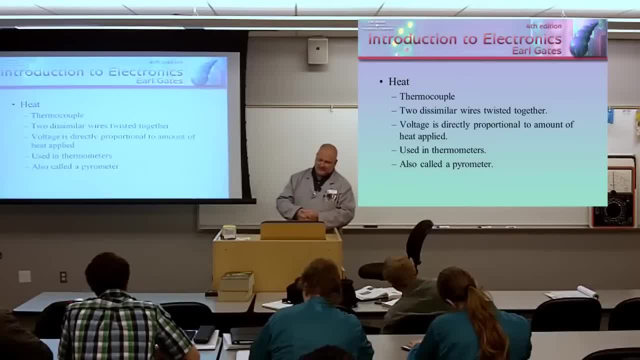 proportional to the amount of heat applied. These are going to be used in thermometers. You've seen a digital thermometer. Typically that's going to be a thermocouple, Because what it does is you apply heat to it. it produces a voltage. The voltage gets converted. 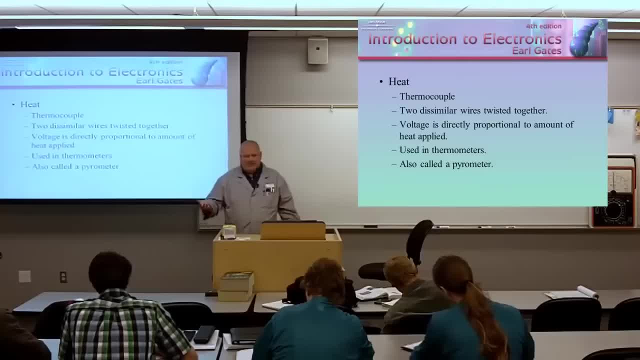 to an equivalency of either Fahrenheit or Centigrade, And then you read it out: Real simple way of doing it, Also called a pyrometer. Pyrometer Had a student in this class several years ago whose father owned a company locally. I forgot. 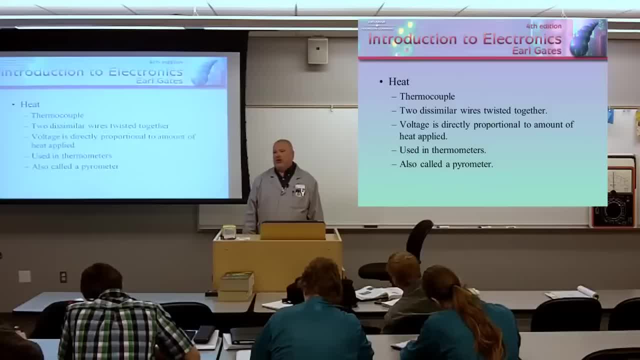 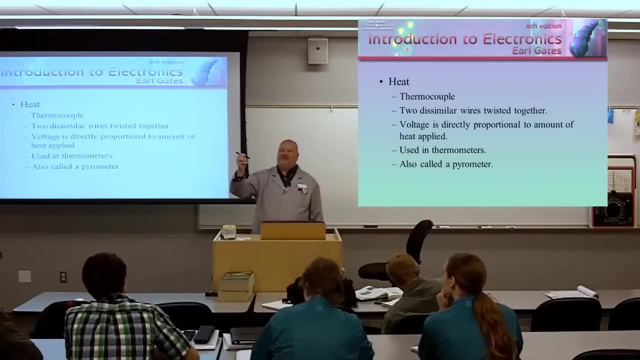 the name of the company, but they basically produced thermocouple sensors, And one of the big products that they were developing was specifically for the racing industry, And what it was is about the size of my laser pointer, It was nice stainless steel and it had a little. 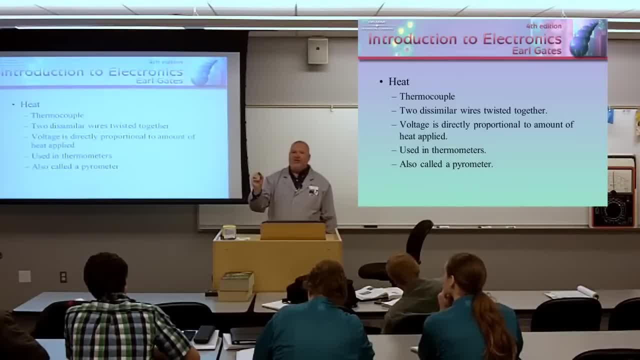 probe on the end and that was the thermocouple And what was so popular in the race industry. if I don't know how many of you are into racing or whatever you know, you take like NASCAR, for example, and ideally, what you want to do with one of those race cars. 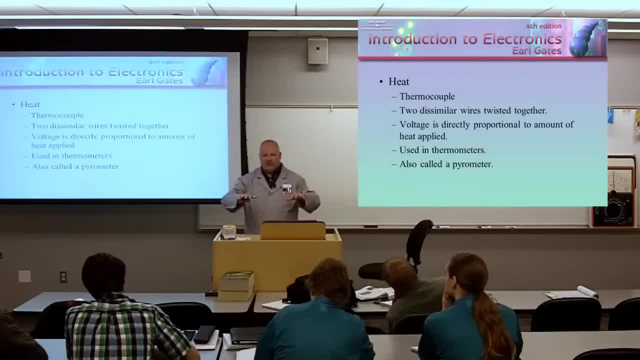 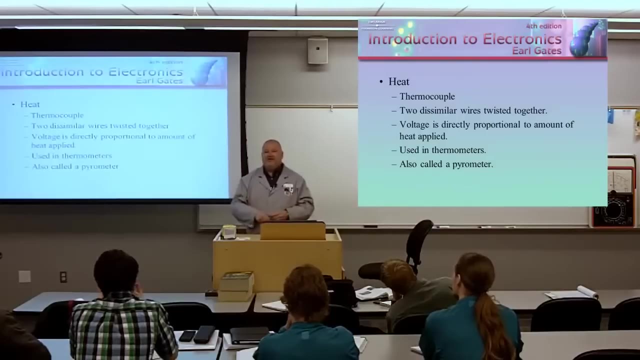 is set it up so that you distribute the weight evenly on every tire, equally across the tire, And if you could do that, obviously you've got the most contact with the road. it's going to give you the most handling on the track. it's going to give you the best performance Generally speaking. 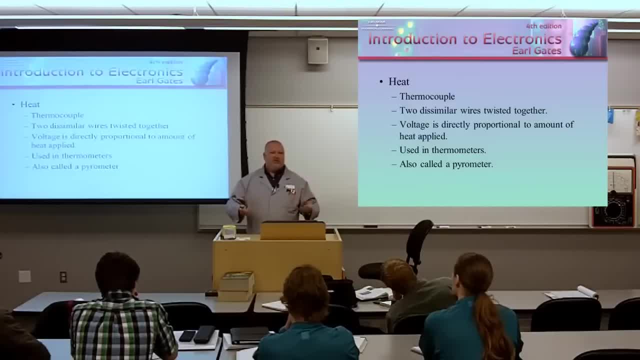 there are some exceptions to that on road course versus whatever, but basically you want full contact with all your tires on the track. Make sense. Also understanding with NASCAR rear wheel drive right, you're going to have a lot more friction on your rear wheels. 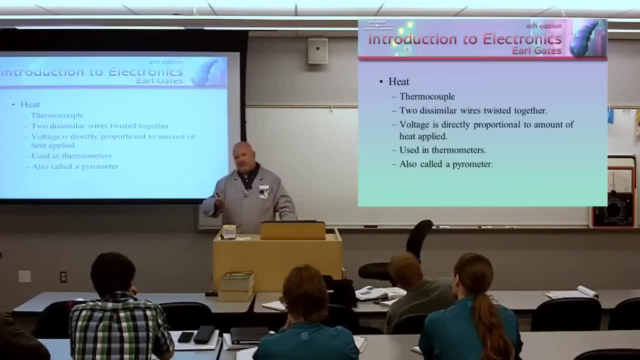 So what happens is when that race car pulls in and they pull the tires off, then they could sit there after they get the car out of the pits with their thermocouple probe and then measure across the tire outside inside or outside middle inside for my left rear. 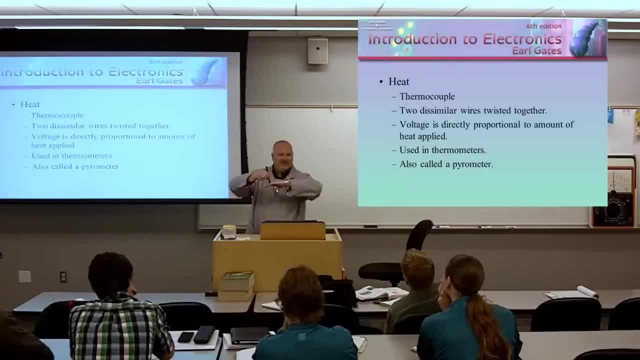 My right rear take the same readings. My front tire take the same readings. My other front tire- same readings. So you should see consistency between the two fronts across temperature wise too, that means you've got the car set up so that the tires are in full contact with the road. 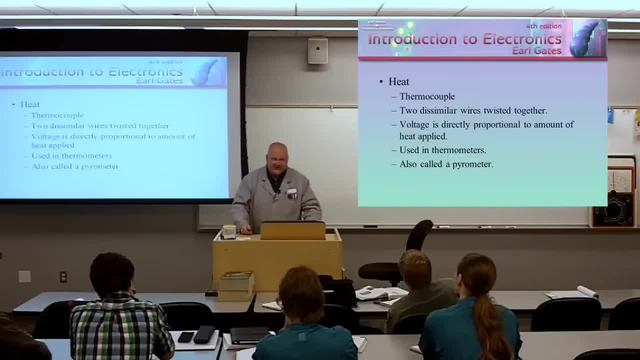 So it's really a poor man's alignment tool. So he gave me one of these. It's kind of cool because it's the OEM. It's just stainless. It doesn't have any decal or sticker on it. I mean, they're the factory that built it. 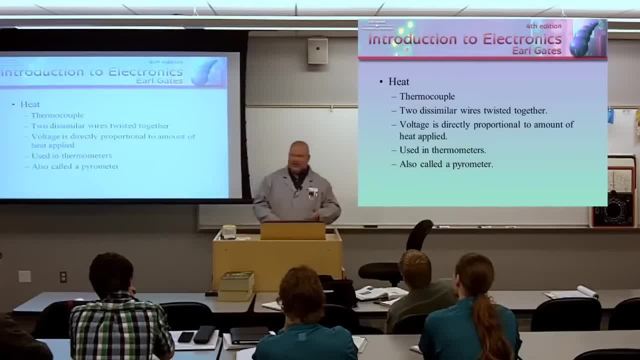 and then sold it to some racing company so they could put their name on it or snap on and charge an arm and a leg for the thing. So he gave me one of these things. So I actually did some experimentation. Since I am a commuter, I did that a couple times on my drive home. 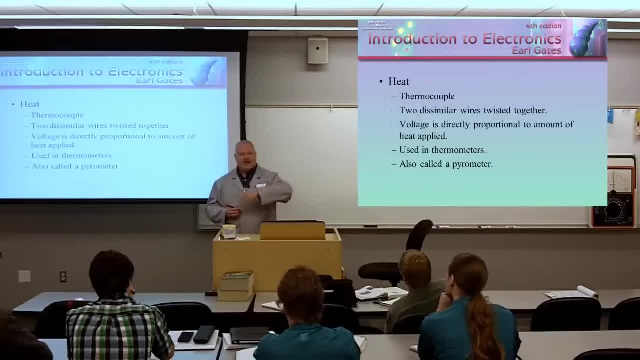 I was wondering what the alignment on my car was. You know I drive home, I pull off the exit hot Federal Way, pull over the side of the road, get out my Fluke meter- with this thing plugged in, take temperature readings. 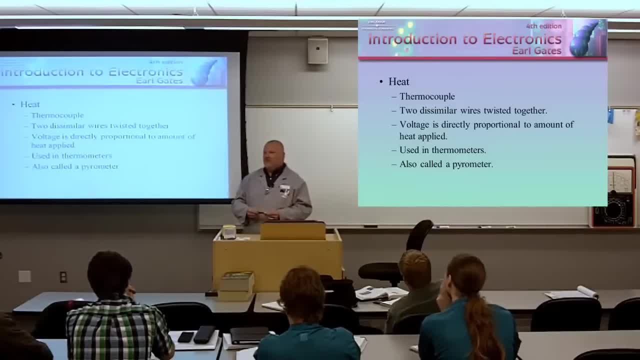 look for consistency. I've basically been tweaking alignment in my vehicles using nothing more than that temperature gauge. Pretty cool, Pretty cool Thermal couple. Simply applying heat to the device produces voltage. That simple Apply heat, it'll produce voltage. This is what the schematic symbol for one looks like. 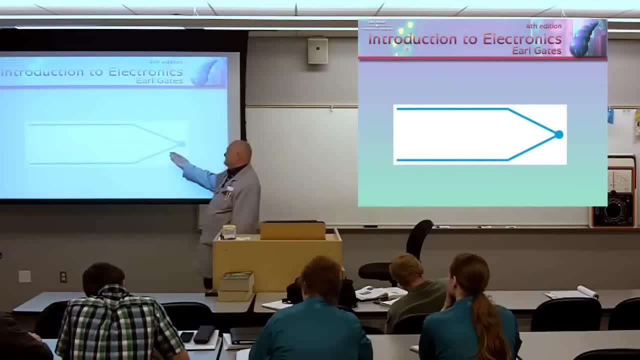 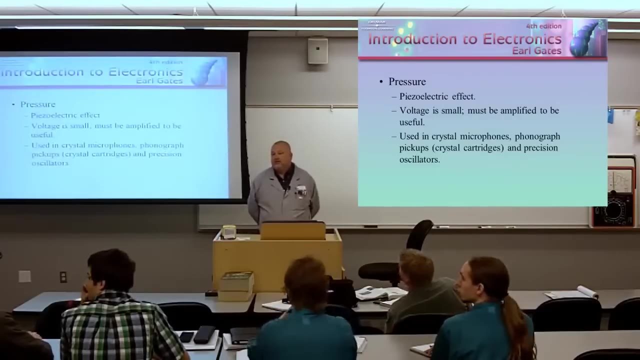 Again, understanding that these are going to be dissimilar metals, Two dissimilar metals, And then you weld this together, the bead Actually, that because they're in contact with each other, it will produce. Where would you take the readings At the very end of it On the tips? 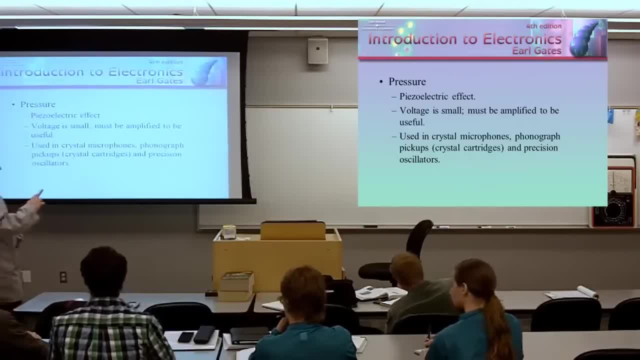 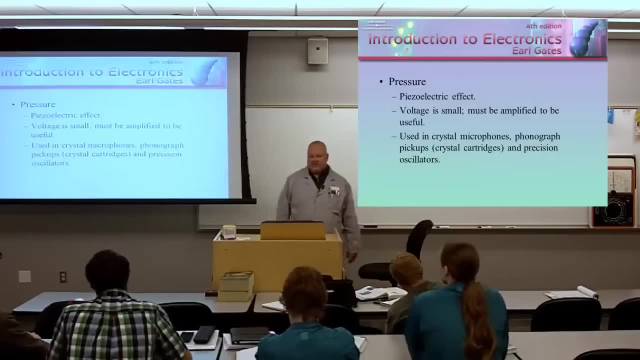 Okay, Yeah. So simply by putting the wires together, they are going to be in contact with each other, so you are going to get some reaction. But these thermal couple probes are actually welded. The tips are welded, Believe it or not. another method of producing. 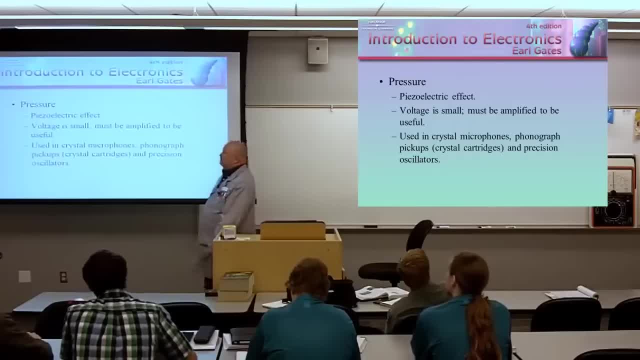 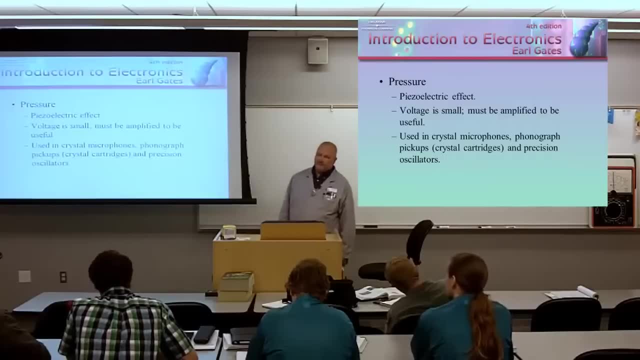 voltage is simply by the use of pressure. This is called the piezoelectric effect. Voltage is going to be very small, so it must be amplified in order for it to be useful. But just a pressure change on a crystal will produce a voltage. This is used for crystal. 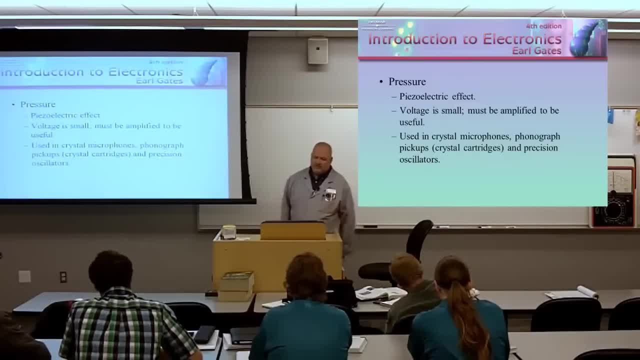 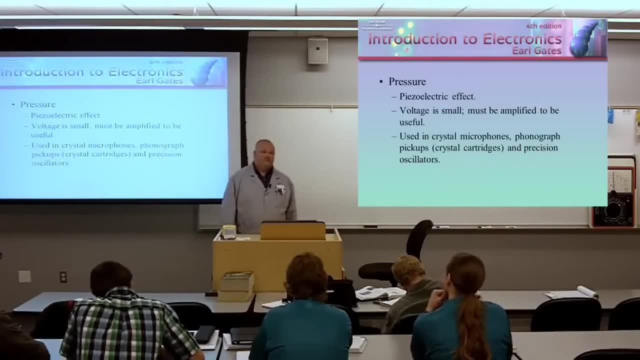 microphones, phonograph pickups and precision oscillators, As well as some sensors, pressure sensors. You could get some really inexpensive pressure sensors now that are calibrated for barometric pressure, standard barometric pressure, So as the Earth's pressure, the atmospheric pressure, changes on it. 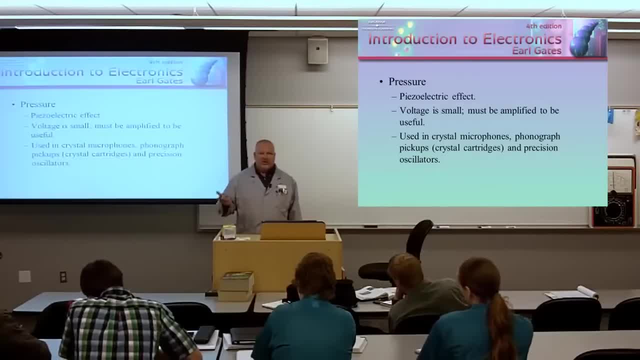 the voltage will change. You couple that with a weather station or couple that with. actually, you could use it for altimeter. If you're sending a rocket up and you want to know how high your rocket goes, you know what your base pressure is. As you go up in altitude, the pressure decreases. 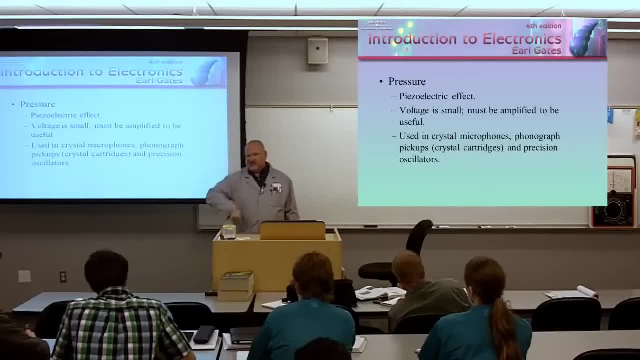 So you can have an inexpensive little sensor that keeps track of your pressure. Also, these are used in a lot of engine sensors. now, right, You could monitor all types of different pressures- Your oil pressure, your pressure of your cooling system on board an aircraft. 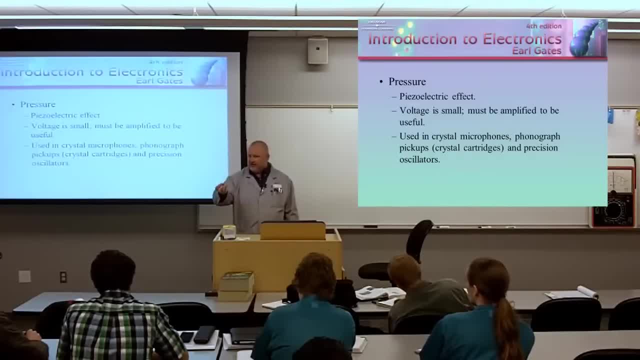 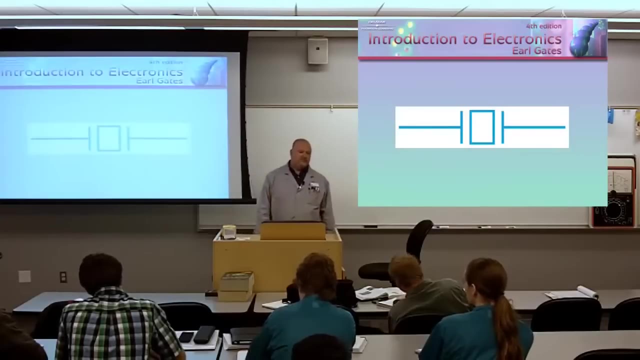 your hydraulic pressures. all of them A little sensor that voltage gets amplified, sent into a computer, and then you could look at all this virtual instrumentation, Simply doing it by applying pressure to a crystal. This is what the schematic symbol looks like for a piezoelectric crystal. 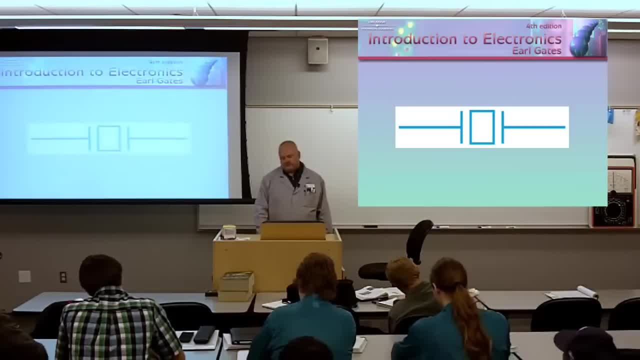 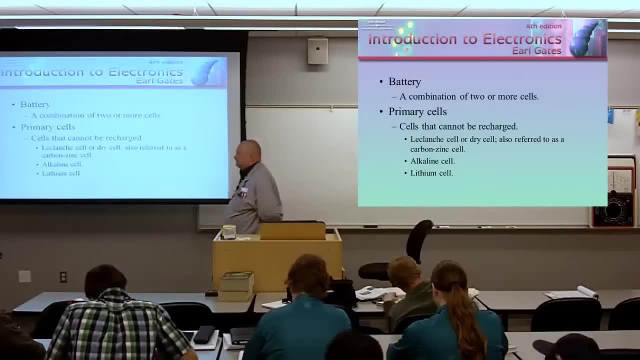 Now we're going to talk about some different types of batteries. Battery, of course, is a combination of two or more cells. Now we have two different choices of cells. One is called a primary cell, the other is called a. 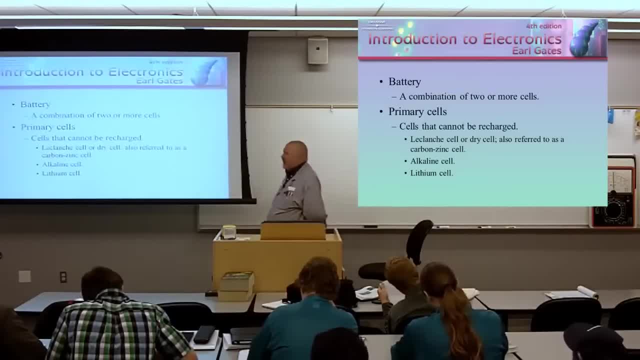 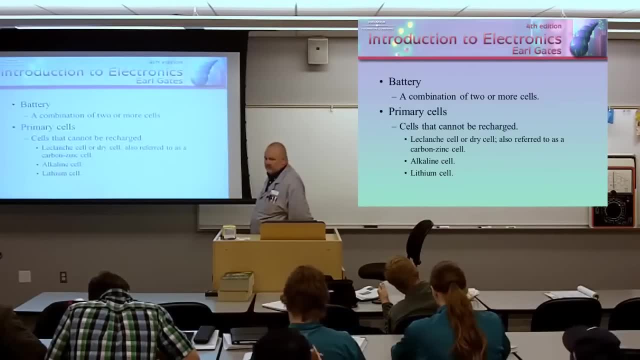 secondary cell. Let's first talk about primary cells. Primary cells are cells that cannot be recharged One time use. These are like most of the cells that you and I buy right. When you're done using them, you recycle them. 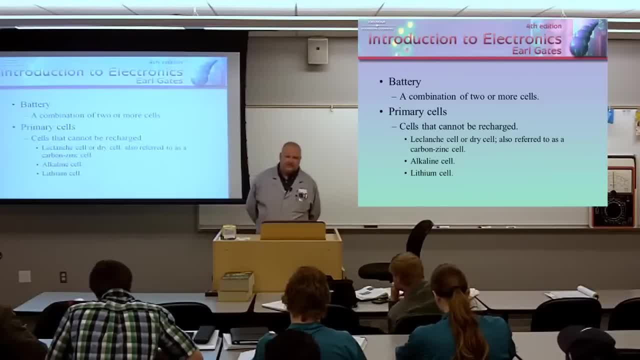 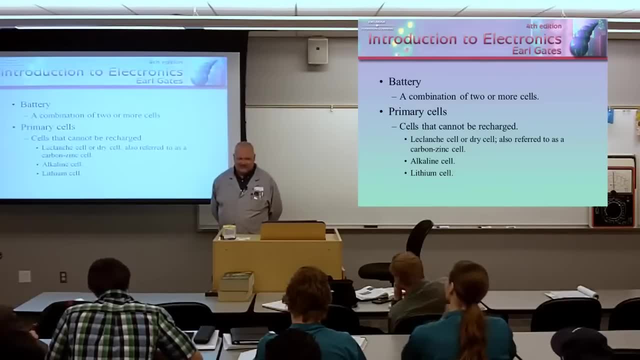 Don't throw them in the landfill right. You recycle them, Bring them to the hazmat place and then they'll turn it in and get money and make your community more profitable based on you turning in your dead batteries, Some of the stuff you don't want, going to the landfill. 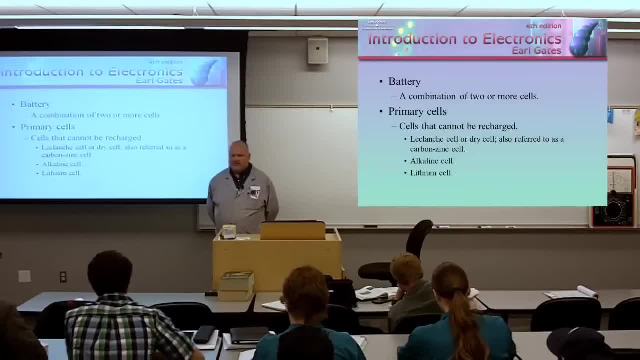 Although they've gotten better with the choice of chemicals that they're using. But primary cells: once you use them, you throw them away. This is designed after what's known as the LaClenche cell, or dry cell, also referred to as the carbon. 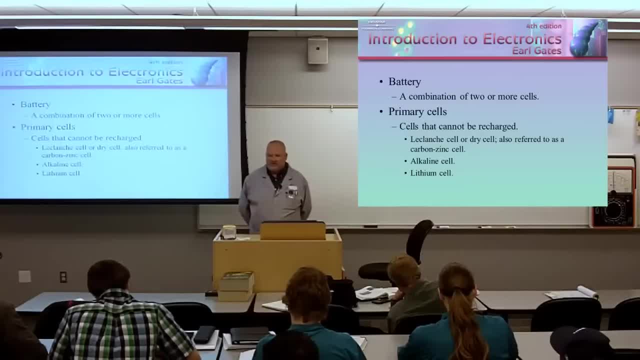 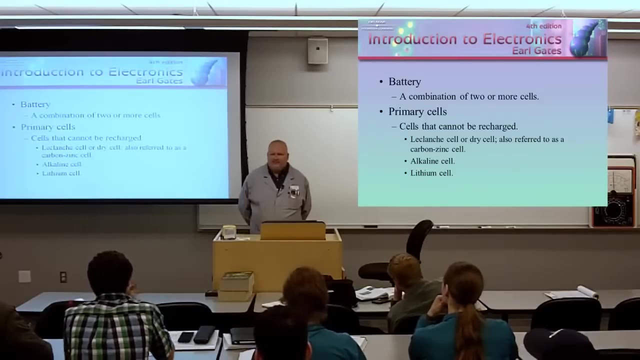 zinc battery. Carbon zinc battery. This is the old school battery that we were talking about earlier. I got a couple old timers in here, Remember, that's all we had. These are the only types of batteries that used to exist, And then I believe it was in the 1970's they came out with. 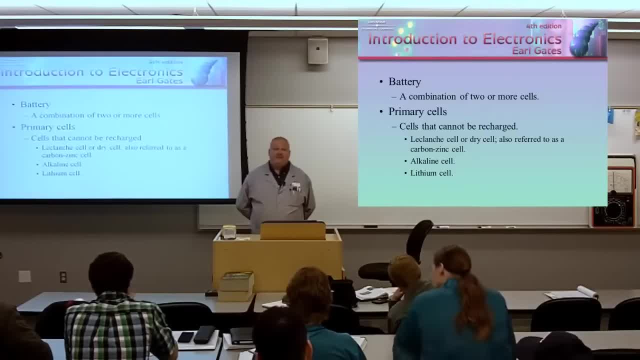 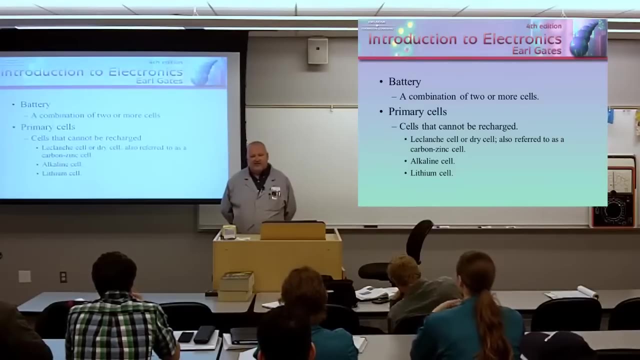 alkaline cells. That's when alkaline became somewhat mainstream, Started to become mainstream. These alkaline cells were still pretty expensive as compared to the carbon zinc batteries. I remember Radio Shack because, again, I was a big electronics guy so I was like hanging out at Radio Shack like looking at all the parts and stuff. 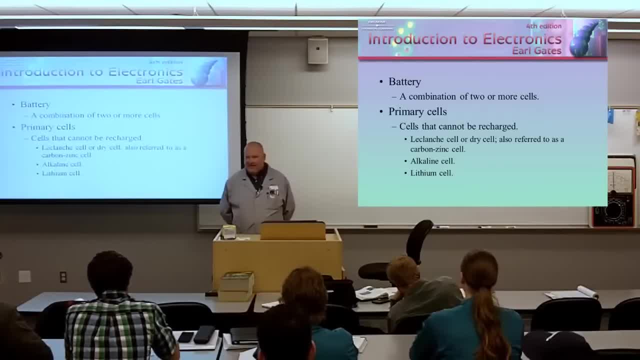 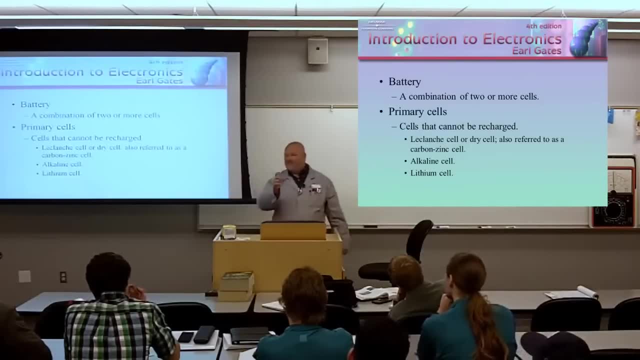 Radio Shack used to have a battery of the month club And you got a little card and you'd go in with the card and you'd pick out the battery that you wanted and then they'd punch your card and you got a free battery. It was a carbon zinc. 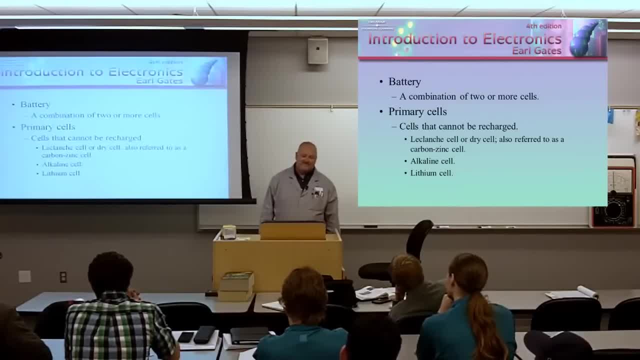 battery, but it got you in the store, Kind of a cool thing. Alkaline cells really, really good. Alkaline cells would work a lot better with a lot of electronic equipment when it came into being The latest cell and my personal favorite. 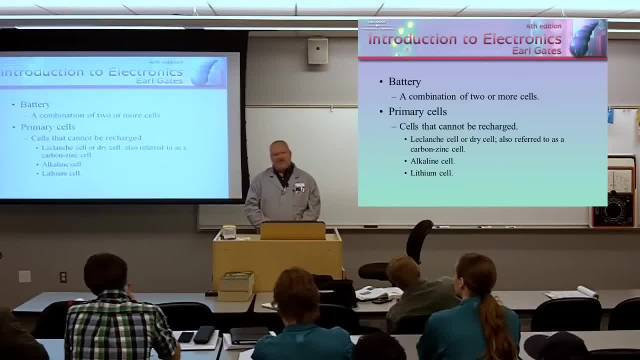 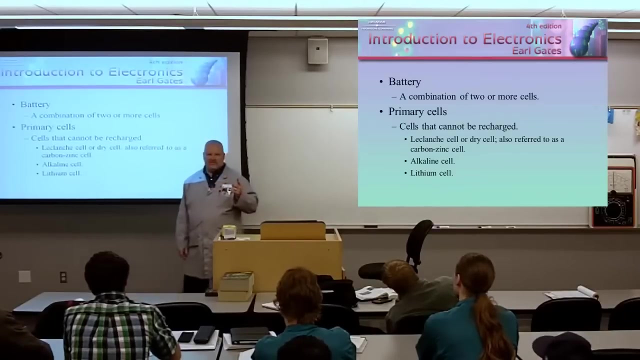 is the lithium cell. These are the high end lithium batteries that Energizer produces. They cost like sixteen bucks for eight batteries. They're very, very pricey, But these lithium batteries will produce a voltage longer than any of these other types of primary cells. They also have a longer shelf life. I'll bring in a package we can look at it. I just I bought some last week and I think it's. the expiration date on them is like 2022.. Some crazy time in the future. 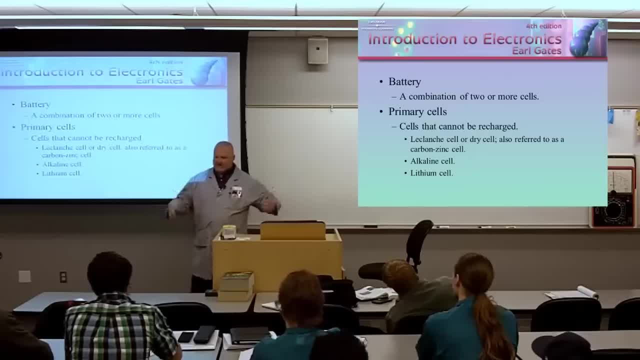 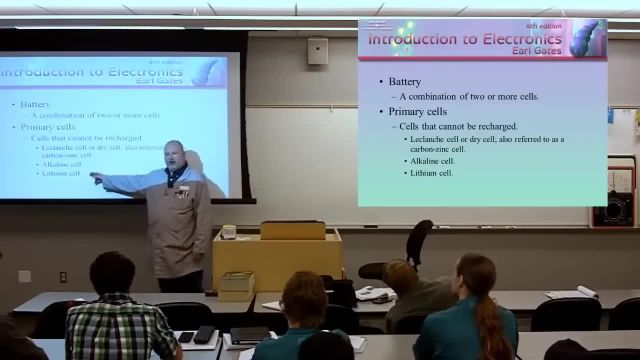 We won't even need batteries. like that We'll be flying to work in jet packs and stuff. We won't even need lithium batteries. And the other thing that these are real great at is working at a variety of different temperatures, from extreme cold. 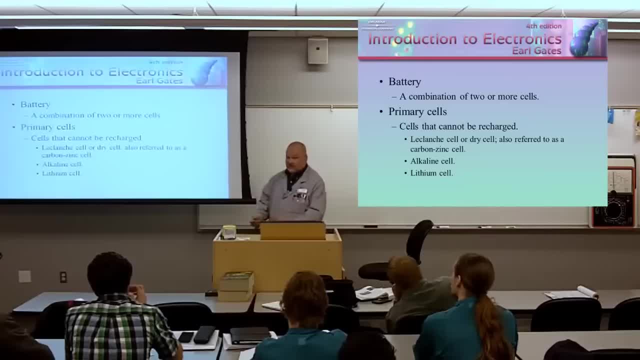 which really kills batteries big time, slows down that chemical reaction to extreme heat. They've kind of known about lithium batteries for a while, lithium cells for a while. On my airplane there's something that's called an ELT emergency locate transmitter In the event of crashing. 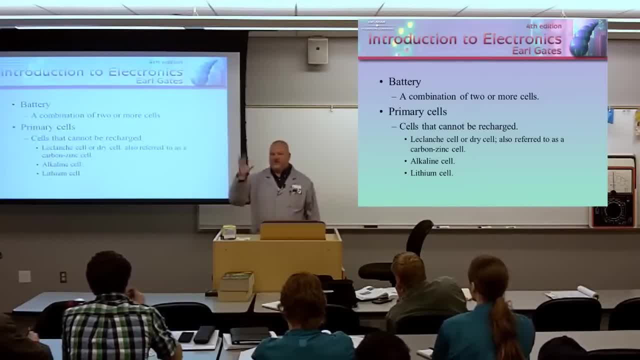 there's a G switch that triggers a transmitter to start transmitting out a beacon That gives your position away. So search aircraft. actually they used to have satellites that looked for that signal, but now they've- long story. they've switched those satellites off. They've gone to some different frequencies now. 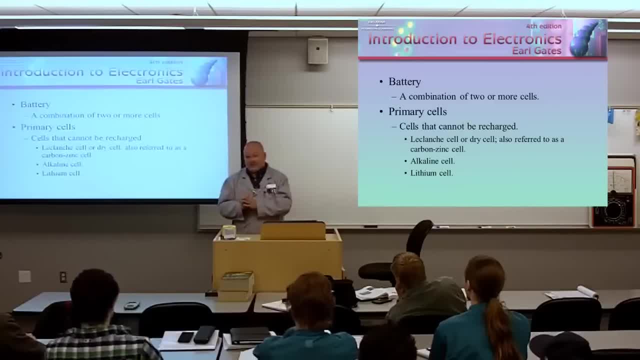 But it would transmit. So when this thing worked, it had to work. It's a safety device, Even like on a ship that goes down. they have these EPIRB systems that transmit to the satellite. You want that when it has. 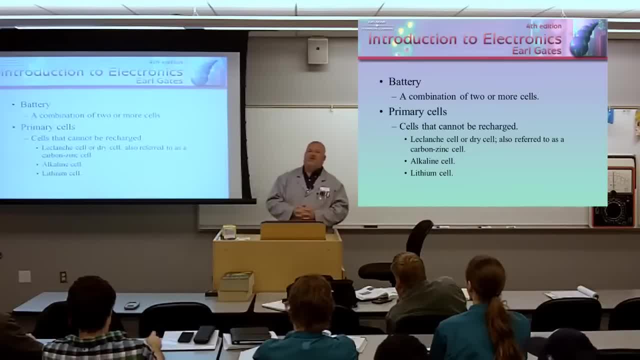 to work. you need the thing to work, So this has always been the choice for those types of applications. lithium cell: I was really, really jazzed and excited when I saw these come on the market for a consumer based product, Because the lithium batteries before were unique To the manufacturer, would put it together and you'd have to buy the replacement from them Because, like the FAA requires, every 24 months, you've got to replace that cell whether you've used it or not. So for them to come out the sizes that I'm aware of they have triple A. 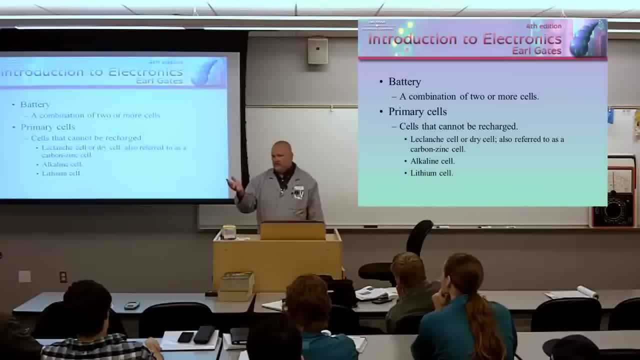 and they have double A size. Have any of you here used any of those? Have you used them? Highly recommend it If you're going on your dream vacation, if you're doing photography and you want something for your flash and you want that flash to keep. 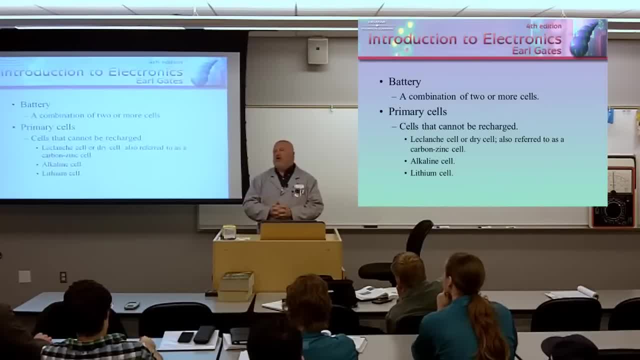 going off and you don't have to worry about it. If you're going hiking, I use it on my GPS. I have a backup GPS that I use whenever I'm going off the grid or anything. I've got a pack that I bought. Energizer will sell you a pack that you could use. 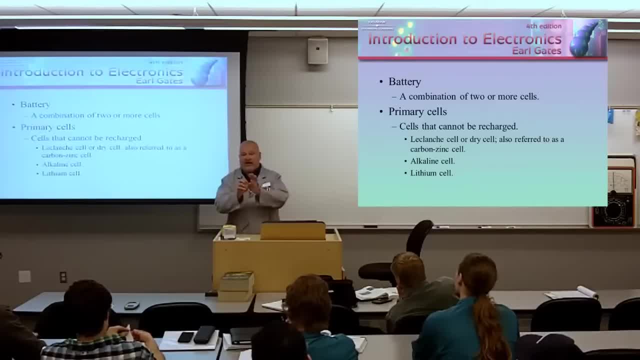 to recharge your cell phone. Have you seen those things? It's like a little pack and it comes with those lithium batteries and it's got a little cord, So like if you're off the grid and you've got to recharge your battery, it comes with that. 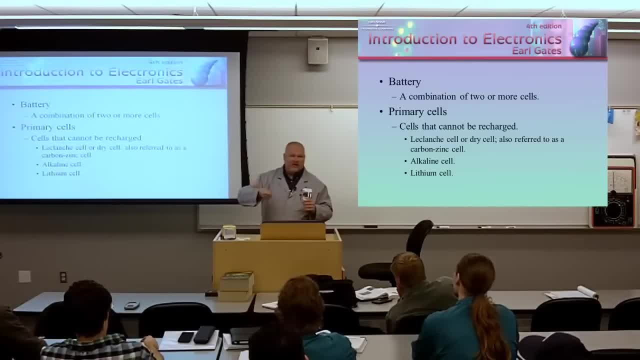 style. You know your micro USB or mini USB plug or your Nokia- Everything now is micro USB. That's kind of the standard for newer cell phones. But you put those lithium batteries in it, You plug it in and it will give you another charge. 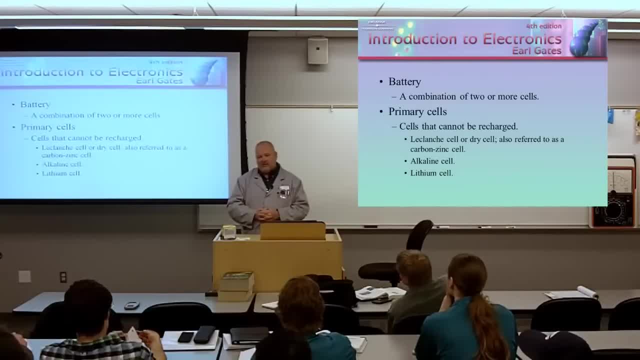 If any of you do any back country stuff or anything like that, I highly recommend you look into them. It's a wise investment, A very wise investment. It's the best primary cell that money will buy. This is kind of you've got the. 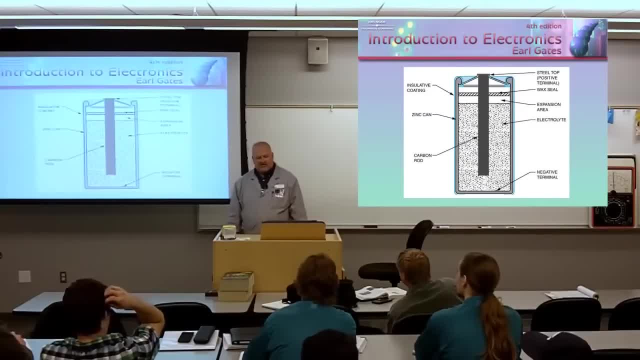 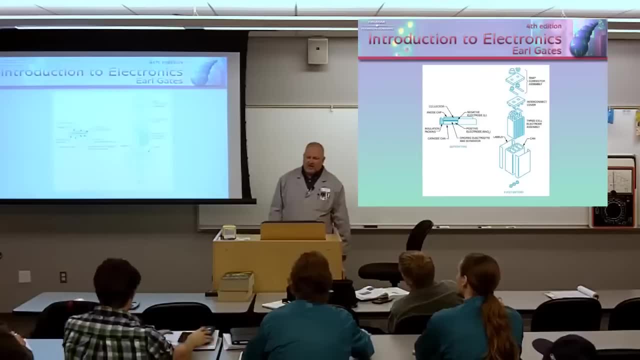 diagrams in your book, kind of a cutaway view of a standard carbon zinc cell. Another cutaway view there: Cutaway view of a 9 volt battery. Is this really a 9 volt battery? Is it really a battery? Yes, it is. It's made up of multiple cells that have been put together. Each cell is capable of 1.5 volt, So they put multiple cells together to give them 9 volts. Why 9 volts? Actually, this 9 volt battery is also synonymous with what was called a transistor battery. 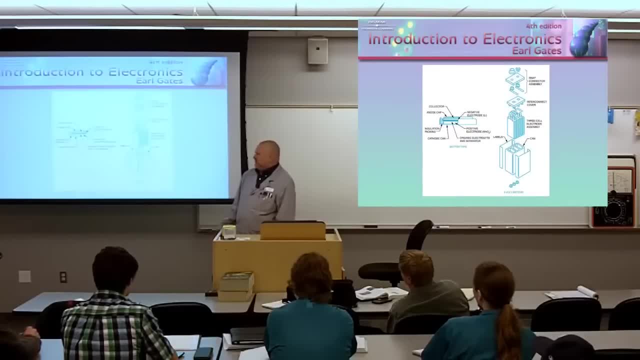 back in the day. There's no transistors in it. Why was it called a transistor battery? Because this is the type of battery that your transistor radio would take. Growing up in Connecticut they used to have a little small 8 transistor radio. 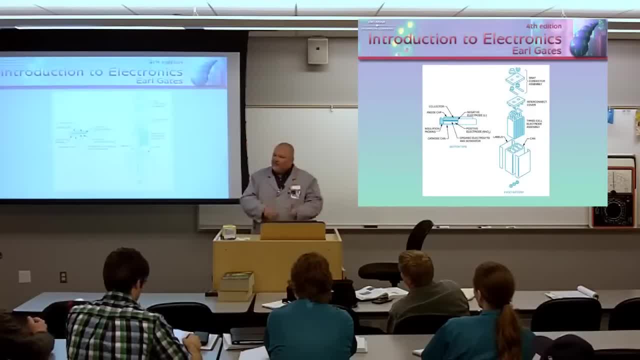 Used to go to the beach and they used to tune in my little radio. Listen to New York radio stations Playing all the top 40 hits and everything. 8 transistor radio. Took a 9 volt battery or transistor battery. This was typically. 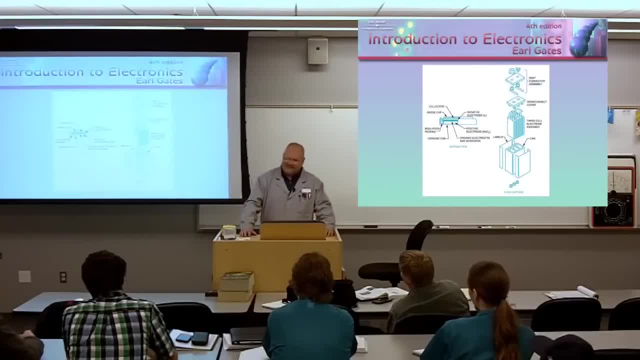 the battery that I would get as a free battery at the Battery of the Month Club from Radio Shack. Why My assumption was it's got 9 volts. The other ones have 1.5 volts, So I'm getting more for my punch- my free battery- than 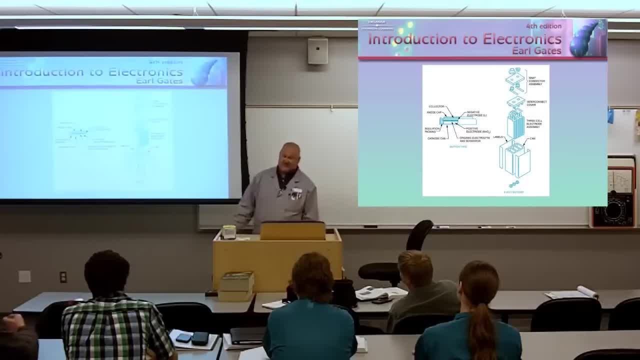 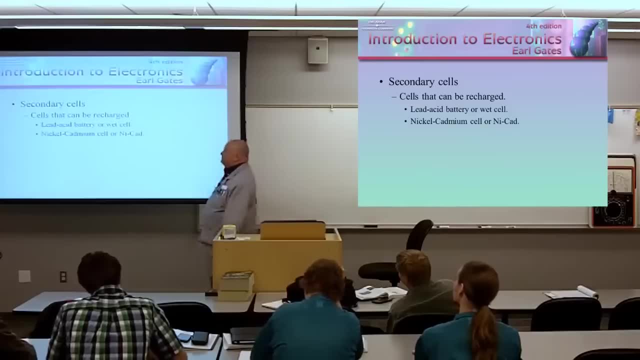 a 1.5 volt battery, So this was typically the bad boy that I always used to get for the purpose of experimenting. Secondary cells are cells that cannot be recharged. You're all familiar with this type of cell: the lead acid battery, or 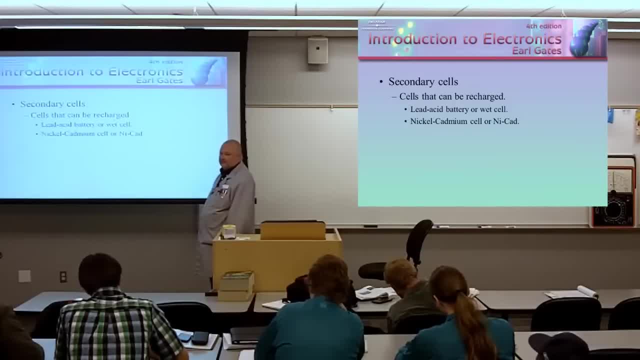 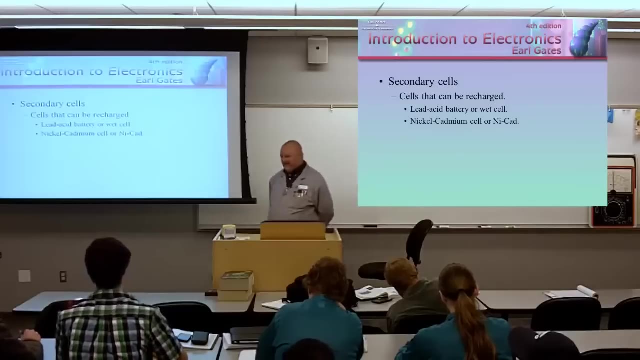 wet cell which is in your car right now. These batteries are not just used for automotive applications. These wet cells, these lead acid cells, are also used for backup power supplies by the phone company For your cell line. They're also used at cellular sites for backup power. 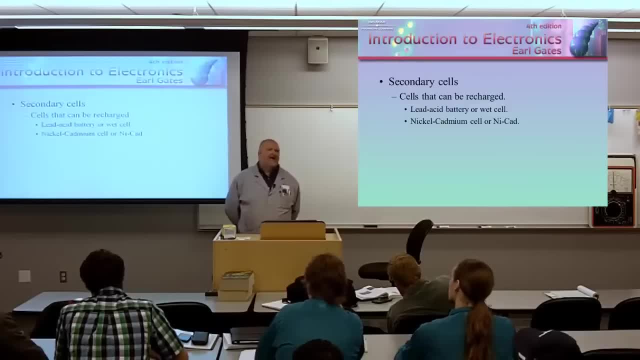 In the event that power is interrupted to the cell sites, automatically they'll switch over to battery backup. They're typically lead acid cells. That's what they use for solar systems too. right, Absolutely. And they use those for solar systems now because they're the cheapest secondary cell that's really on the market. 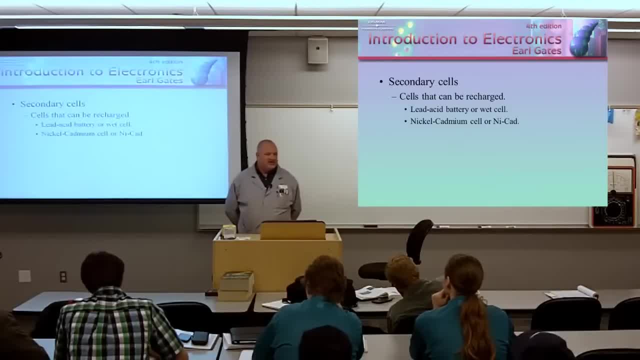 There's other technology that's more efficient, that's more, better, but it costs more. So if you just want to, let's say you live out in the desert and you want to run lights by day and harness the energy by day, and you need a lot of solar panels and you're going to need 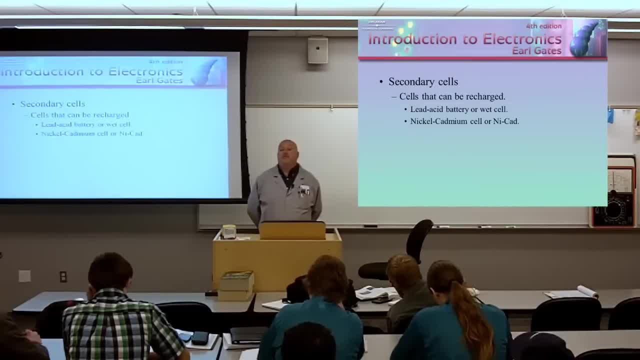 a lot of secondary cells. the cheapest secondary cells that you could buy are lead acid cells. My submarine had a whole bank of lead acid cells Located in the center of the submarine, down in the keel, the very lowest portion of the boat, And it was called, ironically, the 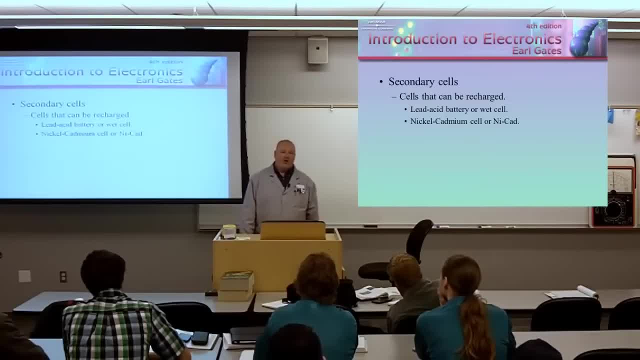 battery well, And in the battery well were batteries that were basically six feet tall and they were about this big around and they were individual cells And it took a crane to be able to lower these things in and move them all in, And then they had wooden 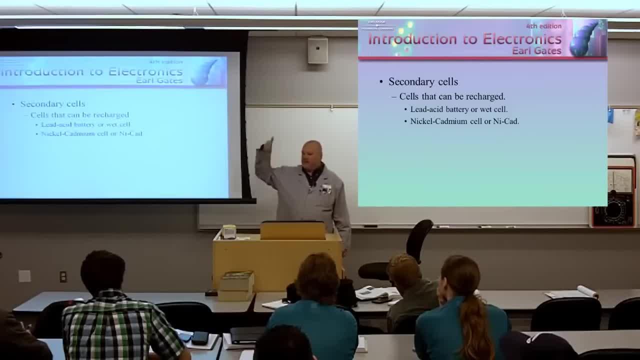 shims, Wax-impregnated maple shims were all put in between these and it was all one giant bank and they were all wired up Lead acid On a daily basis. an electrician would strip all the metal off of their uniform if they had a belt. 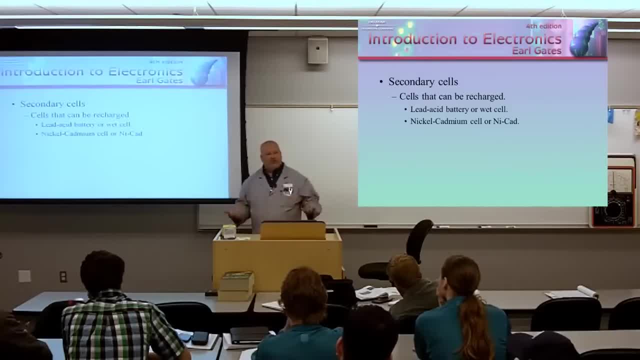 on or anything metal, And typically what they had is a special jumpsuit that they put on that had all acid burns in it, And what they would do is they'd have to climb down in the battery well, and they'd have to check the gravity. 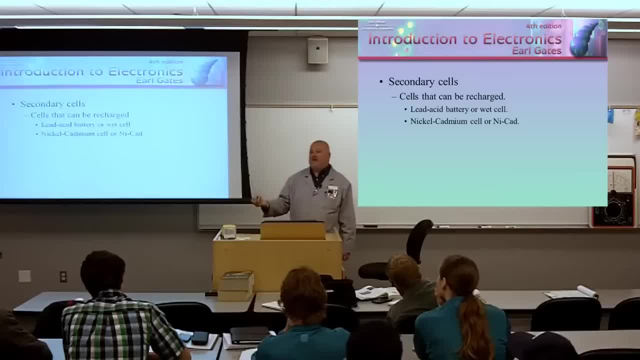 the specific gravity. This is the electrolyte fluid inside. And basically, when we charge a battery, what are we putting into a battery? Who said electrons, Electrons. That's really what we're doing when we charge a battery. We're putting free electrons, we're storing it in an 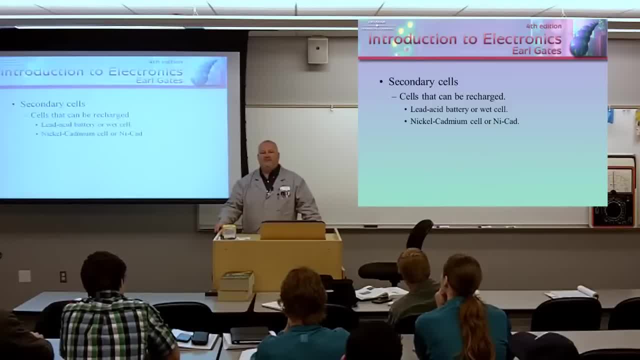 electrolyte solution, Are electrons matter? Absolutely. They're not very dense, but they still are matter. When you charge a battery, what you do is you increase the specific gravity of that fluid, that electrolyte fluid. So what the electricians would do on a daily basis is they had a clipboard and they had a 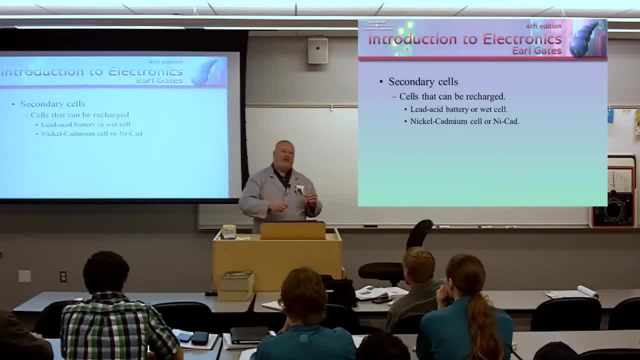 grid that showed all the locations of the battery They would go down in and they would check the specific gravity. You know what I'm talking about with specific gravity. Specific gravity is a comparison of the density of pure water, H2O, at room temperature, standard temperature, The specific gravity. 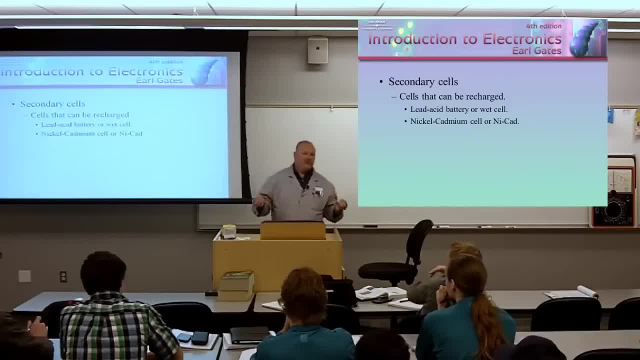 of H2O. pure water at room temperature. standard temperature is one One point: zero, zero, zero, zero, zero, zero, zero. It's one. It's what we compare everything else to. Now, if I have pure water and I start to get some salt and I dissolve salt into the water, what am I going to do? 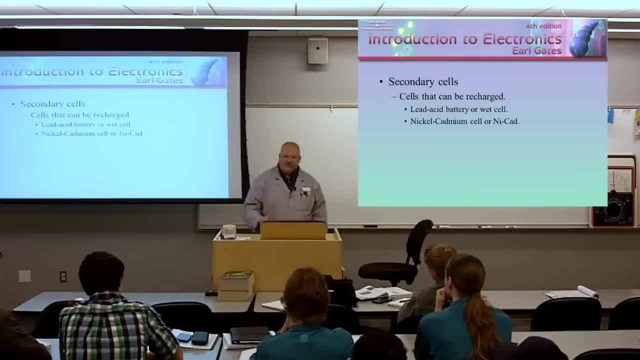 to the specific gravity. I'm going to raise it. I'm going to increase the density of the fluid and by taking a specific gravity reading I'm going to show that it's more dense. That shows me that I've done what. I've put matter into the 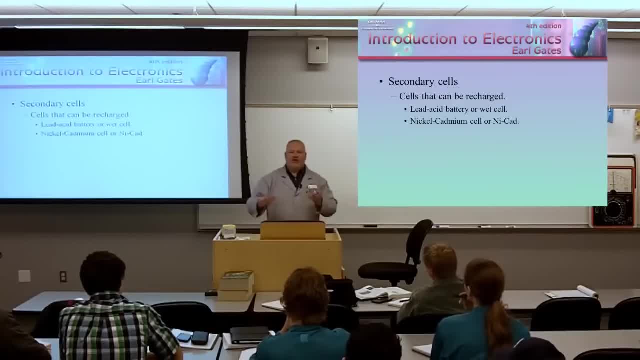 solution. If I dissolve sugar into it? same thing. If I pump electrons into it, what am I going to do? Same thing: I'm going to increase the density of it. I use specific gravity. I brew my own beer And I use specific gravity to tell me what the alcohol content is. 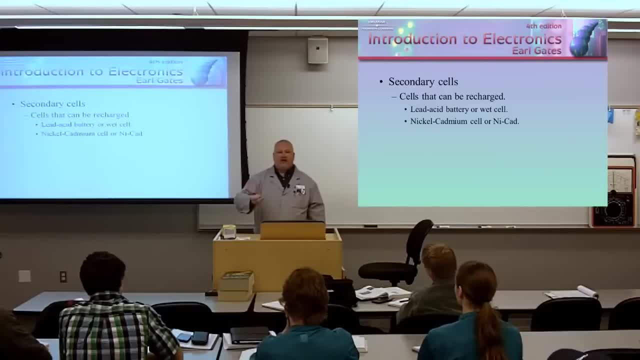 In the brewing process I basically impart a lot of sugars into the beer And I take that reading. The more sugars I put into the beer, the specific gravity increases, The density increases Make sense. Then what I do is I get yeast, I put the yeast into. 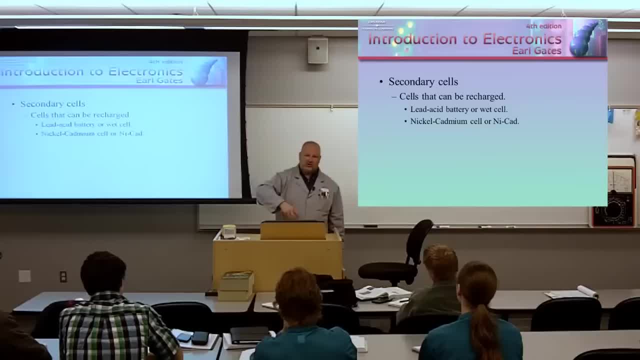 that solution and the yeast consumes the sugar, converting it into CO2 and alcohol. So after the yeast has done its job, I expect to see that specific gravity decrease because alcohol is less dense than water. And then I take my first reading. 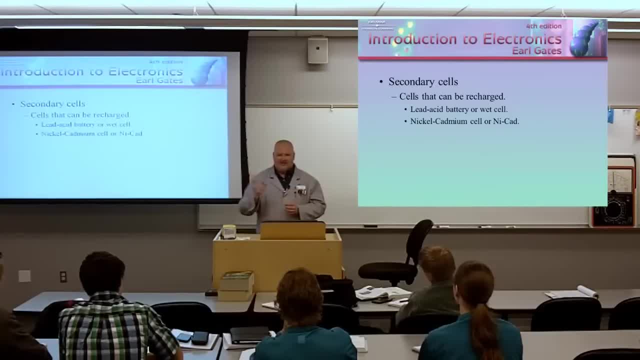 compare it to my last reading. That gives me my alcohol content of what's inside the beer For a battery. your battery in your car has six cells. If you buy a hydrometer and you test those cells, you should get consistency across all of those cells. If you don't. if this cell's good, this cell's good, this cell's a little bit lower, this good good, good, this cell being a little bit lower, you're probably developing an internal short in that cell. You need to replace your battery. 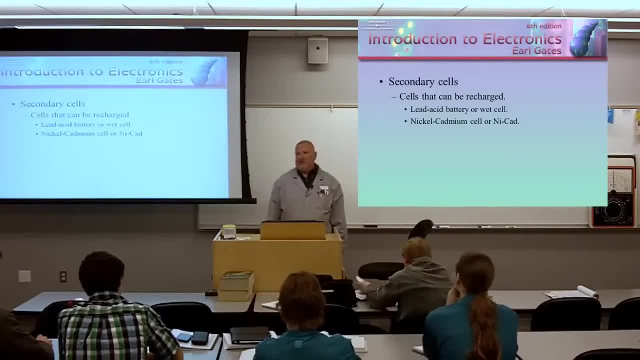 You can't just replace the individual cells, You have to replace the whole entire battery. So back on the submarine, they were really concerned about that on a daily basis. They sent somebody down in the battery well, to take those readings, because if they saw a cell that started to develop an internal short, 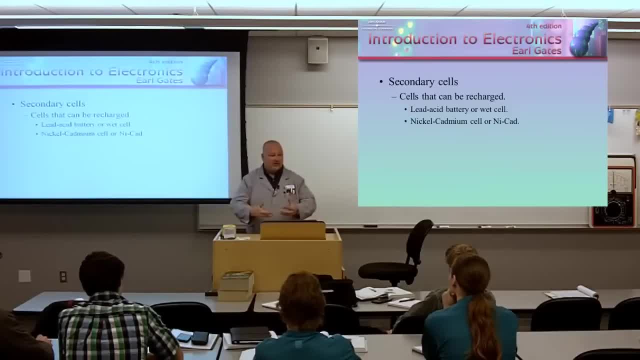 or a problem. conceivably it could take all of that energy and dissipate that energy through that one bad cell. That's bad news Because oh, by the way, you know why we had a battery bank: If our nuclear reactor shut down or we had a problem. 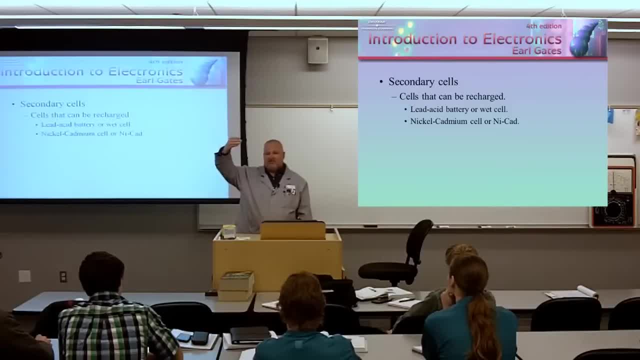 we could get to the surface. When we get to the surface, we could start up a diesel generator. So from that transit, from the deep up to the surface, we needed to be on battery power If you can't get the diesel started while you're on the. 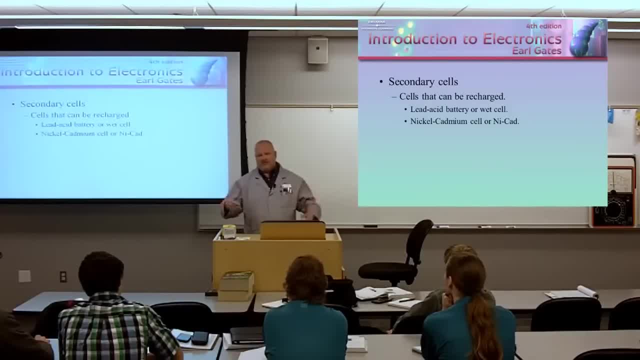 surface or actually at periscope depth, because we had a snorkel, they could just stick up where it's an induction system for the diesel engine run the diesel. We had a generator connected where we could keep not as much power as we'd have to nuclear power, but to keep all vital systems. 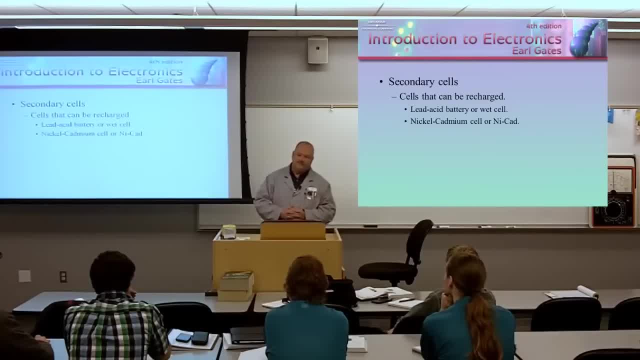 up and operational. Actually, I had a real scare once We were someplace we weren't supposed to be, Like, someplace we were not supposed to be Typically where we always went with my submarine, And it was a national holiday for this. 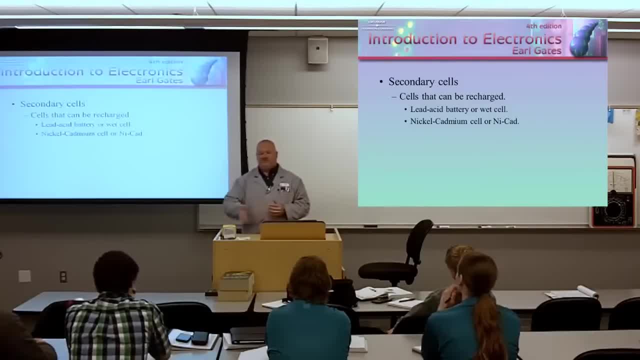 country. So all of their. you know they'd take their submarines and drive them through Red Square and their tanks and their missile launchers and everything, And you know we had nothing better to do So instead of like, hey, you know, we're watching the. 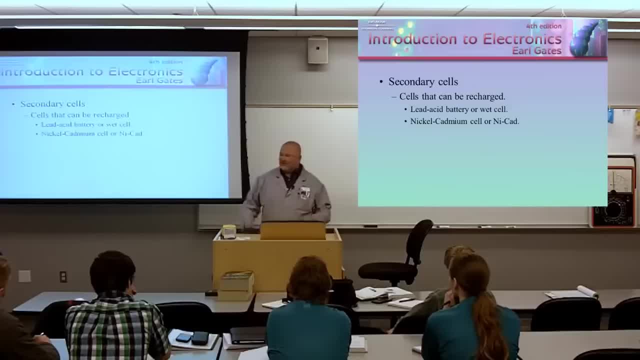 Soviets. They're having a holiday. Let's us have a holiday, Because on the 4th of July we're going to be watching the Soviets and they're not going to take into account our holiday. You know, the captain didn't think it was a very good idea that I had. 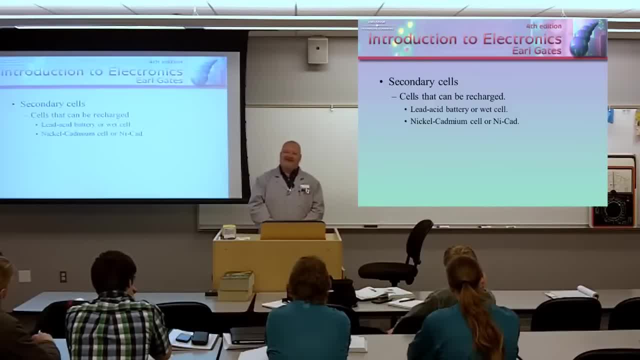 Now, as a matter of fact, Mr Greenock, I think what we're going to do is we're going to do some drilling today, You know, and it's firefighting, whatever. Well, we did a drill, an exercise that involved 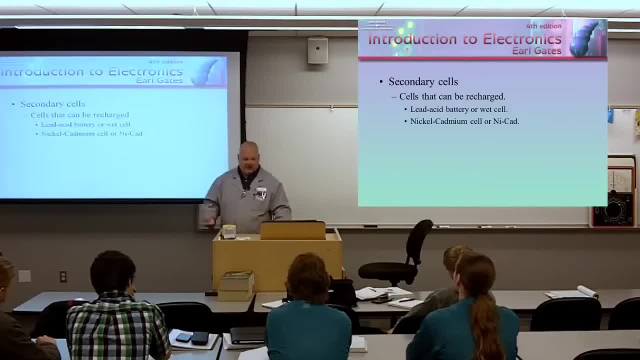 scramming the reactor Sounds ominous, doesn't it? Scram the reactor? Oh no, don't scram the reactor. Scramming the reactor is actually a good thing. Scramming the reactor is when you shut the reactor down. You have control rods. 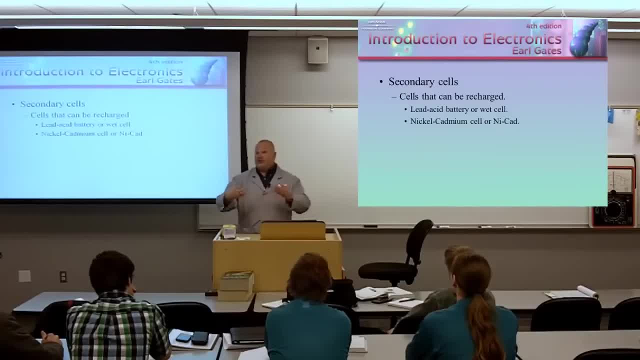 you move the control rods in, you neutralize the reaction, the nuclear reaction. This is actually what they did too in Japan After the earthquake. as soon as there was seismic activity, pow, they shut those reactors down, scrammed the reactors. The problem that they had afterwards was with the 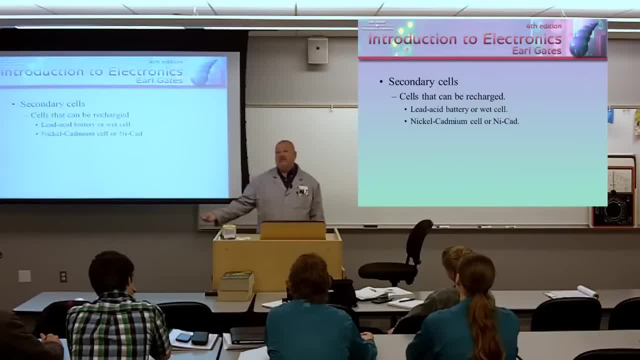 tsunami damaging. I suspect it was their intake, their seawater intake, used for cooling, and they couldn't dissipate all that heat that had already been generated, and then it became an avalanche, so to speak, of circumstances. Anyway, we're somewhere we're not supposed to be, and it was quiet. 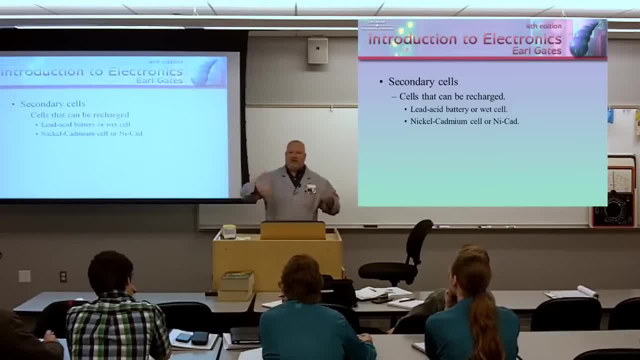 So the captain figures we're going to do some nuclear drills: scram the reactor, pow, scram the reactor. Normal procedure is we start to come up to periscope depth. make sure that we're not going to hit anybody up on the surface. come up, raise the snorkel mast, start the diesel generator. 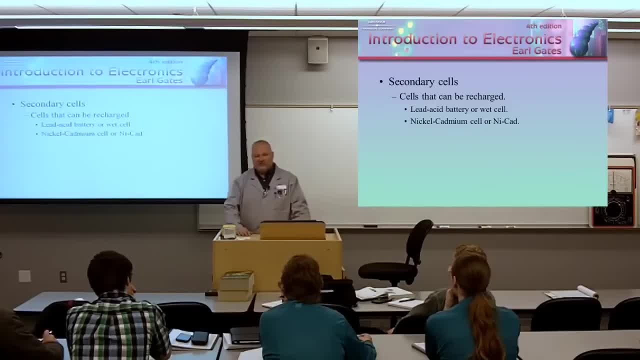 Well, they try starting the diesel generator, which is commonplace- wouldn't start, Wouldn't start. What had happened is there was this multi-pin connector that, for whatever reason, disintegrated in the back of the diesel control panel. So it's kind of like, well, that's going to take two days to put. 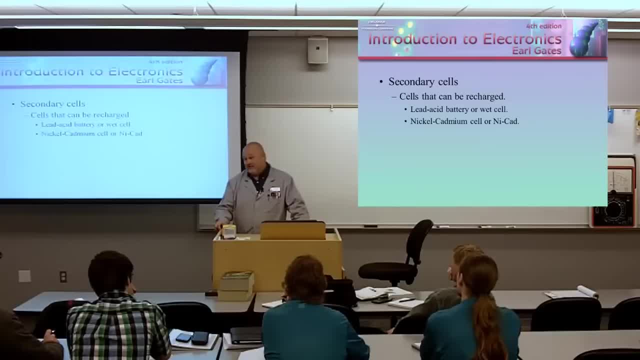 back together, you know. So we're on battery power. To be honest with you, we knew it was a drill and we were all real sloppy rigging for reduced electrical. That's where we shut down all non-vital systems And we knew it was a drill. so 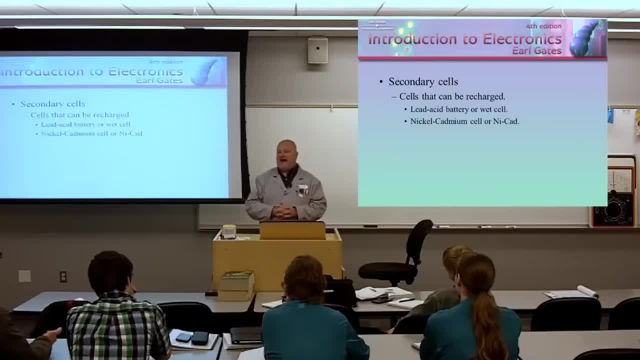 we were very slow in doing it. We expended over half of our battery energy in that period of time. So now, all of a sudden, the reactor shut down. we can't start the diesel generator. we've just consumed 50% of our battery power because we were screwing around. 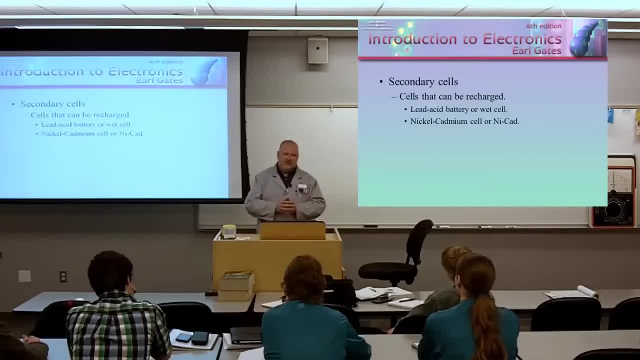 kind of dragging our feet with this exercise. So we realized what was happening and basically the decision was made: restart the reactor. Well, they try restarting the reactor and the reactor won't start And we've consumed all of our battery power. So now we went to this like super, super. 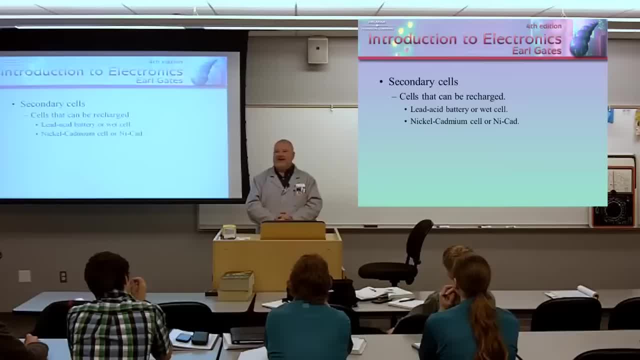 rig for reduced electrical where there's, like you know, emergency lighting and all the environmental systems are down. So the air all of a sudden is almost unbreathable and it's in excess of 120 degrees and it's humid and it's just miserable. Can't get the reactor started. 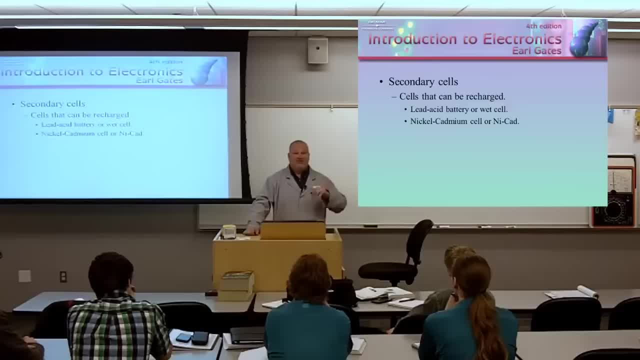 And in my job surveillance I was down to one receiver. I shut all my sophisticated stuff down and I'm down to one receiver. You can't make the story up. It's like: holy crap, Here comes the fleet. It's like: what are you talking about? Here comes the freaking. 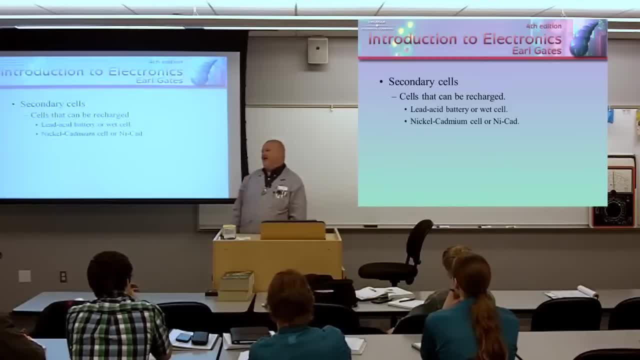 Soviet fleet and they're heading right towards us. I'm like you gotta be kidding. So it got really, really hairy, because this is the type of thing that, like World War III, could start over. What's a submarine doing in our harbor, you know, violating our sovereign territory. 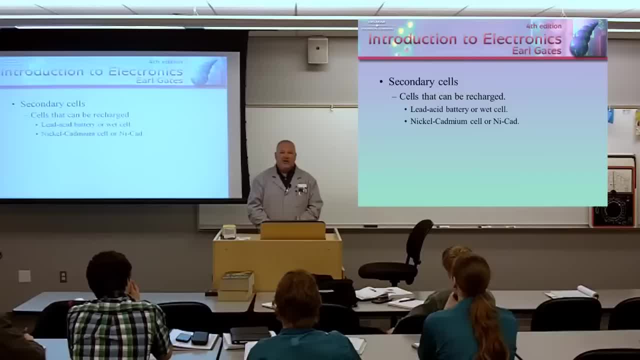 and all of this stuff. You know, we just couldn't get caught. Truth be told, they were able to get the reactor started. They had to kind of amend their procedures And come to find out it was actually a reactor control switch had failed. It was a series of circumstances. We called that. 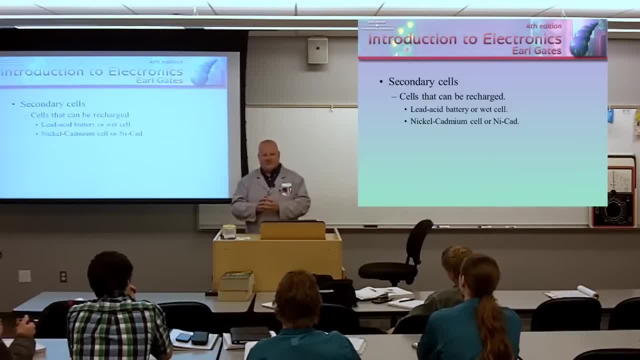 day anybody that served on the boat in that era, affectionately known as Black Tuesday, because things were really really bad And I had it good. I mean my space normally where I worked I had to wear like a foul weather jacket to stay warm because of all the air conditioning. 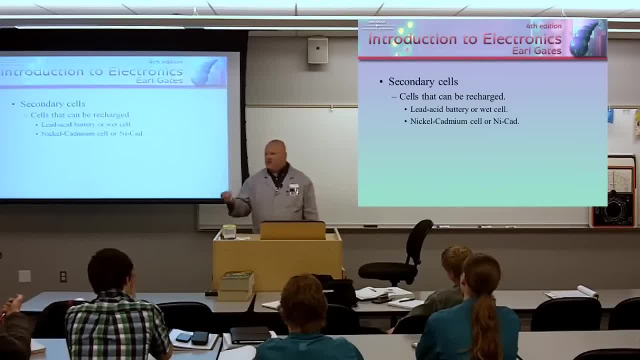 Of course, all the air conditioning was down. but I tell you what the guys in the engineering spaces, I mean they were stripped down to their underwear and no shirts and they were just sweat pouring. sweat pouring, I mean, it's temperature skyrocketed. 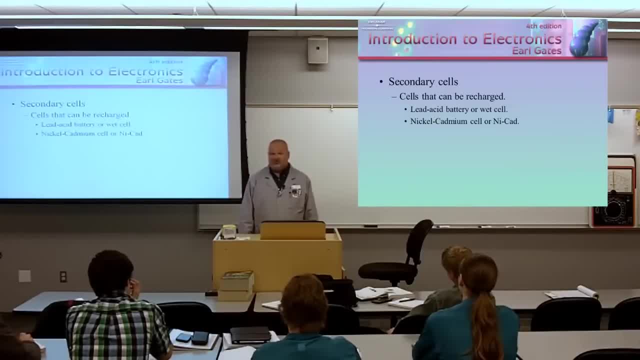 You know 150, 160 degrees back there in the engineering spaces and you're trying to troubleshoot something. But anyway, it all worked out good in the end. But that's the necessity, The necessity of a backup battery. Now a lot of you may be saying: well, I'm never going to go to work on a nuclear. 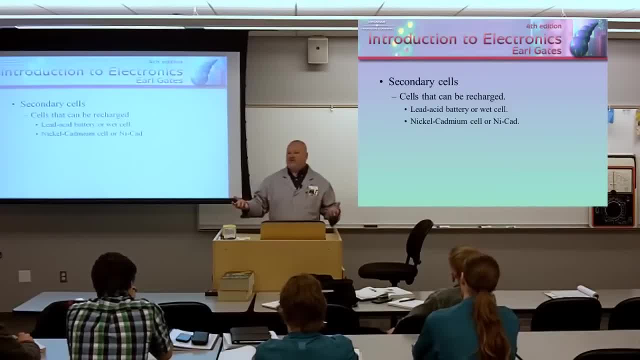 submarine or a ship or whatever. No, you might go to work as a biomedical electronics tech at a hospital. Guess what hospitals have Backup battery banks. You might go to work for the Federal Aviation Administration, Federal Aviation Administration, down in Auburn, Washington, at the Mountain Region. 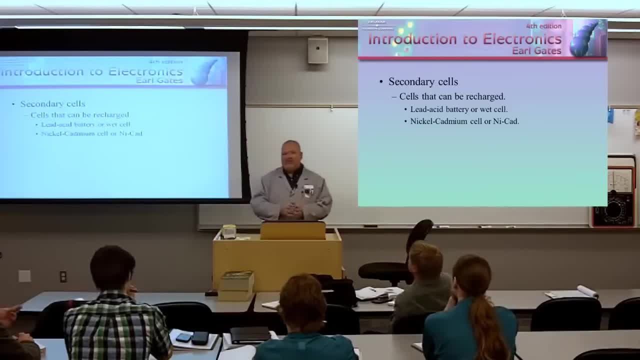 Air Route Traffic Control Center. I don't know if any of you are aware of that facility. If you go to like the Muckleshoot Casino down there, it's like right across the street It's a big building, Fences around it, armed guards, all kinds of stuff like that. That's where they control. 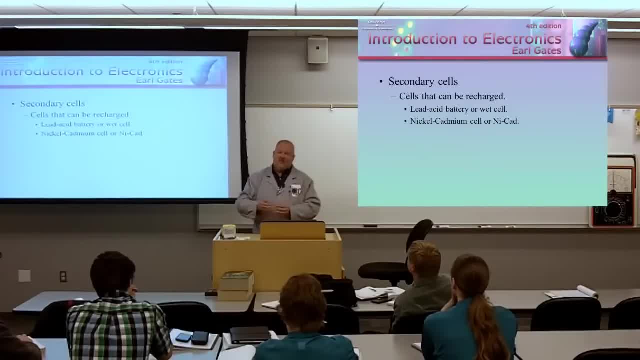 all the air traffic in the northwestern United States, From western Montana to the Pacific Ocean, from the Canadian border all the way to northern California. If you're an airplane in flight, you're talking to somebody in Auburn Washington. They lose the power at that. 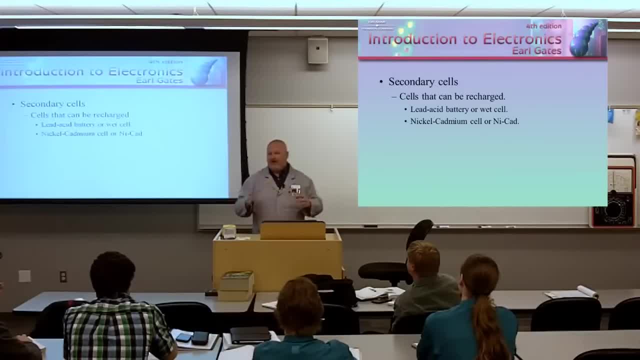 facility. guess what? The whole northwestern United States aircraft are flying blind. So they were kind of smart about this. They put in a battery backup system. So as soon as the power AC crashes, these batteries have power inverters and that brings it back up online. 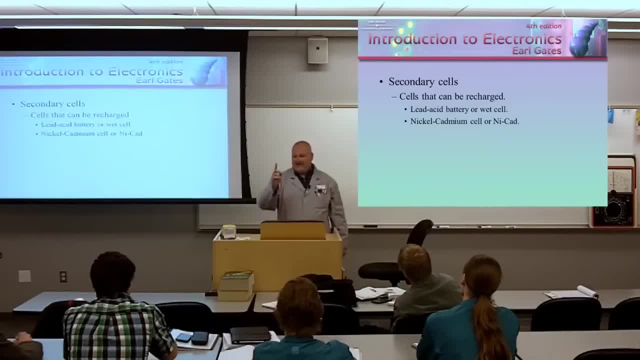 so they don't miss a beat. Once the batteries are up online, then they have diesel generators in another building on the property that will go ahead and kick in and have huge fuel tanks so they can power that for a very, very long period of time. If any of you have ever heard of the news in the past- a lot of 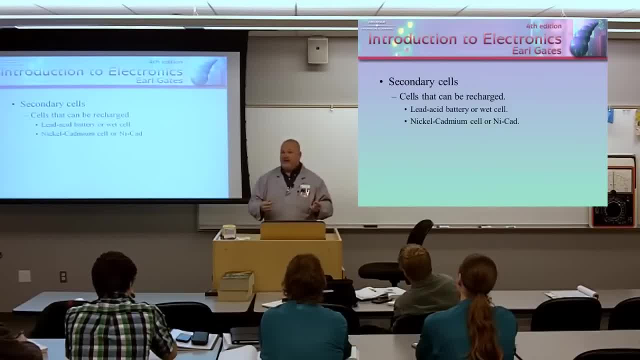 times if they have a glitch, like in the air traffic control system, switching over to backup power. that's actually what the problem is: is going from AC to that battery backup. If it doesn't happen seamlessly, all of those systems go down. You all know, with computers you've got to reboot computers, so you have aircraft. 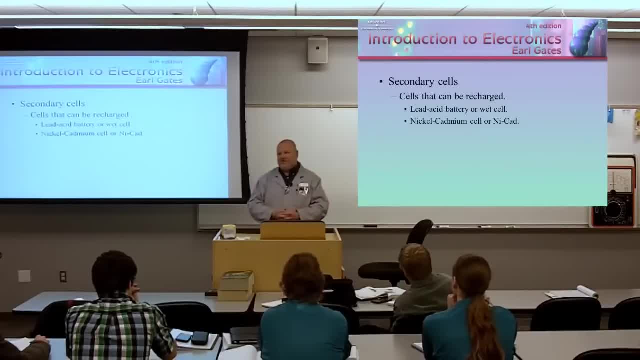 flying blind without air traffic control for a period of time, So it could be somewhat of a inconvenience Safety concern. So a lot of you are going to see this Actually one of the most reliable systems and this is- I don't know how many of you still just have an old fashioned 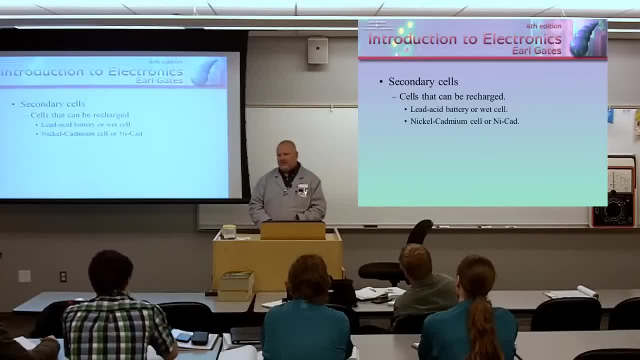 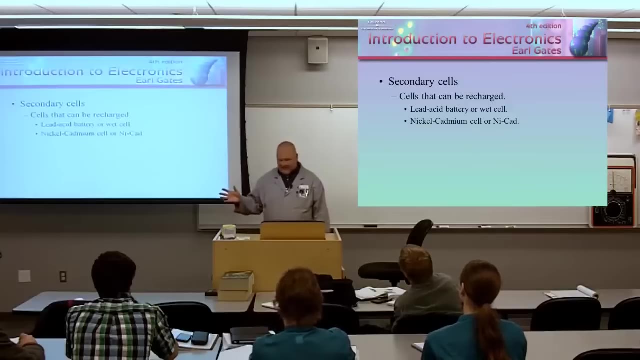 telephone line to your home. POTS is called and basically what that is is an old school just two wires coming to your home. Most of us now are on broadband and voice over IP and all this kind of crap. The old school telephones were the most reliable. You could have a power outage. 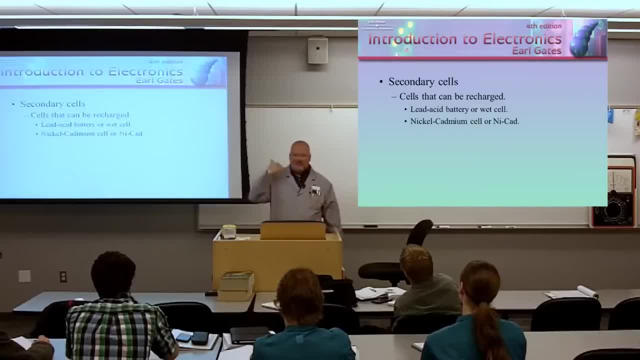 you could have earthquake, whatever, and you pick that phone up and you're still going to get a dial tone, Because that dial tone is being generated by backup battery banks at the central office And that's powering the phone system. So I've experienced a lot of blackouts. 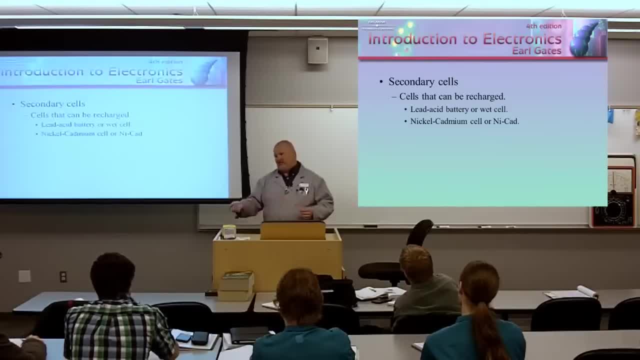 in my life where the power would go out, and I never lost that dial tone on the phone. Now, how many of you are like with Comcast? I mean, what was I thinking when I went to Comcast, Actually, believe it or not, I'm not just talking the talk, I'm walking the walk. 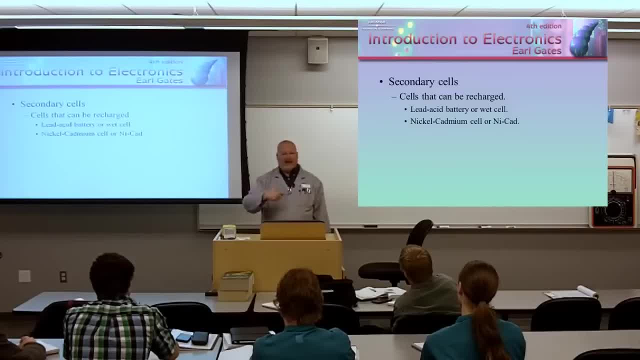 Before I came to work today I actually called Quest. I want to get an old school line back into my house Because I'm looking at my phone bill, My freaking phone bill. I don't know if I'm paying like 70 bucks a month for caller ID and call waiting The only 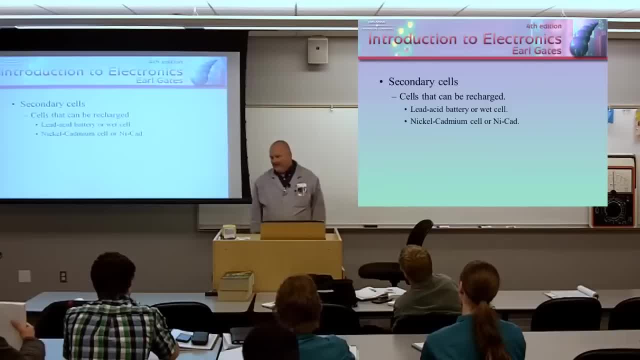 people that call me are people that I don't want calling me. Okay, So why am I paying 70 bucks a month to have something that I don't want, And I don't want to shut the line off because I have some other uses for that line. So I called Quest and I'm like it's kind of an unusual request. Do you have any of the old school lines that I can still have? Yeah, yeah, yeah. And how much? $13.50 a month plus tax. I'm like that's what I want. Can you port my existing number back to it? Yeah, no problem. So I'm going to get that scheduled- $13.50 a month, No long distance or anything, but I don't want it for that. I want it for that 911.. I don't know why I'm going to disconnect the ringer Because, again, the only people, people that want to call me, they call my cell number. But I still need that. If you have an alarm system at your home, you need it. If you've got. 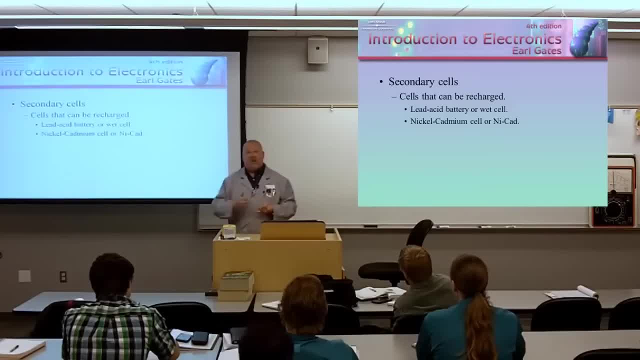 a satellite TV box for updates and pay-per-view. you need it So it could call into the mothership on a daily basis. So battery backups are still out there. So I don't think you're not going to go to work in the industry and never see a battery backup. 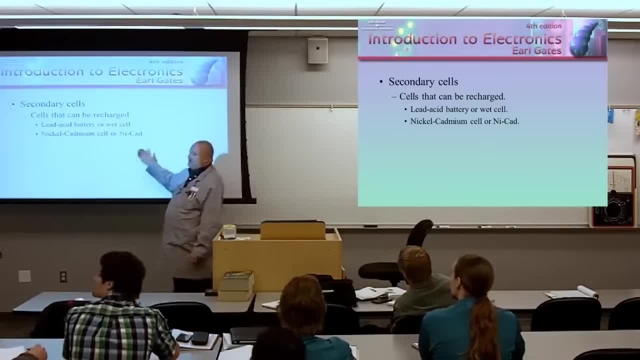 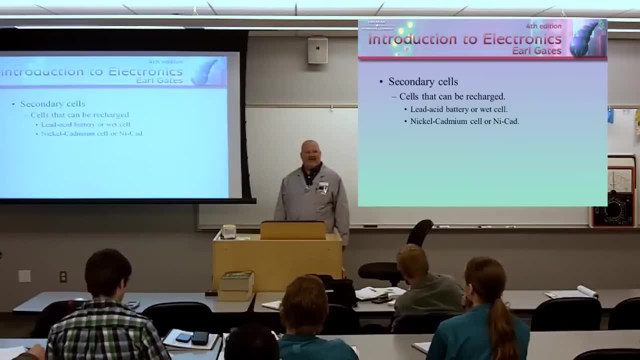 Now, you're all familiar with lead acid, Nickel, cadmium, ni-cad. How many of you are familiar with ni-cad batteries? Ni-cad have been out for a long period of time. Ni-cads had a nasty habit of generating what was called a memory, And what that memory? 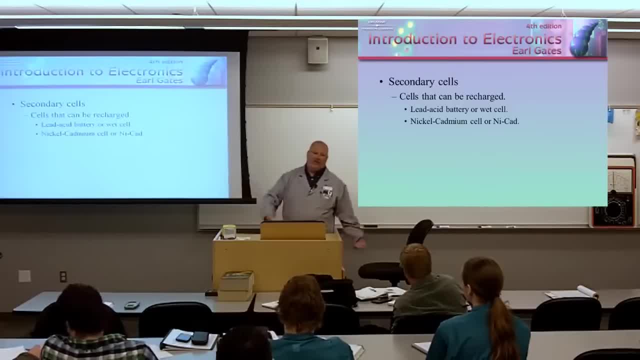 was in essence is if any of you have ever had your arm or leg in a cast and you don't use it. basically, the muscles forget how to fully exercise your range of motion. You've got to go through some therapy to get your arm working again, right? It's kind of the same thing with a ni-cad. A ni-cad, if you didn't fully discharge it and then fully charge it, it would only think that its range was in this narrow margin of performance. So the problem with ni-cads? 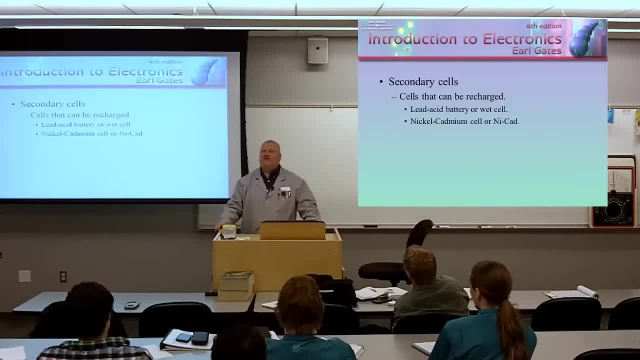 with, like camcorders and cell phones, where as soon as that voltage started to drop a little bit, you start to get the low battery indicator and to preserve the electronic integrity of what you were doing, it would shut off. Then you'd get it, stick it in your charger. 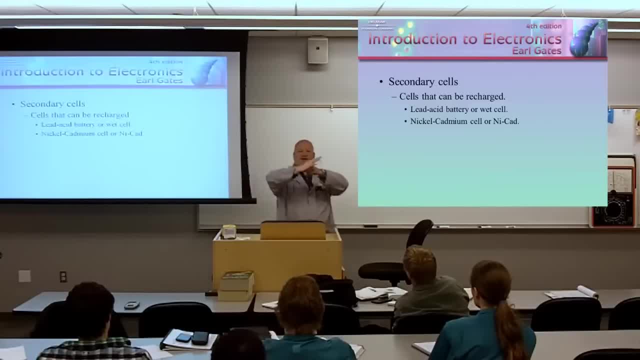 charge it back up. and what would happen? It would only get used to operating in this little realm right here. Some of the manufacturers got smart and they put a little button on there and they could connect it to a load and drag it down. 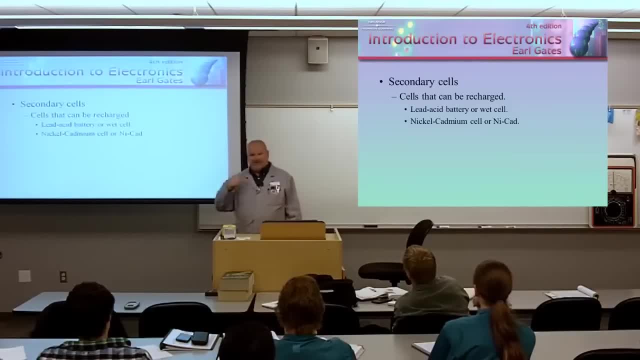 all the way and then recharge it all the way I've gotten- because I understand this stuff. I've gotten exceptional, exceptional use out of ni-cad batteries When my kids were growing up, my first video camera back in the 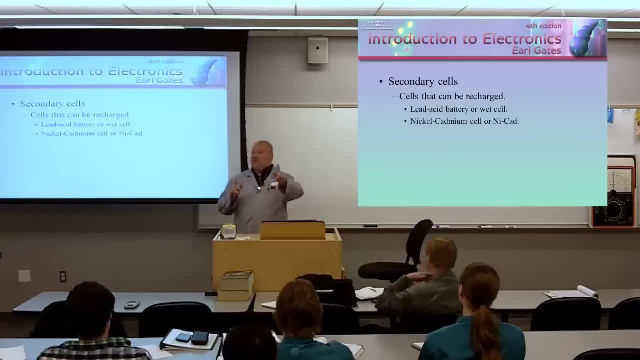 1980s I had one of those big VHS units- Don't laugh, It was VHS. At least it wasn't beta. It should have been beta. Beta was better. but that's another story for another day. But it was one of these big hurricane VHS, you know. 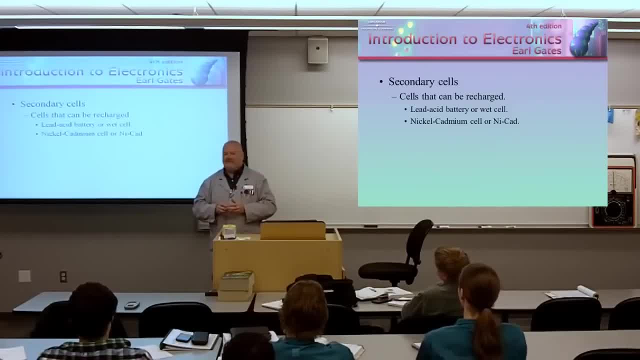 And it took this big 12-volt battery pack and I went to replace it and I was looking at some different vendors and they were looking at me and they couldn't believe that it was the original battery pack. It's like we don't even carry replacements. 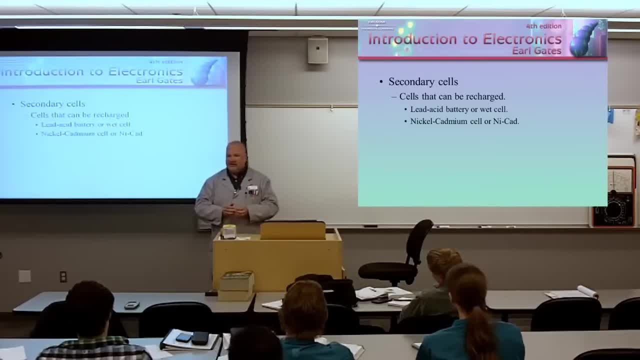 for those anymore. You know how long have you had this? Uh, since the beginning. Well, you know how could this be? It's because I understood how to take care of ni-cads. What I did is I made myself a dummy load, and 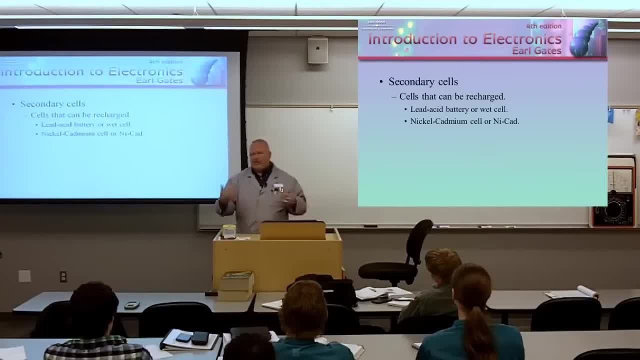 when the battery got low, you know. I mean, obviously if it was a birthday party or something that I wanted a video, I could recharge the battery, But at least on a regular basis. I would discharge it all the way and then 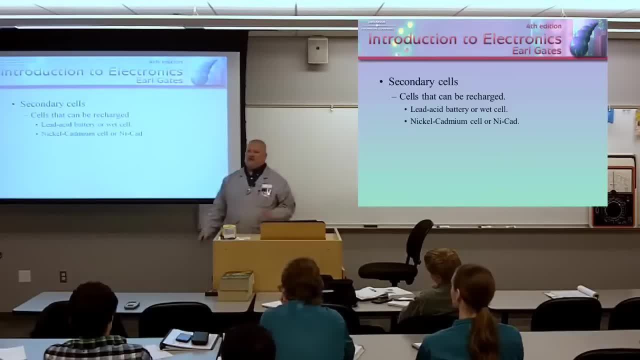 charge it all the way And, by the way, with nickel, cadmium cells. when I say charge it all the way, that doesn't mean slap it in your quick charger, Like, if you I've got a cordless drill at home, a Makita, I got a quick charger for it. Worst thing you could do. Mine still works. but you know, all those quick chargers work. They actually have a temperature sensor in the battery pack. When the battery starts to get hot it must be full, So it cuts the battery off. It's not a full charge. 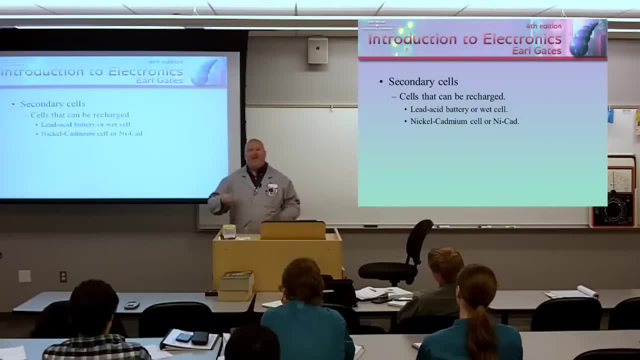 The only true method of charging a ni-cad properly is a timed charge, A trickle charge, where you're trickling in a known amount of current and then you bring it gradually up to that 100%, Not slam it, and then the thing gets hot and then shuts off. Some of the early ones. once it would stop charging, it would cut it off, right. And then what would happen? when the battery cooled down, It'd start charging again, And then it would get hot and shut down. So you ended up with this cycle in it. These were the real cheap. 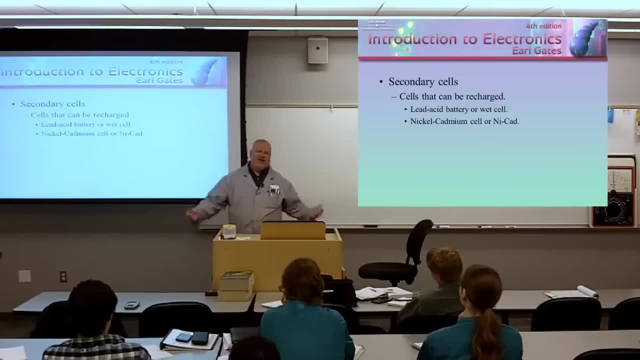 chargers and those would just eat these ni-cads. So if you know about ni-cads, ni-cads weren't that bad, They really weren't. The next thing was nickel metal hydride. Nickel metal hydride. 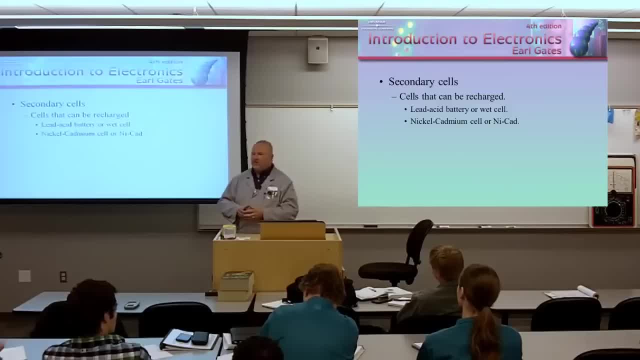 That was the next evolutionary process: Rechargeable batteries, secondary cells. A lot of us had them years ago in our cell phones. Worked very, very well. Less prone to that memory condition. With all these secondary batteries, though, is it an unlimited number of charges, and 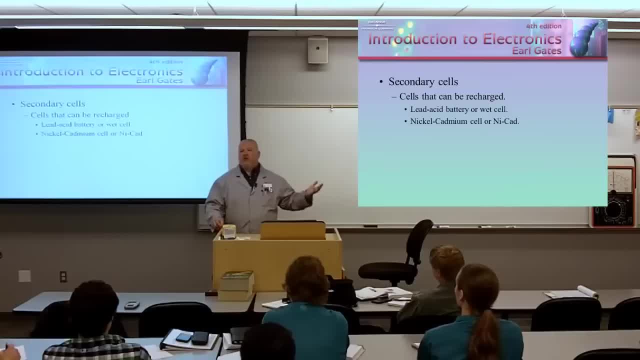 discharges and recharges. No, Every rechargeable battery when it's brand new. you only get so many cycles out of it. They're not gonna last forever, Even if you take good care of them. And then now lithium ion, Lithium ion. If you've got a newer cell phone, probably came with a lithium. 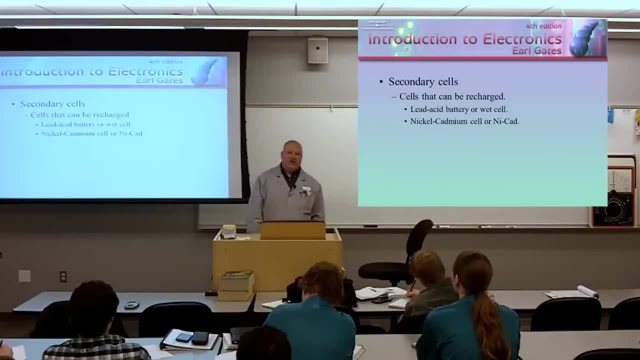 ion. That's really the best that's out there now. I don't know. I was just I don't know. I was thinking about that the other day And I've actually got a new battery put aside that I've never charged yet. 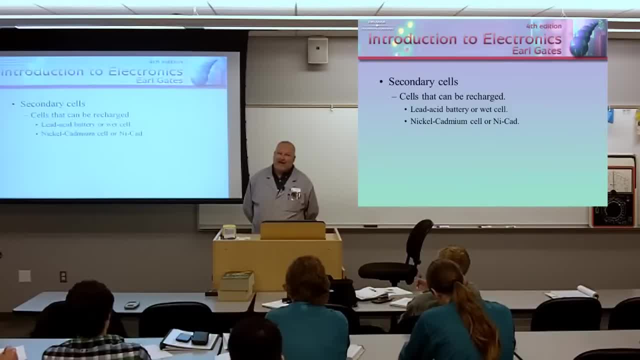 It's still in the package. So, um, I don't know. I've been keeping my eyes open in a store for that style pack And I'm sure it's available on the internet, but what am I gonna have to pay for it? 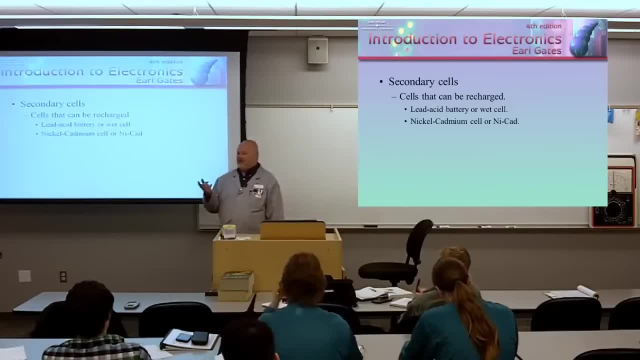 You know The other thing, though, too. check this out, Cause you know I'm not the smartest guy, but I kinda understand some of this stuff. Some of those cases you could actually cut them open and you could replace the cells yourself. 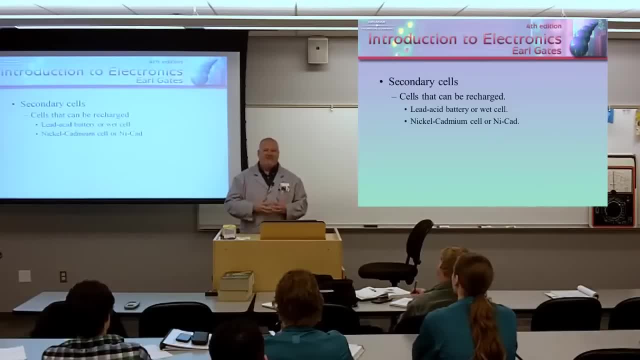 You know, And then re-bond the plastic back together And I've done that on several things myself as I've reconditioned, put in new packs. I had a, I had some, I forgot what the heck it was. It took NICAD batteries. 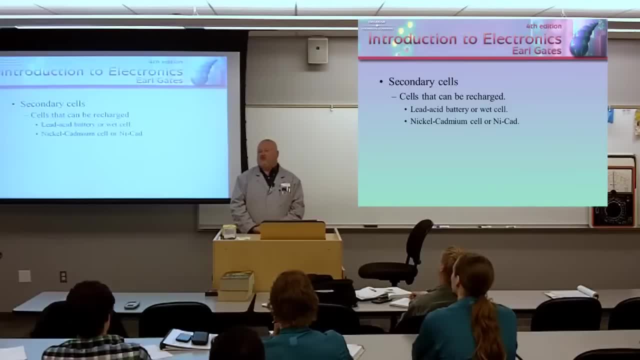 And then what I did is I cut it open and, uh, it was just standard, uh NICAD batteries. Usually it doesn't have the label on it, But the sizes were the same. And then what I did is I went to Harbor Freight. 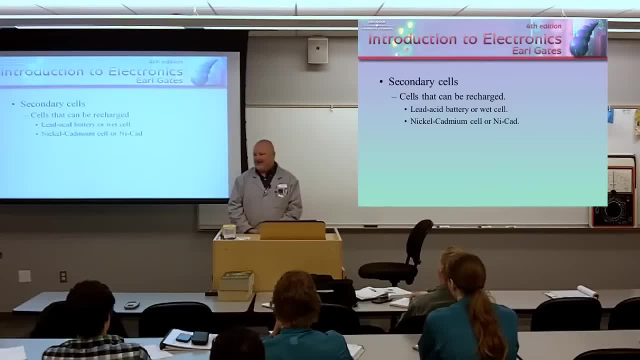 Tools. I bought nickel, metal hydride, rechargeable cells And I put the pack back together, soldered it up. Good to go, Good to go. So in some cases you could do that. A lot of high performance things too, even like jet aircraft. 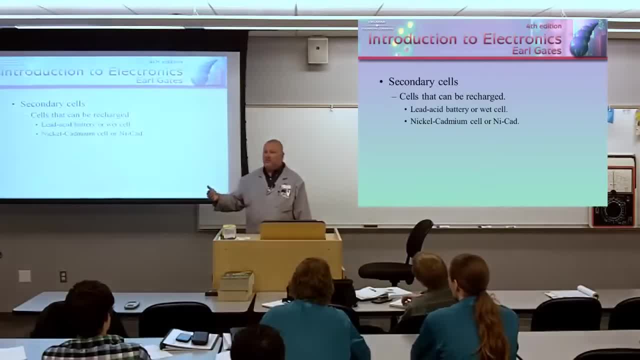 If you're down driving past Boeing Field and you see a Learjet sitting out there, believe it or not, what they're typically gonna use is not the lead acid. They're actually gonna have NICAD packs. So when they start the engines on the jet, 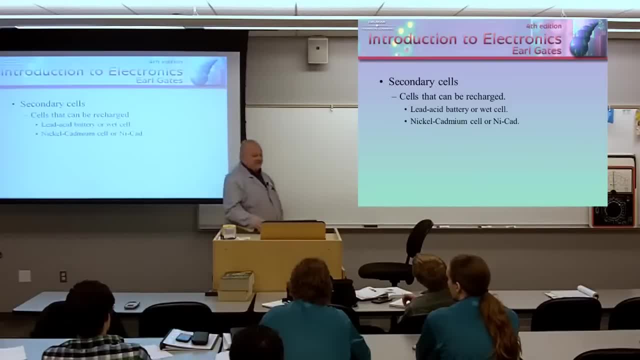 they're starting it off a NICAD, And those are very, very expensive. So it's kind of amazing. You're a multi-millionaire flying around in a Learjet. A lot of times you know what those guys will ask for: They want a starter pack. 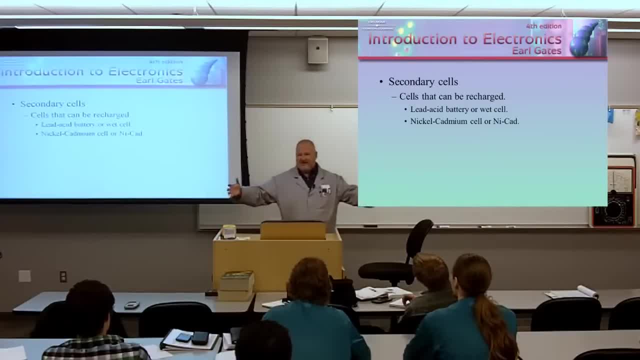 to be brought over with a little tug And there's a cart with a bunch of batteries on it- Lead acid batteries- And then you plug that into the aircraft And then what they'll do is they'll use that so they don't have to put a. 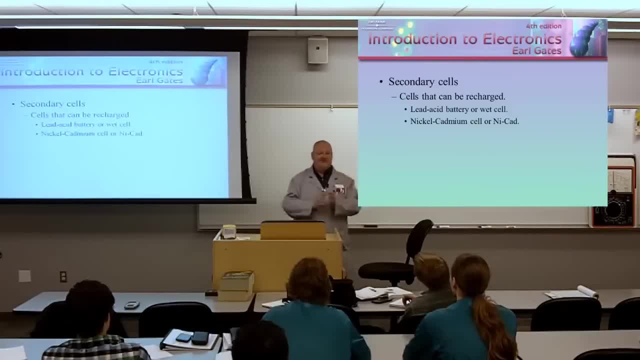 charge-discharge cycle in their NICADs, in their precious Learjet. It's like man: if you can afford a freakin' Learjet, you can afford a new freakin' NICAD. You know I used to work part-. you know the funnest. 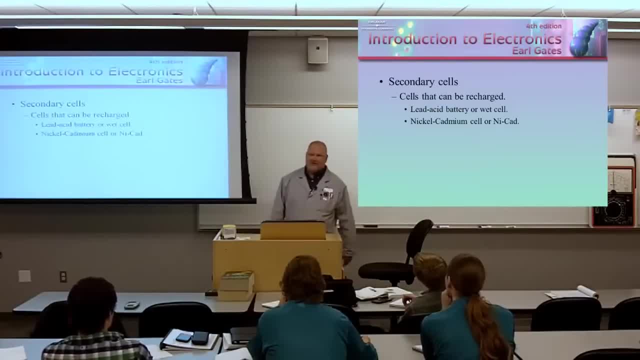 job I ever had. I worked part-time at an airport in Connecticut And those guys always used to amaze me And a lot of them would tip: ya, You know, you bring that pack over or whatever, and here you go. Go buy yourself a good lunch here, son. Oh, thank you sir. 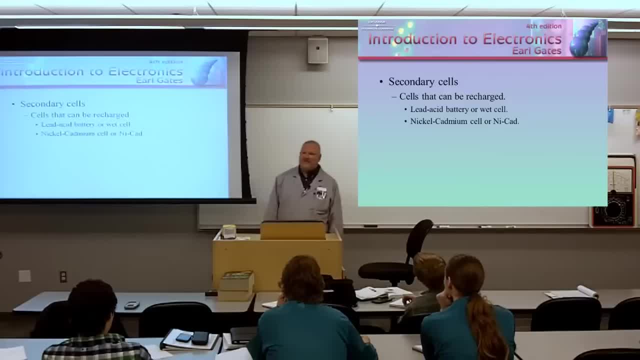 You know, I didn't mind Somebody's dude. So, man, I'm saving you money. You're not even tossing me a bone. Come on, man The heck. Next time I'm gonna park ya out there. This is the cutaway view of a lead-acid cell Now connecting. 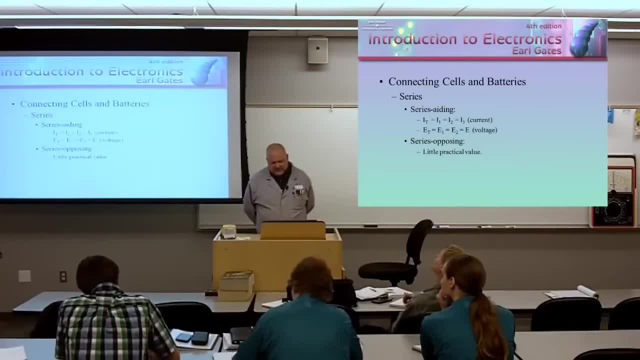 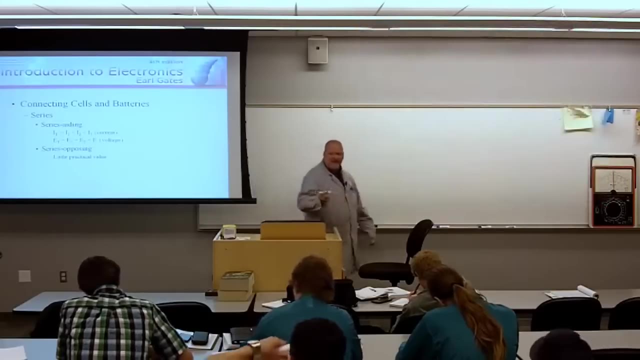 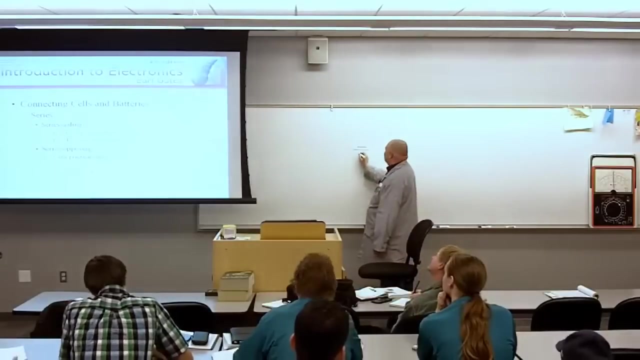 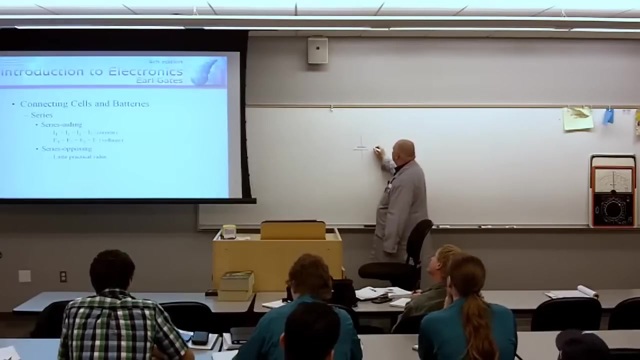 cells and batteries. Connecting cells and batteries. We have series-aiding. This chart here is erroneous. Let me draw this on the board here. what we're talking about here, Series-aiding means negative, positive. I can assume that this is what voltage: 1.5 volts. 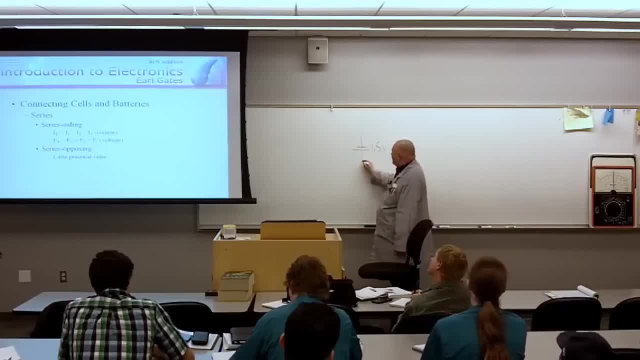 1.5 volts. So if I connect it to another cell, I can assume that this is 1.5 volts. And if I go ahead and even connect the third cell down here, I can assume that this is 1.5 volts. What am I up to, right here? 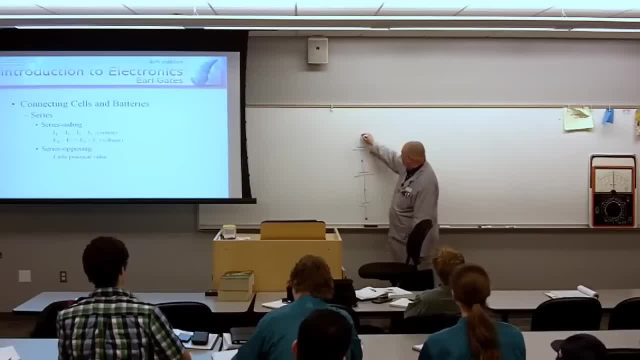 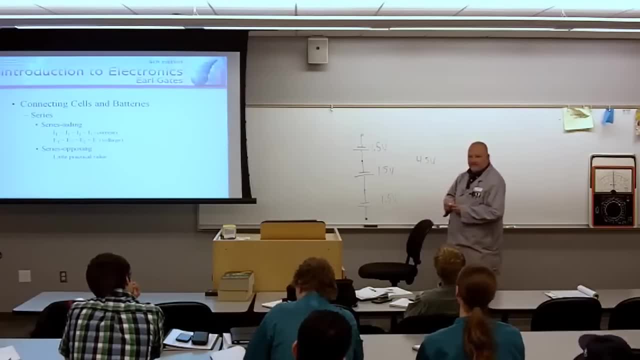 What's my total voltage from this point to this point? Okay, very good, 4.5 volts. Does everybody see that? Everybody see that. So what I'm doing here is, by series- in series-aiding, I am increasing. 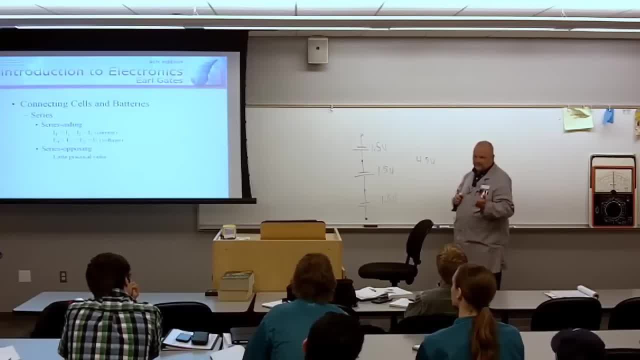 the electrical pressure that's available to me. The amount of current that's available here is going to stay the same, because this is what we call a series configuration, And current will always stay the same in a series configuration. So, by connecting up batteries or cells, 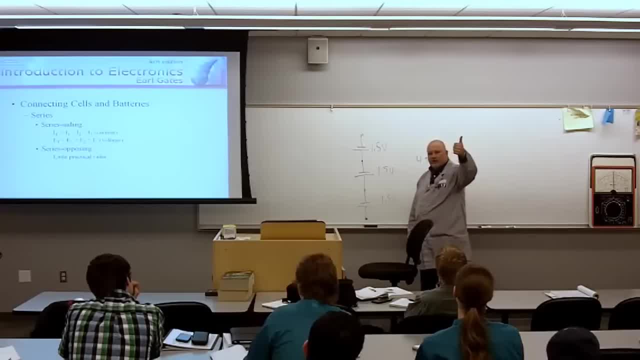 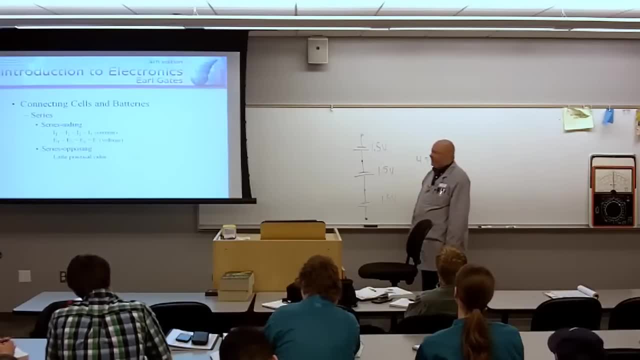 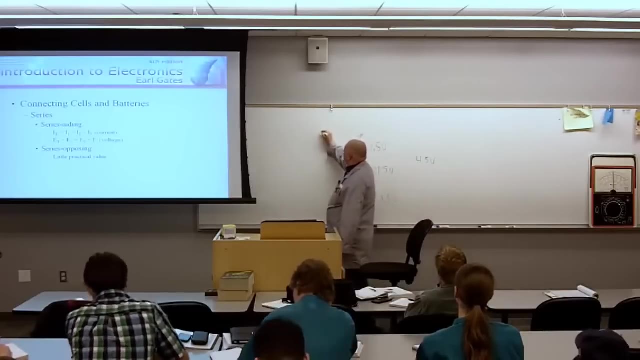 like this: I can get a higher voltage, but current will remain the same. Does that make sense? Now, down below, it talks about series-opposing. Series-opposing would be like: okay, I've got a negative and a positive here You all agree with. 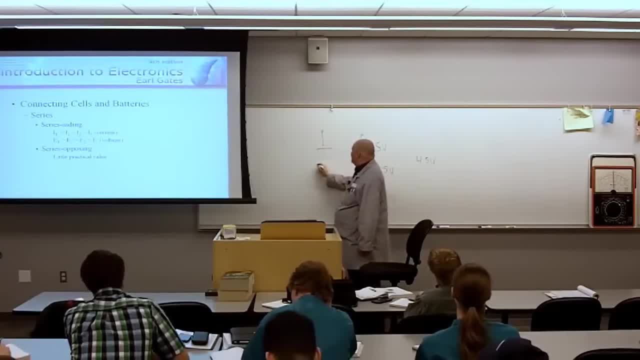 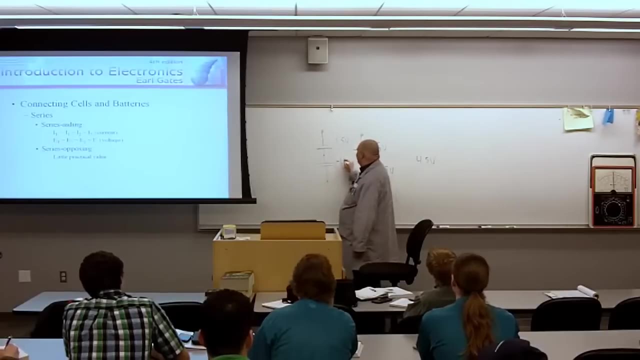 that. Then I'm going to connect a positive and a negative here. So I've got 1.5 volts here, and how many volts do I have here Minus 1.5 volts? So what's my voltage across? 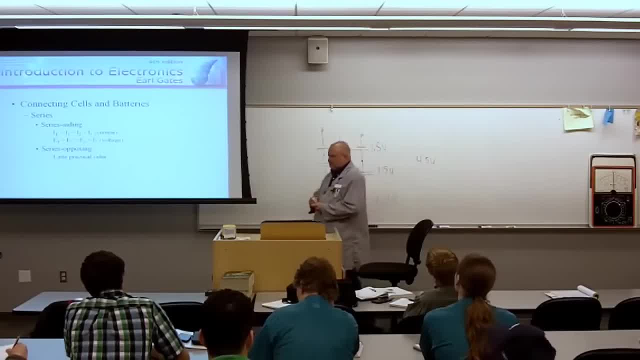 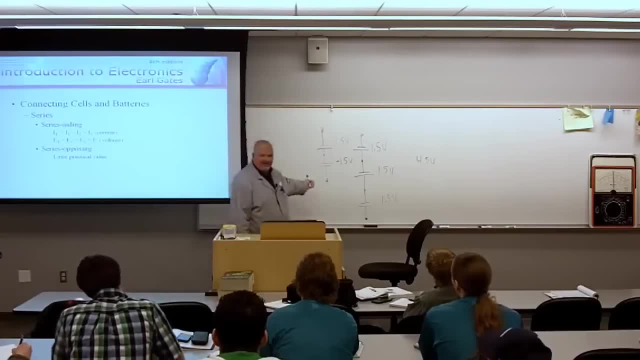 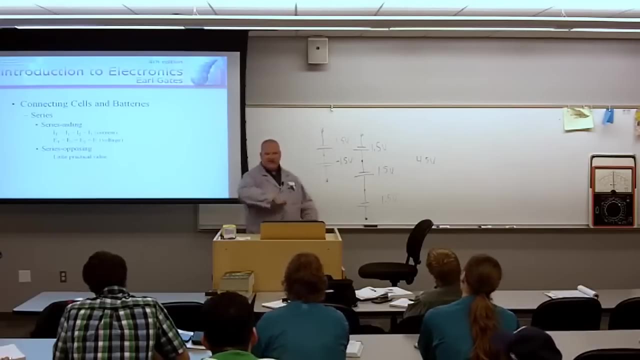 Zero. So my slide, which is politically correct, says it has little practical value. It's actually stupid. This is like you know. you're putting a battery in backwards. Why come my flashlight no work. And you take them out and you realize you put in one of the cells backwards. 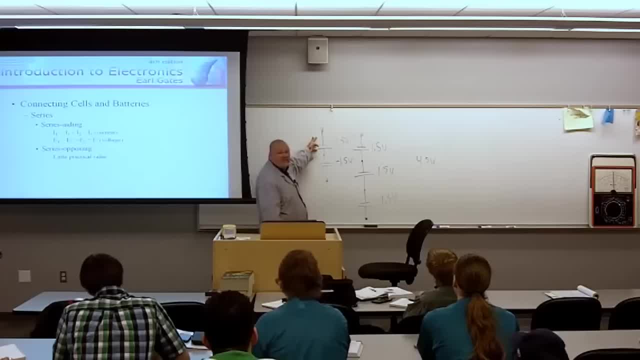 Has little practical value. This one's adding 1.5 volts, This one's taking 1.5 volts away. You're putting a negative and a negative here. Current's not going to want to flow. Again, it has little practical value. 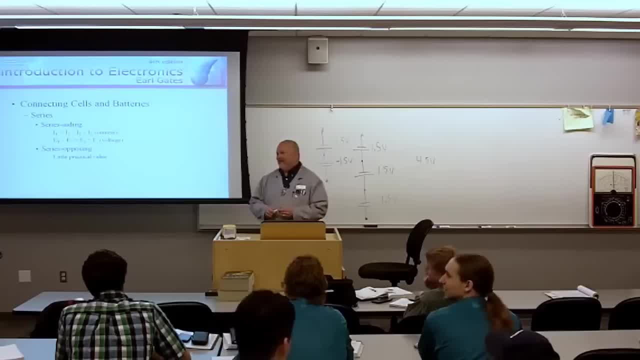 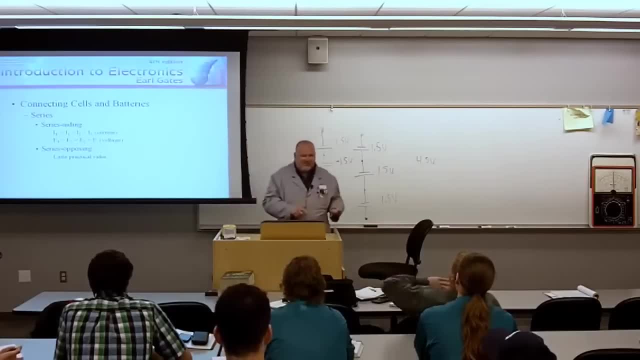 Yeah, challenging electronic students when they're going through a theory course like this. It really is, Because I could draw like five or six of these and you got a- let's see, plus 1.5,, plus 1.5, minus. 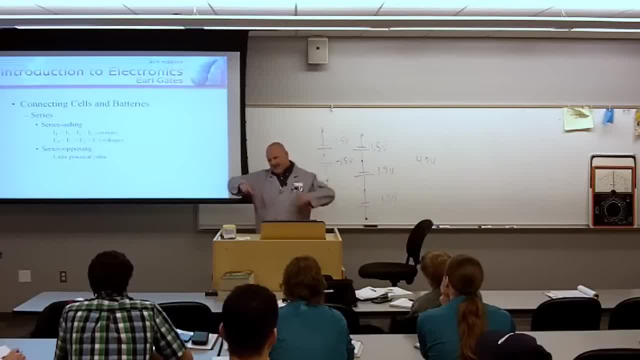 1.5, minus. So we are going to give you some problems like that that have voltages, Because, quite frankly, when you do get into sophisticated electronic equipment, you're going to see that there are some voltages that are being. 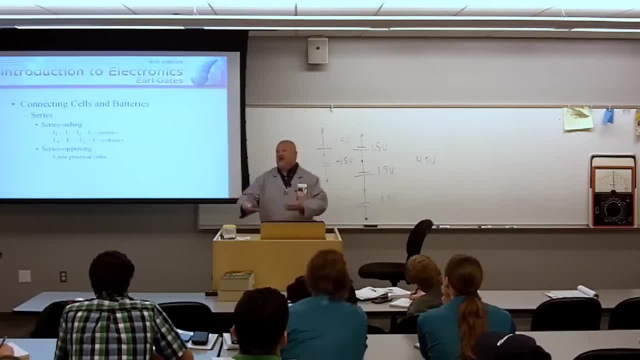 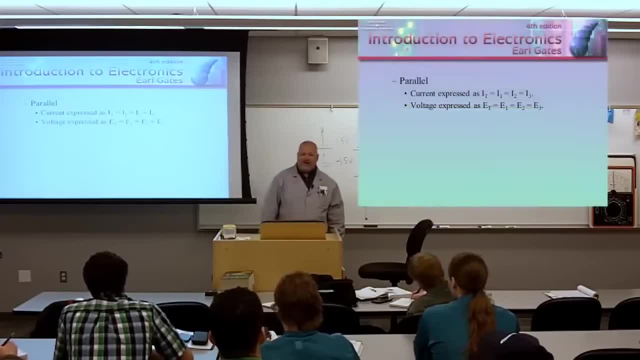 added to a circuit and some that are being taken away from a circuit. So from a math standpoint, a theory standpoint, it does have value in studying it In parallel. and again, this is a typo here. These should not be equal signs. 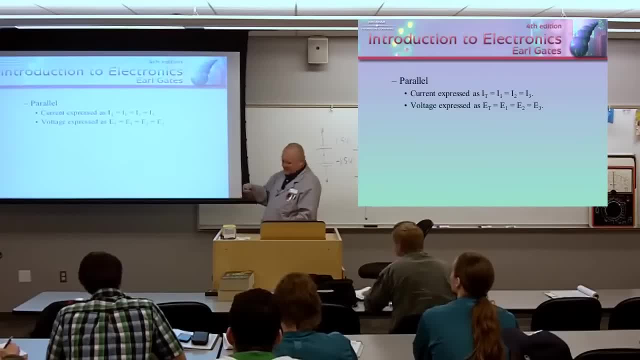 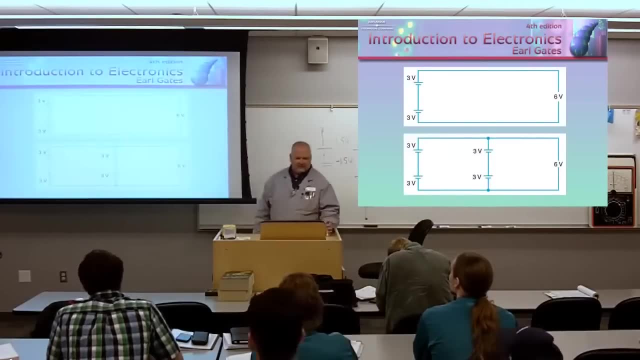 This should be. total current is equal to I1 plus I2 plus I3.. Let me show you this one. Actually, let me just go to the next slide and I'll show you on the slide. This is what we were talking about. 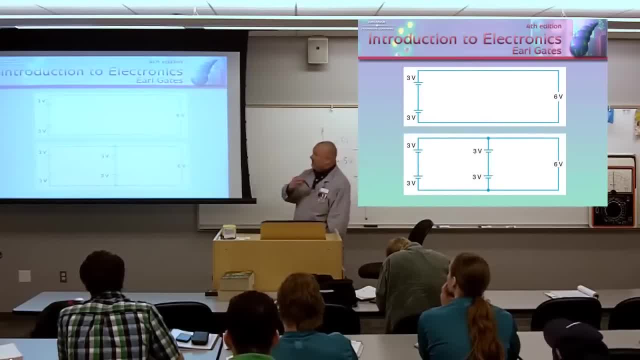 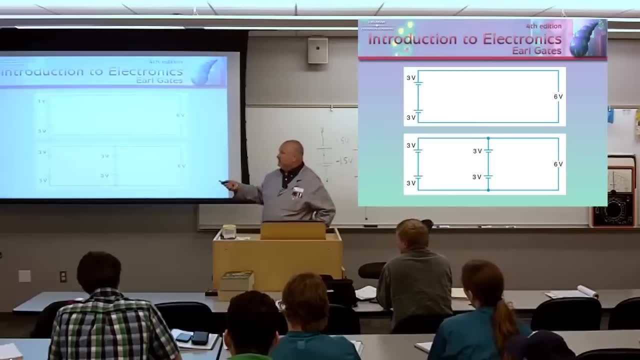 This is what I was talking about. I don't know if we're talking about it. It's what I'm talking about. This is 3 volts, 3 volts and 3 volts is equal to how much across this 6 volts. 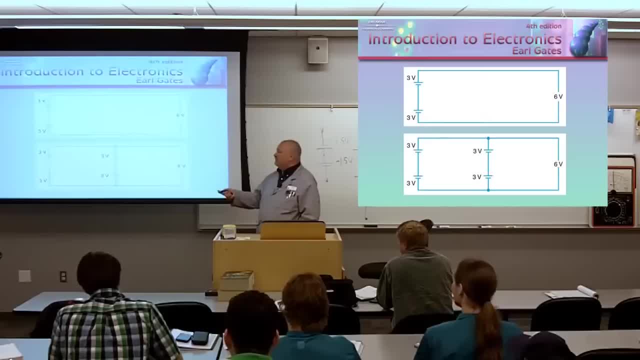 Can you dig it Alright? So here we've got 3 volts and 3 volts, which is equal to 6 volts, connected in parallel with 6 volts. Why, Why come? Why come I do this? Why would I possibly? What is the advantage? 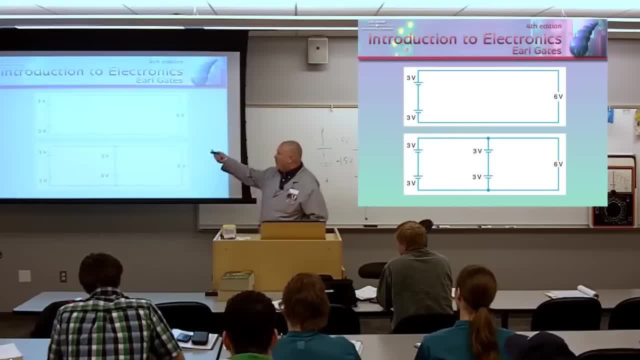 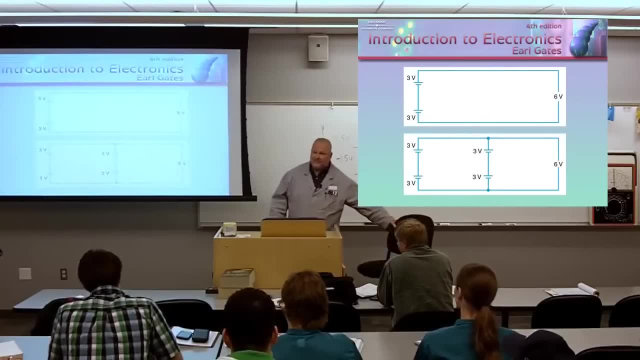 of this Over this. What's that? Is the voltage increased? You said to increase the voltage in the current. Is the voltage increased? No, I still get. how much electrical pressure am I getting out of the circuit? 6 volts. 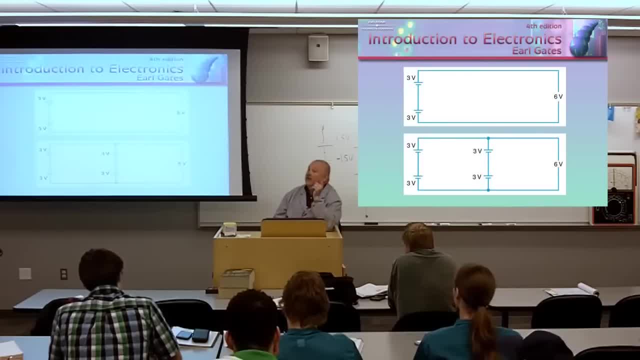 What's that? Increase the capacity? Tell me more about that. I like that Very good. Batteries are measured in in amp hours. How much current over a period of time can they provide us with? So let's look at this scenario for a minute. Let's say that we all 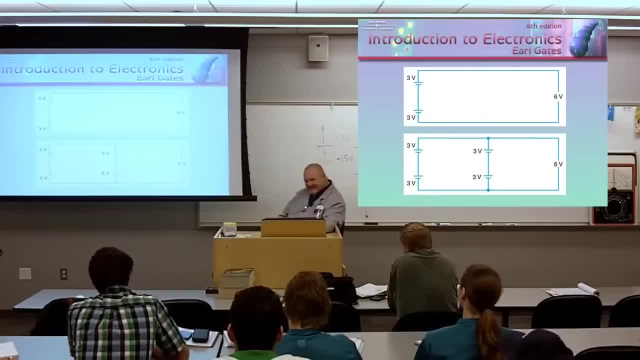 have a sailboat. Wouldn't it be nice if we all had a sailboat. We could sail off to the sunset. Let's sail up to the San Juan Islands And hang out up there. Okay, I've got a 6 volt. It's an unusual sailboat. I've got a 6 volt anchor light. So when I find a nice cove up in the San Juans and I drop my anchor, by coast guard regulations I'm required at night to turn on a light that says I'm anchored And it's a 6 volt light. 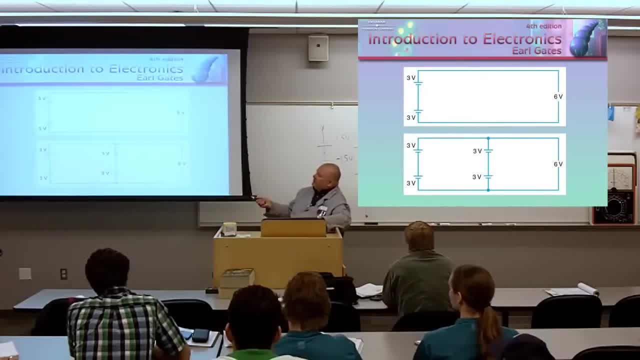 The problem is this: configuration here will only last for 6 hours, And then the light gets dimmer and dimmer and dimmer until it goes out. And shortly after it goes out the fog rolls in, And here comes along a Washington State ferry. 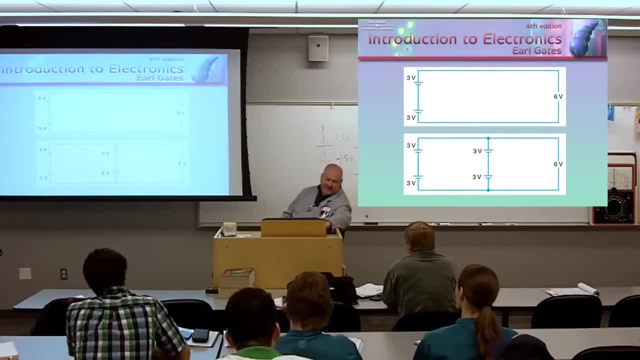 And it runs us down and it ruins all of our fun that we're having on our sailboat in San Juan Islands. So I'm a pretty smart guy. What I did is I went out and I got another battery pack and I put it in parallel with the original battery pack. 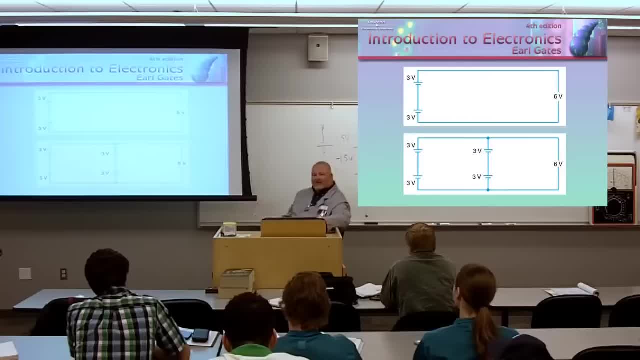 The original battery pack lasted for how many hours? How many is this going to last for? For the same size load, it's going to last twice as long. How's about them, apples? That's how it works. So, basically, he or she who has the most. 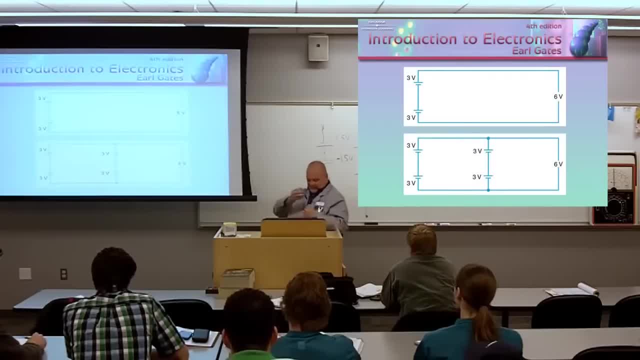 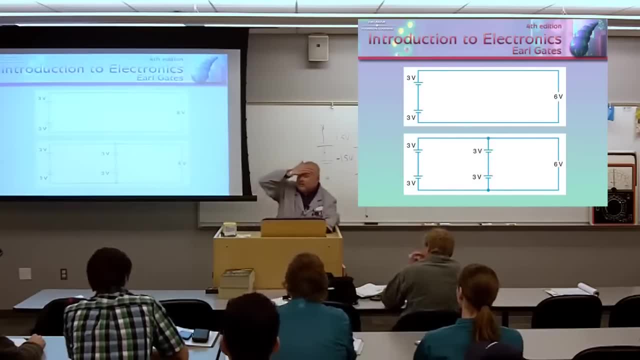 batteries in parallel is going to last the longest, Plain and simple. It was actually kind of a funny story Going to sea for extended periods of time under the water there were very few things, I mean even reading material Books. How many books can you bring with you? What can you do? 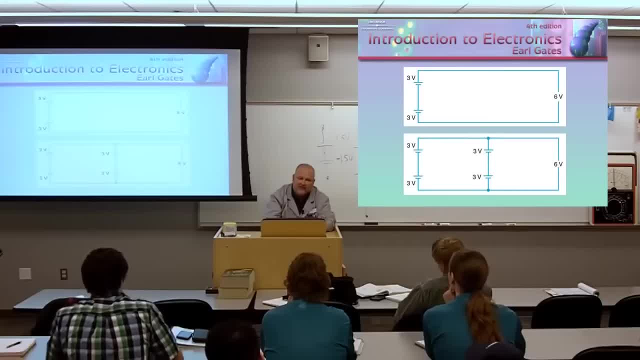 So back in the day the only form of media for me, basically for music, was cassette tapes. So I had my little. I didn't even have a Sony Walkman. I eventually upgraded to a Sony Walkman, but originally I had some, you know. 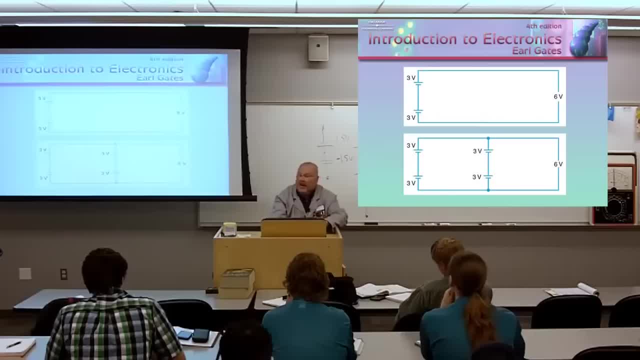 off-brand cassette player And actually that was a big advancement, because prior to that you needed the big cassette player. Put the cassette in headphones, you know? No 8-track, I'm talking strictly the cassettes. This was high-tech Cassettes. 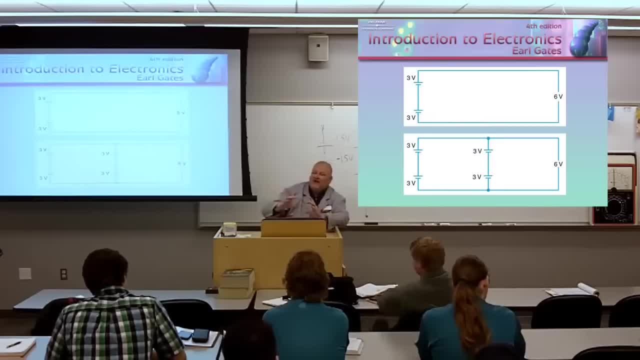 So I bought something that looked like a Walkman, But of course Walkman is a trademark of Sony Corporation. This was some off-brand. So it was so funny too, because you know, everything that we did was super secret. You couldn't tell anybody. 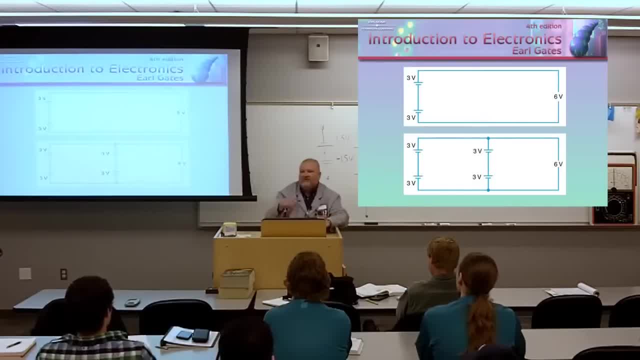 We couldn't even tell our spouses that we were going. So all of a sudden you see a guy in uniform. you know, at the exchange, You know buying like, you know five tubes of toothpaste and seven bars of soap and you know a hundred packs of batteries. 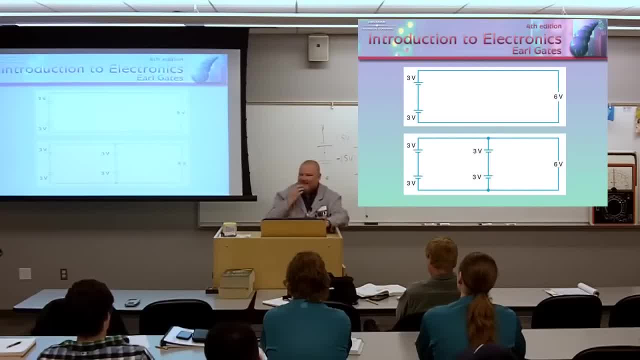 And he's in uniform, with his unit, you know, on his ball cap And you know it's kind of like you're stocking up, You guys are going to sea, You know. so you didn't have to be like an intelligence expert to figure out who's coming and going. So, anyway, we're going to go to sea and it was going to be like a seven month operation. That doesn't mean that we'd be totally incommunicado or away from civilized, you know, shopping or whatever, but for at least a minimum of 90 days we're going to be. 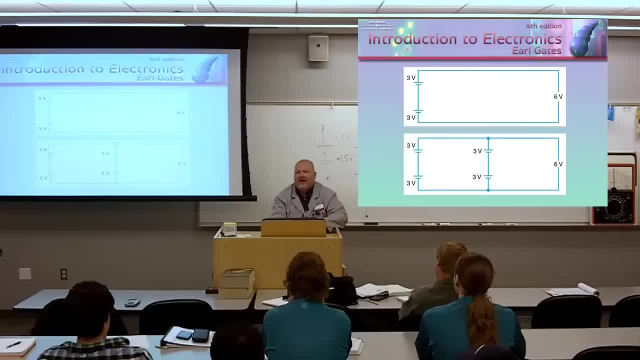 underwater. So I go out and my cassette player took double A batteries, So I bought a bunch of these double A batteries. Well, come to find out that this thing was such a piece of crap that I could listen to 1.5 sides of a cassette tape before the batteries. 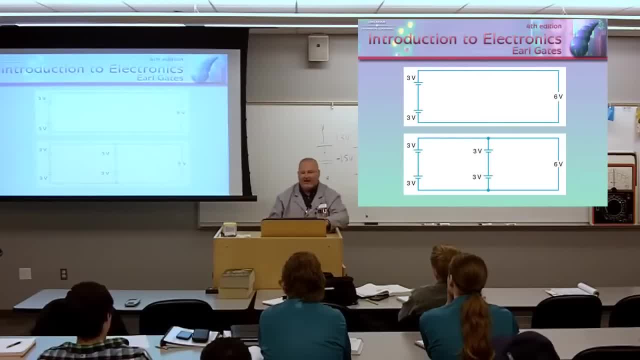 would die And I'm like I'm not a math expert but I'm like I'm going to run out of batteries like really quick. So after I used up all my double A batteries and I still wanted to listen to music, because again you're living with 120 other people in a steel 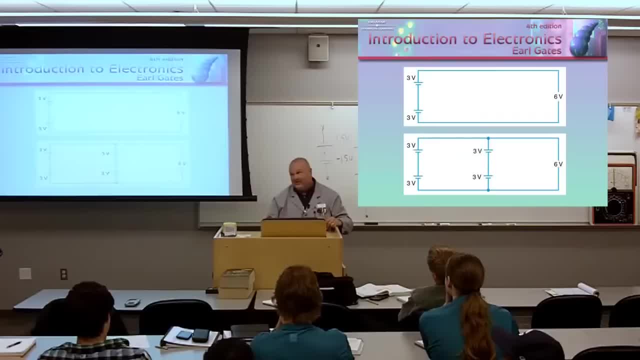 tube, 285 feet long, 28 foot diameter, When you could put those headsets on and you could kind of zone out, that was, you know, a little piece of peace and tranquility you could have. So I'm like, well, I'm a smart guy, I've got an electronics background, How tough can this be? So I cracked the thing off. 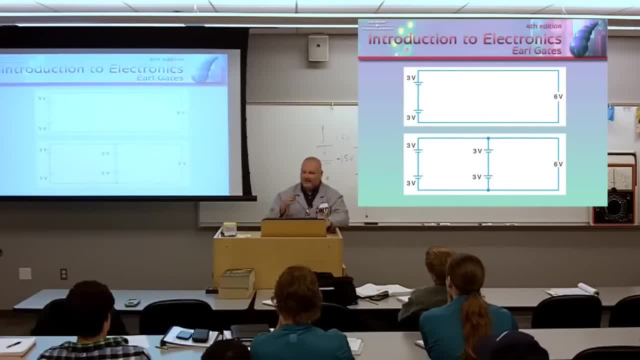 I figured out what voltage I could wire in externally. So then, what I did is every division on the submarine had different consumable products that they were responsible for stocking because you didn't have a store. So actually for my division, 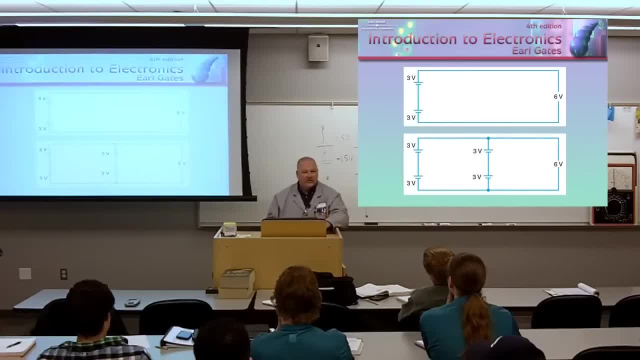 it was pens, pads, paper. So if you were a nuclear reactor guy, you'd come to me and say: hey Joe, you know, can I need some pens? I'd be like, screw you, You know, I'd give you the pens or the paper, whatever you need. Well, ironically, 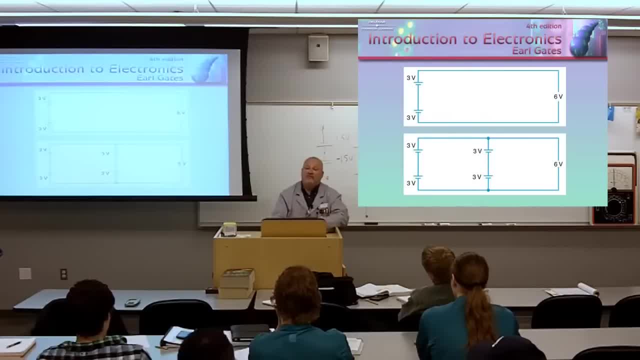 the division that was responsible for providing batteries. ironically were the electricians. So we went back and I said: you know, I need some batteries. What do you guys got? Well, you know, we got these sizes here. They were, you know the big D size and they were military, you know olive. 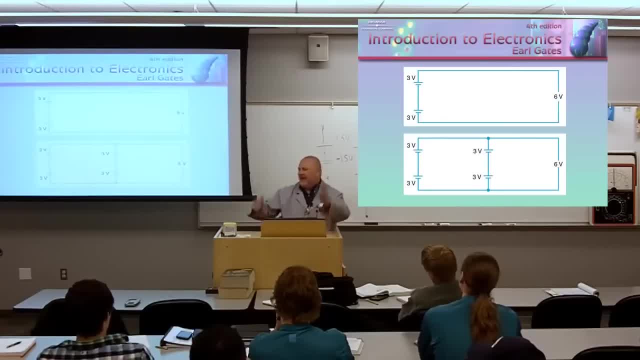 drab green big batteries And I'm like, yeah, give me like eight of them, you know. So I got these eight batteries and I wind them all up, wired them all up combination series parallel, And then I got electrical tape and I like this big freaking brick. 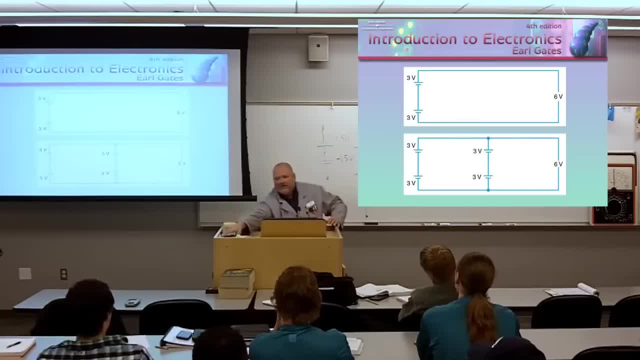 You know, And so I got this nice little portable cassette player that I paid, you know, an exorbitant amount of money for, And then I got this big brick that I like, So it was truly portable device, You know. So, anyway, it worked, And it worked fine. 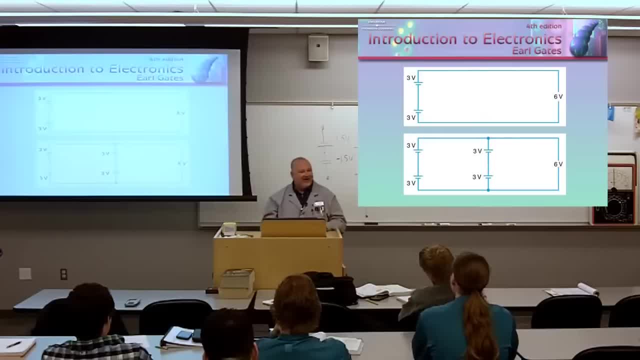 And then I got so used to carrying this thing around that it was like months later we're in port and I'm still carrying this brick And I even had a handle on it And it kept working And I'm like why am I? 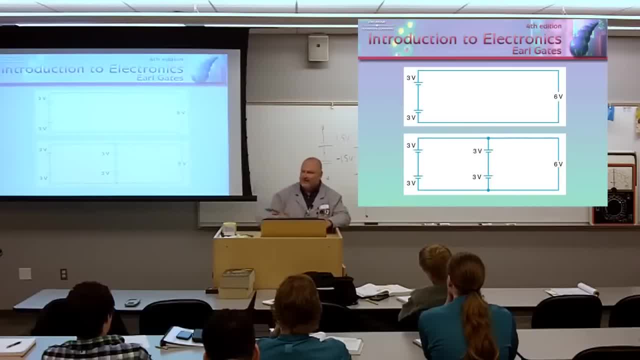 doing this. This thing is stupid. I finally I actually cut it off and I threw it over the side of the boat. that's probably sitting in the bottom of the Thames River in Connecticut still, But the moral of the story is that portable. 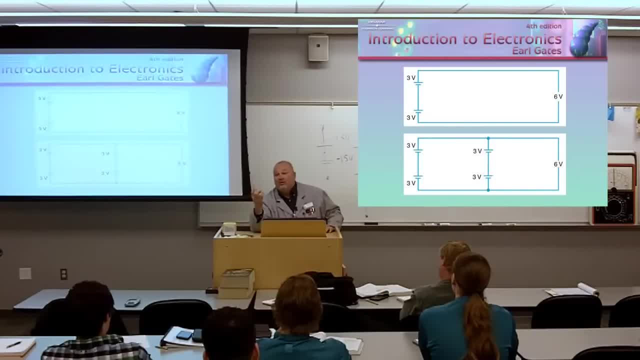 cassette recorder operated off of 1.5 volt cells, did it not? What was the difference when I added the brick to it? Those are 1.5 volt cells, right Capacity Physically more chemical. Physically more capacity, Higher amp hour. 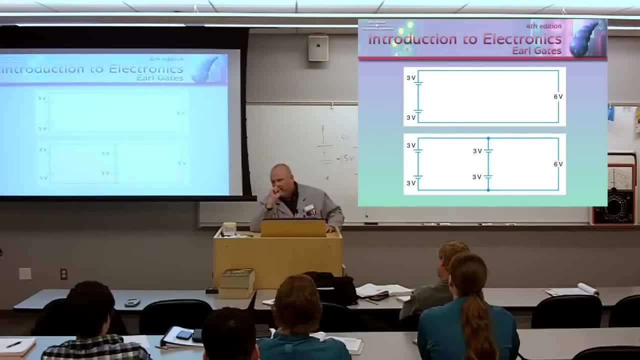 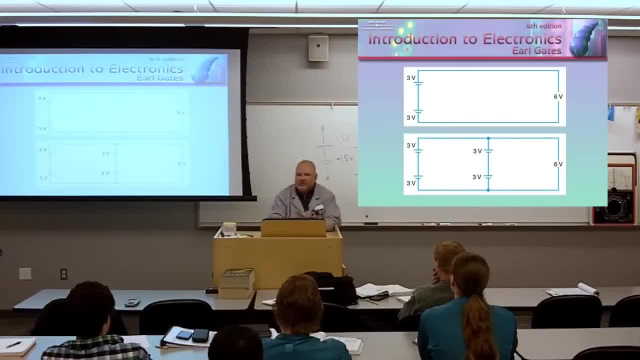 I actually had a student that, as a project, he owns a property in central Washington And, living off the grid, Had a backup generator, Also put in some photovoltaic cells, And, as a project, he basically did the math and figured out like on the shortest day of the year. 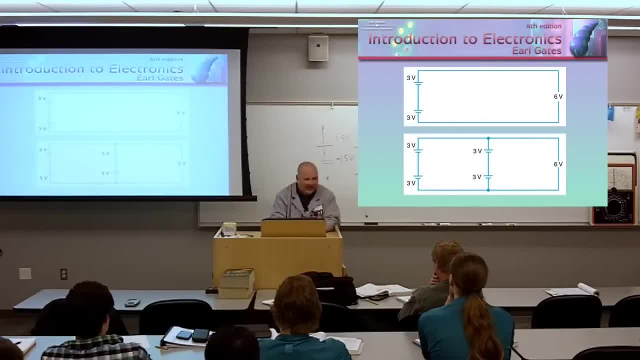 how many appliances am I going to want to run in my little cabin And will I have enough electrical energy to make it through the night? And that's basically what his target was. And he says: I need this much storage capacity. And that's what he used as a 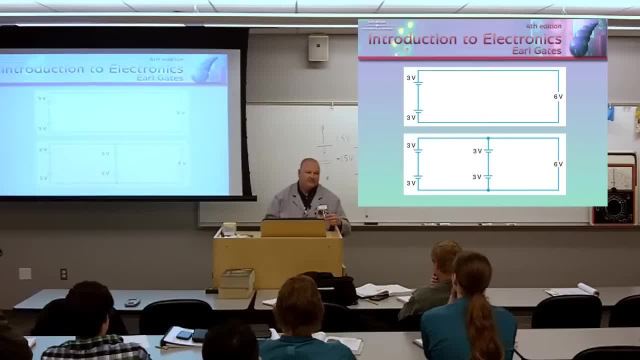 target And actually increased that, I think, by about 20%. And then in the summer how many hours could he use photovoltaic to charge that? And then what's the minimum amount of time that he needs to run his generator to get those batteries up to that full? 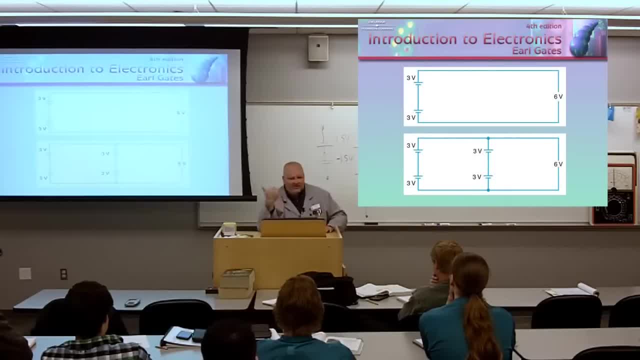 capacity charge. So if you understand the math behind this, let me tell you you're a commodity out there, Because a lot of people don't have a freaking clue. They don't, They don't. When I was on a cruise a couple weeks ago on vacation, I met a 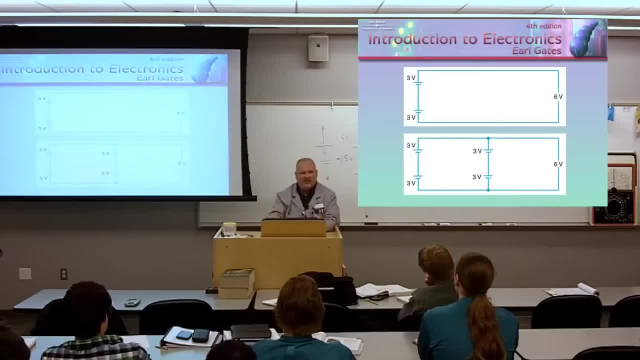 I'm trying to get on better terms with this guy And actually we've been corresponding via email. He owns a 52-foot yacht in Miami And an airplane High performance aircraft And he likes taking his yacht down to the Bahamas and dropping anchor And 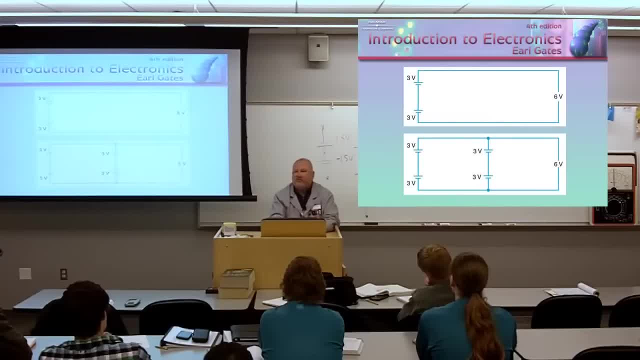 he doesn't like running the generator. So we had a whole discussion about energy management- photovoltaic. what's the minimum amount of time that you could run your generator? can you add batteries to augment the system? And I mean this guy, he's got a couple master's degrees, highly intelligent. 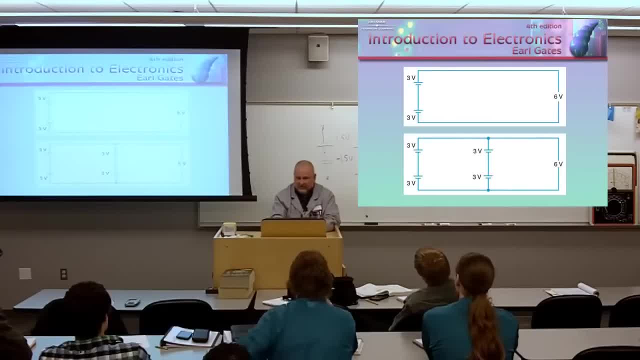 And he didn't have a clue of what I was talking to him about. So if you understand this, let me tell you you got it going on. when it comes to this type of stuff, Make sense. Voltage rise is the energy we put into a circuit. Voltage drop: 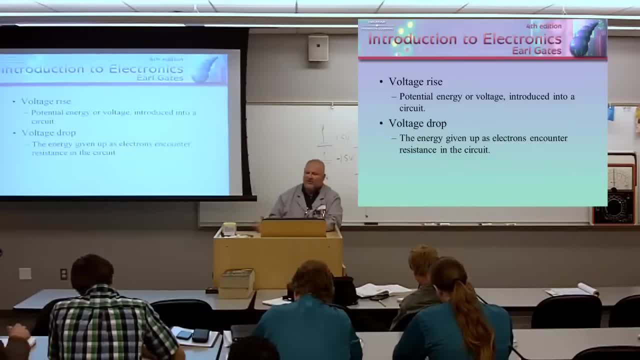 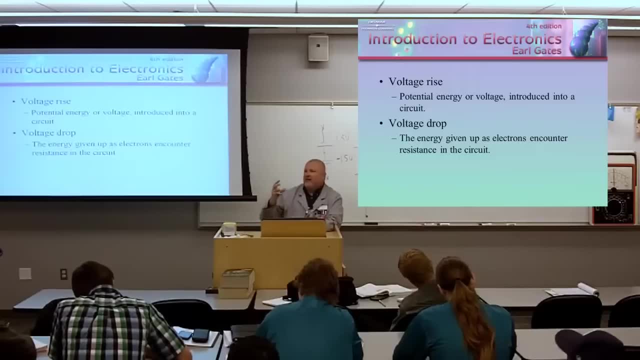 is the energy that we take out of the circuit, if you will, Is given up As the electrons encounter resistance to the circuit. So voltage rise would be like your batteries. Voltage drop is what you're powering, And you know what They should always be equal to. 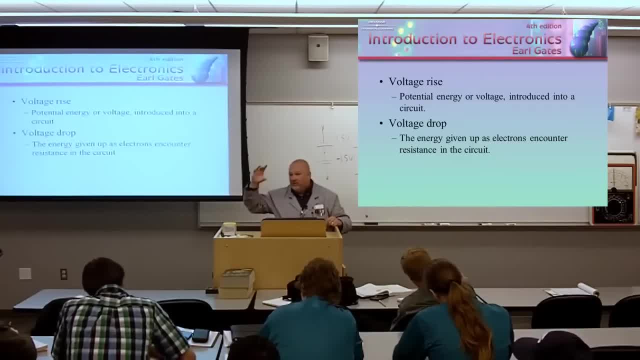 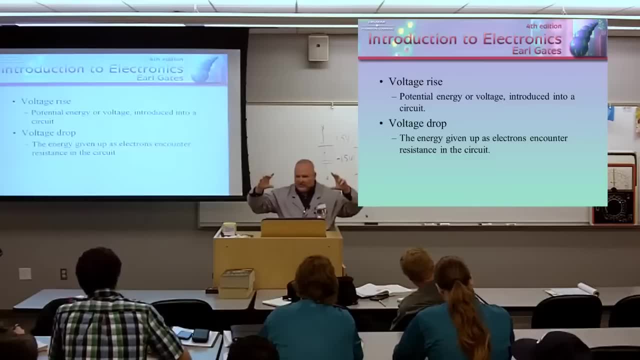 each other. If you've got a 5 volt battery pack and you're powering a radio, that radio should be consuming 5 volts. 5 volt voltage rise, 5 volt voltage drop Make sense. You should never end up with energy left over. 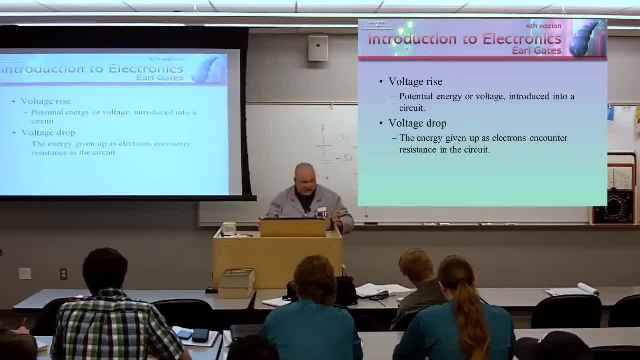 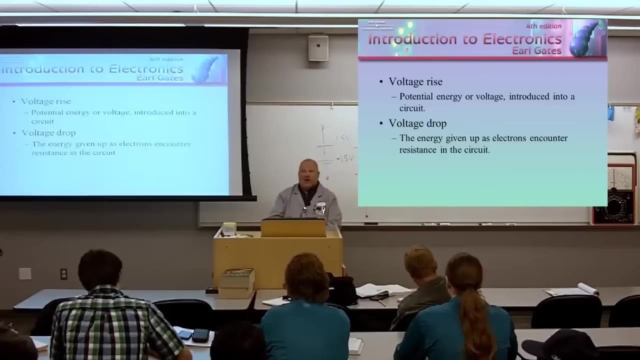 If you are, that's what we call a malfunction. You've got a malfunction. You've got voltage not going from the source to the load. The voltage rise that the power company provides my house with is 240 volts AC. My voltage drop from my home is 240 volts AC. 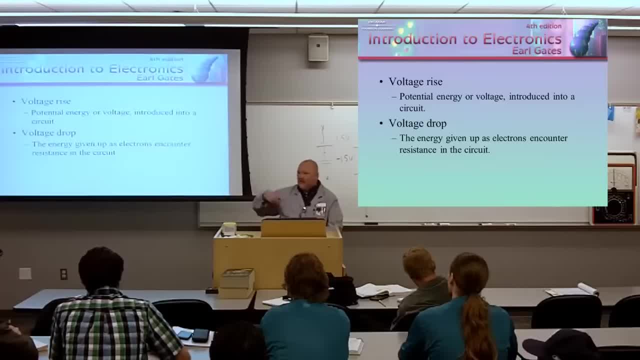 If it was 239,. that means a volt is being dropped somewhere underground or in the overhead. It's not supposed to be getting dropped there. Question: So like if. So like, if our company provided you Voltage rise, Voltage rise, So like if you used more energy, would you be? 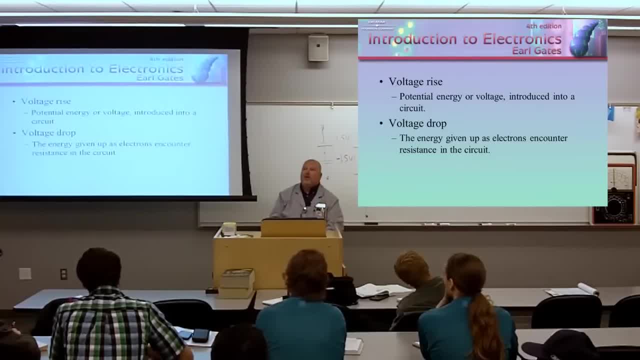 pulling out more current, not more voltage. Yeah, that's, your question is more related to power. I'm talking simply voltage. I'm talking simply voltage So that if I've got- and I'm keeping it real simplistic and you need to understand it in a simplistic manner- If this 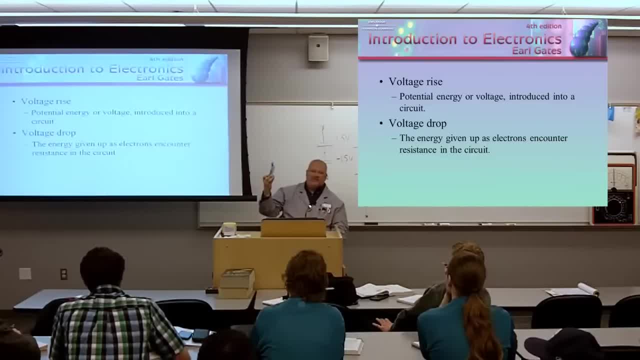 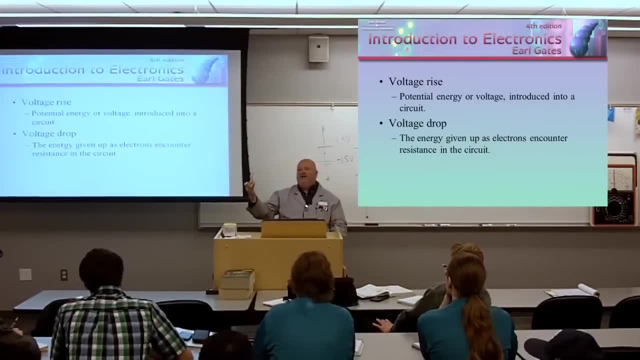 calculator takes 3 volts DC. that 3 volts DC is going to be my voltage drop right. If I want this thing to operate properly, I need to give it a voltage rise of 3 volts. So that's all I'm saying. 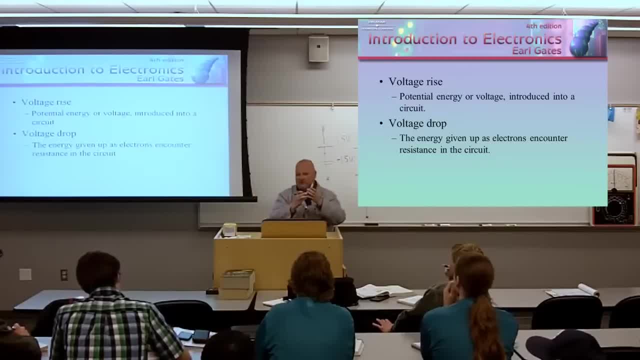 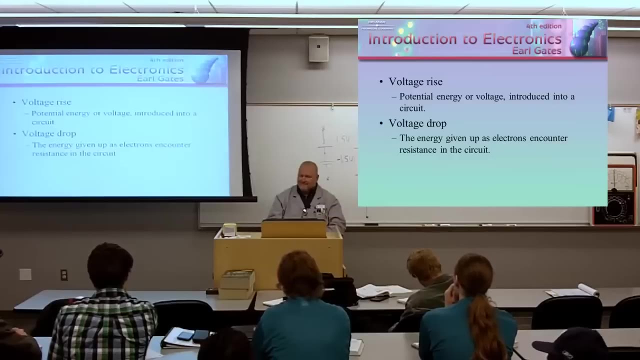 Voltage rise is the voltage pressure you apply to it. The voltage drop is the pressure that gets consumed by the load, And they should always be equal. If they're not, wherever the missing voltage is, that's a problem. So if you consume less voltage, 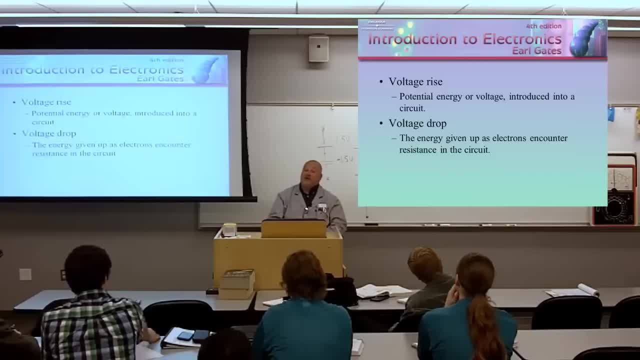 If you're consuming less than what the power company's providing you with, you've got a problem Because that missing voltage has got to be somewhere. And where you find it, that's the problem, Make sense? Okay, we'll talk more about that concept. 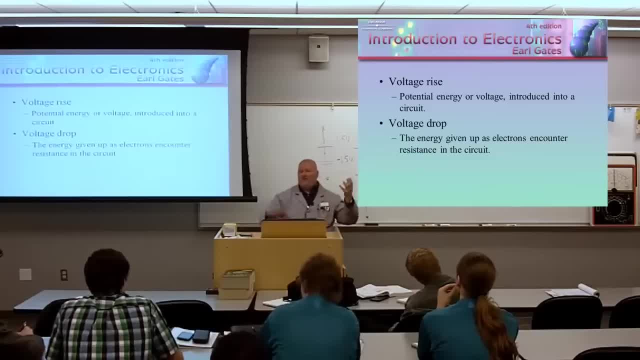 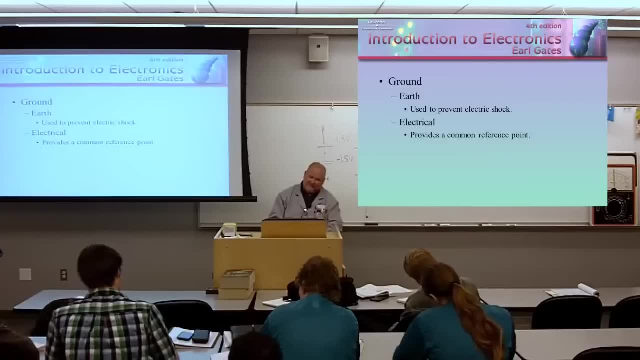 But right now I just want you to understand: voltage rise equals voltage drop, Ground Ground. This is an interesting concept. Any of you here ever driven over Snoqualmie Pass? How do you know you're going over Snoqualmie Pass? It's not a trick question. How do you know you're going over the pass? 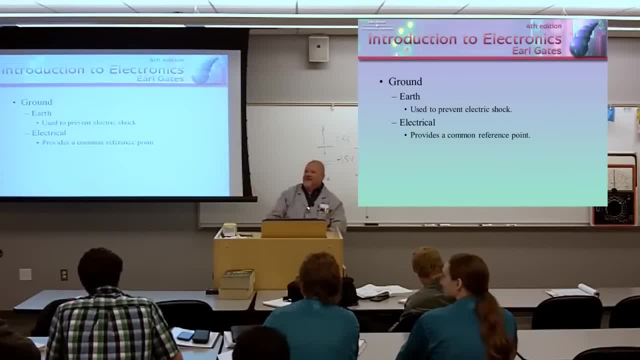 There's a sign on the side of the road that says Snoqualmie Pass. I try to keep it basic here. Now that sign also says Snoqualmie Pass, and there's another bit of information there: Elevation, Elevation, above what? 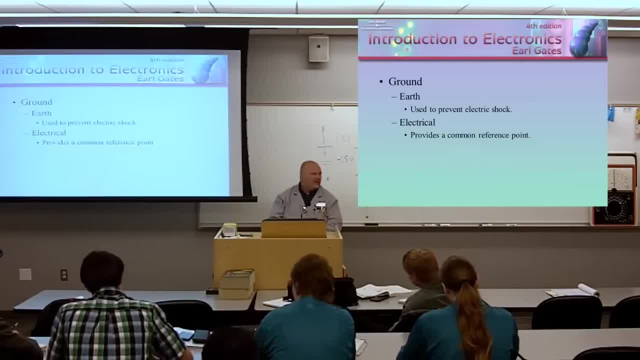 North Bend, Seattle, Above where Sea level? You guys are all smart. You guys are one of my smartest classes here in a while. High tide or low tide, Average, Average, And you know what we call that MSL- Mean sea level. 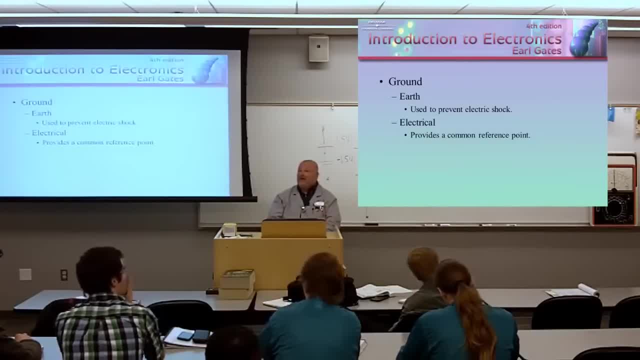 So one of the things Al Gore is talking about, like sea level rising. that's what he's talking about. So his big concern is all the expense of changing all the signs. Now, obviously it's going to cause a lot of problems, if mean sea level. 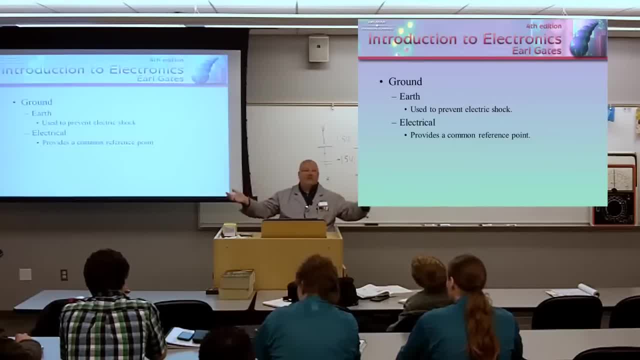 if the polar ice caps melt and sea level rises, it's going to be a lot of flooding and devastation, Especially during hurricanes and high tide events and tsunamis and everything else. So we use the height of the ocean mean sea level as a reference for all of our height measurements. 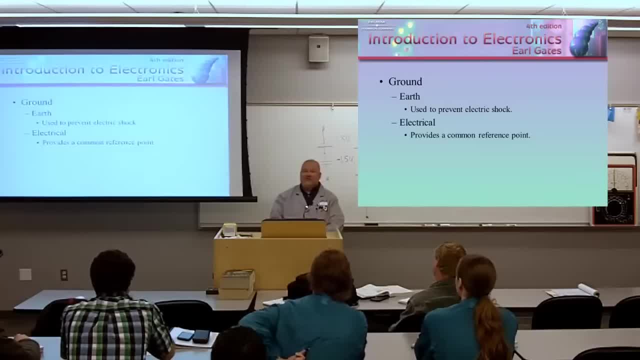 It's actually really important When I fly my airplane. it's one of the first things. instruments I calibrate when I get in is the altimeter, And that shows me how high I am above sea level. It's kind of important. I flew my airplane Friday night. 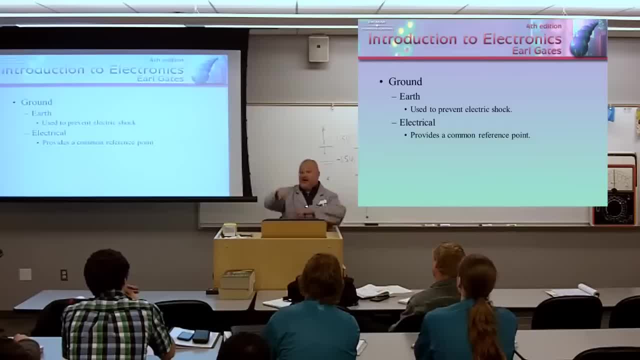 I went across the top of SeaTac airport. I had airplanes taking off and arriving and I'm flying through there in my small plane. You kind of think it's important that I know what altitude I'm at. Yeah, And as a matter of fact, 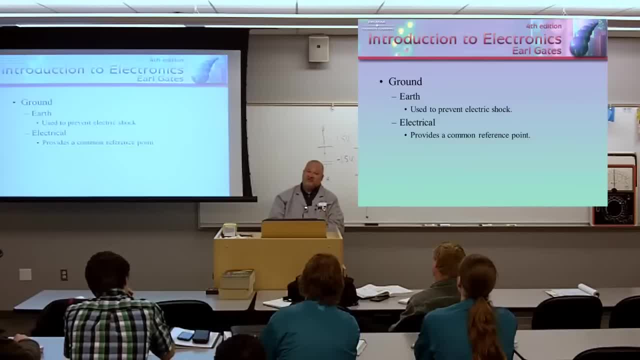 they check back with you When you establish radio communications. they say: you know, hold, maintain 1,500.. Force is kilo. what's your current altitude? 1,500.. Roger, we got you at 1,500.. You're cleared. 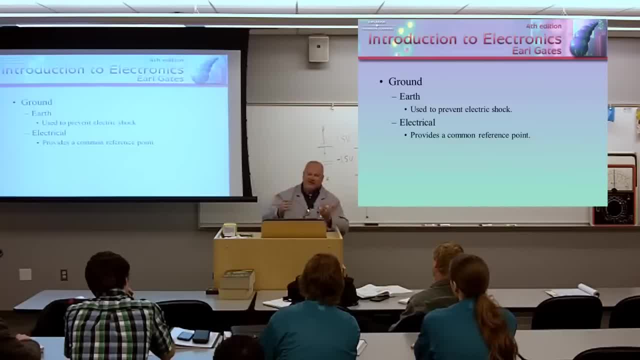 through our airspace Because they want to make sure you're not off. It's important to me, So that's how we calibrate. if you're into hiking, driving, even boating- Mean sea level is kind of critical, isn't it? High tide, low tide If you're at low. 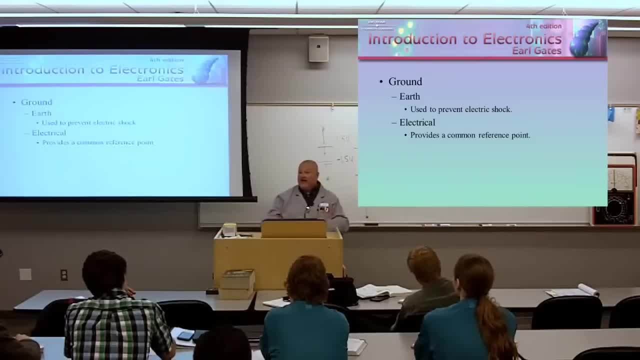 tide and you hit a freaking rock. it's kind of important you have the right charts and you understand low tide. Are you saying mean, Mean, Mean, No, mean, M-E-A-N mean, Which is average. So when we started playing around with electricity, 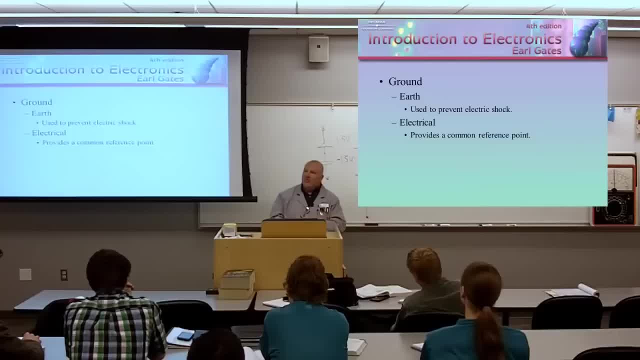 we had to come up with a methodology, if you will, to what's what's. what can we compare? What's a benchmark of something that's in a neutral natural state- Earth? Why? Because this is where we be, Okay, This is where we're standing, So literally what we got. 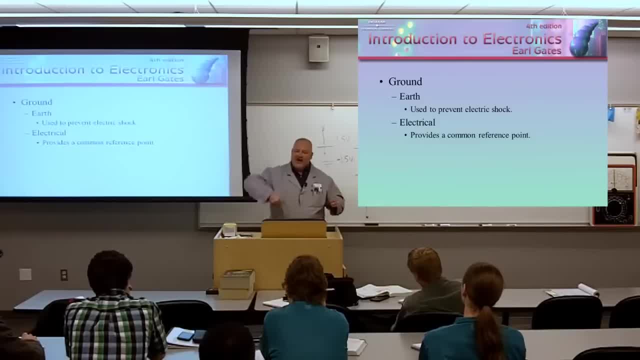 is a ground rod, an eight foot ground rod, drive it into the earth and say you know what you connect to, that you're connected to ground And you're connected to zero potential. It's not positive, it's not negative. 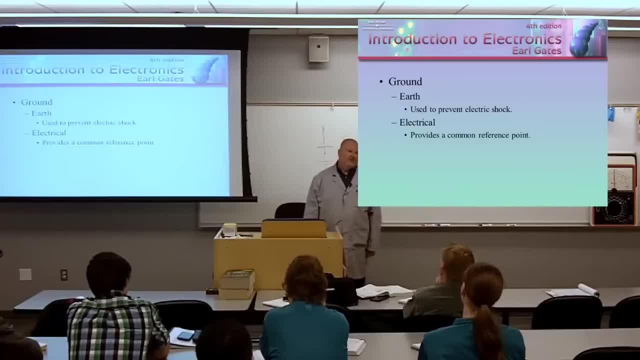 it's neutral. Why? Because it's driven into the freaking ground. So what happens is the idea kind of caught on. So the power company out at the power pole or your transformer, if you have underground, they got a rod and they drove it into the ground. They said: you know what? 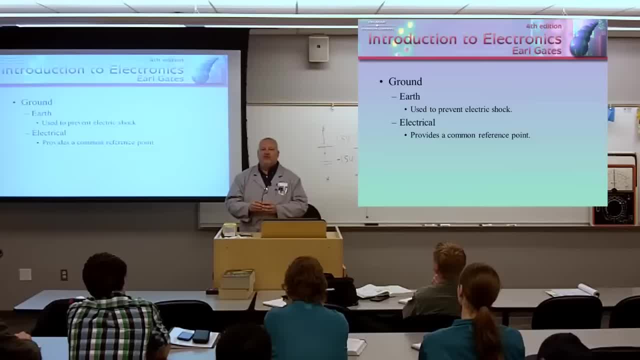 we're going to sell you 240 volts AC in reference to ground At your home. at your load you should get 240 volts in reference to ground, The electrical generating plant where they generate the electricity. they drove a ground rod in and they referenced that voltage. 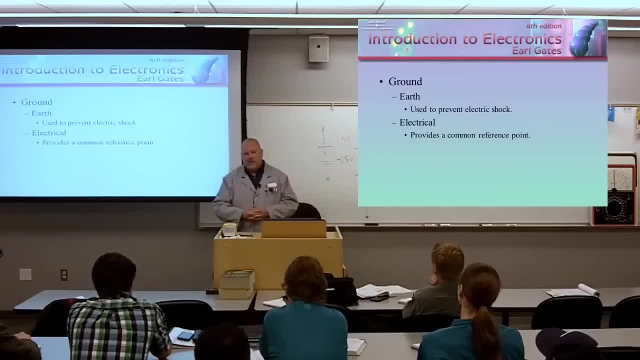 to ground, So we use it as a reference to all of our voltages, which are really quite critical. I'm kind of making fun of this in a goofy way, but in all honesty it's actually really, really critical, Like right. 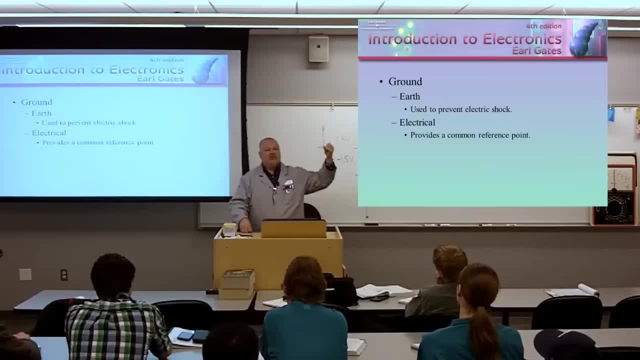 now at my home I've got the electrical connection coming from the power company in reference to, hopefully, ground. I get my telephone line soon to be replaced, kicking it old school and that needs to be referenced to ground. 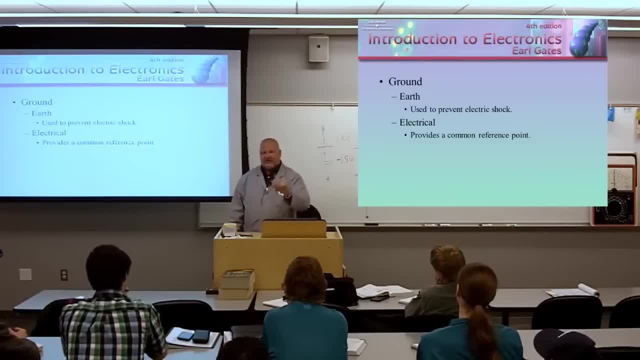 I've got a satellite receiver that has the antenna up on the roof. That antenna needs to be referenced to ground. The satellite receiver also plugs into the electrical outlet. that should be referenced at ground. and it also needs to be plugged into the telephone connection. that should be referenced at ground. 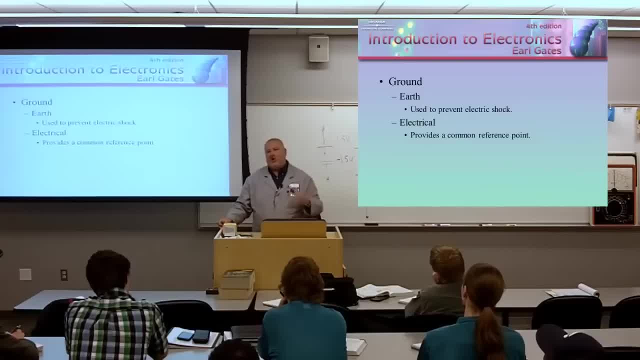 Actually, when I had Comcast installed in my home, it was over the summer, I had time off. I was watching these dudes install it And because I teach electronics, I'd always like to say: hey, dude, what's going on? man, How long you been with Comcast, These people treat you okay. What's the deal? What's your? 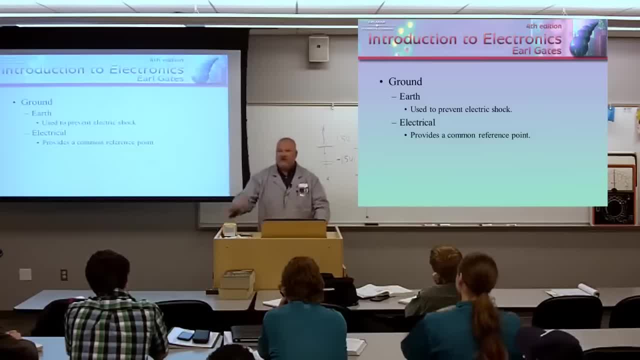 educational background. What's going down? How are you doing that? If I could learn something from you, somebody that does installs all day long, I'm going to pick your brain and see what I can learn. Anyway, I see this dude hooking his freaking contraption up to my 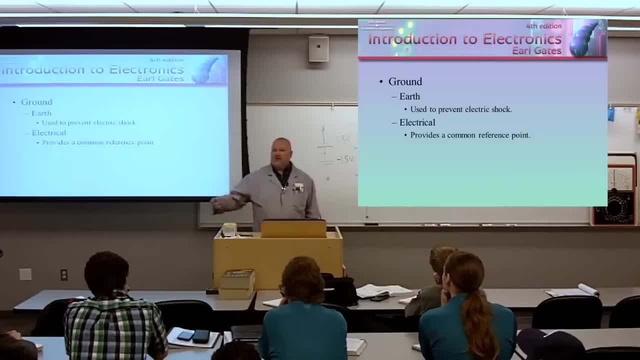 faucet. I'm like: what are you doing? He said: I'm connecting this to ground. We've got to reference it to ground. I'm like: hold on, cease and desist. what are you doing? Well, I've got to connect. 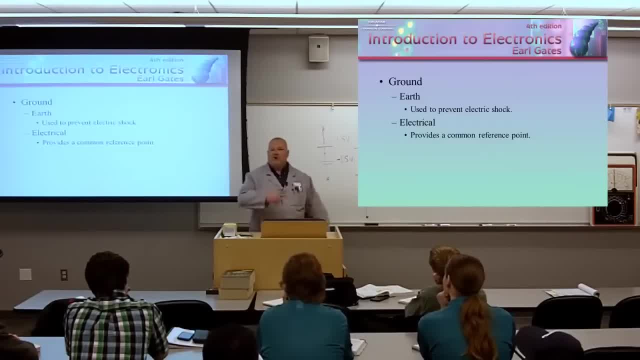 this to ground. I said that's my freaking water connection. Well, yeah, but this is, you know, water pipe is a good ground. No, You see that, right there, driven into the ground, That's a ground rod. okay, That's the same ground rod. 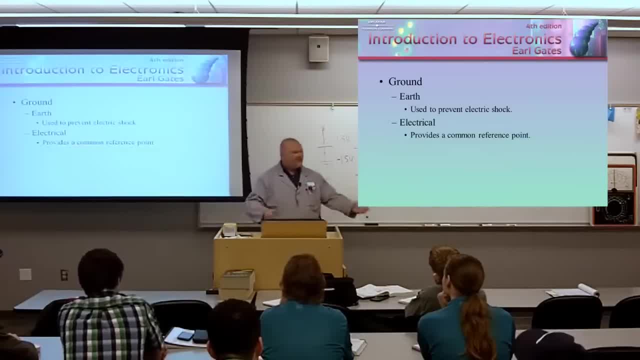 that the power company's providing me with ground. It's the same ground that everything else in the house is connected to, So why are you going to connect it to this faucet coming out of the wall? You don't know if it's PVC inside. He really got an attitude and I'm like no boom. 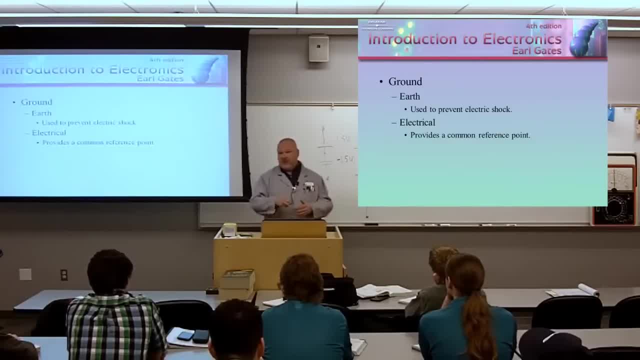 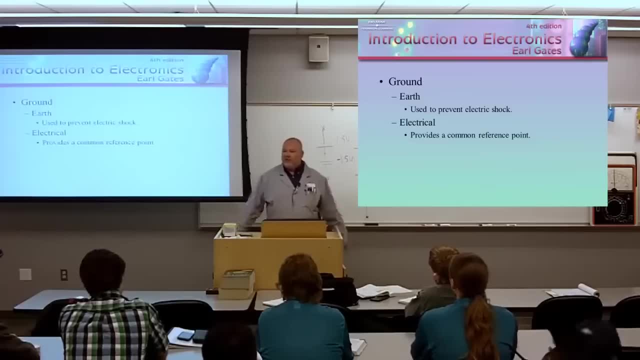 cease and desist. I got a supervisor out there and I had to sign paperwork. Modified install- Modified install- Customer request. I want ground And I wrote that right in there: Me want ground to be connected to ground rod, You know. so they all really got an attitude and stuff, you know, But it's kind of like no, I mean it really needs to. 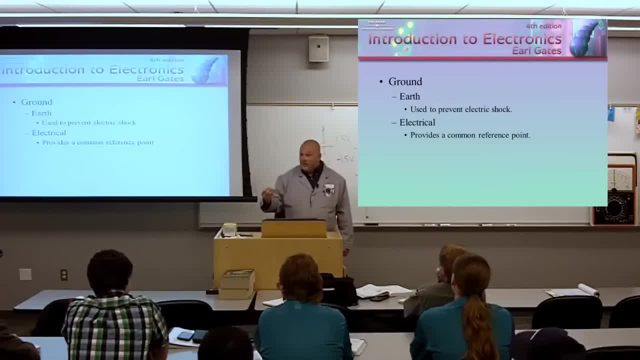 happen Because especially too, this is back in the day when you had a computer modem. You could have that modem, You could have your computer power supply, You could have all these things, And if they're not all connected to ground, they could develop a. 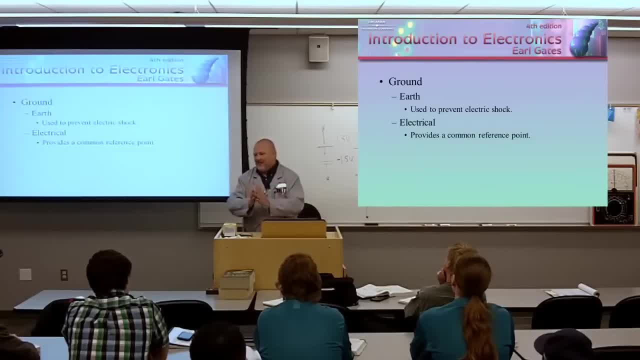 difference in potential. And if they develop a difference in potential, you know how that's going to manifest itself With highly sophisticated electronic systems. Not necessarily sparks of fire, It could be gremlins, It could just be real wacky behavior. All of a sudden, your satellite. receiver starts rebooting itself. All of a sudden your computer reboots itself. All of a sudden your modem kicks you out. So when they started doing all of this- inter-building, networking and everything- it became a real big issue to make sure that ground was really ground Years ago. 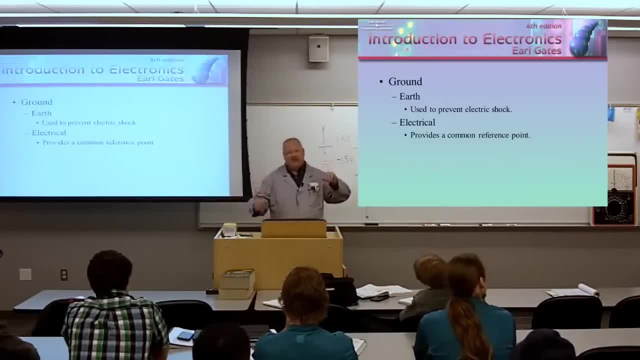 when they built this building. well, actually they renovated this building behind here. they pulled up the concrete and they drilled down into the earth And they put in this huge ground for the school to make sure it wasn't just a standard ground rod. This was like drilled way down into the earth. 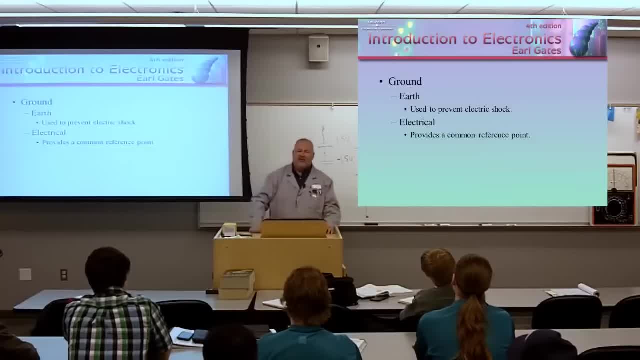 You can see the core and stuff. I'm just kidding, It was pretty far down in. This is actually one of the problems they have in Arizona because of the sand and the desert. We have good ground here because it's all wet. 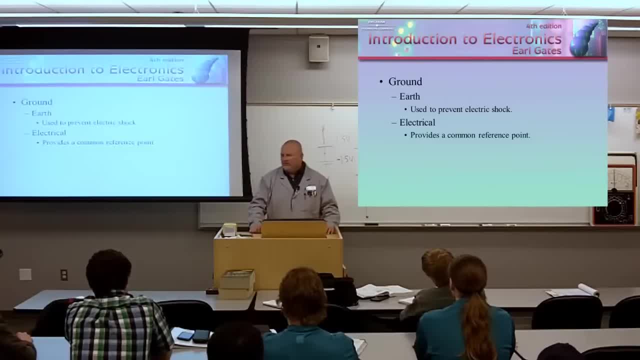 But in Arizona they have some problems. So I think there's some code variants down there where they're actually connecting rebar in the concrete foundation and such. They do some different stuff down there. I'm not totally familiar with it, but some of those drywalls- 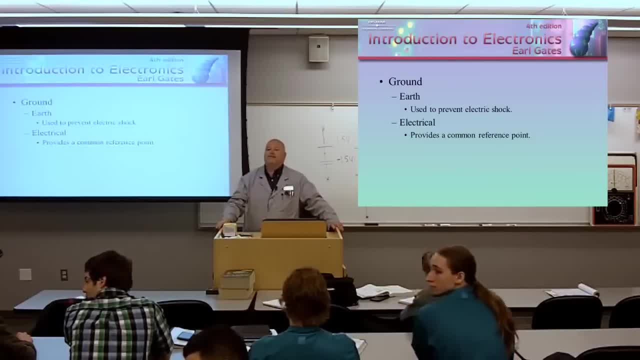 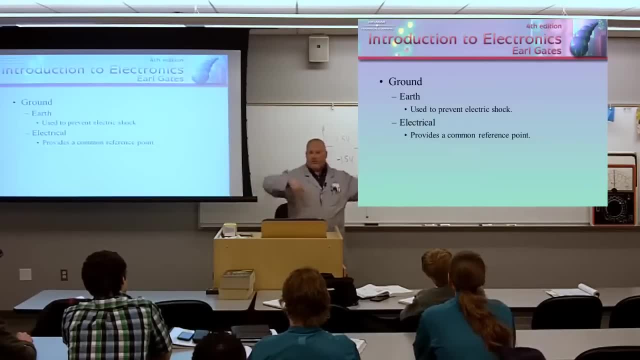 They have to do it, John. It was And they were actually adding chemicals to almost create like a P and an N type material there. so current would only have one way to travel through that: like a giant diode buried in the ground. 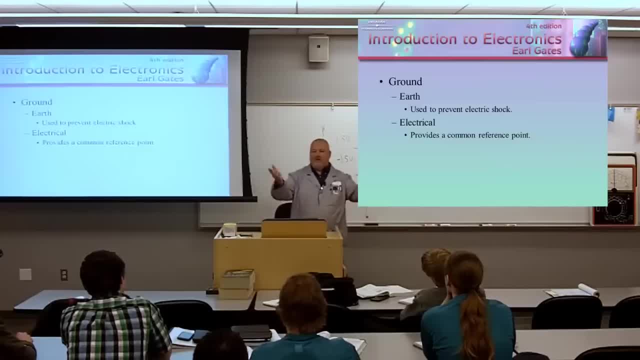 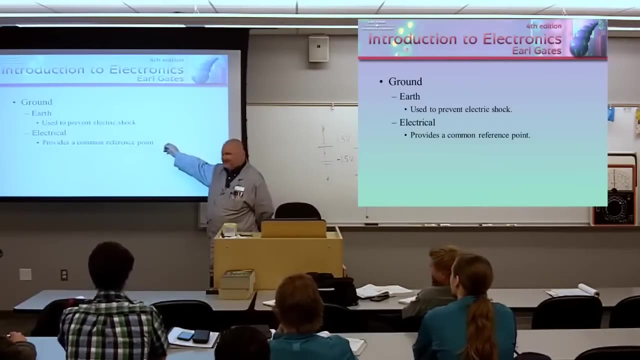 behind here. I wish I had taken pictures. I know you're not believing me, But it was like a drilling rig out there. Black gold, Texas T, We're going to Hollywood, Anyway. the other type of electrical ground is electrical ground And this provides a common reference. 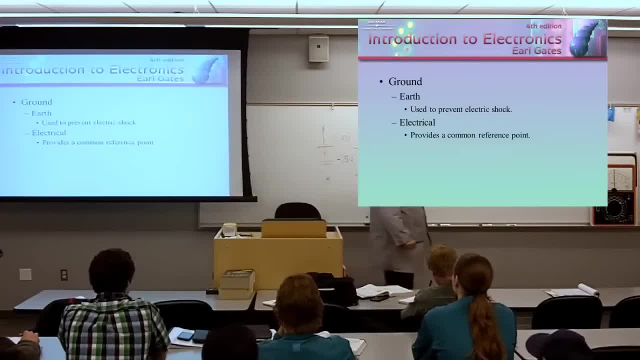 point. We use this electrical ground because a 747 taking off would look stupid with a big reel spool of wire trailing behind it. Okay, It just wouldn't look right. So for pure aesthetic purposes, we can't do this, So we use what's called electrical. 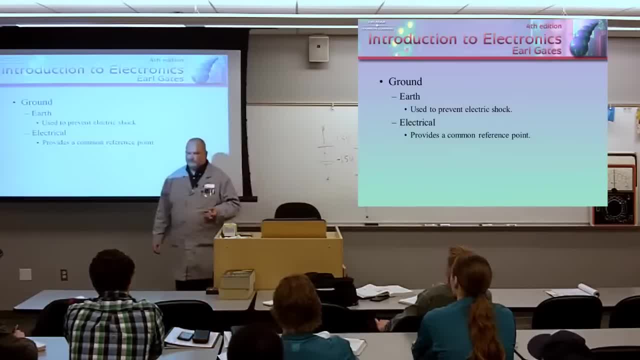 ground. Your car uses electrical ground, Airplanes use electrical ground, Ships use electrical ground, And what that in essence means is a chassis ground. Now, most of our home appliances use both. We ground the chassis, the electrical ground, to earth ground, So that if you have a three prong plug, 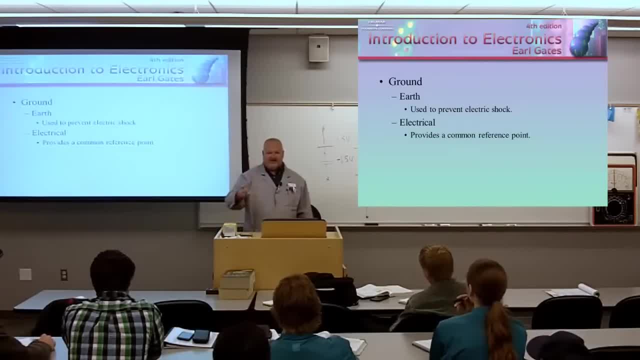 one of those plugs, that round plug, is ground And that's connected to the chassis. So be aware of this. In the lab you're going to have some problems with ground, Because you don't understand what I'm talking about. Some of the 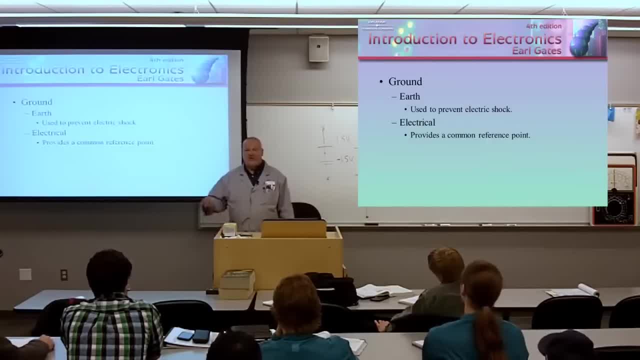 equipment that we have in the lab is isolated from ground. So when you connect the negative lead, like on a power supply, you think you're connecting ground as a. you're not That negative. if you have a DC power supply in the lab, you have a. 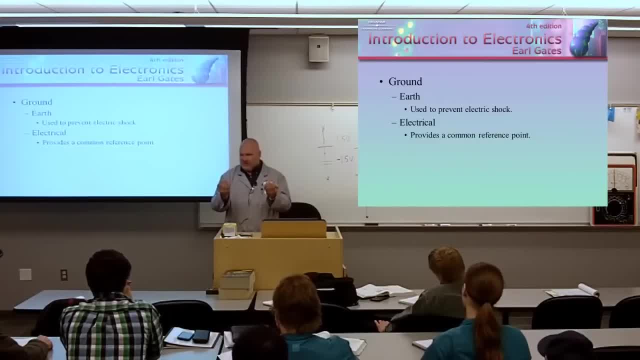 positive, you have a negative. they're isolated from ground. They have nothing to do with earth ground So in some cases you could create a ground loop in there and they get wacky results with your equipment. Most commercial, consumer, industrial products. 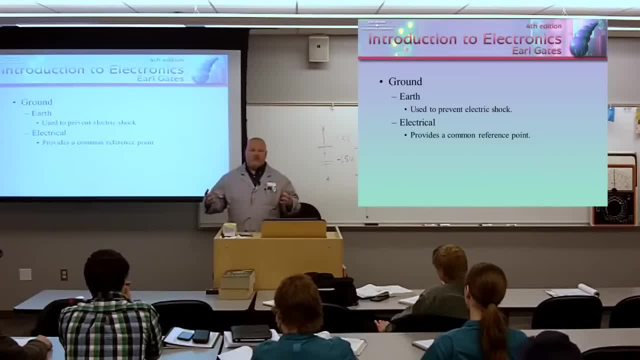 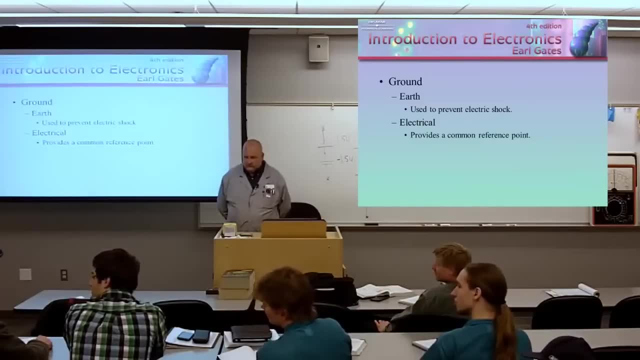 are for the purposes of electrical safety, that chassis will be ground And that's connected also to earth ground Question. So electrical ground can vary from whatever you want, Absolutely, Absolutely. And that's one of the things that can be a real problem Is you might think you get into a piece of equipment. 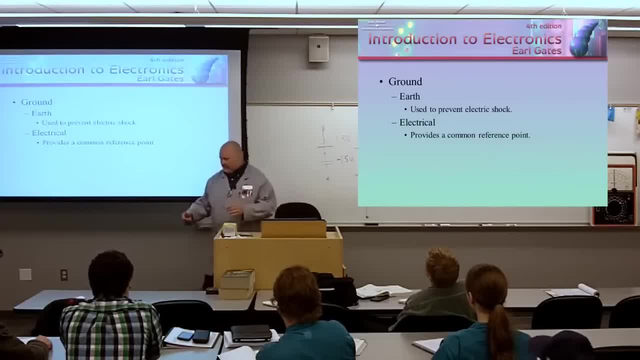 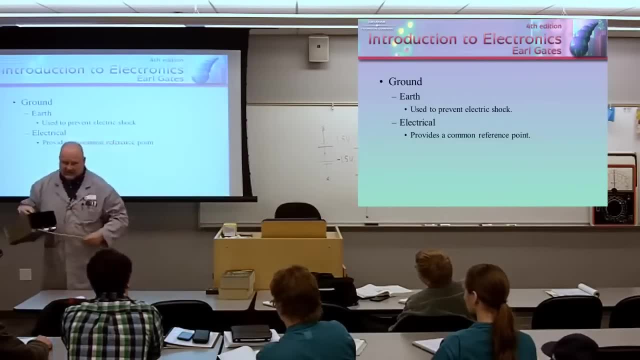 and say, oh wow, look at this big metal, look at this big. if this was inside, this is actually a DC power supply like we use in the lab. This in the back here is a heat sink. If this was installed inside, some big piece of equipment like a radar system, 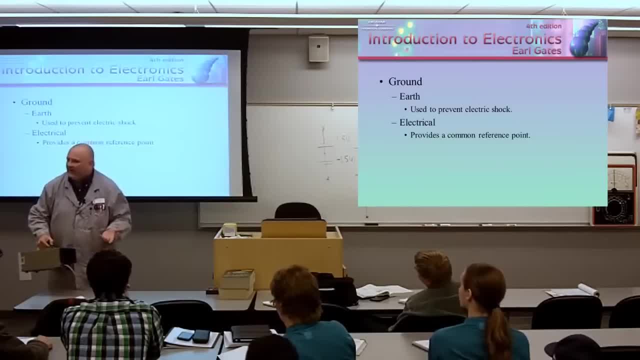 you see this metal, you assume that, oh, this metal here, that's ground, That must be ground because it's metal, Right. And all of a sudden, you know, you put your hand on there, you lean into it and you get. 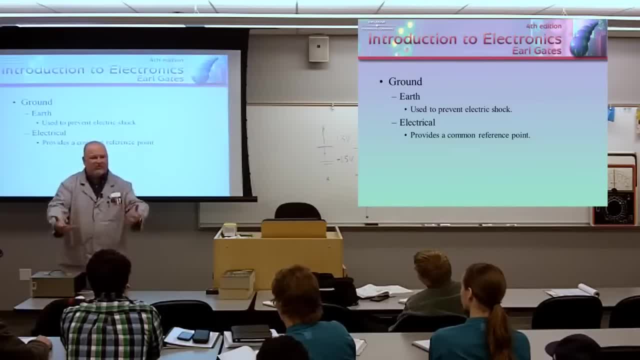 electrocuted. This in some cases could be electrically isolated from ground. This could be connected to some big high power transmitter tube for the purposes of dissipating energy and it could actually have like that mica that I passed around earlier. 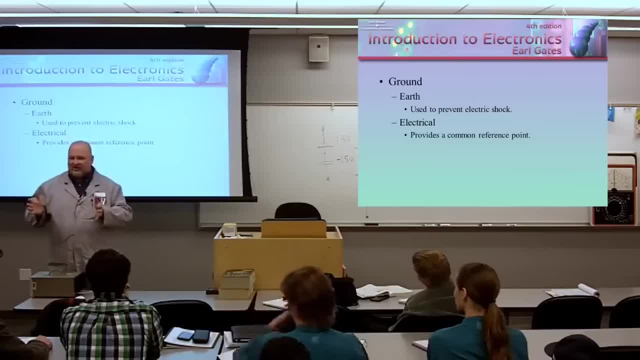 it could have a big sheet of metal and it could actually have like that mica that I passed around earlier. it could have a big sheet of that mica there, electrically insulating it from the rest of the chassis or frame of the piece of equipment. 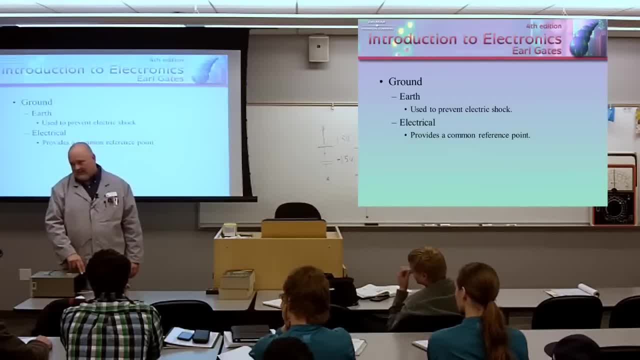 And that's taken out many a good technician. So never assume, Never assume. Generally. yes, Some of the worst shocking experiences I've ever had were working in a lot of tube circuits, Because sometimes those tube circuits were notorious for two prong Old school tube amplifier. 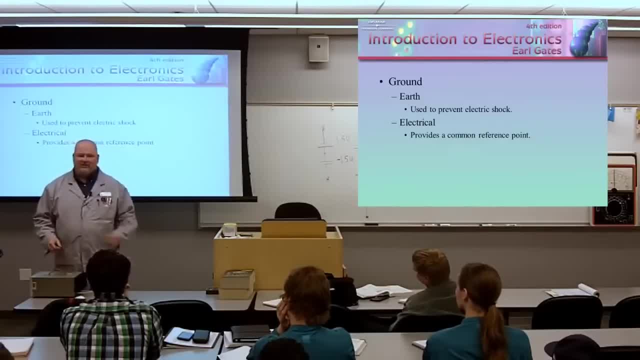 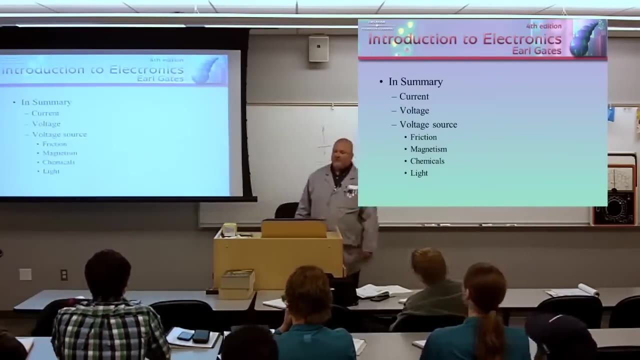 you plug it in two prong and you didn't have that electrical ground in there. All of a sudden you go up against the chassis and you get getting zapped by 300 volts. Make sense, Alright. We talked about current Flow of electrons in a specified. 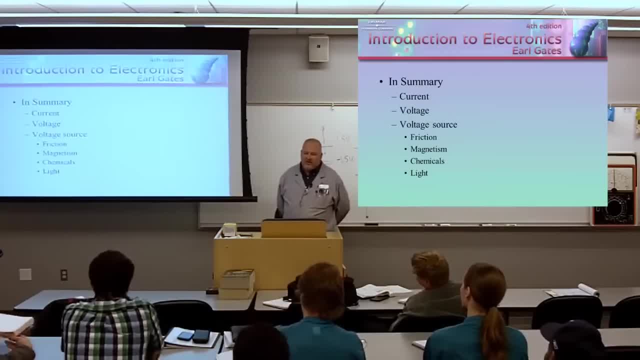 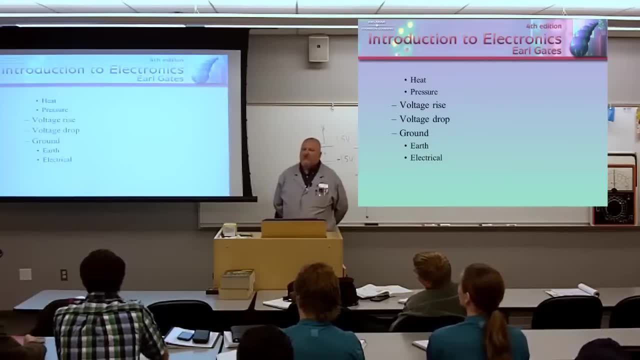 direction happens at the speed of light Voltage, And there's only six different methods of producing voltage: Friction, magnetism, chemicals, light, heat and pressure. We talked about voltage rise. That's the energy that we put into a circuit. Voltage drop is the voltage we get. 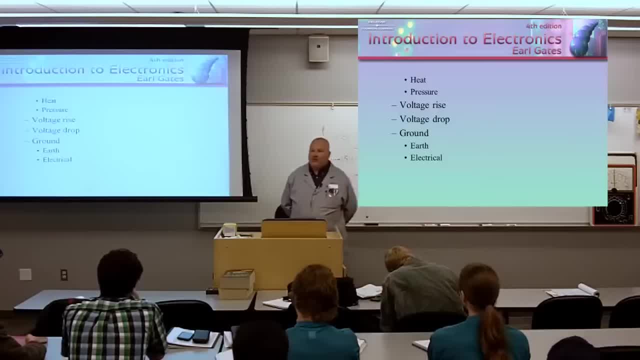 out of the circuit. Voltage rise and voltage drop should equal each other. If they don't, you got a problem. Am I being silly? Am I keeping it basic? Yeah, But you know what I have fixed in my career? dozens of problems, that that was the symptom. 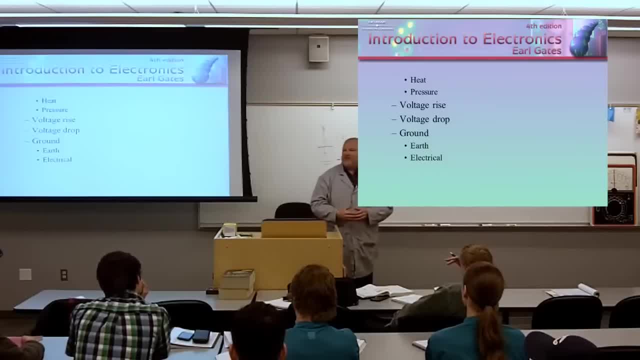 And the symptom is the equipment doesn't work right. What's the first thing that I do? Check the voltage coming in. If the voltage coming in isn't good, it's not gonna work right. Then you gotta find out where the missing voltage is. 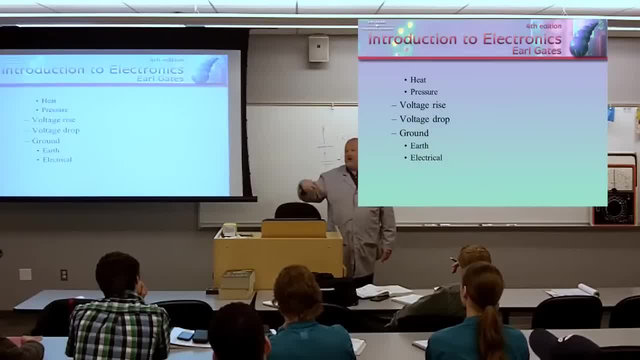 Maybe it's a brownout. Maybe it's a brownout, Maybe the power company they're having a problem with generating power and giving you know the feed, But those two always need to equal each other. We also talked about ground, Earth. ground is a freaking. 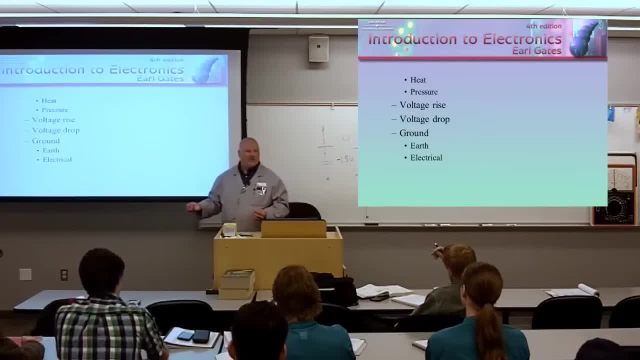 rod driven into the earth. Why the earth? Well, it's where we stand, It's where we live, It is what it is: Neutral natural state. And we talked about electrical ground, which is typically the chassis, Could be the airframe of an airplane, Which is actually. 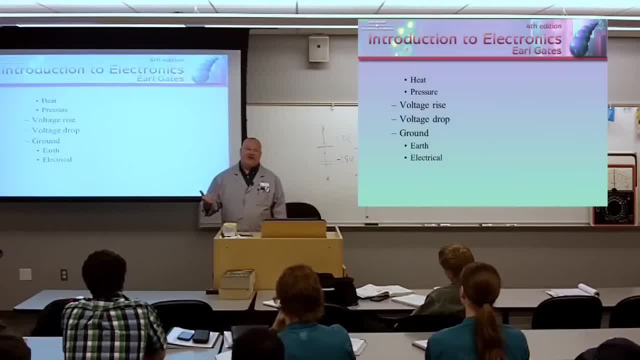 kind of odd. It's kind of odd when I talk about an airplane, Because what's Boeing building? now 787.. What's that thing made out of Aluminum Composite? Think about this one. By using the chassis of your automobile as ground, you know how much wiring it saves on your car. 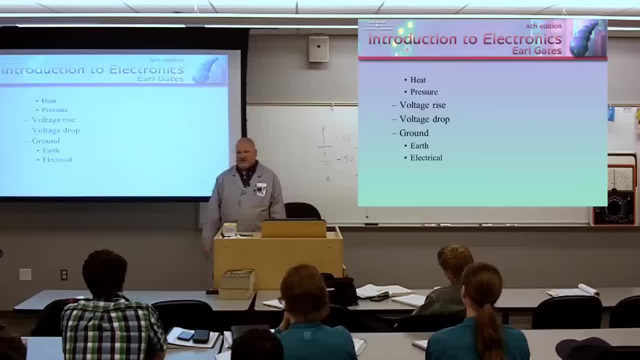 Go ahead, make a stab at it. You know how much wiring it saves on your car. Saves half the wiring. If your car was made out of composites and it was not a conductive material, you would have double the amount of wires. 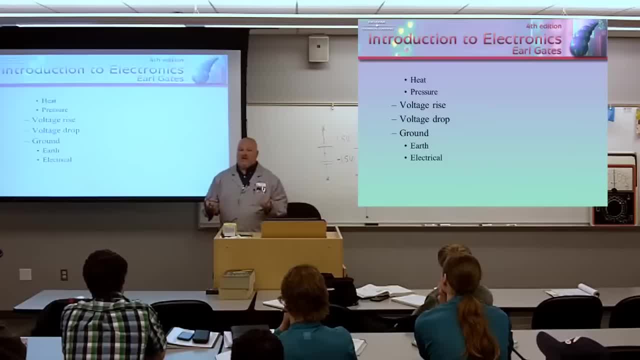 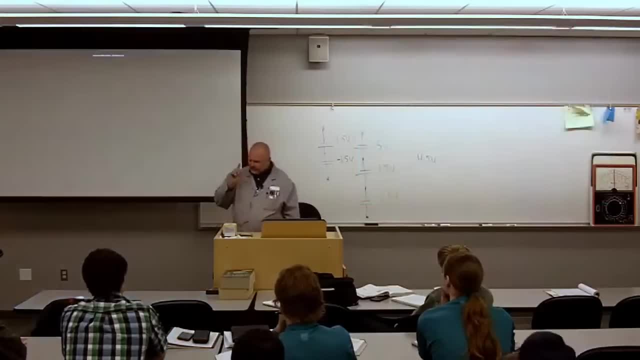 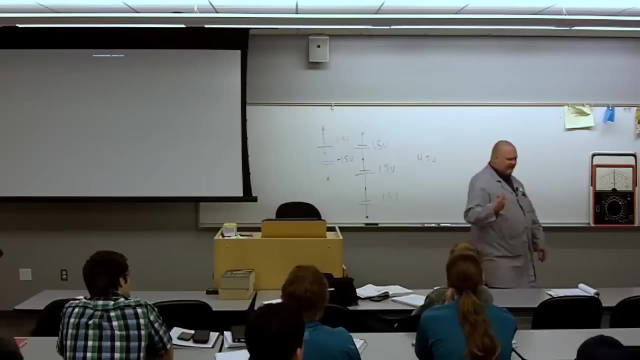 on your car Because we use the chassis as an electrical connection, Make sense? Okay, I've got a question for you And I'm going to ask you about this in our next lecture, And I want you to discuss this in teams and as a class. 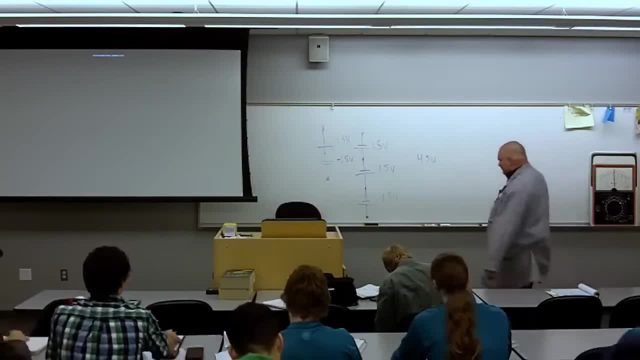 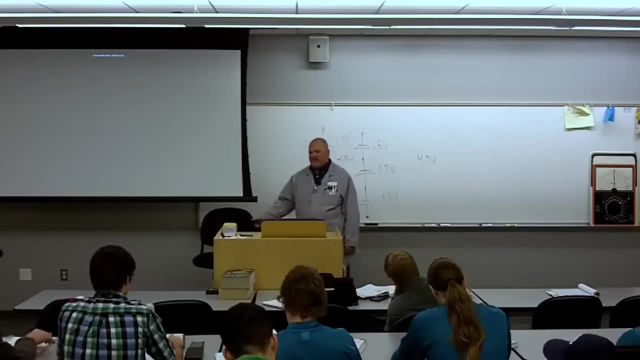 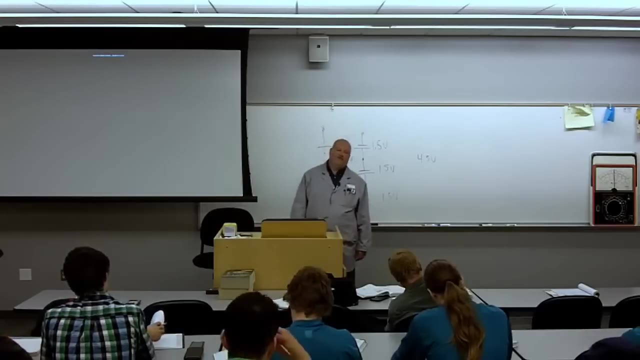 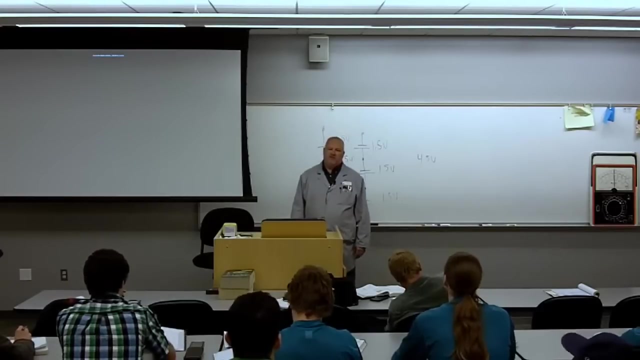 Since there are six different methods of producing voltage, I am going to design a deep space probe To boldly go where no man has gone before. So this deep space probe is going to probe deep space. That's why it's called deep space probe. 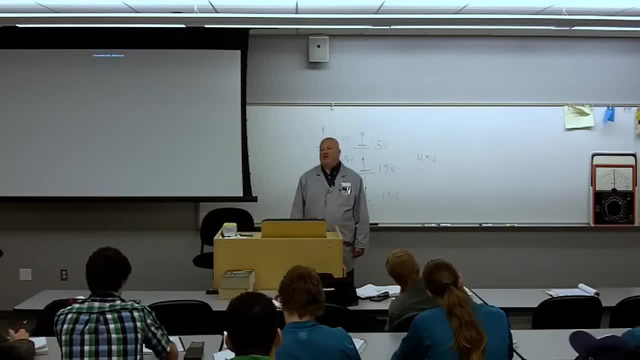 What method should I use to power this thing In outer space So that it keeps going and going and going, And sending data back to earth through a high power transmitter so we could monitor its journey from afar? I want you to think about this. 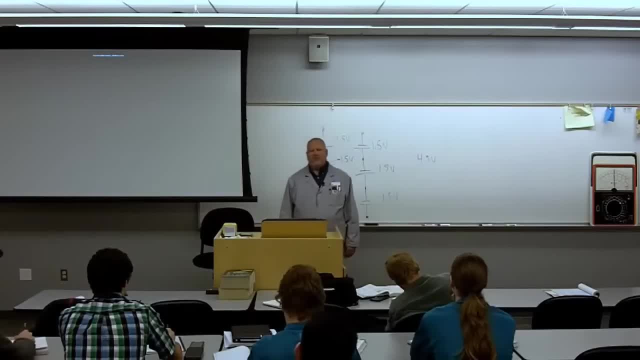 I want you to discuss it as teams And next week when we lecture on ELEC 110, I'm going to expect an answer from you, And it better be the right answer, Or all hell is going to break loose. Any questions? 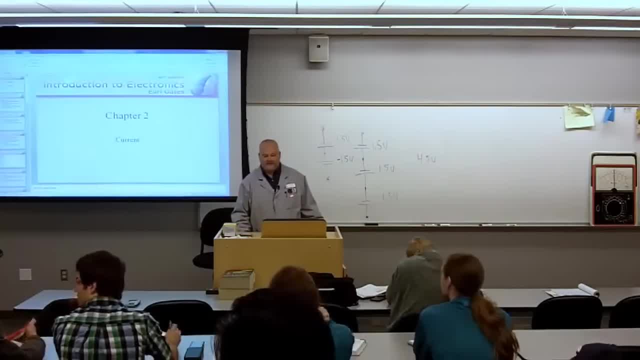 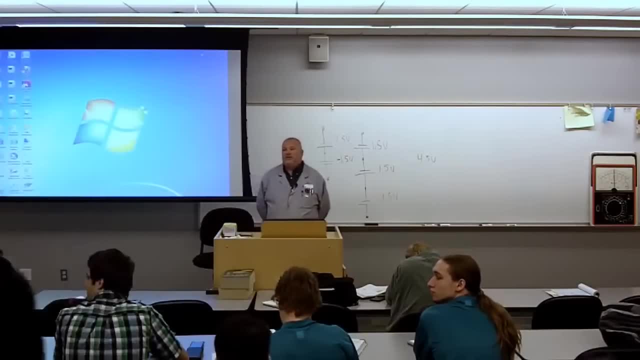 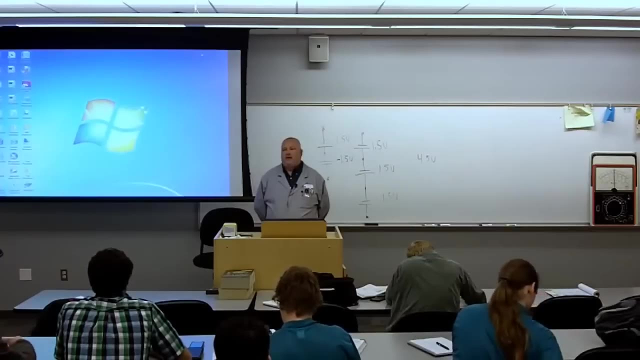 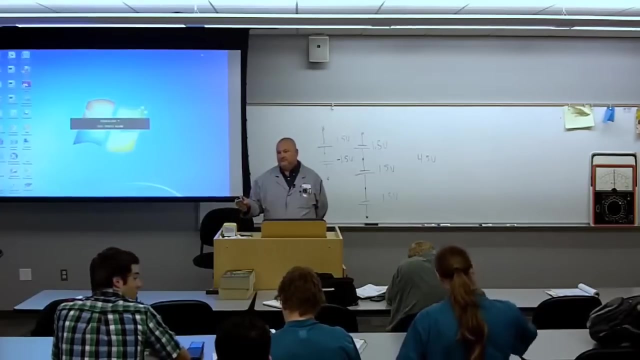 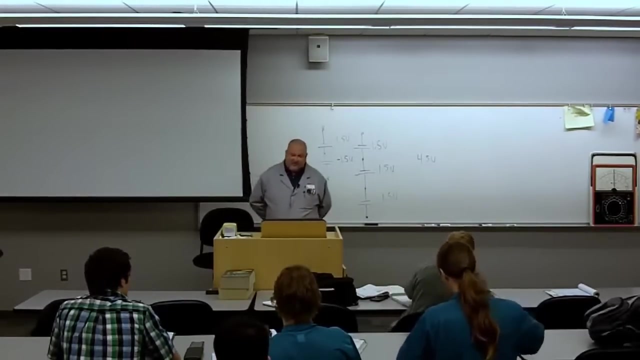 Question: I was wondering why radioactive material is always radiating something. right, It's radiating something absolutely. I always found it strange like we're never able to figure out a way to generate electricity out of the radiation itself. is that at all? 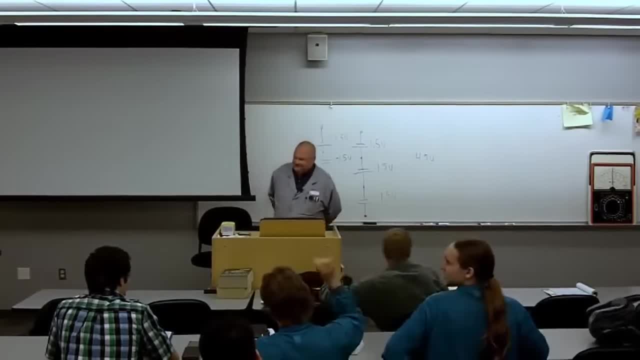 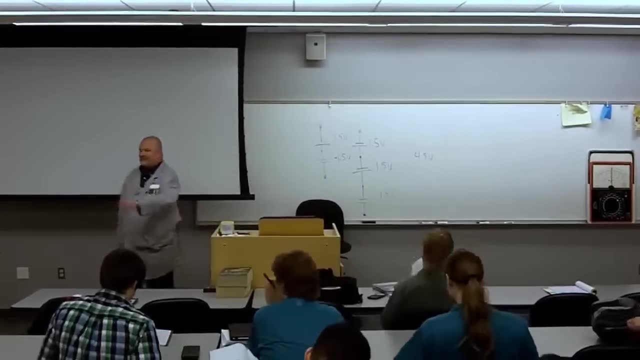 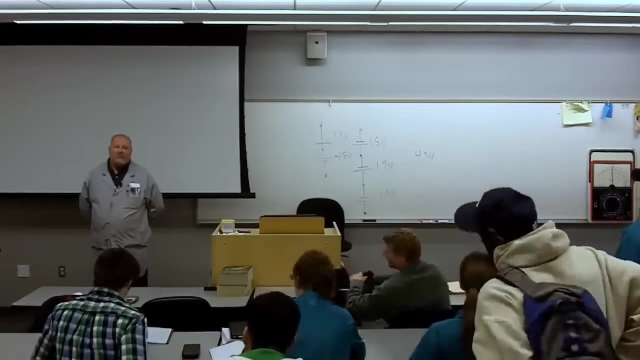 Sounds like you've got some good ideas that are worth pursuing. Enough said, We've got somebody in here that's thinking that's cool. Question: How do you measure ground? It is measured in ohms. What you do is you have to. it's a comparative process. 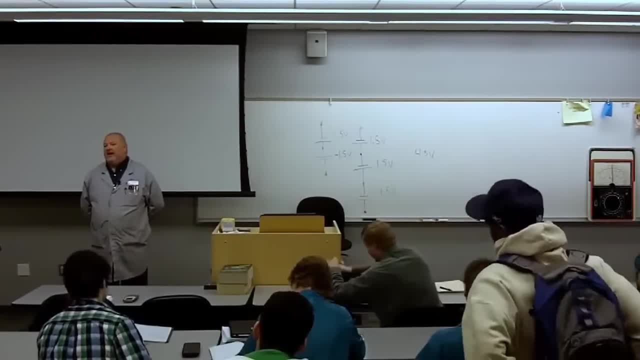 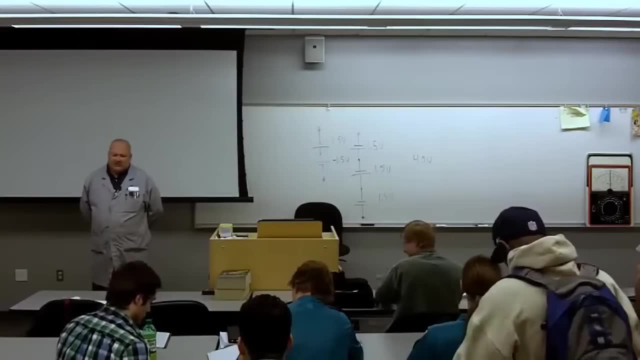 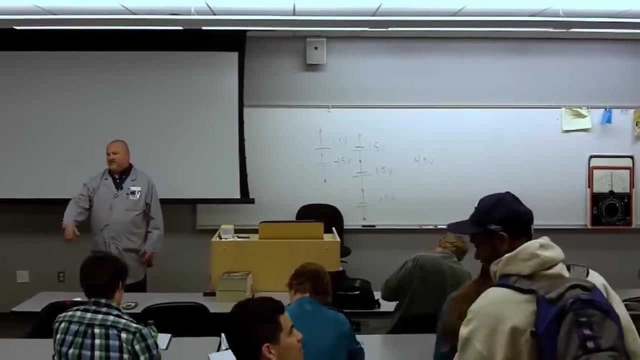 of what you assume is a good ground And you're basically comparing your ground- unknown ground- to that good ground. But there's an assumption made, by getting an eight foot long rod and driving it in, that that is providing you with an adequate 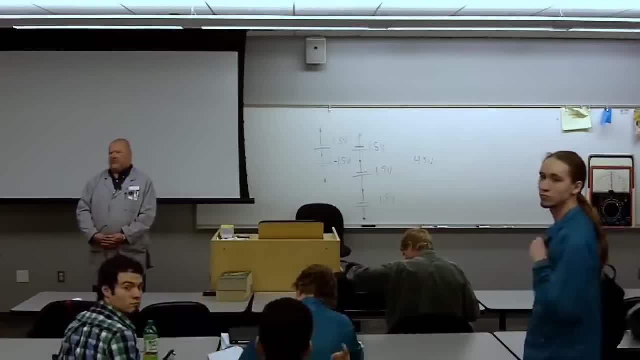 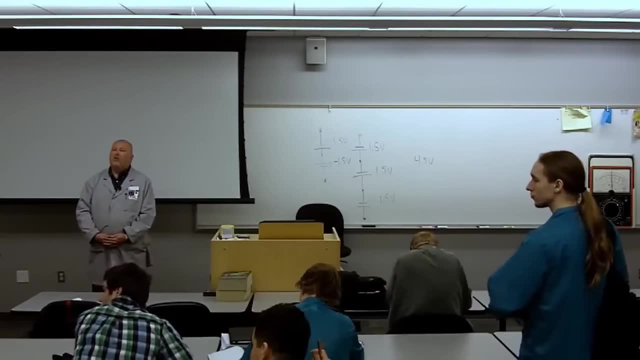 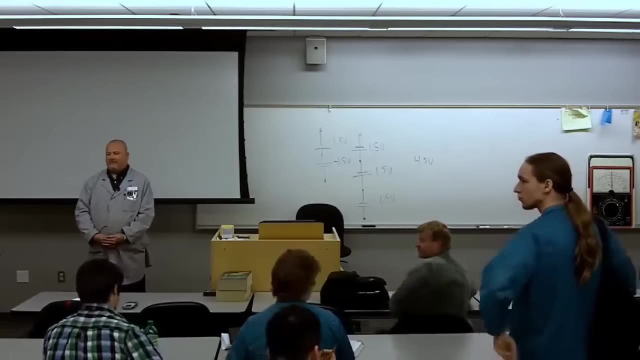 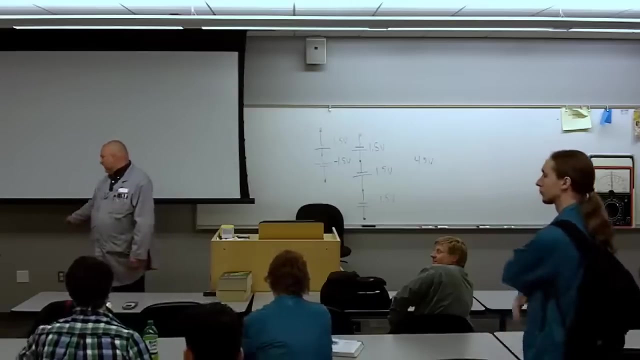 ground. You need something else to compare it to in order for your assessment to be accurate. What are you measuring it in reference to? I don't know An electrical outlet, What you're doing from an electrical outlet. if I wanted to verify that this is a good ground. 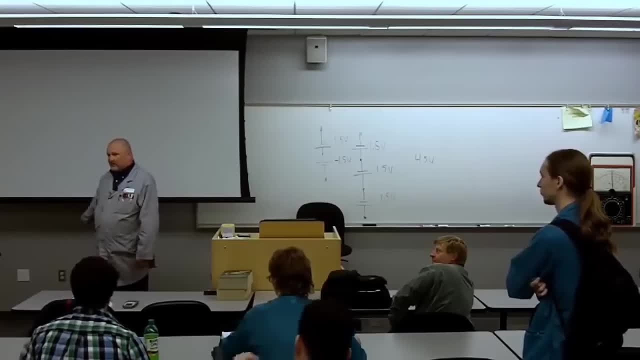 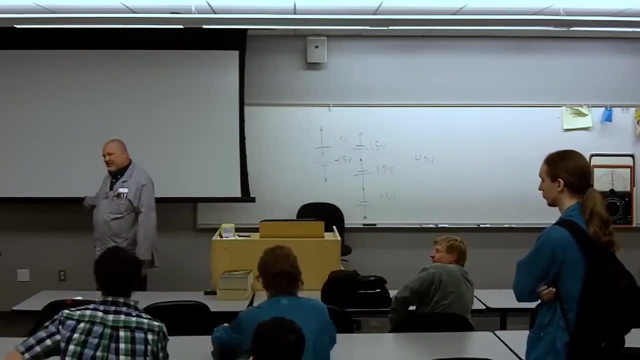 in actuality, what I need to do here is I can measure ground against my neutral. Those two should be connected back at that box. So between the hot lead and ground and between the hot lead and neutral, I should end up with the same difference in. 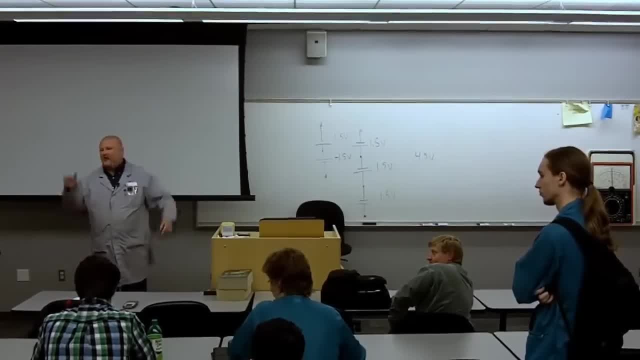 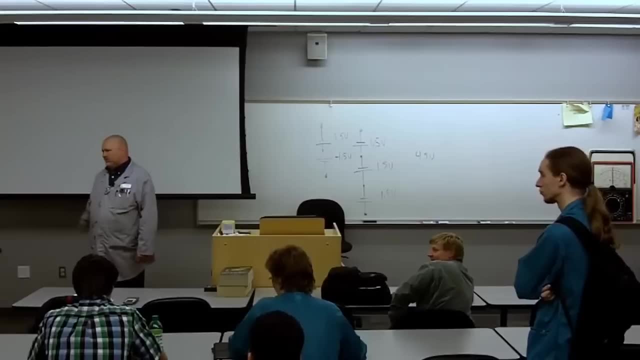 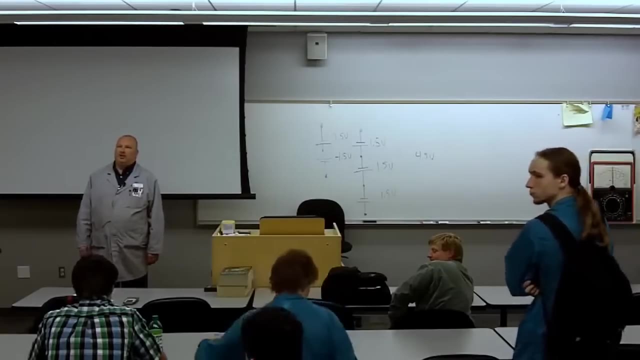 potential. Then going with a multimeter to that box, I should get that same difference in potential across the two. And that basically is letting me know that the ground and the neutral for that particular circuit are valid. But for you to compare a good earth ground to 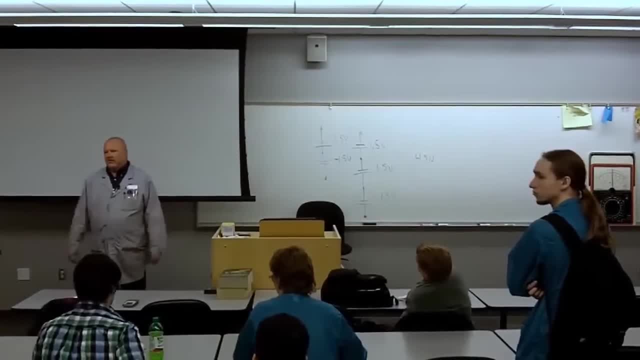 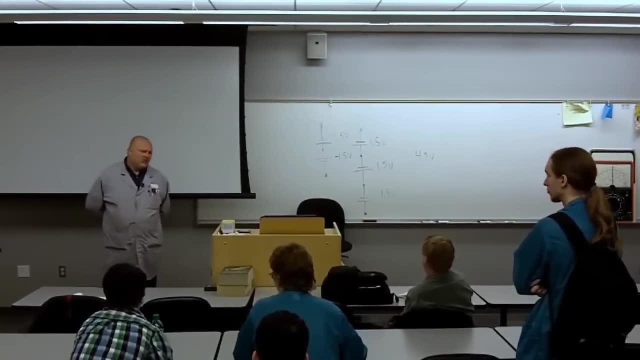 a not so good earth ground. I don't know how you'd go about that other than you've got to basically know that one of them is good, And that's actually one of the things about ground too that I don't know if any of you are aware. 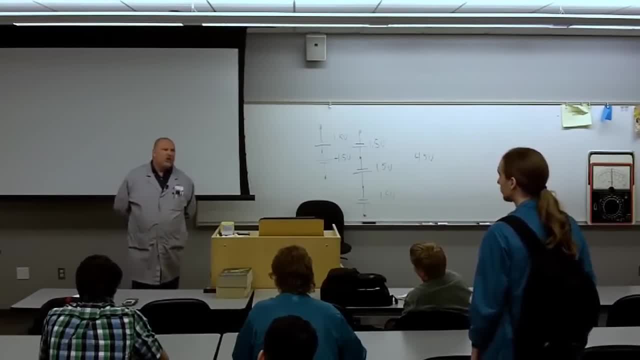 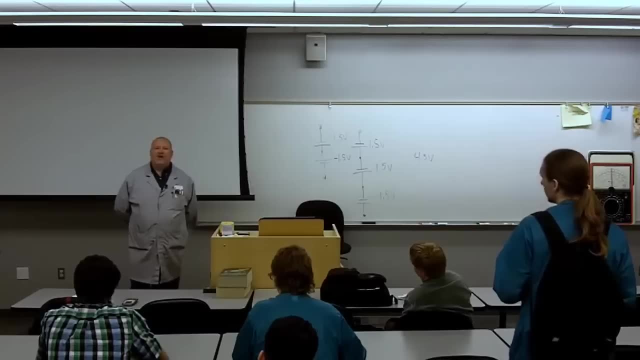 a lot of AM radio stations are located in swamp lands. It's the best place that you could put an AM radio station, Because in a swampy area you get a really good ground, So you get a really good ground plane And because of the frequencies that you radiate at. 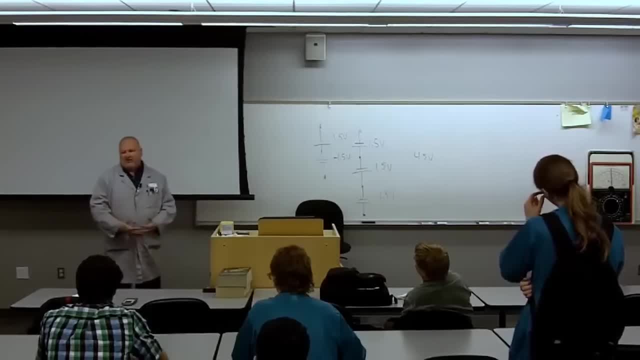 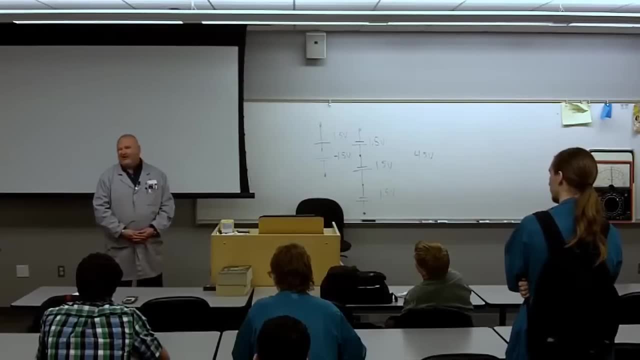 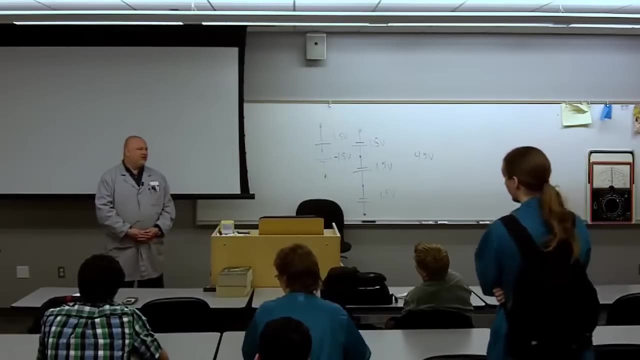 it's going to ensure much better transmission of that RF signal. A second choice is also a field, a pasture, where cows graze and urinate and keep everything nice and moist and healthy. That's why even in New York City- growing up in Connecticut- all the New York City radio. 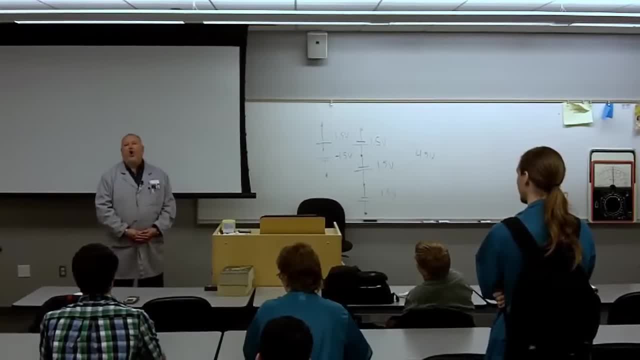 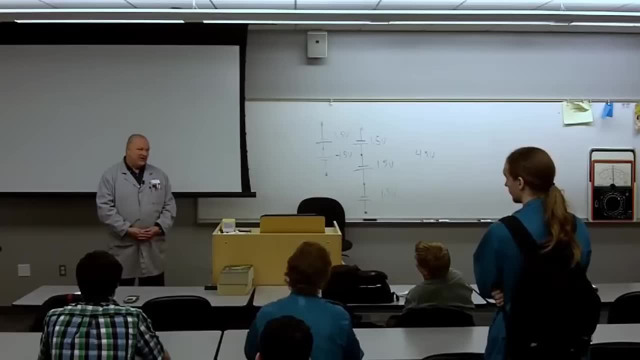 stations- WABC, WNBC, WCBS. all of their transmitters were located in New Jersey, the Meadowlands. If there's any Giant fans here, that's where all their transmitters were located. Why? Because it was a marshy location. FM transmitters. Different. If you're in New York City, where do you want to put an FM transmitter? Top of the Empire State Building? Why? Because it's the highest, It doesn't have as much to do. You still need a good ground, but it's not as essential. 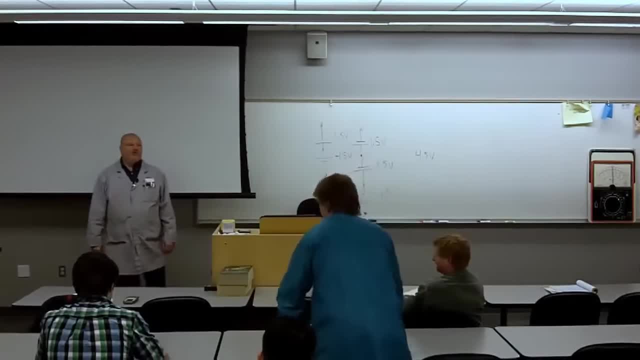 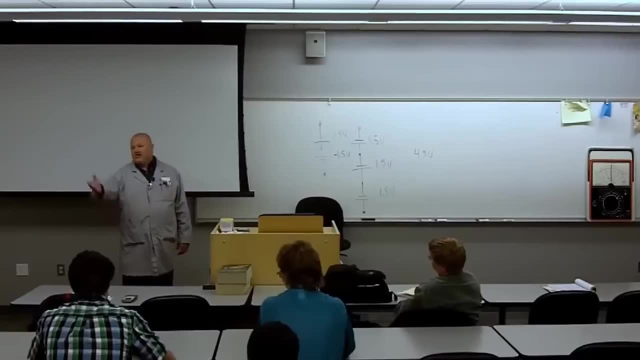 as that low frequency transmitters. So ground is important, folks. We're going to talk more about it. We could have a course in ground. We honestly could Five credit classes just talk about ground Testing processes. you know some of the different things. 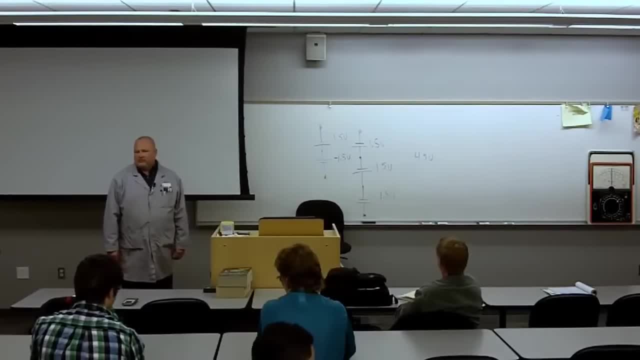 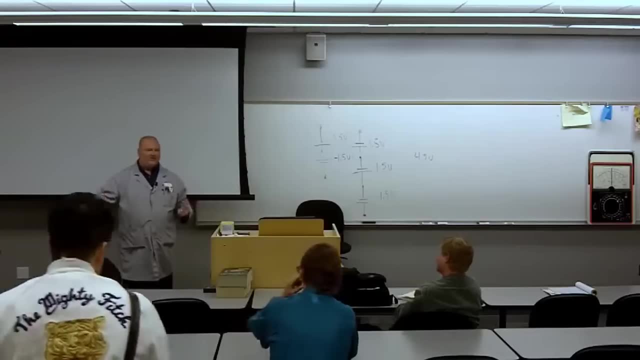 Things that we've encountered with ground. Fifty years ago, thirty years ago, twenty years ago, ground wasn't that big of a deal. Ground right now is very, very big Because a difference equates to a difference in potential And even a small difference in voltage could create. 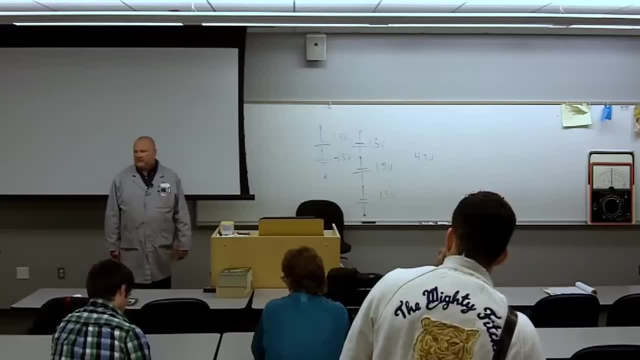 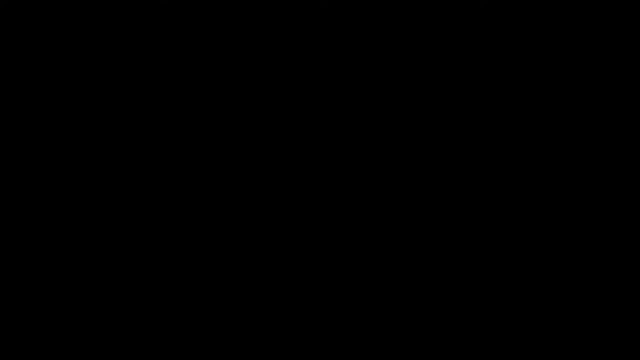 a circuit, It causes that circuit to go. here's your final technical term for the night: cattywampus, Alright, Alright, that's all I got. folks Have a good day. Okay, let's get started. Chapter four: 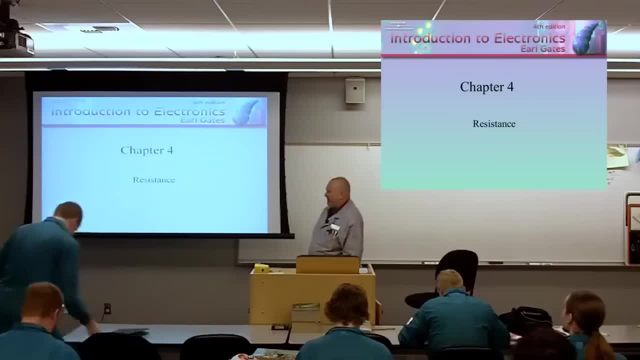 Chapter four, Just kind of as a review to get us up to speed with what we've talked about thus far. We talked about the fundamental physics of electricity: Where does electricity come from and what subatomic properties mean to both materials, the type of materials that we use in. 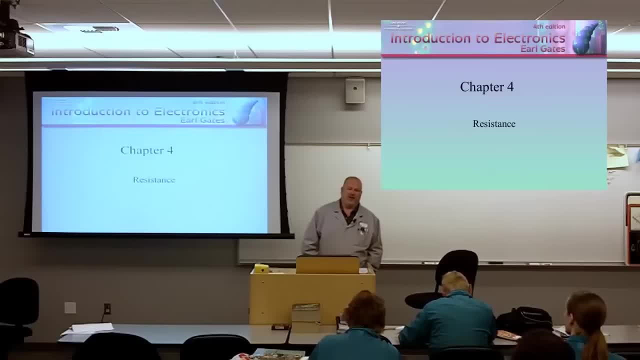 harnessing electricity and electronics and also how materials are affected when we apply energy to them. When we apply energy to matter, we could knock some electrons free from the valence shell. When we knock those electrons free from the valence shell, that represents potential energy right. 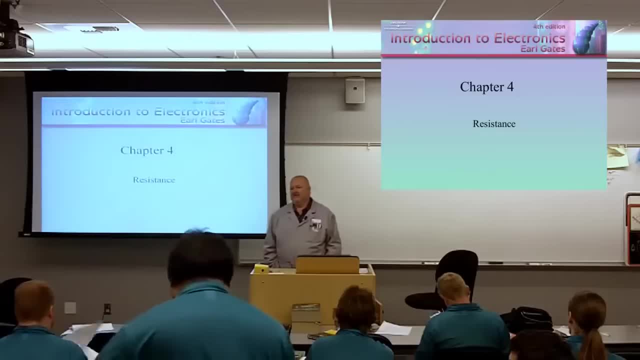 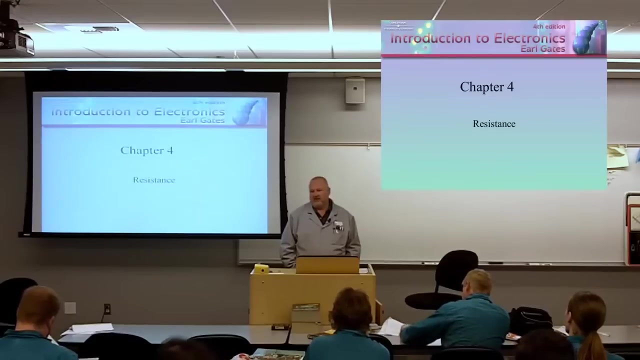 Because we could direct those free electrons through a circuit and make them do some work for us, Right? So we call that flow of electrons, current Current, The flow of electrons in a specified direction. And that specified direction is negative to positive And every 6.24 times 10 to the 18th. 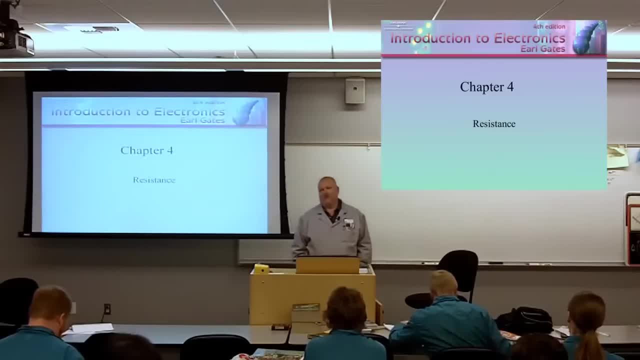 electrons equals one coulomb. One coulomb per second equals one ampere. So we talked about current already. The next thing we're going to talk about tonight in chapter four is resistance, Or as the French would say, resistance, Maybe not Resistance. 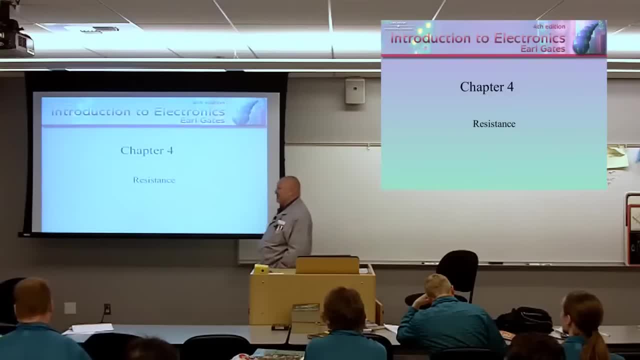 And this is kind of easy to remember. One of the questions that I'm going to ask you in the future in lecture is going to be: what has resistance? And the answer is easy: Everything has resistance, Everything. Some things have more resistance than others, but basically everything. 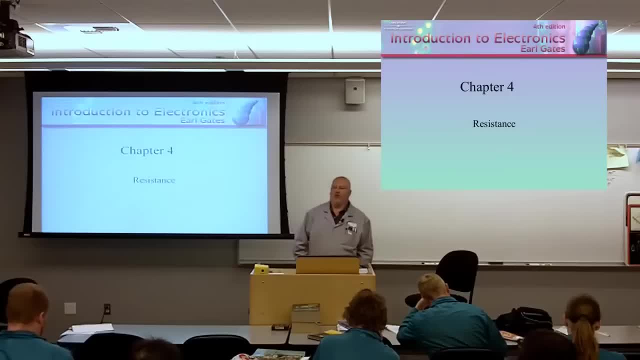 has resistance. There's only one thing that I'm aware of that doesn't have resistance, and it only exists in a laboratory. What am I talking about? Superconductor, Superconductor, Superconductivity is the utilization of materials that have no resistance Zero. 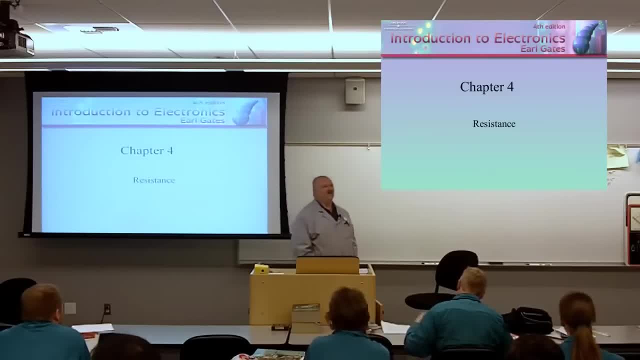 resistance. So once we get that stuff up and running, once science masters that they're going to be dealing with materials that have no resistance, And that's going to revolutionize the industry, Because right now it's something we've just got to deal with and there's a lot of losses. 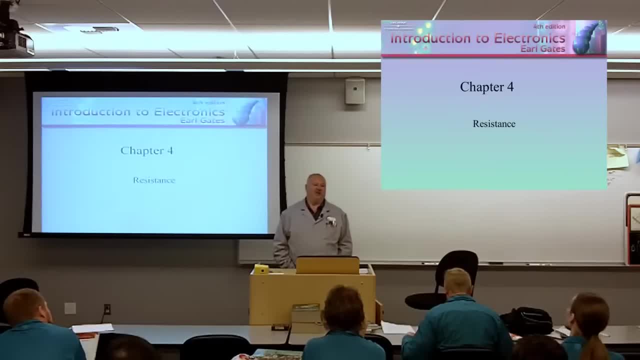 associated with it. The power companies would love to get a hold of superconductivity at room temperature. They'd love to harness that Question. Do modern computers have superconductors? No, No, It is not feasible right now for any everyday use, It only. 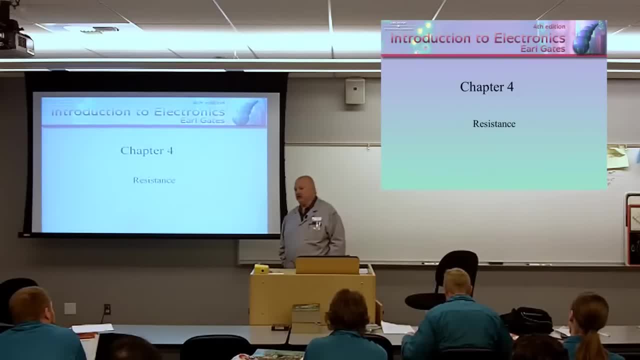 exists in a laboratory, at extremely cold temperatures, The use of a cryogenics, And, believe it or not, I shared with you right. what material are they having the best luck with? Ceramics, Ceramics- Who would have thunk Ceramics? 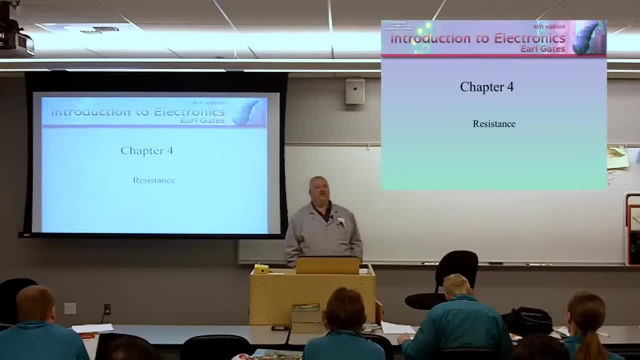 Ceramic, A great insulator at room temperature. but at these extremely cold temperatures some of these ceramics take on superconductive properties. Anyway, we're not going to talk anymore about that. I'd love to, but we just don't have time. What we've got? 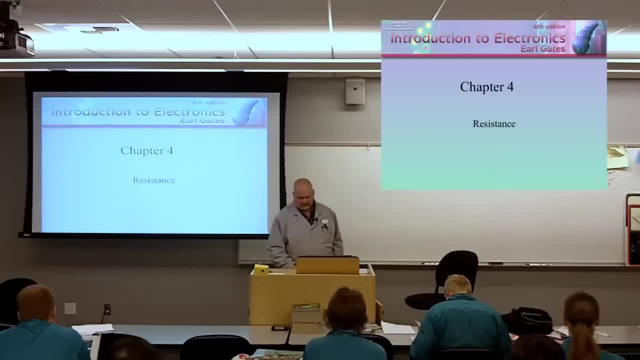 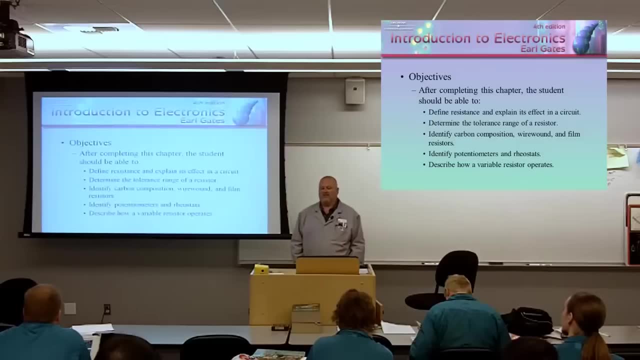 to do is embark on our journey here. Chapter 4, resistance. After completing this chapter, you're going to be able to define resistance and explain its effect in a circuit, Determine the tolerance range of a resistor. Identify carbon composition: wire wound. 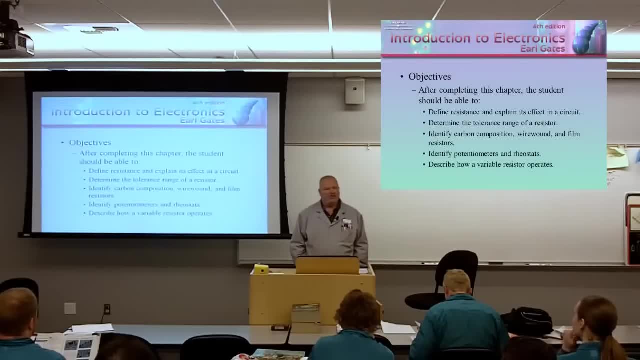 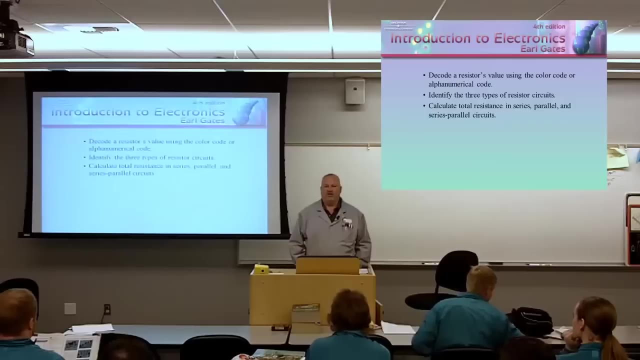 and film resistors. Identify potentiometers and rheostats. Describe how a variable resistor operates. Decode a resistor's value using a color code or alphanumeric code. Identify the three types of resistor circuits and calculate out total resistance in series parallel and series parallel circuits. 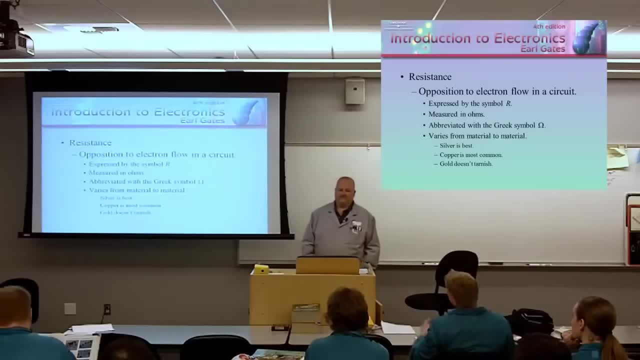 Resistance is the opposition to electron flow in a circuit. What has resistance? Everything Except superconductors. Everything, Everything has resistance. If you went out and bought a new extension cord over the weekend, even though you paid a lot of money and it's a really good, high quality extension. 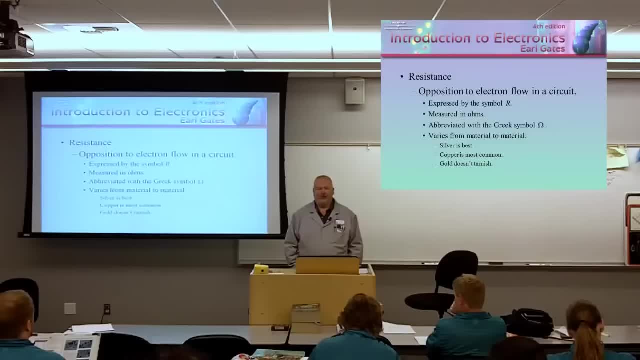 cord, it still has resistance. If you went out and bought cable for your speakers, you're rewiring your house and you're putting in some new speakers and you went out and got some of that monster cable. It cost you a fortune. 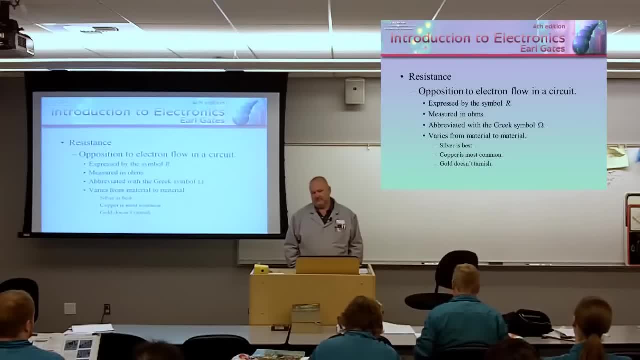 Still has resistance. Everything has resistance. It's expressed by the symbol R. It's measured in ohms O-H-M-S. Ohms Discovered by a guy by the name of John Ohms, Abbreviated with the Greek symbol omega, The Greek. 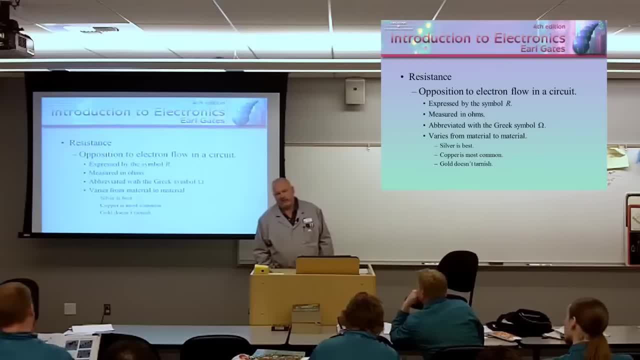 symbol omega. And although everything has resistance, the amount of resistance varies from material to material. Silver is the best meaning it has the least Found in nature. So if you went out to the periodic table, played around with it and tried to find what materials on the periodic table you could, 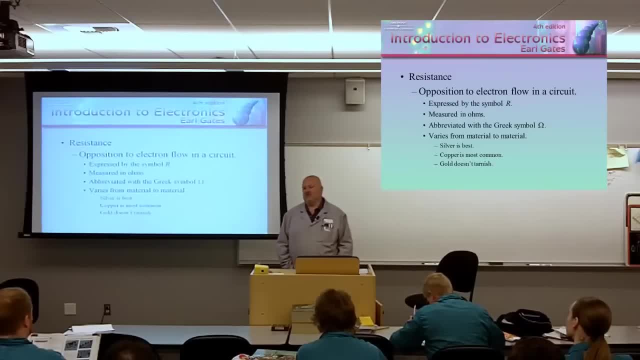 find and which one had the least resistance. it would be silver. Copper is the most common, meaning. it's really the cheapest, even though it's expensive In the grand scheme of things. that's why you've got these people like cannibalizing stuff, taking stuff apart to steal the. 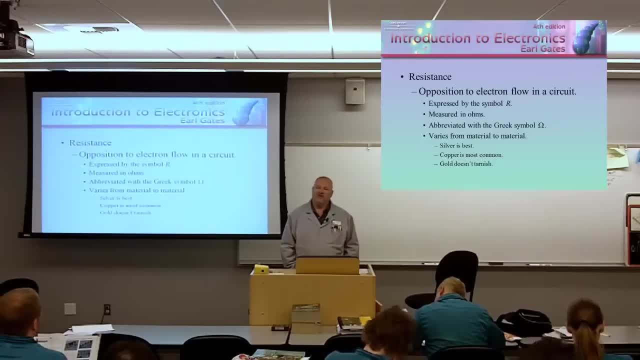 freaking wire. What took the cake was: did you hear down in Tacoma a couple months ago? they've got that drawbridge down by downtown Tacoma. the big ships go underneath The cannibal. they just got in there one night and they tore it all up. 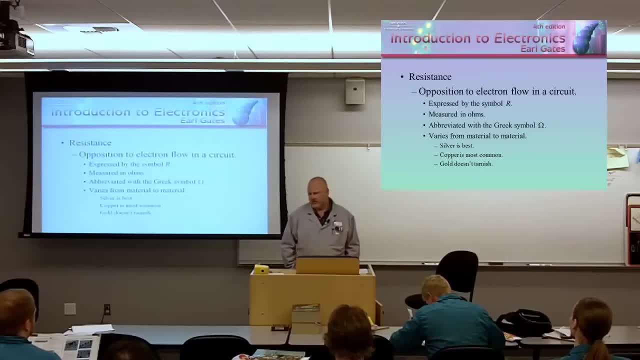 The control panel. it's gonna- I don't know- it's like millions of dollars to rebuild this thing And they just stole all the wire out of it, gutted it and just started turning it into a recycling place. Yeah, I got all this wire. 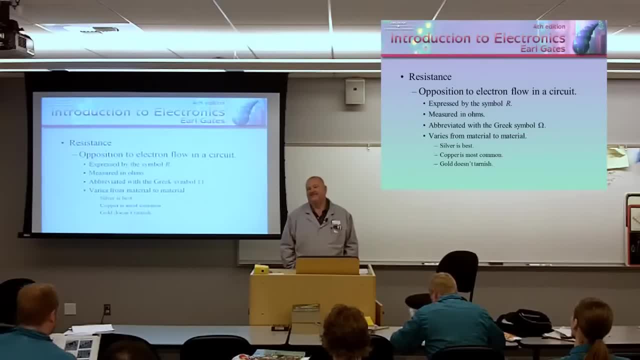 Sure, you know how much You're kidding. Huh, That's nuts For legitimate people. That's nuts. Now, Washington or Oregon Washington? Huh, Alright, Gold doesn't tarnish, So although gold is not as good a conductor as silver, 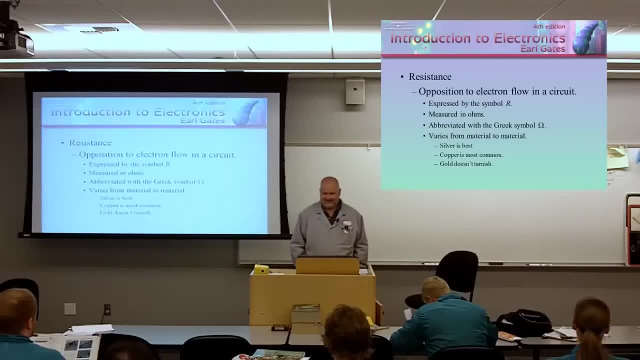 by plating it, by plating copper with gold, then you get the best of both worlds. You have something that doesn't tarnish, Because the problem with silver, if any of you have any silver jewelry or silverware about the same time. 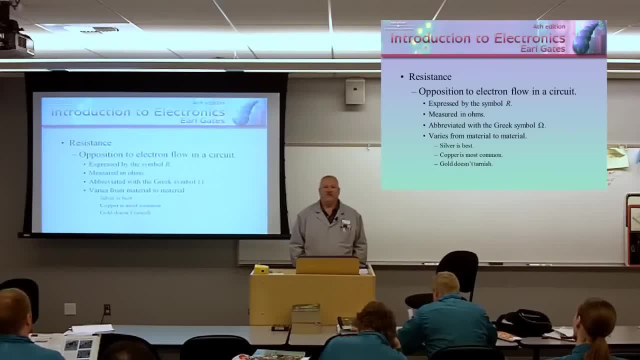 you're done polishing it, you need to polish it again Because being exposed to oxygen oxidizes it. Gold, that doesn't happen. No, oxidation means you get a superior connection when you use it as a termination on an electrical connector. Resistance is affected by temperature. 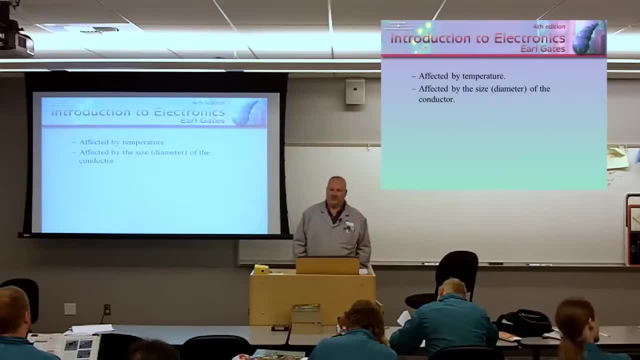 It is affected by temperature. Typically, resistance has a positive temperature coefficient. we call it Positive temperature coefficient, meaning as temperature increases, the amount of resistance in a conductor increases, Which is a problem If you have an extension cord and it starts to get. 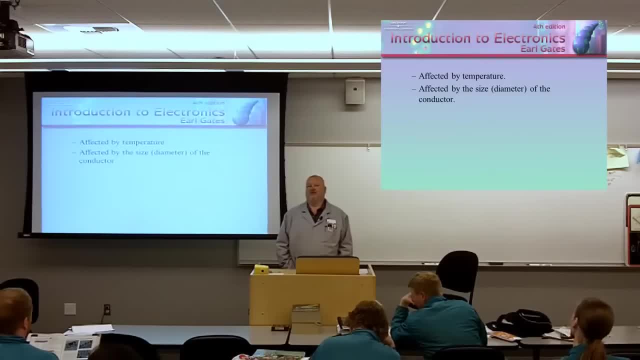 hot, the extension cord is going to possess more resistance. If it possesses more resistance, that means less current makes it to your load and the extension cord is going to get even hotter. If it gets even hotter, its resistance is going to increase more, limiting the amount of current even more. 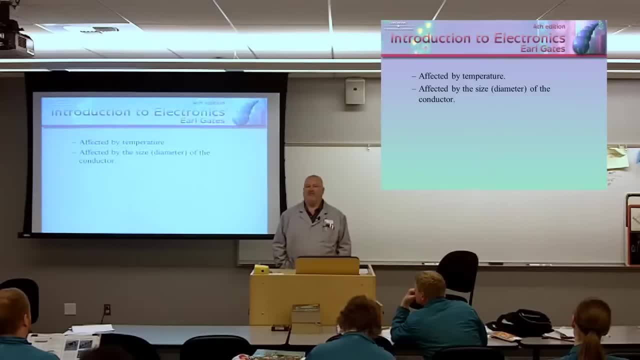 that's going. So that's where you end up with a vicious cycle. You let that go on long enough, you end up with an electrical fire. So keep that in mind. If you've got an extension cord or a cable that's getting warm, getting hot, it's a problem. 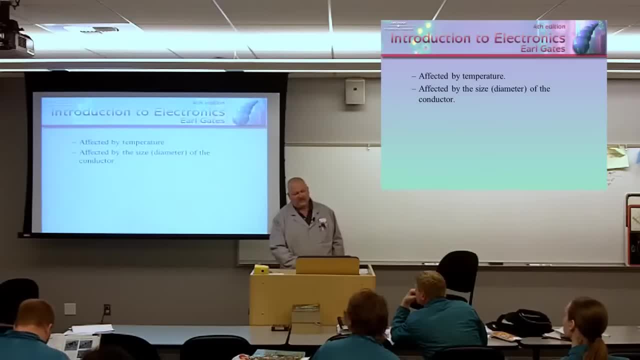 It's also affected by size. Size does matter when it comes to conductors. Basically, the individual that has the thickest conductor will have the least amount of resistance. So earlier in lecture, when I said about connecting up your speakers using that monster cable- if you really are using monster cable- 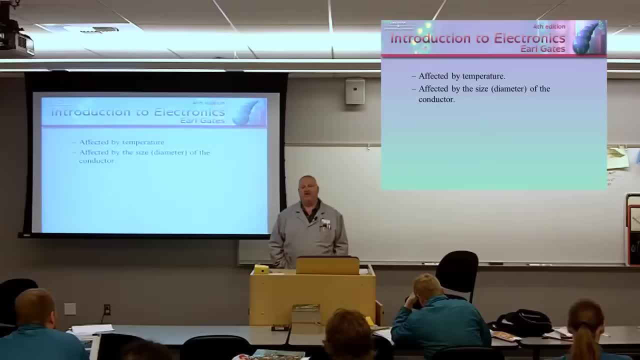 and that cable is really thick. the thicker it is, the least resistance it has, The more energy you transfer from the source to the load, From your amplifier to the speaker, And that's a good thing. So, generally speaking, you want to use the thickest conductor that you can afford. Or, of course, adhere to standard manufacturing processes, And there's tables that you could find that show specifically what is required. Electrical code dictates that In your home. the majority of circuits in your home are 15 amp circuits. They can handle up to 15 amps. 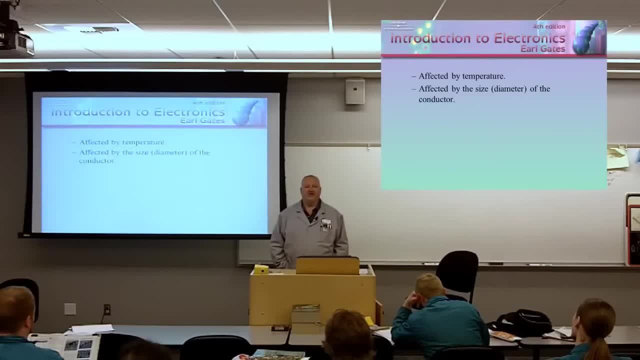 Standard electrical code dictates that you need to use at least 14 gauge wire for those circuits, For 20 amp circuits. you have some 20 amp circuits in your house, maybe in your kitchen or out in your garage, your work room, your. 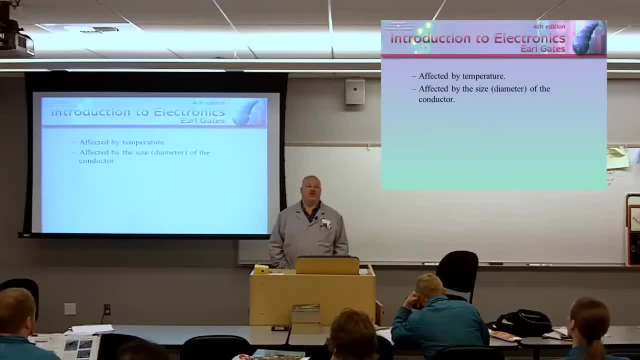 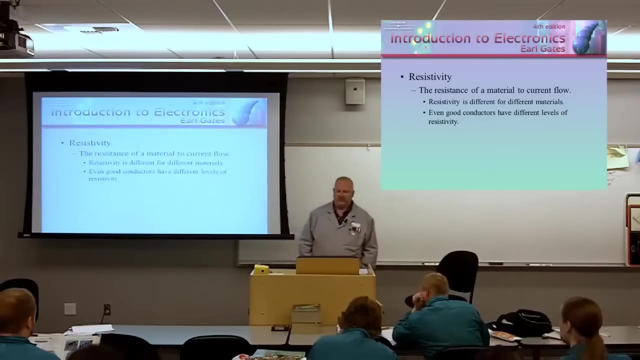 utility room Electrical code dictates that you have 12 gauge wire minimum. That means that the wire is thick enough to support the flow of 20 amps of current. Resistivity is the resistance of a material to current flow. Resistivity is going to be different for different materials. 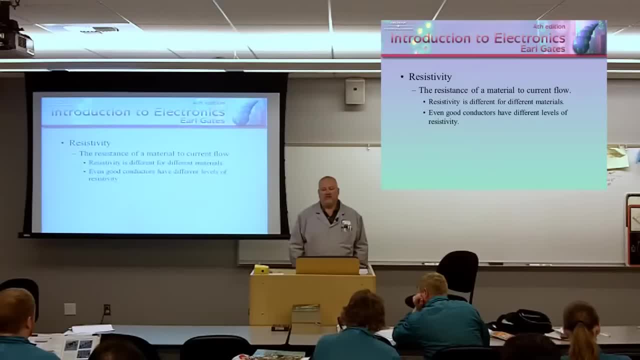 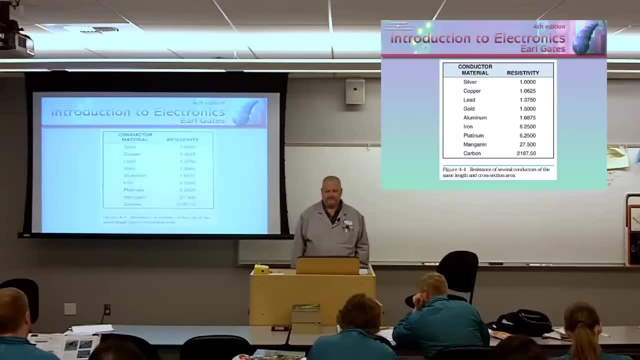 Even good conductors have different levels of resistivity. Here is a table that shows us the resistivity, And what we use as a benchmark is the resistivity of silver. There's a lot of things in science that we do like this One we were talking about last week, Remember? I talked about specific gravity. 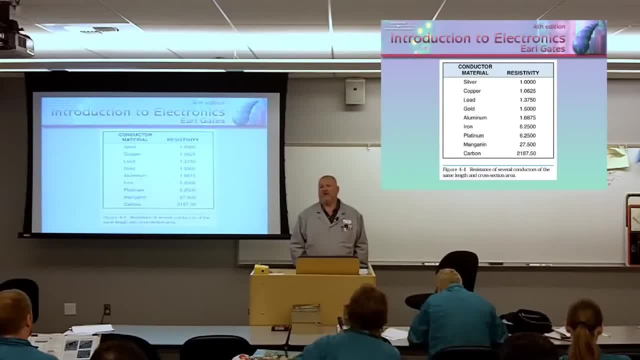 Remember specific gravity. Specific gravity is a benchmark that we use with fluids And we compare everything to the specific gravity of pure water, H2O at room temperature, Typically 65 degrees standard temperature, And we say that it has a specific gravity of. 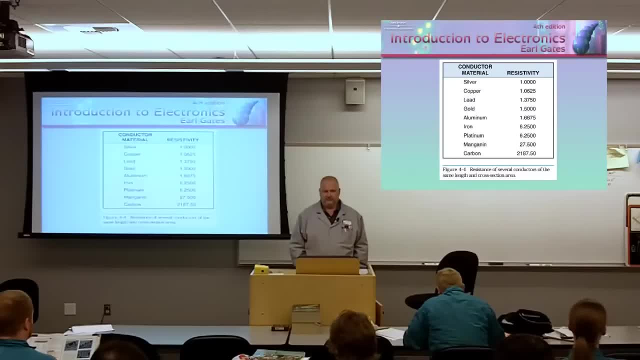 1.000.. In dealing with conductors, we use resistivity, which compares resistivity to that to the best known conductor that we have found in nature, which is silver. So we say that resistivity has a- or, excuse me, silver has a resistivity of. 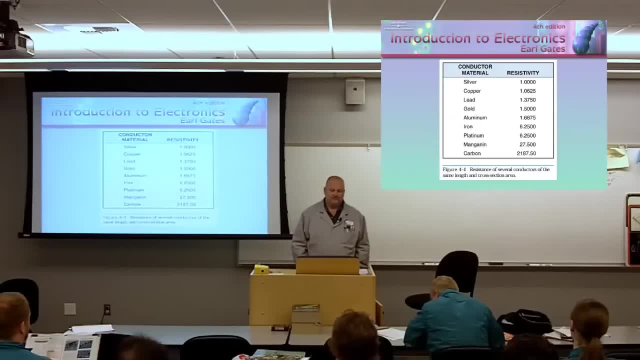 1.0000.. Copper 1.0625.. Lead 1.3750.. Copper 1.0625.. Lead 1.3750.. Gold 1.5.. And you can see the rest of the table there. 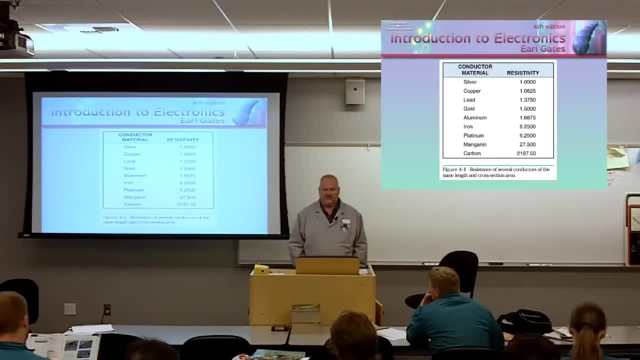 This compares all resistivity of all materials. So silver has the least resistance, it's the best, so therefore it has a resistivity we use as a benchmark of 1.000.. So do you understand the difference between resistivity and resistance? 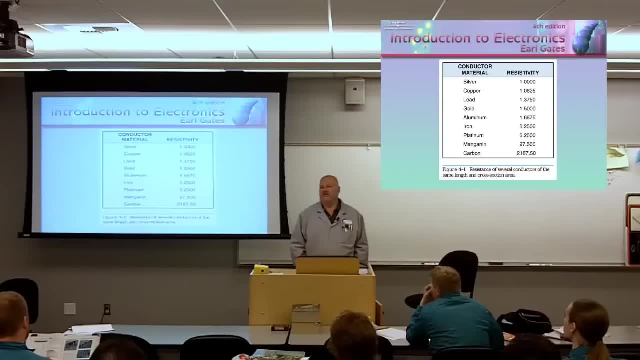 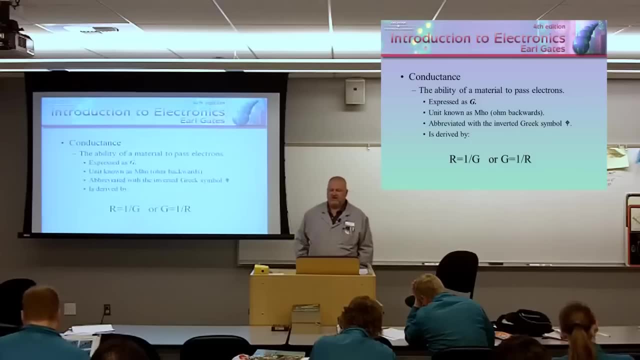 Resistance is measured in ohms. Resistivity compares everything to silver Conductance: The ability of a material to pass electrons Conductance. It's expressed as the capital letter G and, believe it or not, I'm not making this up. 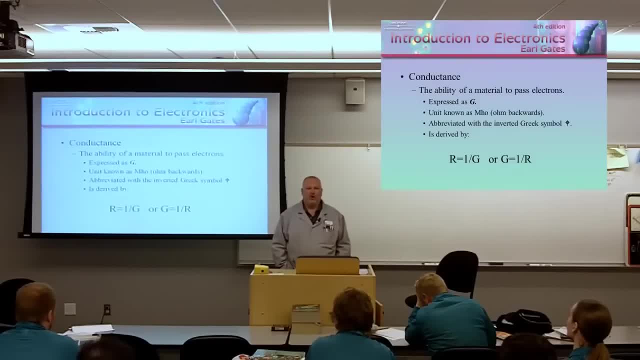 the unit that we measure this in is called the MO M-H-O. It's ohm spelled backwards, And that's not by mistake. Basically, the dude that came up with this said: I'm going to spell ohm backwards. take the reciprocal of resistance and call it the MO. 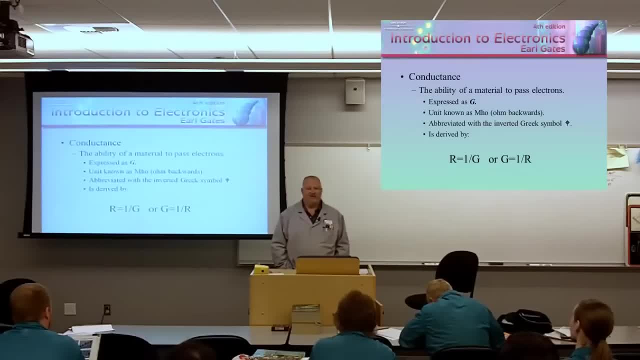 And see if that makes the textbooks. Well, it made the textbooks, but it's not the unit of measure that we've adopted for measuring resistance. It is the unit we measure conductance with. It's abbreviated with the Greek symbol. it should be an upside down omega. 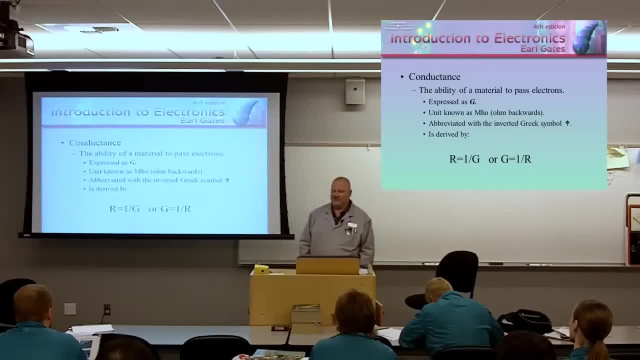 I don't know why. it gives me like an orthodox cross, But since that orthodox cross appeared on my slide, I'm not inclined to remove it. if you know what I mean It's. It may be a sign, But all's it should be is an upside down omega. 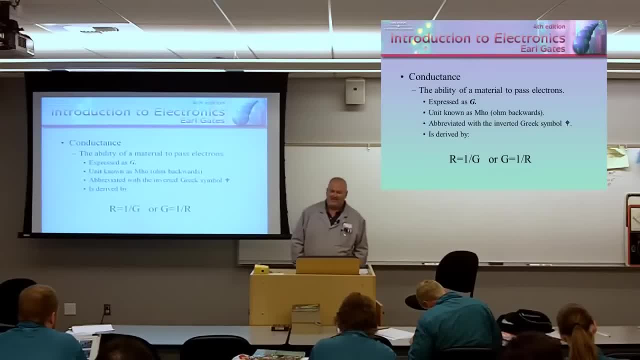 A guy by the name of Siemens came up with this. Have any of you heard of Siemens before Siemens Corporation? Well, this was like great, great, great grandad Siemens, And he made the textbooks by playing around with electrical properties And the rest of that company. 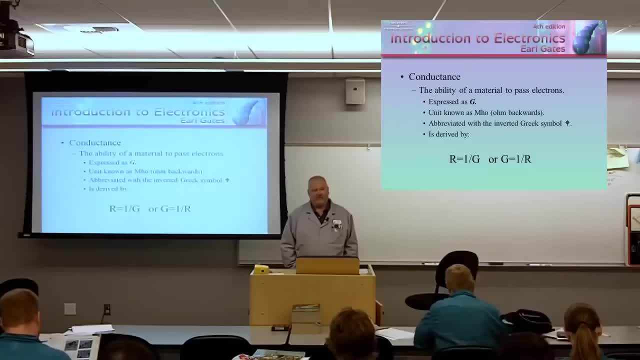 of course, is history And what Siemens said. I guess he was in a big argument with Ohm back in the day. Ohm said we should measure materials all for their resistance. Siemens said, no, we shouldn't. We should measure it all for their conductance. 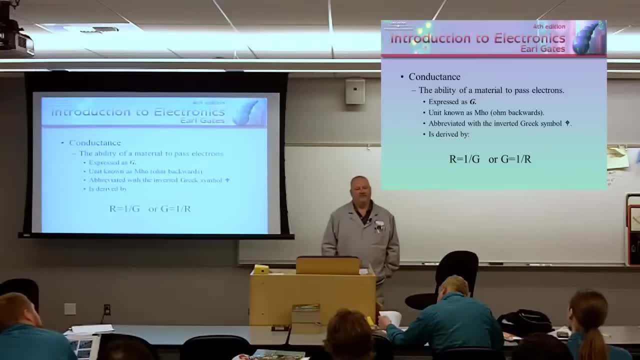 Resistance is measured in Ohms, Siemens is like uh, conductance is measured in Mohs. It's Ohm spelled backwards. Well, how do you calculate it? Well, it's real simple. What you do here is you take the reciprocal of resistance, One over resistance. 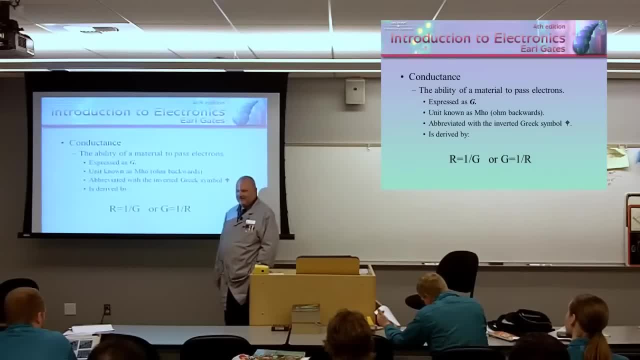 equals conductance, And I guess the guy said this to his face, with a straight face. So what do you say? the answer is, you know, I say the answer is a thousand Ohms. Well, one divided by a thousand. well, that's how many. 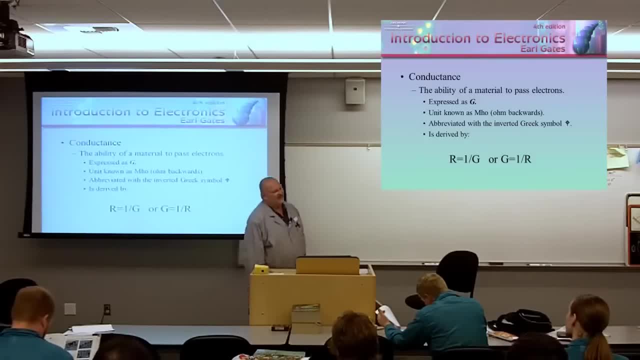 Mohs, I think it is, And actually, since it's thousands of Ohms, taking the reciprocal of it means that most of our answers will actually be in millimohs, Millimohs Or micromohs. You can't make this stuff up. 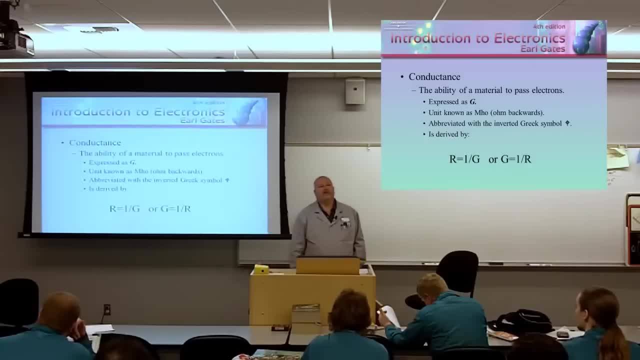 It used to be that I put out in lecture: you will never see a conductivity meter. Anytime I put out any absolutes in lecture, somebody feels compelled to prove the prof wrong. So I stated: you will never see a conductivity meter. and then almost immediately I had a student in my class. 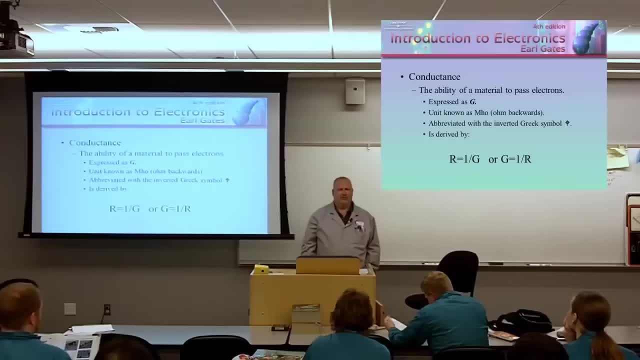 raise their hand And said: I use one every day at work. Really, I've never seen one in my life. Where do you work? And the individual worked actually at a water treatment facility. A water treatment facility, What they use the conductivity meter for, literally. 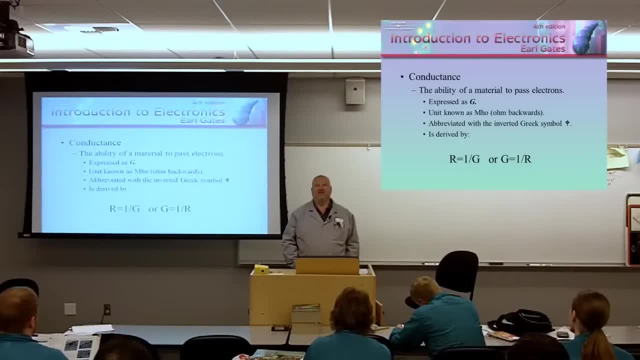 is to see how much stuff is left over in the water after they treat the water, Because I don't know if any of you realize this. is water a conductor or is it an insulator? Semiconductor? Pure water could be an insulator, Not unpure water. would be somewhat of a conductor. 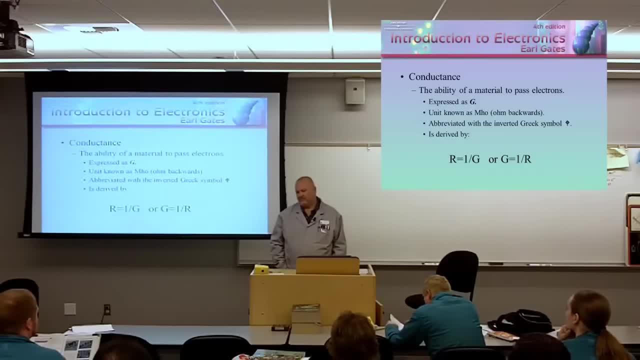 Very good, Very good. Pure water. H2O- Pure water basically, is an insulator. Current will not pass through pure water. So if I'm in my hot tub filled with pure water, my neighbor's wife comes over and joins me. 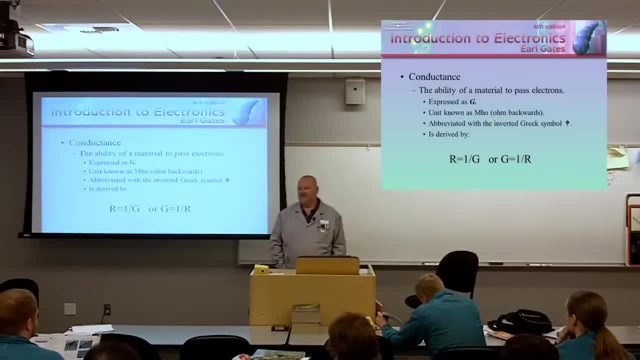 And my wife comes home and says: wow, you look comfortable in there, Would you like a piece of toast? And throws a toaster oven that's plugged in. Provided the tub was filled with pure water- H2O- it wouldn't be a shocking experience. 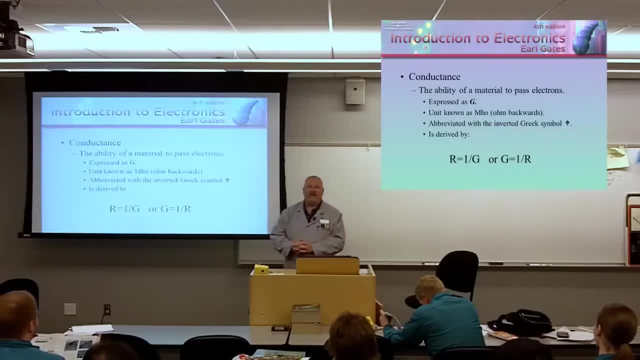 But due to the fact that my water chemistry- actually if I get in the tub, there's going to be salts and oils from my body that are going to contaminate that and immediately take that pure water into the conductive realm. So again, the conductivity meter that my former student was using. 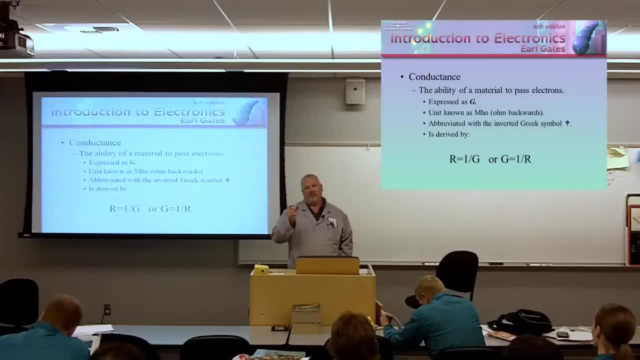 was to measure the conductivity of the water. The more stuff you have in the water, the more conductive it's going to be. I had a terrible bout of bronchitis several years ago- The flu with bronchitis. It was terrible. The verge of pneumonia. I was coughing Fever. Felt miserable. Got up, went to the doctor. It's in the middle of winter. You know how dry our air gets in our homes in the middle of winter. He recommended I go out and get. 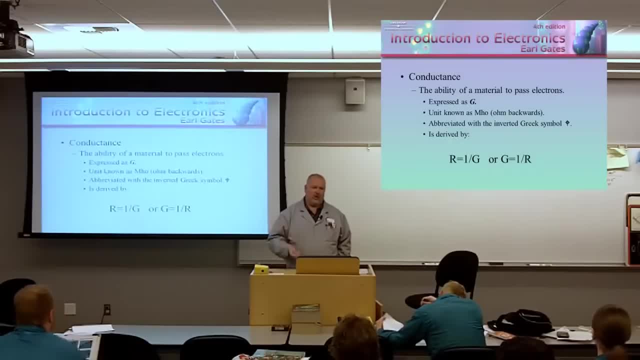 one of those humidifiers. Fill it up with water, plug it in. makes humidity, Puts humidity in the air. So I stopped at Walgreen, picked one up, brought it home. It didn't even have an on-off switch. 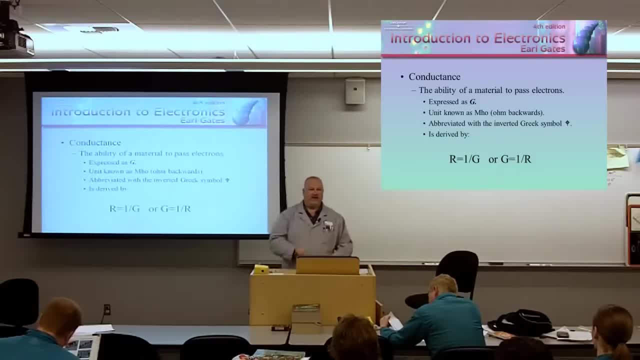 You know it's just a tank of water. You put the thing on, you plug it in and it puts humidity into the air. How tough can this be? So I mustered every ounce of courage that I had, because I really felt like I was dying, Filled the 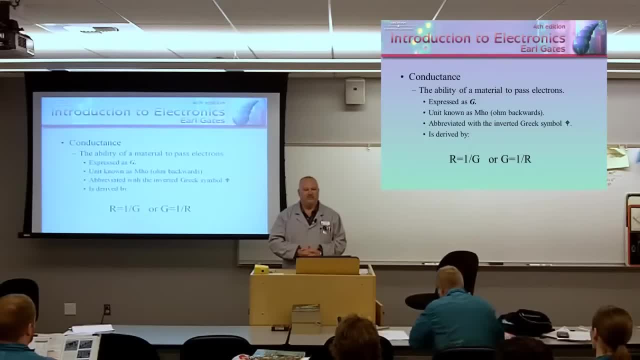 thing up with water Climbed under my covers And I'm looking at the thing sitting over on my nightstand And it's just sitting there. I look at the clock and I continue to watch it. Nothing's happening. I'm like 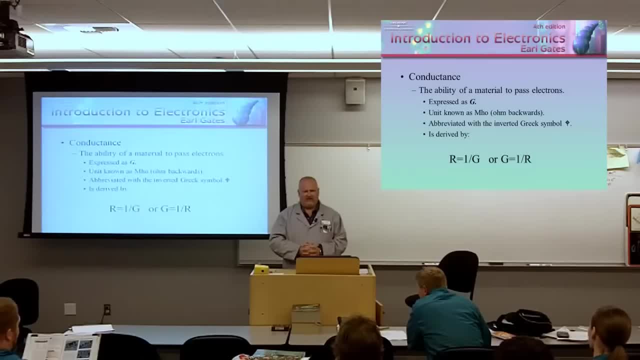 you've got to be kidding me. Okay, This thing's busted, Or worse. yet I've got to read the owner's manual on something that doesn't even have an on-off switch. So I go ahead and I open the owner's manual and I'm reading it and stuff, And they say: 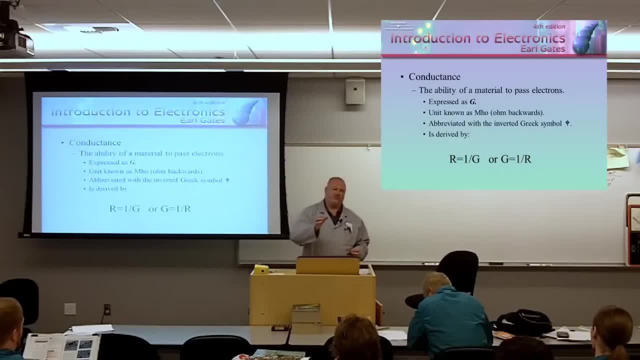 right in there. if you plug this in and it doesn't produce steam in a certain number of minutes- I think it was five minutes- your water may be too soft And add no more than an eighth of a teaspoon of salt to the two and a half gallons in the tank. Any more than 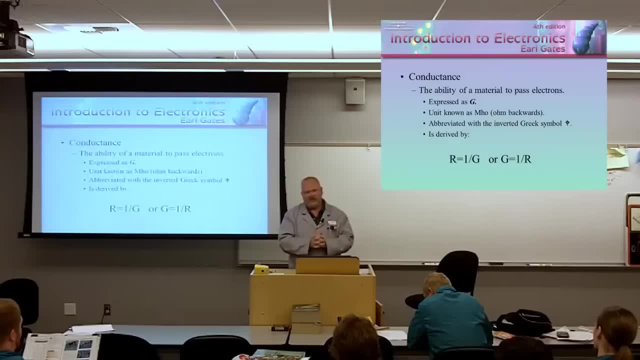 this could corrode the electrodes. blah, blah, blah, blah, blah blah. So I'm like you know, I'll read the instructions, I'll follow the instructions, But I don't think an eighth of a teaspoon of salt in two and a half gallons is going to make. 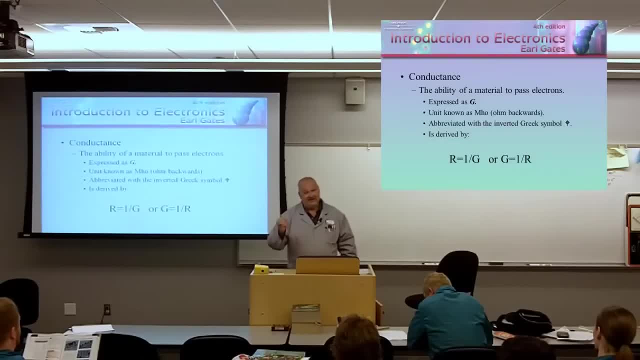 much of a difference. So I got an eighth of a teaspoon, which is a pinch. I mean, that's just a pinch of salt, Put it in there, plug the thing in, got back under the covers. By the time I was tucked in under the covers I looked over to think: 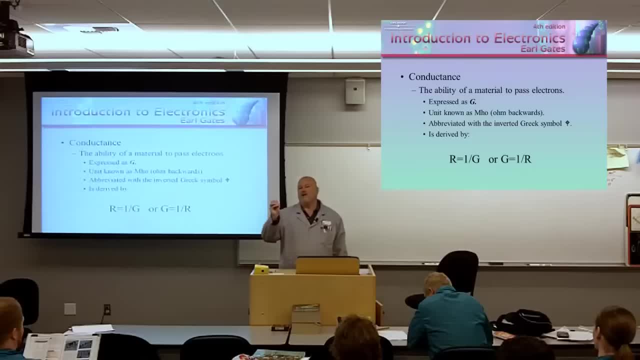 steam's pouring out of it. That small amount of impurity was enough to make that water conductive, Because those don't boil the water. What they physically do, they're electrodes and they flash it to steam, So its operation is contingent on having water that has some impurities in it. That being said, 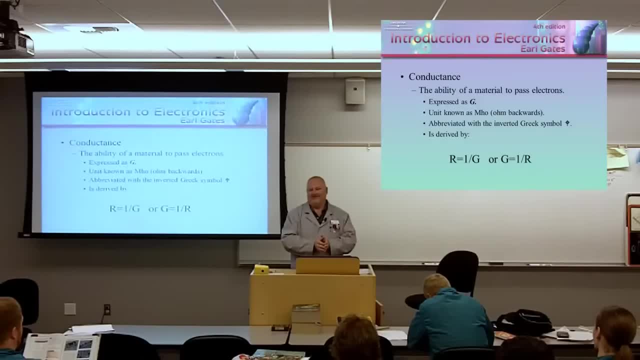 what does this say about our water? tap water here in western Washington- Really good water? What's that Really? Where are you that you don't think the water's that good? They're getting it out of the slough out there, don't they? 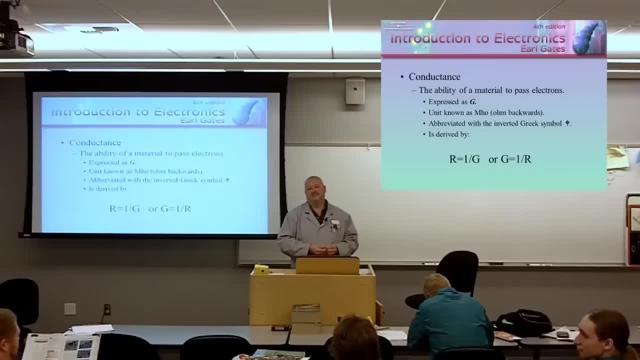 Generally speaking, though, here, generally speaking here in western Washington, in the northwest, in general, we have pretty good water. If any of you have ever lived in southern California, I was buying bottled water back there before bottled water was in vogue. I was buying bottled water because it tasted like it. didn't have a taste to it. Super hard, yeah, In the Midwest. I mean, I stayed with a cup cousin of mine that lives in Missouri once, and you know, hit the water softener, you got like stalactites and stalagmites in the shower. 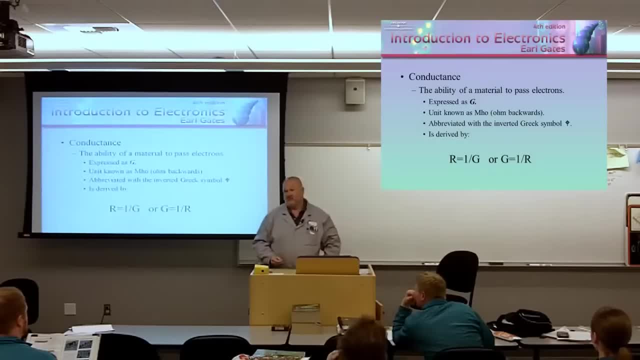 you know, because all the minerals that are, you know, I mean it's just crazy stuff. It's very hard on plumbing. I grew up in the east coast actually in an artesian well, well water, until the city came in and finally put but water. 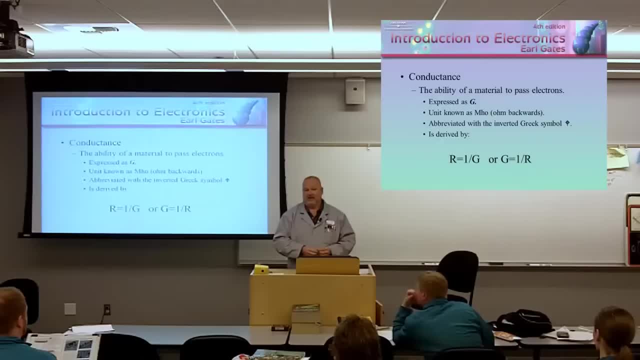 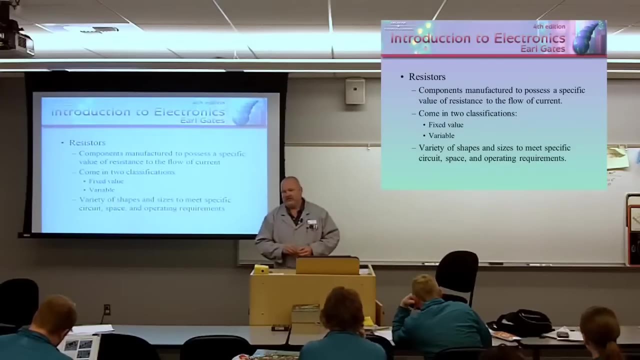 was perfect, So to some areas of the country they're really bad, but keep that in mind. Pure water. H2O is an insulator, So we have to add some impurities to it to be able to convert it. Now, everything has resistance, but we 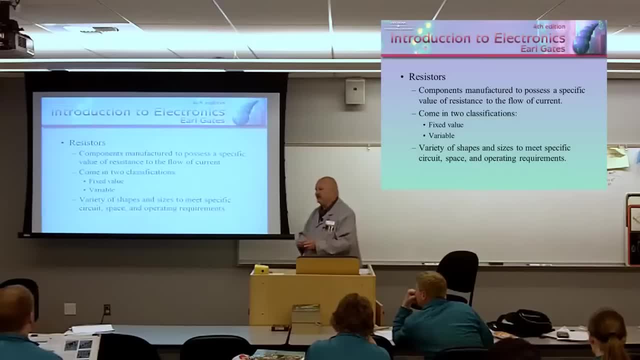 in electricity and electronics have a component that is designed to have this property of resistance And, amazingly enough, you know what they call it: The resistor. So a resistor is a specific device designed to possess the property of resistance. It's designed to have resistance. It's designed 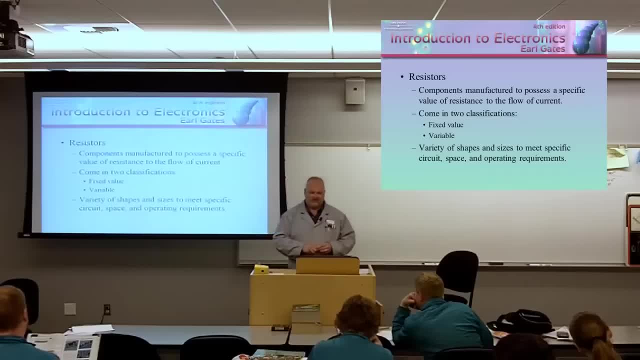 to possess a specific value of resistance that's predictable Comes in two different classifications: One is a fixed value, meaning what you see is what you get, And the other is a variable value, Variable. You can adjust it. Variety of shapes and sizes to meet specific circuit space and 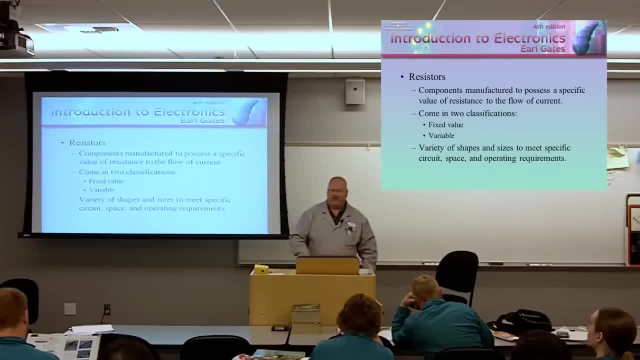 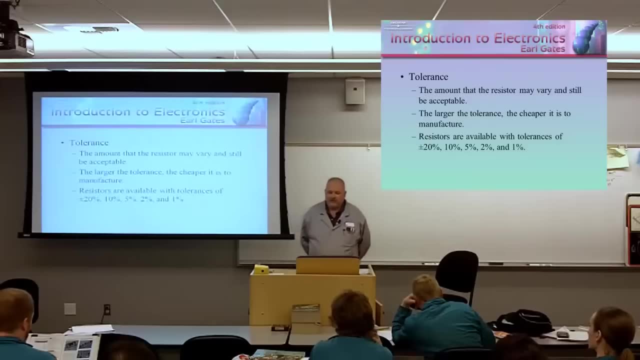 operating requirements. So there are all kinds of resistors on the market. These components all have a tolerance associated with them. Tolerance is the amount that the resistor may vary and still be acceptable. The larger the tolerance, typically the cheaper it is to manufacture. 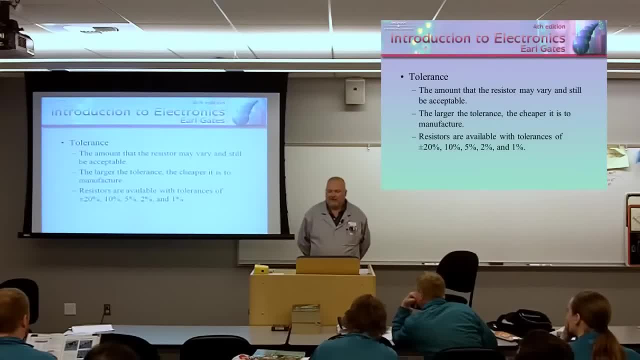 Now, believe it or not, in electronic components we could have values of tolerances that go anywhere from plus or minus 20%, 10%, 5%, 2%, 1%, But 20%. can you imagine that Everybody get their taxes? 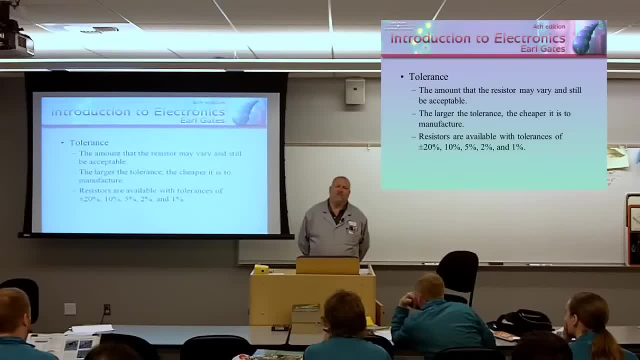 in on time. How do you think that would go over here, IRS? You know I did my taxes and I think they're accurate within 20%. Think that'd go over pretty big. What about if your employer said: you know, here's. 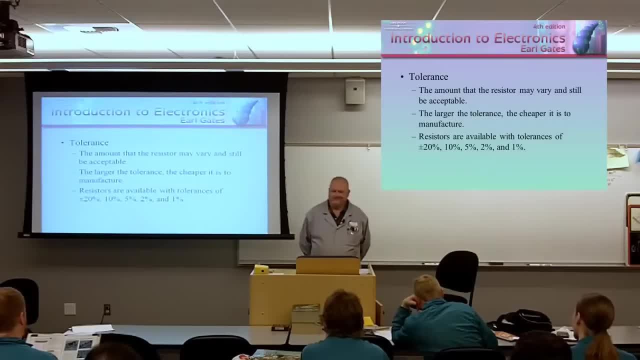 your paycheck on Friday, but plus or minus 20%, we're not really sure if it's accurate, Plus or minus 20.. And if you're on the plus side, cool, But if you're on the negative 20, it's. 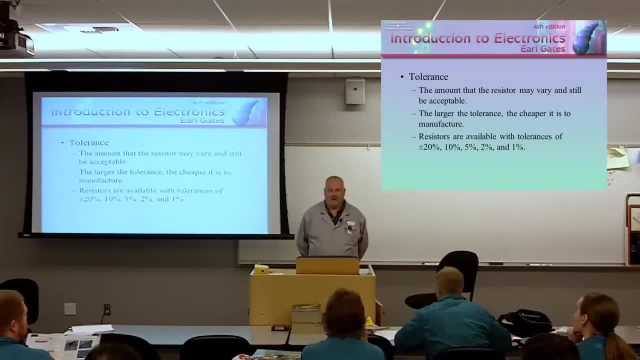 Isn't that technically 40%? No, Either plus 20 or minus 20.. But it's a difference. yeah Well, I don't even know if it's a difference of 40%, Is it? I guess it would be. 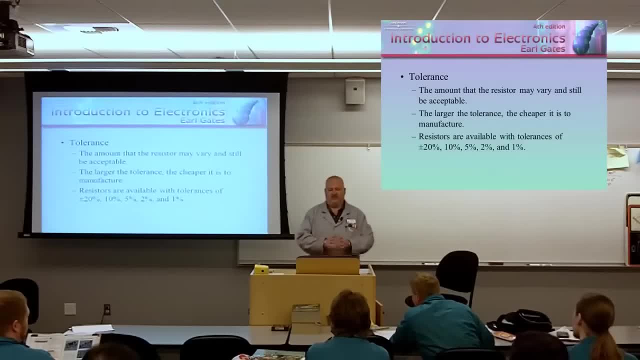 Yeah, But the way we say it. so we're allowed plus 20 or minus 20.. But it's a difference. yeah, If you've got a 100 ohm resistor, keep the math simple, right? That means that that resistor out of the package could be anywhere from 80. 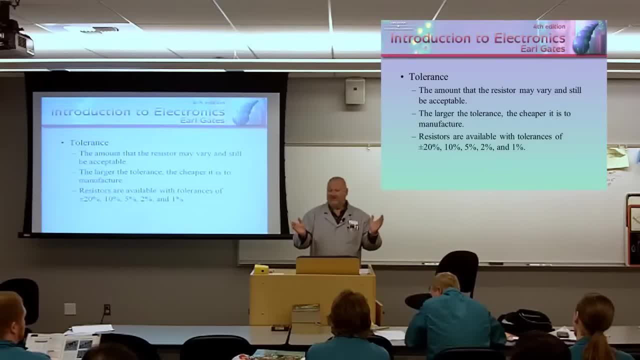 to 120 ohms And it's still okay. You got what you paid for. So it's kind of a wacky thing here because I make you follow all these procedures and policies here: Dot your I's, cross your T's, make sure your paperwork. 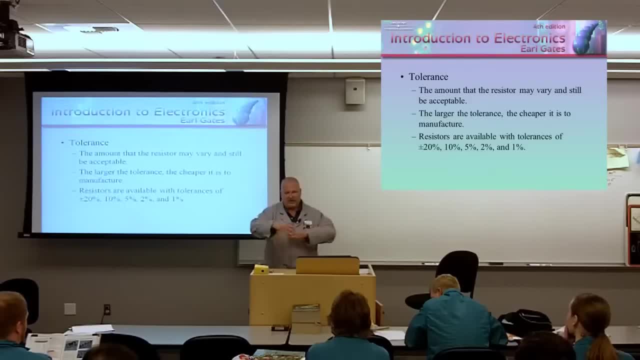 is accurate. You're answering to your team lead, the class lead. We have all this protocol here and everything. I expect your answers to be very, very accurate. But when you get over here to the lab, when you get out into industry, you're going to find that you're working with. 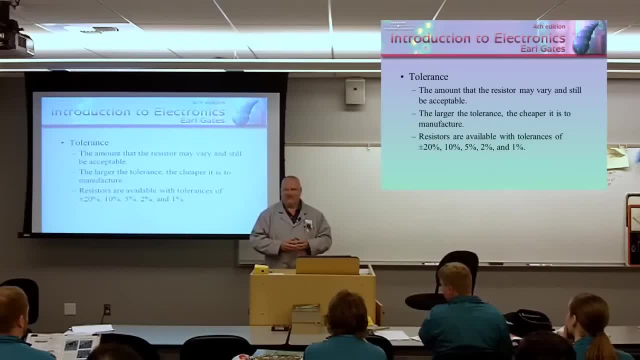 components that have tolerances up to plus or minus 20% Very, very frustrating. It's actually one of the challenges that I had in this industry, Because in here everything we talk about is theoretical Perfect. In industry it's at plus or minus 20%. 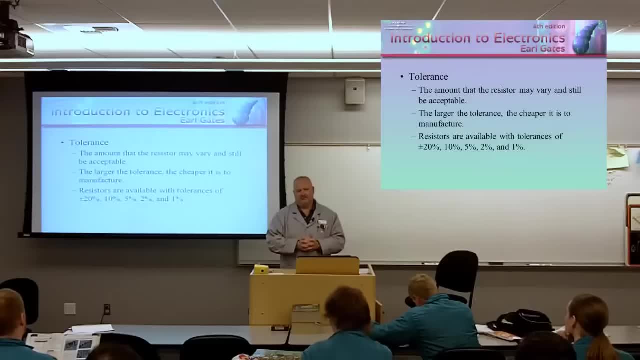 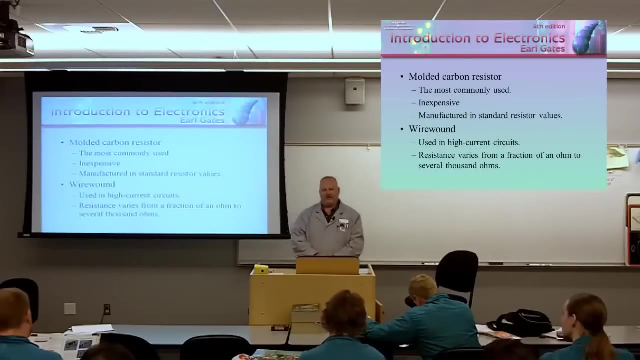 And it's okay. It's okay, So keep that in mind when you're working with any of these components. Some of the different types of resistors We have: molded carbon resistors that are made out of carbon That is molded. It's the most commonly used. It's inexpensive. 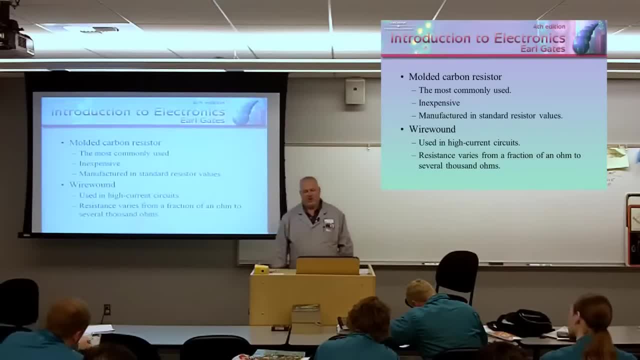 and it's manufactured in standard resistor values By standard resistor values. what I'm talking about, you know like how tires come in different sizes. I'm sure you could, if you wanted to, go, take a machine class and then make your own wheels. 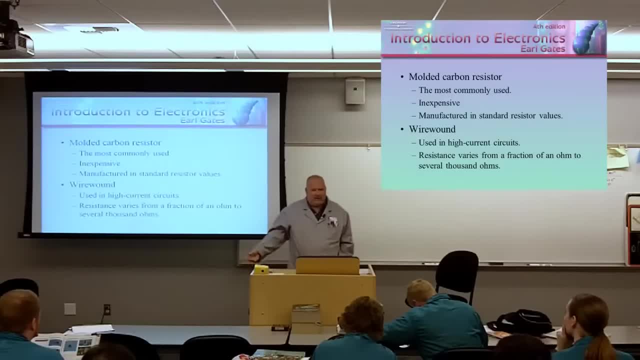 on a lathe or whatever on a milling machine down here? You could make your own wheel Whatever size you want. Knock yourself out, you could make your own wheel. Can you find a tire that's going to fit your wheel? Probably the first. 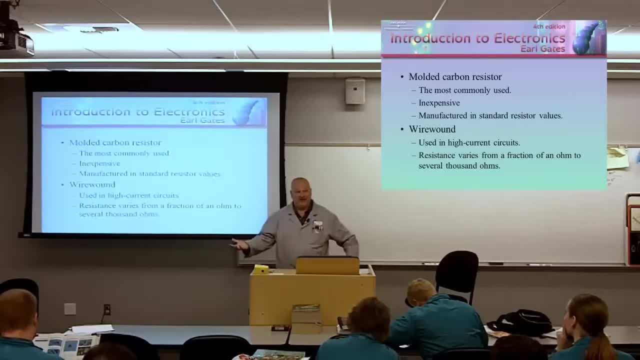 thing that you would do is look and see what standard tire values are and then make a wheel. if you're going to make a custom wheel that fits standard tire sizes, Because you're going to end up making a wheel that you can't even find a tire for, Make sense. 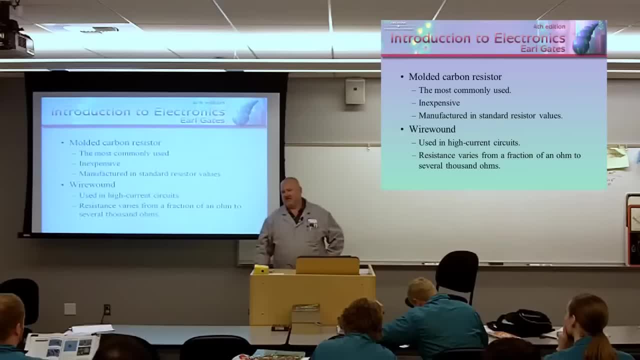 So resistors are the same thing. When we say they come in standard sizes, they come in standard sizes. Don't expect to go out and find a 103.5 ohm resistor. Don't expect to find that on the market. You could go buy a package of resistors that are 100 ohm, resistors that are 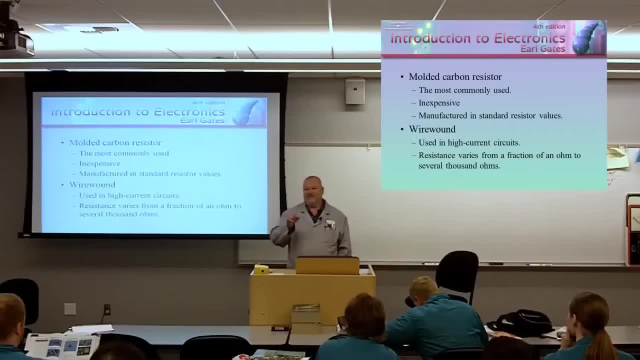 plus or minus 10% and start going through and see if you could find one that's 103.5, but an engineer is never going to specify and say I want a 103.5 ohm resistor in this circuit. They'll say I want a 100 ohm resistor, Standard sizes. 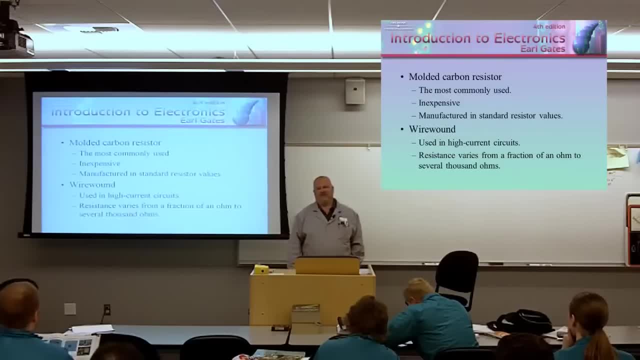 Another type of resistor manufacturing process comes up with what's called a wire wound resistor. These are used in high current circuits And they are made out of wire that is wound Because we know that wire has resistance. so if I get a certain amount of wire, 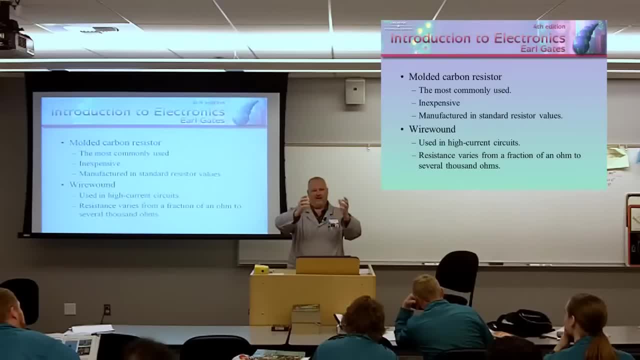 in one turn, then I can make another turn and get twice the amount, And it's literally how it works. The resistance of these varies from a fraction of an ohm to several thousand ohms. Question: When you were talking about the tolerance and you were 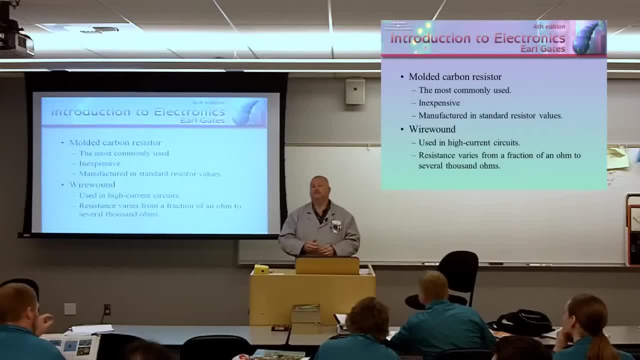 saying, if you bought a 100 ohm resistor and you found this 103.7, will that tolerance change or will that resistor constantly be one of the three? It could change over time. It could. Typically, it's going to stay pretty close to what it was. But again, since these heat up, things could change in the composition of it and alter its characteristics, But that's not a big factor to worry about. There's a lot more components in electronics that are a lot more sensitive than resistors. Good question. 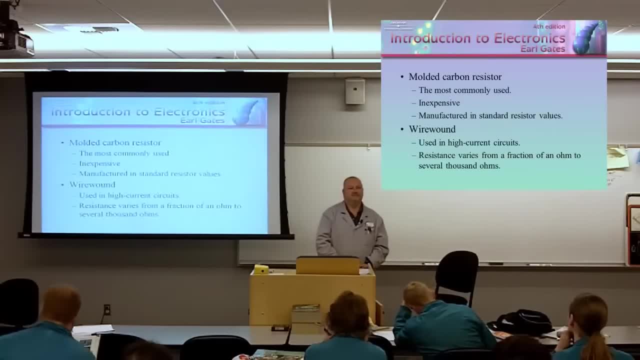 Does the tolerance add up? Because if you have three resistors and you've got 20% of both of them, all three of them, that's 60%. Yeah, the question is: do tolerances add up? Is there a cumulative effect? Yes, I worked. 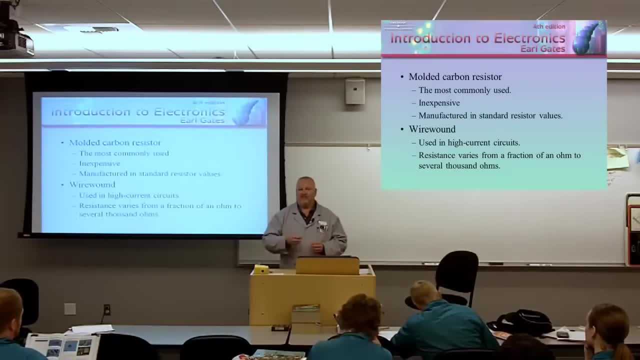 as a contract employee for a biomedical company before I came to teach here at Lake Washington 20 plus years ago And this unmentioned biomedical company I was working on this product and it was pretty expensive: motherboard And every component. this board kicked my butt. I could fix these boards pretty much. 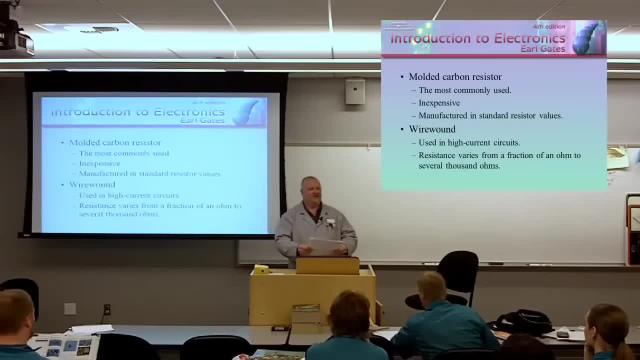 you know a lot of them were common problems. I'd look at the symptoms. you know, kind of hold it to my forehead, Let me guess resistors. you know R22 needs to be replaced. I'd replace it, fire it up. 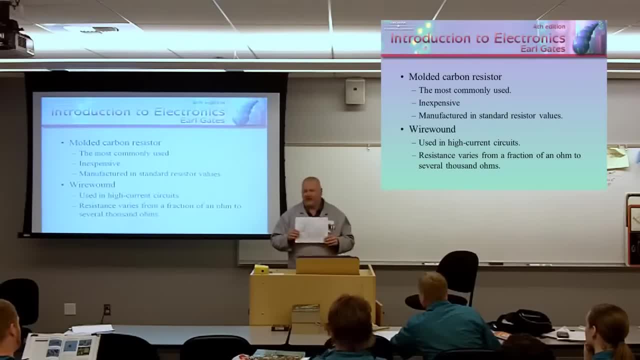 the thing works okay. I had this one board that I couldn't fix. I just could not fix it, And when I looked and evaluated the integrity of every component, every component was within tolerances, But when you put it all together, one. 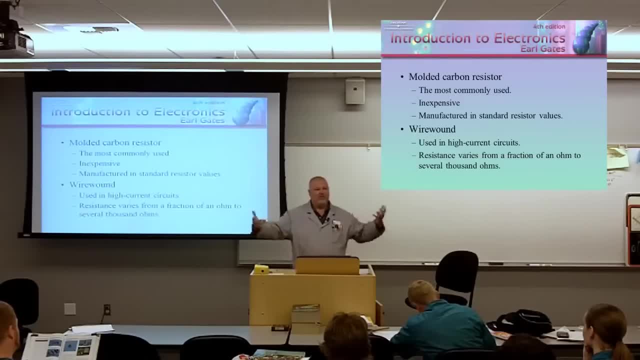 tolerance was pulling it this way, another tolerance was pulling it that way. When you put it all together, the board would not work. It was an anomaly, Because everything individually functioned And I kind of got in trouble over it. It was kind of like my ego, like I'm not going to let no stinking board kick my butt. 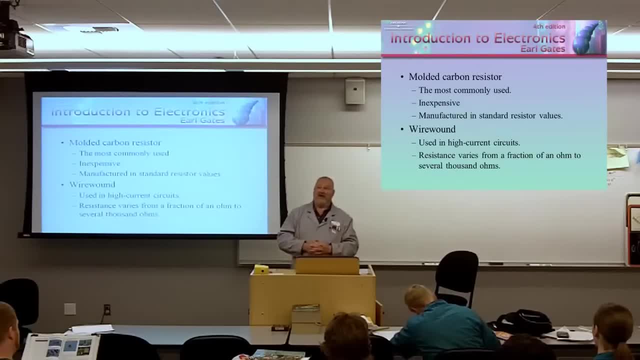 And, believe it or not, this company had it figured out. where every circuit board, a technician was allotted basically .65 hours to troubleshoot it. So what I would do if I was given a big production run to do on racks, what I would go through is fix all the easy problems first and then go to the next. 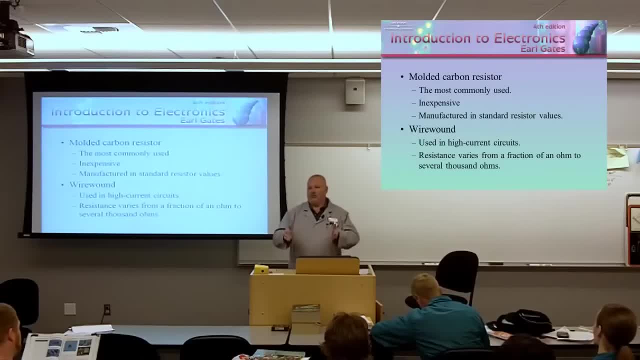 easiest problems and work my way so that when I was done I had all the real difficult problems left And then I'd look and see how much time I had left statistically. See, a lot of you- I don't even think- realize that this is how you're. 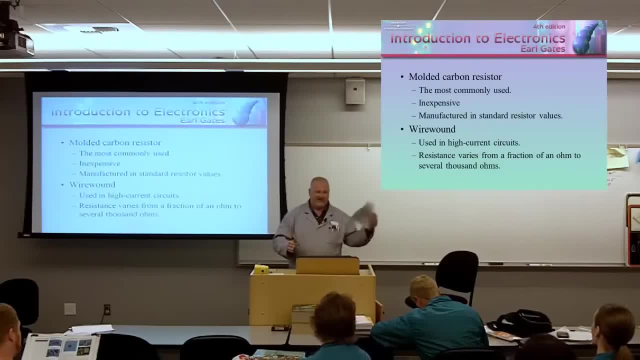 measured. when you get to industry, They know exactly how long it takes to fix this board. So if it's .65 hours and it takes you three hours, you're going to have a discussion with the boss. You're in the wrong profession. 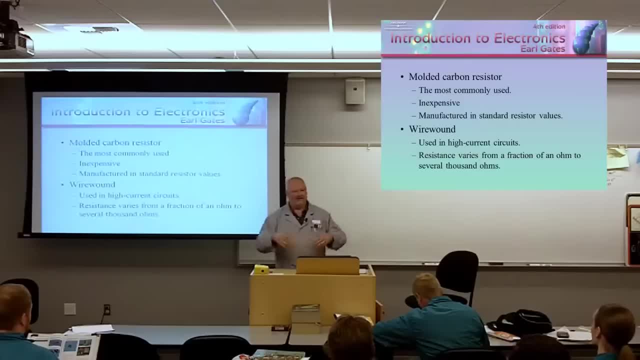 So, anyway, I knocked out all my boards and I ended up with like four days left. So I could go take breaks for four days, goof off and still end up statistically ahead of the game. But I wanted to fix this board. I ended up. 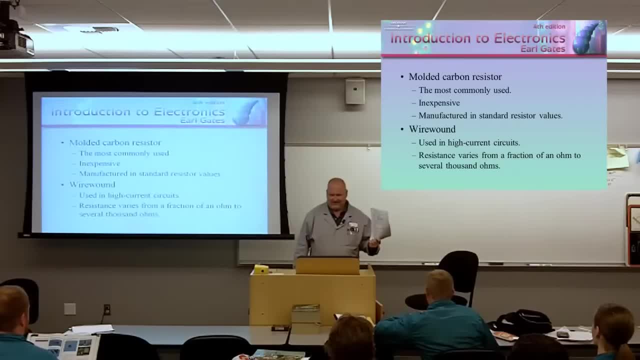 screwing around with this board for two and a half days And then finally my boss saw that I don't have a lot of boards. I'm all, what are you doing? I'm working on this board. This thing's kicking my butt, You know, I've been working on it. 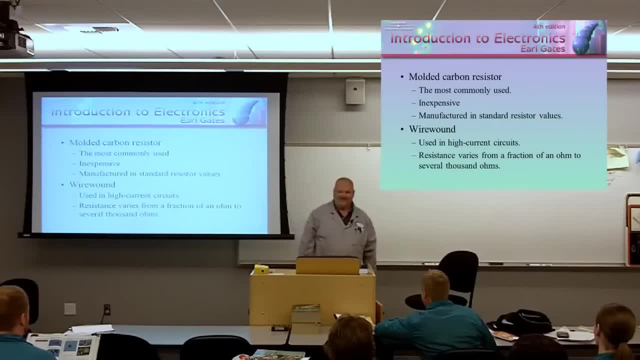 two and a half days. Two and a half days, You know, got the thing, threw it across the freaking floor- We're not paying you to screw with that- And I never was able to fix it. But what it was again were tolerances pulling in different directions. So sometimes 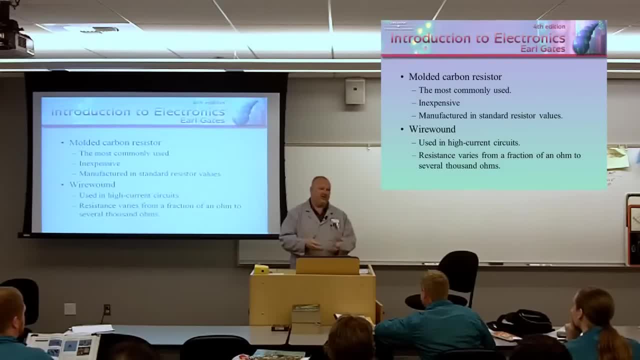 you could have something that, individually, everything is functional. You put it together, integrate it as a system. It just doesn't work. Why? Because of what you said: Tolerances pulling in different directions. That's a pretty uncommon situation, though, huh. 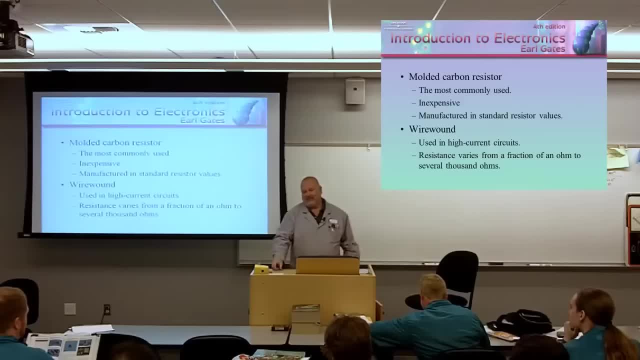 Yeah, You know it's probably more common than we think, But yeah, generally speaking, it's uncommon And that's why I'm not mentioning the name of this company. One of the things that they did is the majority of boards that were. 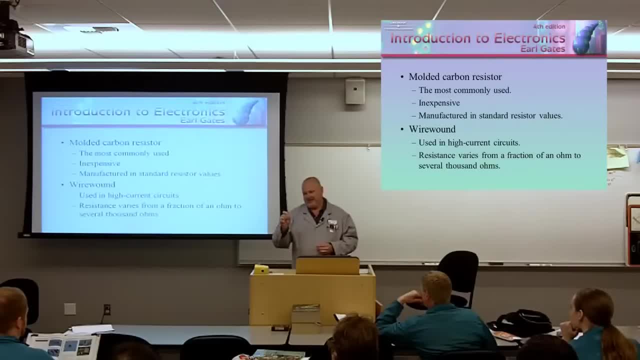 rejected were because of this capacitor, that they used 20% tolerance capacitors And the circuit would not tolerate that. It had to be right in the zone. So what I would do is I would go to stores and I'd get a bin of capacitors, I'd sit there and then I would test every one. 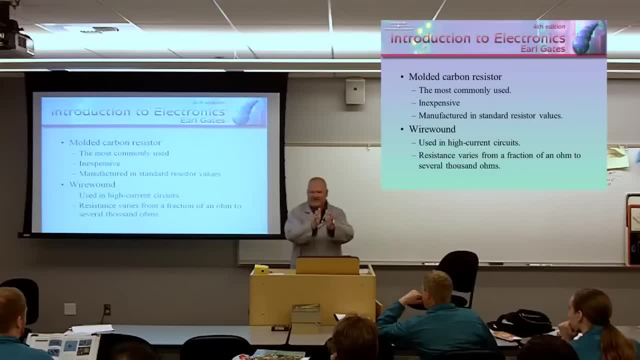 and basically sort from 20% tolerance to like a 5% tolerance and keep those capacitors. So when I ran into that problem I would just unsolder that cap, put the new cap in. Employees wrote a beneficial suggestion to the company saying: you know, why don't we just buy? 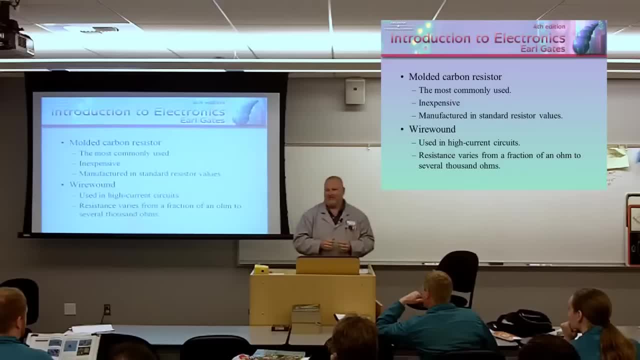 5% tolerance, capacitors and all these things wouldn't have to be reworked. You know? you don't know what you're talking about. You know: just do your own job or whatever, Instead of looking at the big picture. I think it was like a production manager, I think his brother-in-law. 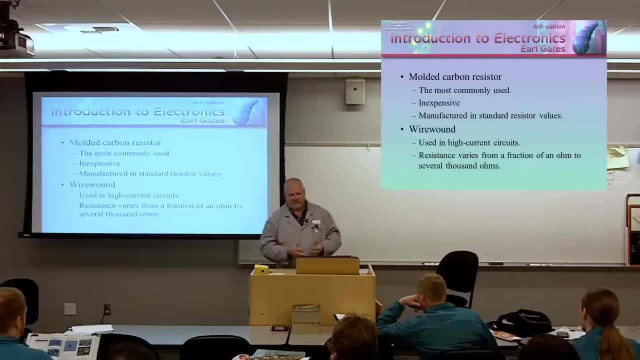 sold cheap capacitors for a living or something and he was buying them by the semi-load. It just made no sense, It just made absolute. this is a well-known biomedical company. It's kind of like: why are you doing this? Why not just use a tight tolerance component to begin with and avoid? 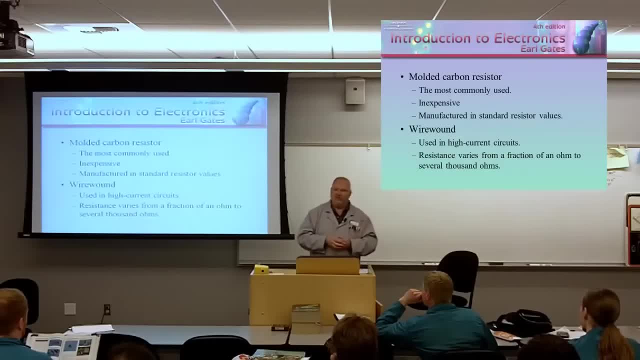 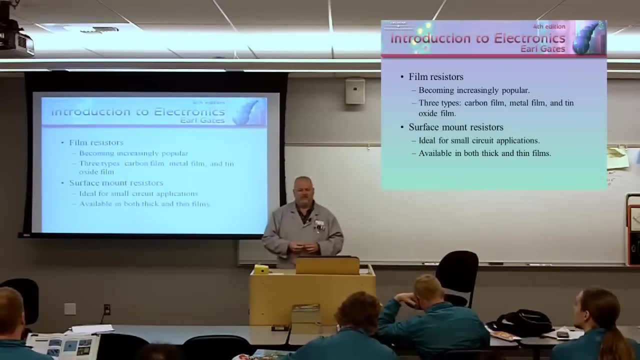 somebody having to solder and unsolder and repair these boards. It's costing them a ton of money. What do I know? Film resistors are becoming increasingly popular. There's three different types: Carbon film, metal film and tin oxide film. 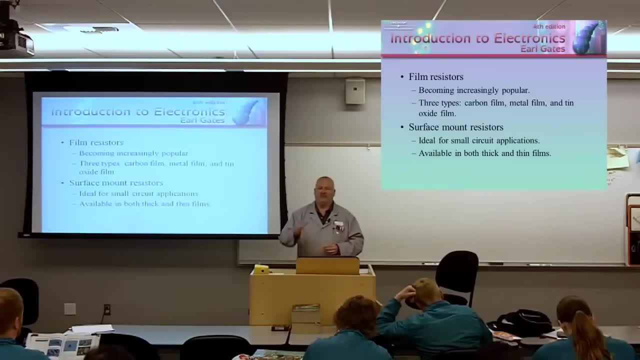 And by film what we mean is a manufacturing process that lays down a thin film of this material on a substrate and then that becomes the resistive material. So it's, some of the manufacturing processes actually are on par with manufacturing solid state semiconductor devices. 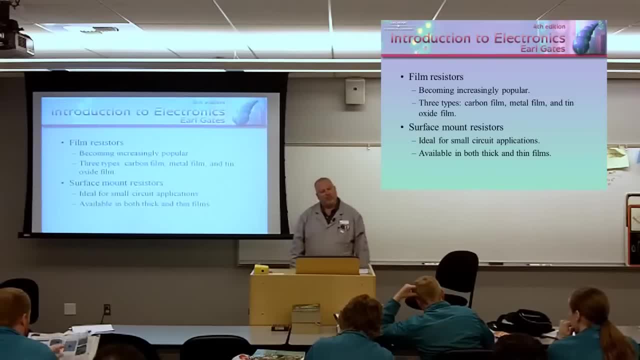 Surface mount resistors, Ideal for small circuit applications, Available in both thick and thin film. If you're working with surface mount resistors and you have a package open and you sneeze, they're gone. So don't sneeze near a package of open. 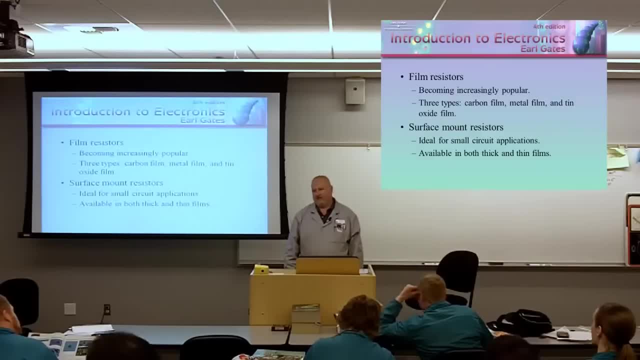 because these are tiny. Some of these are almost the size of the head of a pin. Tiny, tiny components. That's what goes into making your cell phones and digital watches and TVs on your wrist that you can watch and all of that kind of stuff. 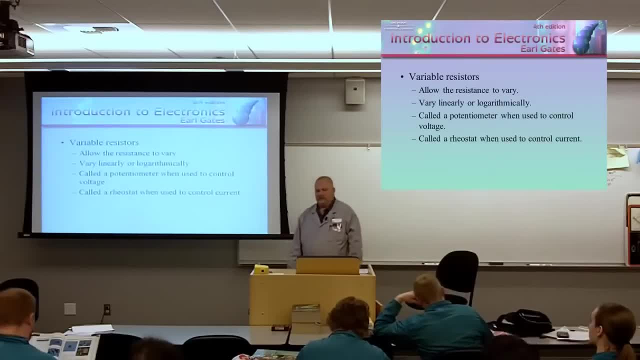 We also have variable resistors. Variable resistors allow resistance to vary, both linear and logarithmically. Linear and logarithmically: When I say linear, do you know what I'm talking about? Linear, Linear means a straight line. So if I 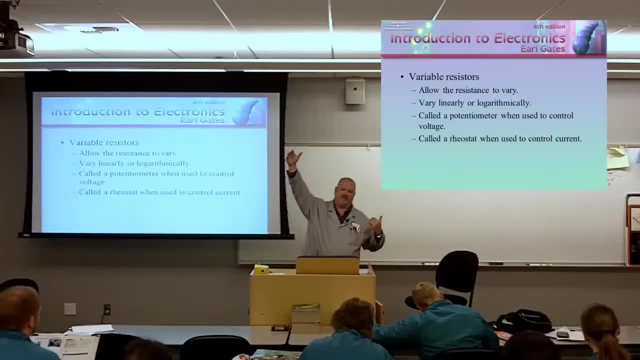 have something on a linear scale. if I adjust it a little bit, I get a little bit of response. If I go to 100%, I get 100%. If I go to 50%, I get half. If I go to 25%, I get a quarter. 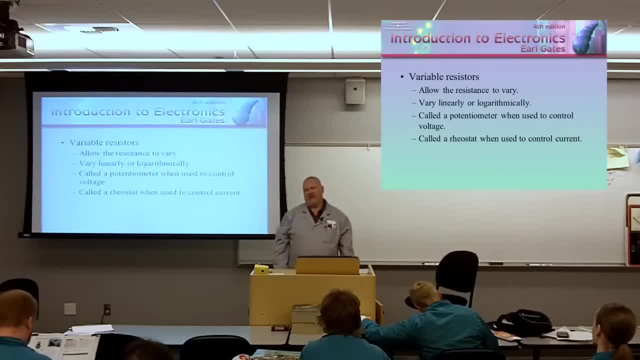 Make sense. That's linear, It's a straight line. Logarithmically is on a curve. It's on a logarithmic curve, So if I turn a little bit, I'm not necessarily the whole response is on a curve. Does anybody know why? we would want to have a control that? 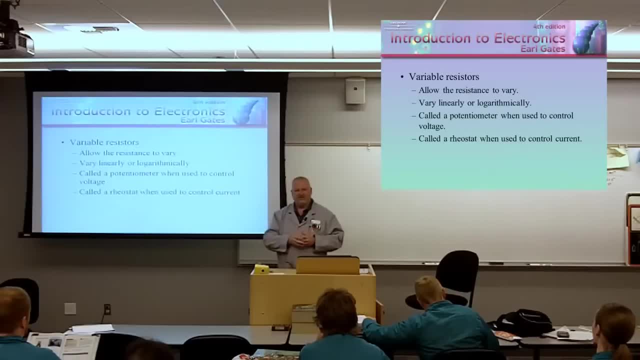 is not linear. that intentionally puts things on a curve for us. Very good. Logarithmic is used for audio applications because audio is not linear. Audio is not linear. Audio, some of you may be aware, is measured in decibels. 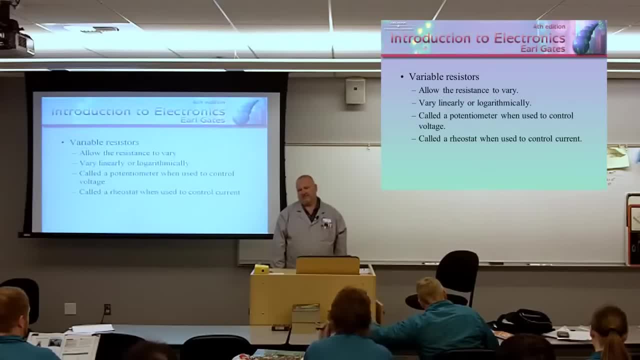 And that's on a logarithmic scale. So if you want to control something that is nonlinear, you need to use a control that's nonlinear, And audio is that example. So that's why we have this logarithmic control- One of the things if you're shopping for these variable. 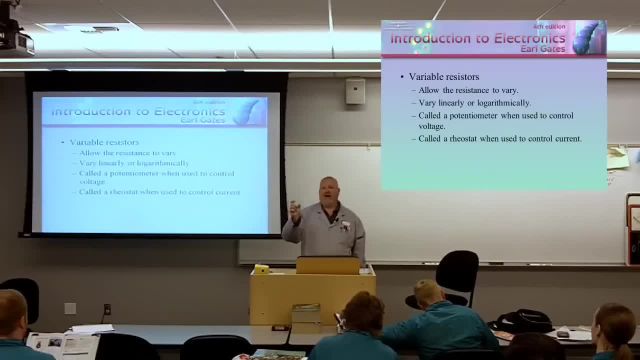 resistors. you may also see it say audio on the box Because it's for use with audio. So volume control on a radio, on a stereo, would be a logarithmic control, Because it's controlling something that's nonlinear And what we're trying to do is get somewhat of a linear response out of it, right? 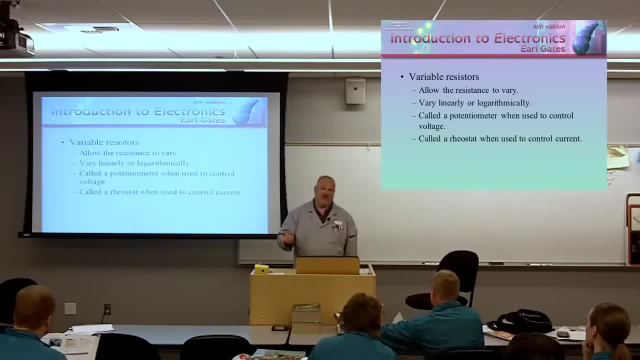 When you turn the volume all the way up to 100%, you expect to get 100%. When you turn to 50%, you expect to get 50%. But since audio is not linear, we need to use a logarithmic control to get a linear type response Make sense. 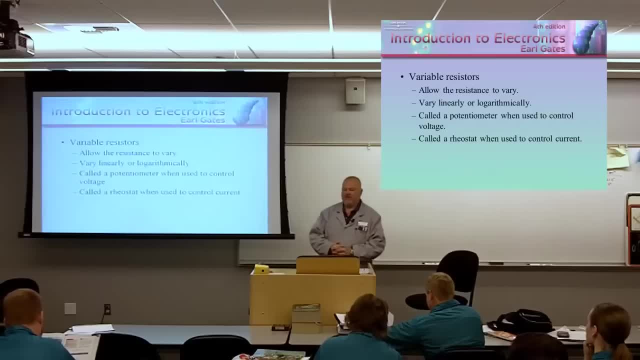 These variable resistors when they're configured as a potentiometer or pot, also known as pot a pot. When we configure it to control voltage, we call it a potentiometer, And I'll show you how we do that in a second. 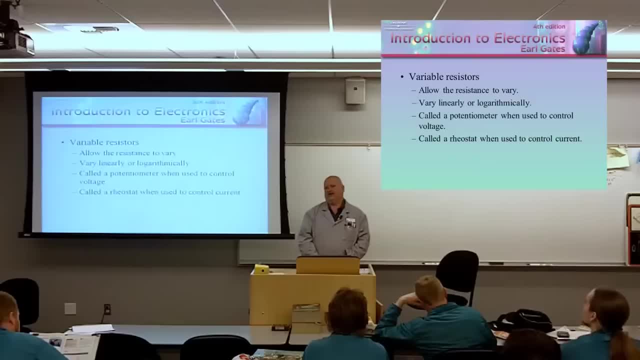 But I want you first to hit the I believe button. What type of a device do we use to control voltage? Variable resistor do we use to control voltage? The answer is potentiometer. When we use a variable resistor to control current, we call it a rheostat. 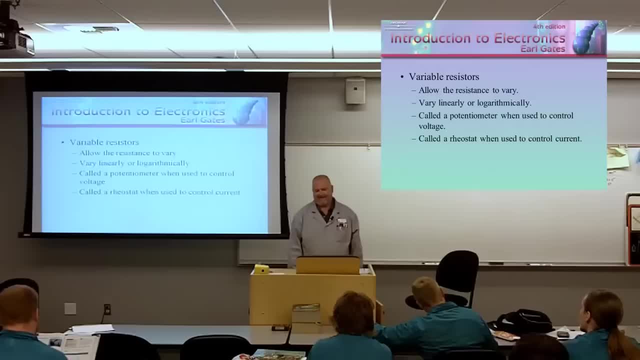 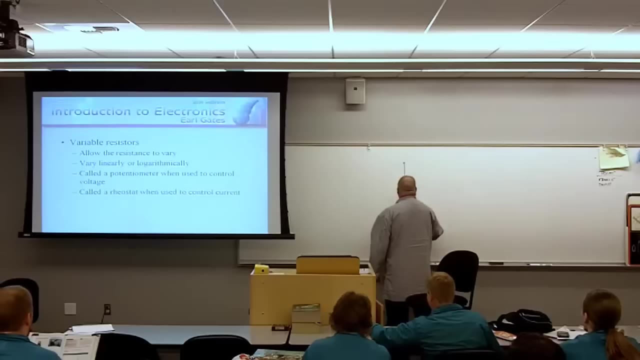 We call it a rheostat And basically the way that this thing works. What I just illustrated here on the board is a resistor right, And what I've got here is I've got terminal A And I've got terminal B. 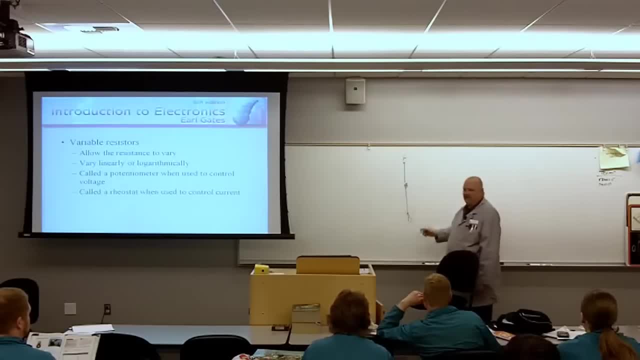 When I put my meter across terminal A and B, what am I going to measure? The resistance, The resistance between A and B, The total resistance? You all agree with me with that. Okay, So if I go ahead now and connect this up to a circuit? 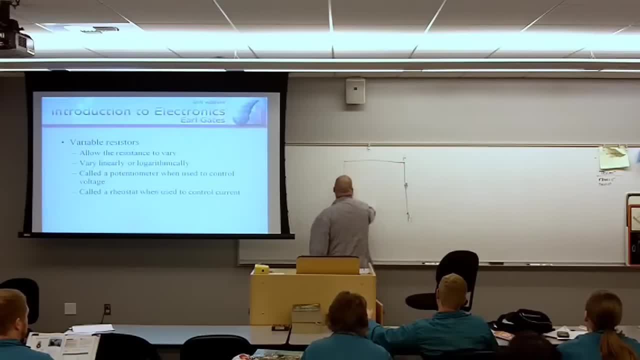 Okay, This is the negative terminal. This is the positive terminal. Okay, Current is going to want to flow in a counterclockwise direction here And it's going to flow through this resistor And when it encounters this resistance, it's going to limit how much current flows. 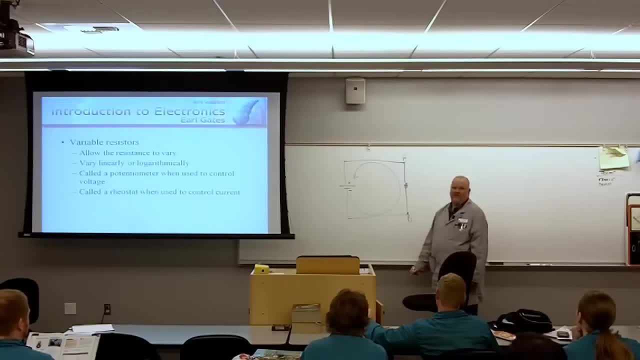 It's going to limit how much current flows through this circuit. Do you agree with me with that? Okay, So if I go ahead now, This is a fixed resistor. If I go ahead and turn this into a variable resistor, A variable resistor has a third lead on it. 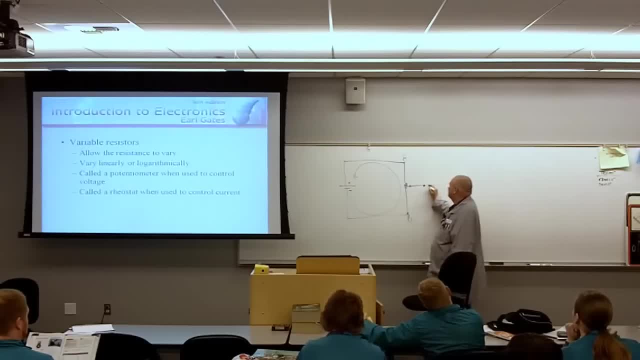 And I'll label this terminal C. So I have between A and B is my total resistance. And then I have C And what this is is a wiper arm. This is a wiper arm And physically what it's going to do is move up and down. 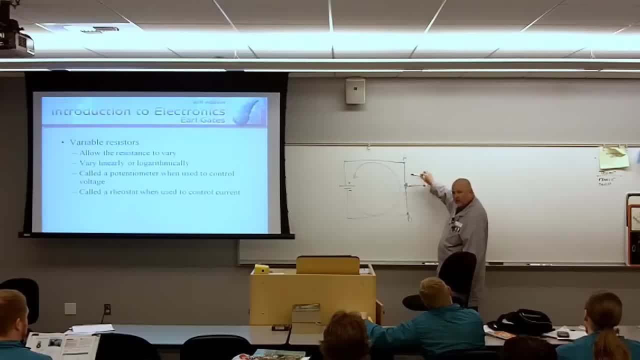 and come in contact with either my resistor or my resistor. Okay, So I'm going to go ahead and connect this. Is there more resistive material or less resistive material? It all depends on your perspective. If I have this adjusted right now, smack dab in the middle. 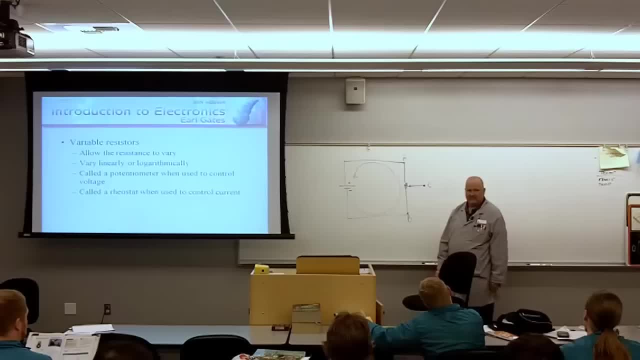 how much resistance do I have between A and C? Half. How much resistance do I have between C and B- Half Half, If I adjust it just barely, touch it just a little bit. now I'm 49% on one side, 51% on the other. 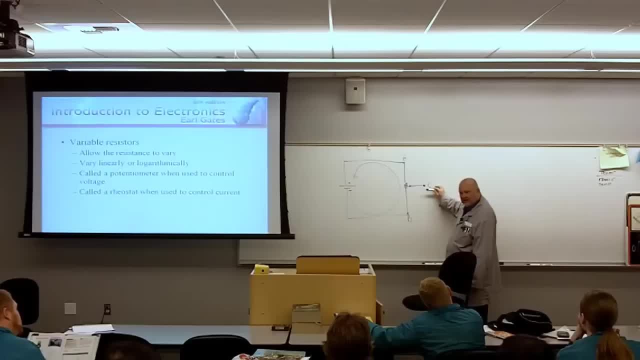 Tweak it more and I'm 40-60.. Right 80-20.. 90-10.. 99-1.. So I'm moving this wiper arm coming in contact with a different amount of resistive material. You all agree with that. 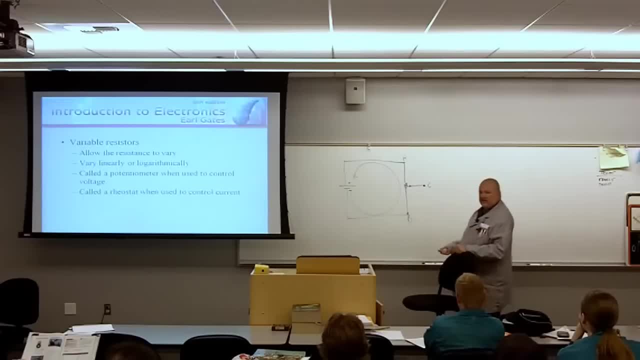 Does that make sense? Okay, Now, in this particular configuration I could move this wiper arm. I'm up and down all day long. Am I going to have any effect on current flowing through the circuit? Why It's just flowing between point A and point C? 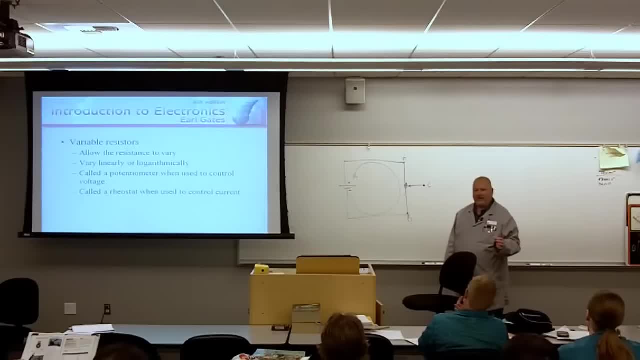 Excuse me, Point A and point B. Point C is effectively not even part of the path, So I can move that wiper arm. Hey look, Mom Right, Nothing's going to change. Nothing's going to happen. 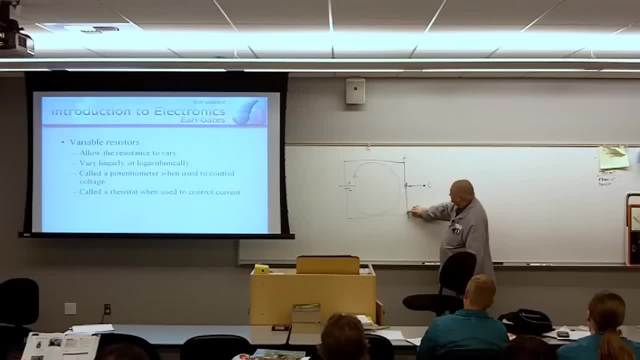 Now what if I break this connection here and come and move this and connect to point C directly? Now what's going to happen when I move that wiper arm? What's that? Total resistance is going to change in the circuit, Absolutely. 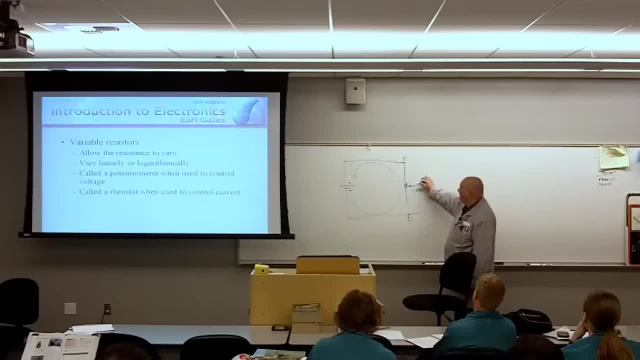 Absolutely. If I adjust this thing all the way to the end right here, I may have what 100%? Well, if I move it all the way here and it's not in contact with any resistance, 100% current flow. 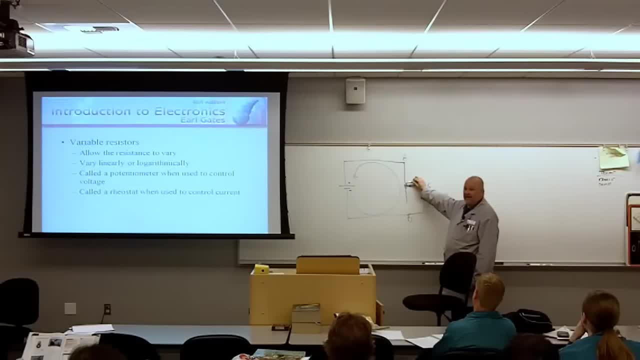 zero resistance, or as close to zero as I could get. When I move the wiper arm all the way to the bottom here now I get 100% resistance, minimum current flow. So literally when I'm adjusting this wiper arm here, 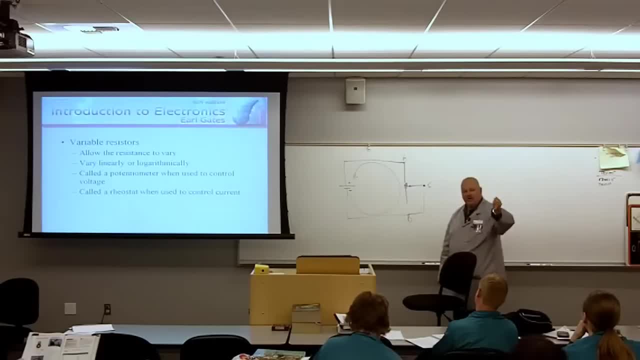 I'm adjusting the current flow, I'm adjusting the amount of- you said it- current in the circuit. So I've got this configured right now as what A rheostat? A rheostat. So when I'm using only two terminals. 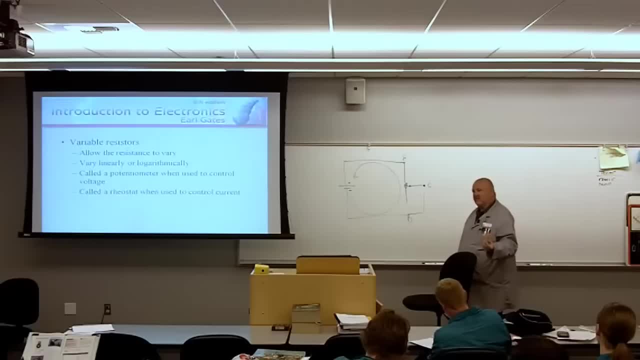 of a three-terminal device. I've got it configured as a rheostat. When I adjust my wiper arm, I'm literally adjusting the total amount of resistance, and that total amount of resistance is going to affect the current flow. It's going to affect the total amount of current. 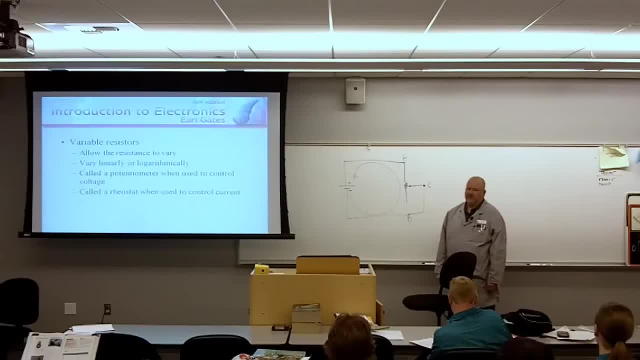 flowing in that circuit Make sense. I'm going to disconnect this, reconnect this and let's assume that I'm going to have make another connection over here and this is going to be a voltmeter. Voltmeter, I'm going to connect. 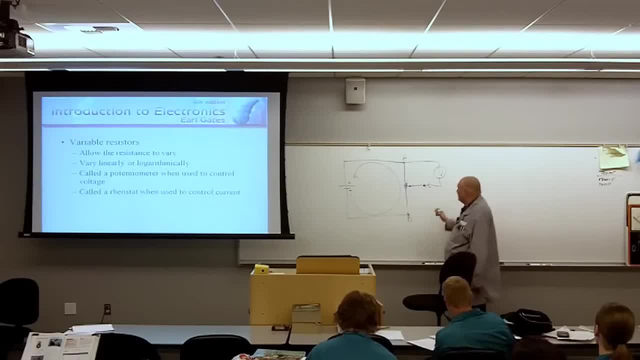 I'm going to connect a voltmeter between A and C and I'm going to connect a voltmeter another voltmeter. why? Because they're cheap right Between B and C. When I have this adjusted, smack dab in the middle. 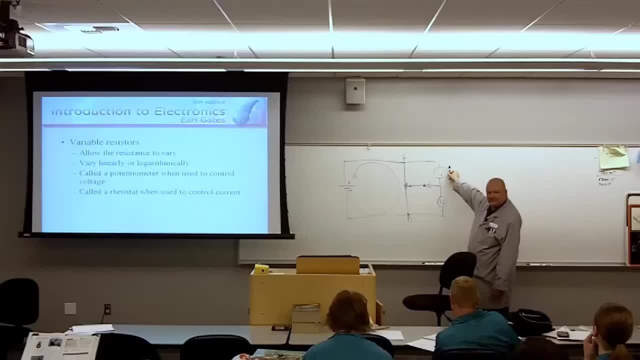 what voltage am I going to get across this voltmeter Half. I, like you, You're keeping it basic Half. That's the way I want you to keep it. you know I ask that question. I see somebody going for their calculator, you know. 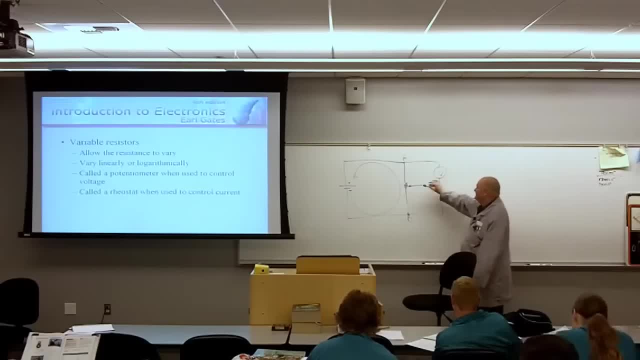 it's like I haven't given you any numbers. you can't calculate this one. If I've got it smack dab in the middle, I'm going to get half my voltage here, which means I'm going to get my other half voltage. 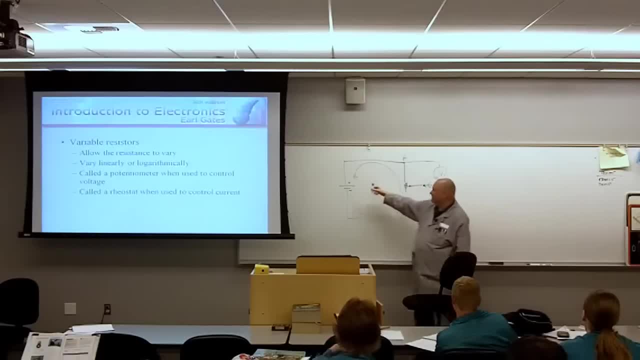 down the bottom. Okay, So if this is 10 volts, I get 5 volts here and 5 volts here As soon as I begin to move that wiper arm slightly. now I'm that 5140,, 69,, 60,, 40. 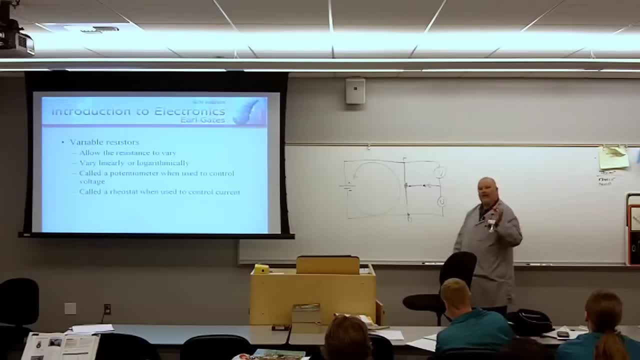 But I'm not talking about resistance now. I'm talking about what Voltage. So when I connect all three, I could use this as a voltage divider. 100% of the voltage that gets applied between A and B gets divided proportionally between the wiper arm and the outer terminals. 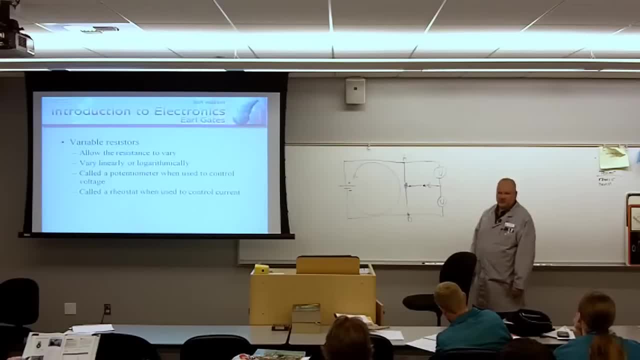 When I have it configured like this and I'm dividing voltage or controlling voltage, we call that a potentiometer. This is how the volume control on your stereo is connected. This is basically what you're doing And that voltage, that voltage that you're controlling- 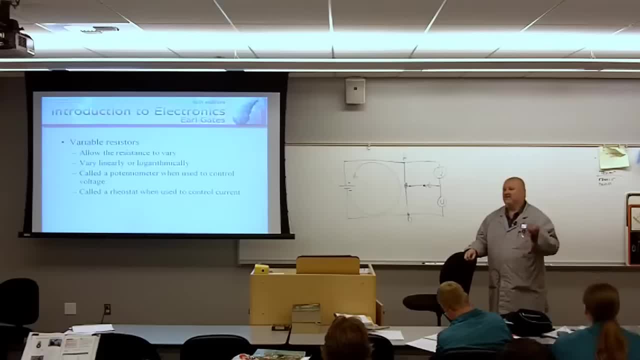 is going typically to a transistor And it's telling that transistor: here's more voltage. I want you to amplify more and make the music louder, Or turn it down and make the music softer. I'm going to give you less voltage to the amplifier. 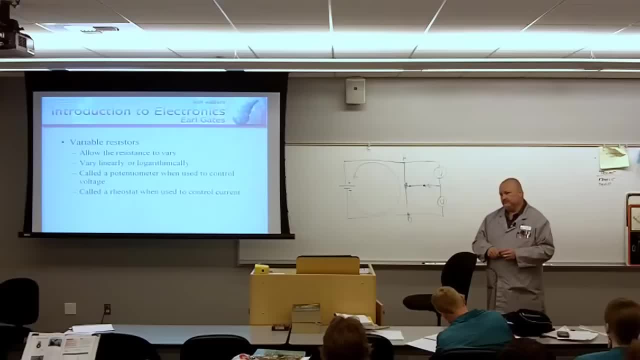 the transistor And this is how it works, So keep that in mind. That's how we say we're either controlling current or voltage. Could I use a potentiometer as a real stat? How would I do that? Only connect two of the terminals. 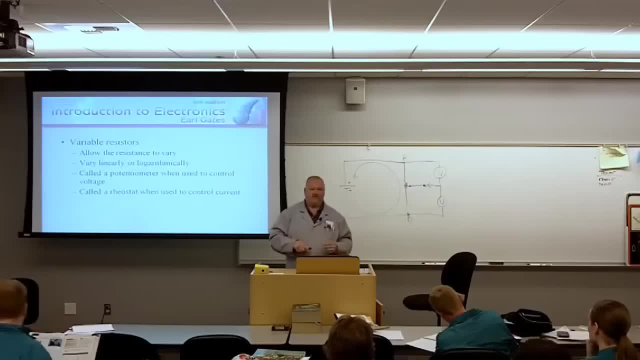 So if you go to Radio Shack and say, do you have any real stats here, That would be a fun question. I should give you that as an out of class assignment. Everybody go to Radio Shack and ask if you've got any real stats. 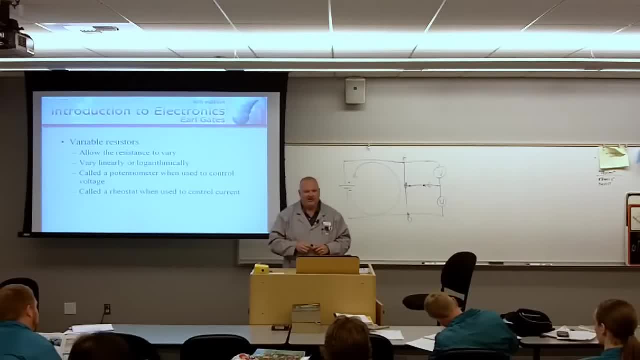 And they'd probably scratch their head and bring in: oh, but we have some potentiometers. You could use a potentiometer as a real stat. You only need to connect two of the terminals. If you went out and bought, special ordered a real stat. 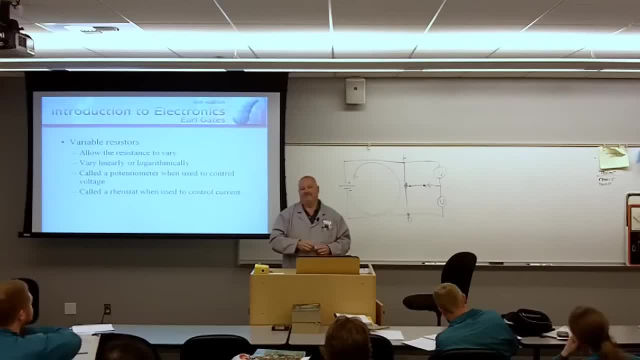 and it came in a box and it said real stat. could you use a real stat as a potentiometer if it only came with two terminals? No, You need that third terminal to be able to divide the voltage. Make sense, Okay? 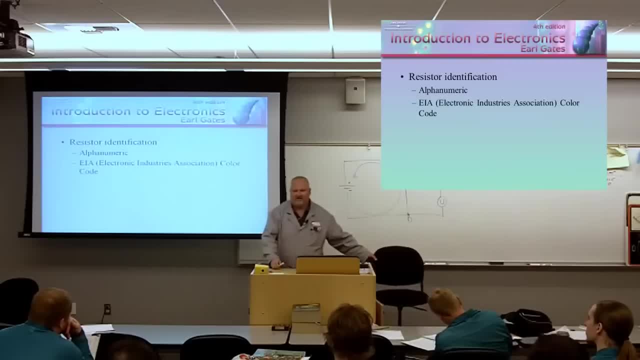 Resistor identification. There's a couple different methods that we use here We use to identify resistors. Does anybody know the easiest method of identifying resistors? I love it Now. the easiest method is when they put the value right on the outside of it. 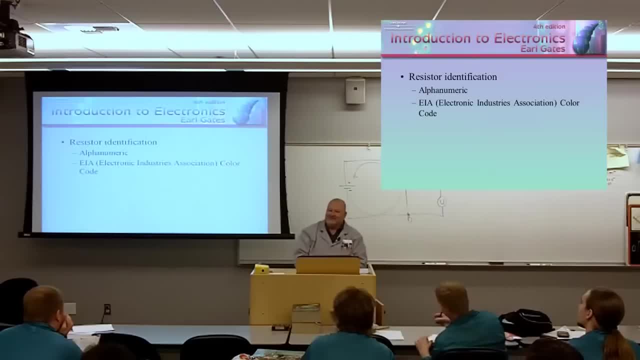 with numbers and letters. I always sucker people in with that one, Because everybody knows resistor color code. Now the easiest method is really when they use numbers and letters and they just say: if it's like a 1,000 ohm resistor. 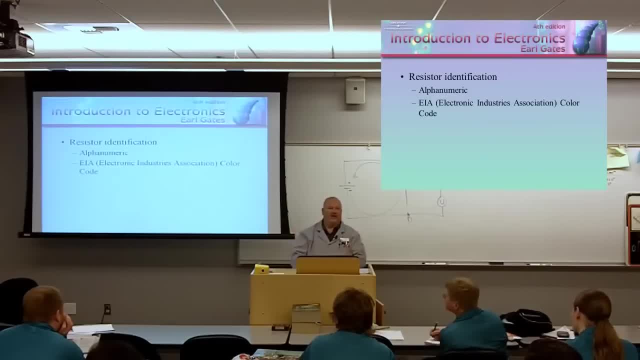 you know 1k ohm. It's right in there in black and white. You read it. you're good to go. Another method that they use is alphanumeric code, And for a lot of these resistors you're going to have to. 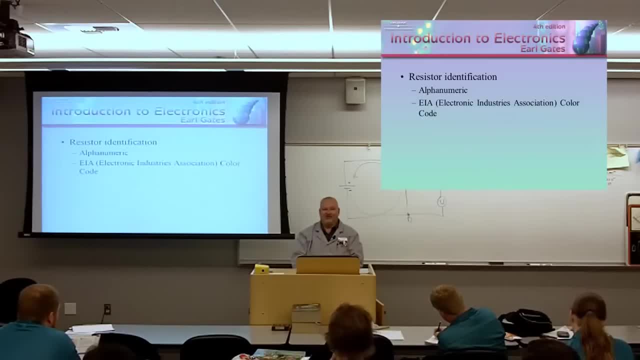 like a secret agent. use a decoder ring or a decoder chart to figure out exactly what the code means. The third easiest method is the color code And, of course, you can't have a successful career in electronics unless you understand the color code. 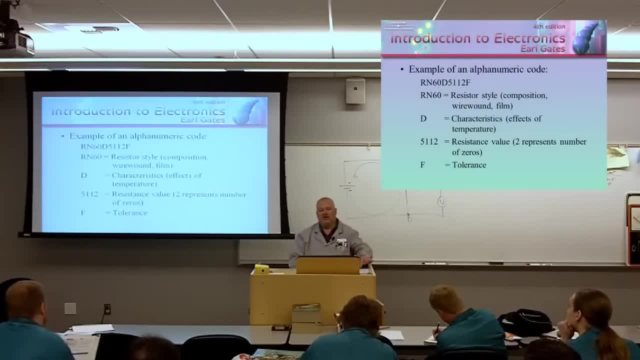 First thing we're going to take a look at here is the alphanumeric code. If you looked at a small resistor and it had an RN60D5112F on it and you came up to me and you said, hey Joe, what kind of a component is this? 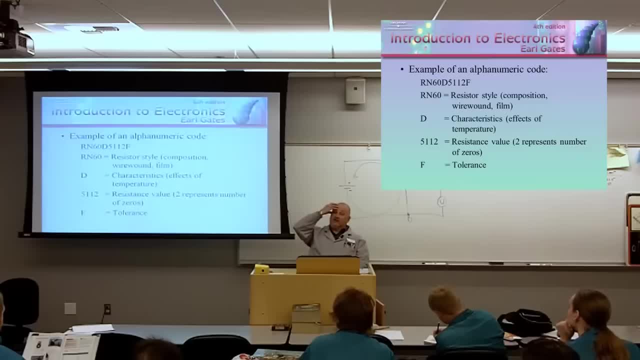 I would probably hold my head and say: I have no freaking idea. What you're going to have to do is you're going to have to call up this code and decipher it. If you work at a company, this is one of the things. 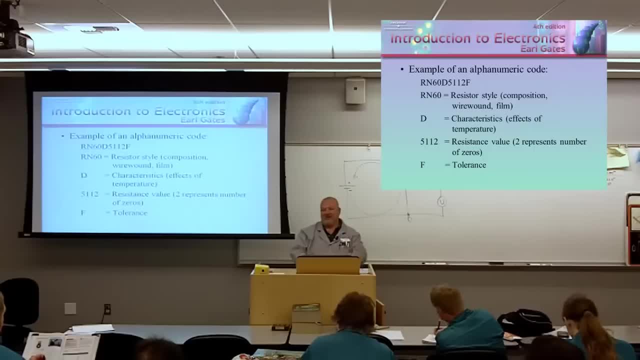 this is a very difficult job. it's a tough job I got. I got to train all of you generically, but what happens is when you go to your specific industries, you're going to see some of the same components day in and day out. 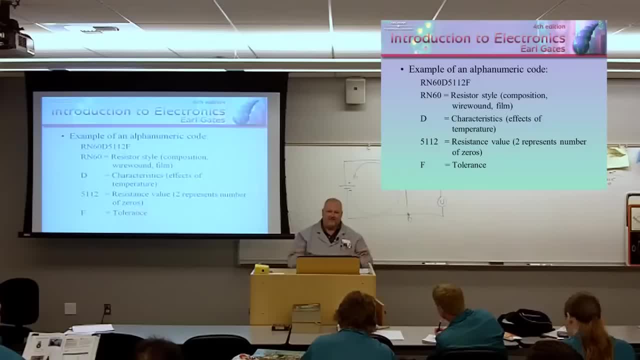 because you're going to get used to your company's product line. But here it's very difficult. I'm teaching you generic electronics and there's a lot of different schemes that they use. This is one of them. So the RN60 identifies the resistor's style. 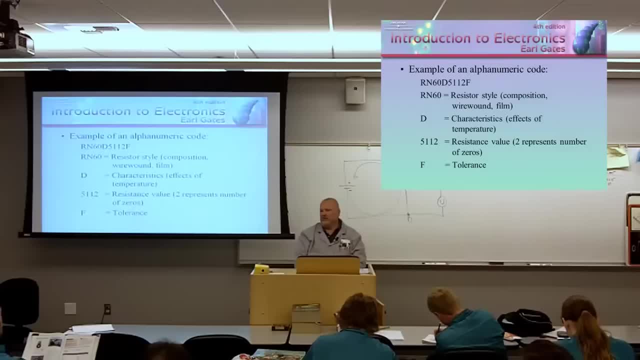 What is it? Carbon comp, Wire wound film. The D are its temperature characteristics. How does this behave? And they'll normally include some tables or charts in there to say, for every five degrees rise in heat, in Fahrenheit, this is how many ohms it's going to change. 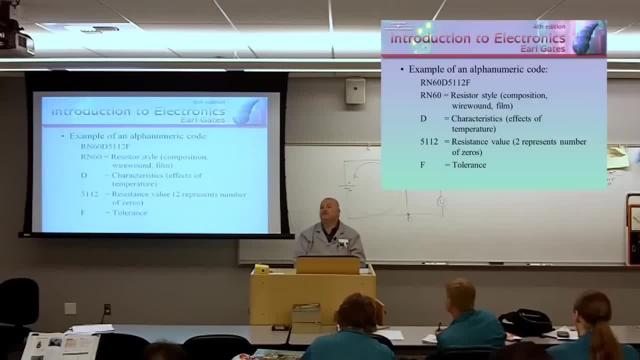 So it's going to be its temperature characteristics Question. Yes, yeah, No, don't memorize this. The point of this is that you're dead in the water unless you get the code The 5112, that shows the resistance value. 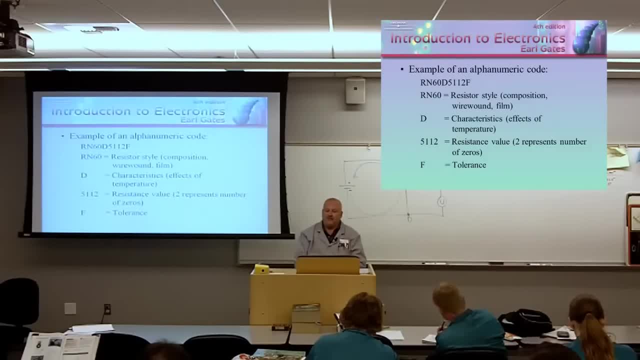 The 511, the 2 represents the number of zeros at the end, So this would be 51100.. Putting that in most common terms would be 51.1k ohms, 51,100 ohms And the tolerance would be F. 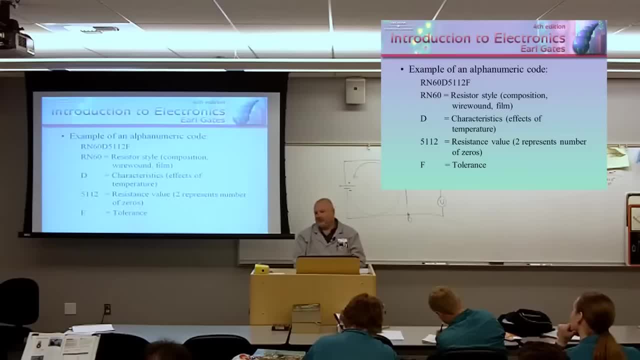 I don't know if that's good, bad. You're going to have to look it up and see what it equates to: 5%, 2%, 10%, 20%. I don't know, But that's how you would decode that. 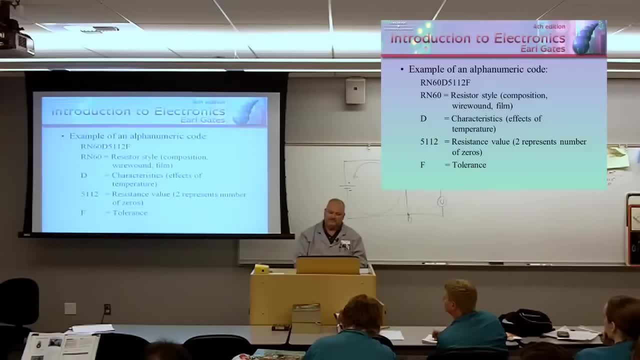 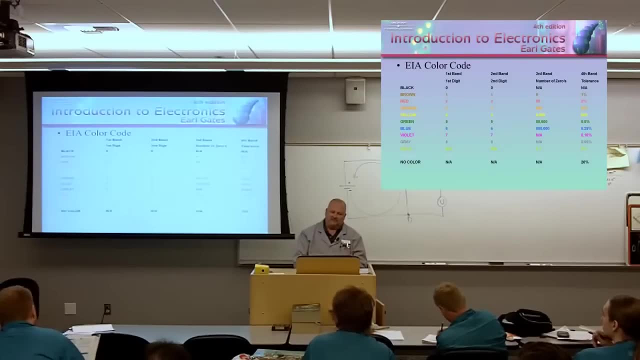 If you saw that on the side of the resistor, If you saw colors on the side of the resistor, well, there they are. You've got this in your book. The way the color code works. you have your first band, second band. 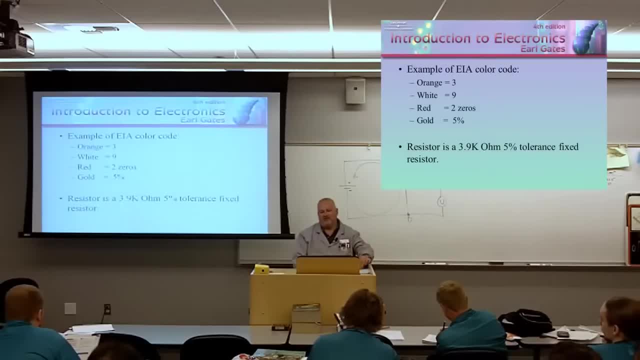 third band. fourth band: If you have a resistor, that's Well. first thing you want to do is hold it so that one of the bands is closest to the edge. You normally want to put that closest on the left and then read it like a book. 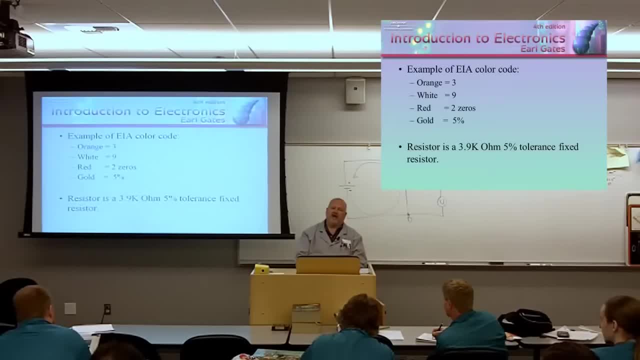 If I had a resistor and I held it in my hand and it was orange, white, red, gold, Orange on the color code equals the number 3.. White is the number 9.. Red is the number 2.. So that means I'm going to add two zeros. 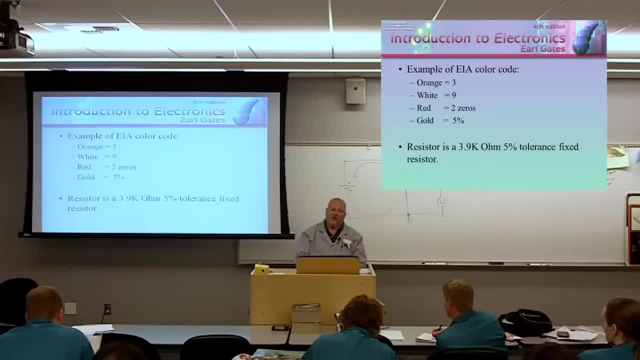 after the 39.. 3900.. That's a 5% tolerance. Putting that in most common terms means this would be a 3900 ohm resistor or a 3.9k ohm resistor. 5% Question. I hate the word memorization. 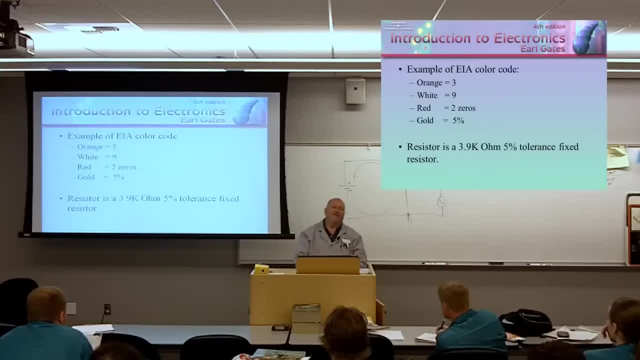 The question is: we have to memorize it. You've got to know it. You've got to know it And, to be honest with you, a lot of job interviews. they're going to ask you to do that. The best thing, though. 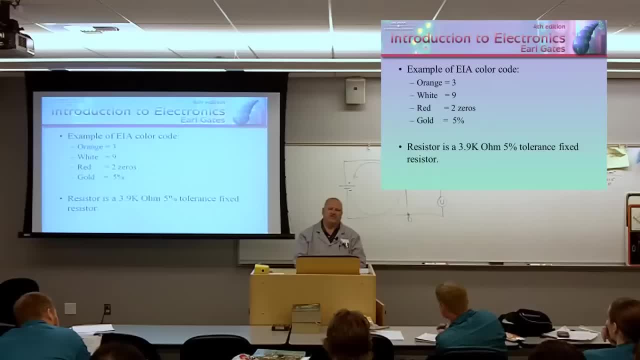 I'm not going to go out of my way. I'm going to be honest with you. I'm not going to go out of my way on a quiz to hammer you on it. You're not going to fail this quiz because you don't know the resistor color code. 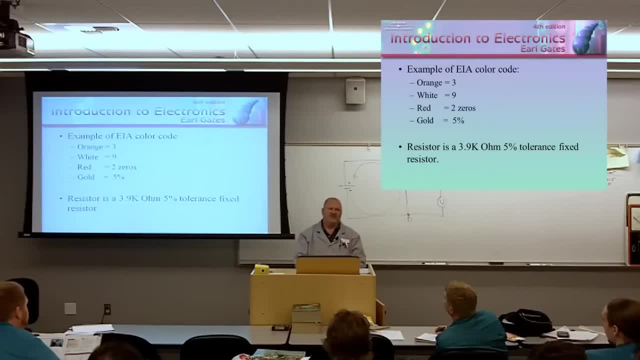 One of the big things with the resistor color code is simply your experience doing your labs. You're going to come to learn this And the more you work with it, you're going to understand it and you're going to remember it. But I don't want to make flashcards. 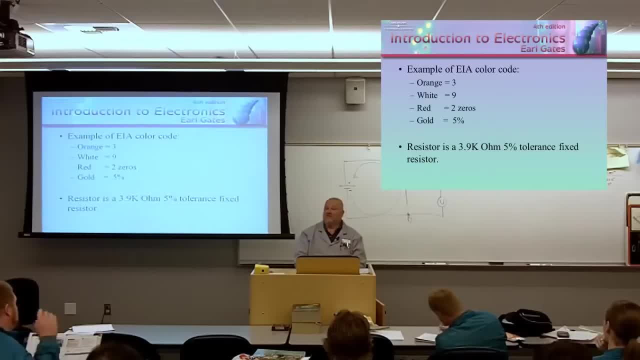 Other programs do that. We could give you flashcards and identify this resistor. I could keep you occupied and entertained. But then, when you're all said and done, you're ready to go get a job and identify resistors for a living. Not a lot of money in that. 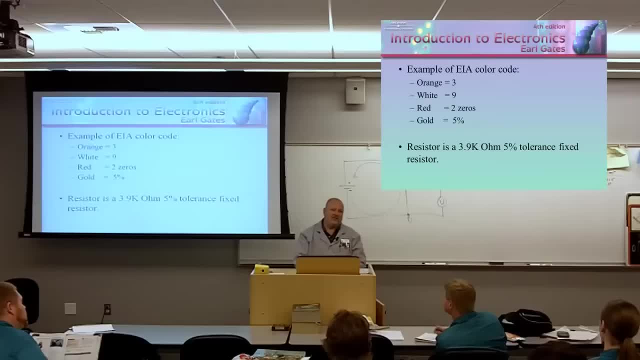 So this is just something that you need to learn, you need to know, you need to be able to decode. it Make sense. I'll let you study the acronyms At your own leisure in a group forum. See, I'm ex-Navy. 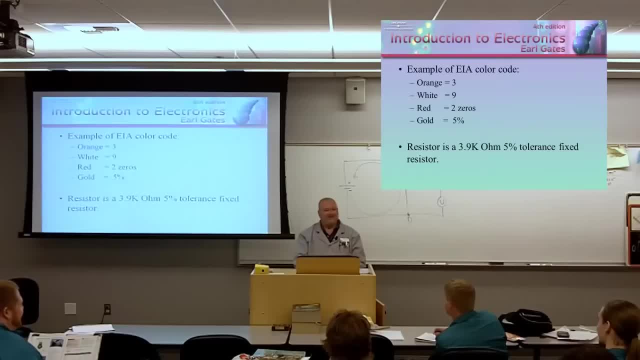 and we had some acronyms that basically if I repeated here I would be handcuffed and dragged off. Start with bad boys. That was one of them. Yeah, that's one I learned, So I'll let you discuss some of these amongst yourselves. 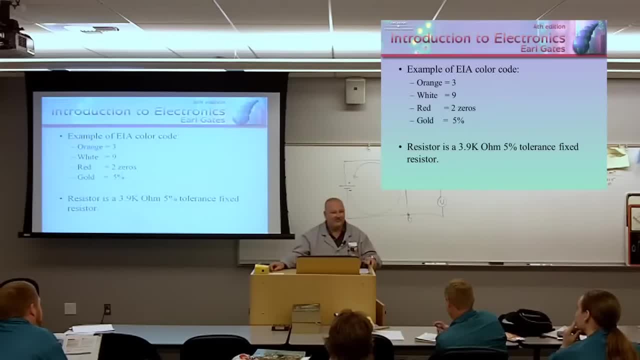 And they do work. It's actually funny because, having interviewed a potential faculty member, I'll of course always throw in there, identify this resistor And you see some making charts. I've never once given anybody a resistor. What size is this resistor? 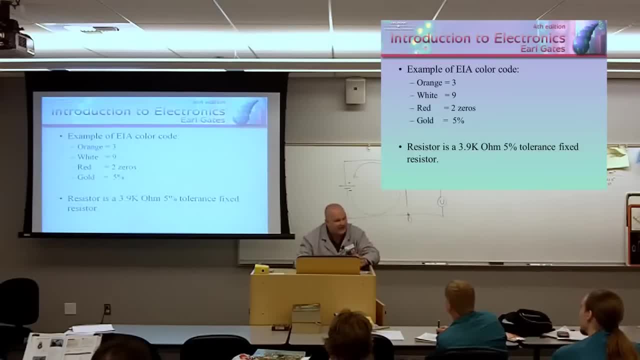 Oh, that's a 1.2K 5% resistor. Actually, if somebody identified it, I'd probably- you're a freak. You're a freak of nature, But it is something that, again, through experience, you're going to get used to. 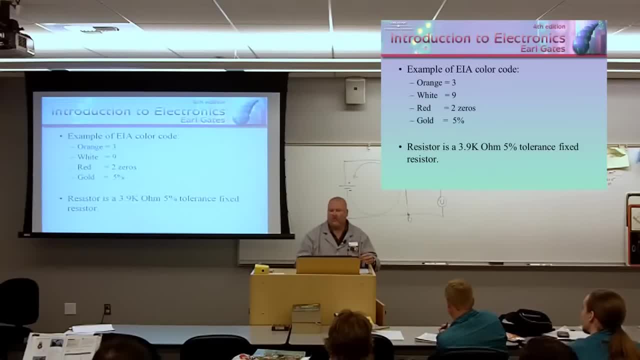 And when you're prototyping a circuit, you're going to say: I'm looking for a 1.5K ohm resistor And you find it, you plug it in your circuit and you move on. So Resistors and circuits. 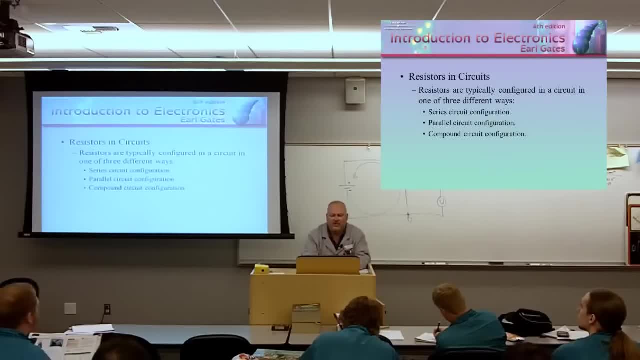 Resistors are typically configured in a circuit in one of three different ways: Either series, parallel or compound. And, to be honest with you, I hate to let the cat out of the bag, put the cart before the horse, But you know what? 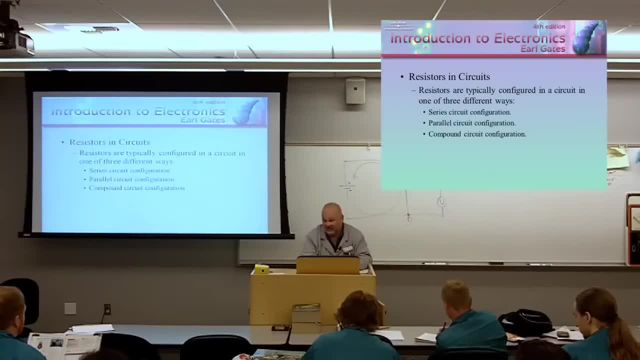 In the entire world of electronics and the entire universe of electronics, there's only three types of circuits. And here you are, week number three, learning about them. It's that simple: The most complex circuit you ever work on in your life. 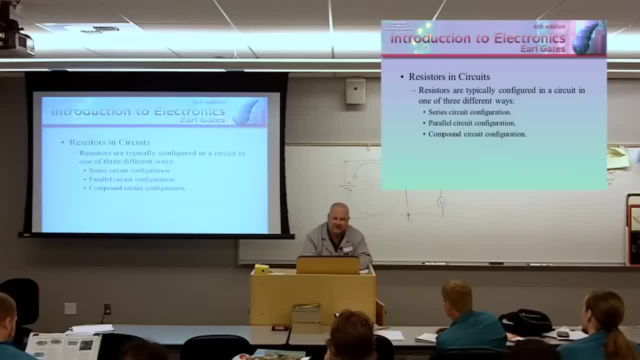 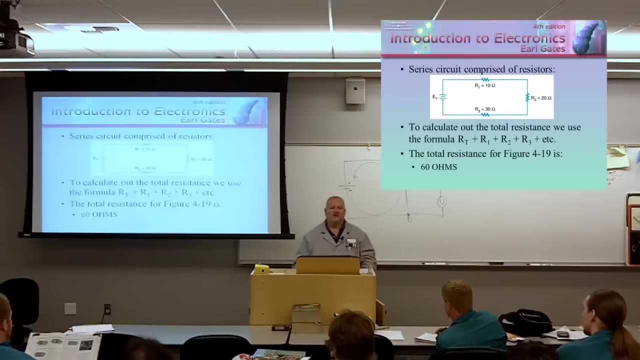 will be one of these three. It's either going to be a series circuit, a parallel circuit, or it's called a compound circuit Or a combination. yeah, The first circuit we're going to talk about is the series circuit, And the simple thing to remember with a series circuit is: resistance is additive. 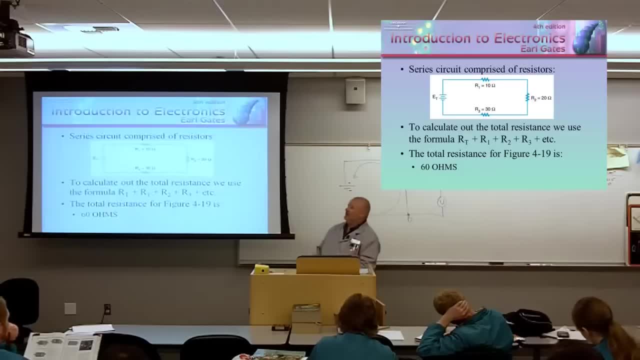 Resistance is additive. So the formula that we need to remember- and this is not accurate- This should have an equal sign. right here There's an error in this formula. It should be: RT. total resistance is equal to resistor 1 plus resistor 2 plus resistor 3 plus, etc. etc. etc. 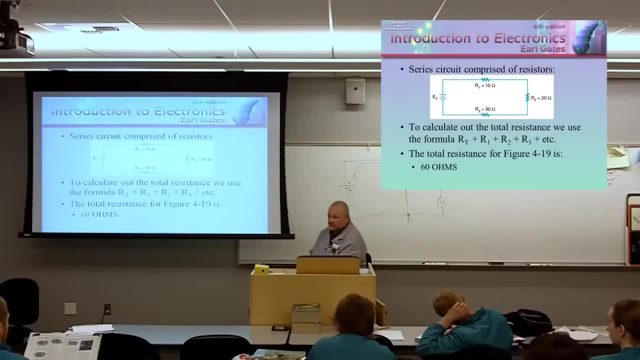 If you've got 5,000 resistors in a circuit, you're going to have 5,000 resistances to add up. It's cumulative. So in this particular circumstance, all we have to do is pick a point in the circuit. 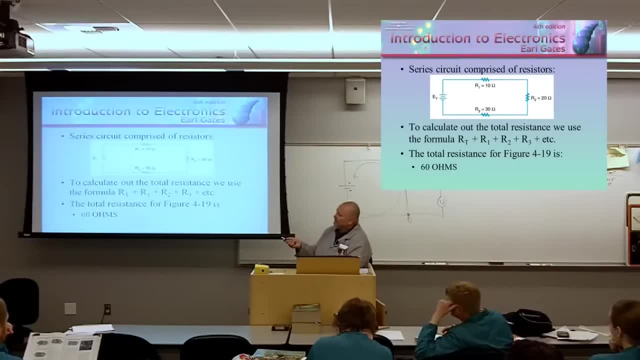 and start to calculate. We'll start right here, at the negative terminal. The first resistor I encounter has 30 ohms of resistance. 30 plus 20 is equal to 50 plus 10 is equal to 60.. That completes the circuit. 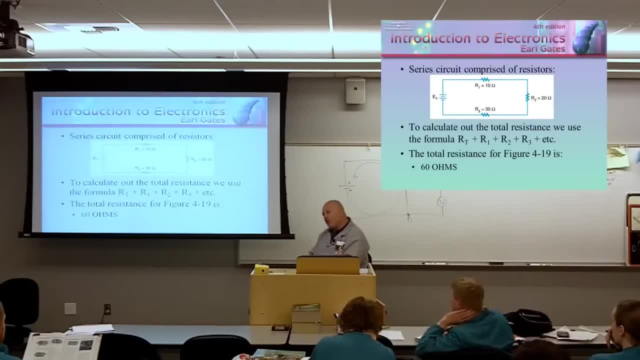 In this circuit there are a total of 60 ohms of resistance. Does that make sense? Sounds real basic, doesn't it? It's all fun and games until you have a bad battery connection. right here There's some corrosion that adds some resistance. 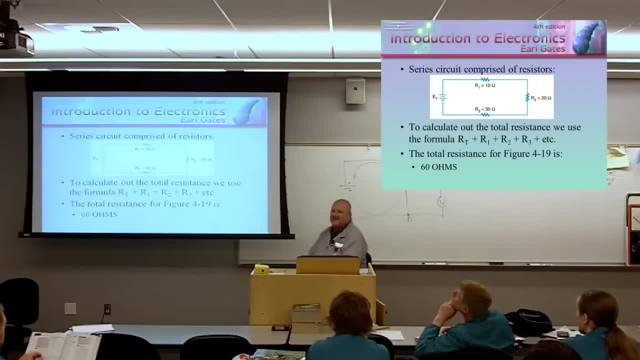 You've got a bad solder joint right here. It adds a little bit more resistance. So in a theory class like this, how many ohms of resistance is there supposed to be in a circuit 60. You get in there and measure it with your meter and you get 67 ohms. 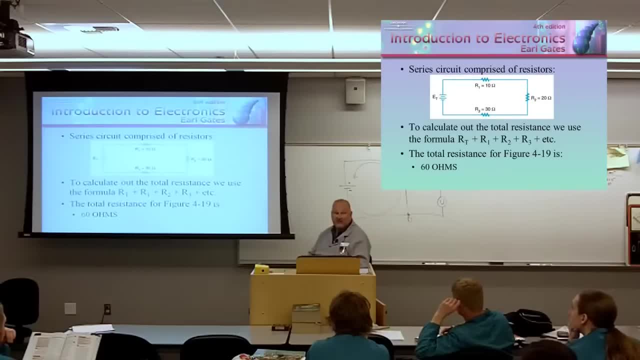 Then you realize you have tolerance of these resistors. Did you take that into account? Yeah, But that only accounts for a small percentage. Then all of a sudden you realize: well, I've got corrosion in the circuit, Or I've got a bad solder joint in the circuit. 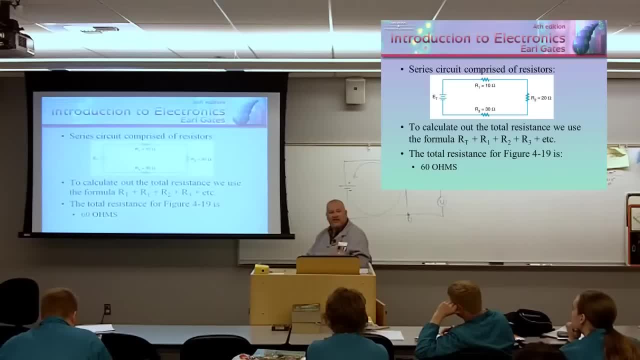 So that's where there's a disconnect sometimes between the world of theory that we live in here in a classroom, a lecture environment, and the world of reality in the lab. That's why I want to see all of you getting in the lab doing your lab assignments. 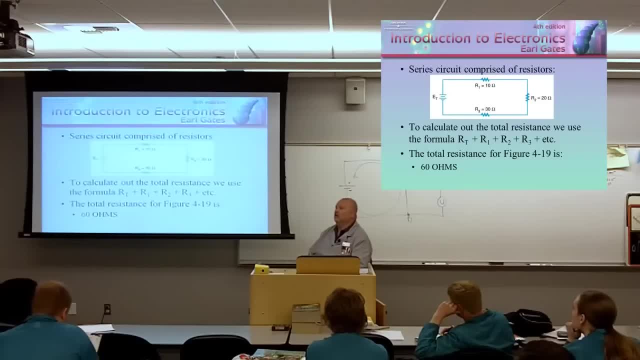 Because you're basically going to start scratching your head saying, Hey, I thought Joe, I kind of believed what Joe was saying in a lecture, but it isn't quite working. I don't like that. It's going to work, like I say, but there's going to be also a lot of variables that take place in the lab. 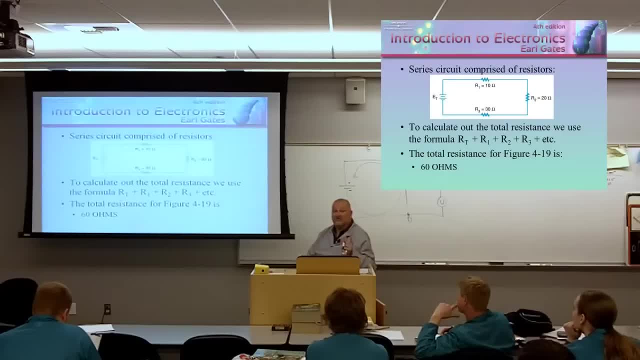 and in the real world. As I said before, that's the toughest thing that I had. when I got out into industry, I went through a bunch of theory schools. When I started seeing things for real, I was like, whoa, this doesn't make sense. 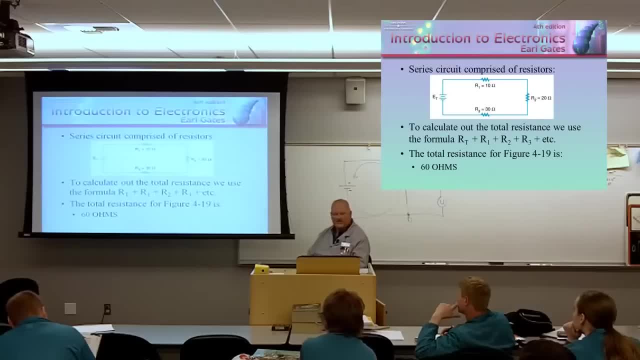 Is this good? Can this possibly be good? This doesn't look like a good reading. I mean, it's not what the book says. How could this be good, You know? So that's the only way you're getting that is experience. 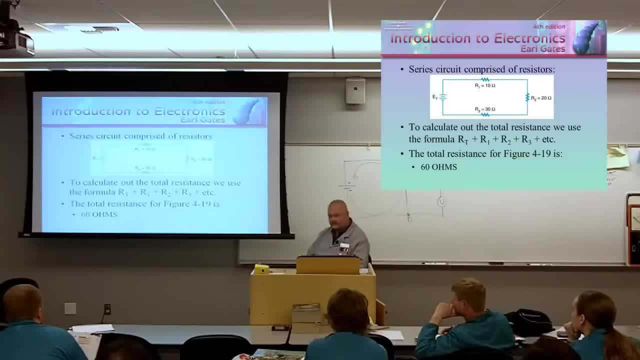 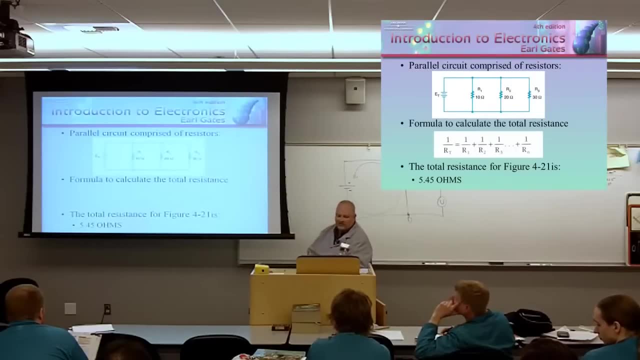 Any questions on series resistance Parallel. This is my favorite slide of the entire quarter Because, like watch, I'm going to hit the key and the formula is going to fly in from the side. Isn't that cool. You ever see how people like abuse PowerPoint and use too much animation. 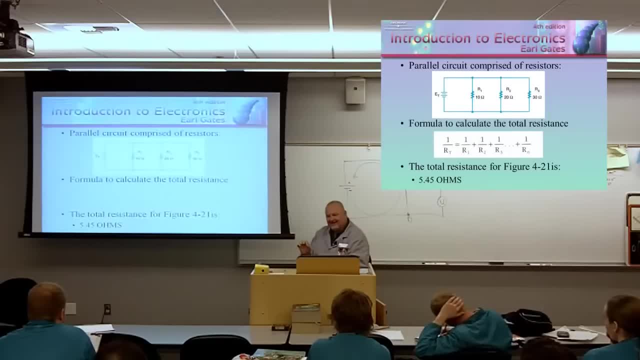 This is just right And I'm going to do it one more time. It's the last time. I'm going to do it The entire quarter. the last slide that I have that's animated is this slide. Okay, you ready. Just kidding. 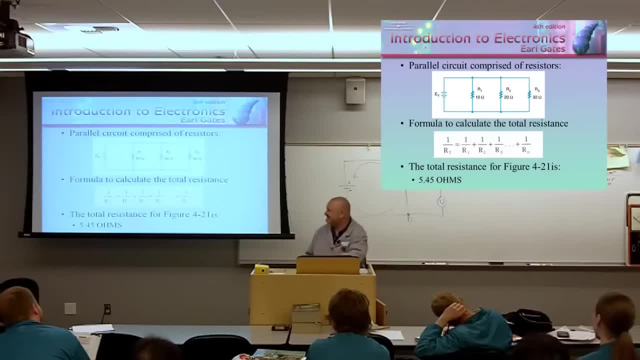 One more time Now, in order for us to calculate out the total resistance in parallel. this is kind of different. This is kind of odd. Right? This is kind of odd. This is kind of odd. What we're going to do is this reciprocal formula, the reciprocal of resistor one plus. 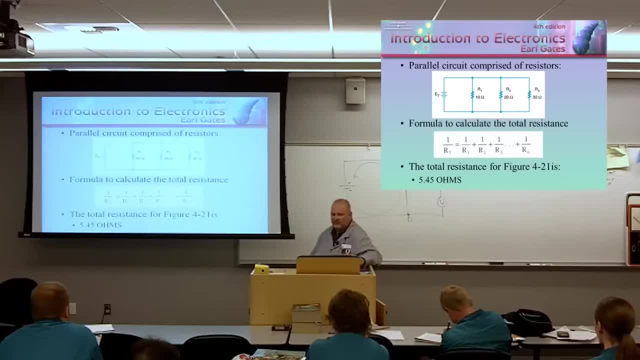 the reciprocal of resistor two plus the reciprocal of resistor three, on and on and on. That sounds awful familiar to me. What is the reciprocal of resistance Conductivity? Remember that One over R equals Conductivity. Conductivity Siemens measured in Mohs. 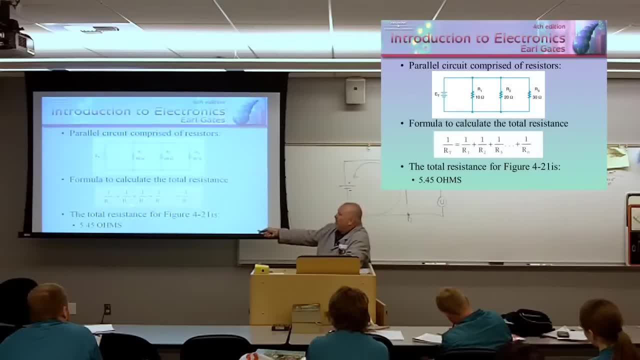 So what we're saying here is by adding up all of the conductivities of all of these branches to a parallel network, then taking the reciprocal of that, we end up with total resistance. So this is kind of like a bar trick. How can you add resistors to a circuit and yet make the resistance of the circuit less? 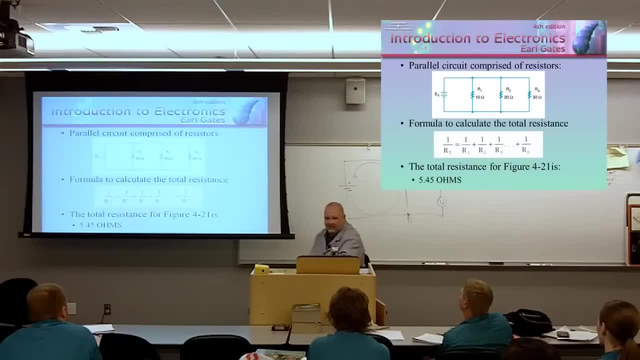 The answer is: add them in parallel, Because that's exactly what we're doing here. It's exactly what we're doing. Think of this as the Seattle traffic system. Seattle traffic system. Okay, Uh-huh, All right, This is a. it's a Friday afternoon before a three-day weekend. 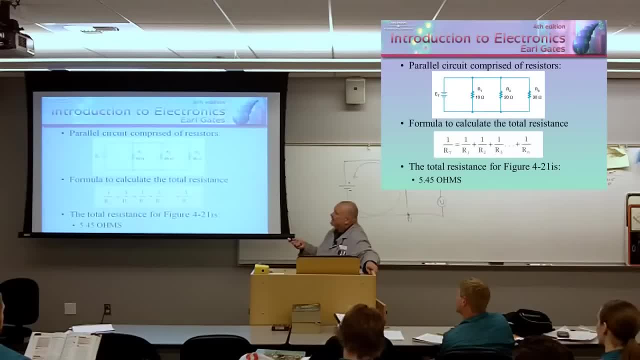 And these are all the people that are in Seattle And they want to get to Bellevue And they've got multiple paths to take. How do you get from Seattle to Bellevue? 520.. How else? I-90.. How else? 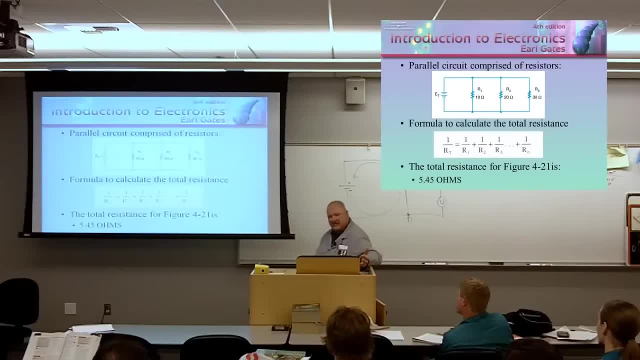 Up and around the north end of the lake Or down around the south end of the lake. So basically we've got four. Let's say let's just talk about three for the case of our example here. If you're in Seattle, I'm a big commuter, so I like these analogies. 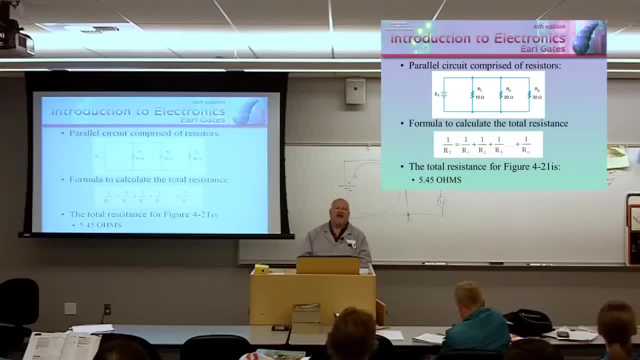 They really work well for me. They work all too well for me. If I'm in Seattle and I want to get to Bellevue and it's a Friday, three-day weekend, what path is probably going to be the best for me to take, and why? 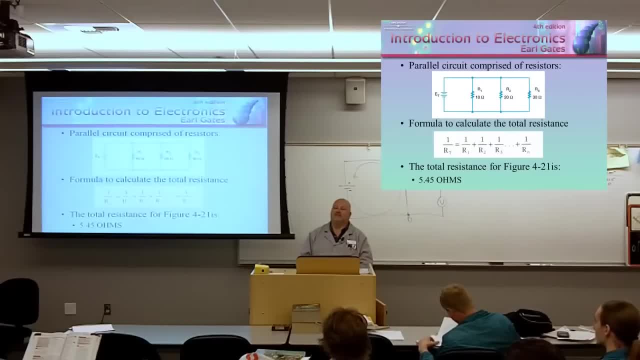 What's that? No, No, No. If I'm in Seattle and I want to go to Bellevue three-day weekend, which is the best path for me to take? and why? Why, Most lanes, Most lanes. It's going to move the most traffic. It's got the least amount of resistance After I-90,. what would be my second choice Before the toll. The toll will quickly make this number three choice, At least for me. I'm a tightwad. I'll take the ferry to Vancouver and drive down and around before I get a boat. 520.. 520 has fewer lanes, It's got more resistance. It doesn't move the same amount of traffic. And then, finally, the other option is driving around the north end or the south end of the lake. Not an easy way of doing it. 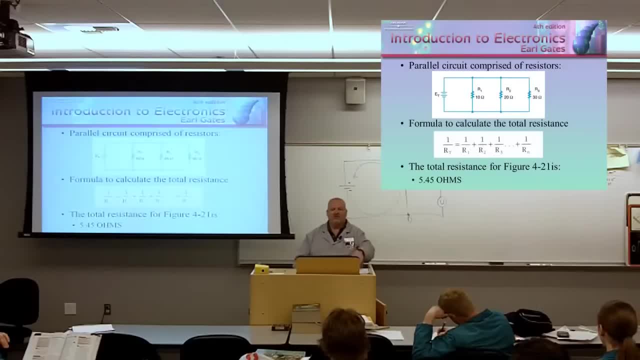 A lot more traffic, Less traffic, Less flow. So comparing that now to this, we could say that I-90 is like the equivalent of 10 ohms of resistance, Because even though I-90, it's a super interstate highway and it's got multiple lanes, does it still have resistance? 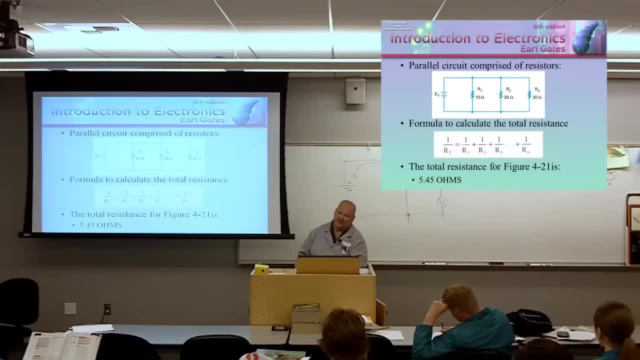 Oh yeah, Oh yeah. If it didn't have resistance, there wouldn't ever be any brake lights on it. This would be like 520, would be like twice the amount of resistance, meaning it moves. It moves half the amount of traffic. 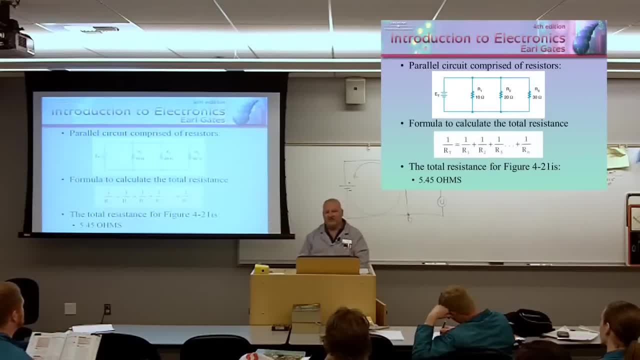 And then the north end of the lake. three times the amount of resistance, meaning even less traffic. Does that make sense? So every one of these is a viable current path. Every one of those routes is a viable traffic path. Let's say, for example: 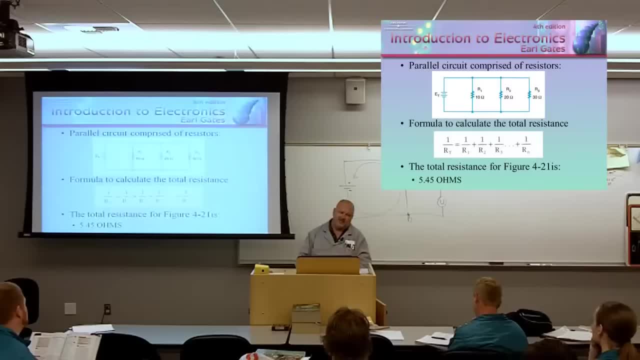 that Bill Gates. he really wanted to give back And he loves the people of the Puget Sound region And he wants to build another bridge across Lake Washington And he is so into it he's even going to let the bridge like come off of his property. okay. 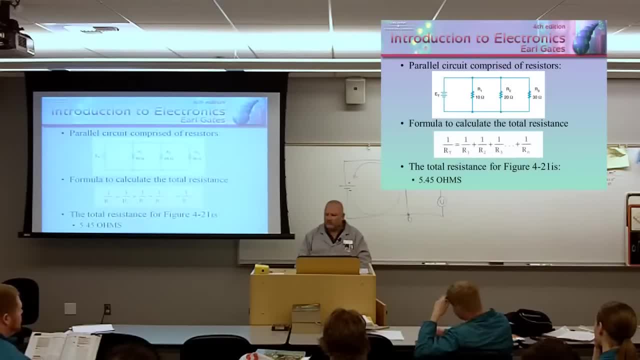 And because he's building the bridge, it's going to be called the Bill Gates Memorial Bridge. When he builds that bridge across Lake Washington, what's it going to do to this flow here? What's it going to do? It's going to make the overall circuit have less resistance. 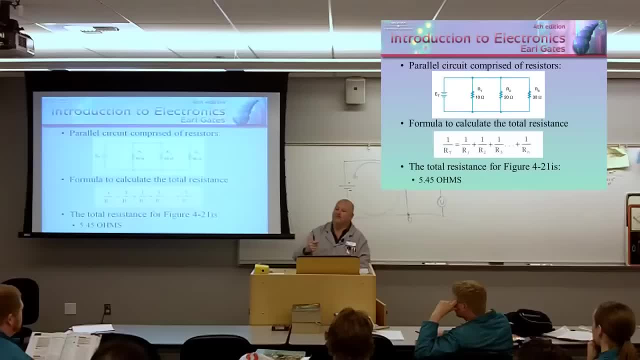 because he built another viable path. Is the path he builds going to be perfect? Is it still going to have resistance? Yes, But is it going to have an overall effect on increasing the flow in the Seattle metropolitan area of traffic? Absolutely, So that's how we can add resistance. 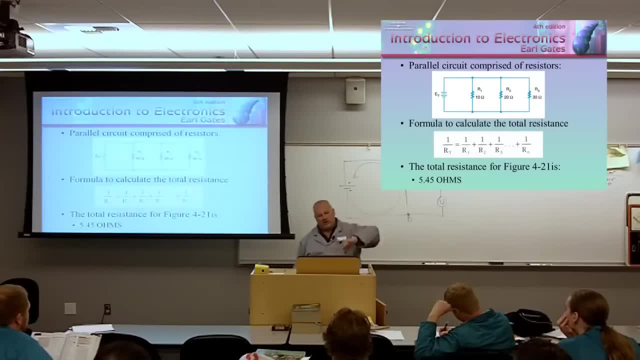 We can add resistances on this circuit yet lower the overall resistance of the total circuit, And that's why we have to use this formula. We're actually adding up the conductivity We end up with the total conductivity for the circuit. Take the reciprocal of that. 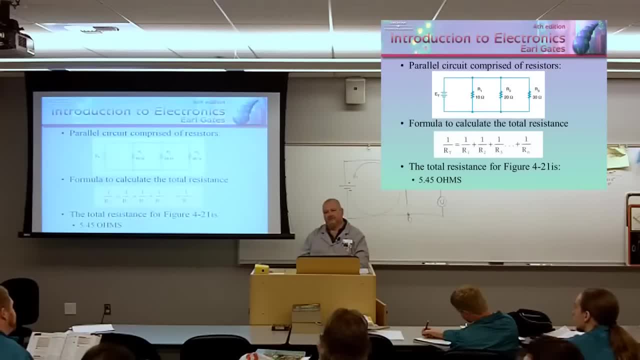 That gives us the total resistance for the circuit Make sense. Okay, Now I'm going to give you some thumb rules. Thumb rules, The first thumb rule that I want to give you. it's very, very important When you're analyzing a circuit like this. 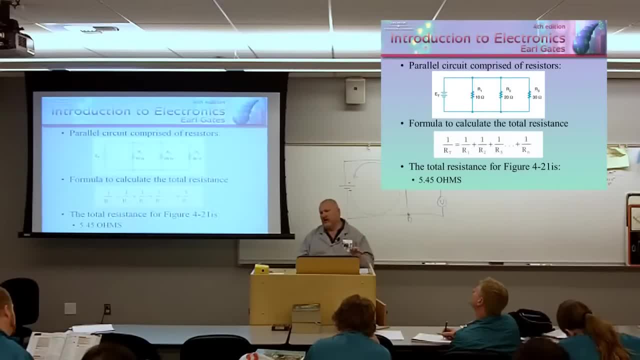 the total resistance of the circuit will always be less than the value of least resistance. If not, you made a mistake, Plain and simple. So you can guarantee the total resistance will be less than 10?? Absolutely. And if you come up with something other than that, 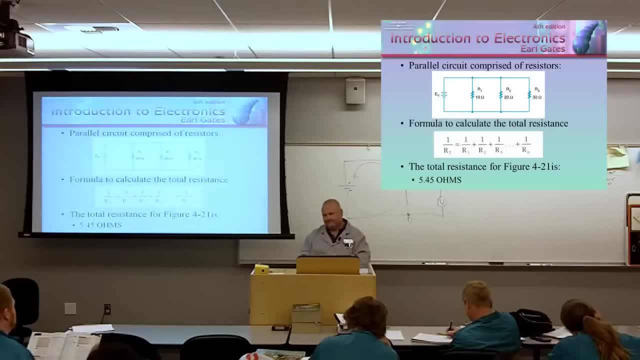 you're done, screwed up, Plain and simple. So the total resistance of a parallel network will always be less than the value of least resistance, And your assumption is correct. In this circuit it's got to be less than 10 ohms. 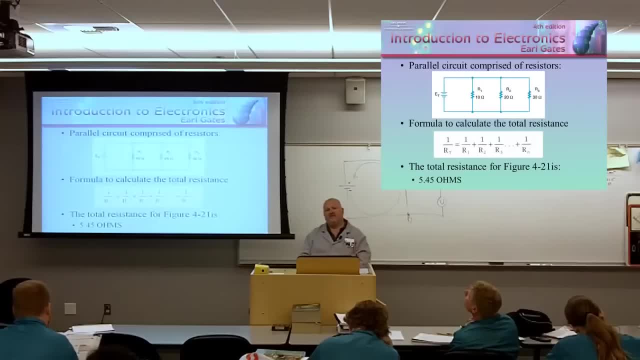 The other thumb rule that I'm going to give you is: if the values of resistance are all equal, you simply count up the number of resistors. take the resistance and divide it by that number. As an example, if R3 is 30 ohms, 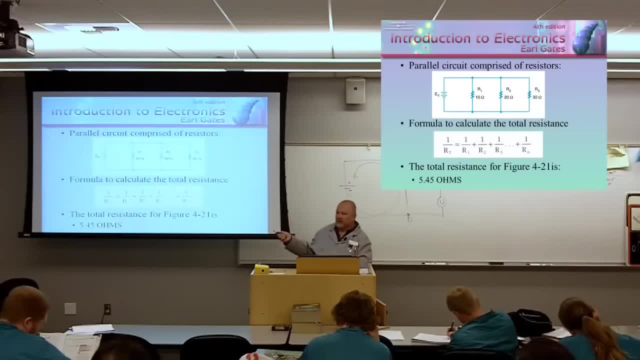 R2 is 30 ohms and R1 is 30 ohms. 30 divided by how many resistors Equals 30 divided by 3 equals 10.. The answer to this is going to be 10 ohms. 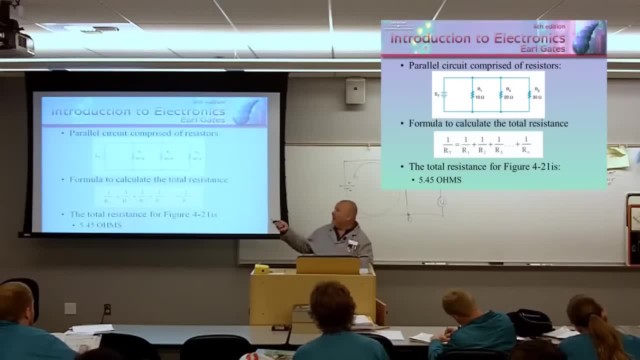 That's a thumb rule. So if I've got four 100 ohm resistors in parallel, 100 ohms divided by 4 equals 25.. If I have two 50 ohm resistors in parallel with each other, two 50 ohm resistors 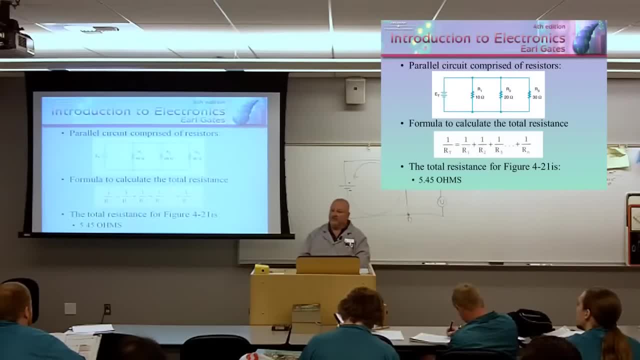 25.. 50 divided by 2? 25.. So that's a thumb rule, Only if the values are equal. So a lot of times in the lab you may be looking for a certain value of resistance. I need 20 ohms of resistance. 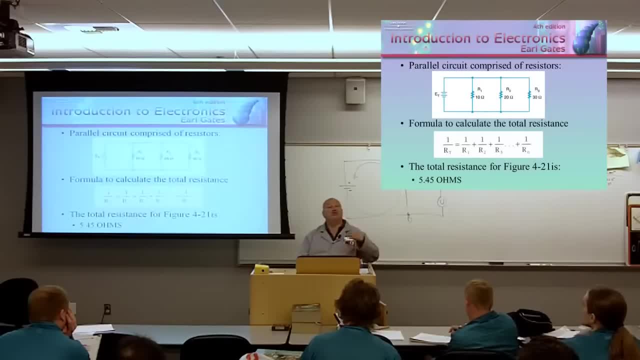 Or you could put two 10s in series with each other, Or you could put two 40s in parallel with each other, So there's a couple different ways of doing it. It's one of the reasons we're teaching about this stuff. 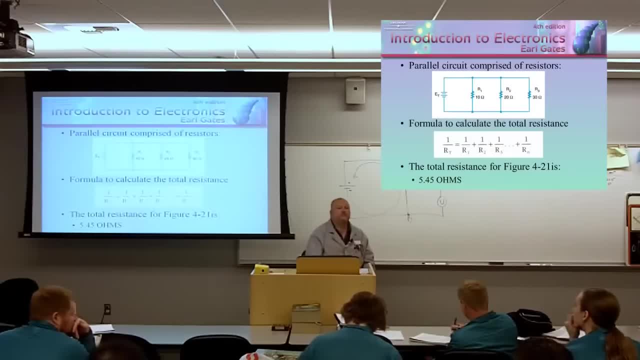 Make sense? Not yet. I'm just trying to synthesize it into a formula now. Okay, Add up all the resistors and then divide by The number of resistors. Only if they're equal. This only works if they're equal. 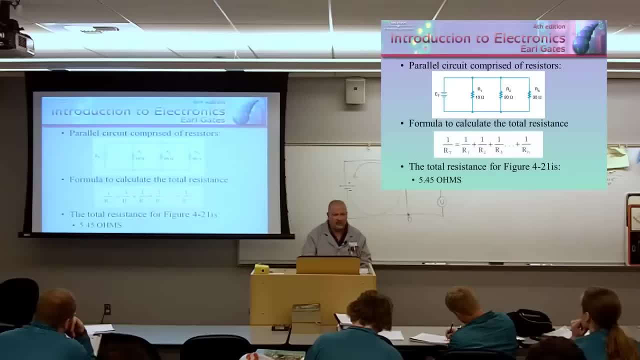 It's a thumb rule. You don't need to use the thumb rule, It's just another tool in your toolbox. Make it easier for you. If you doubt me, well, you could always use that formula. There is another formula I want to show you. 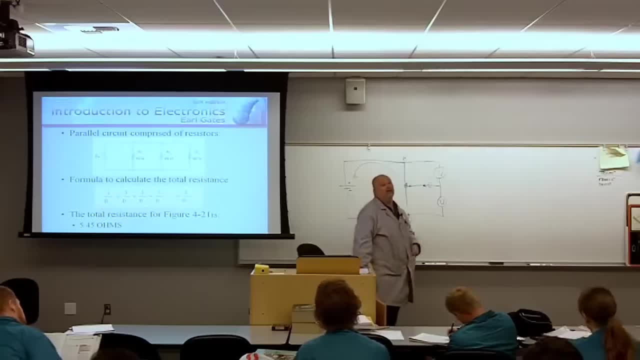 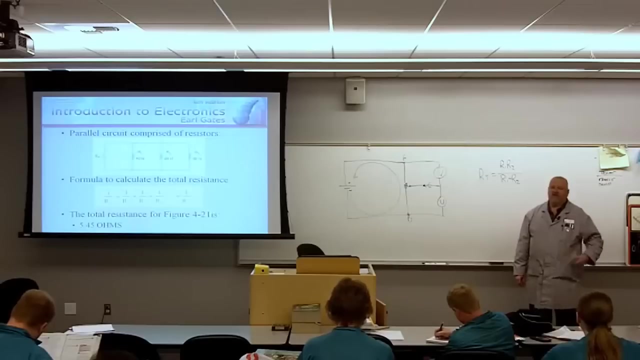 It's not in the book, but I want you to know it, Learn it. This is called the product over sum formula: Product over sum. This only works if we have two resistors in parallel with each other. period: Two resistors in parallel with each other. 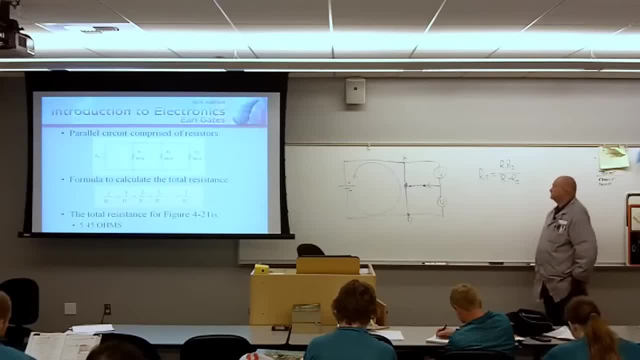 Two resistors in parallel with each other period. So this literally is the product over sum. The product is R1 multiplied by R2.. R1 times R2. Divided by R1 plus R2.. The product over the sum. 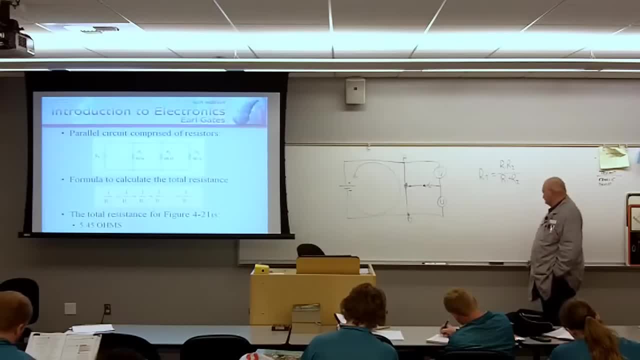 This works if you only have two resistors in parallel with each other. Problem solved. If you've got two or more resistors, you have to use this formula here. I just drew it a little bit differently, but that's basically the same formula. 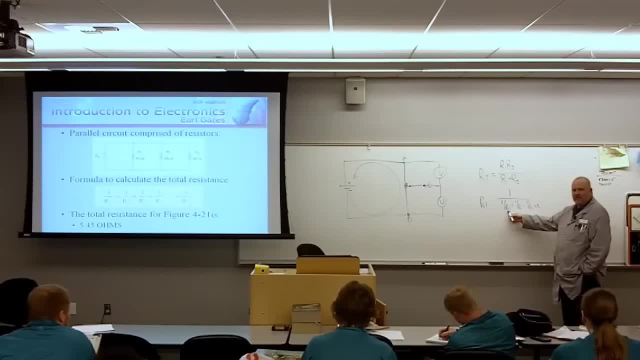 The reciprocal of R1,, which is the conductance of R1, plus the conductance of R2, plus the sum of the conductances, total conductance. the reciprocal 1 over the total conductance equals the total resistance. 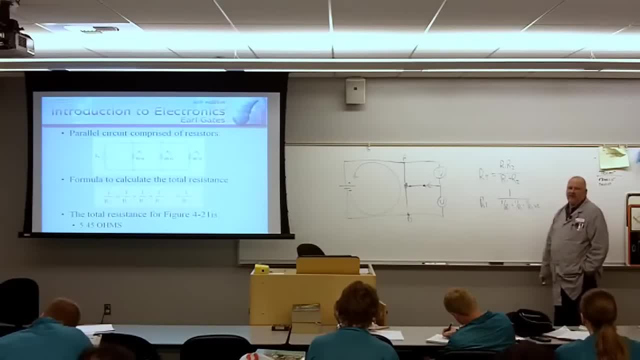 So this formula works for two or more resistors in parallel. Well, this one here works for two resistors in parallel Period. The reason I want you to start using this is because, in the future, we're going to take this formula and we're going to adapt this formula for some other use. 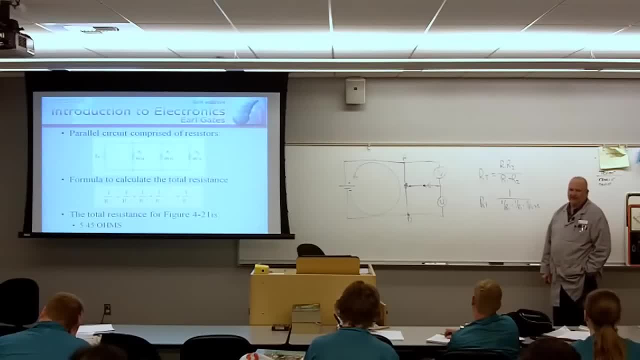 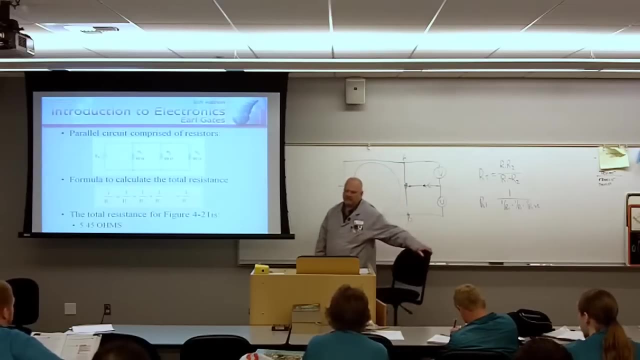 So it's better that you just learn it now and it's another tool in your toolbox. Product over sum- easy enough to remember. Product over sum When we execute the math on this formula here: the reciprocal of R1 plus R2 plus R3,. 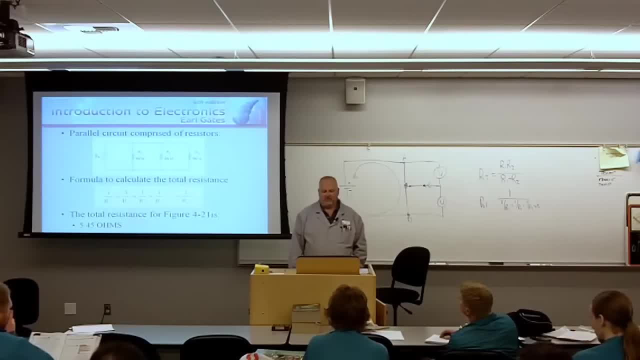 we add those conductances up, take the reciprocal of it, we end up with 5.405 ohms. Does that answer sound right? Why does it sound right? It's less than 10.. Works for me. In that slide. could R3 be considered Rn? 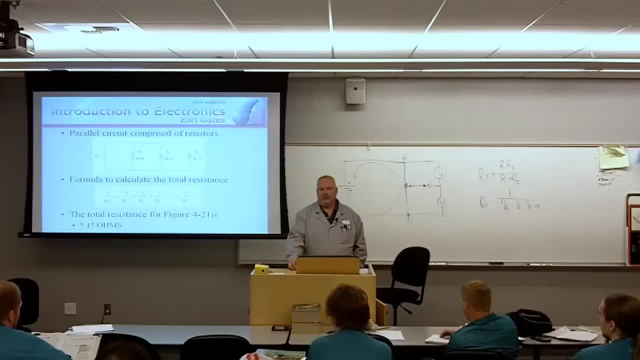 No, Rn would be like R4, 5, R22, R447.. R to the nth degree means to the nth degree. This formula works to infinity. If we keep adding resistors in parallel, we just keep adding the reciprocal of that resistance on it. 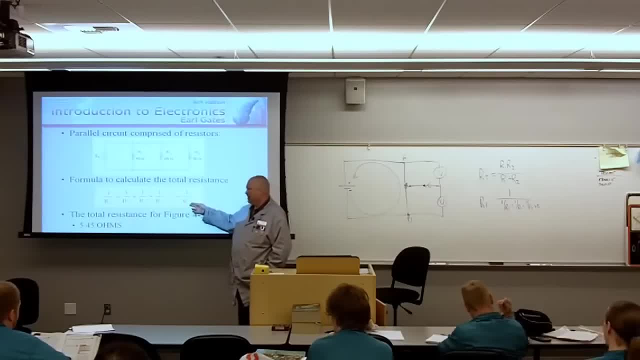 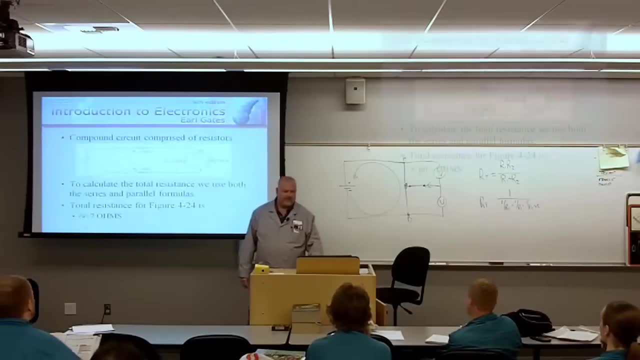 That's what we mean by that. So they drew it like this: plus 1R to the nth. I did it, etc. etc. etc. This is a complex circuit. Now, again, I know you want to do the math, you want to get it right. 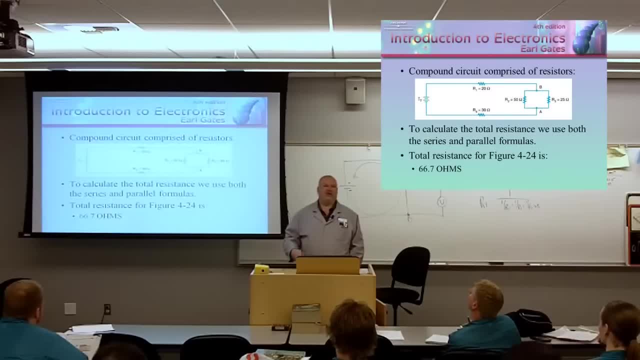 That's cool. okay, I want to keep things real. I want to keep things basic. The first thing that I notice in this circuit is that these two resistors are in parallel with each other, So this is an actual ideal situation for us to use this product over sum formula. 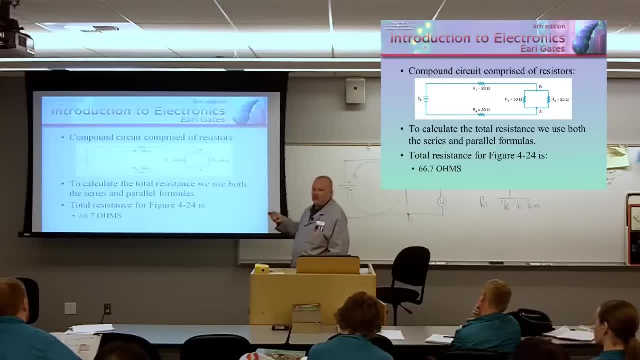 50 times 25, divided by 50 plus 25.. Why don't we just do it right now? You got your calculators, Let's do it, Just do it. But I want to do it in stages here for those folks at home. 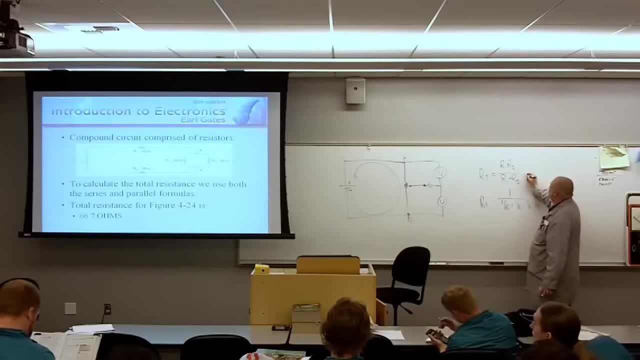 This is how I'm going to start off with the formula. Now what I'm going to do is substitute in my numbers What is that? 50 and 25?? So it's going to be 50 times 25, divided by 50 plus 25, okay. 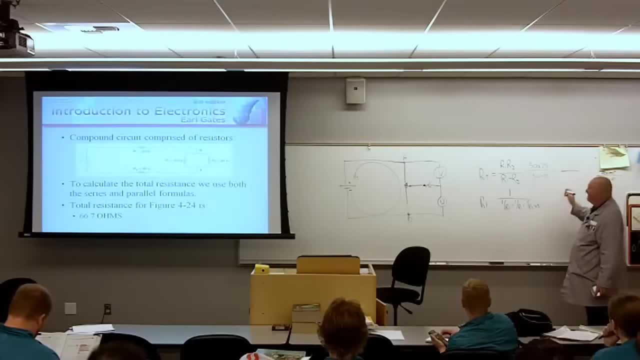 I know that this is going to 50 plus 25, I could do that in my head. right, That's 75, okay, But the 50 plus 25.. 50. Excuse me, Times 25 equals. 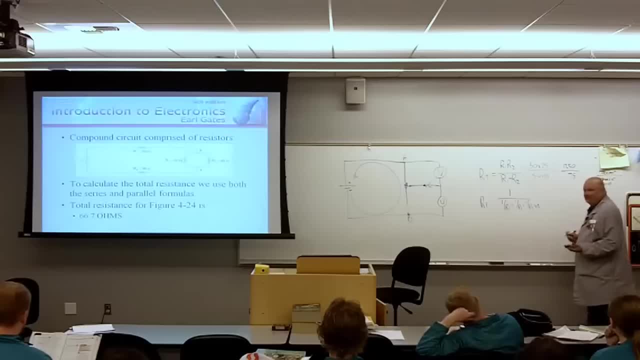 12. 12. 50.. So 12. 50 divided by 75 equals 16.67 ohms. So does everybody see how I did that? Isn't that a cool formula? It's cool, I like that formula. 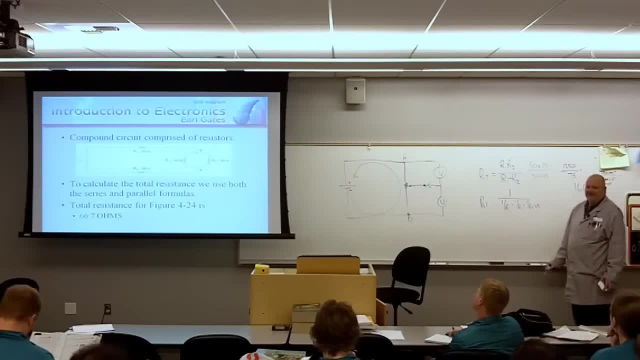 I don't know why, Because the answer is always like: come out, I don't know. I like that formula. You can do the same thing down here and you're going to get the same results. So I know that I've got. 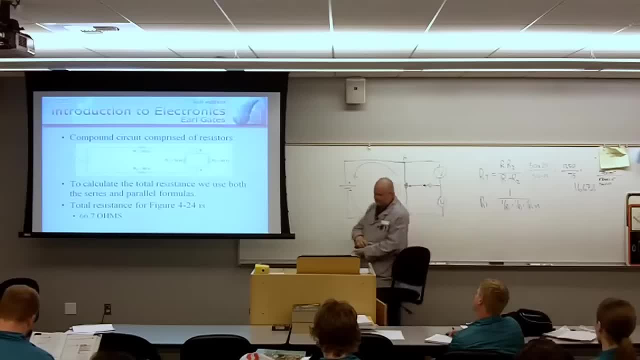 And the way I want you to look at these parallel circuits, The way that I want you to think of these parallel circuits, is: how much resistance is there between this point here And that's actually called a node? A node are where two or more wires are joined together. 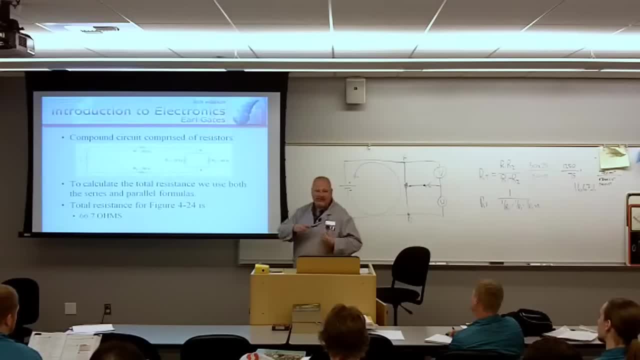 How much resistance is there between node A and node B? So to lay this out mathematically, The way that I would actually calculate out this whole problem is RT. for this circuit, total resistance is going to be equal to the resistance of resistor 1 plus the resistance between node A and B. Plus the resistance of resistor. 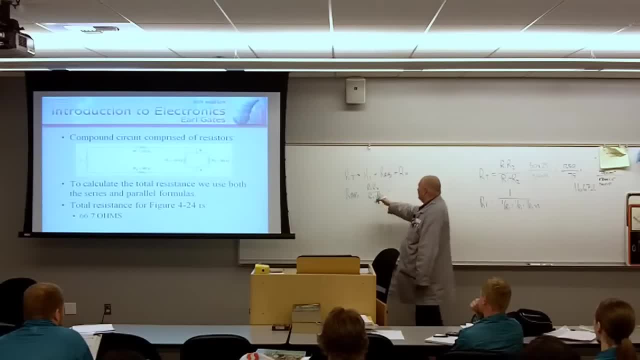 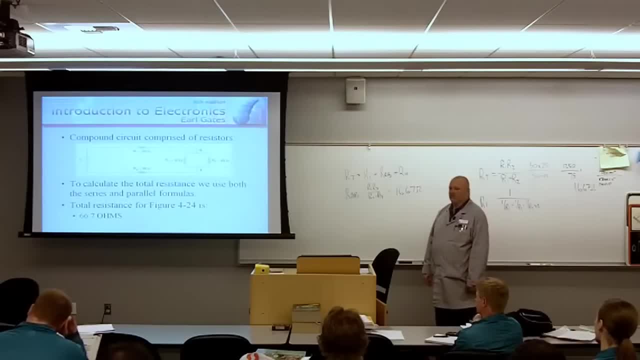 So I highly recommend, until you really got a handle on this, you lay it all out like this: to the problem: Use the right tool, you get the right results. Use the wrong tool on your car. 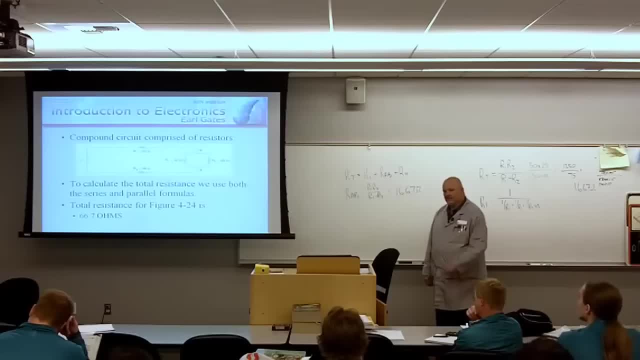 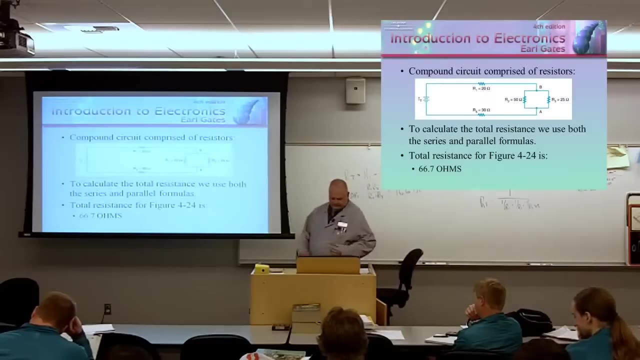 you strip the nut, Use the right tool, you get about the results that you desire Make sense. When you first see a problem like this, though, one of the things that I'm going to stress in this program is that you keep it real. 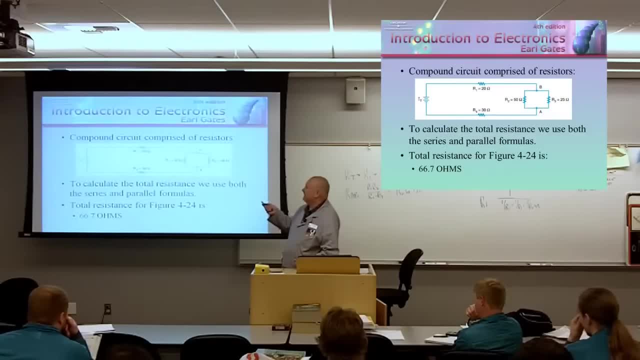 What was this total resistance going to be between this A and B? It's going to be less than 25.. So I've got 30 ohms here and 20 ohms there. 30 plus 20 is 15, and less than 25.. 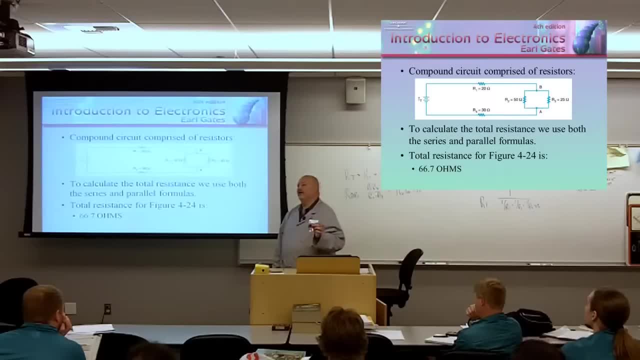 What do I know? my answer is going to be Less than what? Less than 75.. If you could do that in your mind, looking at this, I want you on my team. I'll be honest with you. I want you on my team. 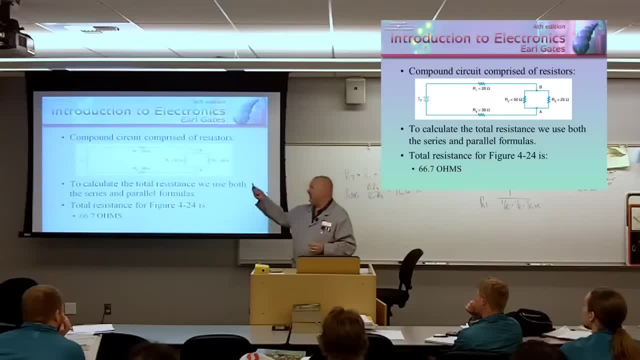 Those are the people that I want. If I give you this problem and immediately you're with the calculator, I don't mind if you use the calculator, but if you're turning it upside down, you're sideways. no, What I want out of all of you is to look at this. 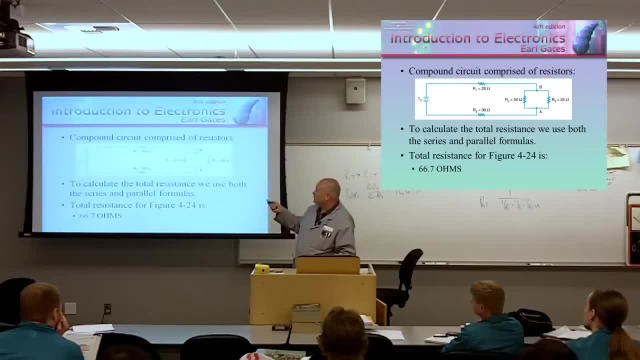 I've got 30 ohms here. I've got 20, that's 50, less than 25, my answer is going to be less than 75 ohms. Do not try to take my quizzes doing that. If you do, you'll probably be very successful. 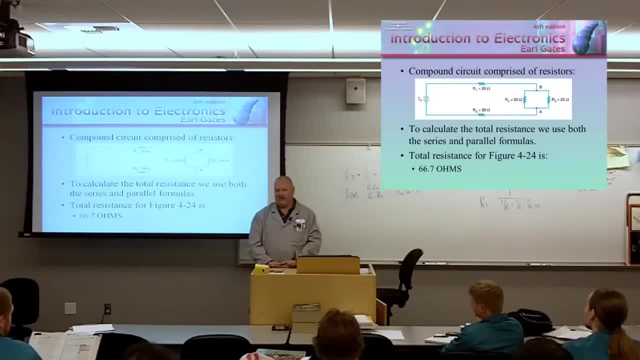 with a lot of my quizzes. I could take most of my quizzes and not even use a calculator and get them all right. Well, that has something to do with the fact that I wrote my quizzes, But what I want you to do is that thumb rule. 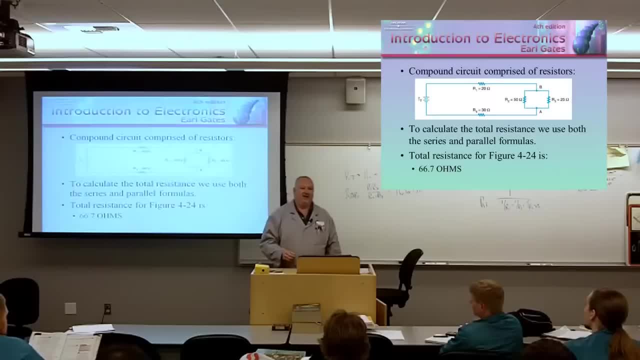 as a litmus test at the end or even before you calculate it. I should get less than 75 ohms as an answer. My answer should be less than 75 ohms. I came up with 66.7 ohms. 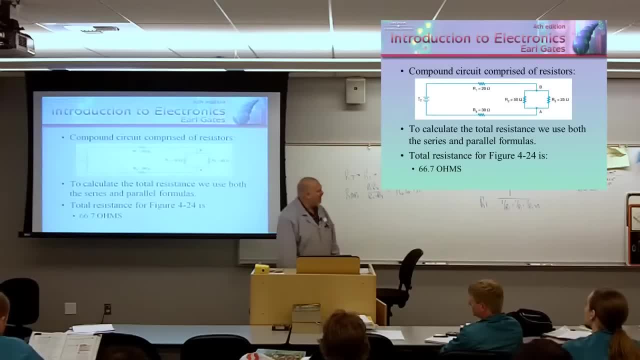 Does that sound about right If you come up with an answer of what's the total resistance in a circuit? 1,250.. Well, that's not less than 75.. Houston, we've got a problem. There's probably a math error. 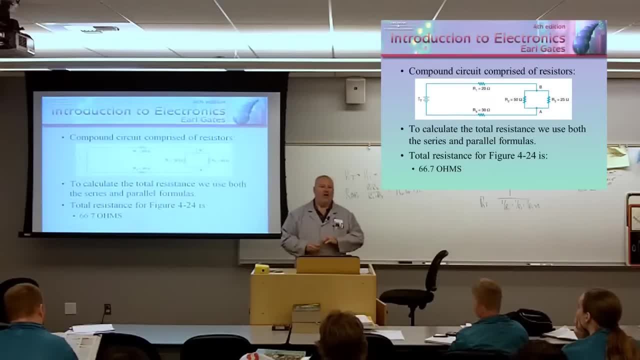 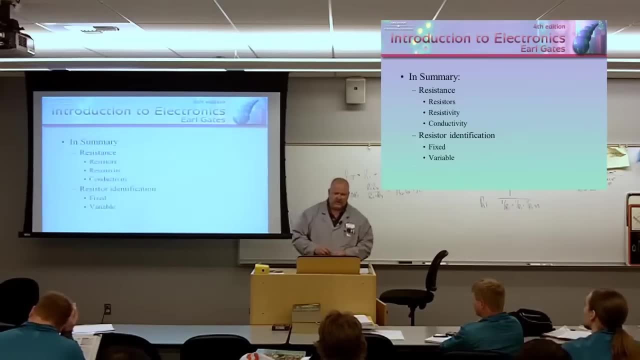 If I were Pope of Electronics, I would require you to all get 100% on all of these quizzes, Because if you use the right tool, you get the right results. Make sense, In summary: we talked about resistance. What has resistance? 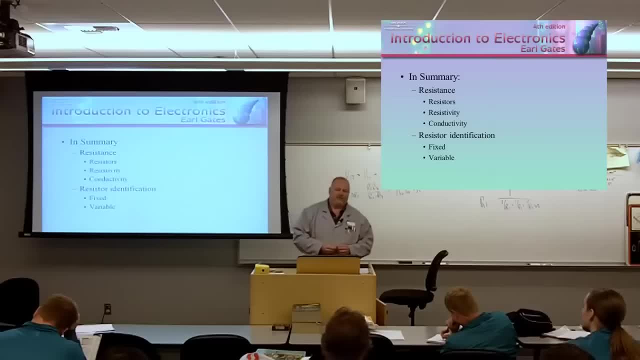 Everything, Everything. We talked about specific devices that are designed to possess the property of resistance- It's known as a resistor. Can you imagine? some dude wakes up every day and, like you know, instead of it's off to make the donuts. 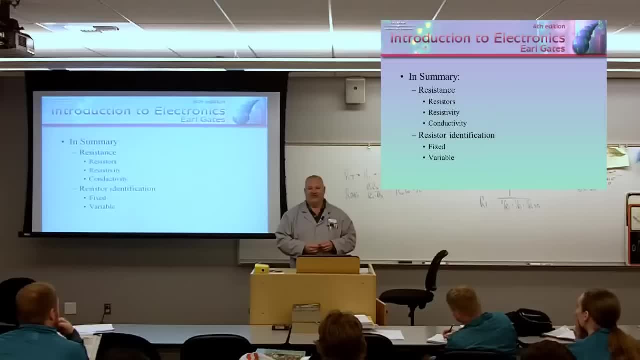 it's off to design the resistors. There are engineers in the world that design resistors for a living. huh Woo, Talk about a crazy career path. Resistivity, That property. that we compare the resistivity of everything to that of silver. 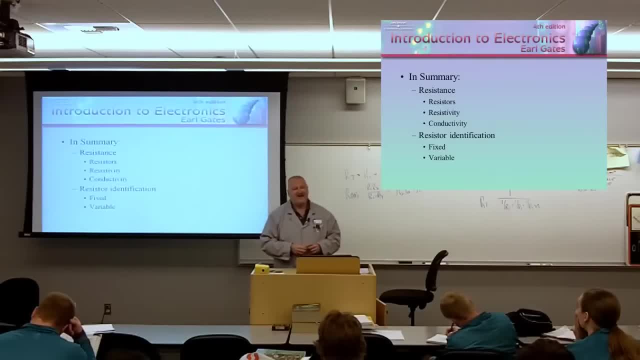 Silver, The best conductor found in nature. Conductivity: Conductivity: The reciprocal of resistance measured in moles, or typically millimoles. Resistor identification for fixed value, variable values: We talked about fixed resistors, variable resistors. 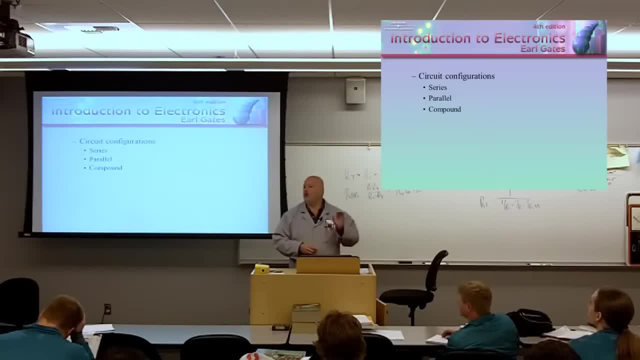 that could be configured as potentiometers. if they're used to control voltage, Rheostats. if they're used to control current. If I'm using three leads, I'm using it to control voltage. If I'm using two leads, I'm using it to control current. 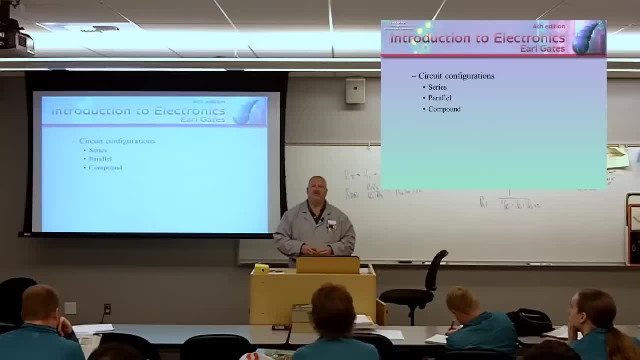 And then, finally, we talked about circuit configurations. First was a series configuration. In a series configuration, how do I determine total total resistance? Simply add it up. It's additive In a parallel circuit. how do I determine total resistance? 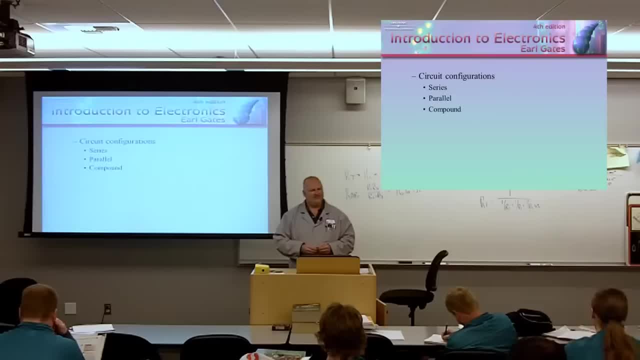 Add up the reciprocals Sounds like I'm adding up the conductivity of the paths In a compound circuit. what do I got to do Both Thumb rules. for parallel circuits, Total resistance will always equal less than the value of least. 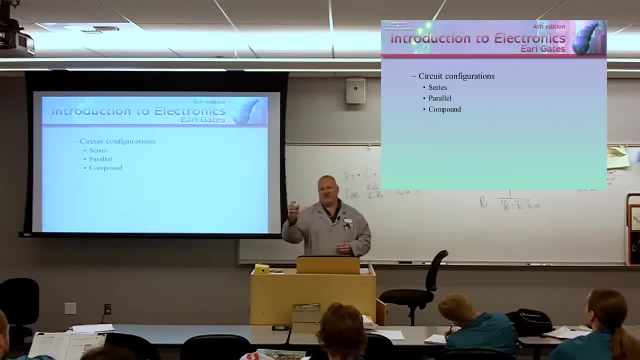 And if I have like resistors same size, then I could simply take that number, take the value, divide it by the number of resistors that I have and that will give me the total resistance. Any questions out of this chapter? 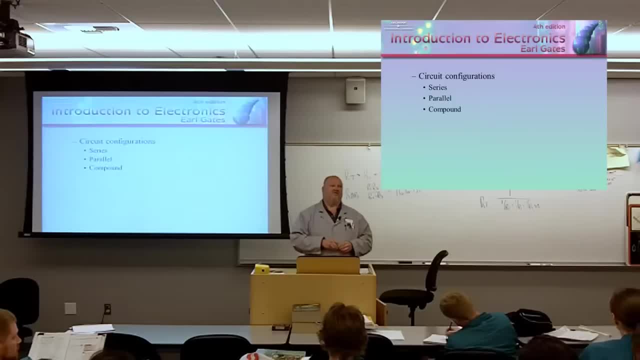 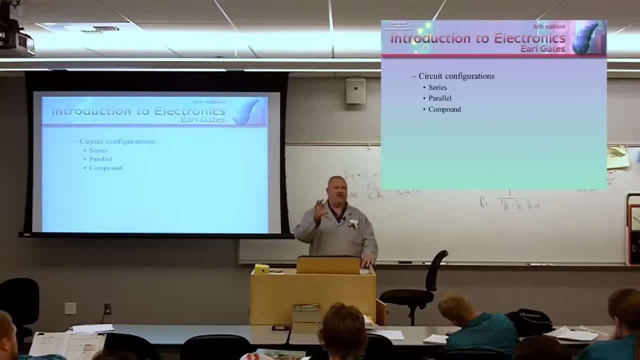 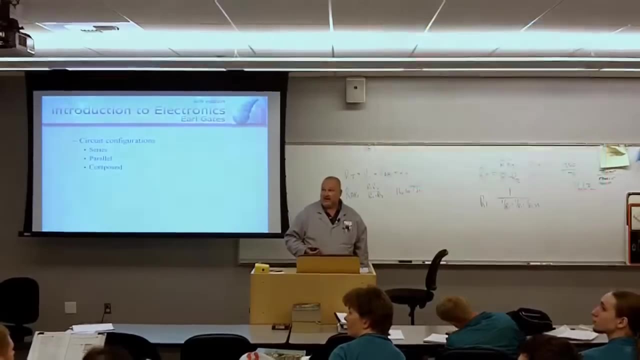 Four. 100 divided by Four equals 25.. I should have approximately 25 ohms across that circuit. All right, Let's go ahead and take a about a 10-minute, 12-minute break And we'll start up at about 10 after. 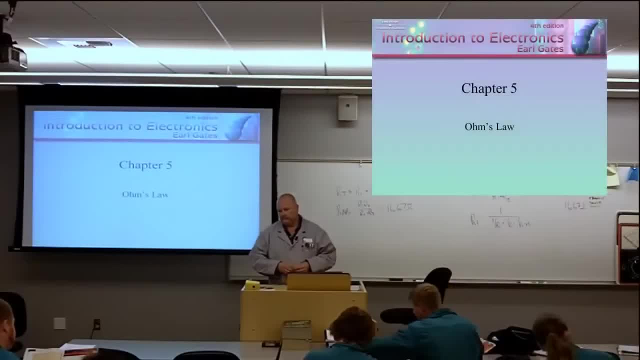 All right, Chapter 5, Ohm's Law. Again, we should like hit a gong, ring a bell, ring some chimes, Ohm's Law. Ohm's Law has more of an effect on being able to predict the behavior. 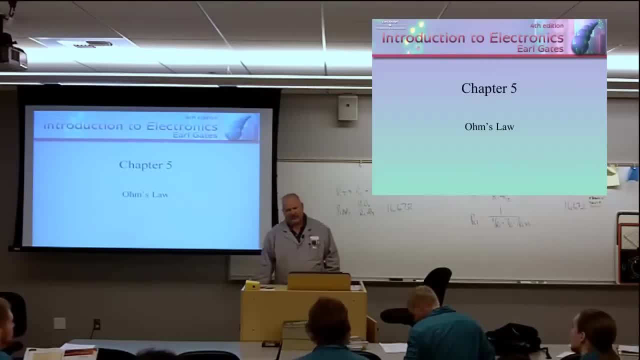 of electricity than really anything else. Does anybody know how predictable the behavior of electricity is Percentage-wise? we're talking about tolerance's last chapter. Anybody know how accurate we could predict the behavior? I'll say 100%, 100%. It's a bold statement. 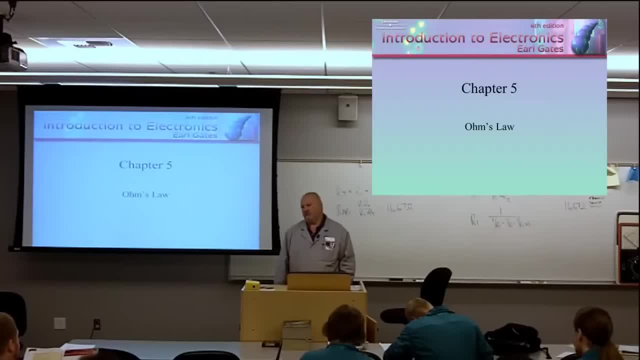 It's absolutely correct, 100%. You use Ohm's Law. you could predict with 100% accuracy what's going to take place inside a circuit. It's pretty powerful. It's a pretty powerful tool, Especially when you're going to be paid. 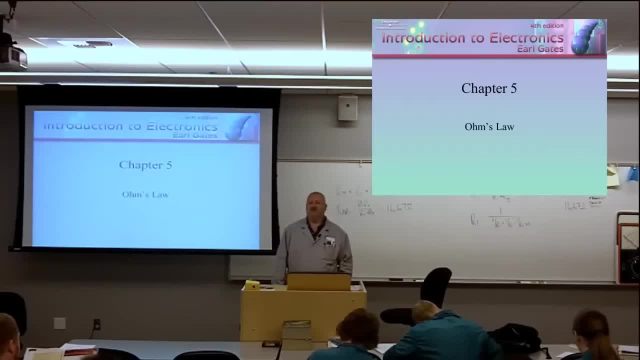 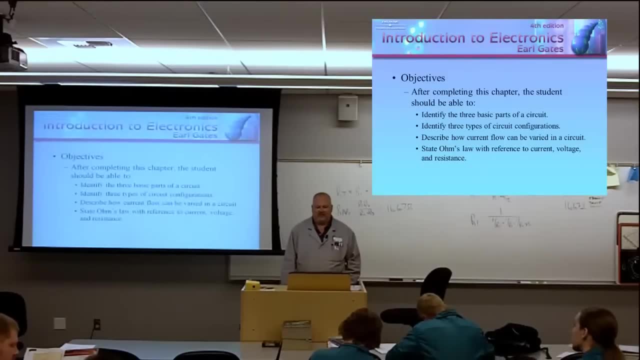 to go out into industry and fix broken electronic equipment. You've got this tool working for you. You've got something. After completing this chapter, you're going to be able to identify the three basic parts of a circuit, Identify three types of circuit configurations. 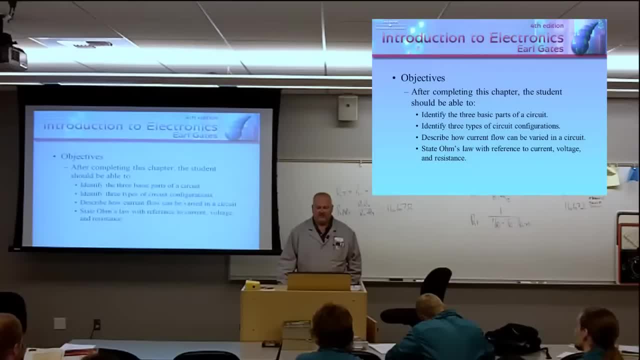 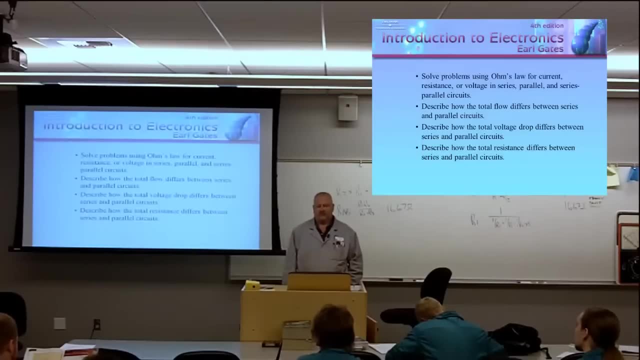 Describe how current flow can be varied in a circuit State Ohm's Law with reference to current voltage and resistance. Solve problems using Ohm's Law for current resistance, voltage and series. parallel circuits. Describe how the total flow differs between the current resistance. 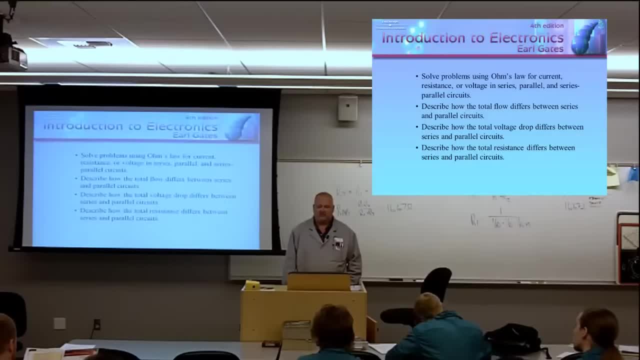 series and parallel circuits. Describe how the total voltage drops differs between series and parallel circuits. Describe how the total resistance differs between series and parallel circuits. State and apply Kirchhoff's current and voltage laws And verify answers using Ohm's Law with Kirchhoff's Law. 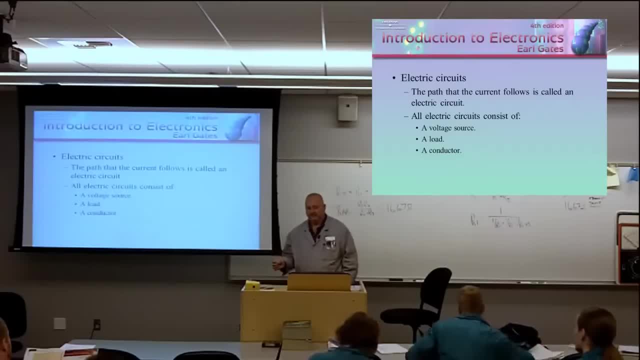 First of all, electric circuits are the path that current current follows is called an electric circuit. All circuits consist of- and this is important and it sounds really basic and it sounds very simplistic, but I'll tell you what Knowing this helped me. 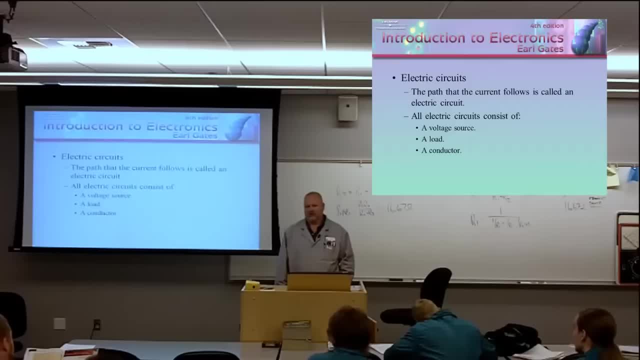 on my worst day of my career as an electronics professional, Because it's so easy to get turned around and lose track of what the problem is. And if you could get back to the basics you're always going to do well, The basics are all electric circuits. 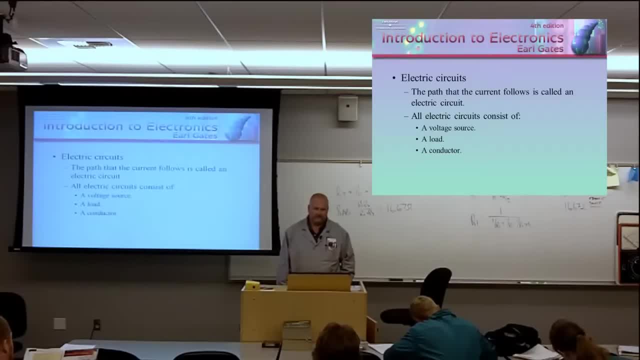 must consist of a voltage source, a load and a conductor. The voltage source is the source of your electric energy. It could be any of those six different types that we talked about last week. The load is what converts the current. It converts one form of energy. 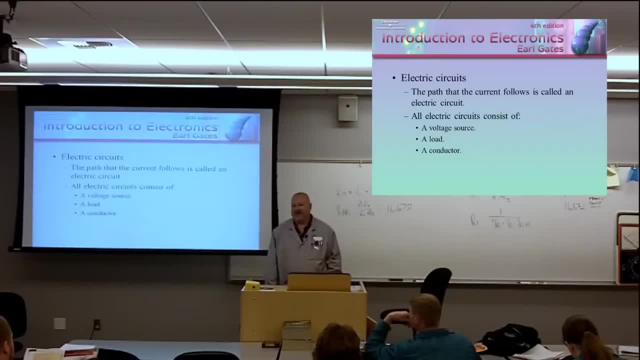 into another form of energy. An example of an electric load would be a light bulb, A motor, A heater. It converts electric energy into light heat, motion. A conductor, A conductor, electrical conductor, transfers the energy, the electric energy. 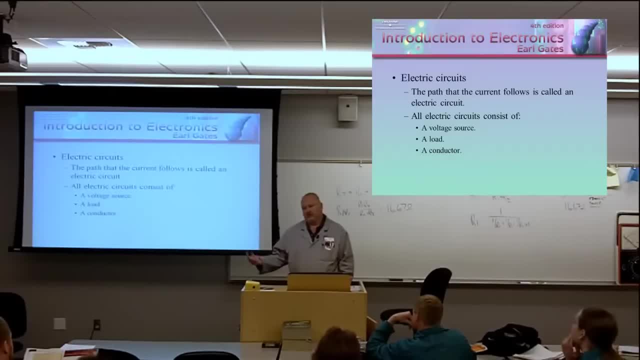 the current from the source to the load. You have to have those three parts of a circuit, Or it's not a circuit. I'm going to add two other optional parts that are not in the book. The other optional device: most circuits. 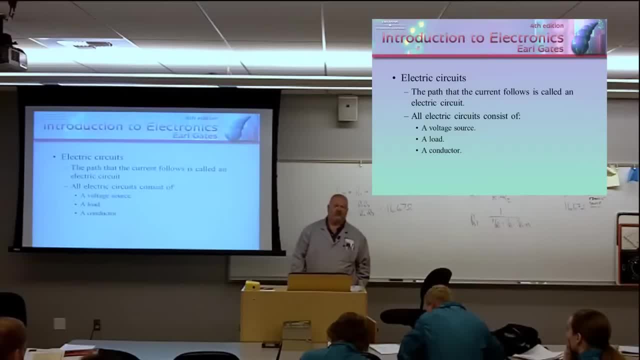 have them. not all do. is a controlling device A control device? A simple example of a controlling device is a switch. A simple example of a complex controlling device is a microprocessor With 1.9 billion transistors on it. 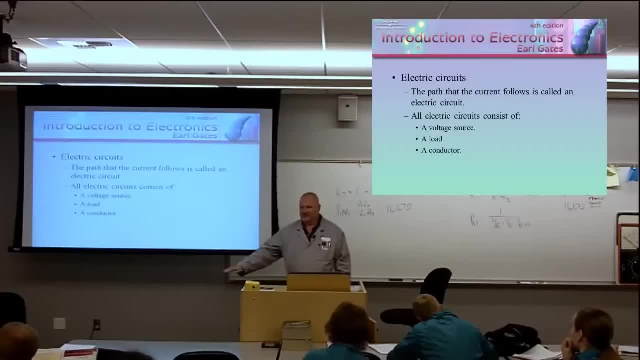 So you see, that's where we're going in this course. by the way, From one switch to 1.9 billion switches in a microprocessor, Controlling devices used to control the flow of current in the circuit, And the fifth optional device that you could have inside a circuit. 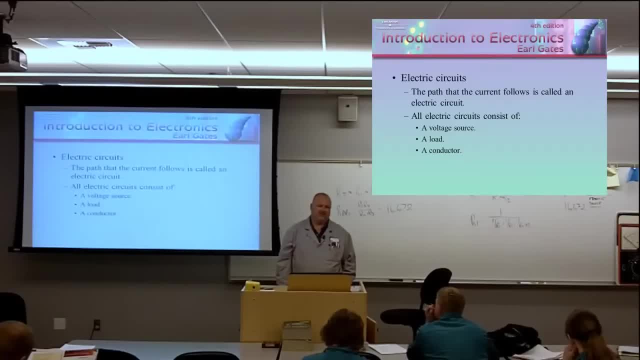 is a protective device. An easy example of this is a fuse, A circuit breaker, A fusible link, A fusible link, A thermal circuit breaker. These are all examples of protective devices. So, on my worst day of my career as an electronics professional, 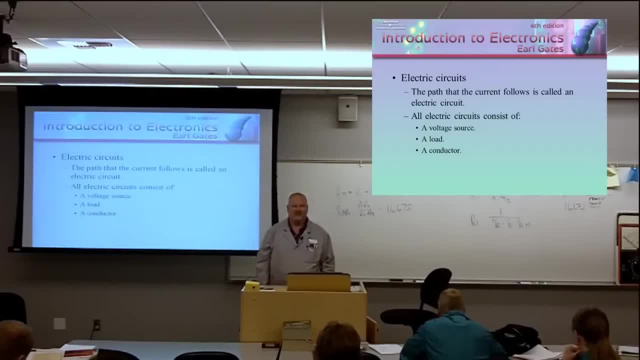 it involved a nuclear submarine someplace we weren't supposed to be, And it involved, unfortunately, my equipment that I was responsible for. There were three of us that were responsible for that system, Big system, Sixteen million dollar system, And that was like in 1982, dollars. 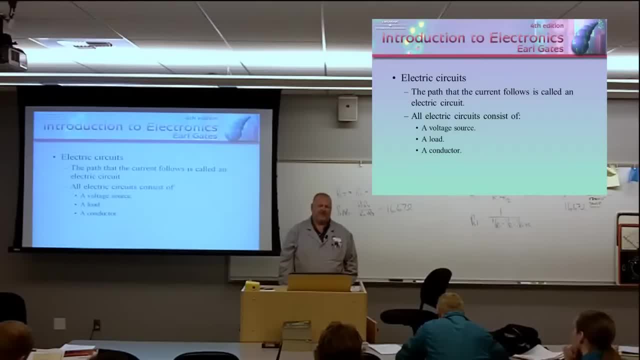 Expensive. This system was sold to the Navy and it was designed with what was called graceful degradation. That means bits and pieces could fail and the whole system would keep up and running. That's what the vendor told the Navy when the Navy bought the system. 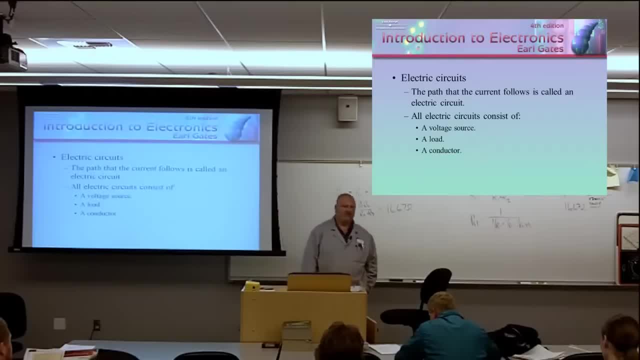 So here we are, someplace we're not supposed to be doing stuff we weren't supposed to be doing, And it was showtime for my equipment to do its thang. Didn't work right, Didn't work at all, As a matter of fact, it was. 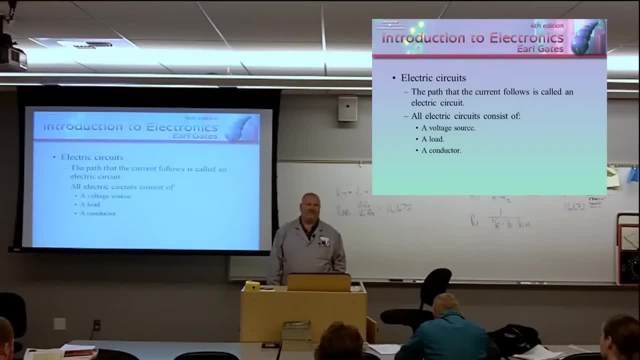 totally down 100%, And the captain like Mr Greenick. how can this be? This system was designed with graceful degradation. It should never be 100% down. Well, Skipper, it's like this, It's totally. 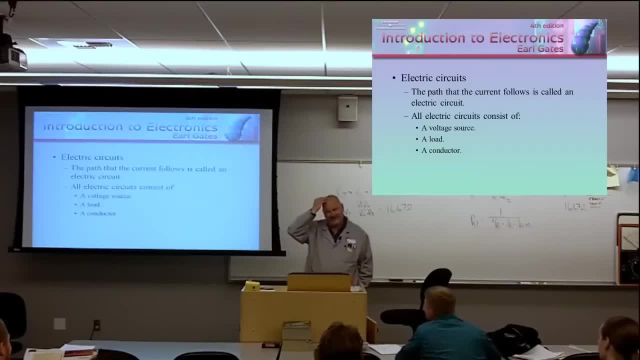 busted. I don't care what you got to do, I want you to fix it. And we literally worked on that system nonstop, three days in a row. Stayed up Popping no-dose, drinking coffee, just working on it, working on it, working on it. 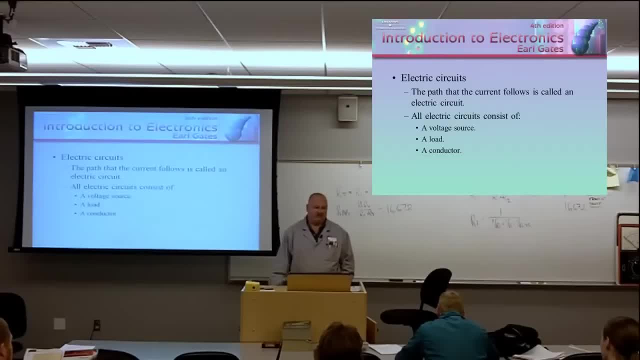 Two other guys. they finally gave up. They're like we just cannot fix this. It's not fixable, It just cannot. we can't bring it back from the dead. Me. I went back to these basics. It's an electronic system. 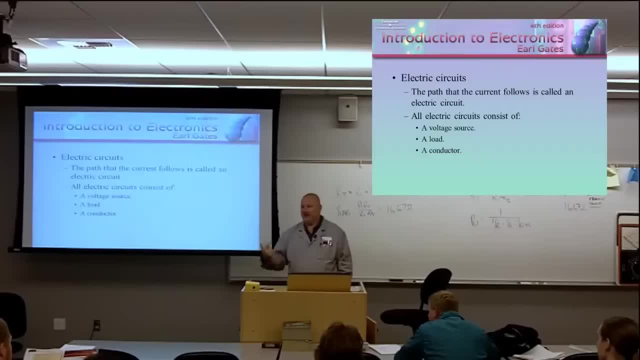 It's made up of nothing but circuits. Circuits have a voltage source, they have a load. you have interconnected with conductors, have controlling devices and have protective devices. It's something not doing what it's supposed to be doing. It's gotta be. That's what's causing the 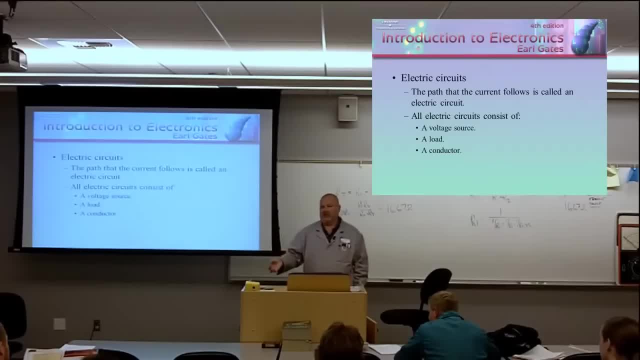 problem. It's narrowing it down, And I stuck with the problem. I ended up fixing the problem, Saved the day, Whoop-de-doo. I basically did my job and fixed the equipment. But I had to take a couple steps back and say: 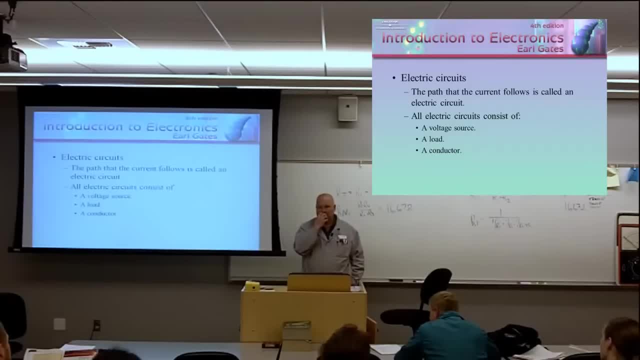 here's a 16 million dollar system. Fills half a room with equipment racks. None of it works. Can I verify the voltage sources for everything? Can I narrow it down and say this stuff's not working? but this stuff is working, Can I? 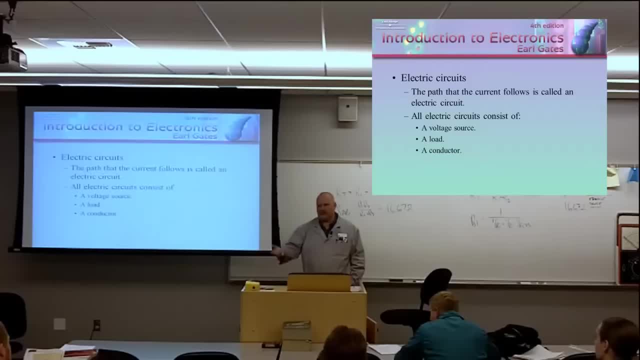 look at the loads: What's not working? What's not converting electric energy into the form of energy that we need to be getting out of it? So if you know all of these systems, then you're gonna be an effective troubleshooter. 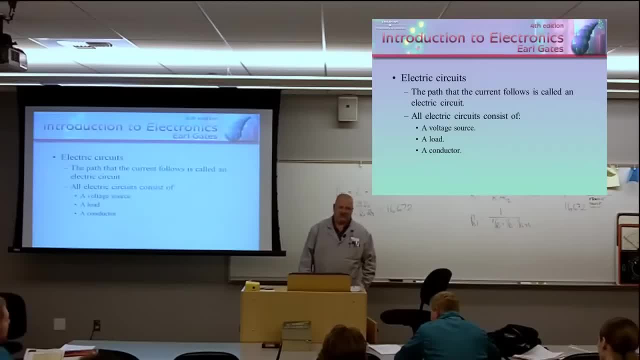 But always go back to basics. Okay, God forbid you get out of class tonight, go out to your car out in the north parking lot, turn the key and you've got an electrical problem. If you do have an electrical problem, approach. 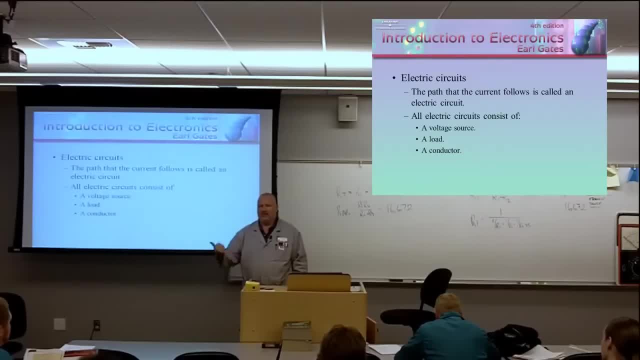 it like this: Do I have a good source? Is my load functional? Is it the interconnects? Can I prove that the interconnects are viable? Is it a controlling device? And, to be honest with you, in this day and age, most of the problems 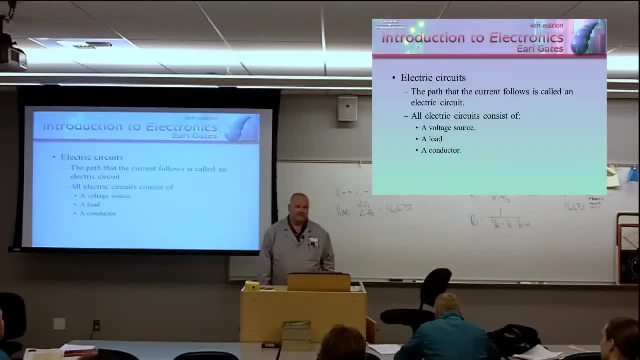 we encounter aren't controlling devices. Okay, It's not a simple switch Toggle switch. That was easy to troubleshoot. I do a lot of traveling. I forgot what brand car it was. I couldn't figure out where I got the rental car. 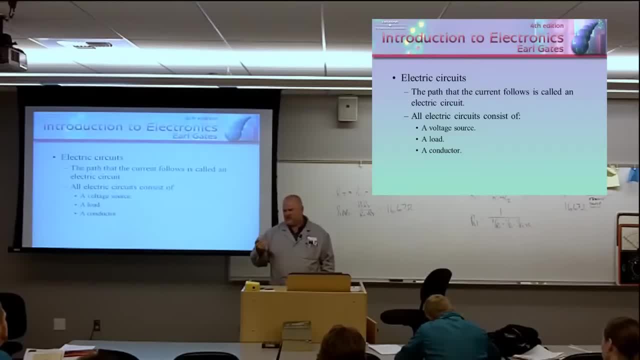 I flew in. It was the east coast and I'm there late at night and I got in and I'm like I couldn't figure out where to put the key. Where do I put the key to start the car? There was no place to put the key. 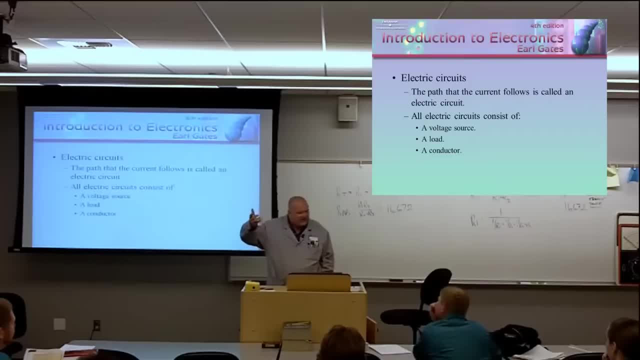 And I'm looking at it. You know, I got a little flashlight and I'm looking. There's no place to put the key. I didn't need a place to put the key. The fact that the key was on my person was good enough for the car. 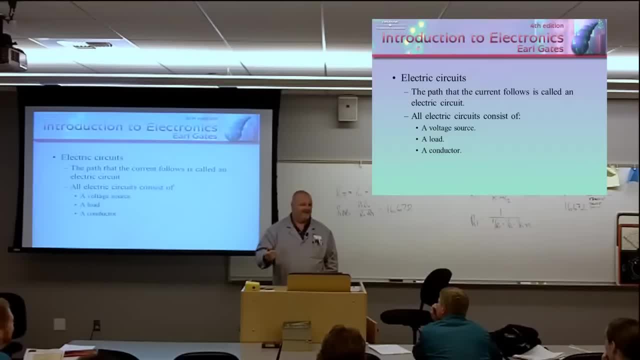 Just hit the start button. Ooh, it started Alright. So the controlling device there was the fob right RFID talking to the computer saying this is a valid operator to be inside the car to operate it. Kind of a complex controlling device. 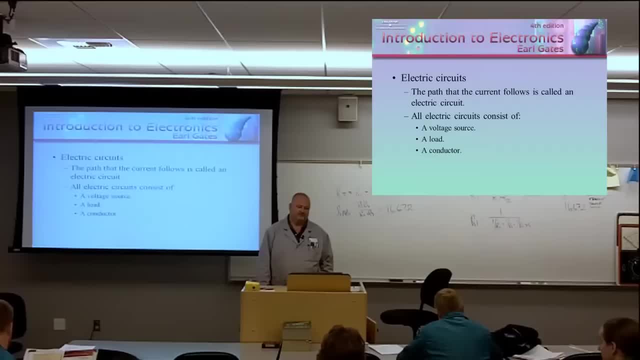 But a controlling device nonetheless. And, of course, protective devices And sometimes wacky stuff is done with protective devices. I was working on my TiVo about a month ago. I had problems with my TiVo and I've got an older TiVo. It's a direct TiVo. 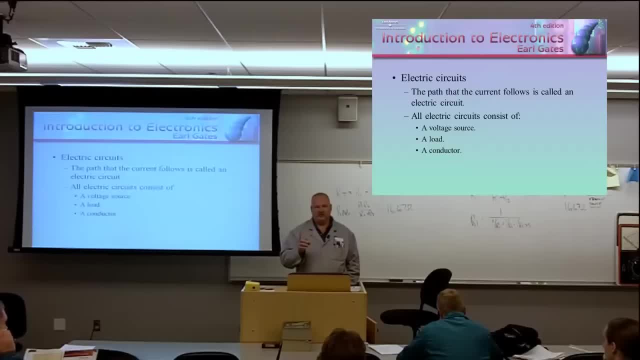 So it's got two dual receivers so I could record two shows and watch another show. It's non-HD Because I don't have HD. I don't want to pay for HD, I'm a cheapskate. Okay, Feed my nice plasma screen. 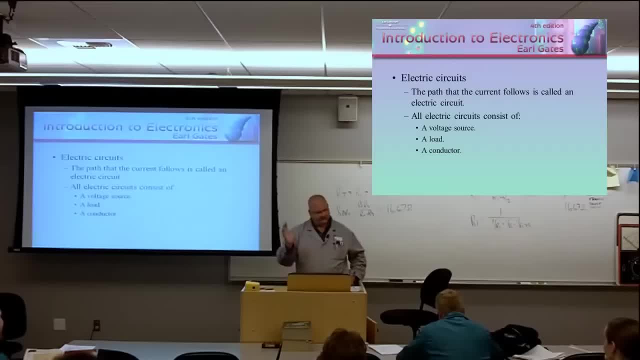 High resolution plasma screen with my basic signal. It's great, It's great, It's all good. My TiVo crapped out, So all the TiVo is it's got a hard drive in there, So I got a new hard drive. 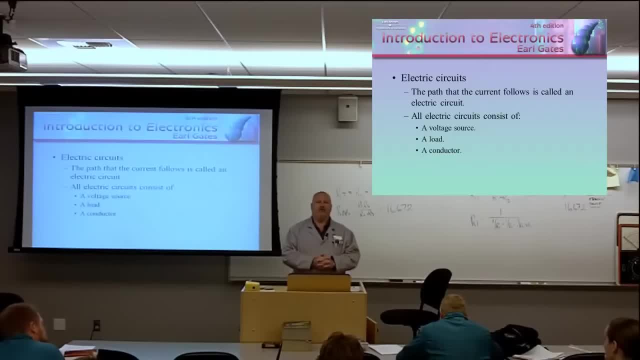 Configured that and everything, And I was just through putting it together and something happened And I heard a pop and all of a sudden TiVo wouldn't fire up anymore And I'm like, oh man, If this thing is dead, I don't want to go out. 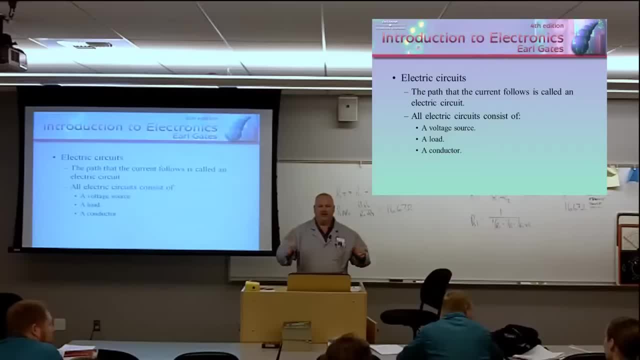 and buy a new direct TV DVR. It's a higher- I'm grandfathered into paying the older TiVo value And plus, quite frankly, I don't know if any TiVo users here. TiVo is the bomb. It truly is, Because it could do words. so 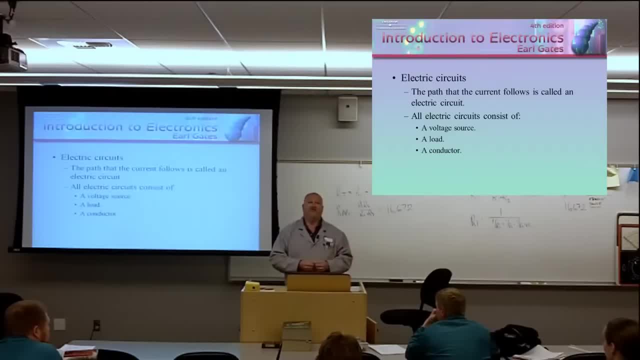 many searches and all kinds of additional stuff that a normal DVR will not necessarily do for you. So I wanted to bring this thing back from the dead And I'm like what the heck? I was pretty ticked off because I already wasted a whole weekend. 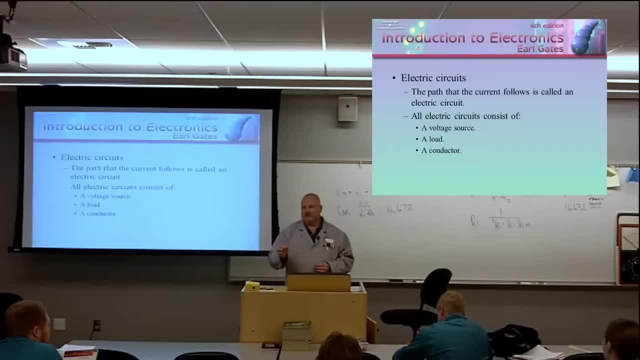 screwing with this thing. So I'm looking through the circuit for something obvious And I find this device And basically it's got shrink wrap, Black shrink wrap over it, Two leads coming out of it And I measure across it and I'm getting it. 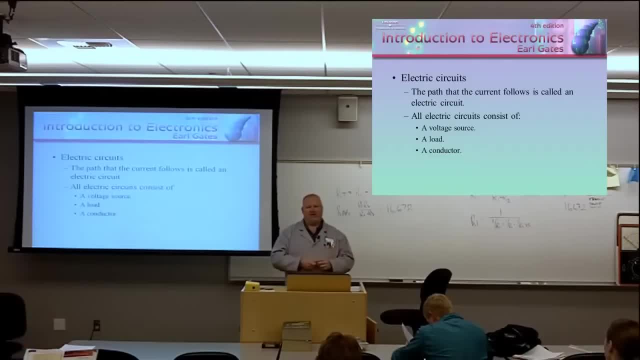 open. I mean, I just got in there with the thing unplugged and I'm poking around. What the heck is this? So, anyway, I unsolder it and I inspect it And, with an exacto knife, I cut the heat, shrink out. You know what it is? It's a fuse. 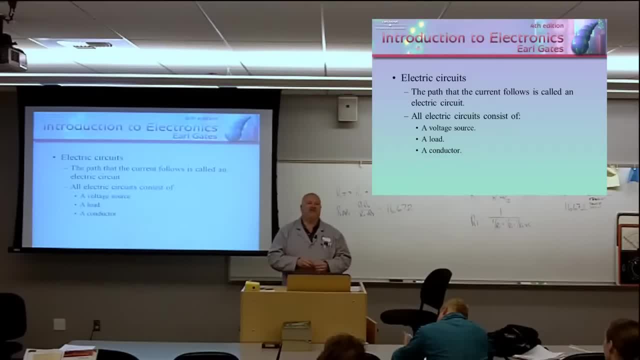 It's a fuse And the manufacturer tried disguising it by putting a piece of heat shrink around it and sticking it on the circuit board, And that's what was burned out. I found a suitable replacement that I had at home in my tin can. 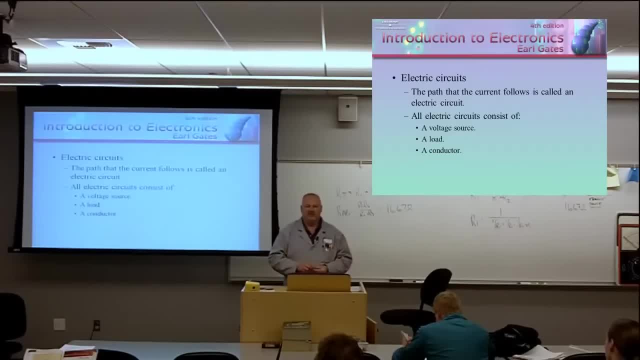 Soldered it back in place, Fired it up. I was good to go. TiVo's been working non-stop ever since, But that's a hidden. A lot of companies do that type of stuff, So that if you don't know, if you're not, 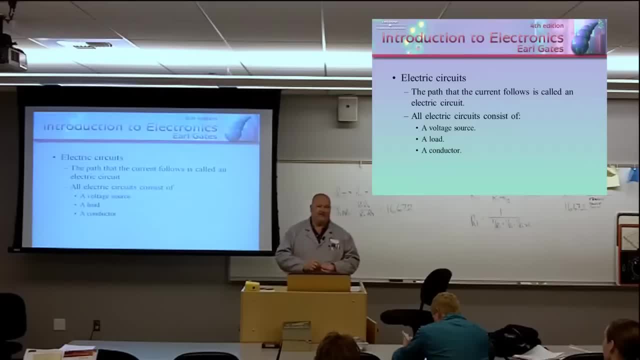 the authorized service center you don't know to get in there and even check that. I've seen some companies that will encapsulate a fuse inside silicon or epoxy. You don't even know it's in there. So keep your eye open for all these. 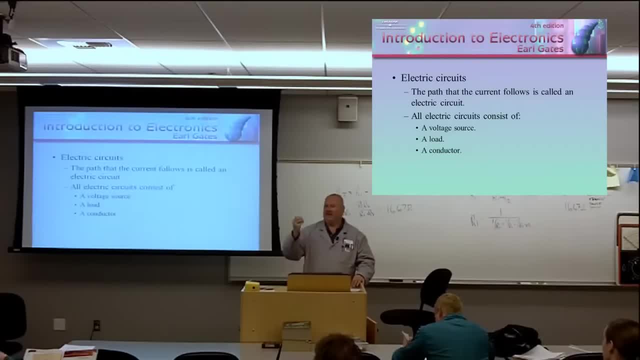 basic parts of a circuit. I know this sounds basic and I'm beating it to death, But I tell you you will deceive me in the future when you get in the lab and it's going to be. I can't fix this, The problem's too complex. 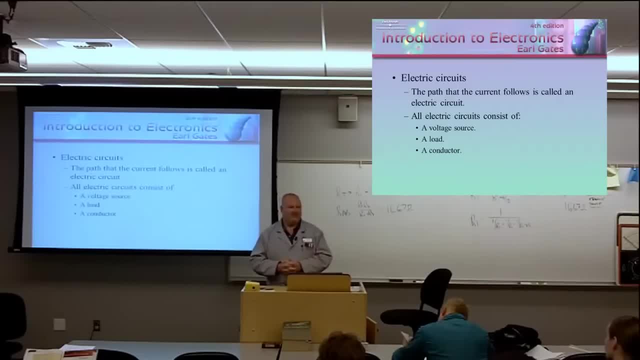 It's never a complex problem. It's usually a real simple problem. Very rarely All of you are here. You want to get into advanced electronics and work on sophisticated equipment. The problems with sophisticated equipment are always very, very simple. Okay, You gotta. 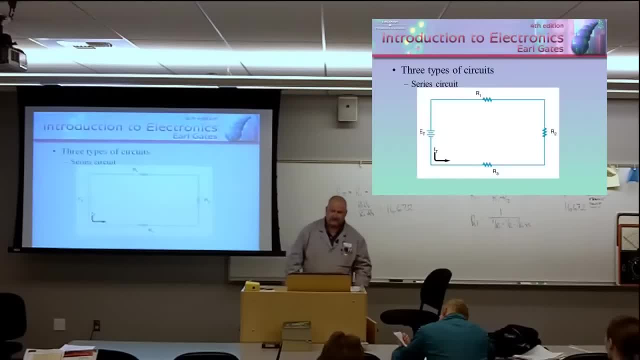 follow this protocol, though, So use this as a checklist. This is a series circuit. We talked about series circuits already. The most important thing for you to remember about a series circuit is that current is constant. in a series circuit, The most important thing to remember is that current 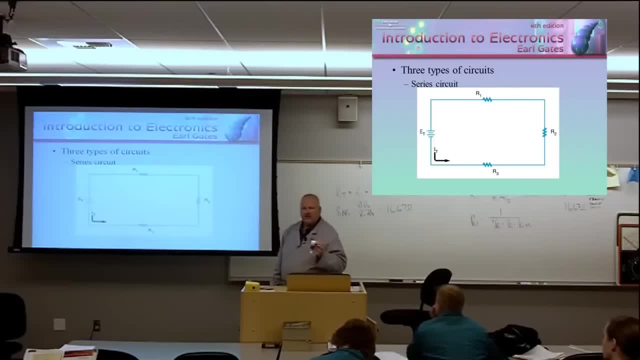 is constant in a series circuit, Meaning I've got a resistor here, a resistor here, a resistor here. These three resistors cumulatively add up to the total amount of resistance in the circuit. This electrical pressure here encounters this total resistance and allows this amount of. 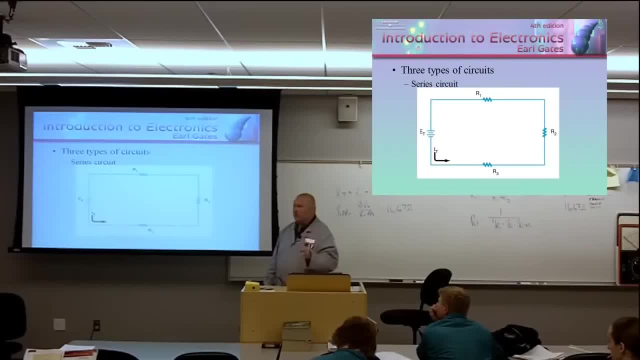 current to flow, This current has to travel the entire path of the circuit. That is the most important thing about a series circuit Period. The second thing I want you to remember about a series circuit is a series circuit is also known as like: 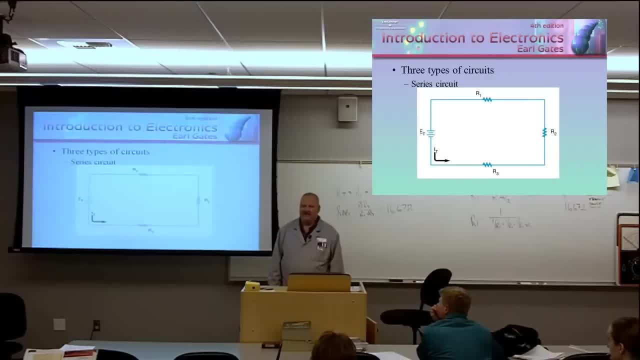 FBI lingo, AKA. AKA. A series circuit is also known as a voltage divider. A voltage divider: What voltage gets divided up? The total voltage. Remember this. We call this voltage rise. How many voltage drops do I have in this circuit? 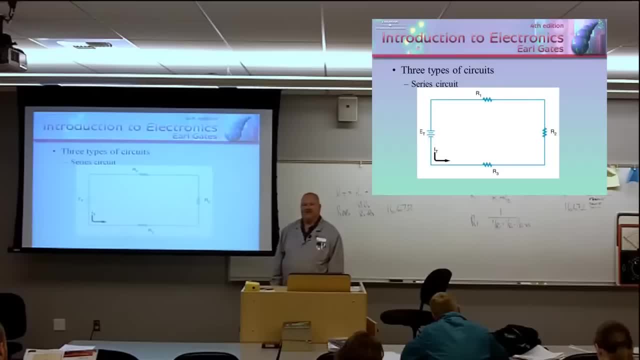 Three. So voltage rise is going to get divided into three proportional values: The biggest resistance gets the biggest voltage drop, The smallest resistance gets the smallest voltage drop. And the resistance- that's just right- gets a voltage drop. that's just right, Make sense. 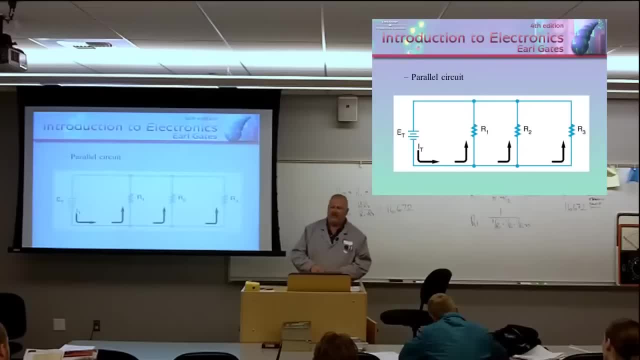 That's the series circuit, The parallel circuit. the most important thing I want you to remember about the parallel circuit is that voltage is constant across a parallel network. This is a parallel network. Here there are three resistors in parallel with each other. 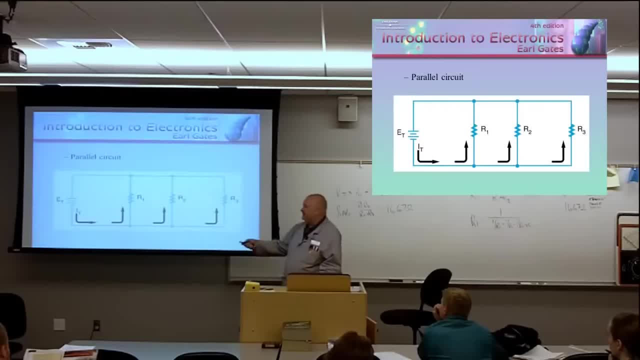 The voltage rise will be distributed equally, equally across all three branches. So, whatever this is, if this is 120 volts, this is going to have 120 volts across it. This is going to have 120 volts across it. This is going to have 120 volts across it. 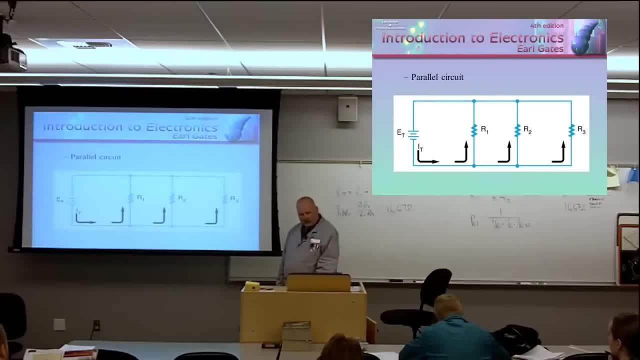 Kind of like how your house is wired. Your house is wired in parallel. Each of the outlets has the same voltage across it, or they should. If not, you've got a problem. That's the most important thing about a parallel network. 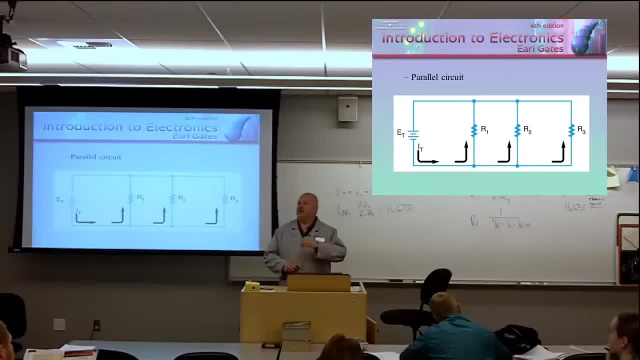 A series circuit was also known as a voltage divider. A parallel circuit is going to be known as a current divider, Because what happens to current in the circuit? This total current here gets divided here, at this node in here. Then current gets divided here. 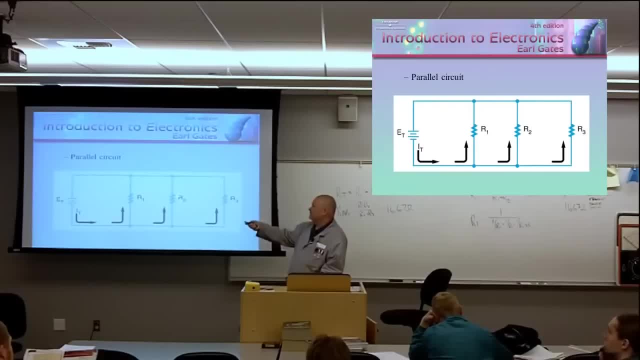 in here. The current flowing through R3 and the current flowing through R2 join up at this node and flow onto this node. This current plus this current equals total current Series circuit, current's constant Series circuit, also known as a voltage. 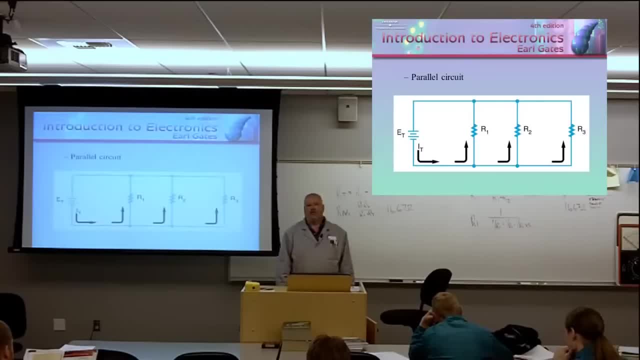 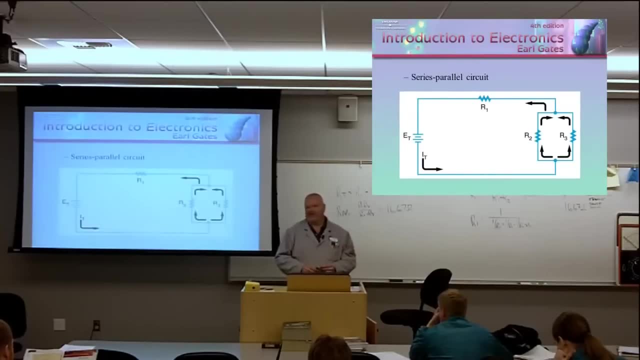 divider Parallel circuit. voltage is constant, also known as a current divider Complex circuit. well, that's got both going on. I've got current division going on here in my parallel network And I've got voltage division going on here between this resistor. 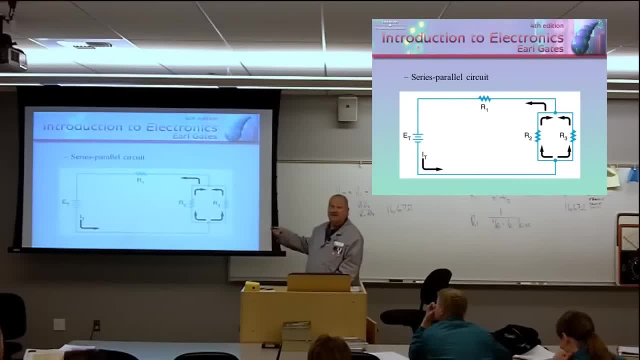 and this resistance, This resistance. The best thing you could do in this circuit is label this: A node A or in B, or X and Z or whatever you want to label it. Give it some. I like using letters, Because numbers typically. 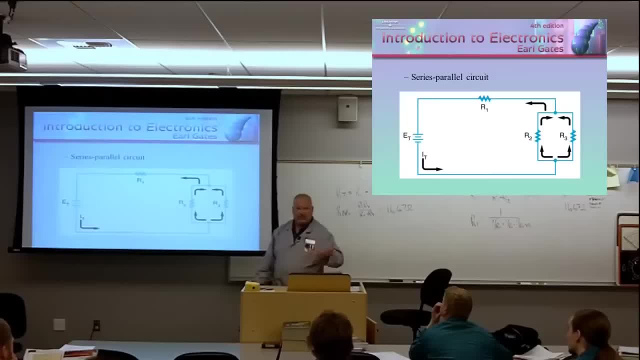 equate to components. Letters I could use to, and there's no rule on this, But it works for me, So I'm going to label this node A and this node B. The resistance between node A and B is equal to the product over sum. 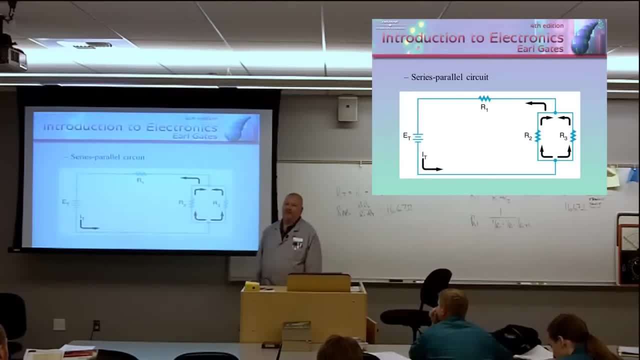 of R2 and 3. Remember that, Studied that last chapter, The total resistance of the circuit is going to be equal to R1 plus RAB. This voltage drop, RAB plus the voltage drop across R1 equals RT Voltage rise. 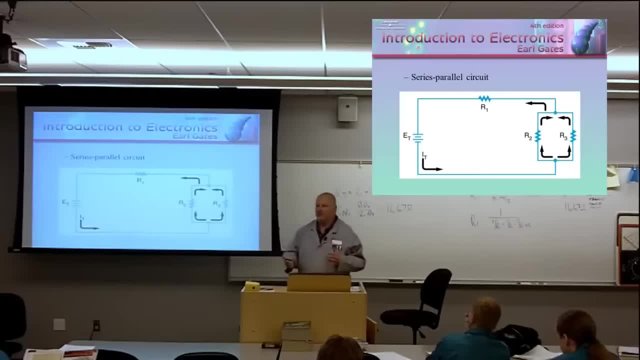 and really, how many voltage drops do I have in the circuit Really? how many voltage drops do I have in the circuit Two And what are they? R1 and R, RAB or R2 and R3.. If I say R2, 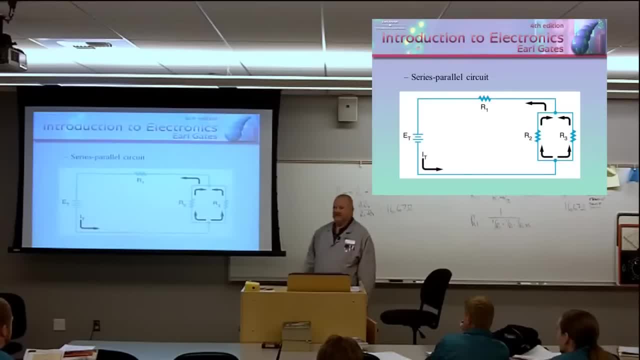 it's really the same thing. R2 is the same as R3.. You could argue and say: well, you really got three voltage drops here, You got a voltage drop here, you got a voltage drop here, and you got a voltage drop here. 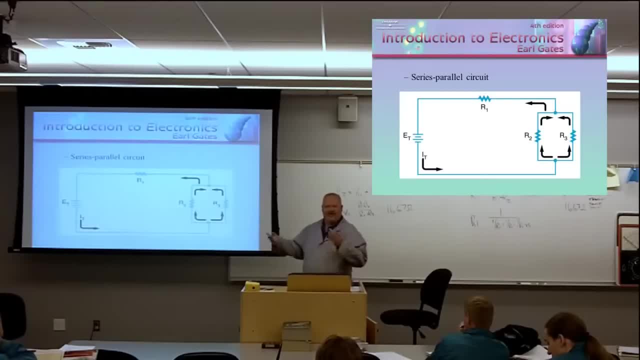 Well, this voltage drop and this voltage drop are the same voltage drop. It's the same difference in potential. So it really I don't want to call it different, It's the same. Make sense, Some different circuit conditions that I want. 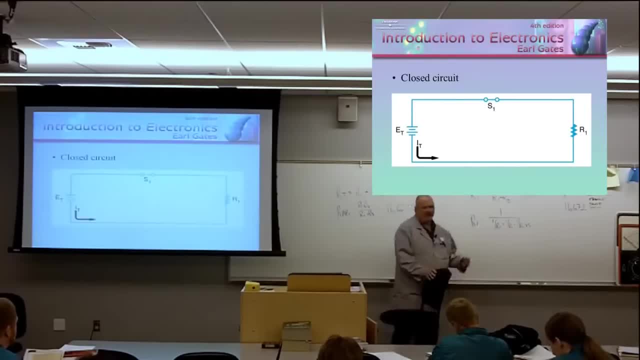 to talk about, And this is very important. I want you to use the proper terminology with me. It's part of why you're here at Lake Washington Technical College studying this stuff Is to learn to speak another language, The language of electronics. 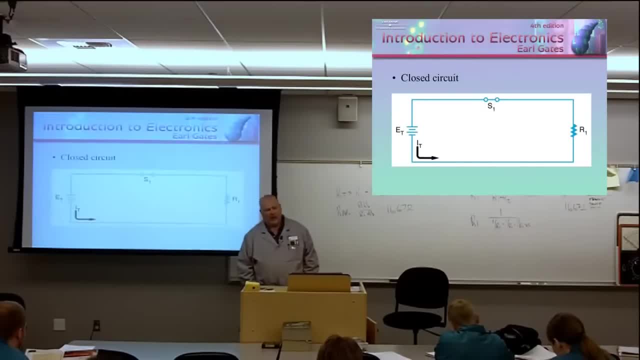 The circuit condition that I want to talk about is called a closed circuit. Is a closed circuit a good thing or is it a bad thing? Depends on what you want. Thank you, Depends on what you want Right now. the circuit in this room for the interior. 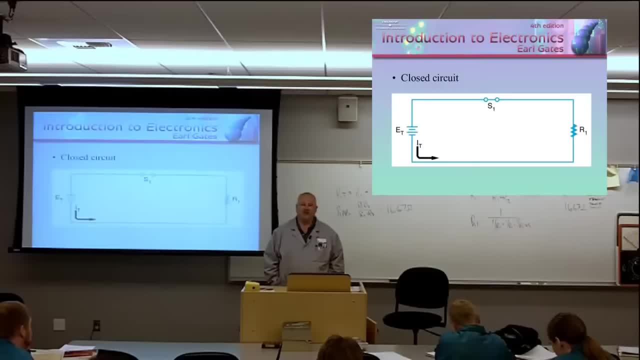 lights is closed, Meaning the circuit's energized and we have an appropriate amount of illumination in here. That's a good thing. If I go and operate the switch and try to open the switch and the lights won't go out, that could be a problem. 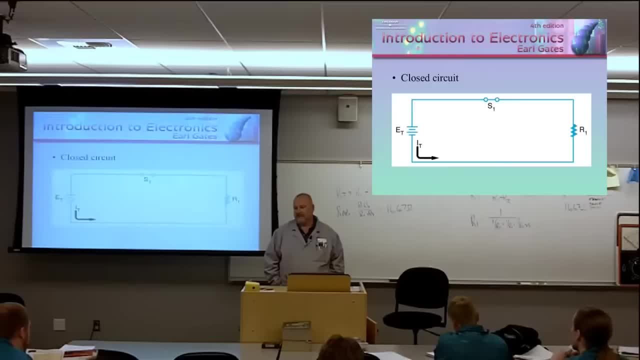 That could be a problem. If you're operating an electric tool and you try to shut it off and you can't shut it off, that's a problem. To be a closed circuit is causing you a problem. I had this problem with a pressure washer. 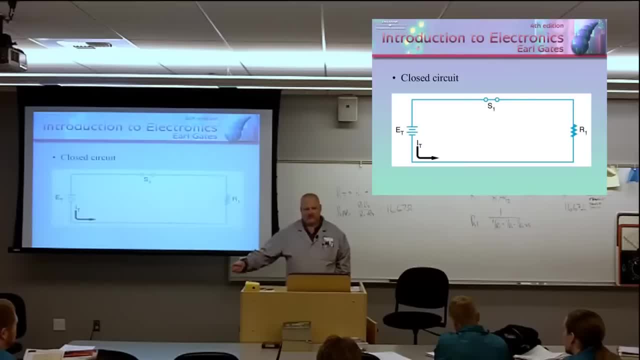 One of these hundred dollar pressure washers- Costco special Great pressure washer. Okay, for what I do, Got a patio, I got a deck, I don't need a. you know, 40 horsepower, fire breathing. you know, peel the paint off. 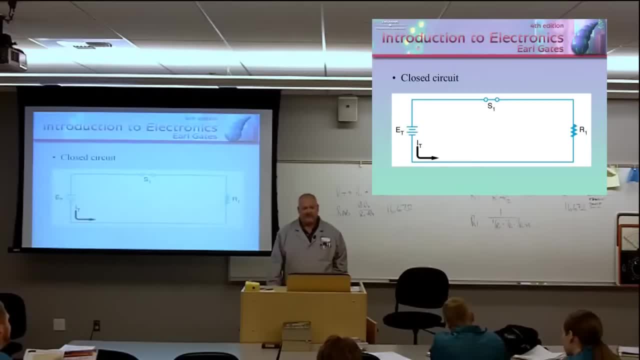 the Queen Mary pressure washer, But it's my pressure washer and I like it. I got a lot of tools. Got a lot of neighbors that know I got a lot of tools- My neighbor Tom. he's since moved. It's another story. 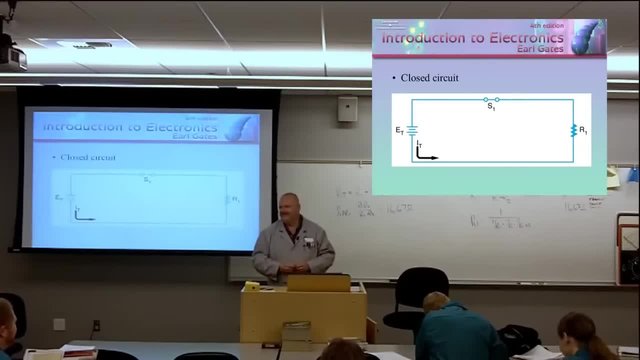 I'll tell you about that some other time. Finally drove him out of the neighborhood. Tom's an engineer, An electrical engineer with Boeing. Hey Joe, I'm going to stain my deck. Can I borrow your pressure washer? I'm a nice guy but I hate loaning. 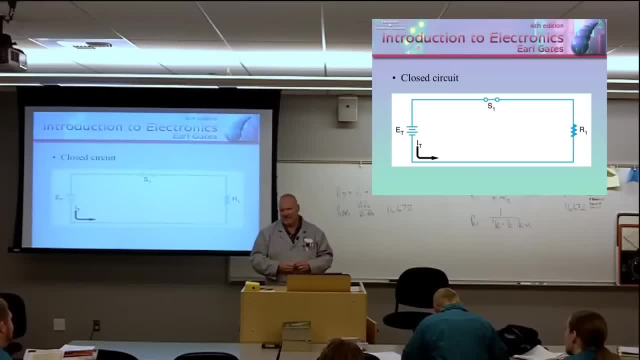 out tools because nobody takes care of stuff like I want it taken care of. I mean, if I borrow somebody's tool, I take care of it ten times better than my own, And if I break it, I buy it, I replace it. 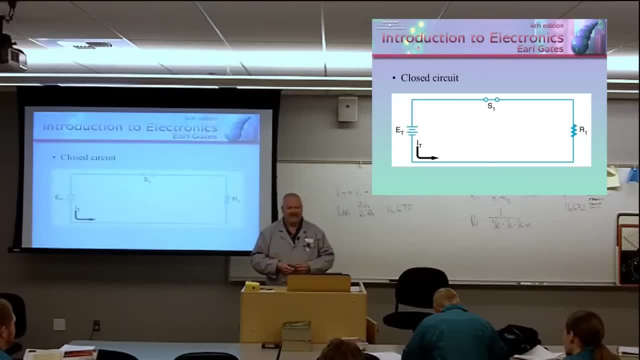 I said, Tom, that's fine, I'll loan you my pressure washer, But but only plug it in a dedicated outlet And do not use any extension cords, Because it's right on the label. It's not that I'm that smart a guy. 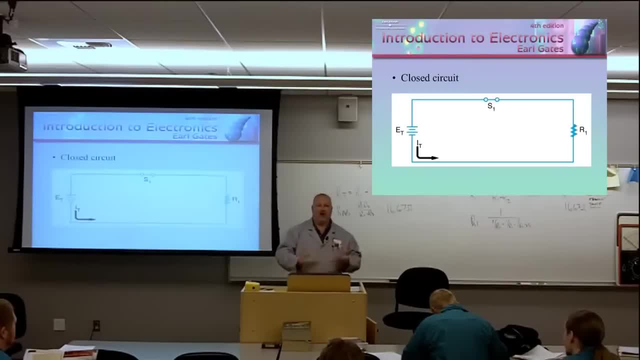 I just read the label, the tag that's on it. Because this motor requires a lot of current to be able to turn and be effective, You plug it in an extension cord. it doesn't get the right amount of current. Remember that whole thing. the cord gets hot. 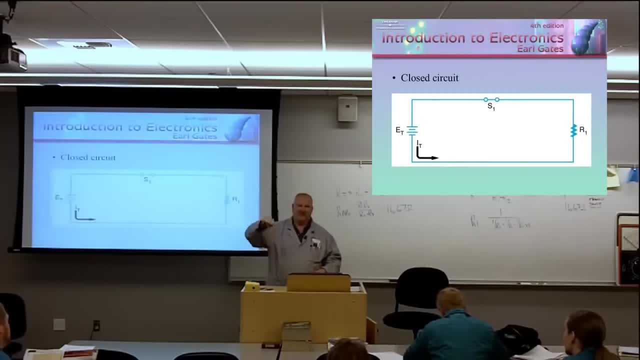 The hotter it gets, the more resistance, The more resistance, less current, The less current, the hotter it gets. It's a vicious cycle. So I loaned him my pressure washer. How did it work out? Oh, pretty good. Thanks, Joe. 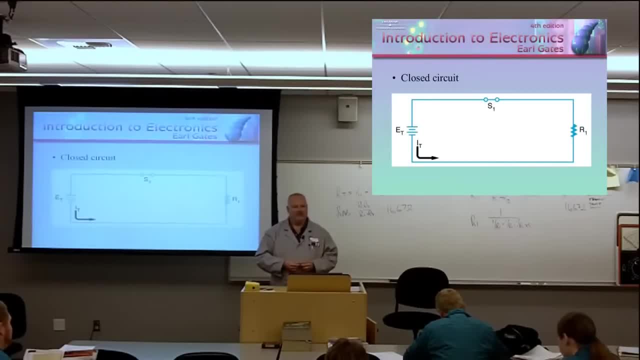 Fast forward. a couple weeks later, I go out to wash my sidewalk, I plug the thing in, turn it on and it's on, Continuously on. It won't shut off. Normally what happens? it's a real simple circuit. 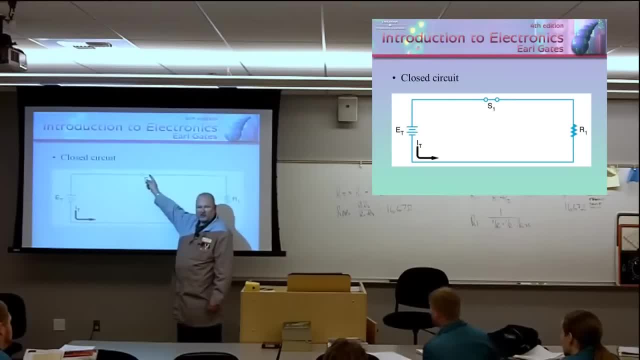 This switch right here on a pressure washer, one of those cheap Costco specials. what it does is there's a water pressure sensor. When the water pressure builds up, what it physically does is open the switch. So what you do in the handle when you release the switch, you release the pressure. As soon as you release the pressure, you close the switch, you turn your motor on. the motor turns the pump on and you're pressure washing. You release the trigger, you build the pressure up, you open. 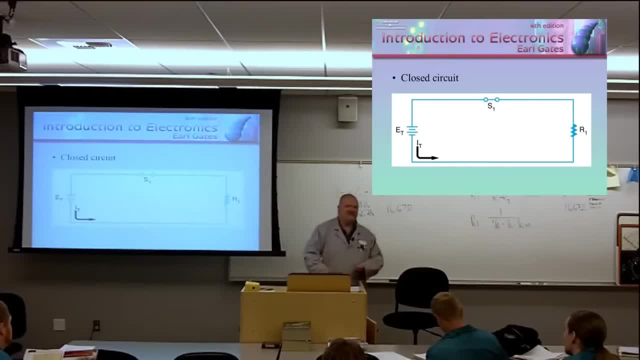 the switch. Mine will never shut off Unless I unplug it. If I unplugged it and it still kept operating, well that'd be something Keeps operating. I'd rip the thing apart. and what had happened was, I guarantee you, I didn't see. 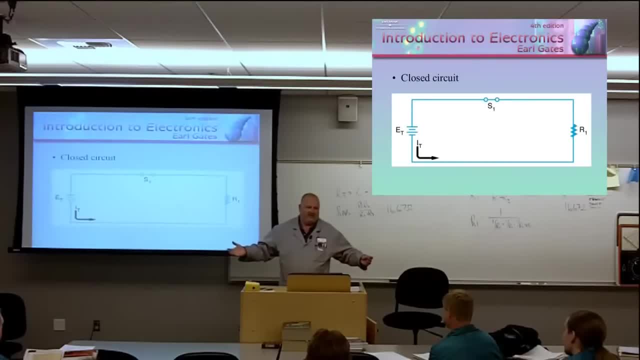 him do it because I had no problem with it and I had it for years. He plugged it in a non-dedicated circuit. it built up a lot of heat and physically, the switch, the contacts got welded. I took the switch apart, the contacts. 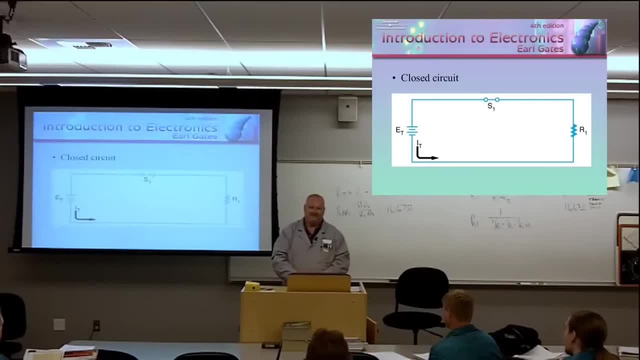 were welded to each other. That's how hot it got. So I went to my file cabinet, opened the drawer, pulled out the manual, got the parts list, contacted the company. The new switch would be $65. Plus shipping. A new pressure washer. at Costco: $109.. I could have it right now. The old one's in a landfill somewhere After I cannibalized some parts off of it. Nah, I ran him out of the neighborhood. I finally ran him out of the neighborhood. 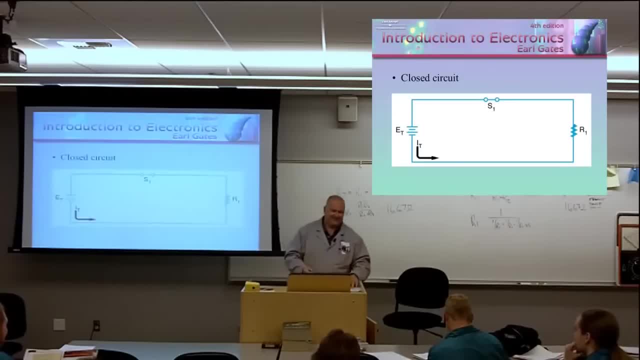 There was a chainsaw involved, Trees falling, Long story. Now. actually, what pushed Tom over the edge was he had problems in his basement flooding split-level house and water would get in. So what he did is he dug a trench around the. 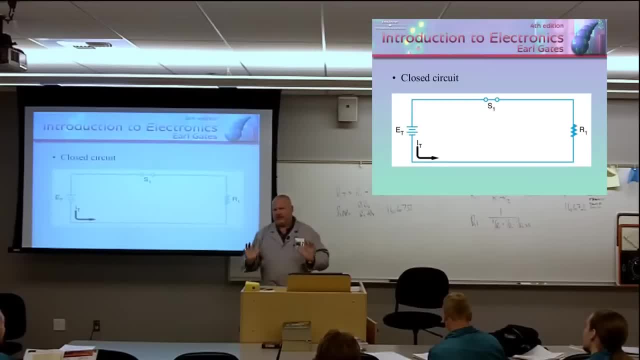 entire foundation of his house and then what he's going to do. he's going to put a treatment on the outside concrete and then he was also going to backfill it, put in drainage and everything. So he had this ditch dug. 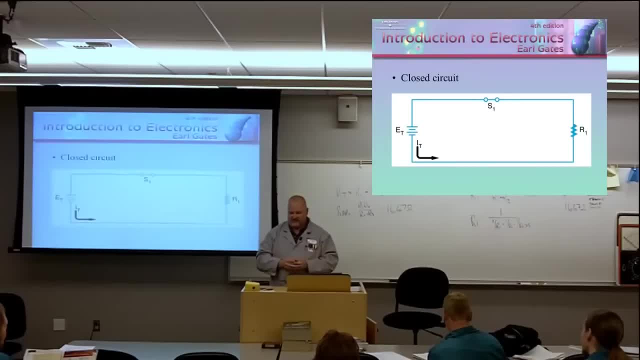 It was a lot of backbreaking work. He did it all by hand. Gotta respect that. But it took him forever to do it. It took him years to do it, So I used to accuse him of having a moat. It's like Tom, what's the deal with the moat? 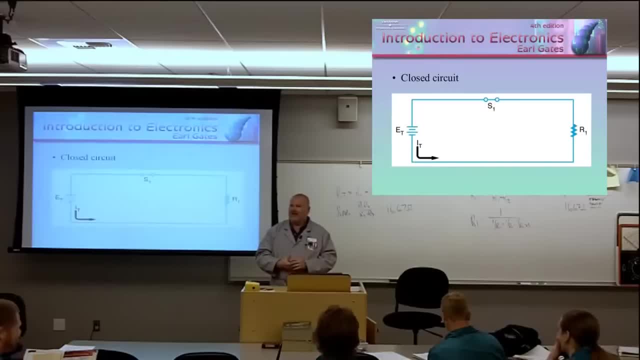 You know. So anyway, again I had a buddy of mine over and it was the wee hours of the morning and we were enjoying some libations And some cigars, And actually my buddy who's got my sense of humor. he's like: 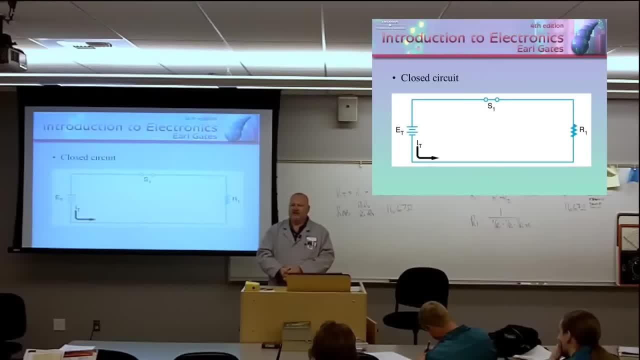 hey Joe, you know, is that Tom's moat? You know what's up with that. Doesn't he want that thing full? I'm like that's a good point. Why have a moat if it's not full? 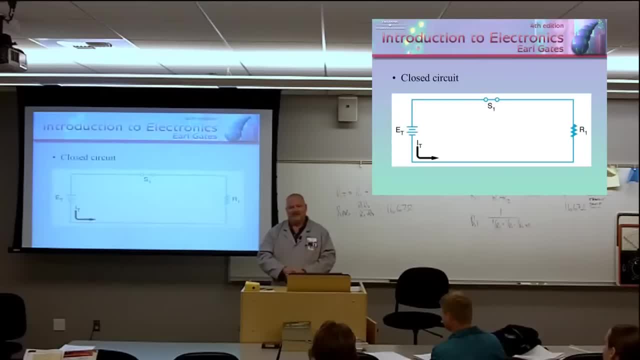 So, anyway, we turned on his garden hose and started filling the moat, and then we're just laughing and like busting a gut. and then Tom came out and he's pretty freaking ticked off that we're filling his moat with water. 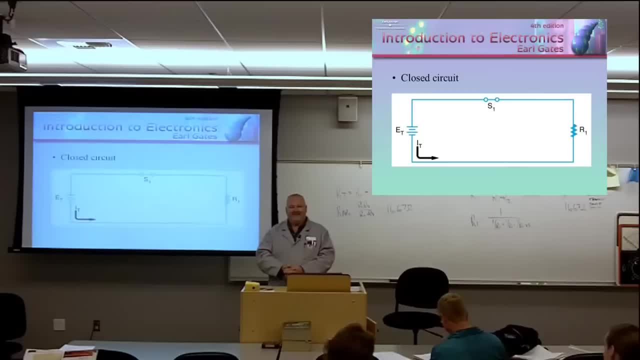 I mean, he woke up to the sound of running water. There's water running in my house and hey man, we thought we were doing you a favor by filling your moat. you know, He was out of there within six months. 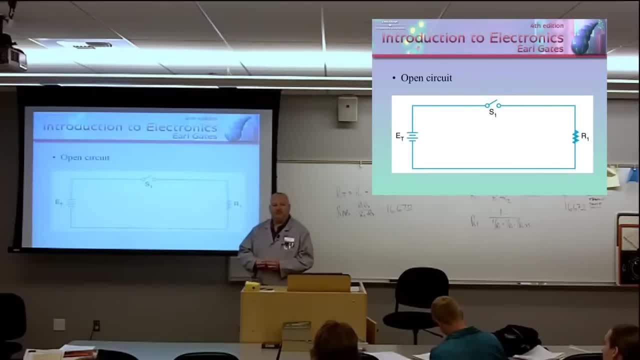 Open circuit. is this good or bad? Depends. Depends On my pressure washer. this would have been highly desirable. When pressure builds up, it opens the switch interrupts the flow of current to the motor right. Another circuit condition is called a short. 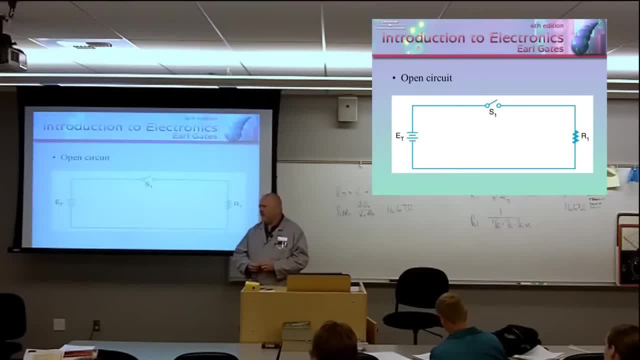 circuit. Have you all heard of a short circuit before? God bless my wife, but she's been my wife now for a long time and I've been in this industry since puberty, so you know hanging out with a guy that teaches electronics. 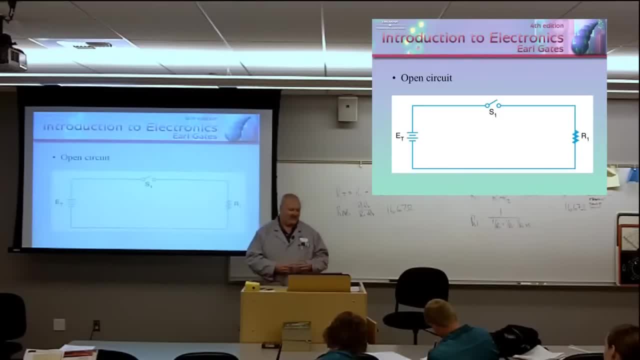 and does electrical stuff, you'd think something would rub off. Constantly I get a call and it's kind of like the blender's not working, I think it's got a short circuit And I'm like, holy crap, you tell short circuit to me. 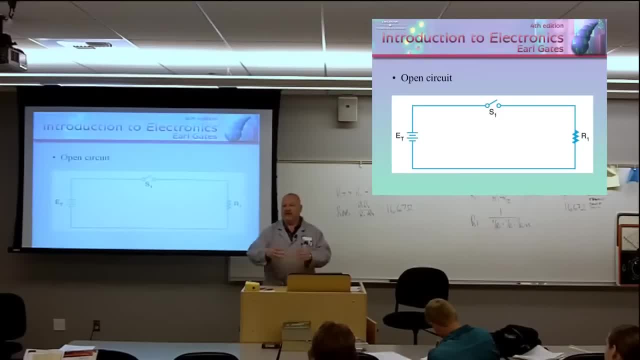 I'm like ready to call the fire department. I mean, short circuit is like what you see in Star Trek when they get hit by a phaser. you know, I mean that's a short circuit. That, literally, is what a short circuit is. 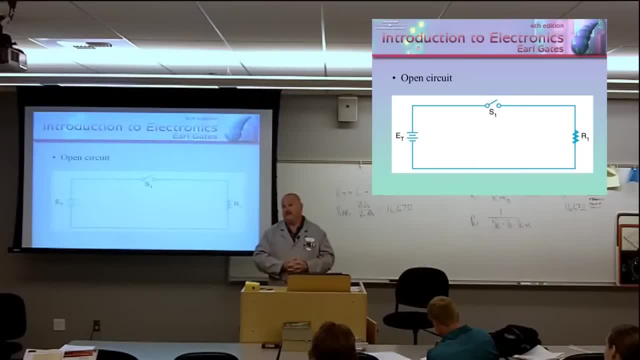 A short circuit will cause an electrical fire. And then, on further probing, what exactly is the blender doing? Well, I plug it in, I hit the button, but nothing happens. Oh, you mean it's an open circuit, not a short circuit, Big difference. 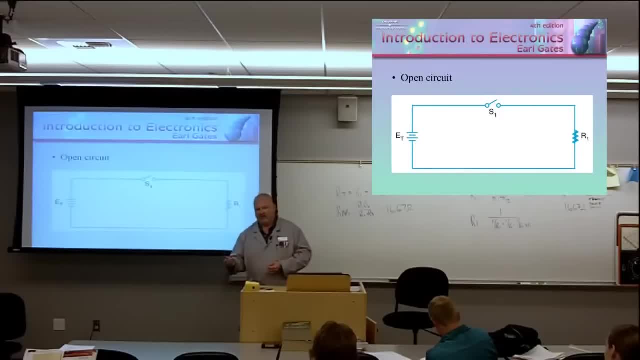 The majority of household appliances that I've encountered that have failed have failed because of an open circuit condition. That's where nothing works. Now you've got to be careful because sometimes a short circuit will cause a protective device to open and render. 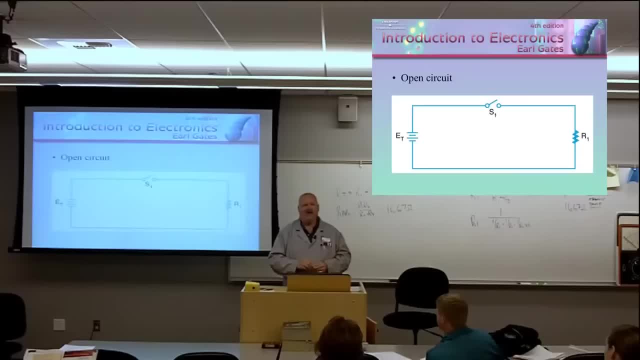 the piece of equipment dead. So you've got to get in and like that: DirecTV, DirecTVo. that was dead. That was open intentionally. I found the open. It was that fuse with heat shrink around it. 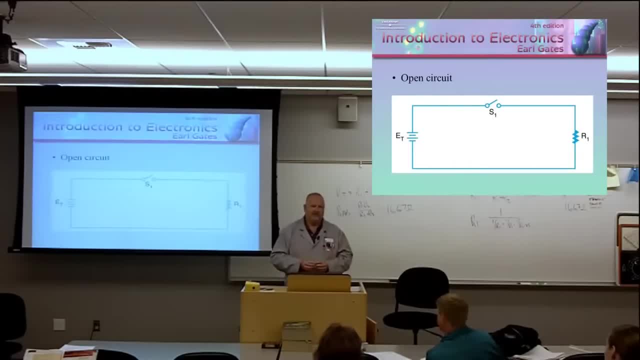 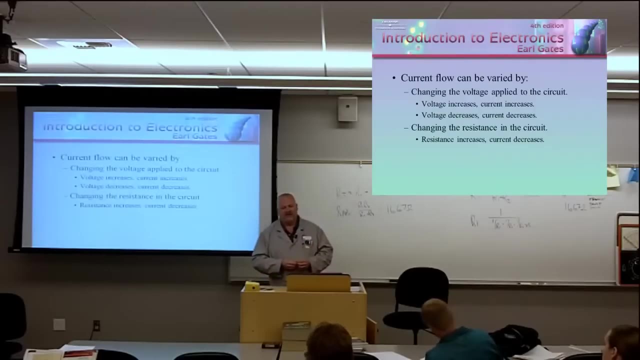 trying to disguise it to make it look like a fuse with heat shrink around it Make sense. So keep that in mind. Open circuit, short circuit is always bad. There's never an intentional reason to short anything. Current flow in a circuit can be varied by changing the voltage. 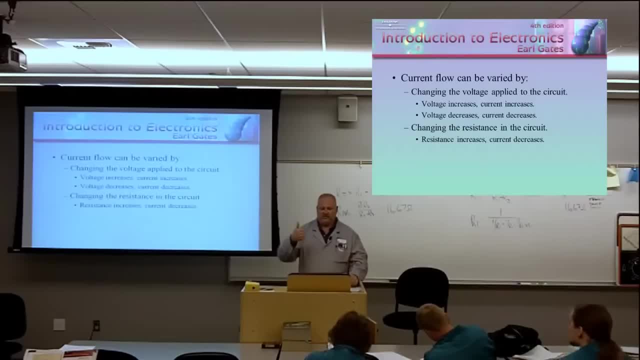 applied to the circuit As voltage increases- current increases. As voltage decreases, current decreases. And also changing the resistance in the circuit. As resistance increases, current's going to decrease. So these first values, we call these directly proportional Right If voltage increases. 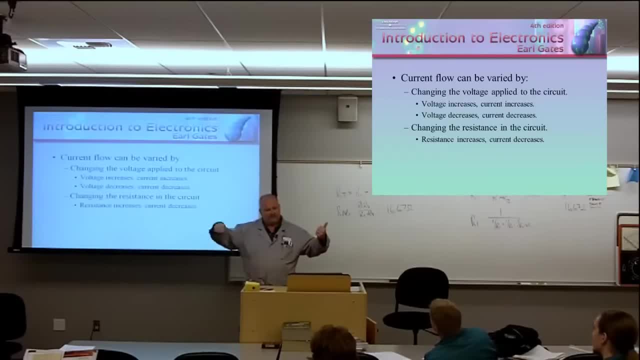 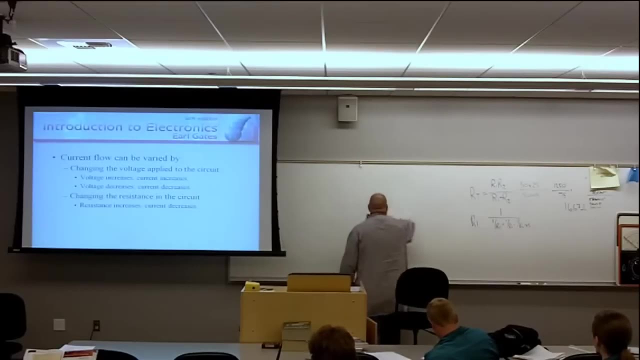 current increases directly proportional. Voltage decreases: current decreases directly proportional. Resistance resistance increases: current decreases Inversely proportional. Now, in the beginning, when Ohm gave his like sermon- I don't know if it was a sermon- 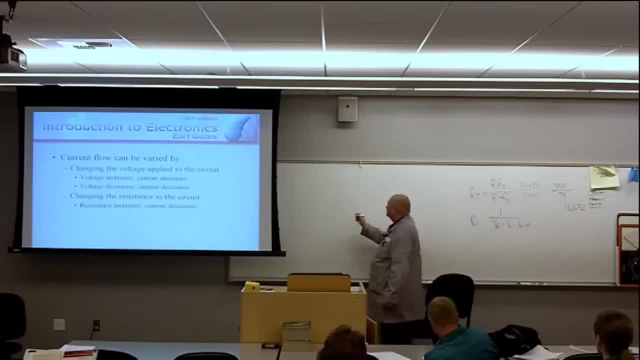 Ohm's Sermon on the Mount. Somehow, I think I'm getting my history messed up. This is what Ohm said. I think the speech was given down at the Kingdome And he got. he was at the Kingdome. 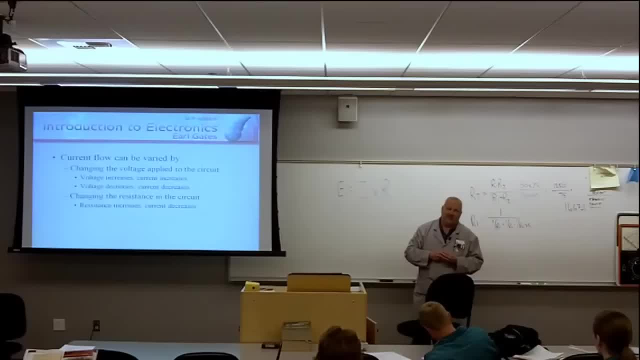 and he got up: hello, hello, hello. This is, this is. I'm the happiest man, man, man alive, Alive, alive, Because, because, because I know, know, know, Ohm's law, law, law, law. 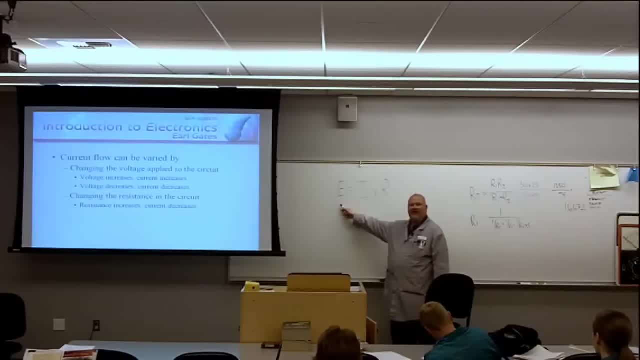 Y'all ready, ready for this, this, this, this, this E, E, E is equal to I, I, I times, times, times, R R, R. And the crowd went nuts: 45,000 people on their feet. 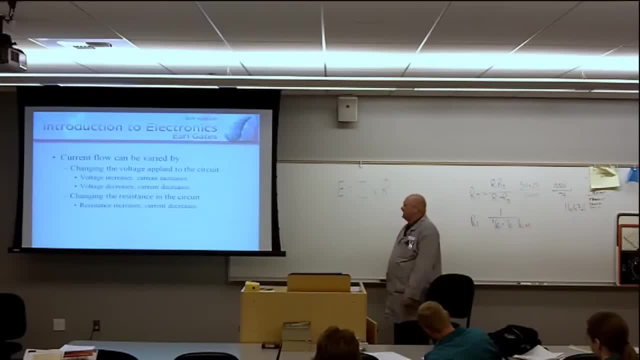 Ohm's law As spoke. Actually, I think I'm getting my history mixed up a little. I don't think it went down like that, quite like that. So this is Ohm's law. This is what Ohm really said. 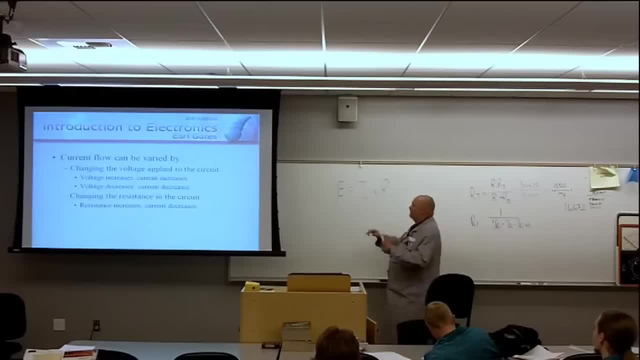 Voltage is equal to current times resistance in a circuit And, of course, instead of the letter E, we could use the letter V. V is equal to I times R. Now remember that trick that I showed you with the triangle T in the center. 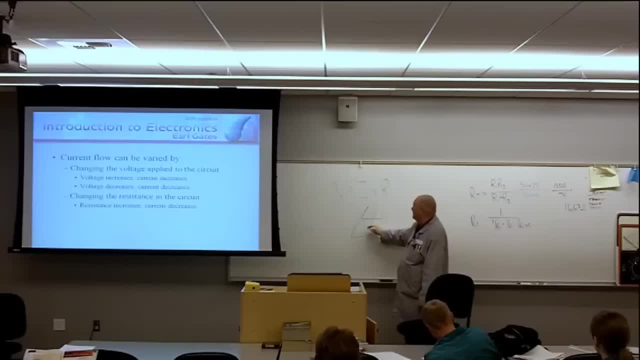 Let's put this in that V I, R. So now you've got all the other variables. If I ask you, how much resistance is in there? in a circuit you cover R up it's voltage divided by current. If I ask you, 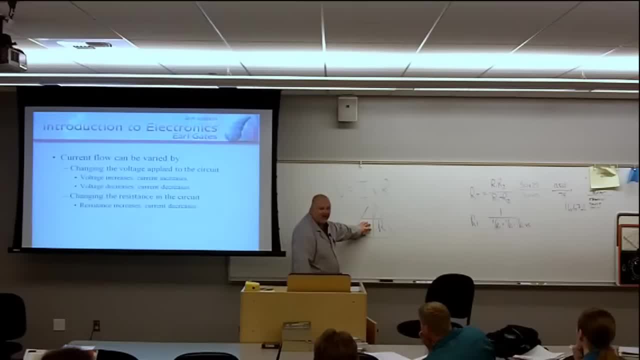 how much current is there in a circuit? you cover up the I and you say it's V over R. If I ask you how much voltage is there in a circuit, it's I times R. So by knowing that one formula you can figure out all the other. 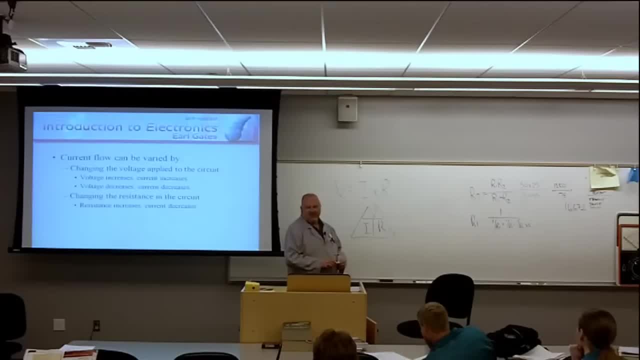 algebraic manipulations of it. Does that make sense? So in essence, that is Ohm's law In all of its variables Or variations, I should say Algebraic variations. So you don't even need to be a math whiz to be able to do it. 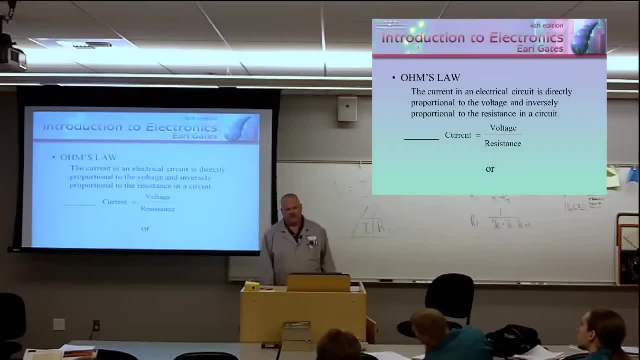 Ohm's law states: relationship between current voltage and resistance. or I is equal to E over R, Or E is equal to I times R, or R is equal to E over I. however you want to look at it, But, but, but, in, in, in the beginning. 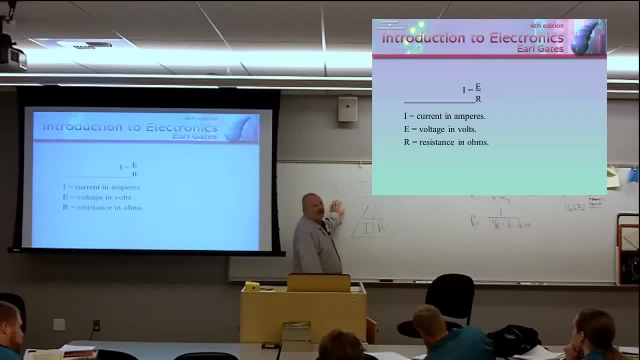 beginning. beginning, it was V, V, V or actually E, E. E is equal to I, I. I times R. 45,000 people on their feet applauding The man with the beret. I don't know if he wore a beret or not. 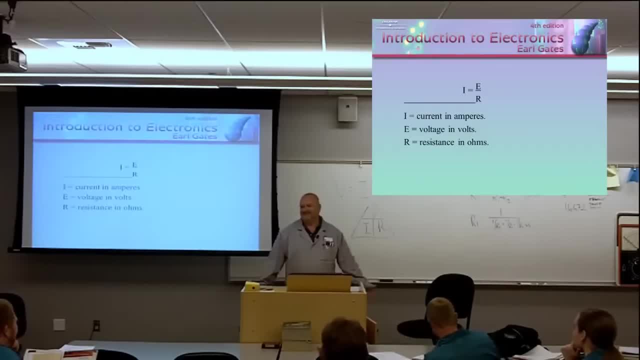 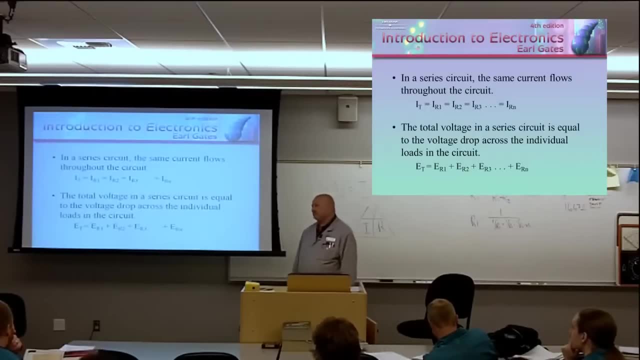 If I was, Ohm, I'd wear a beret, Some of the algebraic formulas, if you will, And when I say that, I know I there's some people in here that cringe like I gotta know all this math or whatever. All this is is a. 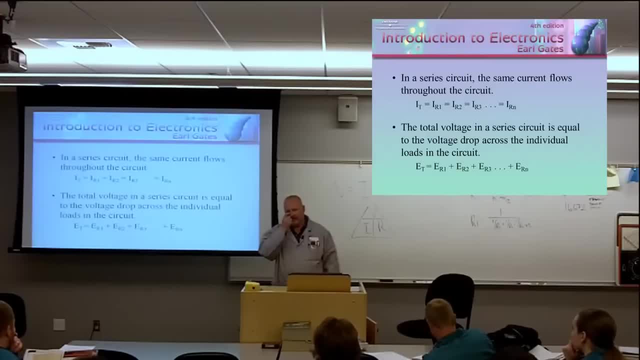 recipe. That's all this is. By laying it out like this, it shows you how it needs to be laid out. to explain the behavior In a series circuit, the same current flows throughout the circuit. Total current is equal to the current through resistor 1,. 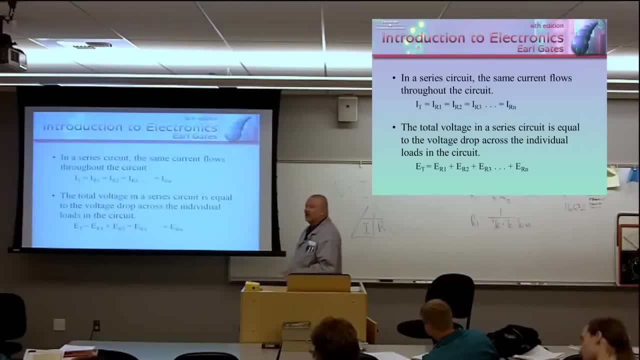 plus the current through resistor 2, plus the current through resistor 3, etc. etc, etc. It's a fancy way of saying current is constant. in a series circuit, Total voltage is equal to voltage drop across 1, across 2, across 3, etc. etc. 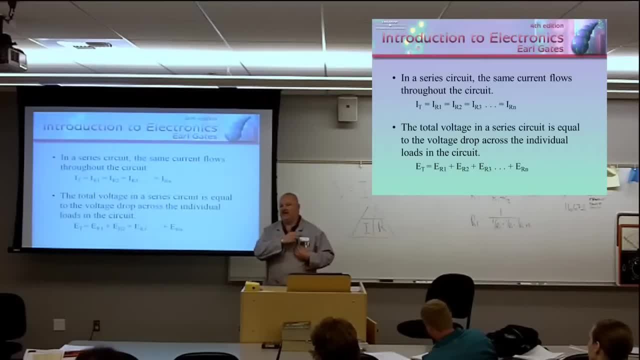 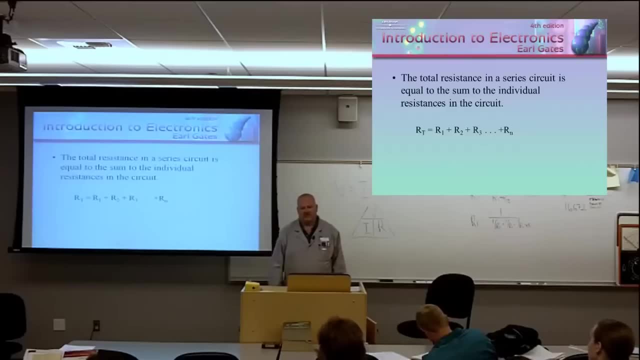 This is a fancy way of saying. a series circuit is also known as a voltage divider. Total resistance in a circuit is the sum of the individual resistances in a circuit. This is a fancy way of saying. you gotta add it all up. Resistance is additive. 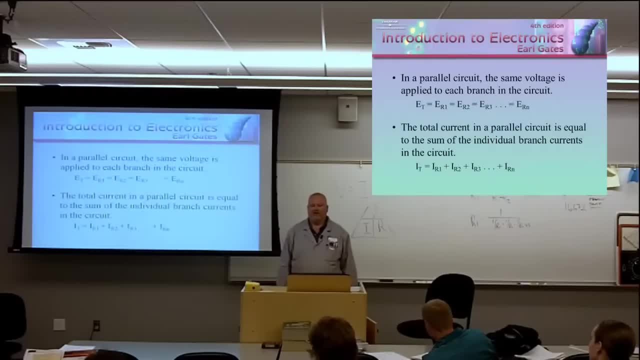 in a series circuit. In a parallel circuit, total voltage is constant across the parallel network. That's this formula Down below: total current is equal to IR1 plus IR2.. This says that a parallel circuit is also known as a current divider. 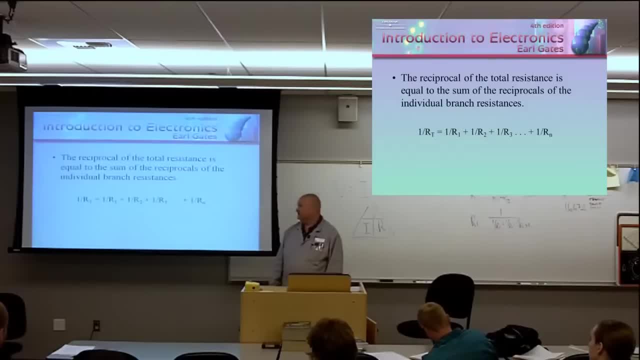 Oops, There it is. There's another formula: The sum of the reciprocal of the resistances equals the reciprocal of the sum of the reciprocals equals the total resistance in the circuit. Because when we add resistors in parallel, what are we doing? We're actually. 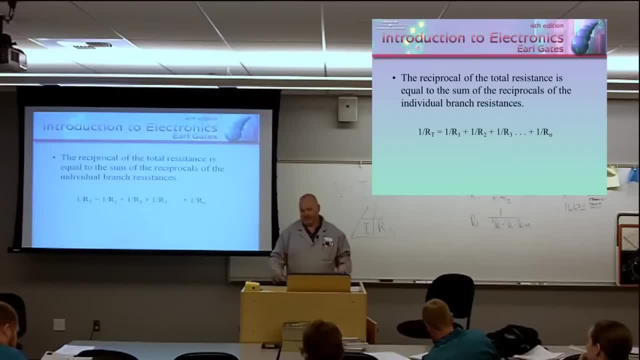 adding up the conductivity of the individual branches To determine unknown quantities in a circuit. you can kind of use this as a checklist Draw a schematic of a circuit. You gotta start off with a schematic of a circuit If one has not been provided to you. 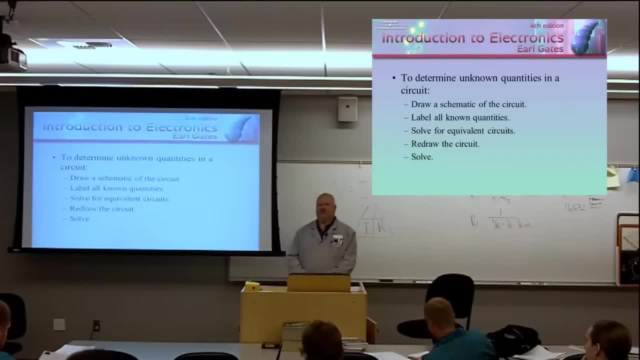 you need to draw one. It's just troubleshooting circuits off the top of your head. Doesn't really work. well, Gotta be looking at the big picture. Pun intended Label: all known quantities. Sometimes you may need to get these known quantities from manufactured data sheets. Solve for equivalent circuits. Solve for equivalent circuits. Redraw the circuit. When I say redraw the circuit, remember like when we were dealing with a parallel network, Two resistors in parallel with each other. You could redraw that circuit and just show one. 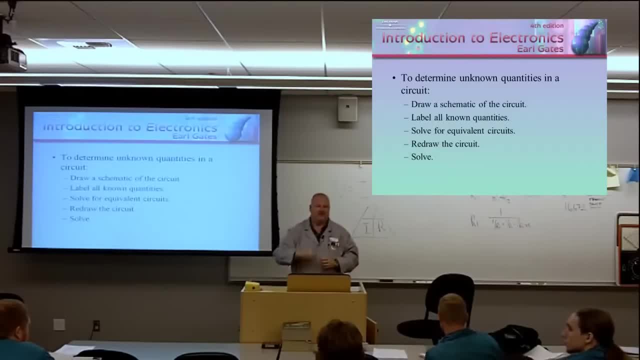 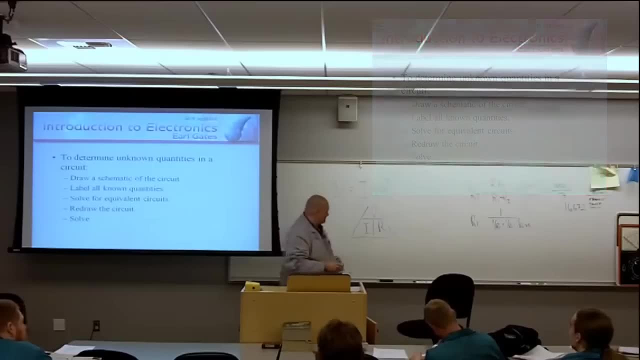 resistance. Two resistors equals one resistance. I could do a simplified. You want me to do a simplified drawing of my car electrical system. right now, Wanna see this Battery Car And, to be honest with you, I'm not being silly. 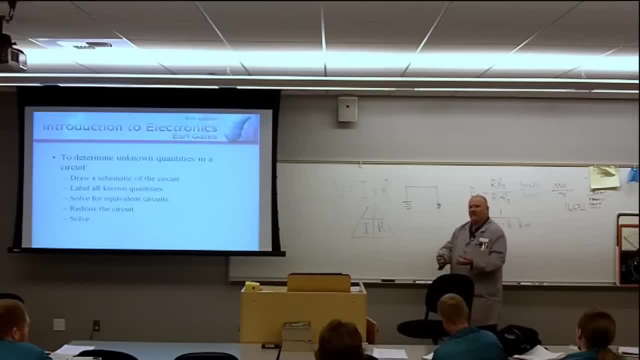 I could redraw every circuit in my car and come up with an equivalency, and this is what it is. And I'll tell you what: if you go out to your car and you turn the key and there's nothing, And you open the door and the dome light doesn't come on. 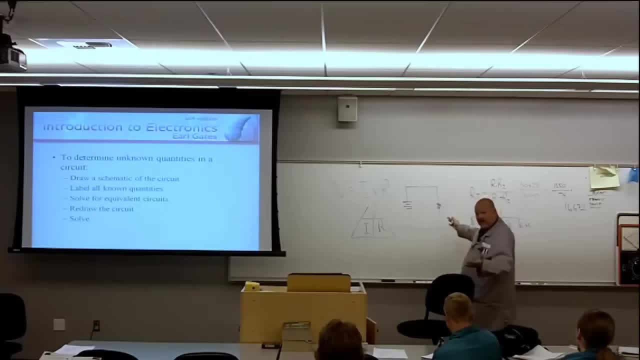 Nothing works in the car and all of a sudden, this is exactly what you've got and there's an open in this circuit, And it's a pretty big open, Or your battery's dead. I don't think your whole load is dead. It's like, oh my goodness, all my load is dead. 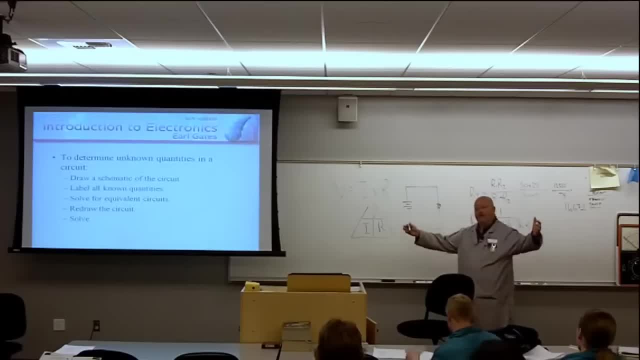 I gotta replace the load, Save the battery. You know what I'm saying. Doesn't work like that. But do you see the power of troubleshooting like that? What's working? My car's dead. What do you mean? it's dead. It's a conversation with my 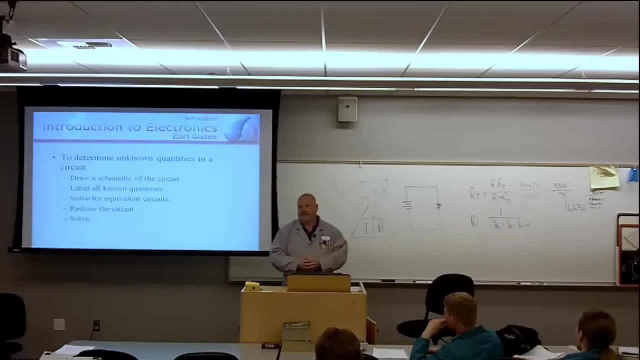 wife, The car's dead. What do you mean? it's dead. It's dead. When you turn the key, does it click? No. When you open the door, does the dome light come on? No, Oh, it's dead. But you gotta ask those questions. 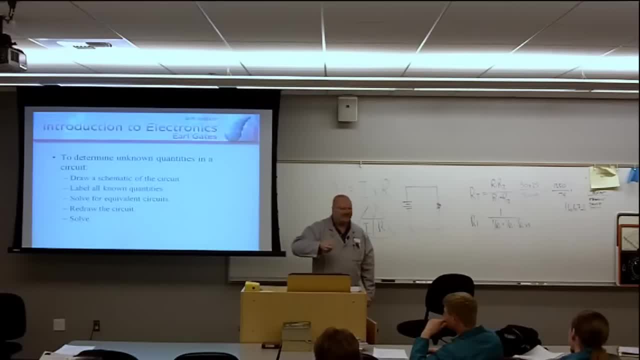 because it's different. When you open the door, the dome light comes in, But you turn the key does anything? do you hear a click or anything? Immediately you're troubleshooting, You're narrowing it down to what circuits perhaps could be faulty. So redraw. 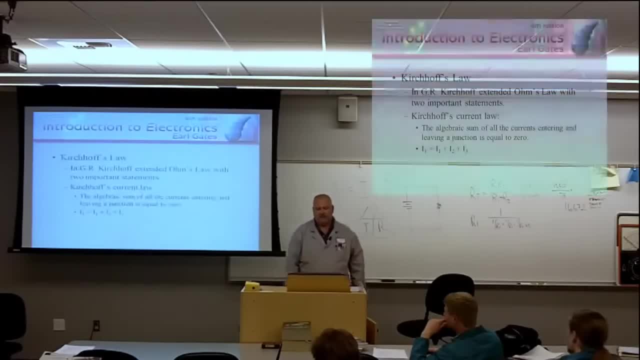 to simplify, There's another big law out there. It's Kirchhoff's law. GR Kirchhoff extended Ohm's law with two important statements. Kirchhoff's current law, The algebraic sum of all currents entering and leaving a junction, is: 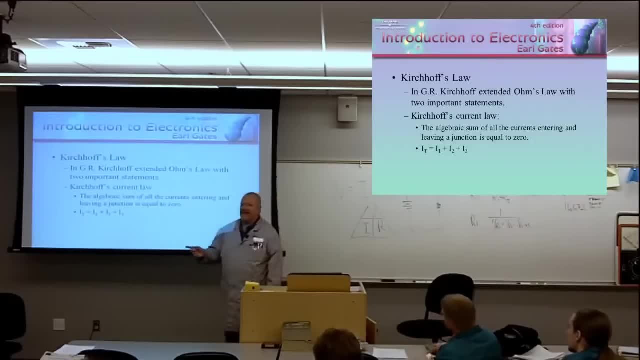 zero Equal to zero. Kirchhoff's law is kind of like this: Everybody know the intersection down here at the bottom of the hill. Okay, Let's say that you're a traffic cop And you're directing traffic down there in the center of the intersection. 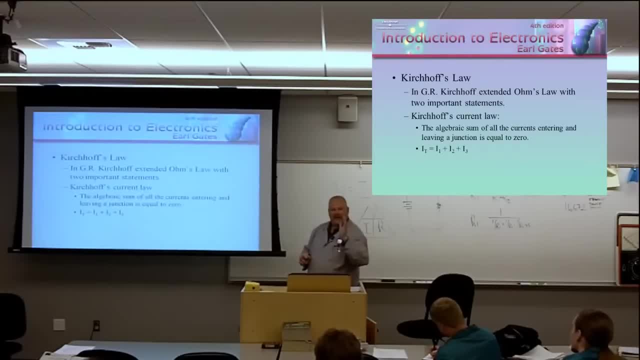 Okay, And you got three cars coming at you this way And you got five cars coming at you this way. In a few moments, how many cars are gonna be going away from you? Eight, Because three are coming from one way. Five are coming the other way. 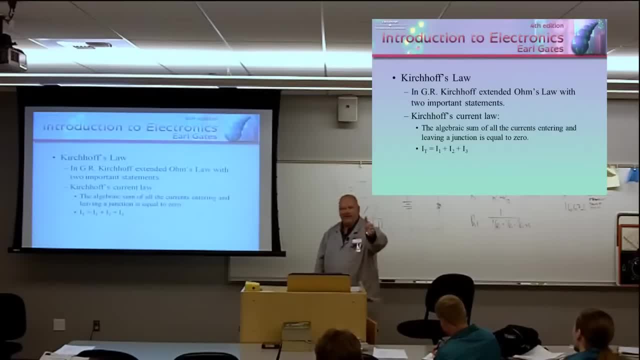 You know, chances are, cars don't come, and then, oh, we're just kidding, We're gonna back up. I've seen them do that down here. But generally speaking, you know, three plus five equals eight. Pretty profound, isn't it? 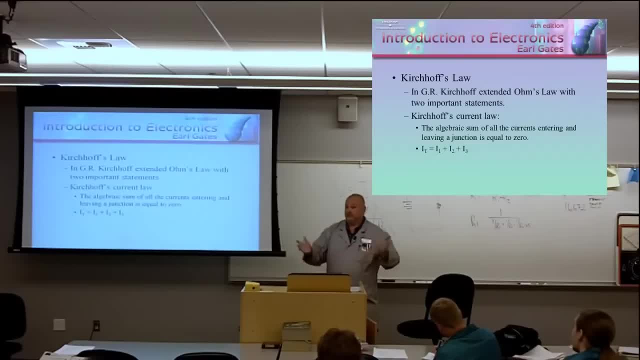 That's what Kirchhoff came up with, And he made the textbooks. You laugh, His name's in the textbook, My name's not. That's Kirchhoff's current law, And what Kirchhoff is saying is again, the total current. 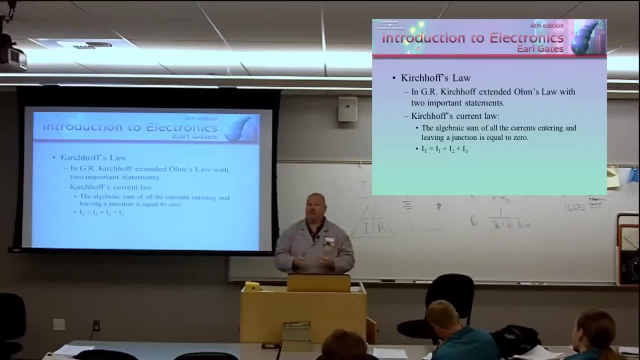 entering has to exit, And it's really a profound troubleshooting tool, Because what you could do, what you could do, is I say I've got three amps of current flowing at me And I've got eight amps flowing away from me. What does that tell me? 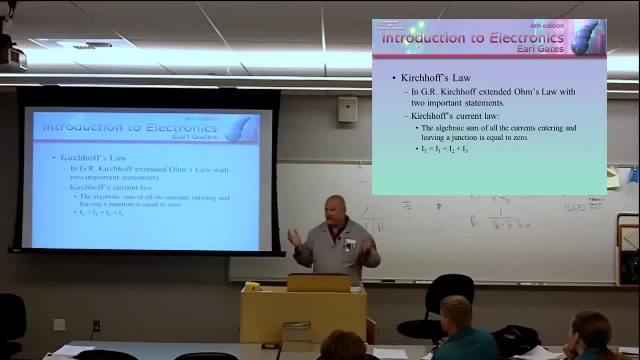 I must have five more amps coming in from another direction that I'm not aware of, And there's only one other circuit. So I must have five amps And I tell you what you could take that information to the bank. It's a law of physics. 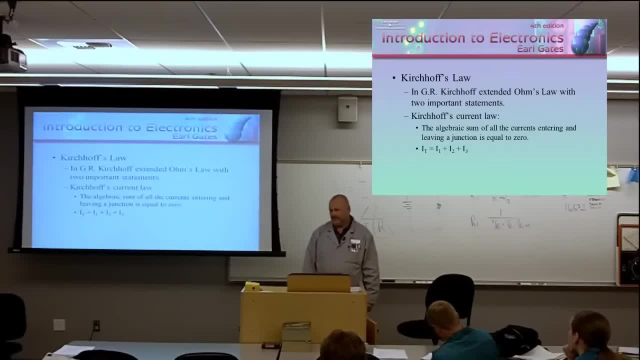 And it's so powerful in troubleshooting. It's extremely powerful in troubleshooting. There was a guy that was in my division, one of our techs in the Navy, Goofy guy. I'll tell you some stories about him and his wife in the future. 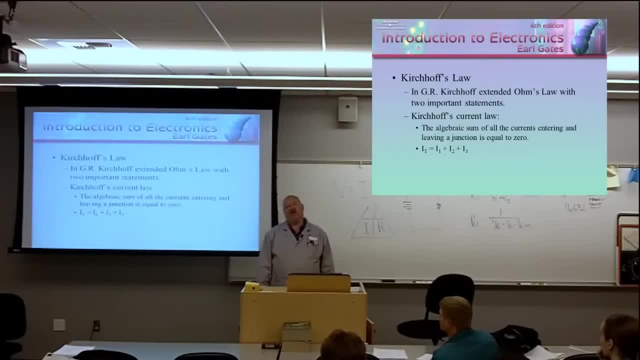 But this dude it just you know every day was a mystery What you'd see this guy into. So military equipment is put together really, really, really well, And we didn't have cordless screwdrivers, So you used to have to take stuff apart by hand. 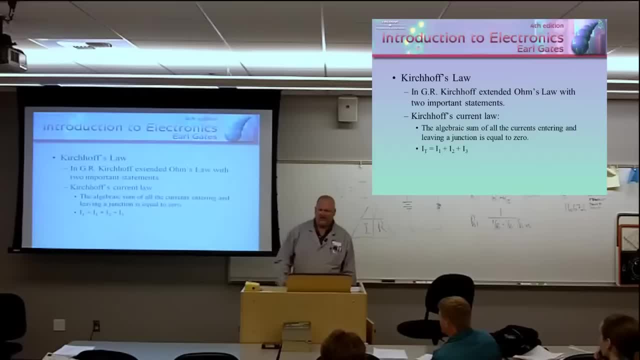 So I come in and I'm like: you know what are you working on? Yeah, we've got a problem with this unit here And I want to take this current reading. you know, And in order to take a current reading, I've got to open the circuit. 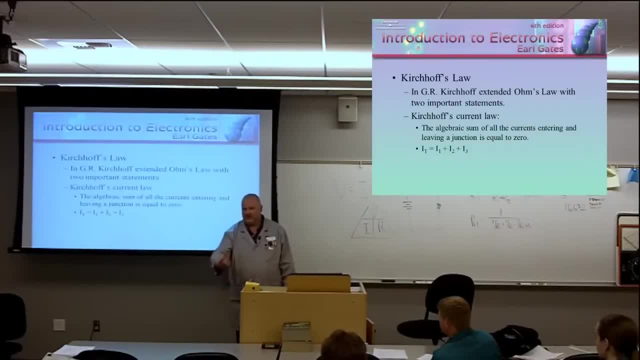 So you're going to remove this access plate here with 64 screws And you're going to remove that. You're going to get in there and take that reading. You know why don't you use this here, which is called Kirchhoff's Law? 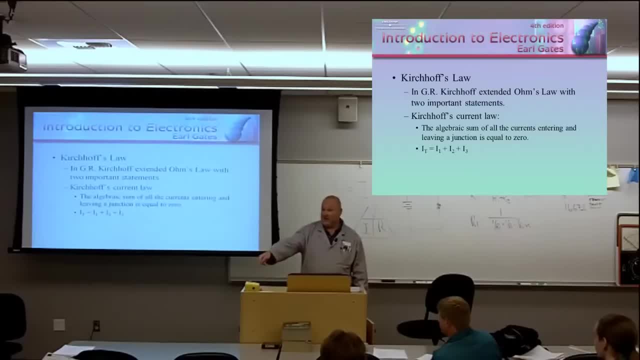 You've got this amount of current going this way, This amount of current coming in, And the unknown is what you want to measure here. You're going to use Kirchhoff's Law and determine with 100% accuracy how much current is flowing through that point. 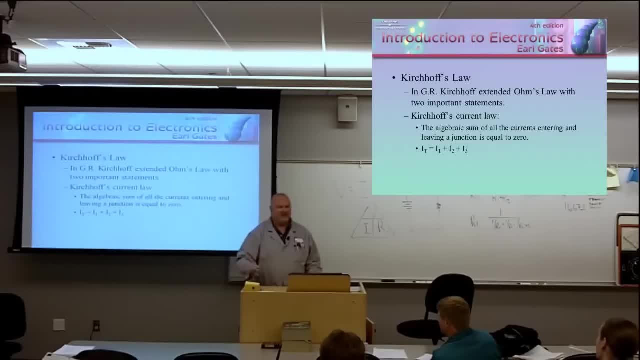 You don't have to take the panel off, You don't have to remove the screws, You don't even have to use a meter. You could use math, Put the meter down, Math Solve the problem And, to be honest with you, these are the technicians that I look for. 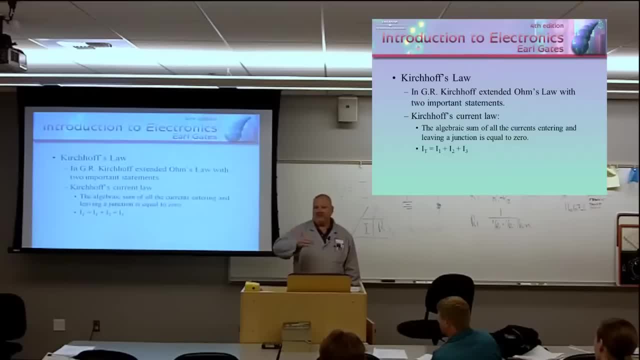 These are the technicians that I want to hire. If you start the troubleshooting process with the manual and then you're going through tracing, redrawing, applying these principles, these laws, before you go ripping into stuff, you're going to save yourself a lot of grief. 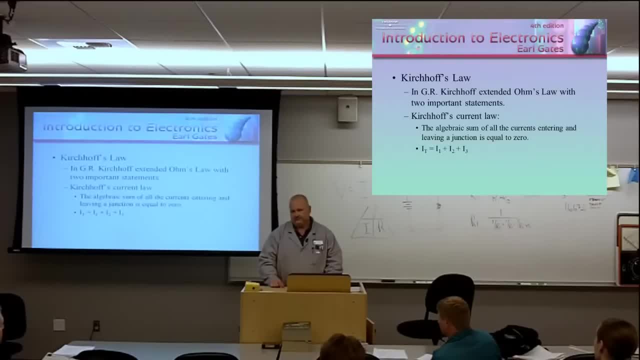 A lot of grief. It's like going to work for Boeing. Boeing builds big airplanes. On the tail of their airplanes they put a light that blinks so other airplanes don't hit their airplane when it's flying. I'm not making this stuff up. 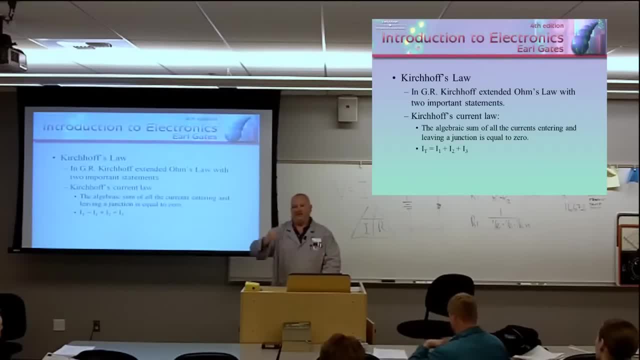 It's kind of like the light doesn't work. Well, let's get a man lift and get up there and take it apart. You get a man lift, You get all harnessed up, You're five stories in the air. You're manipulating the controls. 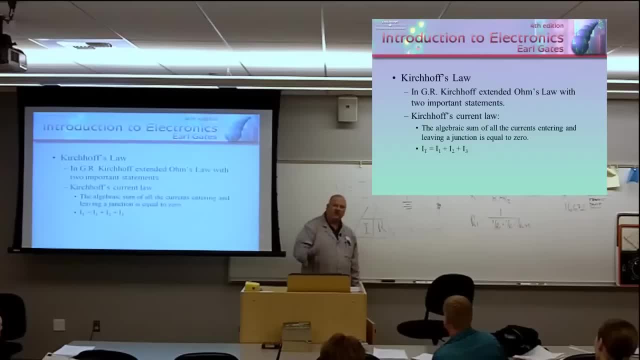 and all of a sudden, oops, You put a dent in the rudder. You've done some troubleshooting, probably through an access panel down below, using Kirchhoff's law. How much current do I have flowing up there? What's going on Then? make some determinations. 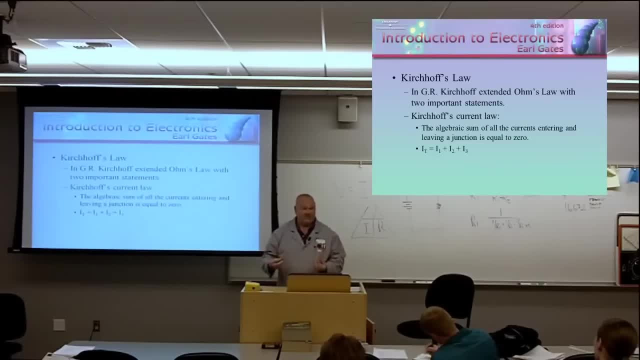 Is it really essential for you to get up there and take that assembly apart? Get a man lift, Harness yourself up, Run the risk of plowing into the rudder- Accidents happen. So always look at that kind of stuff. Is there an easier way of going about? 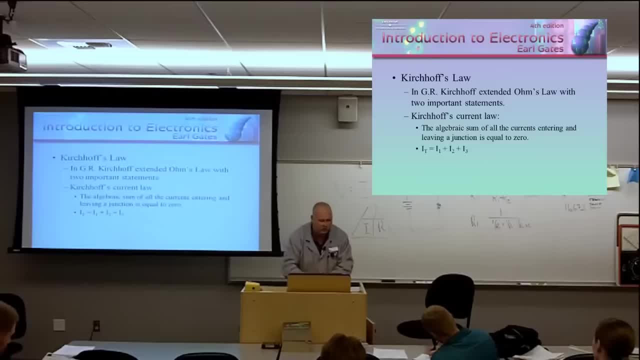 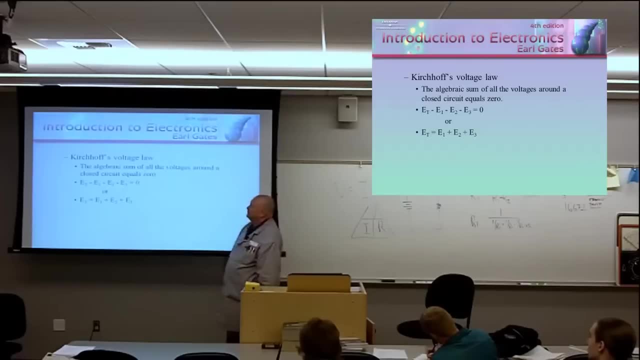 getting the reading that I want. That's the power of Ohm's law, Kirchhoff's law. Kirchhoff's law also has a voltage application And Kirchhoff says: the algebraic sum of all voltages around a closed circuit equals zero. 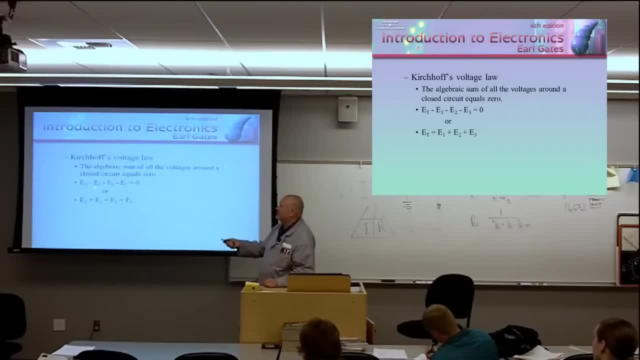 This is a fancy way of saying: voltage rise equals voltage drop, And you know how much you're left over with Zero. We talked about this last week. We talked about this last week. We talked about this last week. If you put 12 volts in, 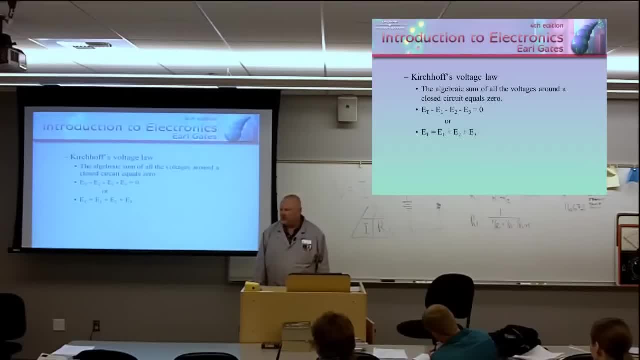 how many volts are going to get used? 12. If you're troubleshooting and you can only account for 11.5 volts, that half a volt is somewhere that it doesn't belong. You got 120 volts that are supposed to be coming out of these outlets. 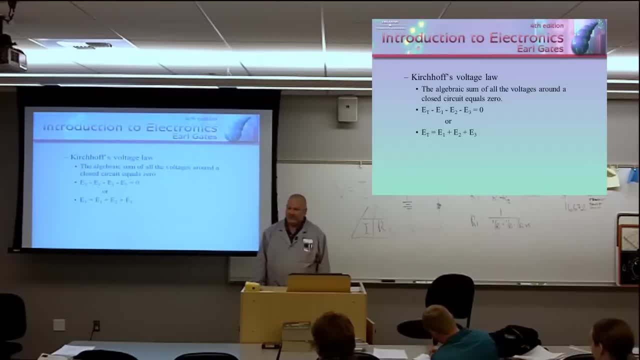 If you plug it in, you only get 98 volts. Something's wrong If you could go to that box and prove that you got 120 across each leg, but you go to an outlet in your home and you get 98, something's wrong. 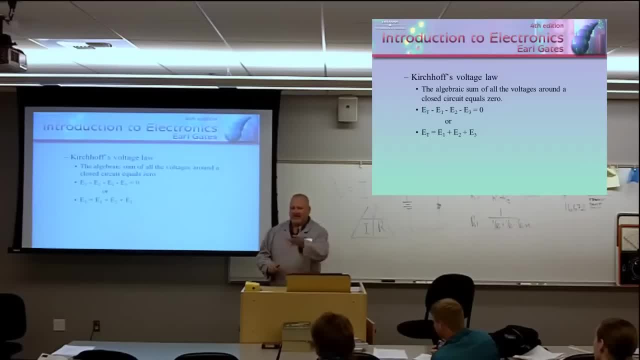 You find where the missing voltage is, you find the problem. So again, does this sound really basic? What goes in must come out. It is, But I'll tell you what. when you get to industry, you'll deceive me. You're going to get your head all. 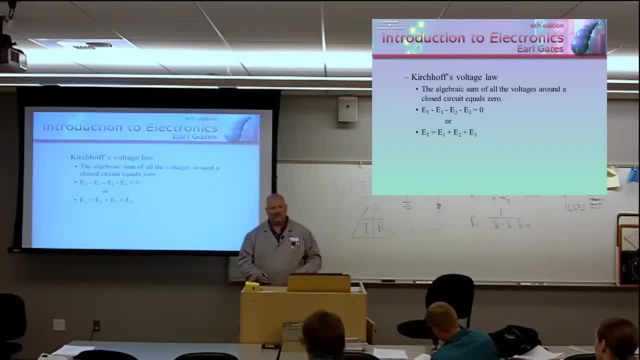 complex. I never worked on one of these before. Oh sheesh, it's got to be something. really it's got to be. the flux capacitor must have failed. I missed that day when Joe talked about the flux capacitor. No, no, no, Keep it basic. 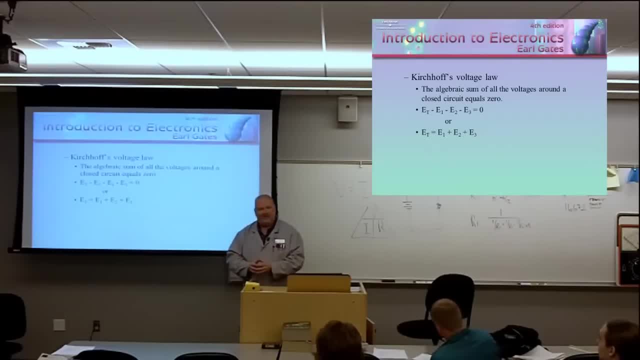 Keep it basic: The fundamental parts of the circuit: the source, the load, the internal wiring, the controlling device, the protective device. You got to be able to prove every one of those parts- functional parts- is functional, And how are you going to learn? 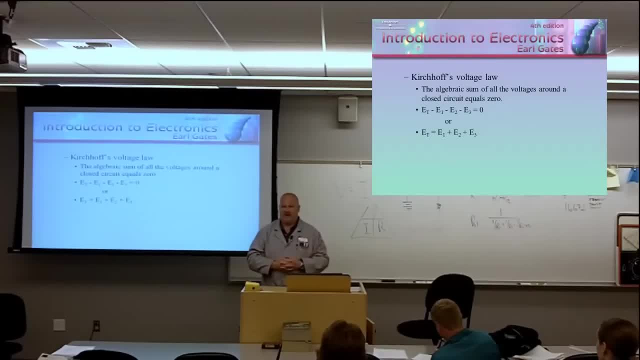 how to do that In the lab, by doing your labs Theoretically. how are you going to come to appreciate that? By attending a lecture and doing your written assignments? Because that's what this industry is about: It's about the written. 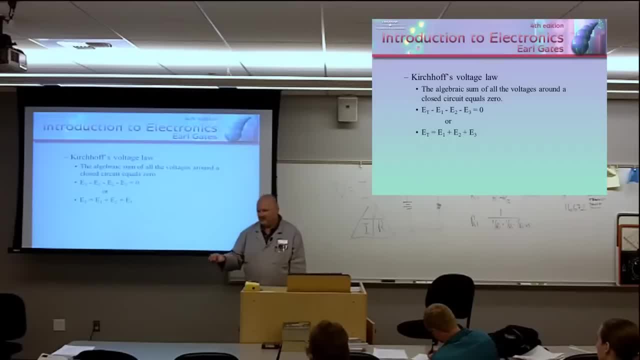 theory, which is kind of cool. Some of you had back-breaking jobs in the past. Okay, I never worked a hard day in my life- Actually I did, but it was all mental, And I'll tell you what. there were days. 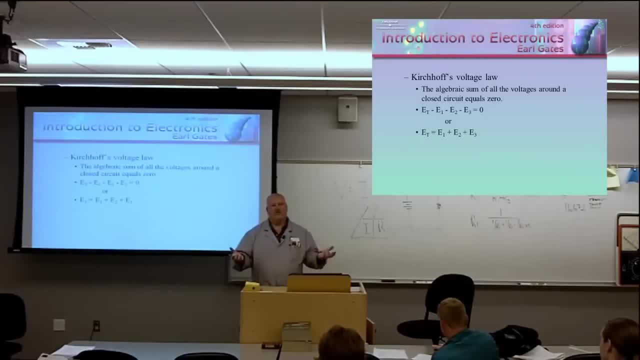 working on my system. That's the other thing too. It's one of the reasons that we all try to treat you as professionals here in this program. When you go to industry, you're going to be professionals If your equipment ain't broke. 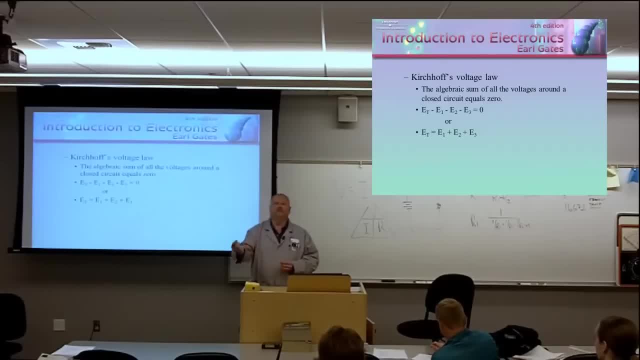 they don't care what you're doing, But when it's broke they expect you to be there bringing it back from the dead, No questions asked. Well, I'm a union guy and do I get time and a half to fix the freaking gear? 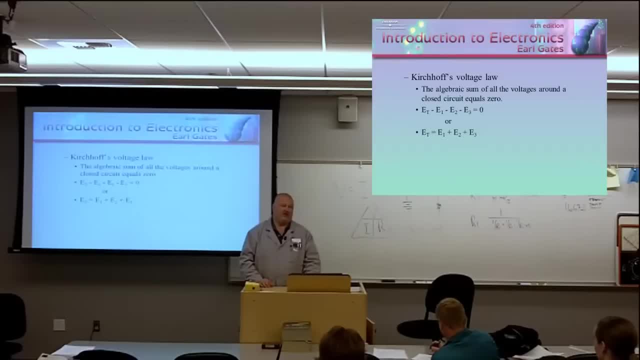 Get it up and running. That's all they care about. And you're actually there are some union maintenance jobs that do pay you well if you've got to put in that overtime, But generally speaking, this is where you make your money. 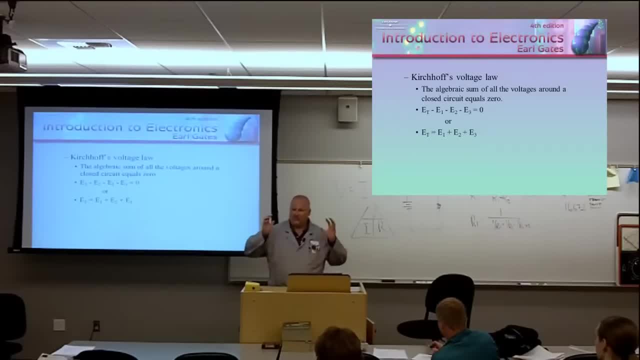 This is the most. I tell you what. I'm taking a lot of time with this chapter. This is one of the most important chapters of the book. It's one of the most important chapters of this entire program. I could talk for a week about just this. 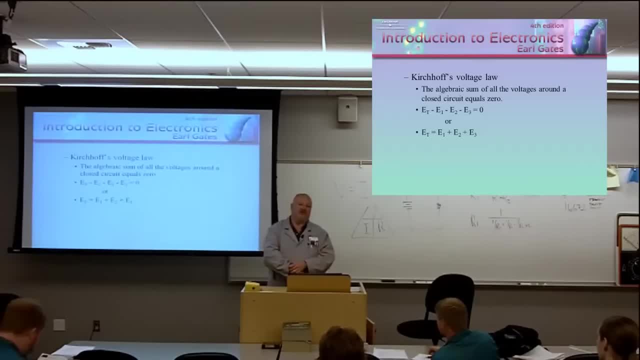 chapter, And you know what the beauty of it is. You've all been here. This is your third week in this program. Do you understand what I'm saying? Do you understand what I'm saying? The message isn't going to get any worse. 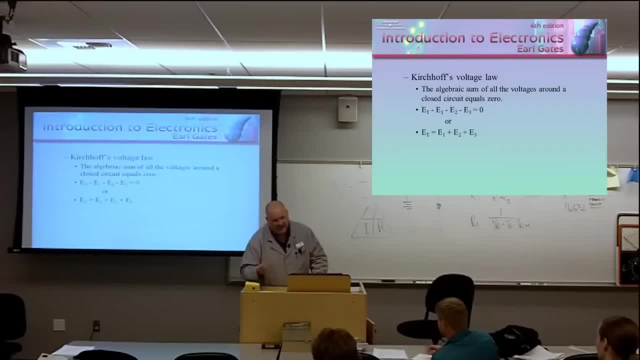 It's not The most complex. electronic systems could be rapidly troubleshot. keeping these fundamental skill sets in mind, Ohm's law, Kirchhoff's law, five basic parts of a circuit, Is my source good? Is my load good? Is it the interconnects? 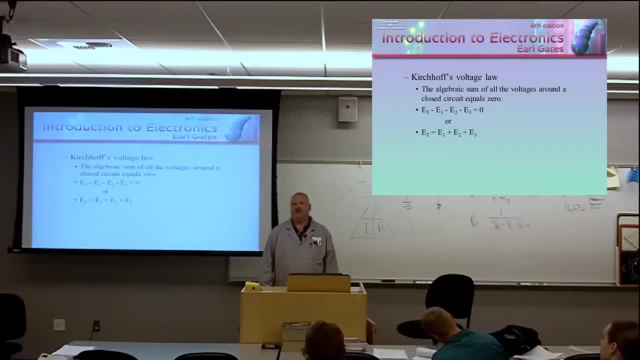 Can I prove that? The other thing you've got to do as a technician is just pay attention to what can you check quickly? What can you check quickly Again, like my former esteemed colleague on the submarine- Mike Weirup was his name Weirup? 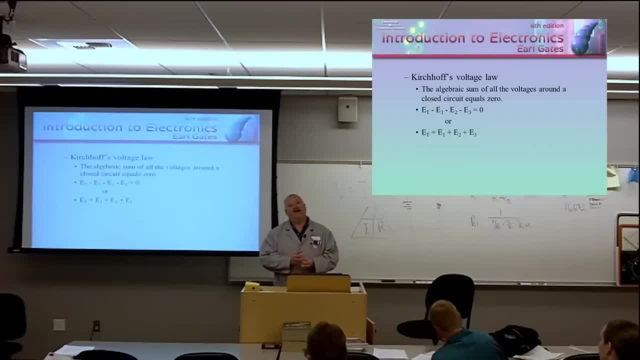 Weird name. He'd be the kind of guy like: well you know, I think it's the wiring Joe. I want to do continuity checks. I mean, you're talking these big multi-pin connectors and you're going to disconnect and check the continuity. It could take months. 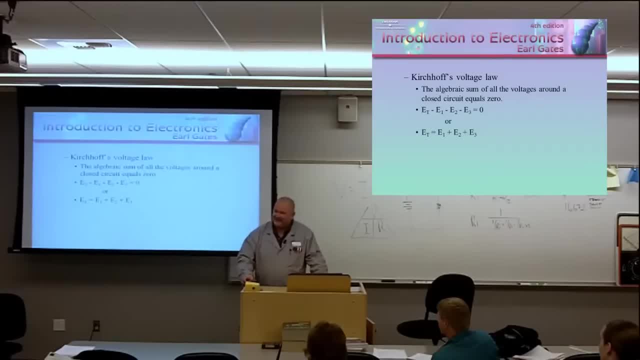 You really think that's the problem? You really think a wire like broke in the middle of the night behind that equipment rack? You know I don't think so. I think it's, you know, maybe something like controlling device. Have you tried reloading the software? 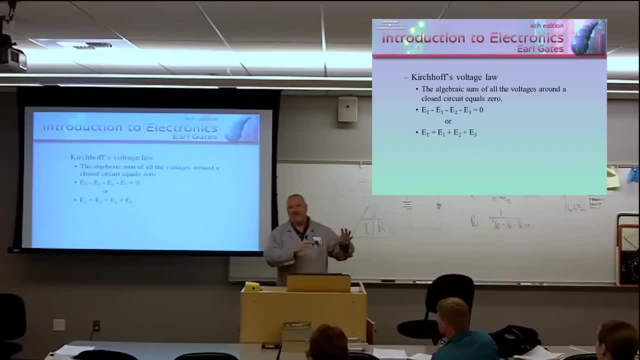 You know the virgin version of software that we have in that safe. Why don't you try reloading the version of software Controlling device? is what I'm thinking right? Reload the firmware software, Reboot the system. See how the problem manifests itself. 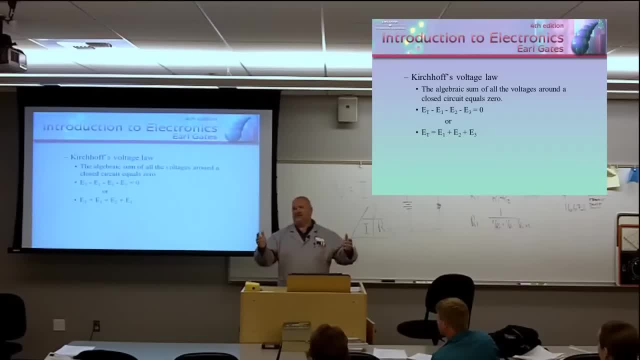 Oh, Joe, The most amazing thing happened. Reloaded the software Started working. Wow, Good thing you didn't like take you know, six months and check the continuity of all them. wires in the back of the equipment rack. 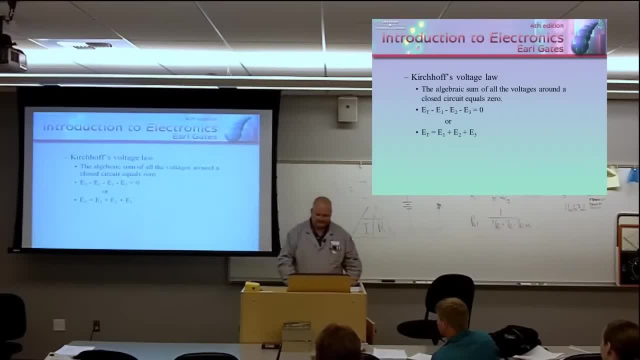 What would the odds have been? In summary, the electric circuit contains a voltage source, a load, a conductor, the two optional ones: controlling device, protective device. Don't second guess those Hey want another troubleshooting hint, Another type of protective. 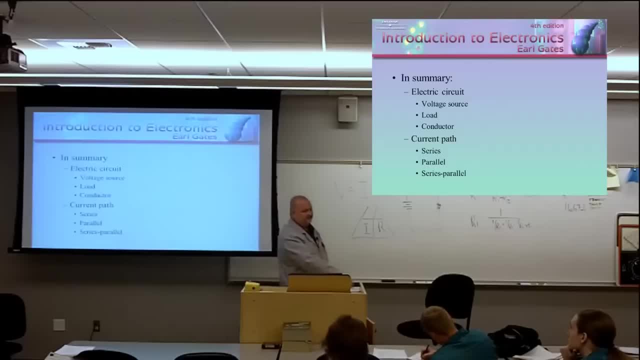 device. It's called a resettable fuse. Resettable fuse: A lot of consumer electronic products- DVD players, VHS players, stuff like that, tuners, TV tuners- have these resettable fuses And a lot of times what happens is the device. 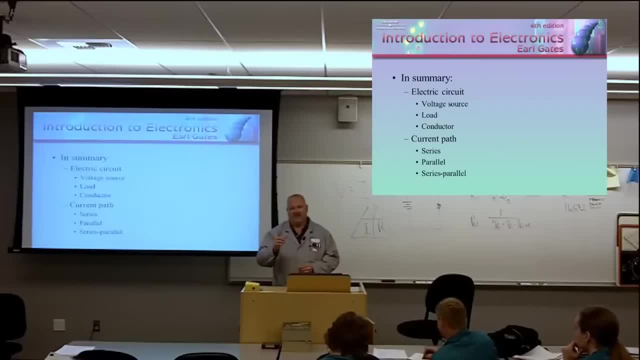 will not work. So it's kind of funny. You know my family, they all know. you know Joe in the family. he's the electronics guy. You got a problem. you know they always call me with the problem. 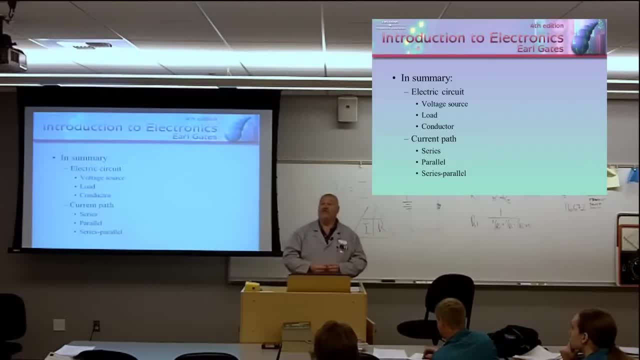 So it's amazing how many things I've fixed from afar. They tell me what the problem is, you know, And a lot of these have been with DVD, VHS players, things like that, in the past. So well, what I'm going to have you do, 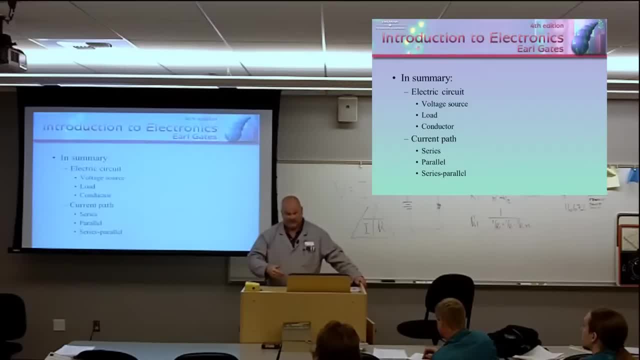 is. I've got a ritual that I'm going to go through here on the West Coast And I want you to unplug that device. okay, And what's the most comfortable chair you have in the house? I want you to remove it and put it in the most comfortable chair. 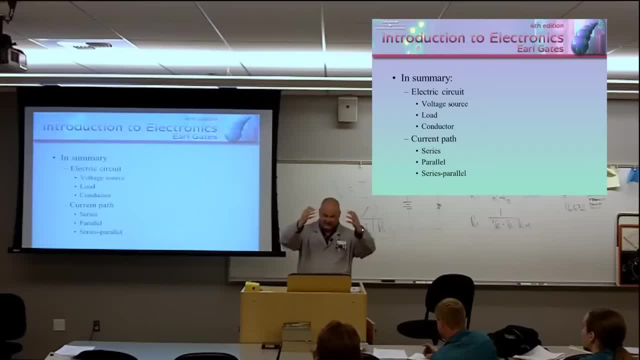 of the house overnight And I've got some rituals and some telepathic, you know things that I'm going to do, And then I'm going to call you back in the morning and let you know when I'm done, Okay, And I'll go plug it in. 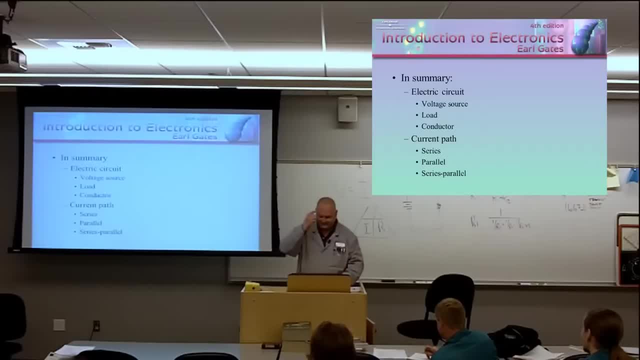 Holy cow, it works. How did you do that? You know It's all about chi. Okay, Freaking resettable fuse. For whatever reason, there was a glitch that tripped that you've got to unplug it totally, discharge the whole unit, plug it back in. It reboots. 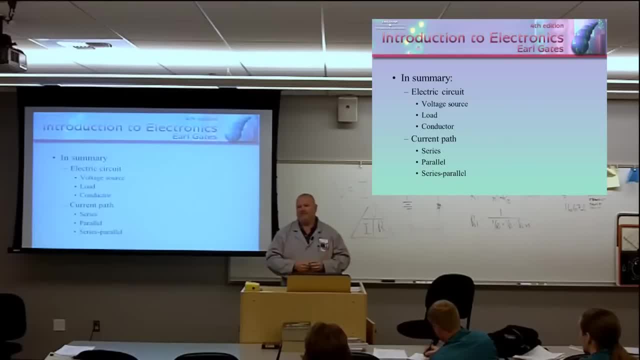 thinking it's back at the factory the first day it was ever made. Problem goes away. You've got to make sure you give it overnight to be able to do that. So I've brought back countless. I've had a lot of people come in here, Colleagues, 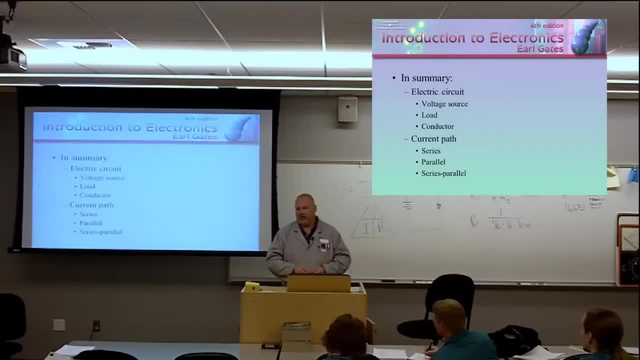 Hey Joe, my amplifier, This amp doesn't work anymore. You could have it if you could fix it. Okay, Because I went out and bought a new one. I figured this thing is toast. I go plug it in, It works. 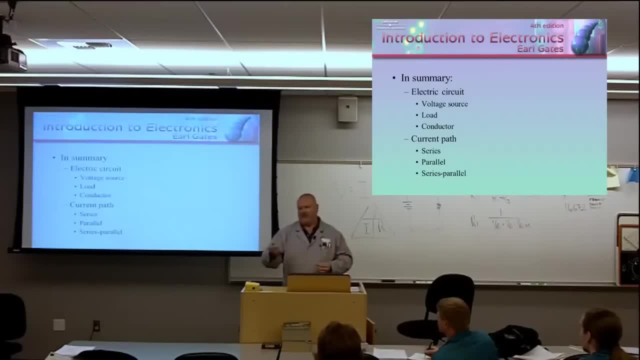 By you unplugging it, you fix it. I don't even go on it with people. You'd be surprised the amount of stuff that you could fix by simply unplugging it for 24 hours. plug it overnight, Not even 24 hours. Plug it back in, you're good. 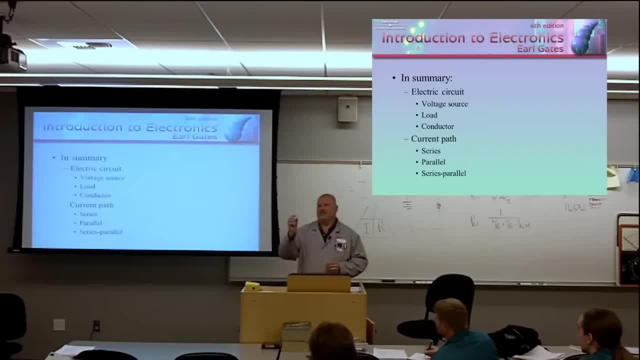 to go. Why does it take time? Because these resettable fuses- there's a time delay before they're actually solid state devices, before they physically reset and allow the circuit to function properly again. So you want to get it back to that neutral state of. 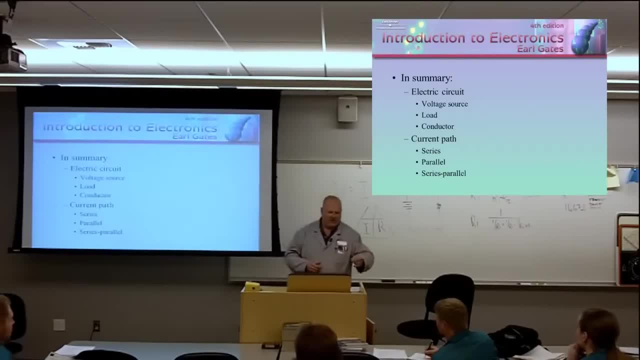 when it left the factory? I don't know, In mobile audio did you encounter any of that stuff Where by disconnecting it for a period of time would fix the problem? Yeah, I mean when, if you did a hard reset? 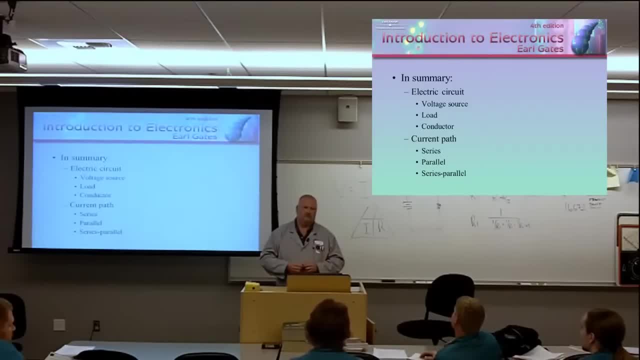 touch the positive and negative together and make sure the circuit's completely different: Unenergized airbag lights, some control systems- if you did a hard reset it would do that. Okay, To make sure that everything dissipates and it's on the fastest. 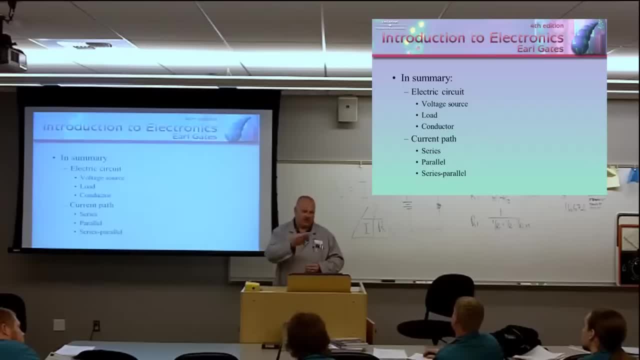 way. Yeah, And that's the other thing that you can do. even with a DVD player, if you just short, not unplug it, make sure it's unplugged and then keep the leads shorted together, then that's kind of a fast track. 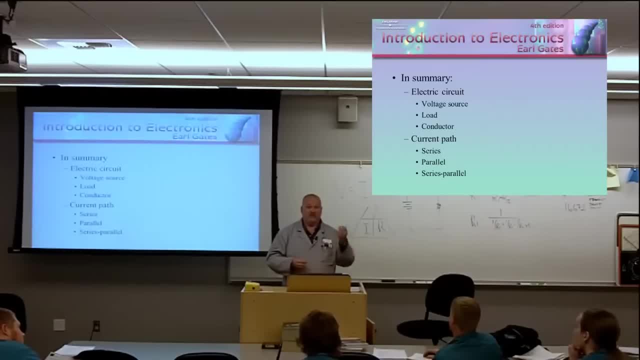 But still, there's some capacitors we'll talk about in the future. store energy in the form of an electrostatic field that may keep stuff alive for a considerable amount of time. Flux capacitors: Don't care. Current path- We talked about series. 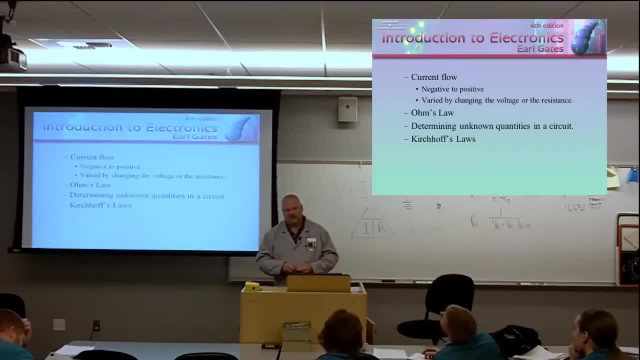 circuits, parallel circuits and complex circuits. series. parallel circuits: We talked about current flow, negative to positive, varied by changing the voltage or the resistance. We talked about Ohm's law And also determining unknown quantities in a circuit, as well as 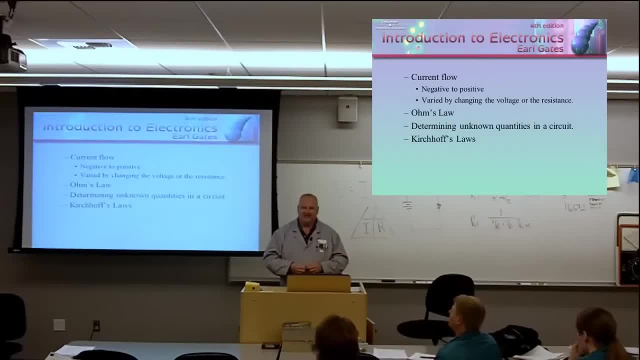 Kirchhoff's law For current: current is constant in a series circuit. Ohm's law: All the current entering a node must exit the node. Kirchhoff's law- Powerful, powerful stuff- Prevent you from removing 64 screws. 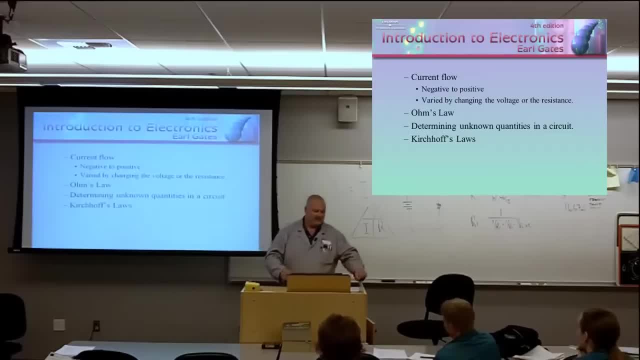 by hand to take one reading. He used to think I was an a-hole. This here is Kirchhoff's law. I stayed awake during that class. You could use this here tool to prevent yourself from removing 64 screws. Chronic, Chronic, here freaking. 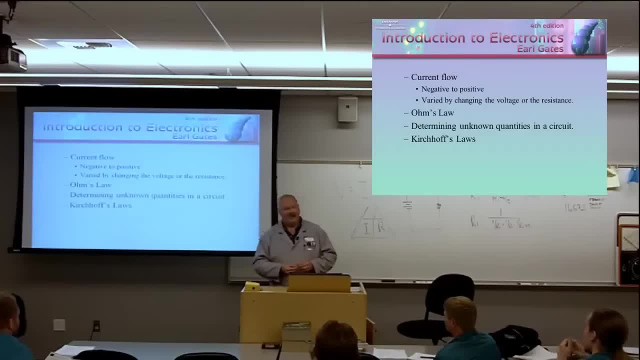 jerk? No, No, I'm not. I think the guy that's removing 64 screws and then is going to strip the screws Break the heads off. That's another story. There was a dude. a local company Can't make this stuff up. 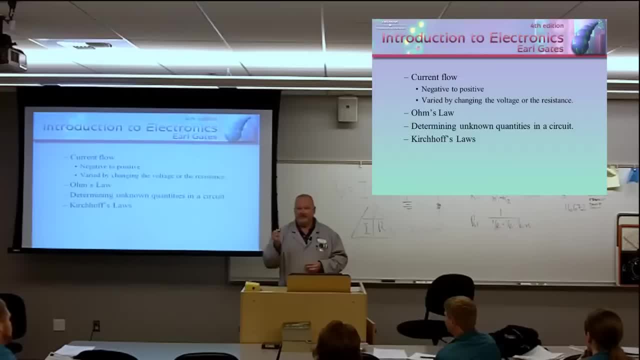 Broke heads of screws off. The product's ready for shipping. Got freaking instant glue. Glue the heads back on First time it was out in the field. then they took a panel off for maintenance. Snap, snap. What the heck is this? What is that on there? 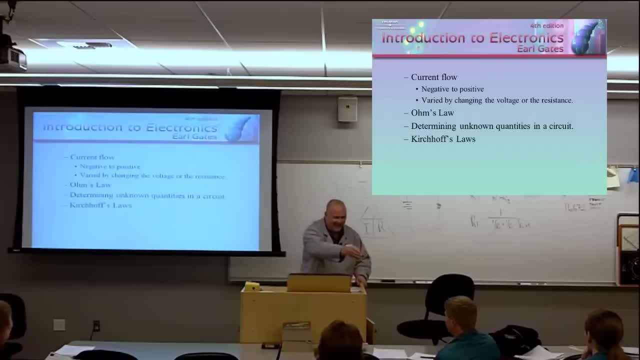 They look at it, It's like this is instant glue. Who worked on it last at a company? Why'd you do that? Well, I didn't want to get in trouble. Peer out of here. You know that instant You can't. 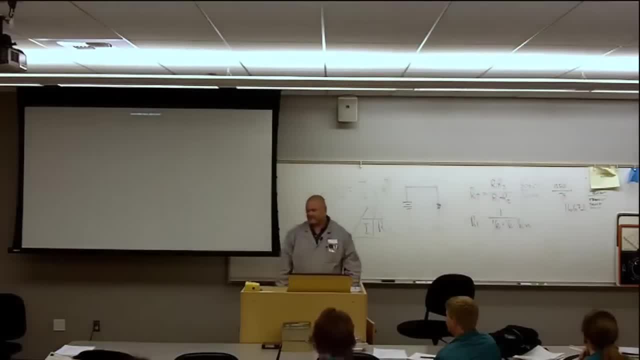 make stuff like this up. Try to avoid it. Questions: Electricity is a theory, right? Yes, and that's basically what we're studying is a theory: Laws of physics. We have proven that, although this is theory, these are laws of physics. 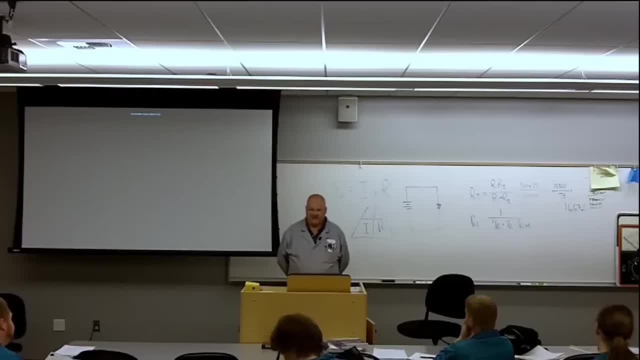 Voltage, the relationship between voltage current and resistance, The relationship between voltage current and power. Kirchhoff's laws: they're laws of physics. We know that we could prove with 100% accuracy that this is how they behave. 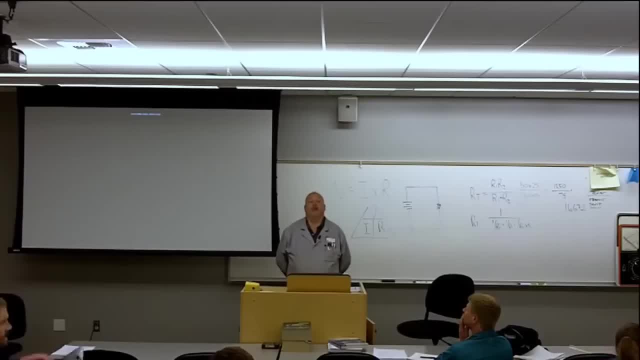 Scram. Also, in science generally, a theory is something that is provable to an infinitesimal degree, and a postulate is something that's unpermissible. Very good, Thank you. Okay, hey, before we wrap things up, because we got. 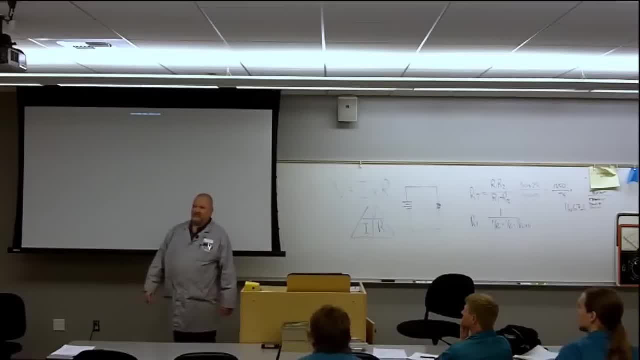 another chapter to do. okay, But fortunately, one of the reasons that I took this amount of time here is: this other chapter is not a chapter that I am going to lecture on. It's another chapter that you've got to watch some videos on. 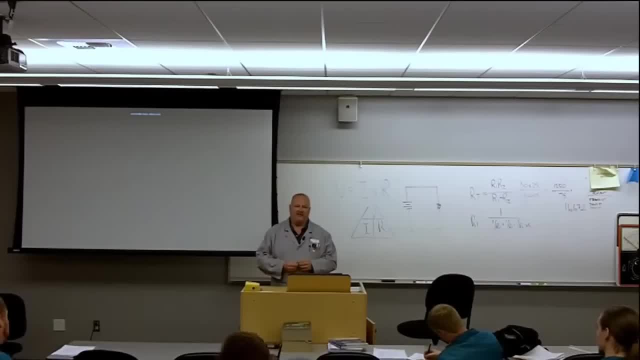 There are four videos. When you go to the Google site, it's going to say: follow this link to watch test equipment videos. Okay, And there are four videos that I want you to watch And you're responsible for the information. I think all of you kind of. 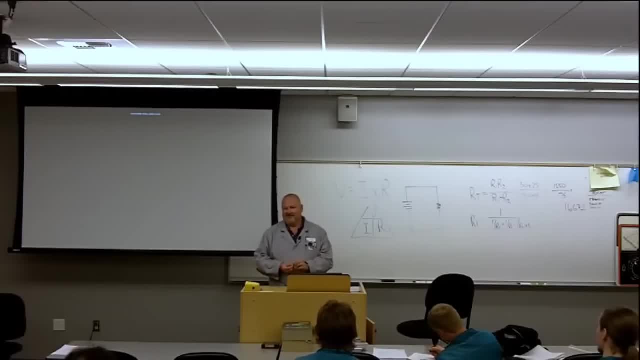 figured out that I'm the kind of guy that likes lectures. Okay, I like to have fun with lecture. Hopefully you're not falling asleep during my lectures, But I like lectures And it gives me quality face-to-face time with all of you. 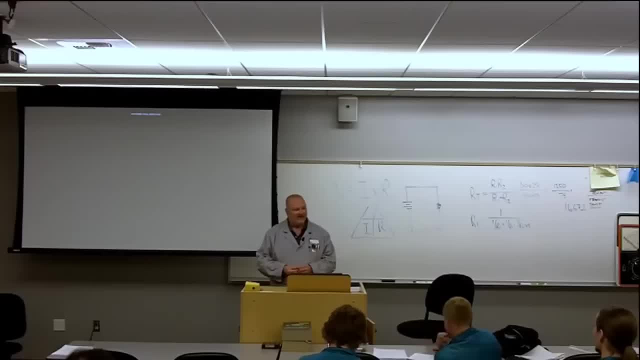 However, that being said, I also am not the smartest guy, but I know that a picture is worth a thousand words. So if I could have you watch a 15 minute video, that's a lot of frames, That's a lot of pictures. 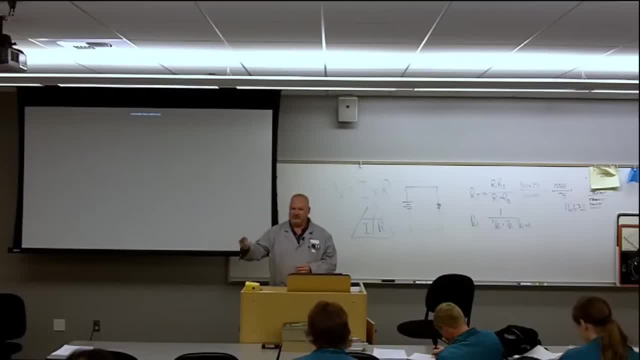 That's a lot of data, More time than I have to preach to you about this stuff. The four videos: The first video is going to be a basic introduction to digital multimeters versus analog meters. Okay, The analog when I speak of analog. 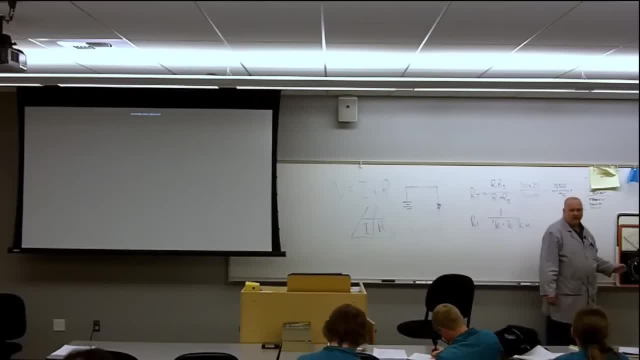 this is what I'm talking about here: Kicking it old school. The digital meter is going to be based on a Fluke 70 series meter that, quite frankly, all meters are really measured against. The second video is going to talk specifically. 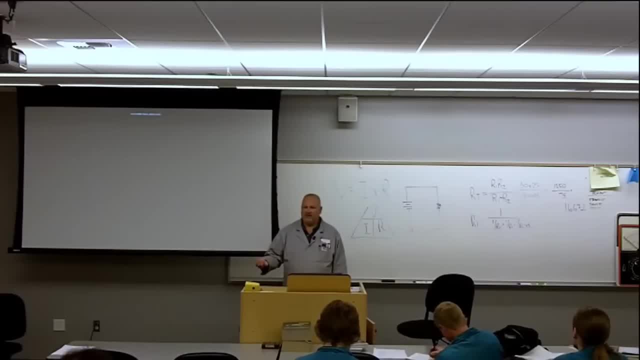 about how to perform resistance and continuity measurements using an analog meter and a digital multimeter. Resistance and continuity. The third video is going to talk about measuring current and voltage. So by the end of those three videos, you're going to know how to measure. 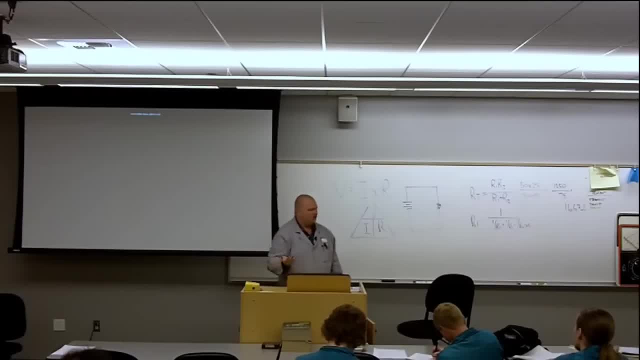 resistance, current and voltage. If you know how to do that, let me tell you you got it going on. You got it going on Because those are three of the big four properties that all of this is based on. So these are. 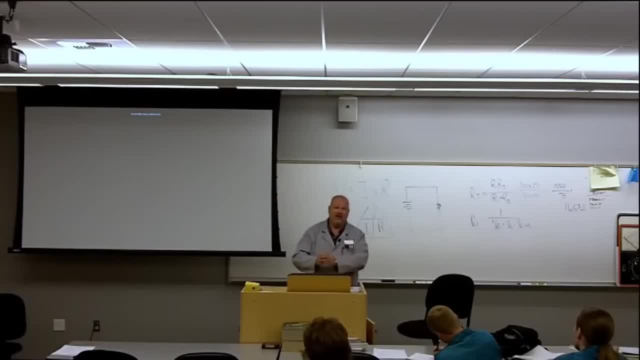 very, very important videos. One of the reasons that we have them in videos and uploaded is so that you can watch over and over again to make sure you understand exactly what the process is. So by the time you get into the lab, you can apply that. 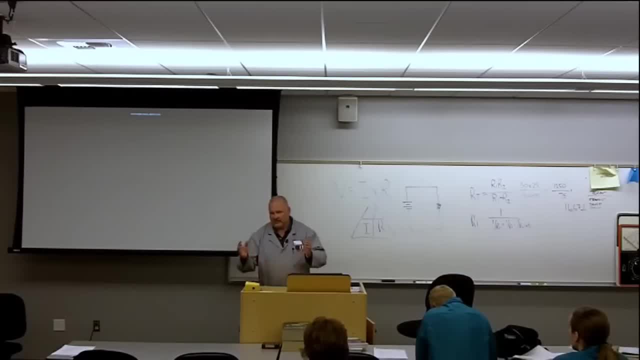 Very, very critical, Like how to defuse a nuclear bomb. You want to get it right the first time. The fourth video is produced by Fluke Corporation. How many of you know about Fluke? Fluke is the real deal, The real deal. 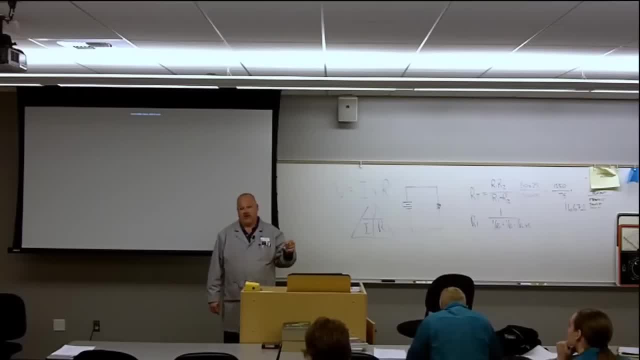 Expensive local company, John Fluke, Former submarine guy, Got to support his product. He was before my time But yeah, John Fluke is a former submariner. They produced this video and it's kind of a drama- Not a drama like. 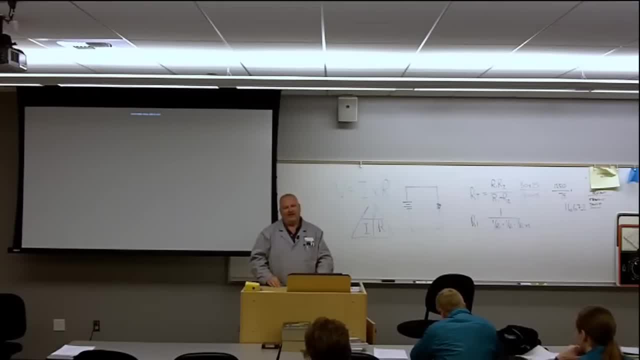 oh, I can't believe he's going to test the voltage. You know it's got a story behind it. There's a kid who's working on the job and he blows up something and his boss is like you need to go out to the community college and talk with. 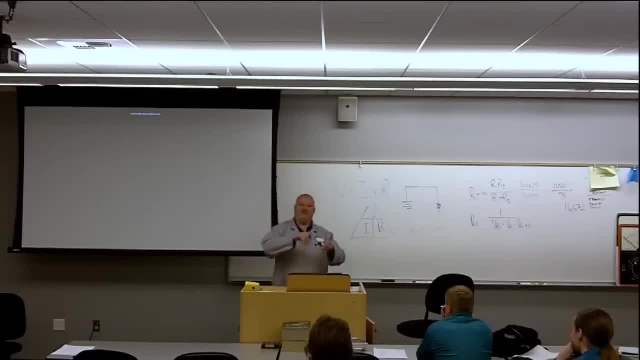 your electronics professor And basically it reviews how to perform basic measurements- Resistance, current and voltage- with a Fluke 70 series DMM. That's the fourth video, So all of the information in those videos is testable. The link is on the Google. 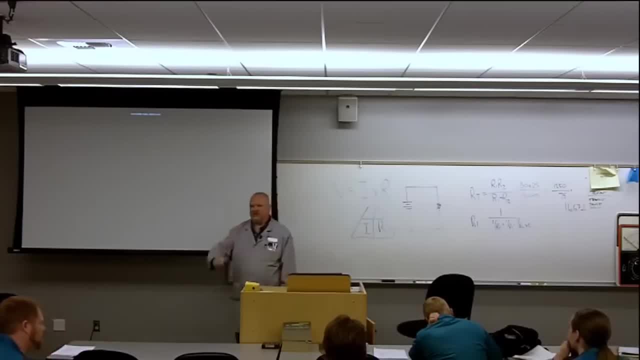 sites. You can watch it in the privacy of your own home, You can watch it on these machines, but that is what we are doing in lieu of this chapter on test equipment. Does anybody have any questions on anything that I covered tonight? Yes, 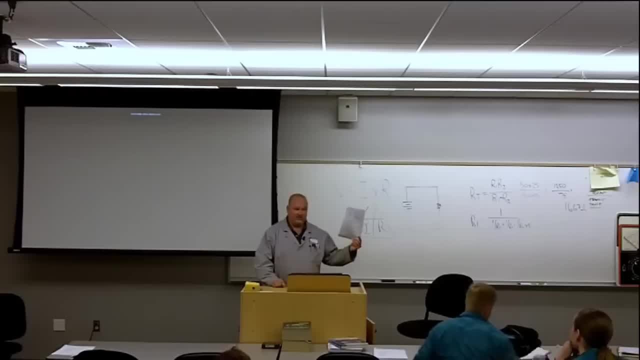 No, the Google site, It's the sites that were in the syllabus. Okay, This right here. If you go to that Google sites- the electronics, LWTC electronics- you're going to see a link in there. Follow this link for test equipment. 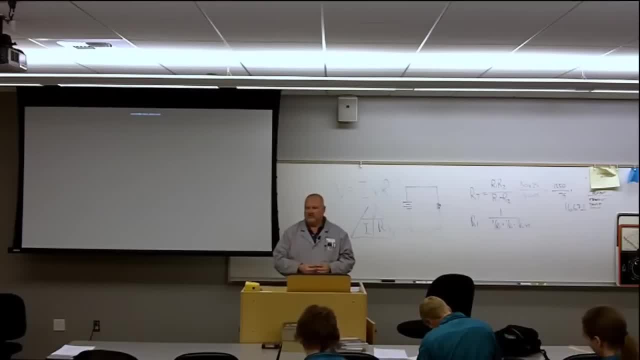 videos. You click on that and then it brings you to some server in Peru that we've uploaded those videos to. We got stuff all over the place, But you know what The alternative is: you got to sit here and watch it all. Okay, We've really tried. I got my. 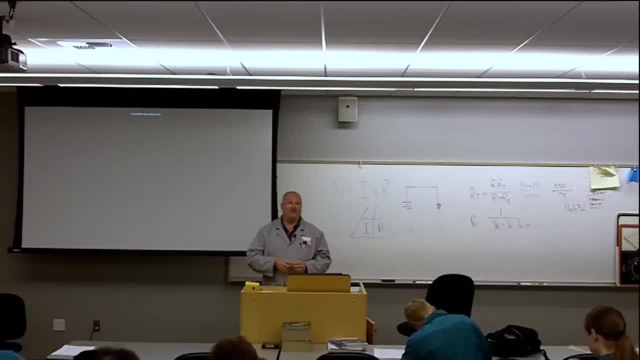 TAs working very, very hard to get as much stuff as we can uploaded to the web so that you could look at this stuff morning, noon and night. Any other questions on anything in general? Okay, Make sure you get that video watched over the next 24. 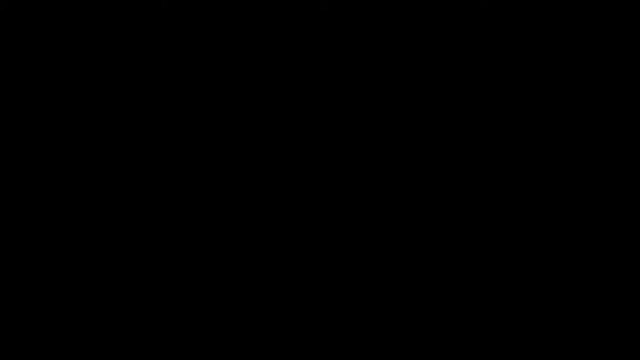 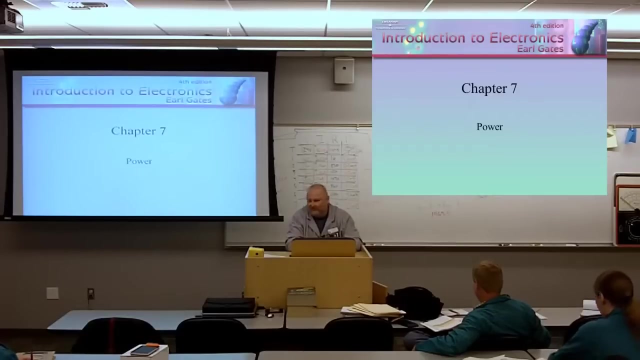 all those videos watched over the next 24 hours. Alright, A chapter that I really like talking about. It's chapter 7.. Because the title is power And I like power. I like power. Remember what was it? Tim the Toolman. 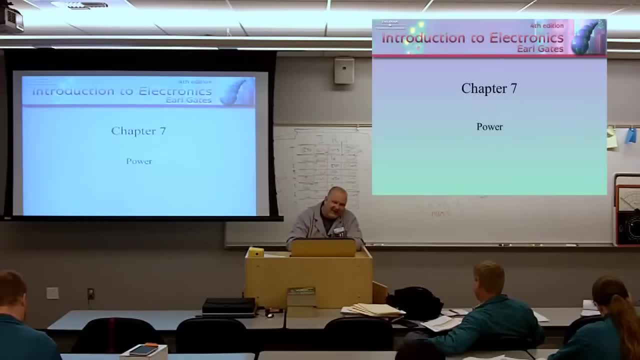 Remember power. You can never have enough power. You know the gas powered blender. I think it's a great idea- You know, if you've ever mixed any frozen concoctions- having a little bit of extra power there to chop that ice up. 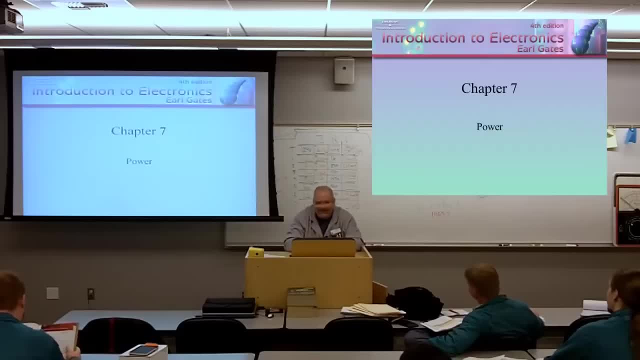 and you know, get just the perfect consistency is not a bad thing. So I've never driven a car. I've never driven a car that's had too much power. Actually no, And I did have the opportunity. I went through Richard Petty's driving school. two years in a row. This was probably about 10 years ago And I thought these cars would have governors on them. You know, you go through and they're going to turn some goofball like me loose in a Winston Cup car. at the time, No governors. 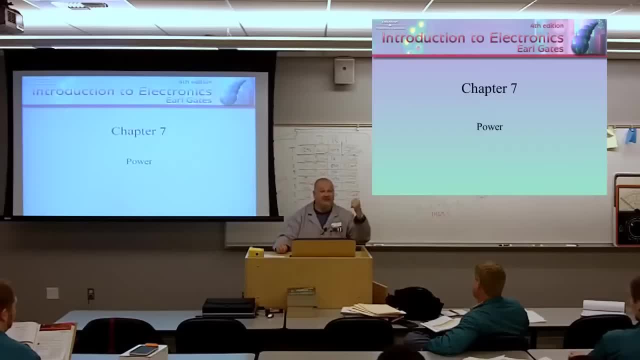 That car had a lot of power. Okay, Put in the right hand, That's the Las Vegas Motor Speedway And I turned the hot. I'll tell you the whole story sometime, But I actually got the fastest times of the day. I was at the top of the reader board. 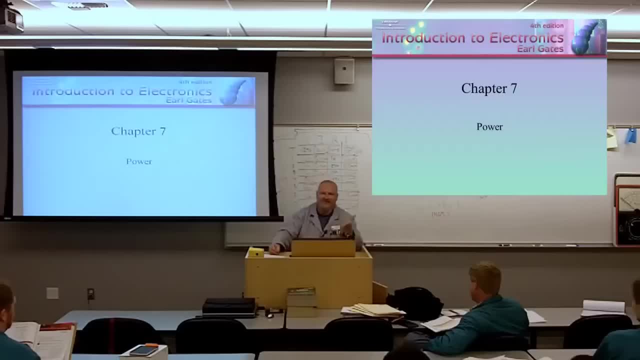 Joe Greinick. You know it was pretty freaking cool. So I was thinking about quitting my day job and becoming a NASCAR driver. Luckily I have good friends that woke me up to reality. But the power, the power was fabulous. So I 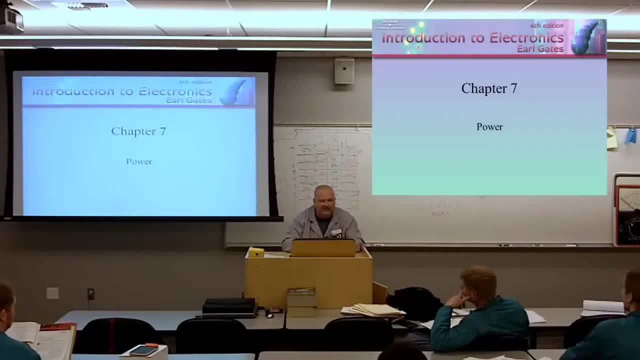 think as much as I love aviation and aerospace- you know I see the Blue Angels in town- I look at those F-18s and knowing my own piloting skills And I think I'm a pretty good pilot, But knowing my own pilot skills I'd probably last. 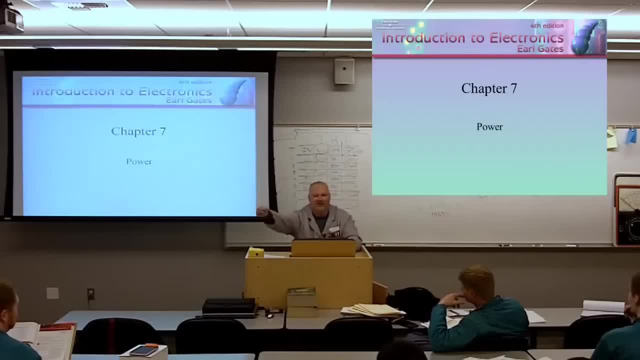 probably five or six seconds in one of those things before there'd be a fireball going down the runway. A little bit too much power for me. Power Power in electronics is in electrical is very, very important because it's the metric that we use to determine. 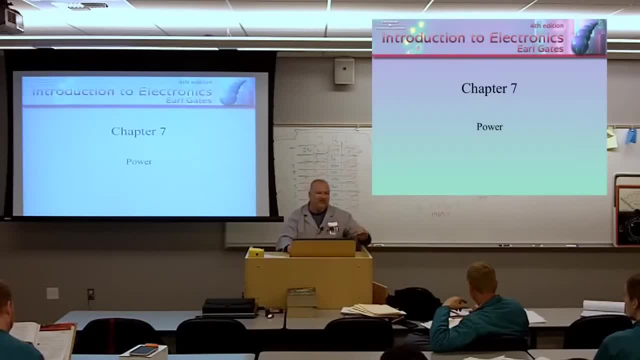 output. It's the metric that we use to determine efficiency. It's the metric that we use to show us how much energy we're converting into work. So this is a really big chapter. If you fully understand the implications of power, you're 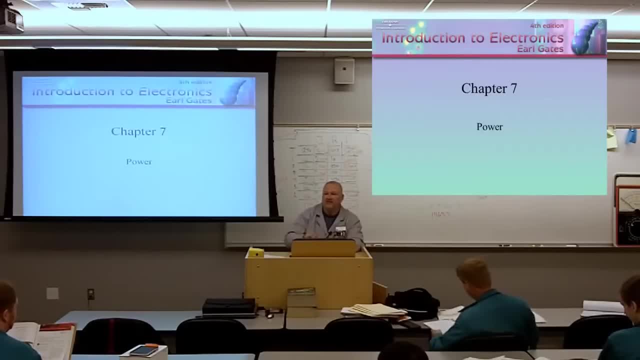 going to be a better technician- You truly are, Because looking at inconsistencies in power output is going to start to paint a story, Tell you a story And paint you a picture of what's taking place with a system. So, with that being said, let's. 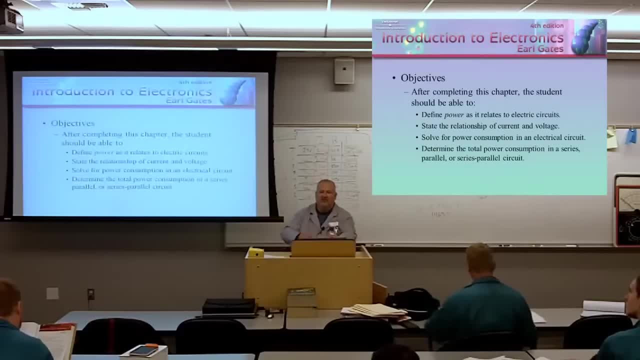 jump and immerse ourselves into chapter seven, power. After completing this chapter, we're going to be able to define power as it relates to electric circuits. State the relationship of current and voltage. Solve for power consumption in an electrical circuit. Determine the total. 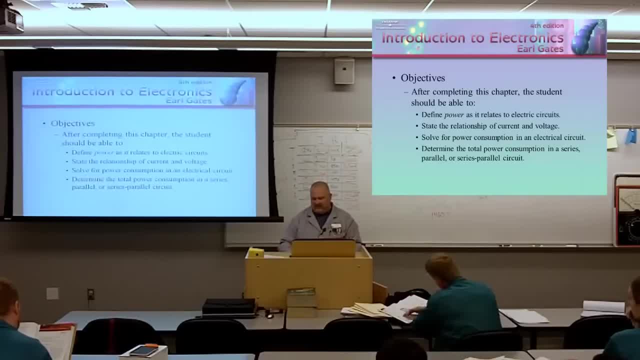 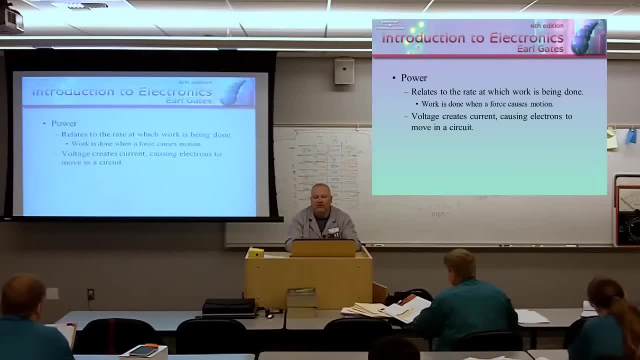 power consumption in a series parallel and a series parallel circuit. Now power relates to the rate at which work is being done. 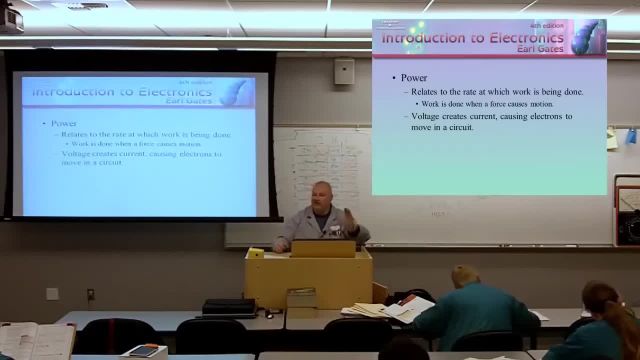 right. so by simply standing there bracing yourself against the rake, you're definitely not working to get back to a raker, and so obviously, me knowing this stuff, they think I'm a jerk. so work is done when a force causes motion. now, 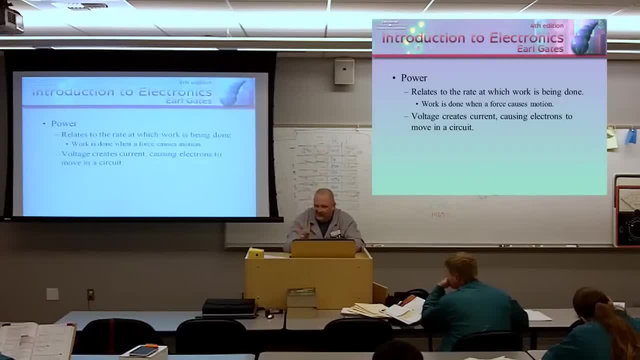 check this out: force voltage, current, motion voltage creates current, causing electrons to move in a circuit. so if you've got a voltage and you've got current, you're doing work. may not be the work you want to get done, but you're doing work because a force causes motion, voltage causes current and we know. 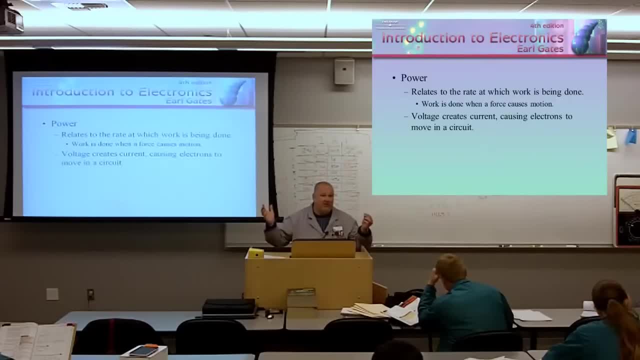 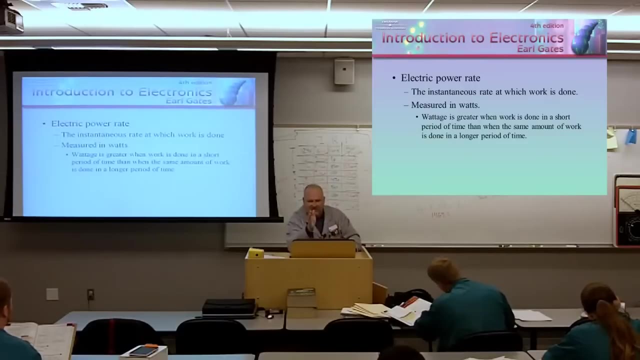 voltage is pressure, current is movement. it's got to be power. make sense now. electric power rate is the instantaneous rate at which work is done. instantaneous, that means take a snapshot right now: how much work is being done right now, right now, right now. what's the pressure? what's the current? right now, instantaneous value. make sense. 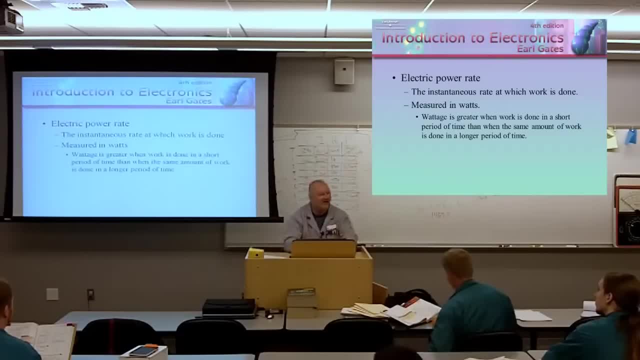 now, that's not how the power company- it's actually odd the power company- is called the power company. let's go back to that. power relates to the rate at which work is being done. work is done when a force causes motion. how many of you here pay money on a monthly basis to the power company? the power company? why? 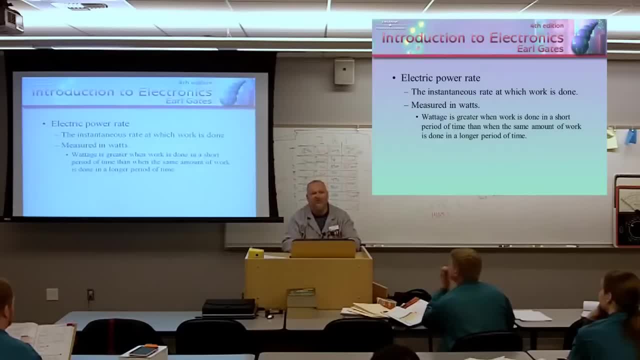 are they called the power company? all is they're really providing us with is voltage. you know who the power company is. it's you. it's to take money out of our wallets- exactly who's the power company? you're actually the power company. you're providing the the current path, if you will, for the current to flow. they're just. 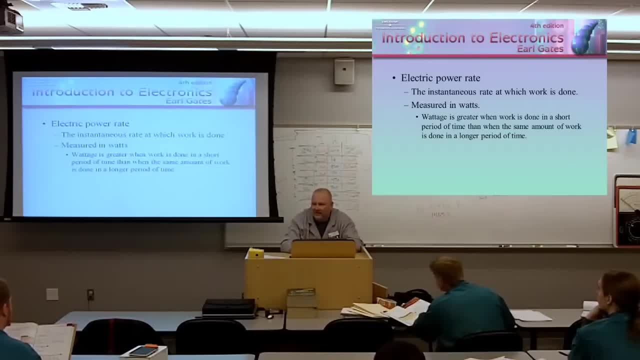 providing you with the voltage. they should be called the voltage company. okay, I mean, realistically, that's all they're doing. when you pay for electrical service to your home, all is they're providing you with is a voltage, a electrical pressure, at your box. it's up to you to hit the breakers, turn the. 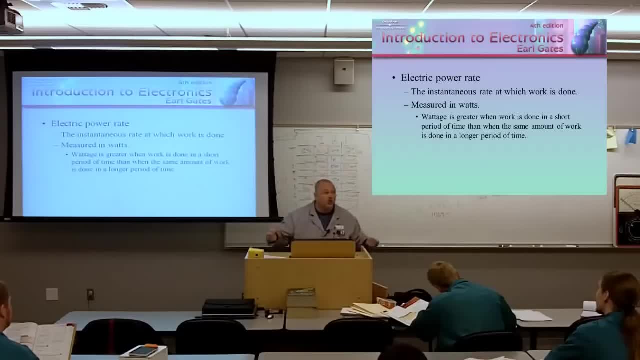 circuits on, turn your lamps on, turn your appliances on, turn your lights on, turn your loads on. that gives current a path to flow. now you're consuming power. power company always. you know. I see I take this stuff too literal, which is one of the reasons that I'm here and you're there. okay, but it just doesn't make. 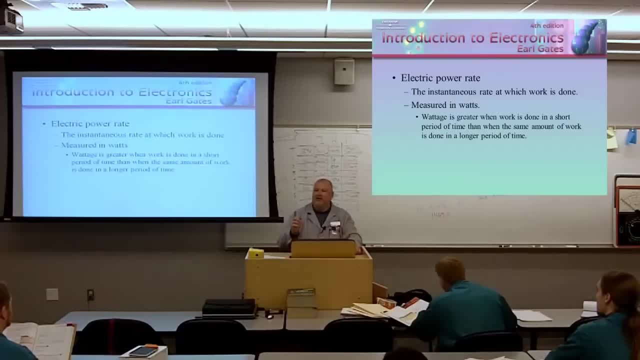 sense, does it? it really doesn't. now the power company, the voltage company, charges you in in watts. actually, the power company charges you in what are called kilowatt hours. kilowatt hours- I'll talk about more of that in a second- measured in watts, wattage is greater when work is done in. 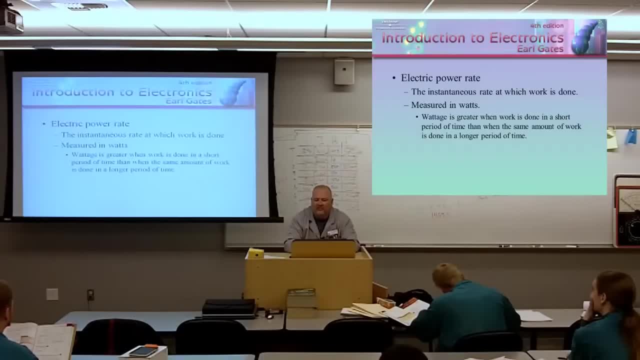 a short period of time than when the same amount of work is done in a longer period of time. wattage is greater when work is done in a short period of time than when the same amount of work is done in a longer period of time. all right, a mild example of this. it's an area of I enjoy motorsports in general. I 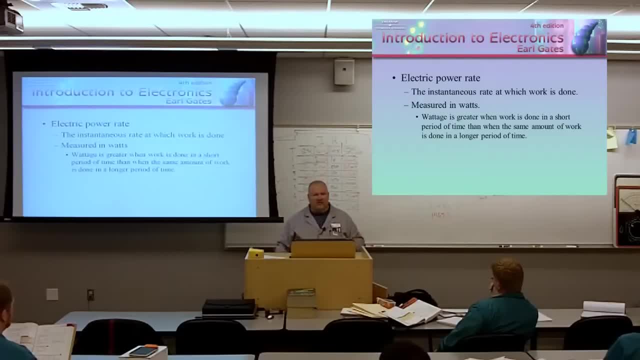 enjoy mechanical things. you know, no offense to any of you here that are into any of the fine arts, but if I had a chance on a on a Sunday afternoon of going to the opera which I've attended- the opera, symphony orchestra, musicals plays not a big 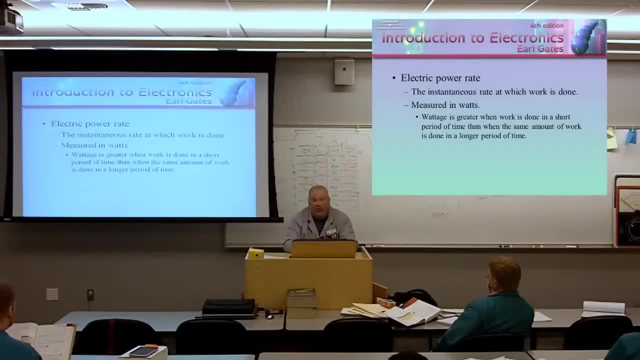 musical guy, no offense, but it's not how I roll. or going down a bowing field and standing at the edge of the fence and watching the heavy metal take off- okay, I'd probably be down a bowing field, it's just how I roll. so I've always been a big advocate of motorsports. one area of motorsports that 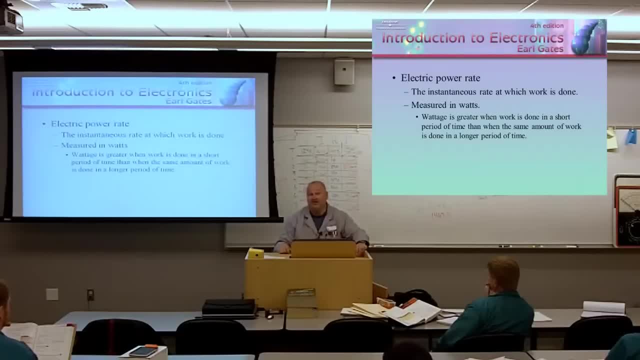 I never was really that intrigued with. I respect it, but I'm not that intrigued with pursuing it is drag racing, but I respect it immensely. drag racing is about getting as much and power out of the engine and coupling it to the wheels and getting the car down the track- quarter mile track- as quickly as you. 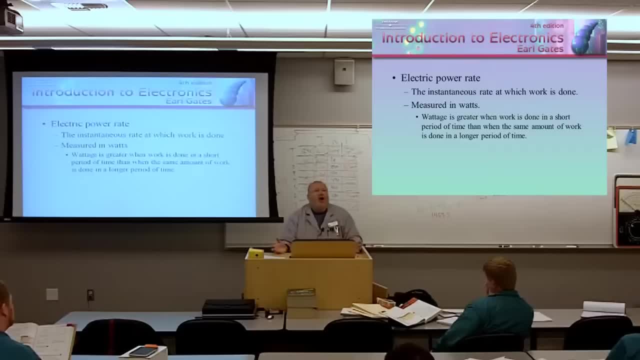 possibly can. and if any of you ever watch drag racing, I'm some of the rocket rocket. strap yourself in, go wow, wow, wow. a matter of seconds. so they're down that quarter mile track. I've always been, I've enjoyed NASCAR racing and Formula One is just Formula One for me. is it because they not only going on the track? 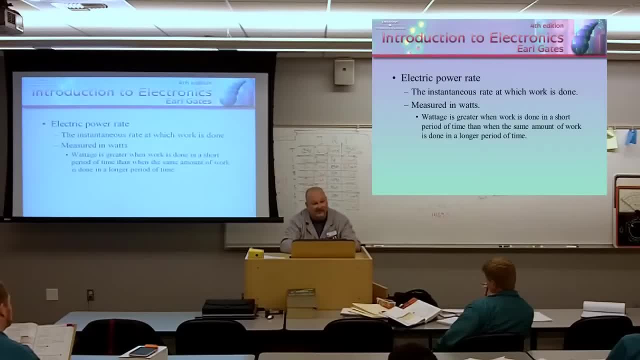 that fast, but they turn around and come back and they make some turns in between. so that's really amazing technology. but follow what I'm saying: drag racing. drag racing takes all of that power, couples it to the wheels, the tires, traction and acceleration, So they're consuming a huge amount of power and converting it into energy to get down the track. 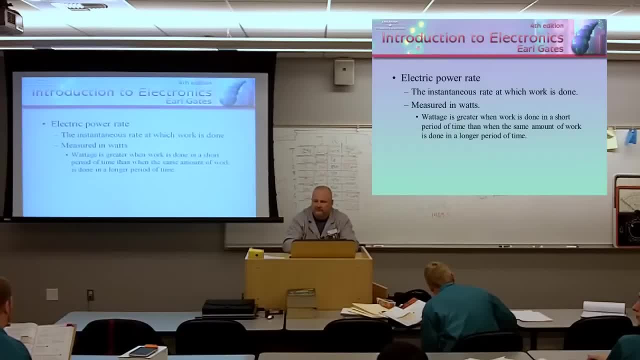 Would that be the same concept if you had a car that did 45 miles in one hour versus a car that did 80 miles in one hour, and you would be consuming more power? Absolutely, You could get there faster, Absolutely, And to get that work done in a shorter period of time, it's going to take you more power. 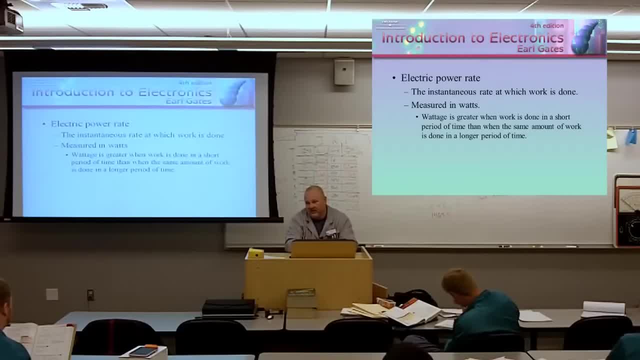 So that's one of the reasons that, with gas prices going up, getting off that pedal, it does make a difference. It does make a difference- The epitome for me, and it's a toss-up. It's a toss-up. NASA was involved in both of them, right? 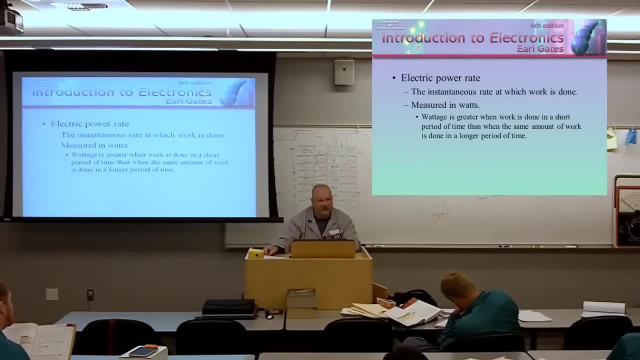 Space shuttle, Space shuttle or kicking it, old school NASA, the Saturn V rockets. Saturn V rockets: a little tiny capsule up on the top, big, huge, freaking rocket, Light it. The dude that lights it lights it and then goes like three miles away and goes into a concrete bunker. 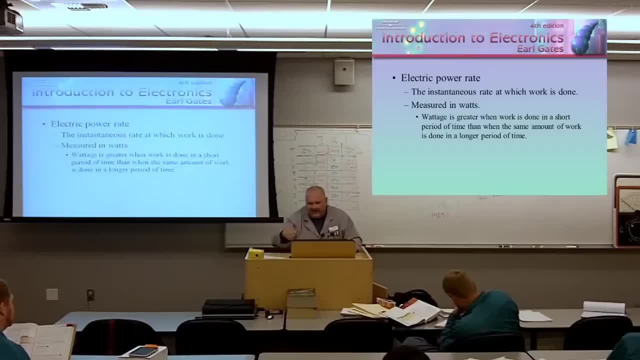 And then, literally with the space shuttle it's the same thing. they light it and then they like run three miles away and you know the thing goes off right. Seven minutes later they're in outer space. Seven minutes later, they're in outer space. 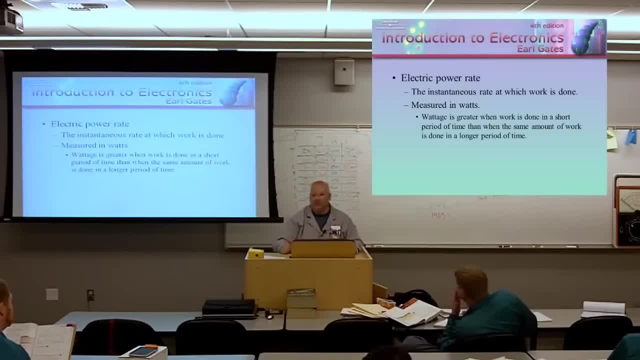 NASA throws power at the problem to get the space shuttle into orbit. okay. So obviously we're talking about if NASA could meter out that power, you know you could probably light several cities for a good deal of time. Instead they say: how can we get that power and concentrate it in liquid fuels? solid rocket boosters. 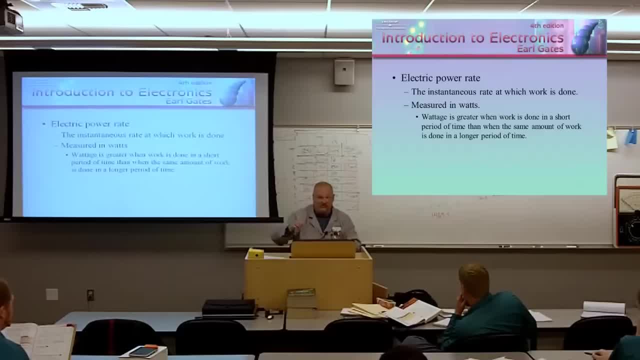 and then be able to concentrate that energy so we could get that space shuttle- which is freaking huge, it's a big thing- into outer space in seven minutes, Not eight minutes, not nine minutes, but in seven minutes they're in orbit. 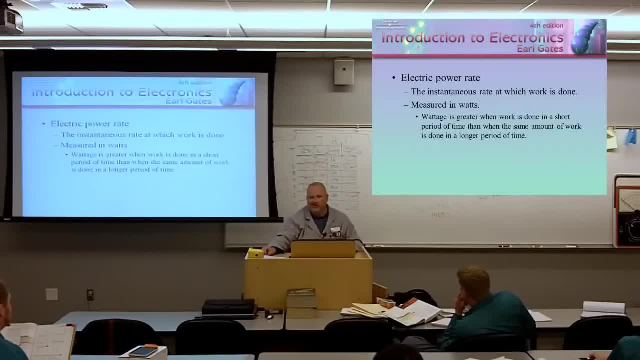 Tremendous amount of power. Have any of you here ever seen a space shuttle launch? Okay, I had the opportunity back in the 80s. I actually saw the Challenger, fortunately not the time that it had its malfunction. I saw it before that. 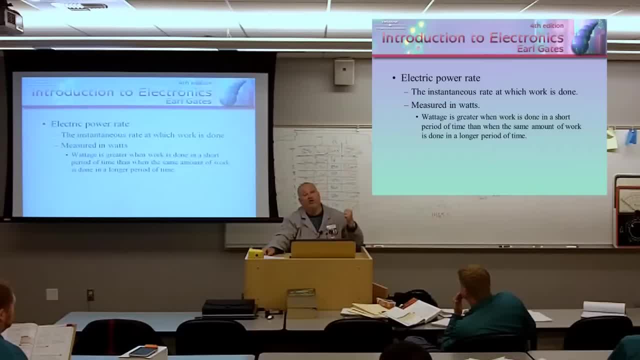 And actually, ironically, Dick Scully Toby, who's from Auburn, Washington. I saw a mission that he flew prior to the catastrophic accident that they had. But I was in Titusville, Florida, And you know you're listening to the radio and you hear the countdown and everything: three, two, one. 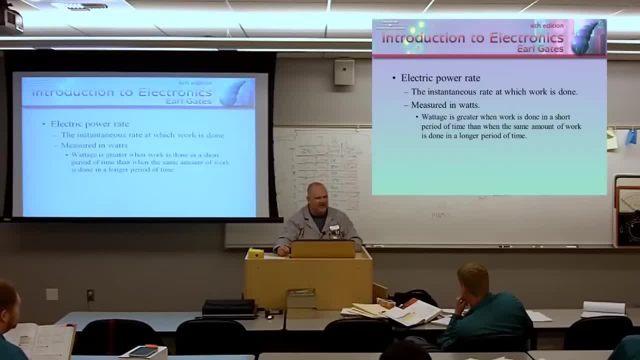 And you know, I don't know how many miles away you are- like 10 miles, 12 miles, You know, you see it going up, going up, And then all of a sudden the wall of sound hits you And it's just a sound like I've never heard before. 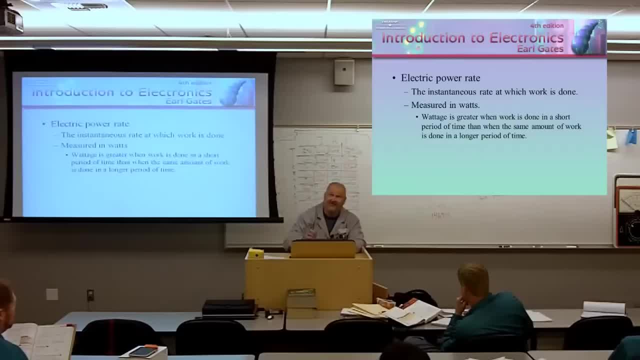 It's like, wow, that is freaking cool, You know. and next thing you know, it's gone, man, It's in orbit. They're in orbit, Orbiting around the Earth. Tremendous amount of power, Okay. 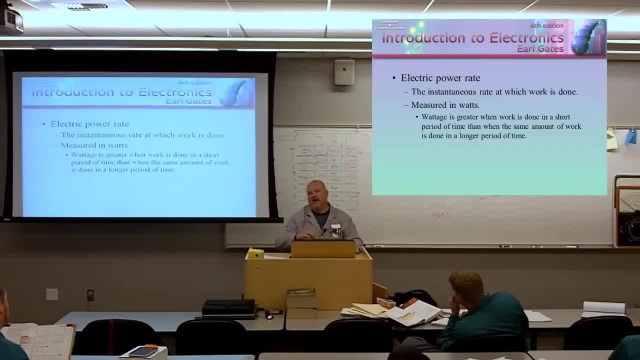 So it's the same thing with electronics. It's the same thing with electronics: The more power we throw at something, the more work we can do. So you know, basically, you know if you're attending a concert. you know the Pink Floyd Orchestra is performing in an auditorium. 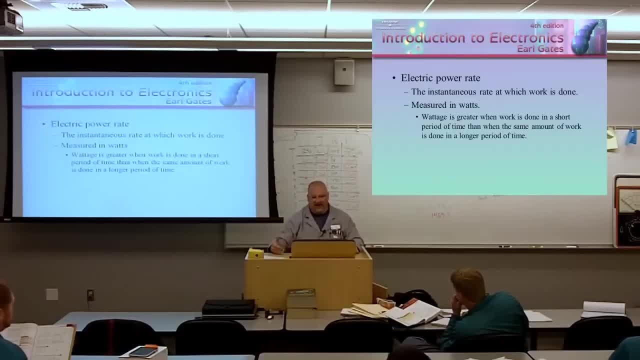 They are going to have to throw a lot of voltage and current at the problem to create a lot of power, To create a lot of acoustic energy, to satisfy the masses, Because that's what we've all grown accustomed to- is loud music Right. 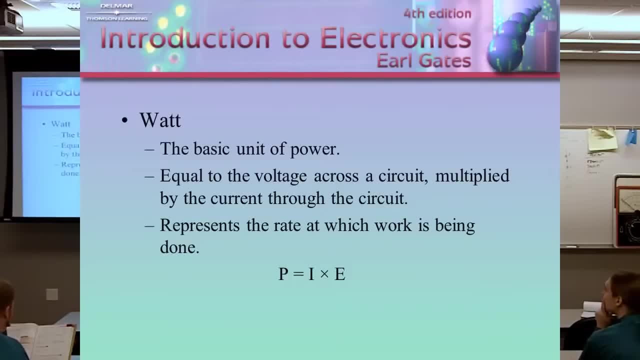 Okay, What is the basic unit of power? That is not a question, it's a statement. What, What is the basic unit of power? It is literally equal to the voltage across a circuit multiplied by the amount of current in the circuit. 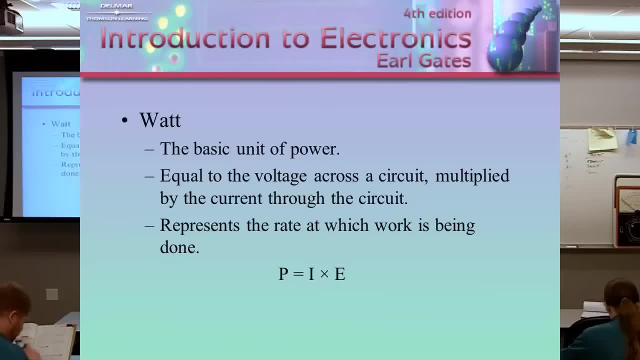 It represents the rate at which work is being done. And what is the guy that came up with it And what he said? I think he gave this presentation down at the Kingdome back in the day- 45,000 people. Ohm gave his spiel. 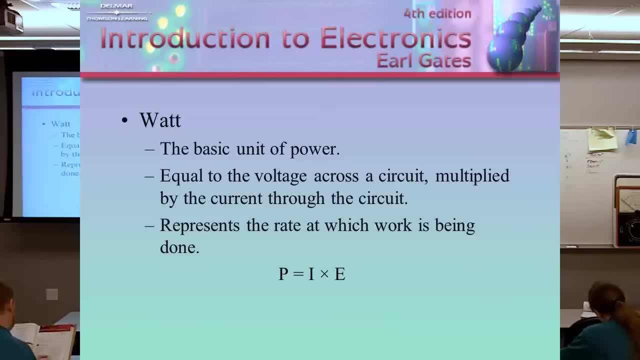 Right, Remember that V, V, V is equal, equal to I. I, I times times R, R, R R. Right, That was Ohm's deal. Watt got up there not to be outdone and he said: 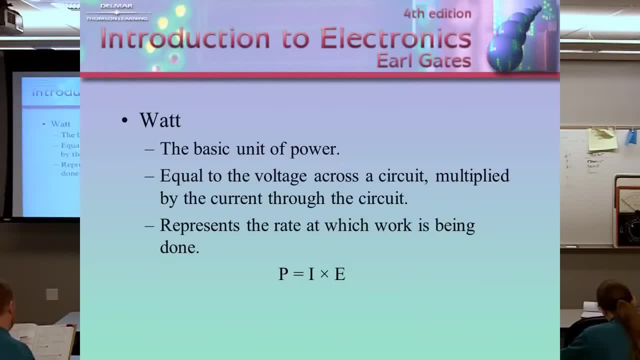 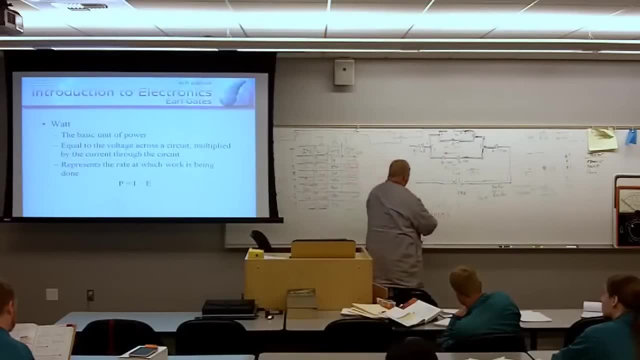 P, P, P is equal to, to, to, I, I, I times V, V, V, And that's what he said. That's what he said. So again, again, again, again, P I V. 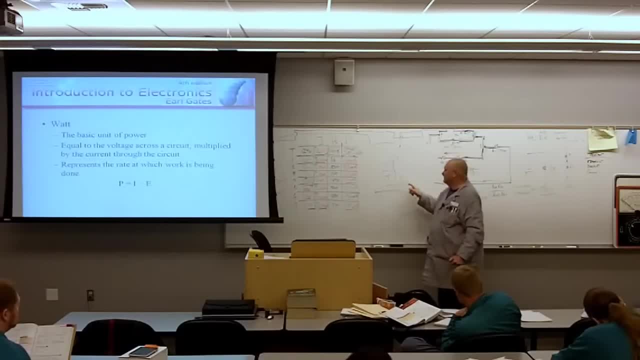 Triangle with a T in the center. Power is equal to voltage times current. If I ask you how much voltage is there and you know how much power there is right in current, then you can calculate out the voltage. If I ask you how much current is there, if you know the power and the voltage, 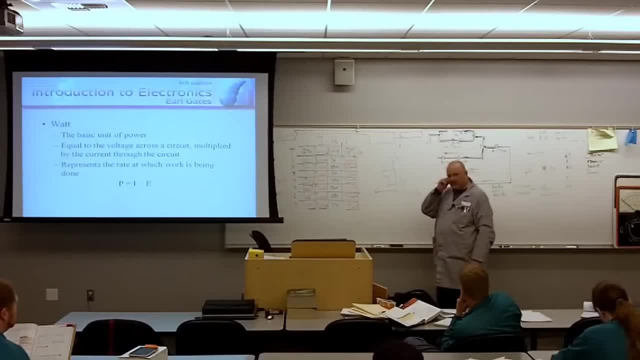 you can calculate out the current And, of course, power, current times, voltage. That's all your variables, Simple math, And this is called Watt's Law. Watt's Law. So so far for those of you at home keeping track of what's going down. 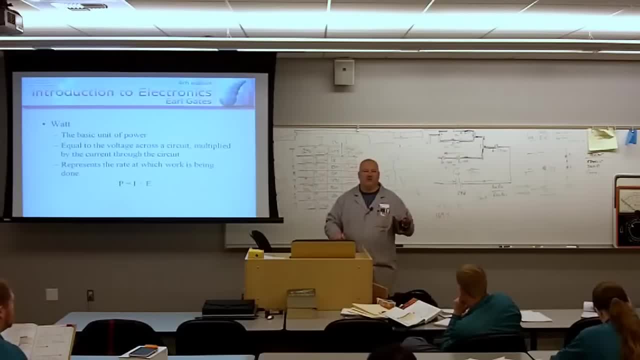 we've gone over Ohm's Law, we've talked about Kirchhoff's Law and this is Watt's Law. These are laws of physics. They allow us to calculate what's going to take place with 100% accuracy. Very, very useful tools. 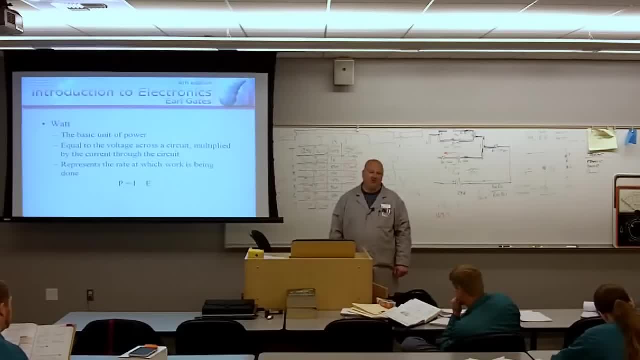 We're not teaching you this stuff because I've got nothing better to do with my time. We're teaching you this stuff because this becomes very valuable for an electronics technician. It paints a picture, tells you what's going on, literally tells you what's going on, okay. 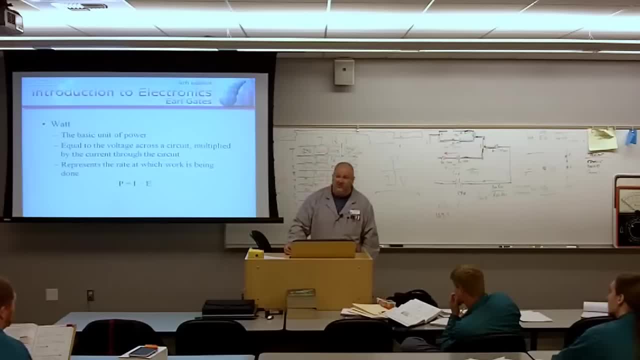 A little-known fact about yours truly. I used to work in radio. okay, I worked on the air. I was an on-the-air personality for an AM radio station in Connecticut And it was one of the things that got me interested in electronics. 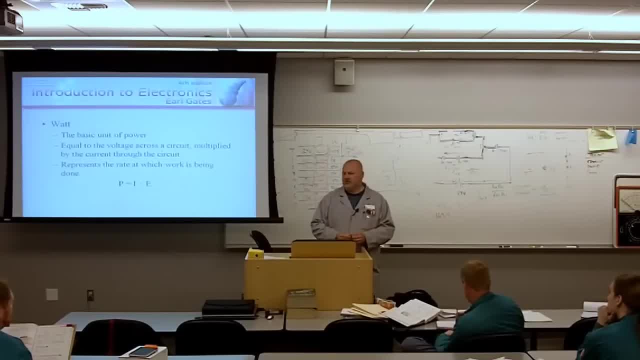 because I worked kind of hard and I didn't have a whole lot of job security. There was a guy at the station, the chief engineer. this guy. every year he'd have a new. he'd buy a Formula Firebird, trade in the old one, get a new Formula Firebird. 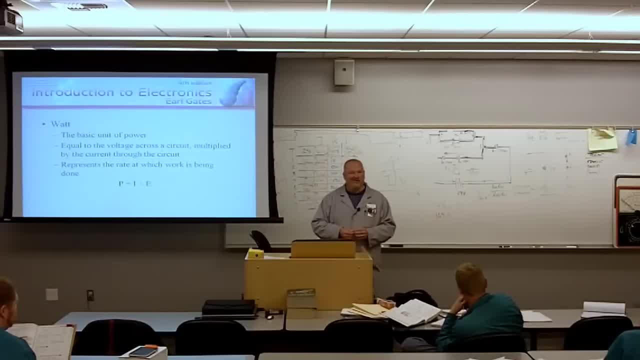 and he always kind of had a girlfriend with him that kind of had it going on, if you know what I mean. okay, And he did very little. He came every week to the station and he'd get all of the readings that all the on-the-air people took from the transmitter. 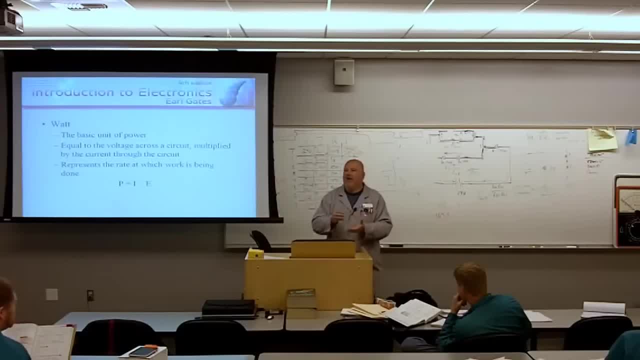 We were able to take the readings from the transmitter remotely, but we had to log in these voltages and these currents. And then he would say he would come, he'd come with a calculator much like this right, And he'd sit there and he'd perform these calculations all the way down. 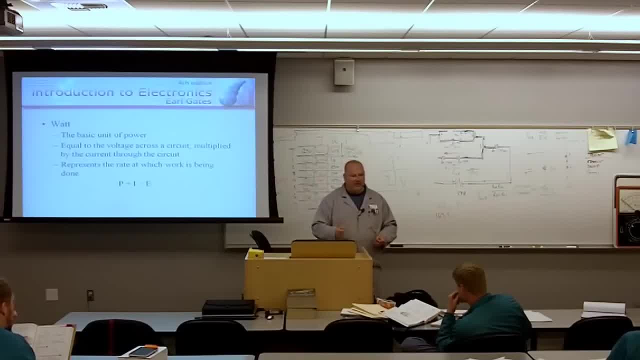 and then he'd sign the logs, take them, stick them in a folder and then they'd be held by the station. What he was doing is that the station- commercial station- was licensed by the Federal Communications Commission to only broadcast so much power. 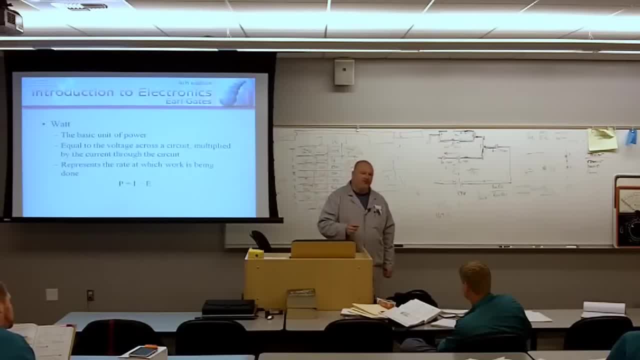 And the proof of how much power was being transmitted was the voltage of the final transmitter tube, the current flowing to that transmitter tube. If you knew those two, you could calculate out the power. And then there was approved engineering design criteria for the antenna system. 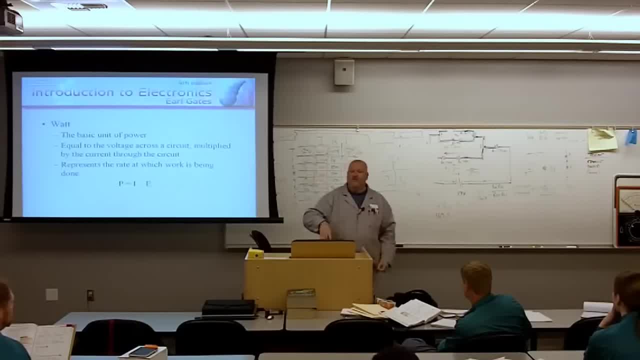 that the antenna system had certain number of losses. so you could prove to the FCC. you see, we were not broadcasting more power than we were allotted, We were not interfering with that station in Pennsylvania. okay, We couldn't have been, because we were only broadcasting power. 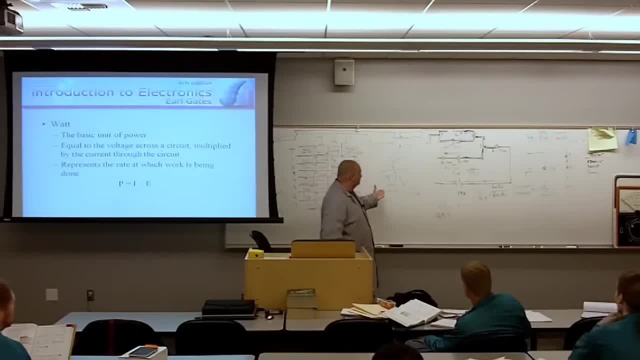 We were only broadcasting out what you've allowed us to broadcast out. So, as a technician calculating this out through the current and voltage readings, that I think it was every four hours, we had to take Every four hours on-air personnel and it was right there in the studio. 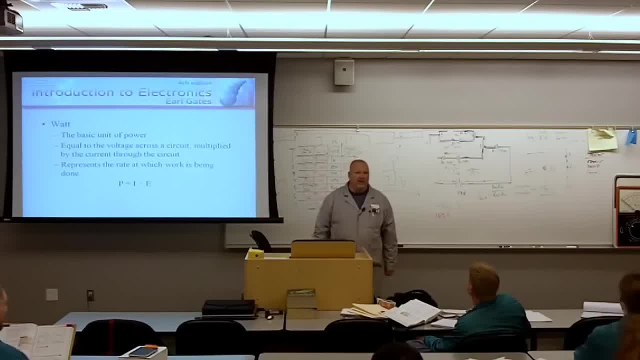 It was an equipment rack and you could go and just sequence through, you know, and take the voltage readings, the current readings, and log those in and that became part of the permanent record. So it was kind of funny. The. 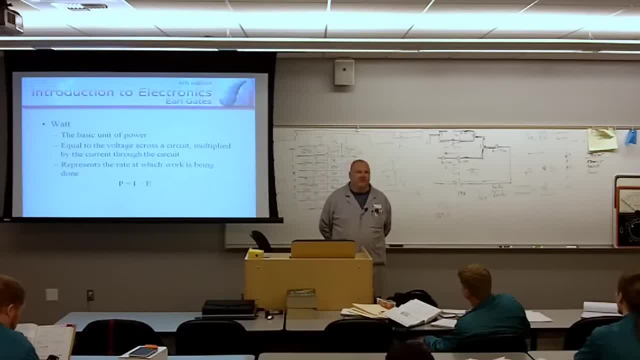 It really was inspirational for me seeing this guy as the chief engineer. He was a chief engineer and he was assigned several radio stations in Connecticut on contract. Guy made really good money, you know, and I'm like: how do I get his job? 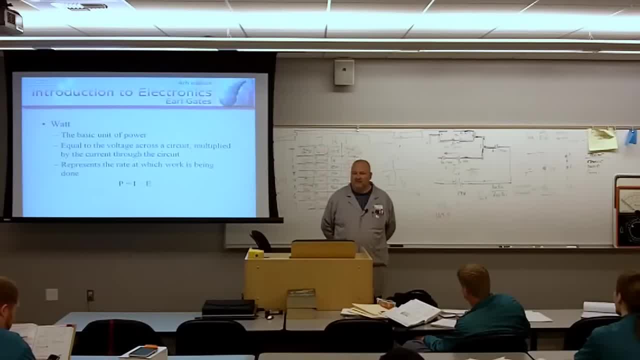 Well, you need an FCC license, you know, basically the general radio operator's license, to be able to maintain a commercial radio station like that. So, anyway, I'm an examiner now for the FCC and I give that exam and I've never in my life owned a Formula Fire radio station. 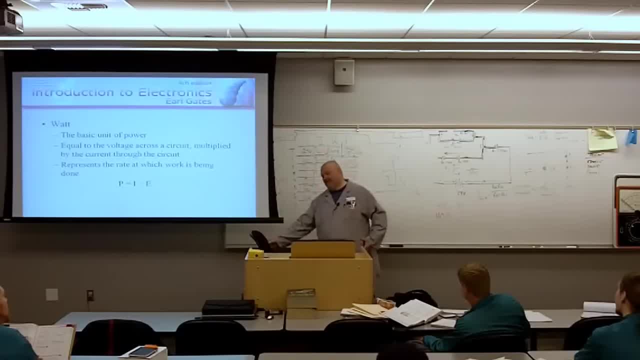 So I have had some girlfriends that kind of had it going on, if you know what I mean. It sounded like a pretty easy job he had, though, huh, Until it hits the fan, Until the station gets hit by lightning, okay. 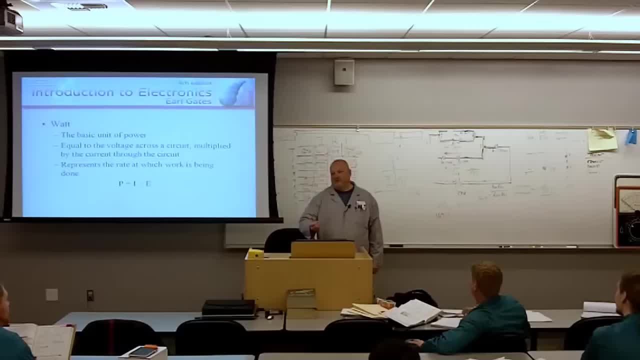 And then it's like ugh. And then you got the general manager right, the program director and all of that advertising dollars that were spent right. you're losing that money because the station is off the air and that's how stations pay the bills- is all the advertising. 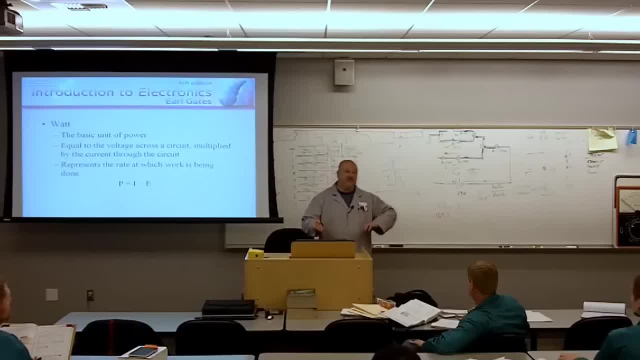 So when you're off the air, you're in a pickle, People will tune to another station or whatever. So it's kind of a big deal. Ironically though- kind of behind-the-scenes story like here- we had a woman in our program that completed this program. 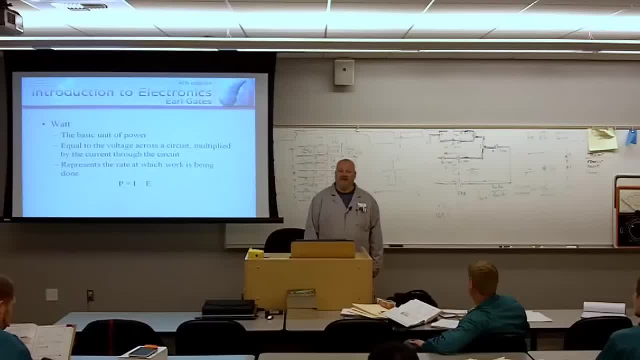 and I got her an internship. She interned for a period of time at KISW And the engineer at the time over there, Brian, he hadn't had a vacation for three years because, again, as a chief engineer, you just don't go on vacation. 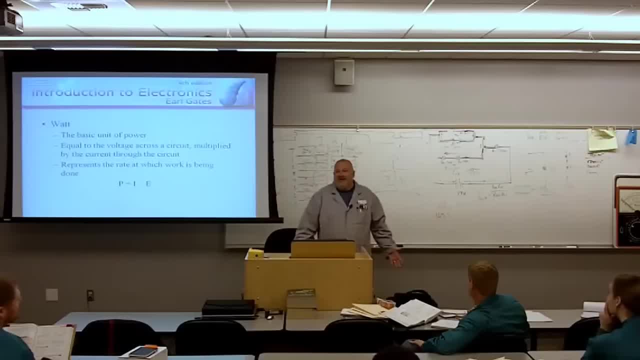 Yeah, I'm taking my vacation next week. You can't do that because if the station goes off the air, who's going to you know? So there was nobody that he could hand the station over to Once she got in there and she built up some credibility. 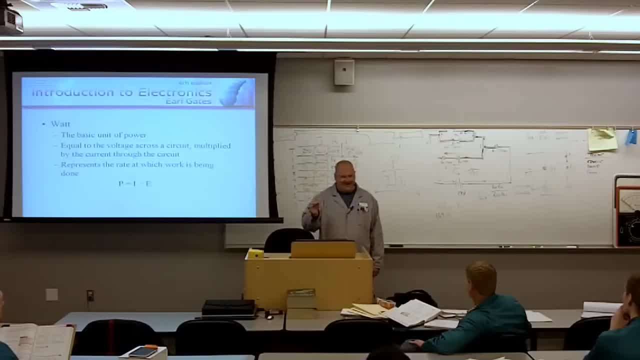 he actually went on vacation and gave her the keys and it's kind of like, hey, you've got it, You've got the stations. She was a student here at Lake Washington Technical College. She was the acting chief engineer for KISW. 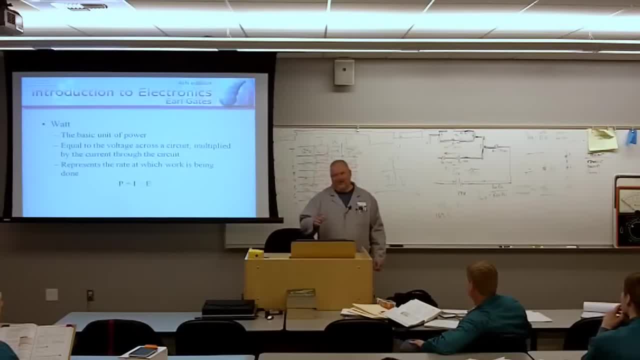 Okay, Also also because all these engineers and all the radio stations in Seattle, they're all in cahoots with each other. okay, So if the station goes off the air, you know, call Tony over at Cairo. 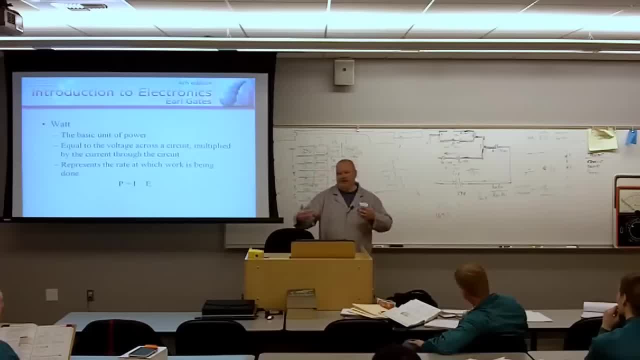 He'll come over and help you out. You know you've got all these engineers that will lend a hand, even though you're the competition on paper. If I need something, you'll help me out. If you need something, I'll help you out. 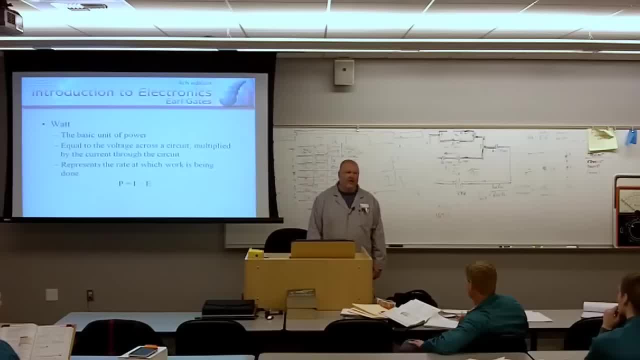 And it kind of goes: it's a you know unwritten law, if you will, in radio to help everybody else out, So kind of exciting. So anyway, This power reading is very, very critical so that you could tell the performance of your equipment. 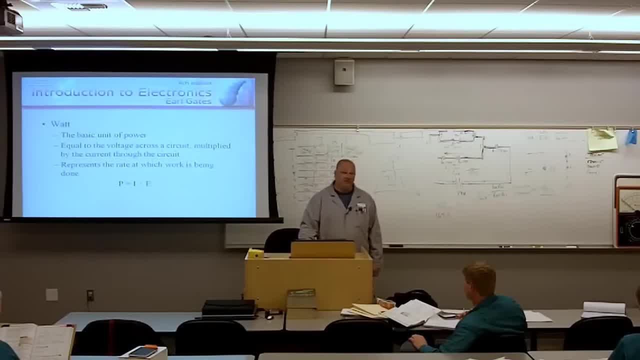 And it's something that, if any of you go into commercial broadcasting, you're going to be doing the exact same thing: taking those power readings. How much energy are we getting off the antenna? The only way of telling is how much voltage you've got. 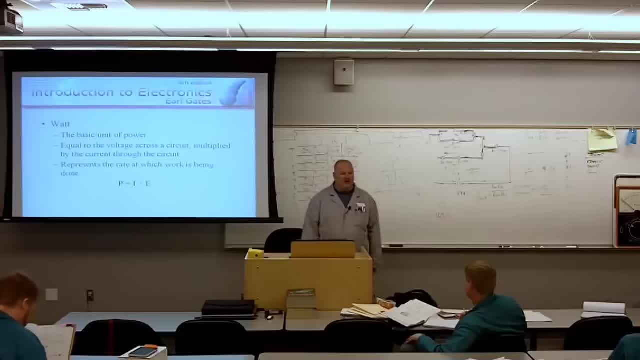 how much current you've got going. Same thing You come from an audio car, audio background. same thing. You've got a 1,000-watt amplifier. It's a math problem. okay, 1,000 watts. you know what this is okay. 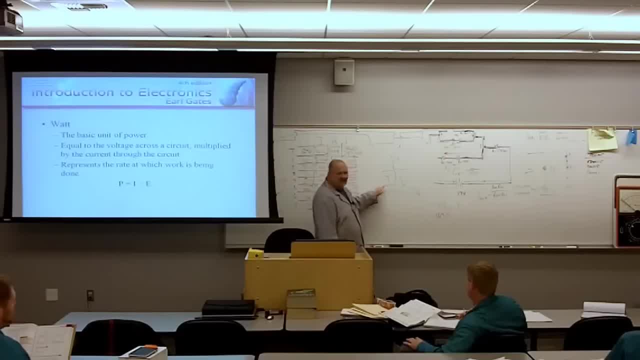 12.6 volts DC. You know what this is? Well, this is going to tell you how much current it is. It's a math problem, you know. Now it's 1,000-watt amplifiers. That's peak performance. 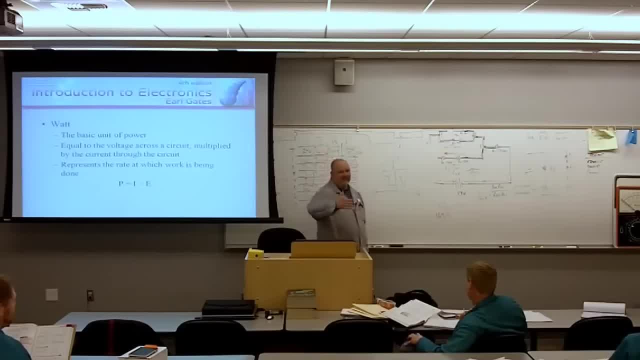 And how often are you going to be cranking out that peak performance? But you've got to design everything backwards to make sure that if you crank it up all the way, you're not going to cause an electrical fire and subsequent meltdown. So you've got to design. 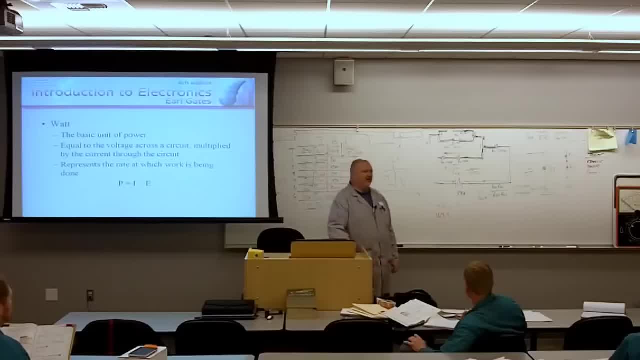 And it all integrates. Really, it's a beautiful thing. Now, the electric company, The electric company, I like that. The voltage company, The voltage company, They charge you, They charge you for kilowatt hours, Kilowatt hours. 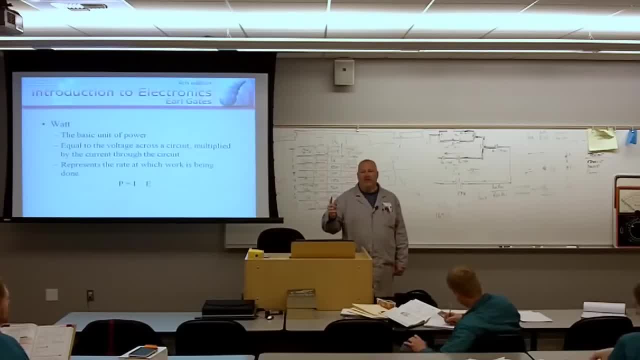 That's 1,000 watts, a kilowatt right per hour. So that's you consuming 1,000 watts over an hour. okay, I don't know if any of you go to the gymnasium periodically. the gym workout. 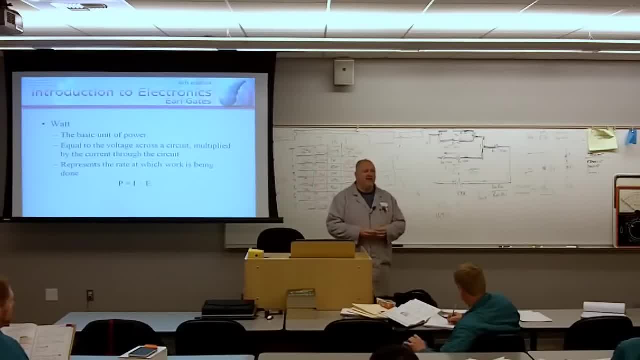 Some of the life cycles, stair-steppers, these things. some of them have integrated in calories that you're consuming. Some of them have a screen that you can go to for watts. okay, So I often thought I hate working out. I really do. 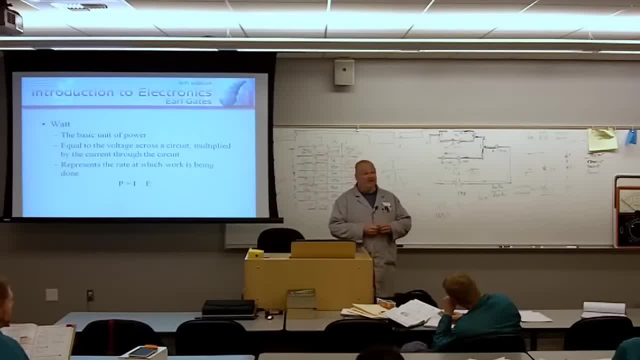 I'm not afraid of hard work. If I got to dig a ditch in the backyard, I love doing it. I'm all about hard work, But going to the gym for an hour just doesn't make sense. At least put the thing up to a generator. 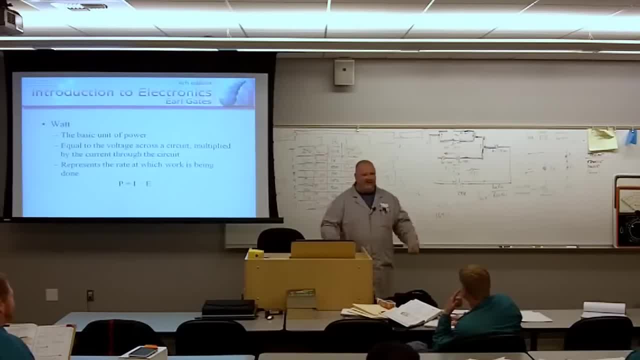 Let me charge my cell phone or something, Let me save a nickel or something. That makes more sense to me. But anyway, some of these screens have watts And if any of you have ever done that, how hard you have to work to generate a watt, I mean it's amazing. 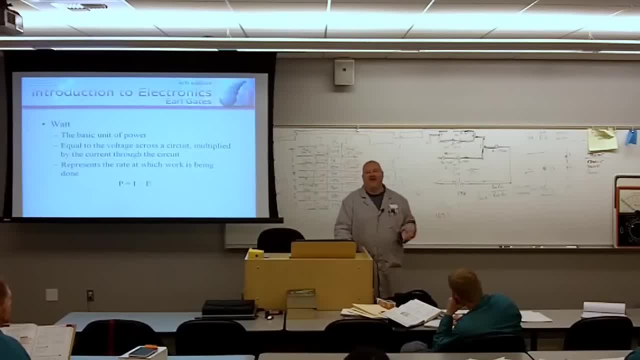 So the electric company, the voltage company, is selling us 1,000 watts per hour. That's the unit of measure that they charge us. okay, Does anybody know off the top of their head about what we're being charged here in the greater Seattle area? 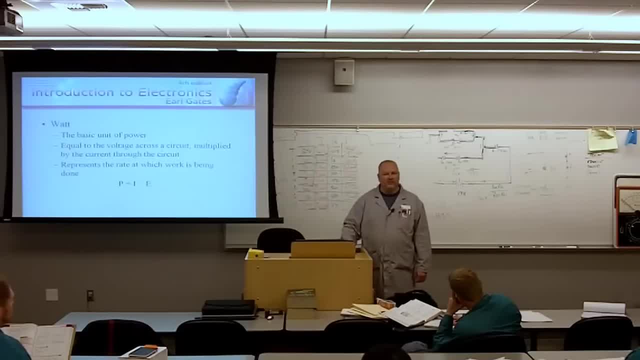 per kilowatt hour. Zzz, Wait, You're being ripped off, man. That's Greenick power and light- About $0.08.. About $0.08.. Some of you, depending on your scale, $0.065, $0.07 per kilowatt hour. 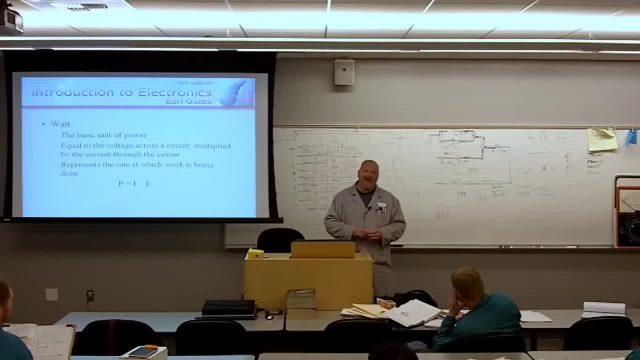 which is the thing that I kind of struggle with. I go this year alone. since January I got invited to attend a green energy conference- Good Jobs, Green Jobs- in Washington DC, And then I went, And then I was invited to be a guest speaker in Milwaukee. 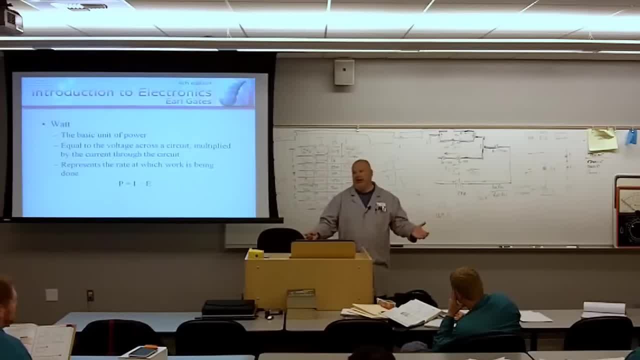 at the Green Summit. So I'm some world-class speakers I get to be in the presence of. So I go to this like Green Summit in Milwaukee and I get seriously jazzed. You know like, yeah, I'm going to go home. 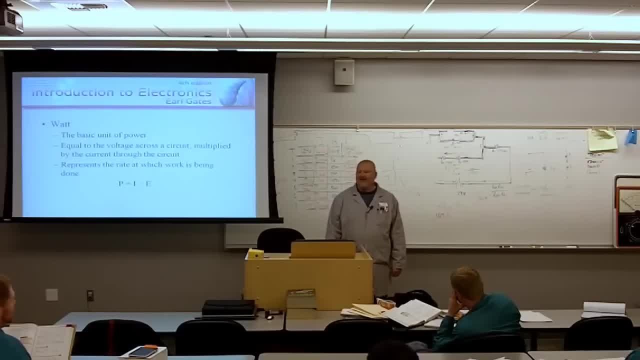 and I'm going to do an energy audit. I'm going to see, But I get lost. I don't get lost to make $0.065 per kilowatt hour. you know How much effort do I have to put into really saving? 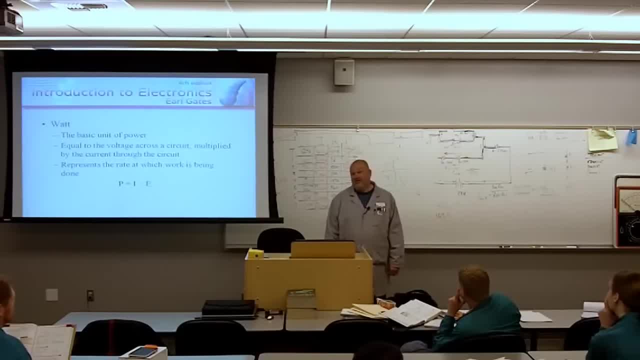 How much am I going to save? It really doesn't make sense. It really doesn't. There needs to be consumer incentive for you to really hunker down and save, because electricity here in the Northwest is very, very inexpensive And that's a good thing. 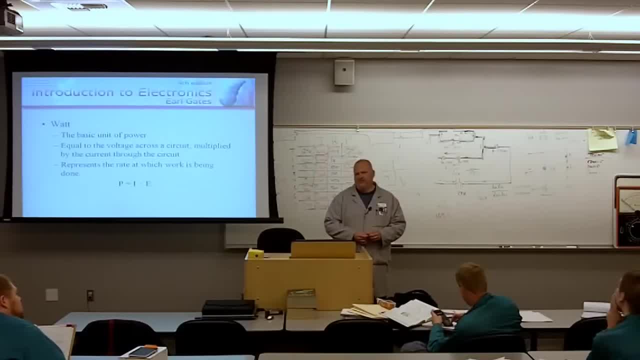 I'm not complaining about it, You know, and there are some things that you could do to save energy, but there's only so much that you could do and we're really not paying that much for it, Even like with electric cars. I know my colleague did some of the math with purely electric cars That we're coming out with And really it equates for the price of gas at $4 a gallon. it comes out to being that it's about 99 miles per gallon. that you would get equivalent to travel 99 miles than it would cost you for that fill-up, And that's about what it equates to when you're paying $0.065, $0.07 per kilowatt hour, which isn't bad. 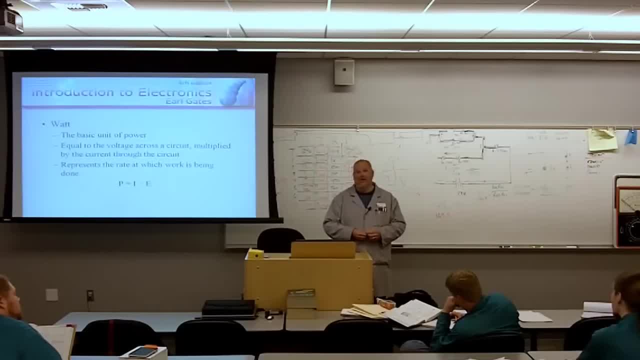 You know, I wouldn't mind having a car that got 99 miles per gallon, 100 miles per gallon, But is it worth the investment Of me scrapping my- you know my- V8? I mean because I don't. 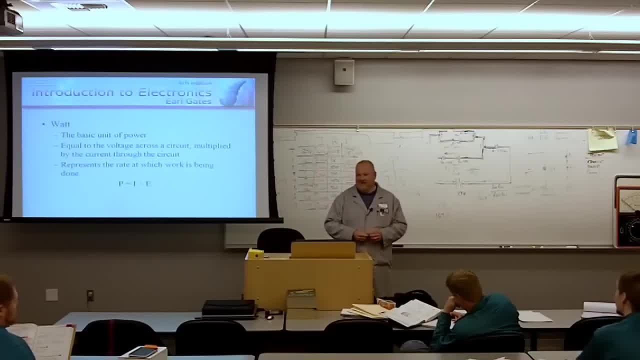 Unless I'm driving a Tesla which is out of my range. you know, I don't think I like that V8. You know, V8, Taurus, Pour some fuel into the situation. a little bit of air, Get out of the freeway. 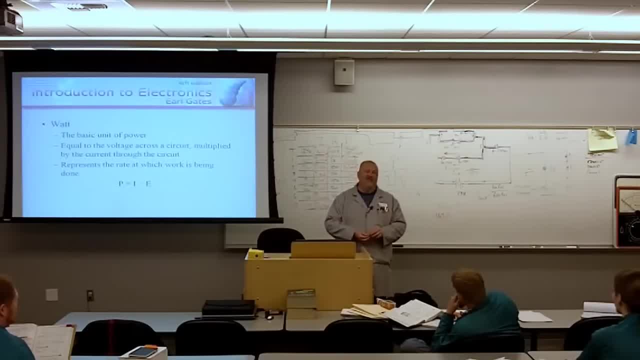 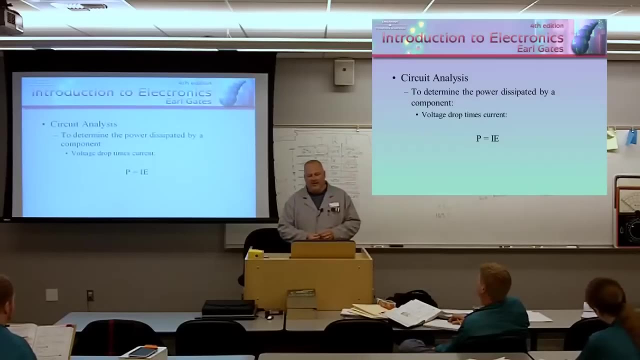 Set the pace, Not keep up with the flow of traffic. Set the pace And I have documentation from Washington State Control that will test that out fast. Okay, Circuit analysis To determine the power dissipated by a component and the voltage drop times current. 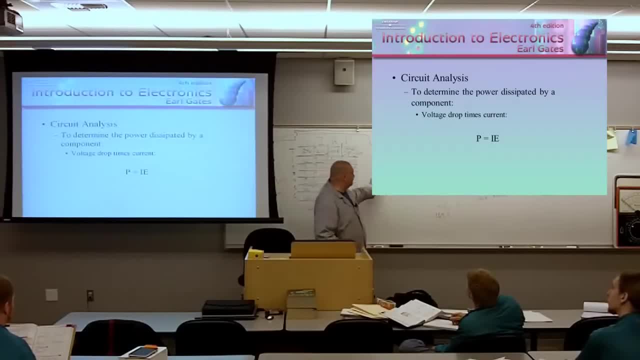 So I'm thinking about for a component now. Okay, This works for loads, This works for, like, an amplifier: If you've got an electric load, an amplifier, A transmitter, you could do this. But this also works for individual components. 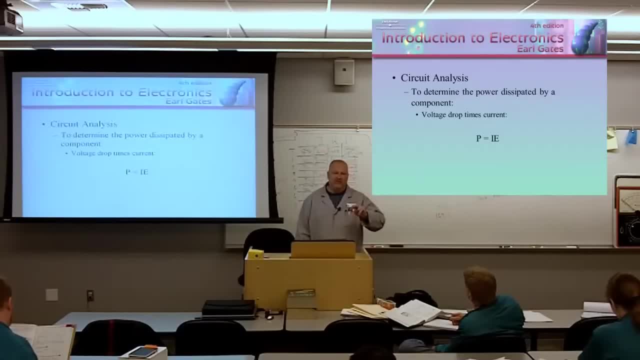 So if you know how much current's going through the component and you know the voltage across the component, then you could figure out exactly how much energy that component is dissipating. Now remember resistors, Remember resistors. Resistors are devices designed. 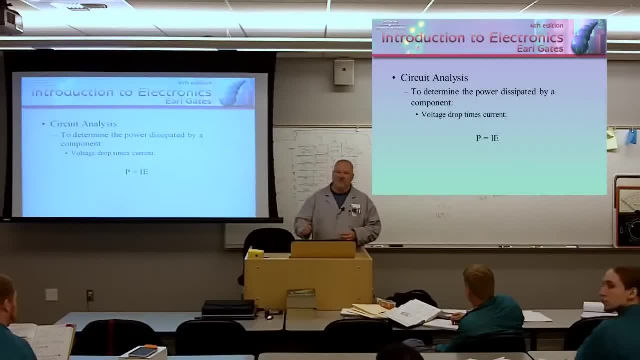 to possess the property of resistance. Resistance is that force which opposes the flow of electrons, The byproduct of resistance. when current encounters resistance, it generates heat. That's how we determine the power of that resistor, Because all resistors are not created equal. 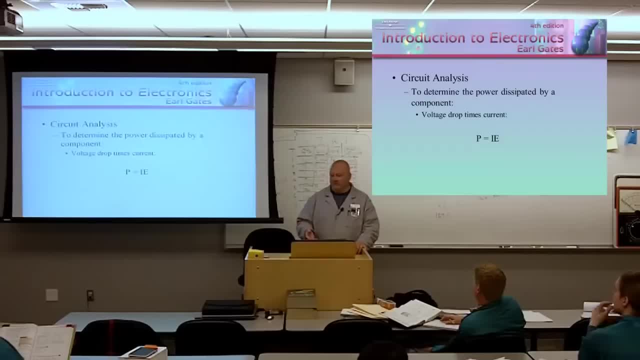 There's eighth-watt resistors, quarter-watt resistors, half-watt resistors, one-watt resistors, five-watt resistors. How much energy could they dissipate? And literally, literally, it's the voltage across the component. 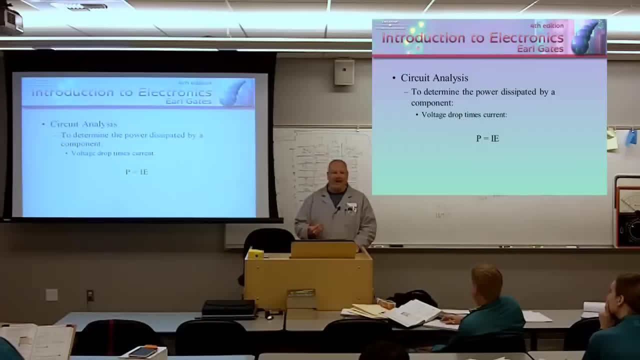 times the current going through the component that's going to give you that power that's being consumed by it. If a resistor, if you ask too much of a resistor, it will fry. It will fail If you exceed its rated capability. So all electronic components are really like that. 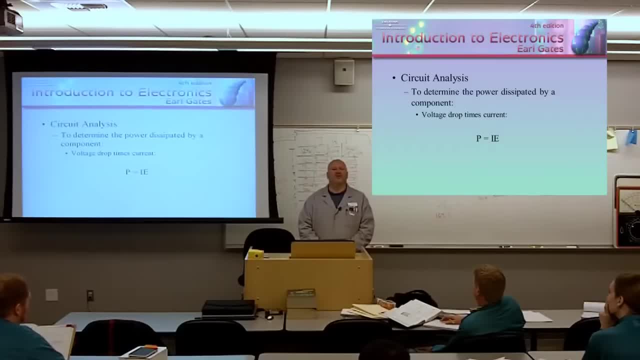 If you know the voltage, you know the current. We're going to talk about some exceptions in the future. They're not resistive components, They're called reactive components. They'll come later this quarter, We'll talk about that. These are components that don't consume energy. 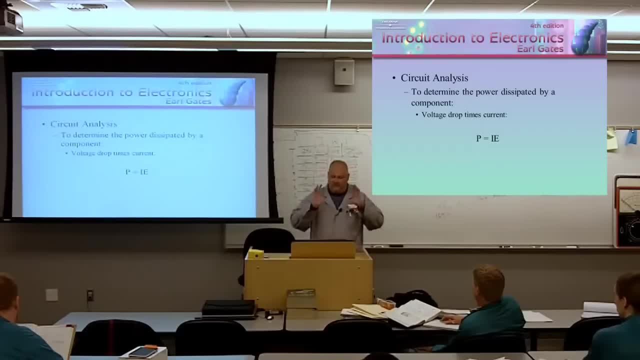 in the form of heat. That's why they're called reactive, Something we'll talk about in the future. Hey, the neat thing with power: power dissipated in series or parallel is equal to the sum of the power dissipated by the individual components. 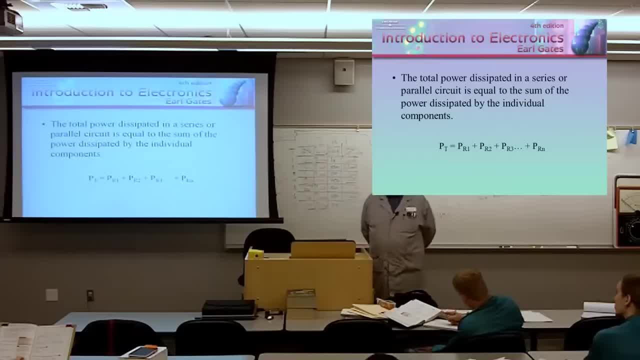 Power is always additive. It doesn't matter if it's series or parallel or whatever, Power is always additive. If I've got a 400 horsepower engine on my airplane and I remove it and get another 400 horsepower engine and mount each engine on each wing, 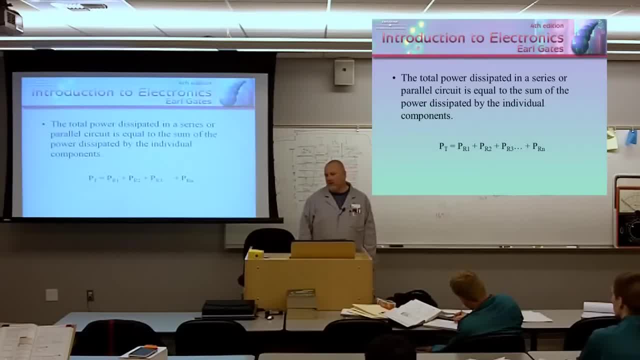 now 400 times 2 is I'm up to 800 horsepower worth of power, As where before, in a single engine aircraft, I was only up to 400 horsepower. Okay, It's kind of funny. I know a little bit about airplanes. but the odd thing about airplanes is when you do that, instead of the airplane costing twice as much, it ends up usually costing you about three times as much. So for a twin engine airplane, you're going to pay through the nose. You know much higher performance. 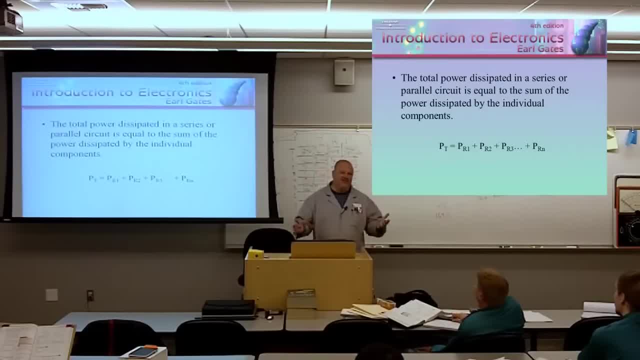 a lot more going on with it, a lot more structural that they have to do. But power is always additive. That's why the space shuttle right Solid rocket boosters on the space shuttle right They have two. You know how much power that is. Twice as much as one. Okay, That's why they put two of them on And actually, from what I understand, I think the space shuttle can. I don't know if it can get a shallow orbit, if it's just on one solid rocket booster or not. 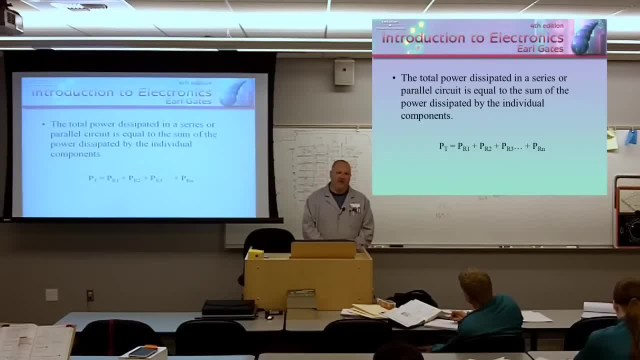 But those things are literally like Roman candles: Once they light up, they're going for a ride. There's no shutting them down. Uh-oh, we changed our mind. Let's back it back to the pad. now You're going for a ride. 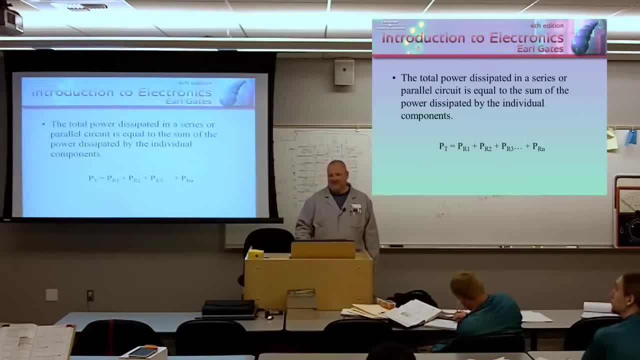 Power. So power is always additive, Always additive. This is the thing like with your Hummer. Forget about what I said. Energy conservation: a bunch of hoaxes in your home. Every device that is on in your home right now that has a voltage across it and current flowing through it. 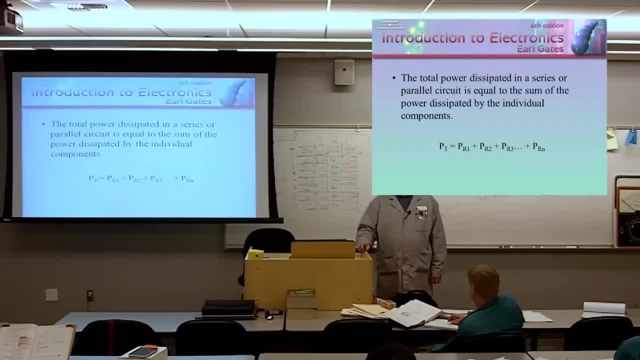 is consuming power. Okay, There's a lot of phantom loads in your home- Stuff that's plugged in but it ain't turned on. but it's still consuming power. Why You got voltage across it. it's got a current flowing through it. 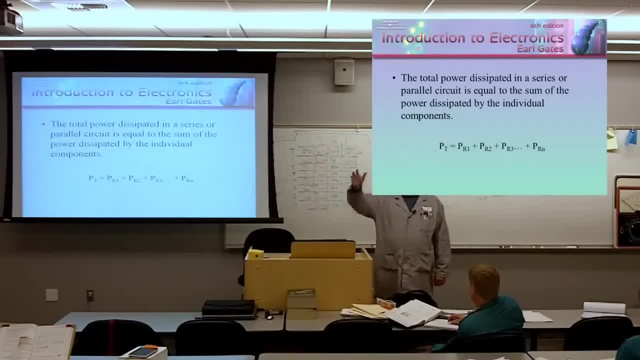 Your plasma is going to go up. How many of you have a nice flat screen TV at home right? How many have it? is it turned on right now- You leave it on 24-7- or is it turned off, Still consuming power? 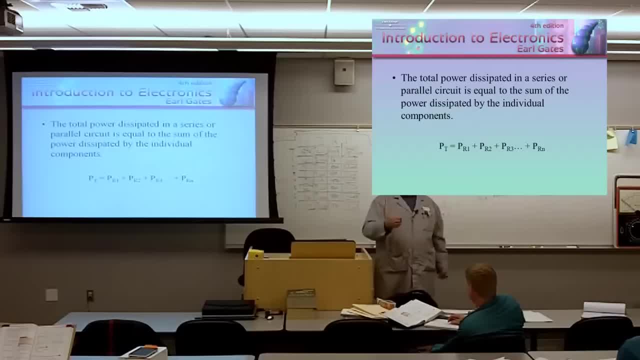 Still consuming power. So that way, when you go home and hit that remote, pow, that screen comes right up. If not, there'd have to be a period of time with some electronics for it to warm up. come up. Everybody wants instant gratification with systems. 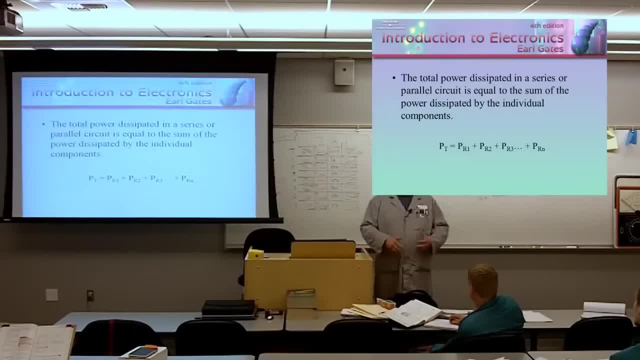 Especially some of the old tube systems. right, Those really consumed a lot. You had to wait for the tubes to heat up and everything. But most electronics are really in a standby mode: Your battery charger right now, your cell phone charger at home, 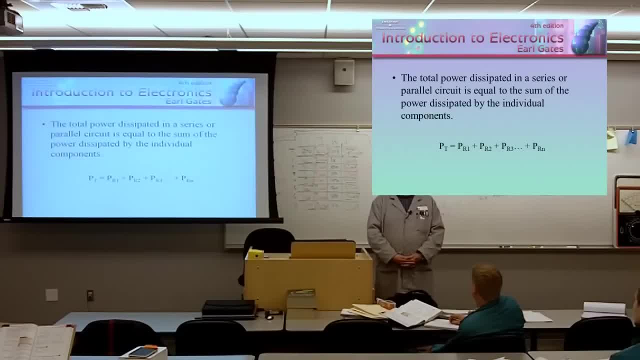 if it's plugged in the wall and it's not plugged into your cell phone, it's still consuming some energy Because it's got current flowing through a coil there. When you plug in your phone, it consumes more current, right? So a lot of these again are phantom loads that exist in your home. 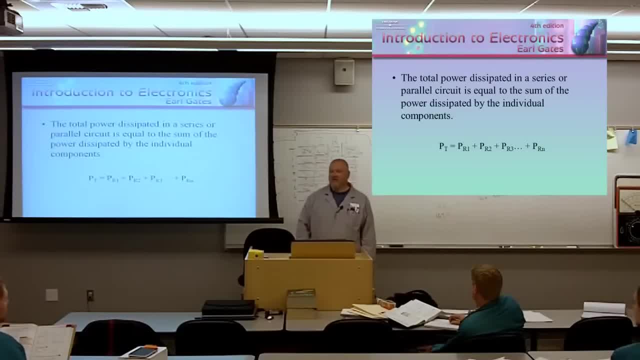 You're consuming energy, A real small amount, But it all adds up, It all adds up. You know, Actually, one of the things I can give you a sales pitch for tomorrow's meeting, where I can watch a documentary called Power Search. 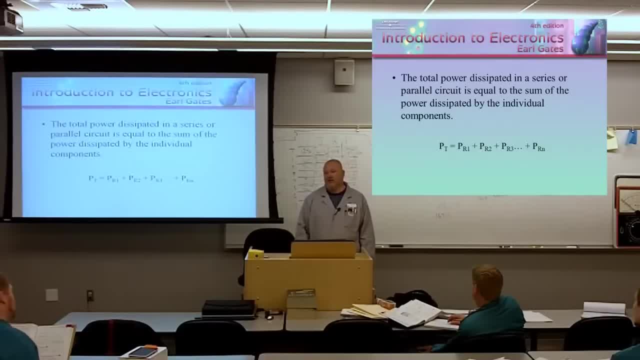 that was just done on public television. They talk a lot about that. You know it all adds up. It's all about power. You know How? about the lady that unplugged everything in our house for a month? Oh, I didn't hear about her. 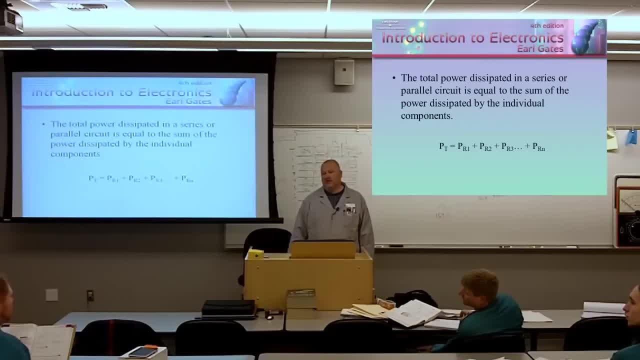 As soon as she was done using it, there was nothing that was plugged in. Did she save money? Yeah, Really A decent amount. yeah, I can do that. All my plugs are like behind the couch and crown. I'm going to climb back there. 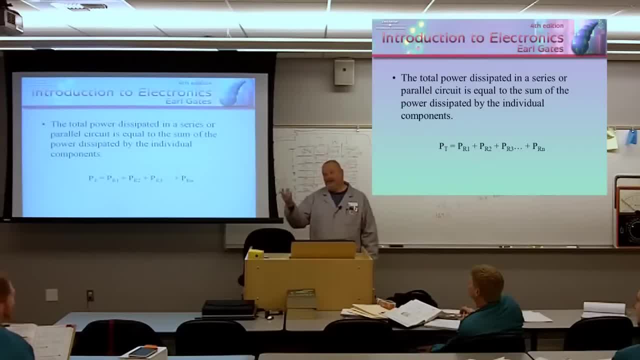 It's all a power strip with an on-off switch. You know that's it, In all honesty, that actually I thought about that. You know my wife and I travel a lot And we, you know, we go away. And it really would make sense to shut off that main breaker of the house. You know, Leave for a month, Come back And then, you know, you go get your electric bill And they still charge you the same, You know. 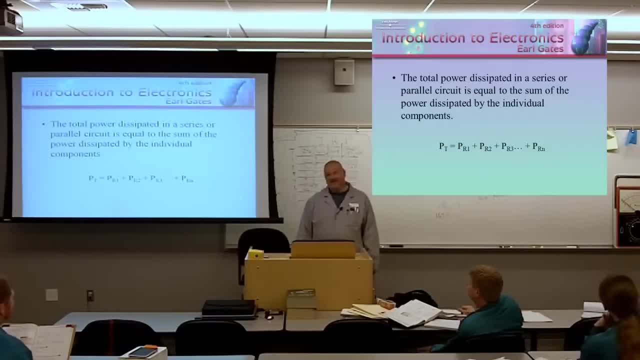 They're just messing with you, man, They're just messing with you. You've got to have your ducks in a row. You've got to pay attention to that meter. So Now, in electronics, the power dissipated in a circuit is often less than one watt. 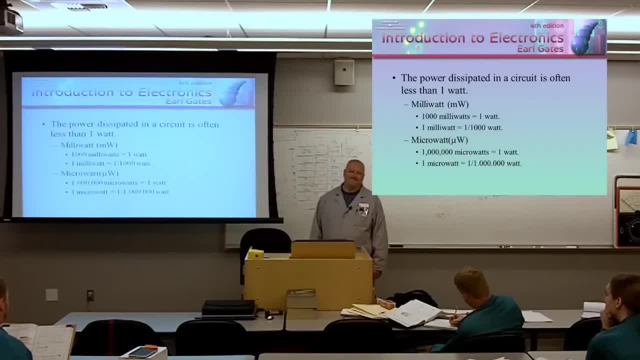 Electronics, microelectronics, like you're studying here. typically, the value is going to be less than a watt. Typical values will be the milliwatt, This is times 10 to the negative third or one thousandth of a watt, And the microwatt. 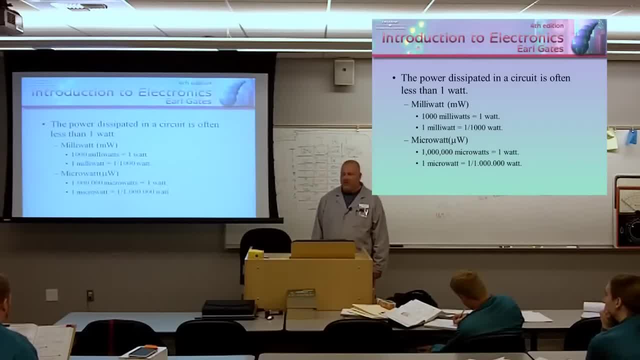 Okay, One million microwatts equals one watt, So we're talking a millionth of a watt. That's typically what's consumed in microelectronics, So it's not going to be energy being consumed. Some of you are playing around with amateur radio. 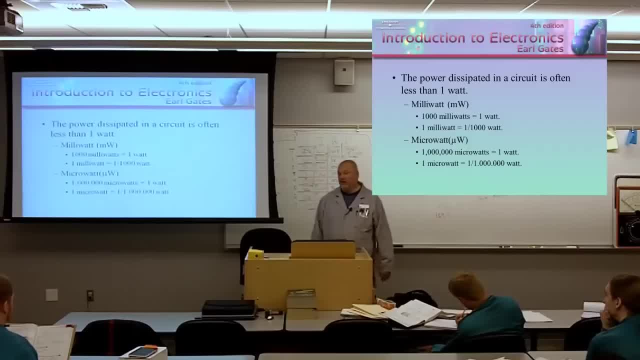 You want to get your amateur radio license and play around with some of that stuff- Some of them are power transmitters- You need to make sure you have the available current. You're not going to be able to do that Because, again, 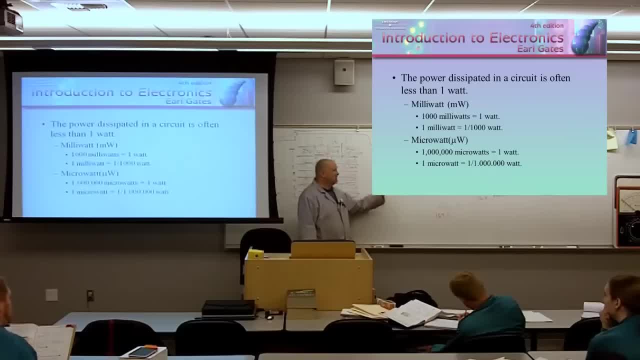 You're going to hear behind me lie. Power is equal to current times voltage. So if you're on a low voltage system, Like car, Like a car or a boat or an airplane, And you want to start jacking this value up, 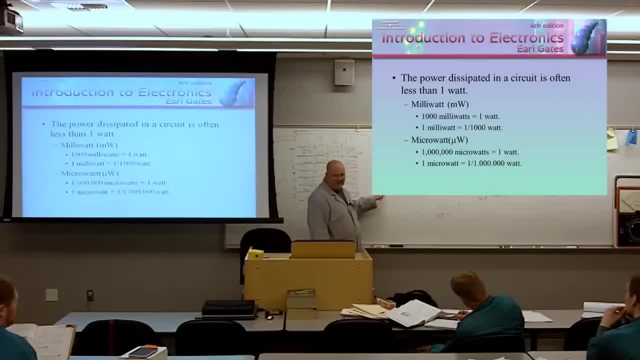 That means you're going to have to start using a bigger cable, A physically bigger cable, Because you have more electrons that you're going to have to transport from the source to the load, And that's what you're measuring. Okay, So the math doesn't lie. 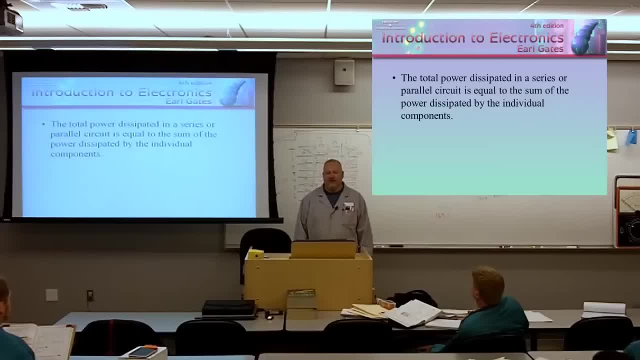 Total power dissipated in a series or parallel circuit is equal to the sum of the power dissipated by the individual components. Meaning: power is additive, Power is additive. There's no such thing as negative power. But this is putting power back in. 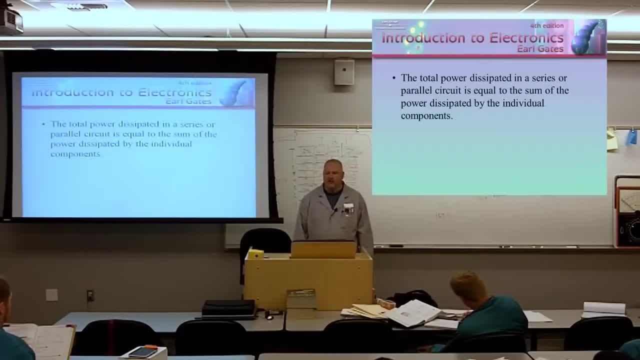 Perpetual motion machine. You get something like that going. Give me a call. Okay, Give me a call, I'll have my attorney contact your attorney And I'll personally fly you to Bimini And you could watch the sunset drinking out of a coconut with one of those screwy straws. 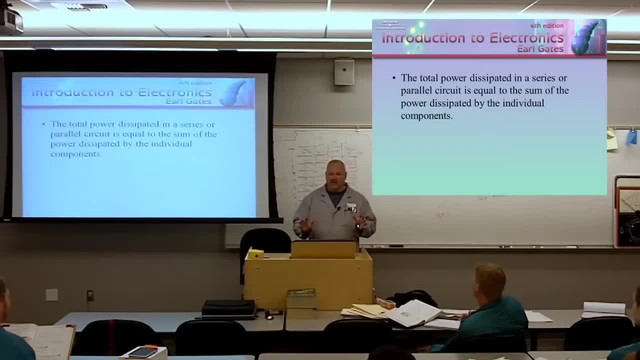 An umbrella on the top of your drink. Okay, Now all we do is consume. We consume power. Nothing puts things back in, So it's not. I guess it would be like me getting an airplane engine. You know, mounting one. 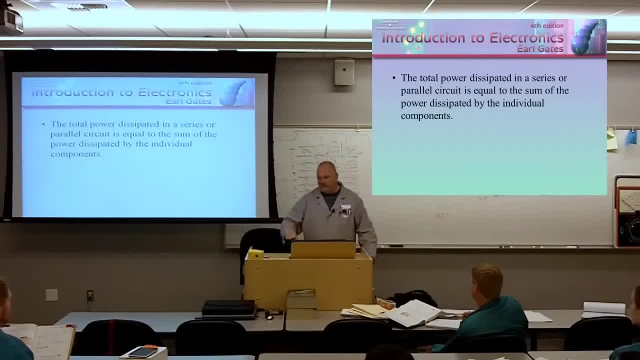 Like going this way And then the other engine going this way. You just sit there, You know, Then they're flipped off. You know It's a UFO now. It's a doofus, It's a doofus. 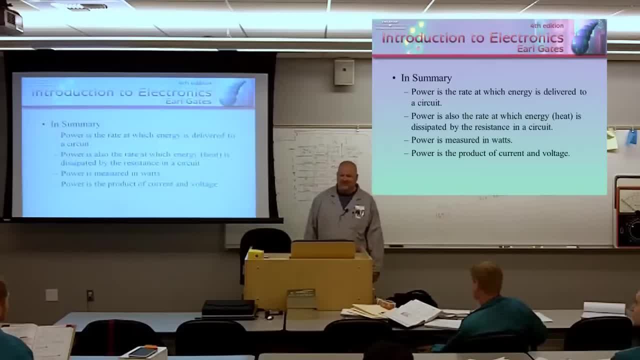 What's that guy doing? That make sense? All right, Summary: Power is the rate at which energy is delivered to a circuit. Power is also the rate at which energy or heat is dissipated By the resistance in a circuit. This isn't. 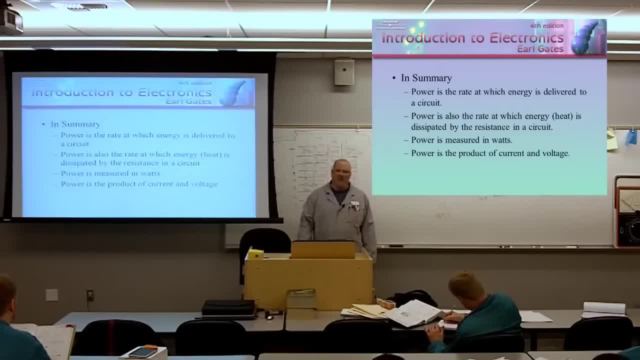 That second bullet statement there. there, It isn't something we dig, It's something we've got to deal with. We don't want our electronic equipment to get hot. It's one of my problems. I've got a lot of electronics in my family room. I've got my audio, I've got surround sound, I've got my plasma screen. 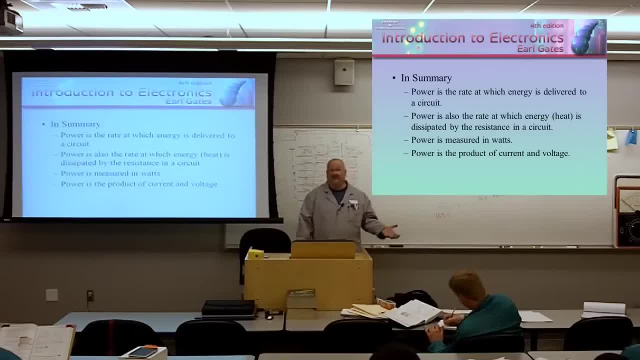 TV. I've got all this equipment. I've got several computers. I've got a computer that monitors the weather at my house. Why? Because I'm just into that kind of stuff. I've got my other main computer. I've got all my network gear for router. I've got a switch. 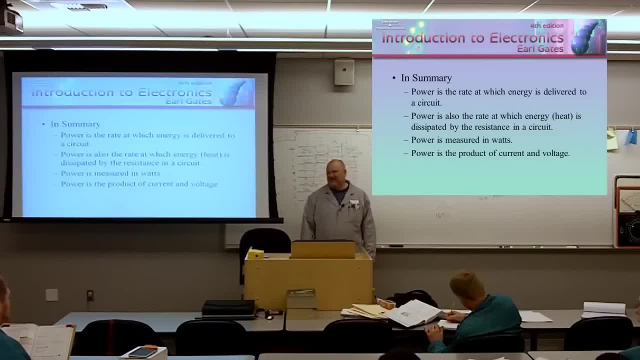 That powers the other internet connections in the house. I've got all that stuff. In the summer that room really gets freaking warm. In the winter it's kind of cool Warm. I mean. You know what I mean. You come in there and I've got all this electronic stuff. 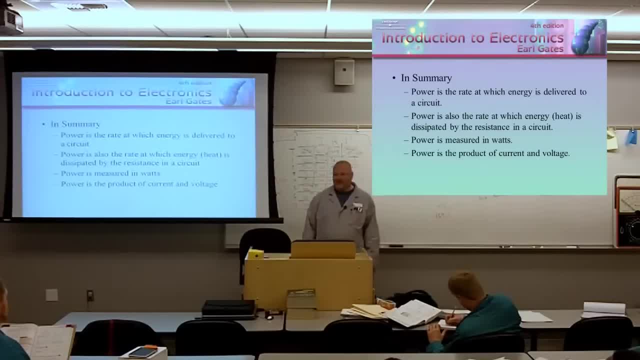 that's keeping that warm relative to temper, Was it last year, two years ago, we had that heat wave. It was like holy cow, man, I've got to start shutting stuff down. I'm like, how important is it? I've got to shut this stuff down so I don't have a Wi-Fi system. 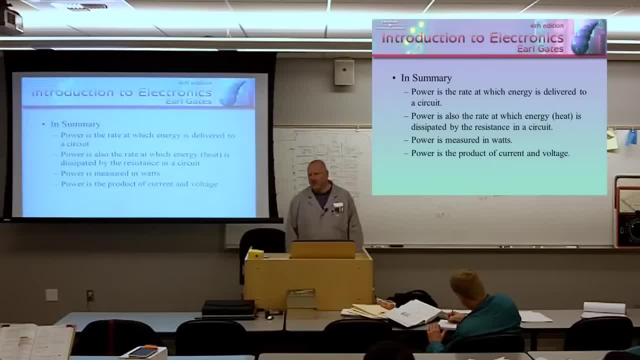 in the house, Not that that generates that much heat, but everything else in there does generate the heat. We don't want that. We don't want that. It's something we have to live with. So a lot of times, when equipment is densely packed, that thermal profile tells us what's going. 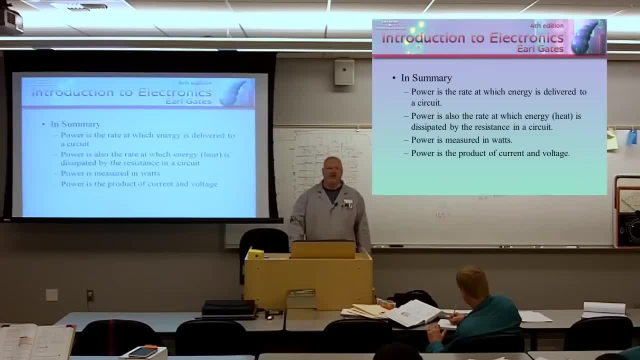 on. Former member of our advisory committee here at Lake Washington Technical College was the chief engineer for Channel 9 out of Seattle And we went down there for a tour one day. Their transmitter's located up on Capitol Hill And he was showing me the air. 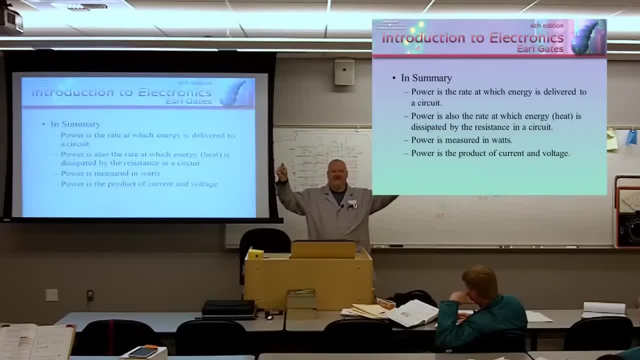 inlet temperature And then the exhaust temperature, Right The air that they're sucking in to run through the transmitter to cool it, And by looking at that you know this is the inlet air temperature, This is the exhaust. By looking at that difference, obviously if it's a warmer day they go up. 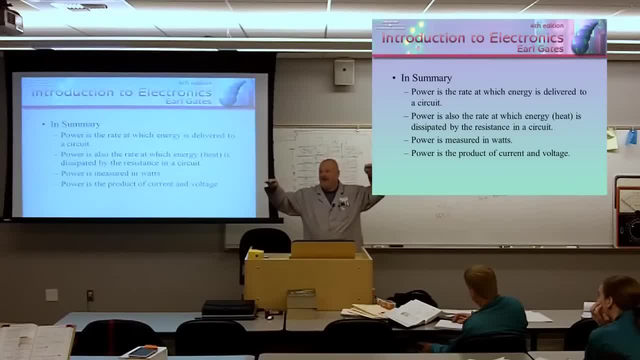 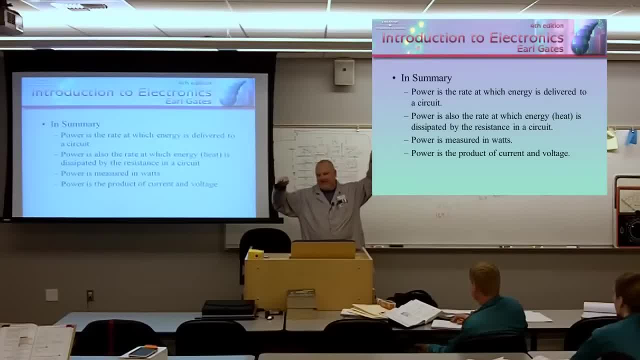 Because when it was brand spanking new, this is what it was. this is the inlet that the difference between the two is a critical number: Temperature You raise the temperature shows you something's not operating efficiently. plain and simple. One of the tricks. because 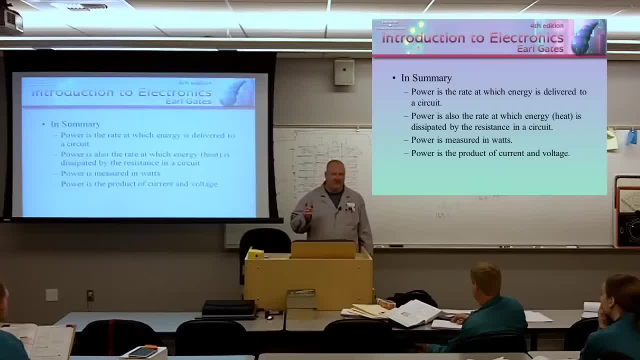 I paid attention. I'm not that smart of a guy, but I did pay attention. when I was in school- Formal schooling lectures- One of the things that I used to do is when I was in the navy. we had very, very complex. 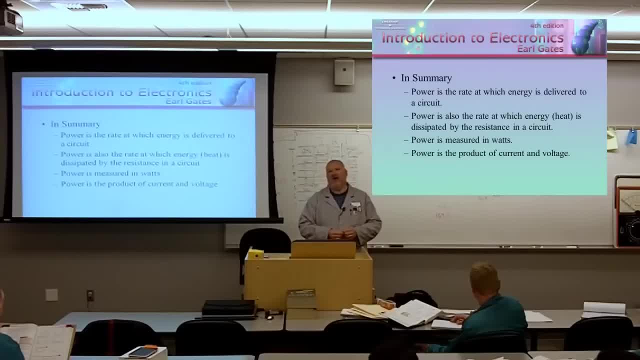 circuits. Ah Right, Yeah, Yeah, Okay, Okay, Okay, Okay. And there was this one board that had memory chips on it And it used to fail, And running the diagnostics to determine which chip it was was just very, very laborious. 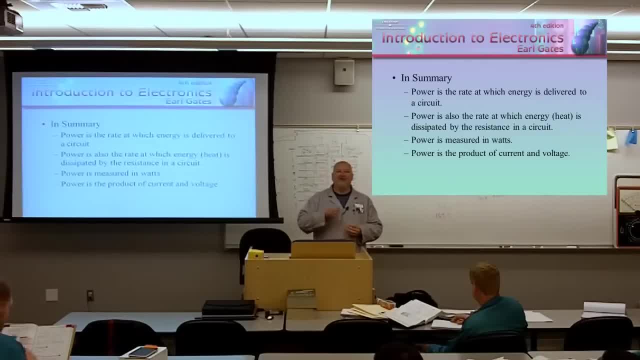 And I've always kind of been a lazy guy And I'm like you know. there's got to be an easier way of doing this. So what I did one day is just for giggles. I knew we had a failure. We already figured out what the chip was. 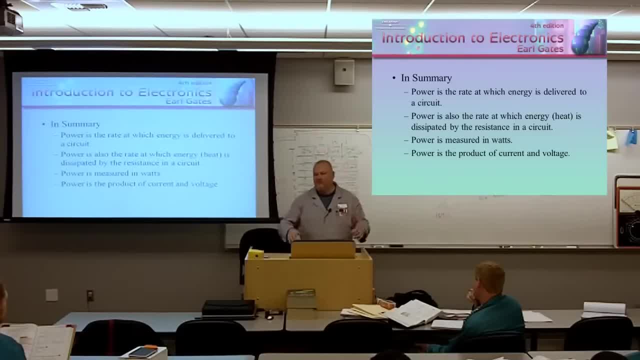 I put it back in and fired the whole system up And then immediately shut the thing down, pulled the circuit card out And I started going across the chips, Got to the hot chip. And guess which chip was the hot chip? The failed component. 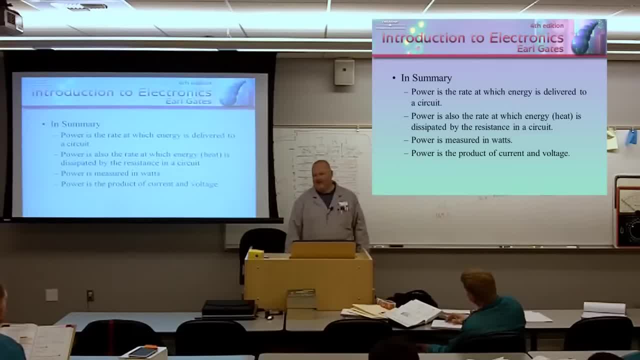 So anyway, it was kind of funny. My colleagues thought I was into black magic and voodoo Because there would be a problem with the chip. And then I'm like, okay, I'll figure out which one it is, But you're all going to have to leave. 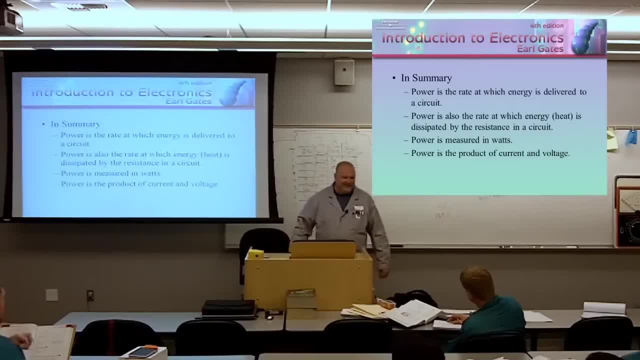 And I actually started doing it. I had a little mojo bag. It has bones in it and a crow's foot And I played the whole thing up, you know, And we'd shut the thing down, I'd come out U-44.. 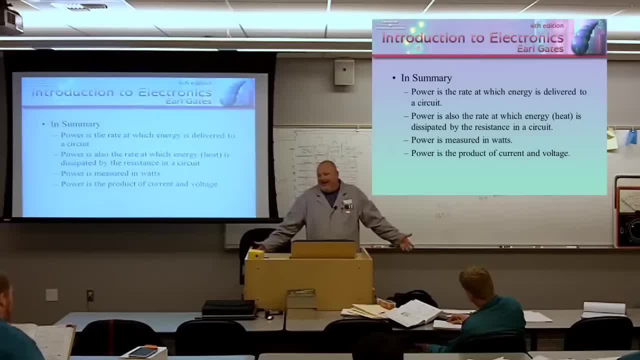 It's like: how the heck did you do that? I was looking at which chip was getting hot. The one that gets hot is the one that failed And it's generating more heat, And that's what the problem is. So you could really determine using a troubleshooting tool later on. 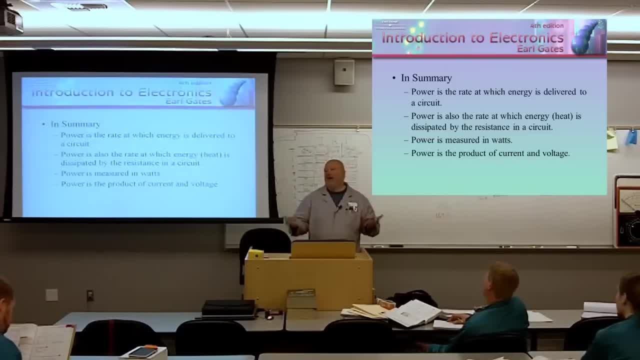 If something's getting hot And if you know what the norm is beyond that. Now they've got stuff on the market. They've got thermal imaging. Power company Actually uses thermal imaging. They'll go ahead with a thermal imaging gun and look at their power runs. 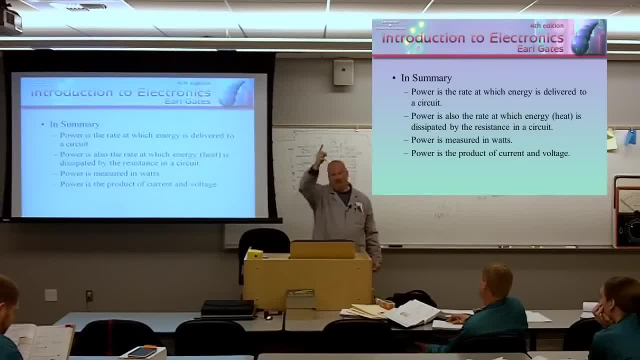 And where two wires are joined together. If it starts to generate a lot of heat, They know there's a problem up there. Okay, Because if it's generating heat, That shows that that connection has too much resistance, Because resistance generates heat. 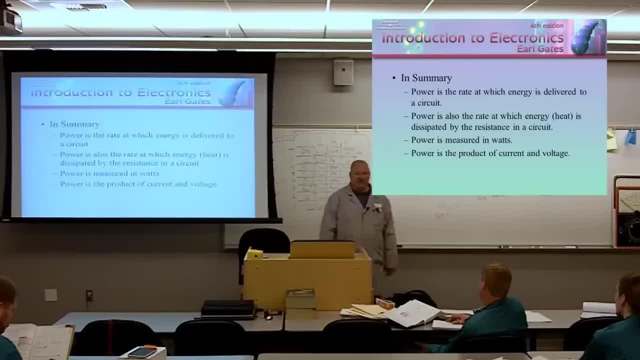 So you could analyze. with thermal imaging You could really see a picture of physically what's working and what's not working. So that's an advancement that's taking place Really. Within the past decade, Thermal imaging Now is pretty much mainstream. 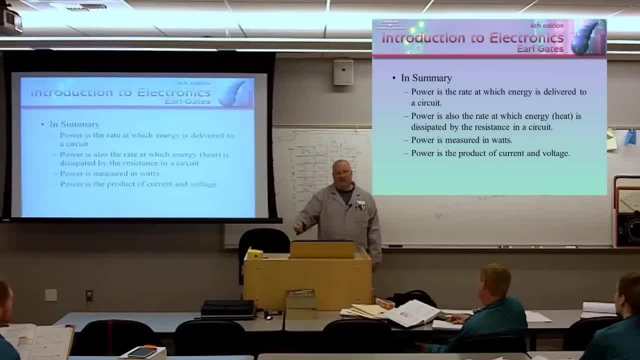 You know, it's not that Heck. you could get a non-contact infrared. get one at Harbor Freight Pools from 1995.. I had to use to burn my fingertips, finding the hot chip. Okay, Now you could just use one of those and say, oh yeah, this chip here is hotter than all the others that are doing the exact same job. 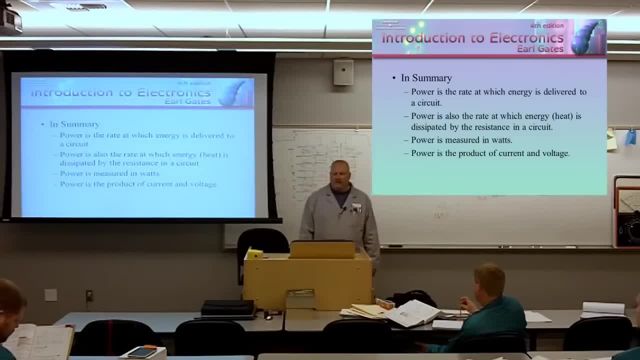 That's where the failure is. Power is measured in watts. Watts is what power is measured in. It's not a question, It's a statement. Power is literally the product of current and voltage: Current times, voltage. Any questions on power? 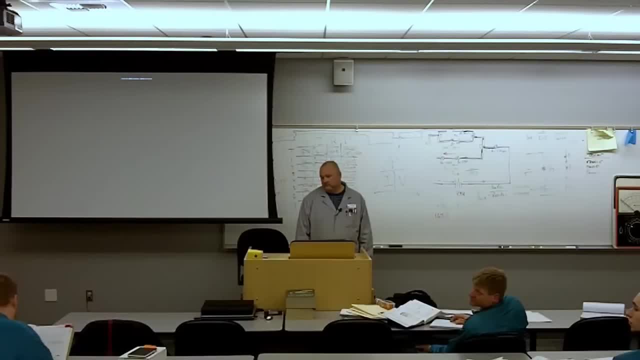 You were saying that to determine the total voltage drop throughout any component is a different formula than what it would be to calculate power. But in the book it says the voltage is equal to I. No, I'm just saying I'm not going to determine how much. 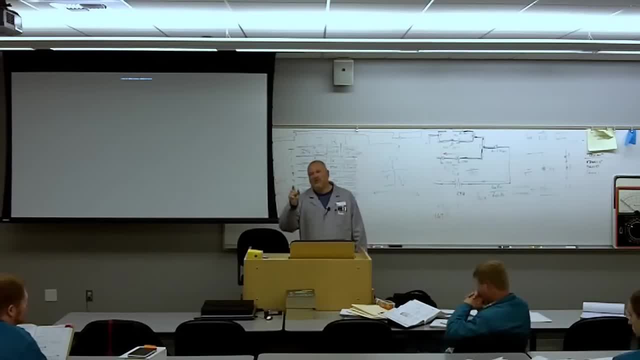 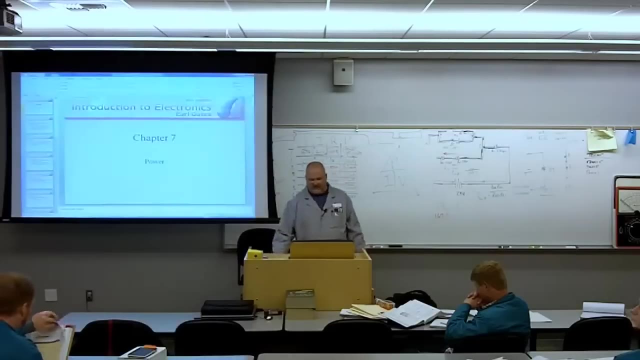 Power is being consumed across a component, You need to use that voltage drop across the component, not the total voltage value. All right, Let's go ahead and take a 13 minute break. We're going to start up again at 635.. 635.. 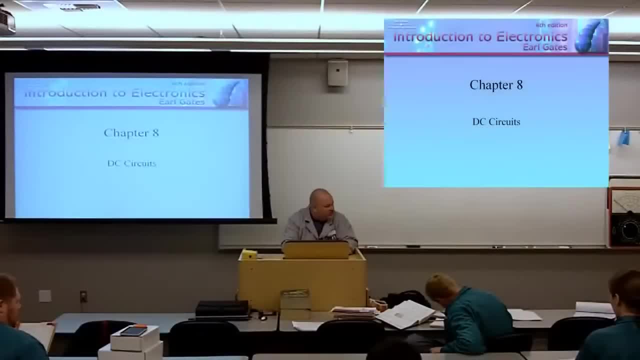 635.. Chapter 8. DC circuits- DC circuits. One of the things that you need to understand about this chapter is it's the concepts that we're going after. We want you to understand the basic concepts. You're not going to make a lot of money necessarily going out and working on circuits like this in industry. 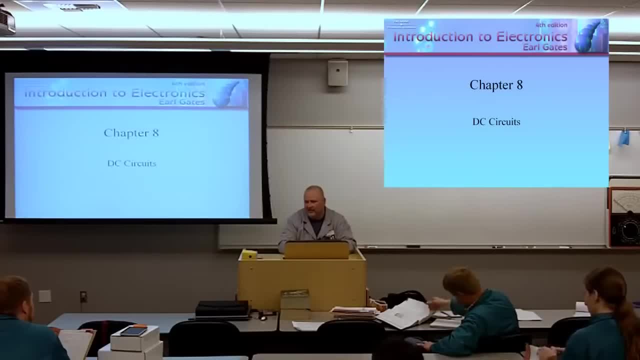 Circuits that are made up of a power source and a bunch of resistors, But what this is designed to do is to show you an approach on circuit analysis. We are going to use circuits That contain a bunch of resistors in industry. 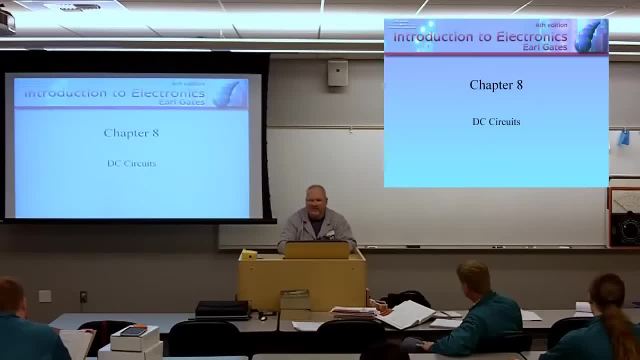 And those resistors are going to be used to establish voltage operating points Around transistors or other semiconductor devices. So, although you're never going to go out and necessarily work on circuits exactly like this, You have to absolutely positively understand the steps and the competencies of circuit analysis. 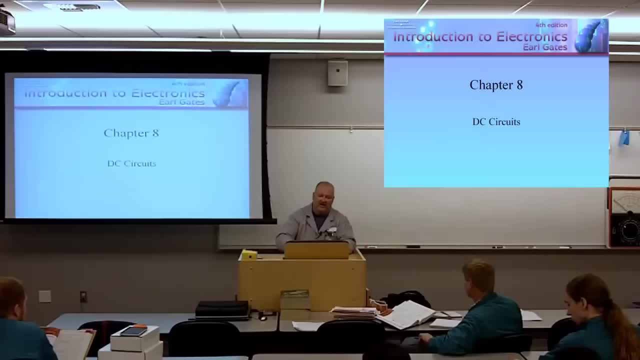 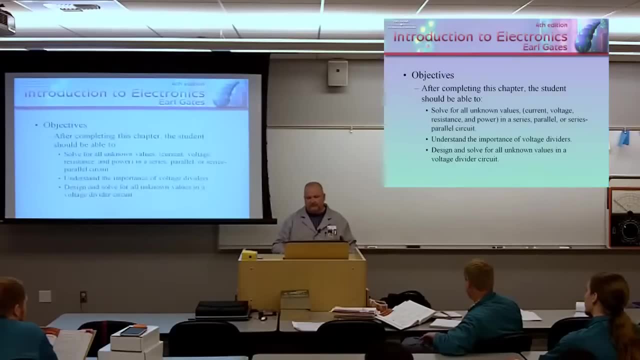 As it pertains to DC circuits. That goes without saying And, quite frankly, we've already talked about these concepts. This is just the chapter where we pull it all together. After completing this chapter, you're going to be able to solve for all. 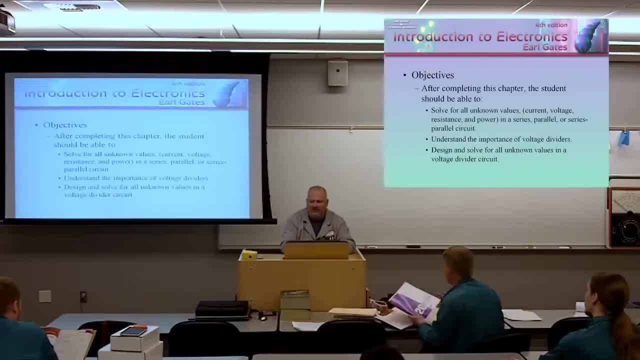 And let me emphasize the words all Unknown values. That means voltage, current resistance and power. Always solve for everything, Because if you know everything, I could never ask you anything that you don't know. Because you know everything In series circuits, parallel and series parallel circuits. 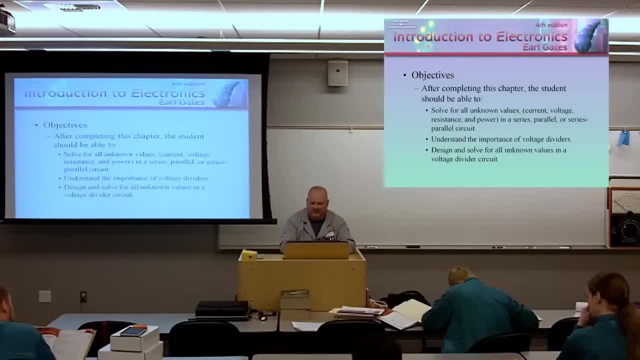 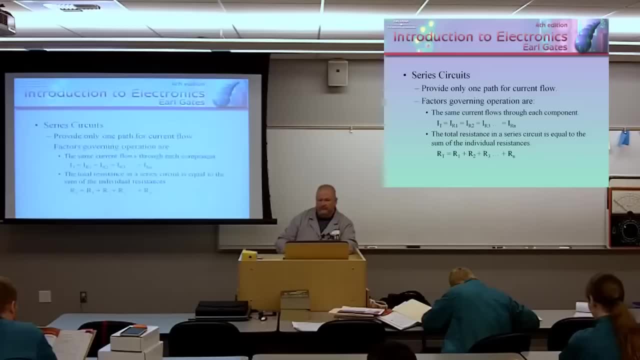 Understand the importance of voltage dividers And design and solve for all unknown values in a voltage divider circuit. We are going to spend time on voltage dividers- Some of the stuff I'm going to blast through- But voltage dividers are something that I'm going to spend some time on the board here. 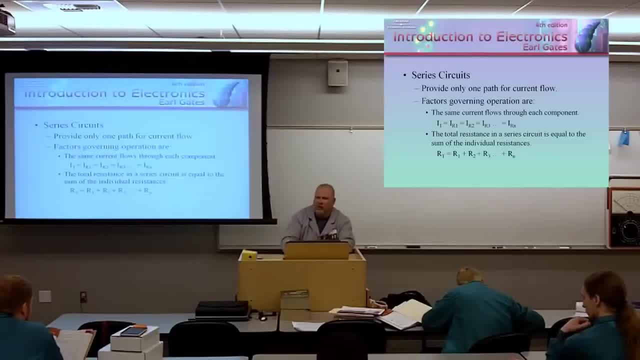 To make sure you've got a handle. It's quite fun And, frankly, the book is okay, But the author really drops the ball with voltage dividers. He pulls a couple numbers out of the air that I still don't have a clue where it comes from. 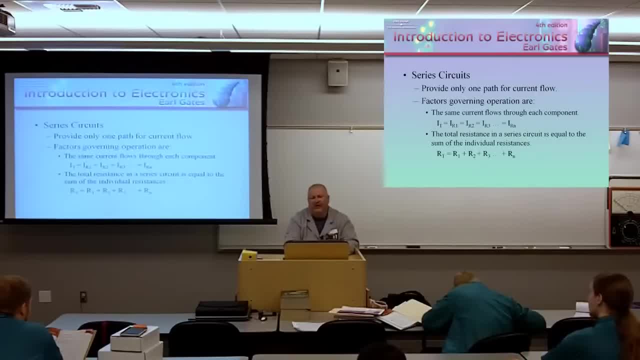 So I'm going to show you how to approach that. As you know, a series circuit is a circuit that provides only one path for current flow. The simplest example of a series circuit You ever have, those holiday lights, The Christmas lights that a bulb burns out and a whole string goes out. 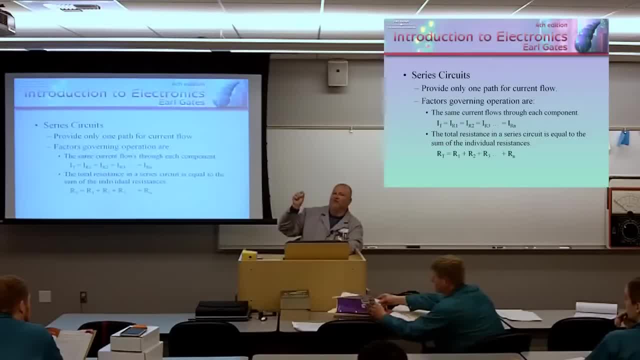 It's a series circuit Because the filament of one bulb Interrupts the flow of current to all the other bulbs. It's a series circuit. If you've got a string that one bulb burns out And maybe ten other bulbs go out. 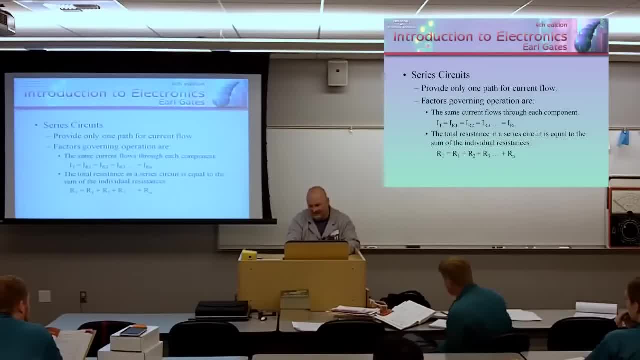 What does it tell you about those ten other bulbs? They're all in series. The whole string may be a combination circuit, But that individual section that went out is in series. So there's a lot of lessons behind looking at festival lighting And when it goes out. 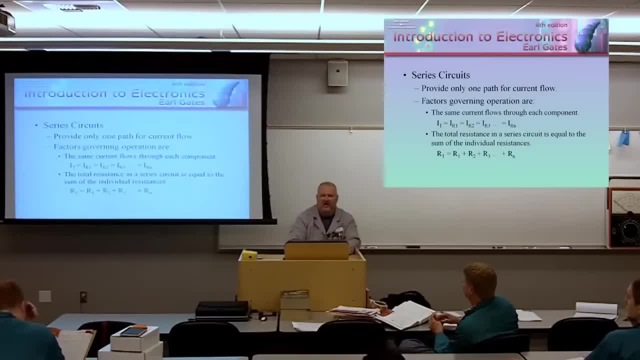 What exactly is taking place there? Factors governing the operation are the same. current flows through each component. Literally the same current, The same electrons. They only have one path to go, That's from negative to positive, So they have to travel the entire route. 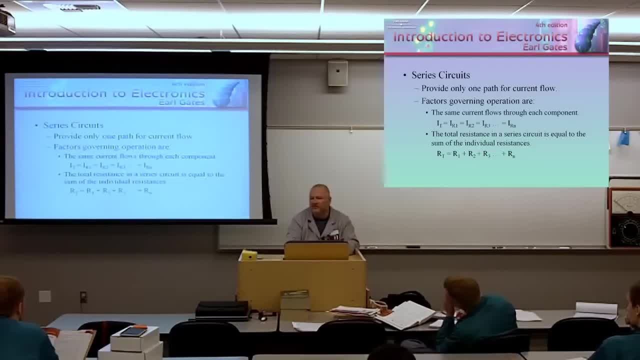 Total resistance in a series circuit is equal to the sum of the individual resistances. This is what chapter three, four review. You got resistance. You add it up In series, Always additive, And that includes the resistance of a bad solder joint. 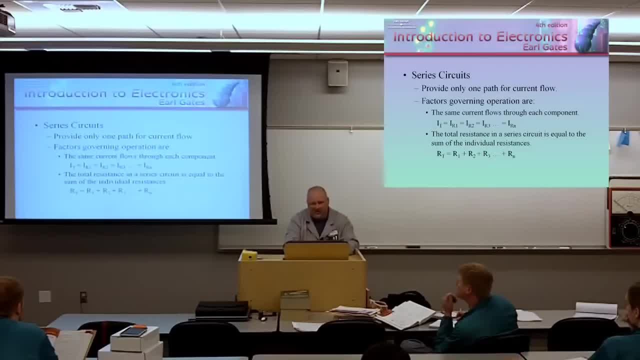 The resistance of a bad splice. Remember how I said: the power company, the voltage company, will actually use thermography and look And say, wow, we've got a splice up there and it's generating a lot of heat. We've got to shut that section down and replace that. 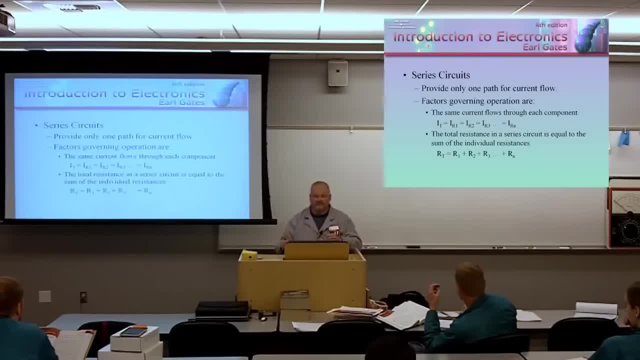 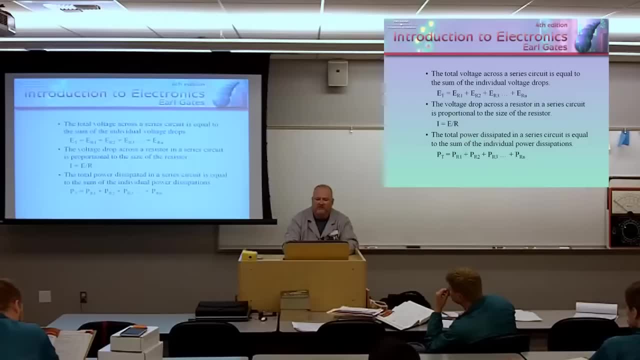 Because it shouldn't be generating any heat. if it's a good splice, The total voltage across a series circuit is equal to the sum Of the individual voltage drops, Meaning total voltage is equal to voltage across component one Plus the voltage across component two. 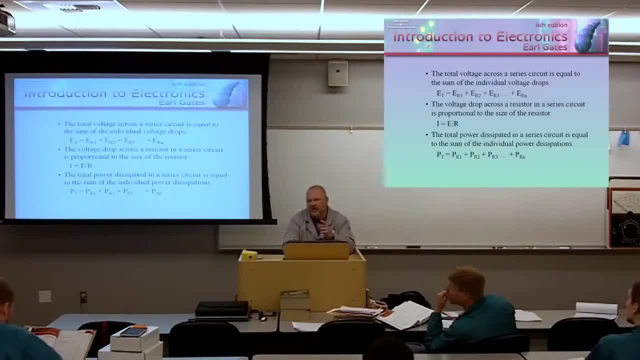 Plus the voltage across component three. This is a review. This is the same thing. you could quote me. I love it when you quote me. Voltage rise equals voltage drop. So here, voltage rise, ET or VT, if you prefer- Equals voltage drops. 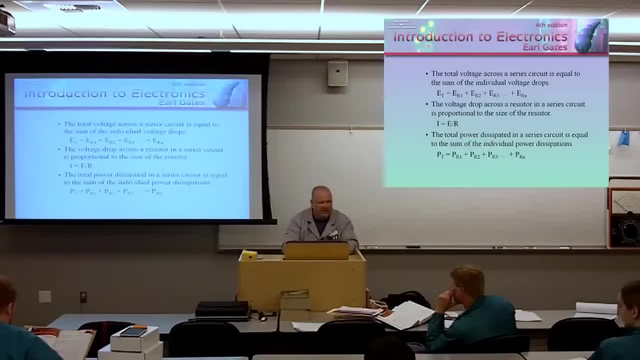 ER1.. ER2.. ER3. Those three voltages better equal what I put into the circuit. If not, you've got a problem. If you find where the missing voltage is, you probably found the problem. Where was the missing voltage? 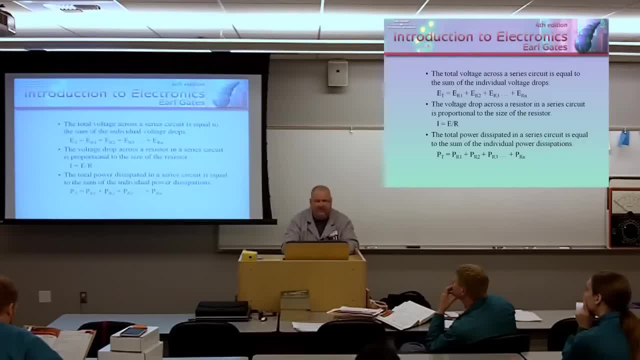 Where was it? Oh, it was on a bad splice. Oh, okay, You fix that problem. Boom, you're up and running. The voltage drop across a resistor in a series circuit is proportional to the size of the resistor, Meaning the bigger the resistor. 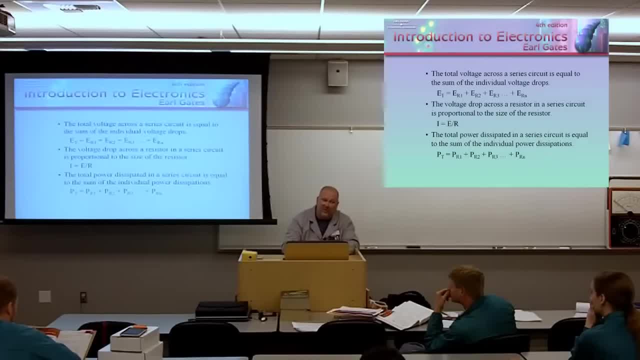 I'm talking about the size of the resistor. I'm not talking about in ohms. I'm not talking about physical size. The more ohms, the less current. The more ohms the higher the resistance, the bigger the voltage drop across that resistor. 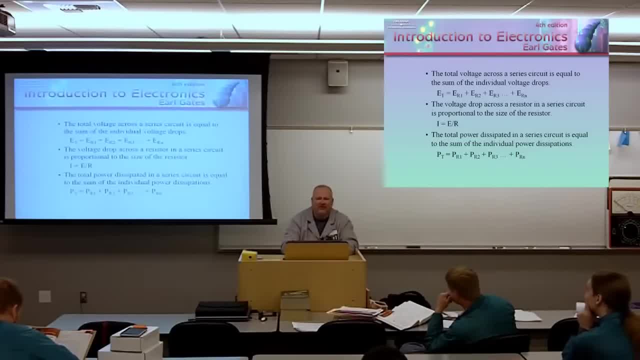 I always think of a resistor. Remember how I used Seattle traffic flow as an analogy. Right, A big resistor is like a big accident. If you just got a fender bender, is that going to slow the traffic down? Yeah, Fender bender, they pull over the side, people start, you know, slow down whatever. 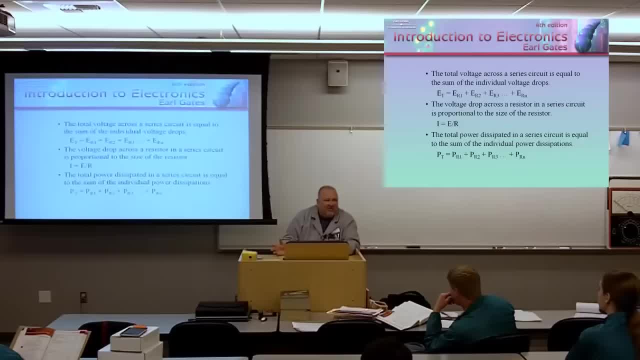 Right, You got a 3-5-3.. You get a 3-5-3.. Three-car, five-car pileup. it's a big accident. That's a big resistance. A big resistance is going to create- I gave it away already- a big backup. 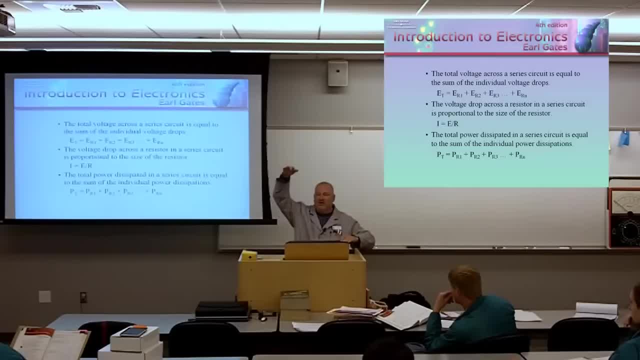 A big backup is a big difference in potential. A bunch of people here that want to get to work and a bunch of people here on the other side of the freeway that an empty freeway. basically That's a big difference in potential. Okay. 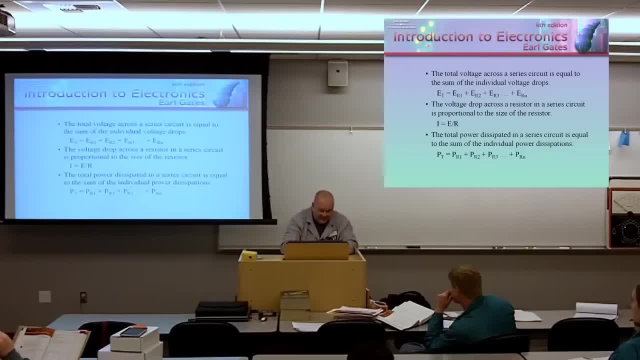 I love flying in my airplane over traffic jams. As a matter of fact, being a pilot owning an airplane, being stuck in a traffic jam drives me freaking nuts Like: why am I stuck in this traffic jam? But from the air it's so obvious where there's an accident or a problem, because all the traffic. 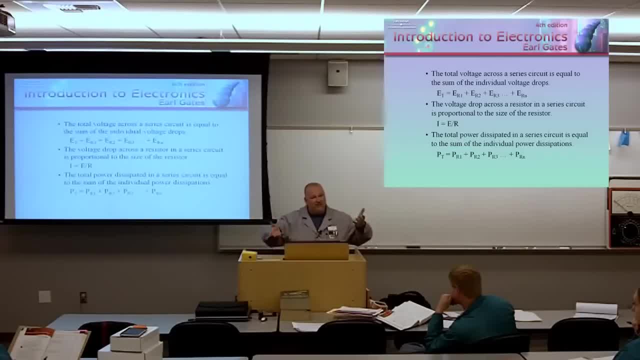 is backed up and then just a few cars are making it through. Difference in potential Big resistance. Make sense. In the book it says ET is equal to ER1,, equal to ER2, equal to ER3. It's a mistake. 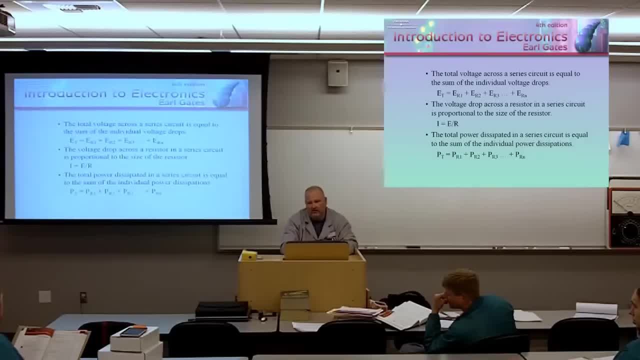 That's for parallel, You sure that's not parallel? you're looking at Total voltage across the series circuit. Typo, Typo, Yeah, Total power in a series circuit or a parallel circuit or a complex circuit, Power is additive. PT is equal to PR1, PR2, PR3, PR4, just add up all the power and that's going to give. 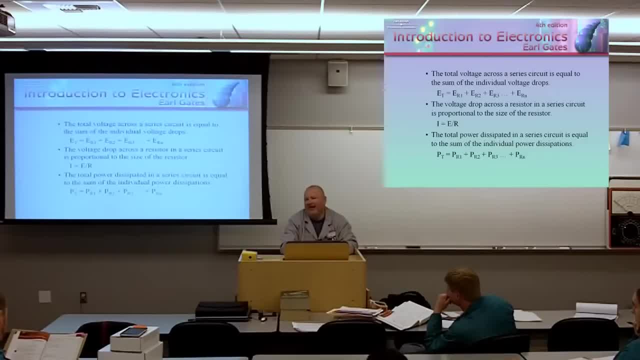 you your total power, The bottom line, You want the bottom line or you want the BS, The bottom line, Bottom line In a series circuit. the most important thing to remember about a series circuit is: current is constant in a series circuit period. 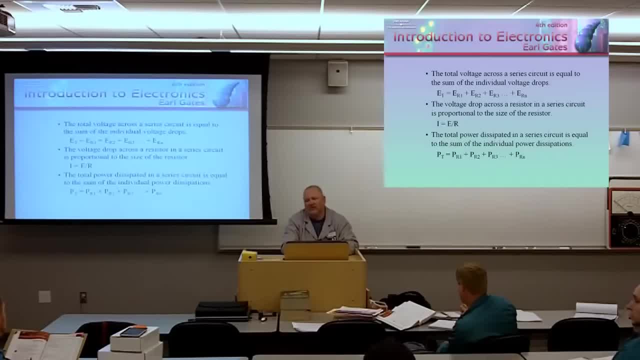 The second most important thing to remember about a series circuit: series circuit is also synonymous with voltage divider. When I say series circuit, I want you to think current's constant and I want you to think voltage divider. That's just how I want you to look at them. 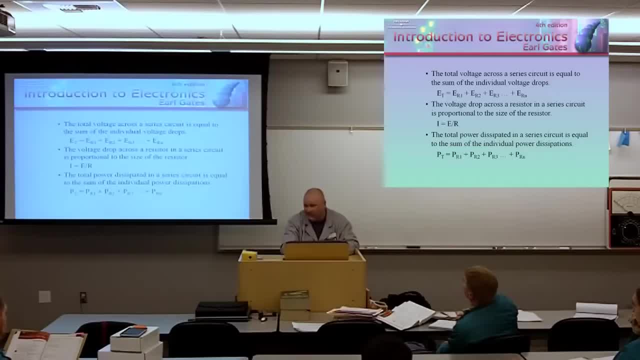 And if you're not looking at them that way, you ain't looking at them right, Houston, we're going to have a problem. Okay, Those are the most important things. I'm going to have you repeat that back to me in the future. 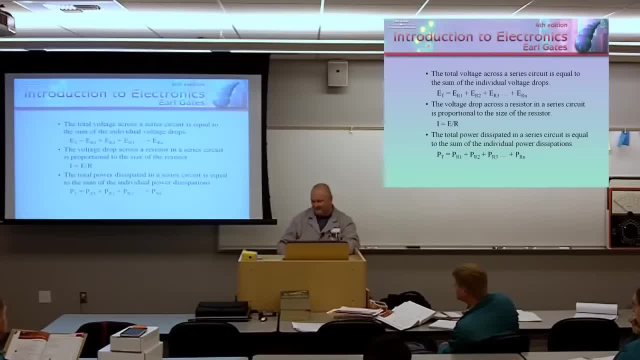 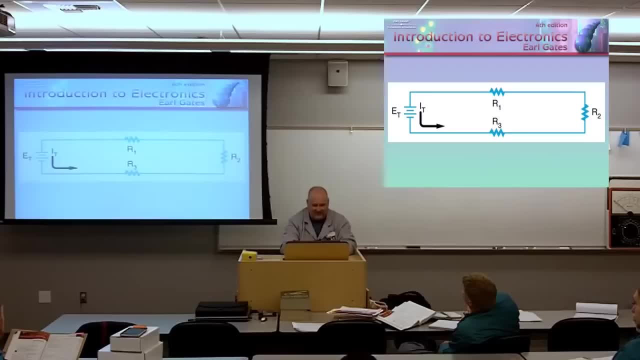 Do not deceive me, Remember that stuff. The most important thing in a series circuit is current is constant. Why is it constant? It's only got one path to flow, so it better be constant. The second most important thing about a series circuit is the cycle. 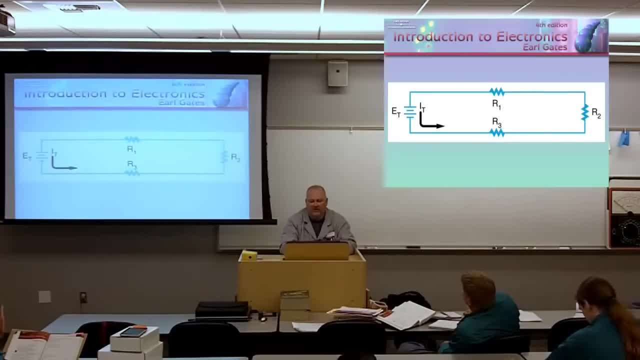 The second most important thing about a series circuit is the cycle. The second most important thing about a series circuit is the cycle. The second most important thing about a series circuit is a series circuit is also known as AKA. like in police lingo, AKA also known as a voltage divider. 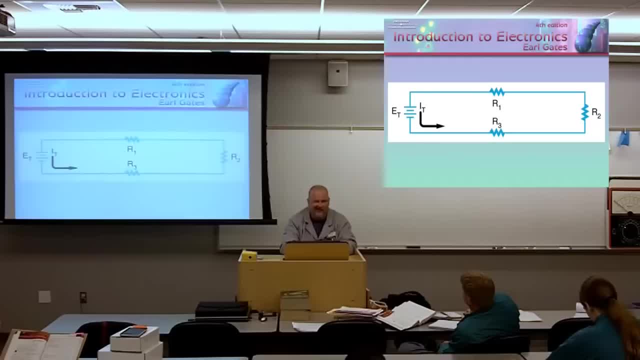 A voltage divider In this particular circuit. I mean, I look at it and yeah, I've been doing this since puberty. but I look at this. What do I see? I see a voltage source and three voltage drops. Voltage rise and three voltage drops. 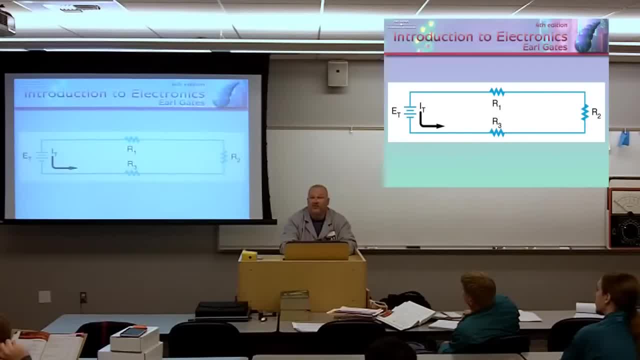 drops Three loads. I don't know what they are, but I know these loads are connected in series And I know that all the current that flows out of the negative terminal of my voltage source has to travel this complete path, No place else for it to go. So the current's 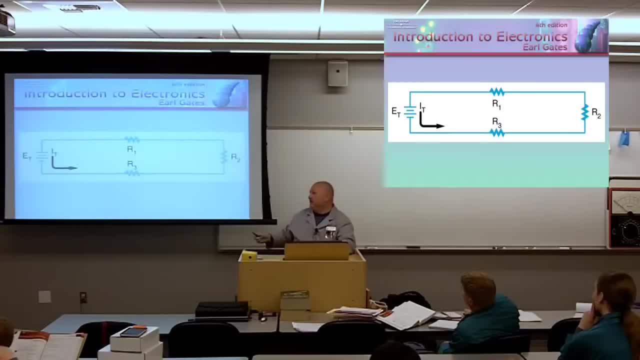 going to leave the negative terminal of the battery. It's going to make this corner, 90 degree corner, at the speed of light. This is cool stuff, isn't it? The speed of light? Come on down through here in the back stretch, hit resistor three and create a voltage drop. 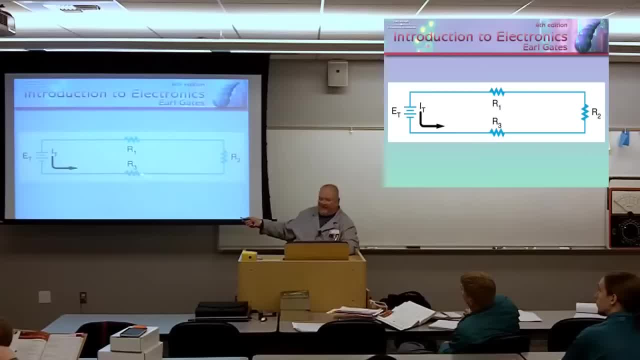 a difference in potential Current's going to finally make it through that obstruction. Another 90 degree corner at the speed of light Come up here to R2.. It's going to create another voltage drop because there's another obstruction. There's more resistance, There's more resistance. 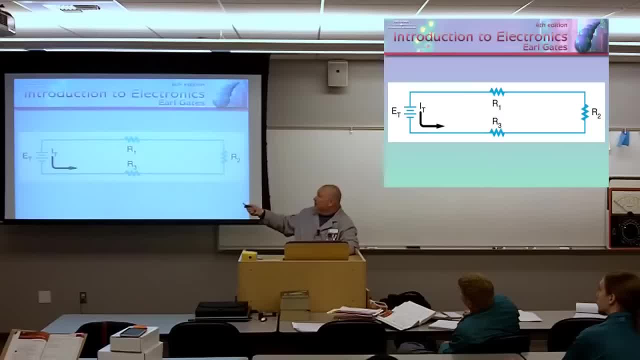 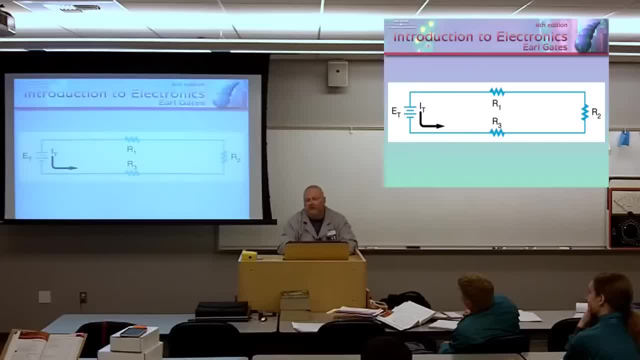 have to equal this voltage rise. If anything's missing, you've got a problem. Find where it's missing and you've found your problem: Power additive, Resistance additive, What else is there? So, anytime you've got the reason I want you to look at it is anytime you've got one way into a circuit and one. 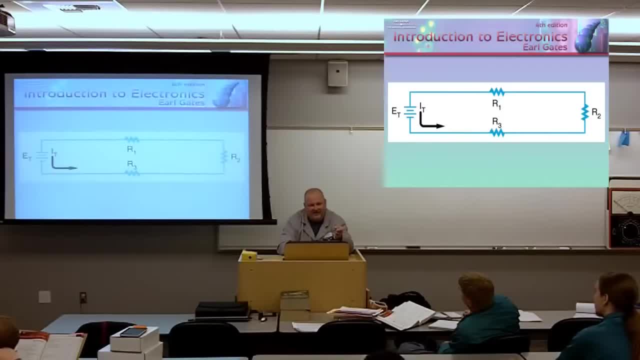 way out. what does that tell you? It's a series circuit. It's a series circuit Because I cannot. I cannot show you every possible series circuit ever invented. If you've got one way in and one way out, it's a series circuit, Even if it's one component, One component. 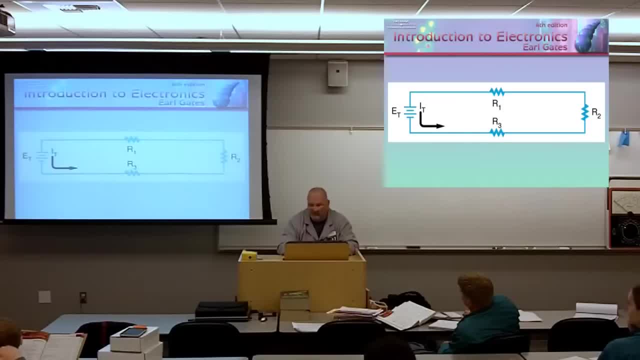 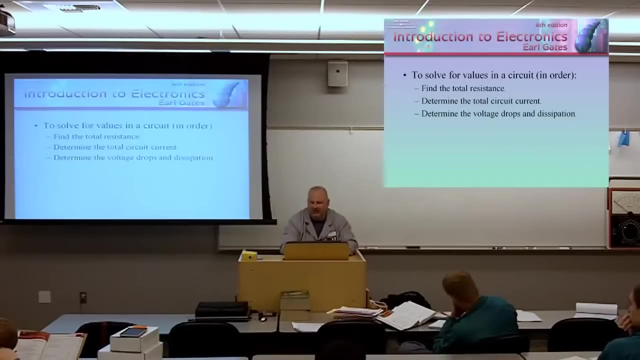 could that be series? Yeah, One way in, one way out, it's series. Is that right? Is that right To solve for values in a circuit in order? the first thing I recommend you do is try to solve for that total resistance Once you determine RT, total resistance in. 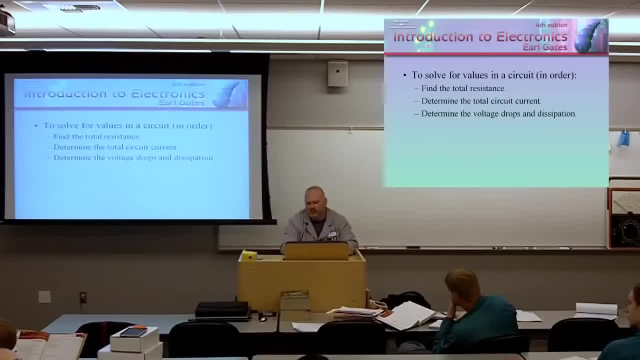 the circuit. then try to solve for total current in the circuit IT. Once you know IT, then you can determine what your individual voltage drops are right. So solve for your total resistance. Total resistance with your total voltage will show you how much current you're allowing. 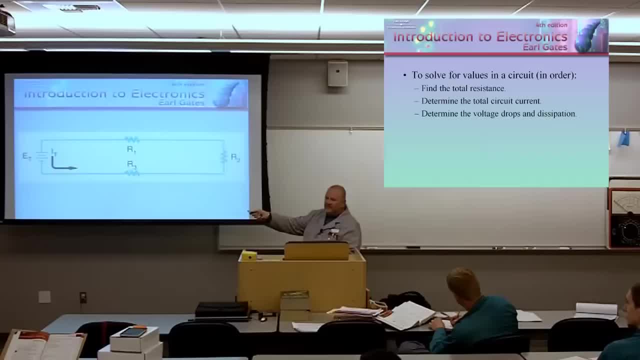 into this circuit. Current flowing through the circuit encountering the resistance V is equal to I times R, The total current. the same current that travels the entire path times the amount of resistance there is in a circuit. So this is going to drop a portion. 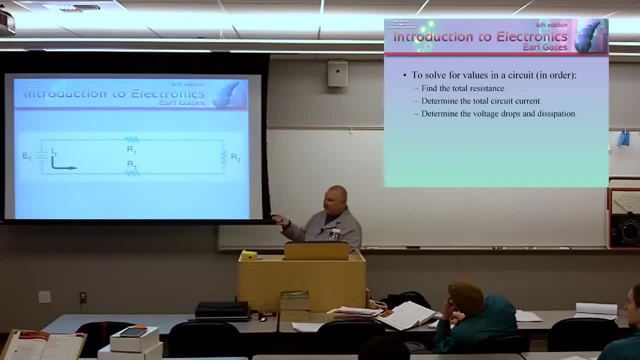 of that voltage. This is going to drop a portion of that voltage. This is going to drop a portion of that voltage. These three portions better equal the voltage that's put into the circuit. In regards to the slide previous to this, which is the three steps, it doesn't say on. 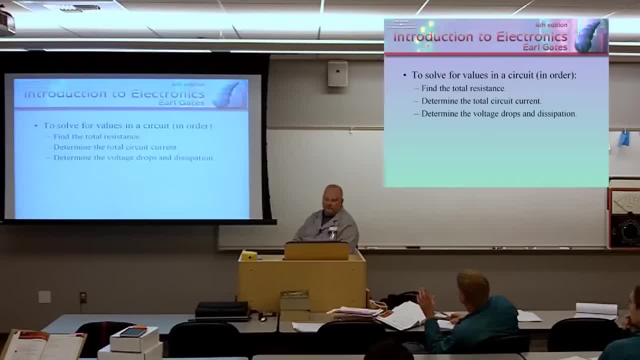 the slide series or parallel. So these will they primarily cross out between the two applications. Yeah, but I got to warn you, This here is just like generic. This is like generic And the thing of it is is, when you get out into industry or in lab, I may give you this, I may give you this, I may give you this, But this is encased in epoxy. You can't even get to it, You can't even get a part number off, You can't even take reading. 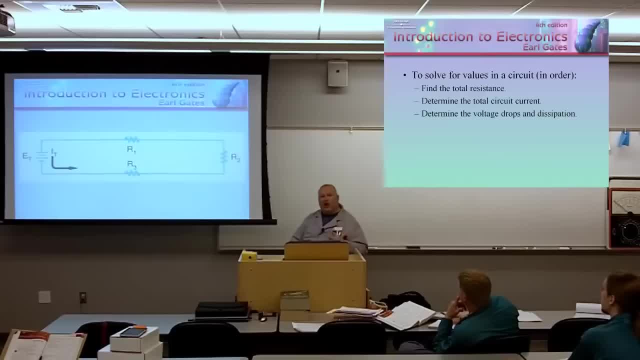 of it. So you're going to have to use these laws and say: well, Sheesh, I remember Joe said that this is equal to this, plus this, plus this. I know what this is is, I know what this is, I know what this is, but I don't know what this is. So then you could say: 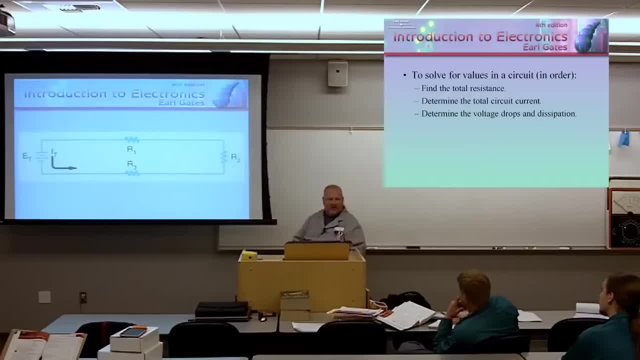 this. minus this, minus this, the remainder is equal to this, And it's a safe assumption, because you're using a law- Kirchhoff's voltage law, basically- to determine what the unknown is, And if you're using a law in industry to figure out what part you need to buy, whose money you need to spend. 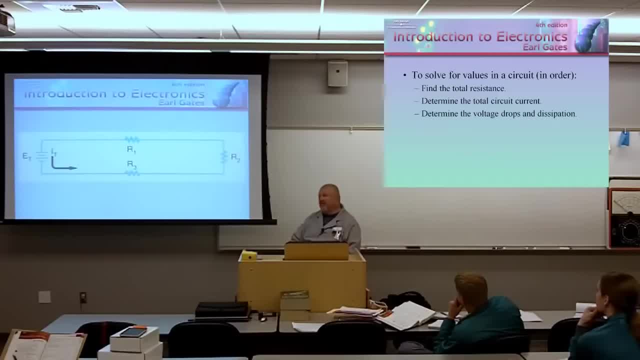 it's a pretty safe assumption. I mean it really is. So that's why we're teaching you this. So don't necessarily use this as a checklist and like: oh yeah, I took copious notes, I listened to what Joe Greenick had to say in lecture. I went home this weekend to try to do my homework. 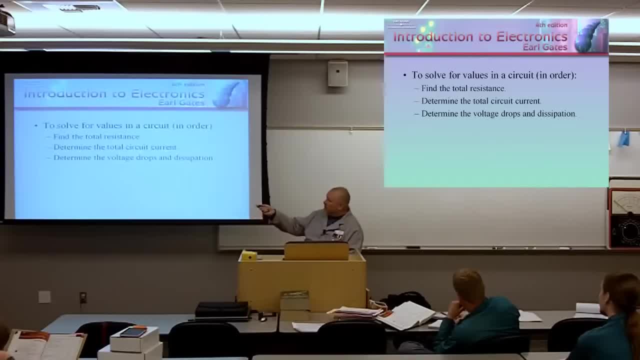 and it didn't work because I couldn't determine total circuit current, because I didn't know what this value was, because Joe didn't say sometimes we might not know what this value is or we need to find it on the internet off of a data sheet from a manufacturer. So the bottom line I want: 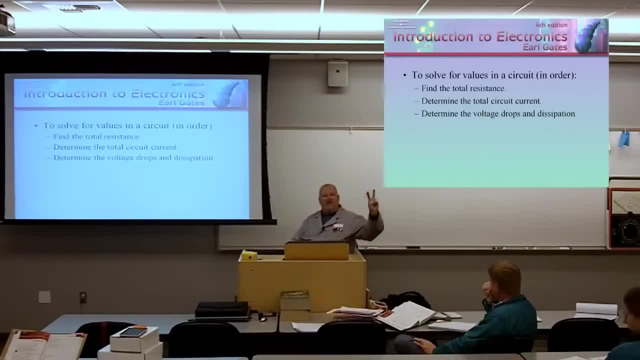 all of you to realize: with these circuits and analyzing the circuits, you always need to find at least two bits of information. If I only give you one piece of information, you're not going to be able to get very far. But if you could extract two bits of 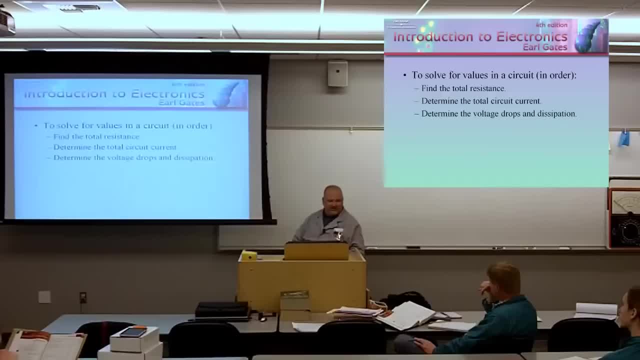 information, then you could re-manipulate these three to suit your needs. as long as you get the right answers, Make sense, Absolutely Okay. Parallel circuits: I might as well get the cat out of the bag right from the get-go. Parallel circuits, the most important thing you need to. 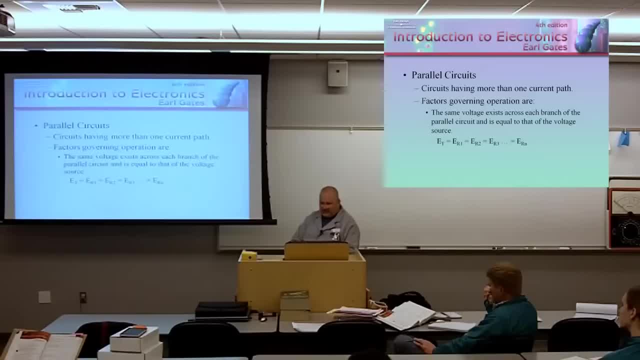 remember about a parallel circuit is: voltage is constant across a parallel network. Voltage is electrical pressure by being constant across a parallel network. What am I talking about? I'm saying that that voltage is constant across all components that are connected in parallel. Your house is wired in parallel. The freaking voltage coming out of the outlets- better all be. 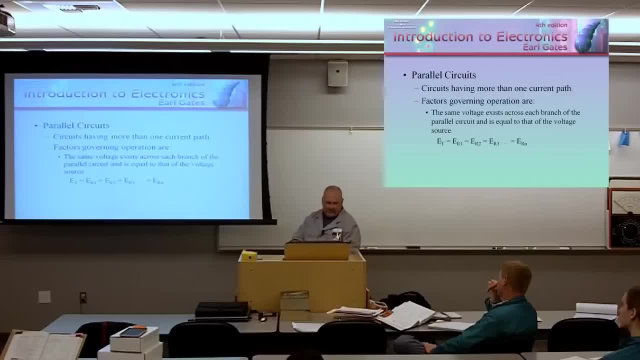 the same. If not, you got a problem. You got a problem. Voltage is constant across a parallel network, Most important thing you need to remember. So when I say that what's the most important thing about a parallel circuit Like church, you all repeat after me. 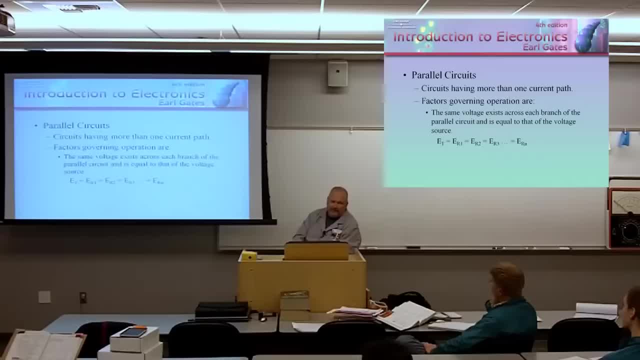 Voltage is constant across a parallel network. Okay, The second most important thing about a parallel circuit is that a parallel circuit is also known as police lingo, aka also known as: what If a series circuit's a voltage divider? what's a parallel circuit? It's a current divider. 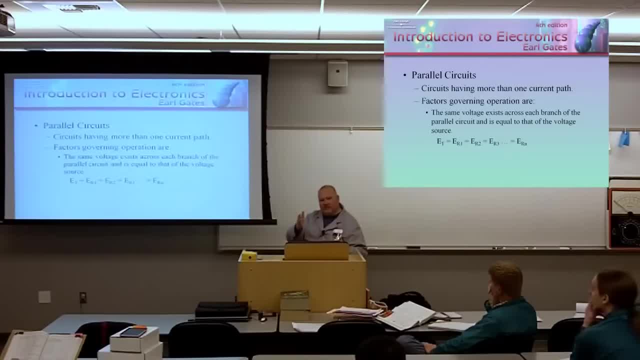 Divides up current. Some of the current goes one path, some of the current goes the other path. Remember the Seattle traffic pattern last week? Was I here talking to you folks? Was I talking about that or was it somebody else? Was it a dream I had? I had a dream. 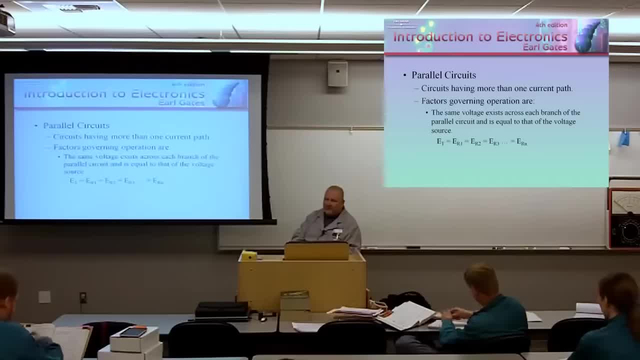 It was about current And it's what it is. So some of the current's gonna take the 90,. some of it's gonna take the 520,. some of it's gonna take the north end of the lake. some of it's gonna take the south end of the lake. Make sense? I've been a commuter for 20 years. 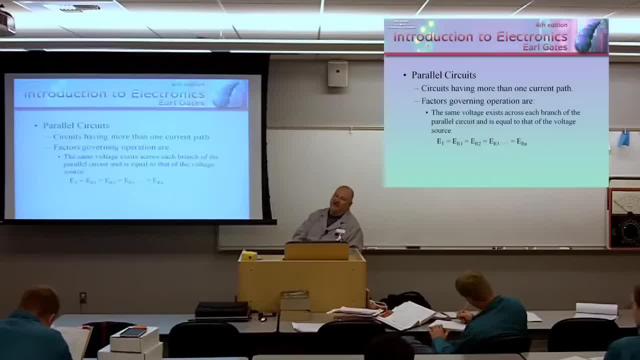 I know Seattle traffic. I've gotten out of here and gotten on I-90 and driven eastbound- Okay, Tacoma to Highway 18, just so I could avoid traffic. So I know a little bit about traffic. Look at these circuits like that. 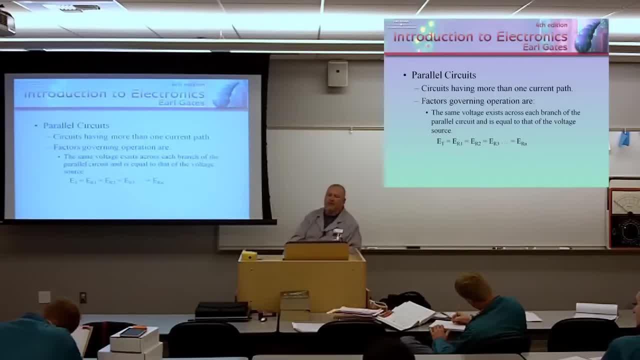 Factors governing the operation of a parallel circuit: the same voltage, the same voltage, not an equivalent voltage. the same voltage exists across each branch of the parallel circuit and is equal to that of the voltage source. So, literally, this is what we're. literally, this is what we're. 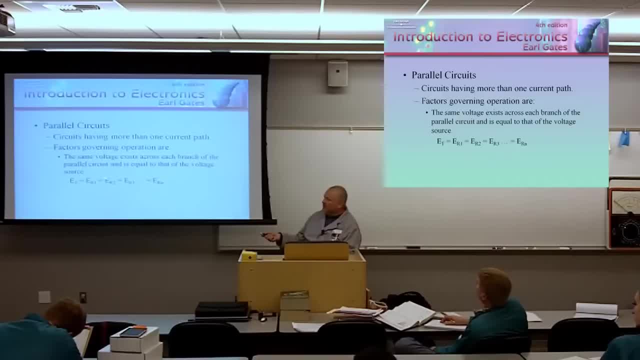 up against Total voltage is equal to voltage across component. 1. It's equal to voltage across component. 2. It's equal to voltage across component 3. It's not only mathematically equal to, it's the same pressure. I'll show you in the schematic: Same pressure. 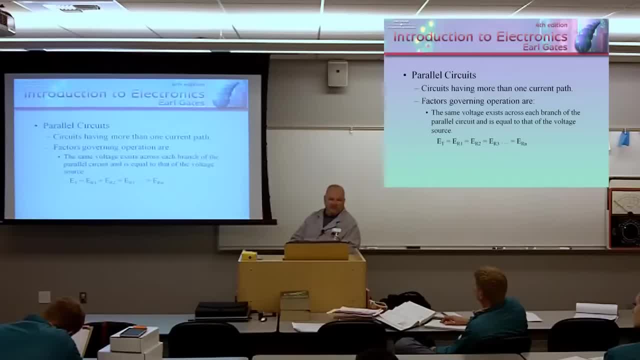 And that in and of itself will help you solve problems. If you know something's in parallel, you could assume If it's connected in parallel, I should have the same voltage across that. Well, sheesh, the thing's still not working. 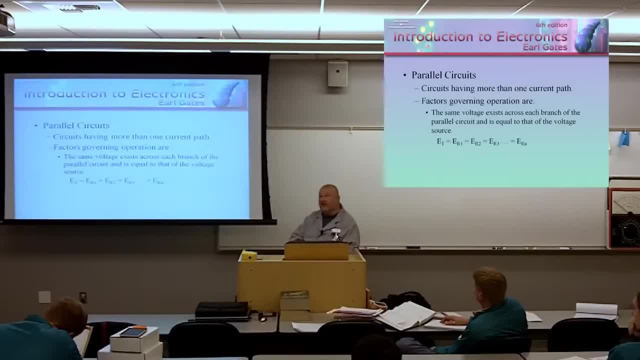 Or it's working kind of goofy, It's hard to get to. Well, sometimes you have to remove that access panel, go in there and take the reading. Holy cow. Everything else in parallel is at 12 volts. This is only at 9 volts. I'm missing. 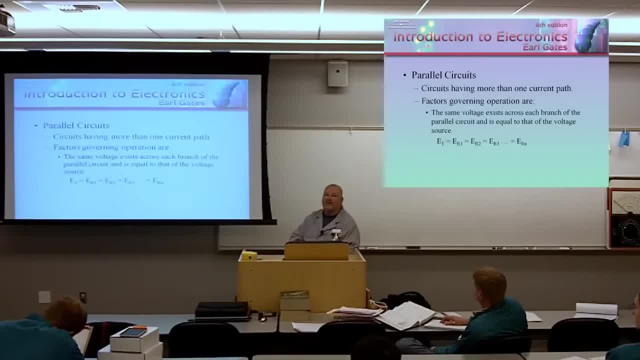 3 volts. You find I'm missing 3 volts. you found the problem. It's that simple. One of the most powerful tools. How many of you here like tools? I got tools. I got like every tool known to man in my garage. Just ask my wife, She'll tell you. 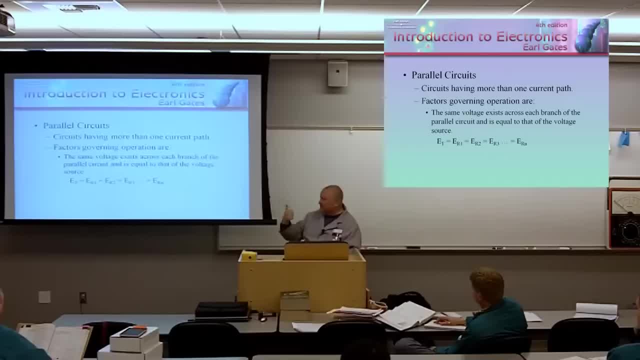 Okay, I like tools. One of the most powerful tools in your box is this stuff right here. The second most powerful tool you're going to have is the digital multimeter, Because the digital multimeter is going to allow you to get out there and find the missing. 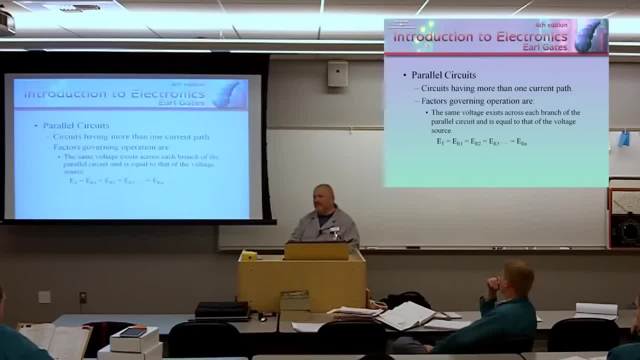 3 volts. Find the missing 3 volts. you found the problem. Found the problem. you save the day. You save the day. you hit your boss up for a raise. he gives you a pink slip, cuts you loose, Just kidding. 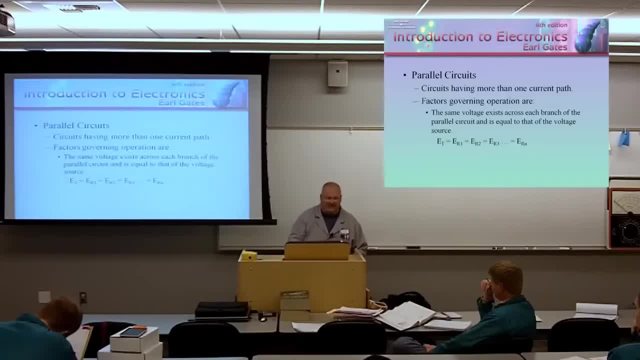 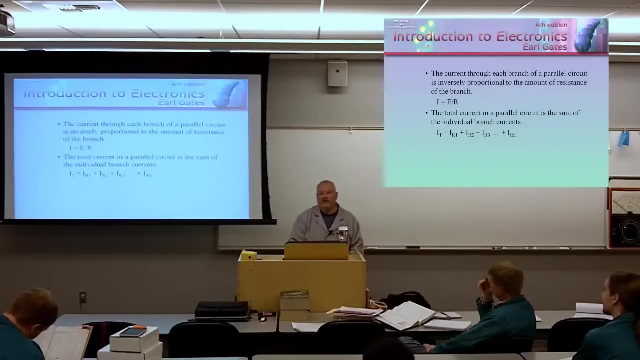 You get a promotion, life is good. Make so much money, get married, start a family, get a girlfriend on the side, it's all good. I don't mean that The current through each branch of a parallel circuit is inversely proportional. 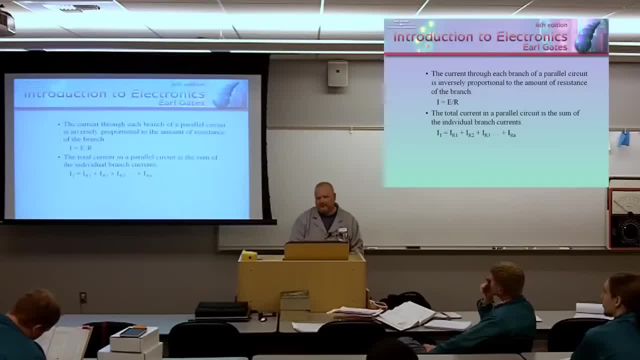 to the amount of resistance of the branch. I is equal to E over R. I is equal to E over R. So that means because R here it means E over R, right, E over R. We use the slash here, But that means that this: 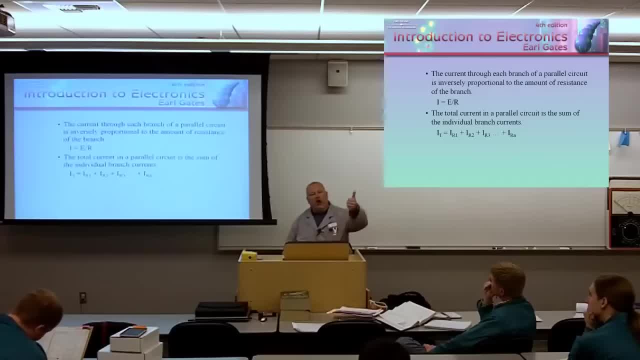 is on the bottom of the slash. So whatever we do to R is going to have an opposite effect on I. We call that an inverse proportional relationship. An inverse proportional relationship. So if resistance increases, current decreases, Bigger accident, less flow of traffic. 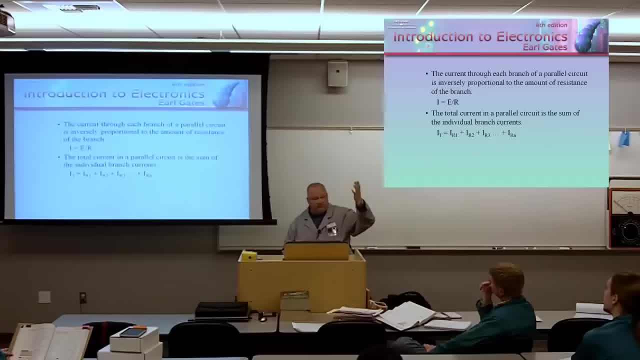 Smaller accident, less flow of traffic. Traffic flow increases- Plain and simple, So keep that in mind. The value of least resistance in a parallel circuit will have the highest current flow through it. The total current in a parallel circuit is the sum. literally. 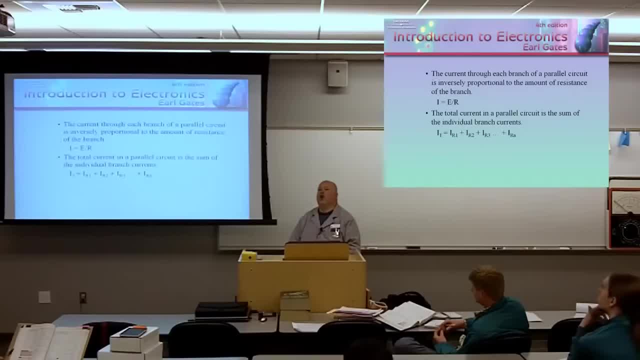 the sum of the individual branch currents. That's why we call parallel circuits current dividers. Thank you. Current dividers, Reciprocal of the total resistance in a parallel circuit, is equal to sum of the reciprocals of the individual resistances. 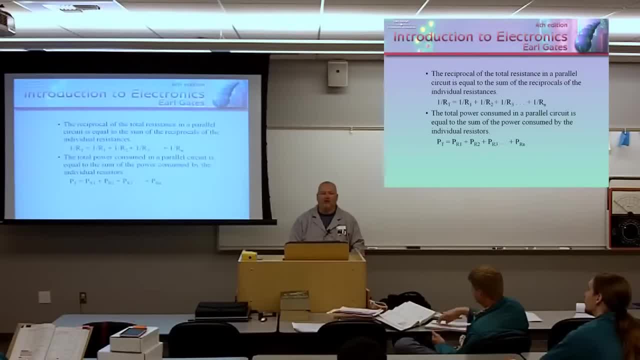 This is a fancy way of saying. when we put resistors in parallel with each other, we actually add up the, the reciprocals. We add up the conductance of those of those paths, not the resistance of those paths And the conductance of those paths. 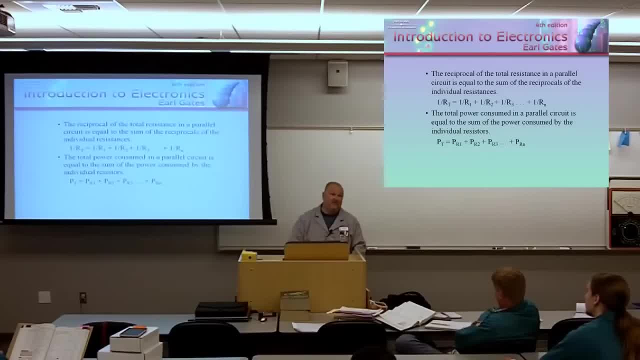 literally, is the reciprocal of the resistance Seaman came up with. right, That was his whole trip. The other formula that I want you to be aware of- and I know some of you are resistant, reluctant to use it- is the product over sum formula. 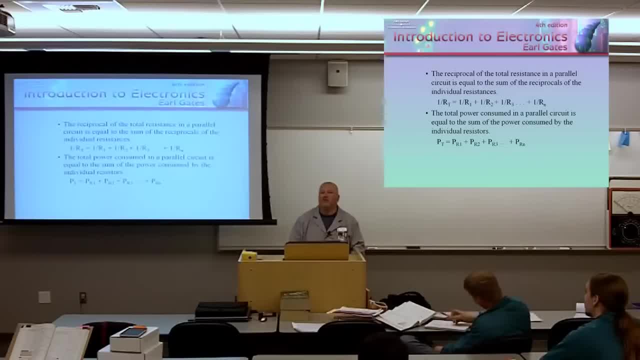 If you've got two resistors or two resistances in parallel, use the product over sum formula. Product means R1 times R2 divided by the sum R1 plus R2.. And it's a real easy way. I mean, it's what's the you know. 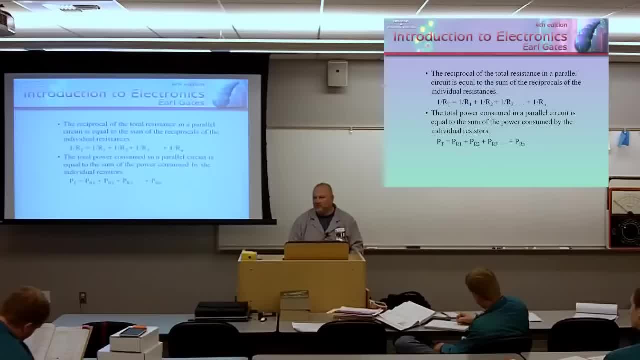 you got a half inch nut that you need to get loose. You know you could either use- you know- the box and the wrench, or you could use your teeth. Use the easiest tool. The easiest tool is the product over some formula. 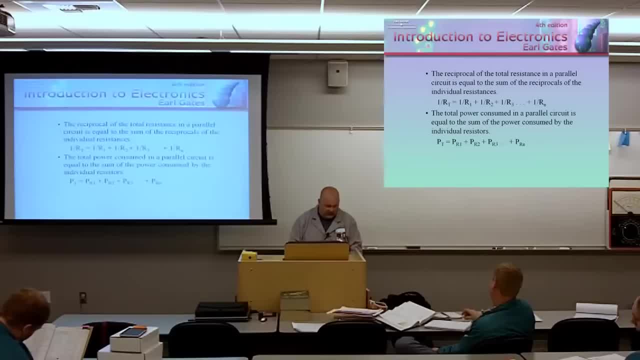 Well, that's another formula we got to memorize. Don't memorize these formulas, Use them and learn them. You understand the difference. Memorizing stuff never worked for me. I mean, that's always my fear that I'm gonna get pulled. 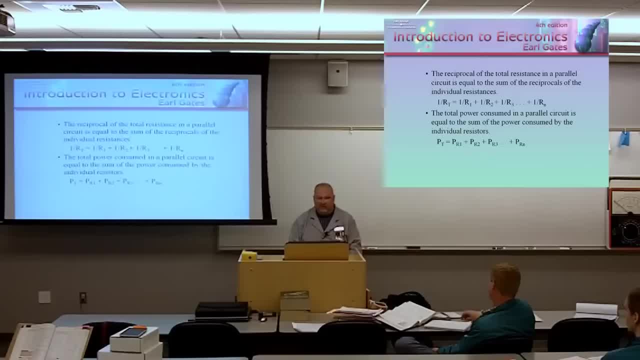 That's why I don't drink and drive, because I get pulled over even if I haven't been or, you know, if I'm not totally under the influence. they're going to ask me to do the ABCs and I'm probably going to screw that up. 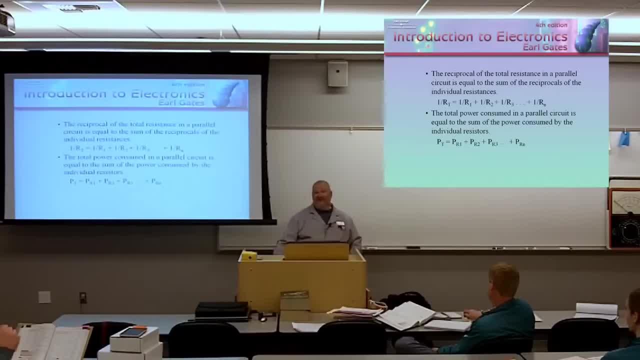 They're going to throw me in the hoose cow because they don't know my ABCs, Because I never really memorized them. I kind of like learned them Saying backwards: I mean, how do you do that crap? You can't freaking do that. What the heck are you. 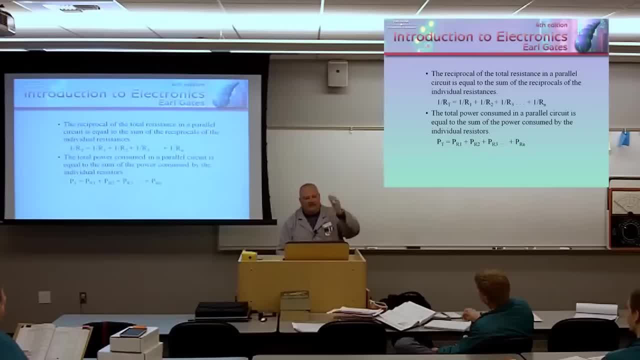 doing While hopping on one foot. you know, recite the alphabet backwards. No man officer, with all due respect, let's see you do that. Huh, Jeez, you're killing me. Total power consumed in a. 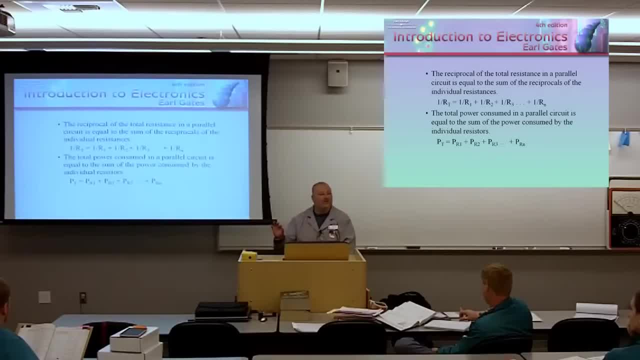 parallel circuit is equal to the sum of the power consumed by the individual resistors. No mystery here. We just talked about it last chapter. Power is always. That's beautiful. What were you saying about the part of some formula when you can only use that in a parallel? 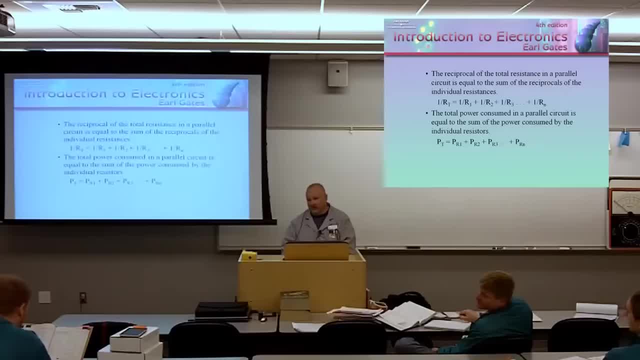 circuit Correct. If you only have two components in parallel, Two or more, you gotta use your favorite formula. The reciprocal of the total resistance of parallel is equal to the sum of the reciprocals of the individual resistances. A lot of. 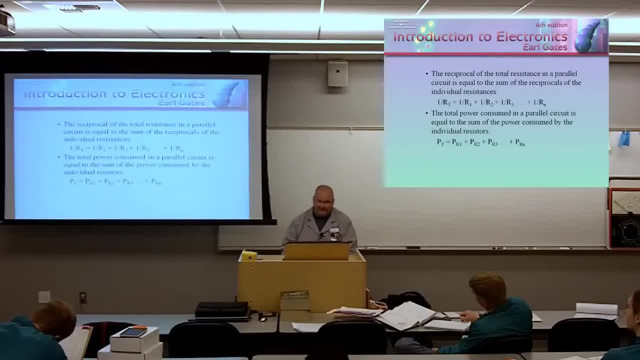 people like that one more than mine. Mine is only good for two. Also, with that, don't forget your thumb rules. Remember your thumb rules? Right, If it's equal resistance, you simply count up the number of resistors, that value of resistance and divide. 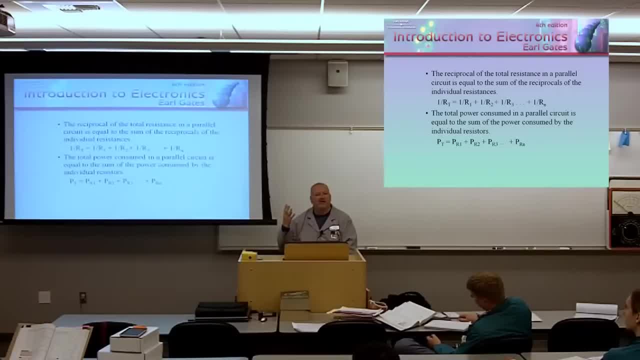 it by that number. If I have four 100-ohm resistors in parallel with each other, what's the total resistance? Four 100-ohm resistors in parallel with each other, 100 divided by equals 25 ohms of. 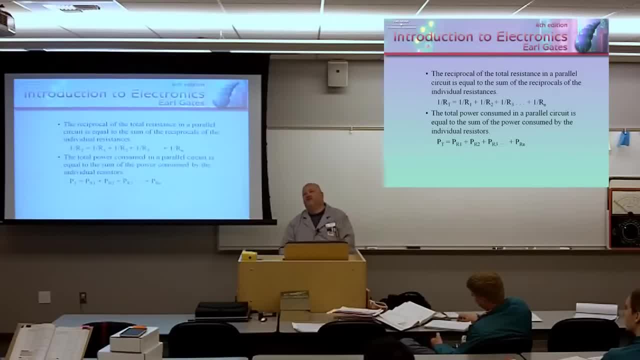 resistance, The other thing for resistors. in parallel, the total resistance will always be less than the value of least resistance. It'll always be less than the value of least resistance. Thumb rules. You pay attention to those thumb rules? your GPA is going to increase drastically. 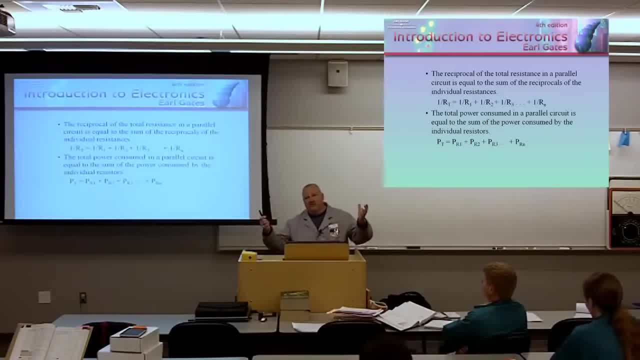 Because you're going to have something to check yourself against. I don't know if I used the right formula, but I remembered you always said the value of least resistance will be less than the value of least. My answer meets that. I'm comfortable with that. 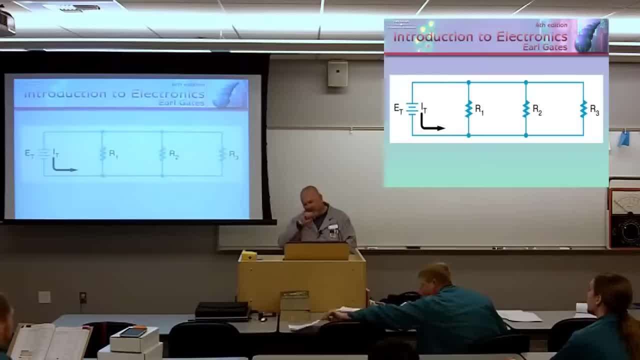 answer. Stick with that answer. Power is additive. It's a parallel circuit. Remember how we said: voltage is constant across a parallel network. That's because this electrical pressure being exerted by this source is distributed equally across these three loads period. 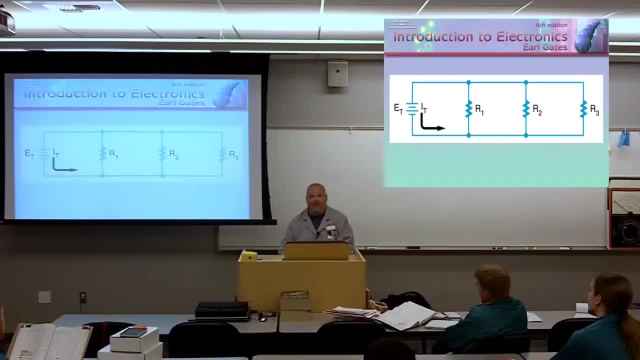 It's the same. It better be the same. If it's not, we got a problem. If it's not, we got a problem. Where's the missing voltage? This is how your house is wired in parallel: The outlet in your bathroom. 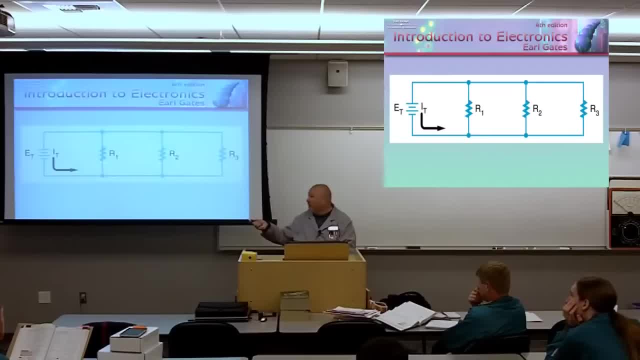 better have the same voltage across it as the outlet in your family room, as the outlet in your garage. If not, it's not wired properly. Something's up. I got a big circuit like this at home Because I do everything big. That's how I roll. 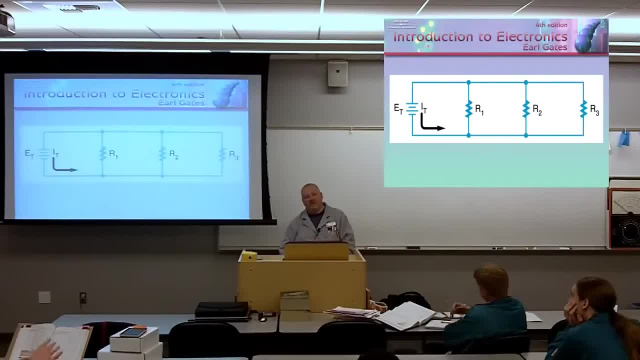 I made some significant improvements to my backyard about ten years ago. My backyard used to come out and it used to drop off- Drop off a hill- and it was just an unusable backyard. I wanted to like, do stuff back there. You know what I'm saying. 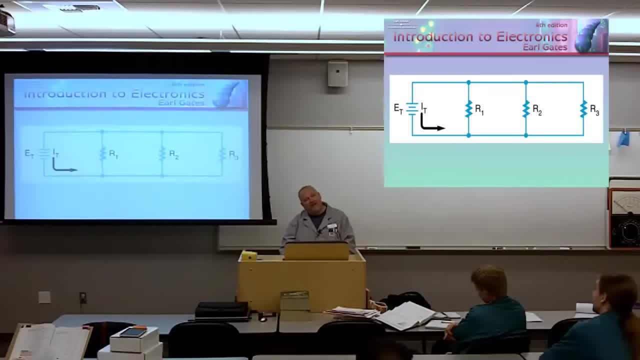 You know what I'm saying. So I was looking at- I had to build a retaining wall, Talk a big box to put in a nice retaining wall. So I was looking at different options And I like to utilize the resources that are. 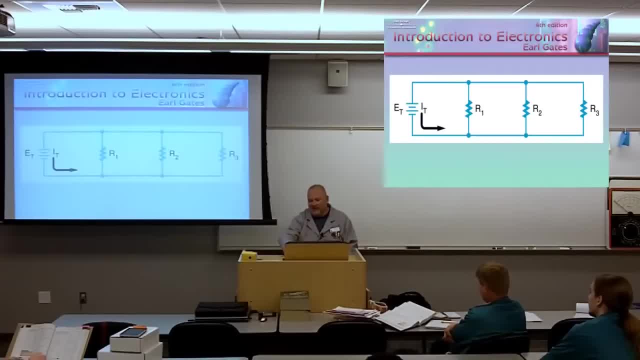 available to me. So I have a good friend of mine that worked for the railroad Burlington Northern And I said, hey, you know, you guys use those railroad ties. You know what are the chances of getting some of those railroad ties. 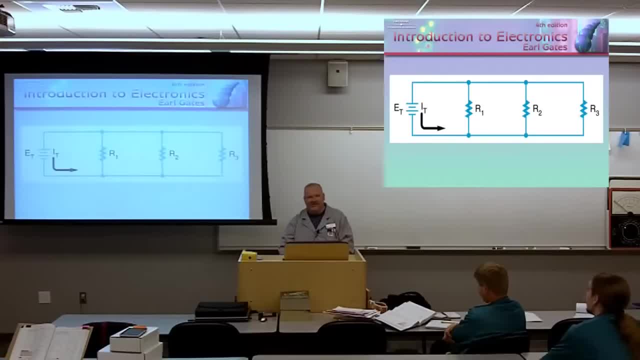 You know like what are you talking about? Oh, like a truckload. You know those are hard to come by, Joe. You know it ain't what it used to be. So for like three years I kept hitting him up for railroad ties and wasn't. 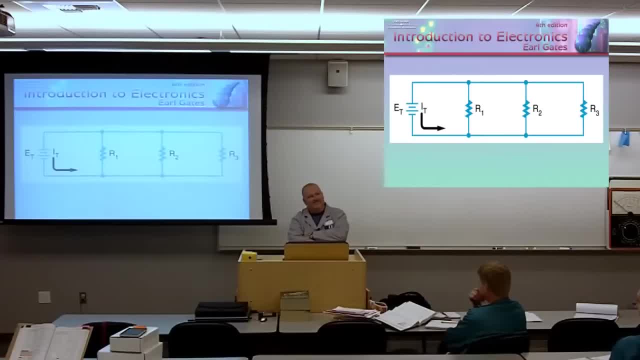 getting anywhere. And you know we had a great relationship. Finally, he said something He was kind of hitting around about going for an airplane ride. You know he was hitting me up for an airplane ride. And finally, and I'm not the quickest- 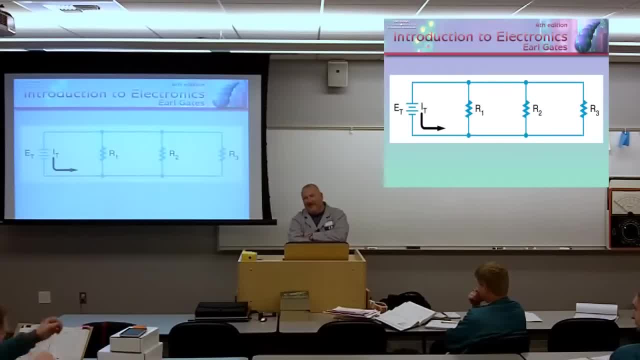 study the smartest guy out there, sharpest tool in the shed. I finally like, oh, I get it. So I gave him a call like: hey, Larry, what are you doing Monday night? You know, want to go. 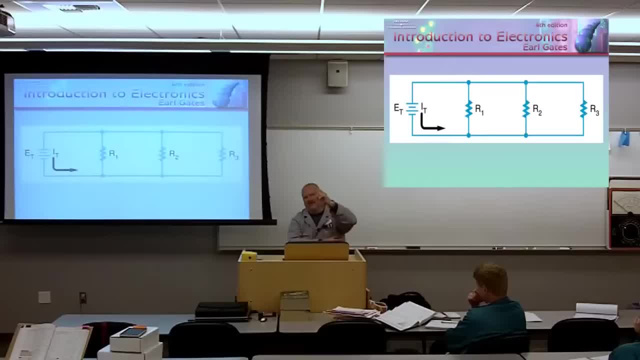 for an airplane ride. I picked him up in Arlington and we went out over the Cascades- beautiful sunset. whatever landed Right That Wednesday. my cell phone is ringing. Hey Joe, still want those railroad ties? Yeah Well, I got clearance, not only to give you the railroad. 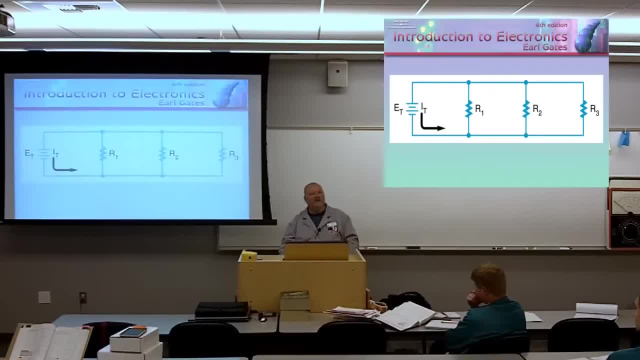 ties. but I got clearance to use a Burlington Northern crane to load them on a truck for you. Okay, You just got to get the flatbed. So I went out and rented a flat. I drove literally. it was funny, it's Burlington Northern but it was a yard up. 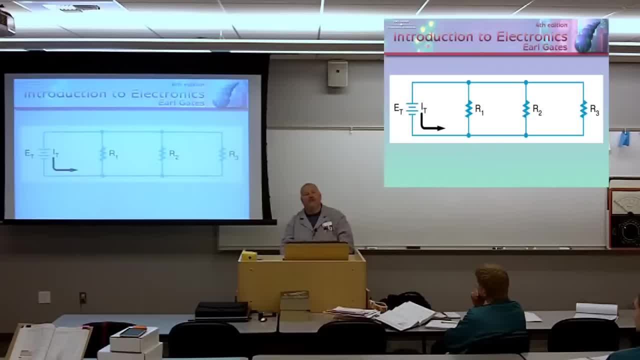 in Burlington, So I had to drive all the way up there. He loaded them on 148 ties. Long story short, I built a beautiful retaining wall. Actually, I had a former student of mine that was an engineer. He designed the wall for me. 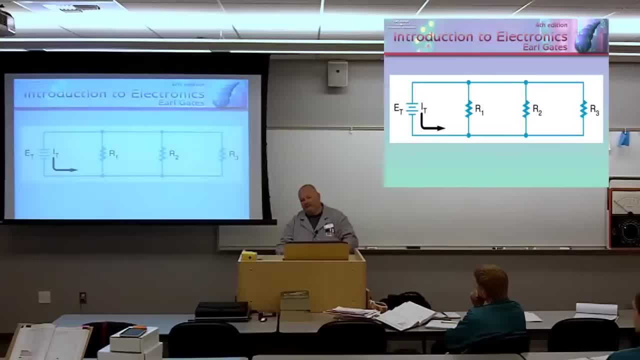 You know, did the prints and everything, Built this wall and landscaped it beautiful. So now I have a backyard. My neighbors, they weren't digging it, Because now they're looking at like, you know, he's got a perfect yard, Are we still, you know? 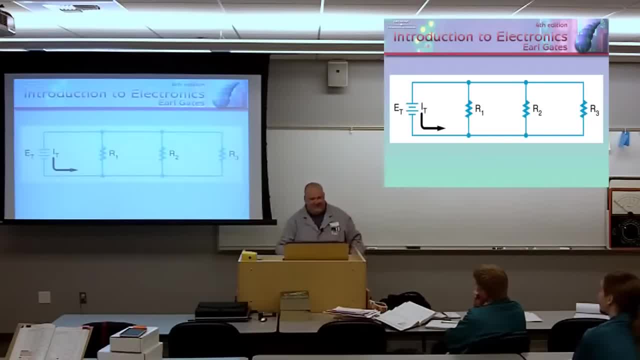 just like a wall. you know railroad ties- Funny part of that story too: that entire. I built that by hand- 148 ties. I don't know if you've ever picked up a railroad tie. They are heavy. I built that by hand. 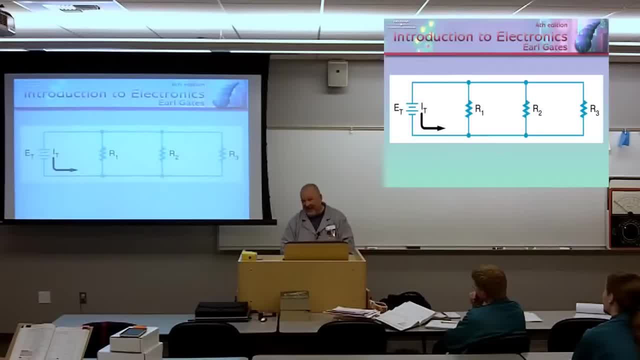 Backfilled it by hand with a wheel barrel Gravel Drainage By hand. You know how much weight I lost that summer Zero. Probably had something to do with the pizzas and beer I was consuming while I did it, But anyway. 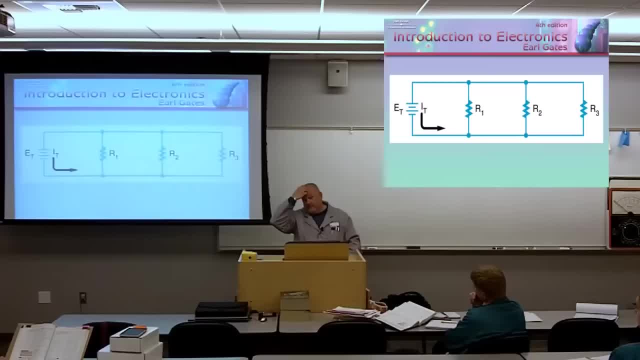 what I wanted to do is I wanted when I was, when I was all landscaped and everything in the process before landscaping, I wanted to put in low voltage lighting. Low voltage lighting around the perimeter. So you know, like these, the goofy- 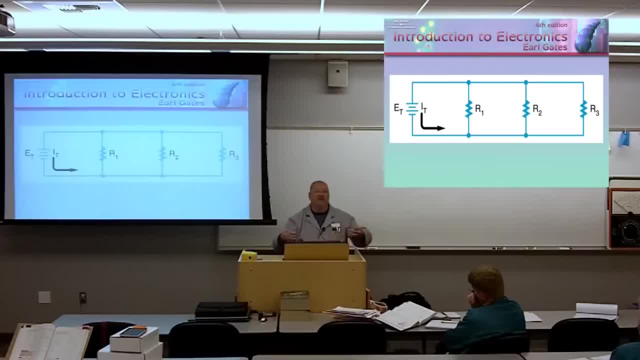 lights you stick in and you know the. but I wanted to put in conduit. I wanted to do this right And as a pilot, I kind of wanted it almost to look like a runway and you know an airport. You know the. 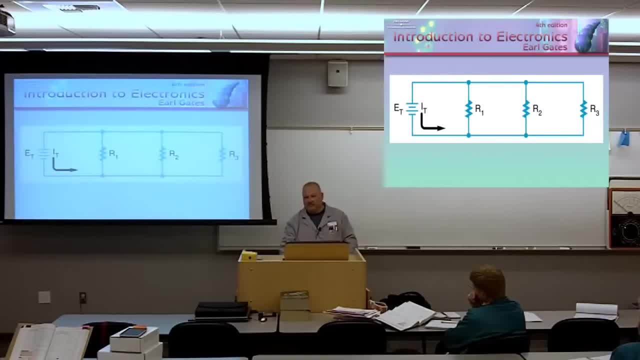 lights around the periphery, So I used these low voltage lights. I had a big power supply in my garage and an equipment rack, Dug conduit all the way back, Did my calculations And the other thing about calculations, determining what size wire you should use. 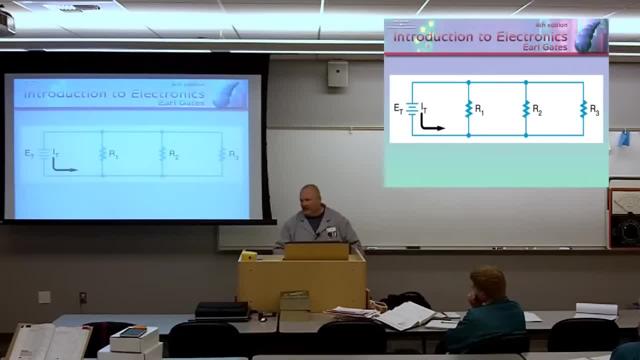 The kind of wire that I use is the kind that falls off the back of a truck, You know, and the kind that contacts provide me with. So I went with this gauge of wire. It was a little bit substandard, but you know. 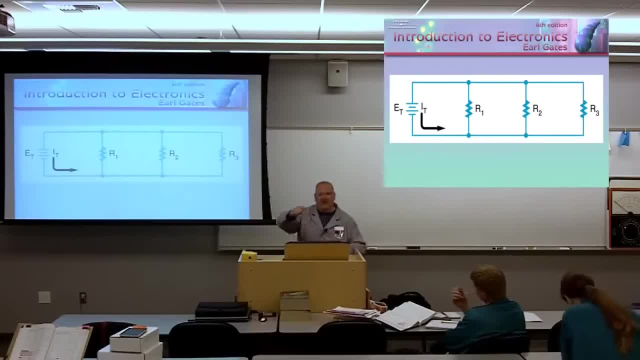 the math kind of works out and it's kind of good. So I've got all these low voltage lights and ironically, ironically, it came out nice, Came out really really nice, Nice backyard. But I could tell, If I brought you back there you probably 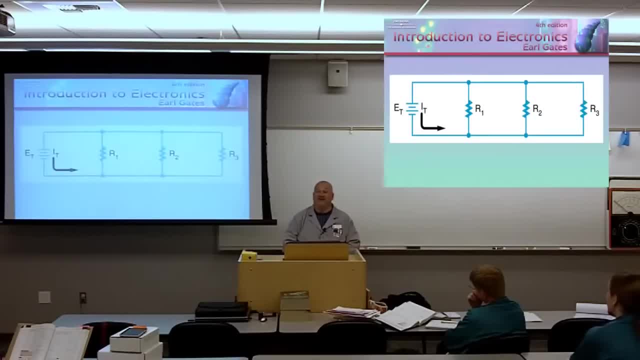 wouldn't even notice it, But I could tell which light is the furthest from the power supply, Just looking at it And it kind of bothers me. It doesn't bother me enough to rip up the conduit and pull new cable, okay. 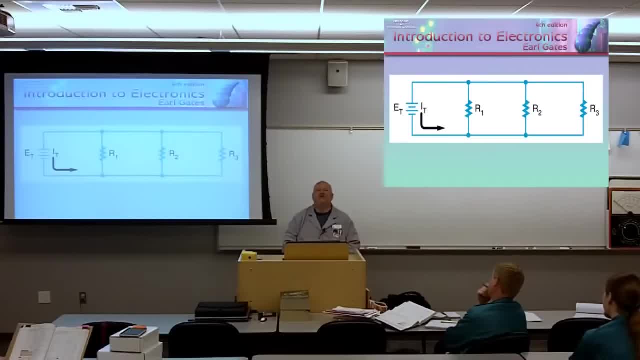 But I know, I know by looking at it. And what does that tell me? That tells me that the load furthest down the line is not getting the same voltage as the load closest to the source And gradually, as you get further away from it, you just notice. 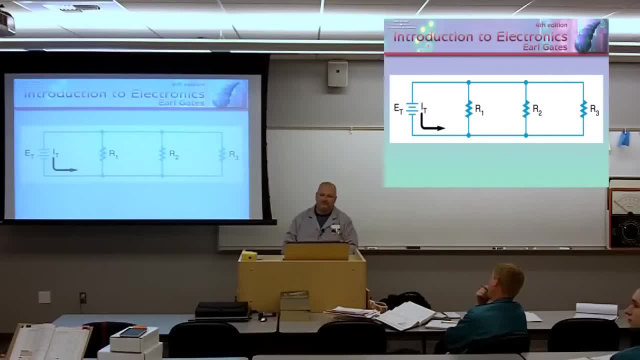 a little difference in illumination. Shouldn't voltage remain the same in a parallel? Yes, That's my whole point. Why doesn't it So? as long as it's distant, you just need a different bulb that's more efficient. I needed. 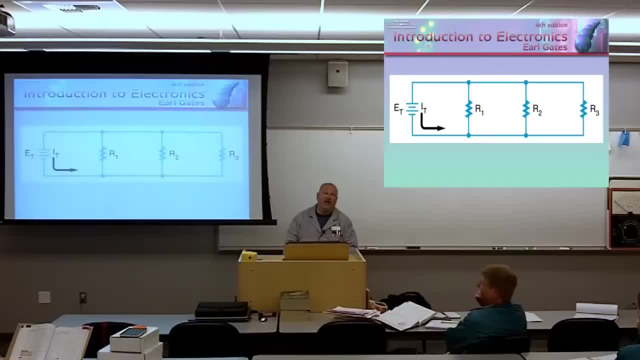 to use basically a heavier gauge of wire And in doing that, if I had done that, then I could. yeah, there's ways I could fake it: Soldering- What are you doing out there? I'm soldering in resistors to these other lamps. 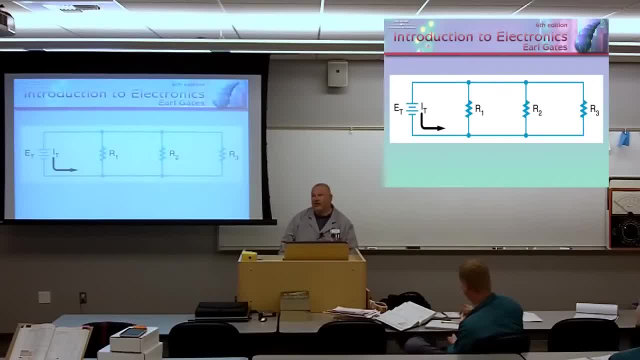 Why'd I get it? My wife would probably finally really give me the boot, But it bothers me. It bothers me because I like doing things right, And I guess I did do it right Because you know how much that wire that I used cost me. 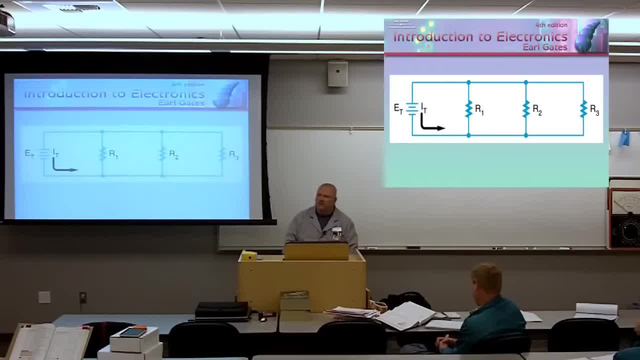 Literally fell off the back of a truck. So you know, Don't judge me- I have a friend that's a police officer. I asked him. I said: you know what's the whole deal Like if I got something that fell off the back of the truck? 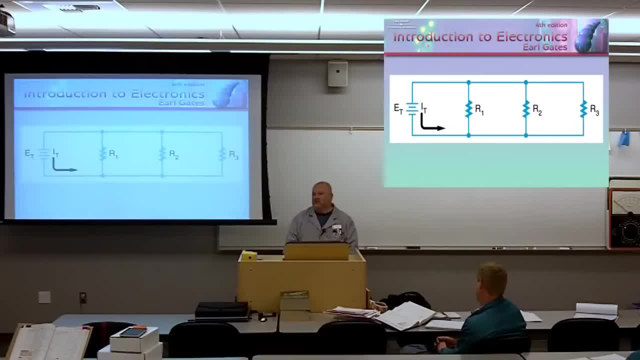 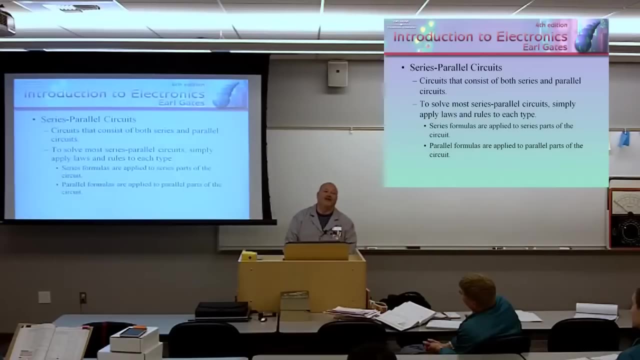 He like sat up and he's like, you know, I'd love to cite the driver for driving an unsecured load, You know. Anyway, so this is a parallel circuit. Now, yes, You know, that's one of the other things I was kicking around. 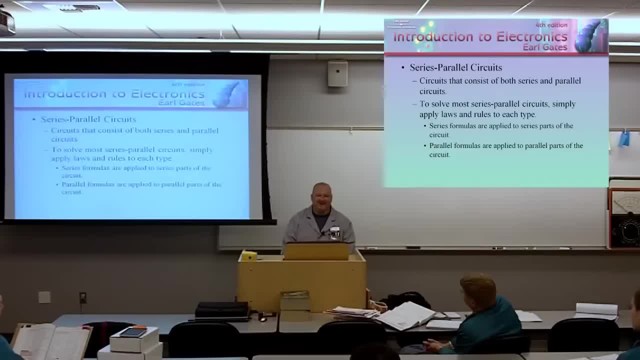 Can I stick an inert gas in there? and you know, increase the dielectric properties and you know She'd throw me out. man, She'd throw me out, And you know what. I know you find this hard to believe. Maybe you won't. 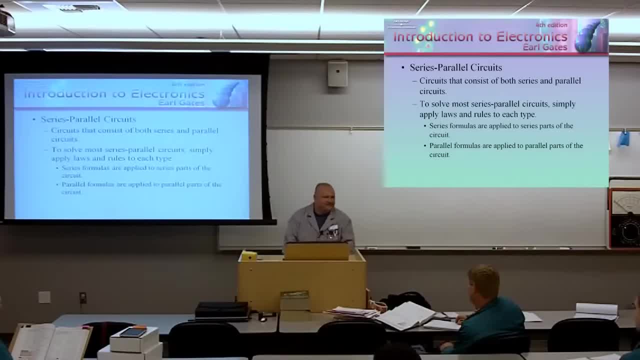 But I actually have a nitrogen bottle at home, Doesn't everybody? And I don't necessarily use it for welding Series parallel circuits- This is the easiest part of this entire chapter: Circuits that consist of both series and parallel circuits. To solve most series parallel circuits, simply apply the laws. 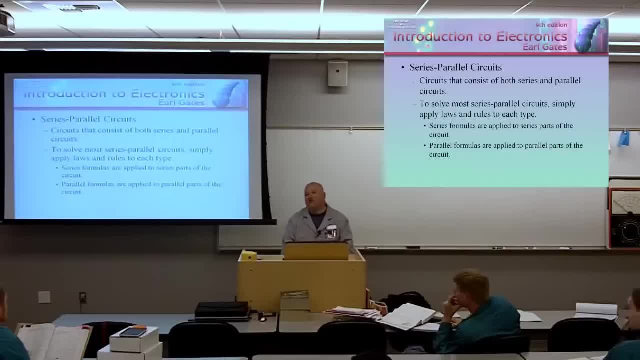 and rules of each type. There's no mystery. There's no silver bullet. There's no easy way for me to describe it to you. Use series formulas for the series parts of the circuit. Use the parallel for the parallel parts Period. 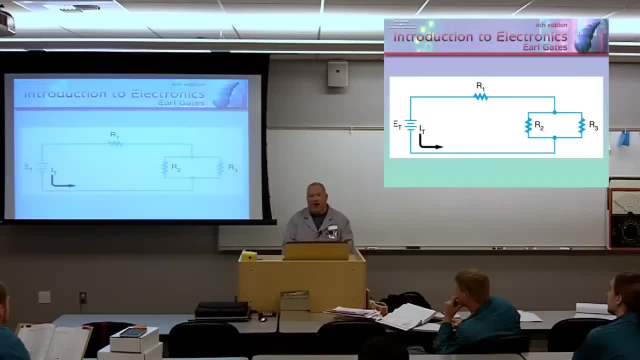 That's all it is. That's all a series parallel circuit is. That's what it looks like. R2 and R3 are in parallel with each other. You've got to solve for that before you can solve the total resistance, Because R2 and R3,. 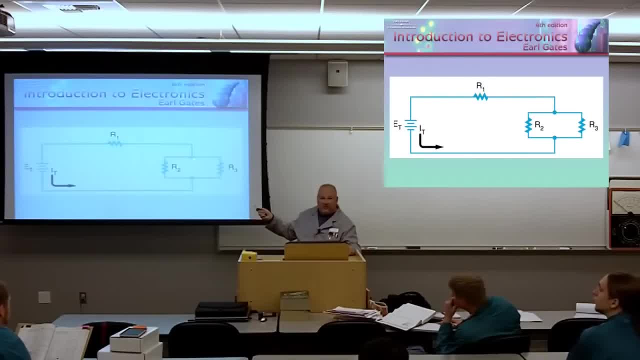 one of the things that I like to do is identify these points right here. These are called nodes. I'm going to call this node A and node B. The resistance between node A and node B is equal to the parallel resistance of R2 in parallel with R3.. 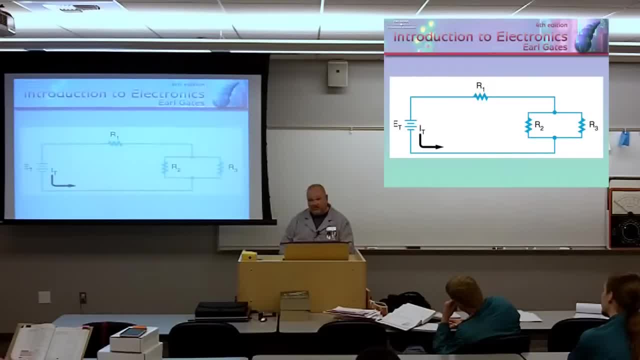 I'd use the product over sum formula to determine what RAB is. Follow what I'm saying. RAB: the resistance between node A and node B. The total resistance in the circuit is equal to R1 plus RAB- RAB. 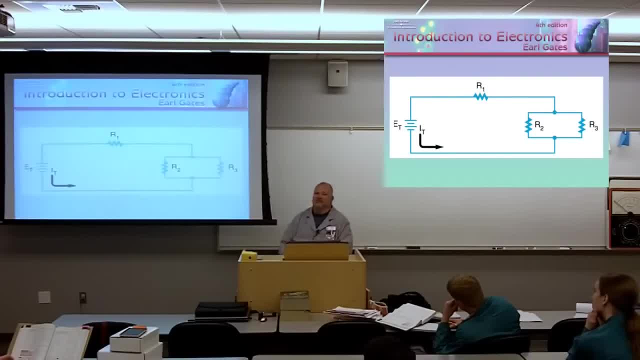 that's what equals total- Excuse me, total resistance. Total current can be determined by that. Once I know what total current in the circuit is, total current is going to create. a voltage drop across this resistor, Total current is going to create. 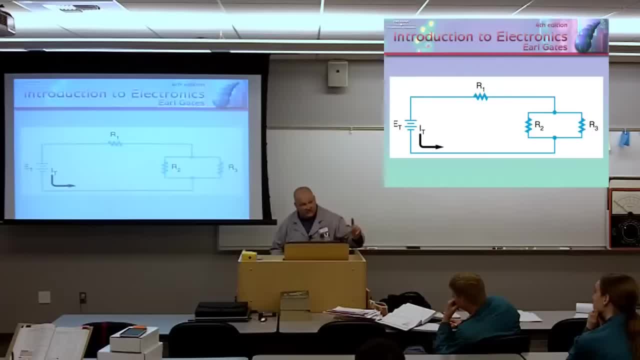 a voltage, drop across this resistance. The resistance I'm talking about is the resistance of AB, which is the combination of two in parallel with three. Make sense. Once you do that, it's just easy to slice and dice. The worst thing is: 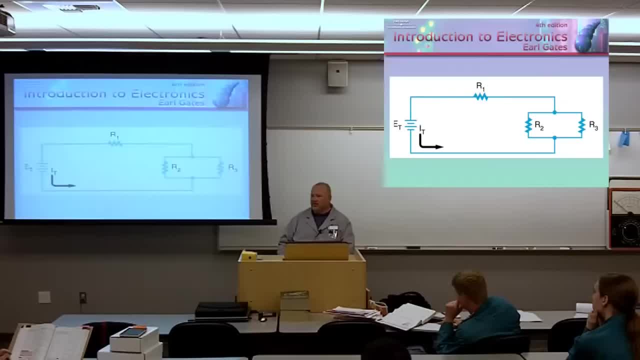 when you see, Obviously we gave you some problems in the assignments of the book that take time for you to solve, But the first thing you've got to do is break it down. The other thing, too, is if I had a resistor. 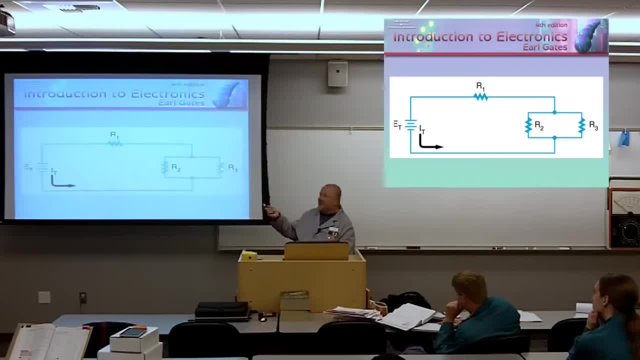 in series with another resistor. here I'd need to solve for these two first, because they're in series with each other, But in parallel with this. So then I need to solve for this series, This section of the circuit which is in series. 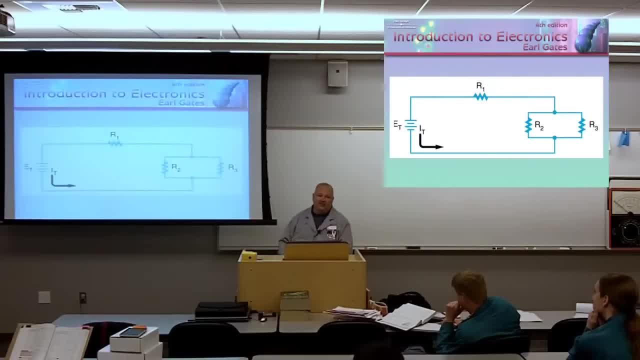 with this section of the circuit. So you know a lot of students get frustrated and think there's a checklist they could follow or a protocol. No, you've just got to pay attention to the individual laws and rules that we establish. But there are no two circuits alike. 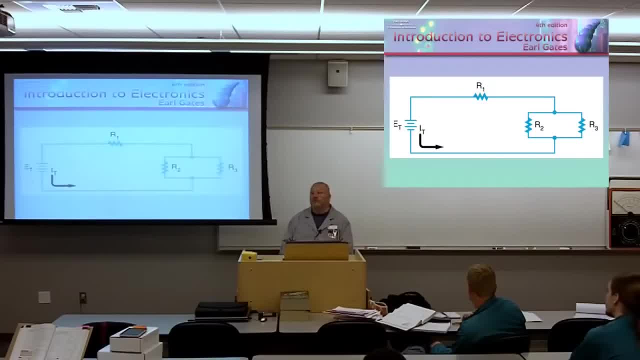 One of the things that I've heard over the years of teaching here. I get a lot of new students that come and or you know, quite frankly, a lot of people they're working in industry already and they want to come in. 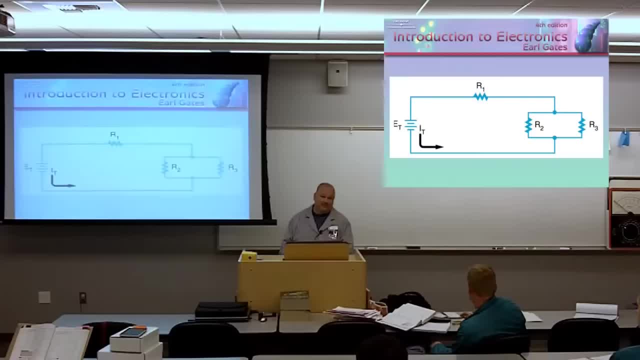 and they want to learn how to read schematics. Joe, if I come to your program, can I learn how to read schematics? Well, yeah, but we don't have a schematic reading class. There's no schematic reading class And, quite frankly, 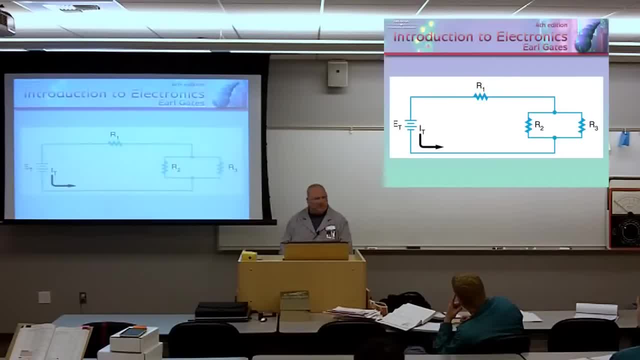 I wouldn't want to have a schematic reading class- even if I could fill a schematic reading class- because you wouldn't learn anything. What are you doing here? by studying this, You're learning how to read a schematic. You're learning to differentiate between those sections of the circuit. 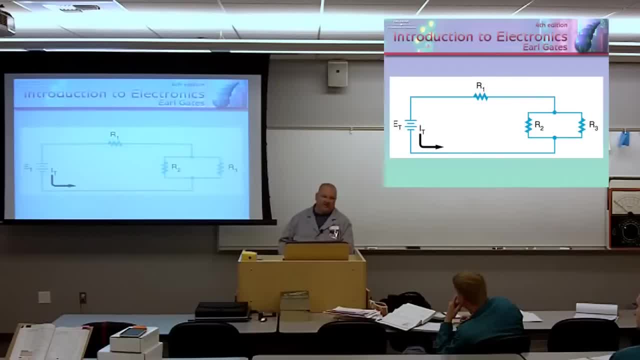 that are in parallel with each other and those sections that are series components Later on, when we talk about transistors right now, those of you in the full-time program did a component ID test today to be able to recognize different types of components. 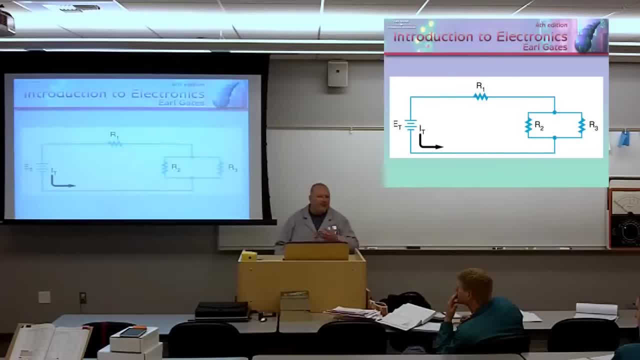 You're going to see what happens when we put a transistor, a diode, a capacitor, different components in different configurations. If I put a capacitor in series, all as it is is a capacitor in series. It's still a series circuit. 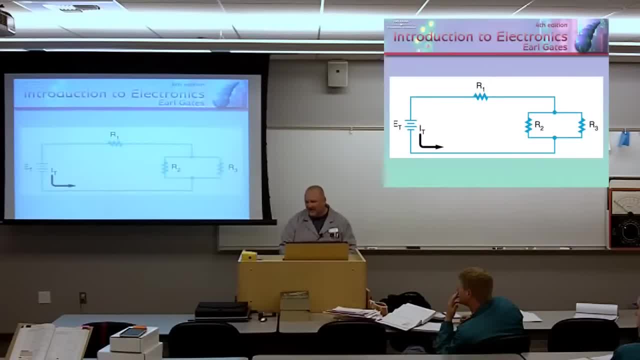 And everything that we've talked about this week still applies. There's going to be some things that are going to be a little bit different with a capacitor in a circuit. We'll cross that bridge when we come to it, but it's still a capacitor. 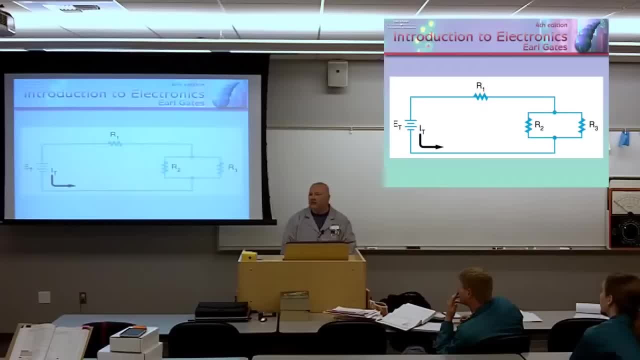 connected in series And there's really only three types of circuits that you're ever going to deal with in your entire career, And that is series, parallel and complex. So if any of you this week have been grunting, groaning- 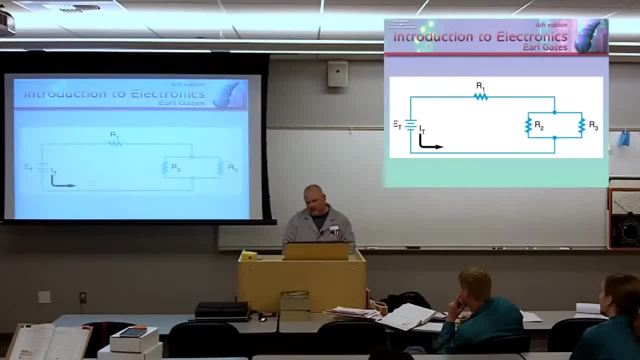 outside weeping, gnashing your teeth. you know what? It's all right, Because once you master series parallel complex, there's nothing else I'm going to throw at you. There's nothing else that Peter's going to throw at you. 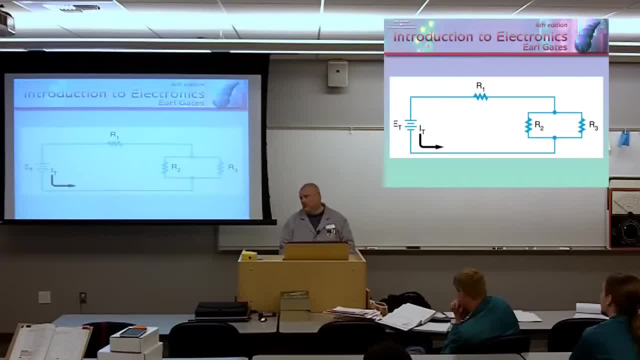 Now, that being said, we're going to have you looking at some complex circuits in the future And you know what? You will deceive me As much as you could pass this test on series, parallel complex circuits. you're going to forget about it. 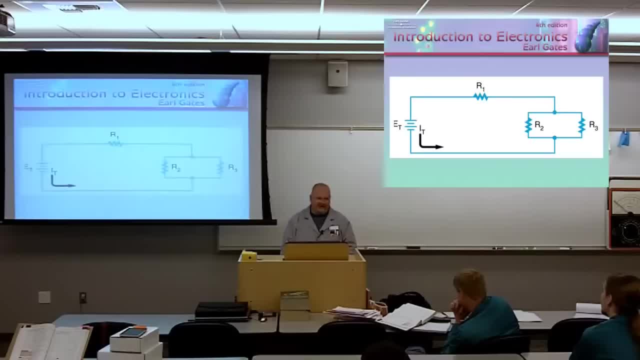 in the future, Because we're going to give you some schematic to read: that's got some different components on it, or it's got some components drawn at weird angles or something, and you're going to get your freak on And you're going to say: 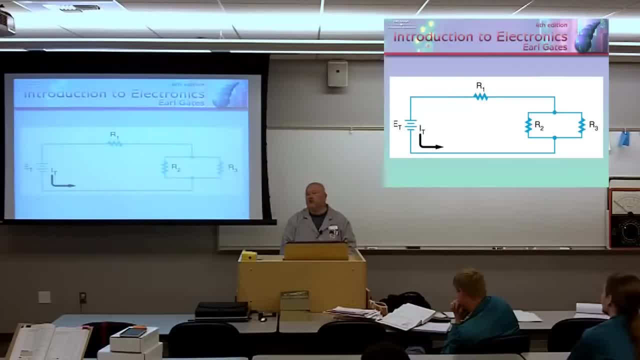 boy. they never taught me that I don't know what to do. You know what you do. You fall back to the base. The only circuits you're going to encounter in industry are series, parallel, complex. And if it's complex, 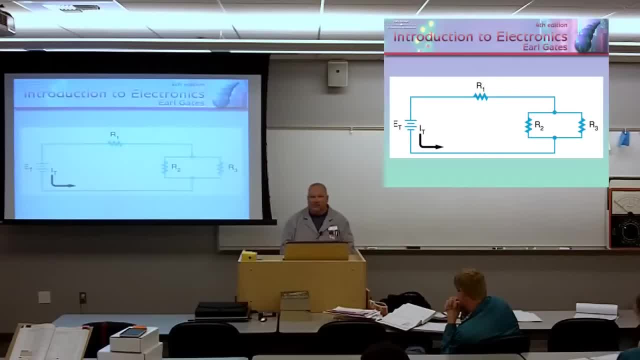 what laws do you use, Those of series and parallel? You've just got to figure out which components are in series and which ones are in parallel. I can't say it any stronger: If it's in series, there's one way in. 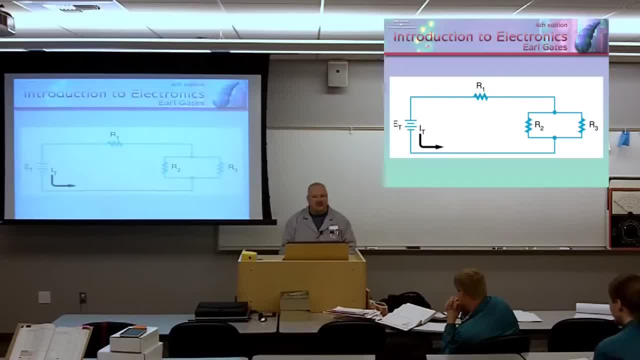 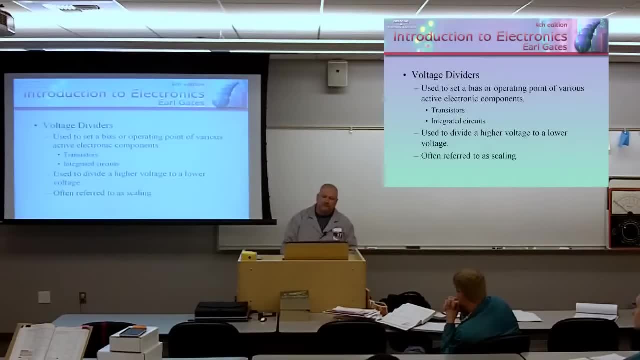 there's one way out. If it's in parallel, that means there's interconnection of all the components. Make sense: Voltage dividers Used to set a bias or operating system point of various active electronic components. We use voltage dividers to create the voltages. 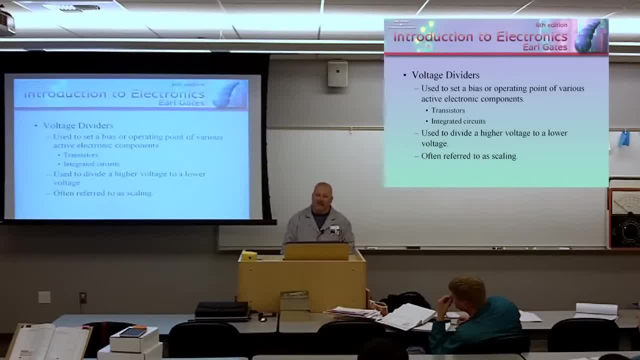 that turn on transistors and integrated circuits. They're used to divide a higher voltage to a lower voltage, And this process is often called scaling. Because what are we doing? Voltage rise equals voltage drop or voltage drops, So voltage drops will always be. 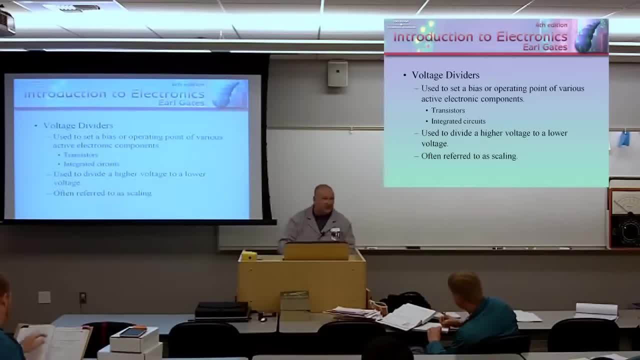 a fraction or scaling of the total voltage that we apply to the circuit. Does that make sense? We're going to use Ohm's Law to solve that. That's the current to a circuit. I'm not done with voltage dividers, Trust me, I'm not done. 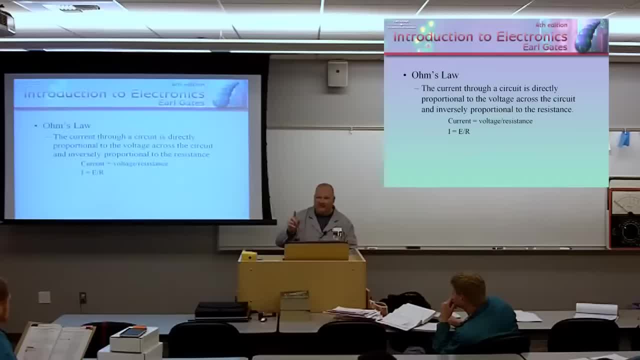 I'm done when the screen goes black. No, I'm not done. when the screen goes black, Then I'm going to show you some stuff on the board. So sit tight, That's not my spiel on voltage dividers. Ohm's Law. 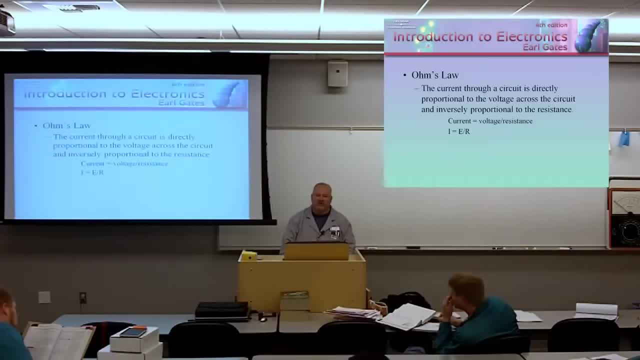 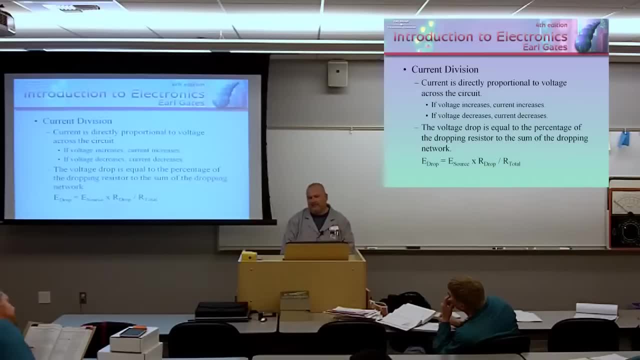 the current through a circuit is directly proportional across the circuit and inversely proportional to the resistance. Ohm's Law I is equal to E over R. Current division: current is directly proportional to voltage across the circuit. If a voltage increases, current increases. 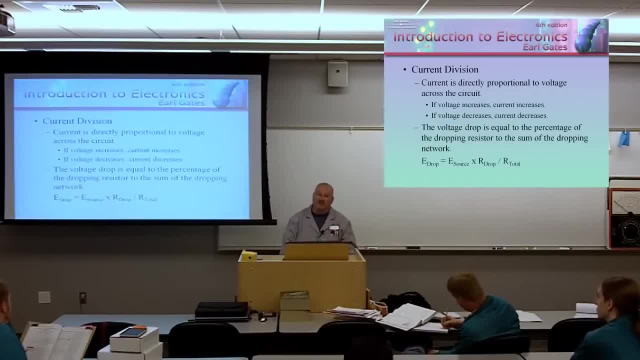 If a voltage decreases- current decreases- The voltage drop is equal to the percentage of the dropping resistor to the sum of the dropping network. You know what I'm giving you this formula. If you dig math, great. If this confuses you, 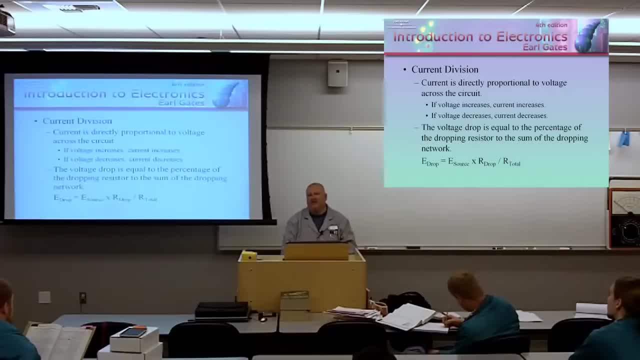 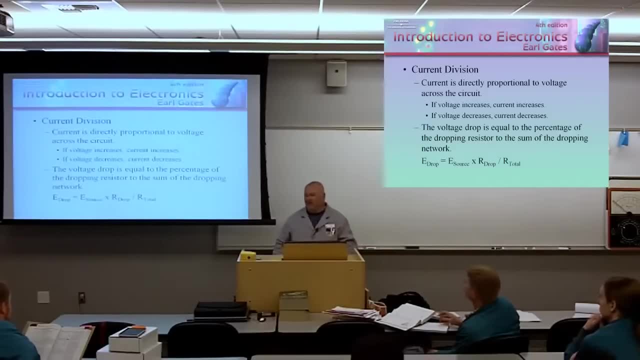 just tune me out, Because everything could be solved with Ohm's Law and Watt's Law. If you dig math, this is another tool in your box. Let me show you how this thing works If I want to calculate out my voltage drop. 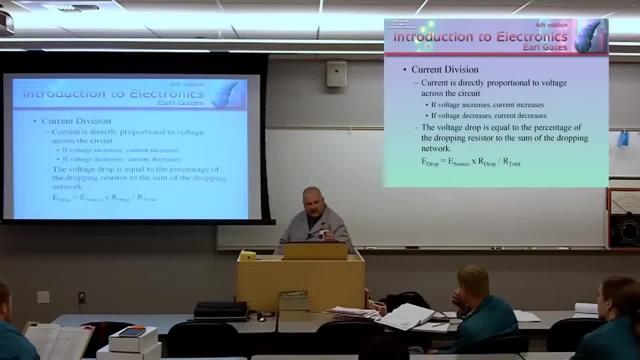 across a load, across a resistor. this voltage is going to be equal to my voltage source, multiplied by the voltage drop, divided by the voltage total. Okay, Let's keep this really, really simple so we can understand how this formula works. If I've got 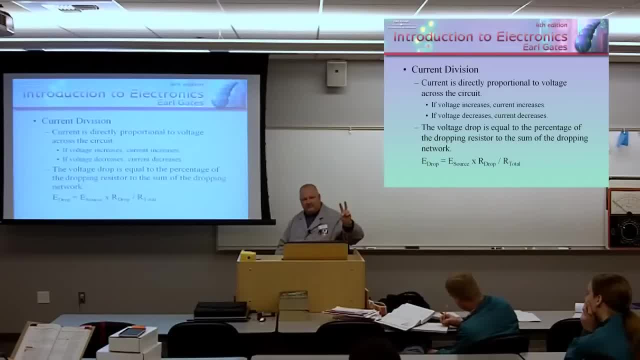 two 100-ohm resistors. if I have two 100-ohm resistors in series with each other and I want to know what voltage I'm dropping across one of those, I'm going to draw that You know what I'm talking about. 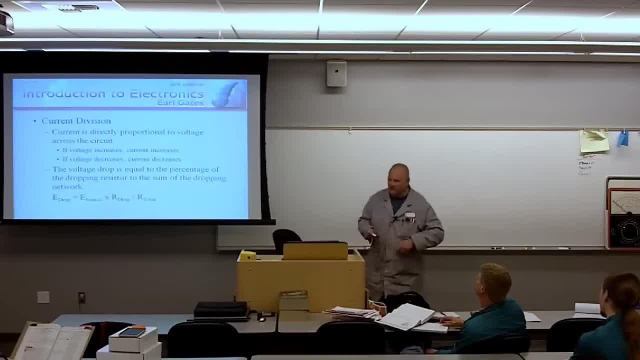 I should be able to use words, because the test I give you, the quiz, is going to be words. That's why I try not to draw too much on the board. I'll draw some stuff on the board, but I don't want to draw too much. 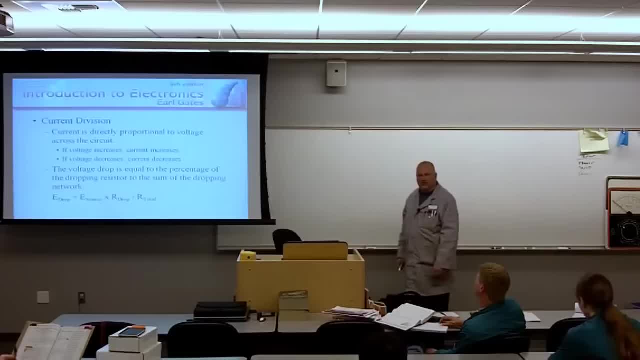 because, Joe, all week you've been drawing stuff on the board and then you ask me a bunch of words: Okay, You've got to pass the quizzes and they're words, word problems, Okay, But if I've got, If I've got this, 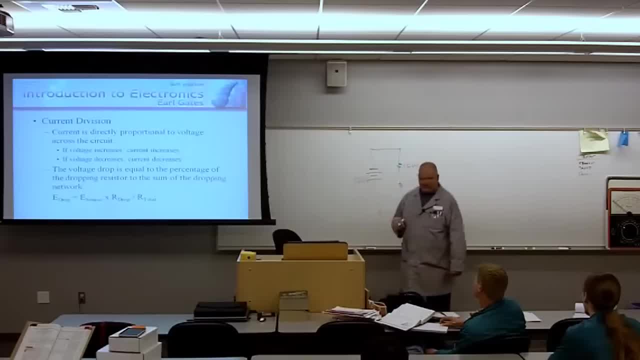 if I've got this and I've got 100 volts, let's keep this real simple. Okay, What this formula is showing me is: what is R drop? R drop here, V drop is equal to voltage total times R drop over R total. 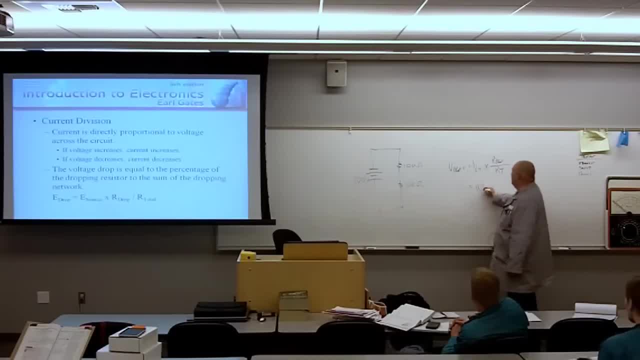 Okay, So let's take a look at that. Voltage total is going to be 100.. 100 volts times our drop, which is one of these voltage drops, whichever one you're trying to calculate for, Let's say it's this one. 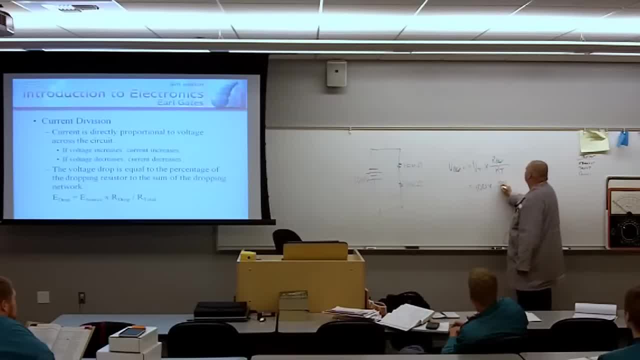 It's going to be 100 divided by What's my total resistance in a circuit? 200.. Okay, What's 100 divided by 200?? What is it? 0.5. 0.5.. What does 0.5 mean? 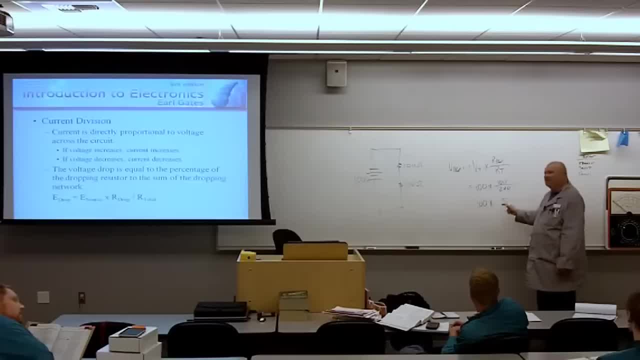 What percentage? Half Half, It means 50%. So 100 times 50% equals what? 100 divided by 0.5.. What does it equal? 50 volts? We could do this one in our head. That's why I want you to do this in your head. 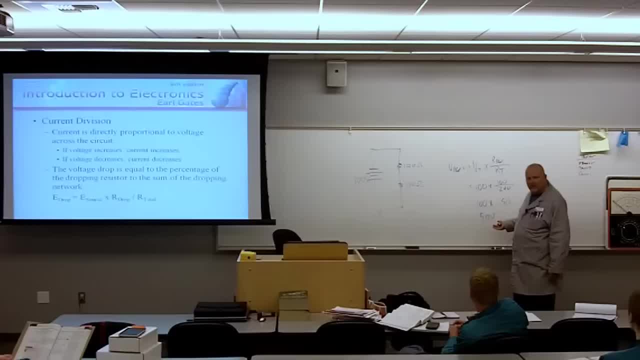 so you understand the formula, You understand how the formula works. So if you know what this value of total is and you want to calculate out, let's say that I went ahead and I changed this. now that this is This is You know, this is 500 ohms. 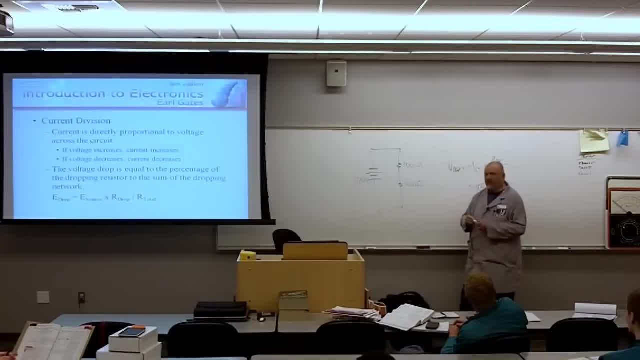 and this is 100 ohms And I'm asking you what voltage is going to be across this voltage drop here 100 divided by 5, basically 1 fifth, 1 fifth right. What percentage is 1 fifth? 2,, 4, 6, 8, 10,, 20%, right? 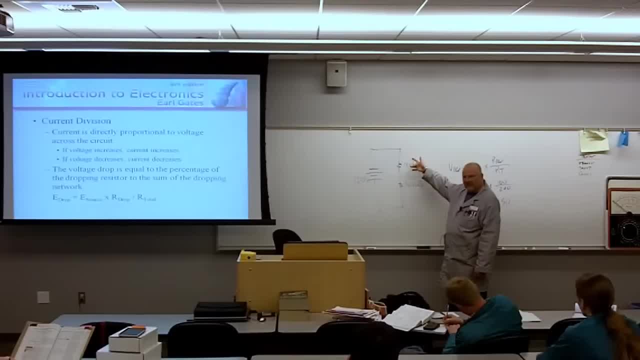 So that means 20% of my voltage is going to be dropped across this. If 20% is being dropped here, actually no right, Because this is 100 over 6. 600.. So what percentage is that? I was off on my math. 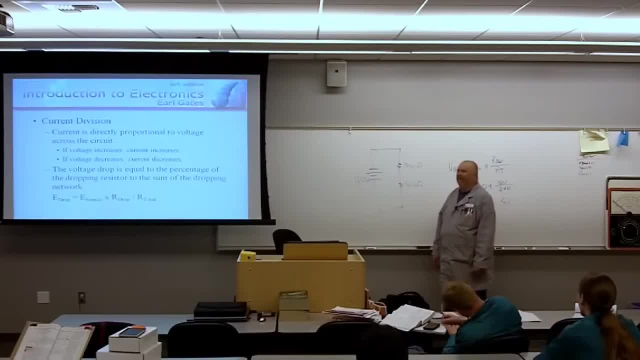 I'm sorry, You guys were buying it. man, I want to be your banker. What's 100 divided by 600? Because total resistance is 600.. 17? So basically, 17% is going to be dropped right here. 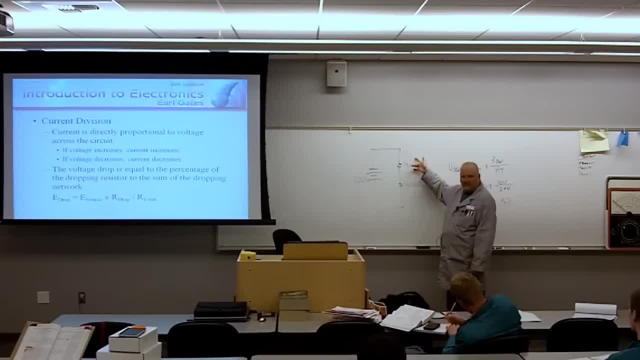 100, 17 volts is going to be here. The remainder is going to be: Where's the remainder voltage going to be dropped? This is an easy question. Right here It's got to be, Because this plus this has to equal this. 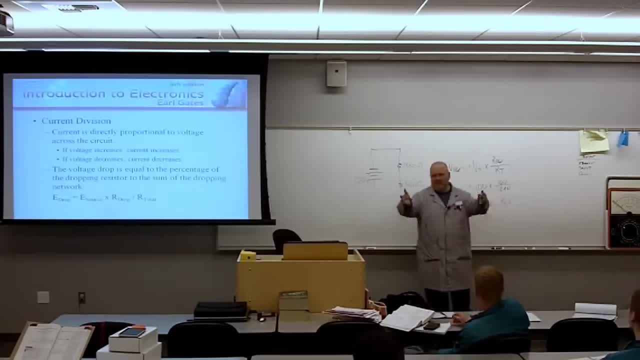 Does that make sense? So this is just another formula for those of you, the math addicts want another tool. I like tools. Just ask my wife. Got every tool right. This is another tool for you. So if I'm giving you, 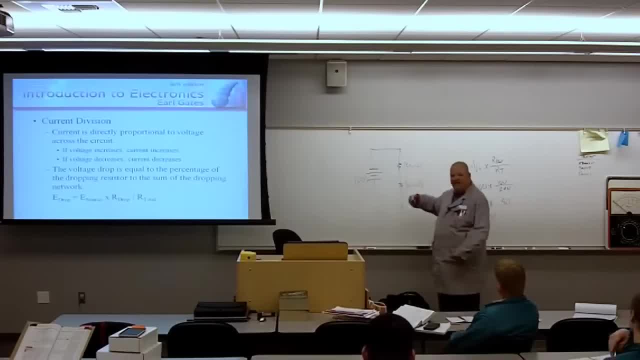 I could sit here all day long and tell you how much voltage is dropped here, how much is here. It's a lot easier to use this form, Although you could calculate the same thing using straight Ohm's law. It's just going to take you a little bit longer. 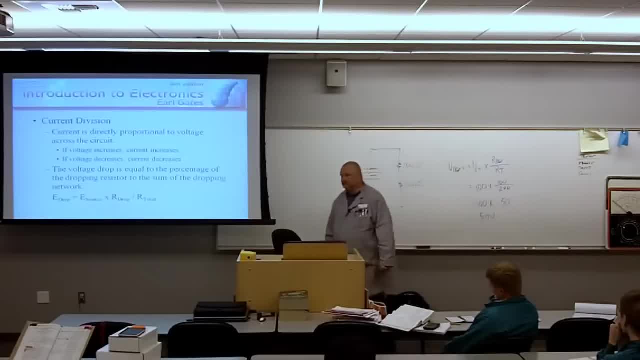 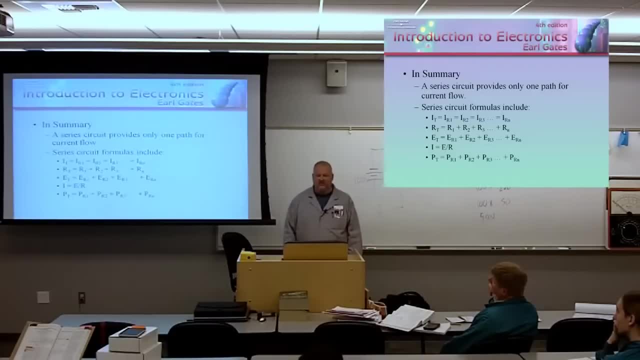 to get to the answer. Make sense, All right. In summary, a series circuit provides only one path for current flow. Series circuit formulas include: IT is equal to IR1,, equal to IR2,, equal to IR3,, et cetera, et cetera, et cetera. 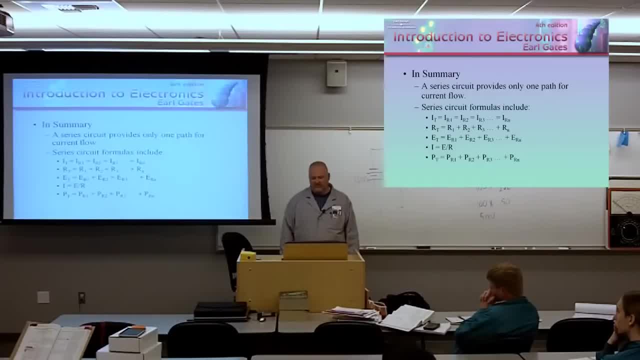 RT is equal to R1 plus R2 plus R3, et cetera, et cetera, et cetera. Voltage A series circuit is also known as a voltage divider, So therefore the sum of the individual voltages. 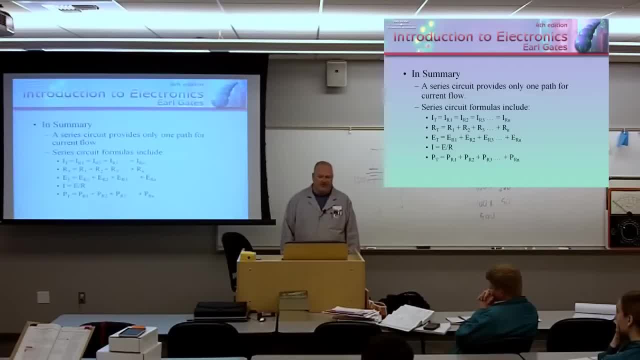 must equal source voltage. I is equal to E over R. Well, that's Ohm's law. Power is additive in a series circuit. Power is additive in a parallel circuit. A parallel circuit provides more than one path for current flow. Parallel circuit formulas include: 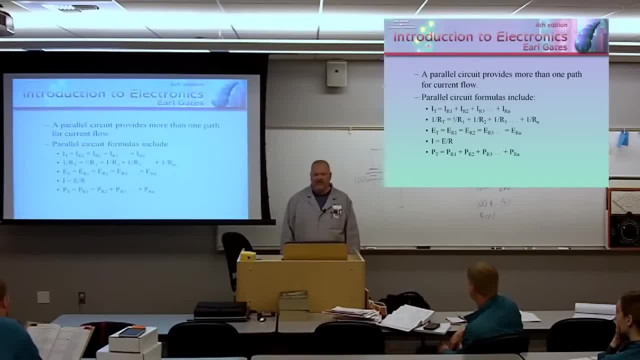 IT is equal to IR1 plus IR2 plus IR3.. The reciprocal formula for resistance Voltage is constant across a parallel network. Again, I is equal to E over R If you want to calculate how much current is flowing through an individual path. 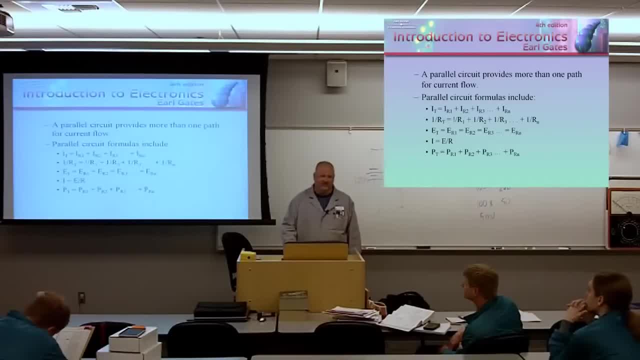 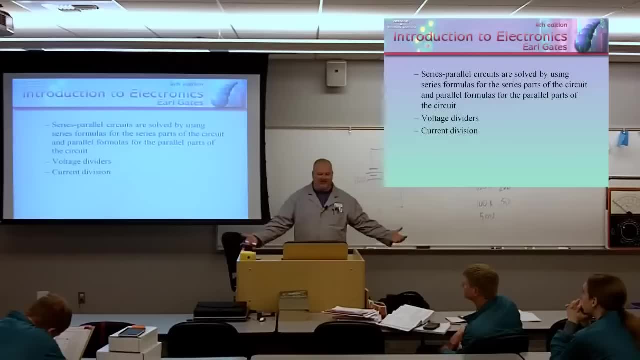 And power total is equal to PR1 plus PR2 plus PR3,, et cetera, et cetera, et cetera. Series, parallel circuits are solved by using series formulas for the series parts of the circuit. Parallel formulas for the parallel parts of the circuit. 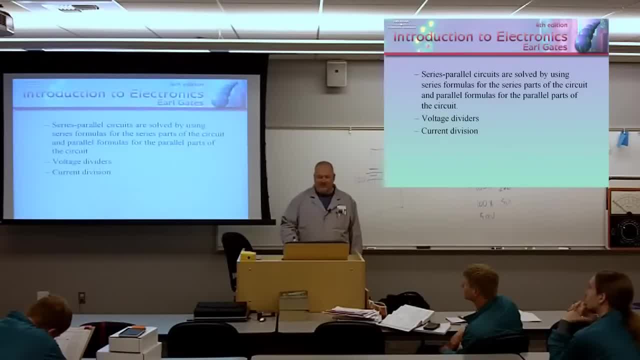 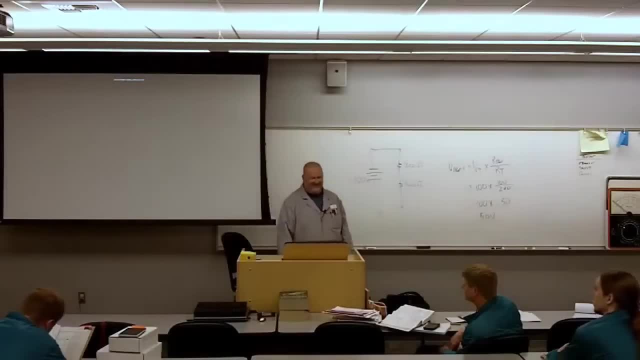 We talked about voltage dividers- More to come- And we talked about current division, The process of- excuse me, the process of current division in a parallel circuit. Any questions on this? Okay, Let's talk about voltage dividers. Kind of get emotional. 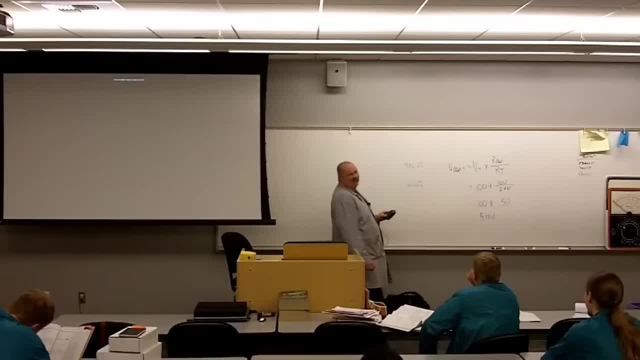 when I talk about voltage dividers, It's kind of like your first real circuit that really does something. Trust me, it'll be good. We're going to need some help, though, because we've got some electronic experts in here. We're going to need some help. 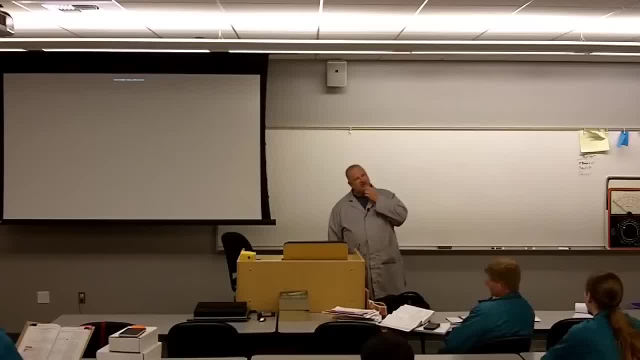 What kind of a circuit would I use to divide voltage? Series Series. You've got three to choose from. Multiple choice answer: Series circuits, parallel circuits or complex circuits. The correct answer is ding ding, ding, ding ding. 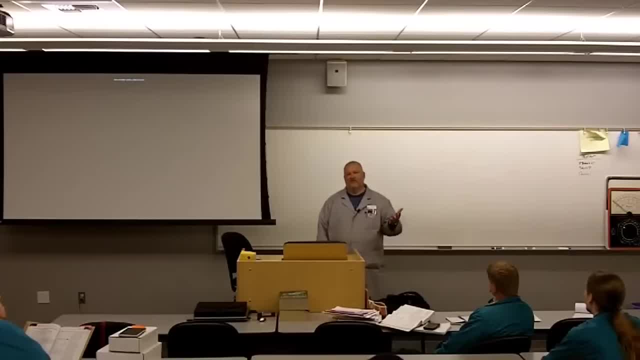 series. Okay, So a series circuit is also known as a voltage divider. right? You all believe me? Okay, so let's go ahead and draw that This is a voltage divider. Any questions? Unfortunately, this is a voltage divider. 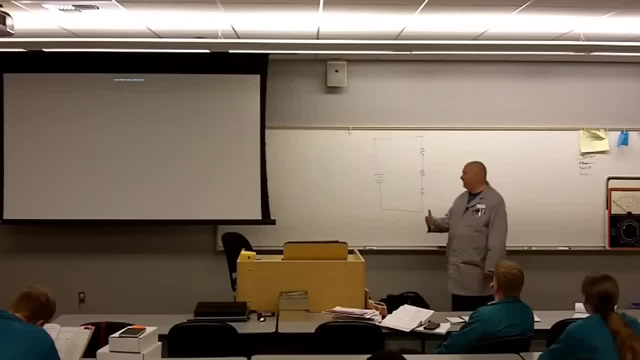 but unfortunately this isn't going to do much for us. This will do a lot for us, but if we effectively want to use it, it really can't be represented like this. Can't be represented like this. First of all, we've got to ask ourselves: 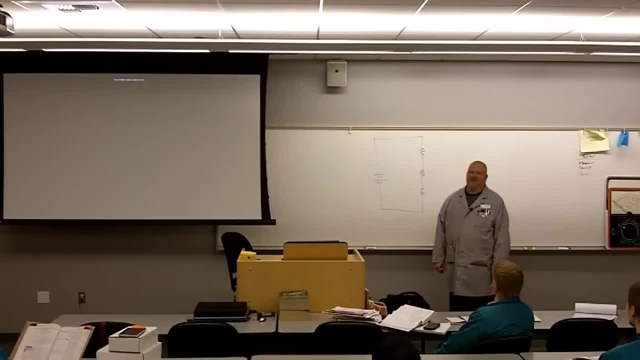 why would we want to divide up voltage? We want to divide up voltage, like I said in here, to power transistors, to power integrated circuits, to power different types of loads, to power different types of devices. Make sense, Okay. 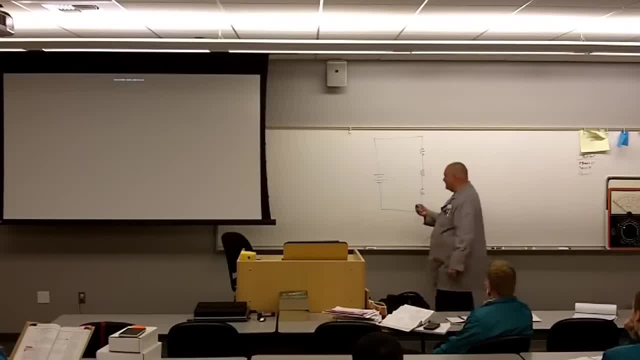 So let's say as an example that I have a 48-volt power supply. This is a big rack-mounted power supply that sits there and drones. it puts out 48-volts DC, But I've got some different appliances. 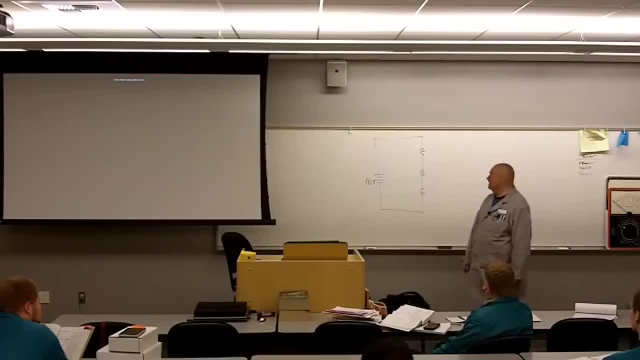 that I want to power from it. Okay. One of the devices that I want to power from it is a 12-volt radio, a simple 12-volt radio, Okay, And that 12-volt radio is a citizen band radio. 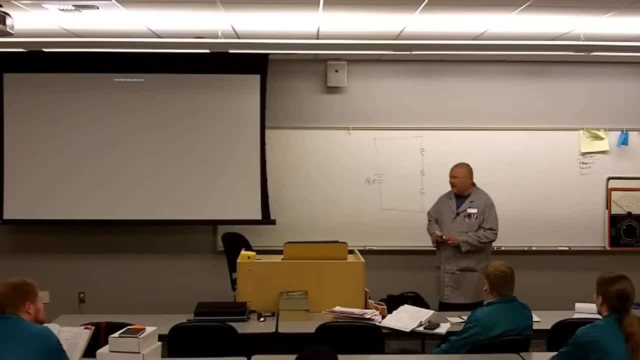 CB radio. So what I need to do is I want to connect that radio to this resistor right here and have this resistor produce 12 volts across it. So when I go out here and connect my radio, which I'm going to represent, Anybody know a symbol that I could use? 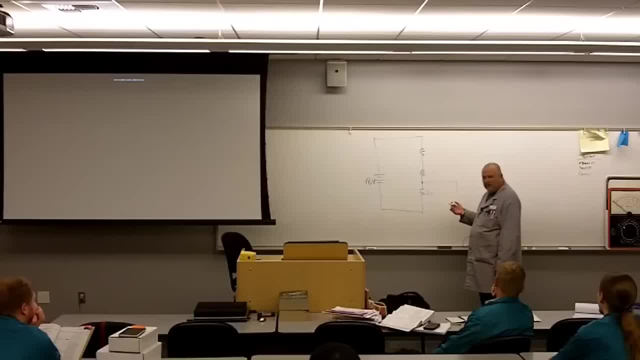 to represent a radio. What's that R? Yeah Yeah, There's no special schematic. What I'm going to do here is I'm going to draw a resistor, and that represents the load that a CB radio has, And I'm going to connect it in parallel. 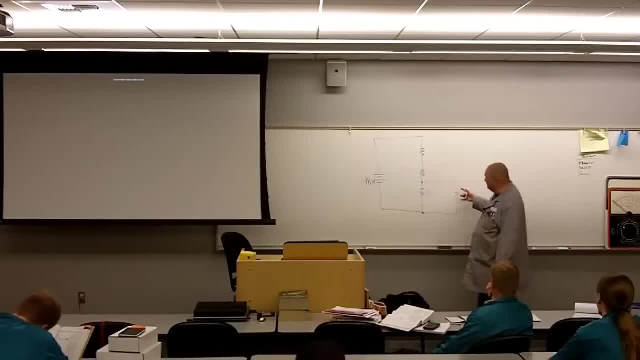 Do you agree that that's in parallel? So whatever voltage is here is going to be right here. When I did this, I just changed the dynamics of the circuit. I just changed the dynamics of the circuit. What I just did is I just loaded the voltage divider. 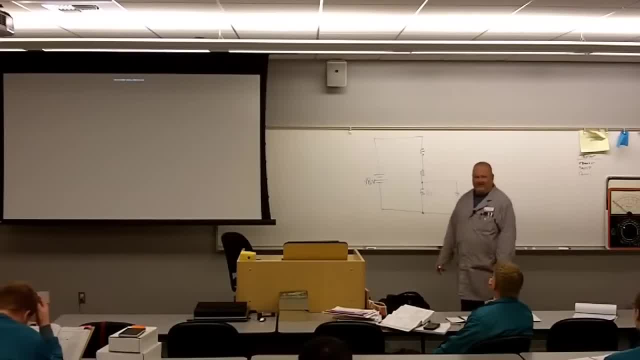 So we're going to call this a loaded voltage divider now And, quite frankly, a voltage divider in and of itself, without any of the loads connected to it. it's kind of stupid. So, you guys, if you had read ahead and you really had mastery of it, 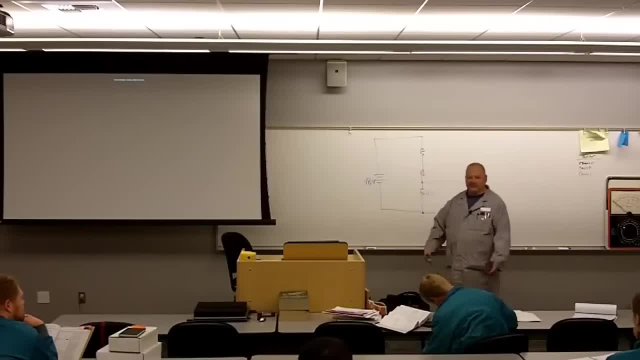 when I'm showing you the voltage divider, you could have said, Joe, that's stupid. What are you going to do? Put three resistors divide the voltage. What good is that? What you've got to do to make it viable. 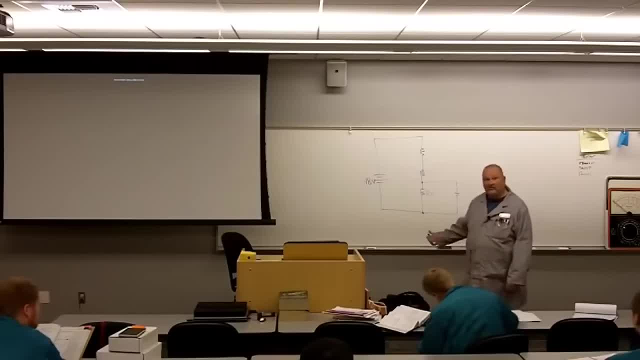 is connect a load to it, a loaded voltage divider. This is a real circuit. We're really going to do something here. We're really going to power a CB radio. So to figure out, we know that this is 12 volts because the manufacturer said: 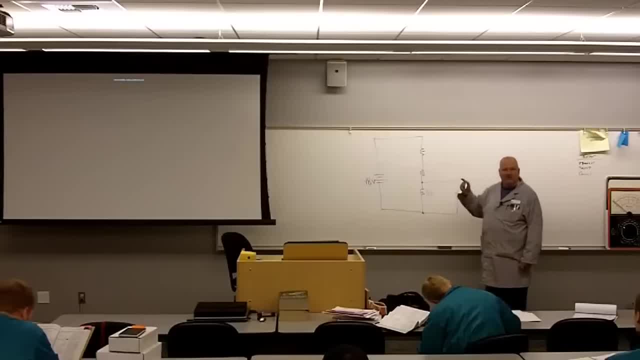 this is a 12-volt CB radio. You plug it in your cigarette lighter, you could wire it into your car and you too could be breaker breaker. one nine Make sense, So we know the voltage is going to be. 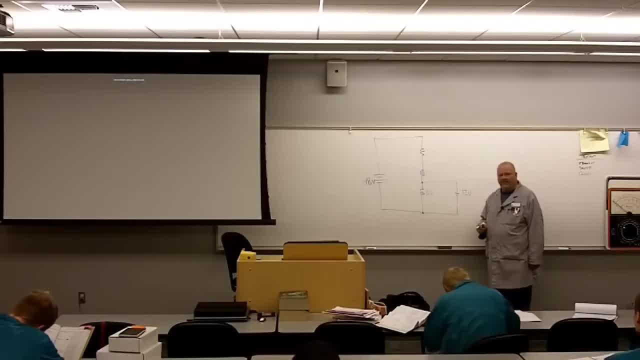 12 volts. The other piece of information that is critical for us is we have to know how much current is required by the CB radio to operate properly. So what we're going to do over here, okay, okay, P-I-V- Okay. 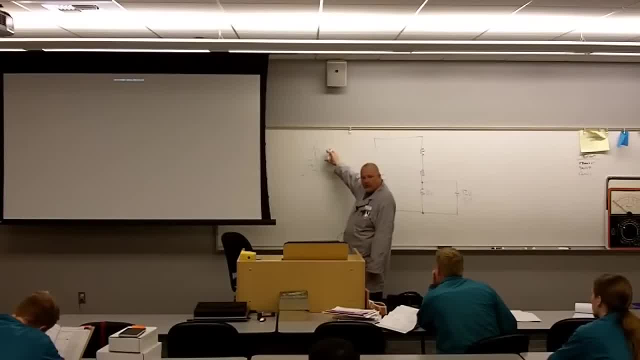 I know that the CB radio right, a typical CB radio is about five watts. And I know that that CB radio because I got the box and the salesperson at Radio Shack- we know how smart they are- said I could wire it up into my car. 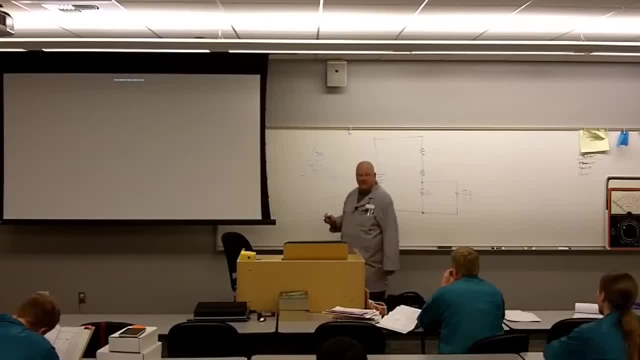 It's a 12-volt system. Okay, So this is going to be 12 volts. So how much current is going to be required to power that radio when I key the microphone and I bring it to the car, When I broadcast out five watts? 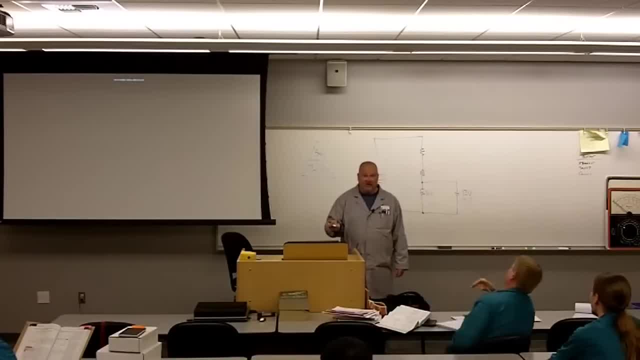 What's the and that's the. by the way, that's the maximum you'll ever consume in a CB radio. If it's a five-watt radio, the maximum you're ever going to consume is when you're transmitting. If you're just receiving, 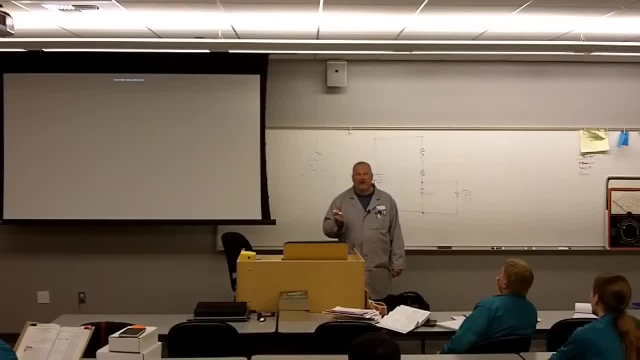 that doesn't consume much energy at all. It's when you key that mic and transmit that you're going to start consuming the most power. So I'm thinking worst-case scenario here. Okay, So all we need to do here, right with your calculator. 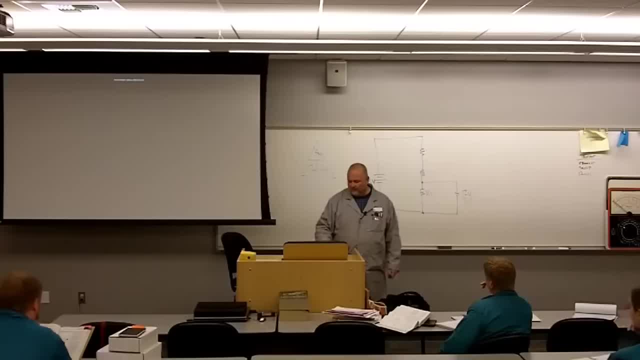 go, five divided by by 12.. What did I come up with? 0.42, rounding off right 0.411, 0.4166666.. Right, That's what I got. Everybody get that. 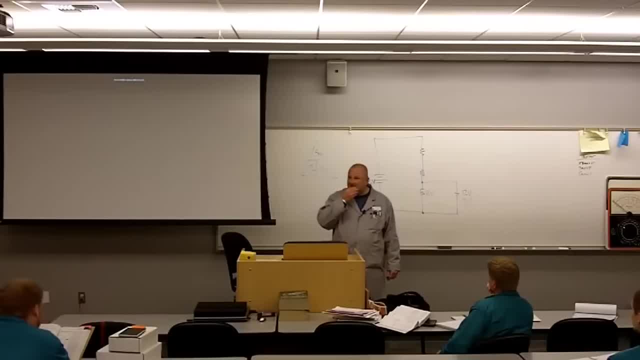 Everybody say I came with that. Okay, That's assuming the radio is 100% efficient. You know what I mean. Like every ounce of current is going into generating that which there's going to be losses. How do I know there's going to be losses? 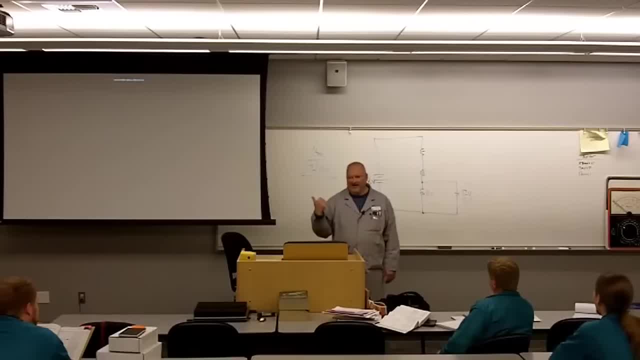 When I use the radio, it's going to get. it's going to get hot. All that energy is not going to get out the antenna. If you get that working, you get all the energy getting out the antenna. give me a call. 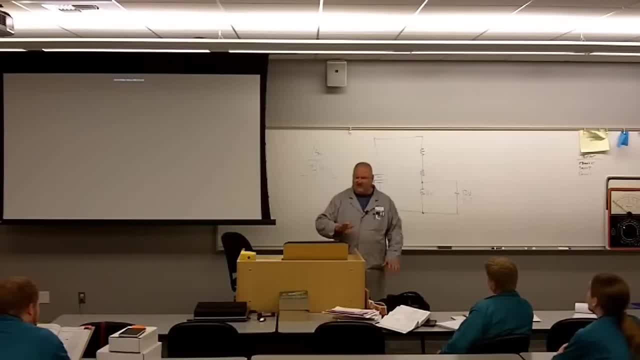 I have my attorney contact you. I personally fly at a Bimini. I'll set you up, Pour you your first cocktail. Okay, I'll set the tab up for you. So what I'm going to do with this, just for the case of example. is. I'm going to round this. Generally speaking, a CB radio is going to take a minimum of half an amp at 12 volts. Minimum half an amp, But probably it's going to be even more than that. But in order for it to transmit out 5 watts. 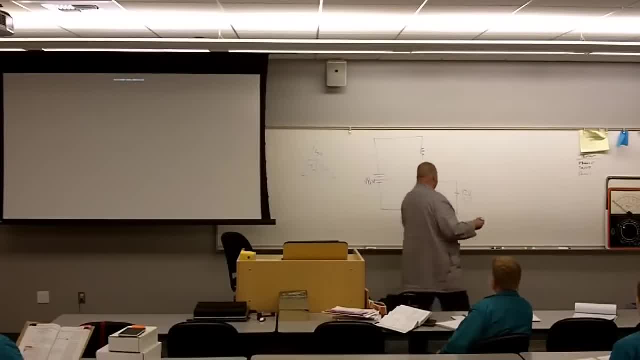 you see the math? Does everybody see the math? Okay, So I am going to assume that this here is 0.5 amps Amps. So we know everything about the CB radio. now It's a 12 volt, 5 amps, 5 watt radio. 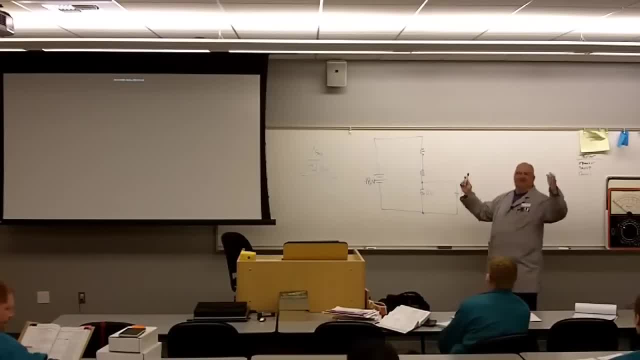 I feel pretty good about it. We can calculate out the internal resistance of it if we wanted to. I don't see the benefit of doing that now. We don't need to do that right now. Make sense, Okay. Voltage divider. Voltage divider. 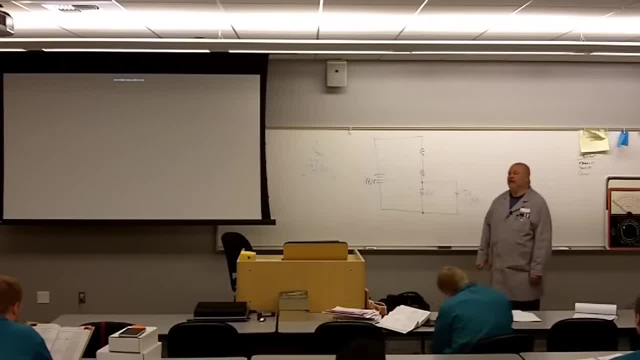 I've got another device. I've got another device, And this other device that I have is, by the way. by the way, we're not going to put this in your car anymore, We're going to put this radio, CB radio, on my boat. 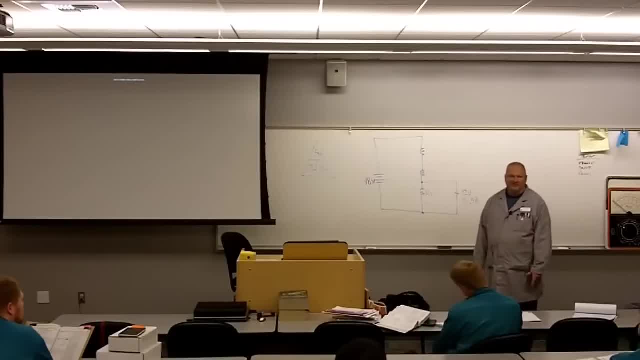 Why I want a CB radio on a boat. I do not know. It's a power thing, man. I want to talk with truckers because I'm going underneath the bridge. Ha ha, You start the traffic, I'm going underneath it. 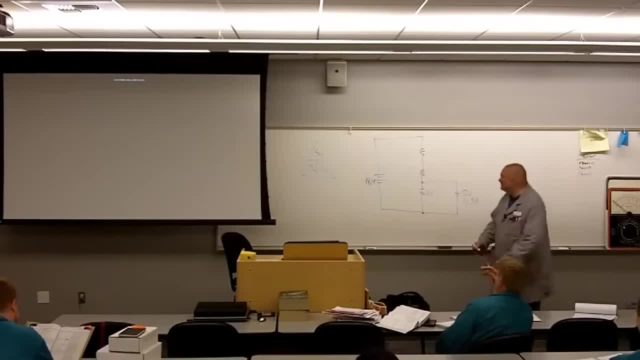 Ha ha, I'm on my boat. Okay, I'm going to install a. I'm going to install a radar system And the radar system that I could represent with a resistor is going to be connected across these two resistors. 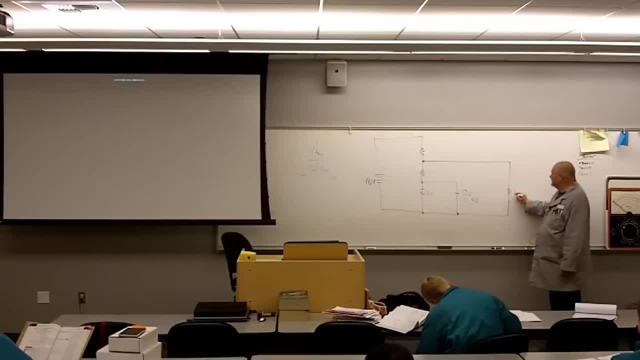 The voltage of my commercial radar system is 24 volts DC And it puts out 200 watts. How much current is going to be needed to go through this device in order for it to transmit out 200 watts? Again, if you get confused, 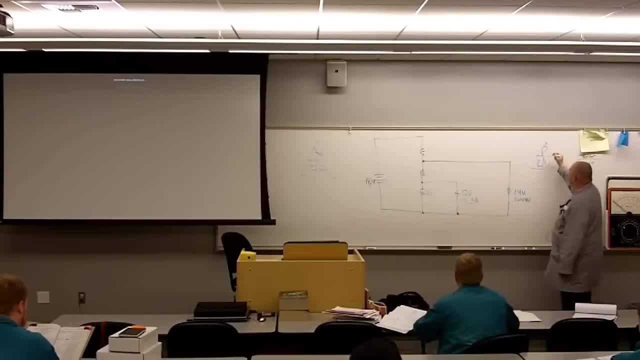 draw the triangle P-I-V, 200 watts divided by 24.. What do you come up with? How much? 0.12? 0.12? 120 milliamps, 8.33.. How much. We got a big disparity here. 8.33.. That makes sense, right. If a half an amp can power a CB radio, it's going to have to be more than a half an amp to power a 200 watt transmitter, right Even at double the voltage. 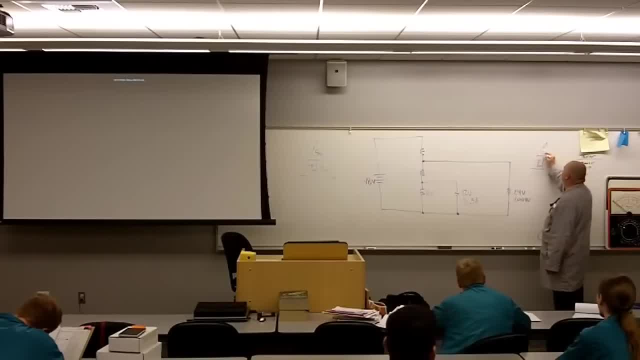 So all I got to do here is: power is 200 divided by how much. What's our voltage? 24., 24., 8.33.. And that assumes what. That assumes 100% efficiency. Do we get 100% efficiency out of this stuff? 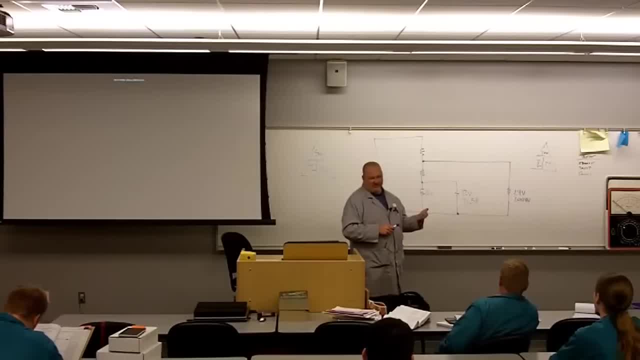 To be honest with you, if we're lucky, if some of this stuff operates at 80% efficiency, 20% of the energy gets consumed as heat. So just for the case of example, I'm going to say that this thing 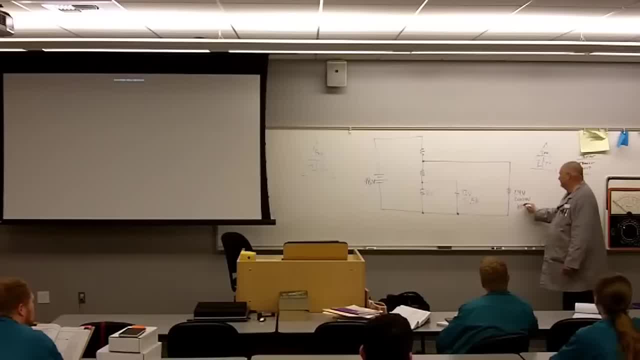 really, in order for it to work properly, is going to need 10 amps, And this might be what the placard data on the back of the radar says or the manual says. But you understand that which one of these are real If you do the math. 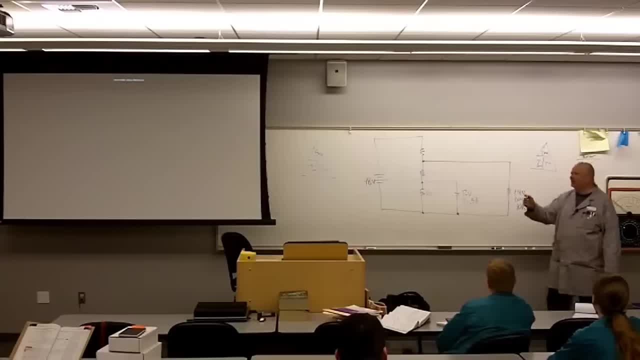 this number could be good. this number could be good, And if that's the case, then we know that the answer is going to be 8. 8.33 amps. But in reality, because of the losses, because of the property of resistance, 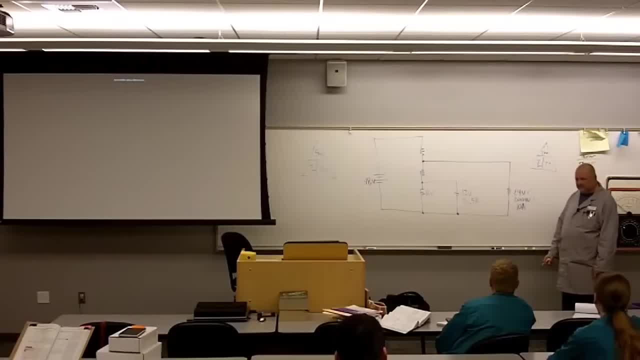 we're probably going to be consuming, really about 10 amps, Make sense, Okay, So now what I have is a circuit, a viable circuit, And, by the way, if I want 24 volts here- and I am getting this voltage across- 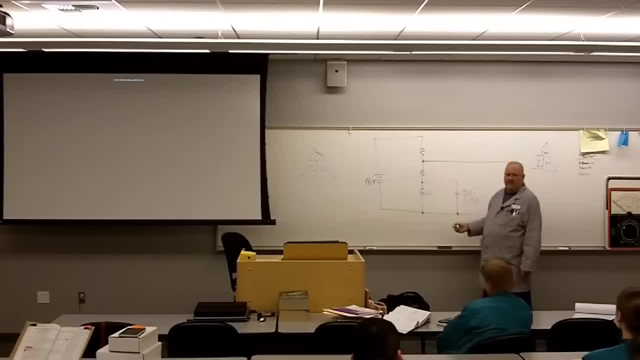 these two resistors. what voltage must I be dropping across this resistor right here? How much? Why 12?? Yeah, And I am connecting this radar unit in parallel- I love it when you talk that way- Parallel with these two resistors. 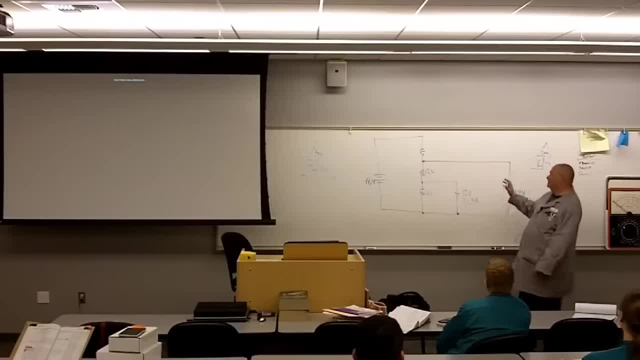 that are in a voltage divider network. Okay, So what we did is we just built. we built a voltage divider, a loaded voltage divider, But we've got to analyze it now. We've got to analyze it, And this is where the author like 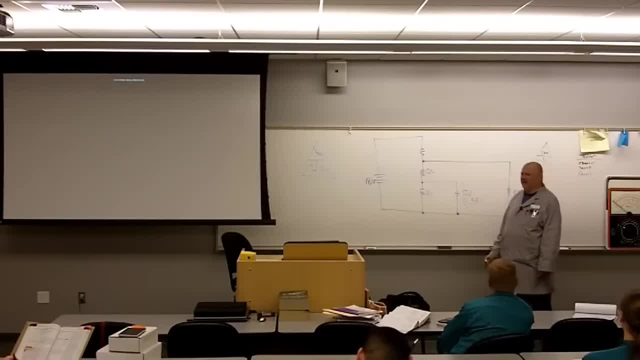 pulled numbers out of his backside and he really didn't justify it, and I don't even know where that's coming from. That's why we're having this lesson Question, Question: Is there another resistor up there that's hanging out by itself to another 24?? 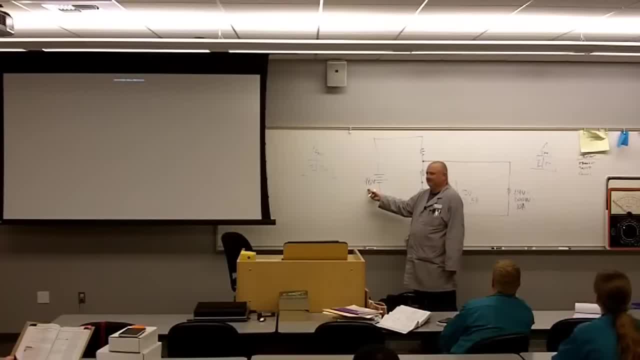 It has to be 24, right, It gets 48.. Why wouldn't that This? remember This here. I bought this. It's military surplus. This is a 48-volt power supply. Okay, So it converts my ship's power to 48 volts DC. 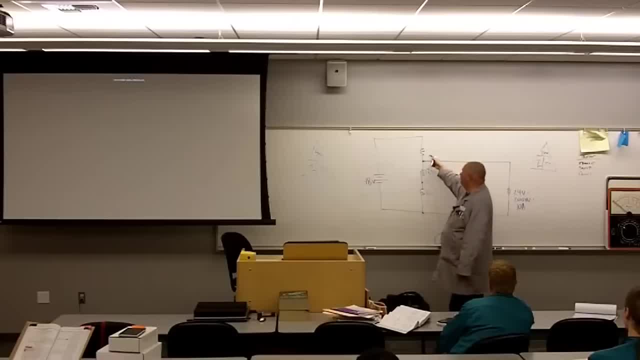 Yeah, So if this is 48, and this is 12, and this is 12,, what's this got to be 24.. Why, Come on, guys, Quote me what I've been quoting you? Your drop has to equal the rise. 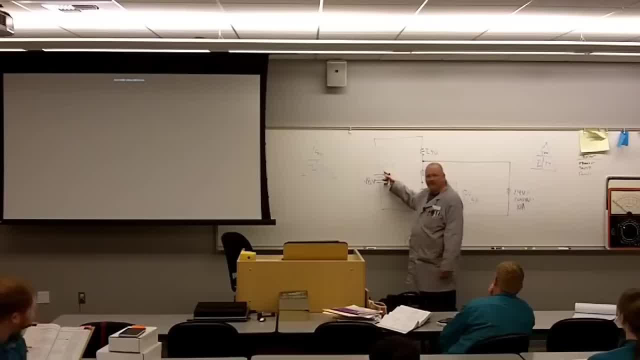 Absolutely, Because the drops have to equal the rise. I'm putting 48-volt rise in, I'm getting 48 volts a drop. 12 here, 12 here, 24 here. All voltage drops present and accounted for Make sense. 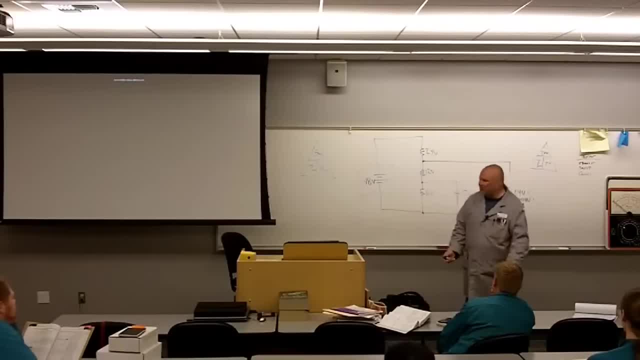 Okay, so this is cool. It's really going to work like this, But we don't know the math. We don't know what values of resistance to use here. This is where it gets tricky. This is where there's another thumb rule. 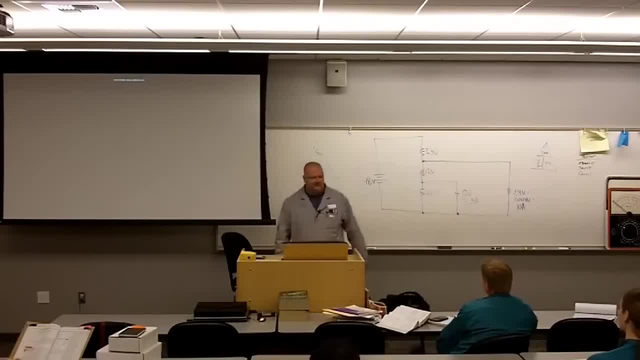 That's why you come to lecture. Okay, If the book was that good, if the book was that good, you could be home in your underwear studying right now, and I could be home in my underwear correcting your work. Instead, here I'm dressed up, wearing lab coats. 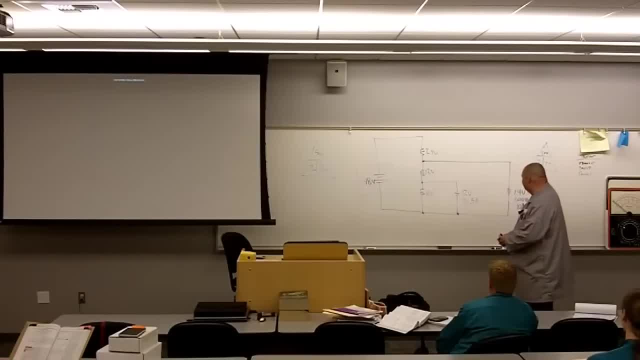 you're wearing lab coats and we're having this interactive lesson, The thumb rule. is you ready for this? The bleeder current needs to be one-tenth of the total load current. The bleeder current needs to be one-tenth of the total load current. 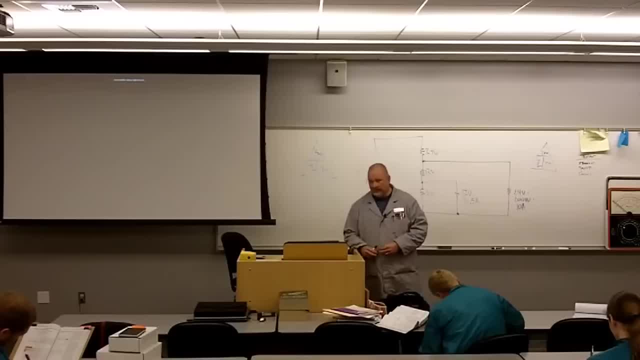 The bleeder current needs to be one-tenth of the total load current. How many of you buy that? You better buy it. I just sold it to you Now. the question is: what the heck is he talking about? bleeder current. 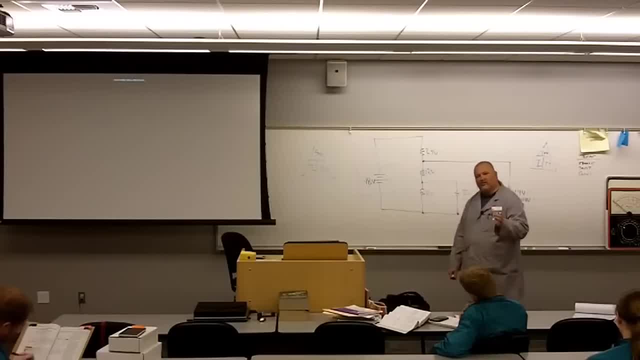 The bleeder current is the current flowing through the first resistor that starts the voltage division process. So by me saying that first of all we've got to determine what is our total load current, What's our total load current in this circuit? 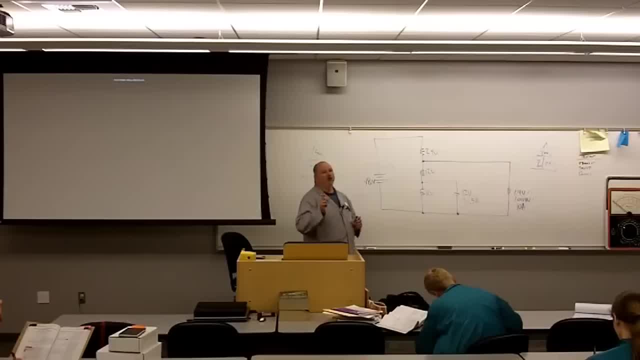 28? 48?. Total load current- Current- is measured in amps. What is my total load current in this circuit? 10.5.. What Pounds, ounces, kilograms, amps? I love it when you talk that way. 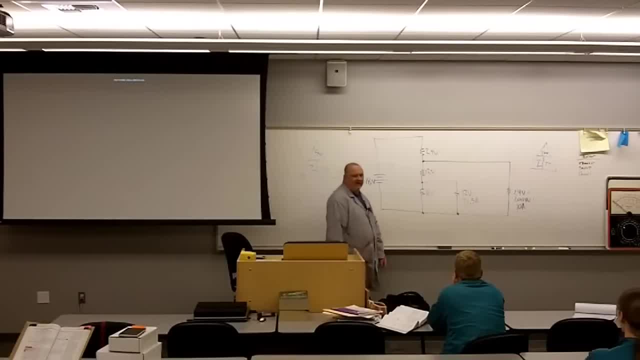 Total load current is 10.5 amps. Everybody see how we did that. The only loads in this circuit. this is a voltage divider. These are my loads, The only loads in the circuit. here are what the heck was this? A CB radio. 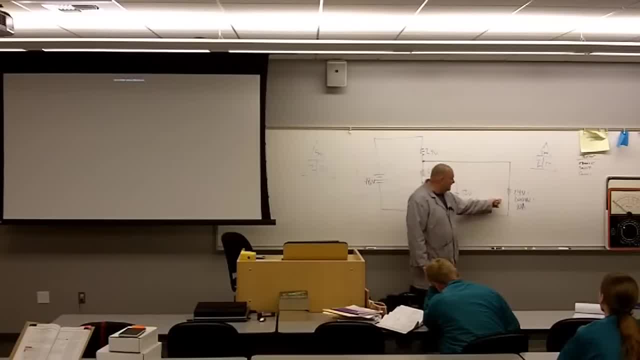 Breaker breaker one nine CB, All right, And then this was a radar system. Radar system consumes 10 amps. This consumes a half an amp. So by total load, current is 10.5 amps. Do you all agree with that? 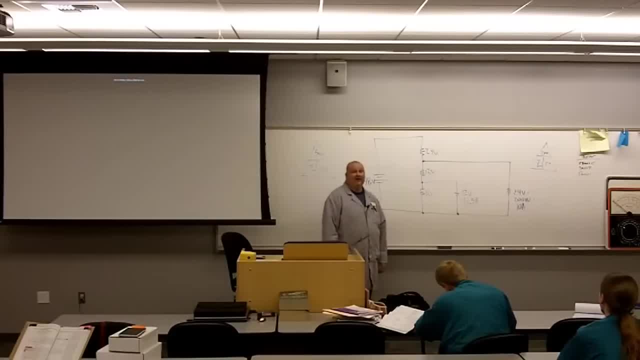 Okay, So I said the thumb rule is that the bleeder current is one tenth of the total load current. What's one tenth of 10.5?? One tenth of 10.5 is 1.05 amps. Okay, So 10.5 divided by 10,. 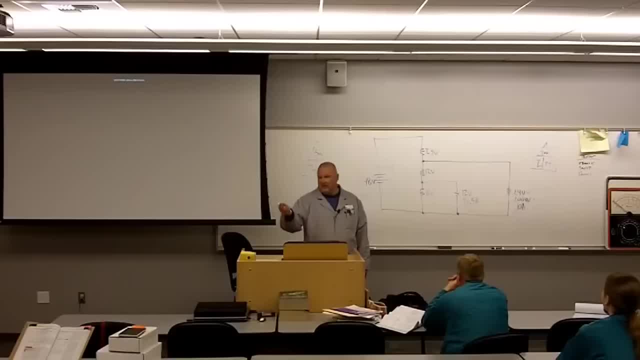 10 point. all right, one tenth, So 1.05 amps. Do you all agree with that? Getting some puzzled looks. One tenth of my total load. One tenth of 10.5 is 1.05.. Agree with that? 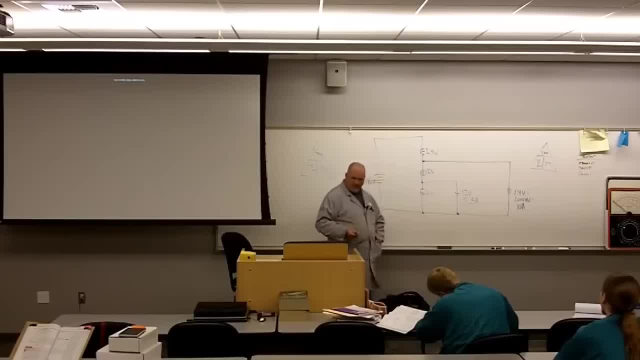 So that's how much current. I'm going to do something here. I'm going to change the color to make it stand out. Okay, It's going to be passing through this first resistor. Very good, Okay, And this is going to be 1.05 amps. 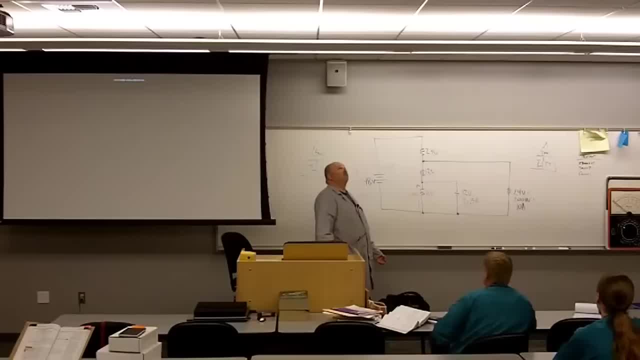 And again, where's that coming from? It's exactly the text that we're stating on that, So at least remember my, my deal. So, right there, we just unlocked the entire circuit. We just unlocked the entire circuit, Because what we've got here is 1.05 amps. 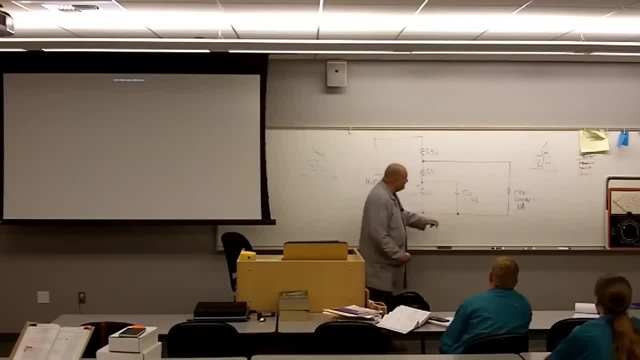 coming up out of this node. How much current do we have coming up through here? Where'd that number come from? Thank you, The paperwork Okay, Or your calculation based on, if the paperwork left out, the current demand. you know it's a 5 watt radio. 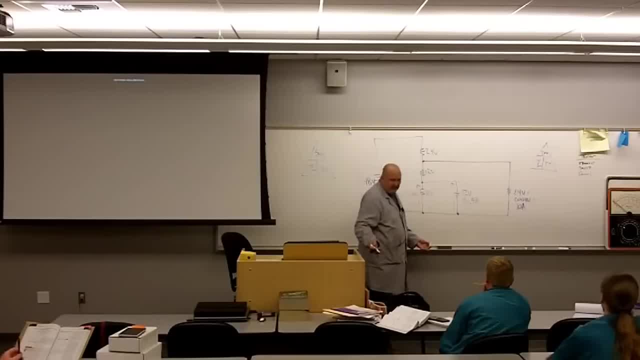 And again, as long as you can prove, you've got to be able to prove to somebody. Okay, So we call that 0.5.. So we've got 0.5 amps coming up through here, All the current that comes up through the radio. 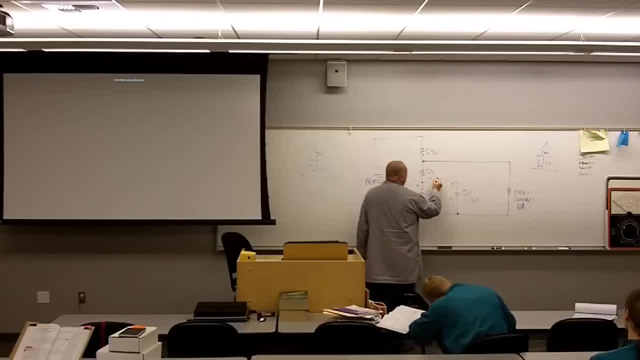 is going to come here, into this node right here. So I've got 0.5 amps coming in from this angle. I've got 1.05 coming in from this angle. Can anybody tell me about how much current's going to be going through this? 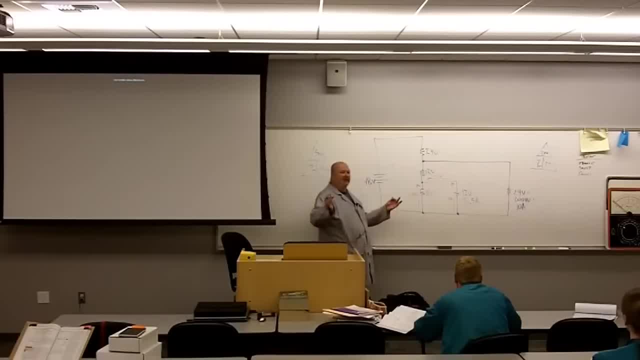 How'd you come up with that? And how'd you come up with that? Is that a notion? It's a current divider. It is a current divider, Okay, But again, what's going to bring tears to my eyes is, if you quote me, laws. 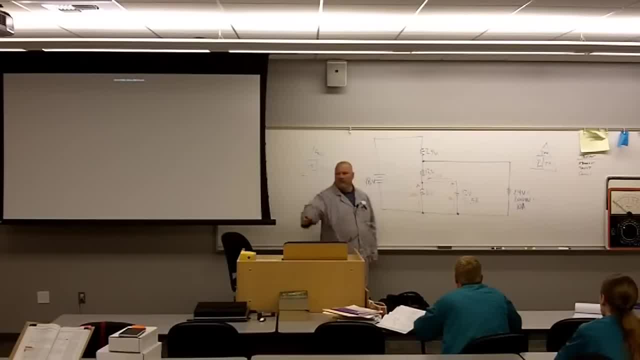 Are there any laws that govern what's happening here in this node? What is it? Absolutely Kirchhoff's Law. I got 1.05 coming up here. I got 0.5 here. We've got a traffic cop standing in the middle of that intersection. 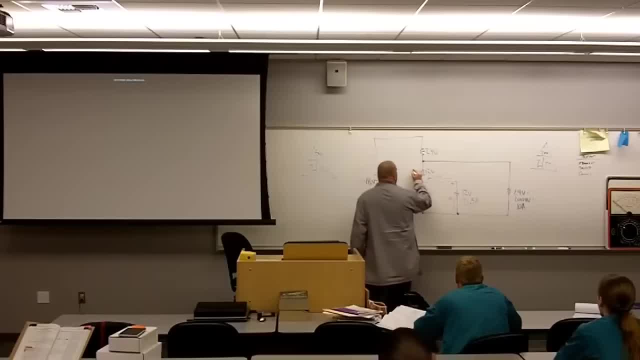 How much current's driving away from him. 1.55 amps, It's gotta. It's gotta. If this thing's functioning, it's gotta work like this. So I've got 1.55 amps coming up through here, Okay. 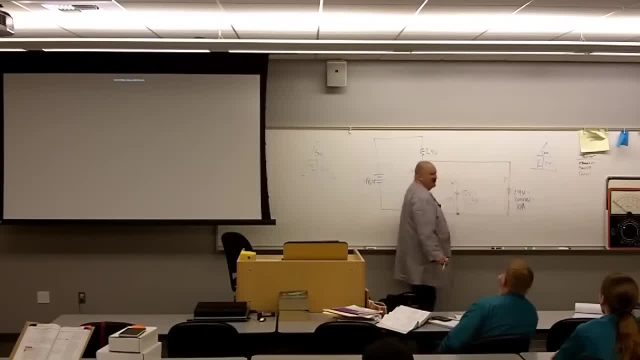 How much current is coming up through this load? How do we know that Placard data, technical documentation, calculation utilizing Watt's Law? I don't know, Because Joe said so. Actually I didn't. All I gave you is that 24 volts and the 200 watts. 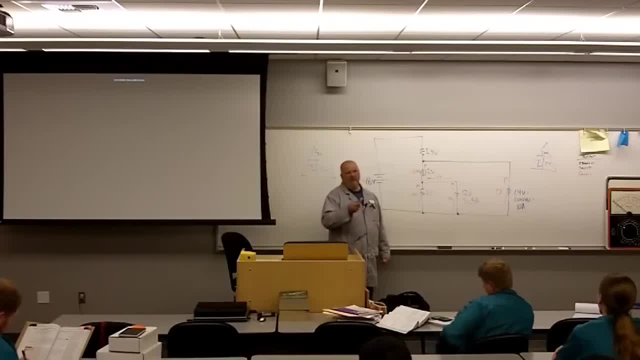 You folks really calculated that out. The only curveball that I shot you in any of this was the efficiency bit. I'm talking about efficiency. The book doesn't even talk about that. But you, just you don't get 100% of anything. 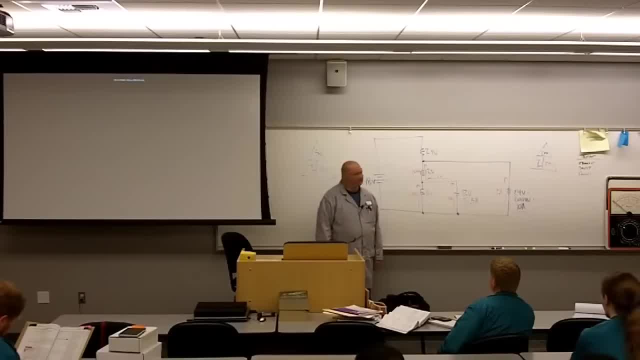 You don't. There's nothing that's 100% efficient. So I got 10 amps coming up through my radar system. That means that 10 amps makes a 90 degree corner at the speed of light. Right, 10 amps. 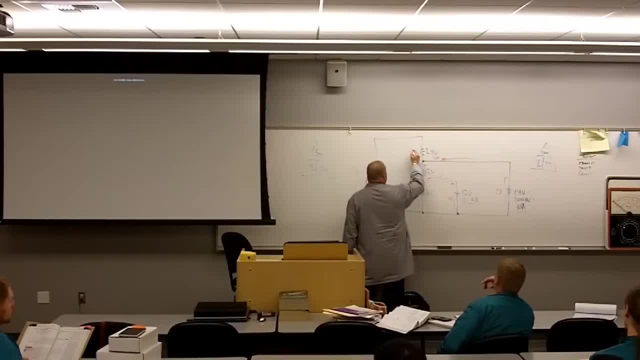 11.55 amps. How do we get an extra amp? How'd you get an extra amp with Watt? We got .5 amps a half an amp. What was the rule here? What was the whole thing on unlocking this entire circuit? 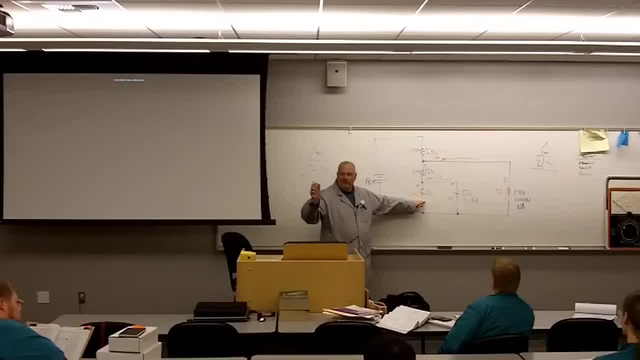 What did I call this resistor, The bleeder resistor, And that's what's starting the whole process. We have to have some current going through that to create, And the reason that we use one-tenth so is that these loads come on and off line. 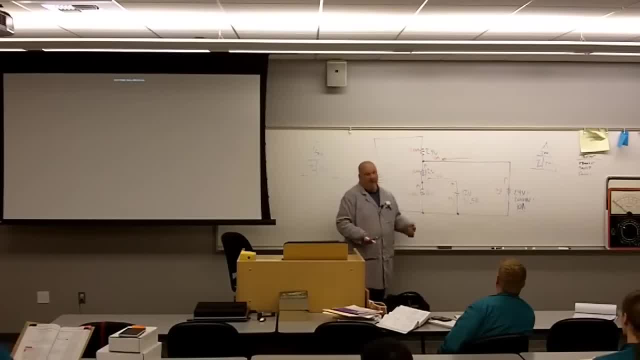 the circuit's going to have stability, Because that CB's not always going to be on, And when we turn the circuit on, we're going to have stability. And when we turn the circuit on, we're going to have stability. And when we turn the circuit on, 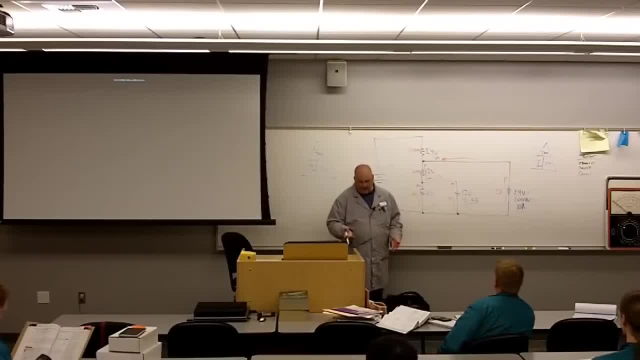 we don't want the whole circuit to go cattywampus, We want it to be somewhat balanced. Same thing with the radar system. So it's a thumb rule. It's not an absolute. It's a thumb rule that should give us consistency of operation. 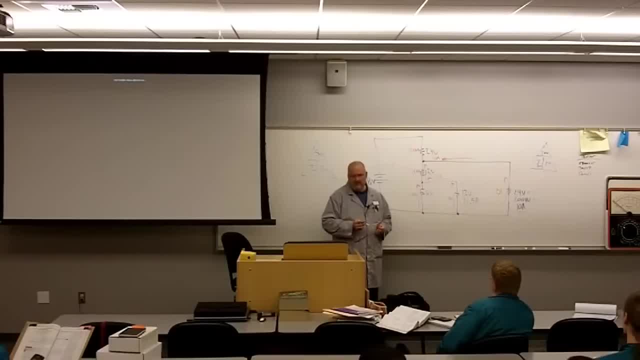 for this circuit Make sense. So we know that we have 11.55 amps coming up through here. Boom. If I've got 11.55 amps flowing into my power supply, how many amps must I have flowing out of my power supply? The same. Okay, So that means I've got 11.55 amps flowing into this node. If I've got 11.55 amps flowing into this node and 1.05 amps flowing out of this node, how much current do I have flowing in this direction? 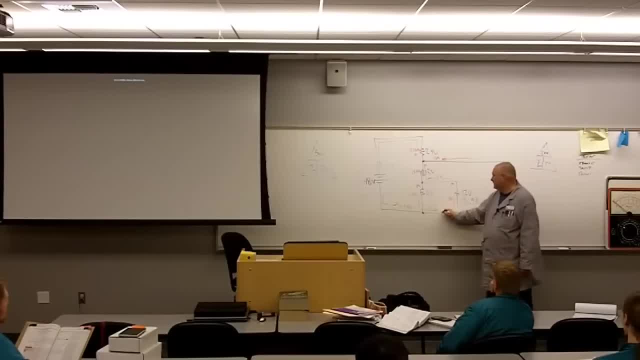 How much 10.5 amps. Do you agree with that? If I've got 10.5 amps flowing into this node and I've got 0.5 flowing in this node, how much current am I going to have flowing in this direction? 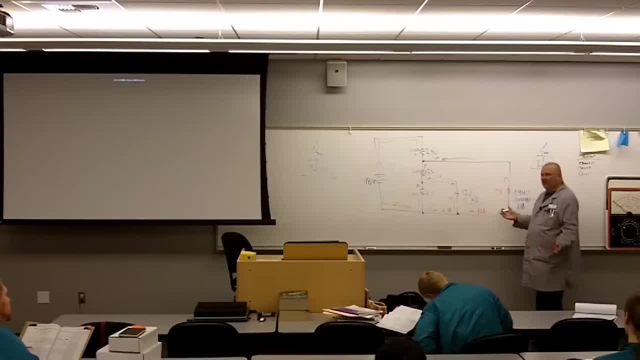 Isn't that the same number we started off with? So I just proved that this works. I just traced all the current through this circuit in doing this. Now, the easy part of the analysis is this: V I, R, Let's calculate out resistance voltage over current. 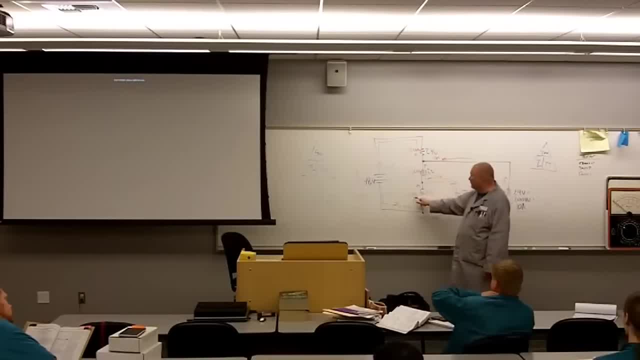 Voltage over current right Voltage: 12 over 1.05.. 12 over 1.05 is going to give me this value of resistance: R is going to be equal to 1.40 volts. 11.428 ohms. That's what I came up with. Are we going to find an 11.428 ohm resistor? Can we find something close? Maybe we could find one with tolerance as a 10 ohm resistor. that's on the high side: 20% tolerance. 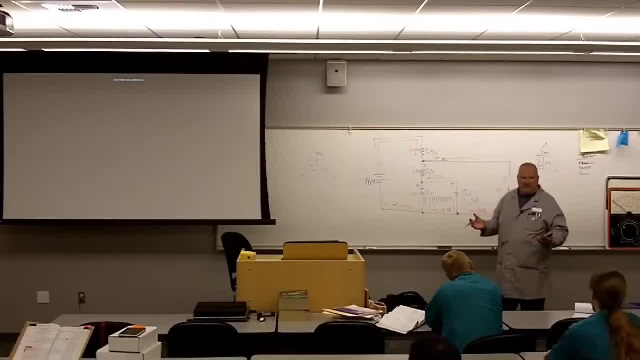 We could find one that's within that right, Because a 10 ohm resistor could be anywhere from 12 ohms to 8 ohms, So, yeah, we might be able to find something close to that. It's not going to be that critical. 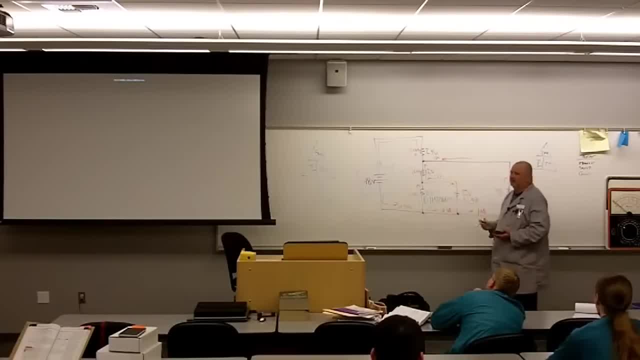 You're going to get less of a voltage drop there, So that is kind of critical. The bigger the resistor, the bigger the voltage drop. The smaller the resistor, the smaller. So we could do the same thing up here: 12 volts divided by 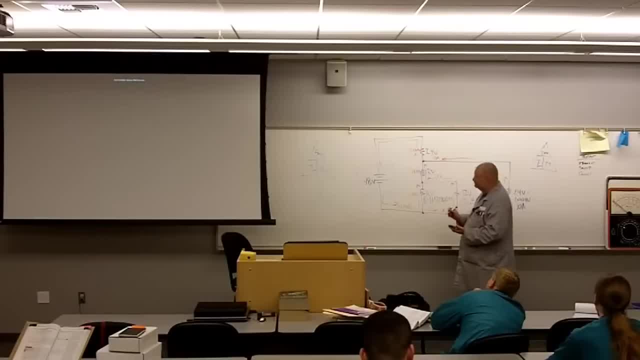 1.55 amps, 7.7 ohms, And then finally here up at the top, 24, divided by 11.55.. 2.08 ohms, And this is how you analyze a loaded voltage divider. It's really nothing unique, is it? 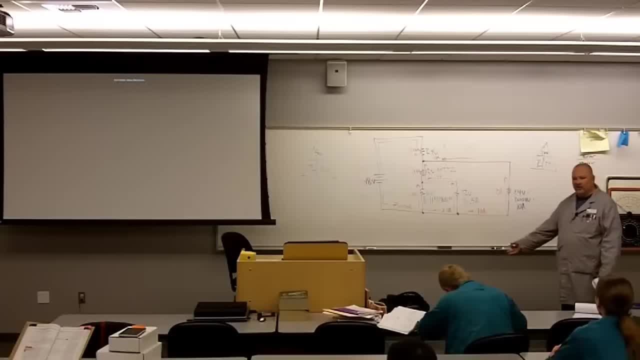 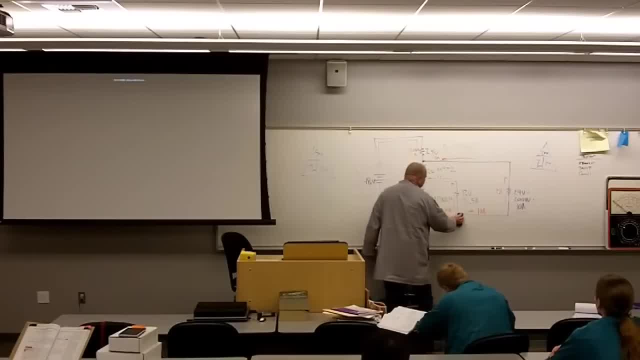 All right, let's go ahead and take a look at this. Thank you. What is it? It's the exact same circuit And, to be honest with you, this is how this thing would really be connected. This is how it would be really connected. 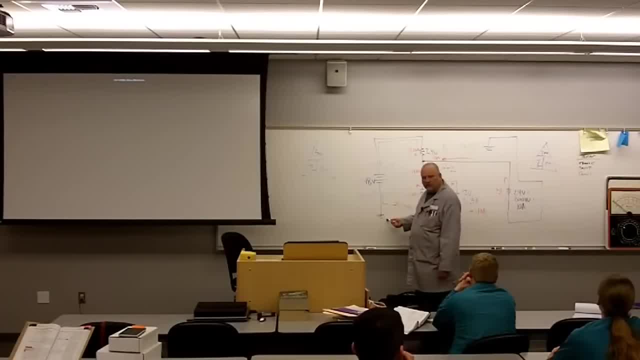 Your 48 volt power supply would be connected to what kind of ground? Electrical ground, Not necessarily earth ground. electrical ground, which is typically a chassis ground or a frame of a vehicle or a boat, the hull of a ship, the frame of a train car. 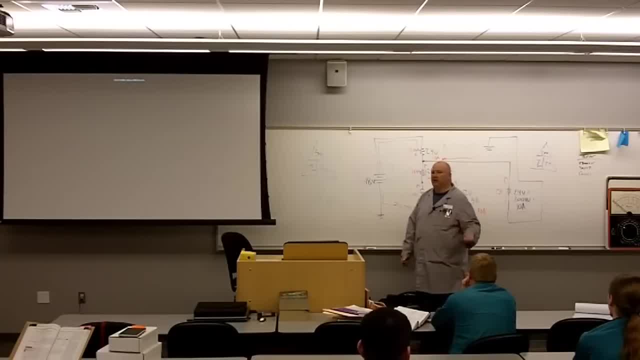 This is how it's going to be done, because we're going to use the frame as a conductor. The circuit's going to operate exactly the same. We're going to get the bottom of the circuit here, the bleeder resistor, connect that also to ground chassis ground. 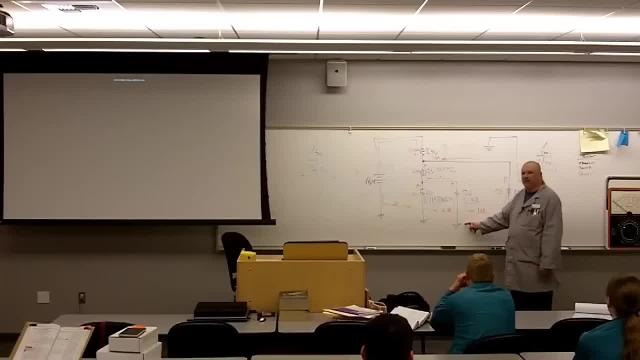 We're going to connect the negative lead of our radio directly to chassis ground. We're going to connect the negative lead of our radar. The radar's kind of mounted in an unusual position. you know, I got that. you know the pulpit up there. 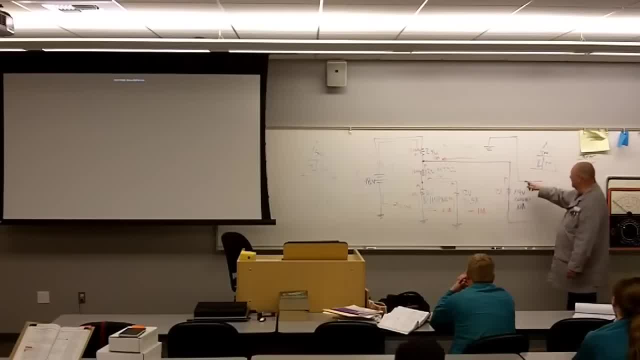 I drive the boat. I want the little radar there, So I'm going to have to run quite a bit of cable, but I'm still going to connect it to chassis ground. And this is the exact same circuit that you just analyzed. I just made it more complex, complicated, looking by putting these grounds in 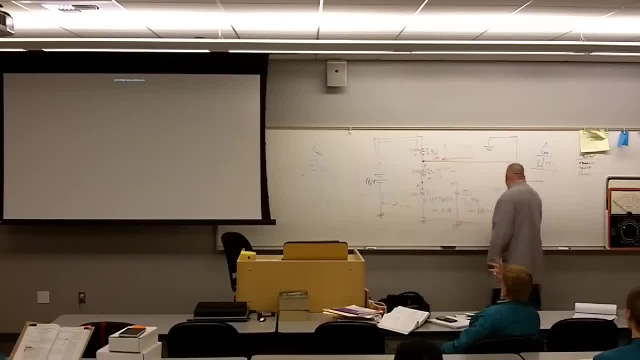 Basically, when you see this in a circuit, you know that, electrically, all of these- whatever the heck that thing is right- All of these are interconnected. Don't let me screw you up with this kind of stuff. And it's assumed that you know how to interpret this type of stuff. 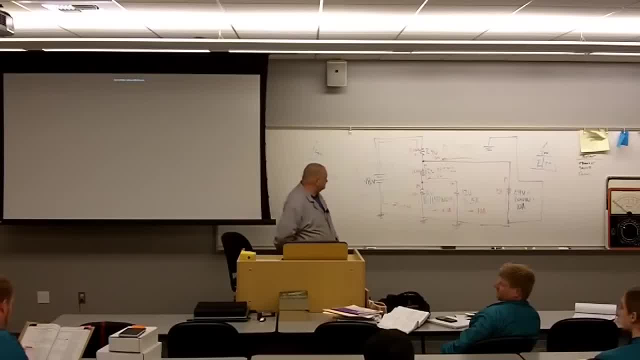 Questions. Questions Yep: 10.5 divided by 10. One-tenth is 10, right One-tenth is 10.. Makes sense 10.5? 1.05.. You can multiply it by .1.. 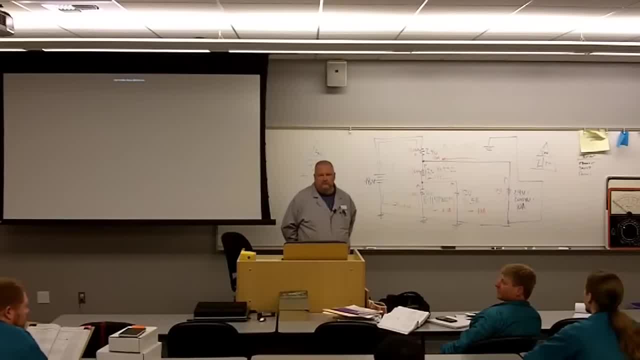 You get the same answer. Another question: No Questions. Yeah, 10.5.. Yeah, You could sit here all And again. that's a thumb rule, but you could use it for analysis and then if somebody asks you: how the heck did you come up with that? 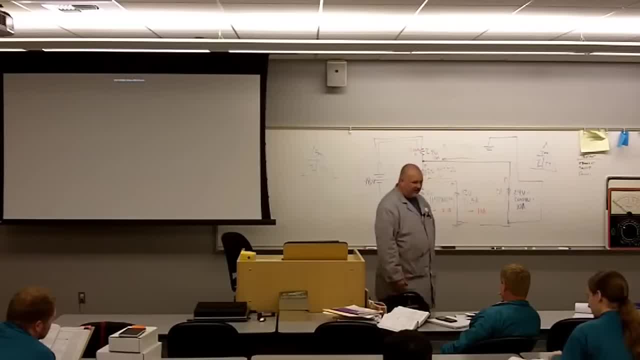 How did you What? You want me to buy these parts? Well, how'd you come up with that? Well, I used it as a thumb rule that I want my bleeder current. Okay, As opposed to the author who, just again, I don't know where those numbers came from. 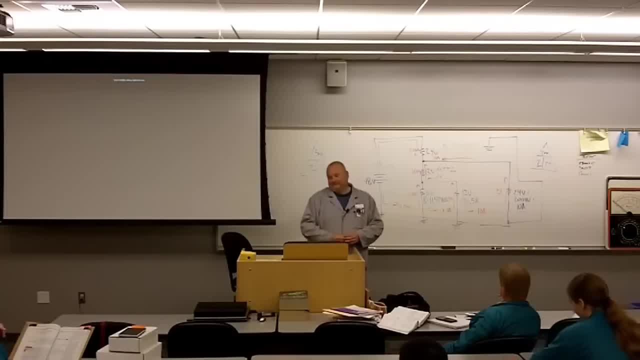 I don't know, I don't want to know. It is what it is. So in the future, use that one-tenth, I use that one-tenth. you're not even going to get the. I mean, you won't get the answer. 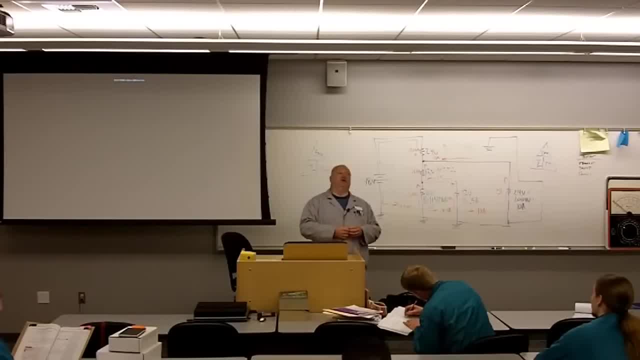 that the author gets in the book. I don't know what you. You got to do it wrong to get the number that the author gets in the book. So there's In the future, when you see loaded voltage dividers, use that one-tenth rule unless. 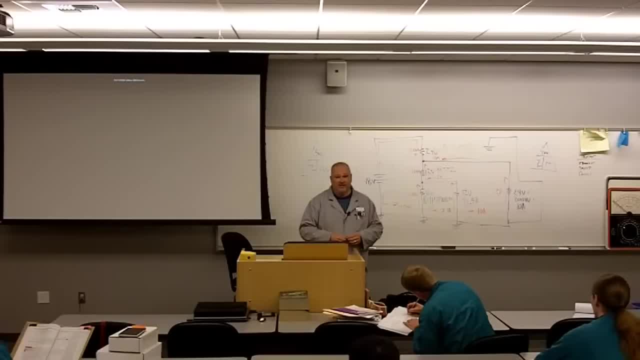 you're told, otherwise You know there might be an engineer that knows a lot more math than we know. They say no, we want you to assume 15% or 20% or whatever, But you need some guidance. We're not engineers. 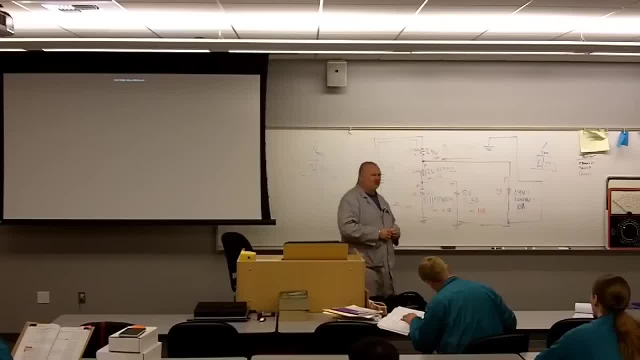 You guys remember that. You know that We're not engineers. Anybody here want to be an engineer? honestly, No offense, honestly Okay, If you want to be an engineer, that's, you know, that's good. You're going to immerse yourself more in the world of theory. 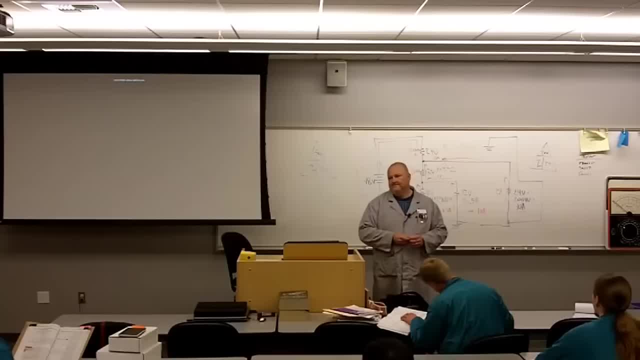 We immerse ourselves more in the world of reality. So we're going to do what we're told to do. I actually had a meeting today with an engineer. We're looking at some engineering, starting some engineering classes here at Lake Washington, a parallel program to pursue your engineering degree, and the way he was talking about too. 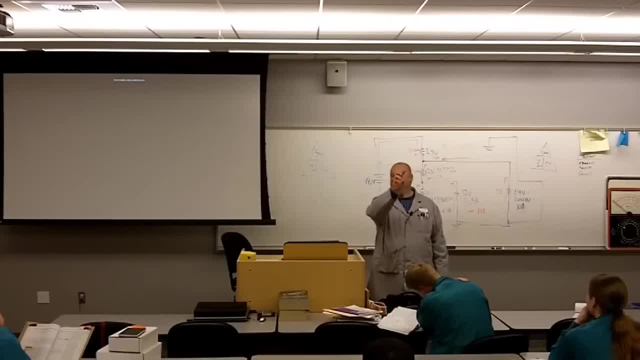 like a pyramid. It's like a pyramid. You get to research science A handful of research people up here at the top of the pyramid, then you've got engineers designing the stuff and then you've got technicians making the stuff work. So there's a lot more technician jobs out there to support engineering and the engineering. 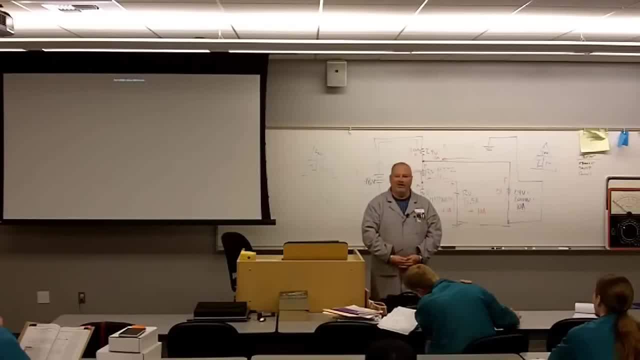 supports R&D. You know, Boeing only has a handful of people that sit around and think about weird crap all day long. Thank God right, Because then what they do is they farm it out to the engineers and say, hey, make this. 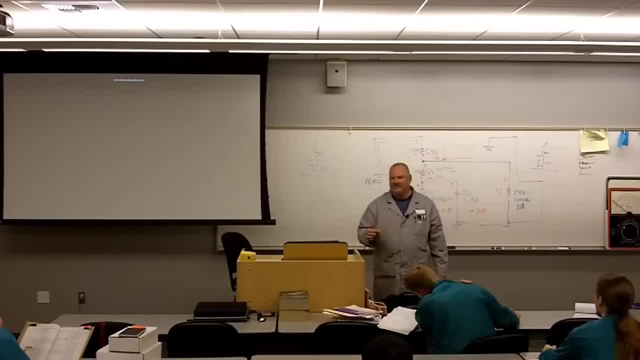 work, And then the engineers figure it out, the calculations and everything, and then they give it to the technicians and they say: make this work. And then we are the last line of defense And the only thing that we have to fall back on are the laws of physics and the theory. 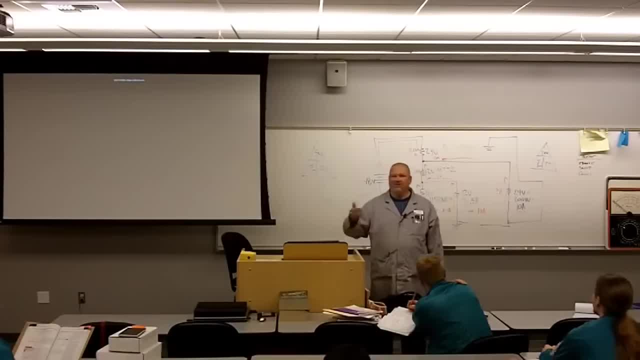 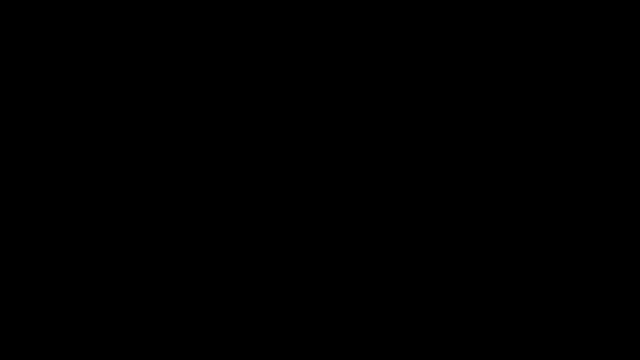 of operation. That's all we have to fall back on, And if you can apply that, then you're going to be ahead of the game. There's no question about it. No question about it. This actually worked out pretty well for us. 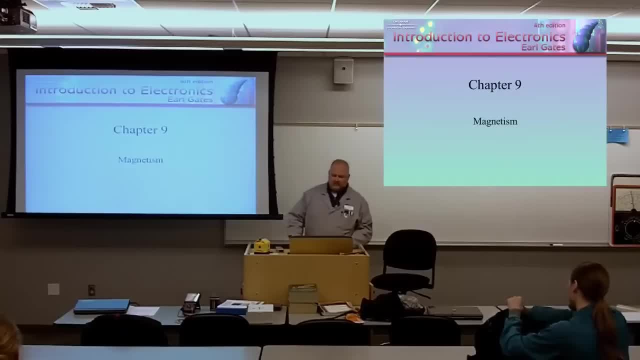 I'm going to go back to the last slide With last week, doing 7 and 8, and then saving chapter 9 for this week, because that's the only thing that we're going to do. tonight is going to be chapter 9, magnetism. 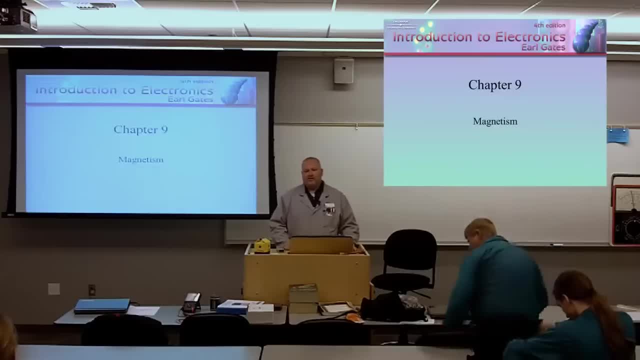 And this is a huge chapter. I don't think there's any other property that has had such a profound impact on society as magnetism, as you're soon going to see. I mean, if it weren't for the property of magnetism, we wouldn't be here today. 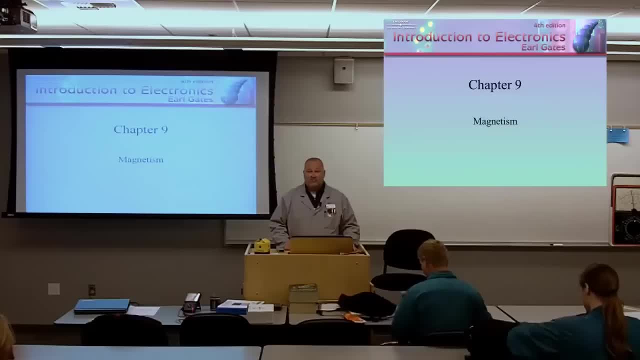 I mean, if it weren't for the property of magnetism, we wouldn't be here today. I mean, if it weren't for the property of magnetism, we wouldn't be here today. So much more than magnetism, Electronics and electricity would not be what it is today. 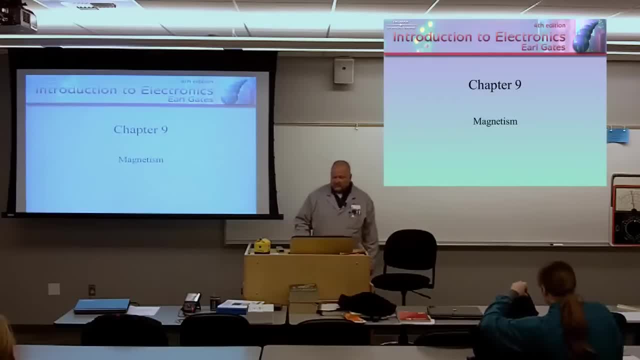 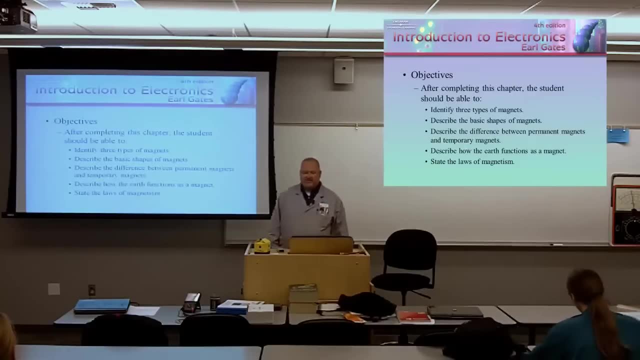 It's really that simple. So, with that introduction, let's forge ahead with chapter 9, magnetism. After completing this chapter, you're going to be able to identify three types of magnets, Describe the basic shapes of magnets. Describe the difference between permanent magnets and temporary magnets. 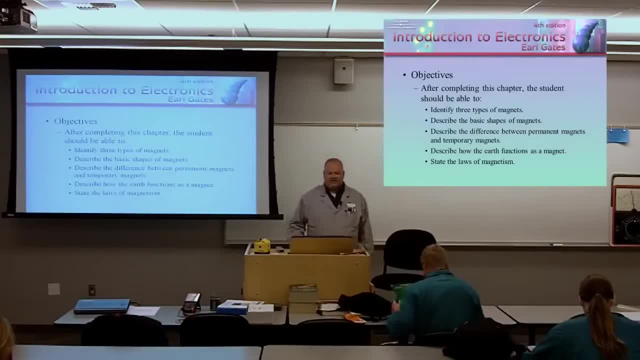 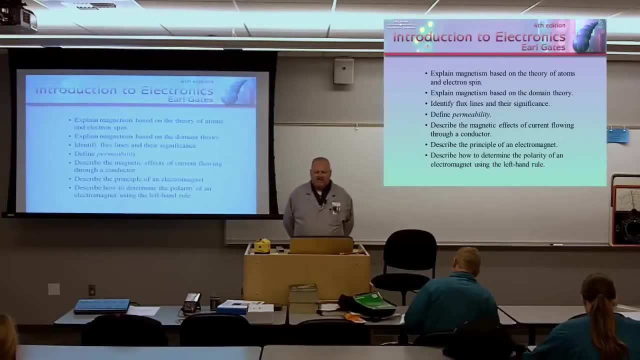 how the earth functions as a magnet State. the laws of magnetism. Explain magnetism based on the theory of atoms and electron spin. Explain magnetism based on the domain theory. Identify flux lines and their significance. Define permeability. Describe the magnetic. 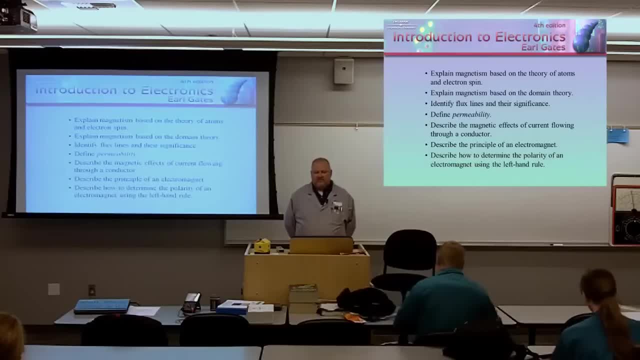 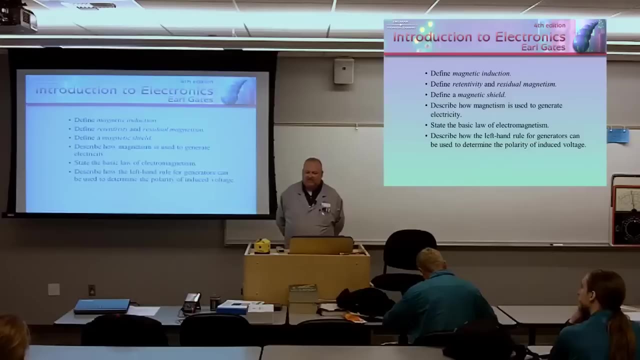 effects of current flowing through a conductor. Describe the principle of an electromagnet. Describe how to determine the polarity of an electromagnet using the left-hand rule. Define magnetic induction. Define retentivity and residual magnetism. Define a magnetic shield. Describe how magnetism is used to generate electricity. State the basic laws of magnetism. 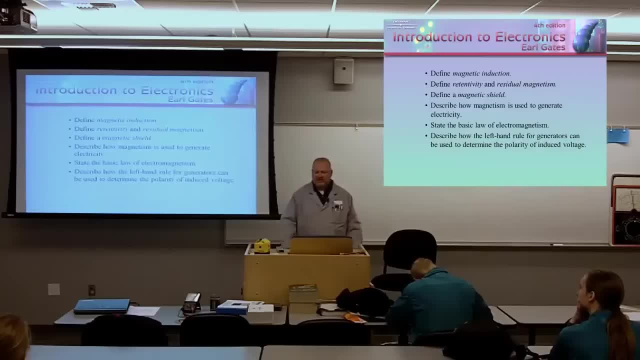 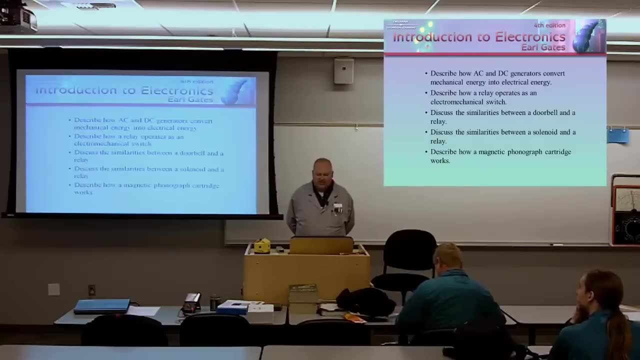 Describe how the left-hand rule for generators can be used to determine the polarity of induced voltage. Describe how AC and DC generators convert mechanical energy into electrical energy. Describe how a relay operates as an electromechanical switch. Discuss the similarities between a doorbell and a relay. Discuss the similarities between a solenoid and a relay. Describe how 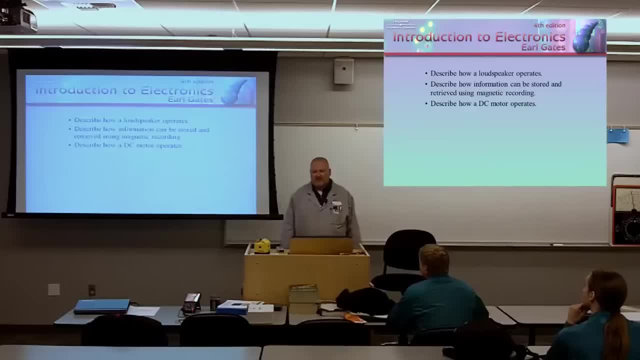 a magnetic phonograph cartridge works, Describe how a loudspeaker works, Describe how information can be stored and retrieved using magnetic recording. And describe how a DC motor operates. I don't think we've had any chapter up to this point that has had so many. 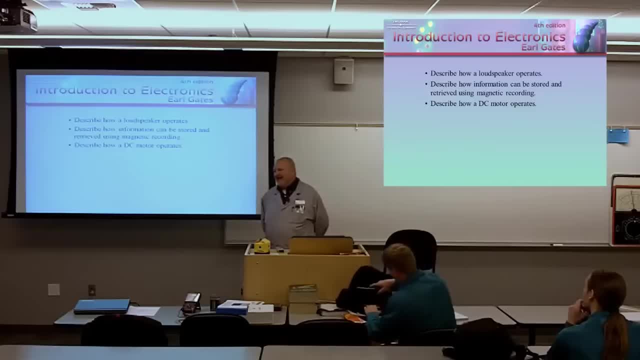 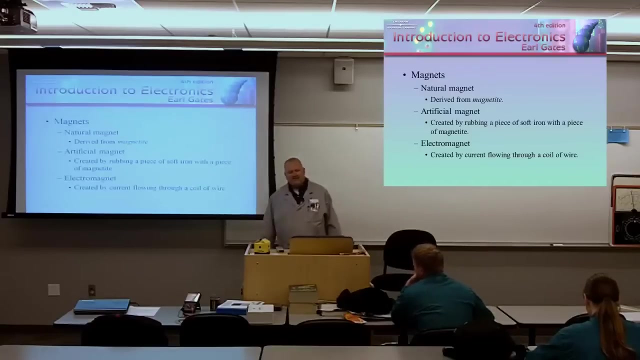 objectives, and this just shows us the far-reaching hand of the property of magnetism. It's everywhere. All the magic that's done in today's society is brought to us really by magnetism. I'm not bragging about it, It's really what takes place. Magnets- Natural. 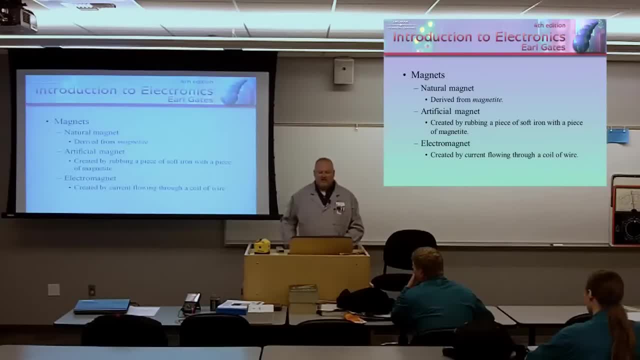 There's really several different types, three types: Natural Magnet: It's a magnet. I'm not going to talk about magnetism, because magnetism is actuallyら ketene. Magnetism is a material. Magnetism is other words that is derived from. 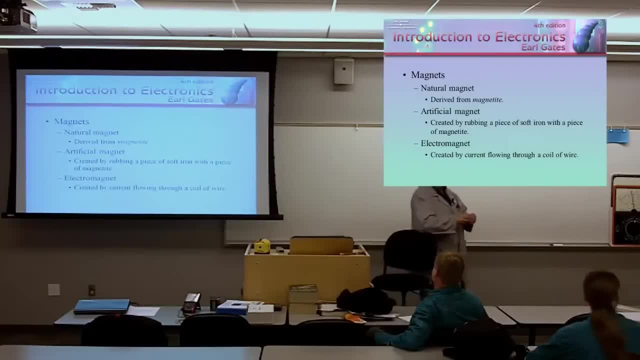 magnetite, Magnetite, And it just so happens that I've got a couple pieces of magnetite in my pocket. These are natural magnets, okay, that's like found in the earth's crust. Here it is, So we'll pass this around and we'll let you play with a, with polished 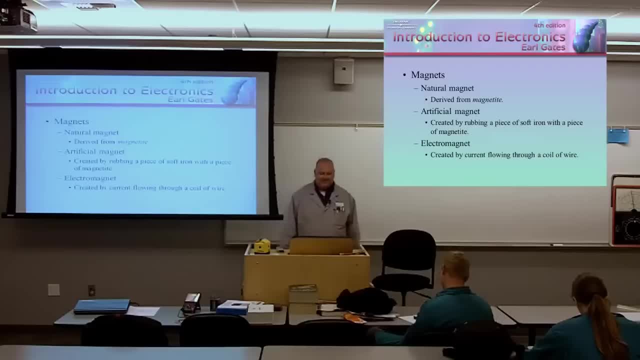 magnetite. Okay, So that's kinda cool stuff. So that's found in the earth's crust and it's be created by rubbing a piece of soft iron with a piece of magnetite. So if you've got a piece of soft iron and you know, I see underneath the 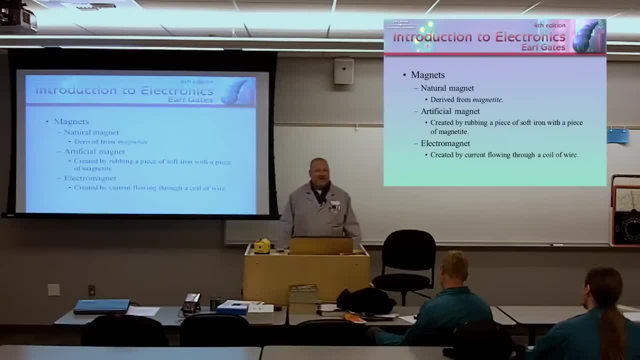 you know what the heck are you doing under there? I'm creating an artificial magnet by rubbing a piece of soft iron with a piece of magnetite, And what it's going to do is it's going to pull that magnetic property off of the magnetite. 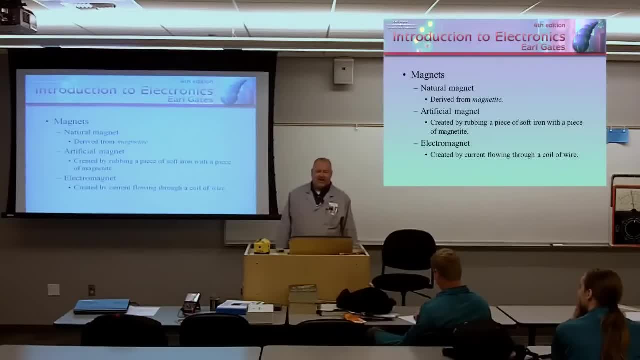 and transfer it to your piece of soft metal. Actually, that's a trick with a lot of mechanics, right? If you magnetize the tip of a screwdriver, it comes in handy for picking up things that you drop into odd places. Finally, the third type of a magnet is an electromagnet. 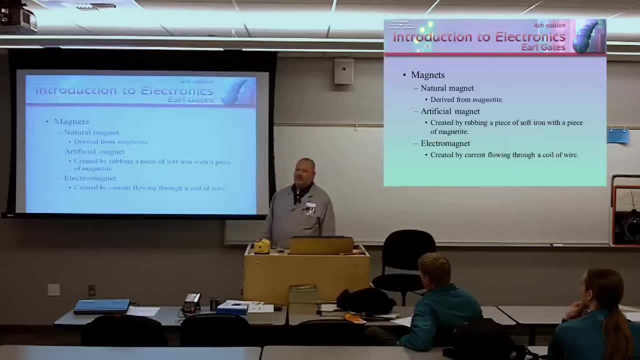 This is created by current flowing through a coil of wire. Basically, when we pass current through a coil of wire, we're going to develop a magnetic field And in concentrating that, that's how we have an electromagnet. So electromagnets range. 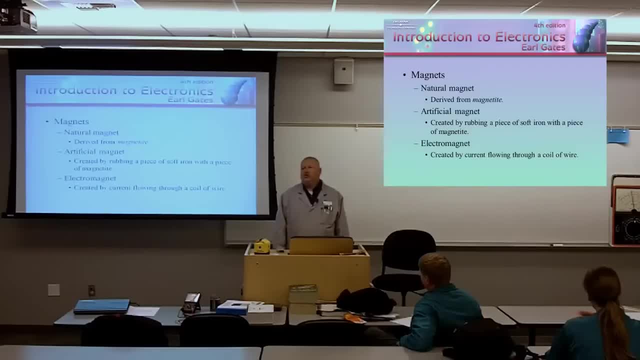 They range in size from very, very small to. if you've ever seen like at a junkyard, a scrapyard on a crane, they've got an electromagnet. You turn it on it like you know picks up a car or whatever. 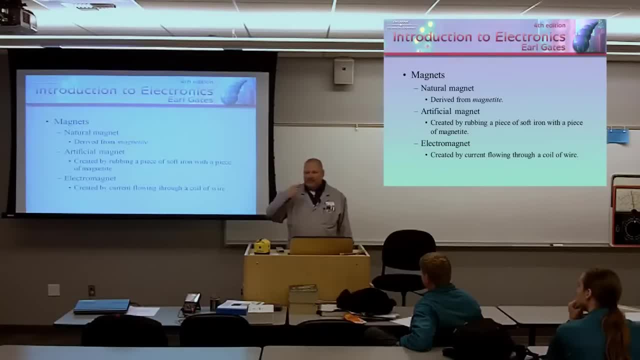 Actually my favorite application. I'm a big James Bond fan. Remember that Jaws dude who was, like you know, like biting things like train cars and stuff. And you know they turned on the big electromagnet and boom pow. 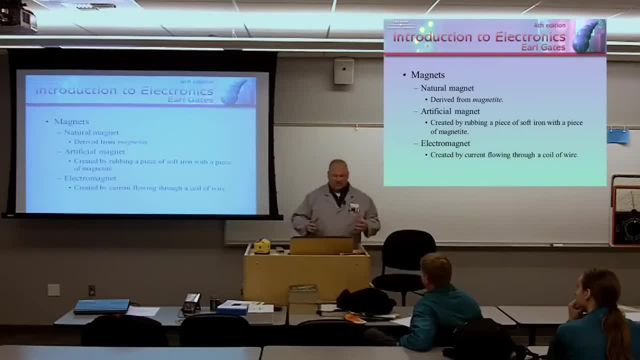 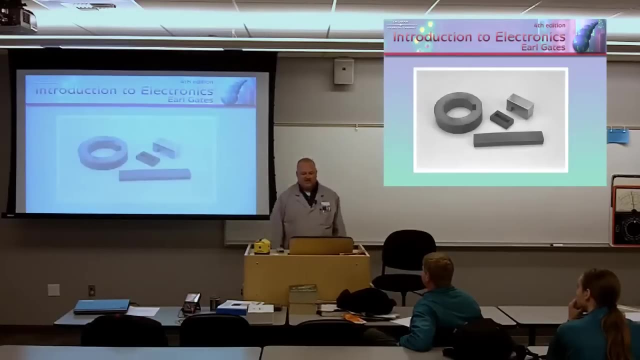 he gets pulled right up to the ceiling on that. So that was a giant electromagnet. I'd hate to have that. You don't have your credit cards anywhere near that, as your credit cards have magnetic strips on it And a strong electromagnet will probably desensitize those cards. 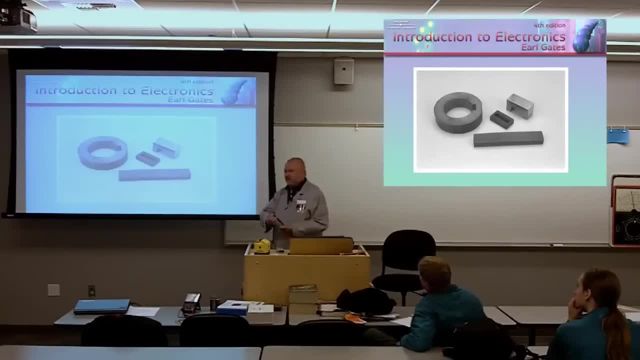 Here's some examples of some magnets. Come in variety. It's my personal collection, Just kidding. This is torrid core, meaning it's a donut-shaped, It's circular. This is a standard bar magnet. This would be like a horseshoe magnet because it kind of looks like a horseshoe. 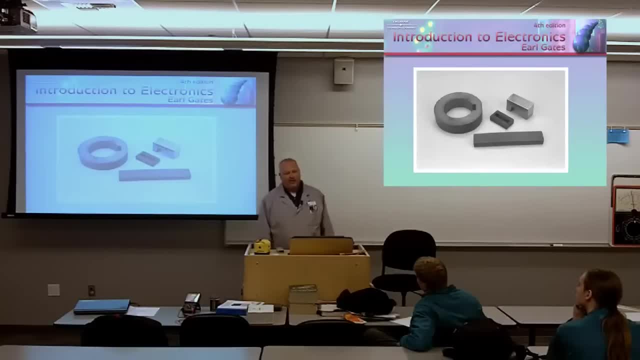 The thing to remember is that all these magnets are going to have a north pole and a south pole. Even that magnetite that we're passing around there, if you try holding it unusual- it won't even attach each other. Basically the reason that those four pieces of magnetite are attracted to each other. 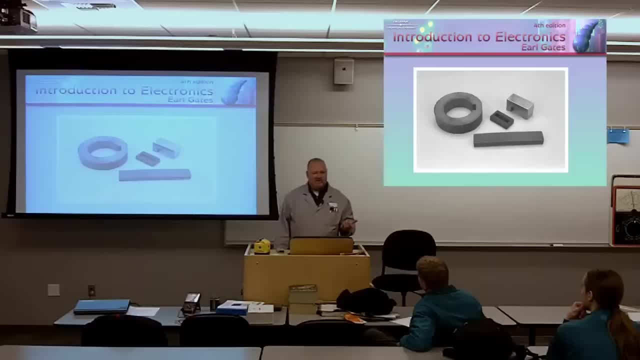 is because the north pole is attracted to the south pole of the other magnet which is attracted to the north pole, the south pole of the other magnet, North and north ain't going to work. Permanent magnets retain their magnetism. That's why they're called permanent magnets. 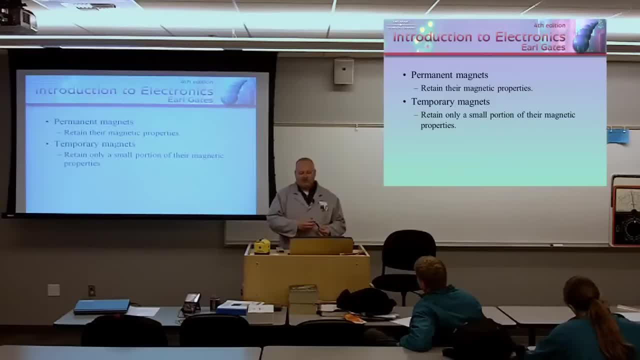 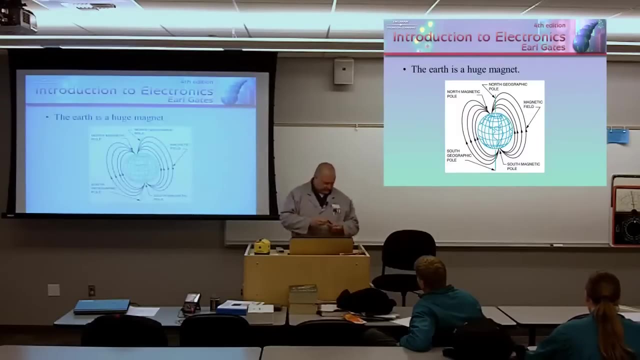 Temporary magnets are only going to retain a small portion of their magnetic properties- That's why they're called temporary Okay, and over time that magnetic field may deteriorate or be altered. So permanent magnet will retain the magnetic properties. Now, this is kind of cool and I'm sure it's no surprise to any of you. 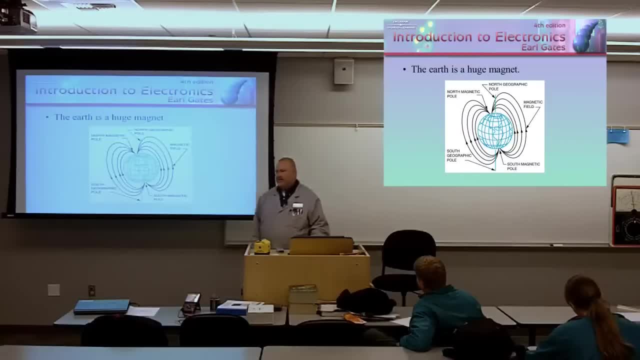 The Earth is a giant freakin' magnet. Okay, and it has to do with the core of the Earth and then the crust right, But we basically have a giant north pole and we have a giant south pole. The problem about the north pole and the south pole: I've got to give you a geography lesson here. 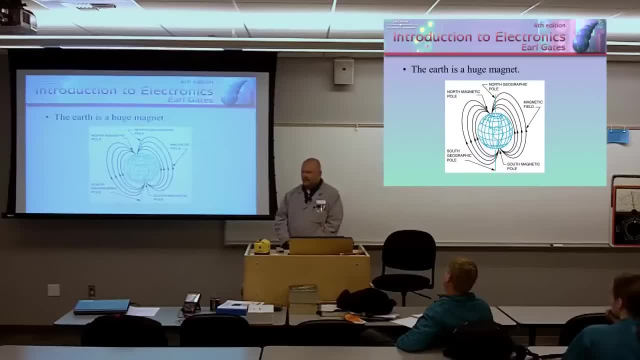 If I wanted to go find Santa Claus? if I wanted to find Santa Claus, where would I look and how would I get there? How could I navigate my way to this place With a compass, and where am I trying to get to? 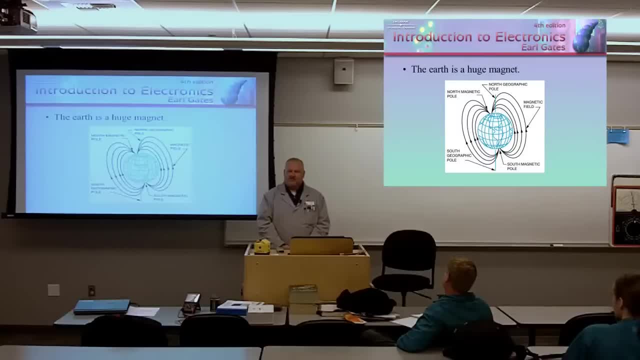 Okay, so you want me to use a compass to try to get to the north pole, to try to find Santa Claus, To get to the magnetic north pole. If I get to the magnetic north pole, am I going to find Santa Claus? No, Nowhere to be found. 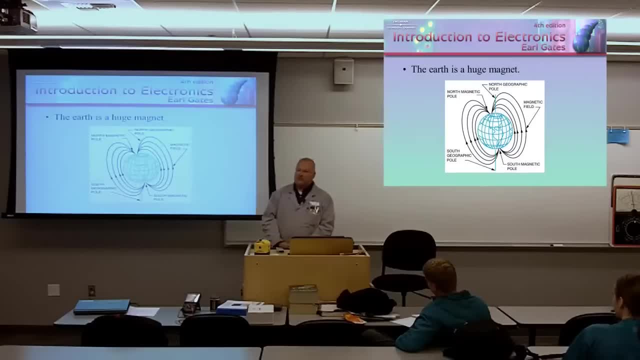 In order for me to find Santa Claus. what am I going to have to do? I'm going to have to go to the True north pole. True north pole Or the north, The north geographic pole, The north geographic pole, which is literally the top of the earth. 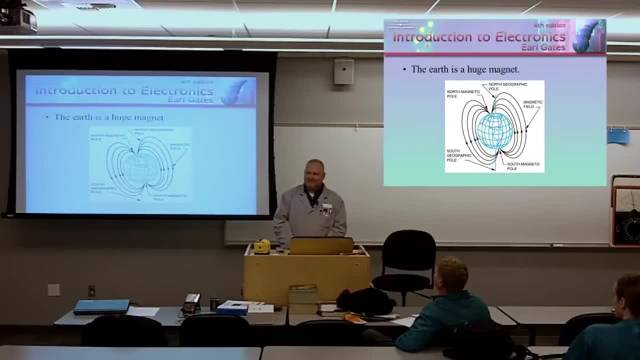 Anybody want to take a wild guess what the best way of getting up there might be? What's that? Well, I'm talking about means of transportation. What's that? Uh, Uh, Uh, Submarine, Submarine, Submarine, yeah. 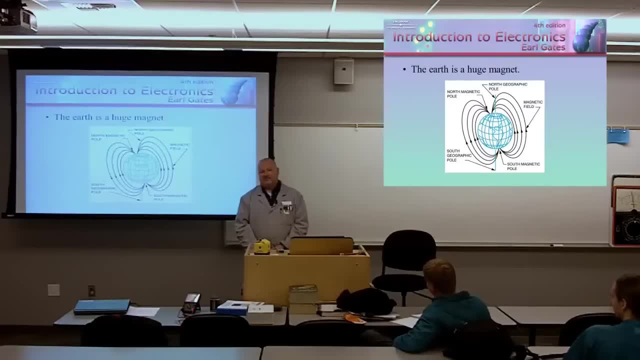 You could be in a short-sleeved shirt and go up there. surface at the north pole, because it's underneath the Arctic Ocean, So you could surface at the north pole. I just happened to flaunt that I actually have never been to the north pole. 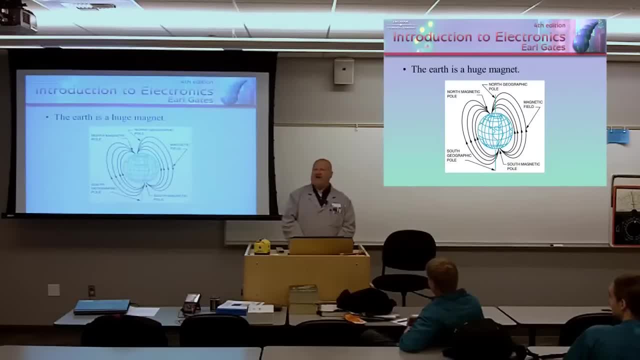 My submarine has been to the north pole. At home I've got water from the north pole in a vital, in a vial from my submarine that went to the north pole. My submarine actually delivered, believe it or not, Al Gore to the north pole. 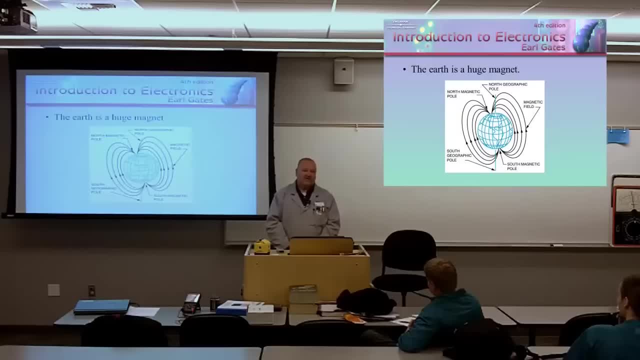 It was after I was off the sub, But they did a mission and went to the north geographic pole And typically on the ice, they put a lot of research camps to conduct research, magnetic research, And that's the place to do it. 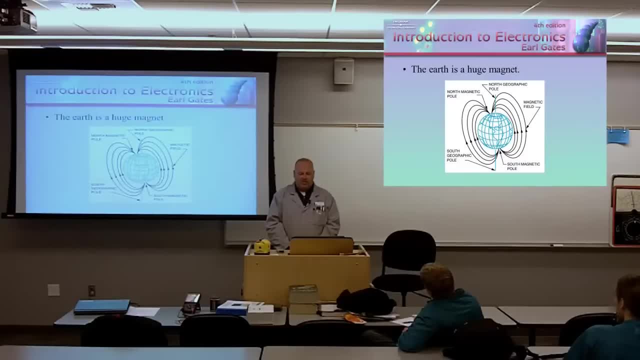 So the north magnetic pole is this illustration. it's an artist's depiction. It's not very accurate. The north geographic pole is here. The north geographic pole is going to be somewhere up here, up north of Labrador, And it moves about two kilometers per year. 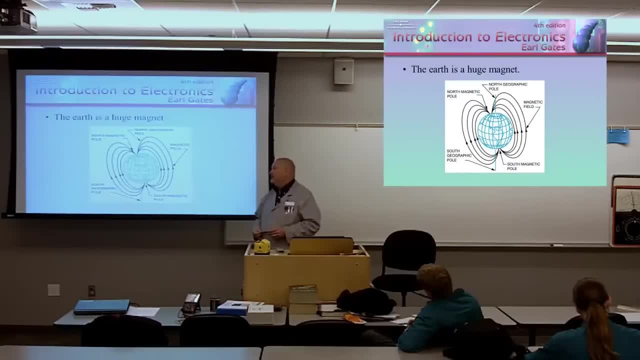 And it's actually moving in a northwesterly direction. And the variance, the magnetic variance. does anybody know the magnetic variance, The difference here between the north pole geographic pole and where the north magnetic pole is? I know because I'm a pilot. 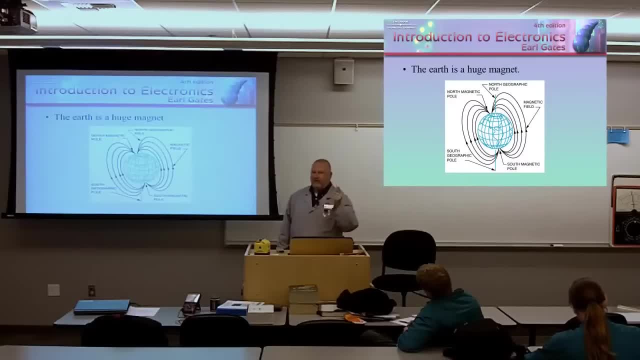 And it's kind of important. Okay, If I'm flying northbound or whatever which- am I going geographic north or am I going magnetic north? And the difference here in the Seattle area is between 19 and 20 degrees difference. It's pretty significant. 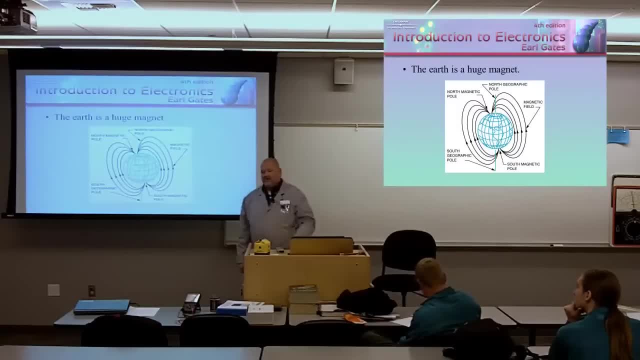 So this hallway right out here in this wing is aligned pretty much with the north geographic pole. If you could walk straight, which none of us could do, we've got a dominant leg And you walked out this hall and just kept walking north. 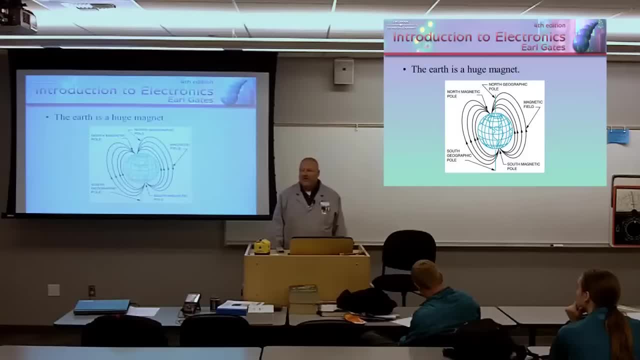 Eventually you're going to get to the north pole. find, Santa Claus, It's all going to be good. If you had a compass and you stepped outside the door here and you looked, that north magnetic pole is going to be literally over in this direction here. 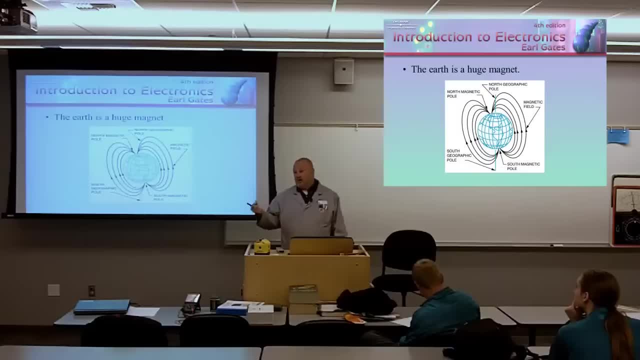 So it's very important because again in the aircraft you've got a compass. You set your gyro compass for that magnetic heading And I bet you folks never realized magnetic properties had such a profound impact on all these different things. If any of you are familiar with airports, airport runways are designated based on their magnetic heading. So Sea-Tac Airport. Sea-Tac Airport's got three runways, But they're all parallel with each other, so they all have the same numbers If you're headed southbound, like typically when we have crappy weather here in Seattle. 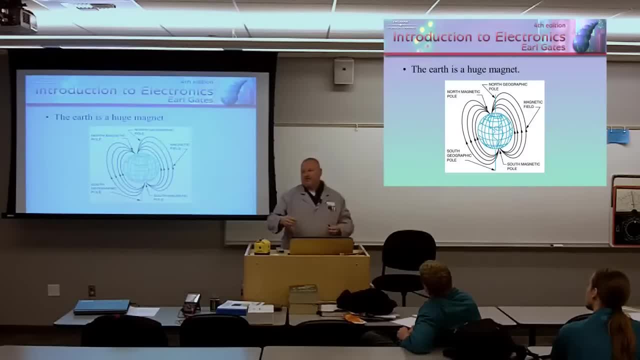 if you look up and you see an airport, you're going southbound. There's a plane going on the Sea-Tac. What he's going to do is he's going to fly out over Lake Magnolia. right then turn inbound. 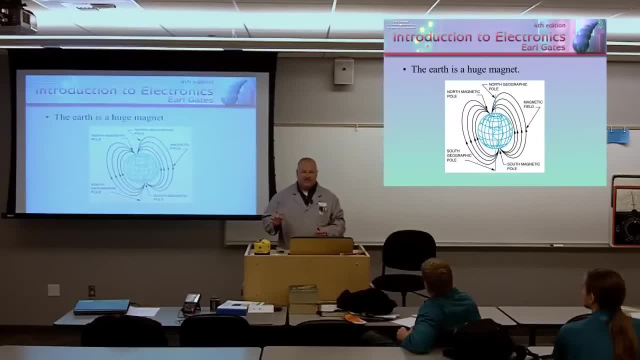 And then what he's going to do is land on runway 16.. Because if you rounded that, it's on a compass heading of 160.. So how do you make sure you're you know, since there's three runways down there? 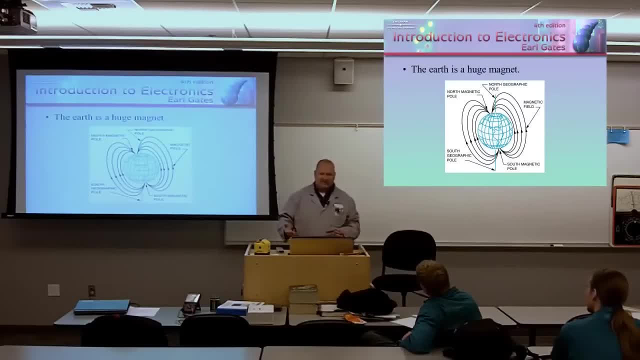 because we all remember those of us that have lived in the area a while, that third runway- when they put it in it was very controversial. It's 16 left, 16 center and 16 right, So you're going to have a compass heading of 160.. 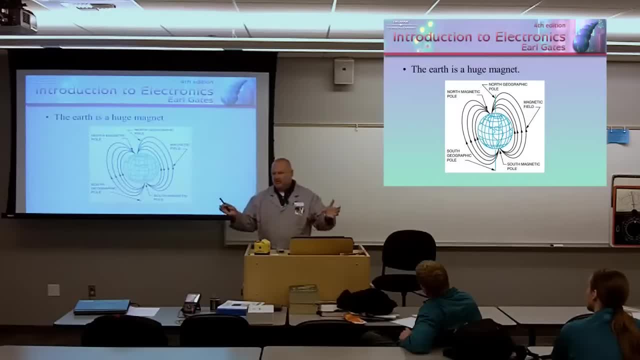 So how do you make sure you're you know, since there's three runways down there, you're going to land on runway 16.. Right, That's how they designate which runway you're cleared to land on. Add 180 degrees to that and you end up with what. 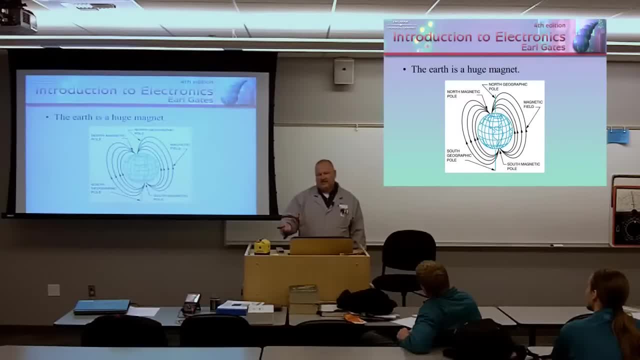 Runway No 16 plus 180 degrees Runway 34.. So if you're landing northbound at Sea-Tac Airport, you're cleared to land on runway 34 center, 34 left or 34 right. Okay that they select runways is they do wind studies to determine where the prevailing winds are. You want to take off into the wind and you want to land into the wind, So primarily here in central Puget Sound, that's pretty much how all the runways are. Auburn Airport: 1634.. Renton Airport: 1634.. SeaTac: 1634.. Boeing Field is a little bit different. It's runway 31 northbound, so there's going to be a slight variance in runway 13 in the opposite direction. That's just how the winds are kind of funneled there by the location of Boeing Field. But 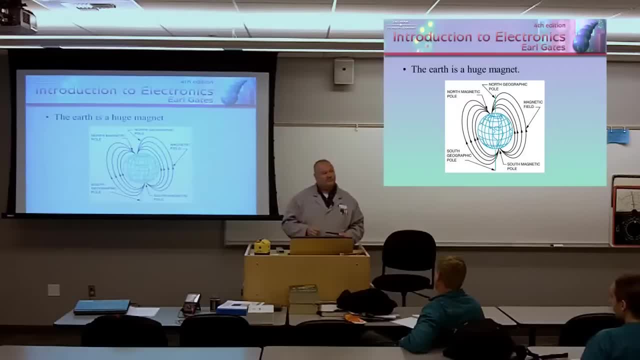 Renton Airport used to be runway 33, but because of that magnetic precession, what they've had to do is they've had to renumber And you think, oh, it's no big deal, You send a guy out there with a can of paint and you paint the new number on the runway. It's not. that It's not that easy. All of the procedures, all of the approach procedures, all of the publications, all of the databases, all have to be updated. It's really a big thing. So eventually, all runways are going to have to change their number as that north magnetic. 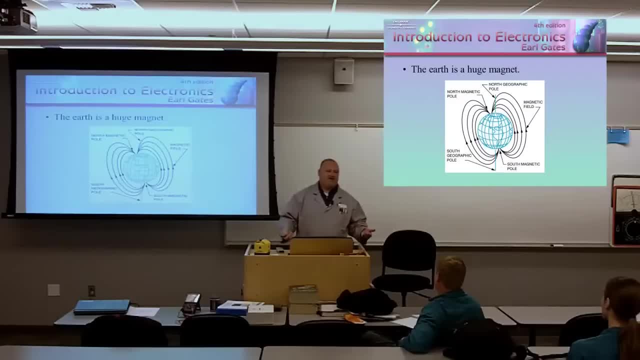 pole continues to fluctuate. Why am I telling you this? in an electronics class, A lot of you are going to go to work in industries that are associated with electronic navigation And you've got to know this. I mean you don't have to memorize it. I'm not going to quiz. 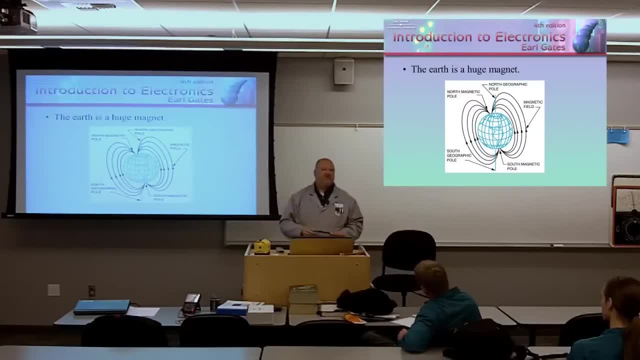 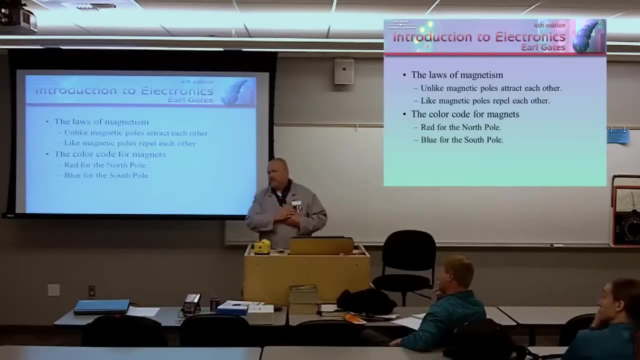 you on this magnetic precession in the 19. 20 degrees variance here in Seattle. but a lot of you are going to go to work in electronic navigation systems And you need to understand the difference between the two. Make sense The laws of magnetism. I think most of you probably remember this from elementary school. 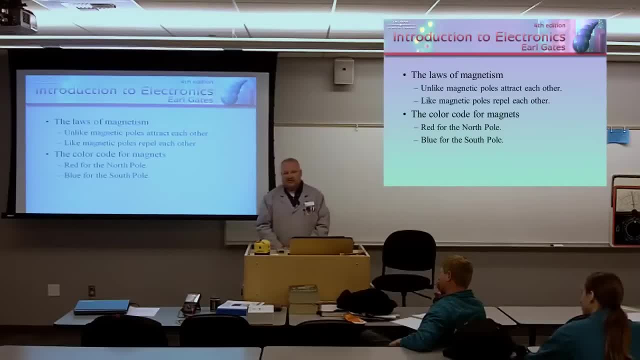 Unlike magnetic poles, attract each other right. Unlike attracts. So a north is going to be attracted to a south, A south is going to be attracted to a north. Like magnetic poles repel each other, North and a north. They're going to push each other away. 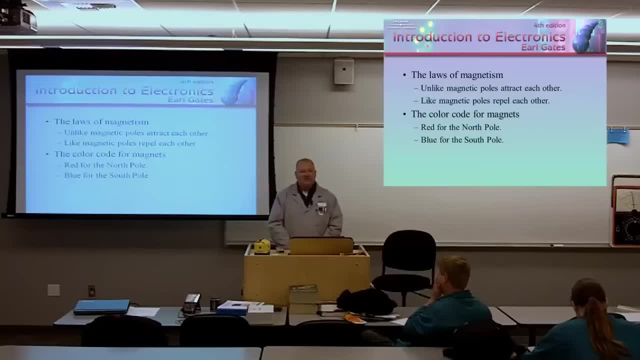 South and the south put each other away. This is actually kind of interesting too, because it has some applications now, like magnetic levitation. Some of these rail systems- that they're actually the whole train- levitates magnetically. That's how they're doing it. 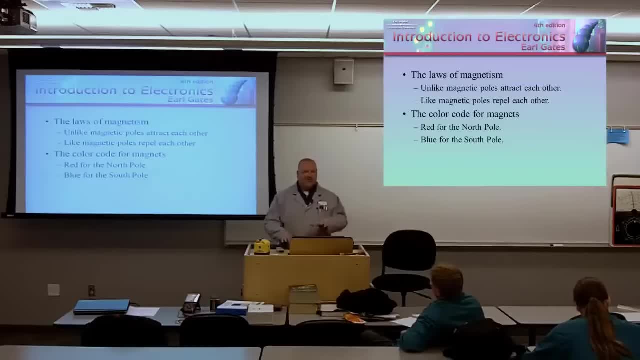 That's how you get a whole train to levitate, because North Pole and the North Pole, they'll basically push each other away. And then, once you've got something floating like that, it doesn't take a whole lot of energy to move a train. 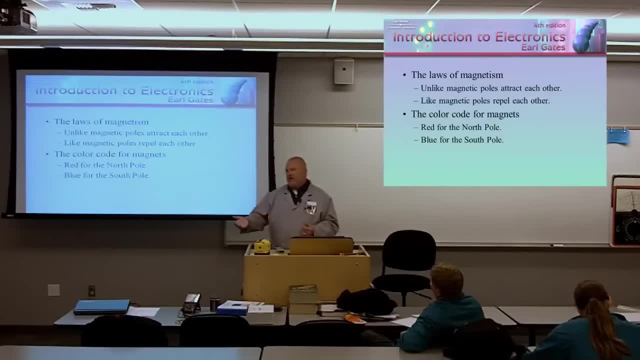 I mean think about that. I don't know if you've ever even thought about why do we use trains? I mean trains that wheel on a rail, very little friction, So it takes very little energy to move a bunch of stuff. 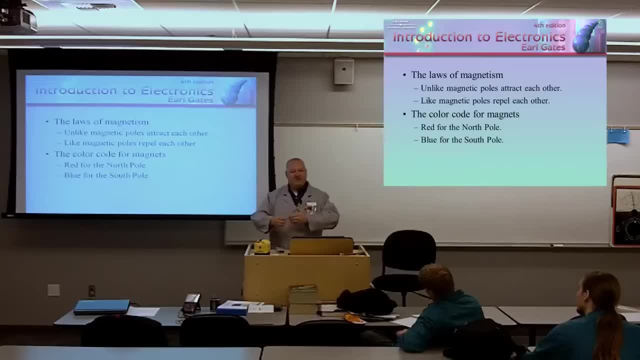 If you could kick it up even a notch further. I mean, we still have to overcome the friction of the bearings and the axle and the wheels on the track. Now, if you could levitate the entire, the entire train magnetically, then just give it a little push. 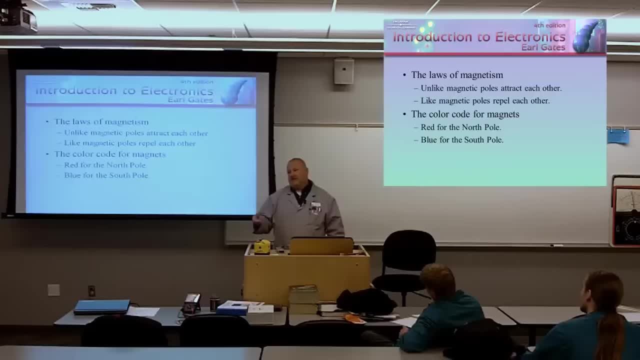 and that thing's going to be able to move with hardly any energy. So these are a lot of the advancements that we probably want to stay tuned for, because, in the name of efficiency, we're trying to play with a lot of this stuff. 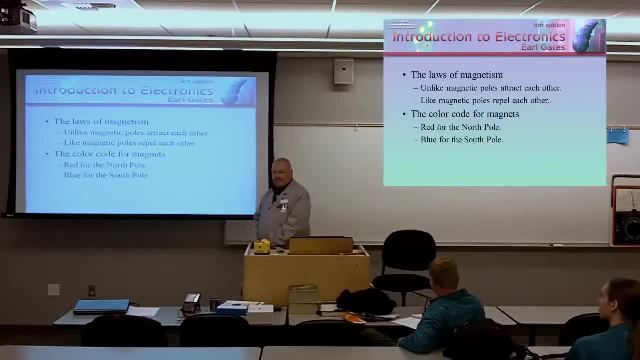 Color code for magnets. Color code for magnets: Red is the color code that we use for North Pole. Blue is the color code that we use for the South Pole. So if we were going in search of Santa Claus and we got to the North Geographic Pole, 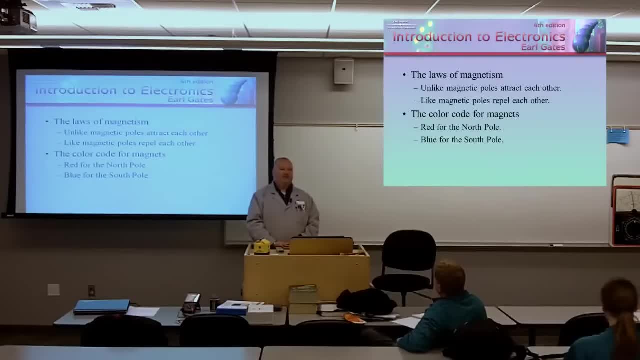 what? how would we know we got there? What would we see? Bzzz, There'd probably be reindeer. but what color pole would there be? Red and white. very good, Red and white pole. we know that Candy cane right. 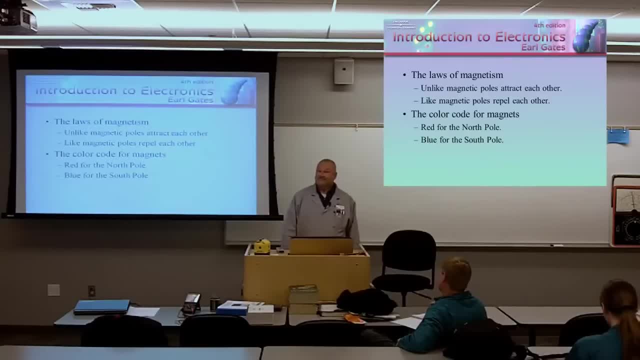 If you were at the South Pole, what color would the pole be? Blue and white Stripe pole. Yeah right, I mean you've got to follow that same tradition. If you're outside a place that has a pole that's red, white and blue, where are you? 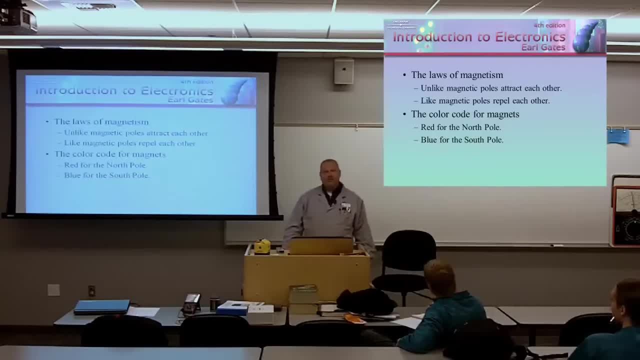 Bingo. Excellent, very good. I've got students that just Same students that don't know what a barbershop is. I like the barbershop, That's how I roll, That's my thing. So yeah, that's the color code for magnets. Magnetism. the property of magnetism can be traced to the atom. As electrons orbit the nucleus, they also spin on their axis. This electrostatic charge produces a magnetic field. So even these electrons are going to have magnetic properties. The direction of the magnetic field. 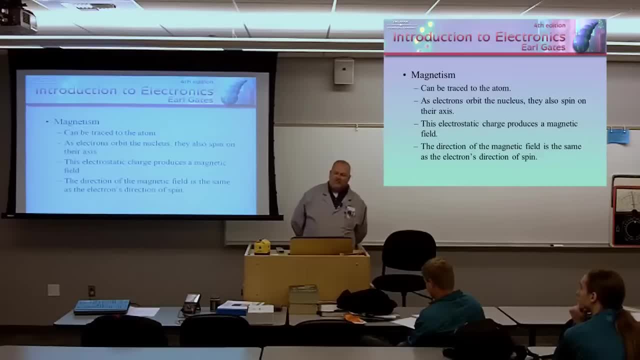 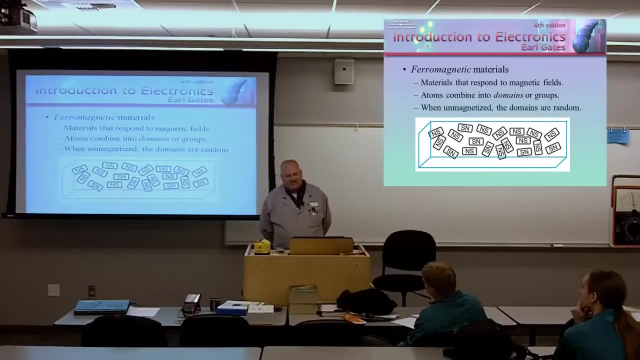 is the same as the electron's direction of spin. So even at a subatomic level we're going to have properties of magnetism. Ferromagnetic materials- ferro meaning materials that contain ferrite- this is the stuff that will rust. 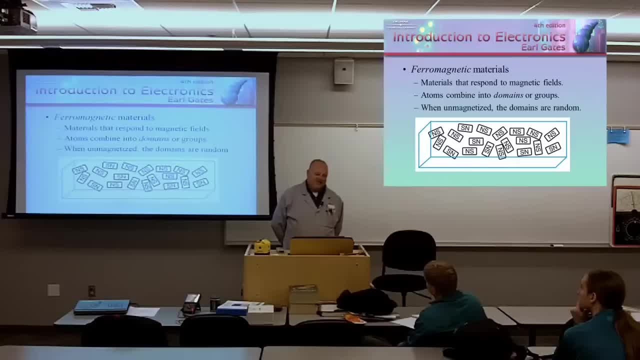 If the metal will rust, it contains a high amount of ferrite, So any ferromagnetic materials are materials that respond to magnetic fields. Any of you have magnets- Magnets at home- stuck to your refrigerator. Okay, your refrigerator is made out of a ferromagnetic material. If it were not painted, it would rust, Plain and simple. If not, the magnets wouldn't stick to it. That's actually the old trick too, if you're going and buying a used car or whatever and you're looking for bondo, right. 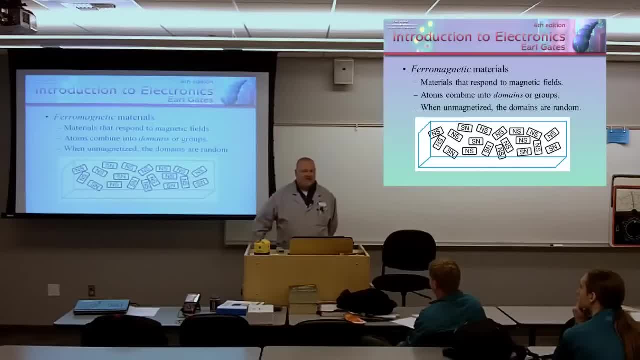 Put a magnet over it and obviously, if it sticks, you know that that's all original with no bondo. You know you all of a sudden get to an area and that magnet doesn't work, It doesn't want to stick. Don't try this with a Corvette, of course. Corvette is fiberglass And actually with all the cars now, with all the plastic on them, magnets aren't going to stick well to plastic. Atoms combine into domains or groups. When unmagnetized, the domains are random. This is what we're looking at here in this illustration. 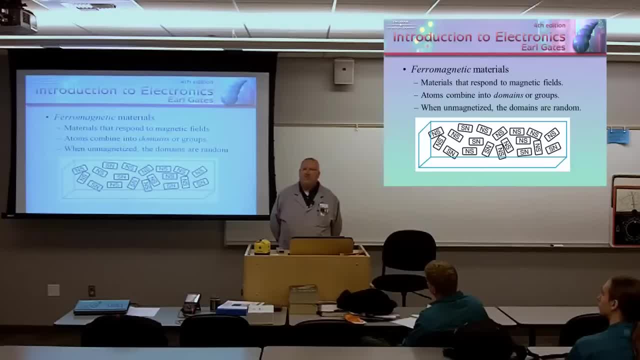 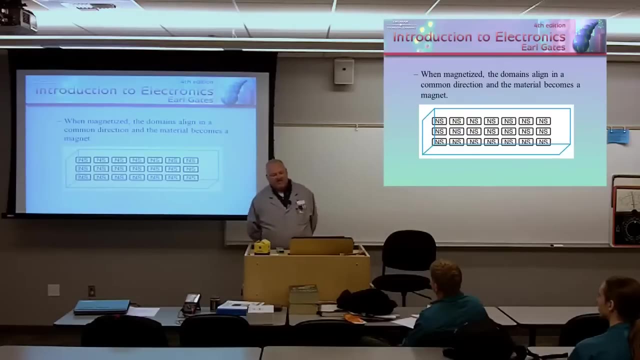 This is random domains. okay, This is an unmagnetized piece of ferro magnetic material. As soon as we magnetize it- watch This is kind of cool- Boom. When magnetized, the domains align in a common direction and the material becomes a magnet. 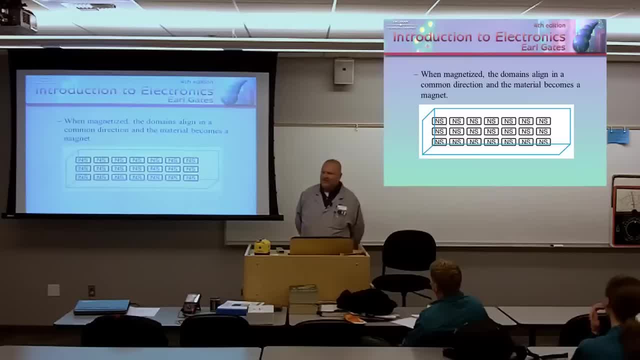 So if you've got my magnetite that we're passing around and you rub a screwdriver up against that, this is ultimately what's going to happen: You're going to align those domains and it's going to become magnetized, Magnetic. What would it do to a ferrous and a non-ferrous metal again? 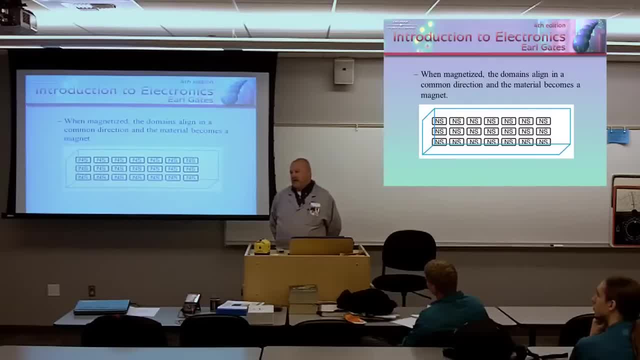 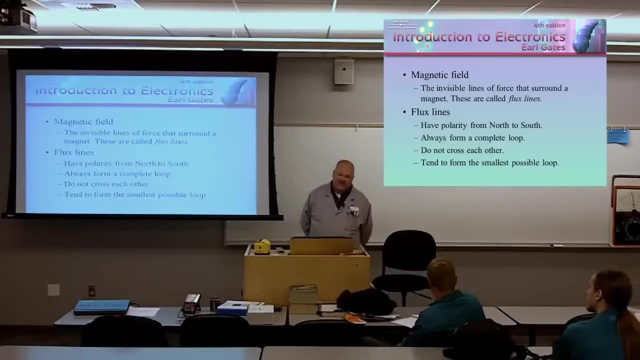 Ferro. Ferro contains ferrite and that's the iron content that makes stuff rust. basically, Now, a magnetic field, a magnetic field. this is kind of where you've got to hit the I believe button. right, It's invisible lines of force. 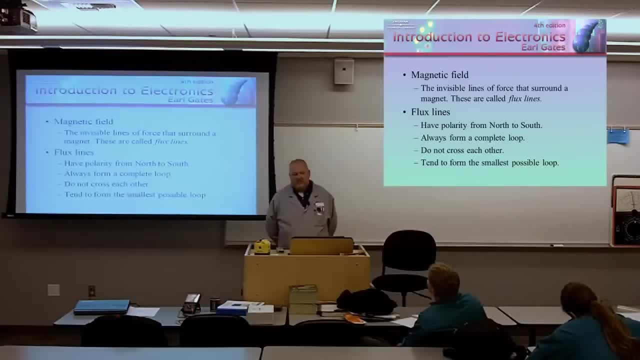 That surround a magnet. These invisible lines are called flux lines. We've got to be careful, because those of you in ELEC 115 are learning about flux right, It's a different kind of flux. There's two types of flux in electronics. 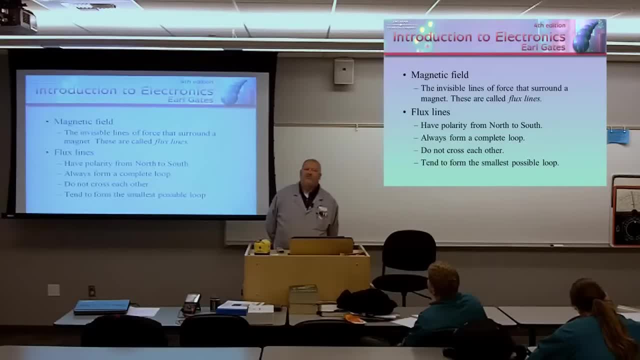 There's magnetic flux that we're talking about tonight and there's also flux that we use as a cleaning agent for soldering. Okay, You're not going to use a magnetic field for cleaning and soldering, to the best of my knowledge. 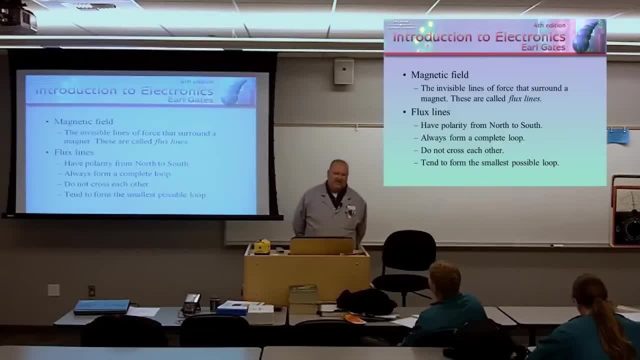 and a magnetic field has never been used as a cleaning agent. Flux, however, is used as a cleaning agent, a different type of flux. Okay, So this word has two meanings in electronics, And don't forget, one of the reasons that you're here is to learn the language of electronics. 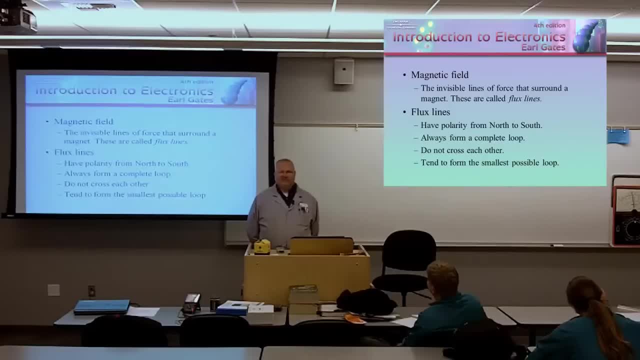 I wish I had had me as an instructor, okay, Because I was kind of like flux and I was like why are we going to use magnetic lines of force? to, you know, clean something to make it more solderable? Just you know. 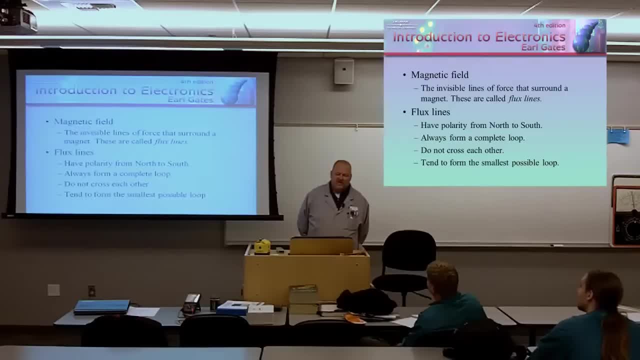 nobody ever explained that to me and I wasn't the smartest student. These flux lines, these flux lines have polarity and that polarity is north to south, North to south and it always forms a complete loop. They do not cross each other. 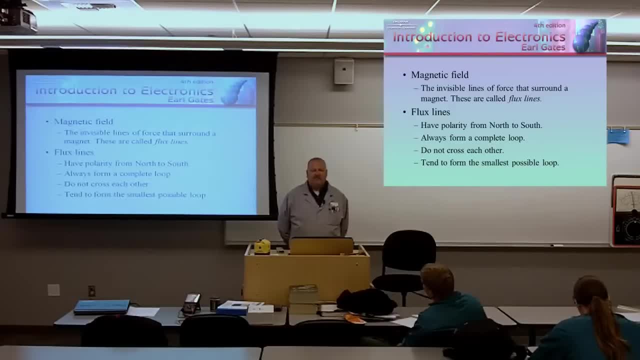 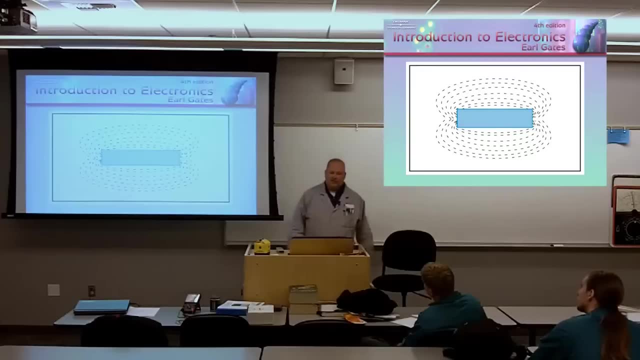 And they tend to form the smallest possible loop. Some of you may have done this, like in third grade: You got a magnet, bar magnet, you got a piece of paper and on top of that piece of paper you sprinkle iron filings. 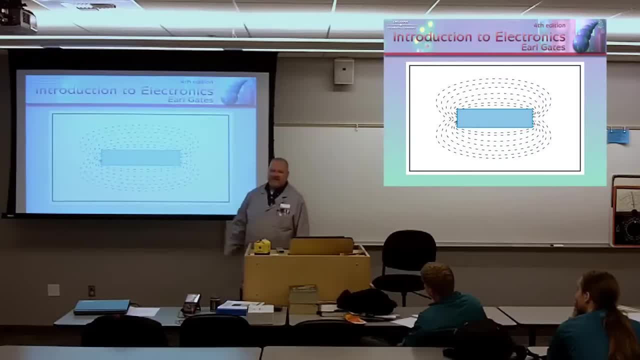 The iron filings will actually form a pattern, and that pattern that you see is the invisible lines of force. It is the flux lines. That's exactly what you're doing by spreading those iron filings on. that is seeing the lines of flux. 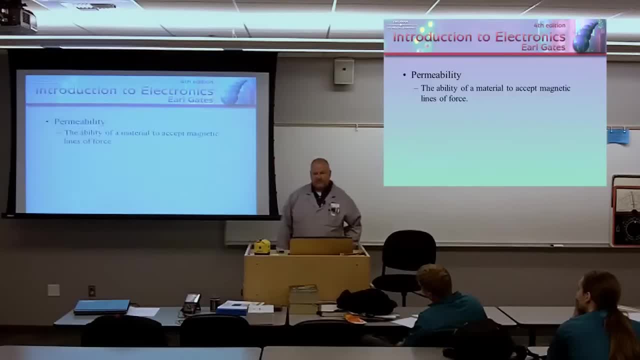 as a visual aid, if you will. Permeability: there's a new word for you. Permeability is the ability of a material to accept magnetic lines of force. An example of something that has a high level of permeability would be your refrigerator at home. 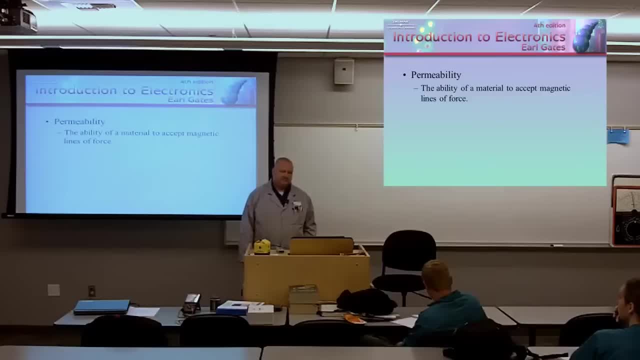 If you've got magnets stuck to it. My last refrigerator that I bought and you never. how many of you here like buy a refrigerator because, like you've got nothing better to do, And like how many of you like buy a refrigerator. 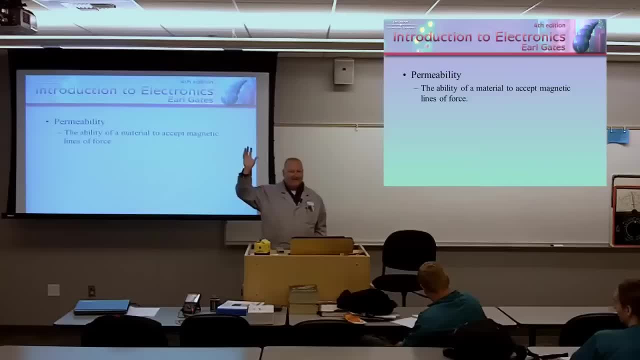 because your food is all spoiled and your old one died. You know, I mean, that's normally how you go about it. So you know, my last refrigerator. I was like in a panic and I found one. 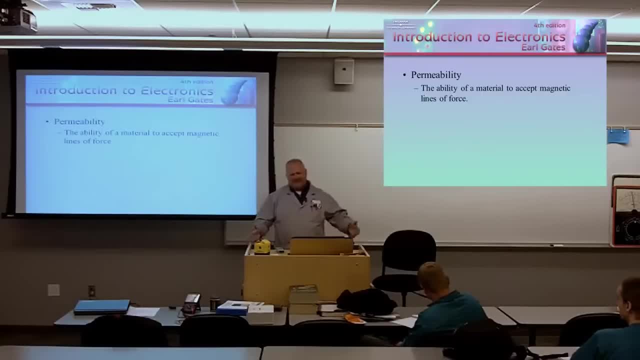 and um what, uh, and they never fit right. You know they've actually made them bigger, so if you want one to fit into the small hole, you've got to get a custom refrigerator. So a smaller custom refrigerator costs more. 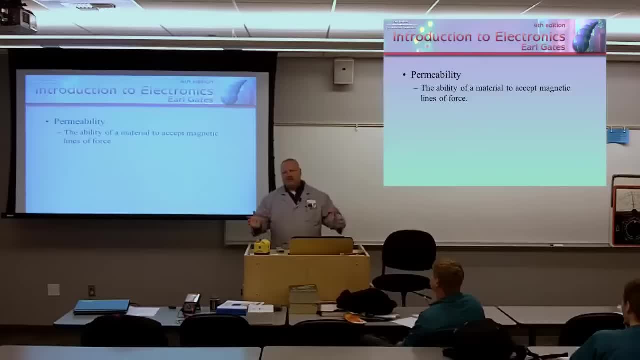 than the big one. that doesn't fit right. Right, The big one. it doesn't fit right, It's bigger, whatever. But I get home and I paid a lot of money for this thing and then I get my magnets. 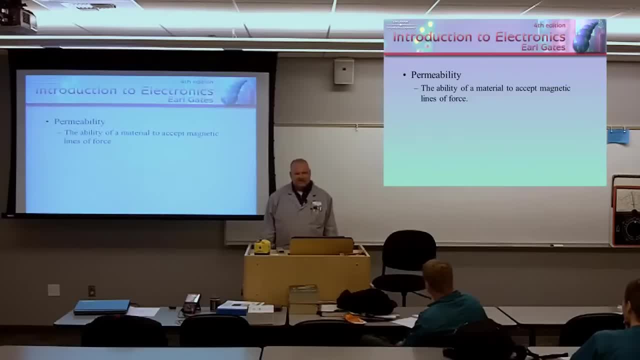 and I got, you know, the magnets to put Junior's work up on and everything else and my favorite pizza place Magnets won't even stick to this thing because it's like this designer facade. so you could. what the heck is this? 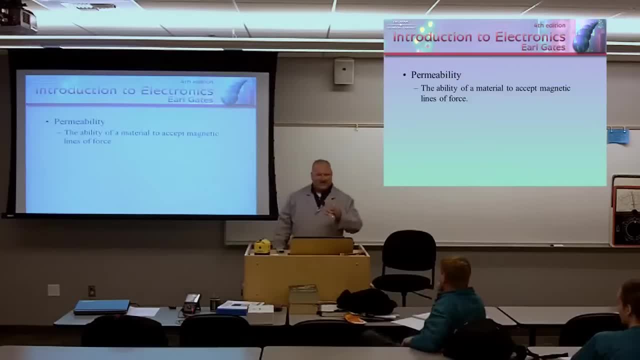 You know. So you've got to put the magnets on the side. You've got to put them on the side because the front is, so that you could make it. you know, I don't know, I just want something to keep my stuff cold. 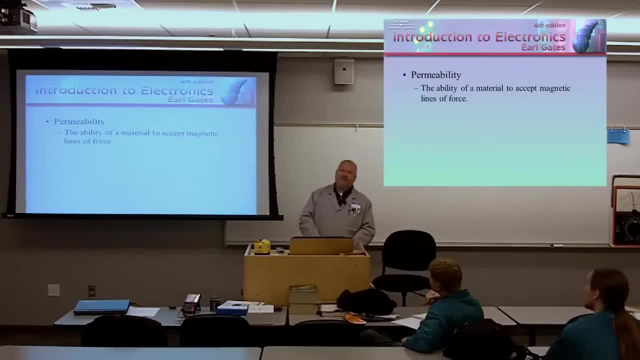 That's all I want. So permeability is a material that readily accepts these lines of force. If a magnet will stick to it, it has a high level of permeability. Now there's a direct correlation between electricity and magnetism, probably why we're talking about it tonight. 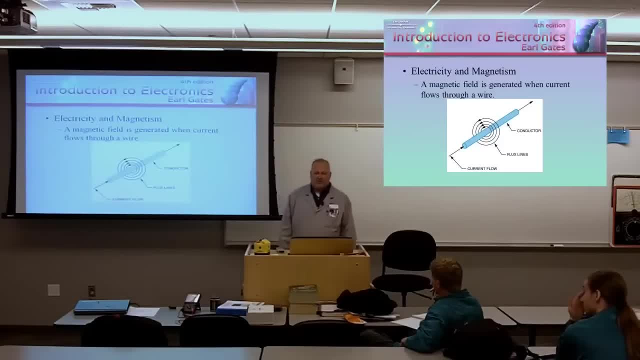 right in the electronics program. A magnetic field is generated when current flows through a wire period, Period Period. Let me say that again: A magnetic field is generated when current flows through a wire period, So when you plug something into an extension cord. 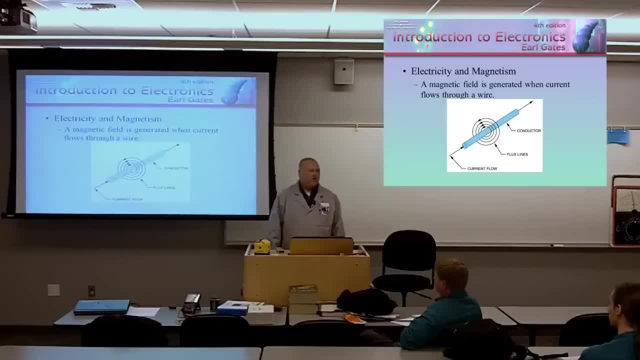 is it generating a magnetic field? You betcha, When you have, when you connect a speaker up to an amplifier and you've got current flowing through that wire to the speaker, are you generating a magnetic field? Yeah, Okay, Anytime current flows. 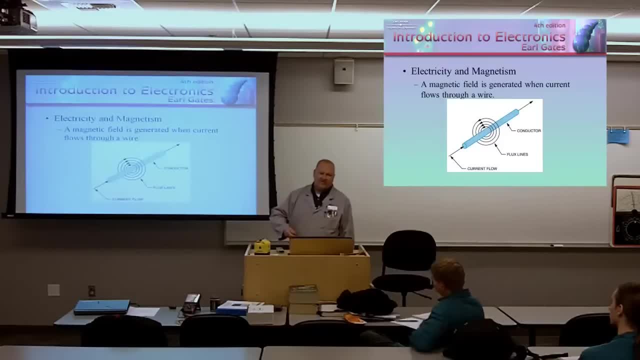 through a conductor, you generate a magnetic field. So if you could see magnetic fields and you had an energized piece of equipment, you would see all of these lines of flux that are being formed by simply turning a piece of electronics on. 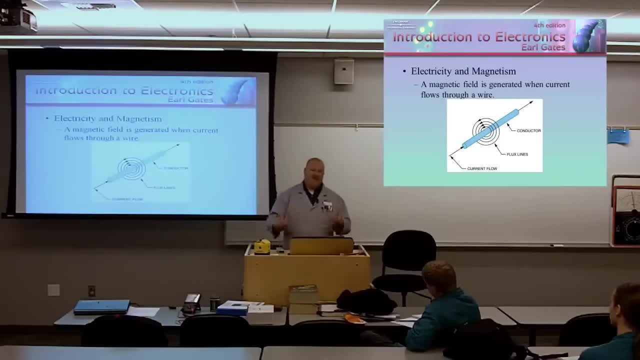 By simply turning a piece of electronics on or an electrical circuit on, you're generating lines of flux. Sometimes it's something that we need to be aware of. other times it's something we need to discount. An example would be in your home, okay. 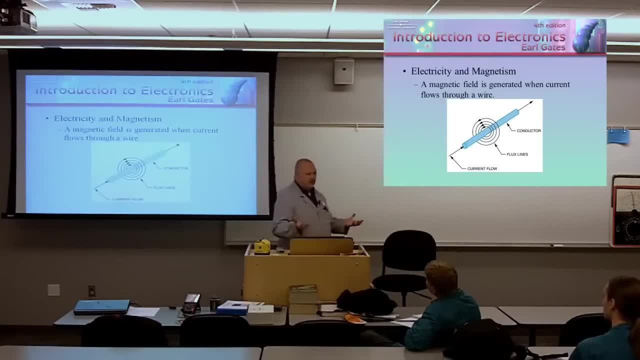 Typically how your house is wired up. the magnetic fields that are generated by your home are not sufficient enough to cause you any worries. They're not going to demagnetize your credit cards. they're not going to. you know. screw up your brain, you know. 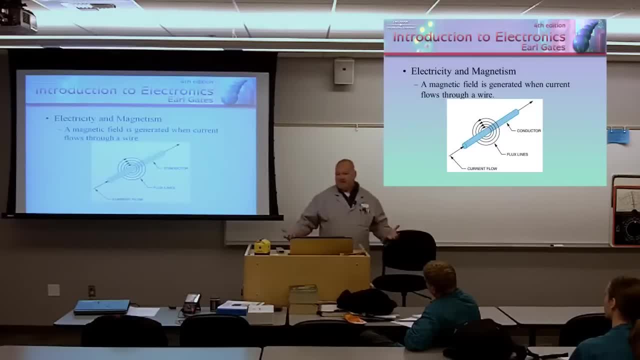 But still they are generating magnetic fields. There's no way around it. We were going to talk a while ago about staring at a computer screen for too long, so the magnetic field could affect you after a while. Yeah, and again with some computer screens. 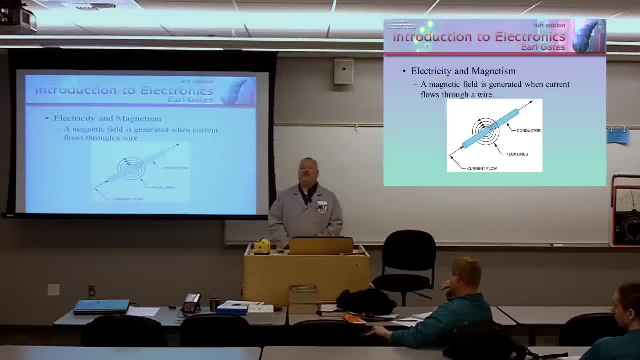 there's some higher frequencies that are used and I mean it's the same thing, You know. is it harmful or harmless, I don't know. There's also some laws on the books about building schools underneath power lines, you know. 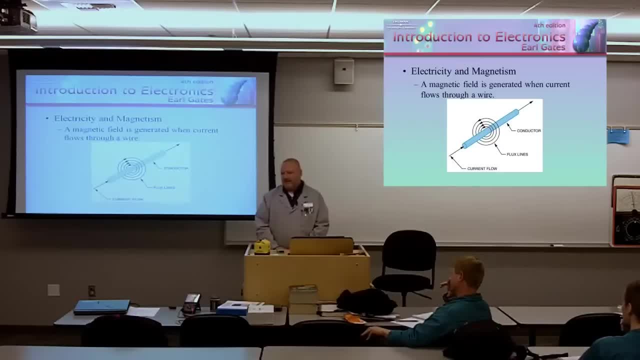 So if there was nothing there, why are there laws on the book about that? you know I've never had an interest of well, my only interest of living underneath a power line would be able to perhaps tap into that magnetic field and lower my power bill. 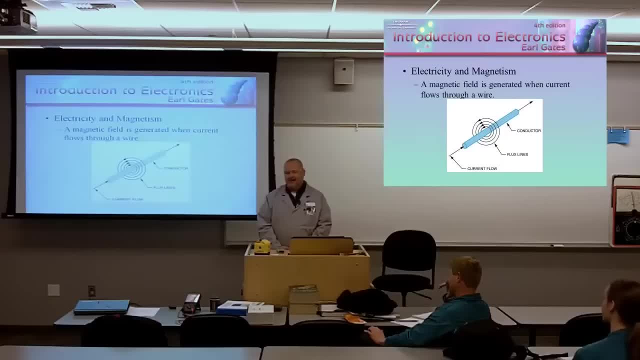 which of course would be illegal and not above board and I would never do that. But I never really had a whole lot of interest of like living underneath power lines, you know, because it's just an unknown, You just don't know. 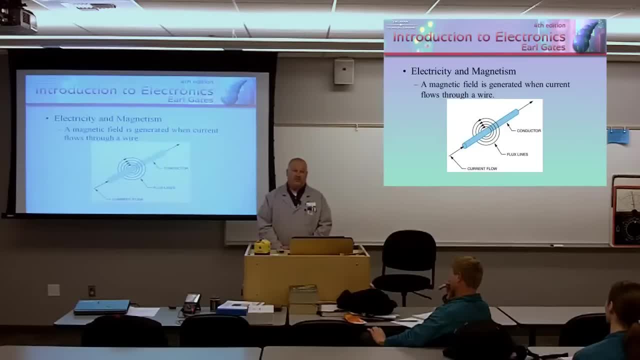 Because those high-voltage wires they move a lot of current through it. I mean you create huge magnetic fields. I don't know if you realize this, but if you get a fluorescent tube and you go underneath a lot of these high-voltage wires, 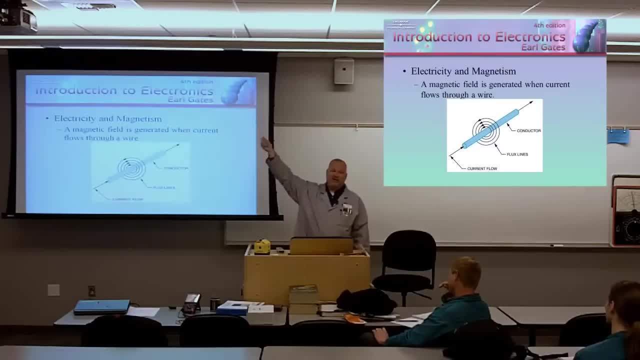 you could excite the gases inside the fluorescent tube and light it up. Look, Mom, It's lighting up with no strings attached. So if it could ionize gas inside a fluorescent tube, you know what's it doing to your And I don't know about you, you know. 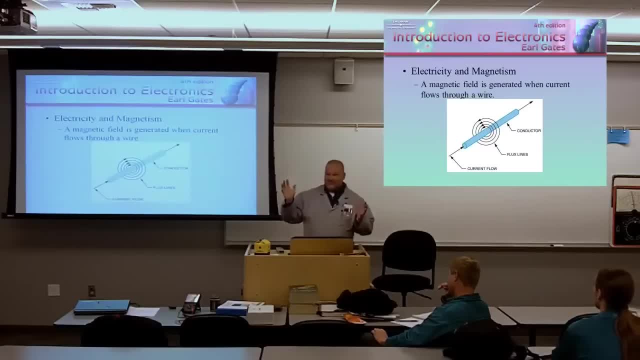 but I've had a pretty good life. I've got a lot of good memories. I do not want to scramble those memories So I'm going to keep my brain away from magnetic fields and anything else that will alter some of these fond memories that I have from my youth. 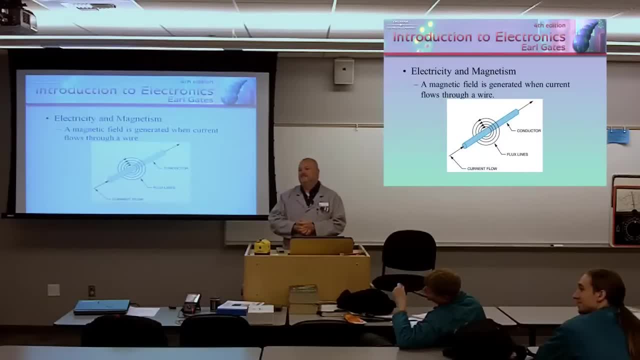 Well, yeah, my journeyman told me that exact same thing. My mom was going to buy a house by a power line. She said we'll go out there with a fluorescent tube and hang it up If it lights up. she don't want the house. 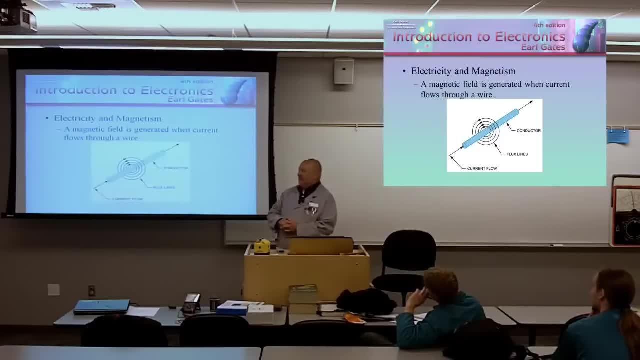 Yeah, yeah. So this is exactly what it would look like. here We have current flowing through a conductor and we're going to generate this magnetic field around the outside. If the magnetic field is strong enough, stuff would stick to it- Normally the magnetic field. 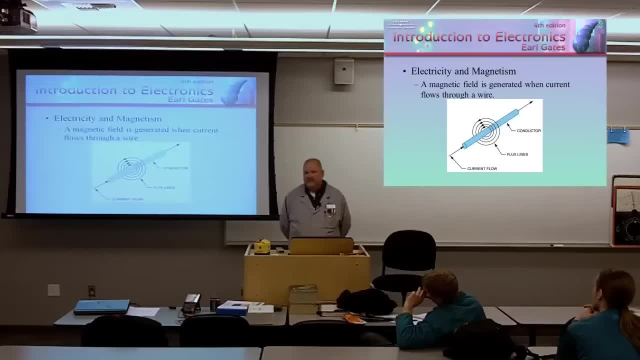 The magnetic field is not that strong, so stuff won't necessarily stick to it. Like iron filings are not necessarily going to be attracted to a low-energy circuit that's energized. But that being said, there's still a magnetic field there. It's just not strong enough to attract an iron filing. 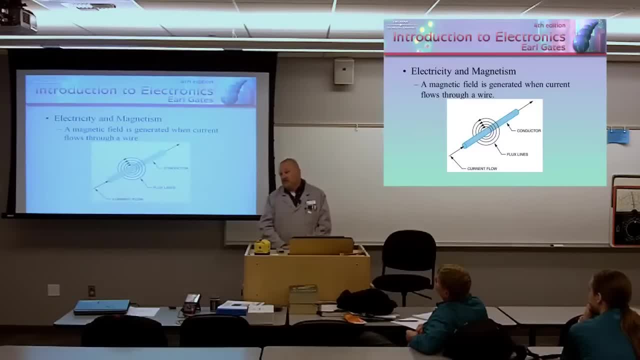 to stick to the circuit, Thank goodness, Or whenever we turn anything on, it would be Now. Yeah, it would have to be a significant enough field to attract, you know, current. to do that, The current going through it would have to be sufficient enough. 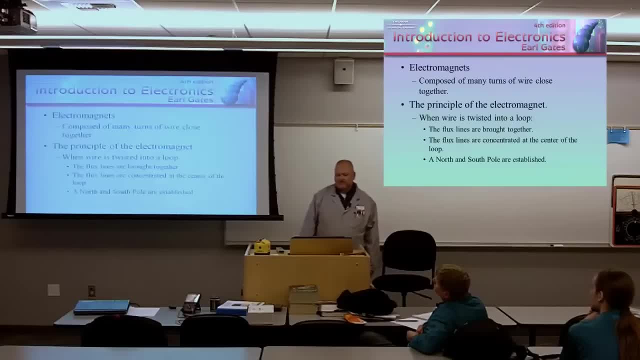 to create a big enough magnetic field to attract an iron filing Electromagnets composed of many turns of wire close together, Because, as I just said, one piece of wire may not be strong enough. What happens if you get that and then you wrap it around again? 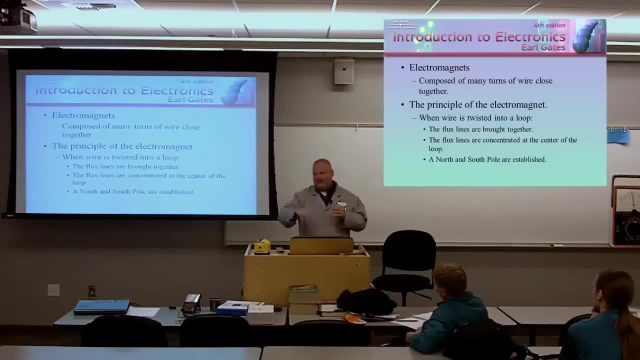 Now you just doubled it. You do it a third time, you triple, fourth time, quadruple it. The math is simple. The math is that simple. So every time with a winding you add a winding, you're increasing that magnetic field that you're generating by it. 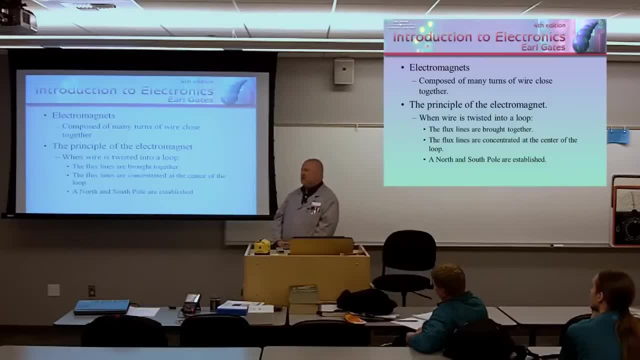 So the principle of an electromagnet. when wire is twisted into a loop, the flux lines are brought together. The flux lines are then concentrated at the center of the loop and we establish a north and south pole. Any time you create a magnetic field, you're creating both a north pole and a south pole. The strength of the magnetic field can be increased three ways. The more turns of wire, the more flux lines are going to be added together and concentrated. The greater the current, the greater the number of flux lines that are going to be generated. 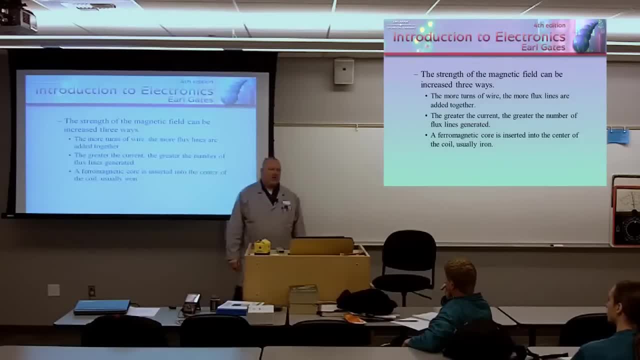 This only carries you so far, though, Because what happens? you're passing current through. what A piece of wire? What property does wire have associated with it? Resistance. So you just can't keep increasing the current, Because if you keep increasing the current, 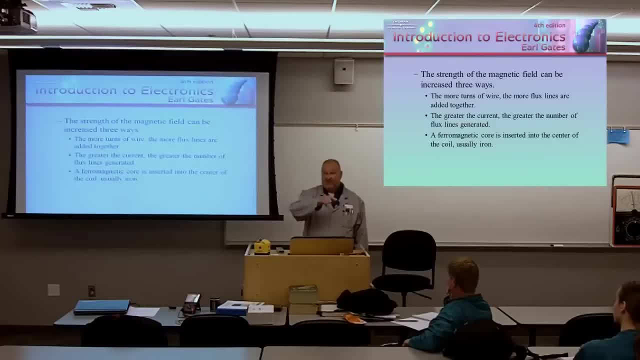 eventually, what's going to happen? It's going to become a fuse. I mean, even if the wire is this thick, you have enough current. go through wire that's this thick. eventually you're going to part that wire, Okay, Okay. 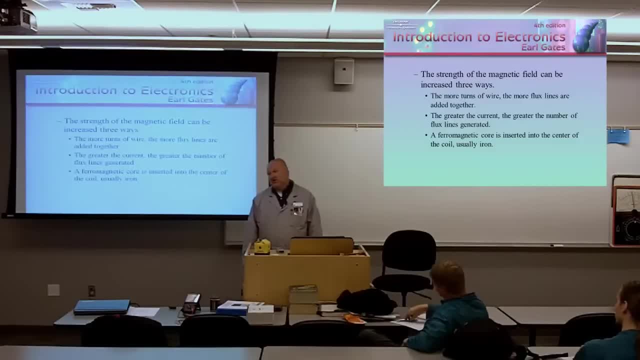 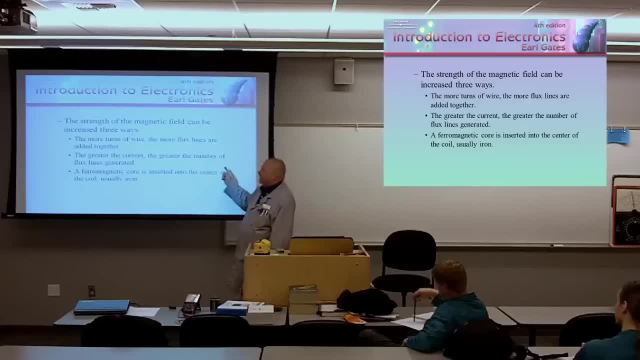 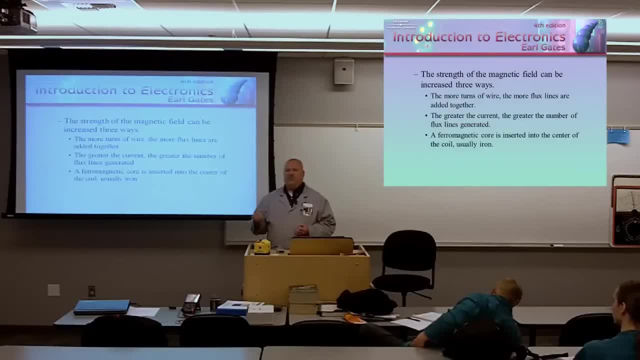 Magnetic wire is wire that's used to make windings, And what it is is thin copper wire, but it has a lacquer coating on the outside. Okay, There's an example right there Outstanding. That's magnetic wire, Okay, And it looks like copper wire and it is copper wire. 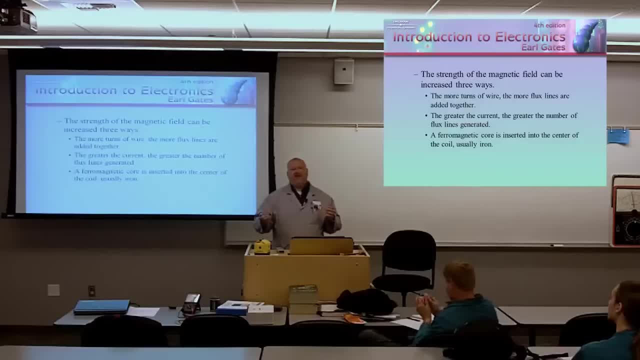 But on the outside is a thin lacquer coating. That lacquer coating acts as an insulator, an electrical insulator, to prevent the wire from shorting. Because if I wound wire over itself, why would current want to go all the way, keep going through the wire? 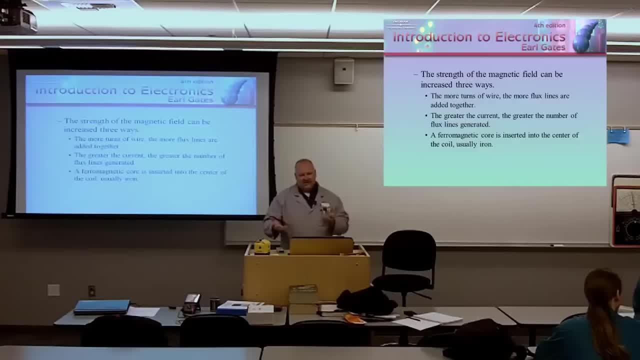 It would just short right out. Okay, so we have to keep it insulated by using that lacquer on it. So let's get back to this bullet statement here: The greater the current, the greater the number of flux lines generated. I'm going to get to a point that I cram so much current through that coil. 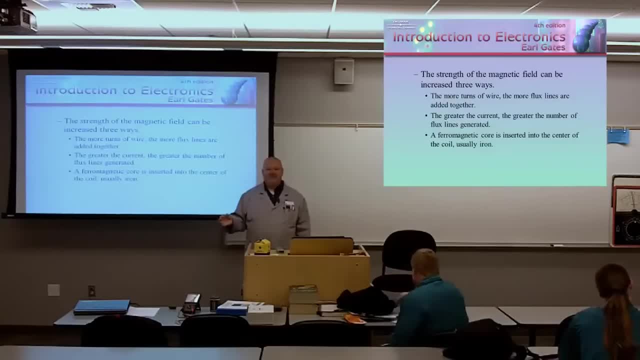 it's going to begin to get hot. If any of you have ever done paint removal, you know that that paint removal when you're using a heat gun works really, really good for removing paint. It works good on removing lacquer too. So once you have too much current, go through that coil. 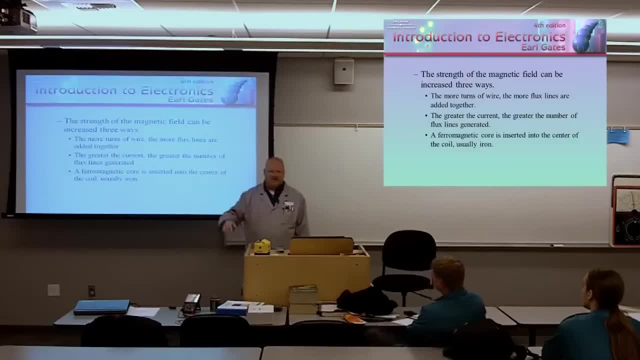 you're going to compromise that lacquer coating and that's the end of your coil. By the way, if any of you have ever smelt a coil, that's the end of the coil. By the time you smell it, it's over with. 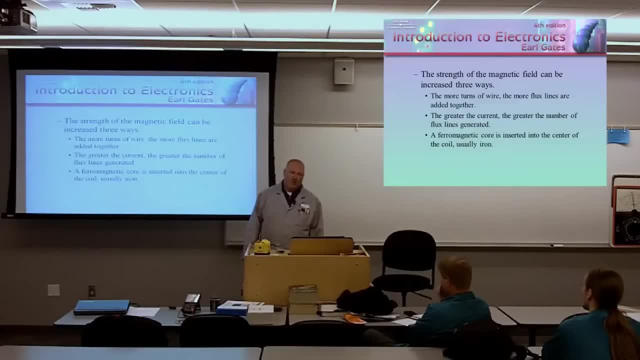 You've already compromised the integrity of it. It'll never work right again. Transformers, motors, coils, any of that stuff, Any of that stuff. If you smell it, if it gets that hot, forget it. Another way that we could increase the magnetic field: 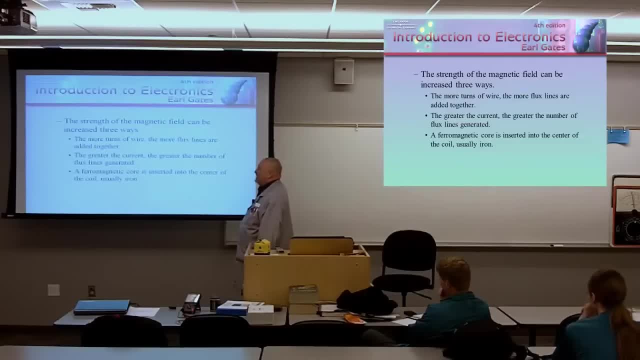 is, we could insert a ferromagnetic core into the center of the coil, usually iron. Iron has a high level of permeability. By putting it into the center of the coil and unwrapping the coil around it, it's going to enhance the magnetic characteristics. 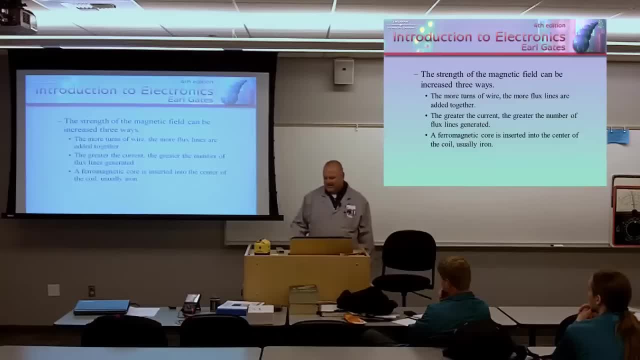 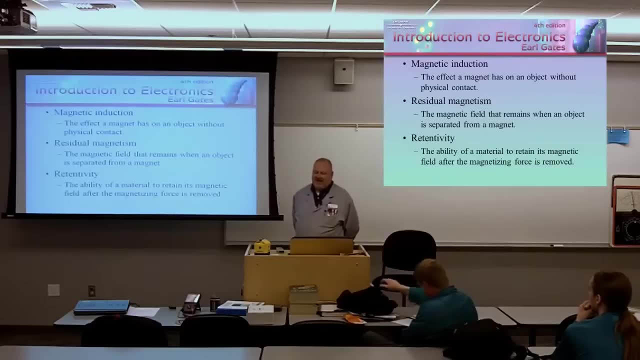 So by putting in a ferromagnetic core it's going to enhance the characteristics. Now, magnetic induction is the effect a magnet has on the coil, On an object without physical contact. The effect a magnet has on an object without physical contact. This is the cool thing. 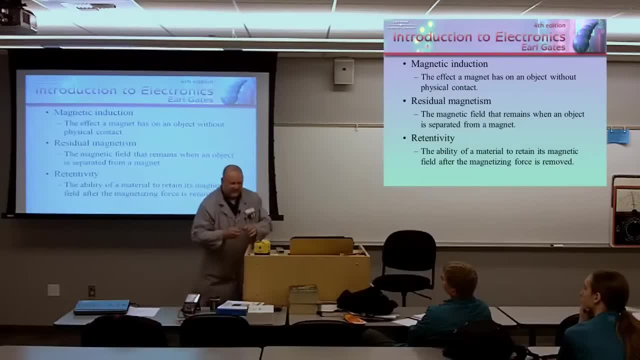 And I think some of you were playing around- even with these magnets here, right, And how they're not even touching, But yet it's having an effect on the other magnet, That's magnetic induction. Residual magnetism is the magnetic field. 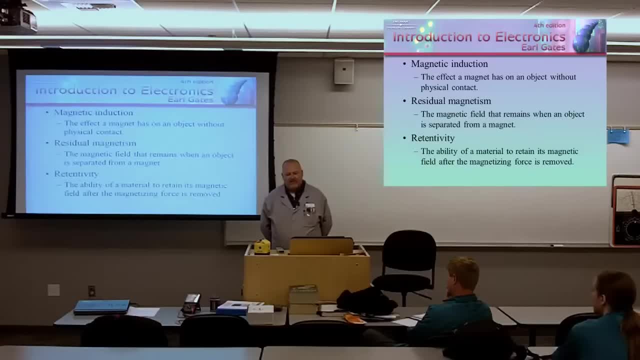 that remains when an object is separated from a magnet. We used to have literally a big problem with residual magnetism. This is something that I might. I don't know if any of you want to make a wild guess at this. here I'm thinking of a very, very large object. 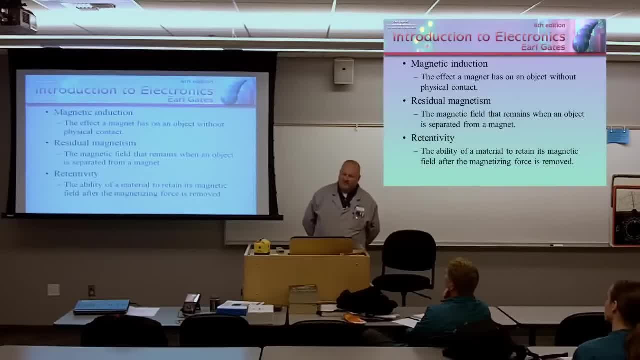 that developed magnetic properties And those magnetic properties needed to be removed, or it could compromise the position of this large steel cylindrical object. Submarine, Submarine, Big, big, big problem in submarining Because the submarine being made out of a ferromagnetic material. 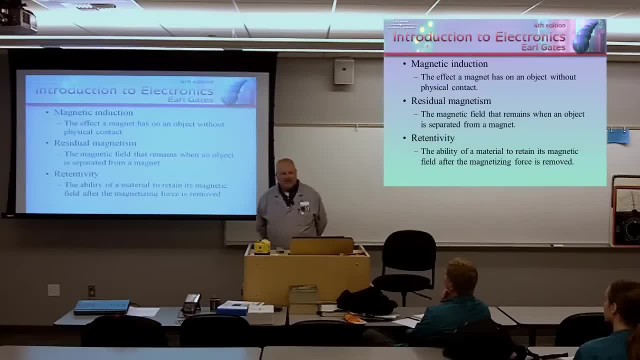 would pick up the Earth's magnetic field and gradually it would become magnetized. And the problem was there was equipment that would detect the magnetic anomaly. So there's no way of seeing a submarine, And some of our submarines are so quiet you would never even hear the submarine. 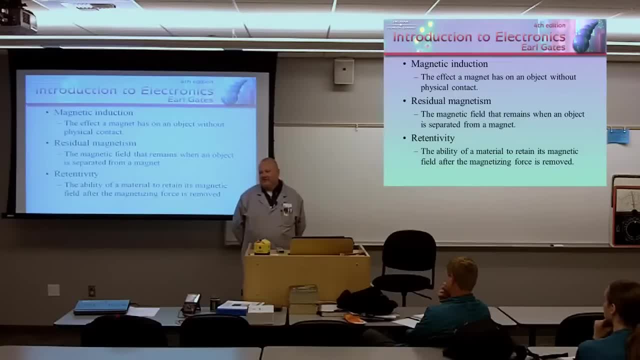 But if you're flying in an anti-submarine warfare aircraft and you pick up a magnetic anomaly, a large submerged contact that's creating a magnetic variation, chances are you found a submarine. So this is exactly what, If any of you ever go up around Whidbey Island. 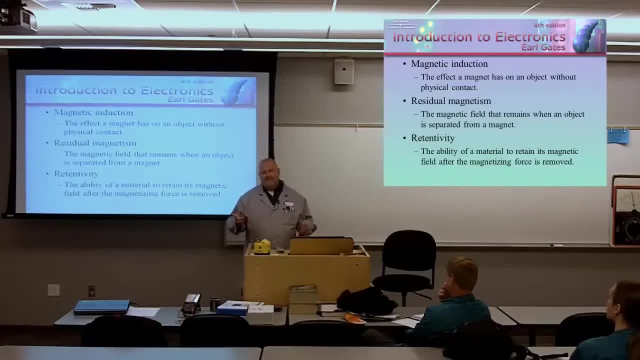 and you see those big four-engine turboprop aircraft P-3s. No, not those, Those are AWACS, Those are like airborne command posts. The P-3 Orion is a submarine hunter, And off the back of it. 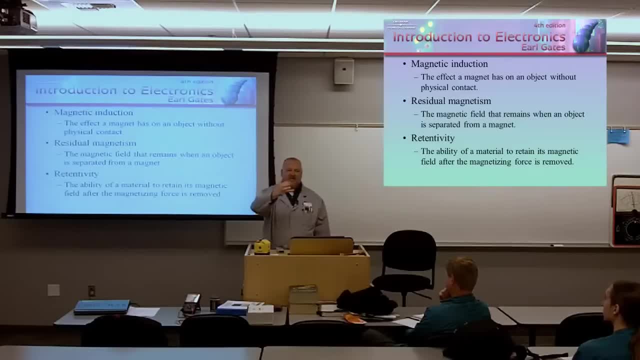 you'll see like this little thing that looks like a stinger, And that's what that is. It's called MADGEAR, Magnetic Anomaly Detection. So when you're flying around, typically what they? They just wouldn't be looking for a magnetic anomaly. What they would typically do is have a circular scan radar on radar. So when they stick up a periscope all of a sudden they get a blip, blip. If it's a good radar operator, that's all it takes. 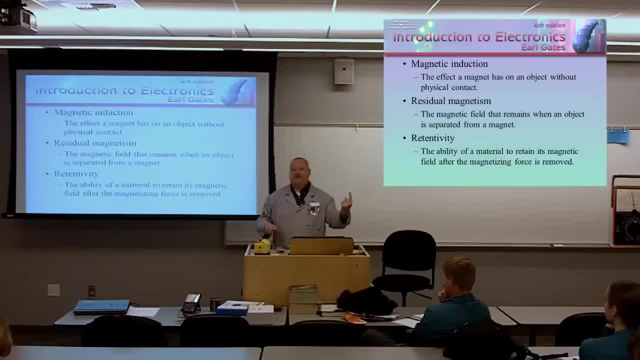 Two blips And then he'll shut the radar down. So what they'll do is they'll continue to fly and then he'll go to a sector scan. Okay, So, from a circular scan, blip, blip, then he'll shut it off. 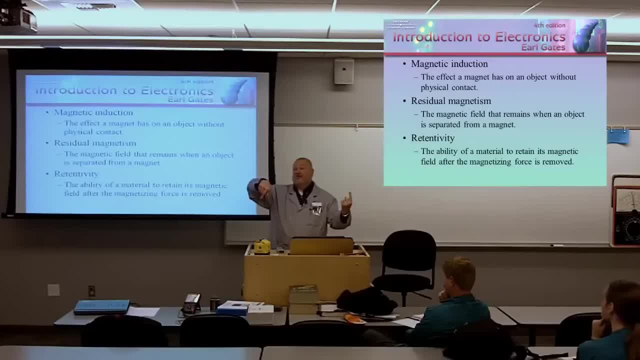 Then he'll get. He knows where he's looking for it, because he saw it on the radar screen. He'll go to a sector scan. Right, A sector scan is back and forth like this: So then off it's going to be. eh, eh, eh, eh. 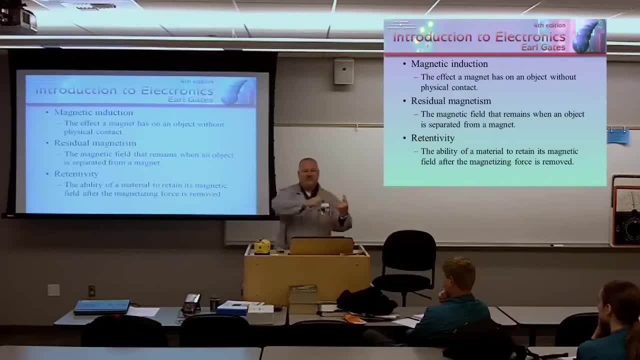 Then he'll shut the radar off And then he'll drive his cursor over to where he had that contact And hit enter. Autopilot will bring the airplane to that point in the ocean. And then the operator is looking at the NAD gear. 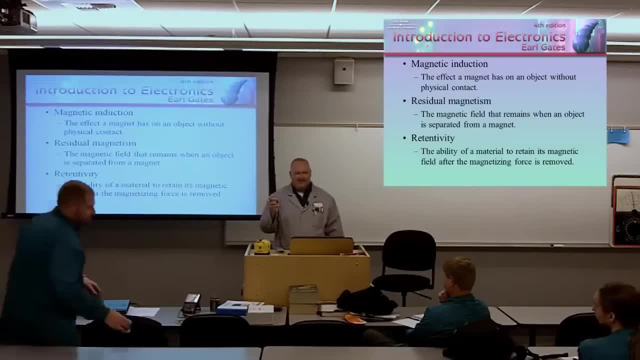 And then all of a sudden they start to get a magnetic anomaly. At that point they pop a flare out over the target. If you're at war, at that point the aircraft is going to go into a bank. start to open the bomb bay doors. 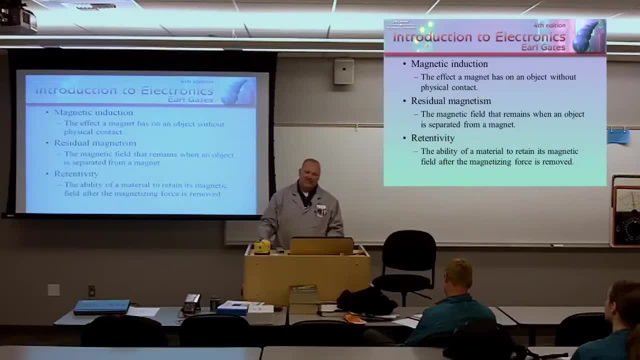 fly right over that point. put a torpedo in the water. It's a smart torpedo. It's going to find the target and blow it up. That's how you die in a submarine, in a combat situation. The only thing that we would know. 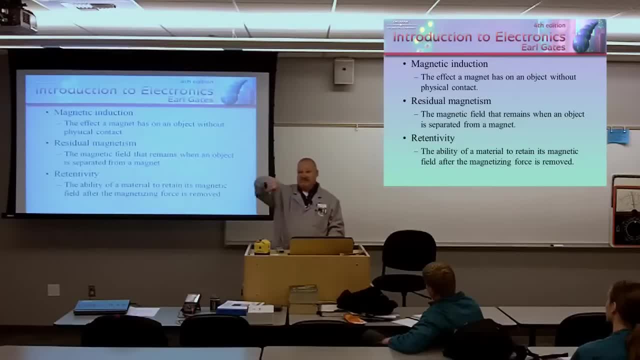 my job was to detect that, So I was good at picking up the blip, blip. But again, the good guys, the good operators: two sweeps, Two sweeps and they'd pick you up. The British came out with a radar that basically 400 miles away. 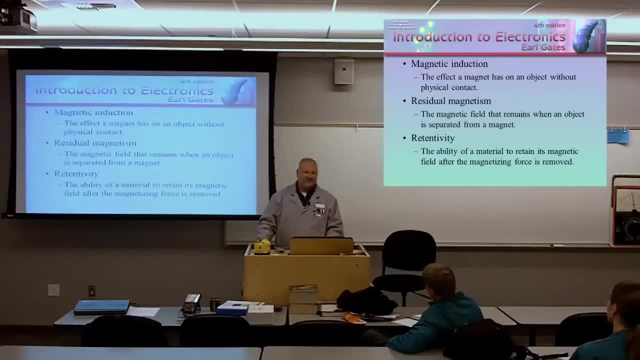 could spot a beer can floating in the water. So it's kind of like when I saw that technology come out, I'm like you know, I think it's time for me to move on to a different career Because if this turns into a shooting war, 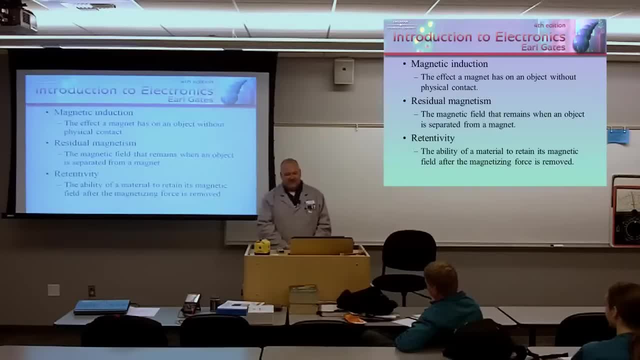 we're dead really quick, You know, really really quick. So to get rid of this residual magnetism, if any of you aren't into boating or fishing and you ever have the opportunity to get on Hood Canal, don't get too close to the submarine base. 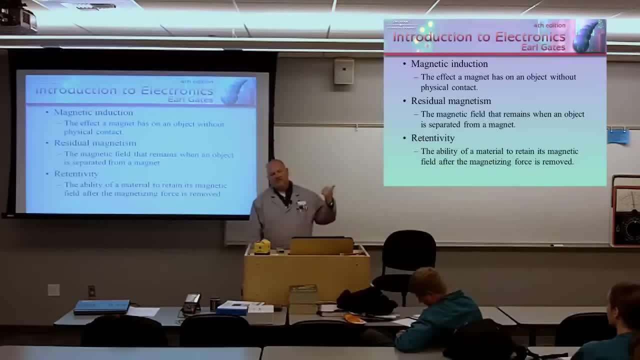 because they have gunboats and stuff and it's all restricted area. But over at the submarine base in Bangor they've got a giant pier. It's a degaussing pier And what they'll do is pull an entire Trident submarine into it. 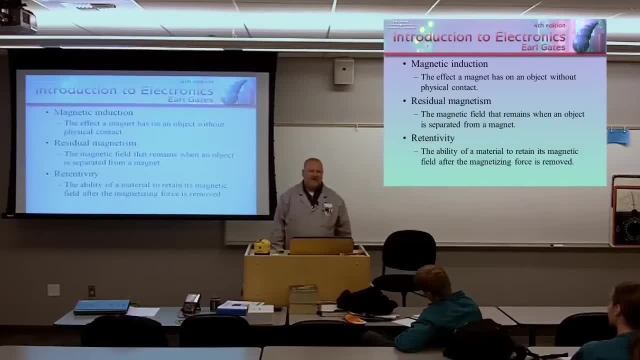 and pull off that magnetic field and get it back to just an unmagnetized piece of steel. But over time that magnetic field will build up again and it needs to be stripped off periodically or you're going to have a real profound magnetic signature. Correct. yeah, If I told you I'd have to kill you. A lot of. it depends where you operate to and what the magnetic field is. But you know, if you're doing a lot of stuff up north and there's some stronger magnetic variants. 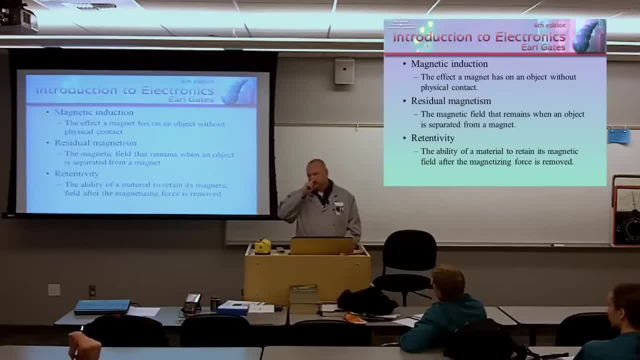 you're going to pick that up a lot quicker. Is that stuff really classified on how long it is here? Oh, yeah, Yeah, because then if you keep track of what boats go in, then it begins to paint an image, So somewhere you get magnetized. 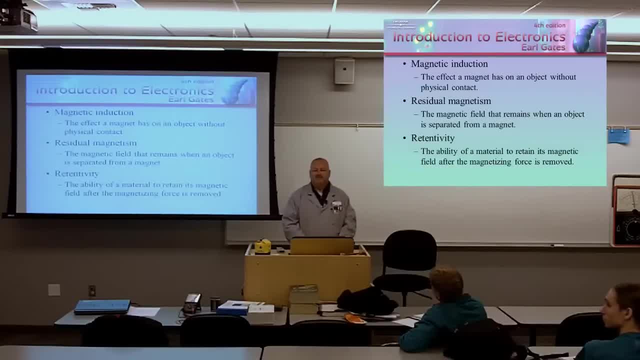 I mean you're not running into metal or another magnet. Earth's magnetic field, Yeah, Earth's magnetic, giant magnetic field. So theoretically, you're going to be able to see what the magnetic field looks like and what the magnetic field looks like. 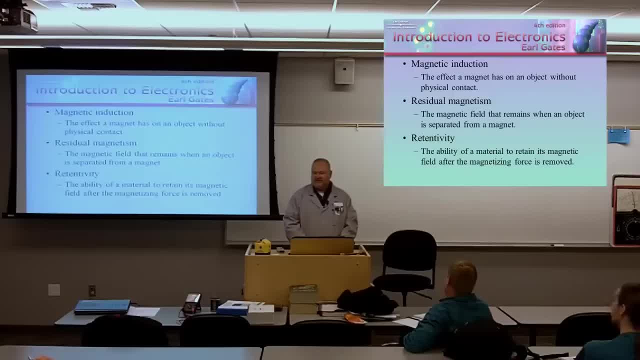 Yeah, Yeah. And then again we see this manifest itself, like with the Aurora Borealis. If any of you have ever seen the Aurora Borealis, I had the opportunity in February. I went up to Fairbanks and they say that if you're up there, between October and April for three nights. basically, you stand a 90% chance of seeing the Aurora Borealis. So we were up there for four. the flight up there, we saw them from the airplane The first two nights. I mean it was phenomenal. 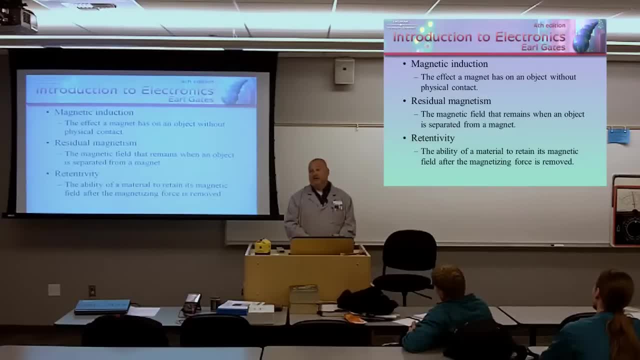 I mean we couldn't have planned it any better, because there was a huge solar flare. And that's exactly that Earth's magnetic field is attracting the charged particles. So as soon as they get the upper regions of the atmosphere, they ionize. 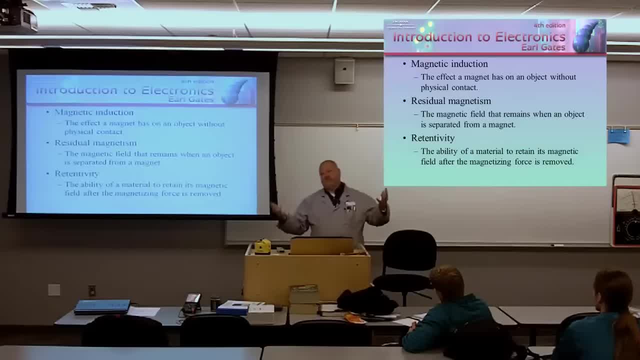 So literally it's like a neon light, except it's in the sky. So I should bring in some pictures and show you. I mean it was breathtaking, just phenomenal. You know, you're just standing there minus 23 degrees. 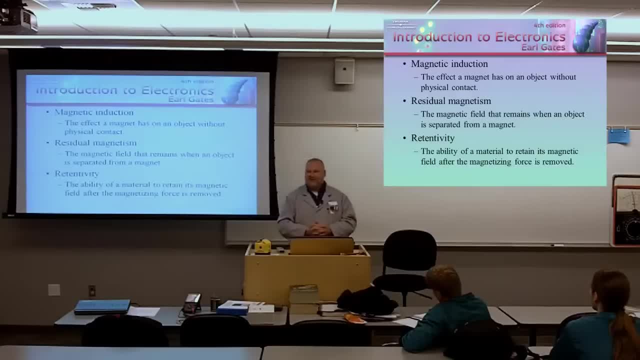 It warmed up The week prior. it was like minus 47 or whatever And I- seriously, even though I had gloves on and everything, I had to take off my gloves to manipulate the camera, I ended up burning the tips of my fingers. 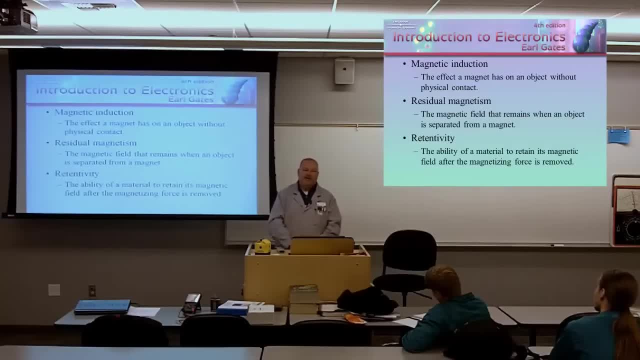 And it took about a week for me to get the feeling back. And it's very, very dangerous, but way cool. you know way cool to see this And you know people spend thousands and thousands of dollars to go up there and see that. 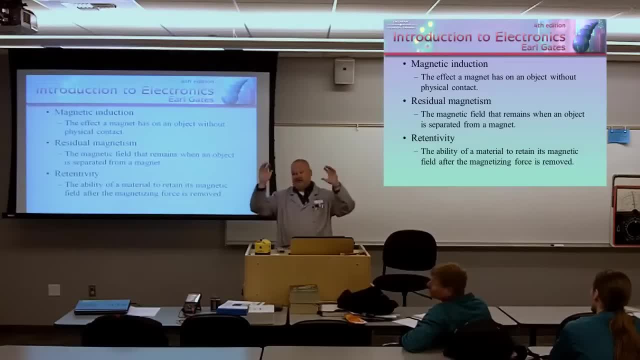 But it's the magnetic field that's actually attracting that near the poles. Retentivity is the ability of a material to retain its magnetic field after the magnetizing force is removed. So, unfortunately, a submarine hull has a high level of retentivity. 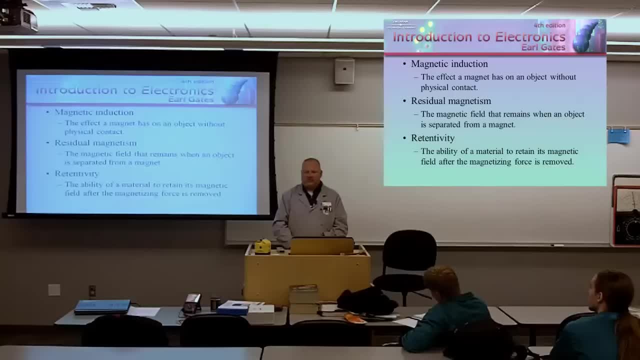 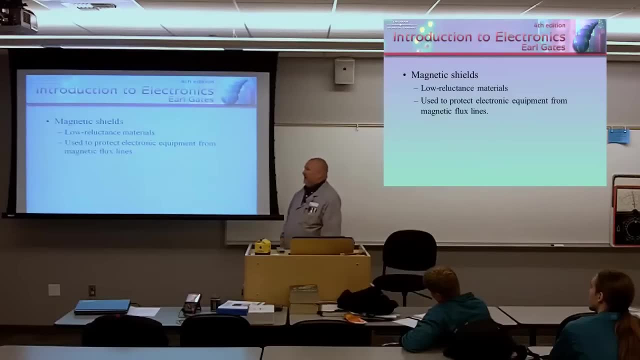 And that magnetic signature. you want to strip that off, because it's not desirable to have a submarine magnetized. Now magnetic shielding. now, magnetic shields are made of low reluctance materials. They're used to protect electronic equipment from magnetic flux lines. 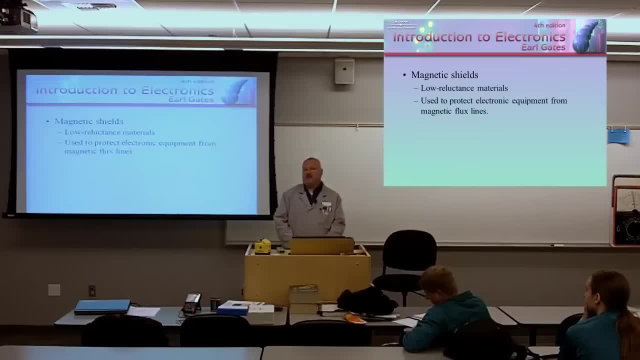 Okay. Sometimes we need to protect the equipment from these lines of flux because they could cause interference or even worse. Let me kind of back up for a second and see if you could connect the dots on this. We all understand that when we apply current to a conductor, 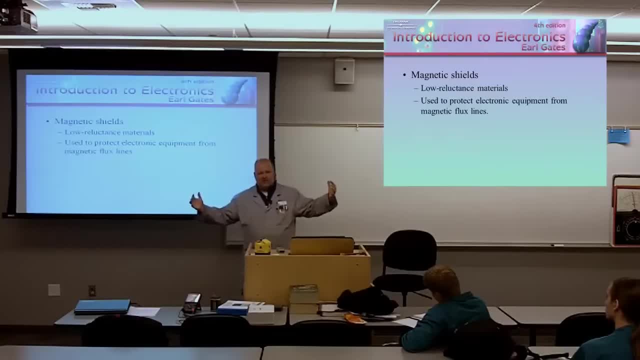 we create a magnetic field, right? So bear with me. If we have a magnetic field that happens to pass through a conductor, what do you think we're going to do? I'm going to create current, Yeah, so basically, if current creates a magnetic field, 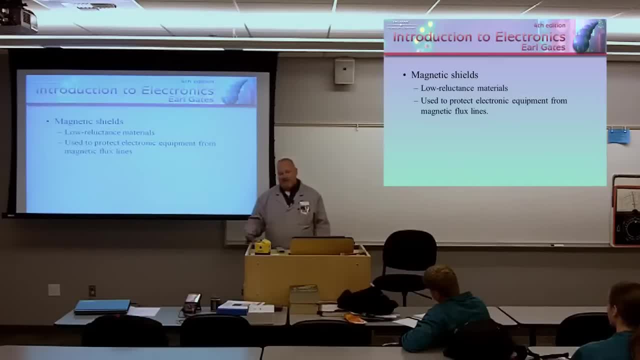 an electromagnetic field can create current. This is one of the things that they kind of figured out the hard way when we started lighting off nuclear weapons. One of the side effects of a nuclear weapon was an EMP, an electromagnetic pulse, And this electromagnetic pulse. 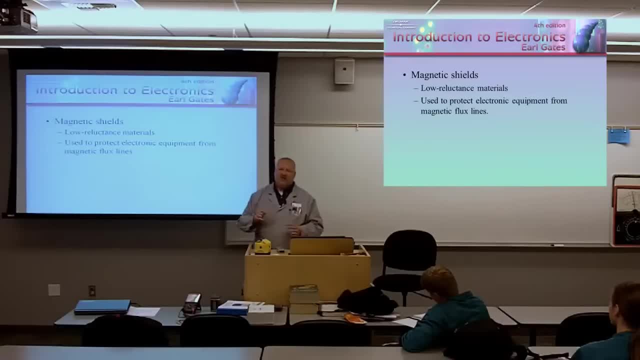 was a giant magnetic pulse that would go through the atmosphere and when it contacted, came in contact with a conductor, it induced a current where current didn't belong. Fry radios Back in the day, when they first started lighting off nukes- basically we all used tubes. 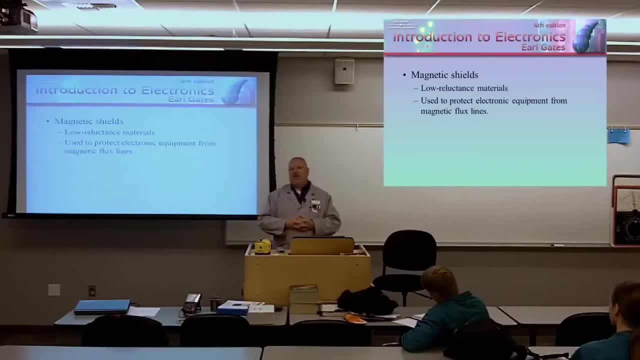 and tubes are high voltage devices and it would cause some interference and some wacky symptoms. and that was about it. With us going to microchips now and integrated circuits, that amount of current is going to fry. That's our technical term for the night. 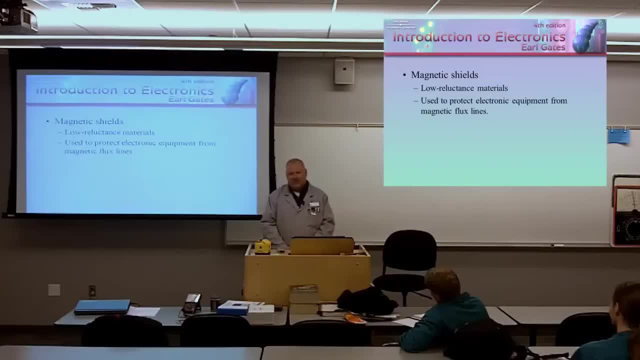 Fry these circuits because we're dealing with minute amounts of current to get the job done. So all of a sudden you have an EMP, you're going to fry stuff And, quite frankly, it really concerns me. I know enough about this where, basically, if you had, 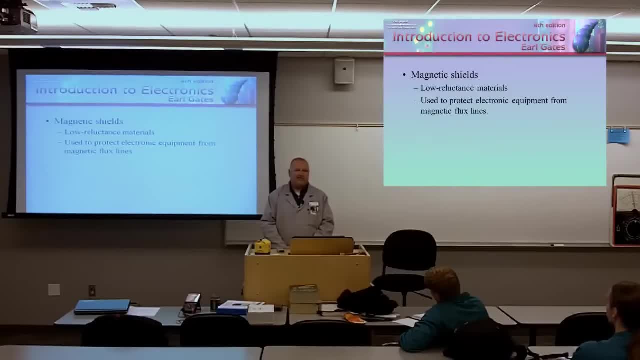 everybody's afraid of a dirty bomb and everything, and that's really bad news. but I tell you what one strategically placed high altitude nuke going off over the centuries in the central US is going to totally wipe us out and set us back into the stone age. 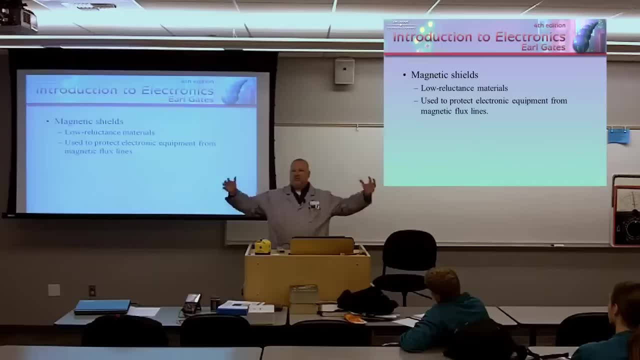 And it's the high altitude ones that really screw things up, because they're far reaching, because of the line of sight. And can you imagine a world? in a world that your ATM doesn't work, in a world that your grocery store, which uses a computer to order, 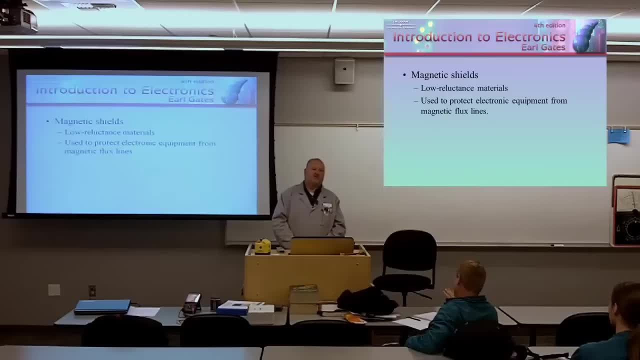 new food and supplies from the distribution center doesn't work. Your cell phones don't work. Your internet doesn't work. Your computers don't work. Your car computers don't work. The only people that are going to be driving around are the old people kicking old school diesel. 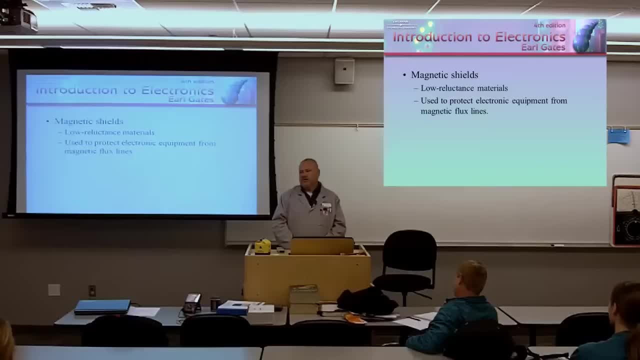 where you know compression and fuel and you've got the diesel engine running. Okay, Science fiction, No pure science. This is how it works. So these magnetic shields are actually used in some military applications for hardening the sites, because we know that this EMP. 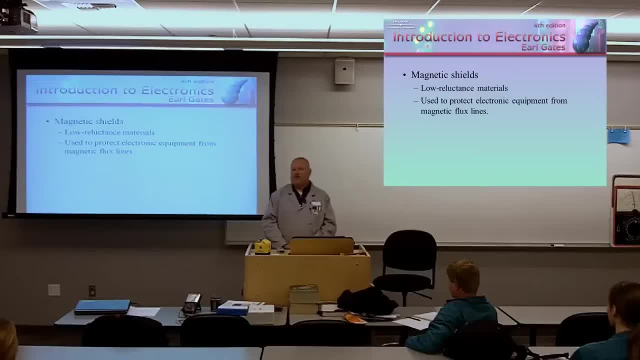 is going to cause problems. None of the consumer stuff that we use is hardened Air Force One- what the president flies around in, is hardened. Okay, They brought that down to Kirtland Air Force Base outside Albuquerque, New Mexico, and that's where they do this EMP testing. 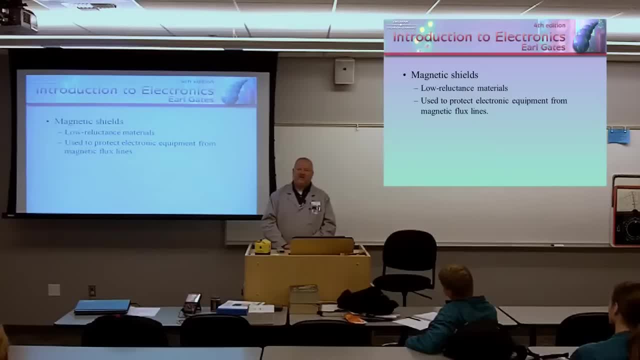 and basically prove what it's able to withstand. And again, that's all really highly classified information. The same thing with the autopilots, the you know. now it's all fly-by-wire technology, So this electromagnetic interference could cause big problems. 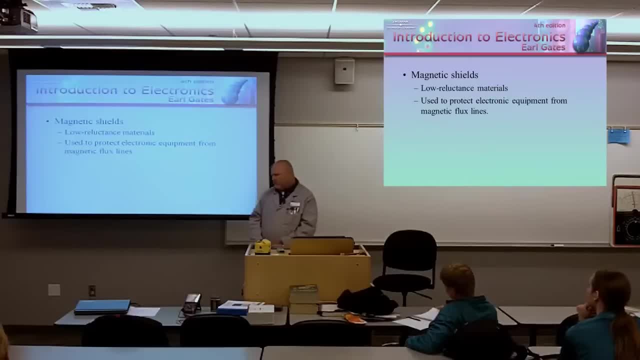 I don't know if any of you remember, years ago there was a problem with the Airbus. Well, there's always been a problem with Airbus, Just different problems as time progresses. But this was the problem with Airbus, was with the A320 aircraft. 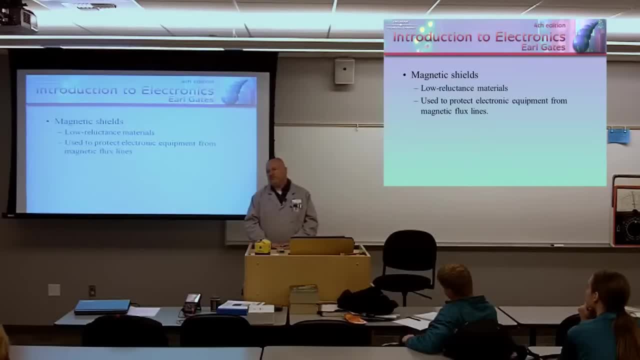 And the A320 was the first commercial aircraft to use what was called fly-by-wire technology And it's actually funny. I like messing with people that are flying on it. A lot of people don't realize that up in the country they don't realize that up in the cockpit. 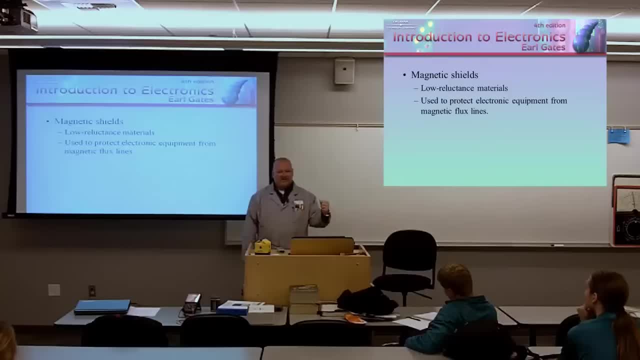 there's no control yoke like this on an A320.. They're flying with a joystick And you know the pilot's seat and he's got the instrument panel in front and right off to his left. here is a joystick. 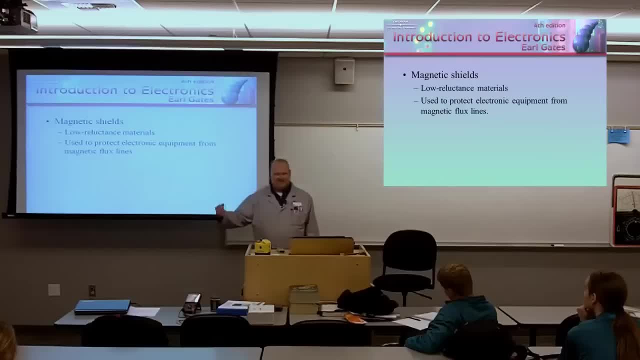 And that's how the pilot captain has got his on the left, the co-pilot's got his on the right. So there was an air show that they were doing a fly-by, And what happened is the airplane came died. 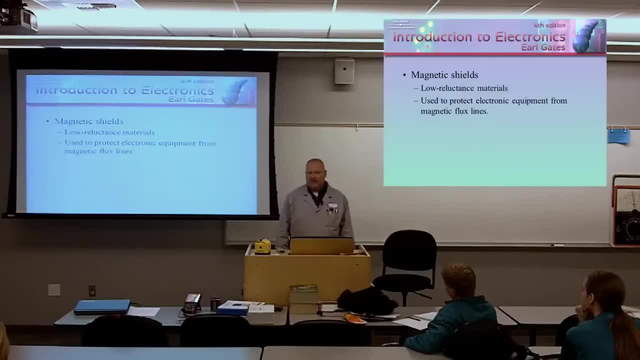 you know the symbolic low pass and then kept going and going and going right into the trees at the end of the runway And there was a huge fireball and explosion and a bunch of people got killed. But there were a bunch of people. 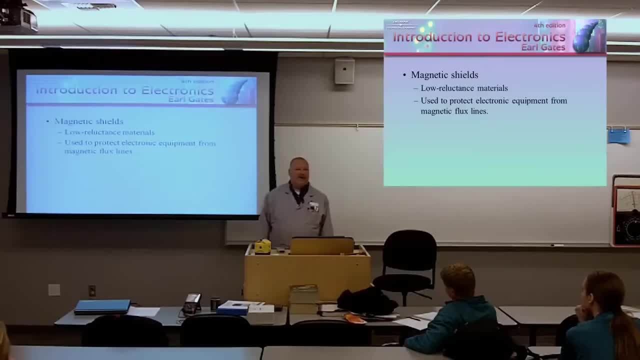 including the pilot that survived And he was like man. he said I don't know what happened. You know I was pulling up the whole time The aircraft was not responding. So in basically the investigation they determined at this big air show in Europe. 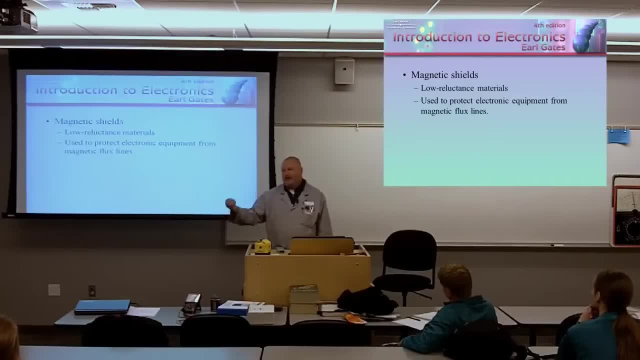 there were military aircraft that were present and they had their high-energy weapons fire control radars turned on And they think that high energy got into the computers and basically put current where current and it got confused. So he's pulling up on the stick, you know. 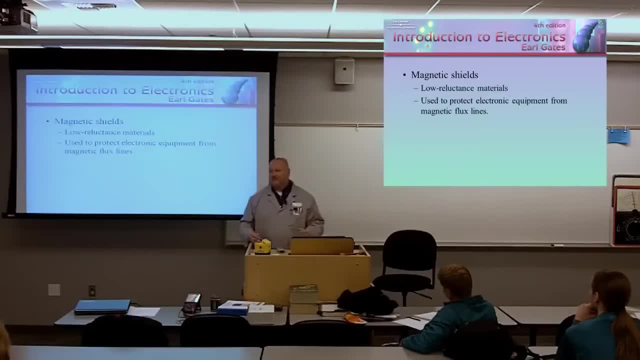 to pull up and you know dip the wing and you know the maneuver. At least I know the maneuver, It's a classic maneuver. Instead, he's pulling up and just right into the freaking trees. You look that up on YouTube: A320 crash. 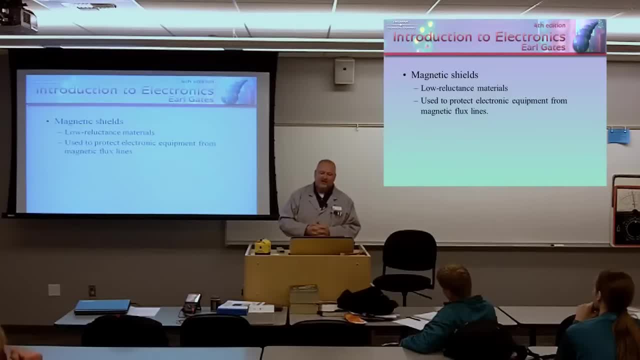 and you know they very well documented crash. They added a lot more magnetic shielding to it. Boeing's first airplane to dabble with fly-by-wire was the 777. And it was kind of a gamble. Military aircraft have used it for years. 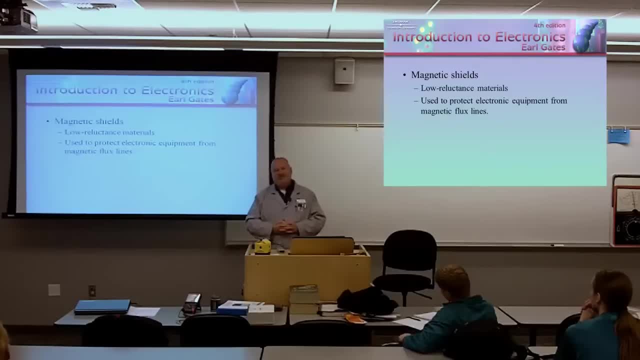 but military aircraft are kind of a different animal. You know, if you got a problem in a military aircraft, you know: eject, eject, eject, pow, you punch out, And you know you live to fight another day In a commercial airliner. 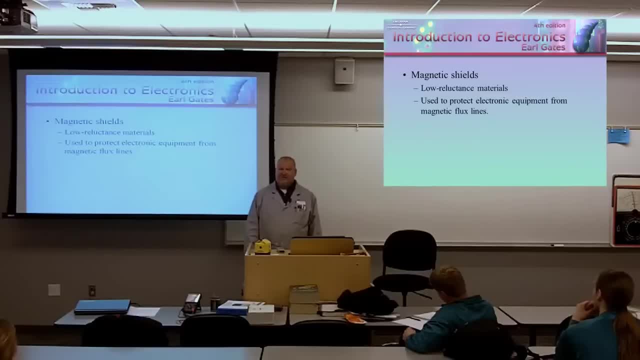 you got hundreds of people behind you. There's no eject, eject, eject. It's like you got to ride it out and you fix the problem. So Boeing's first airplane with fly-by-wire technology was the 777.. Was the 777.. 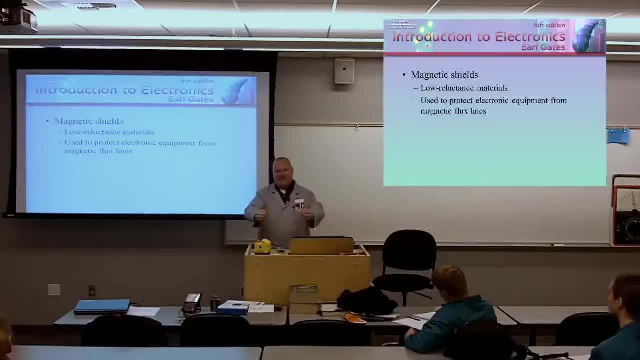 And, believe it or not, it was kind of funny because Boeing opted for standard controls, not the joystick. They could have done the joystick because basically the standard controls are controlling the equivalent of a joystick, But it makes a pilot feel like they're kicking it old school. 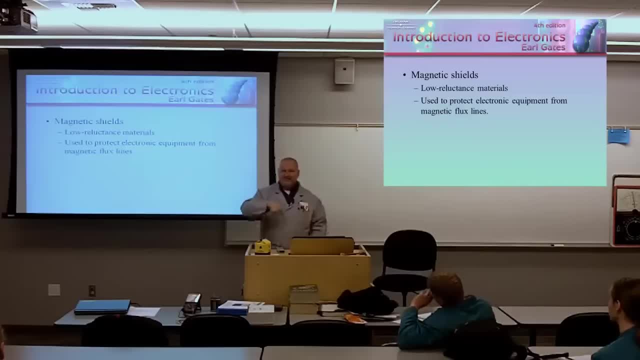 And they're not kicking it old school. They're still putting in inputs that create small currents to feed a computer and then the computer controls the control surfaces of the aircraft. So in a lot of cases like that, suffice to say you reckon Boeing's got some really good magnetic shielding. on their flight control systems? fly-by-wire? Absolutely, It's to prevent current from being where current doesn't belong, And any time there is a magnetic field, you run the risk of putting current where current doesn't belong. So what? like a lightning strike? Absolutely, Absolutely. And that was actually one of the other problems too that Boeing had. You know, every commercial airliner statistically gets struck by lightning once a year. So next time you go on your dream vacation, or whatever, you got on that airplane. 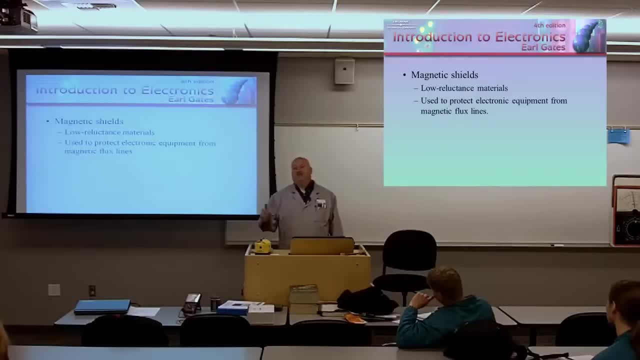 suffice to say that airplane was probably struck by lightning in the past year, As Boeing went to, And for most aircraft it's not that big of a deal, because what happens is when an aircraft is struck by lightning, it follows what's called skin effect. 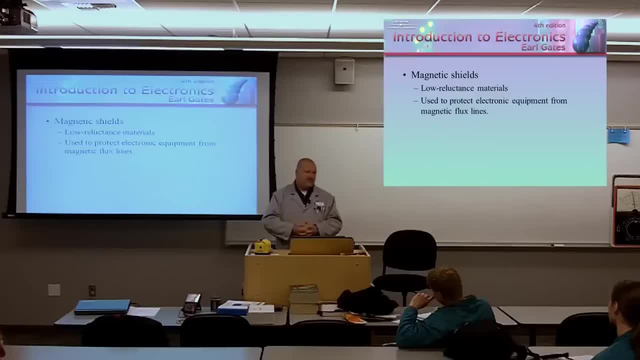 and that current passes over the skin of the aircraft. I mean it could scare the dickens out of you if you're on board. It's going to be a big, you know, and in some cases fireball coming through the cabin. 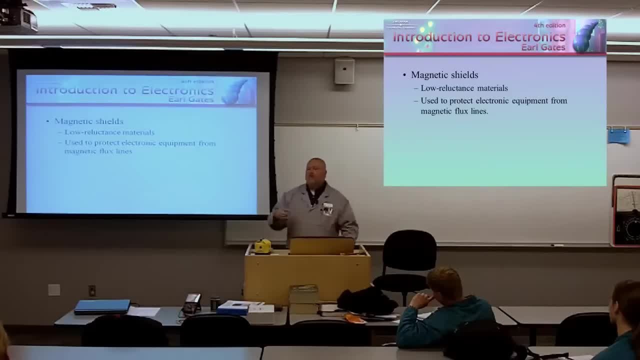 and you know it's going to scare the dickens out of you, but it's not going to bring the airplane down. One of the manufacturing trends now with aircraft, though, is not to build airplanes out of aluminum. It's to build it out of composites. 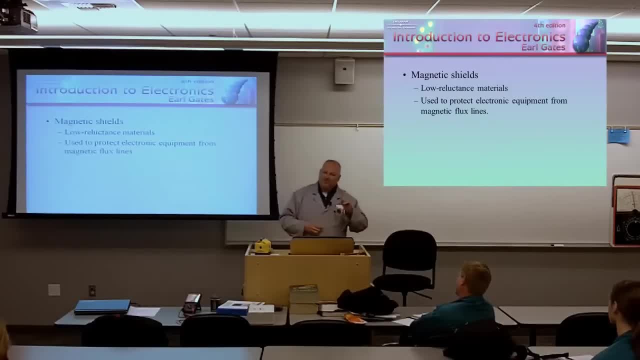 Okay, If you're using carbon. they're not always using carbon, They're just using various composites. So one of the things that they're doing on aircraft now, especially control surfaces, flaps, ailerons that control the roll of the aircraft and such. 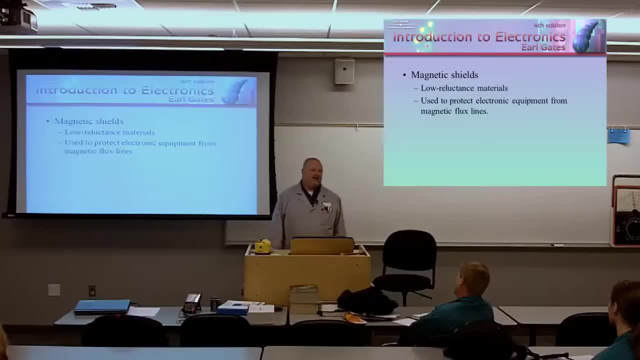 these would typically be made out of composites. So you get struck by lightning. it's quite simple: The lightning. The lightning gets in, there has nowhere to go. it blows the control surface apart. Not good if you're in the airplane, okay. 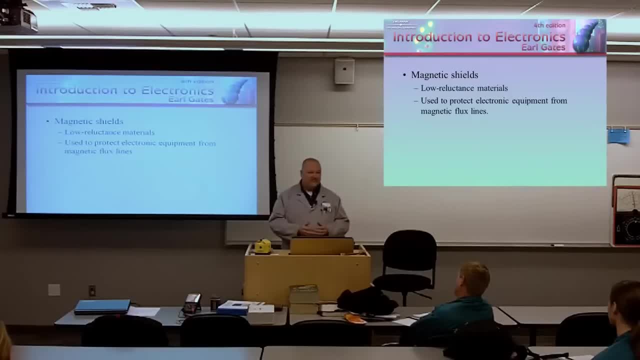 Because now you're going to lose control, because you don't have the ability to control the aircraft anymore. So what Boeing actually started doing is by basically putting in a conductive layer into the composites so that will allow current from a lightning strike a place to dissipate. 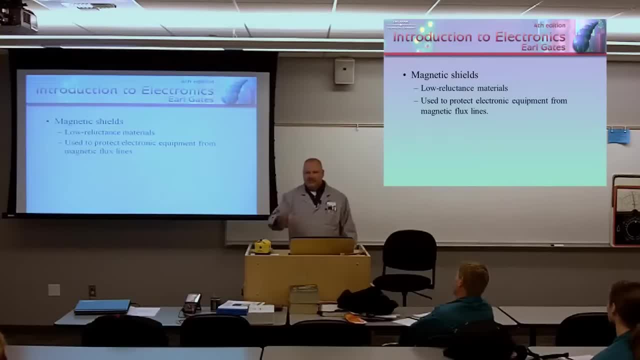 So kind of get rid of the aluminum only to put a conductor back in to the composite. It's still highly efficient and lighter and stronger and everything else I guess lighter and stronger, I don't know. When they fail, they fail big. 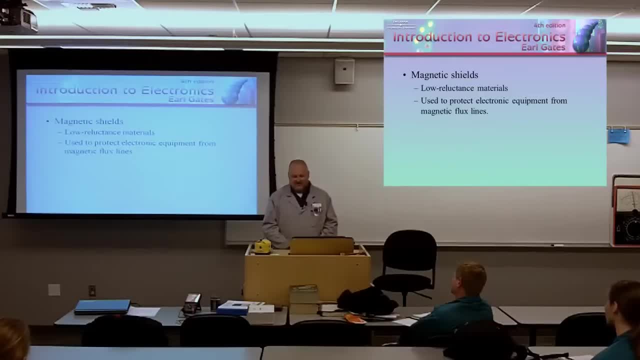 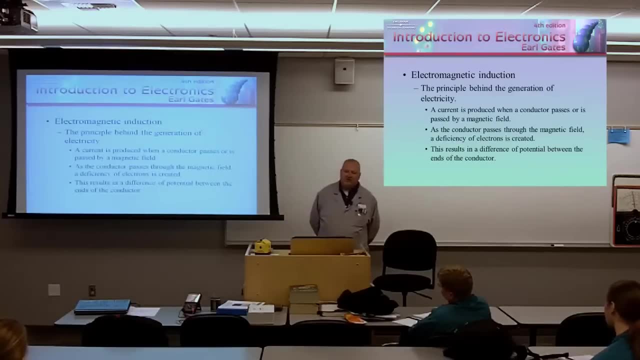 But I guess aluminum. When aluminum fails, it fails big too. So I don't know. I like kicking it old school. Electromagnetic induction is the principle behind the generation of electricity And I think all of you know where I'm going with this. 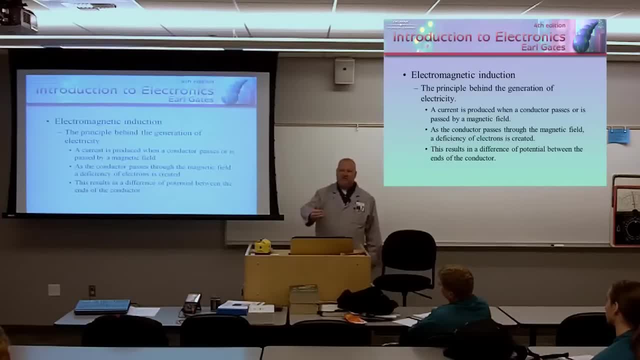 because we just talked about EMP. A magnetic field passing through a conductor is going to induce current. Current is produced when a conductor passes or is passed by a magnetic field. As the conductor passes through the magnetic field, a deficiency of electrons is going to be created. 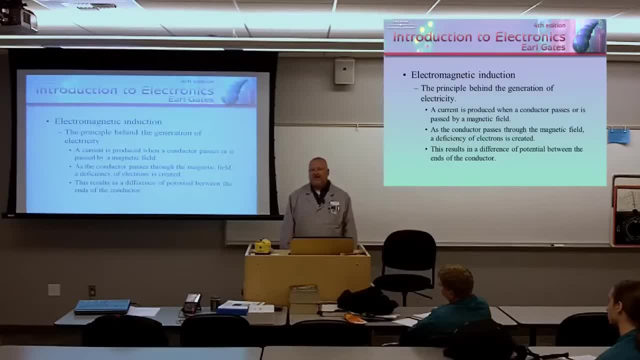 This results in a difference of potential between the ends of the conductor. So again, if you've got a long piece of wire, you pass a magnetic field through it. you're going to induce current, Many years ago I think, the space shuttle. 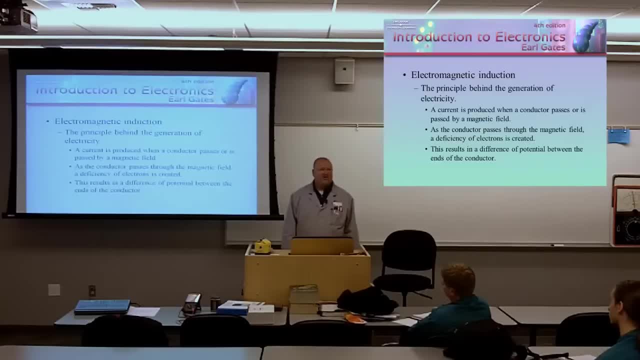 conducted an experiment like that, and literally what they did is they trailed a long wire loop And what their goal was to try to drag it through the Earth's magnetic field and see if they could generate current from that. Basically, they vaporized the wire. 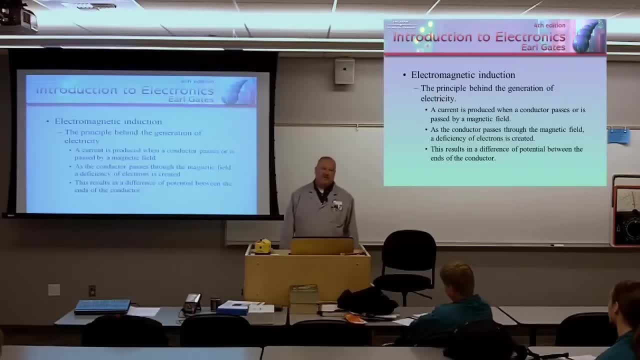 That's how much current they generated from the Earth's magnetic field. So if there was a way of harnessing the Earth's magnetic field as a generator, our energy woes would be over. But I don't think there's an adequate way of harnessing it at this point. 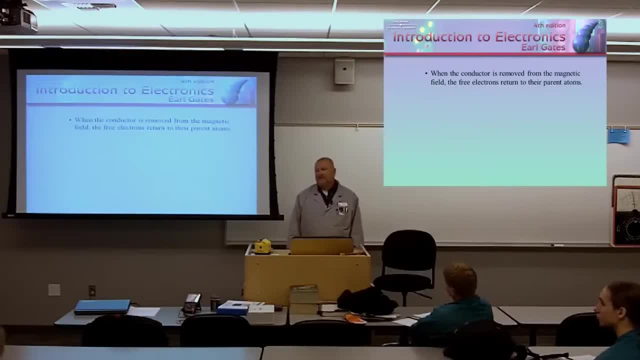 Basically trailed a wire and pulled it through the Earth's magnetic field and vaporized the wire. So when the conductor is removed from the magnetic field, the free electrons return to their parent atoms. So what we're doing is we're getting electrons to move in a conductor. 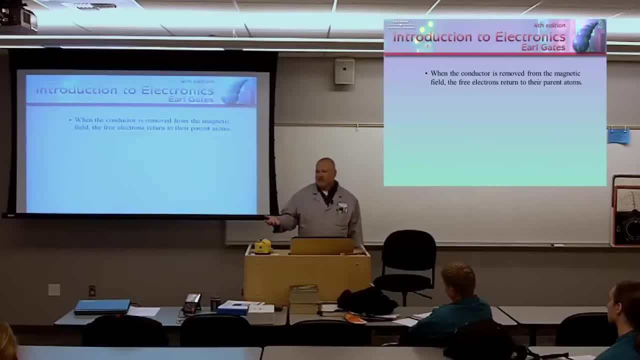 By getting electrons to move in a conductor. we call that current, Call that current. That's the current Faraday's Law. The induced voltage in a conductor is directly proportional to the rate at which the conductor cuts the magnetic lines of force. 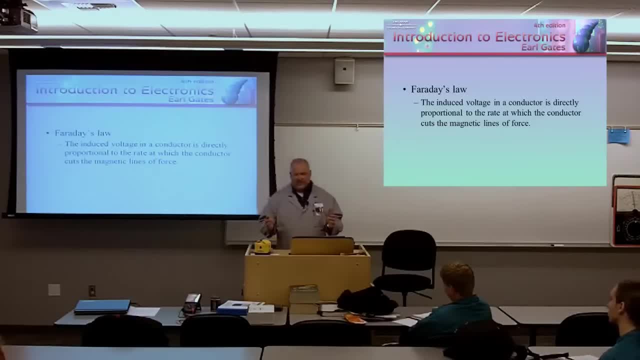 I'm going to make this real simple for you to understand. Faraday's Law here. Envision up here that I have a big north pole, Big magnet sitting here, Boom, Big Giant, And here I have a big south pole. You all agree that I've got lines of flux that are going. 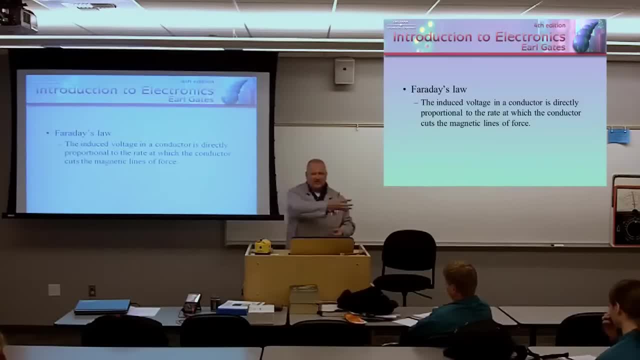 from the north pole to the south pole And all that stuff that I talked about earlier. the straightest line, the shortest distance, right. So in between here I'm going to have a strong magnetic field. if I had a giant magnet right here. 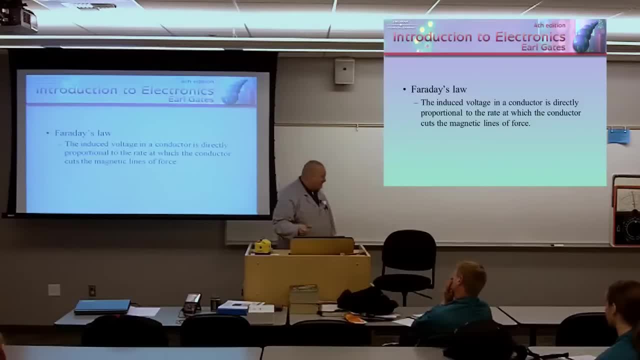 Do you agree with that? Faraday's Law says that if I my conductor, if I've got a conductor, this is a conductor. When I say conductor, I'm not talking just a piece of wire, I'm talking about a piece of wire that has a loop in it. 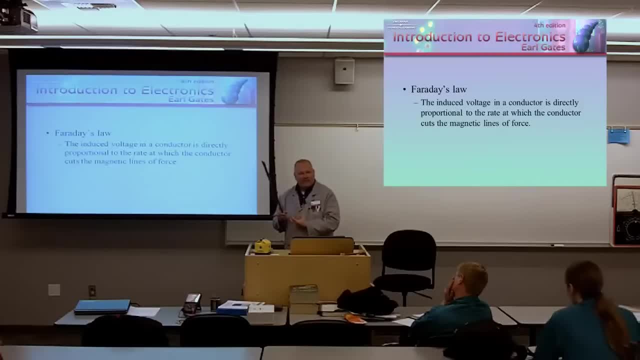 So the current's got to have somewhere to go And it has to have a load right. If I get this and I move it perpendicular to the lines of flux, I'm going to generate my maximum amount of current, Because I'm doing what. 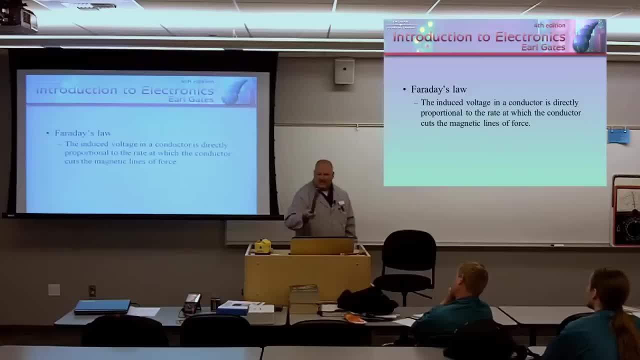 I'm cutting the lines of flux. If I get the conductor and I move it parallel to the lines of flux, nothing's going to happen. I mean nothing is going to happen Because the lines of flux are going north pole to south pole. 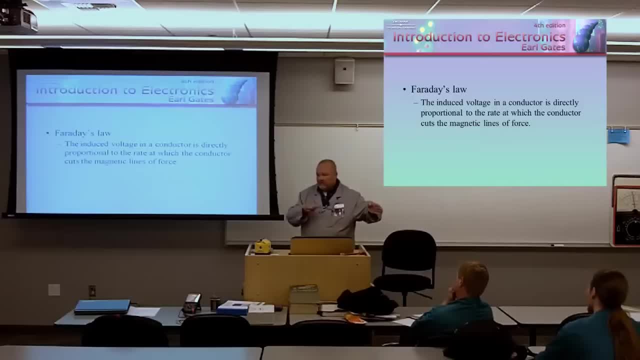 So me, with the conductor moving it like this all day long, nothing's going to happen. All of a sudden, I move it like this. I'm moving it right through those lines of flux, Perpendicular, So I'm going to get maximum effect. 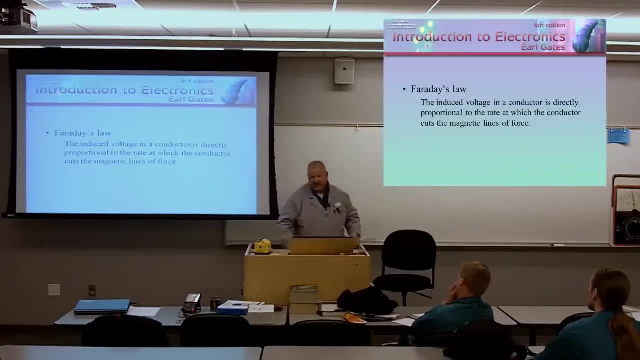 of cutting those lines of flux. So that's, in essence, Faraday's Law. It's me cutting those lines of flux, So I'm still going to have a strong effect by simply cutting it, Now if I'm doing it at a 45 degree angle. 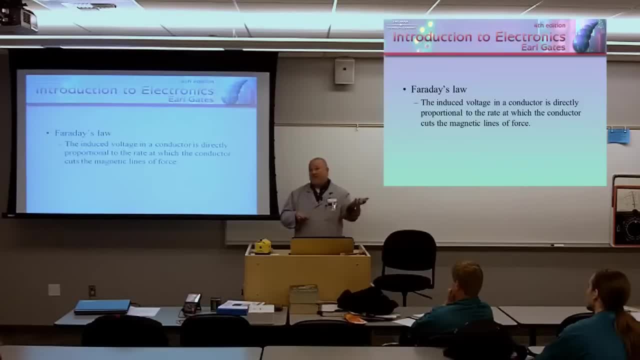 what am I going to be doing? I'm really half effective. It's not this and it's not this. I'm going to cut it in half at 45 degrees- Faraday's Law, But I'm cutting it at a 45 degree angle. 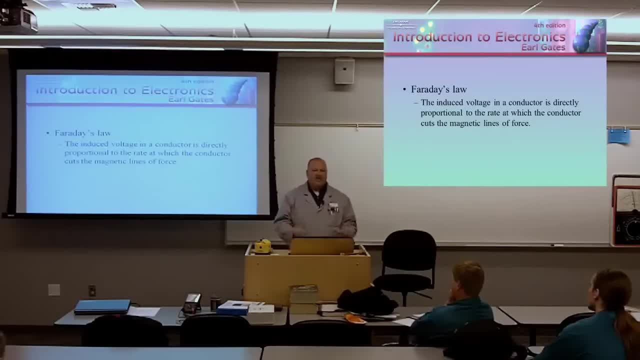 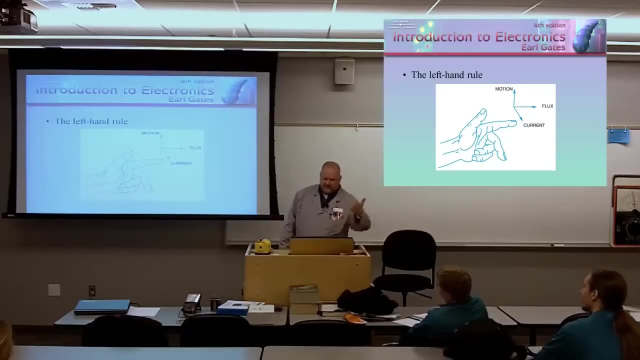 so I'm not cutting the maximum lines of flux By cutting it at 90, I'm getting the maximum out of it. So that's Faraday's Law. This here. don't try this in your car on the way home. Somebody will think you're doing gang signs or something. 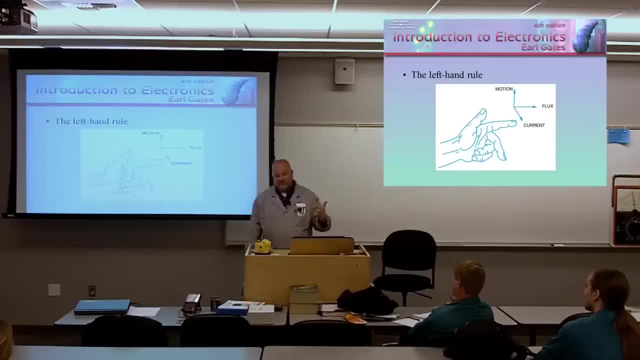 Yo, I'm an electronics student. Yo, This is called the left hand rule, And the way that this thing works is that your finger points in the direction of flux. Which way does flux go? Which way does flux go? From where to where? 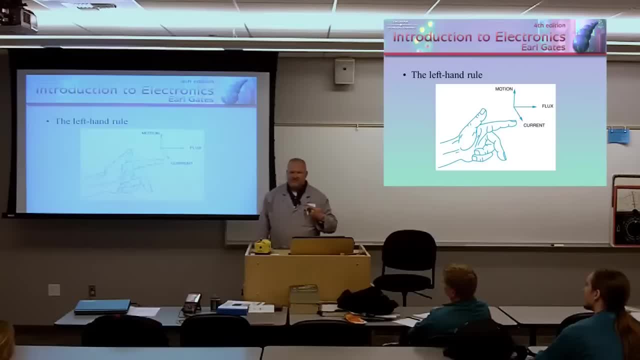 Positive to negative, East to west, North to south. I said that earlier. right Flux goes north to south, North pole, south pole. So this means north to south. That's the direction that the flux is pointing in Make sense. 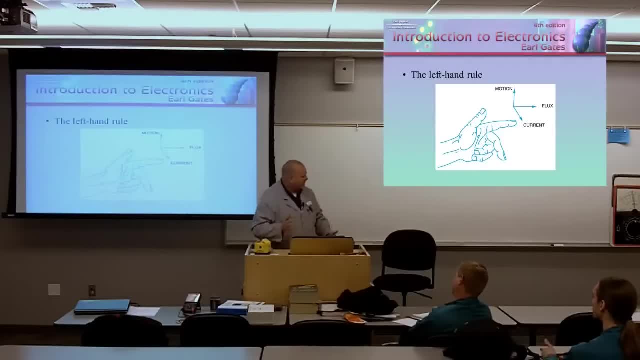 My thumb is going to point in the direction of motion, So, as an example, let's go back to me wielding the yardstick. here Is this the yard? This is the yardstick: 36 inches. That's one of the reasons that I'm real happy that we're not on the metric system. 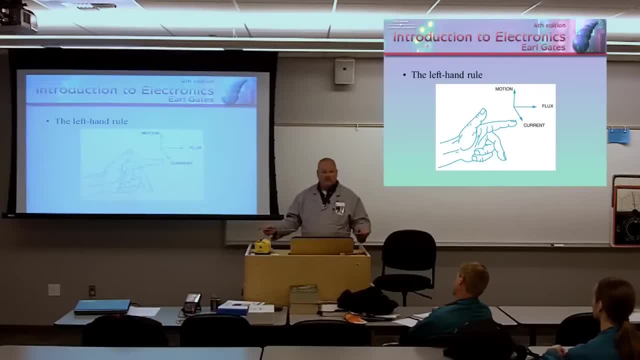 or we weren't when I grew up, Because, having attended a Catholic church school for a period of time, the nuns. if the nuns had been equipped with meter sticks as opposed to yardsticks, there's a good chance I wouldn't be. 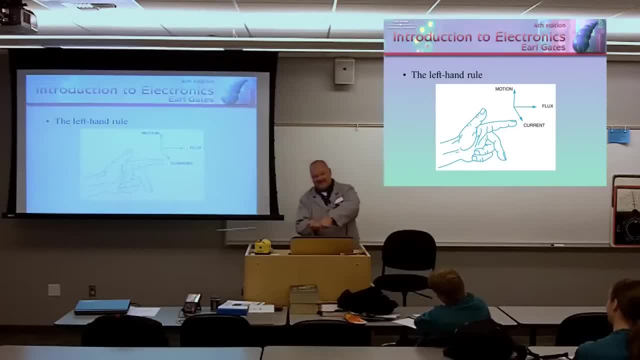 here with you today, Because that additional three inches would have been just enough, probably, for them to connect. Yes, I was beaten by the nuns, Anyway. so I've got a north pole here, a south pole here. Remember that north here, south here. 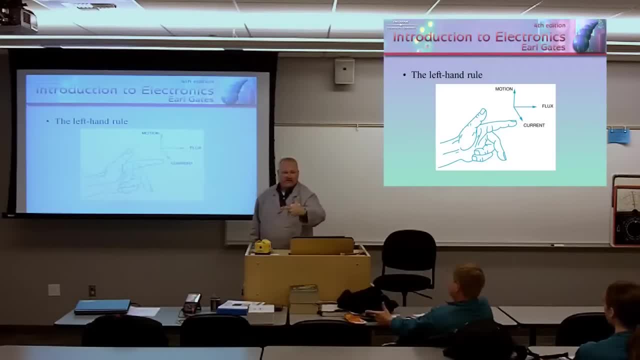 So that means the lines of flux are going which way? North to south. So I've got to do what Make sense. I'm going in this direction. So with the left hand rule, Now my thumb is going to point in the direction of motion. 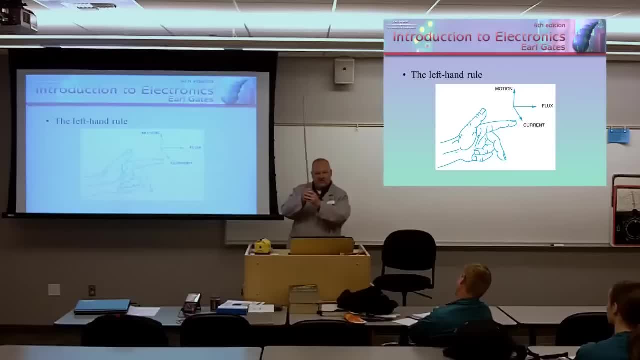 So this means the conductor is moving down through this scenario, And if that's the case, if that's the case, my middle finger is pointing towards me. Which way does current flow? This is not a trick question, folks. Negative to positive. 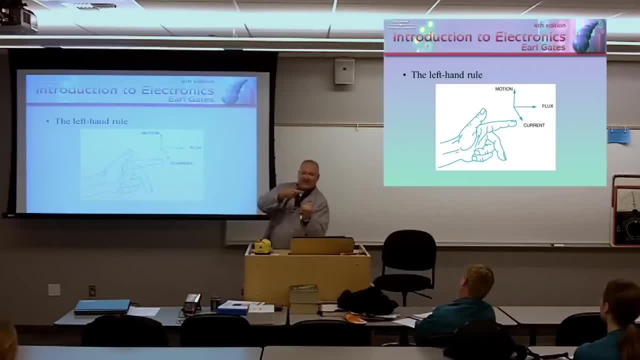 So that means I am positive with respect to my finger, negative to positive current flow towards me. To make it easier, let's make this the north pole, let's make this the south pole. Let's move our conductor. let's move our conductor down. 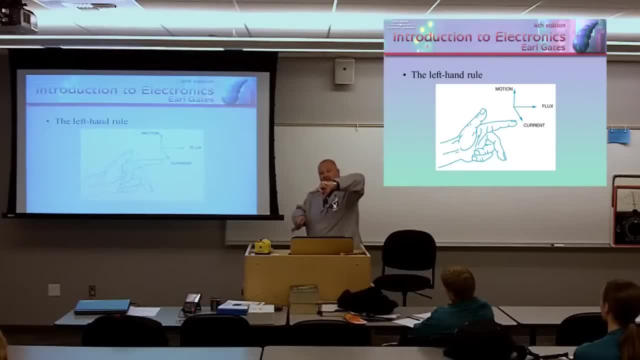 By moving the conductor down. current now is going to be flowing away from me. Negative to positive Make sense. So again, will you ever use this in industry? I doubt it, But this is a way of determining which direction we're going to. 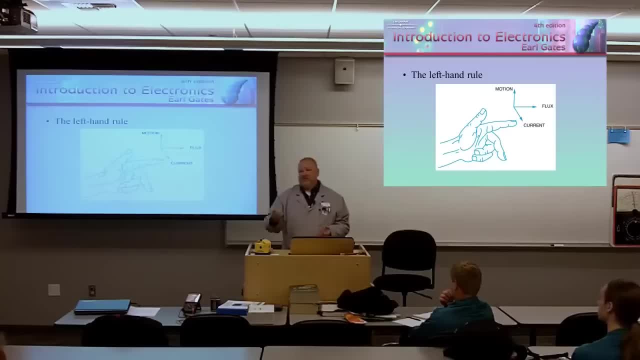 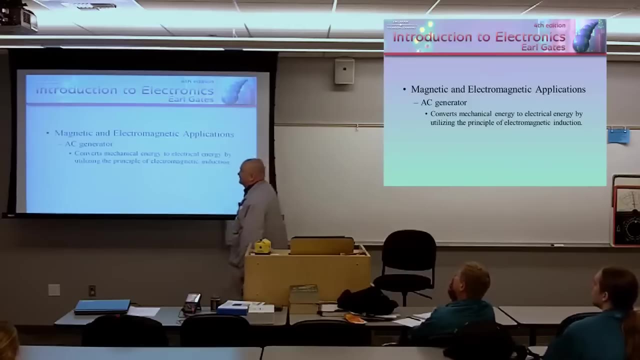 induce current in a generator based on positive motion. Now magnetic and electromagnetic applications- Probably the biggest and most important is the AC generator. AC generator converts mechanical energy to electrical energy by utilizing the principle of electromagnetic induction, And this is the most popular way of producing electricity. 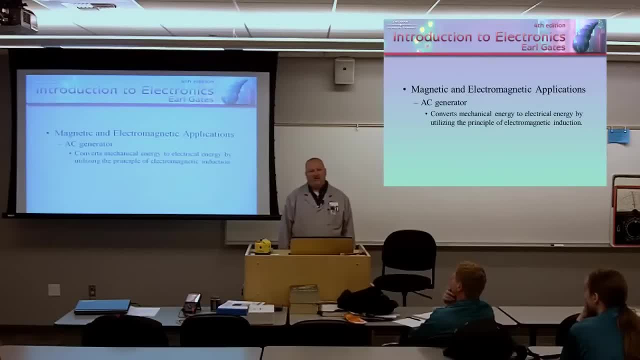 Now, whether we turn this AC generator, we're going to turn it by the shaft Right. Whether we turn that shaft from steam in a turbine that's generated from coal, oil, nuclear, hydroelectric, it's irrelevant. The key is that we're turning the shaft. 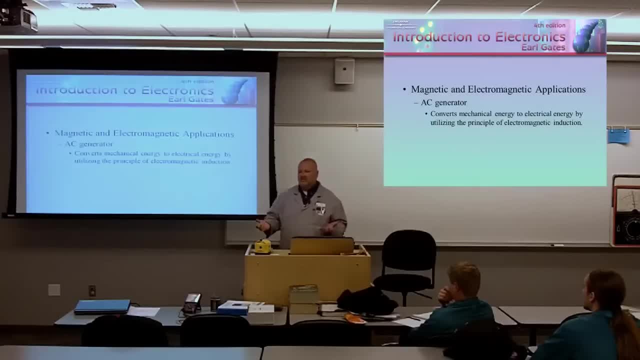 And turning the shaft, we turn the generator. That's what produces the electricity. Now, if we take that another step, are there means that are more efficient than others? Are there means that are more ecologically minded than others? Are there, you know? 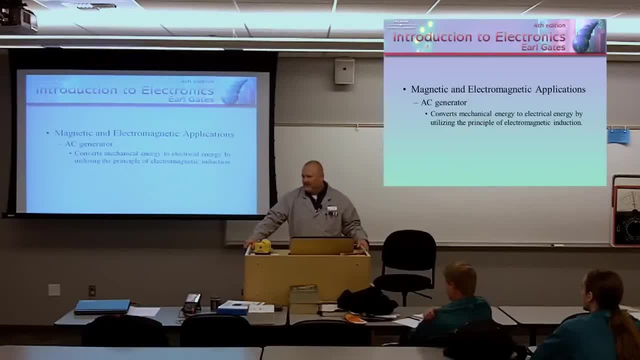 what we watched last week in our program meeting on Wednesday. I mean, even that dude, you know, who was pretty much a tree-hugging kind of guy saying hey, I've rethought nuclear, You know, And although nuclear is dangerous and it's something we need, 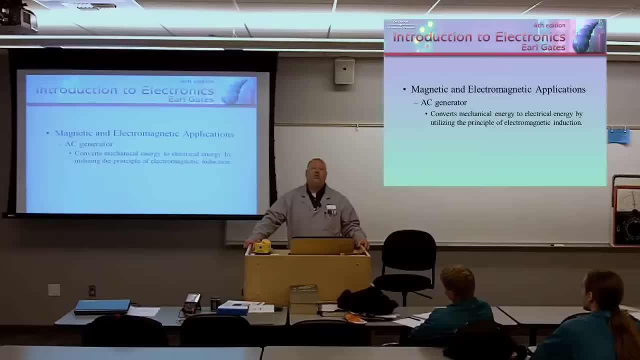 to be aware of. you know, polluting the environment with coal is worse. So things for us to think about, But the key here is, by turning that shaft, we generate AC electricity with an AC generator. This is how it works. This is how 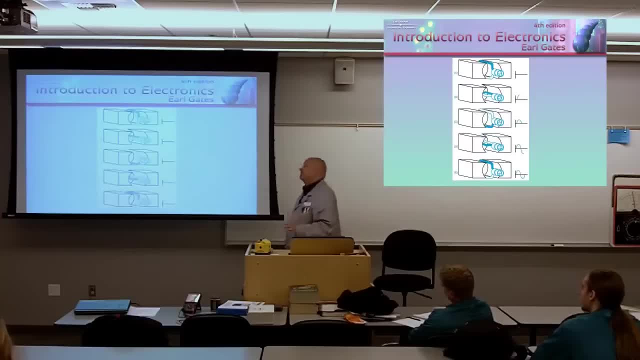 an AC generator works, And the thing that I want to point out to you here is that these are the magnets, And these magnets could be permanent or they could be electromagnets. They could be permanent or they could be electromagnets. As a matter of fact, this is: 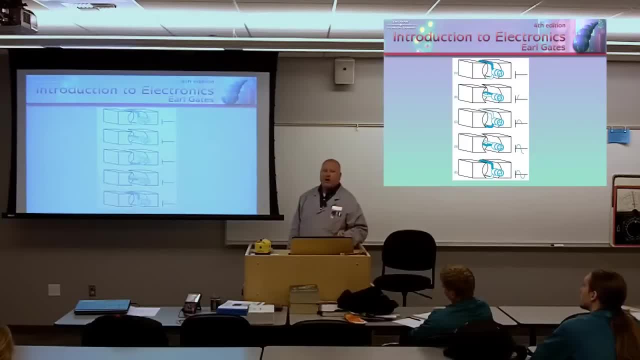 exactly what is taking place in your alternator in your car. Okay, In your alternator in your car, are those permanent magnets or are they electromagnets? Does anybody know Alternator in your car which produces voltage for us? It's a generator, Are they? 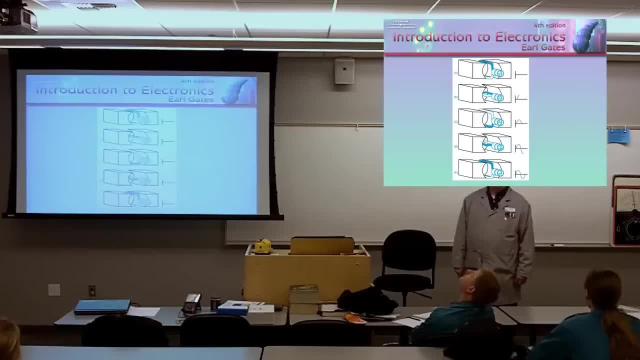 permanent magnets or are they electromagnets? Are they electromagnets? That's my question to you. What's that? I think they're natural magnets. No, No, because there's a power going to it. And what do you call? 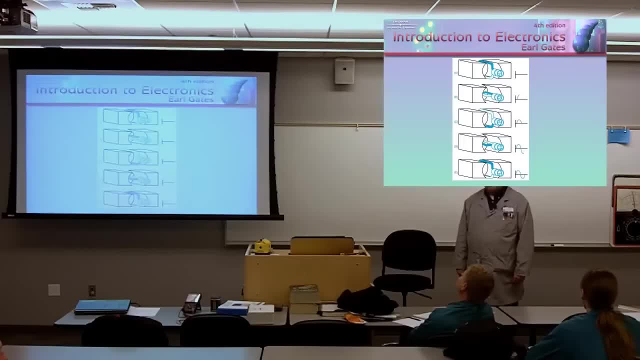 that If some of you have ever played around with an alternator, you might remember As soon as I say it. you're going to know if you've played around with it before. It's called your field windings, Your field windings, Your field. 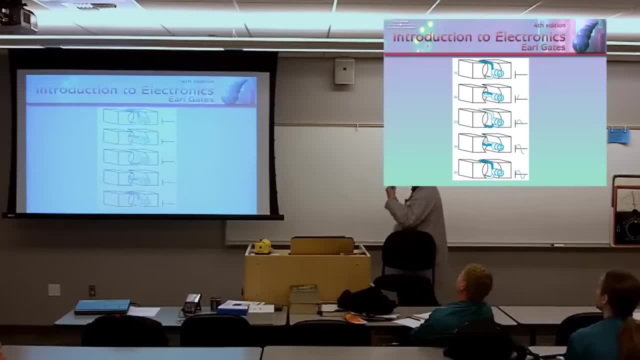 windings produce an electromagnetic field. You know how you can push start a car. You can push start a car if it's dead. You can push start a car if it's dead. If the battery is totally dead, you're not going to push start a car. Some of the older VWs are different: Different magnetos, different system, Different on my aircraft. My aircraft doesn't have a system like that. It has a magneto. If I get that prop rotating, I'm creating a spark that will. 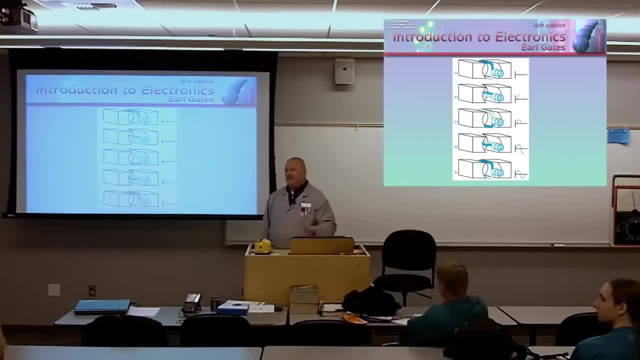 support the combustion process. Kickstart, motorcycle Your car if your battery is totally dead. if you remove your battery and try to push, start your car, pop, start it. it ain't going to work. If your battery is kind of dead, not enough to crank. 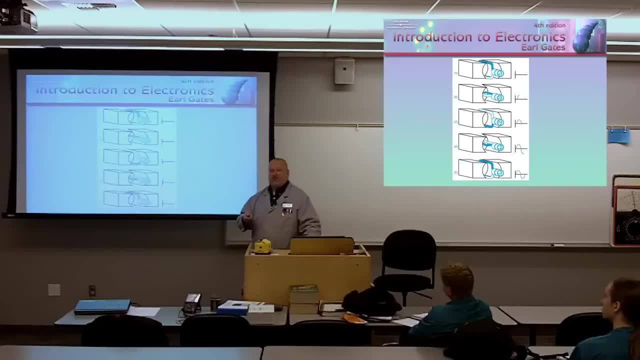 the starter. but enough to go. click, click, click, click, click. that's probably enough to create enough of a magnetic field. so when you push the car, pop the clutch, start the combustion process, get the engine turning immediately, you're going to start to. 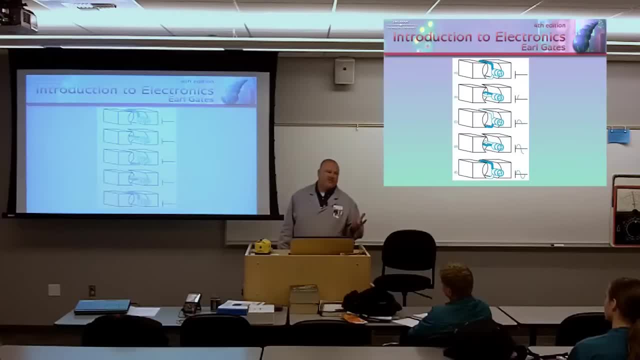 increase the voltage to these windings, So these windings could be very. I don't really know of any applications that use permanent magnets here. Most all use windings. The same thing for a power generating plant like at Grand Coulee Dam. 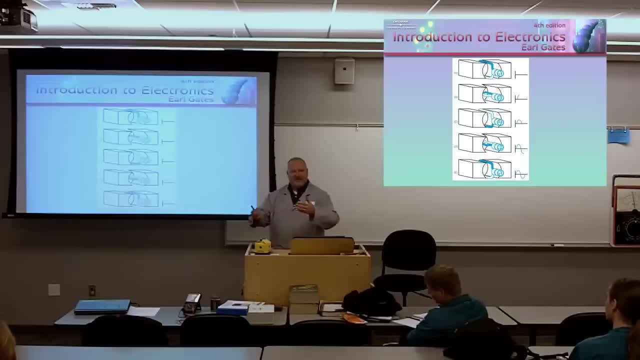 They got to start off with a little bit of voltage to create the magnetic field and then get the generation process going. They're not permanent magnets. Okay, so this here, this loop of wire- this is an artist's depiction- this loop of wire. 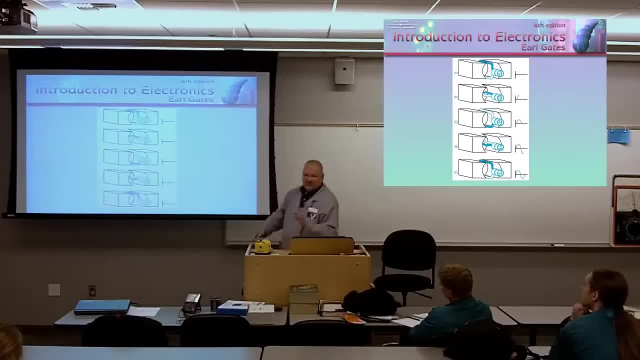 has a light side and a dark side. This is just so you could see it for the purposes of illustration. But this here is actually a loop of wire. The loop, the armature here, is connected to these slip rings. These slip rings allow the 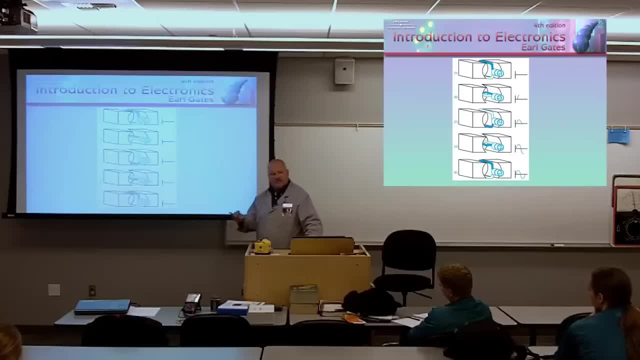 armature to stay connected, 360 degrees of the rotation. So if we look at this right now, North Pole, South Pole, North Pole, South Pole, The armature right here with the winding here at the top and the winding at the bottom Is the winding. 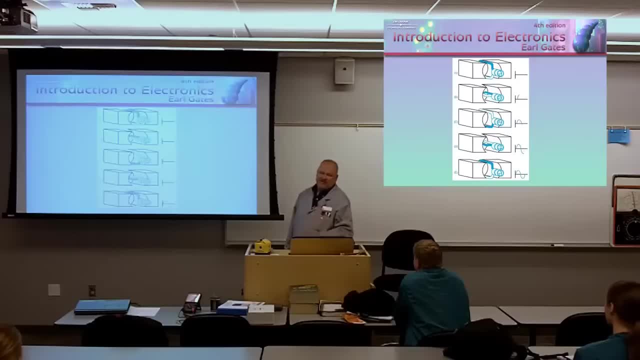 right now, parallel to the lines of flux or perpendicular to the lines of flux. Parallel, It's right at the top, See how it's right at the apex, here at the top. So right at this moment in time, it's parallel to the. 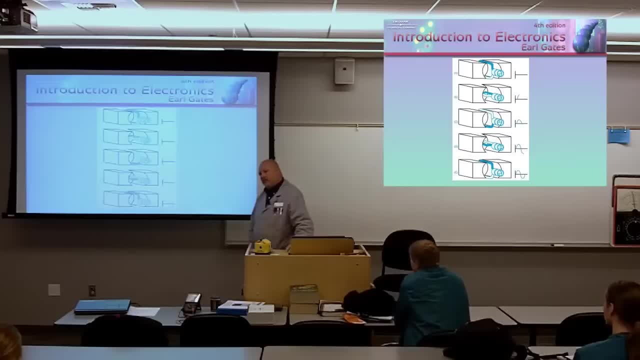 lines of flux. How much current do we generate when we're parallel to the lines of flux? Faraday's Law: How much Zero. And look what we're generating right here: Zero When we rotate that armature. now we're going to rotate it. 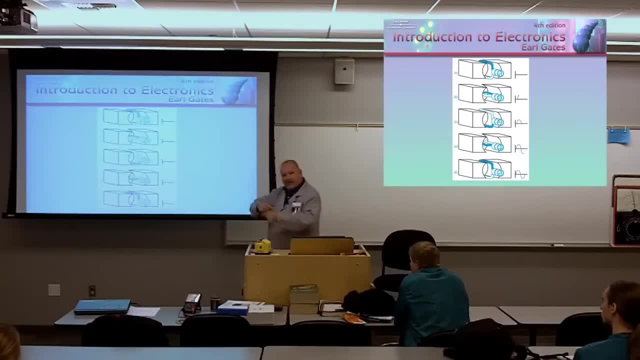 We're going to connect the shaft to this and we're going to blow on it and make the shaft turn through a wind turbine, or we're going to steam and rotate the shaft through a steam turbine or whatever. But when we rotate the shaft now how many degrees? 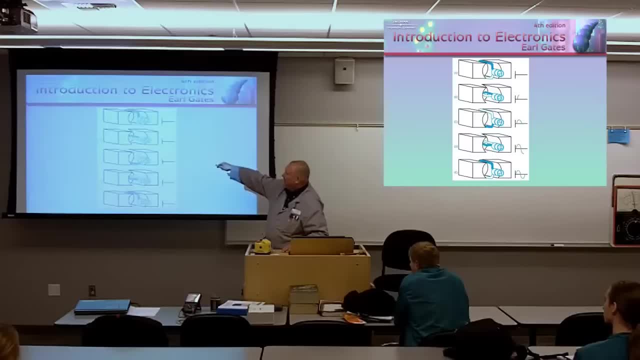 have I rotated it from my peak 90. So right now, is the armature parallel or perpendicular? Perpendicular: What does Faraday's Law say? When I'm perpendicular to the lines of flux, I generate my maximum amount of current. Well, look what we. 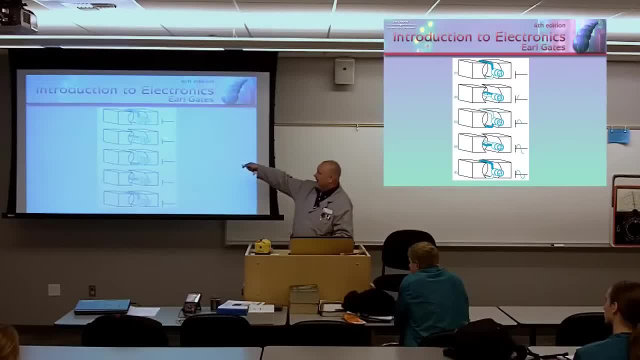 did When we rotated it 90 degrees. now I'm at my maximum peak value When I rotate my armature another 90 degrees. see how I started out here at the top. Then I rotated it 90. Now I rotate it another. 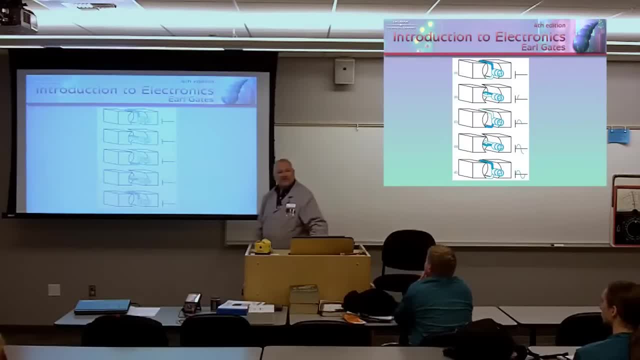 90, so I'm actually 180 degrees from where I started off. Am I parallel or perpendicular to the lines of flux? Parallel? What does Faraday's Law say? Zero. What am I generating? Zero, I rotate it another 90 degrees. now I'm coming up on. 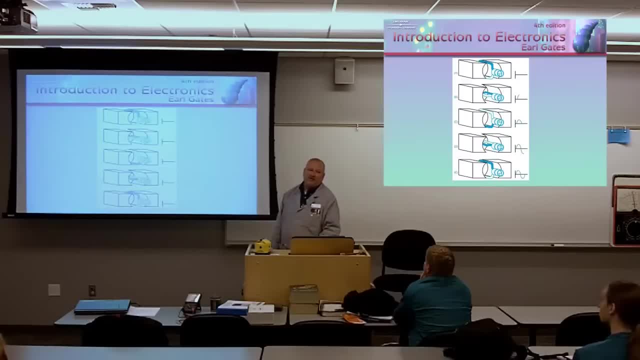 the backside: 270.. Parallel or perpendicular. Perpendicular- What am I going to do? Generating Faraday's Law maximum, cutting my maximum field. I'm right here. I complete that cycle. I've just created 360 degrees of a sinusoidal. 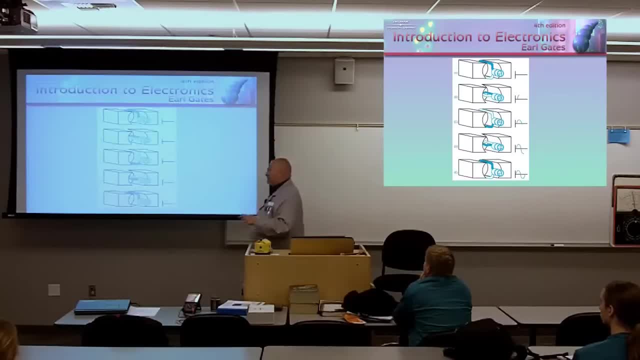 waveform. This is an AC generator. Half of this is positive, half of this is negative. If you're actually an electron, if you're actually an electron caught in this whole thing, basically, what happens is you get moved X amount in this direction. 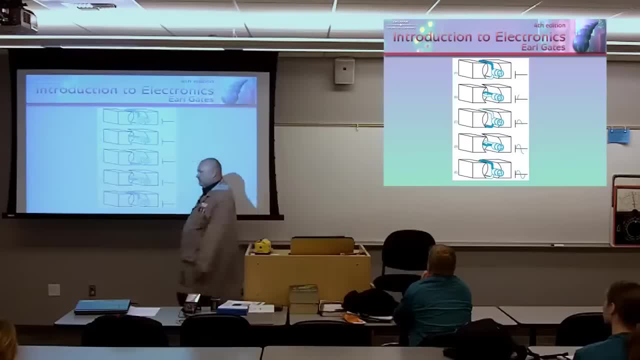 then you go back to zero, and then you get moved X amount in this direction and then you go back to zero. You never really go anywhere, but you do get shaken back and forth. back and forth. back and forth Make sense. 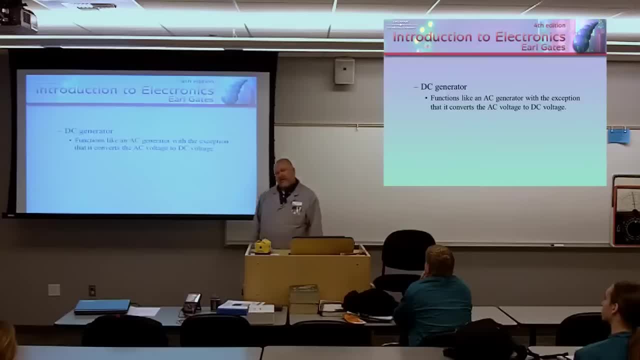 It's an AC generator, A DC generator and actually, by the way, does anybody know who the father of the AC generator was? Who do we give credit to AC generation? Tesla? Very good, Nikola Tesla. He said AC was the way to go. There was another. 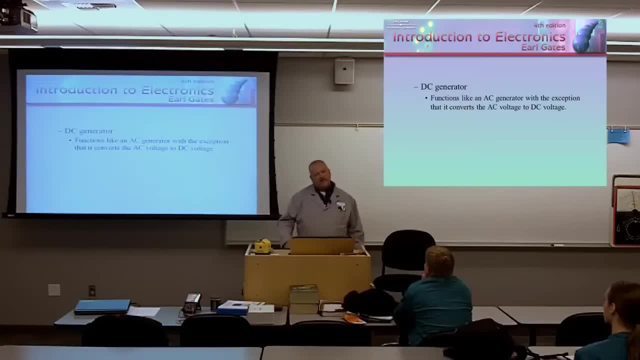 guy big in history who said DC is the way to go. Anybody know who that dude was. Edison, Actually more of a household name. Everybody knows Thomas Edison. Actually, when I first entered this industry, nobody even knew Tesla, Tesla recently. 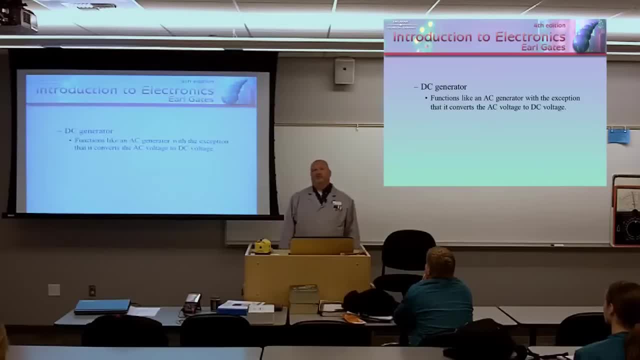 has gained some acclaim or a cult following, depending on how you want to look at it. But Thomas Edison, he wanted to wire up everything in DC. If you go back to New York City, which actually the power company back there, is Consolidated. 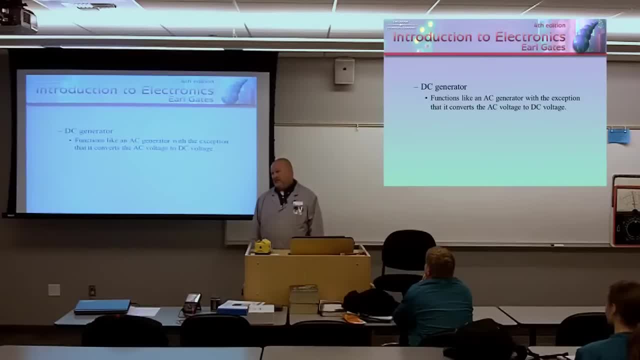 Edison Con. Edison really started out by Edison. Edison got the first contract to wire up New York City and he wired up a lot of the buildings for DC. And again, we're not going to get into it here in class. You can look at: 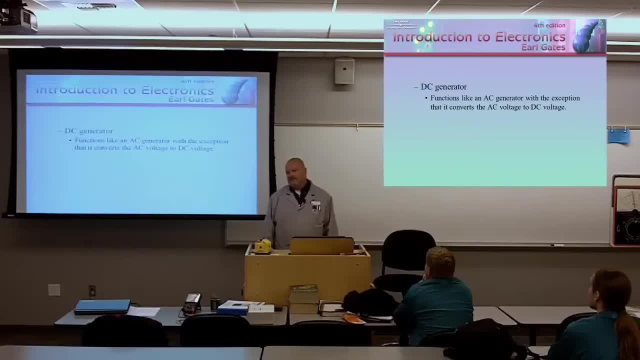 YouTube Edison experiments, electrocuting animals, Tesla experiments- and they were. They'd get like an elephant and electrocute it and kill it dead and say, see, this is why you don't want to use DC, This is why you want to use 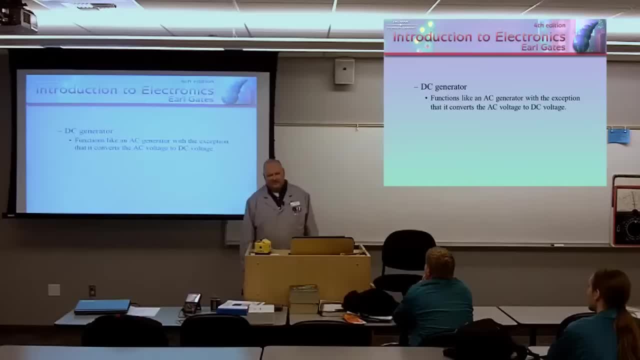 AC. AC is much safer, Sort of like killing animals and stuff. So you can look that up on your own YouTube. We're not going to do it here, But I mean it was These dudes were at each other because that meant world. 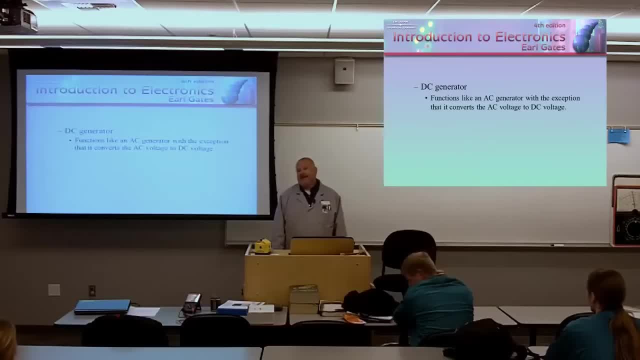 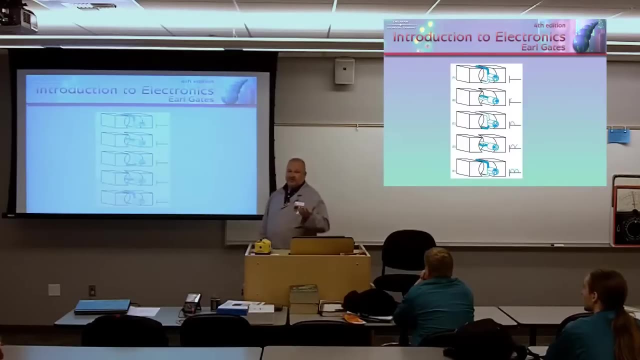 domination, Who's going to get the contracts? And again, Tesla was right. AC is much more efficient to transmit. We'll talk about that later on. So DC never really caught on, But a DC generator. this is how what a DC generator looks like. 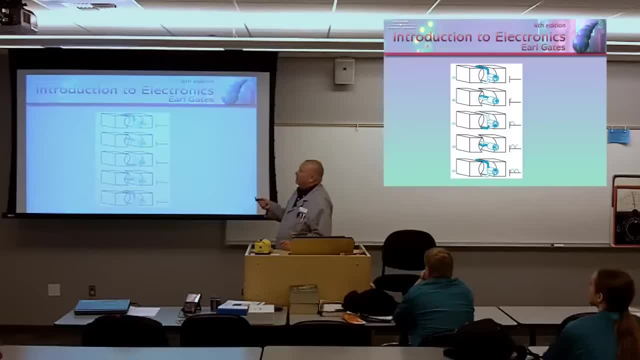 Again you've got an armature. but what note here, as we rotate, this we're coming in contact here with this is called a commutator, And the commutator only makes contact for 180 degrees. So what happens is: 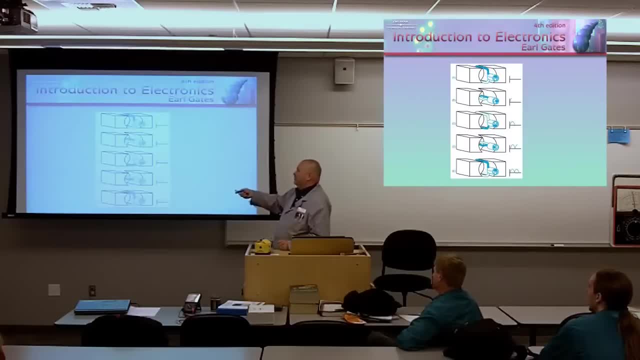 as we rotate the armature through, we're going to generate a positive pulse, Then what's going to happen is we're going to break that electrical connection, because the commutator only makes contact for 180 degrees, And then what we're going to do is harness another positive 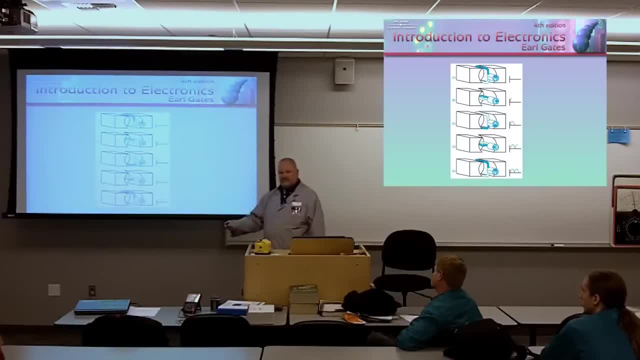 pulse. So it's positive pulse, positive pulse, positive pulse. It's a definition of DC, Definition of DC. AC is half positive, half negative Alternation. This is positive, positive, positive. This is almost like a battery. 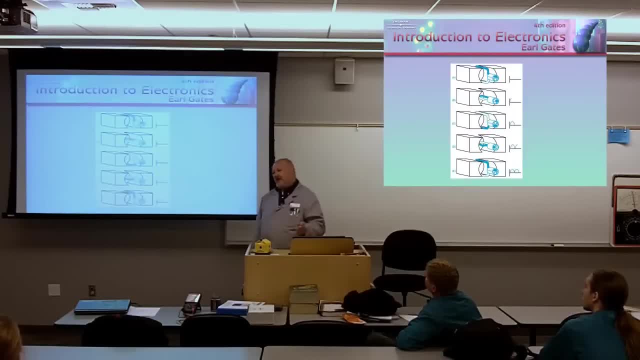 Not quite. This is a pulsating DC, as where a battery would be constant DC created chemically. So the big thing you need to remember is that an AC generator has slip rings and it maintains contact for 360 degrees of the rotation of the armature. 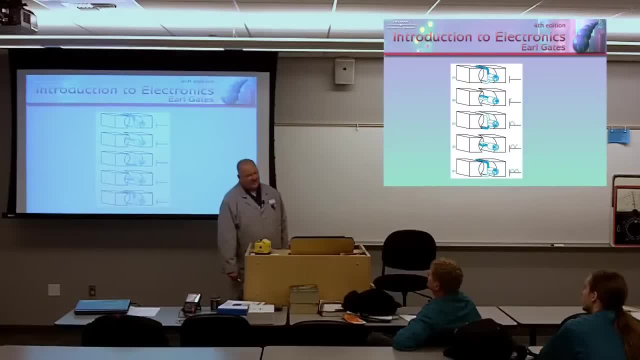 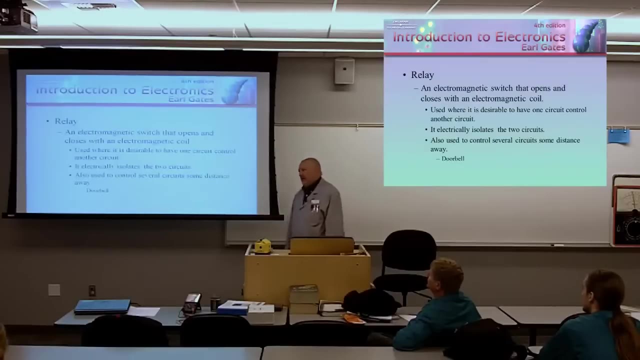 A DC generator has a commutator and it maintains contact for 180 degrees, But the same principle is applied: We're either cutting the lines of flux or we're not. Now a relay A relay. Anybody here have any experience working on any relays? 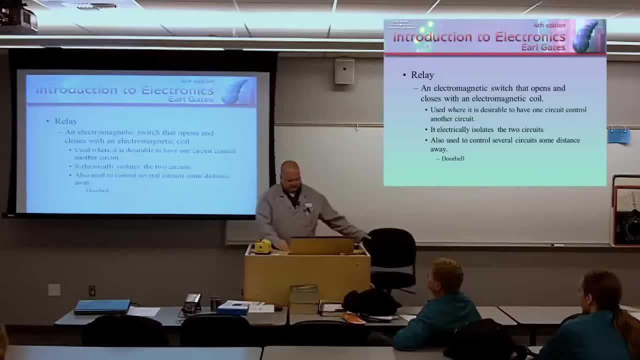 Relays are popular And they still are popular Because for handling high amounts of current it's still a very viable way of control. A relay is an electromagnetic switch that opens and closes with an electromagnetic coil. So real simple With a relay I create. 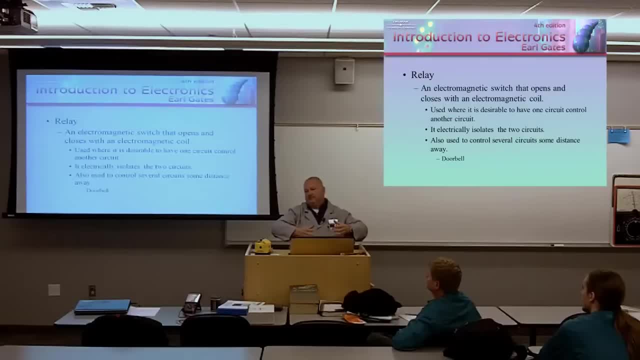 an electromagnetic field with a coil. What I have is an armature above that coil And that armature has a contact on it And it has a spring that basically, when the electromagnetic field is energized, it pulls the armature down, making an electrical contact. 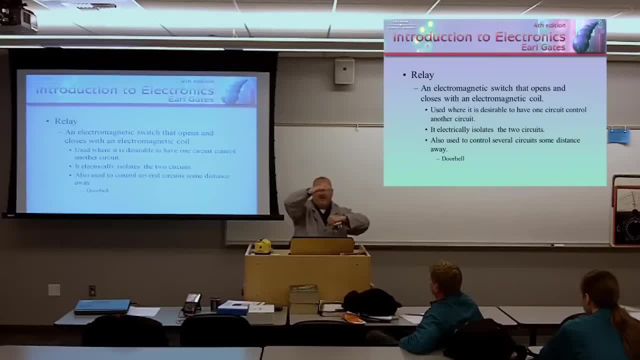 When I de-energize it, it has a spring that opens it back up. Energize makes electrical contact, De-energize opens up the circuit. Or I could do it the opposite way: I could be making electrical contact and when I 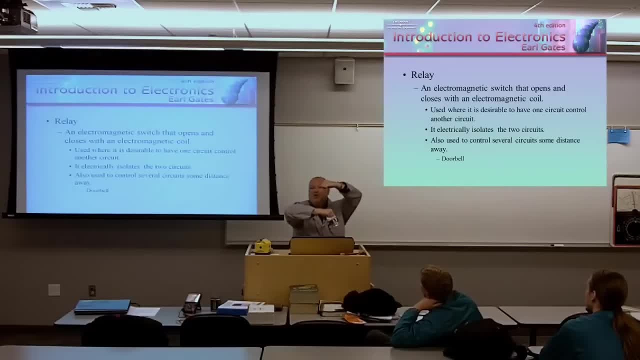 energize the electrical circuit, it's going to open the circuit. Relays also could have multiple ganged contacts. So when I energize it I'm opening and closing a bunch of contacts. But a relay is an electromechanical switch. 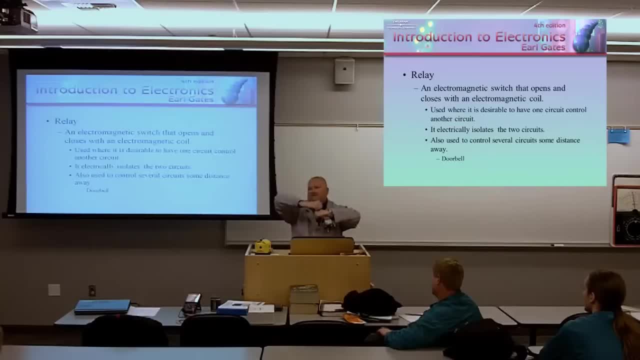 It's using electromagnetism to move that armature up and down. The good news is it's an electromechanical switch. It's going to fail often And you're going to need highly qualified, competent technicians to go in and troubleshoot it. It's called job security. They replace that with something that's solid state. it's not going to need to be replaced. So as long as there are relays, there's stuff for us to fix. We use relays when it's desirable to have one circuit. 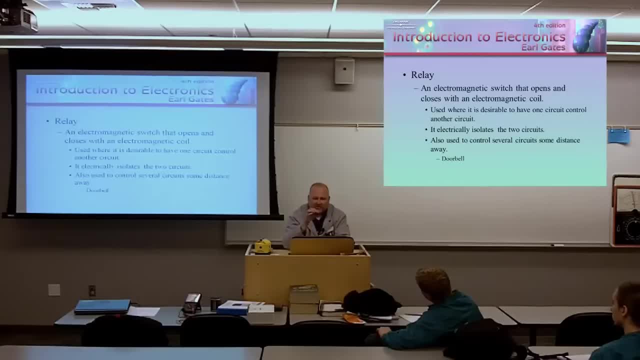 control another circuit, Typically one low power circuit controlling another high power circuit. These lights would be an example. although I don't know if we've got a relay integrated, I know there's a relay that's integrated with a motion sensor, So when the switch 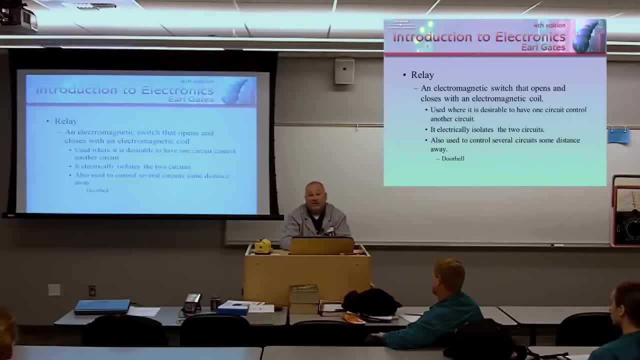 is energized, that motion sensor you'll actually hear. if you walk in here and the lights are off, especially over here, you'll hear the click. Isn't that obnoxious? Somebody's looking for a project to rewire this thing to keep that thing from ever shutting off. 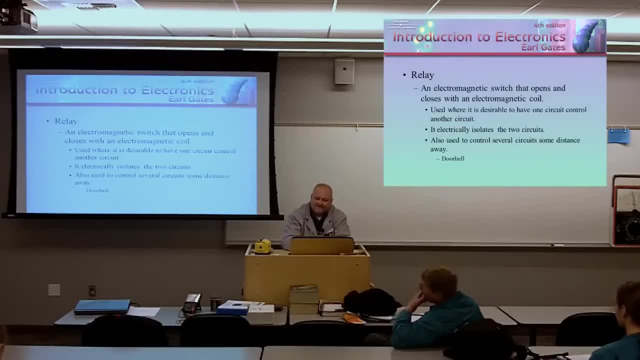 when you're in the lab It becomes pretty obnoxious. It's also used to control several circuits some distance away. So an example of a relay would be: anybody here play with model trains at all. Model trains are nothing more than a small example. 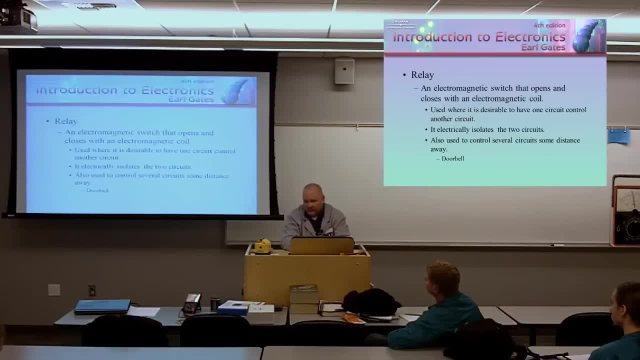 of the real thing. If you look at a freight yard on how they switch and build trains, they basically have switches that move an entire. it's a motor that will move an entire railroad track so that trains could be built on different sightings and such. 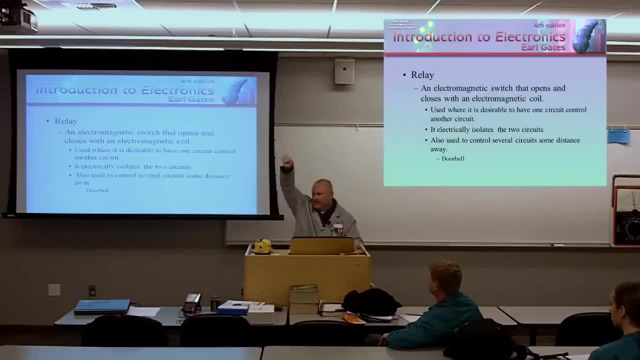 Well how do you control that? The switch alone would be like a Frankenstein you know switch. You can't do that Typically in a switching yard. you'll have up in a control tower a small switch that they throw that sends a small signal out to a big relay that. 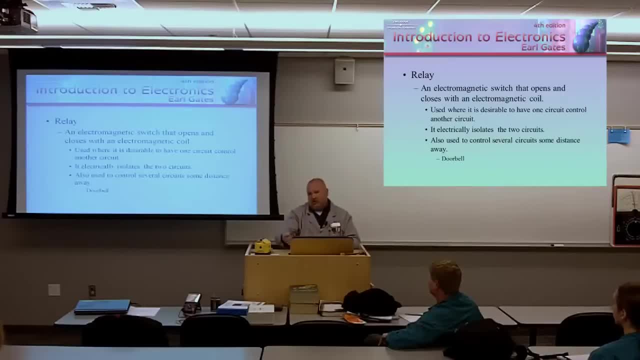 makes connection and allows all that current to flow and turn the motor which boom, switches the track. It wouldn't be practical to have wire this thick going to a control tower knocking. you know it would pull the control tower down, Wouldn't make sense. 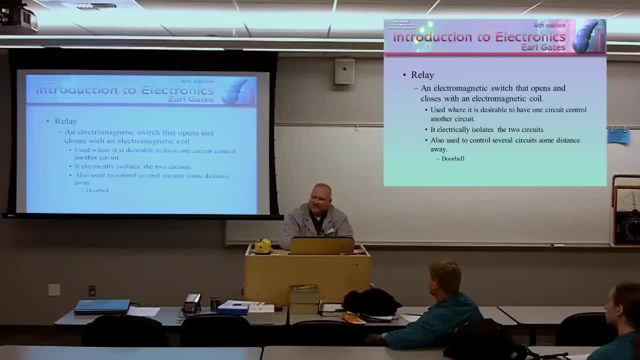 So it's used to electrically isolate the two circuits. Make sense, Okay, Example of this would be a door bell: Small signal voltage, bringing about a large change. The large change is you get woke up out of a sound sleep because the delivery. 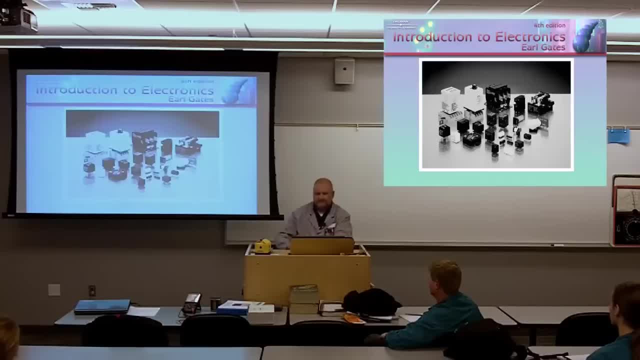 man's outside delivering a package. Here's some examples of relays. Some of these relays are actually encapsulated, so they could be put in a explosive environment, because when you open and close that contact, what are you doing? There could be a spark. 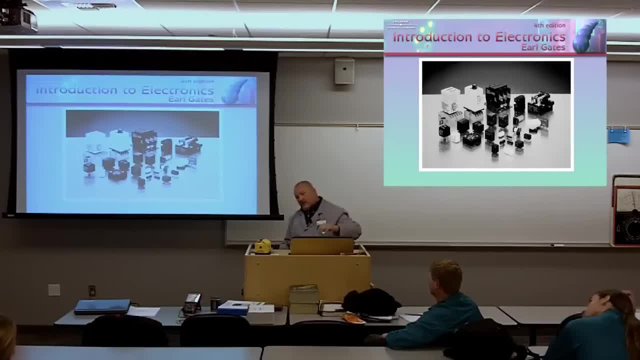 There could be a spark. So if you're working at an oil refinery, you probably don't want that spark. You want that spark to be contained, so it's going to be in a sealed relay, This one right here. you can probably see the contacts. 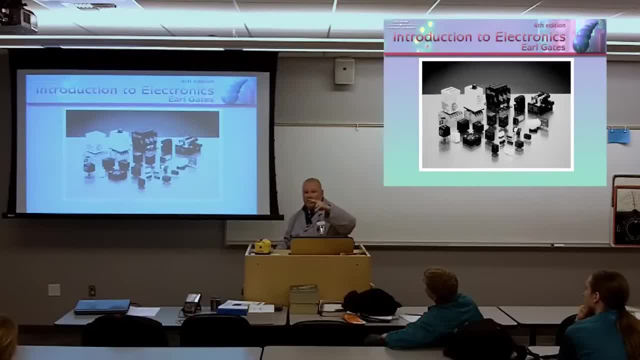 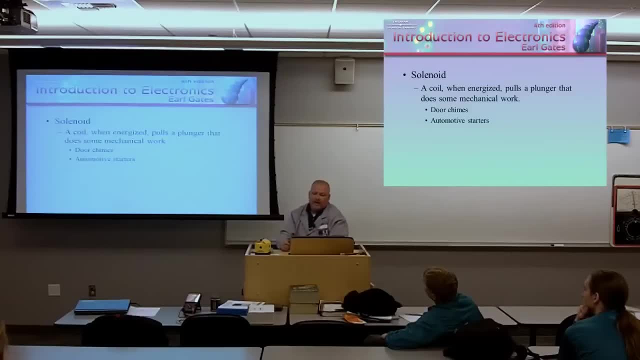 There's two contacts here and that thing is going to open and close Big sparks. Now a solenoid is a coil, when energized pulls a plunger that does some mechanical work. An example of this might be door chimes, I'm talking. 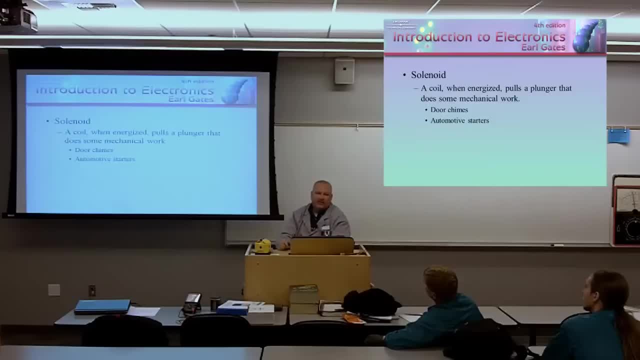 about the old school ding, dong ding, dong right. Those are physically little hammers hitting chimes. Now, most of the stuff, even like clocks- if you buy a clock that has chimes, it's not chimes, it's a recording of chimes. Synthesized. There's very few examples of real chimes being struck by solenoids. Another example is your automotive starter. When you turn the key- typically you turn the key that energizes a starter relay. The starter relay energizes the starter. 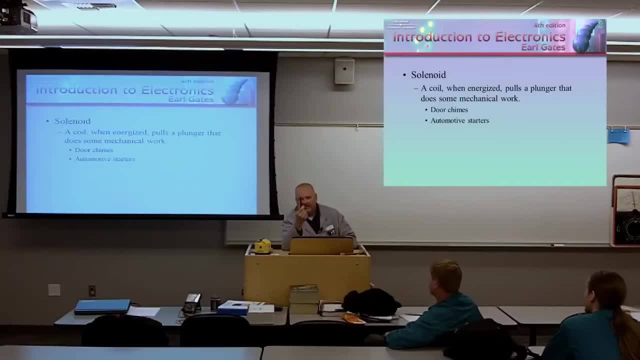 solenoid. The starter solenoid on your car is probably about the thickness of this laser pointer and on the top is going to be a big piece of metal that when you energize it it's going to pull that metal down and make a. 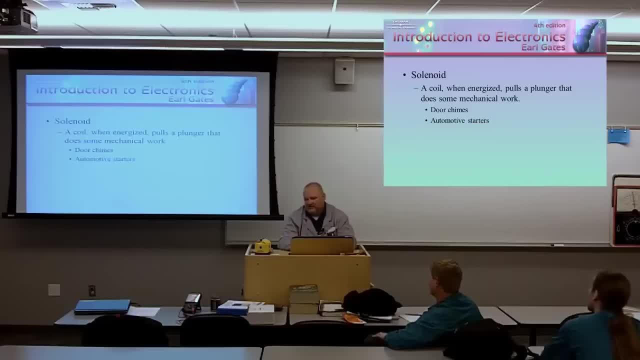 big electrical connection. That big electrical connection basically takes all of the energy from your battery and dumps it into your starter. There has to be physically a lot of metal present to make that electrical connection. So a relay has a moving armature, A solenoid has a 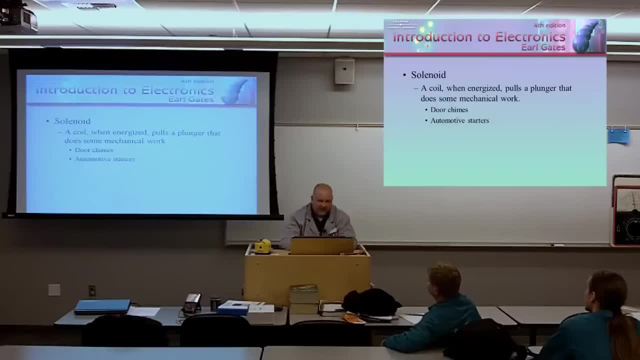 moving plunger a moving core, if you will. If any of you have ever played a pinball machine- the flippers solenoids. When you hit the button, the flipper, it's energizing a solenoid. 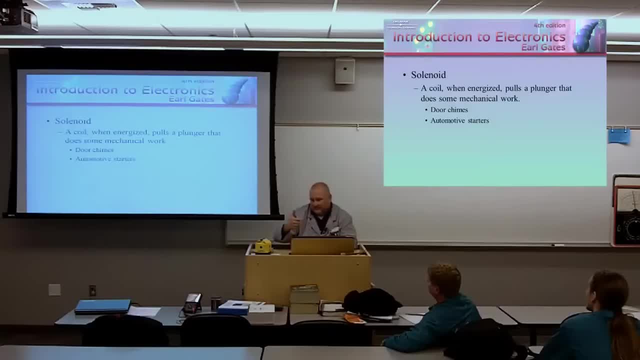 That solenoid is attached physically to the flipper that's going to move back and forth, back and forth. Energize, de-energize, Energize, de-energize, Energize, energize, de-energize. 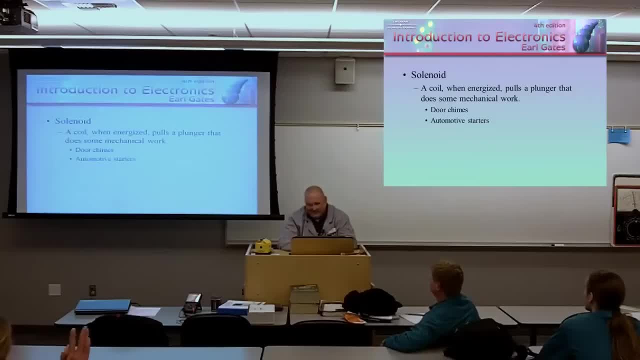 Pinball- Anybody here like pinball. It's the bomb, It's pure, It's the pure game. Look for a project: There you go: Restore a pinball machine. You could restore a pinball machine, contemporary pinball machine. 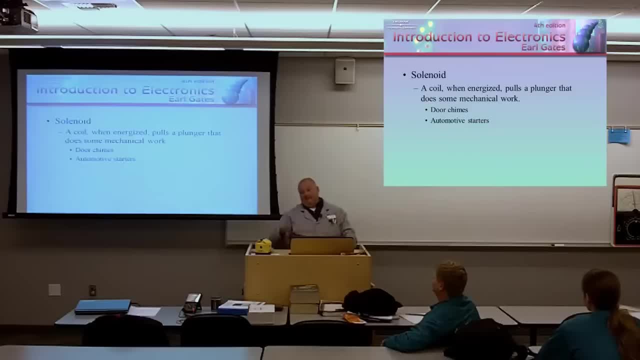 It's got everything: Electrical, mechanical. You've restored one. Really, There you go, There's projects, There's projects Right there. What era, Really? Huh, I've got one. I've got F-14 Tomcat. 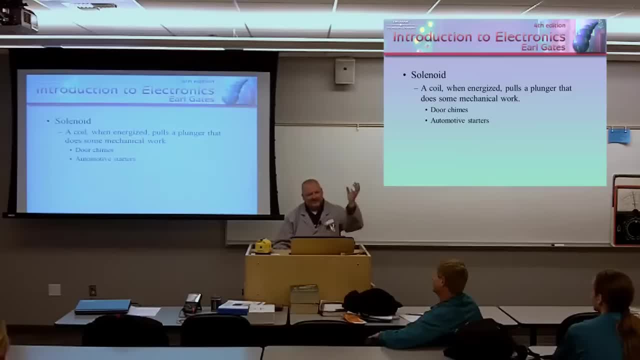 It's the real deal, man. If any of you remember that one, it had the big gumballs on the top: red, white and blue. When you get it into the advanced levels, those things light up. It was actually considered. 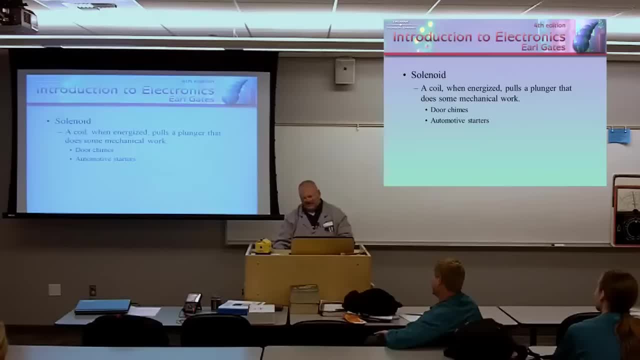 the most obnoxious pinball machine ever created. Because if you're in a bar, you know those freaking lights, you know looks like a police car parked there or whatever. when you get into the, you know multi-ball- It's pretty slick. 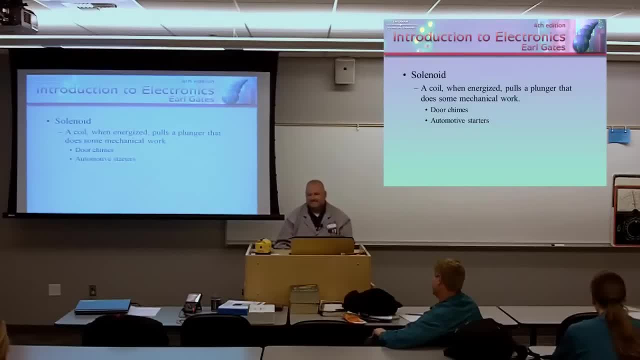 What's that? Williams Williams, Yeah, Good stuff. Um 87? One of my other favorites. I've been keeping my eyes open. If I find one, if I find one and bring it home, my wife will kill me. 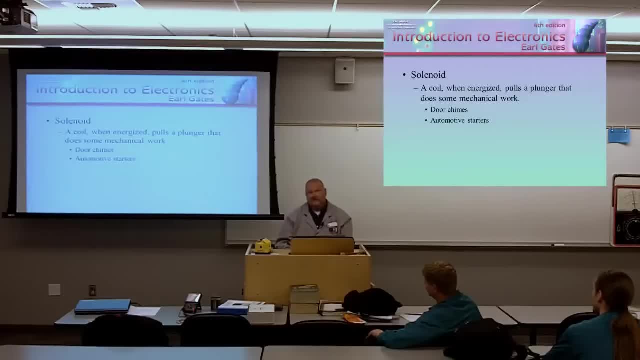 Because that one pinball machine. she's freaking. when are you going to get rid of that thing? Never, I mean, it's so freaking cool man And I keep it operational, you know, Um, but the other one I'm always looking for is Cyclone. 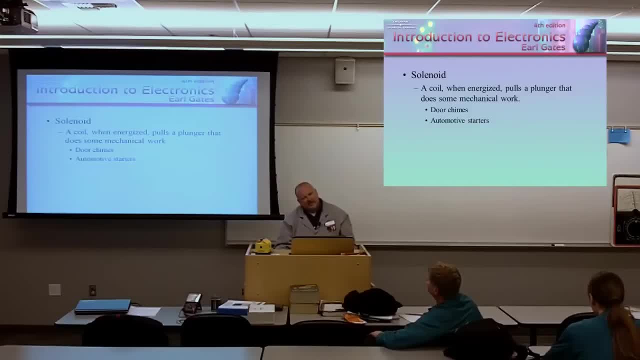 Any of you remember Cyclone And it was a big, uh, you know, during the Cold War. Ronald Reagan And actually the Cyclone rollercoaster. and then the front car is Ronald and Nancy Reagan Holding on for dear life. 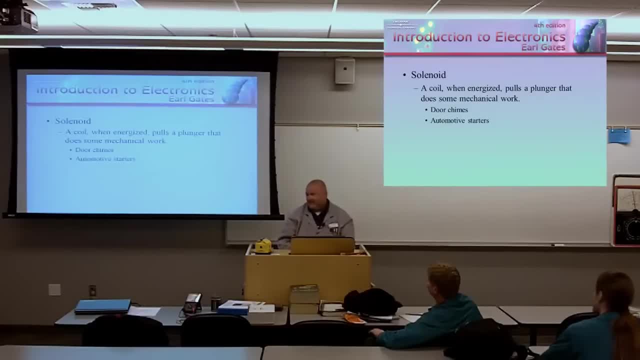 Great pin, Great pin, Anyway pinball brought to you by the amazing solenoid and relays. I love the applications for these things. Actually, one of the things too with relays that's kind of fun is some airports. 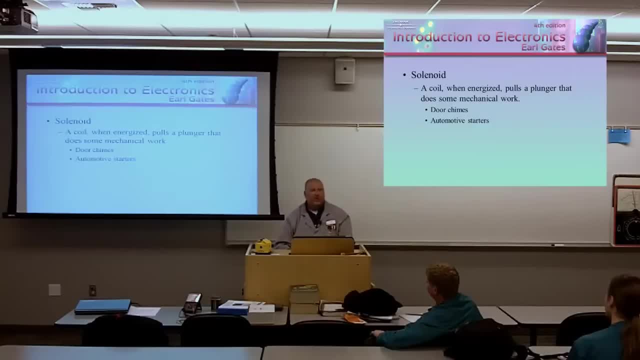 have what's called pilot control lighting, And one of the local airports here is Bremerton, Bremerton National. You know probably a lot of you don't even know Bremerton National. You can land a 737 over there. 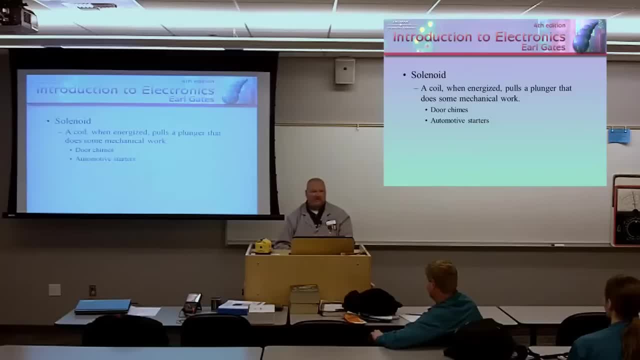 It's a big airport. you know They don't have any commercial traffic in and out. They've actually tried in the past- but it's just not that big of a market. But it's a big runway: Pilot control lighting. So one of the things that I've 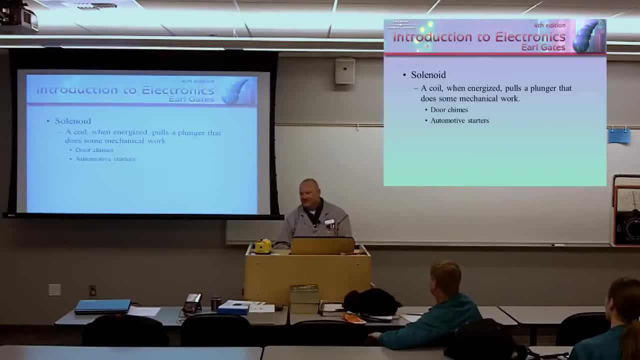 been known to do in the past. if I'm bringing somebody that's not accustomed to aviation is what I'll do, is I'll start the approach and I'm flying the instrument approach. so I'm following an invisible glide path down to the runway. 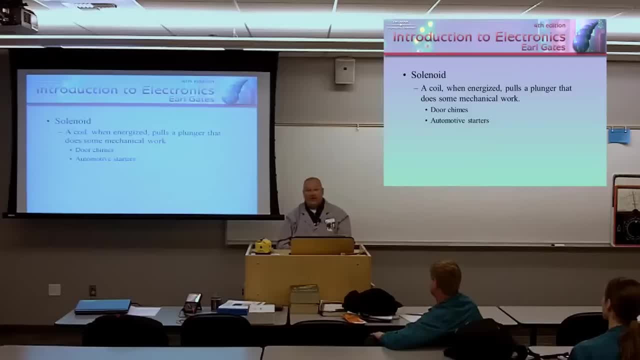 So when the lights are turned off at the airport, it's just a black hole. You're just descending into this black void And then usually about a half a mile out. what I'll do is I'll dial in the frequency and then I'll hit the code And basically, 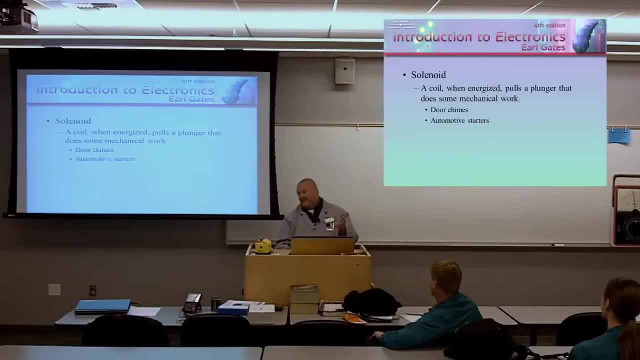 it's a matter of me. just turning my transmitter on and off, on and off, on and off five times Turns it to high intensity. So all of a sudden you're descending into this black hole and then before you, this runway appears. 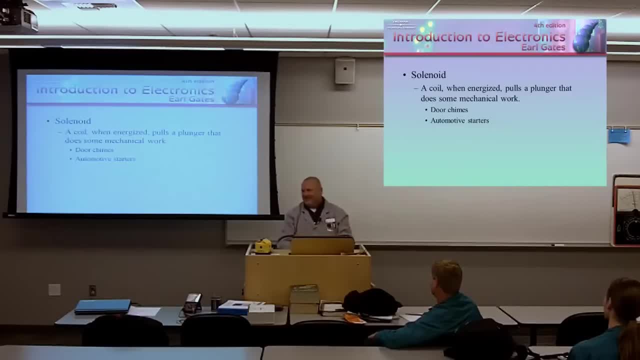 with the chaser lights and everything And it's kind of a power trip. you know, I think it's kind of cool, you know, by me simply, you know, clicking my radio I just turned on, you know, this huge airport, you know. 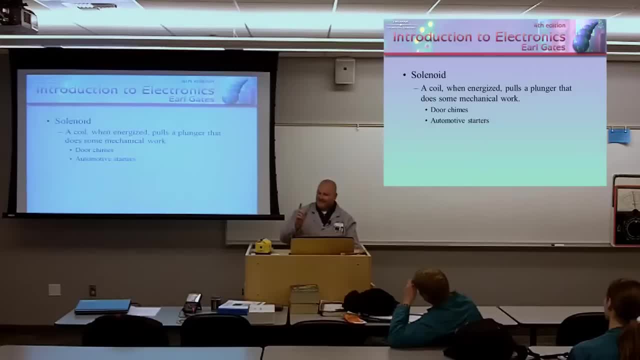 5,000 feet of runway lights. That's all brought to you by well. there's the pilot control lights, There's the lighting aspect of the radio, But what really makes it happen is relays. You know, really relays. 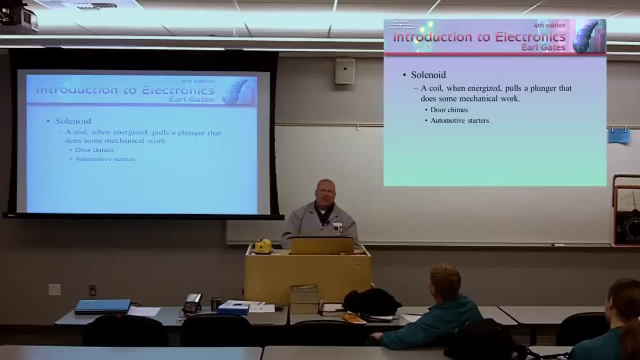 It was actually fun with relays too. Also called could be called an industrial contactor. Industrial contactor: I used to be really in the. I guess I've gotten old and I'm out of the swing of things with holiday lighting. 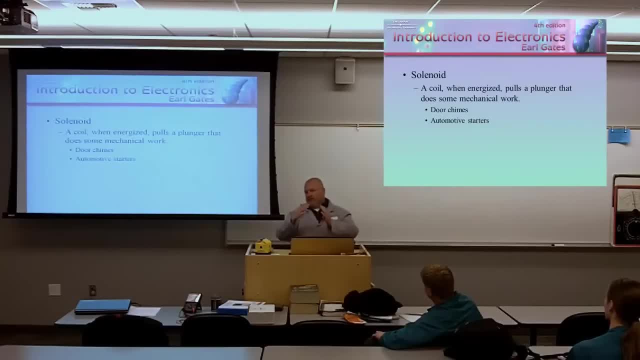 I used to cover every right angle of my house. I mean it looked like you know Christmas vacation material And it was kind of funny because my next-door neighbor, he worked for Boeing. He was an electrical engineer for Boeing, The guy across the street. 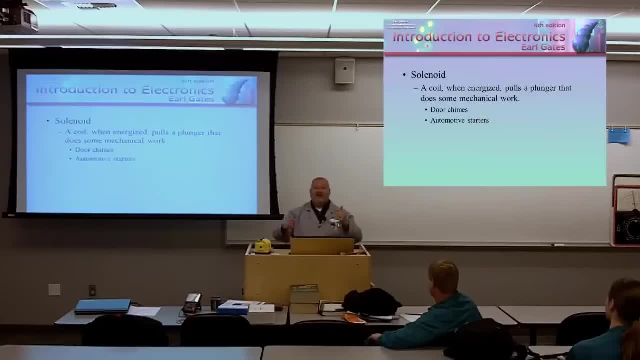 was an electrical engineer for the Federal Aviation Administration. So these guys, you know I'm out there kind of messing with them and stuff, And you know you see them plugging in an extension cord and a bush lights up And you know you plug in another extension. 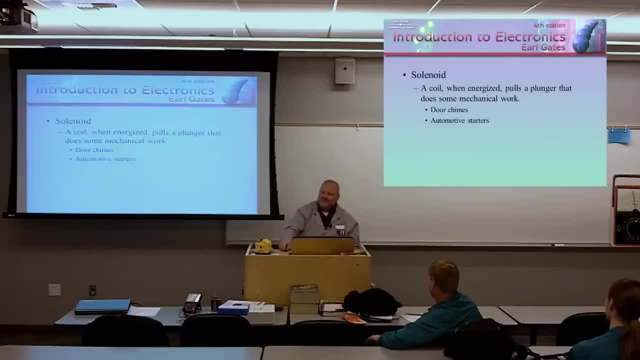 cord Another. you know, the roof line lights up, And with me I wanted to control everything simultaneously. So I got this big industrial contactor that fell off the back of a truck And what I have are four separate circuits. Each circuit is up the 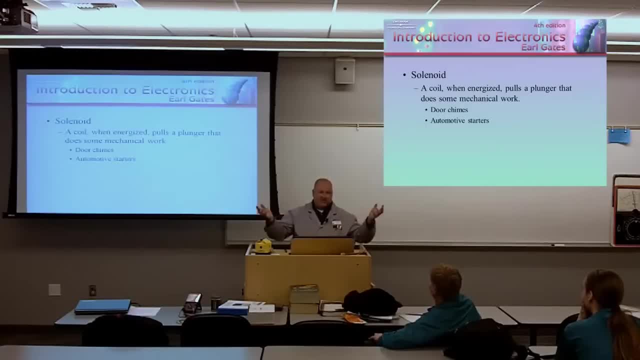 20 amps each. So what I did is I put in, I basically rewired my home and I have separate circuits for the outside lights, And then I have it on a timer. I mean I could connect it to the freaking, you know, clapper. 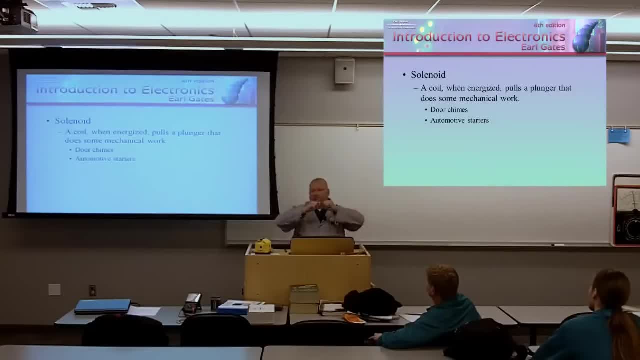 if I wanted to Right. So, simply, when that turns on, everything is on at once. It's like: how did you do that? This here is an industrial contactor, you know, It's kind of a cool system. Yeah, yep, absolutely. 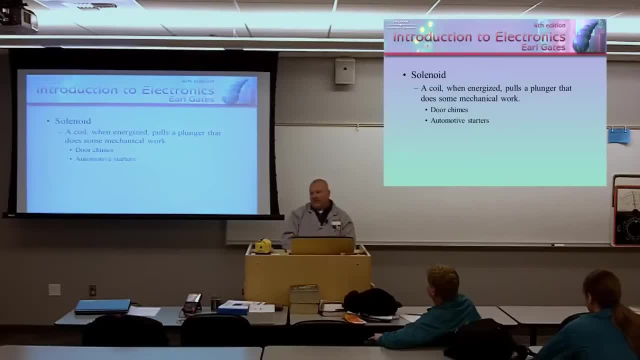 Yep, yep, And actually one of the things that brings that about- and this was kind of where I was segwaying into- is normally for a first quarter student, you'd be taking the PLC class, ELEC 116. 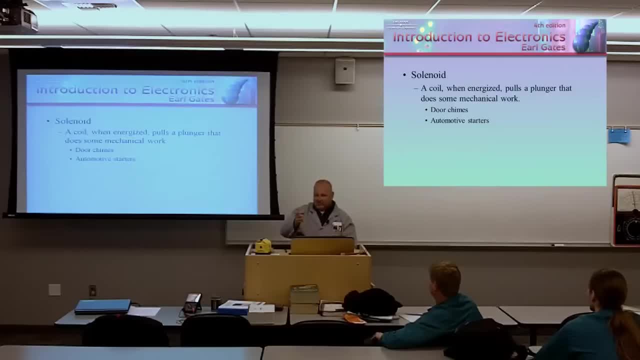 PLC basically is an industrial computer that controls, open and closes, basically relays for industrial control. So after taking that ELEC 116 class, if you wanted you could buy a PLC and basically set up a Christmas display on par with you. 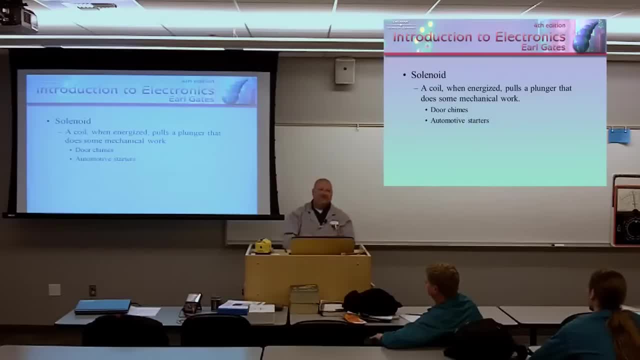 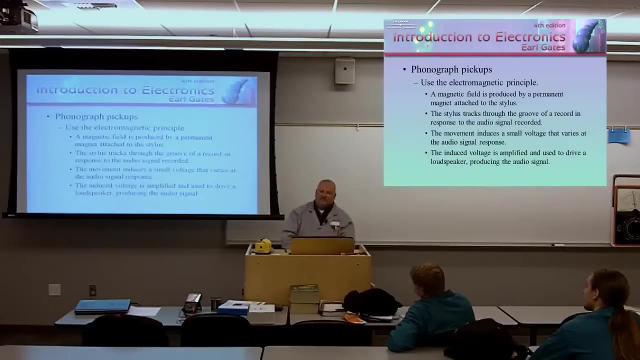 know, what we've seen on video is that, with the light synchronized to music and everything, Really easy to do with PLCs- Real easy to do- Well, not easy, but doable with PLCs, Phonograph pickups. I'm sure some of the younger students are sitting in here and saying: 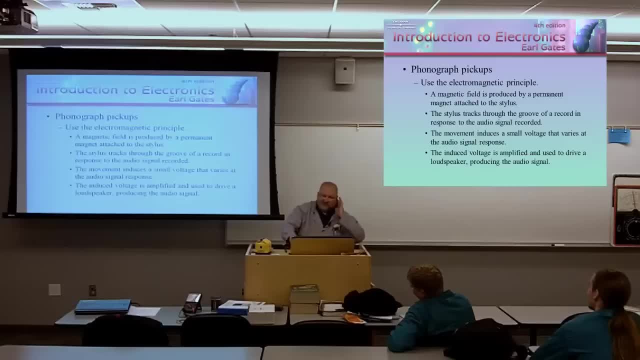 what is a phonograph Right? What's this with the scratching right? That's what they're scratching on. a phonograph right Uses an electromagnetic principle. believe it or not, A magnetic field is produced by a permanent magnet attached to a. 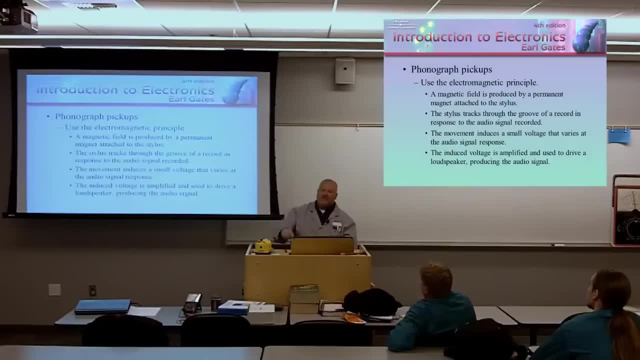 stylus. The stylus tracks through the groove of a record in response to the audio signal recorded. Basically back in the day- some of you are probably familiar with this- like a musical group were cutting an album And literally what they were doing. 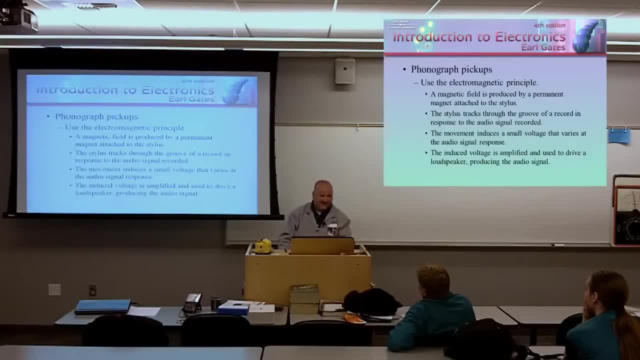 was cutting a groove into a blank and they're cutting an album, They're recording an album. This is how it was done back in the day. Then what that would be is a negative. Then, with the positive, you could start stamping out albums. 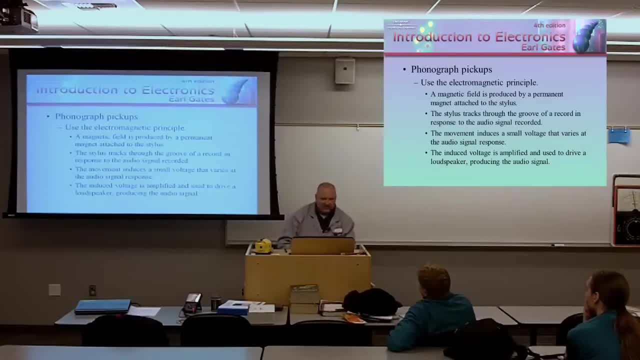 all day long and getting them to radio stations, play your music and start selling it, and that's how you'd make the big time. Well, with the MP3, that's all changed. We won't comment on that. But the stylus, literally. 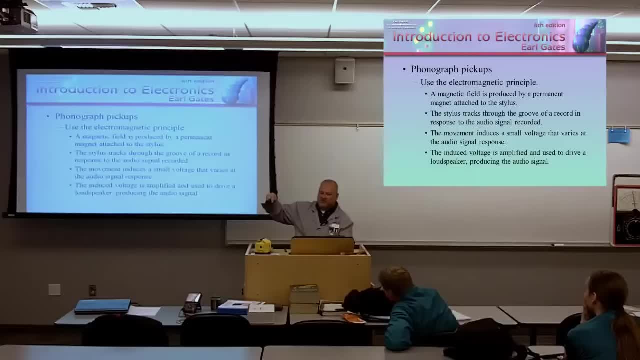 tracks through that groove in the record. in response to the audio signal, The movement creates a small voltage that varies at the audio signal response to replicate the wave pattern that originally created it. The induced voltage is then amplified and used to drive a loudspeaker producing the audio- a facsimile. 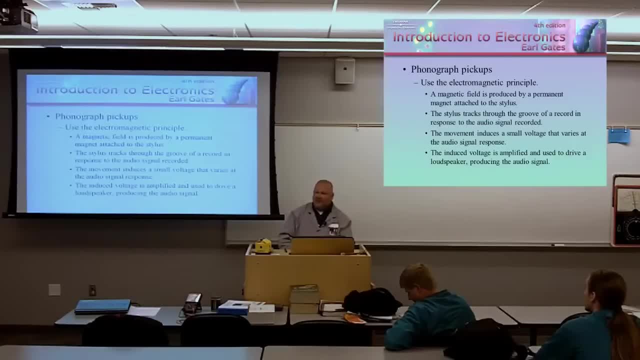 of the audio signal that produced it. Anybody here own any albums. Do you have the ability to play any of those albums? I actually bought a phonograph a couple years ago because I had some older records and all the stuff is available as MP3 now. 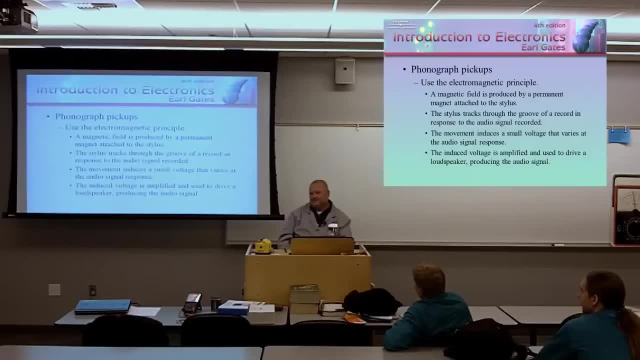 They don't. They don't. For that full experience you need a phonograph player to play it, Kind of a classic old school retro way of going. No, It's almost too clear. I'll tell you some of the stuff. I have a hard time. 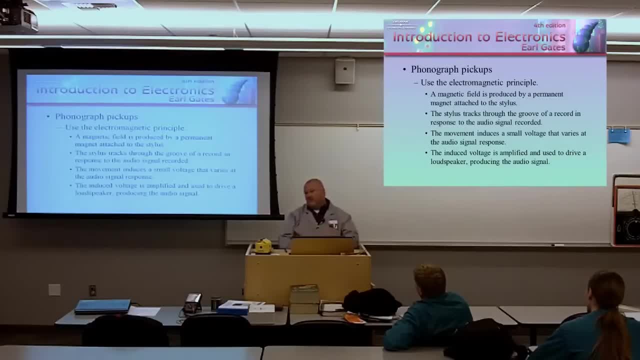 because growing up in Connecticut I had my little eight transistor radio. we'd go down to the beach in Connecticut Shore, Rhode Island, Musquamaca Beach. we'd go down there and whatever. you're listening to the New York radio station, you're listening to the hits, the top 40 hits. 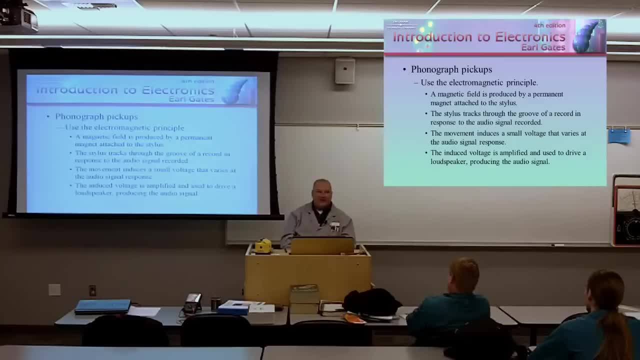 you know, now I listen to some of the high quality recordings. it's kind of like: is this a remake, The original? because the original I was listening to out of a little speaker like this, eight transistors, mono. now the stereo version of it. 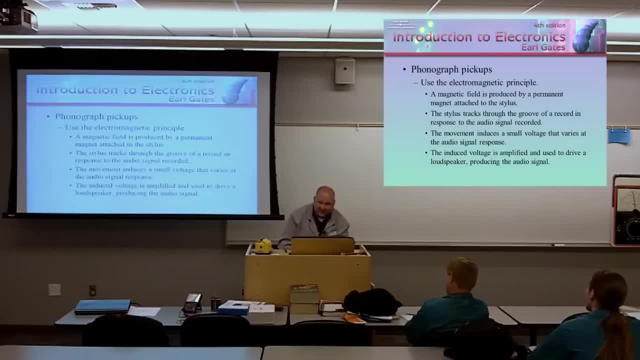 it's a little bit different and of course I was on a limited budget so I wasn't always going out and buying the albums or certain albums that you had and that was high fidelity back in the day. so how a record player would work magnetic, that little stylus tracking in there. 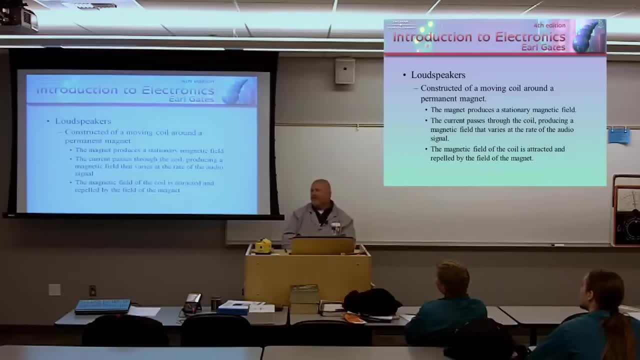 magnetic cartridge loudspeaker- basically the opposite, Constructed of a moving coil around a permanent magnet. so basically, if any of you have ever bought speakers before, one of the attributes you look in, basically he or she who has the heaviest magnet, the biggest magnet, wins, because that's the permanent magnet. 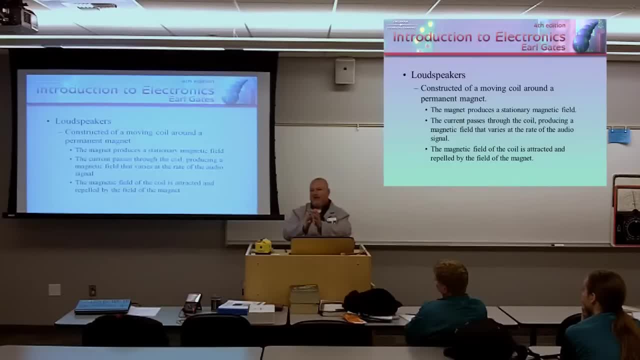 and what that means is that you could throw more energy in there to create either an attraction or a repulsion and move the cone of the speaker back and forth rapidly, replicating the original sound that created it. so that's how a loudspeaker works. so the key components: the size of the magnet. 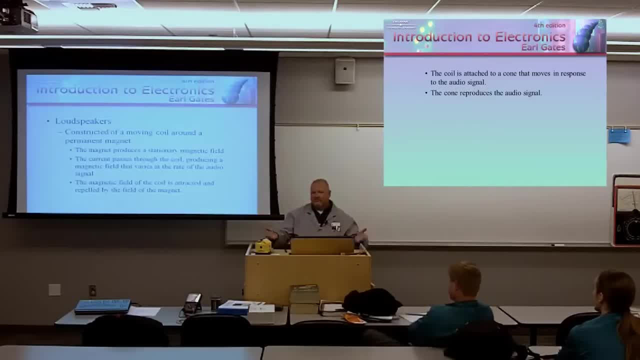 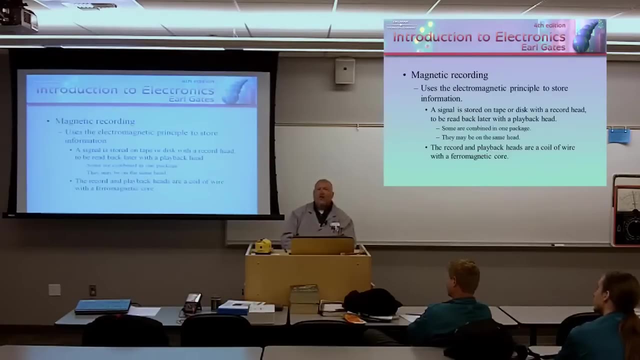 the coil. how much energy? how much energy measured in watts, acoustic energy? but again, it's a magnetic device. that's how it works. magnetic recording using uses the electromagnetic principle to store information. a signal is stored on tape or disc with a record head to be read back. 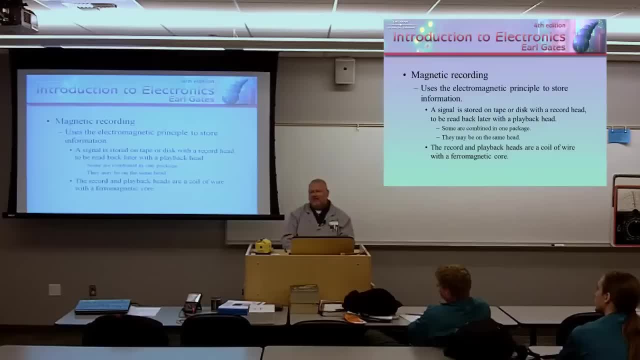 later with a playback head. some can be combined in one package. that means record head and playback head on the same head. the way that this works, and it's kind of important that you understand this- basically it's like getting a piece of tape and sprinkling a bunch of iron filings. 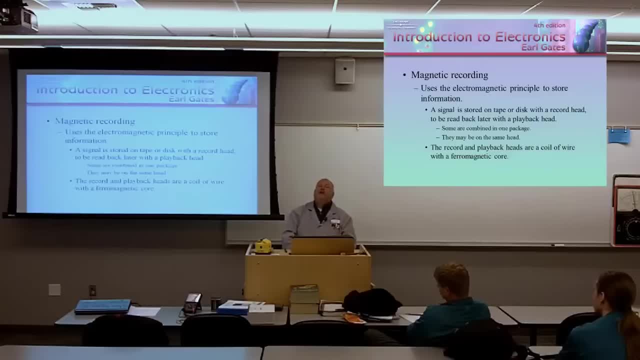 on that piece of tape. by passing that tape over record head. when I speak into a microphone, I'm creating a signal in the wire because the microphone, which also is a magnetic device, the vibration, the air molecules moving back and forth create that vibration. the microphone picks it up. 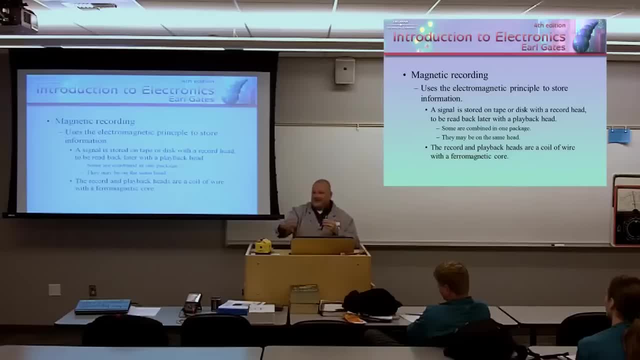 and transforms that into a small electrical signal that goes in, gets amplified and gets connected to the record head. the record head is going to fluctuate its magnetic field, putting those iron filings on the tape into a unique pattern. into a unique pattern. that pattern will be stored on that tape. not indefinitely, because if it's stored here on planet earth, what's one of the things that it could be under the influence of the earth's magnetic field? if you put it in close proximity to any other electromagnetic device, it could alter that, so magnetic recordings will not. 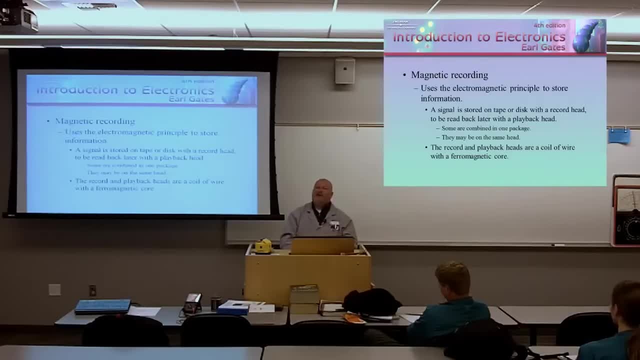 last forever, as a matter of fact, a magnetic recording. every time you play it back and you try to read that fluctuation in the particles that was put on there, it loses a little bit of what it was originally. remember how the video stores get younger students now. what's a? 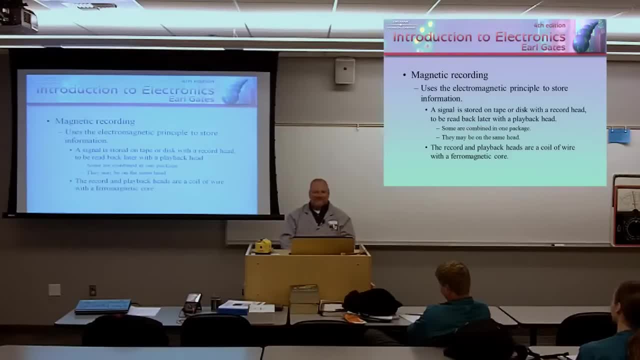 video store. well, back in the day, you used to have to go to places and rent VHS tapes. why would you have to rent tapes when it's just to get it on demand? well, that didn't exist back then. you used to have to rent it on tapes. 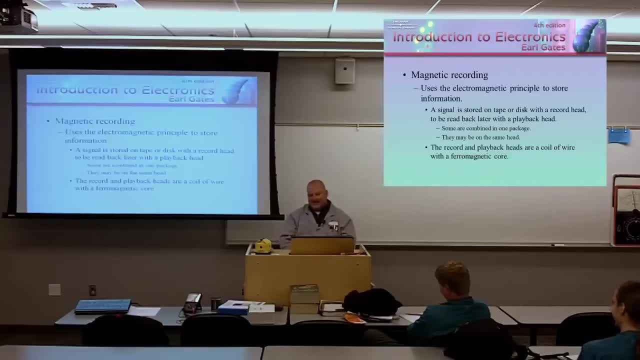 be kind and rewind. be kind and rewind. absolutely. those were the good old days. they really were, I think, those tapes they used to sell. they'd only get so many uses out of them and then they would sell them as previously viewed. you know, and I used to capitalize. 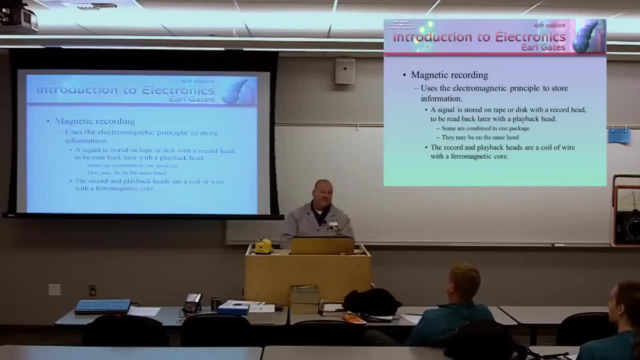 and add to my library if there's a movie I really liked by it previously viewed, but you know what the quality was. always on its way out, because every time you use that play, that tape you'll lose a little bit of it. so, like for high end production, 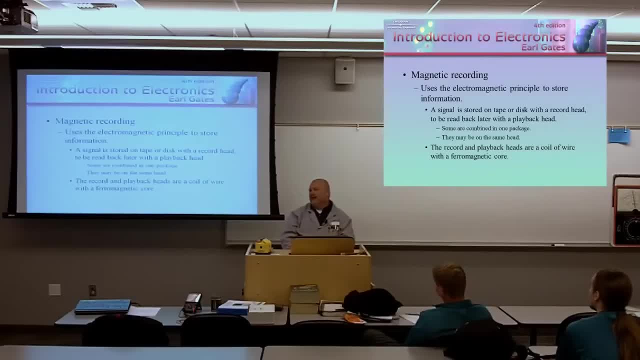 in video. what they would do is: let's say, you're making a documentary for the Discovery Channel and you're shooting it on video. now, there's some different ways of doing it, but if you're shooting it on videotape, what they would do is they'd go out. 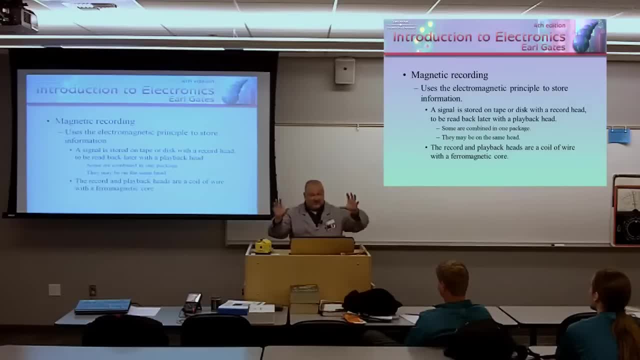 and they'd shoot with a helicopter and these beautiful shots or whatever. they'd get the original tape. they'd make one copy for the purposes of editing. then they'd put the originals in a vault and they wouldn't touch the originals. then they would figure out. 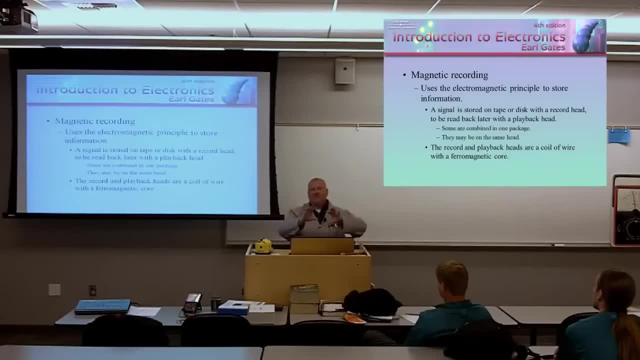 well, we want to edit this scene, we want to edit that scene. we want to do this once they figured out where all the edits were. then they'd go back to the master tapes and they would make a recording of the segments that they want and produce. 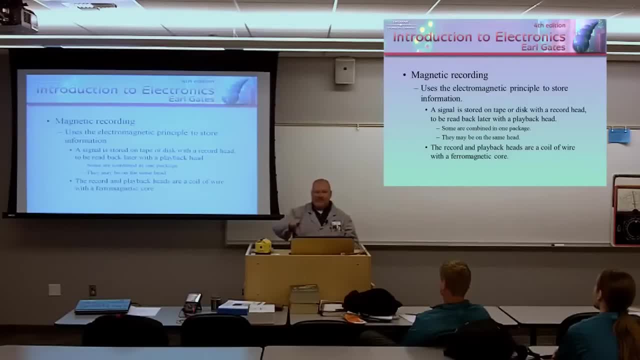 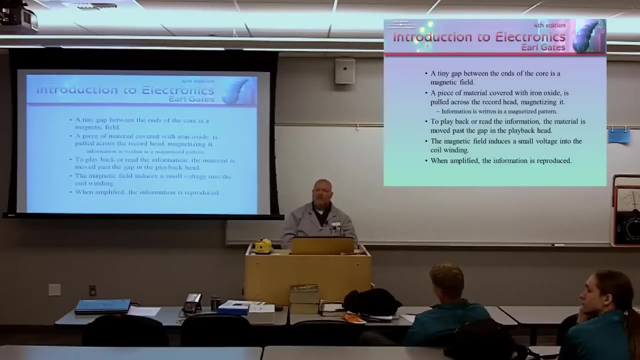 a video production showing that every time they run that tape through the machine they're lessening the video quality of what was on that tape. so videotape, any magnetic recording media, will over time lose its integrity. there's no way around it. yup, if you're burning them. 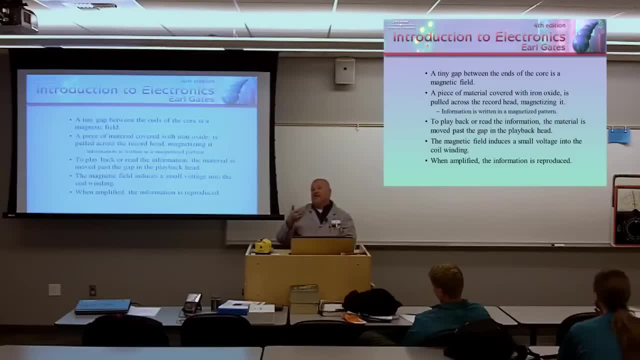 with. basically, traditionally it's not magnetic per se, but over time it will deteriorate. the best method is what's known as actual RAM, like DVD RAM, and that's for archival purposes. you want to do DVD RAM, so that's one of the problems that I actually 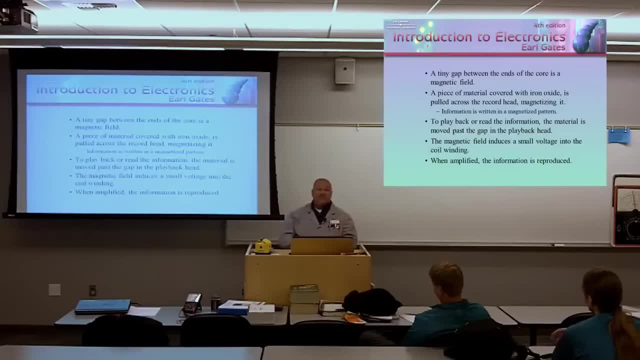 as soon as they had a DVD burner that was on the market. that was reasonable, like VHS to DVD, because when my kids growing up I shot a lot of home movies and stuff and over time I knew those tapes were going to diminish. every time I watched them those tapes were going to diminish. 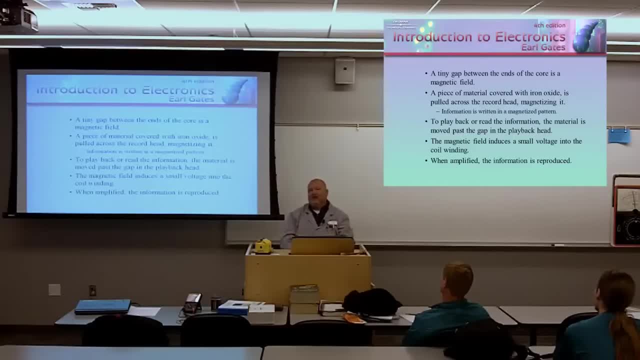 so I got them and then transferred them. but to be honest with you, I should have transferred them to DVD RAM and it's kind of a niche thing, but that's going to last the best and it won't experience degradation, all these other forms of media, even if you're burning. 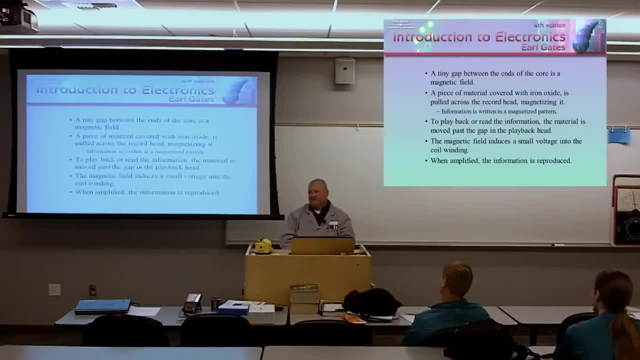 your own DVDs. they will degrade over time. so the way that magnetic tape works, that tiny gap between the ends of the core is a magnetic field. a piece of material covered with iron oxide, basically iron filings, is pulled across the record head, magnetizing it. information is written. 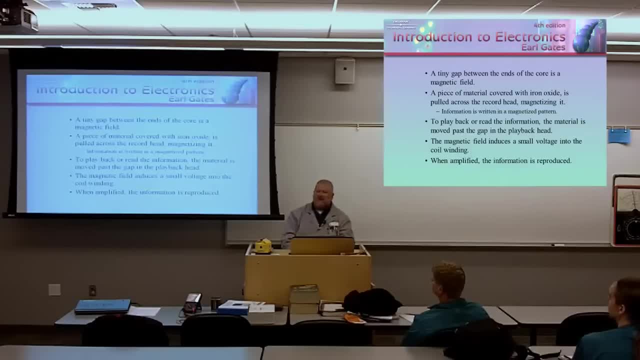 in a magnetized pattern to play back or read the information. the material is moved past the gap in a playback head. the magnetic field induces a small voltage into the coil winding. when amplified, the information is reproduced, and this really revolutionized the recording industry, being able to. 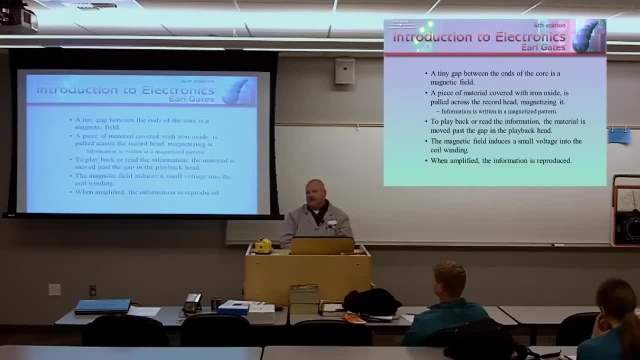 I mean, I remember back in the day I'm dating myself, but wow, could I actually own a cassette recorder and I could speak into a microphone and record my voice on magnetic tape and then you could put it in at a later date and hear yourself. wow, that was really the big deal. 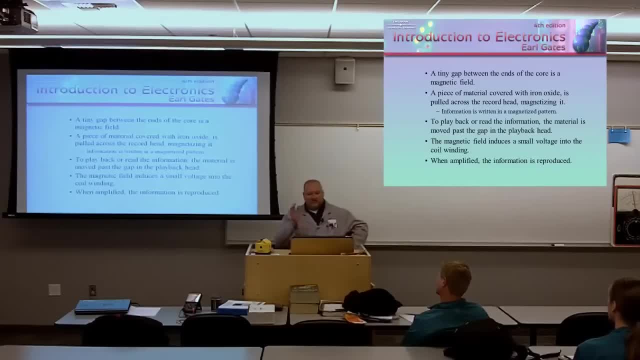 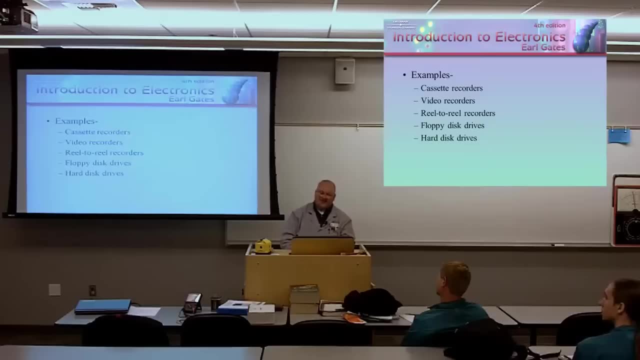 now we have cell phones that we talk into and digitally record that. examples that used this technology on tape would be cassette recorders, video recorders, reel to reel recorders that were used in a lot of production studios, and such floppy disk drives. floppy disk drives is nothing more than a 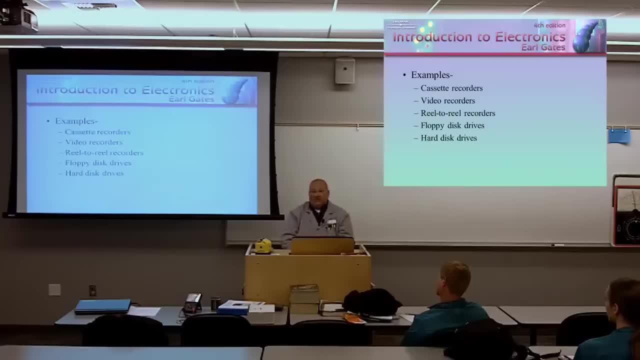 disk with particle on it, with iron particles on it and, believe it or not, hard disk drives. if you've got a hard drive in your computer using the same technology, a little bit better- no, a lot bit better- okay, because now you could go out and buy a terabyte. 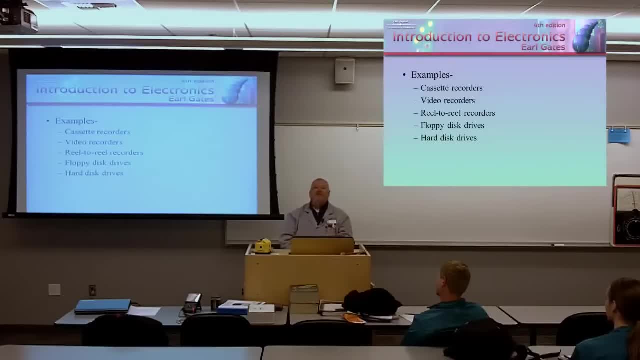 drive for $49 and the reliability of that data is extremely high and if it's properly maintained, you're really not going to lose integrity of that data and that's really, as far as I'm concerned, this is really. that's the best method of storage my wife and I really enjoy. 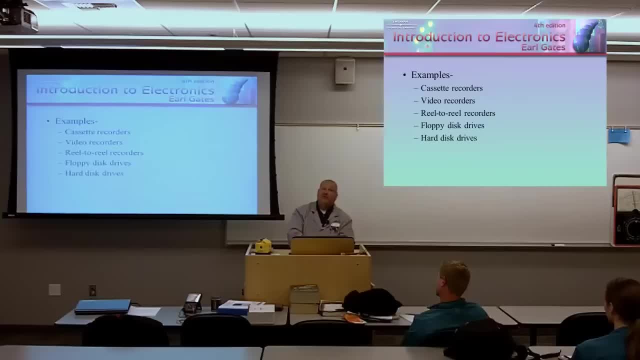 amateur digital photography and when we go out and shoot something when it's on the card, we're at risk as soon as we plug that card in and we copy it to one drive, my primary drive. okay, then what I do is I mirror that on a secondary drive. 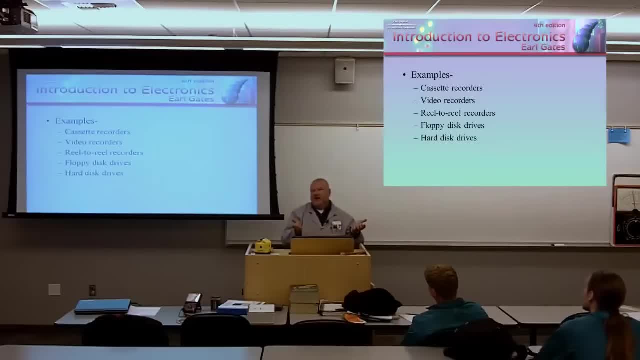 and I mirror that on a tertiary drive and I also pay for a service to go back to that primary drive and back it up off site. okay, let me tell you, in the middle of February, in the middle of February, I fly to Fairbanks, Alaska, minus 23 degrees to see. 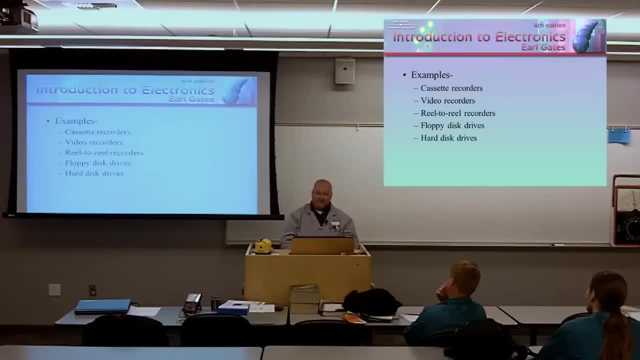 the Aurora Borealis to get some pictures. I don't want to lose those pictures because my hard drive fails, so I want to make sure I have backups to backups to backups. so as long as you do that, you're good with me just transferring a home movie. 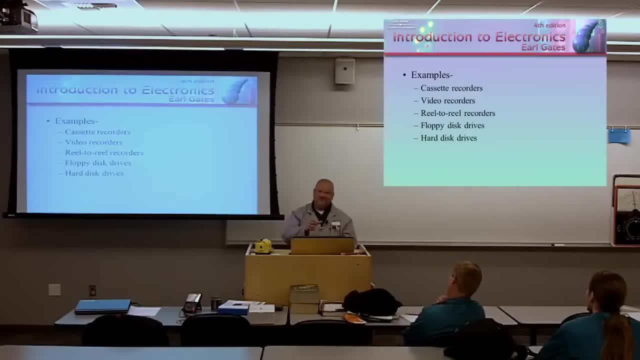 to a DVD, I could lose integrity of that over time. if it's backed up digitally on a hard drive and you could again mirror that, then you're good. DC motor operation depends on a principle that a current carrying conductor placed in and at right angles to a magnetic 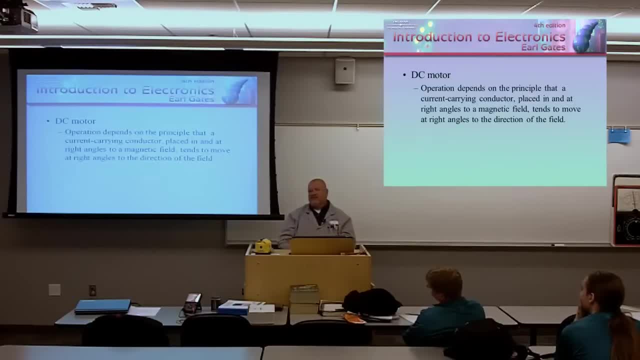 field tends to move at right angles in the direction of the field. basically, what we're saying is: if we could rotate a shaft and create DC, why can't we apply a voltage to a winding and create motion? so the difference between a DC motor and a DC 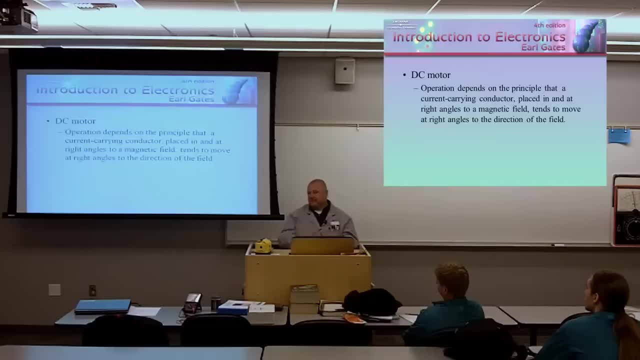 generator is perception. most cases they could be used either way. it's actually one of the things that they use for power management over at the Grand Coulee Dam. I don't know if any of you go recreating over in central Washington. you ever go camping or anything out there. 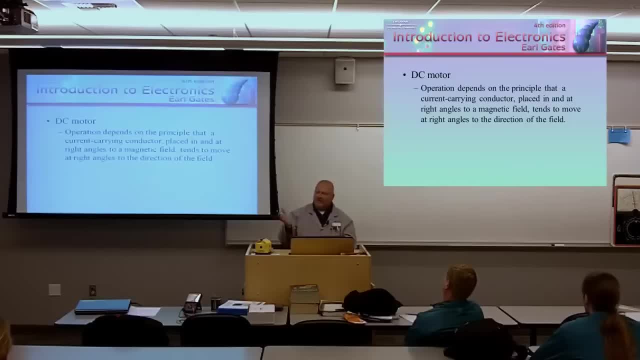 it's really amazing if you have a chance to go out there. this is stuff again they were thinking about in the early 1900s. you got the Columbia River. they built a dam on it, not just any dam- the Grand Coulee Dam- and what they did behind the dam. 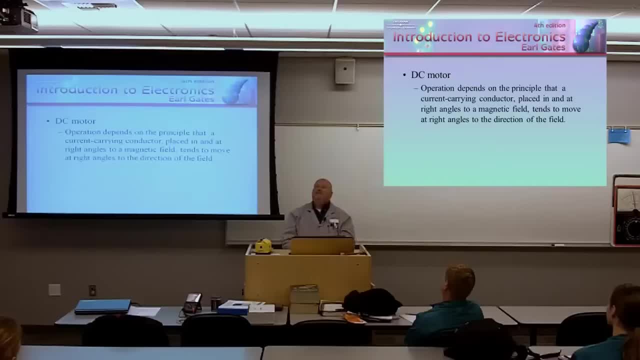 is they created Lake Roosevelt for the purposes of irrigation and to store energy- to store energy during low demand times. what they did is they have the generators. you can't stop the Columbia River. it's a river. you're going to kill all the fish, so you can't just shut the river off. 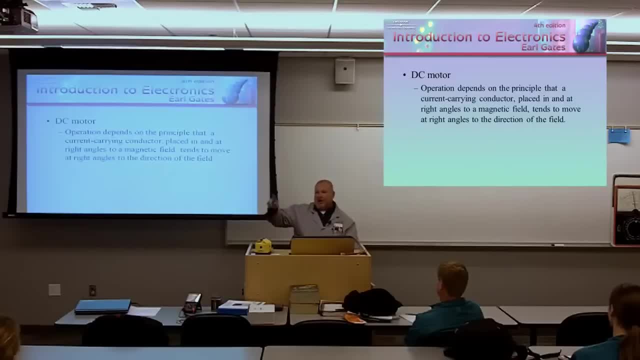 you got to keep the water flowing, but if it's low demand time, get that. harness the electricity. then with the electricity drive pumps, drive pumps and they pump the water from Lake Roosevelt up to Banks Lake. Banks Lake, very popular for water skiing and recreating. Banks Lake goes to feed 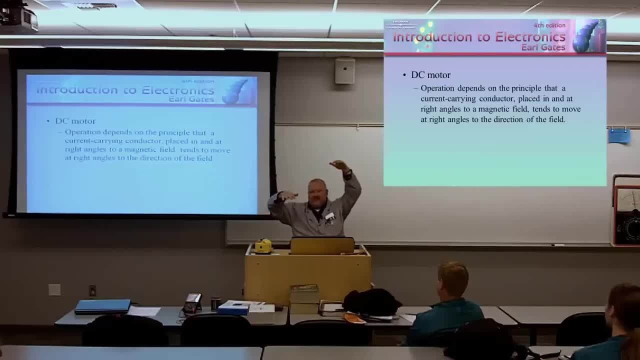 agriculture and then, during peak demand times, what they could do is turn it backwards and catch the energy flowing back to Lake Roosevelt, producing energy, and then catch it falling back into the Columbia River and harnessing it twice. so basically, you're using the water to store the energy by simply pumping it. 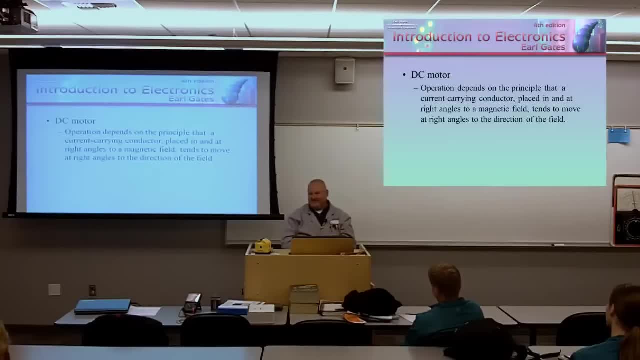 to a higher elevation during that low demand time. brilliant, brilliant. and again, they figured this stuff all out in the early 1900s. so that's what they've got between Lake Roosevelt and Banks Lake. basically are motor generators that you can turn either way and either turn it. 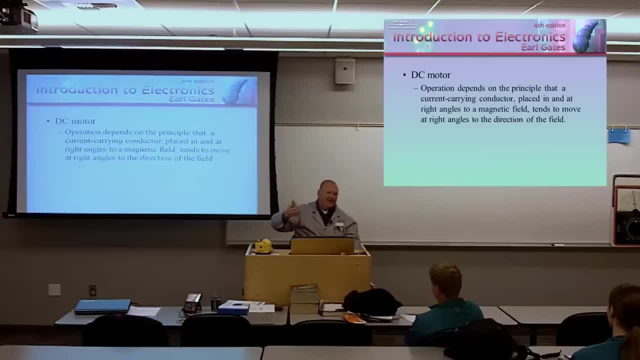 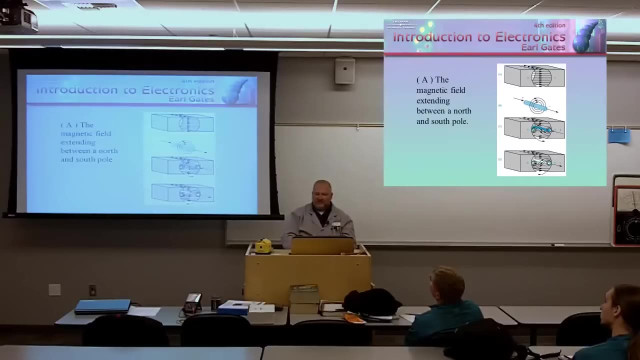 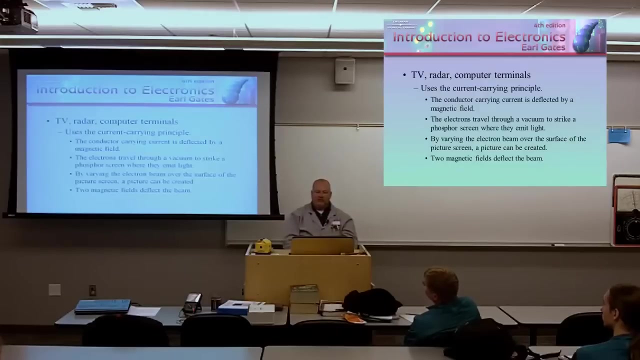 backwards, pump the water up or catch the water falling and generate electricity, and this is simply the process of creating a magnetic field that attracts and opposes, and creating motion. instead of motion being used to create a magnetic field, now we're harnessing the magnetic field to create motion with a DC motor. 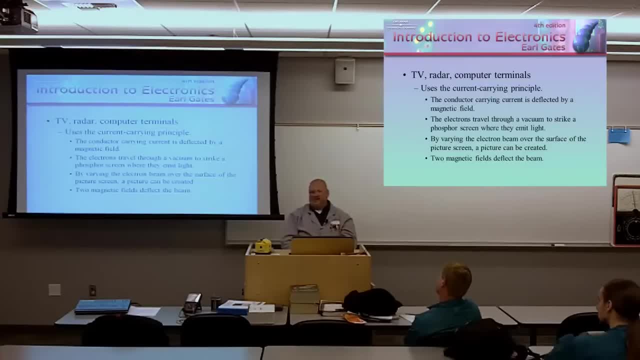 another area that uses electromagnetic fields: TV radar, computer terminals. what we're talking about is the old school monitor like that. old school monitor like that. basically, in the back of a monitor like that there's an electron gun. so you get to go home tonight. what did you learn about in school? 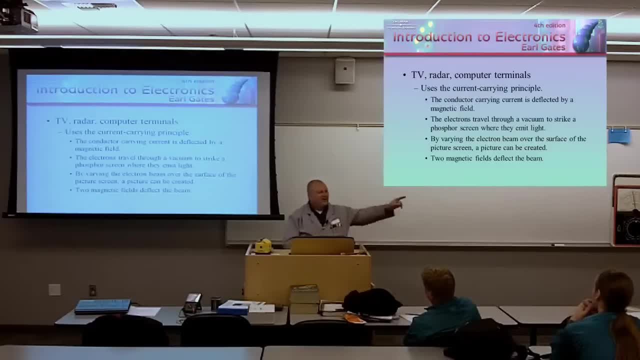 my instructor was talking about them, their electron guns. now, an electron gun basically sits in the back of a cathode ray tube and shoots an electron beam out towards the screen. that electron beam is going to be controlled through deflection windings. the deflection windings are horizontal. 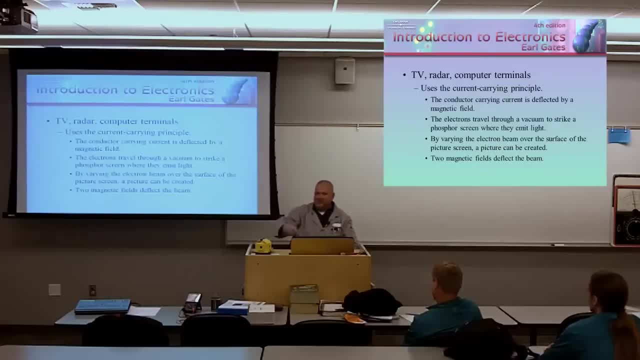 and vertical, and that's what's going to be used to basically paint the image on the screen. it's your x-axis and your y-axis, so that's how we'd use that to paint an image. now with flat screen monitors we're doing things a little bit different, but it's kind of an. 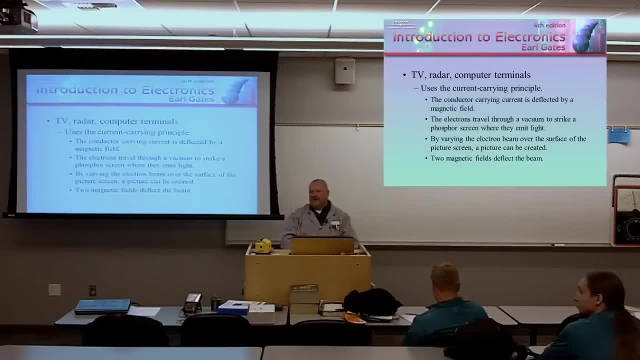 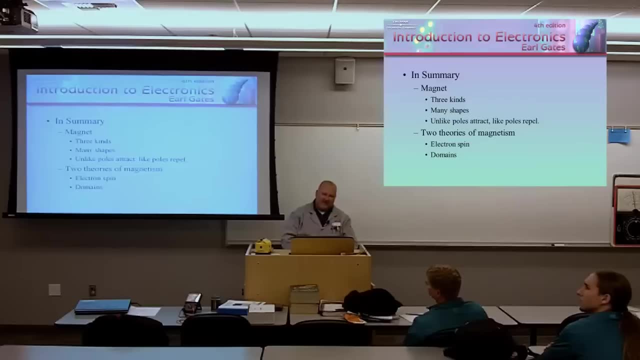 evolutionary process based on what we were doing with that magnetic field. in summary, we talked about magnets, natural magnets, unnatural magnets, artificial magnets and electromagnets come in many shapes and sizes, big thing to remember. unlike poles attract, like poles repel, two theories of magnetism: electron, spin and domains. 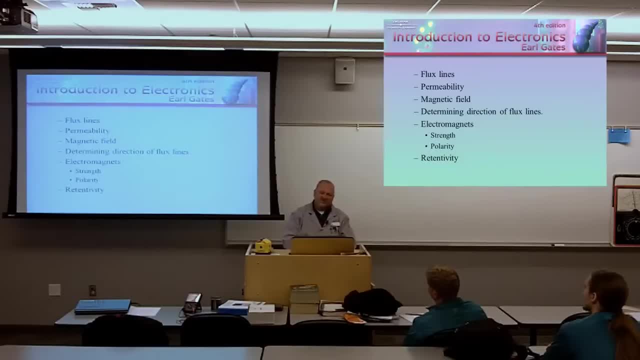 flux lines are those invisible forces that we can't see. you know, this lecture wouldn't be complete if we didn't talk about, you know, anomalies. you've all heard of the Bermuda triangle, right well, science- or science fiction, I mean- they've got some really good hard evidence of. magnetic anomalies that occur there. so if you're navigating solely by compass and you encounter unusual magnetic fields or you're flying an airplane that's again has a gyro compass in it, it could cause problems, big problems, for you. magnetic disturbances there's actually on aeronautical charts. 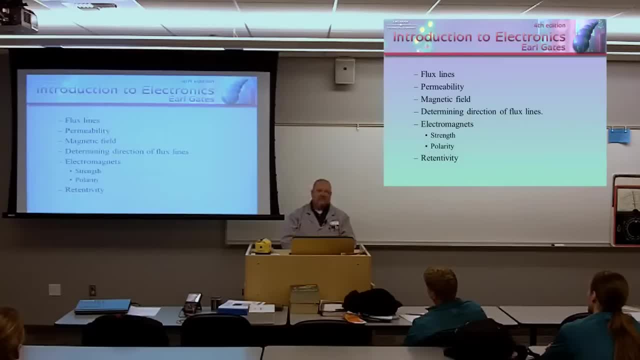 they put down areas that have big magnetic disturbance, areas that they're used to. the Bermuda triangle is one of them. it's actually one of the things that's kind of interesting, too, that I see a lot of these like ghost hunters using is equipment to basically sense magnetic. 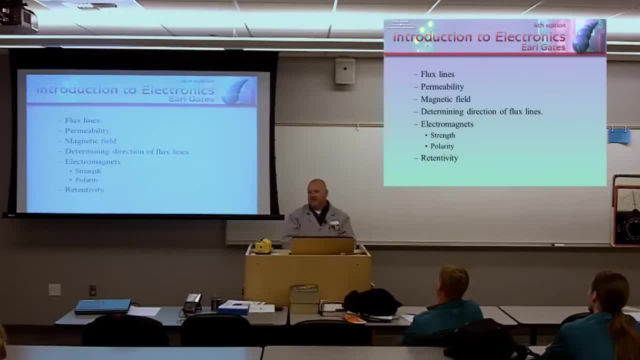 fields and there's, you know, a school out there that basically says that you know, spirits possess this energy and this energy manifests itself as a magnetic field. so if you have sensitive enough equipment- and you know I've, I don't know anybody watch any of those shows on TV. you know I've watched enough that something's. 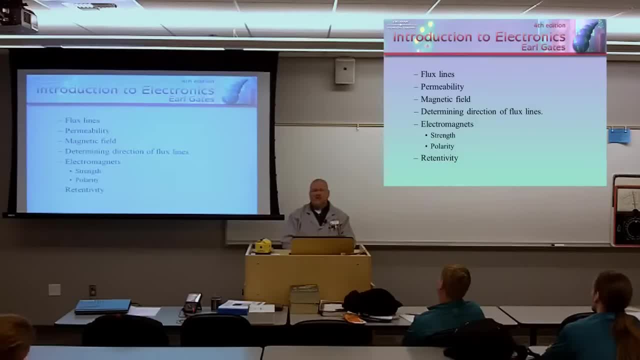 going on. something's going on and actually, quite frankly, I think we're very, we're very naive. if you know, we only believe what we could see with our five senses, you know. so you know, I think there's probably some truth in some of this stuff. we talked about the magnetic field. 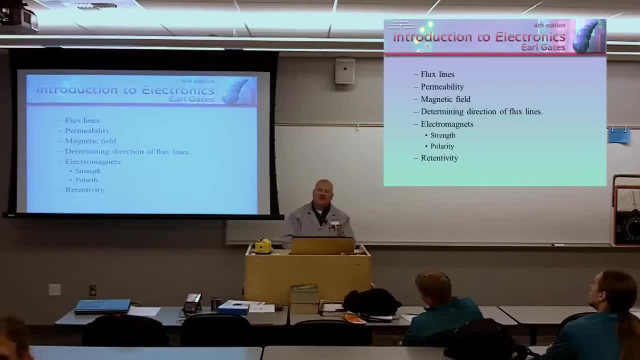 determining direction of flux lines. we talked about electromagnets: strength, polarity, retentivity, electromagnetic induction. we talked about Faraday's law: right, parallel, perpendicular. we not only talked about the left hand rule for generators, but I gave you a specific warning and not doing that in your car, on your drive home. 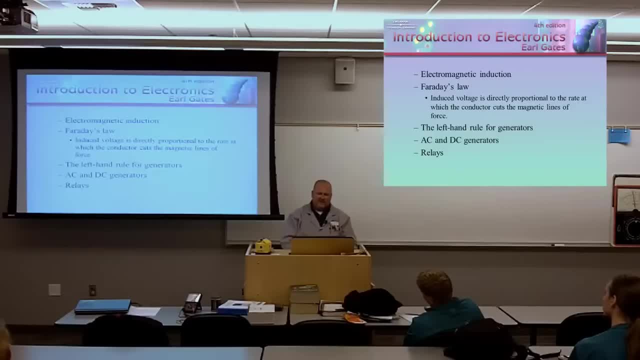 as someone might think you're giving gang signs. we talked about AC and DC generators. big thing to remember about an AC generator: right slip rings. DC generator, commutator. AC generator makes a wave that's half positive, half negative. DC generator makes pulsating positive waves. relays basically. 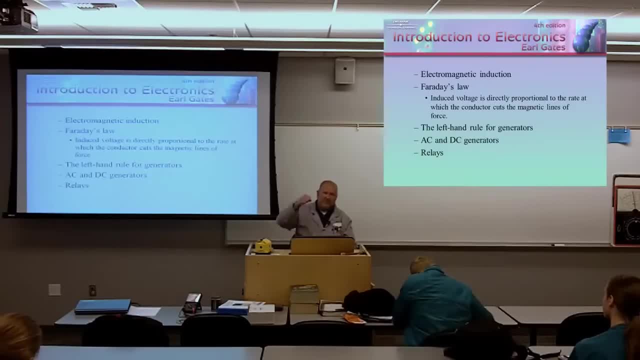 electromechanical switches, a moving armature or a series of ganged armatures, contacts on armature. we talked about how we could use this for doorbell solenoids, phonograph pickups, loudspeakers, magnetic recordings, and then, finally, we talked about DC motors and yes, 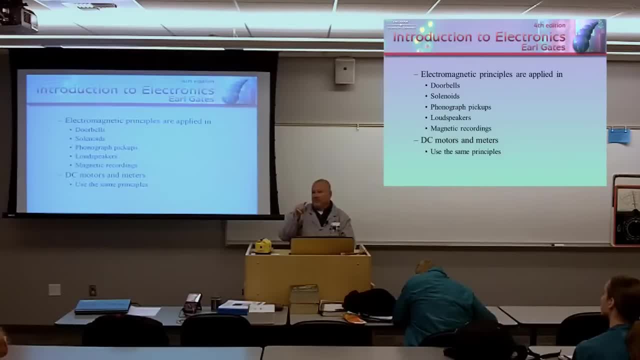 meters- that DRs involve meter movement is nothing more than a permanent magnets and a coil. when you pass current through that coil, you either attract or oppose, causing the needle move. and then, finally, we talked about the electron beams created by electron guns, which are in the back of a CRT. 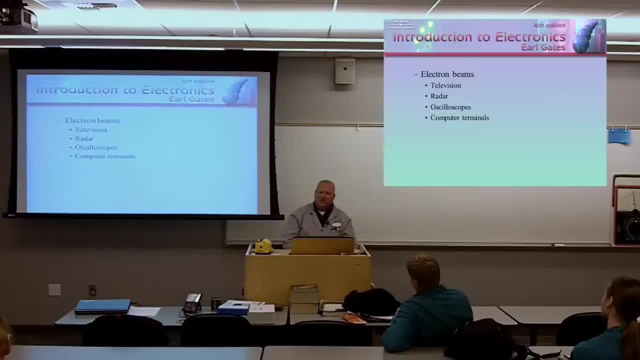 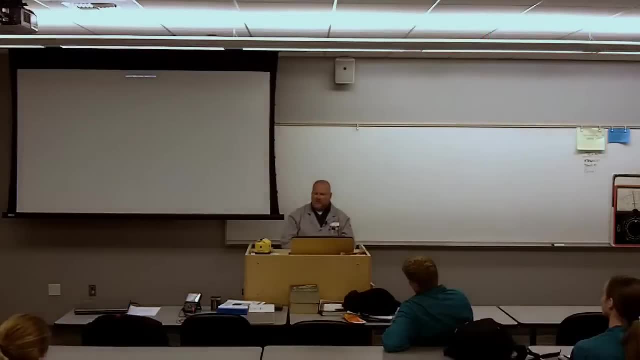 that's how we used to create television signals, radar displays, oscilloscopes and computer terminals. anybody have any questions on anything that we covered in this chapter? there's a lot of new terms. to familiarize yourself with this: less math, more remembering new terms question. this doesn't have to do with this topic, but do. 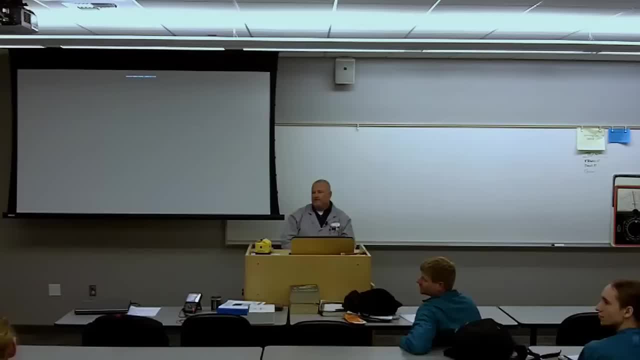 flux lines in here have anything to do with the flux capacitor and that kind of stuff. I have the flux capacitor in back to the future. I have no idea what that is and I probably wouldn't recognize it, you know, if I saw it. so, um yeah, there's no reference. 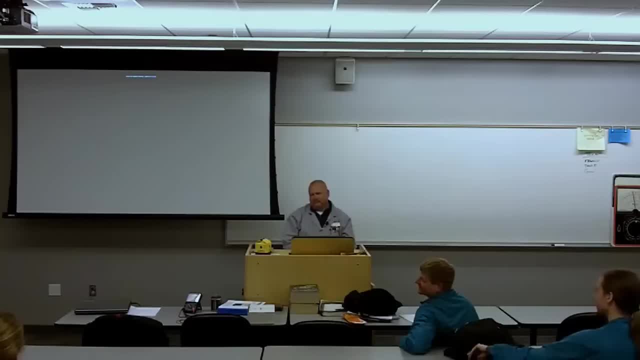 to the flux capacitor. it's just a completely made up thing that they came up with. huh, pretty much. I don't know if there's any Wikipedia references to it. you know could be a fun project to try to build one. I reckon laughter. I was just wondering. 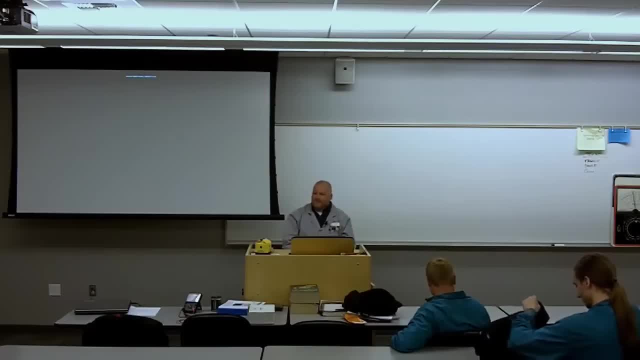 you know, you know electron beams. well, you guys are stumping me tonight. laughter. I don't know. that's what they've always caused. yeah, it should be like an electron beam tube cathode, ray tube cathode sends out an electron ray and it's a vacuum tube cathode. 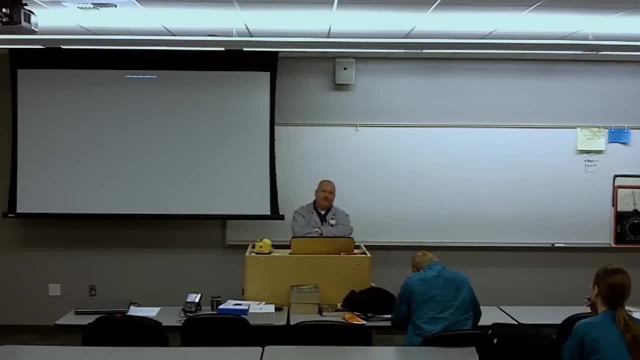 ray tube, electron beam, I don't know? got me good question. yeah, let me tell you, if I was the pope of electronics, all of this stuff would have been called something easier, simpler, laughter. some of this stuff, you just gotta hit the I believe button but suffice to say like, say, magnetism, it is really. 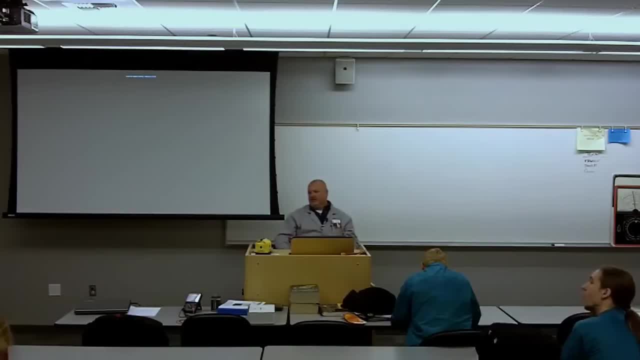 really critical. um, that's actually one of the things, too that I don't know if you, um, I can't confirm or deny, but the movie Hunt for Red October you know? um, that was basically a hydro dynamic drive that was based on magnetic field, and um, you know, you could look at that and say science. 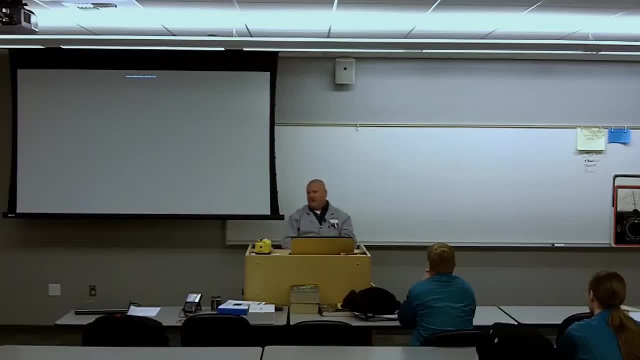 fiction, science or science fiction. I of course, cannot comment on it. um, but if you research that type of technology, the Japanese- and the Japanese, of course, is an island nation- they're very dependent and always have been dependent on trade. they've played around with that technology on. 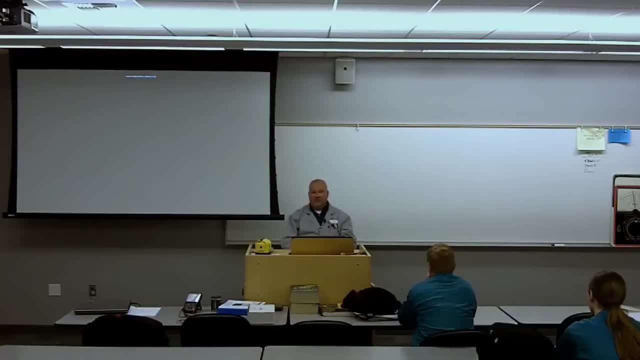 barges to see if they could, you know, move a barge using this. you know hydrodynamic drive system and, um, you know again, it's not mainstream, but they've played around enough with it. so I heard that, yeah, I would think that it might be possible to think it's really silent. 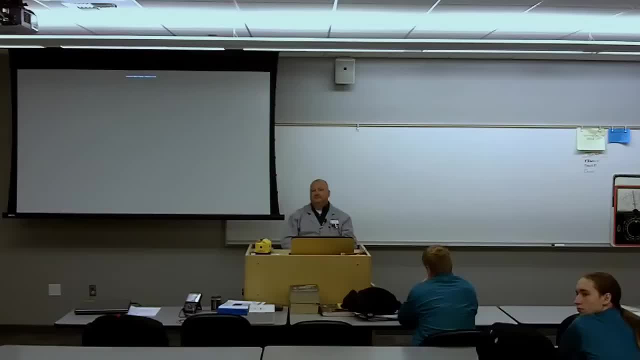 but it's basically setting up a flare in the magnetic field because it's creating some huge magnetic disturbance that is not going to make disturbance anymore. and, to be honest with you, um, you know, and I haven't- I haven't rode a nuclear submarine in over 20. 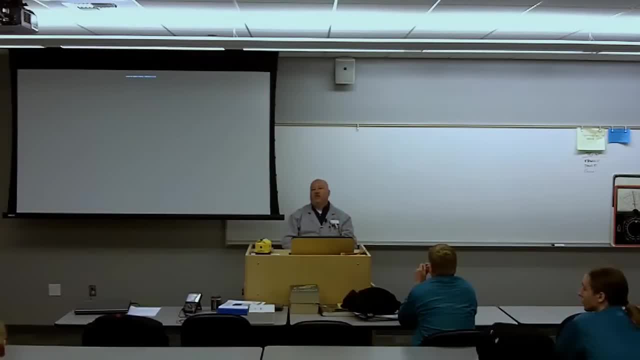 years. um, I know that we had submarines out there that were so quiet you wouldn't hear the submarine. what you would hear is the submarine blocking biological noise behind it. so it's like if you had something big going past your ear. you know something is there because 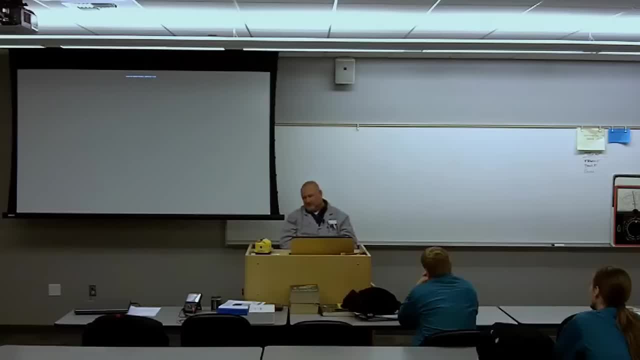 it's blocking the sound. so I mean, that was 20 plus years ago, so we've never had a problem keeping quiet and keeping things real quiet, um, but performance is another issue. so if you want to go fast underwater, you're going to make some noise and that will give a locate. 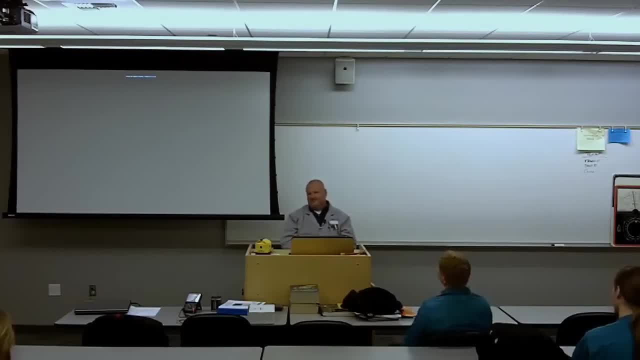 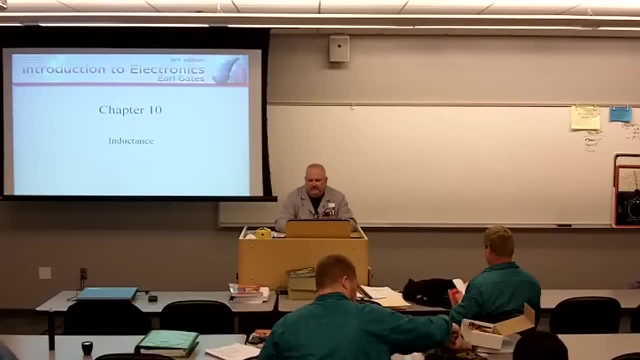 you know, give your tell, basically so, any questions. any other questions comments? concerns: alright, the long anticipated lecture, chapter 10, inductance. this is, uh, this is going to be an unusual property for us to discuss compared to what we've talked about up to this point. 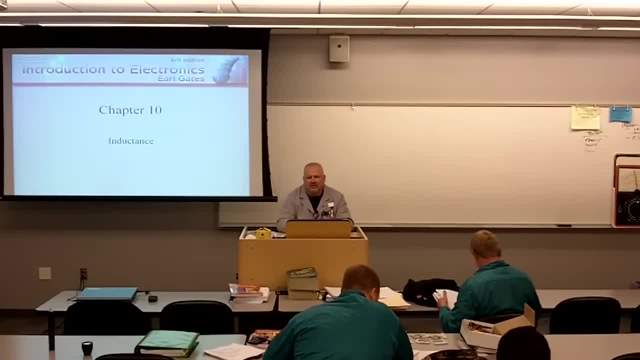 what we've talked about up to this point really is conductance resistance period. in discussing inductance, you're going to see that things with inductance change over time. ok, the property actually changes. the influence it has in the circuit changes over time. so you're going to see that this is uh. 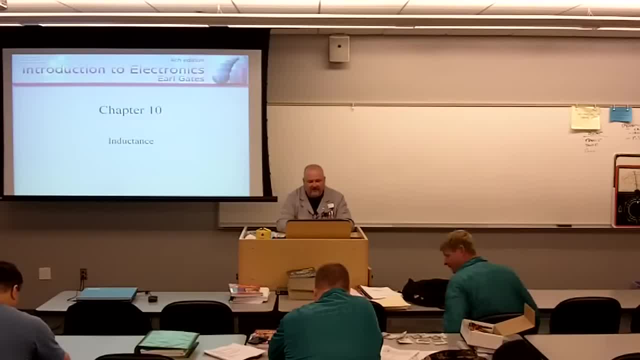 very dynamic, literally dynamic- component and property. chapter 10: inductance. after completing this chapter, you're going to be able to explain the principles of inductance, identify the basic units of inductance, identify different types of cores, determine the total inductance in series. 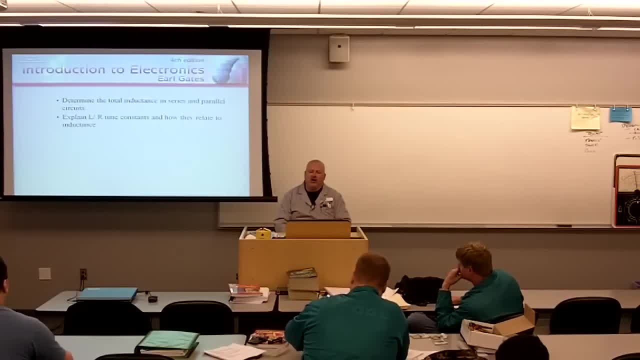 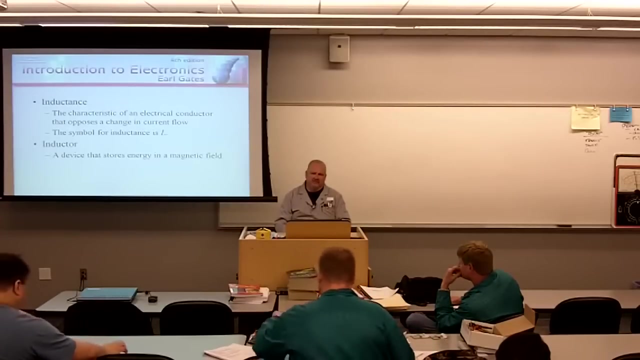 parallel circuits. explain LR time constants and how they relate to inductance. now, the property of inductance is that characteristic of an electrical conductor that opposes a change in current flow. opposes a change in current flow. ok, the symbol that we use is the capital letter L. 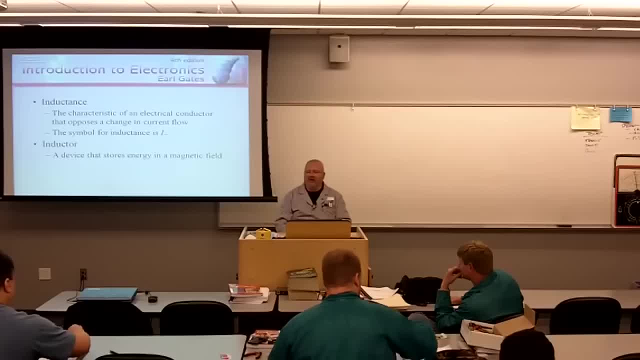 so in a circuit, if you see on a schematic diagram, L equals. that means inductance is equal to whatever specific amount is identified. now. an inductor is a specific device designed to possess this property of inductance. an inductor is a device that stores energy. 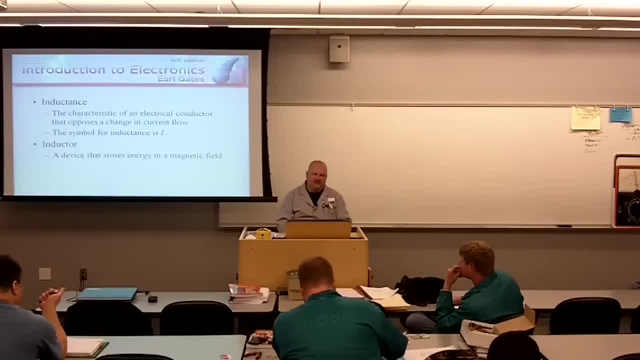 in a magnetic field, and it's important for us to understand this property because we're going to counter this next chapter when we talk about capacitance. right, I'll let the cat out of the bag. capacitance is an electro static field. inductance is an electro magnetic. 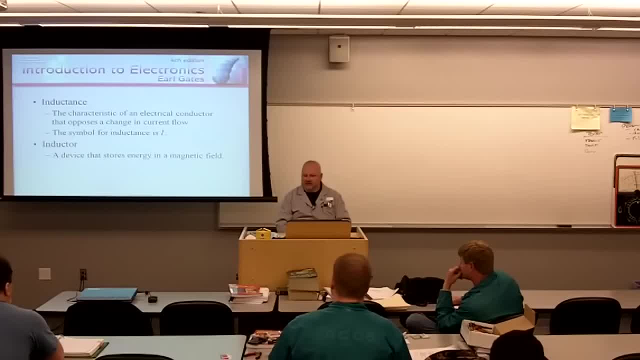 field. that's what's the magic behind an inductor. now, once current is moving through a conductor, inductance helps to keep it moving. as the magnetic flux lines build up, they create an opposition to the flow of current, an opposition to the flow of current Lenz's. 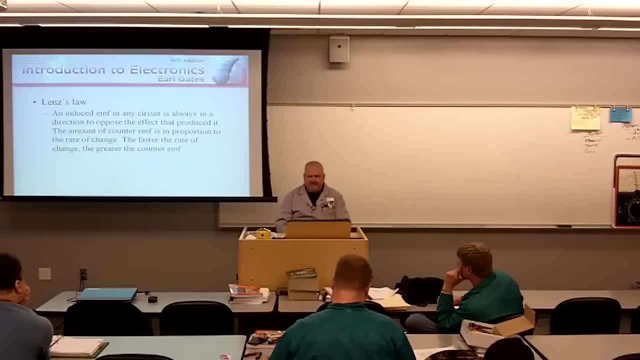 law talks about that. Lenz's law states: an induced EMF in any circuit is always in a direction to oppose the effect that produced it. the amount of counter EMF is proportional to the rate of change. the faster the rate of change, the greater the counter EMF. 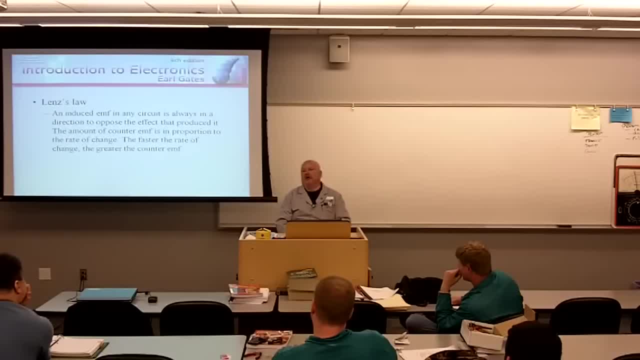 so what this means. let's go back last chapter that we talked about. remember magnetism. remember when we pass current through a conductor, we create a magnetic field. Lenz's law says if the current was going that away, it's going to create an electro magnetic field like this: 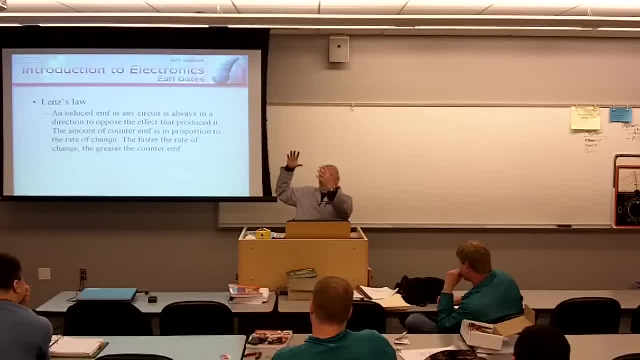 make sense. if we shut the circuit off, that electro magnetic field is going to collapse and it's going to produce a counter electro motive force that goes that way, the opposite way of what created it. so if the EMF goes that way and it creates some magnetic field like this: 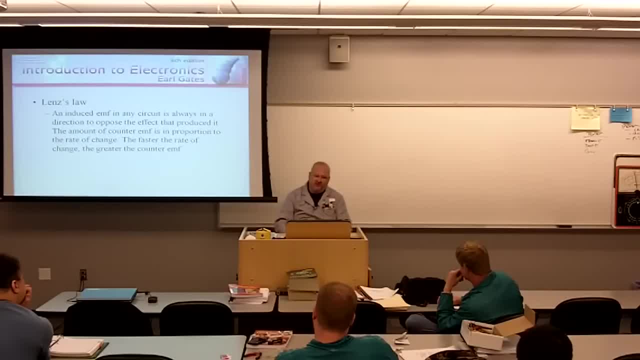 magnetic field collapses, it creates a counter EMF that goes in the opposite direction. so the second part there talks about the rate of change. the faster we turn that on and off, on and off, on and off, expand collapse, expand collapse, the more. the faster we do it, the more pronounced 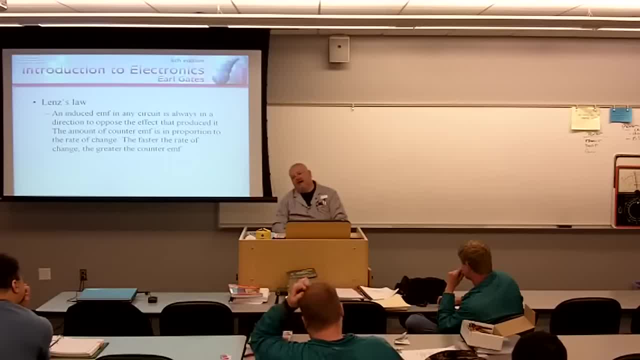 that effect is going to be if you connect one of these- one of them there inductors- to a DC circuit. it's going to happen once when you close the circuit and energize it and when you de-energize it, that field is going to collapse and create that counter current. 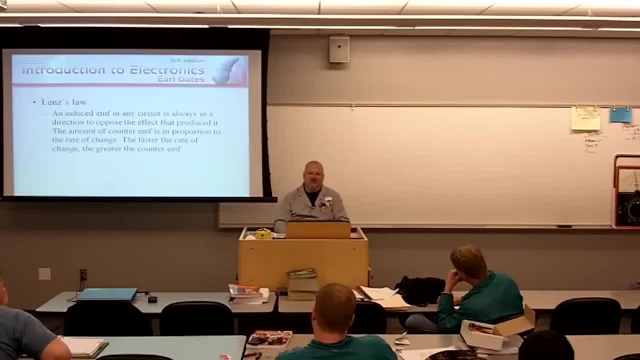 so it's only going to happen once. it's going to expand once and it's going to collapse once. now I'm going to let out a little secret, because you guys have all read ahead: AC: what's one thing that's constant about AC? it's constantly. 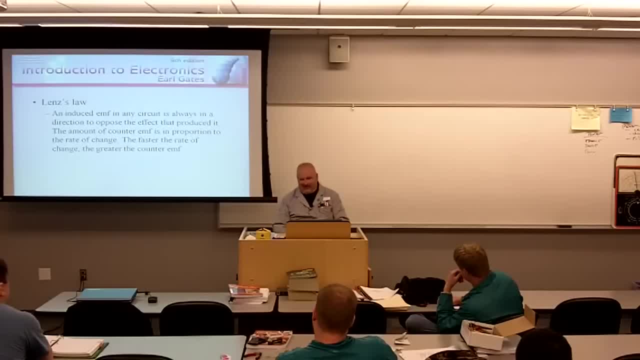 changing. very good, constantly changing. so the higher the AC frequency is that we apply to one of these devices, the more pronounced this effect is going to be. does that make sense? goes back to Lenz's law and again, anytime that in class I say anything about a law, 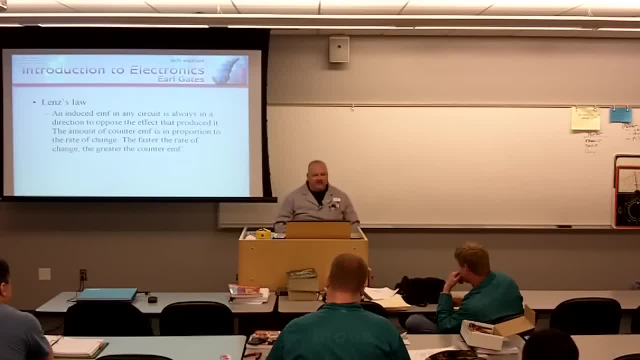 we should like ring a bell. dim the lights, hit some chimes. you know, you know. hit a gong because laws you can take to the bank. you answer a question on your quiz using a law. on an exam. using a law, you approach a project or a lab assignment. 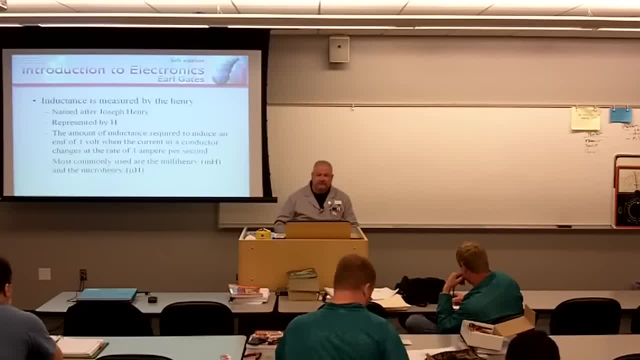 using a law, you're going to get good results. now, inductance is measured by the Henry, and this was invented by a guy whose name was George, a guy by the name of Joe Henry, my main man. Henry, ironically, is abbreviated with the letter H and one. 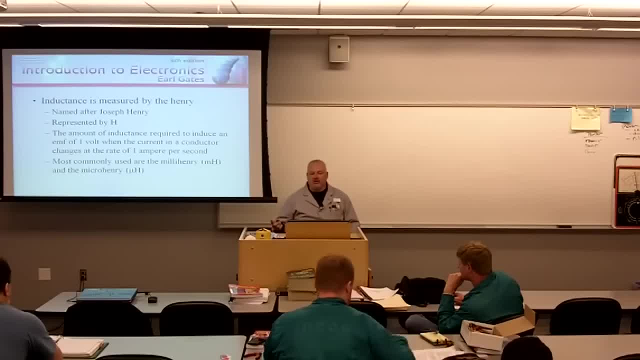 Henry is the amount of inductance required to induce an EMF of one volt when the current in the conductor changes at a rate of one amp per second. so one Henry is equal to one volt of EMF at one amp per second. one is equal to one over. 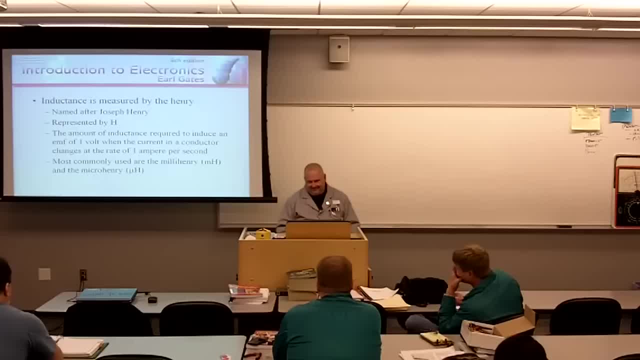 one over one second. now, in electronics the typical values that we're going to see will be the milli Henry times ten to the negative. third, the micro Henry times ten to the negative. sixth, in some high power applications you may see Henrys, but generally speaking, most of the stuff that we're working with in micro 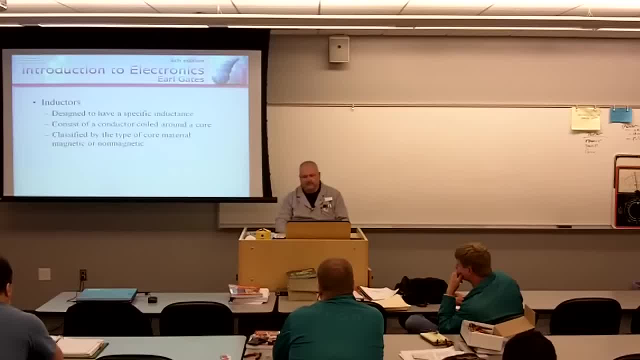 electronics, milli Henrys, micro Henrys, now, inductors are those specific devices designed to possess the property of inductance, so they're designed to have a specific inductance. that's why come they be invented. they consist of a conductor coiled around. 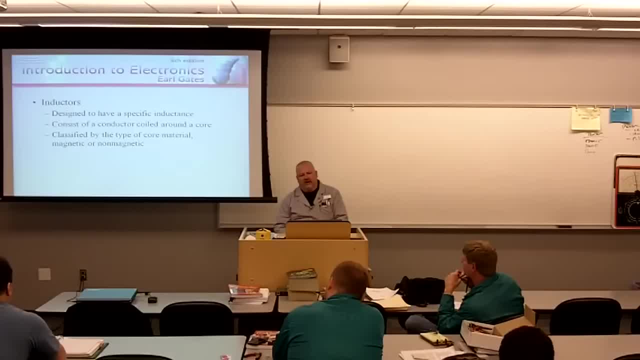 a core. remember: if we got like X amount of magnetism by creating one turn, how much would we get if we make two turns twice as much? it's that simple. it's easy. math consists of a conductor coiled around a core and it's classified by the type of 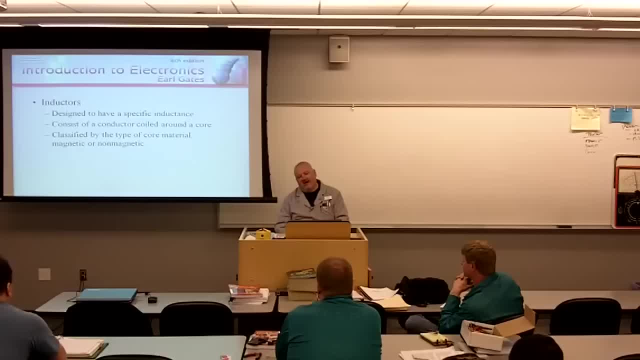 core material, whether it's magnetic or non-magnetic. if we use a magnetic core material we're going to get a higher amount of inductance out of it. if we use non-magnetic, we're going to get a little bit lower out of it. so sometimes they'll use that core material. 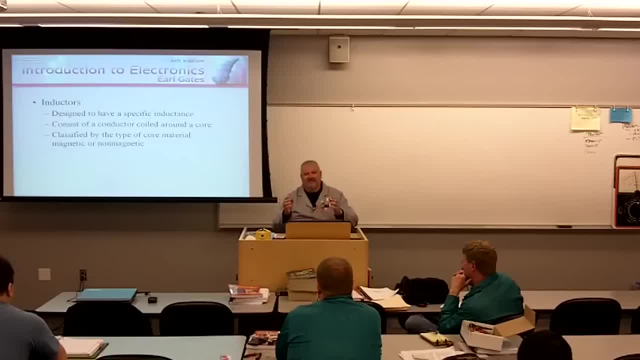 to get it just: not too much, not too little, but just right. this is the schematic diagram for a fixed inductor, and for those of you out there that want to go home and roll your own, you could do that. you just need magnetic wire. magnetic wire is basically. 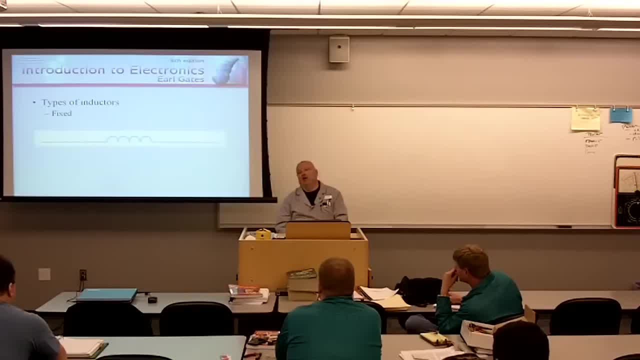 thin copper wire, solid core that has a lacquer coating on it. if you've ever looked into a transformer or a motor and you see the windings, that's magnetic wire. it's all you need. some cases you don't even need magnetic wire because you could. 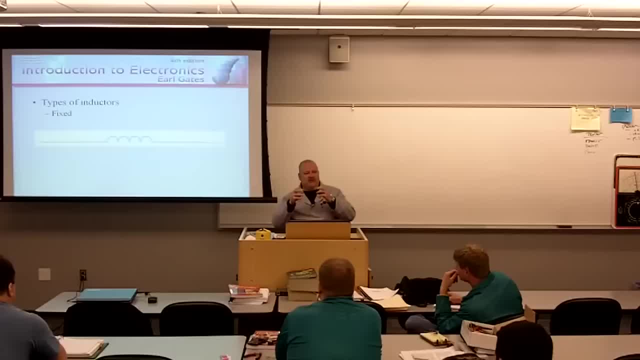 roll a coil and as long as the wires aren't touching each other, you're using air as an insulation. you could roll your own. I've been known to roll my own on a few times with mixed results. I have no idea what I'm talking about. actually, I know exactly. 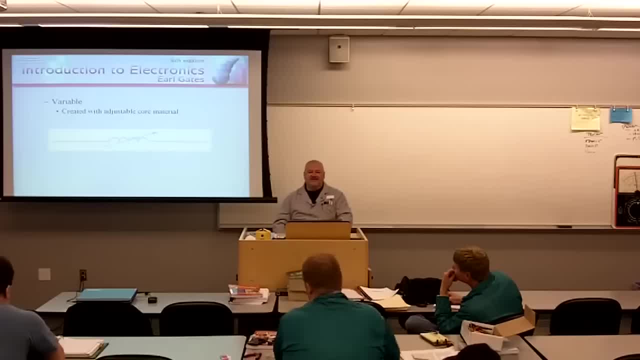 what I'm talking about. this is a variable inductor created with an adjustable core material. now, the way they come up with this is pretty fascinating. what they'll do is they'll get a ferromagnetic core material, typically like powdered iron, and then they basically form it into a material. 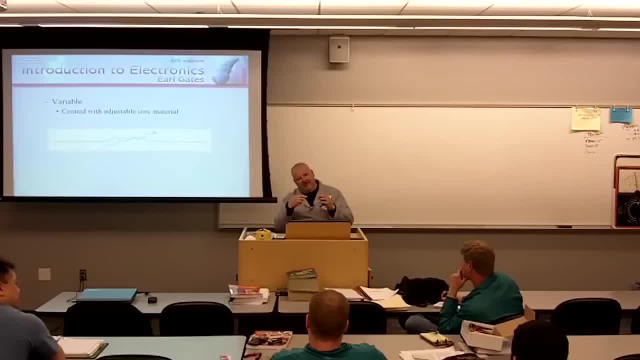 press it into a material, and then they thread it, and then they thread the center of the core, and what you could actually do with it is righty tighty, lefty, loosey. screw it in. and as you screw it in, what are you doing? you're increasing the magnetic 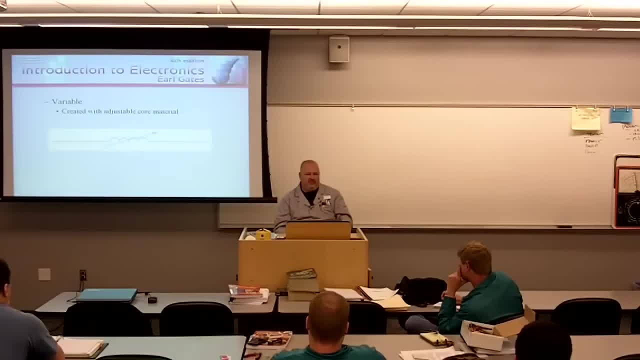 influence of the iron core. so by simply adjusting that, this is used for fine tuning in a lot of circuits that contain these very fine, subtle tuning. another thing that you could do- and I used to see this old school not as much now- they would use a brass insert. 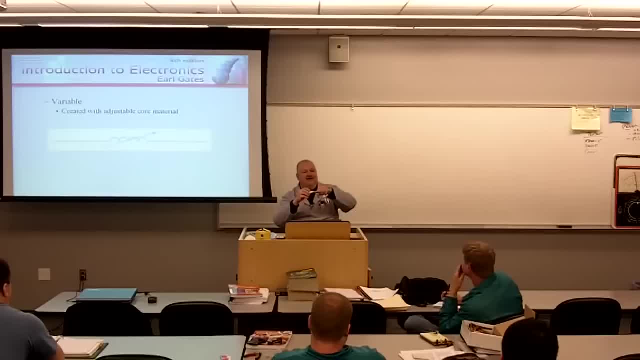 and when you screw brass in, what are you doing? brass has a high level of reluctance, so it's going to oppose that magnetic field. so by screwing it in, you're lowering the amount of inductance. if it was iron core and you screwed it in, you'd be increasing it. 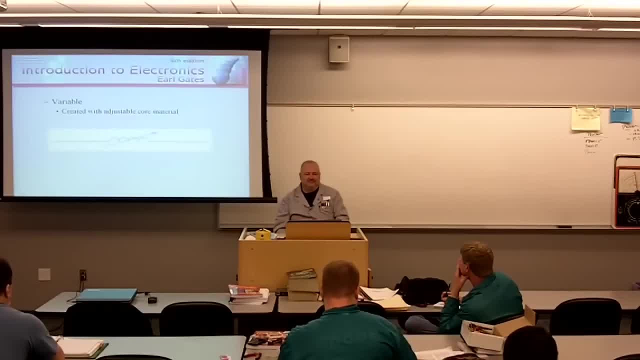 so it's counterintuitive and it gets worse because what would happen is typically the questions that I used to be asked in a lot of my military navy equipment schools. what we would have were circuit card extenders. so what you would do is take the circuit card out, put it in the 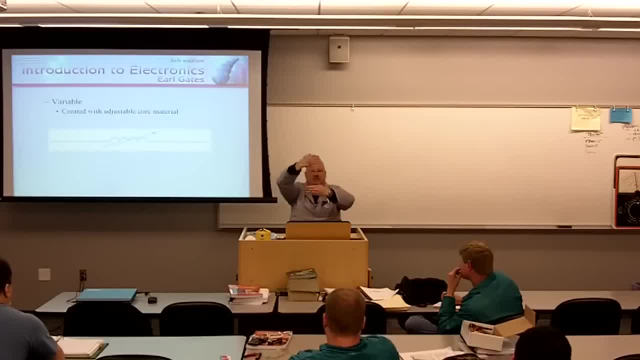 extender and then now the circuit card was was mounted above the rest so that you could get in there and adjust, make adjustments. a lot of times you'd have to make the adjustments from the back side. they'd have a little hole physically in the board that you could put your adjustment. 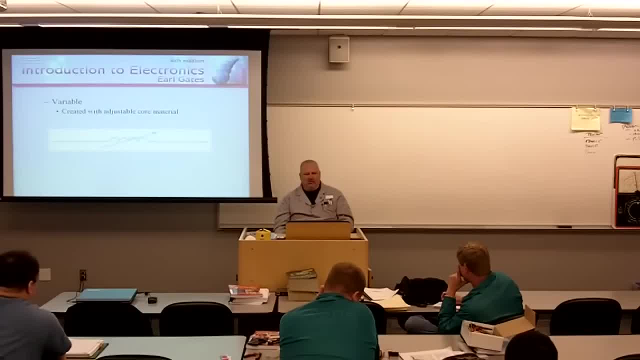 alignment tool in. so then they'd ask if, approaching it from the back side, which direction need you turn the inductor to see a decrease in inductance? so it's one of those things that you know kind of. let's see if I'm turning it. 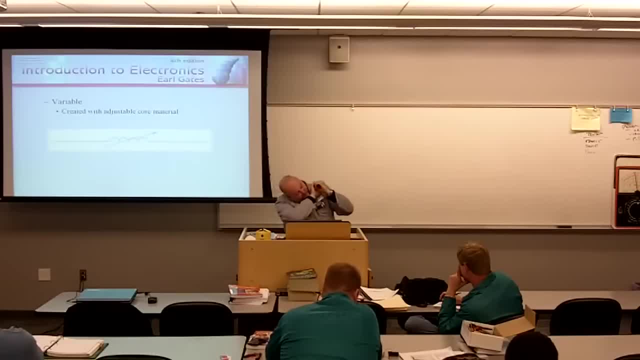 clockwise from the top. that's going to be counter clockwise from the back side, but it's brass core, so as I'm turning it counter clockwise, I'm really moving. I mean, it's just these questions that, like you, thought your head was going to explode, but you know. 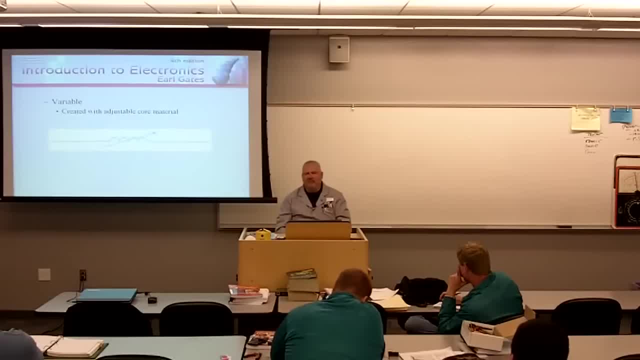 what you kind of had a. well I don't see how that really ever helped me in life knowing that stuff. because basically when you got out to the fleet you put a circuit and you set up your test fixture. basically as soon as you start turning it the wrong way, you see needles go the. 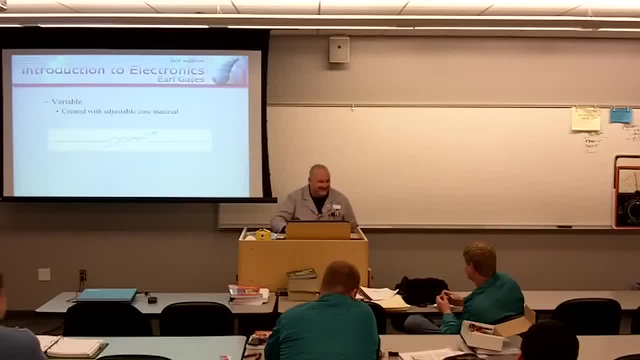 wrong way and you turn it back and you get it to where it needs to be and you're done with it. you don't sit there. well, let's see. if I approach and if I'm using a mirror, I'm actually seeing the inverse. I mean just. 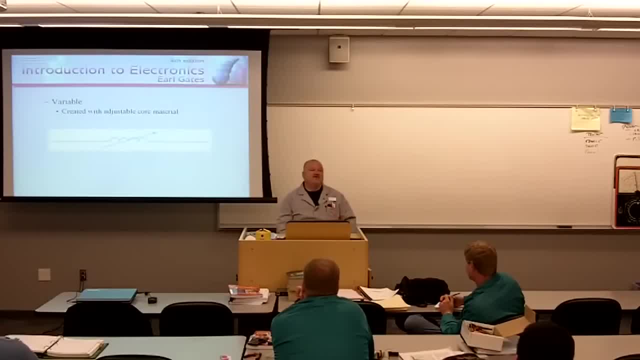 crazy stuff. but think about that because these still- and some of you may work on- some legacy equipment. it's fun to repair legacy equipment, to retrofit, to do things like that, so you may end up finding some of this stuff. this is my personal collection of inductors. 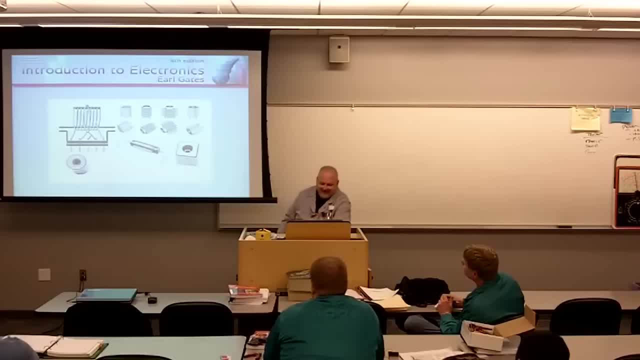 you guys actually believe me. this is an air core inductor, this is a fixed value inductor and that's all it is is just wire wound around a magnetic core. that's all it is. all of these can type here are adjustable and actually, if you could look here, this almost looks like this. 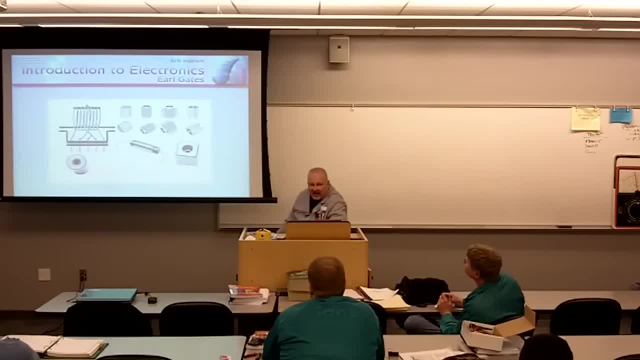 takes a hex head right like an allen, an allen head. whatever you do, don't use an allen wrench to try to adjust this, because typically the allen wrench in your tool kit is made out of iron steel ferromagnetic material. so as soon as you get it in close, 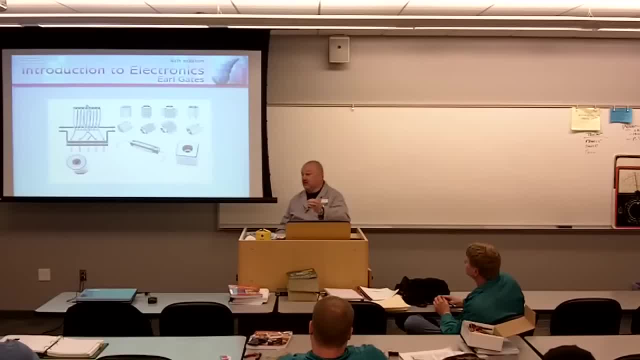 proximity and you adjust it and get it just so you're going to remove part of the magnetic influence and your numbers are going to go cattywampus. so all of these need to be adjusted with non-magnetic alignment tools. I've got a tool roll at home from back. 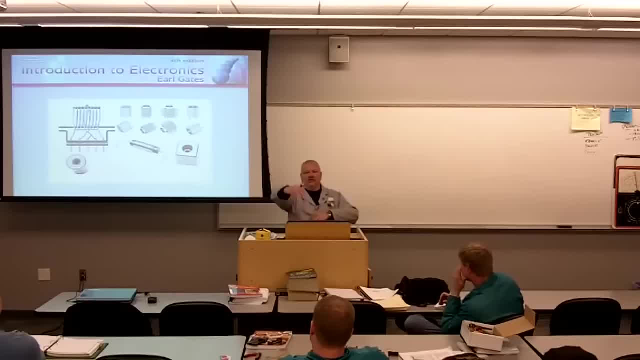 in the day. I should bring it in as an example. it's this big tool roll. it's like every alignment tool known to human kind, and they're basically all plastic heads. the other thing, too, is you stick your hex head in there. you stand a chance of damaging that. 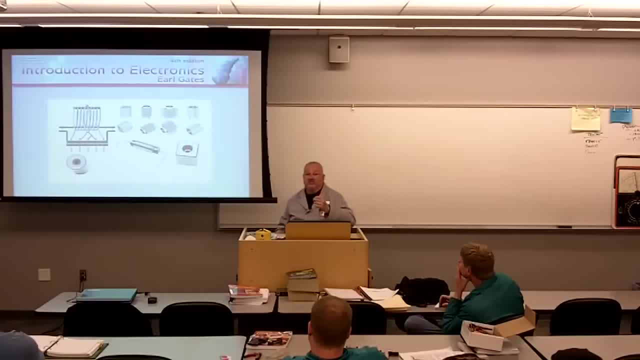 and even if you break off a little bit of material, that amount of material was designed, engineered to be there to create x amount of magnetic field. so you kind of got to get it right. so don't start. if you don't have the right tool, don't touch this stuff. 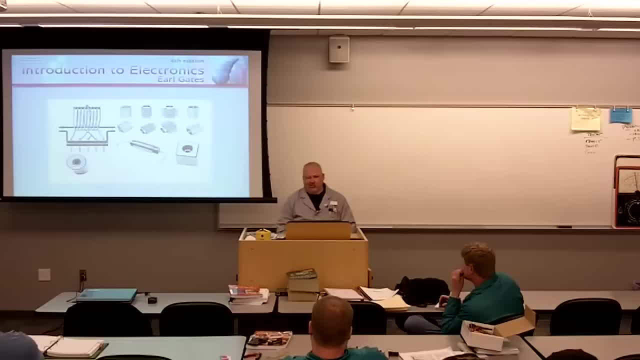 so it's typically called an alignment tool or actually a tweaker in a classical sense of the word- a tweaker- and you could always tell who the technicians were. you know because they'd always have the tweaker in their pockets and you knew it was kind of funny back in uniform. 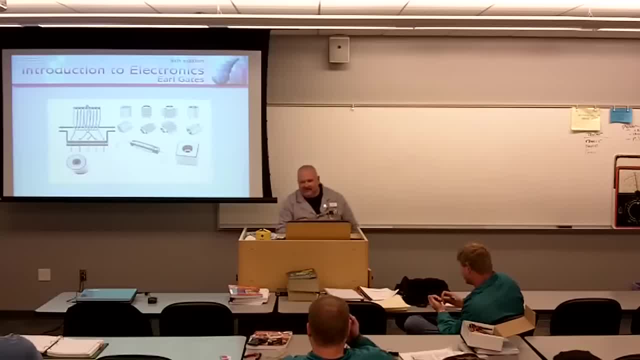 submarine base in Connecticut, I'd be walking around. I'd see you with a tweaker in your pocket, you know, at the deli or whatever, and I knew exactly what you did for a living: the only goofballs running around with tweakers in their freaking pocket. 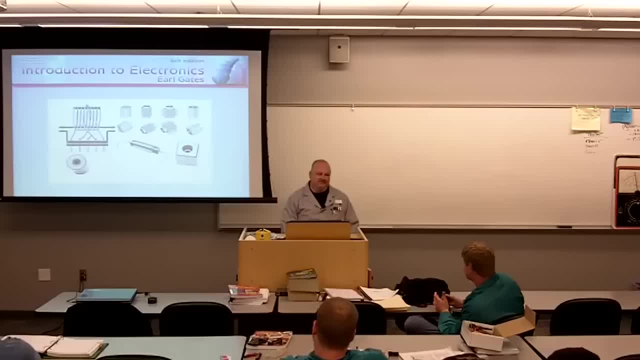 were electronics techs that were regularly aligning equipment. air core: this is an inductor- well, not without core material, because it has air in the core. that's why it's called air core. it's used for values up to 5 millihenries of inductance. 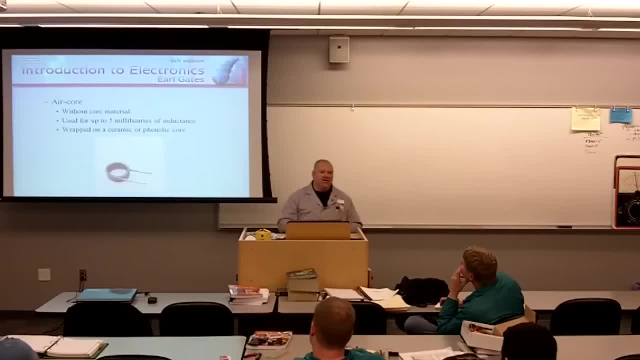 wrapped on ceramic or phenolic core. in this case it was probably wrapped around a dowel or something and then removed and it has form in and of itself. this is actually a really good photograph, because you can see the magnetic wire here and you can see where the insulation 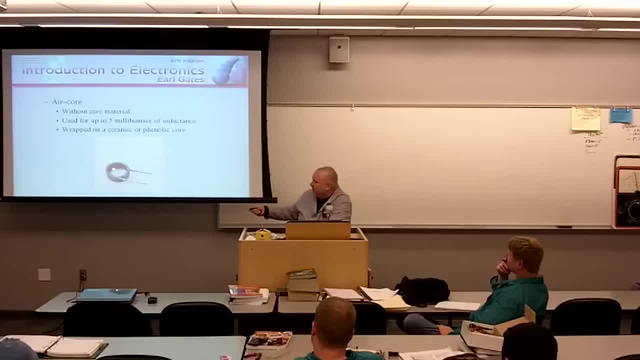 has been stripped. this is bare wire, and then this is insulated. a lot of times people see this and they think that it's bare wire. it's not bare wire, it's insulated. one of the best ways of getting this insulation off if you're going to do a lot of this, 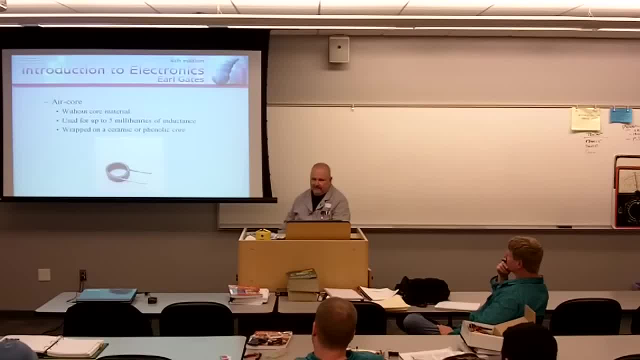 is with a chemical stripper- chemical stripper and basically it's like a thinning agent. you dip it in paint- thinner paint remover- and it removes that right down to the metal and it makes it solderable. you have to put a neutralizing agent on it, but that's the best way of doing it. 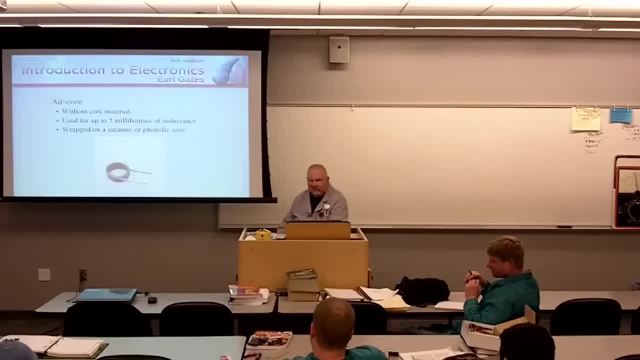 other than that you're going to get your wire strippers and your wire strippers are just basically going to scratch the stuff off. it's not going to, really, because this is a lacquer coating on it, but this is an inductor, believe it or not. just a piece of wire. 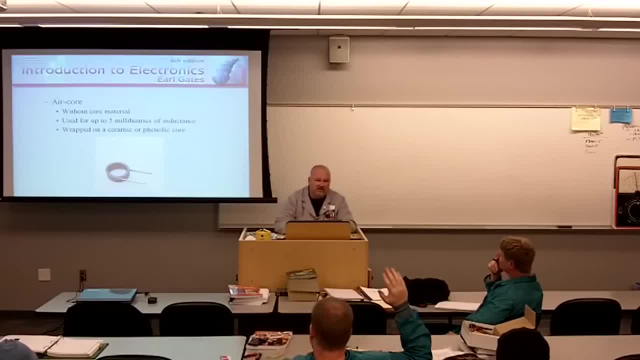 making those five turns. it's going to give you x amount of inductance. might be enough for you to get the job done. on the last air core picture that you had, there was a piece of metal going through it. what's that for this piece right here? 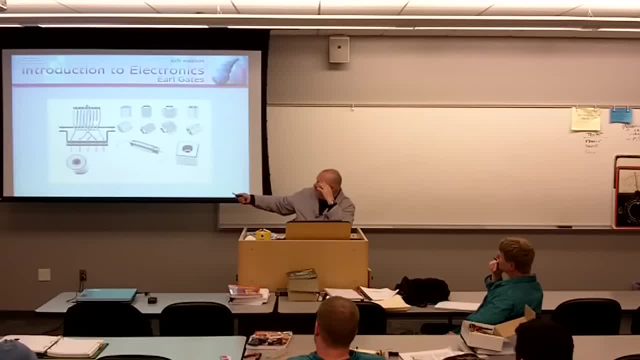 I think somehow this is mounted, this serves as a form, somehow to keep the shape of it. I really don't know. yeah, oh, yeah, yeah, this is not here to influence the magnetic. it's either there for aesthetics or to help the way that's mounted, or what have you. 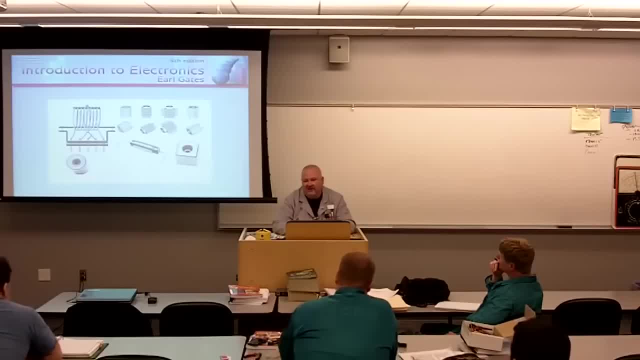 it's a good observation. some of these things are actually pretty cool looking again when you get into some of that older equipment. they made it with a certain level of elegance, you know, and this would be an example of that if you were told in a 1930s radio. 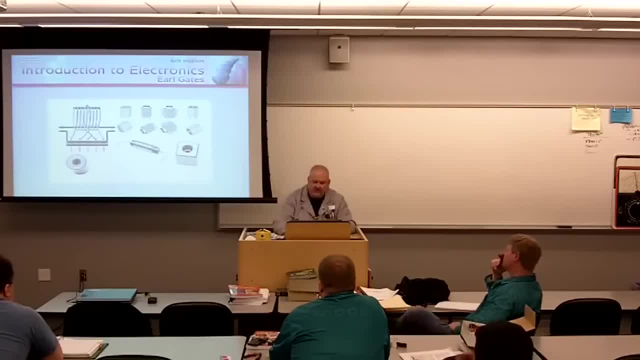 you'd probably find an inductor that looks like that in there 1970s radio. no, you're not going to find that in there. iron core. iron core could be either ferrite or powdered iron. it's a typo, not ion ion core captain. the ion core is melting down. 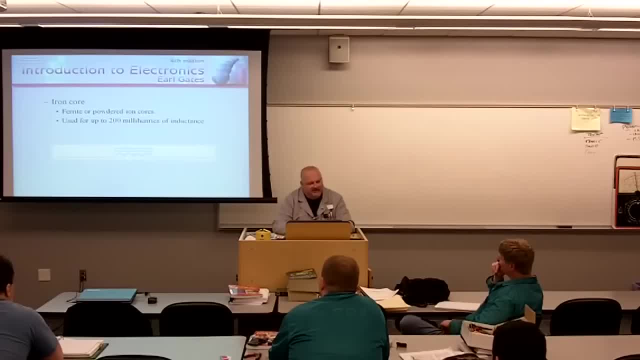 damn damn you, Scotty. that's why I'm not into drama. not a very dramatic kind of guy. it's iron core used for values of 200 millihenries of inductance, typically up to 200 millihenries of inductance. 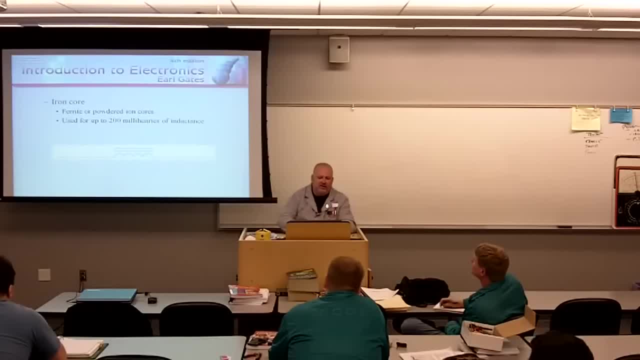 schematic symbol shows these two parallel lines next to the coil. that shows that there's an iron core next to the coil- torrid core. these are donut shaped, but do not try to eat them. they offer a high inductance. for a small size, these are very prolific. 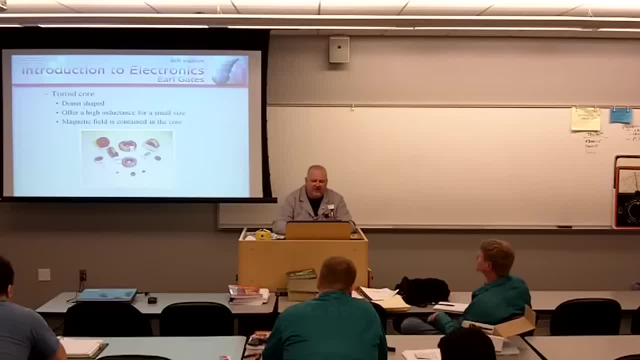 in a lot of contemporary electronic applications because the magnetic field is contained in the core, offers a very high inductance for a very small size. if you opened up a computer power supply you'd find a bunch of these inside. a lot of inductance for a relatively small package. 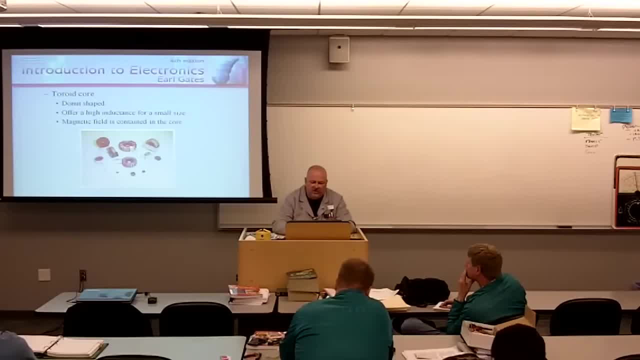 I've had graduates that have gone to work for companies and they had to do this as part of their job. roll their own. they're given the blank core spool of wire and you sit there and you thread it through, tighten it up, clean the lead, solder it in the boards. 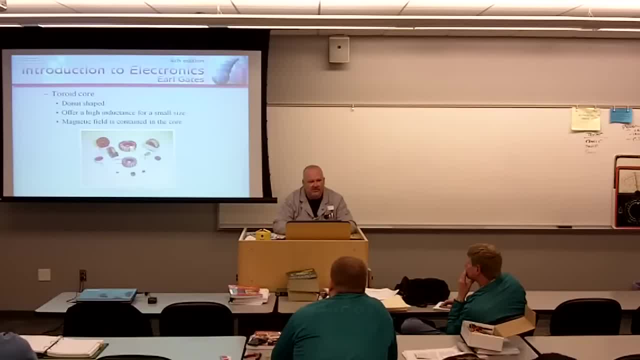 actually pretty good jobs. high frequency, high energy, radio frequency. Mr Graham, what's going on? man got a question. you're just back there waving man. it's like what's up? magnetic field contained in the core. basically, the significance of that is that it's not going to. 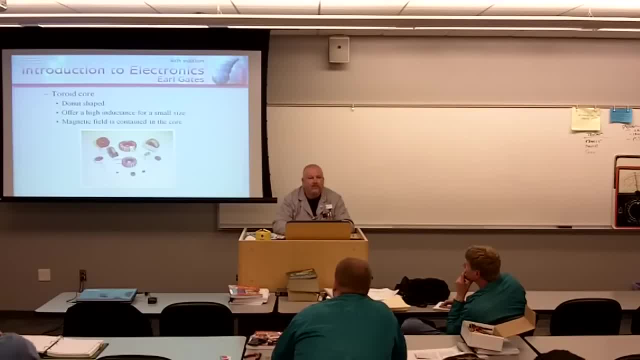 the inductance is not going to stray into things around it, it's just going to be contained in the core so, like a normal transformer is going to have a field around it, inside it's containing. it basically increases the efficiency, which makes it more better. this is a shielded core. 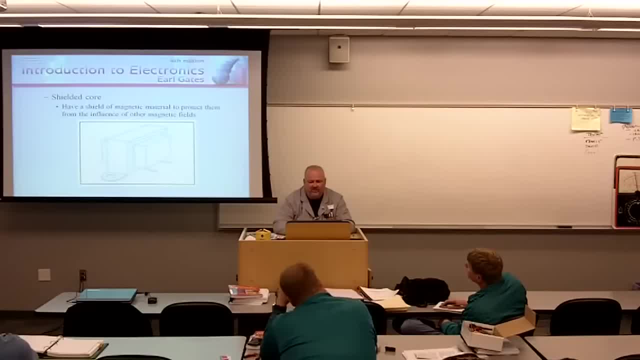 shielded core have a shield of magnetic material to protect them from the influence of other magnetic fields, because if you've got a couple of these in close proximity to each other, one field could influence another device. if you didn't know any better, what would you think this device was? 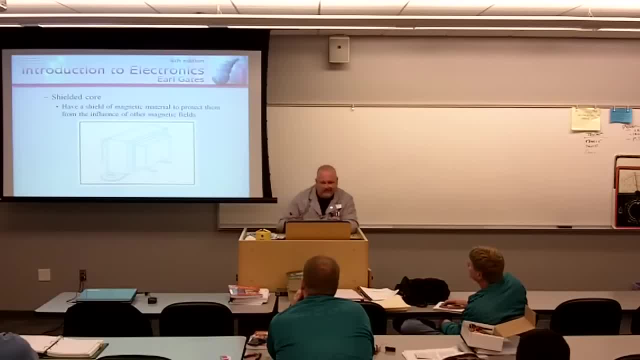 it looks like a transformer and the only tell that there is on this is there's only two wires. if you look on the other side, you wouldn't find any other wires, but it would look exactly like a transformer. as a matter of fact, you can use a transformer. 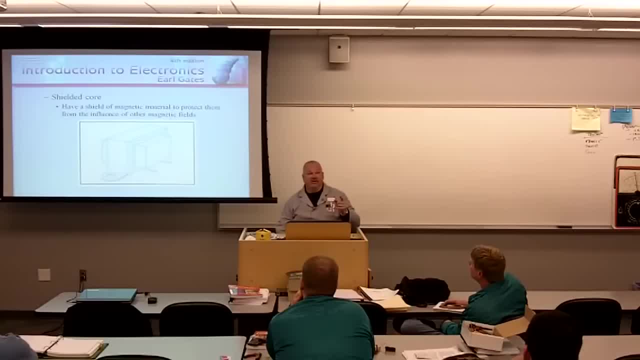 as an inductor, if you don't connect the secondary leads to the primary, if you only use just the coil as an inductor for some applications. that's why I've got a garage full of junk, because I won't throw a transformer away because someday I may want to use it. 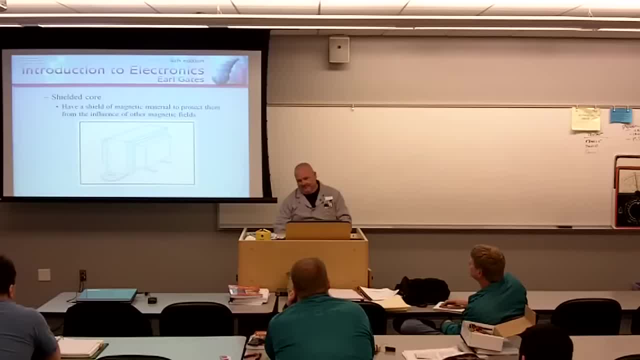 as an inductor. this is laminated core and again, if you didn't know any better, you'd think it was a transformer. we know it's an inductor because there's only two wires coming out of it. on the top is stamped 4.5 henries. 4.5 h. this was going to vary from .1 henries all the way up to 100 henries. this is also sometimes referred to as a choke, as a choke used as a choke in automotive applications- noise filters, meaning to choke off a chain. 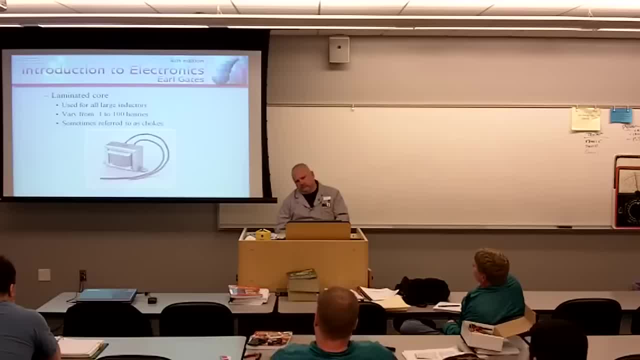 it's going to choke the change. just like resistors, inductors can be connected in series parallel or series parallel. when you're dealing with inductors measured in henries in series, you treat them exactly like resistors, plain and simple. if I've got two henries, and I put it in series with four henries. two plus four equals six. I now get six henries worth of inductance in parallel. you treat them like resistors in parallel, so the total inductance will always be less than the value of least. 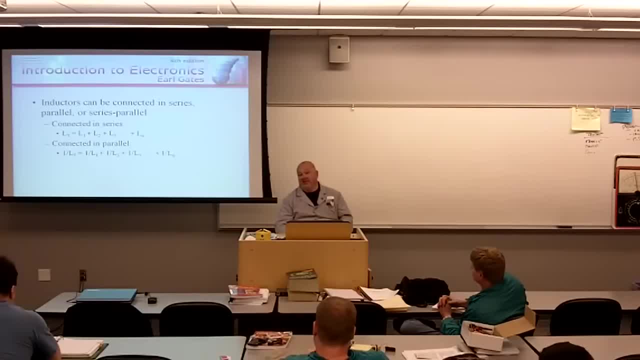 as long as you're dealing with the property measured in henries. now this is where things get interesting. everything else I've been talking up to this point has just been kind of hey, just trying to get to know you. this, the real deal, DIS D-I-S. 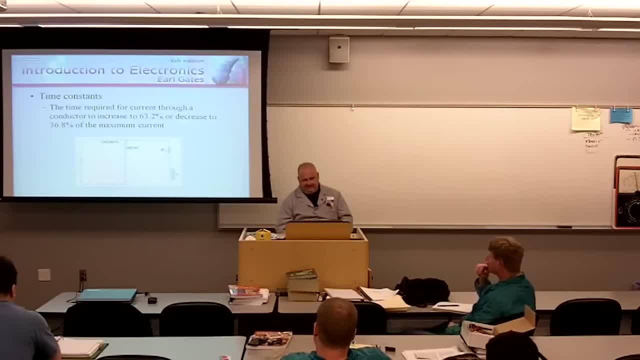 is what it's all about. it's a series circuit. it's a series circuit. I've got a switch that has two positions. one is called the ground growth mode and the other is the decay mode. so this switch I can toggle from either growth to decay when it's in the growth mode. 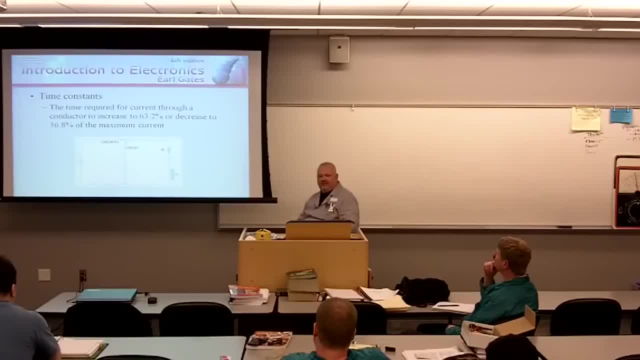 I have a simple series circuit, do I not? and the circuit contains an inductor. actually what an iron core inductor? because I see the parallel lines to the inductor in series with a resistor make sense when I close the switch, as soon as I close the switch. 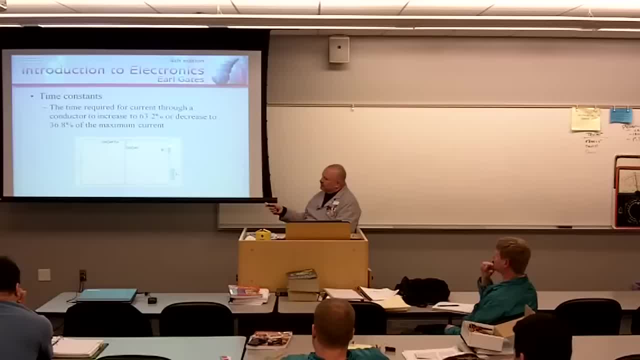 it's going to allow current to flow through this circuit. do you agree with me? what's going to happen is that current is going to come racing through the circuit negative to positive, and all of a sudden it's going to hit this curly piece of wire. 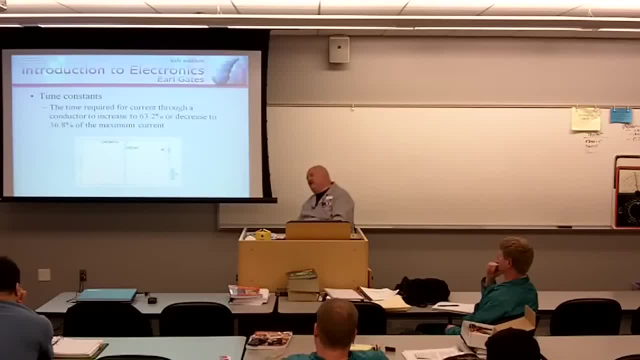 and that curly piece of wire it's hitting is an inductor. an inductor is a specific device designed to possess the property of inductance. inductance is that property which tries to oppose a change in current. so current was at zero. it wants to go to 100%. 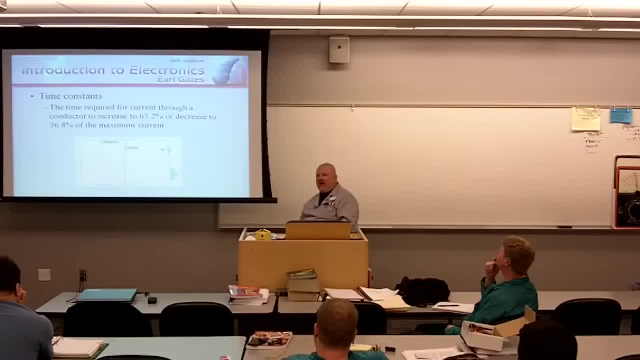 and this device is going to say: uh, uh, I want you to stay at zero. why? because you've been at zero and I like it like that. but eventually, as the current continues to come, that magnetic field builds and current eventually goes to maximum, it goes to 100% for this circuit. 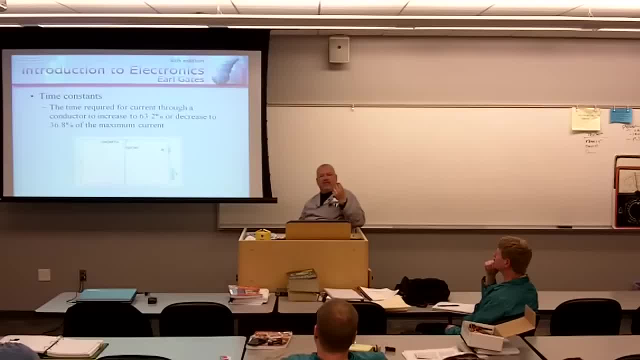 but the inductor, because of its property of inductance, is going to fight the whole time to try to prevent that change from occurring, but eventually it's going to lose. so close the switch turn the circuit on the inductor is going to fight, fight, fight, fight, fight, fight, fight. 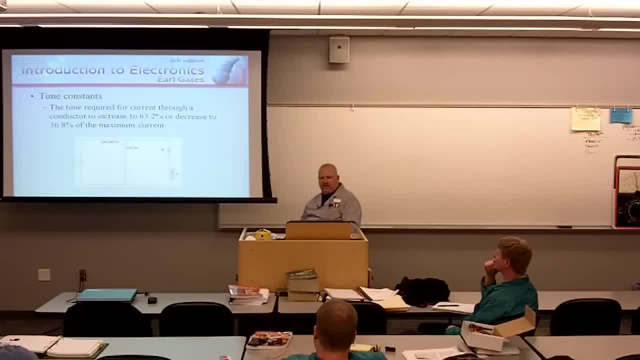 and eventually give up and current is going to be at 100% flowing through this circuit. when current is at 100% flowing through this inductor, electrons are like what is up with that? it's a piece of curly wire after a period of time. 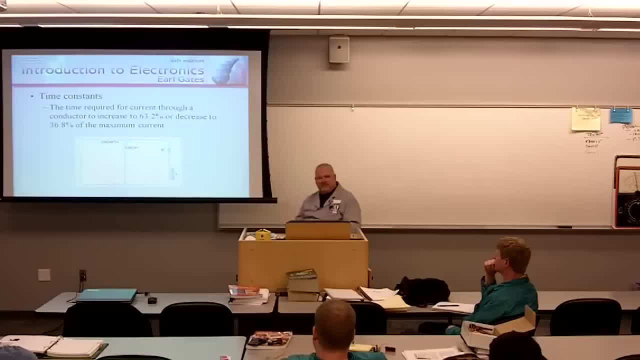 the electrons, it's like: why am I going through a piece of curly wire? it just has no effect on them whatsoever. and the circuit runs and runs, and runs. soon as we get the switch and move the switch from the growth mode to the decay mode, the magnetic field that was built up 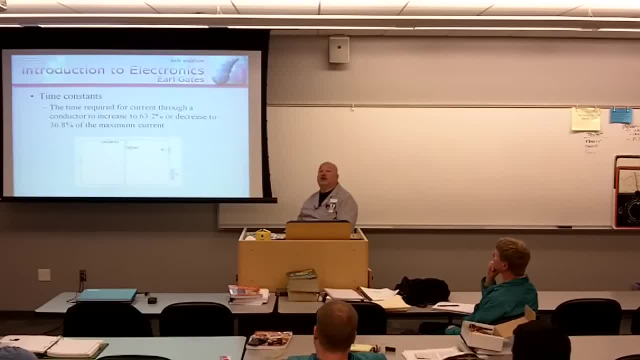 around. inductor L1 is going to collapse and it's going to collapse into itself. when it collapses into itself, what is it going to do? it's going to act like a. what happens when a magnetic field passes through a conductor? we induce current. if we move a conductor, 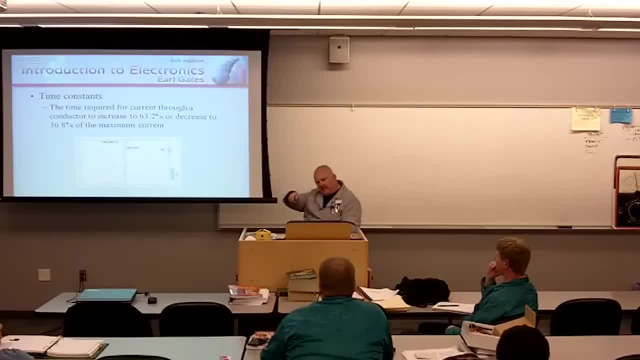 through a magnetic field, we induce current. if the conductor is stationary and the magnetic field moves through a conductor, we're going to generate current right. so as soon as I move this to the decay mode, this magnetic field is going to collapse into itself, creating a counter current. 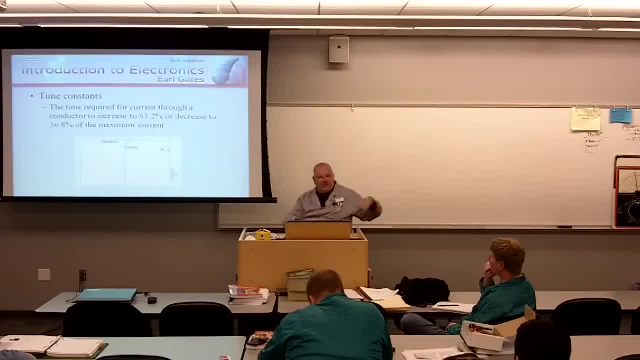 Lenz's law, the opposite of the force that created it, and then that current is basically going to flow through the circuit until it dissipates. but if this was just a series circuit made up of a resistor and a switch, you turn it on, boom, you go to 100%. 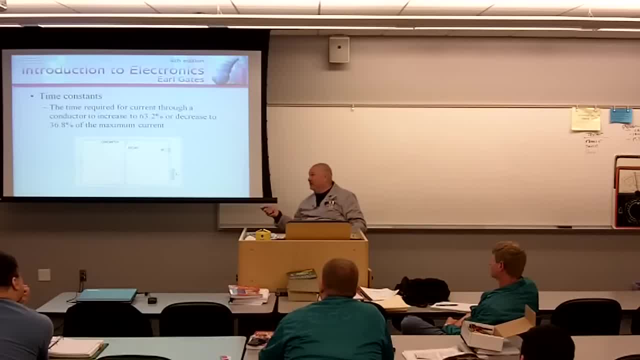 you turn it off, pow, you go to zero. now, with an inductor in here, you turn it on, it's going to come up and eventually get to 100%. you turn it off, that magnetic field is going to collapse and eventually it's going to get down to 0%. 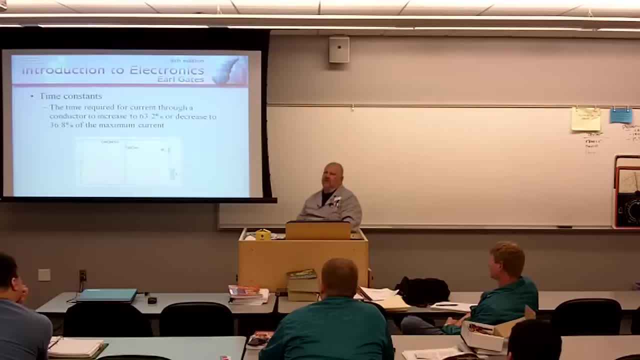 you follow what I'm talking about. you guys know what I'm talking about. I'm beating around the bush. what am I talking about? time constants, the time required for current through a conductor to increase to 63.2%. so if I apply 100%. 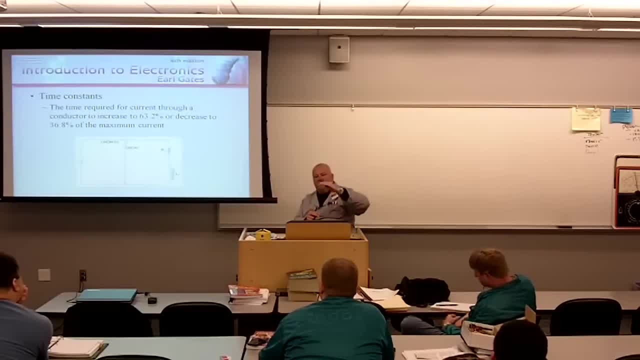 to it in that first time, constant, it's going to rise to 63.2% and the next time, constant, it's going to gain 63.2% of that is what's remaining. the next time, constant- 63.2% of what's remaining. 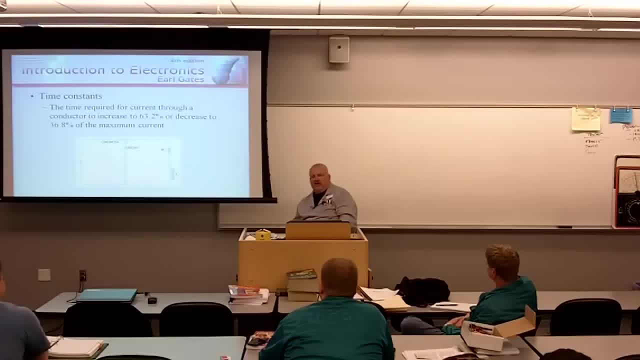 the next time constant 63.2% of what's remaining. the next time constant basically after five time constants. we say enough is enough, it's 100%. but is it really at 100%? no, because it's non-linear, so really it never reaches. 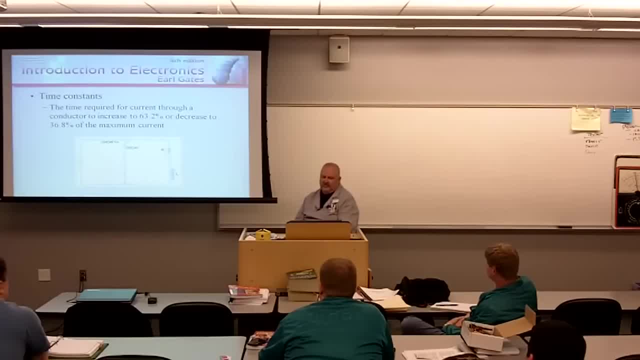 100%. we say after five time constants it's reached 100%. it's good enough for what we do to calculate out this time constant. it's actually relatively easy. LR is the symbol used for the time constant of an RL circuit and the formula is: 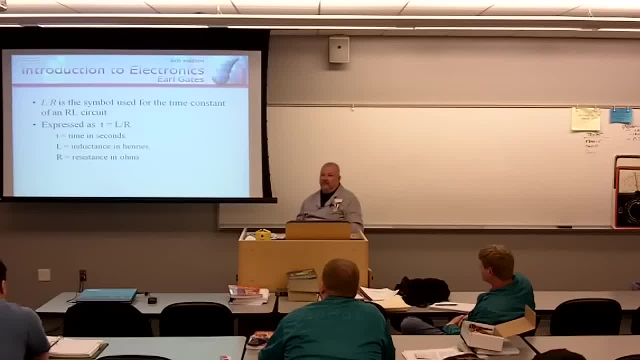 T is equal to L divided by R period. take the amount of inductance, divide it by the amount of resistance. that would be the time constant measured in seconds. that's what we use as our base unit of measurement in electronics. the second T is equal to L over R. 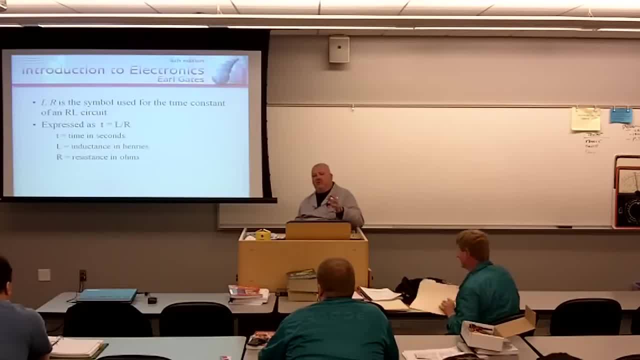 yes, if I gave you four inductors, you'd have to calculate out the total inductance and plug that in the circuit right there. so I could give you some real nightmare circuits right now. think about it, it'd be fair game. I could give you a circuit that's got 13 inductors. 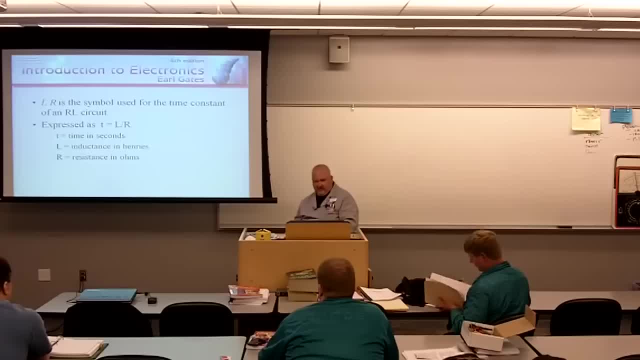 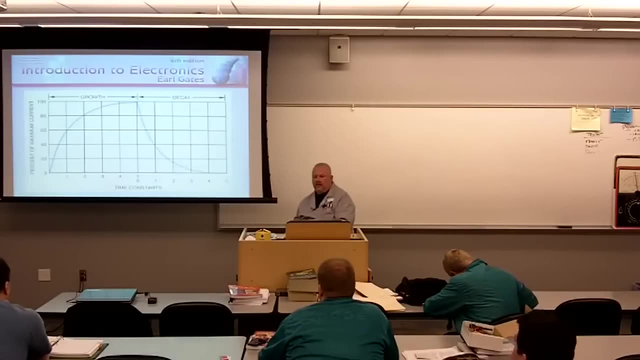 in combination series parallel and 22 resistors in combination series parallel. the bottom line is it's equivalent to this circuit here. you've got to figure that out, but you should be able to do so without a whole lot of fuss. this is what a time constant. 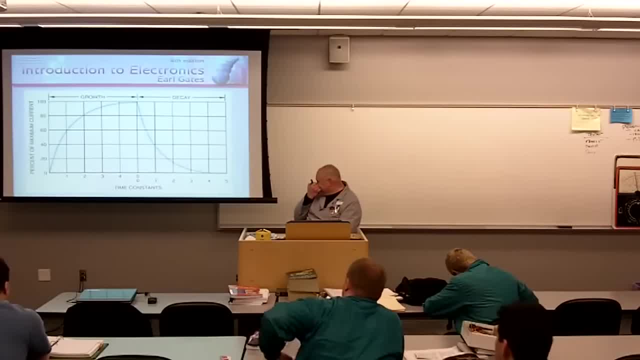 curve looks like. here's that first time: constant 63.2%. 63.2% of what's remaining, 63.2% of what's remaining, 63.2% of what's remaining, what's remaining, and what is it that I'm? 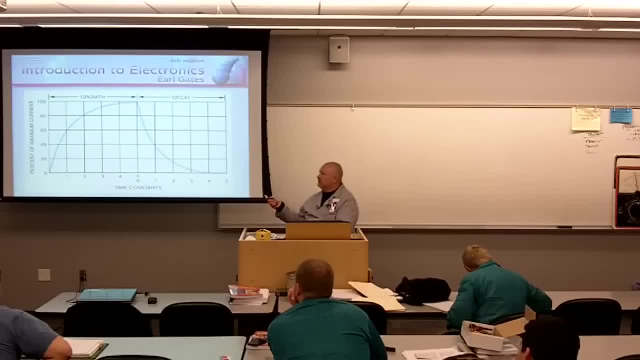 actually looking at here? what is this blue? is this voltage? What is this? It's a current, current. number one because the slide says so. number two, most importantly, most importantly, because it's current, that's going from zero. the inductor is trying to prevent the change. 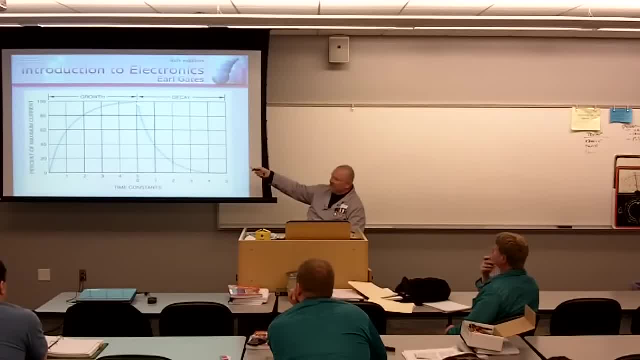 trying to prevent the change. trying to prevent the change, all right, current wins. then as soon as you shut that circuit off, current's going to try to go from 100% to zero, but because that magnetic field is collapsing, ah, I don't want to decrease, I want to keep it 100%. 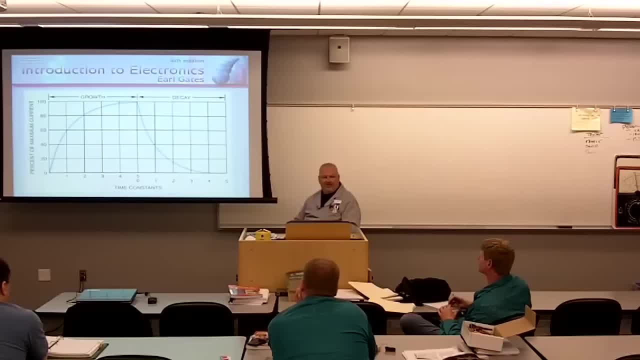 but I can't, oh crap, oh, all the way down to zero. But because that field is collapsing, it's going to try to prevent that change. That's why we use these. That's why we use these Absolutely. 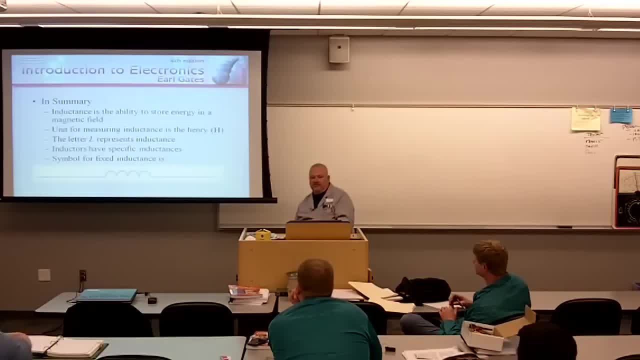 If we're affecting current, definitely we'll have an effect on voltage. In summary, inductance is the ability to store energy in a magnetic field. Just remember: the key word for inductance is magnetic. That's how they do their magic. 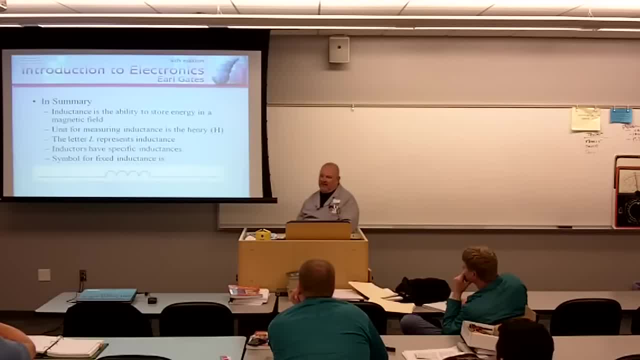 The unit for measuring inductance is the Henry, measured by the capital letter H. The letter L represents inductance. Inductors have specific inductances. That's why they're designed. The symbol for a fixed inductor is down here at the bottom. 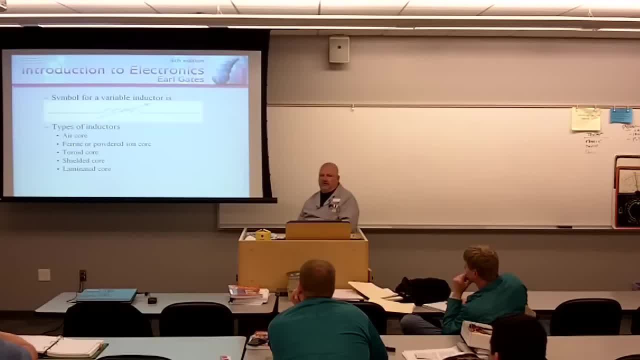 The symbol for a variable inductor has an arrow going through it. The arrow means it's adjustable. Types of inductors include iron core, ferrite or powdered iron core, torrid core, shielded core, laminated core. 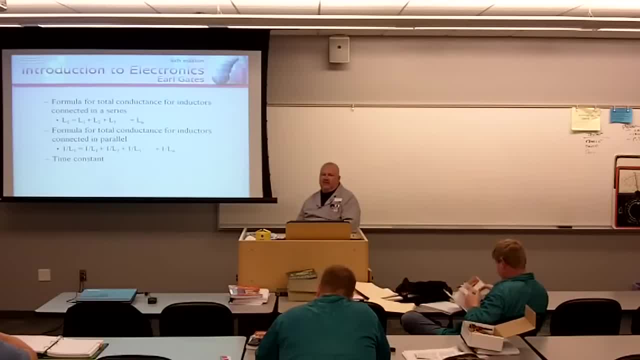 Formula for adding them up in series is like the same formula for adding up resistors in series. The only thing you need to be aware of you're adding up inductance measured in Henry's. If it's not in Henry's, you can't use this formula. 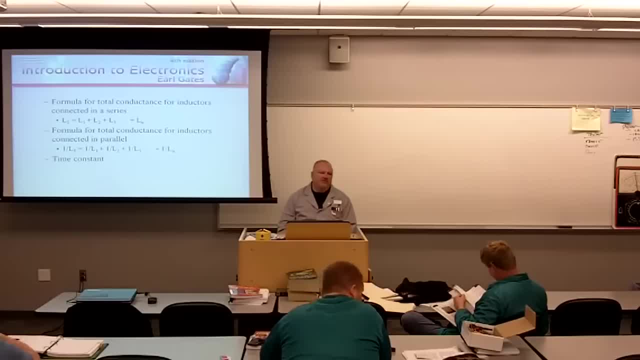 The formula for total conductance in inductors in parallel is the reciprocal formula. Use it the same as you would for resistors in parallel. Time constant formula T is equal to L over R. You run this calculation. it shows you what one time constant is worth. 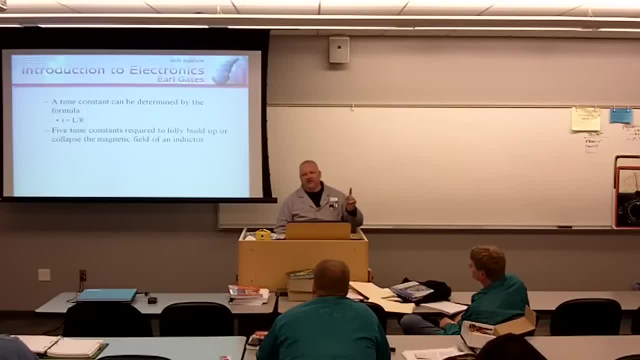 I need to multiply that by how many to figure out how long it's going to take to get to 100%. Five, Because it takes five time constants to reach 100%. So understand that when you do this math you only end up with one time constant. 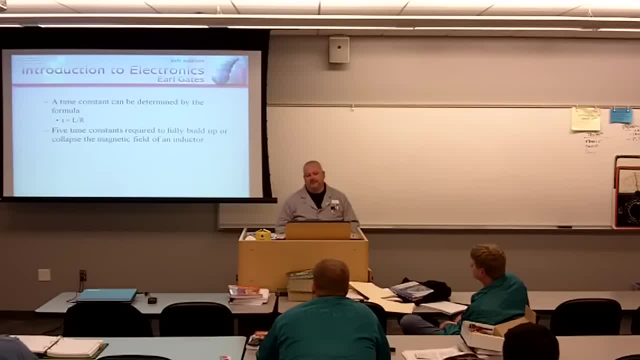 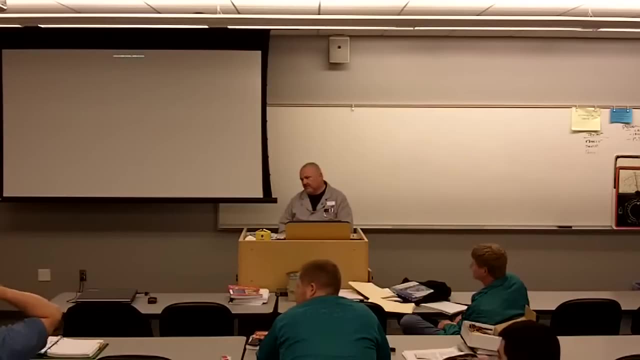 It takes five To get the job done. Or, as it says here, five time constants required to fully build up or collapse the magnetic field of an inductor. Any questions on anything that we discussed with the inductors? Yes, Yes. 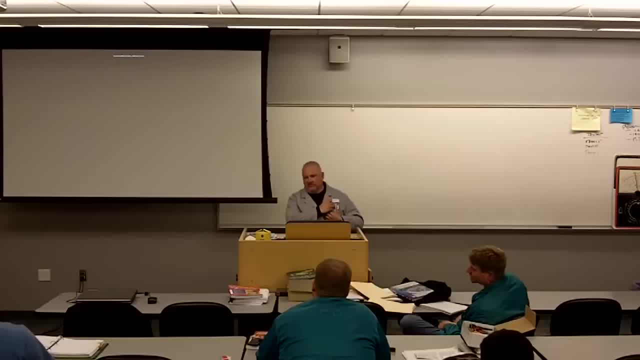 Yep, and that's it. We have inductors because they create inductance, And inductance is that property which tries to oppose a change in current. So we're going to have a lot of different components that are going to want to bring about. 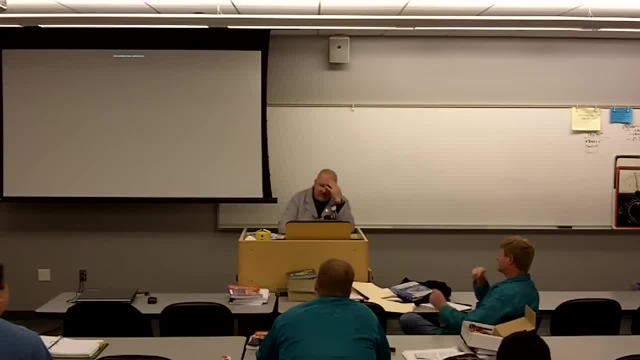 a change in current in a circuit And if we put an inductor in there, an inductor could help stabilize that current flow because of that electromagnetic property. So it's going to help stabilize current levels in a circuit. The majority of applications that we're going to use inductors for 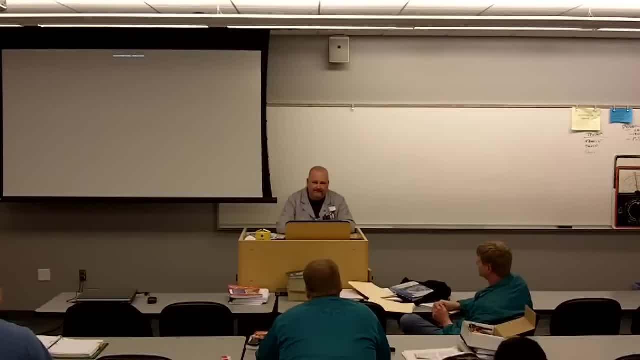 is really going to be filtration, Because, once we're not there yet, some of you may have read far enough ahead that when we apply an inductor to an AC circuit it starts doing some wacky stuff And by harnessing that wacky property, 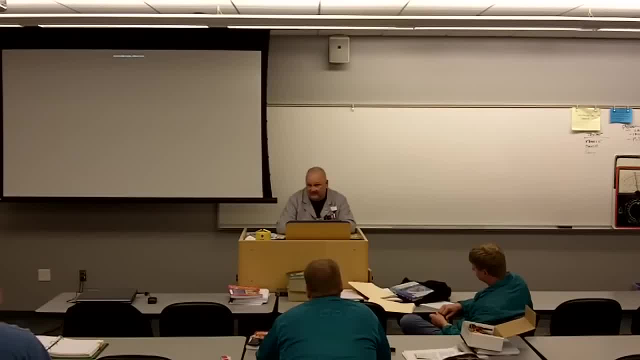 called inductive reactance. we can use inductance, We can use that to filter. We could use it in audio applications where we want only certain frequencies to go to certain speakers. Heck, I knew a guy that was getting some interference on one of his cable channels back in the day. 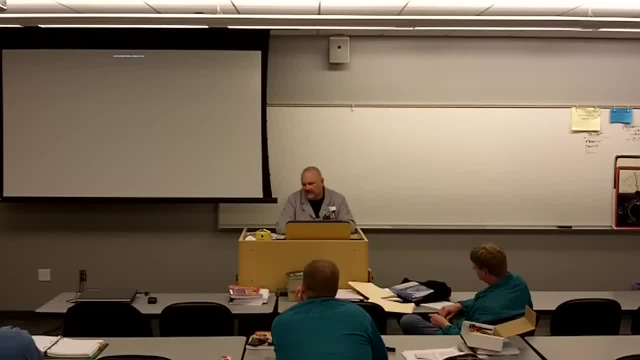 And because this friend of mine had extensive electronics background, he said he didn't want to call the cable company and have them waste their time and come out. and Exactly So this friend of mine built a filter circuit to filter out the garbage signal. 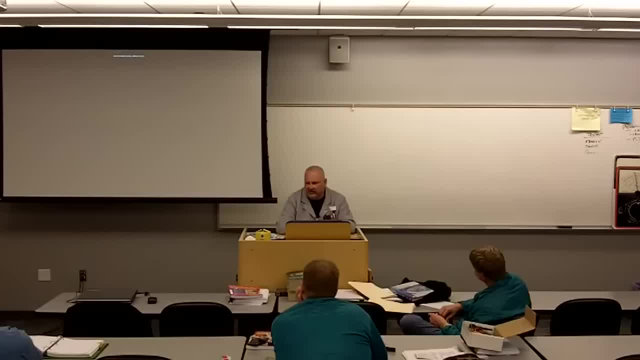 that somebody was putting on this pay-per-view channel And by filtering out the garbage that got put on the channel, the reception was enhanced and made the station viewable. And the key component in that whole- so I'm told project- is an inductor. 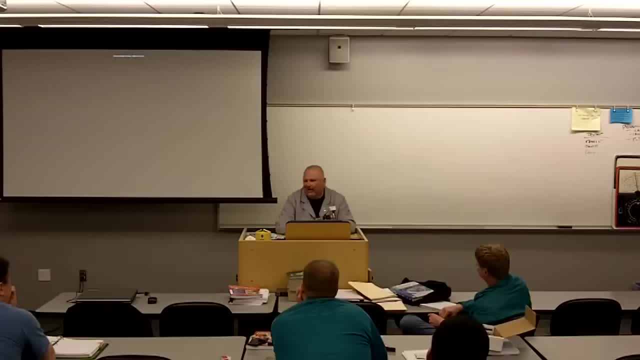 And ironically it was an inductor that was like three turns of wire- One, two, three turns of wire was adequate enough for the reception to be enhanced, Mind-boggling. so I'm told Question: Yeah, Yeah, Oh, really. 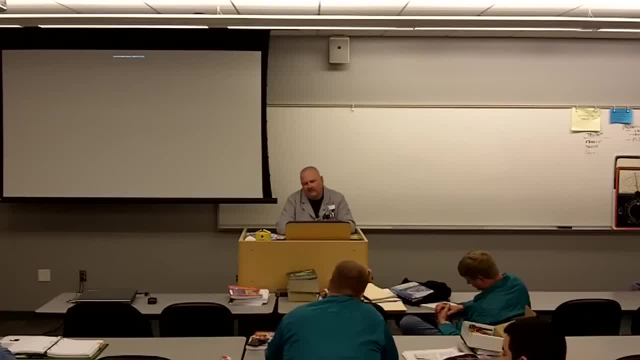 Interesting, Yeah, And a little. did you realize what you were doing at the time? Yeah, Nobody knew why, but it worked. Now you know. All right, let's go ahead and take a break, And at about 6.20,. 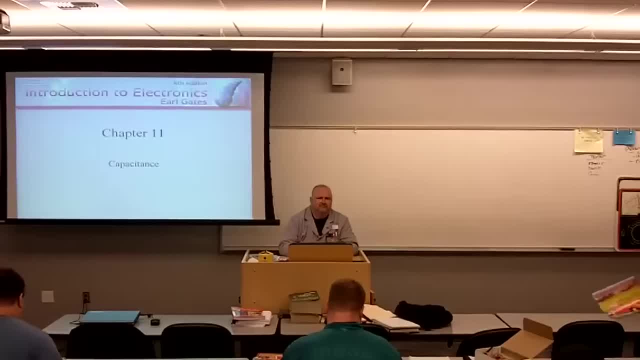 we'll start up with Chapter 17.. Y'all ready for this? Chapter 11,, Capacitance, Capacitance. If you believed what I sold you last chapter, this should not be a stretch for you, Because it's kind of like the same thing is happening. 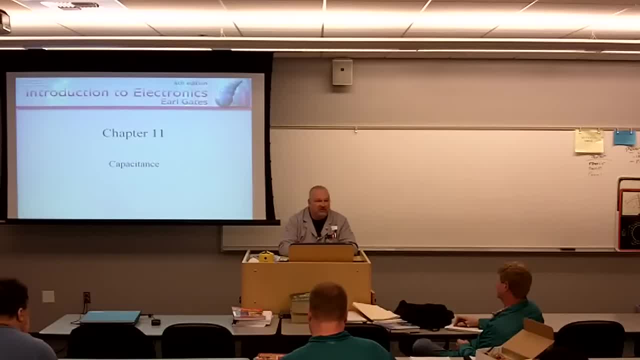 but with a different property. It's really what it's all about, But Capacitance is actually kind of cool. We'll talk about it. A lot of uses for Capacitance After completing this chapter. the student, you, the student. 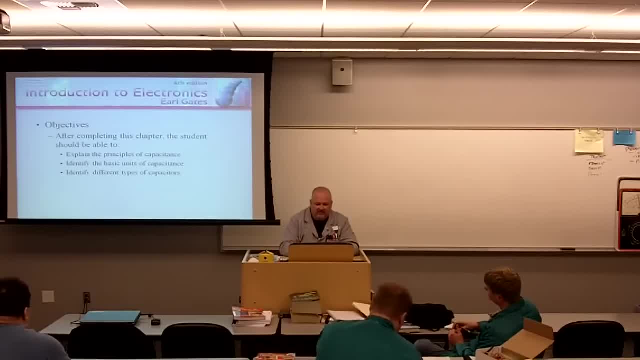 will be able to explain the principles of Capacitance. Identify the basic units of Capacitance. Identify different types of Capacitors. Determine total Capacitance in series and parallel circuits. Explain RC time constants and how they relate to Capacitance. 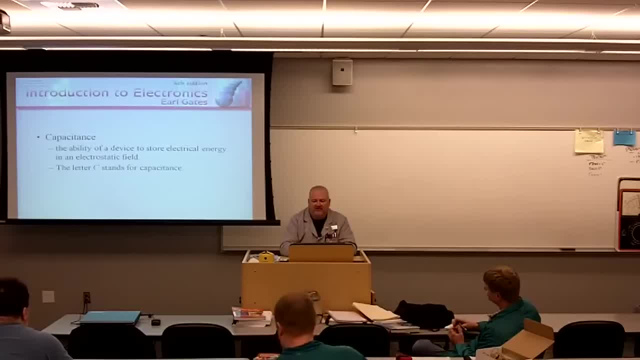 Capacitance is the ability of a device to store electrical energy. Let me stop. The ability of a device to store electrical energy. What does that sound like? the definition of Mr Carter? That sounds like the definition of a battery, doesn't it? 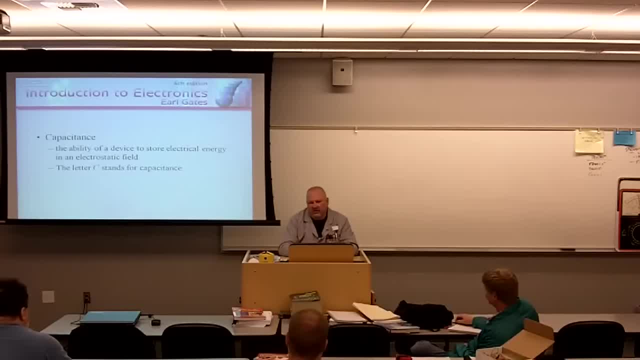 The ability to store electrical energy. So there's really not that big of a difference between a capacitor and a storage cell. Typically, a storage cell is a battery. A storage cell is a small amount of current over a long period of time, Unless you're a car battery. 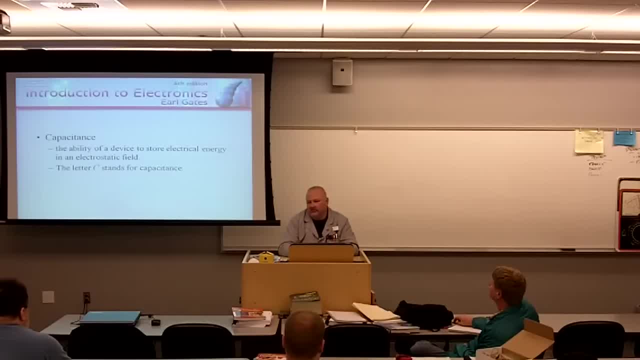 But a capacitor generally is a large amount of current over a short period of time that it's designed to expend, if you will. The definitions are very, very, very similar very close. The key word on how a capacitor works is: is that electrostatic field? 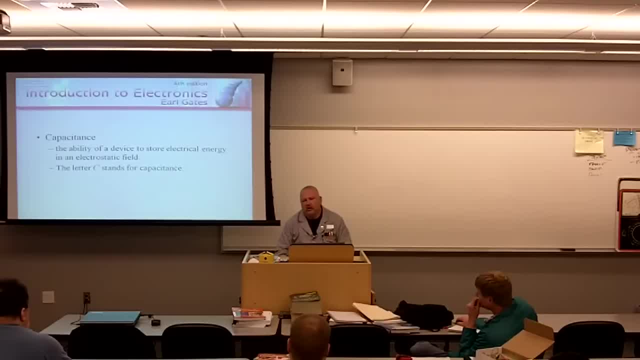 Electrostatic field. Remember inductors? They were electromagnetic. This is electrostatic- Electrostatic. Talk about that property a little bit more in a bit. The letter C stands for Capacitance. So inside a schematic diagram, if you see, a letter C equals. 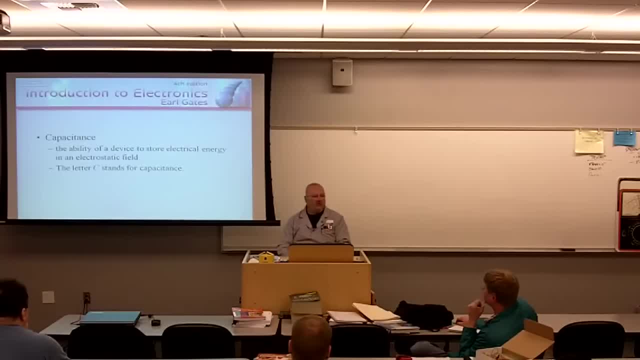 it's Capacitor. If you see C22, it's Capacitor number 22.. C22 in the circuit C47, Capacitor number 47. A capacitor is a device that possesses a specific amount of capacitance. How these things are made. 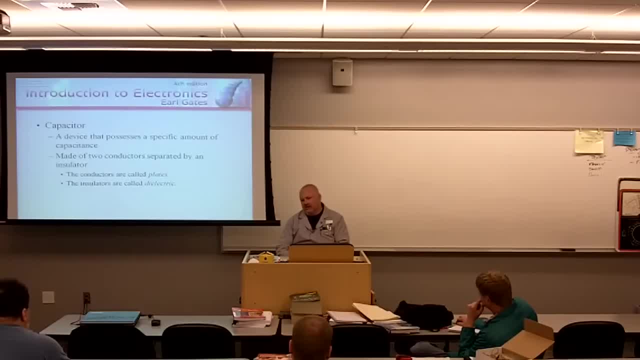 are two conductors separated by an insulator. Two conductors separated by an insulator. What does that sound like? the definition, for Close your eyes and think about it. Two conductors separated, Two conductors separated by an insulator. What does that sound like? 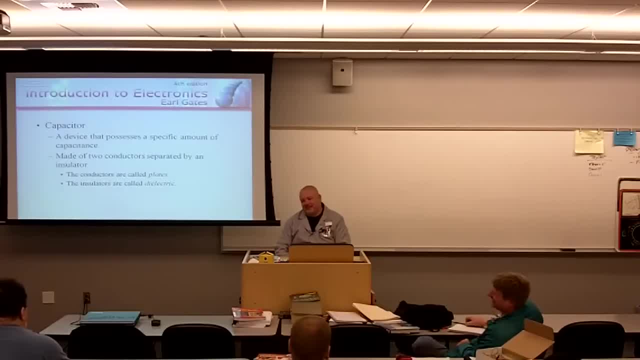 You made that up, man. What would the definition of an extension cord be? Two conductors separated by an insulator? What would speaker wire be? Yeah, so you know what. There are going to be a lot of things that have capacitive properties. 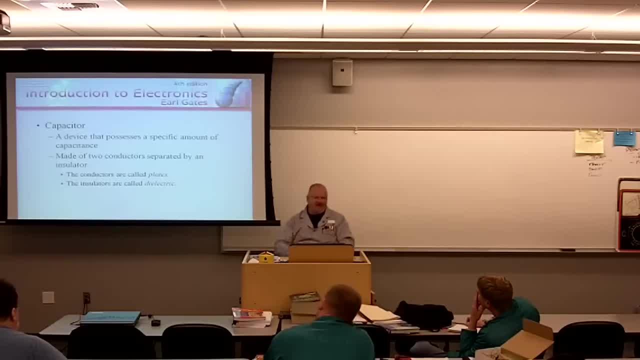 Because they're two electrical conductors separated by an insulator, And a lot of these things that have capacitance is stray capacitance, and capacitance that we don't necessarily want, Engineers don't want, But we have to deal with it because it's two conductors. 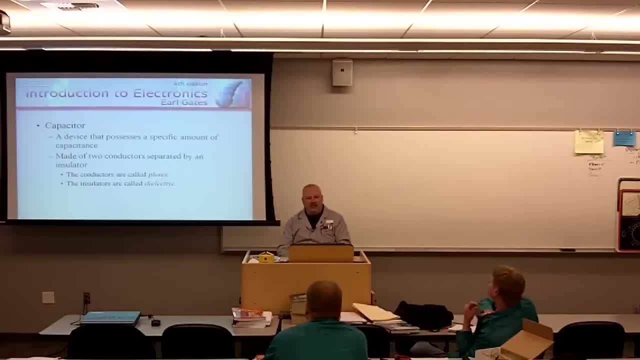 separated by an insulator. Anytime you do that, you're going to end up with the property of capacitance. Anytime you coil up your welding wire, your welding leads, electro-leads- you're going to create some inductive properties. 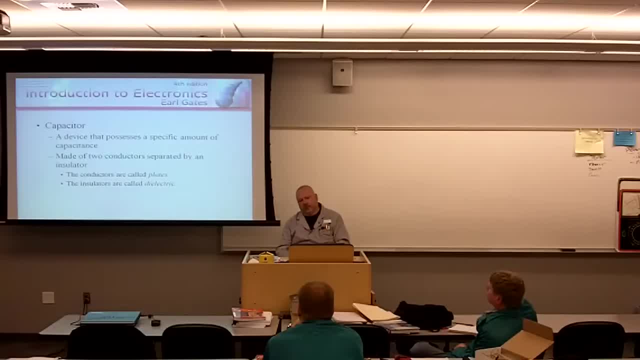 Yep, Yep, And that actually- believe it or not, that style of twin-lead antenna cable. it was some of the most efficient. When properly installed, it had higher efficiency than coaxial cable. The only thing is people would get that nice ribbon cable. 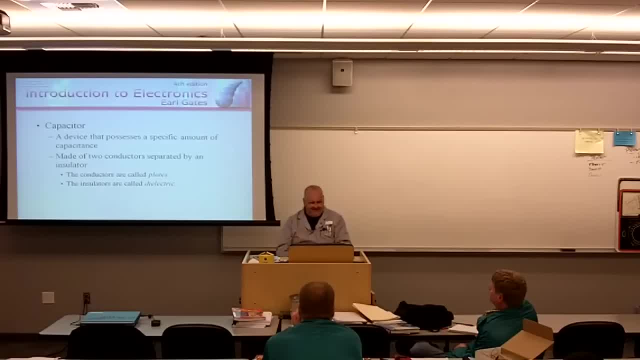 and then back in the day, right growing up in Connecticut, you know we had aluminum windows and you'd run it through the window and then slam the window down on it and there goes any advantage that you had. But when you used the proper stand-offs, 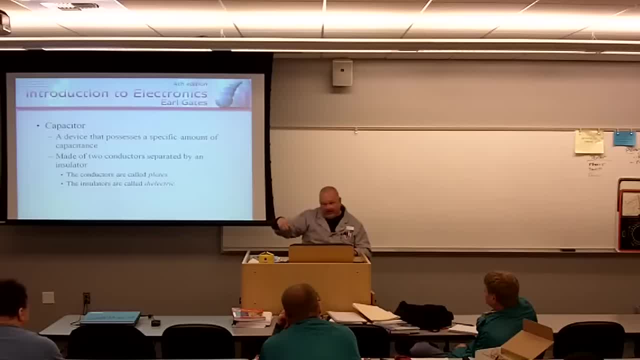 and you, you know, had it. you used the proper bend radius and everything else directly to the back of the set. that had higher efficiency. it would get more RF energy into the back of that tunnel, into the back of that television set. 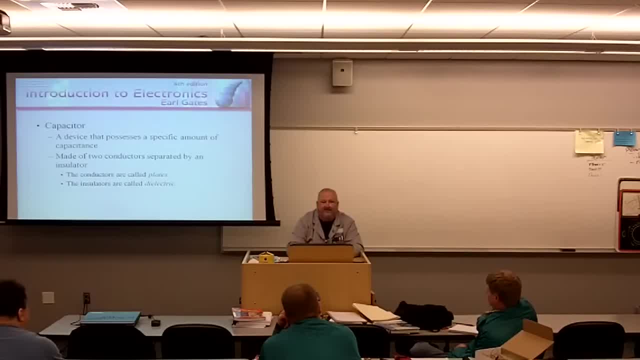 than using coaxial cable. But it was two conductors separated by a thick dielectric, thick insulator material. So that's one of the things I really want you to come out of these lectures with is understanding that. you know this is not a lecture about capacitors. 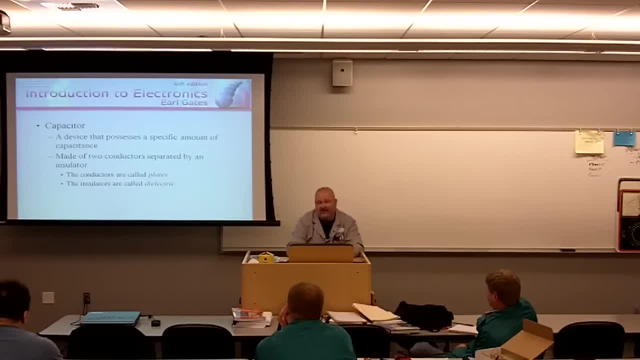 This is a discussion about capacitance And capacitors, But the biggest thing is when you get into some of the advanced classes, like Peter Welty and his PCB design class, one of the biggest challenges is determining stray capacitance inside a circuit. 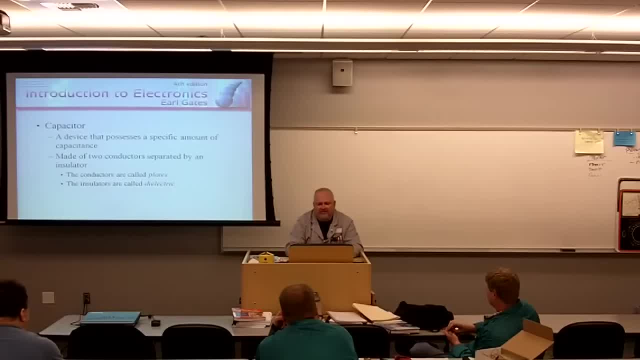 When we're physically trying to create capacitance. we're going to call the conductors plates And we're going to call the insulator dielectric, So two plates separated by a dielectric. Now that, Mr Carter, is the definition of a capacitor. 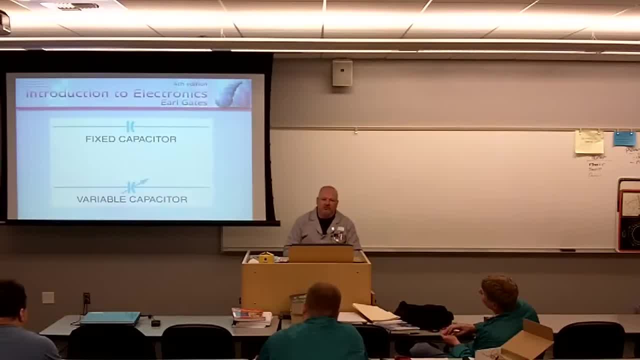 Schematic diagram. up at the top is a fixed capacitor, meaning what you see is what you get With intolerances. of course, Down below is a variable capacitor. There's actually different ways that they're going to be able to vary the capacitance. 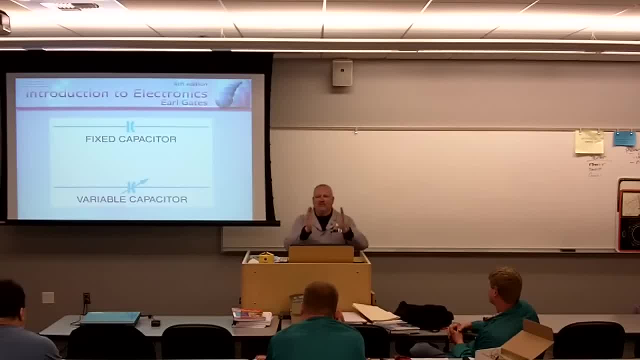 One is going to be varying the distance between the plates- We'll talk about this more in a bit- And the other is meshing the plates where they don't physically touch, but they're just closer proximity, More and closer proximity to each other. 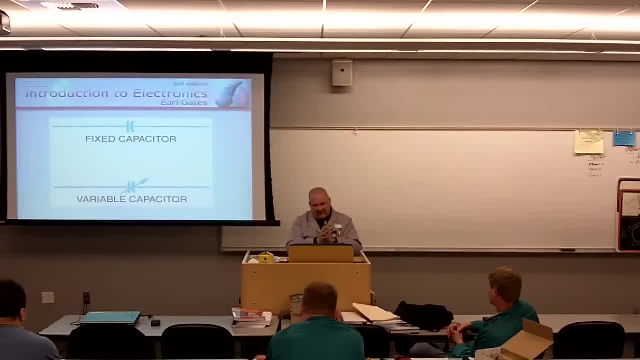 Less and less proximity to each other Make sense. Treat all capacitors as though they were charged. Never touch both leads of a capacitor with your hands. I've got a capacitor. Where the heck it went? I've got to get my stash better organized. 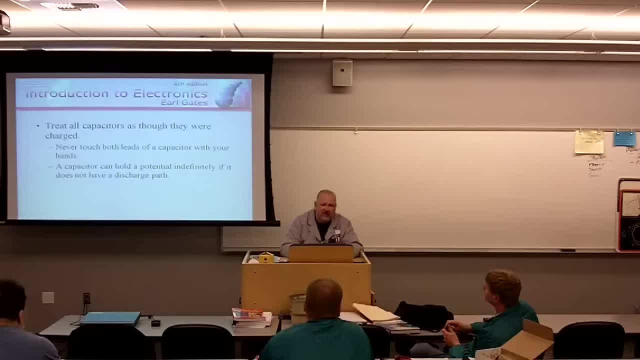 Stuff disappears in here. I actually had a student that worked for one of the biomedical companies, Medtronic, and they had the starter jumper kits for when you die. It's great I see them. They got like Costco, you know. 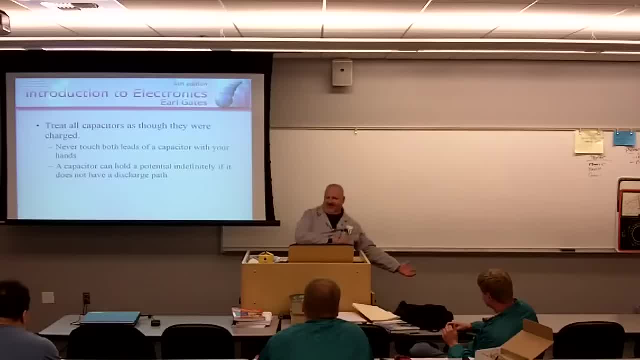 You just got $680 worth of stuff in your cart at Costco. They revive you on the spot. Make sure you pay your bill. Airlines got them. now We're going to charge you $25 for that bag to check it. You know you have a heart attack. they revive you. 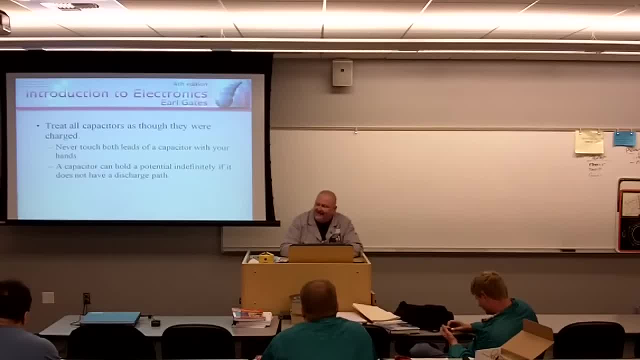 Just let me die here. Anyway, had a student that worked there- an evening student of mine, and he brought me a capacitor That was a key component in that And right on the capacitor was a label. The energy stored in this device could be lethal. 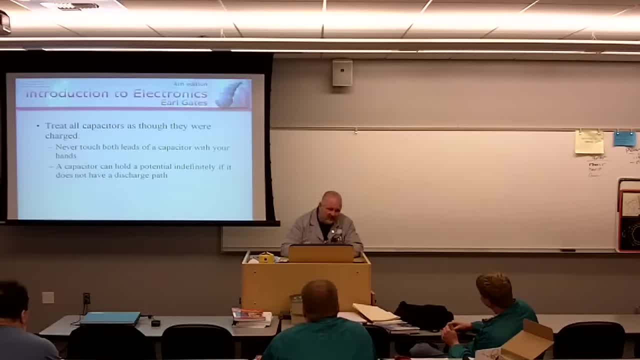 The energy stored in this device could be lethal. So if that capacitor's charged up and I toss it until you touch it, it'll kill you dead Because you're building up all of that charge and then rapidly discharging it through your body. which it's not designed to do, Which it's not designed to do. Capacitor can hold that charge potential indefinitely if it doesn't have a discharge path. A perfect, a theoretically perfect capacitor will hold the charge forever Because of manufacturing flaws and defects and stuff. 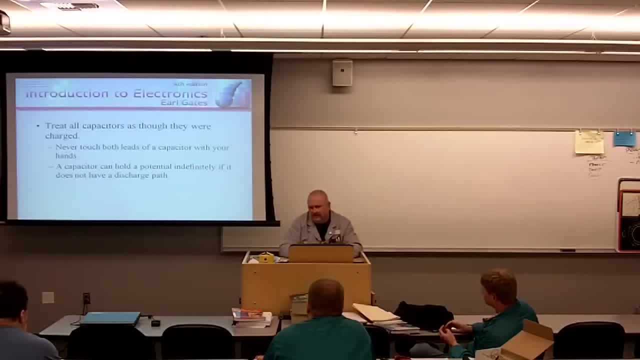 eventually that current will dissipate. I remember when they were- I've been here for a while, Not when they were building this building, Not when they were building that building, The new one, Not when they were building this building, But when they were building that building. 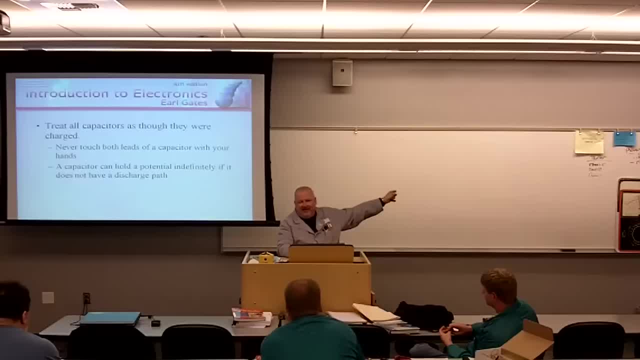 like 20 years ago, And there's actually a time capsule buried out there somewhere And they were looking for ideas from you know, I'm like let's charge up a capacitor and put it in the time capsule. I mean as an electronics guy. 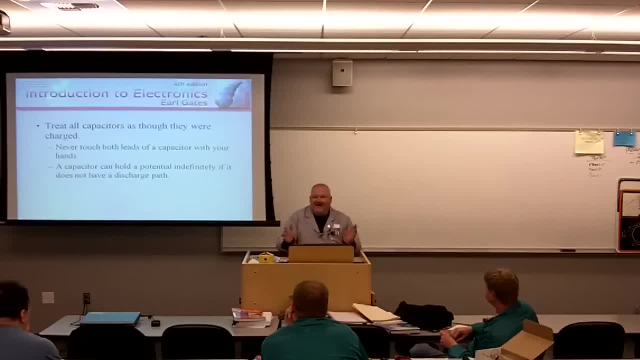 I think that'd be cool Like great. let's take it out of its protective covering and see if any voltage is still present. I mean, I would've gotten a kick out of it. They're all looking at me like I'm a goofball. 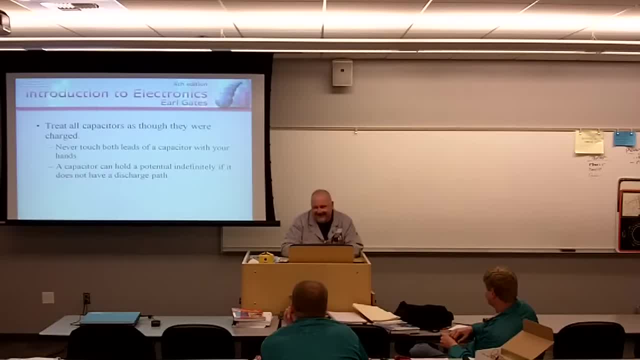 You know I mean, don't you think that would've been an outstanding, freaking idea? Because of the chemicals, a chemical cell will eventually dissipate, So it has a shelf life. Lithium batteries have the longest shelf life. I mean those. 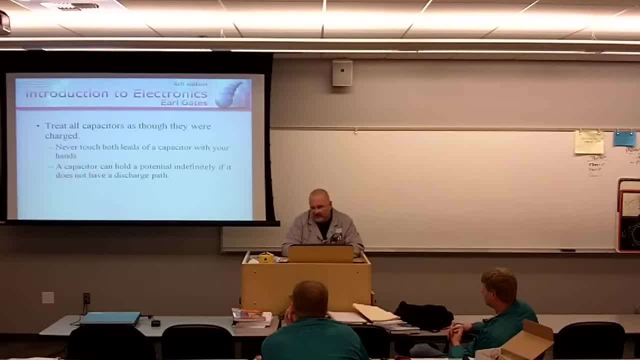 What are they? The Energizer or whatever that you could buy. Lithium, The best batteries that you could buy. Very great product, Innovative product If you absolutely positively have to have a portable electronic device, work, operate under extreme temperature conditions. 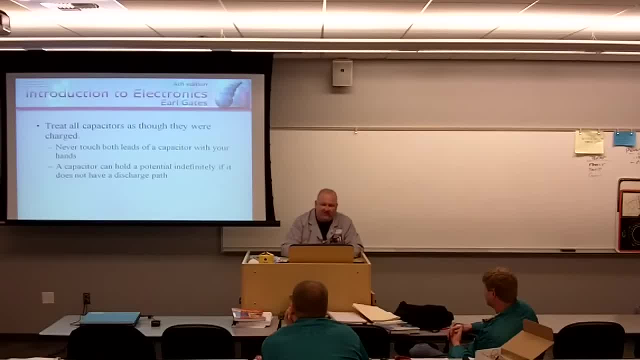 whatever great shelf life use those batteries. So I just bought some and I think that it's good to the year 2025 or something on it. It's like, wow, That's a shelf life. The basic unit of capacitance is the farad. 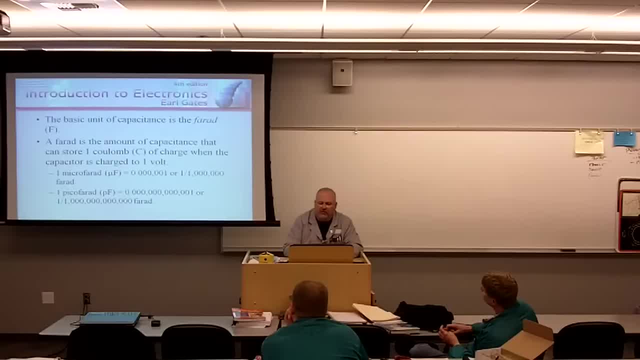 A farad is the amount of capacitance that can store one coulomb. Remember the coulomb 6.24 times 10 to the 18th electrons of charge when a capacitor is charged to one volt. So you got a couple different things going on there. 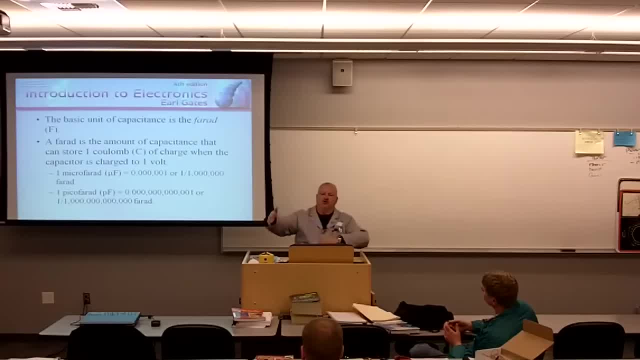 You got these two plates and what you're doing is you're charging it and what it's doing is you're physically loading those plates up with a large number of electrons And then you're building up an electrostatic, an electrostatic field across those two plates. 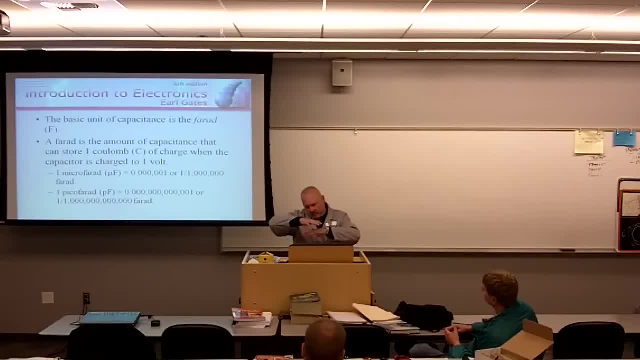 So when you build up one coulomb across the plates, we're able to store one coulomb of charge and bring the capacitor up to one volt. We call that a farad Now typically the values that we're going to work with in electronics. 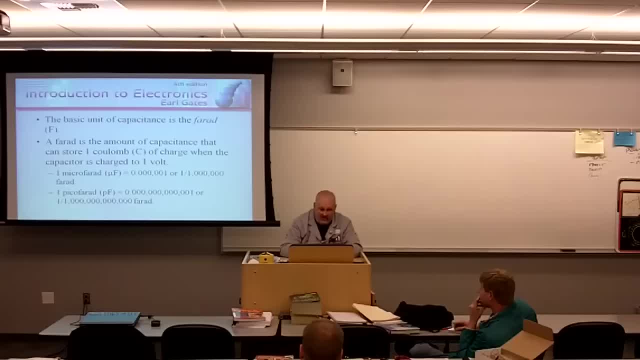 are going to be centered around the microfarad. The typical value of measurement of capacitance is the microfarad, Which is times 10 to the negative 6th, And also the picofarad, which is times 10 to the negative 12th. 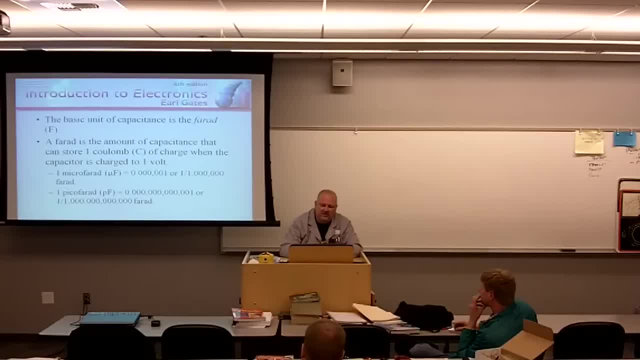 So we go from the 6th to the 12th. What's between 6 and 12? Nano. You know, for the longest time I used to put out in lecture, you will never see a nanofarad capacitor. 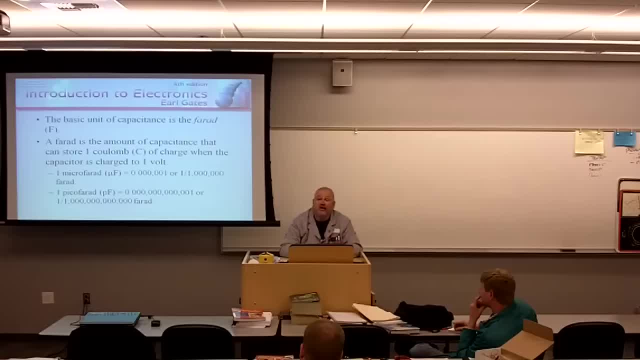 because they didn't use to make nanofarad. Actually, you know what they used to call nanofarad capacitors: Millimicro, Millimicro, Three places past Milli, No micro, Millimicro. 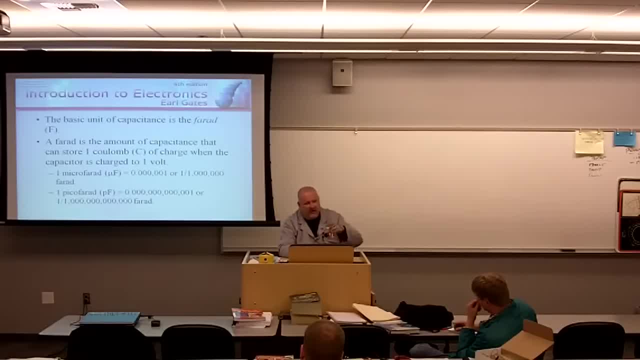 Three places past micro, which would be nano. So we call that, they'd call it millimicrofarad, MMF, Millimicrofarad, Or they would call it tens of thousands of picofarad. Why did they refuse to use nano? 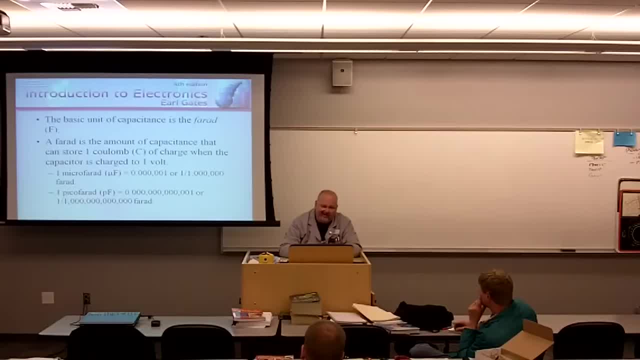 I don't know, I don't know if it was a small letter N that just like freaked them out Seriously. I mean, sometimes it boils down to that It was. you know, they'd have this congress that would meet and analyze this stuff. 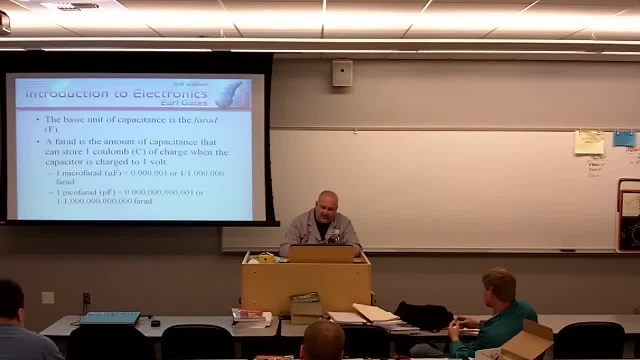 and they just wouldn't. So I used to put it out in lecture: you will never see a nanofarad capacitor. Whenever I put out absolute, somebody feels compelled to prove geogrenic wrong. So the next day, Stu. 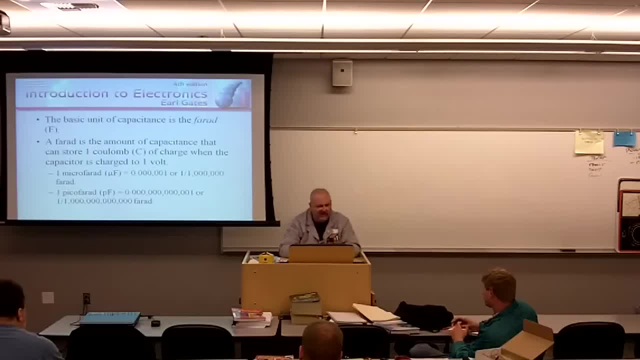 hey, you know, I found this. my company's using these. what's this? You know showed it to me. It was like a 20 nanofarad capacitor. Great, They're doing it. It should be a 20,000 picofarad capacitor. 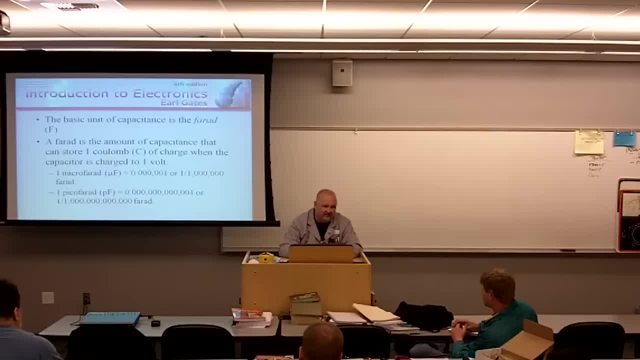 Or a 20 millimicrofarad capacitor, But- and that's I'm intentionally talking to you about this, because traditionally capacitor values have been all over the place as far as how they label them and how they identify them and sometimes determining. 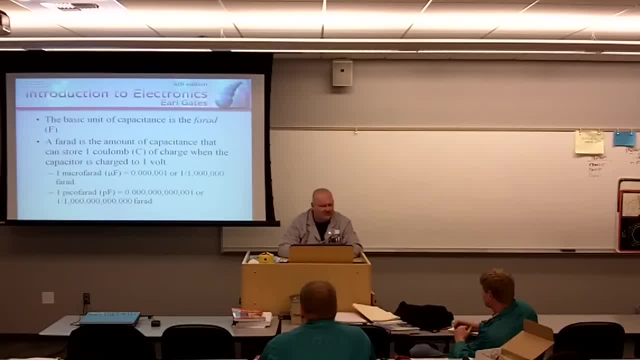 what size capacitor is it is is very, very difficult. And what a manufacturer labels it, as I mean resistors, were easy with color code. Sometimes you gotta trust the packaging on these things. What's up? Do you remember what? the third rating? 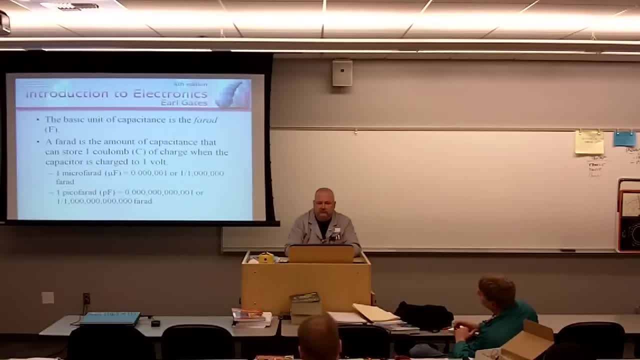 of the capacitor that the guy brought in from the defibrillator was No High Yeah. Yeah, I mean enough to kill you, But yeah, you could really don't do the stuff here. I mean, that's one of the things. 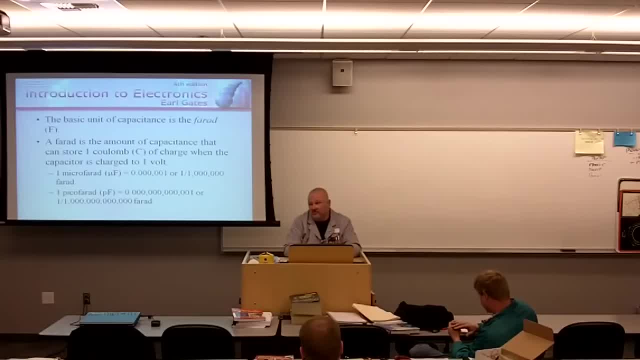 Again, we take safety seriously, But some of those big capacitors charge that up, leave that there. or you know, In the Navy, which was different, we were government property, you know? Oh, you used to do that crap. 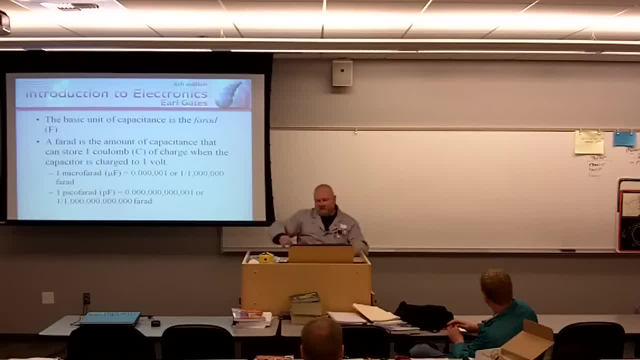 you know, charge it up. It's like, hey, check this out. you know, here catch Psh. ah, you know, Stuff freaking hurt man. You know you're gonna have to put a cap on your neck. 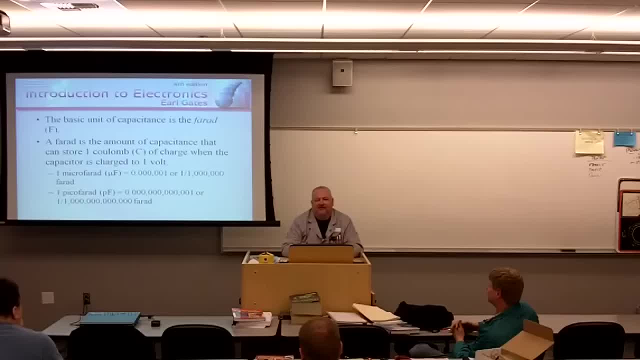 Chah Yup, these people weren't trusted with our nuclear arsenal. Basically, that's a high discharge device. You're using capacitors and inductors in there to create a high voltage to make someone compliant. A capacitor is either fixed or variable. 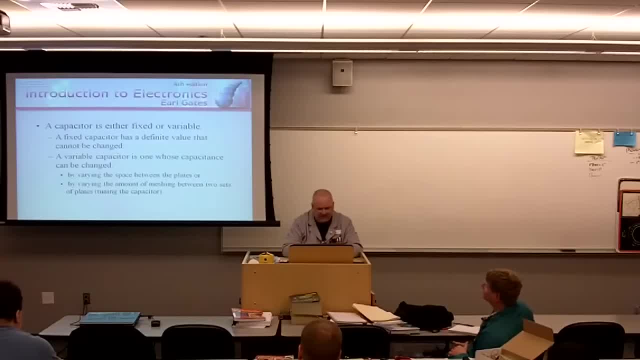 A fixed capacitor has a definite value that cannot be changed. It's made a certain way. if you will, A variable. a variable capacitor is one whose capacitance can be changed by varying the space between the plates or by varying the amount of meshing between. 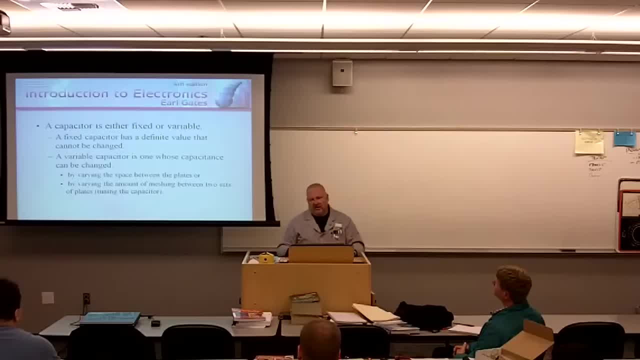 two sets of plates. Although they say mesh, the plates never touch. They have to be kept electrically isolated with an insulator in between, and that insulator could be air. Fact of the matter, you know if you have an insulator. 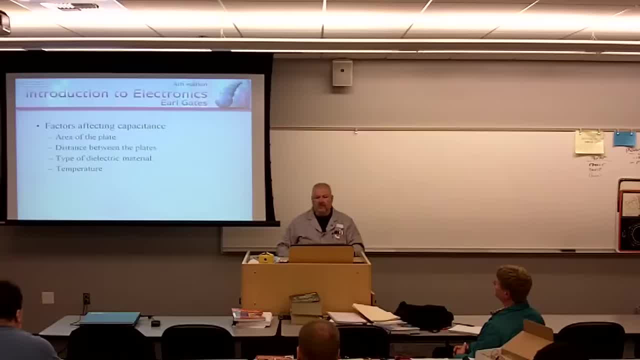 in between that insulator could be air. Fact of the matter, that insulator could be air Factors affecting capacitance. Now, this is kind of important to understand these. If you understand these, the math makes a lot of sense. The area of the plates. 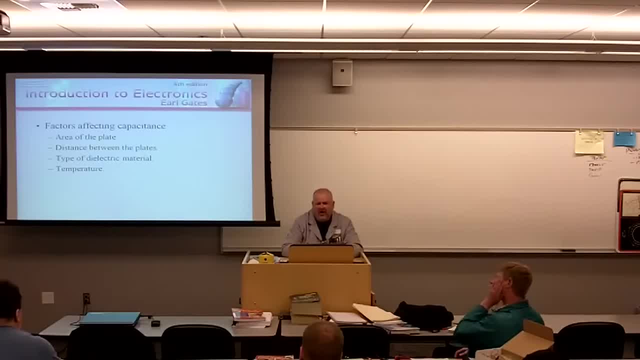 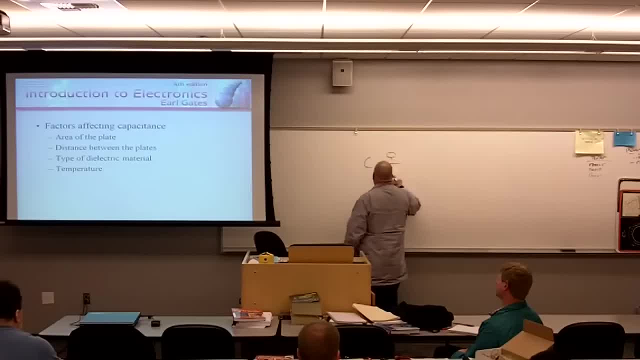 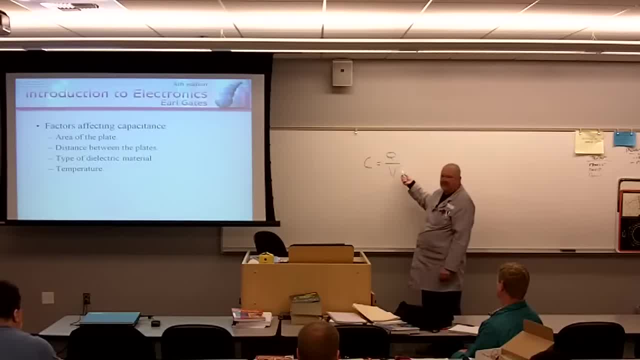 So area of the plate. What effect is that going to have? Is that going to affect Q or is that going to affect V, Q, Q? The bigger the plate, the more electrons that could park on the plate, physically, Right. 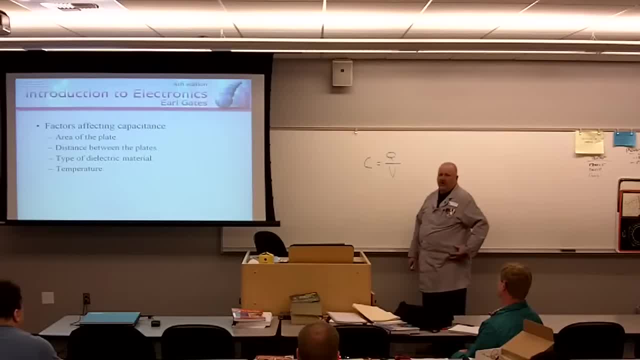 Because even though electrons are electrons, they still take up space, They still are comprised of matter. So very good. So the bigger the plates, what effect is that going to have on capacitance? Bigger plate, More capacitance, Smaller plate. 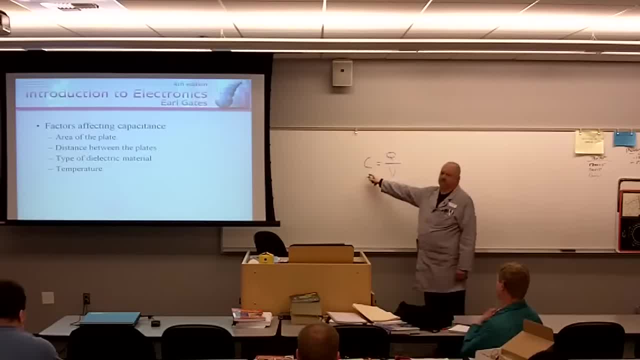 Smaller capacitance. Right Because Q and C are directly proportional. Right Because Q is sitting up on top of this here. Distance between the plates. Distance between the plates: What's that going to affect? It's going to affect the. 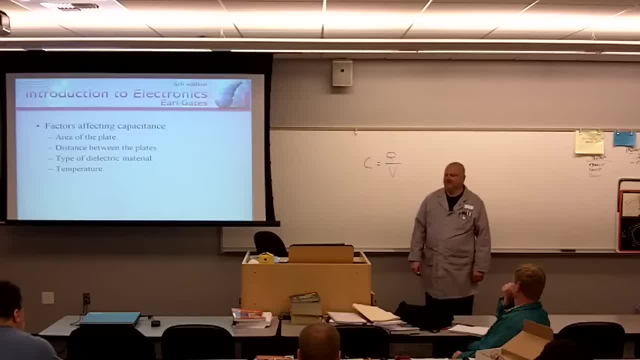 static field. So what's that going to affect Q or V? V? Think of the distance between the plates as like regapping a spark plug. That's the distance between the electrodes. This is the distance between the plates, The further that you move. 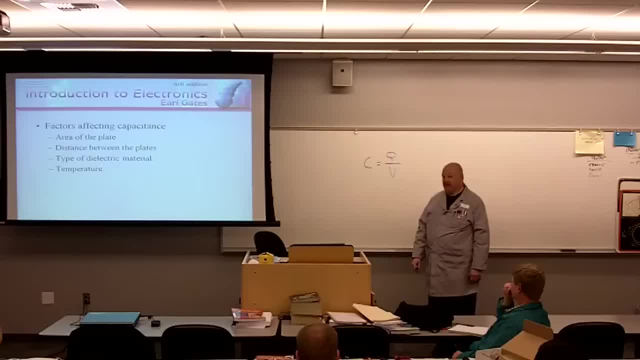 those plates away from each other, the higher the voltage you could store on those plates. And that's where engineers come in. Am I trying to store a lot of electrons? Am I trying to have a high voltage that I'm trying to build up across? 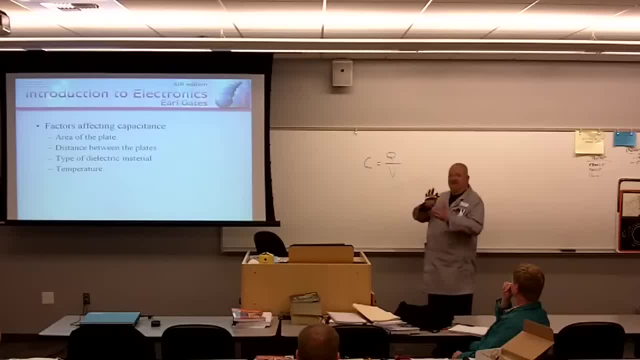 it. What am I trying to do? So engineers have to take that into account. So if I separate the two plates, that means my voltage that I could store is going to go down. So I'm going to start facing this compromise: Higher voltage. 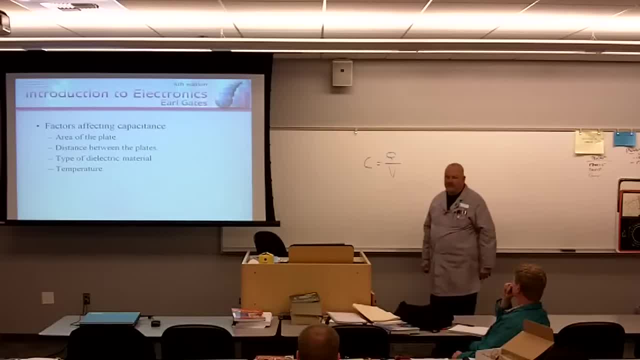 I could store, but I'm going to get less capacitance out of it. Why is capacitance going to go down too? Well, when I separate those plates, that electrostatic material is going to go down at a certain point, So I'm. 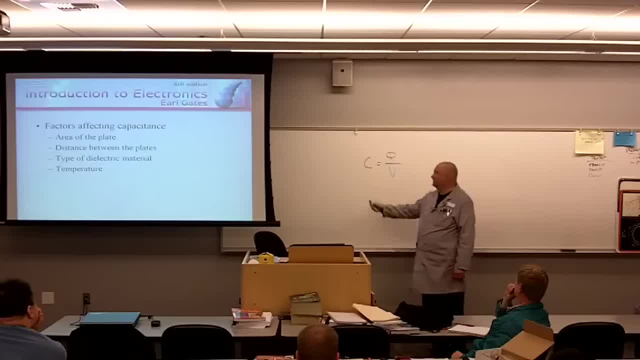 going to separate the two plates and I'm going to get less capacitance out of it. So I'm going to separate the two plates and I'm going to separate the two plates and I'm going to get less capacitance out of it. It's. 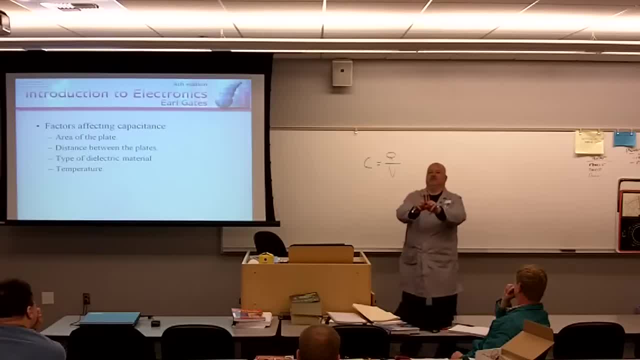 going to affect the voltage, because if I've got two plates separated by air and then now, instead of the air I slip in a piece of mica, mica has a higher dielectric constant than air. does it not Remember those two plates of insulators? 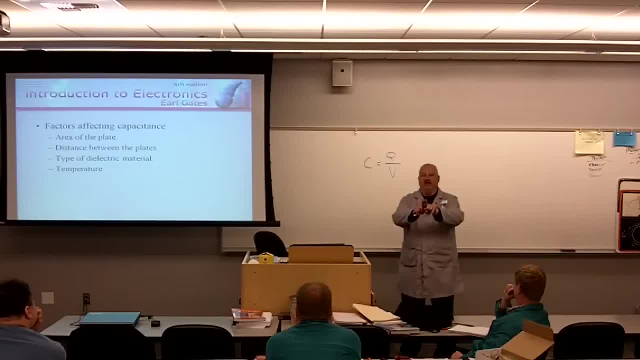 Mica was at the top of the chart. So if I slip a piece of mica between those two plates now, I can actually have those plates real close to each other and slip some mica in there and really get a high voltage across those plates. 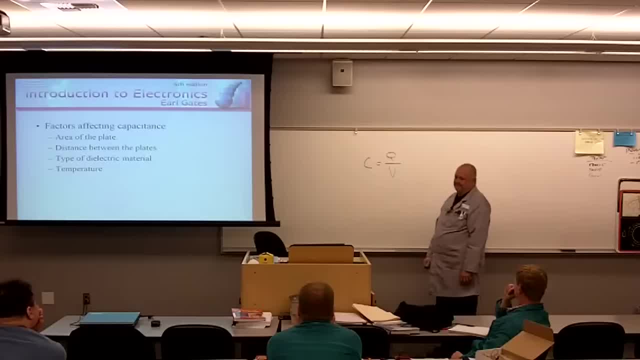 Get a higher voltage for the distance, and then temperature: Temperature. How is temperature going to affect this? What changes with temperature? Yeah, but we're not talking about resistance here, so It's actually simpler than that. It's something, probably, that you 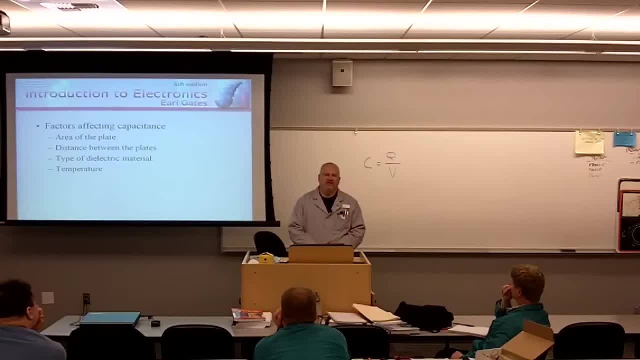 all knew even before you walked in here: Things expand and contract with temperature, right. That's why there's expansion joints on bridges. right, Because bridges expand and contract and if not, they'd break, you know, Oh no, it got over 70 degrees today. the bridge broke. It's going to affect V. So the bottom line is the amount of capacitance will vary with temperature. For some circuits, like at room temperature, it's not that big of a deal. 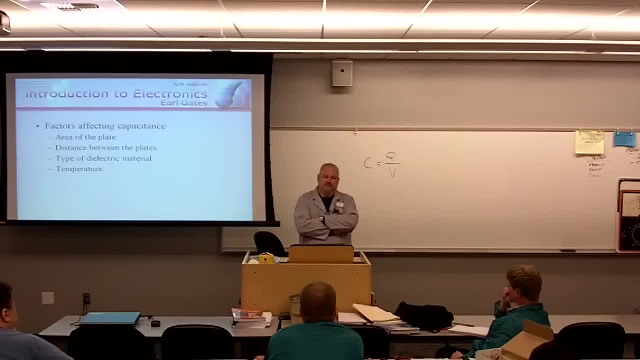 For some stuff. I don't think it's going to affect the temperature of the air system. So I think it's going to affect the temperature of the air system. So you know, I think it's going to affect the temperature of the. 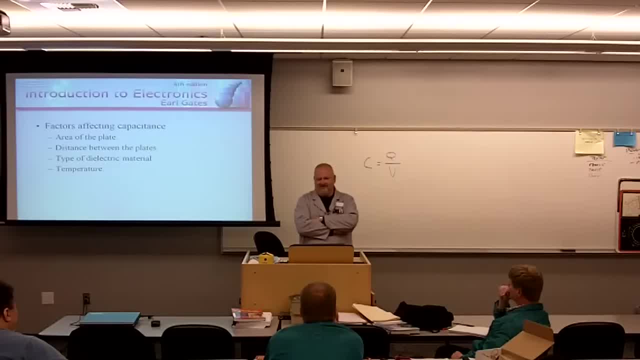 air And I think that's going to affect the temperature of the air. So for some of these circuits, I think that's going to affect the temperature of the air. So I think that's going to affect the temperature of the air. So I 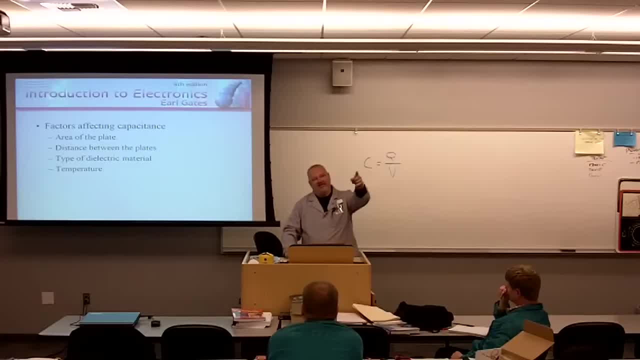 think that's going to affect the temperature of the air. I think that's going to affect the air And I think that's going to affect the temperature. are like woohoo, Because what they did is they not only got to take off, but they got to go supersonic, They got. 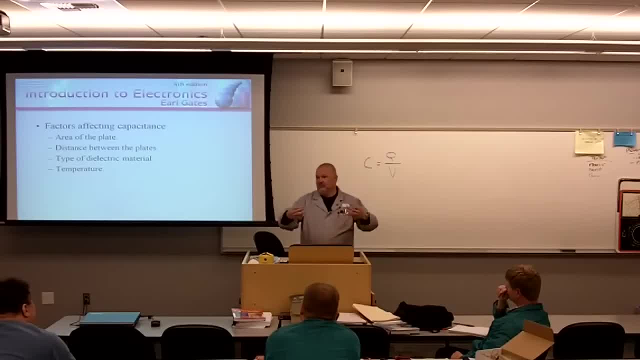 to go on an intercept call. So what they did is they went supersonic- I'm sure you all heard about it- with the windows getting knocked out and the sonic booms. Okay, Where I'm going with this, though, is imagine that airplane sitting on the runway down there. 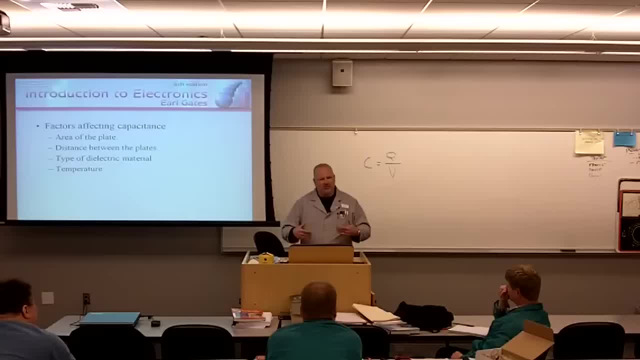 in the middle of summer sitting on the tarmac 115,, 120 degrees, and then 60 seconds later he's at 45,000 feet where it's negative 45. If electronics are not all in heated areas of that aircraft. so if you've got a 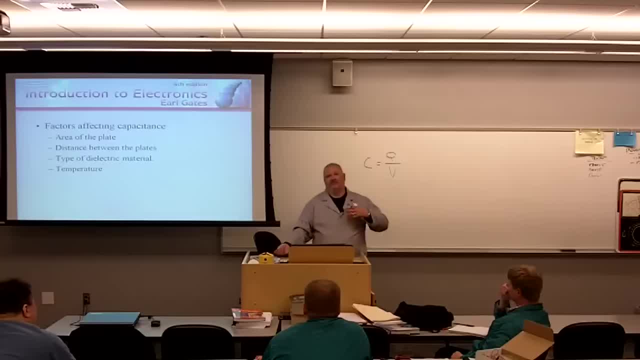 capacitor that is, in an area that is prone to temperature change, you're going to get different results. Hopefully that's not part of a targeting system on that aircraft where all of a sudden, the military is smarter than that. The reason: temperature that it always strikes a chord with me. 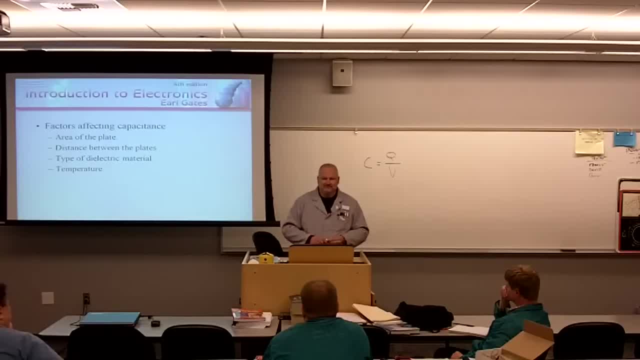 I was not always the best student, Especially when I was in a lot of military schools. I went through over 4,500 hours of military schools, Different systems. I was in a great position because as soon as the Russians came up with something, we had to come up with something to detect it and counter it, and I was constantly in school. 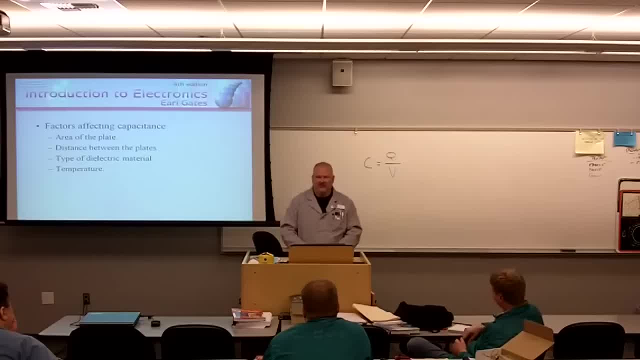 Traveled through 46 of the 50 states on official business, going to school. A lot of factory schools, a lot of stuff, Long schools, And it was not a school day like yours. These are eight hour days, Eight hour days, five days a week. 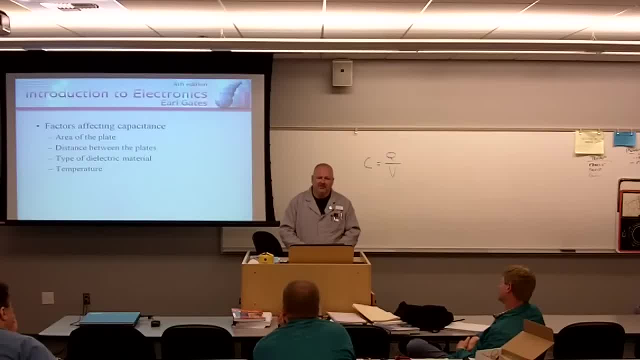 And it was back in the day, old school, So we used to go out for liquid lunches And I used to sit in the back. and I was sitting there one day and I'm, like you know, falling asleep and hopefully not snoring too loud- And I wake up and the instructor is showing. 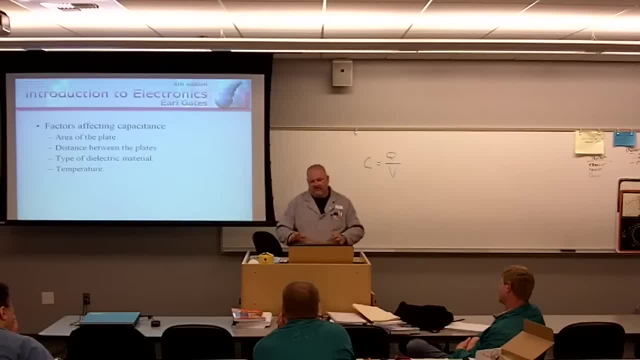 me this: you know they have the presentation and they had not PowerPoint. they had the view foils And they're showing this oven ready light coming on And I'm like oven ready light, Oven ready light. I like I'm in electronic. 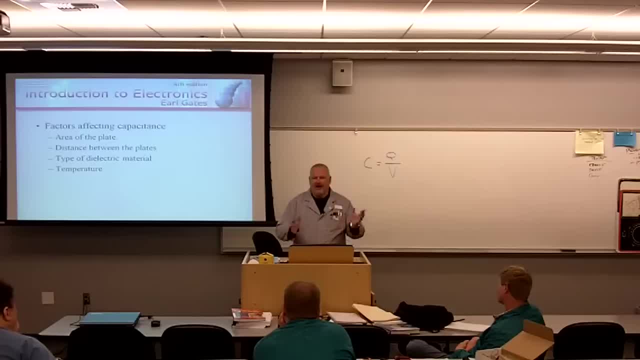 intercept and analysis. Why is he talking about an oven ready light coming on? I mean, if this is like, I picked the wrong time to wake up because I don't have a freaking clue what he's talking about- An oven ready light, And I'm just trying to wrap. 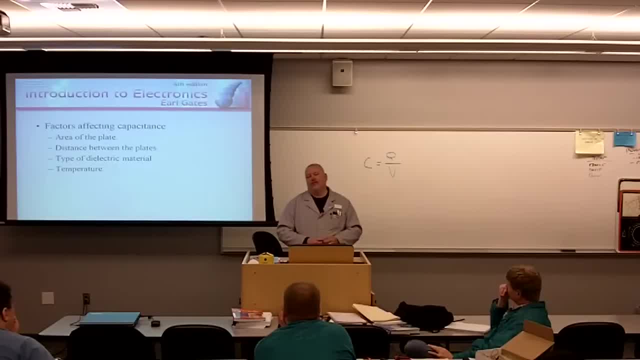 my mind around it. Actually, what happened is this equipment was so sensitive- it was very secret, special equipment for measuring these very specific emissions from Soviet equipment- that they put key sensitive temperature components in what was called an oven, And what it was is a small metal box inside. 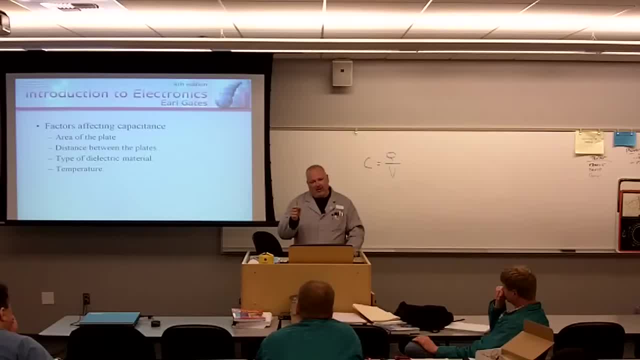 the piece of equipment And it had a heating coil and it had a thermostat and it would keep that temperature stable So that the readings would be stable. And if that oven ready light was not on, that told the technician that the oven wasn't on and the numbers the results. 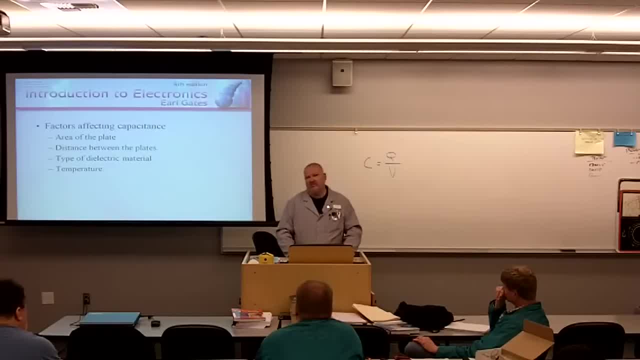 could not be trusted. So that was a big thing. before you use that equipment is verifying that oven ready light was on. It was like it's funny because even though I slept through the lecture, I still remember it, like it happened yesterday. 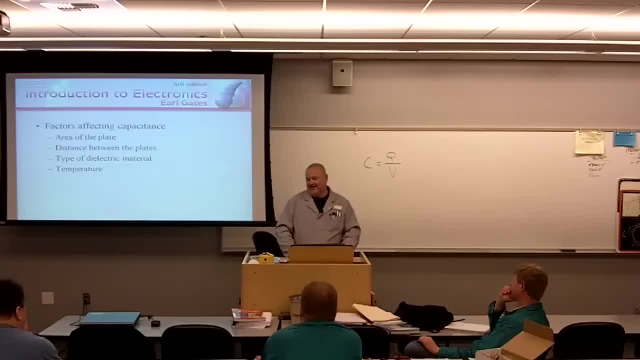 This is not an endorsement to fall asleep in class, But it was a blue light. It was this blue light And I always remember, because I'll tell you what we had. our labs were written tests and then we had practical labs that you had to go in and troubleshoot that equipment. 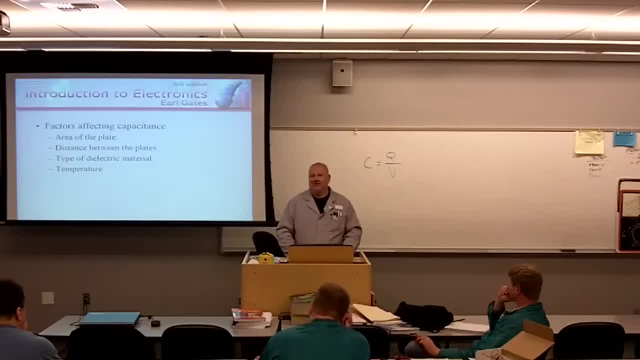 And I remember that the day I went into- you know I was basically being evaluated- I had two instructors standing in there with clipboards and you know let's see how Petty Officer Greinick evaluates this problem here. So I walked in and the first thing I noticed is the blue oven ready light was not on. 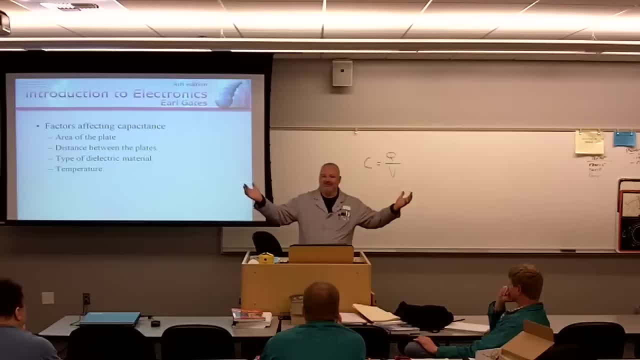 So I knew immediately where the problem was And I you know, I told them: oven ready light's not on, There's a problem with that circuitry. got in there and basically it was like a fuse that was blown. replaced the fuse boom fixed the problem. 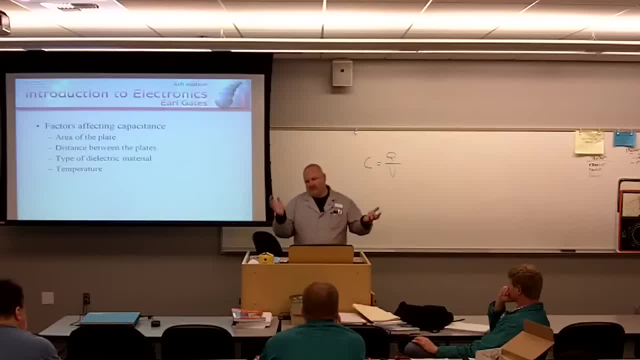 If you're not a vigilant technician paying attention to that. oh yeah, you could run through all the tests. oh, everything's working okay. So some key components like capacitors that are in real critical roles in circuits may be put in a circuit. 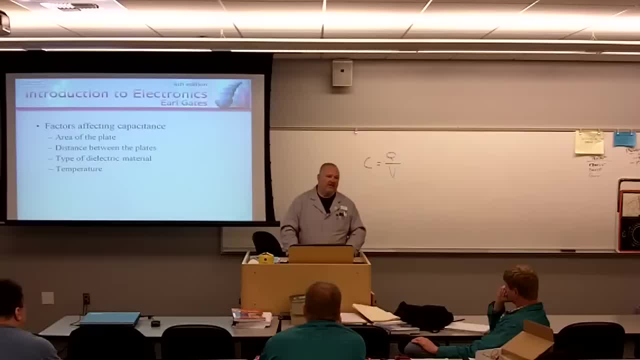 or in a box called an oven where they keep that temperature really stable. For most stuff like this, you know inside buildings and you know whatever industrial controls. it's normally not an issue, Normally even an automotive application. I've never heard about anybody. 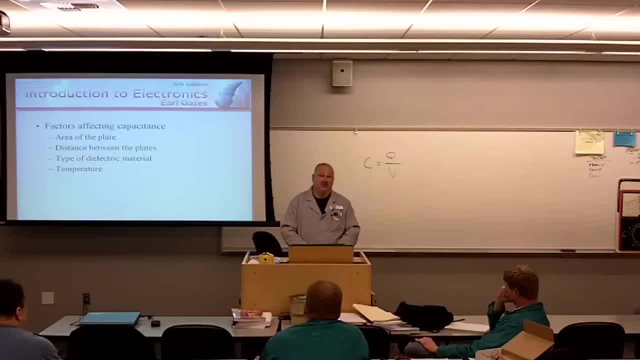 you know, and actually cars are pretty freaking robust when you think about it. I mean from you know, I've been down in Arizona in the summer. you know it's like stuff is melting. plastic is melting. you know your tires are melting on the cars. 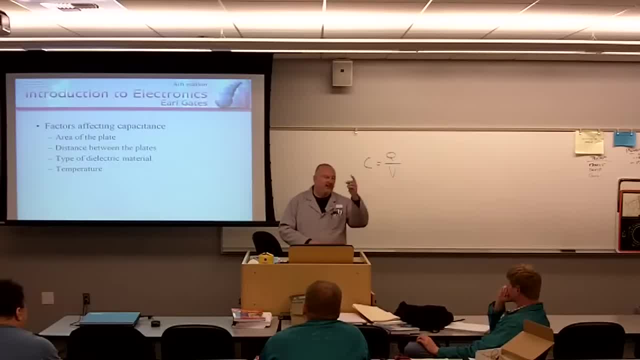 it's just nuts, you know, And I went up to Alaska here in February and you know that was like the week before I was up there was negative 47. So you go to Fairbanks Airport, you land, you're going to rent a car and it's buried in snow. 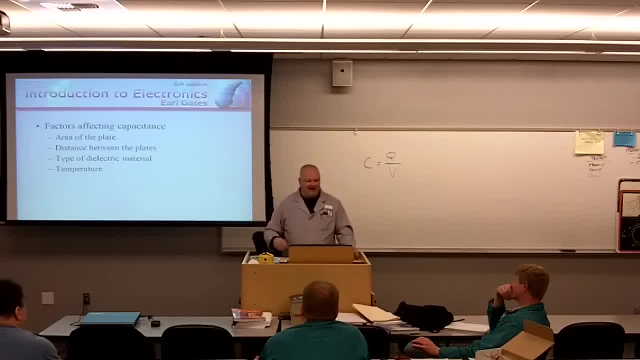 but you just follow the extension cord from the post and it's all on a block heater. you can dust it all off. it's all powder snow up there because it's so cold and so dry. Turn the key, fire it up Every place you go. the hotels all have a place to plug into the. 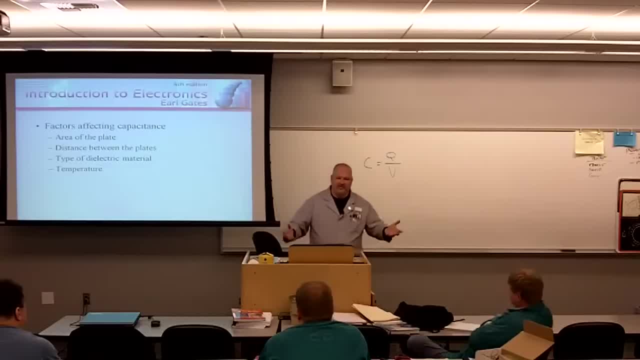 I mean, it's just you know, but still that extreme cold is like wow, the electronics work reasonably well From Arizona to Alaska. Keep these four factors in mind. they're critical Dielectric constant: this is the measure of the effectiveness of a material as an insulator. 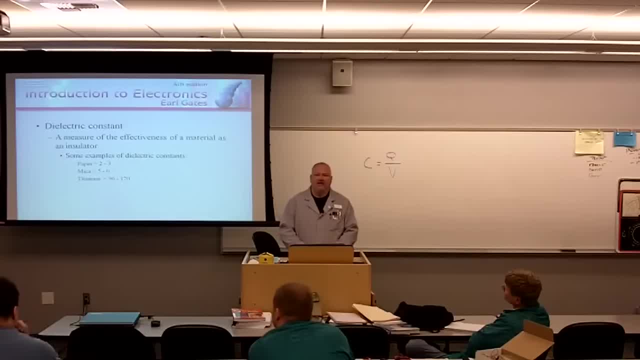 Some materials have dielectric constants. paper has a dielectric constant between two and three. Typically, what they're talking about here is wax paper, Wax paper- Wax paper used to be used as the dielectric, as the insulator, in a lot of capacitors prior to World War II. I've actually restored many an antique radio by simply going in, removing the paper caps that have deteriorated and putting in mica caps of the same value. Just that easy remove it. Everybody always gets an old radio and oh yeah, it must be them. there tubes. Them tubes there need to be replaced. I've restored a handful of radios, haven't replaced one tube. Got in there, replaced the capacitors. Why Paper capacitors? What happens to paper over time? Deteriorates It deteriorates, loses its dielectric constant. 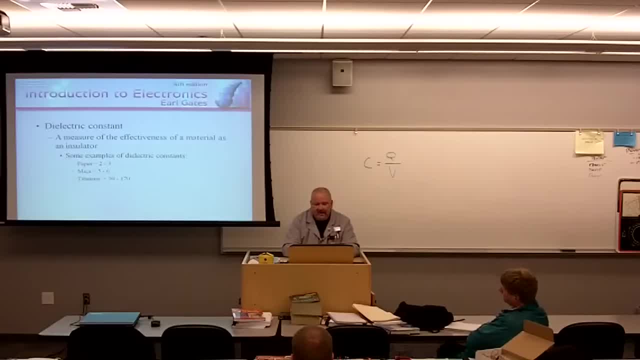 capacitor shorts out doesn't work. Mica dielectric constant between five and six. This should be tantalum, not tantalum Titanium Titanium. they're using that in golf clubs and Soviet submarines. This is tantalum. Tantalum is a material that has a high dielectric property. So by putting it in a tantalum capacitor it gives you a big bang for the buck. Some of the best capacitors that money will buy: Tantalum Electrolytic capacitors. These are large capacitance for size and weight. 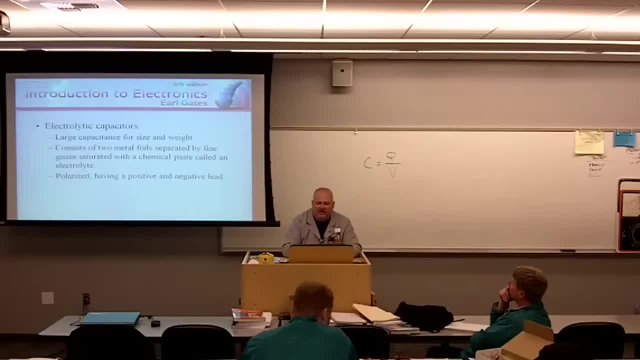 Consist of two metal foils separated by fine gold saturated with a chemical paste called an electrolyte. They're polarized, having a positive and negative lead. If you put a electrolytic capacitor into a circuit, backwards it will splode. 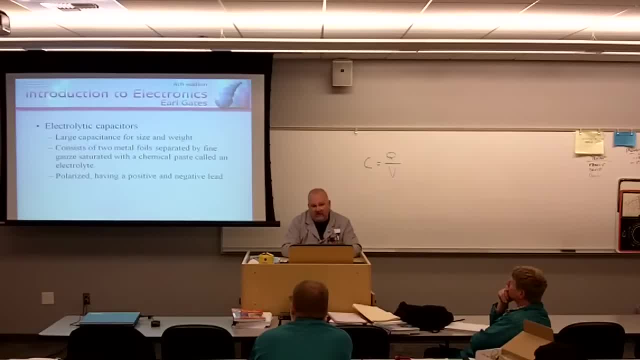 Literally, If you put one of these in a circuit backwards, it will explode. Some of the smaller caps actually have where, like, there's an X etched on the top, so when it blows it'll blow outward and not necessarily build. 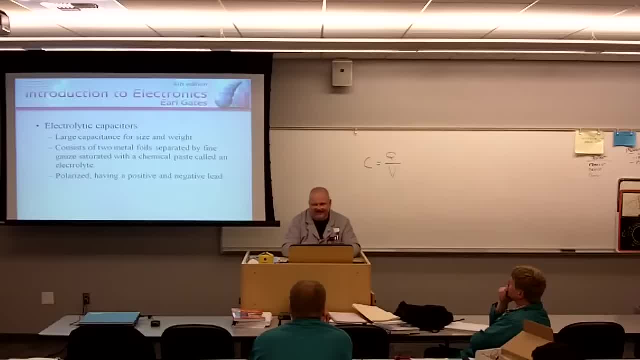 I don't know. I knew a guy that likes to play around with explosives and stuff in the past. You know it's all about keeping it compressed, Those gases you know compressed, And that's going to give you a bigger bang. So some of those small caps that don't have a little release mechanism on that you can throw some shrapnel. Some of the big caps actually have a release valve on it, So if you put it in backwards, pow. But I've seen smoke pouring out of them like a smoke bomb. 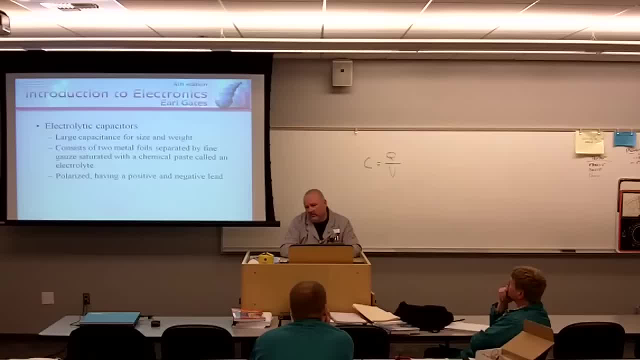 If you ever want to blow up caps, let Peter or myself know, And we want to do it in a controlled, contained environment. You just do it for kicks in the lab. somebody could lose an eye seriously, You know, because they're little metal cans. 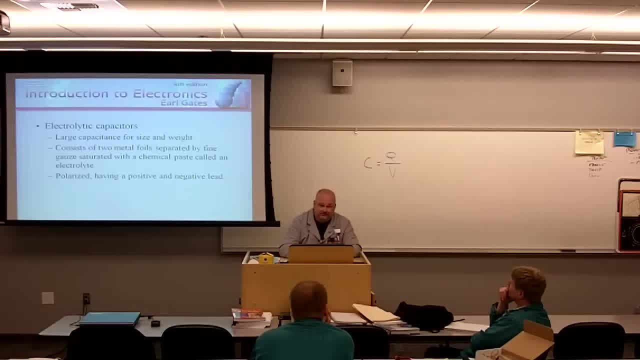 And you put it in backwards. these things blow, Shrapnel is going to go flying. I've done it before. out in the back, You know, we rope off an area. It was actually funny. We were doing that One evening years ago, blowing up capacitors, you know. 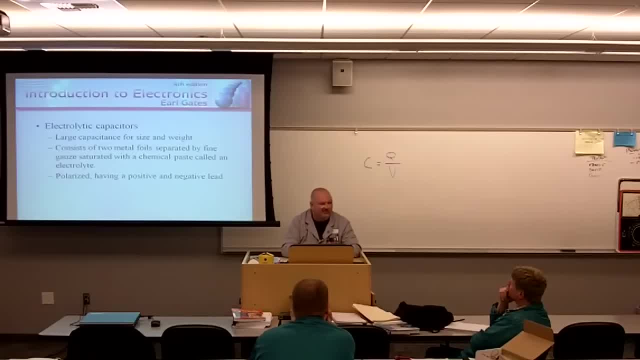 And pow, pow, pow, pow. We're putting them in series and parallel and doing all kinds of wacky stuff. you know, And literally I had, We were doing it in the back here And you know the second floor up above the restaurant. 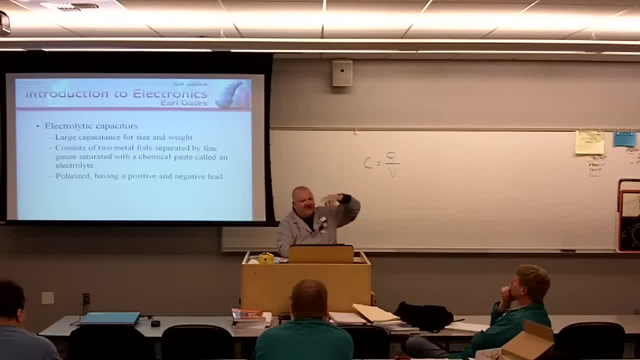 that patio area between the two buildings. I had debris raining down on that So nobody really cared any about it until I went to the custodians and I asked for, like some you know, brooms and stuff to clean it up. 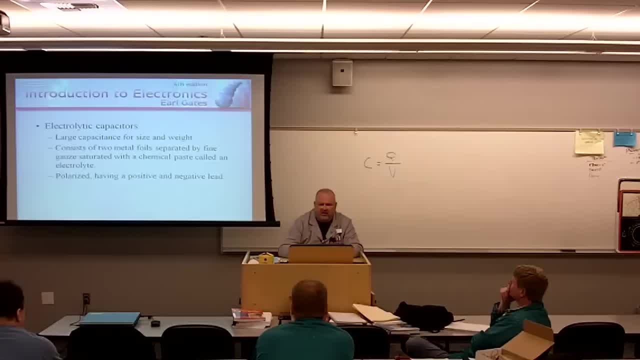 And then it was kind of like: well, they all got puzzled and stuff, because they're like all union here And they're like if it's a mess, you know we need to clean it up. It's like: well, my students made this. 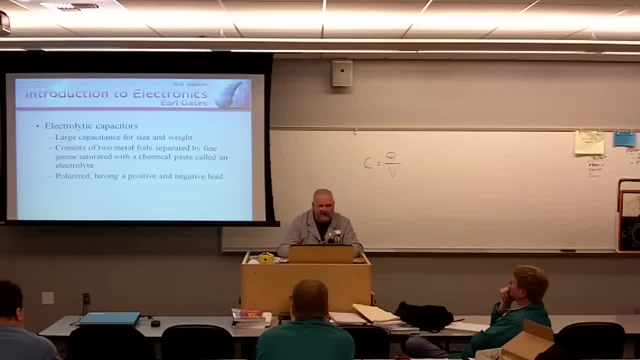 freaking huge mess out here from blowing up crap. Well, no, no, we'll clean it up, you know. Oh, I'm sorry, you know, File a grievance because we're going to clean up the mess we made, you know. 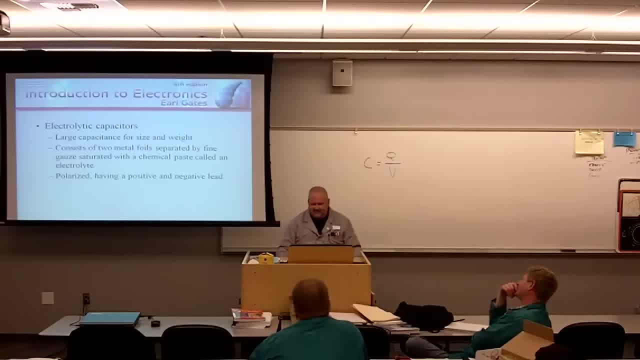 So it was just an odd time. I guess it's still an odd time you know here, But it's my personal collection of capacitors. These are all electrolytic capacitors, And on the electrolytic capacitors you've got to look for the markings here. 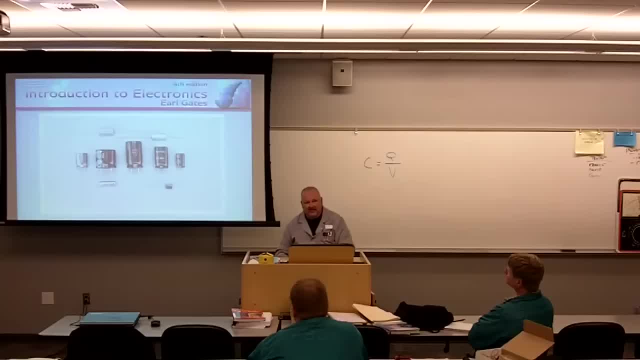 to find which lead is the negative lead and which one is the positive lead, And there will be some discerning mark on it. Some manufacturers identify the negative lead, some identify the positive lead. You've just got to pay particular attention. This here like with the band on it. 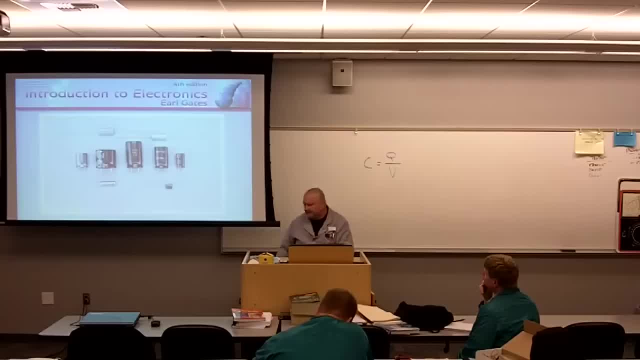 that would signify the negative lead. See that solid band. You've just got to look and be observant. Put it in backwards, It will explode. Paper and plastic caps. construction by a rolled foil technique. Plastic film is used more often. 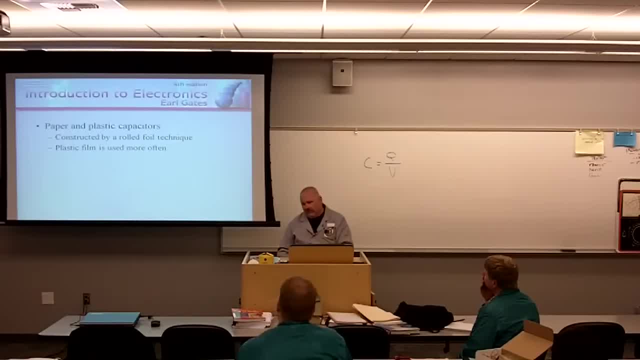 Basically, if you went and got two rolls of aluminum foil and a roll of wax paper or a roll of saran wrap, right laid out one roll, put the insulator on top of it, laid the other roll out, rolled it all up. 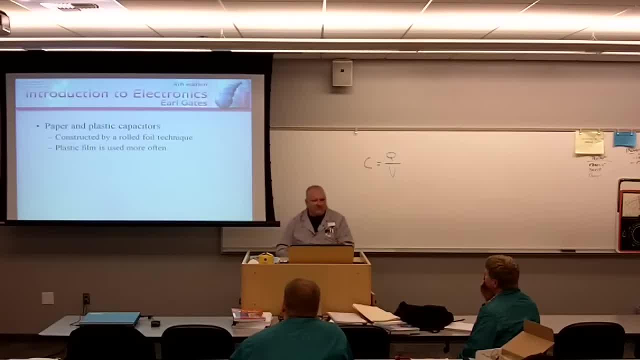 dipped it in wax. attached leads to it. dipped it in wax, you just made yourself a capacitor. So if you want to roll your own, you can roll your own. You make it out of paper. same thing, And that's exactly what paper caps were. 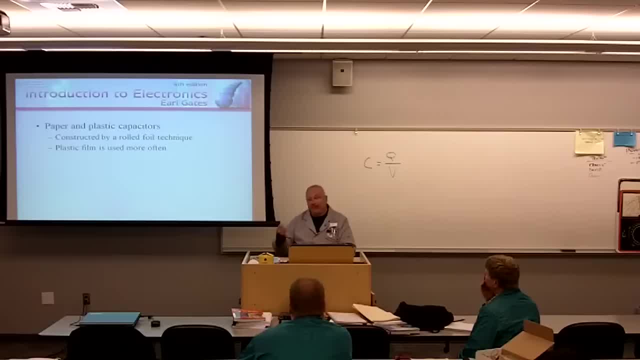 Two pieces of foil with wax paper between them, the leads attached dipped in wax zip And that wax didn't prevent that paper from deteriorating over time. These are plastic caps here, Basically. if you slice that open with an exacto knife, 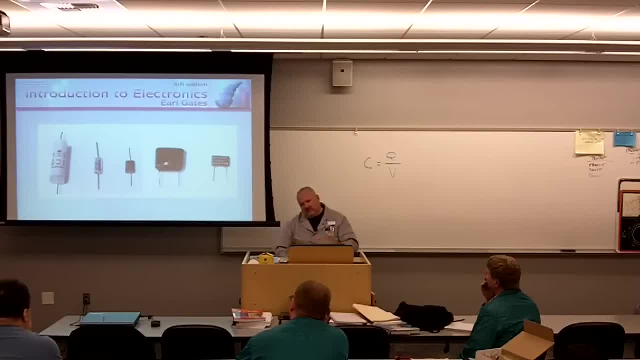 you'd find nothing but rolls of aluminum foil wrapped around plastic Ceramic disc capacitors. popular because they're inexpensive to produce. They're used for values .1, microfarad and smaller. Ceramic is the dielectric. They're reliable general-purpose capacitors. 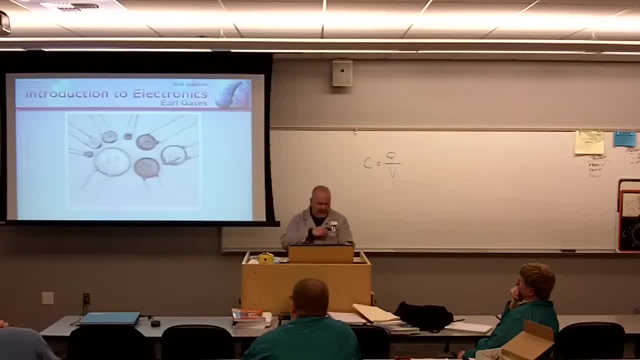 This is my personal collection. I get all my ceramics from Mexico. I get a lot of them manufactured there. It's not electrolytic Ceramic. These don't have a positive or negative lead. It's only the electrolytic that does. Check out the value of this. 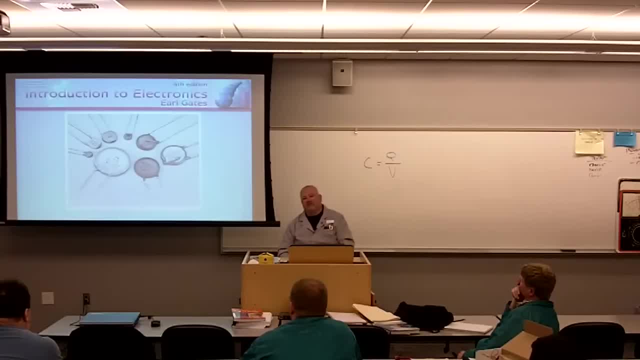 This will have 3 kV. It'll hand up to 3,000 volts. You exceed that, you destroy the capacitor. You operate all day long underneath that. Variable capacitors are also known as patters, trimmers or tuners. 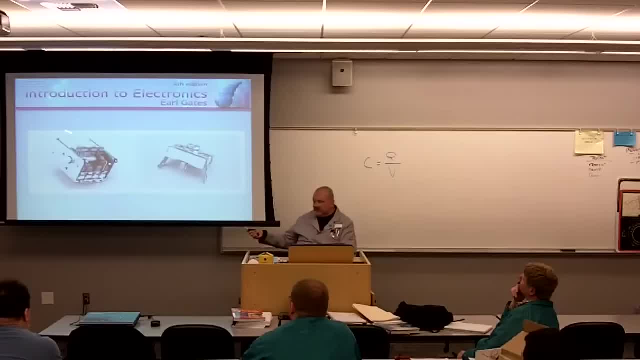 This is a tuning capacitor. This is something you'd find in a 1960s, 50s, 60s, 70s radio: Elegant, Elegant in design. They don't make stuff like this no more. How many of these went to the landfill? 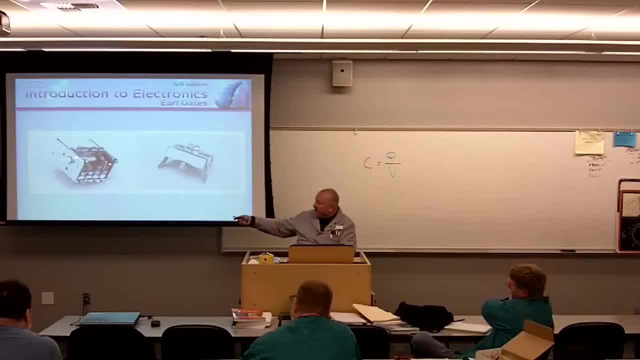 A lot of these. the shaft right here- this would actually be ball bearing movement right there with the heavy grease in there and you turn it ever so slightly. Actually, what they would do with this, they'd put a big pulley on here. 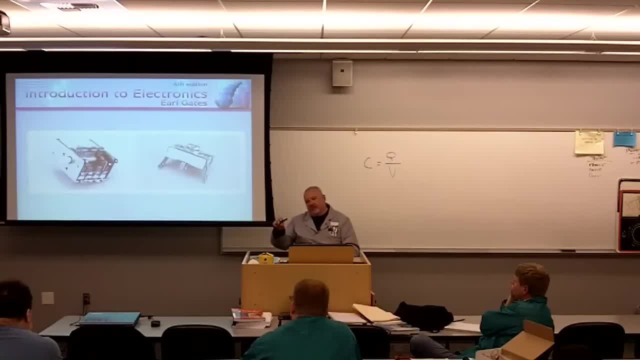 and then there'd be a string that was attached to your tuning dial. When you move that knob just a little bit, it would ever so slightly move that tuning cap, and that's how you would adjust. by adjusting the capacitance you would tune your radio. 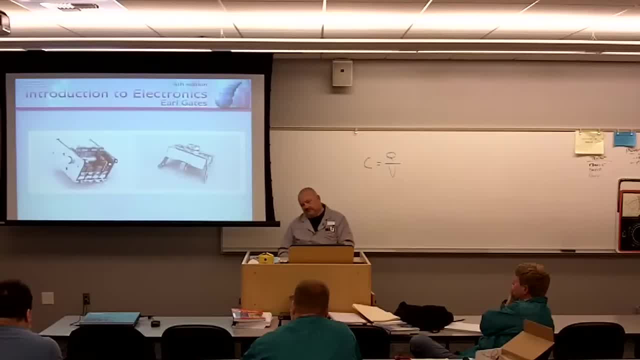 Now it's done all electronically, So this is something kind of from a bygone era, Which is good and bad in some ways. I don't know. Well, I don't think these new tuners have the sensitivity that those old tuners had. 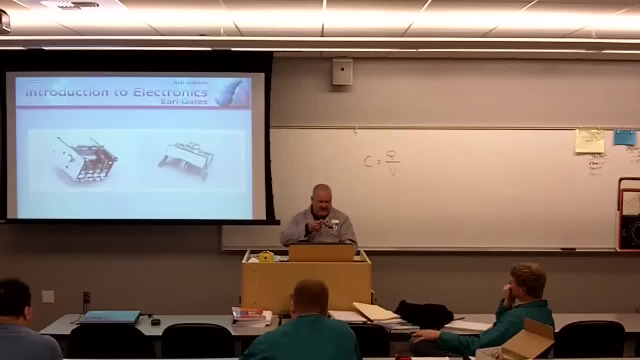 And I saw the transition of the military When I first got into electronic intelligence gathering. they were manually operated tuners. I mean I used to have to sit there and manually tune through, find a target of interest, intercept it, analyze it. 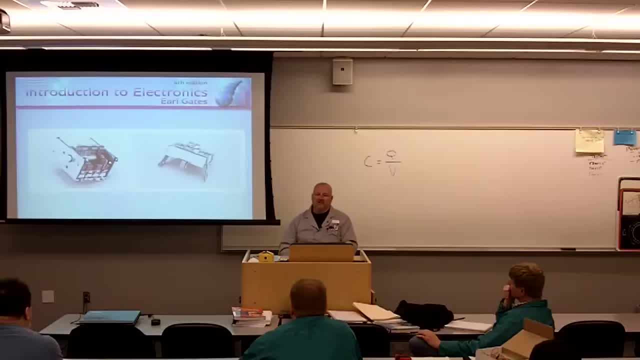 I saw the transition to computer operated systems And it boggled my mind. I was actually. I rode my submarine out here. my sub was going to get a new system, so I rode it here. the work was being done in Bremerton. 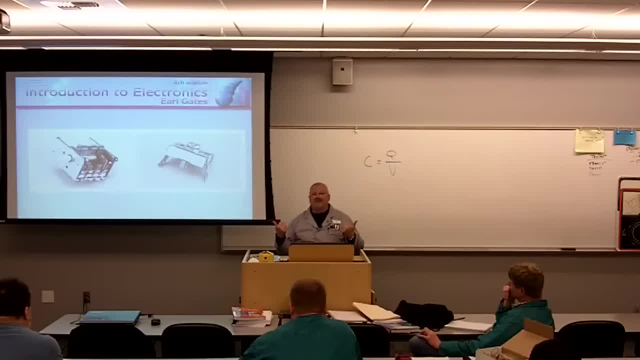 then they flew me back to Connecticut for the summer. Actually I drove. It was kind of funny. I used to tell the Navy I had a fear of flying. That's why I'm in the Navy. So because I would go to so many schools. they would always they'd pay me to travel, So it was like I don't know 300 miles a day, per diem and hotels and whatever. So I used to like get like 14 days off the drive to Connecticut So I'd like go to San Diego. 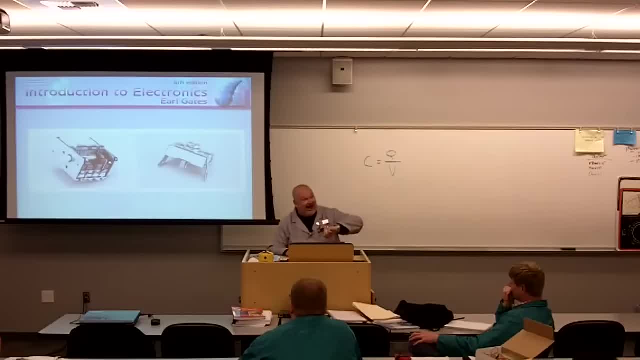 and goof off for a week and a half. Crap And I'd like marathon across the country or whatever you know. Anyway, I was getting sent to this school where it was going to be computer-controlled receivers And my computer-controlled receivers. 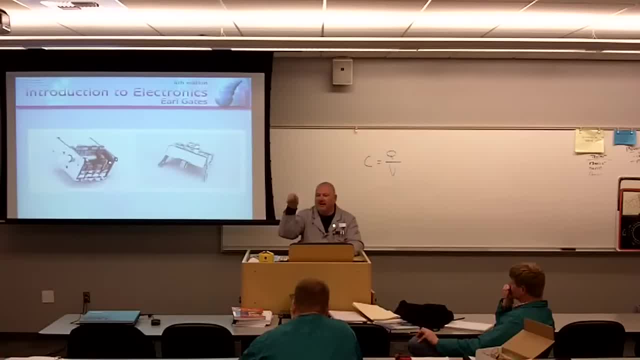 I mean it was like it's like some robotic arm is going to come out and like tune the dial. I mean how do you do that? I mean I'm serious. I was just. I had no freaking clue what they were talking about. 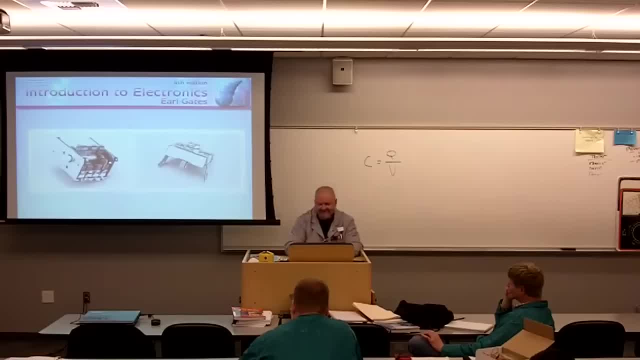 And that's not what they were talking about. But I just don't think we ever had the sensitivity that those old manual tuners had. The newer systems, of course, were much more efficient And they, you know, once you integrate computers. 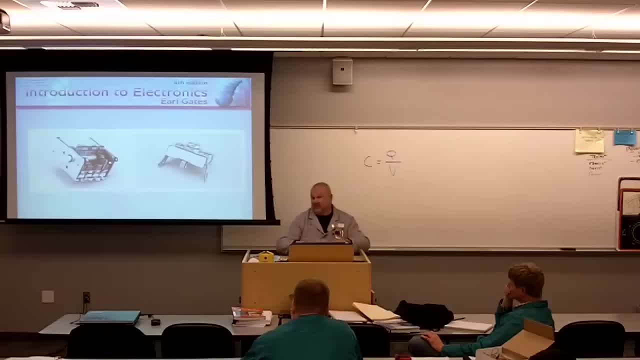 you can process the data. The data's only getting processed as well, as it was programmed. But yeah, those old tuners Boy, I could listen to some stuff way out, way out there. We'd be way the heck out in the middle of nowhere. 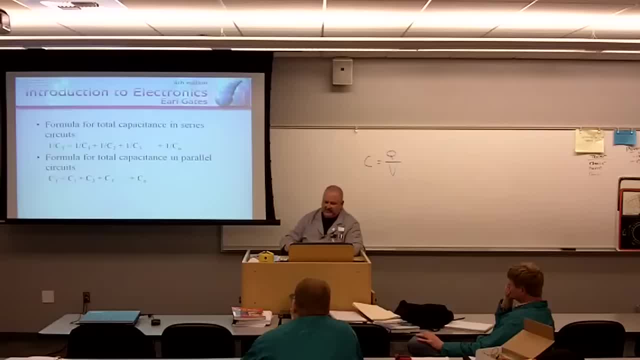 and I could tune stuff in with a good antenna and good receiver. Series capacitors- Yeah, you're not looking at a 10-inch one, That's a typo. When you have capacitors in series, you treat them like resistors in parallel. 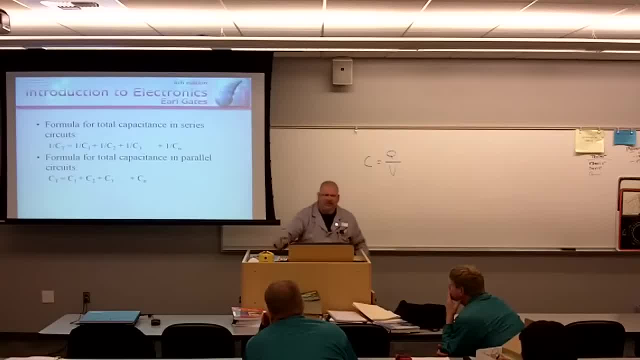 Does anybody know why that is? Why do you suppose It's a good try? Okay, these three capacitors are in series, are they not? What am I really limited to here? I'm limited to this plate area here, am I not? 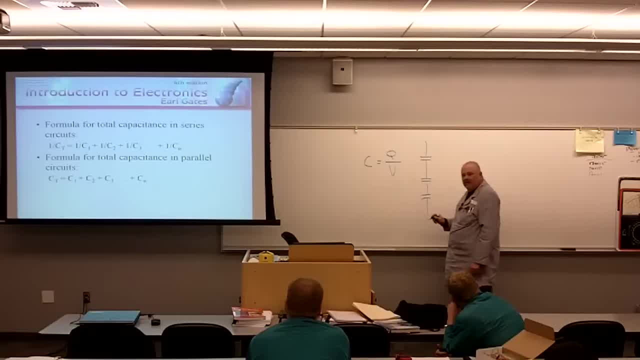 And this plate area here? What am I actually doing? I'm increasing the distance between the plates, which means my voltage goes up. That means my capacitance has to go down. Make sense. That's why that formula works: Plus I got. now I'm getting one, two, three times. 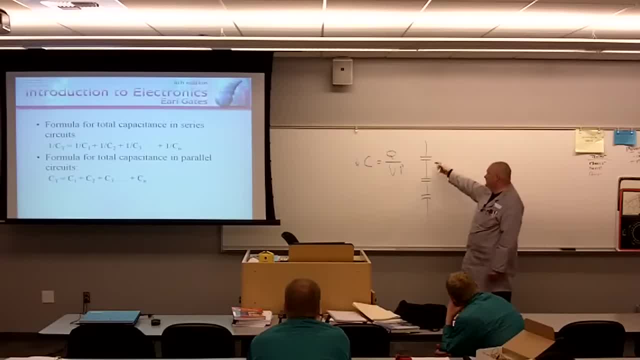 the insulated material, as opposed to one time the insulated material Make sense. So everything always goes back to this formula. Everything in electronics always is explained away with a formula In parallel. What am I doing here? I've got this plate, this plate and this plate. 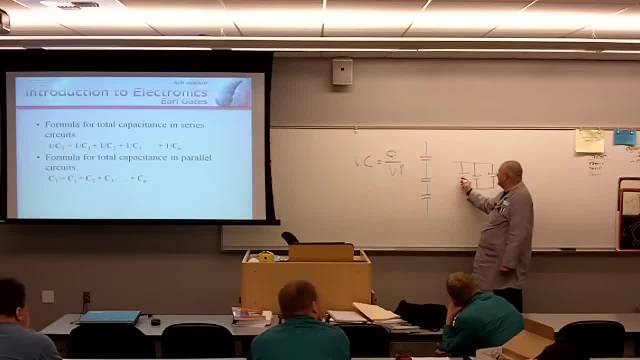 Now here: I triple the size of my plates. I tripled the size of my electrostatic field that I could build up across the two. So what am I doing? I'm increasing my Q, which increases my C. That's why that formula works. 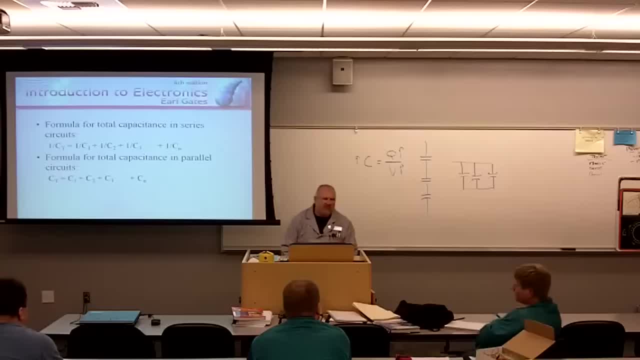 So I don't know if that helps you, but it helps me remember formulas, if I understand how the formula works. If I just give you a formula, C is equal to Q over V. Okay, I'll remember that. That's not going to do you any good. 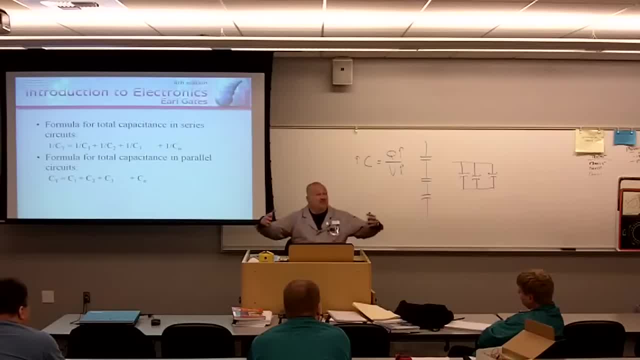 If you remember, C is equal to Q over V. Increase the area of the plates. I could store more Q. Q goes up, C goes up. Distance between the plates increases. V goes up, C goes down. Inverse proportional relationship. 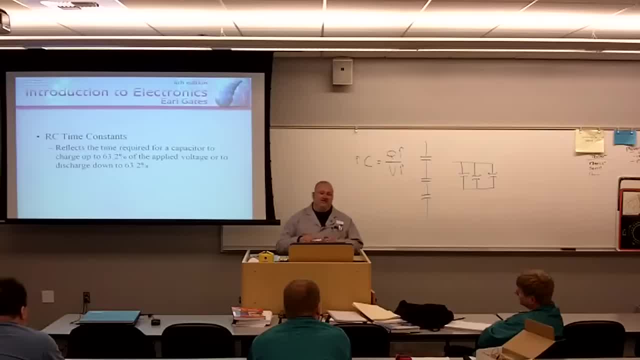 Make sense. RC time constants reflects the time required for a capacitor to charge 63.2% of the applied voltage or to discharge down 63.2%. It's not a typo. It's the way I worded it intentionally on this slide. 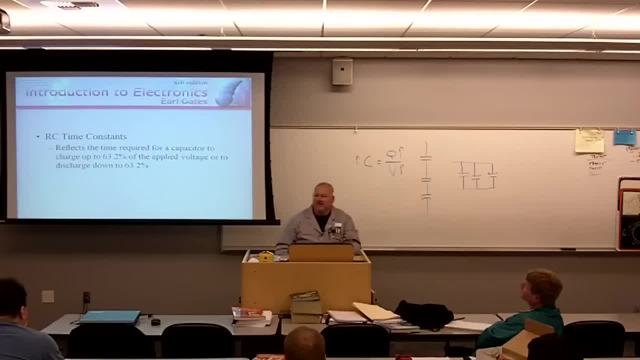 You're decreasing down 63.2% to 36.8%. This is what the circuit's going to look like. This is the formula. T is equal to R times C, It's going to take five time constants. And physically, what's happening with this? 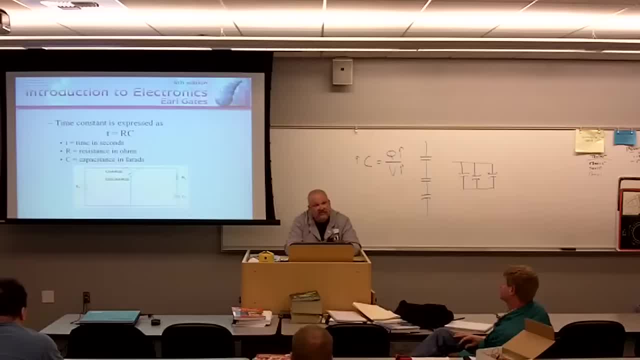 what kind of a circuit is this Series Series RC circuit? It's a series RC circuit And when I close this switch, this capacitor here is going to be at zero volts and it's going to start charging up to 100%. How long is it going to take to get to 100%? 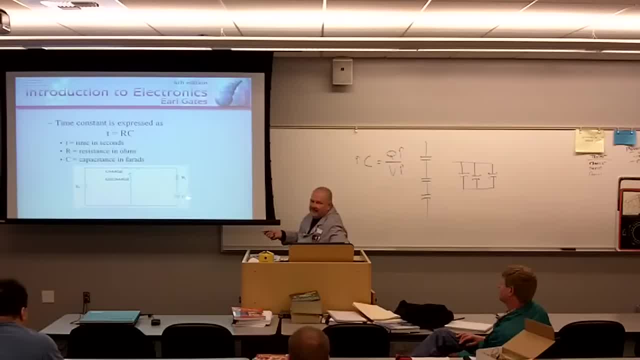 Five time constants. How do I figure out what one time constant is equal to? T is equal to R times C When this capacitor is at 100%. what voltage is going to be across R1? Zero When capacitor C1 is at 100%. 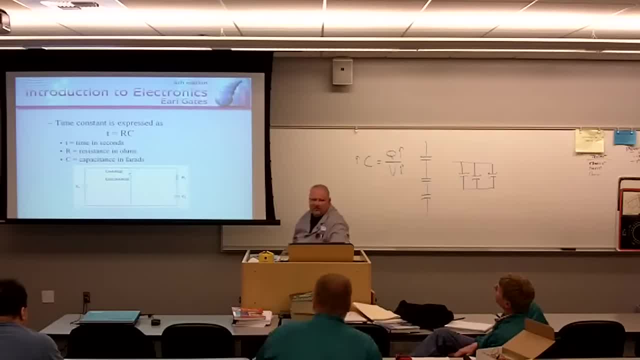 after the passage of five time constants, what voltage is going to be present across R1? Zero? When 63.2% of the voltage is across C1, where's the remaining voltage going to be Across R1.. So basically, as the capacitor is increasing in voltage, 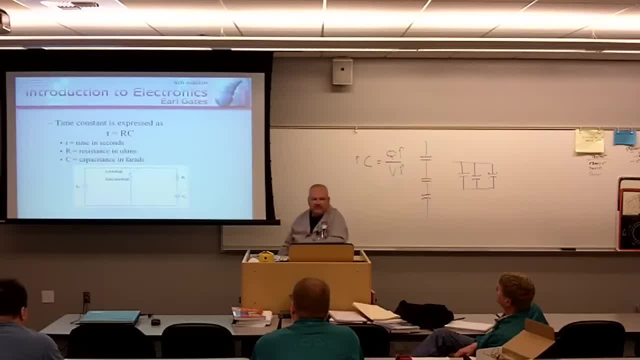 the resistor is decreasing in voltage Because this is not only a series circuit, it's also a voltage divider. It's a voltage divider After five time constants. this voltage will be equal to this voltage. Voltage rise, voltage drop- After five time constants. 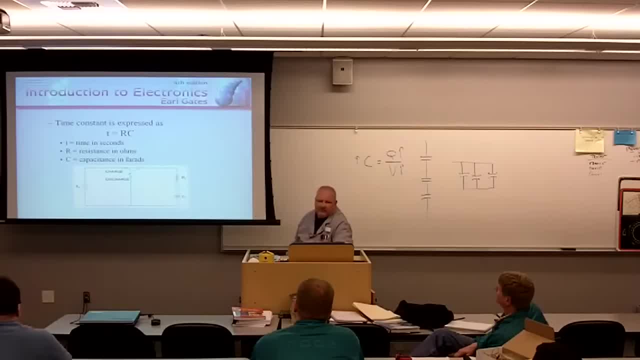 this is equal to this, which means there's zero left over Kirchhoff's Voltage Law. Everything always goes back to what we talked about. I'm really not talking about a whole lot of new stuff here. I'm getting paid to talk about the same old stuff. 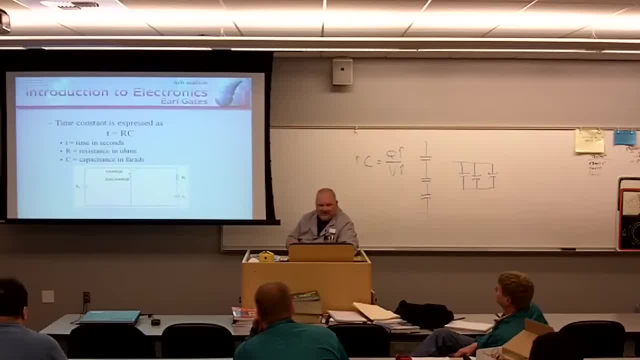 Just every week I introduce a new word. This week it was inductance Capacitance. Why? Because in five times you basically get close to 100%. That's why we call it five times. It's really between five and six times. 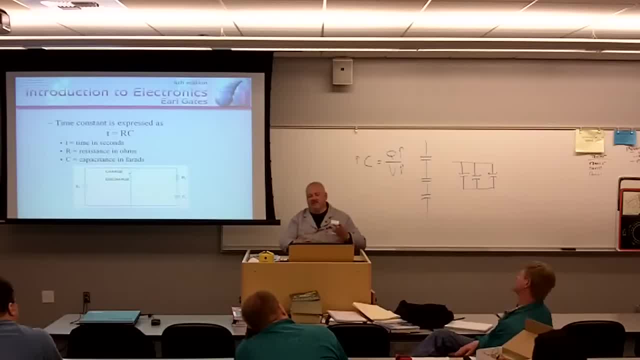 Some books say six time constants, Some say five, But you're so close to 100% Because the six would be 63% of 99.3%. then For the sixth consonant, Because on the fifth consonant it would be 99.3% right. 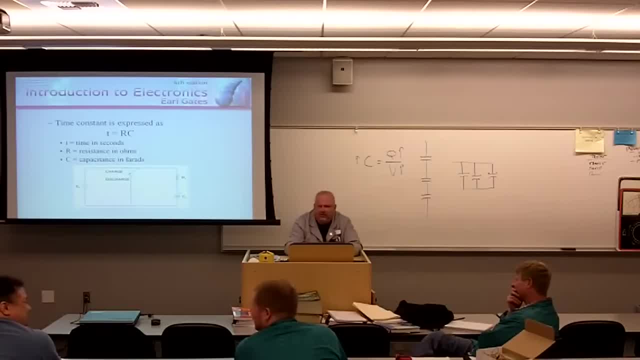 Right After five time constants. we call it even. We just say The books that you say do sometimes have a six time constant. Well, yeah, I mean, if you're dealing with real high power stuff, that could be a difference. 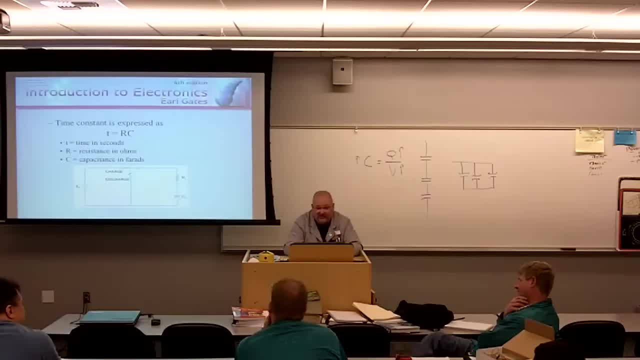 If it was high power and a high voltage it could be the difference of a couple volts, That small percentage, But generally it's accepted five time constants. Every exam you take here it can be five time constants. In summary: capacitance is that property? 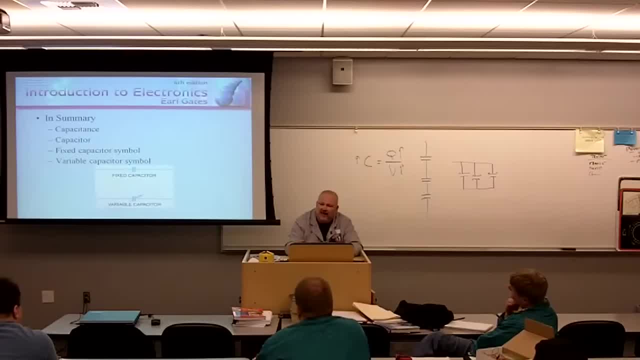 that stores energy in the form of an electrostatic field. A capacitor is a specific device designed to possess the property of capacitance. Fixed capacitor symbol on the top. variable capacitor symbol on the bottom. Capacitance is measured in farads, developed by a guy by the name of Joe Farad.